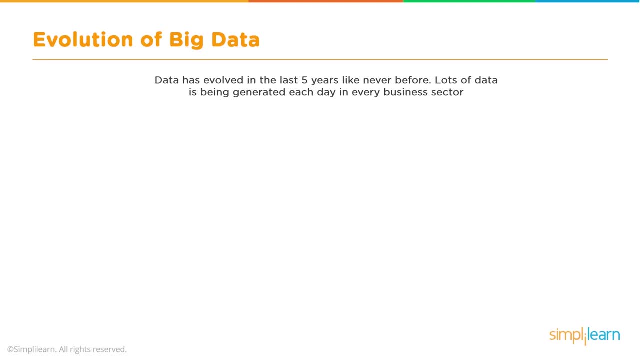 data has evolved in last five years like never before Now, in fact, before going to big data or before understanding these solutions and the need and why there is a rush towards big data technology and solution, I would like to ask a question, Take a couple of minutes and think. 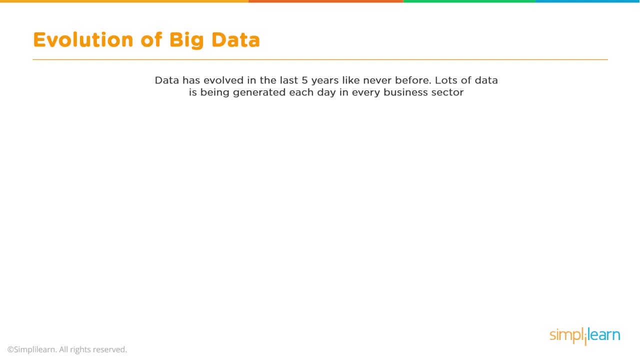 why are organizations interested in big data? Why is there a sudden rush in industry where everyone would want to ramp up their current infrastructure or would want to be working on technologies which allow them to use this big data? Think about it: What is happening and why are organizations interested in this? And if you think on this, you will start thinking about. 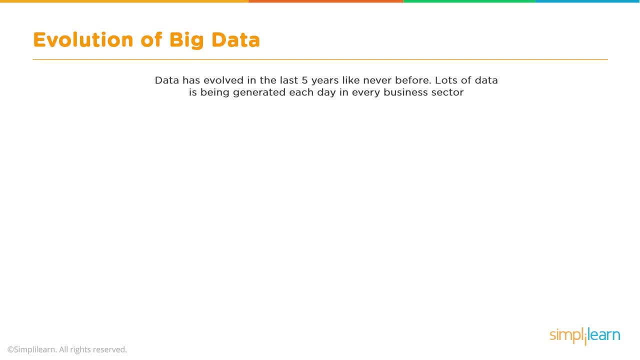 what organizations have been doing in past, what organizations have not done, and why are organizations interested in big data Now, before we learn on big data, we can always look into internet and check for use cases where organizations have failed to use legacy systems or relational databases to work on their data requirements. 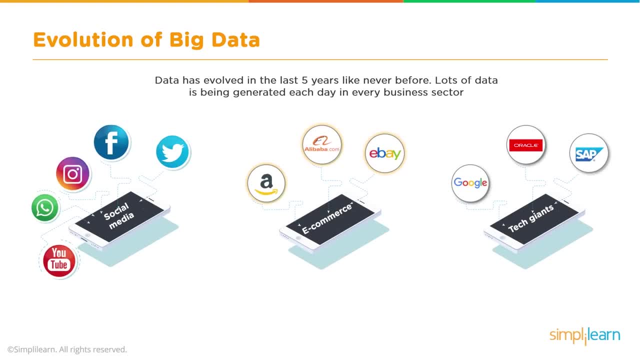 Now over in recent, or over past five years or in recent decade. what has happened is, organizations have started understanding the value of data and they have decided not to ignore any data as being uneconomical. Now we can talk about different platforms through which data is generated. 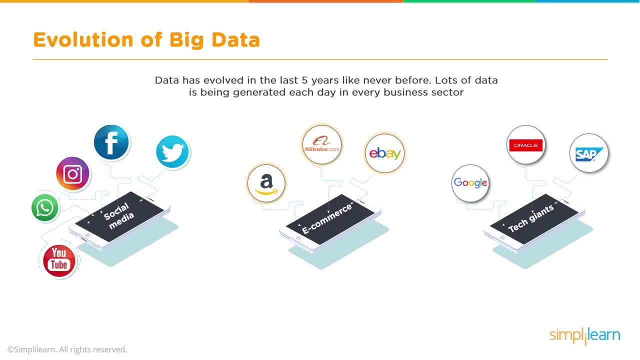 take an example of social media like Twitter, Facebook, Instagram, WhatsApp, YouTube. you have e-commerce and various portals, say eBay, Amazon, Flipkart, Alibabacom, and then you have various tech giants such as Google, Oracle, SAP, Amazon, Microsoft and so on. 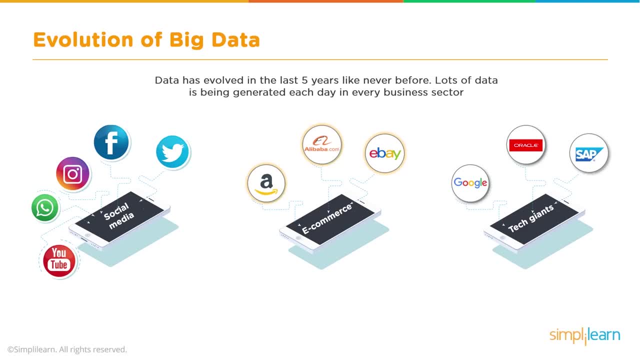 So lots of data is getting generated every day in every business sector. The point here is that organizations have slowly started realizing that these are not just virtual technologies, but these are data from real, that they would be interested in working on all the data. Now the question which I asked was why. 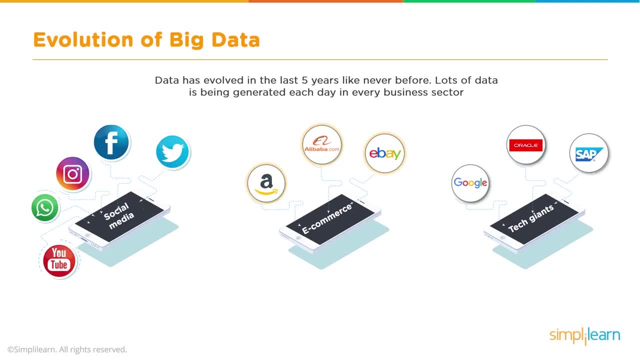 are organizations interested in big data, and some of you might have already answered or thought about that. organizations are interested in doing precise analysis or they want to work on different formats of data, such as structured, unstructured, semi-structured data. Organizations are interested in gaining insights or finding the hidden treasure in the so-called big data, and this is the main. 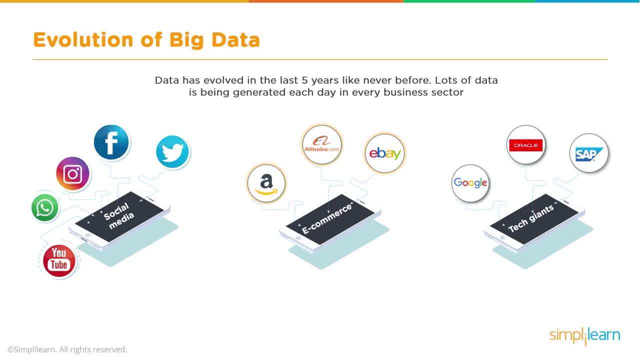 reason where organizations are interested in big data. Now there are various use cases. There are various use cases. We can compare that organizations from past 50 or more than 50 years have been handling huge amount of data. They have been working on huge volume of data. but the question: 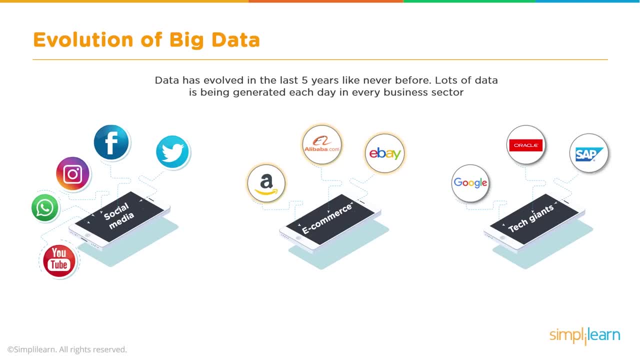 here is: have they worked on all the data or have they worked on some portion of it? What have they used to store this data? and if they have used something to store this data, what is happening? What is changing now? When we talk about the businesses, we cannot avoid talking about 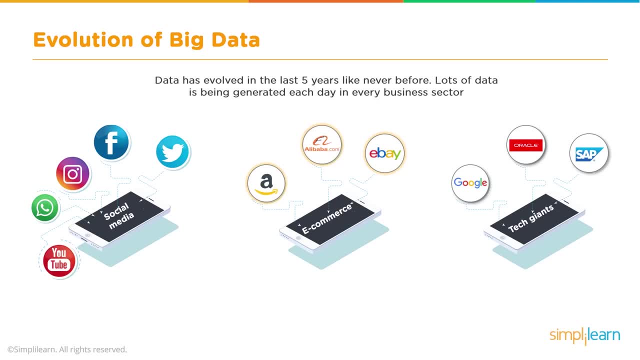 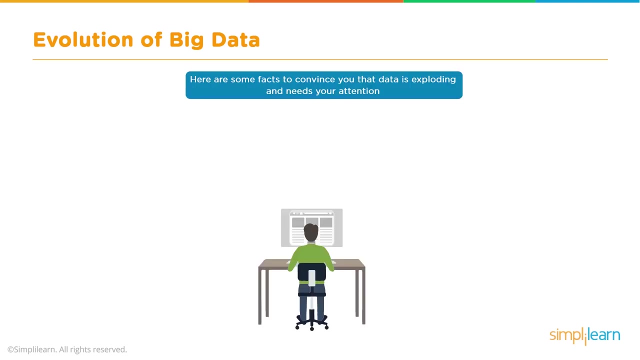 the dynamism involved. Now any organization would want to have a solution which allows them to store data- and store huge amount of data, capture it, process it, analyze it and also look into the data to give more value to the data. Organizations have, then been looking for solutions. Now let's look at some facts that can convince you. 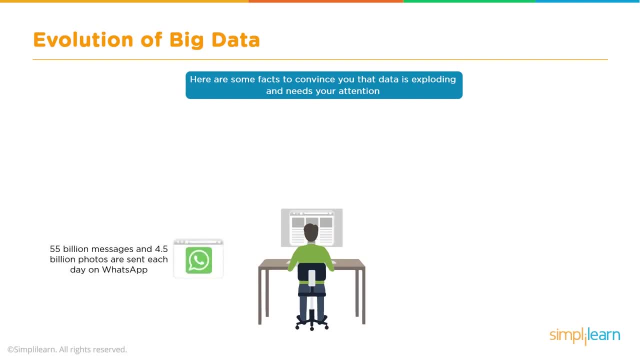 or that would convince you that data is exploding and needs your attention Right. 55 billion messages and 4.5 billion photos are sent each day on WhatsApp. 300 hours of video are uploaded every minute on YouTube. Did you guys know that YouTube is the second largest search engine after Google? Every? 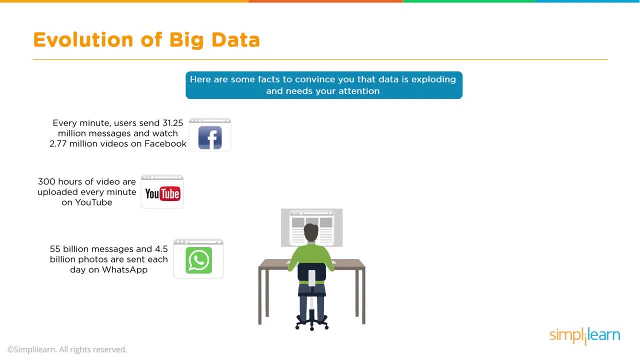 minute. users send 31.25 million messages and watch 2.6 million videos a day. 3.77 million videos on Facebook. Walmart handles more than 1 million customer transactions every hour. Google: 40,000 search queries are performed on Google per second. That is 3.46 million searches a day. 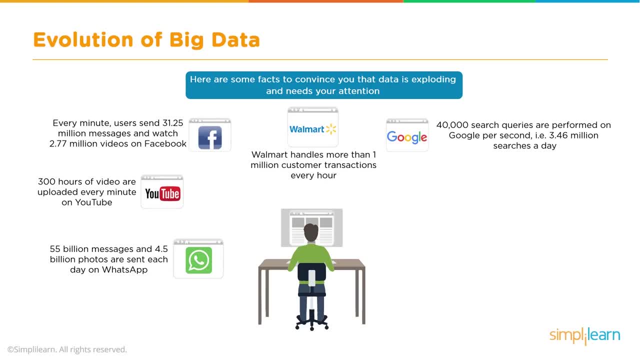 In fact, you could also say that a lot of times, people, when they are loading up the Google page, is basically just to check their internet connection. However, that is also generating data. IDC reports that by 2025, real-time data is going to be used to generate data. IDC reports that by 2025, real-time data is going to be used to generate data. IDC reports that by 2025, real-time data. 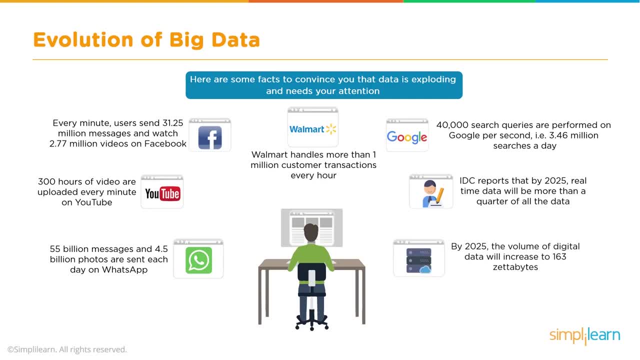 will be more than a quarter of all the data And by 2025, the volume of digital data will increase to 163 zettabytes. That is, we are not even talking about gigabytes or terabytes anymore. We are talking about petabytes, exabytes and zettabytes, And zettabytes means 10 to the power of 21 bytes. 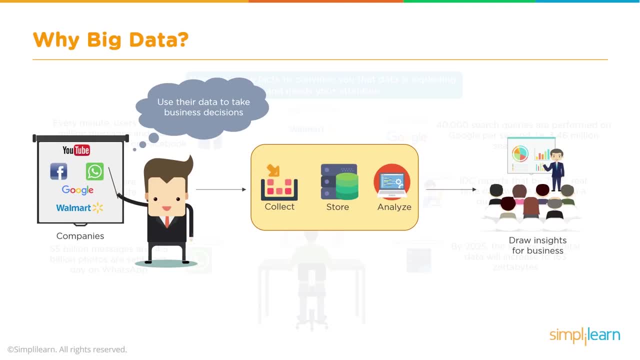 So this is how data has evolved. Now you can talk about different companies which would want to use their data to take business decisions. They would want to collect the data to their, store it and analyze it, and that's how they would be interested in drawing insights for the business. 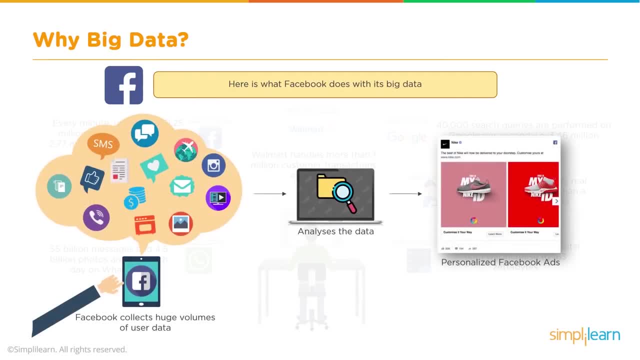 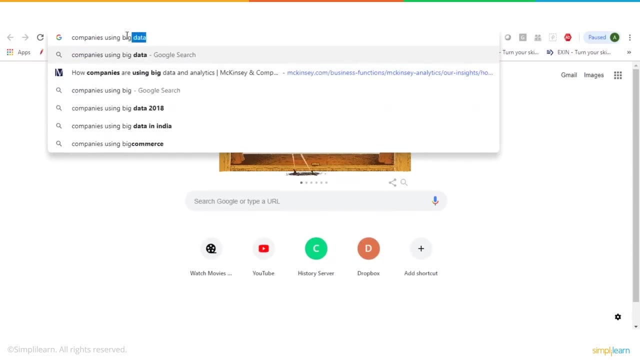 now, this is just a simple example about facebook and what it does to work on the data. now, before we go to facebook, you could always check in google by just typing in companies using big data, and if we say companies using big data, we should be able to find a list of different companies which are: 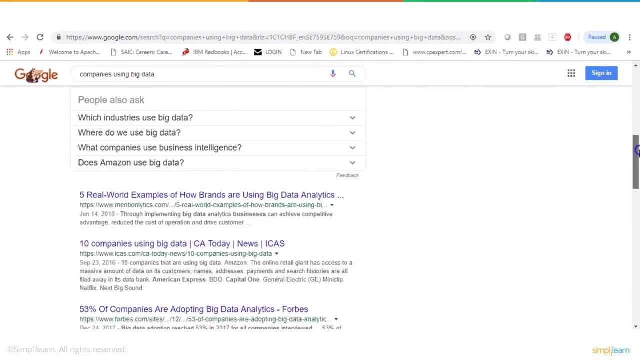 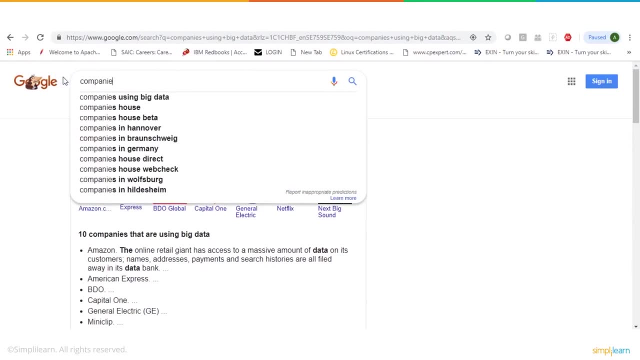 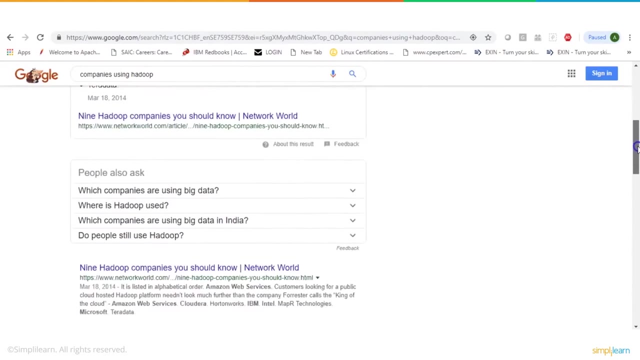 using big data for different use cases. there are various sources from where you can find. we could also search for solution- that is hadoop, which we'll discuss later, but you could always say companies using hadoop and that should take you to the wiki page, which will basically help you. 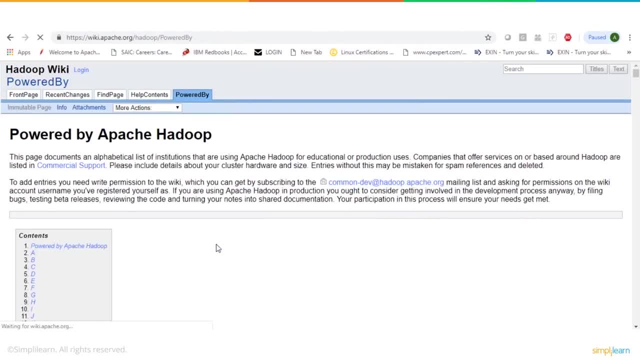 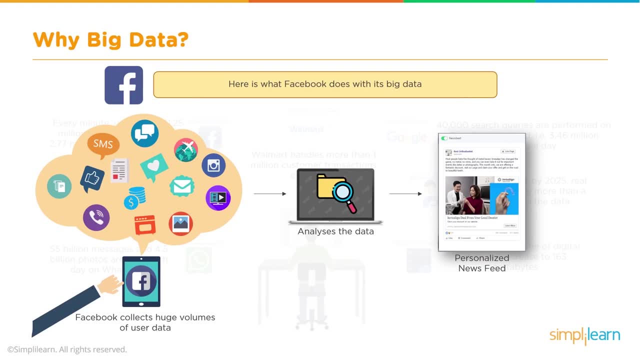 know what are the different companies which are using this so-called solution called hadoop. okay, now coming back to what we were discussing about. so organizations are in in big data, as we discussed. in gaining insights, they would want to use the data to find hidden information which probably they ignored earlier. now take an example of rdbms. what is biggest? 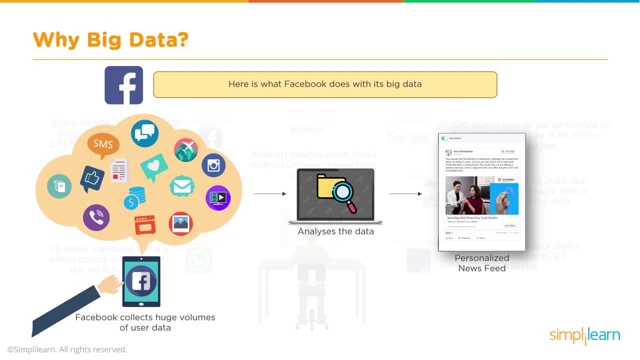 drawback in using an rdbms? now you might think that rdbms is known for stability and consistency, and organizations would be interested in storing their data in oracle or db2 or mysql or microsoft sql server, and they have been doing that for many years now. so what has changed now? now when we talk, 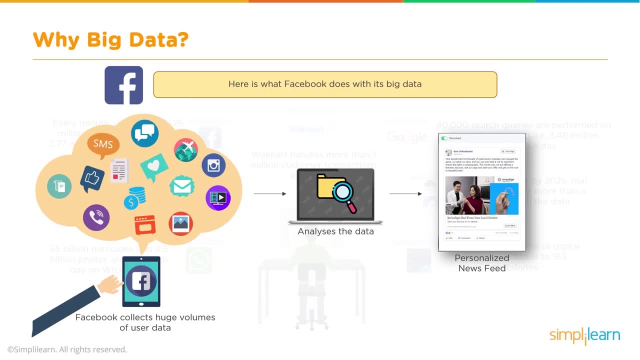 about rdbms. the first question which i would ask is: do we have access to 100% of data being online in rdbms? the answer is no. we would only have 10 or 20 or 30 percent of data online and the rest? 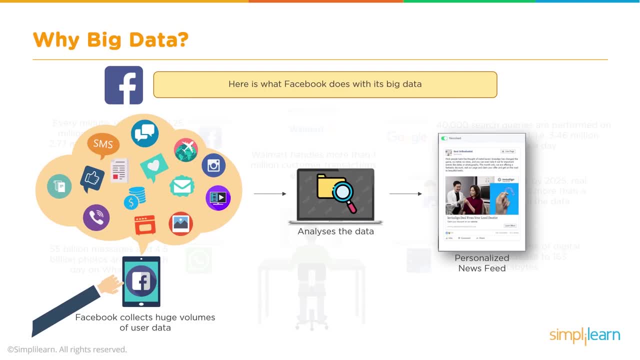 of the data would be archived, which means that if an organization is interested in working on all the data, they would have to move the data from the to the processing layer, and that would involve bandwidth consumption. Now, this is one of the biggest drawbacks of RDBMS: You do not have access to 100% of data online In many of the cases. 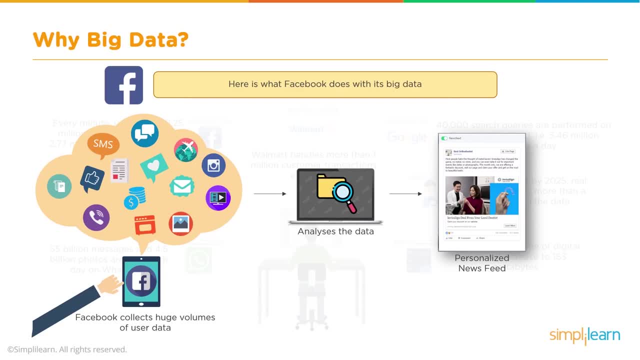 organizations started realizing that the data which they were ignoring as being uneconomical had hidden value which they had never exploited. I had read a presentation somewhere which said: torture the data and it will confess to anything. Now that's the value of data which organizations 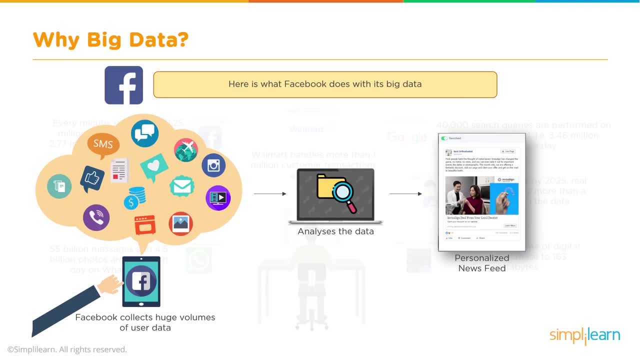 have realized in recent past. Take an example of Facebook. Now. this shows what Facebook does with its big data, and we'll come to what is big data. but let's understand the use case Now. Facebook collects huge volumes of user data, whether that is SMS, whether that is likes. 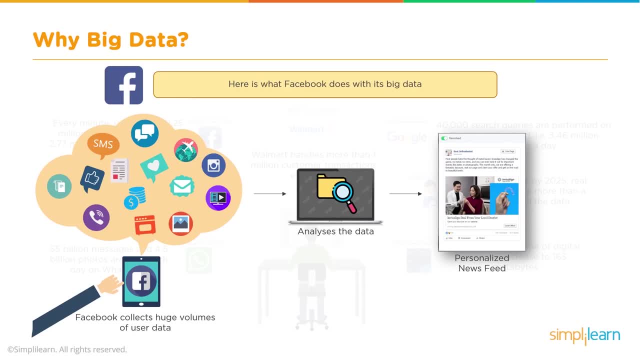 whether that is advertisements, whether that is features which people are liking, or photographs, or even user profiles. Now, by collecting this data and providing a portal which people can use to connect, Facebook is also accumulating huge volume of data, and that's way beyond petabytes. They would also be interested in analyzing this data, and one. 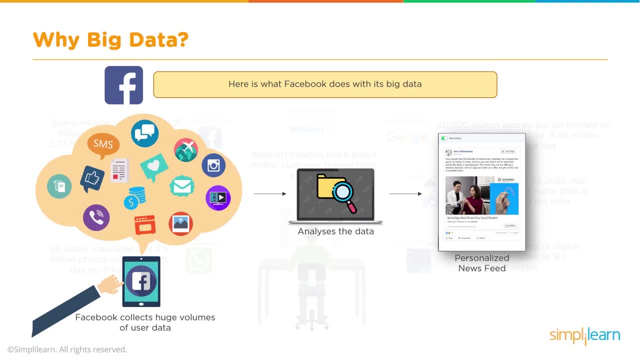 of the reasons would be they would want to personalize the experience. Take an example of personalized news feed: Depending on a user behavior, depending on what a user likes, what a user would want to know about, they can recommend a personalized news feed to every. 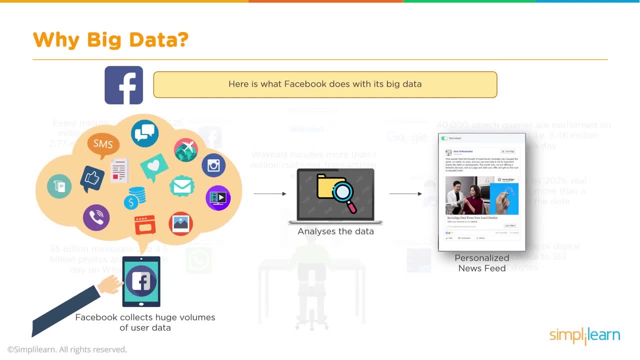 particular user. That's just one example of what Facebook does with its data. Take an example of photo tag suggestions. Now, when you login to Facebook account, you could also get suggestions on different friends whom you would like to connect to or you would want to tag so that. 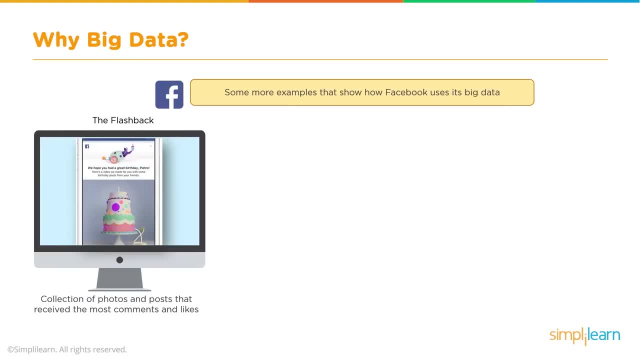 they could be known by others. Some more examples which show how Facebook uses its data are very useful. Apple muchís Sharing The peoples this week. Where did you live So that information comes from friends that you are not familiar with? 영상을 afterward. But very good news to everyone. That's what Facebook is all about. news feeds is showing what a user wants to know about. They can recommend personalized news feeds to every particular user. That's just one example of what Facebook does with its data. taking this data, take an example of photo tag suggestions. Now, 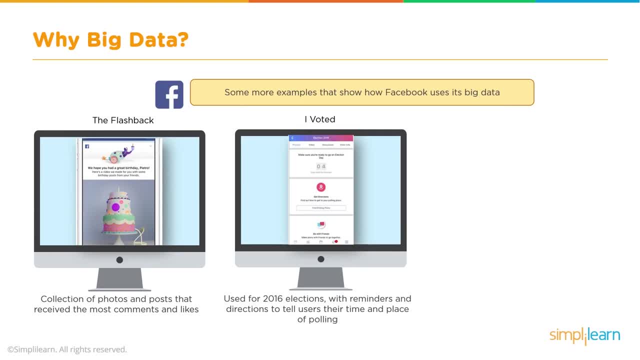 as follows. so the flashback collection of photos and posts that received the most comments and likes. okay, there was something called as I voted that was used for 2016 elections, with reminders and directions to tell users their time and place of polling. also, something called a safety checks in incidents such 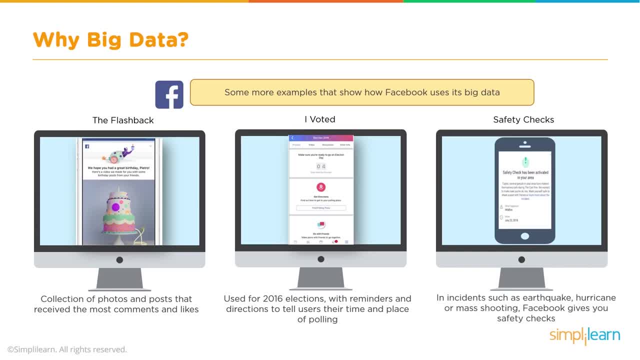 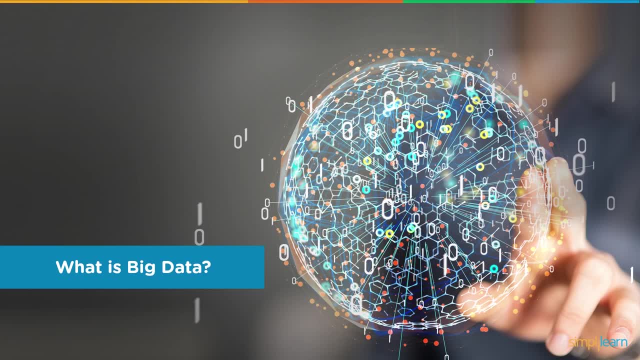 as earthquake, hurricane or mass shooting. Facebook gives you safety checks. now these are some examples where Facebook is using big data, and that brings us to the question: what is big data? this was just an example where we discussed about one company which is making use of that data which has been accumulated and it's 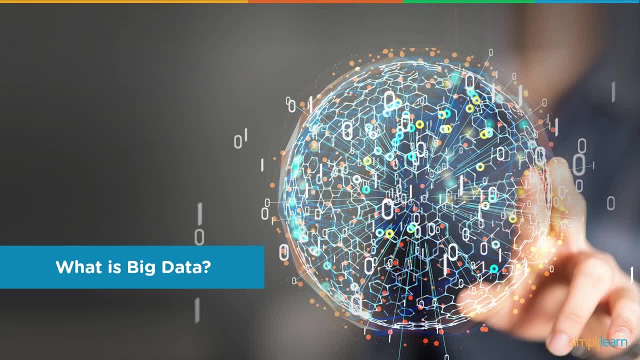 not only for companies which are social media oriented, like Facebook, where data is important. take an example of IBM, take an example of JP Morgan Chase, take an example of GE or any other organization. take an example of IBM. take an example of JP Morgan Chase, take an example of GE or any other organization. 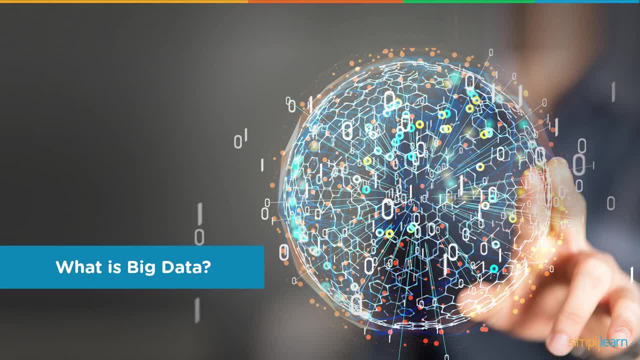 organization which is collecting huge amount of data. They would all want to gather insights, They would want to analyze the data, They would want to be more precise in building their services or solutions which can take care of their customers. So what is big data? Big data is: 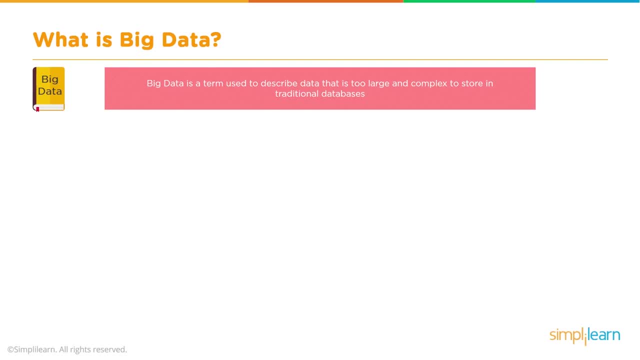 basically a term. It is used to describe the data that is too large and complex to store in traditional databases And, as I gave an example, it's not just about storing the data. It is also about what you can do with the data. It also means that if there is a lot of dynamism, 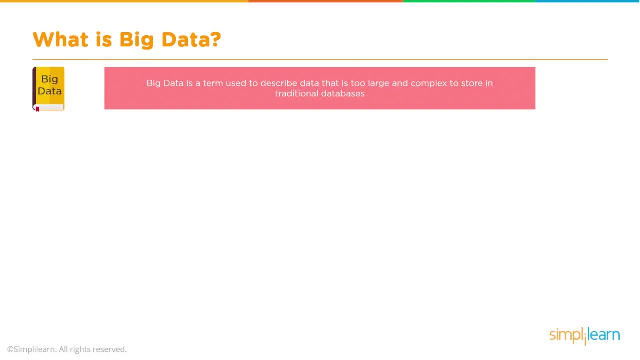 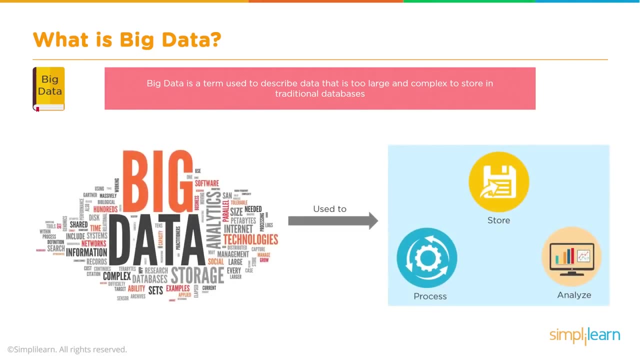 involved. can you change the underlying storage and handle any kind of data that comes in? Now, before we get into that, let's just understand what is big data. So big data is basically a term which has been given to categorize the data if it has different. 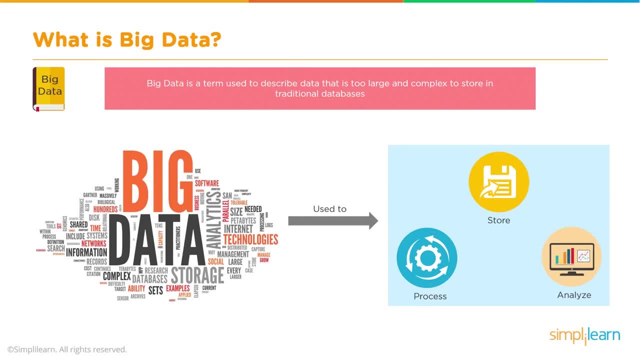 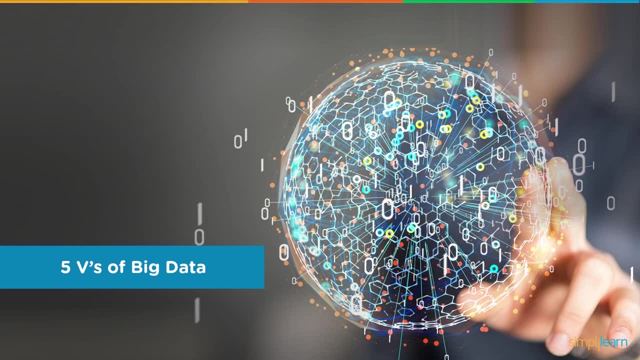 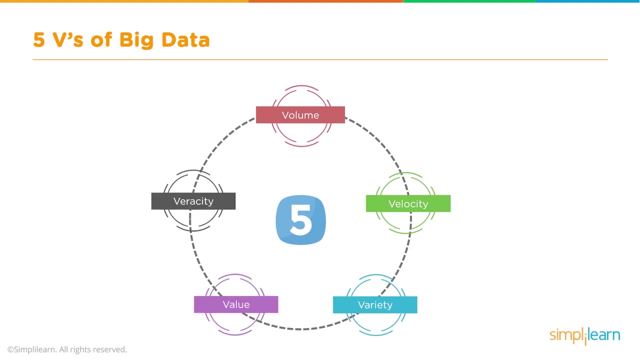 characteristics. Organizations would want to have the big data stored, processed and then analyzed to get whatever useful information they can get from this data. Now there are five V's of big data: volume, velocity, variety, value, veracity. Although 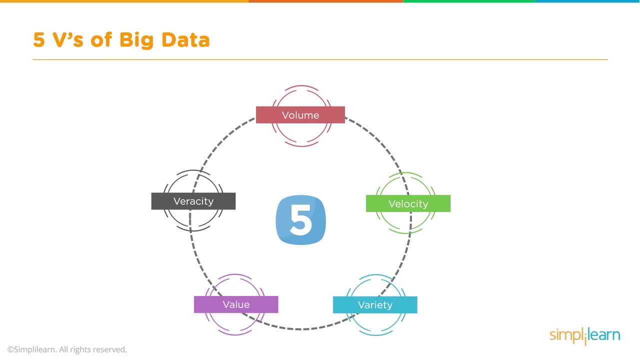 these are five V's, but then there are other V's which also categorize the data as big data, such as volatility, validity, viscosity, virality of data. So these are five V's of big data, And if the data has one, 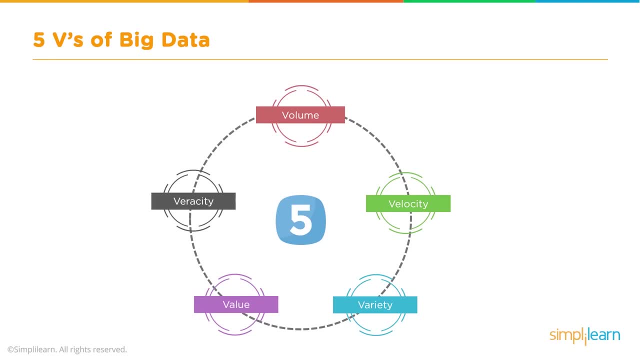 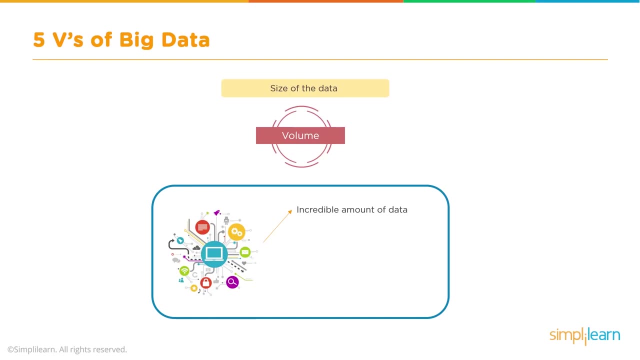 or all of these characteristics, then it can be considered as big data, including the other V's which I just mentioned. So volume basically means incredible amount of data, huge volumes of data, data generated every second. Now that could be used for batch processing, That could. 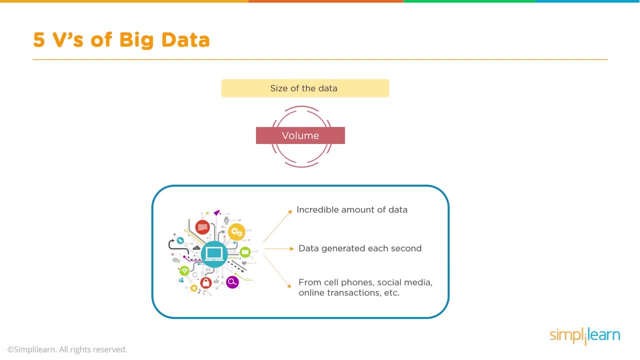 be used for real-time stream processing. You might have data being generated from different kind of devices, like your cell phones, your social media websites, online transactions, wearable devices, servers, And these days, with IoT, we are also talking about data getting generated via Internet of Things, That is, you could have different devices which could be. 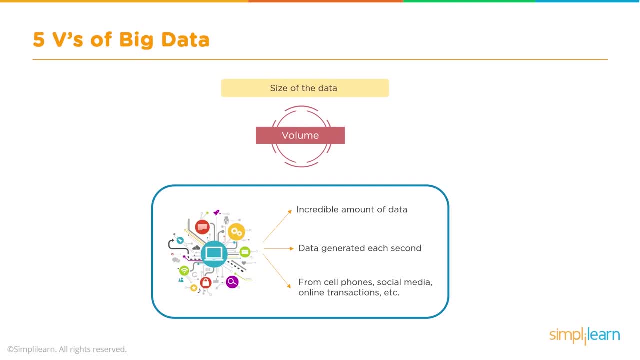 communicating to each other. You could be getting data from radars or lidars or even camera sensors. So there is a huge volume of data which is getting generated. And if we are talking about data which has huge volume, which is getting generated constantly or has huge volumes of data, 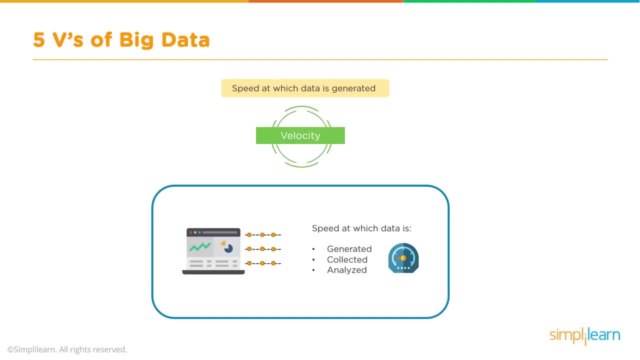 or has been accumulated over a period of time. we would say that is big data Velocity. Now, this is one more important aspect of big data: Speed with which the data is getting generated. Think about stock markets, Think about social media websites, Think about 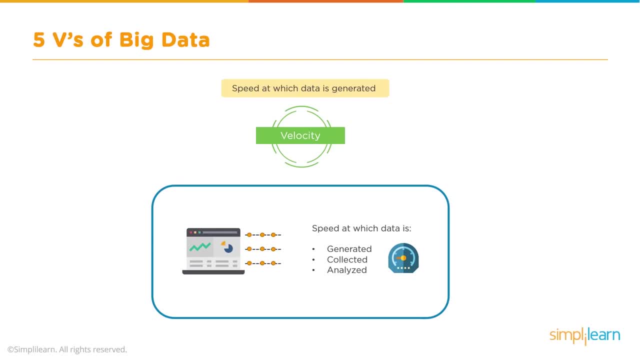 online surveys or marketing campaigns or airline industry. So if the data is getting generated with a lot of speed where it becomes difficult to capture, collect, process, cure, mine or analyze the data, then we are certainly talking about big data. The next aspect of big 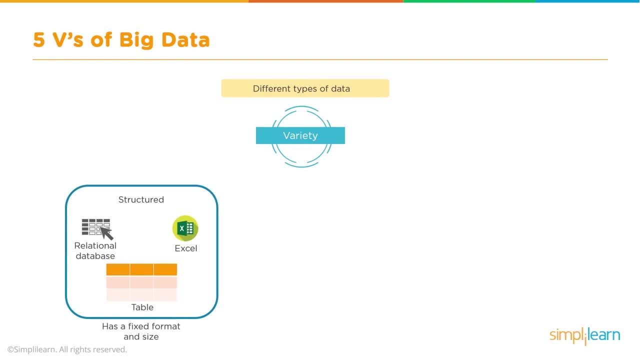 data is variety. Now this is where we talk about structured data, semi-structured data or unstructured data, And here I would like to ask a question: What is the difference? When do you call the data as structured, semi-structured or unstructured? Now let's look at an example. 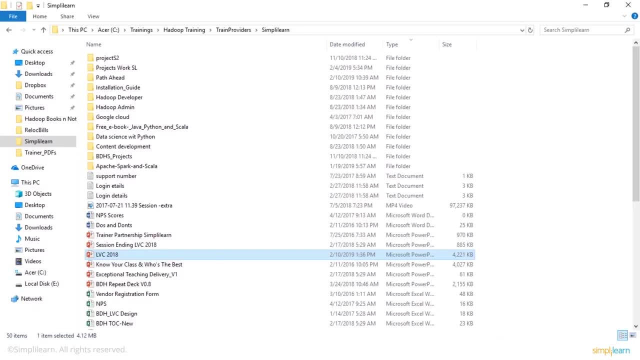 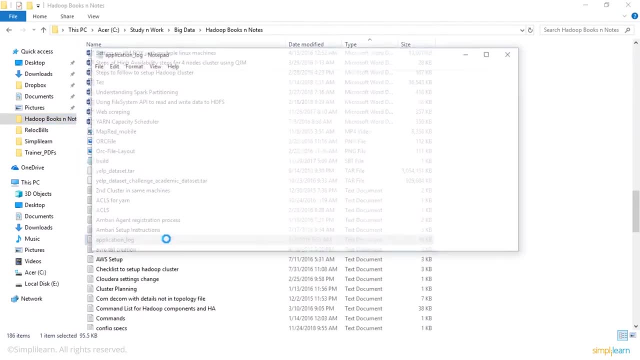 before we theoretically discuss about this, I always would like to use some examples. Let's look at a log, Let's call a file and let's see what is it. So if I look at this log file and if I would say: 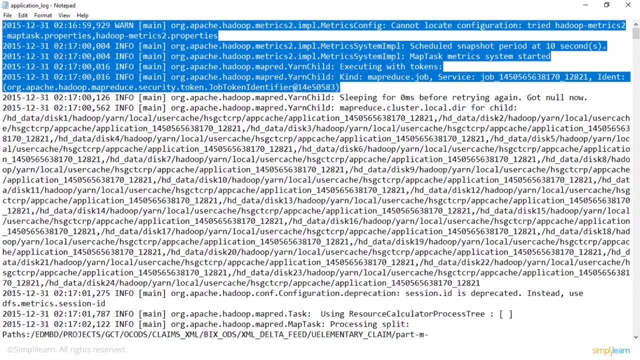 what kind of data is this? which is the highlighted one? The answer would be: it is structured data. It has specific delimiters, such as space. It has data which is separated by space, And if I had a hundred or thousand or million rows which had similar kind of data, I could certainly store that. 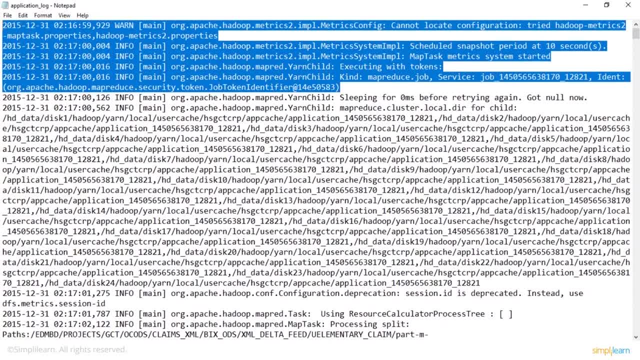 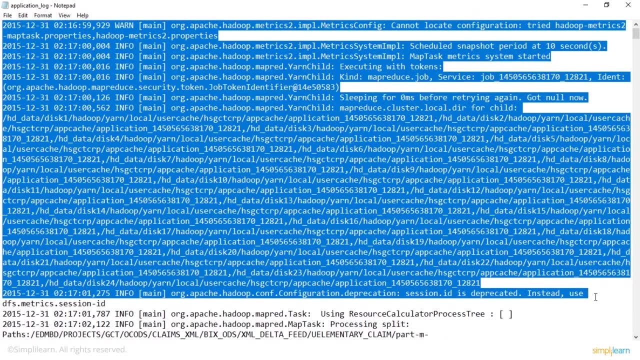 in a table, I could have a predefined schema to store this data, so I would call the one which is highlighted as structured. but if I look at this portion where I would look at a combination of this kind of data, where some data has a pattern and some data doesn't, now this is an example of semi-structured. 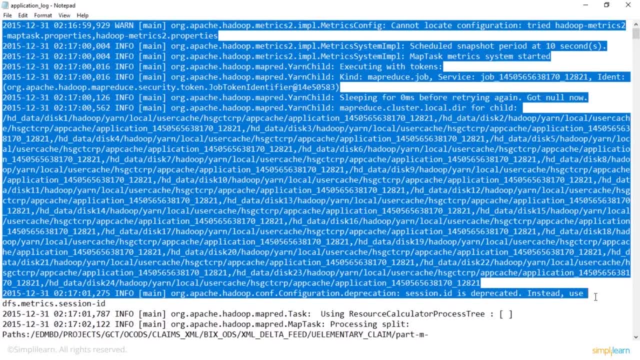 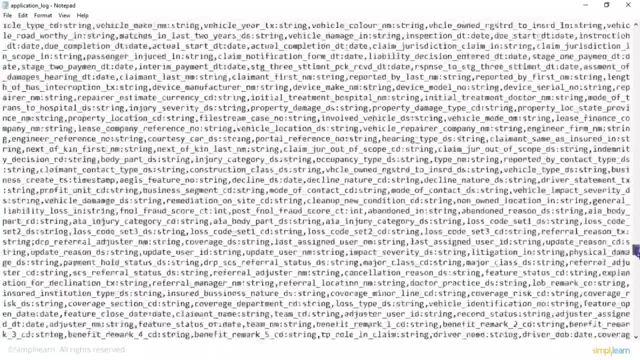 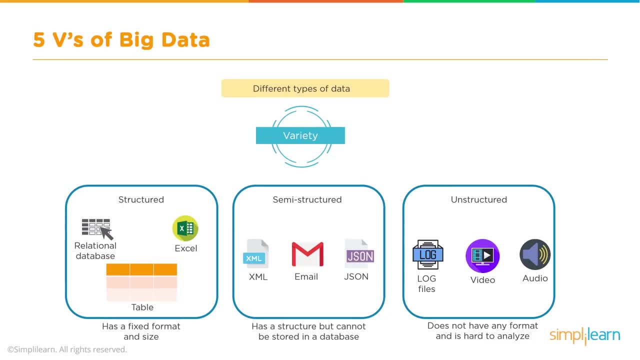 data. so if I would have a predefined structure to store this data, probably the pattern of data would break the structure. and if I look at all the data, then I would certainly call it unstructured data, because there is no clear schema which can define this data. now, this is what I mean by 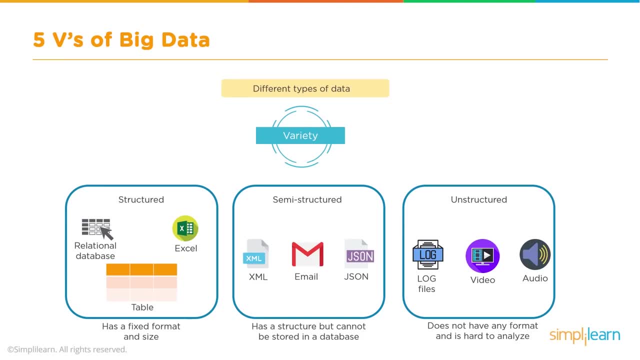 variety of data that is, structured, data which basically has a schema or has a format which could be easily understood. you have semi-structured, which could be like an xml or json or even your excel sheets, where you could have some data which is structured and the other. 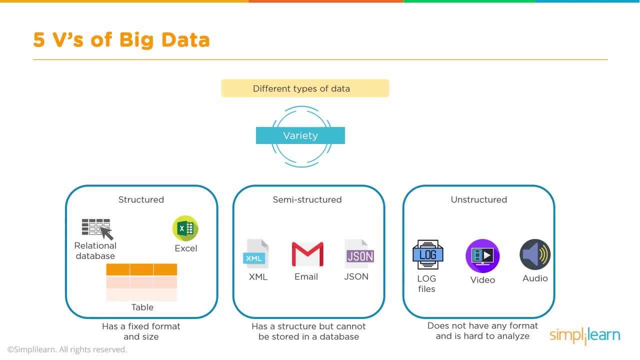 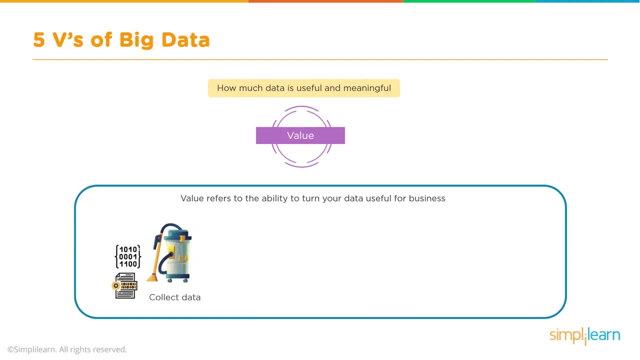 is unstructured, and when we talk about unstructured, we are talking about absence of schema. it does not have a format, it does not have a schema and it is hard to analyze, which brings its own challenges. the next aspect is value. now, value refers to the ability to turn your data useful for business. 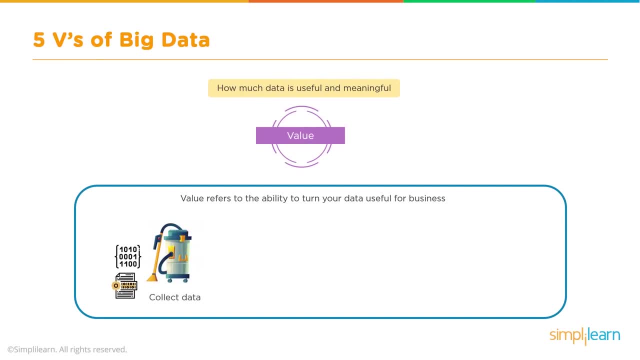 you would have a lot of data which is being collected, as we mentioned in previous slides. right, there would be a lot of data wrangling or data pre-processing or cleaning up of data happening and then, finally, you would want to draw value from that data, but from all the data. 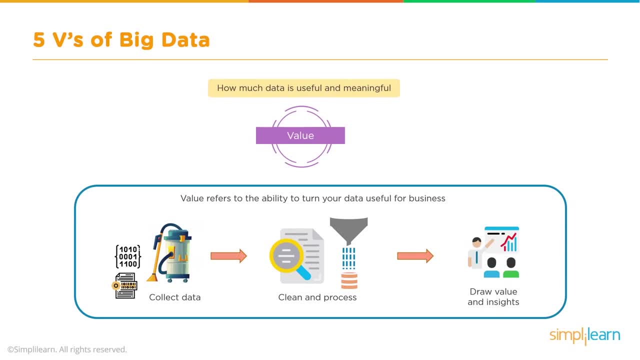 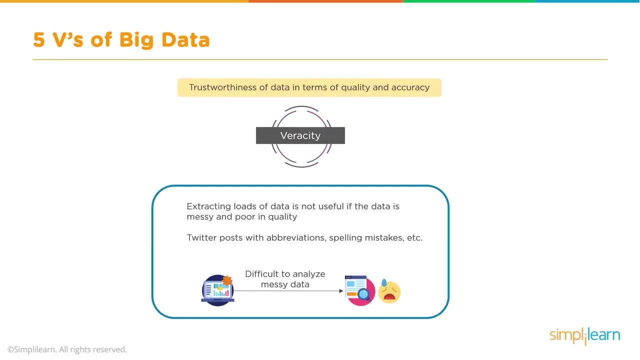 collected? what percentage of data gives us value? and if all my data can give me value, then why wouldn't i use it? this is an aspect of big data right veracity. now this means the quality of data. billions of dollars are lost every year by organizations because the data which was 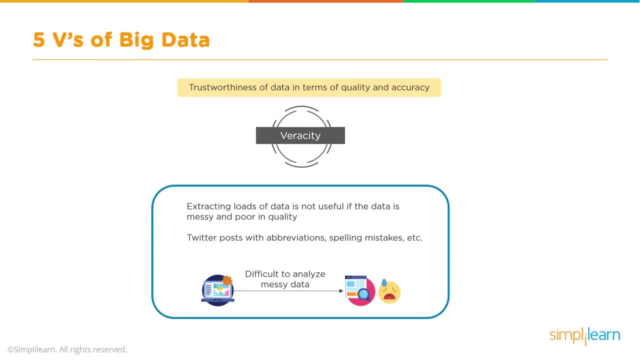 collected was not of good quality or probably they collected lost every year by organizations because the data which was collected was not of good quality- lot of data- and then it was erroneous. take an example of autonomous driving projects which are happening in europe or us, where there are car fleets which are on the road collecting data via 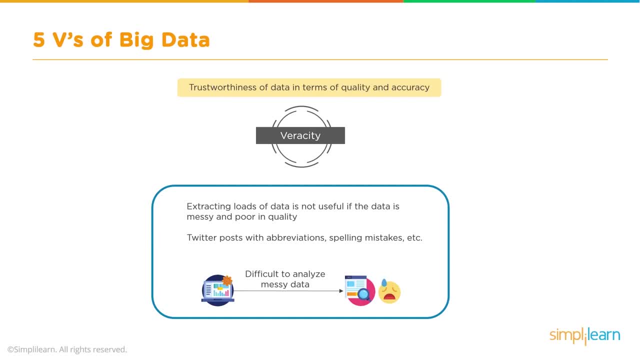 radar sensors and camera sensors. and when this data has to be processed to train algorithms, it is realized that sometimes the data which was collected was missing in some values, might be, was not appropriate or had a lot of errors. and all this process of collecting the data becomes a repetitive task because the quality of data was 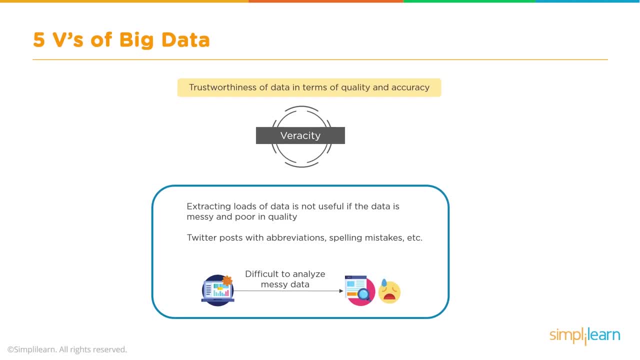 not good. this is just one example. we can take example from healthcare industry or stock markets or financial institutions and so on. so extracting loads of data is not useful if the data is messy or poor in quality, and that basically means that veracity is a very important v of big data. now 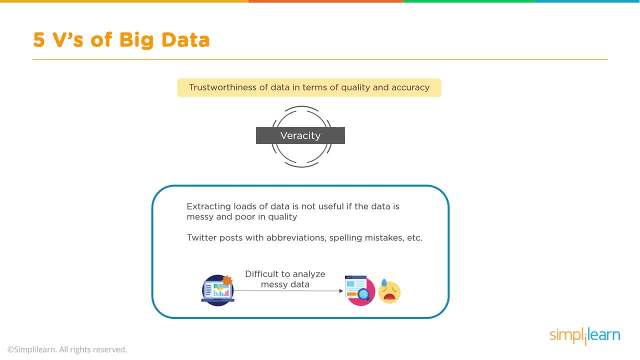 apart from veracity, volume, variety, velocity and value, we have the other v's, such as viscosity- how dense the data is. validity- is the data still valid? volatility- is my data volatile? or virality- is the data viral now? all of these different v's categorize the data as big data. we would like to talk on a big data case study and 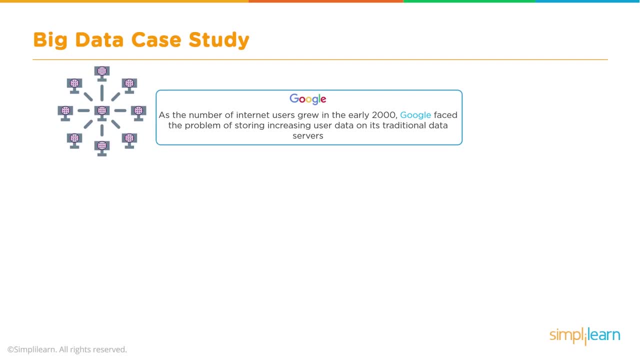 we have taken an example of google, which obviously is one of the companies which is churning and working on huge amount of data. now it's actually said that if you compare one grain of sand with one bite of data, then google is processing, or google is handling, whole world's sand every week. that is the kind of 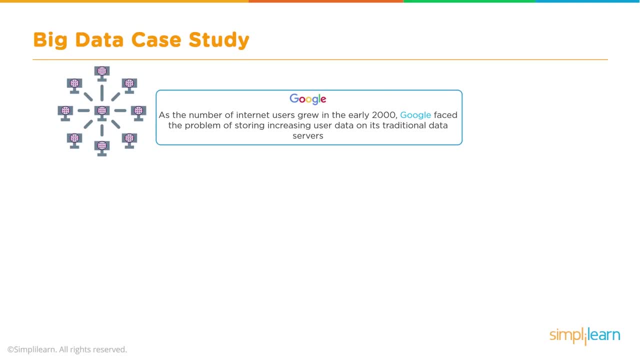 data which google is processing now. in early 2000 and since then, when the number of internet users started growing, google also faced a lot of problems in storing increasing user data and using the traditional server to manage that. now that was a challenge which google started facing. could they use traditional? 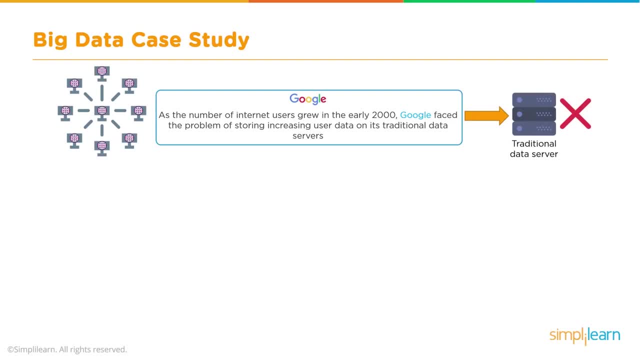 data server to store the data. well, yes, they could right. storage devices have been getting cheaper day by day, but then how much time does it take to retrieve that data? what is the seek time? what is the time taken to read and process that data? thousands of search queries were raised. 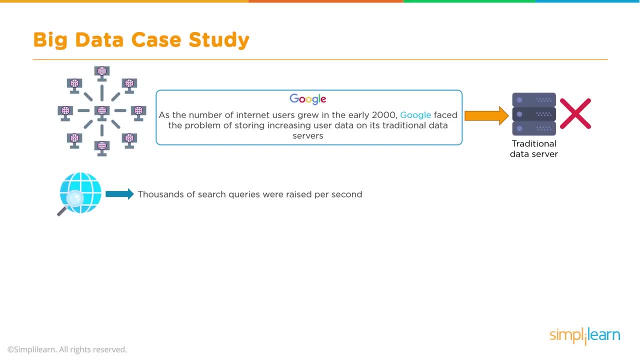 per second. no doubt now we could say millions and billions of queries are raised per second. every query read 100 mbs of data and consumed tens of billions of cpu cycles based on these queries. so the requirement was that they wanted to have a large, distributed, highly fault tolerant file. 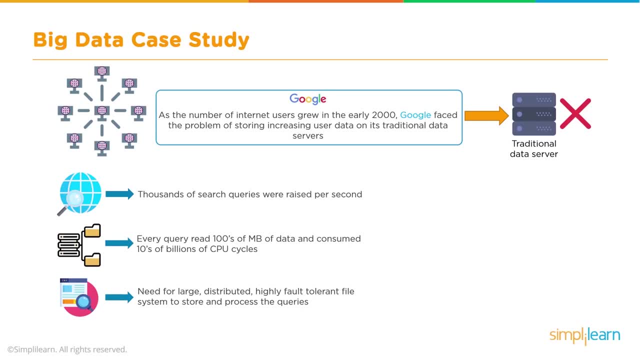 system, large to store, to capture, process huge amount of data distributed, because they could not rely just on one server, even if that had multiple disks stacked up. that was not an efficient choice. what would happen if this particular machine failed? what would happen if the whole server was down? so they needed a distributed storage and a distributed computing environment. 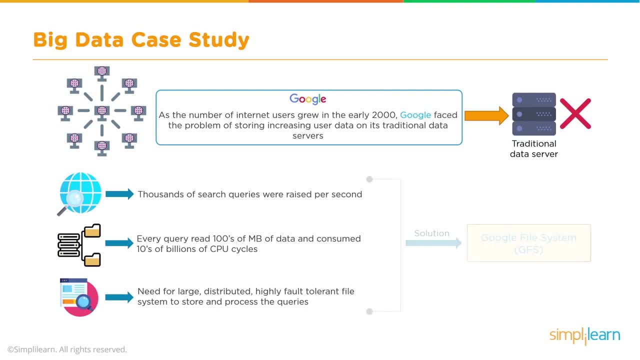 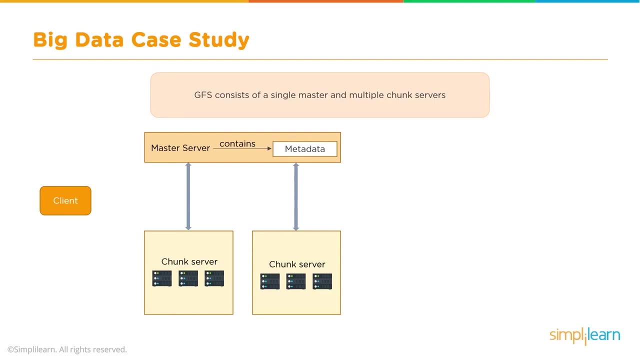 they needed something which can be highly fault tolerant, right? so this was the requirement which google had, and the solution which came out as a result was gfs- google file system. now let's look at how gfs works so normally in any particular linux system or linux server. 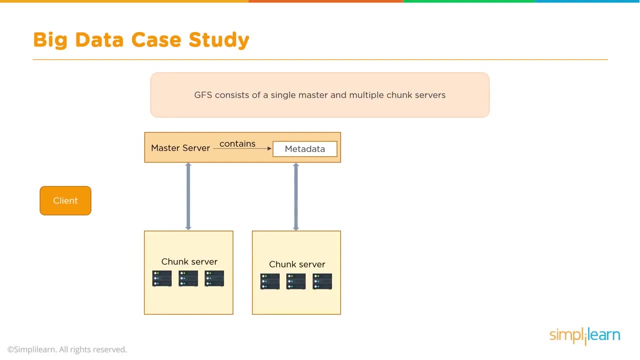 you would have a file system, you would have set of processes, you would have set of files and directories which could store the data. gfs was different. so to facilitate gfs, which could store huge amount of data, there was an architecture, an architecture which had one master and multiple. 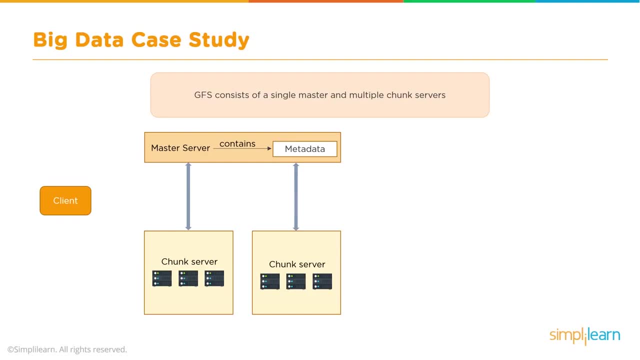 chunk servers, or you can say slave servers or slave machines. master machine was to contain metadata, was to contain data about data. when we say metadata, we are talking about information about data. and then you have the chunk servers or the slave machines which could be storing data in a distributed fashion. now, any 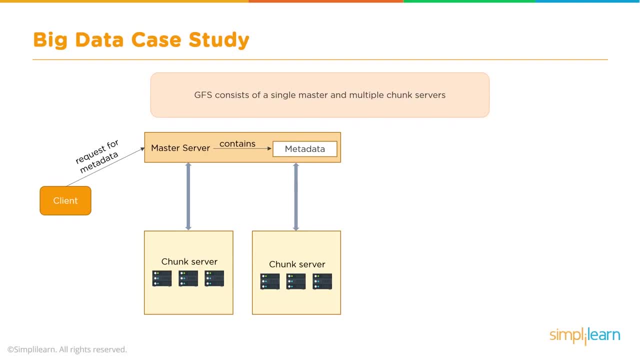 client or an api or an application which would want to read the data would first contact the master server. it would contact the machine where the master process was running and client would place a request of reading the data or showing an interest of reading the data internally. what it is doing is it is requesting for metadata. 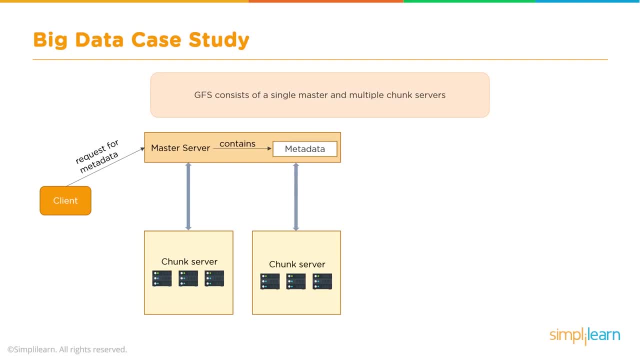 your api or an application would want to know from where it can read the data master server which has metadata, whether that is in ram or disk- we can discuss that later- but then master server would have the metadata and it would know which are the chunk servers or the slave machines where the data was stored in a distributed fashion. 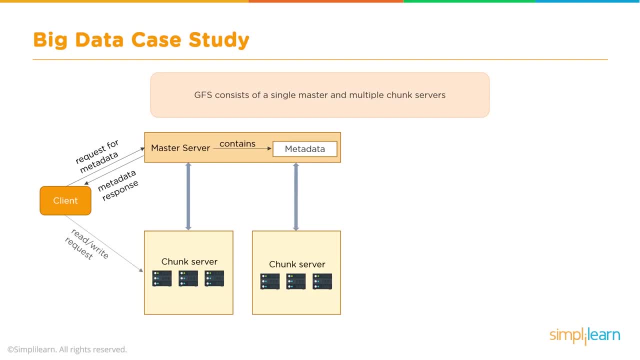 master would respond back with the metadata information to the client and then client could use that information to read or write to these slave machines where actually the data was stored. Now, this is what the process, or set of processes work together to make: GFS. So when you 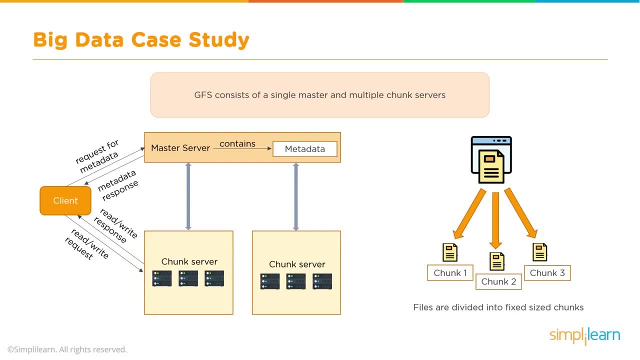 say a chunk server. we would basically have the files getting divided into fixed size chunks. Now how would they get divided? So there would be some kind of chunk size or a block size which would determine that If the file is bigger than the pre-decided chunk size, then it would be split. 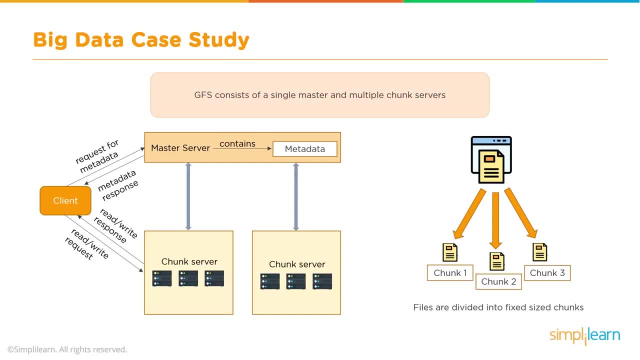 into smaller chunks and be distributed across the chunk servers or the slave machines. If the file was smaller, then it would still use one chunk or a block to get stored on the underlying slave machines. So these chunk servers or slave machines are the ones which actually store the data on. 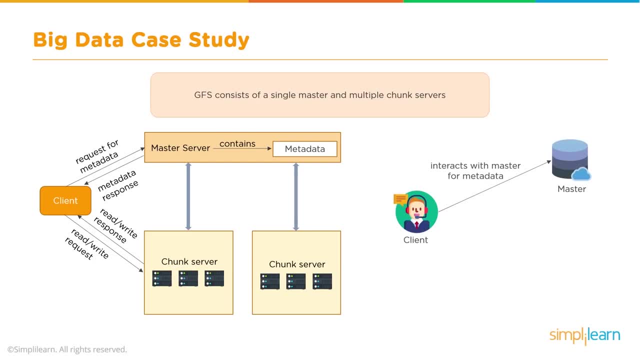 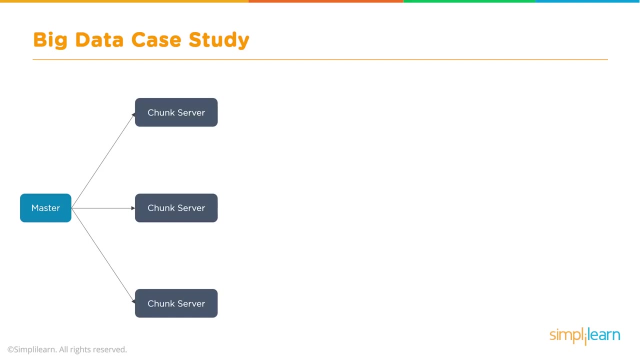 local disks as your Linux files Client, which is interacting with Microsoft Master for metadata and then interacting with chunk servers for read- write operations, would be the one which would be externally connecting to the cluster. So this is how it would look. So you have a master which would obviously be receiving some kind of heartbeats from the chunk servers to 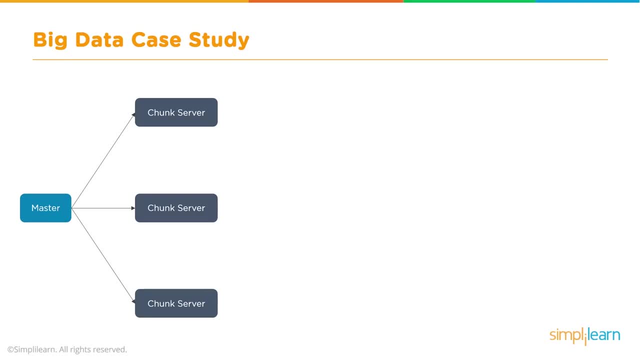 know their status and receive information in the form of packets, which would let the master know which machines were available for storage, which machines already had data, and master would build up the metadata within. It says the files would be broken down into chunks. For example, we can look at file one. It is broken down into: 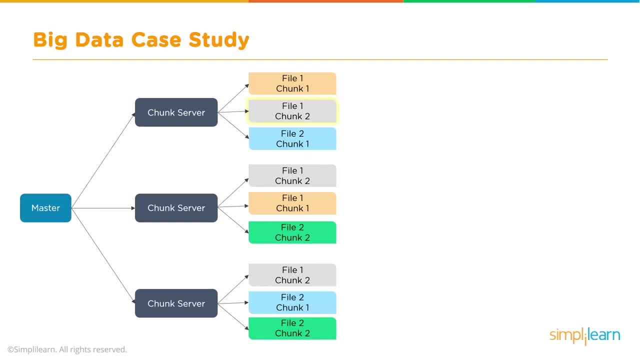 chunk one and chunk two, and file two has one chunk which is one portion of it, And then you have file two residing on some other chunk server, which also lets us know that there is some kind of auto replication for this file system. Right, And the data which is getting stored in the chunk could have a data of 64 MB. Now that chunk size could. 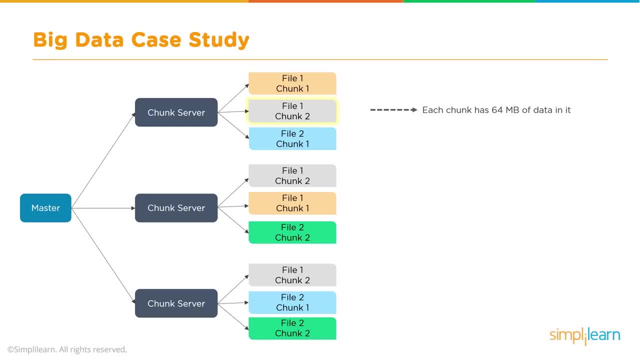 be changed based on the data size, But Google file system had the basic size of the chunk as 64 MB. Each chunk would be replicated on multiple servers. The default replication was three, and that could again be increased or decreased as per requirement. This would also mean that if a particular slave machine or a 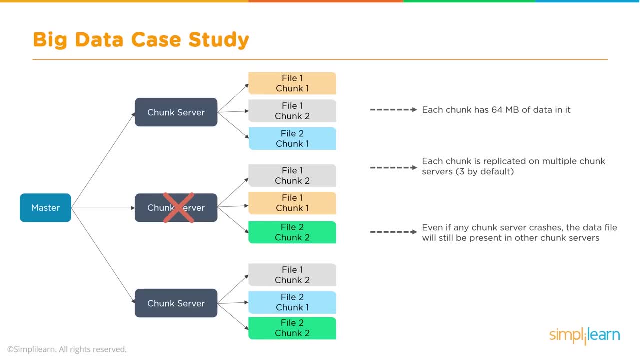 chunk server would die or would get killed or would crash. there would never be any data loss because a replica of data residing on a chunk server would not be able to be replicated on multiple servers, So the data residing on the failed machine would still be available on some other slave server, chunk server or 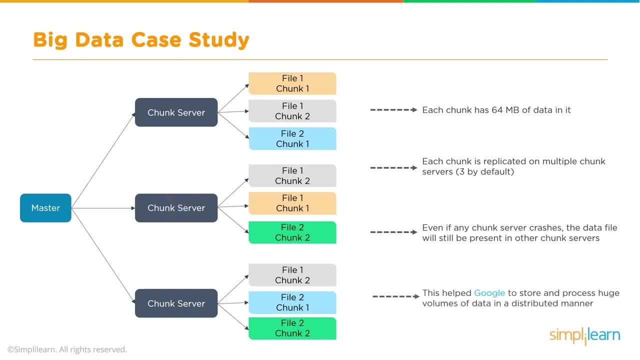 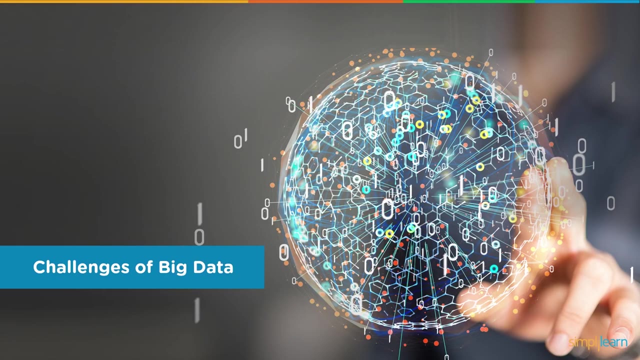 slave machine. Now, this helped Google to store and process huge volumes of data in a distributed manner and thus have a fault tolerant, distributed, scalable storage which could allow them to store a huge amount of data. Now, that was just one example which actually led to the solution which today we call as Hadoop. Now, when we 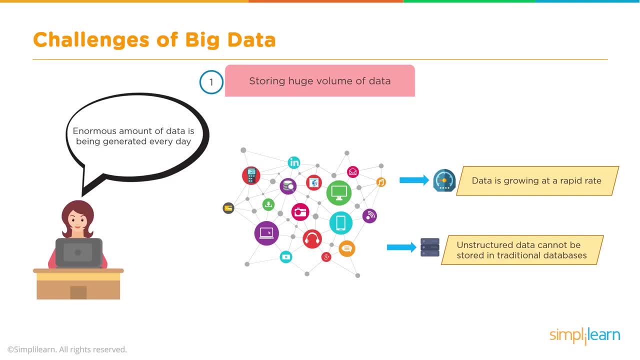 talk about big data here. I would like to ask you some questions. that, if we were talking about the RDBMS case, take an example of something like NASA which was working on a project called SETI- search of extraterrestrial intelligence. Now, this was a 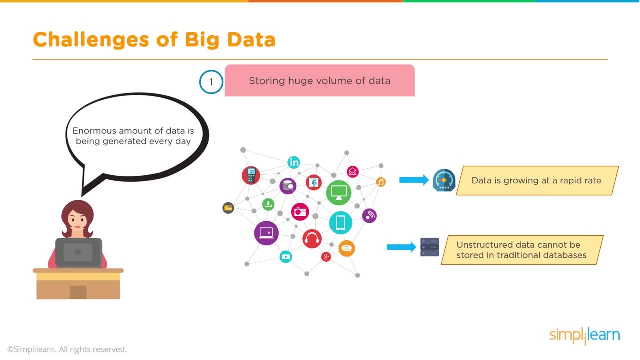 project where they were looking for a solution to take care of their problem. The problem was that they would roughly send some waves in space, capture those waves back and then analyze this data to find if there was any extraterrestrial object in space. Now they had two options for it. 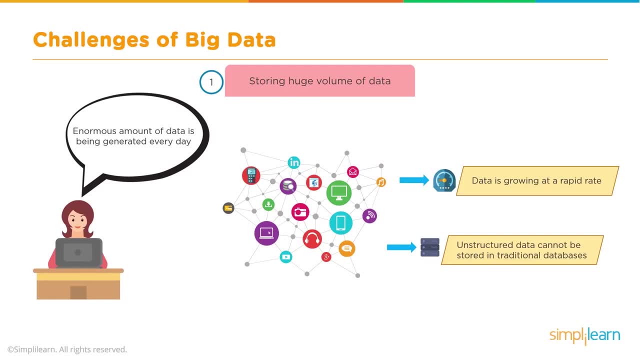 They could either have a huge server built which could take care of storing the data and processing it, or they could go for volunteer computing. Now, volunteer computing basically means that you could have a lot of people volunteering and being part of this project, And what they would, in turn, do is they would be donating their RAM and storage from their machines when they are not using it. 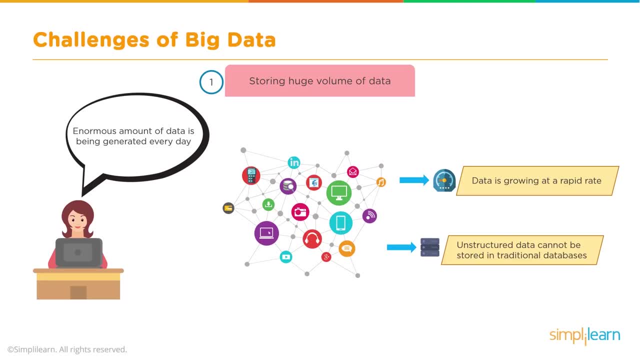 How would that happen? Basically, download some kind of patch on their machine which would run as a screensaver, And if the user is not using his machine, some portion of data could be transferred to these machines for intermittent storage and processing using RAM. 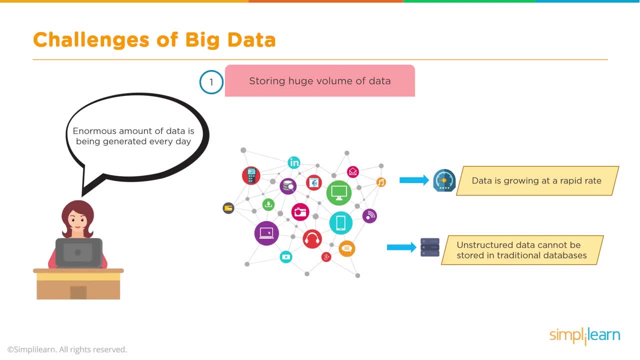 Now, this sounds very interesting and this sounds very easy. However, it would have its own challenges, right, Think about security, Think about integrity, But those problems are not bigger as much as is the requirement of bandwidth, And this is the same thing which happens in RDBMS. 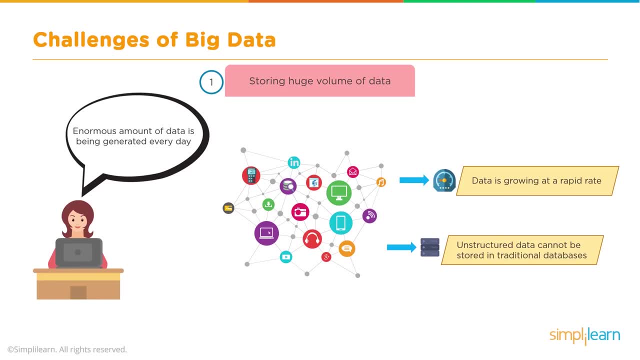 If you would have to move data from archived solution to the processing layer, that would consume huge amount of bandwidth. Big data brings its own challenges. Huge amount of data is getting generated every day. Now the biggest challenge is storing this huge volume of data. 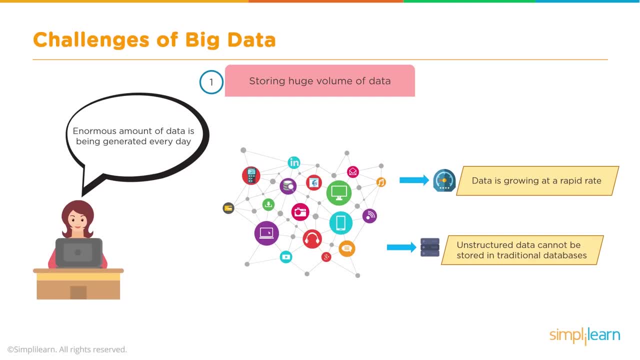 And especially when this data is getting generated with a lot of variety, where it can have different kind of formats, where it could be viral, it could be having a lot of value and nobody has looked into the veracity of data. but the primary problem would be handling this. 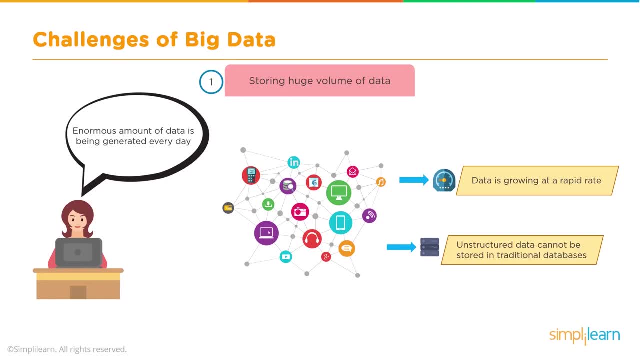 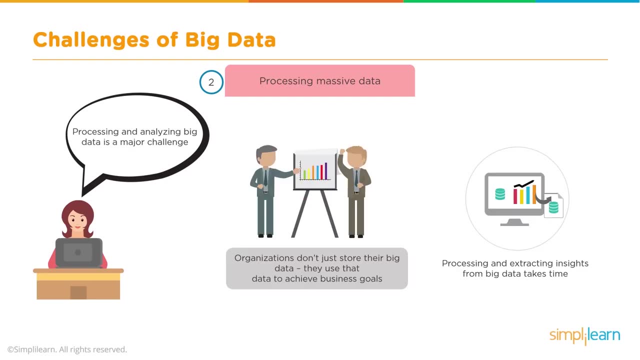 huge volume of data. Variety of the data would bring in challenges of storing it in legacy systems. if processing of the data was required Now, here again, I would suggest you need to think. what is the difference between reading a data and processing a data? 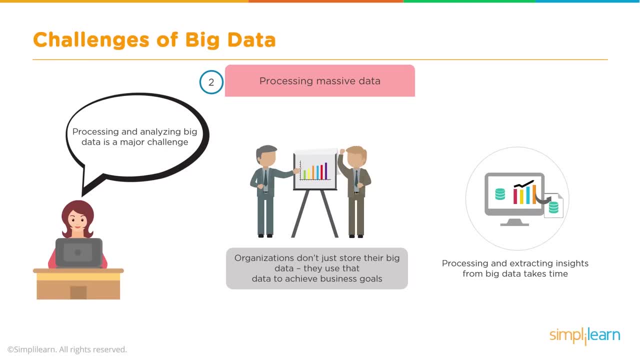 So reading might just mean bringing in the data from desk and doing some IO operations, and processing would mean reading the data, probably doing some transformations on it, extracting some useful information from it and then storing it in the same format or probably in a different format. 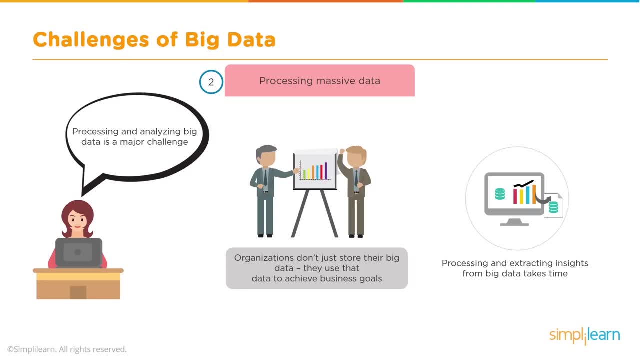 So processing this massive volume of data is the second challenge. Organizations don't just store their big data. They would eventually want to use it, to process it, to gather some insights. Now, processing and extracting insights from big data would take huge amount of time unless 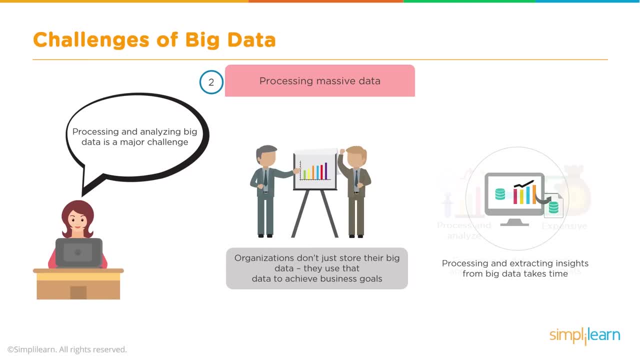 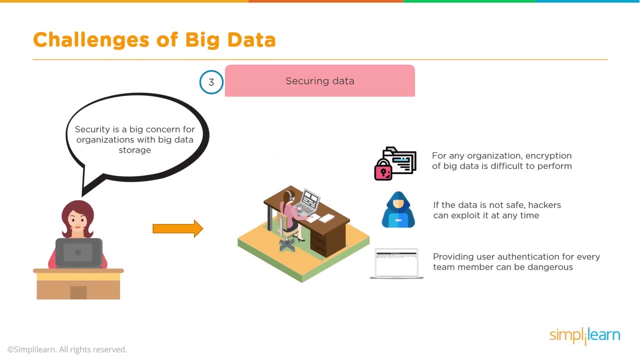 and until, However, there was an efficient solution to handle and process this big data. Securing the data- that's again a concern for organizations. right Encryption of big data is difficult to perform. If you would think about different compression mechanisms, then that would also mean decompressing. 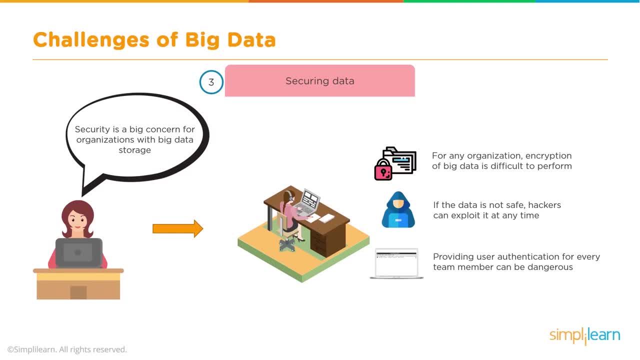 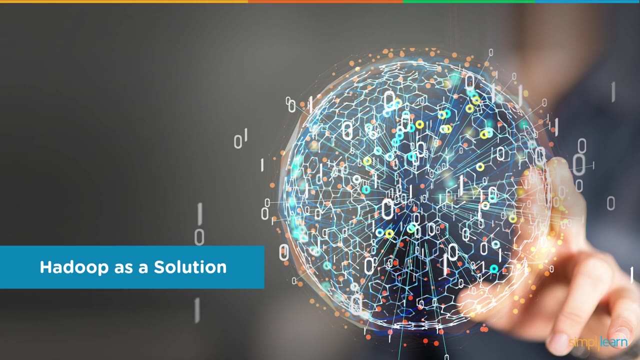 of data, which would also mean that you could take a hit on the CPU cycles or on disk usage, Providing user authentication for every team member. now, that could also be dangerous. So that led to Hadoop as a solution. So big data brings its own challenges. 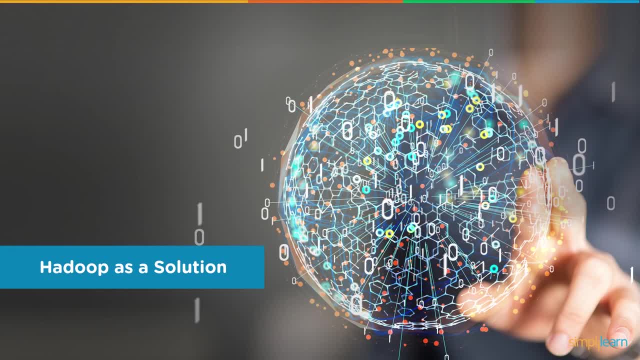 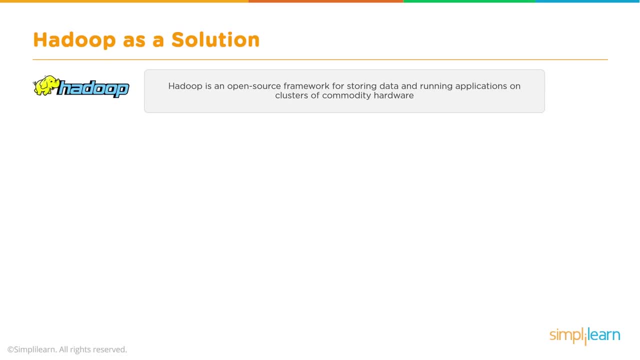 Big data brings its own benefits, And here we have a solution, which is Hadoop. Now, what is Hadoop? It's an open source framework for storing data and running applications on clusters of commodity hardware. Hadoop is an open source framework. 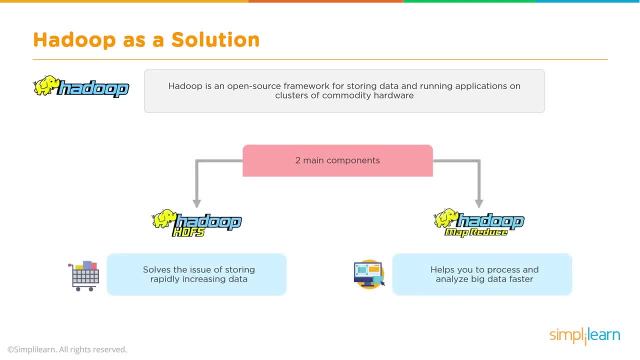 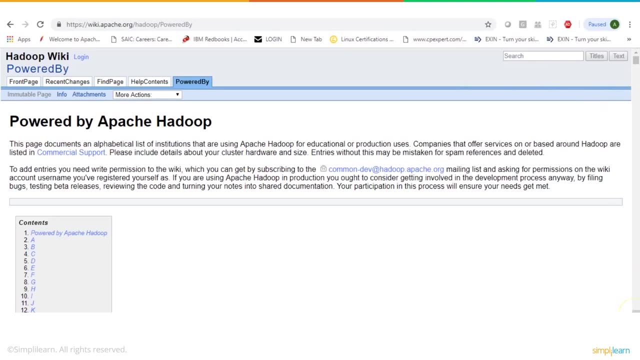 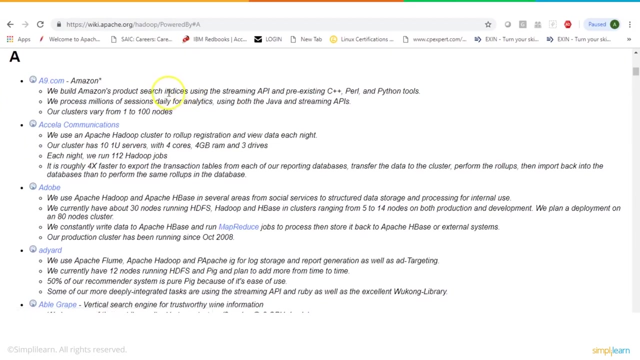 And before we discuss on two main components of Hadoop, it would be good to look into the link which I was suggesting earlier, That is, companies using Hadoop and any person who would be interested in learning big data should start somewhere here where you could list down different companies, what kind of 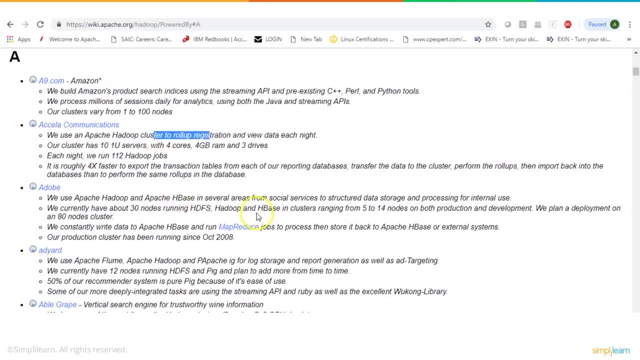 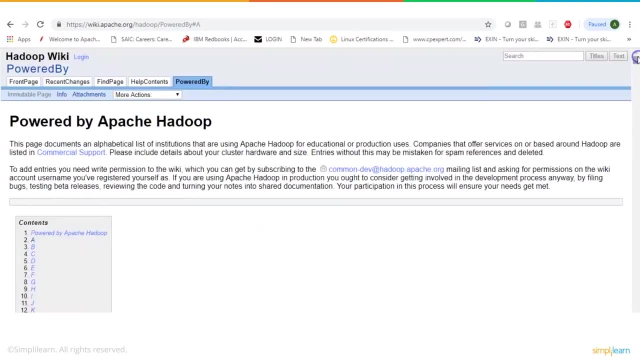 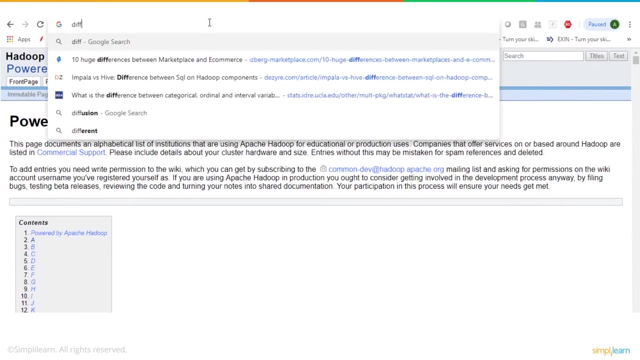 setup they have, why are they having Hadoop, what kind of processing they are doing and how are they using these so-called Hadoop clusters to process- and, in fact, store, capture and process- huge amount of data? Another link which I would suggest is looking at different distributions. 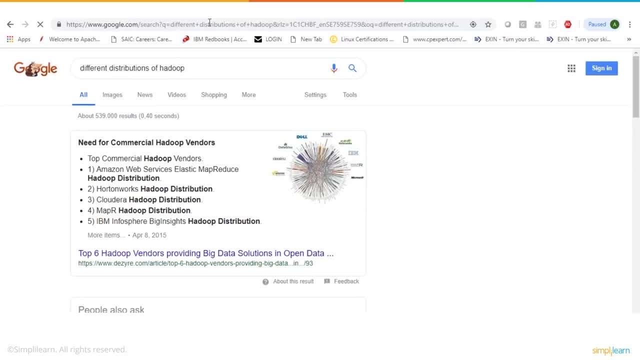 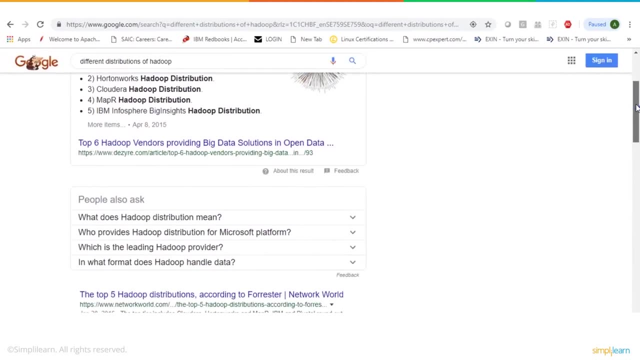 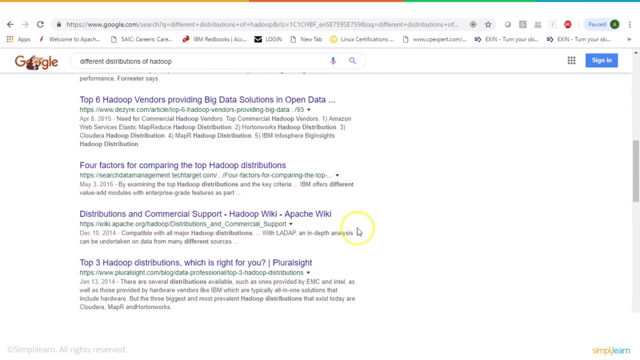 Distributions of Hadoop. Any person who is interested in learning big data should know about different distributions of Hadoop. Now in Linux we have different distributions like Ubuntu, CentOS, Red Hat, SUSE, DBN. In the same way, you have different distributions of Hadoop which we can look on the wiki page. 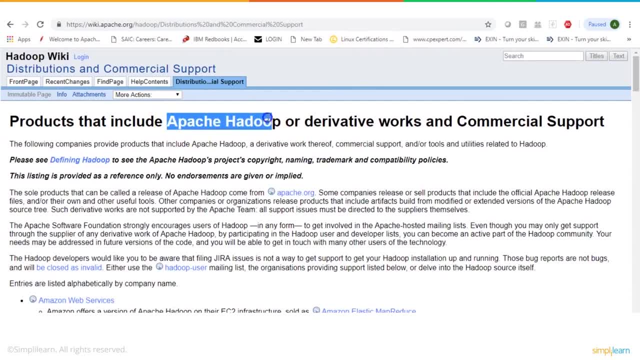 And this is the link which talks about products that include Apache Hadoop or Derivative Works and Commercial Support, Which basically means that Apache Hadoop is a distribution of Hadoop, Apache Hadoop. the sole products that can be called a release of Apache Hadoop come from: 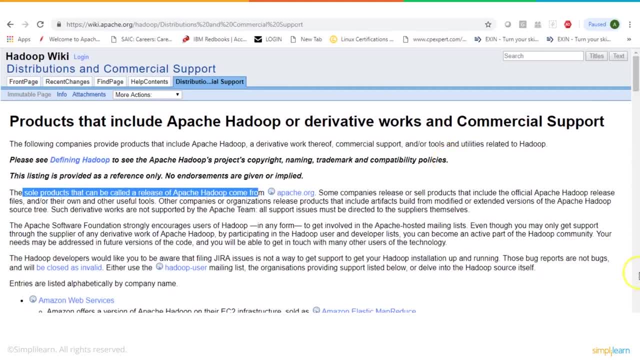 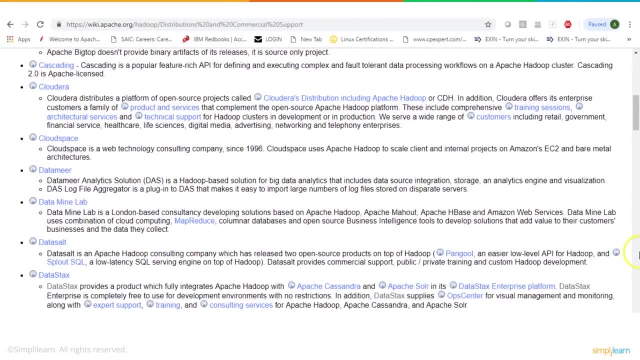 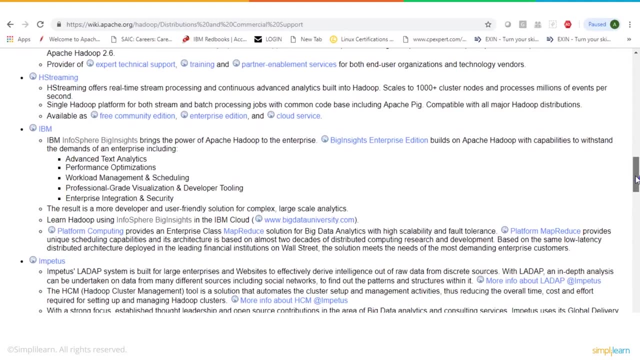 Apacheorg. That's an open source community, And then you have various vendor-specific distributions like Amazon Web Services. you have Cloudera, you have Hortonworks, you have IBM's Big Insight, you have MapR. all these are different distributions of Hadoop. 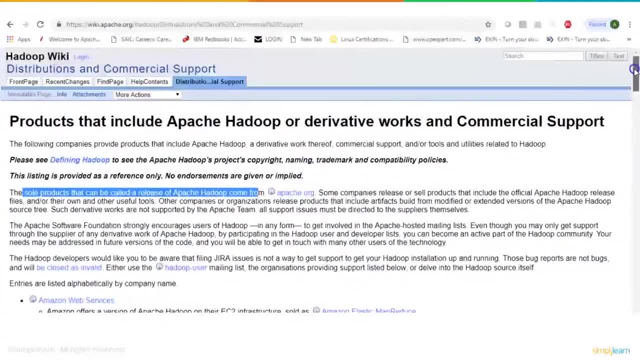 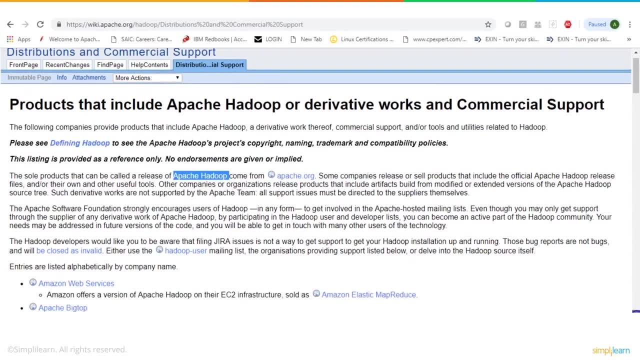 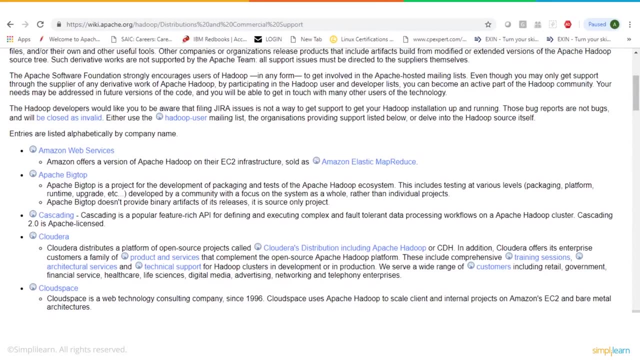 So basically, all of these vendor-specific distributions are depending or using on core Apache Hadoop. In brief, we can say that these are the vendors which take up Apache Hadoop, package it within a cluster management solution so that users who intend to use Apache Hadoop would not. 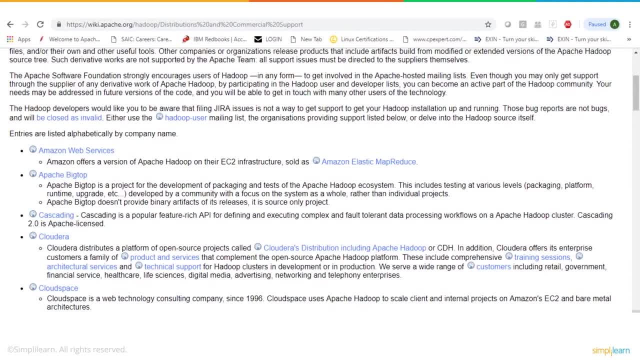 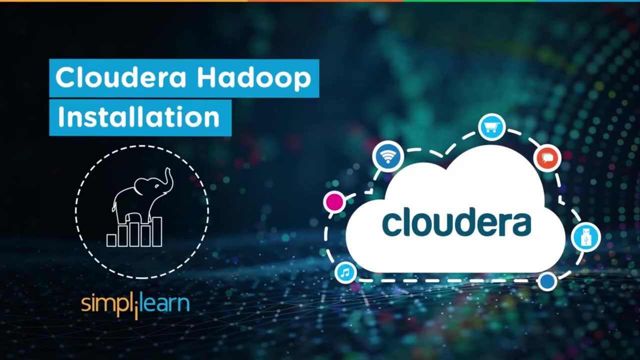 have difficulties of setting up a cluster, setting up a framework. They could just use a vendor-specific distribution with its cluster installation solutions, cluster management solution and easily plan, deploy, install and manage a cluster. Here is a quick summary, A quick demo on setting up Cloudera Quick Start VM. 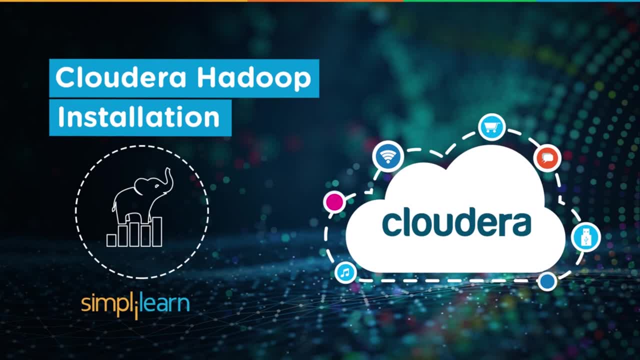 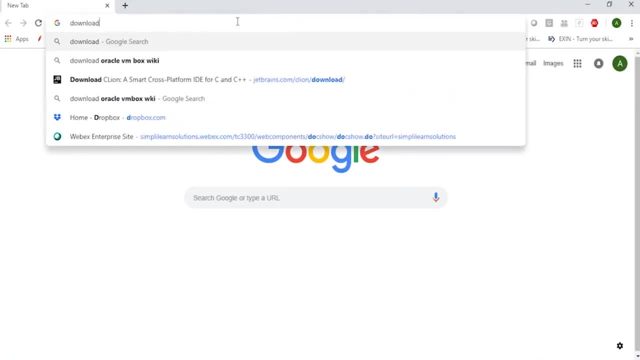 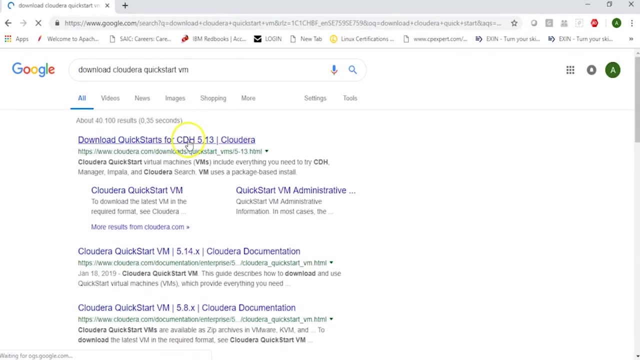 In case you are interested in working on a standalone cluster, you can download the Cloudera Quick Start VM. So you can just type in download Cloudera Quick Start VM and you can search for package Now. this can be used to set up a Quick Start VM, which would be a single node, Cloudera-based. 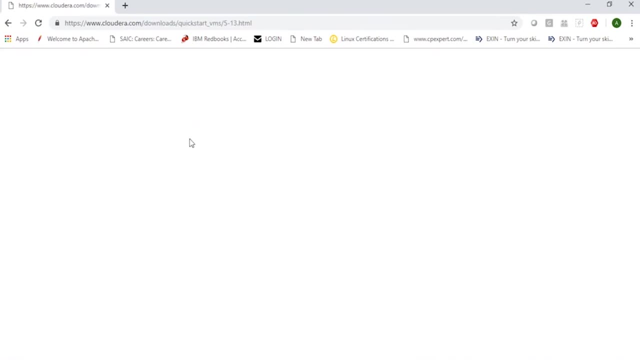 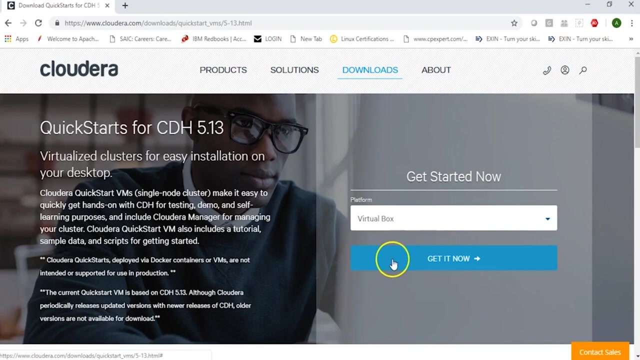 cluster, So you can click on this link And then, basically based on the platform Which you would be choosing to install, such as using a VM box, or which version of Cloudera you would install, So here I can select a platform, so I can choose virtual box, and then you can click on get. 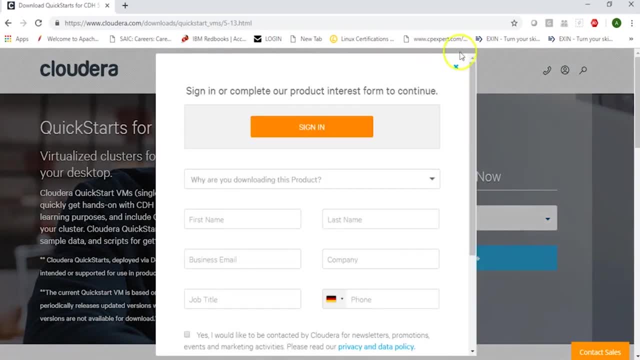 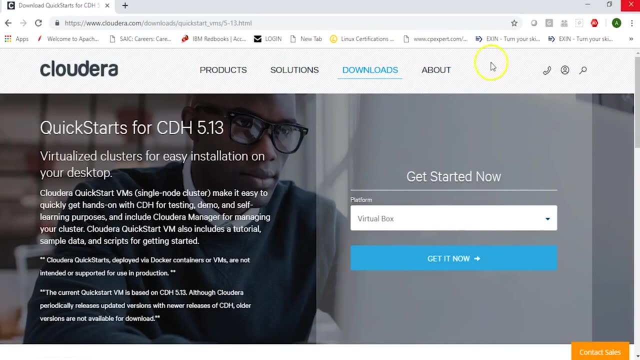 it now. So give your details and, basically, then it should allow you to download the Quick Start VM, which would look something like this, And once you have the zip file which is downloaded, you can unzip it, which can then be used to. 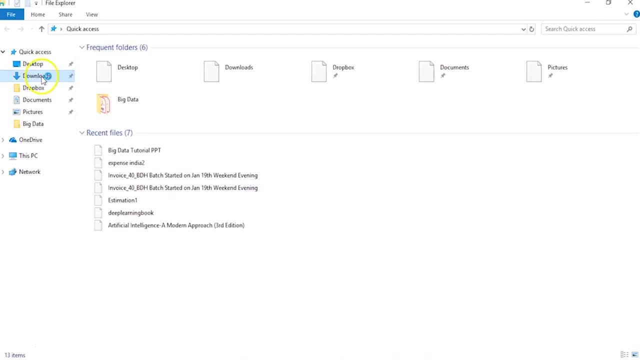 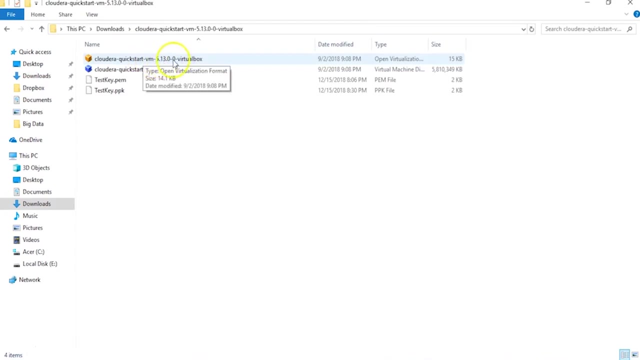 set up a single node Cloudera cluster. So once you have downloaded the zip file, that would look something like this: So you would have a Quick Start virtual box and then a virtual box disk. Now this can be used to set up a cluster. 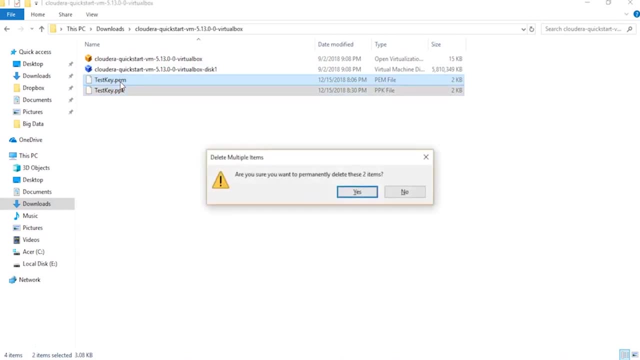 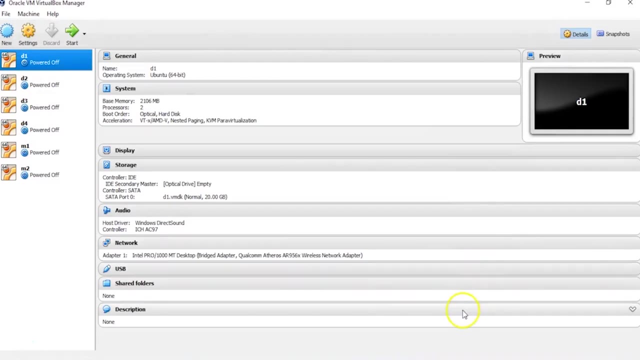 Ignore these files which are related to Amazon machines, and you don't need to have that, So you would just have this, and this can be used to set up a Cloudera cluster. So for this to be set up, You can click on file. 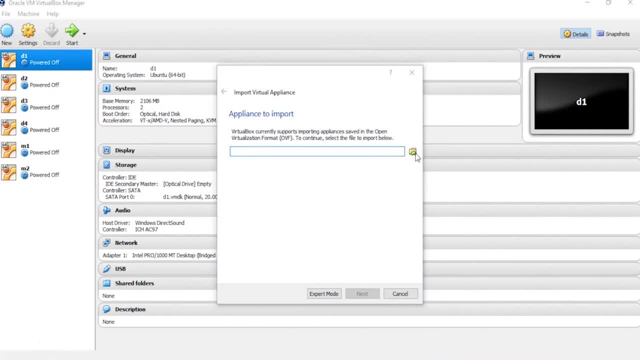 Import appliance and here you can choose your Quick Start VM by looking into downloads, Quick Start VM. select this and click on open. Now you can click on next and that shows you the specifications of CPU RAM, which we can then change later, and click on import. 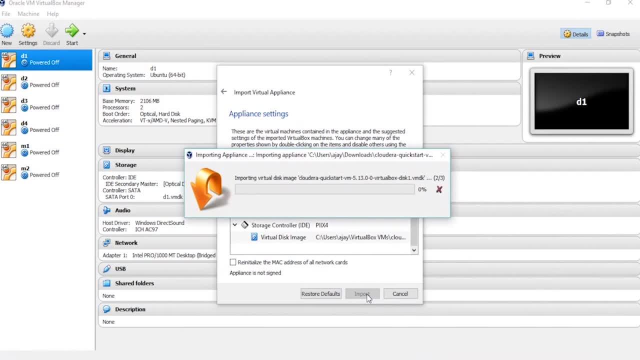 This will start importing virtual disk image dot VMDK file into your VM box. Once this is done, We will have to change the specifications of machines to use two CPU cores minimum and give a little more RAM, because Cloudera Quick Start VM is very CPU intensive and it needs. 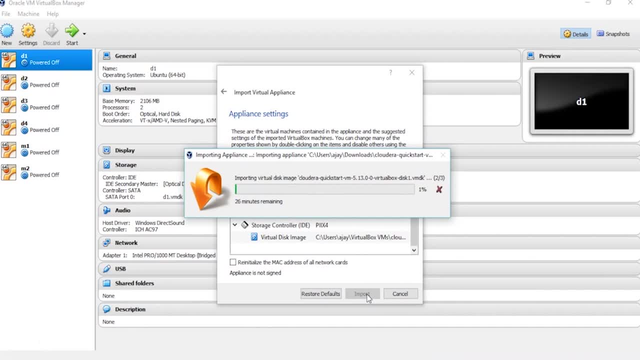 good amount of RAM. So to survive, I will give two CPU cores and 5 GB RAM, and that should be enough for us to bring up a Quick Start VM which gives us a Cloudera distribution of Hadoop in a single node cluster setup which can be used for working, learning about different distros. 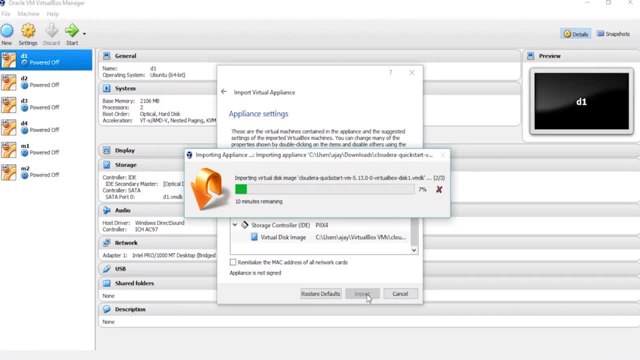 and so on. You can see the distributions in Cloudera clusters working with SDFS and other Hadoop ecosystem components. Let's just wait for this importing to finish and then we will go ahead and set up a Quick Start VM for our practice. 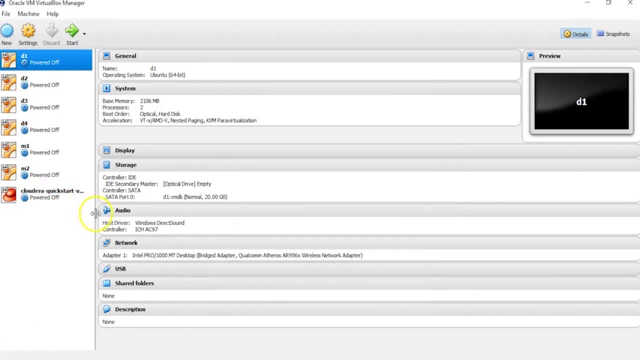 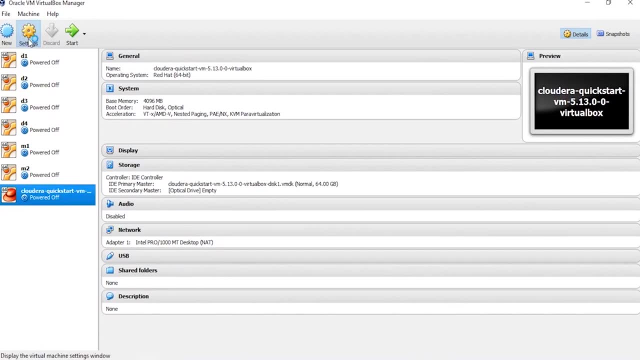 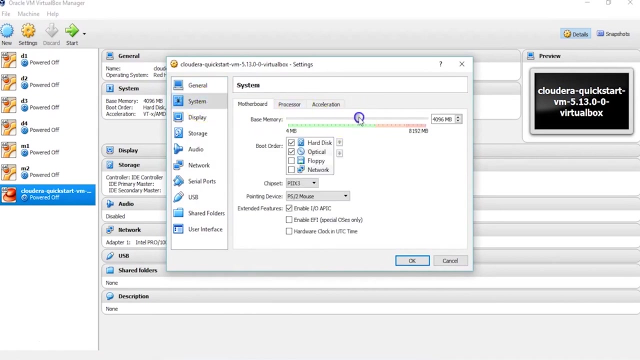 Here the importing of appliance is done and we see Cloudera Quick Start machine is added to my list of machines. I can click on this and click on settings. As mentioned, I would like to give it more RAM and more CPU cores. So click on system and here let's increase the RAM to at least 5, and click on processor. 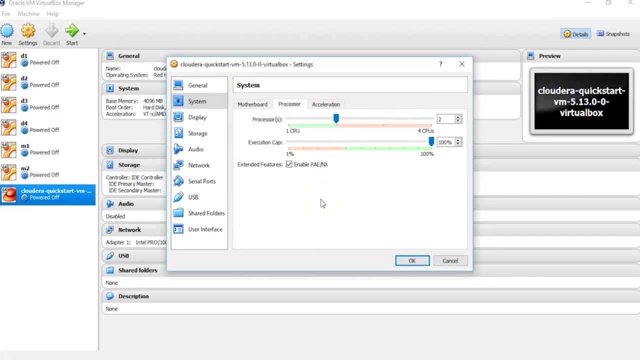 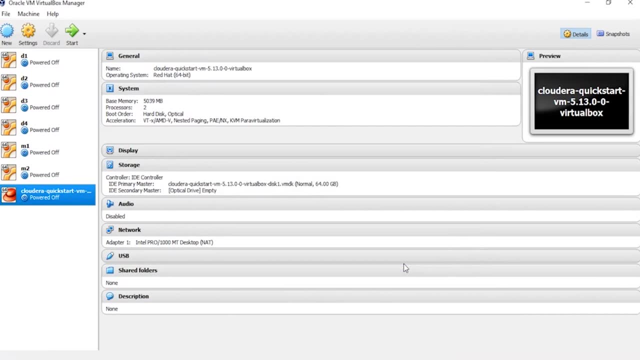 and let's give it two CPU cores, which would at least be better than using one CPU core Network. it goes for NAT and that's fine. Click on OK, and we would want to start this machine so that it uses two CPU cores. 5 GB. 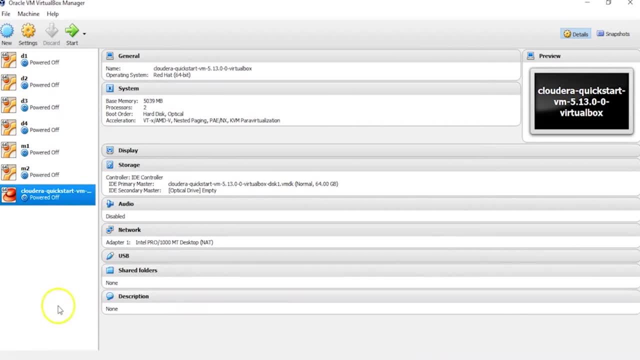 RAM and it should bring up my Cloudera Quick Start VM. Now let's go ahead and start this process. So let's go ahead and start this machine, which has our Quick Start VM. It might take initially some time to start up because internally there will be various 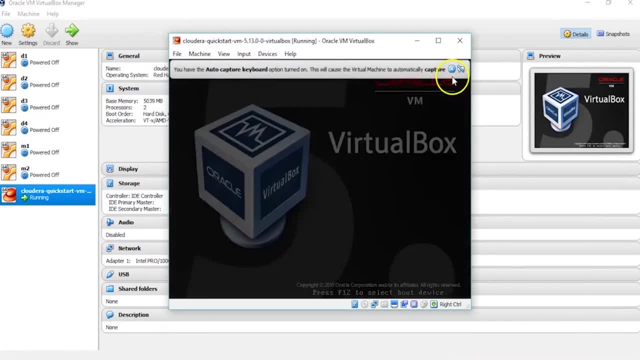 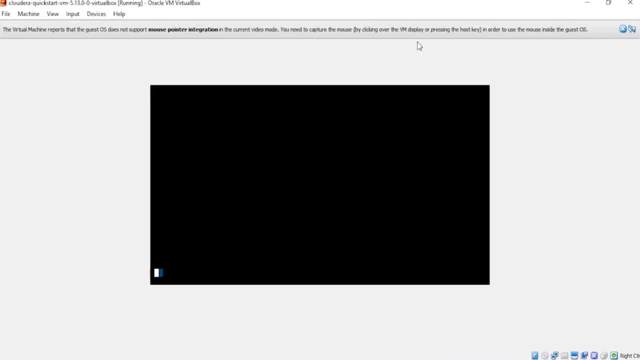 Cloudera services which will be starting up and those services need to be up for our Cloudera Quick Start VM to be accessible. So, unlike your Apache Hadoop cluster, where we start our cluster and we will be starting all our processes, in case of Cloudera, it is your Cloudera SCM server and agents which 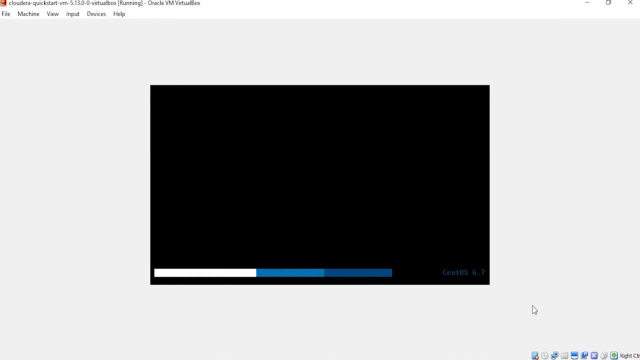 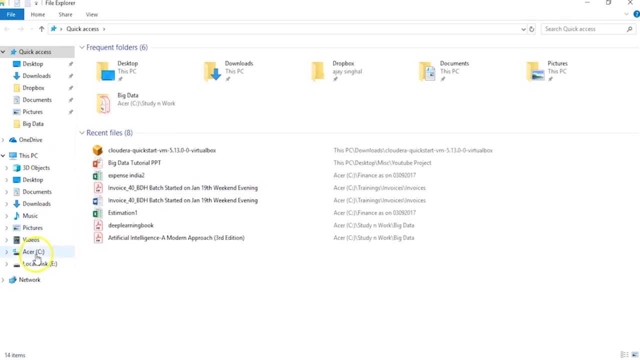 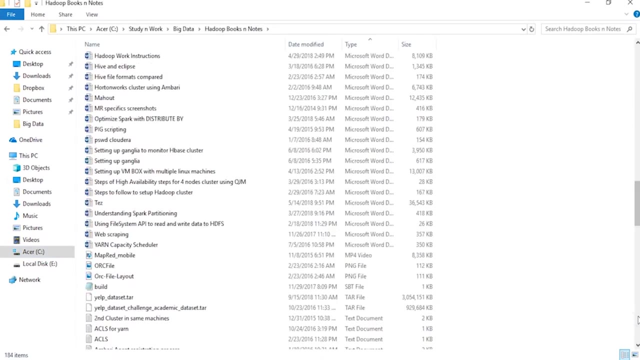 take care of Starting up of your services and starting up of your different roles for those services. I explained in my previous session that for a Cloudera cluster it would be these services. Let me just show you that. So in case of Apache cluster, we start our services, that is, we start our cluster by 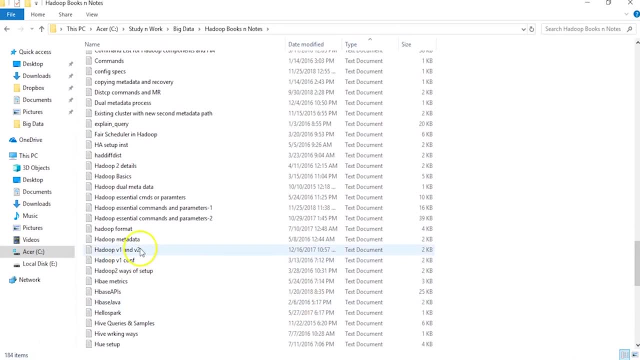 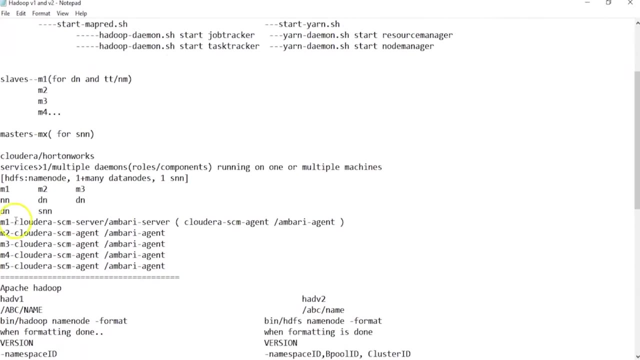 running script and then basically those scripts will individually start the different processes on different nodes. In case of Cloudera, We would- We would always have a Cloudera SCM server which would be running on one machine and then, including that machine, we would have Cloudera SCM agents which would be running. 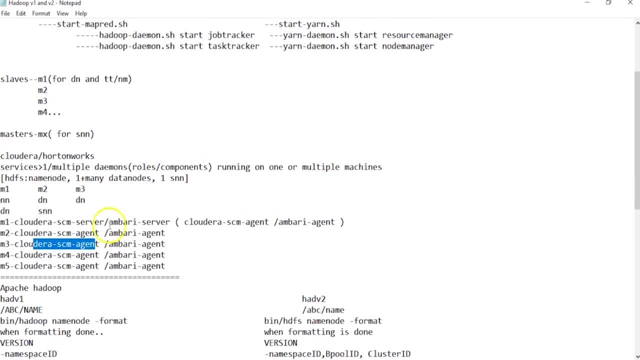 on multiple machines. Similarly, if we had a Hortonworks cluster, we would have Ambari server starting up on the first machine and then Ambari agents running on other machines. So your server component knows what are the services which are set up, what are their. configurations, And agents running on every node are responsible To send heartbeats to the server, receive instructions and then take care of starting and stopping off of individual roles on different machines. In case of our single node cluster set up in quick start VM, we would just have one. 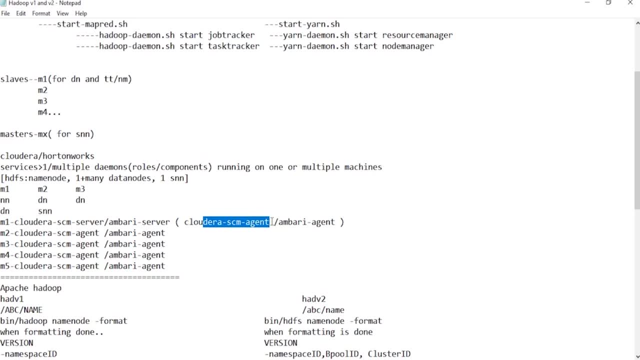 SCM server and one SCM agent which will start on the machine, which will then take care of all the roles which need to be started for your different services. So we will just wait for our machine to come up. And basically, we will just wait for our machine to come up. 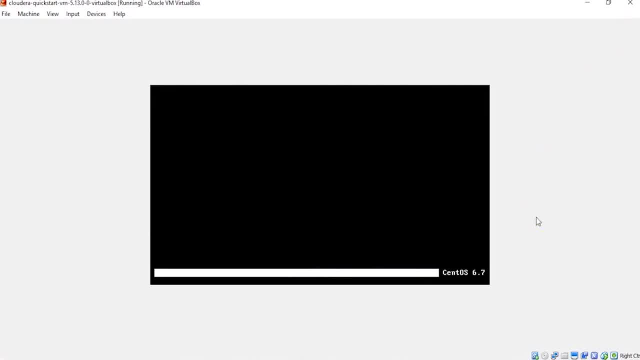 And basically we will just wait for our machine to come up And basically we will just wait for our machine to come up. So we will just wait for our machine to come up And basically we will just wait for our machine to come up. 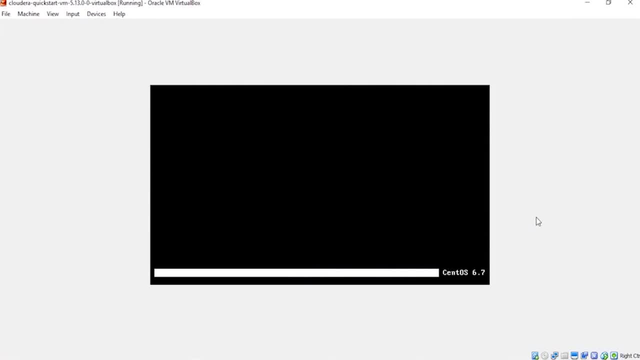 And basically, we will just wait for our machine to come up. And we will just wait for our machine to come up And once we have that, we need to follow few steps so that we can have the Cloudera admin console accessible, which allows you to browse the cluster. look at different services. look. 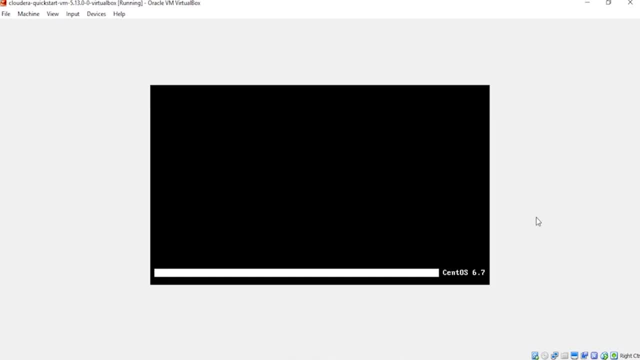 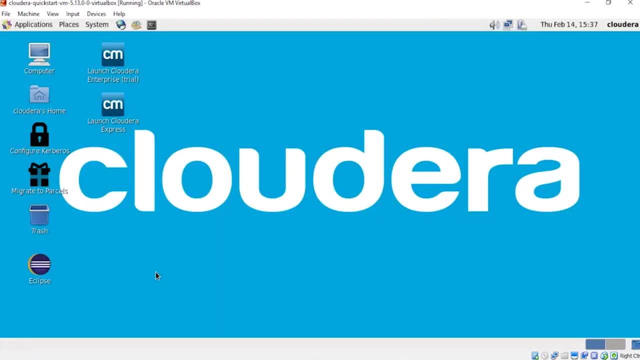 at the roles for different services and also work with your cluster either using command line or using the web interface that is Hue. Now that my machine has come up and it already is connected to the internet, which we can see here, We need to do certain things so that we can have our admin console. 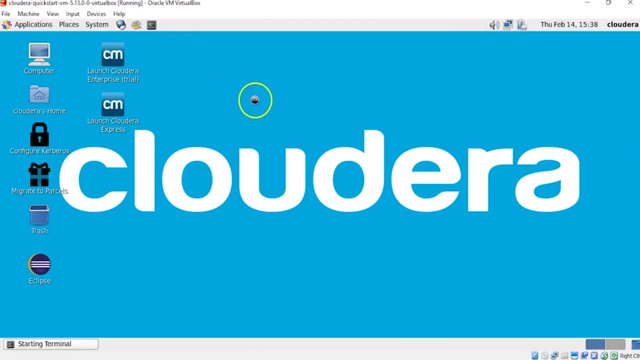 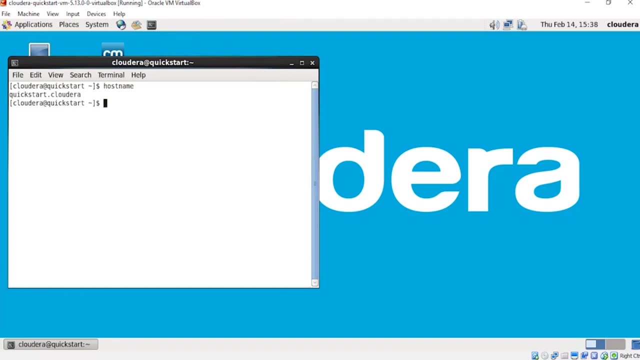 accessible At this point of time. you can click on terminal and check if you have access to the cluster. So here type in host name and that shows you your host name, which is quickstartcloudera. We can also type in HDFS command to see if we have access and if my cluster is working. These: 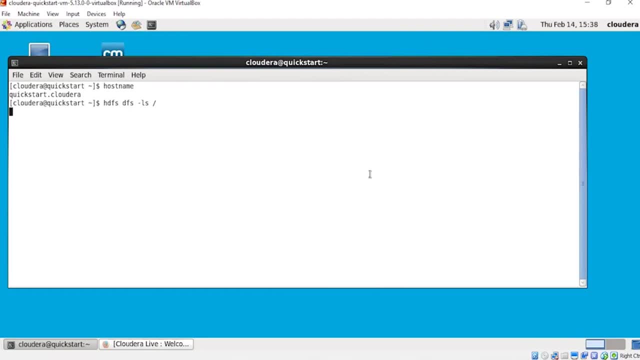 commands are same as you would give them in a Apache Hadoop cluster or in any other distribution of Hadoop. Sometimes, when your cluster is up and you have access to the terminal, it might take few seconds or few minutes before there is a connection established between clouderascm. 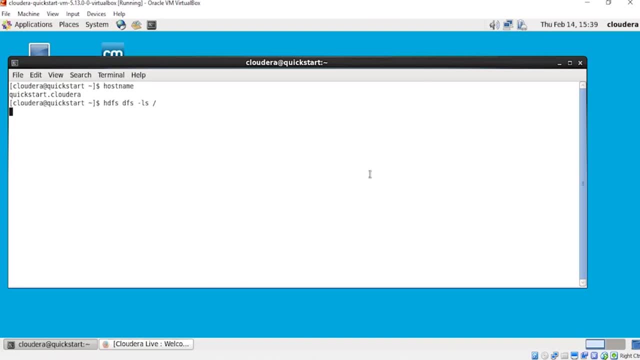 server and clouderascm agent running in the background which takes care of your cluster. I have given a HDFS DFS list command which basically should show me what by default exists. Let's just give it a couple of seconds before it shows us the output. We can also check by giving: 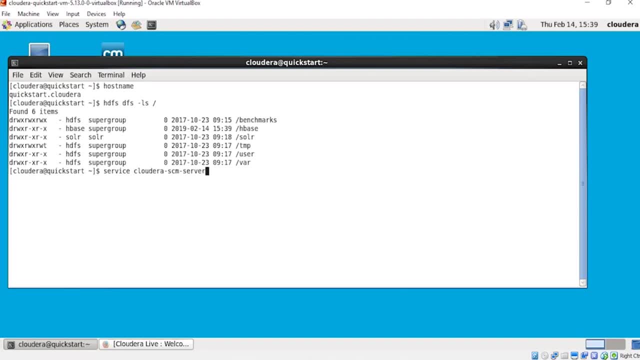 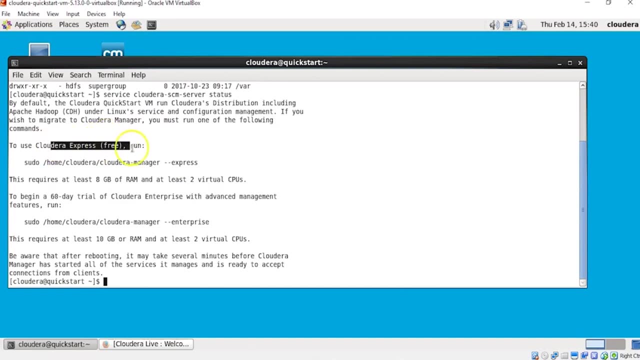 a service, clouderascm server status. And here it tells me that if you would want to use cloudera express, free, run this command. It needs 8GB of RAM and at least two virtual CPU cores, And it also mentions it may take several minutes before cloudera manager has started. 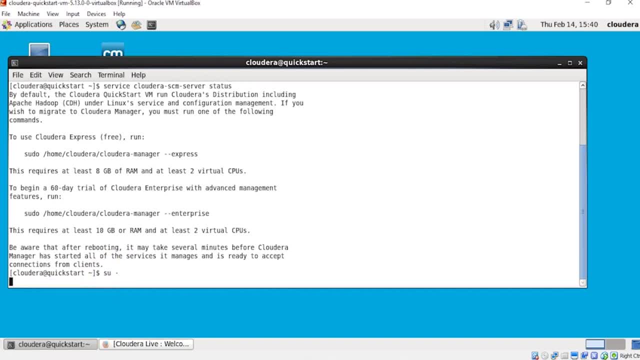 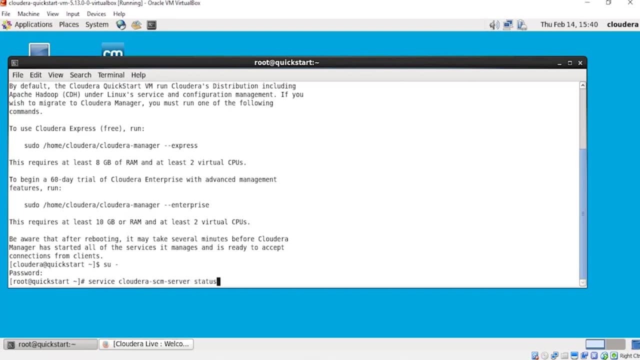 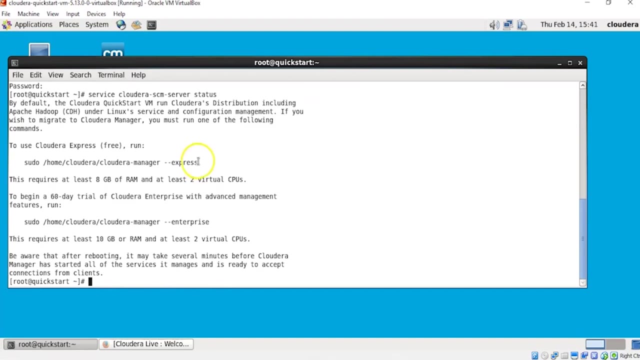 I can log in as root here and then give the command service clouderascm server status. Remember, the password for root is cloudera. So it basically says that if you would want to check the settings, it is good to have express edition running so we can close this. My HDFS access is: 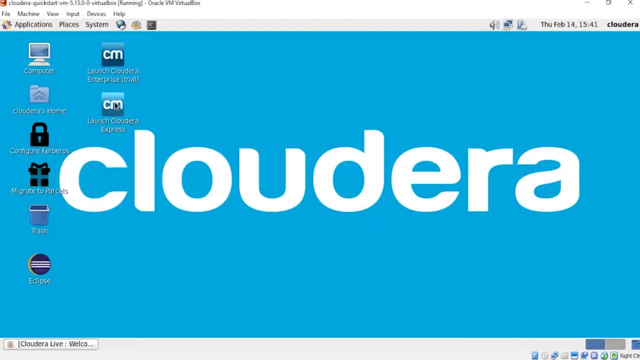 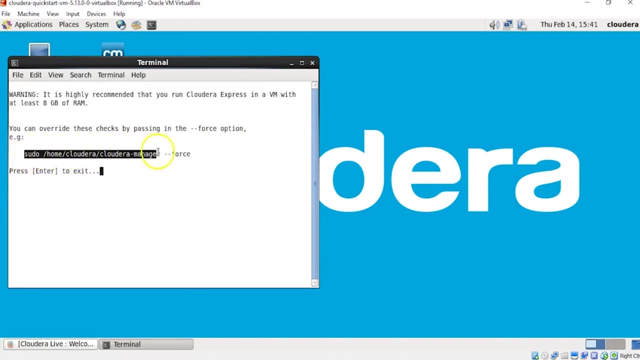 working fine. Let's close the terminal And here we have launch clouderaexpress. Click on this and that will give you That you need to give a command which is force. Let's copy this command. Let's open up a different. 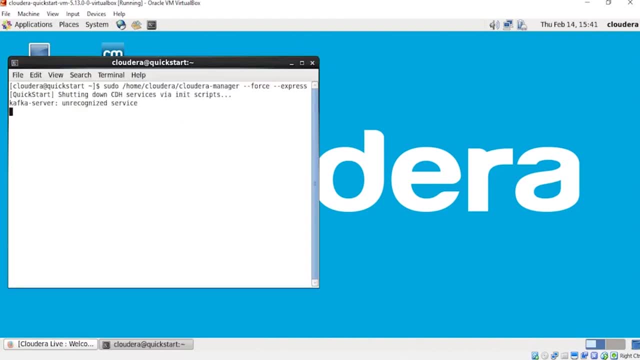 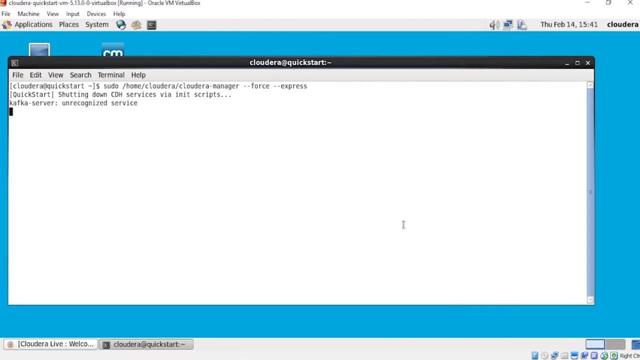 terminal and let's give this command like this, which will then go ahead and shut down your cloudera based services, and then it will restart it, only after which you will be able to access your admin console. So let's just give it a couple of minutes before it does this, and then we will have access to our 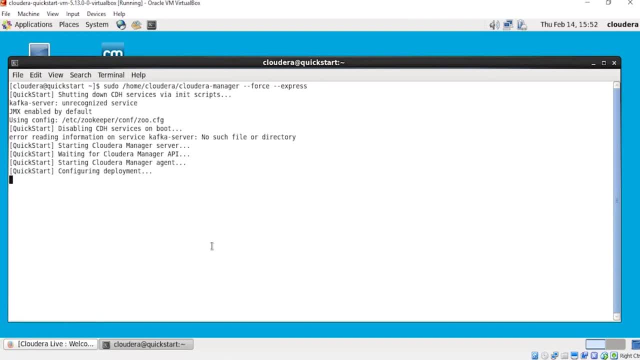 admin console here. If you see, it is Starting the clouderamanager server again. it is waiting for clouderamanager API, then starting the clouderamanager agents and then configuring the deployment as per the new settings which we have given as to use the express edition of cloudera. 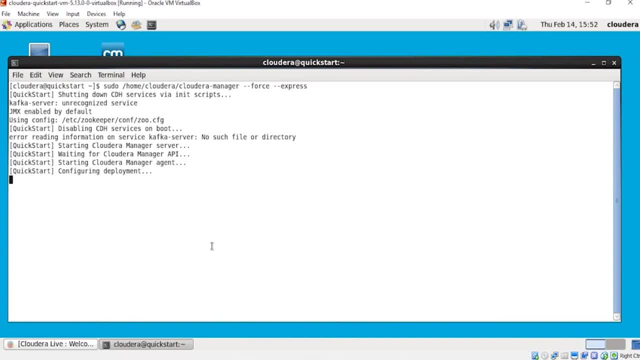 Once all this is done, it will say the cluster has been restarted and the admin console can be accessed by ID and password as cloudera. We'll give it a couple of more minutes and once this is done, we are ready to use our admin console. 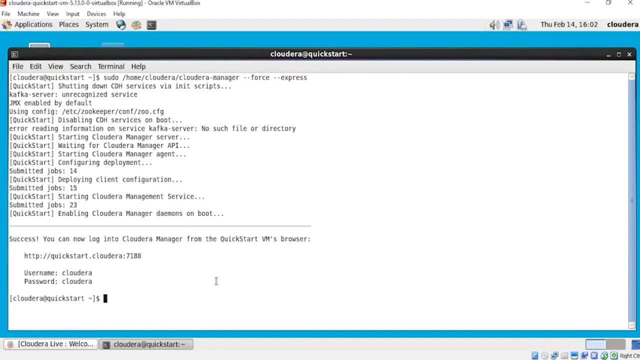 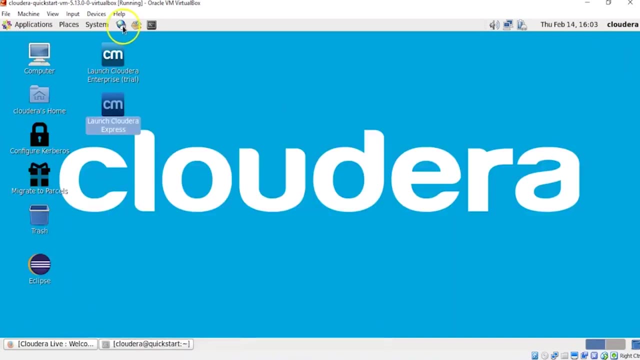 Now that deployment has been configured, client configurations have also been deployed and it has restarted the clouderamanager service. It gives you an access to quick start admin console using username and password as cloudera. Let's try accessing it so we can open up the browser here and let's change this to 7180. 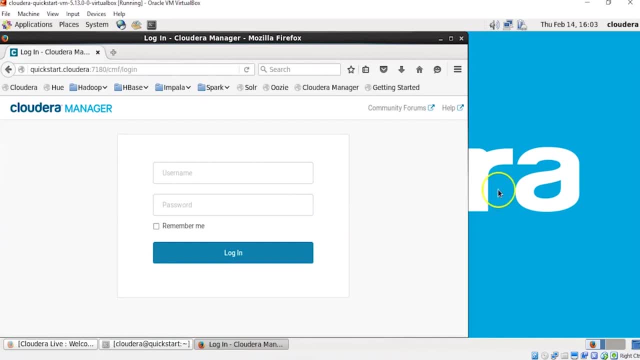 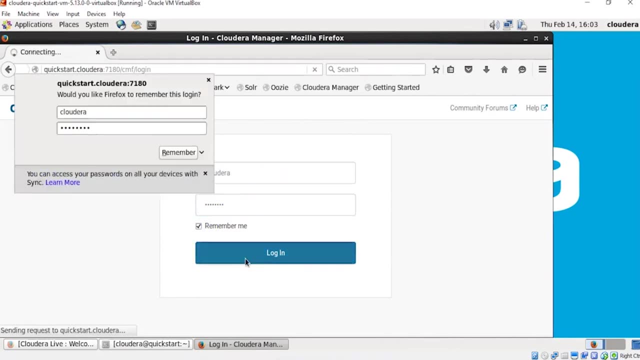 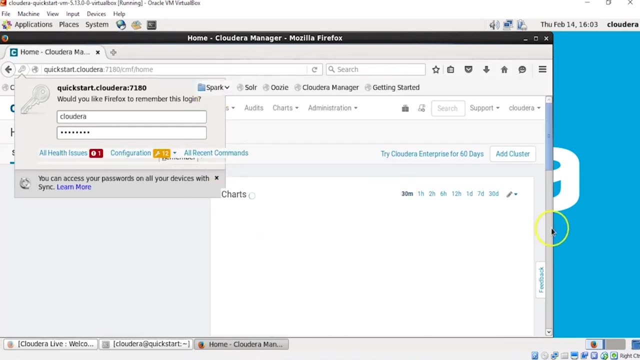 That's the default port and that shows the admin console- admin console Which is coming up now. here we can log in as cloudera cloudera and then let's click on login Now. as I said, cloudera is very CPU intensive and memory intensive, so it would slow down, since we have not given enough. 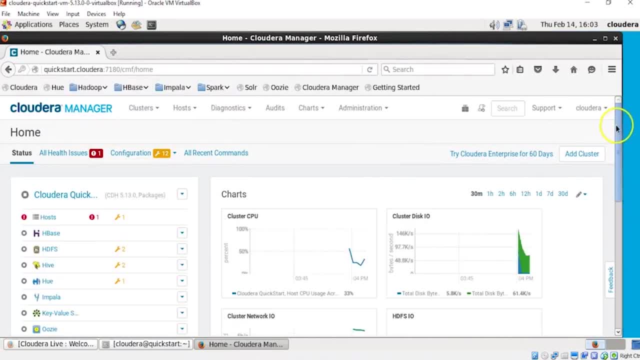 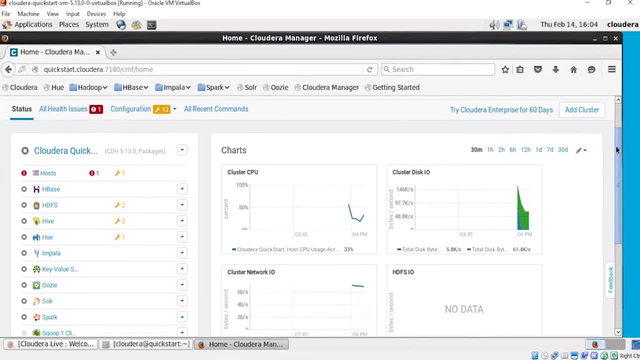 gb ram to our cloudera cluster, and thus it will be advisable to stop or even remove the services which we don't need Now. as of now, if we look at the services, all of them look in a stop status, and that's good. 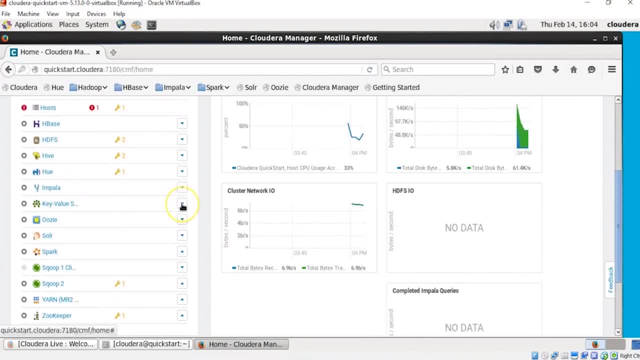 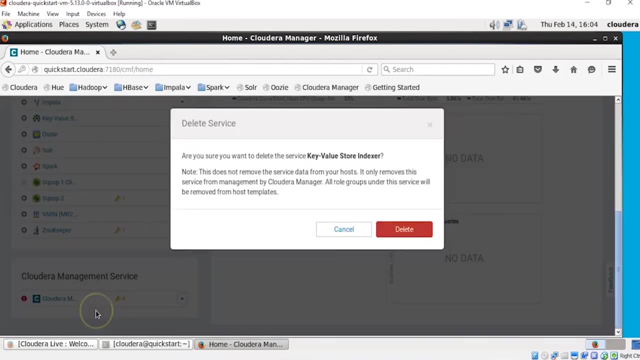 In one way because we can then go ahead and remove the services which we will not use in the beginning and later. we can anytime add services to the cluster. So, for example, I can click on key value store here and then I can scroll down where it says delete to remove this service from the admin console. 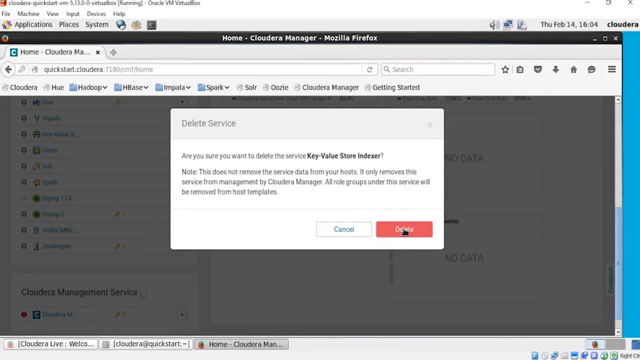 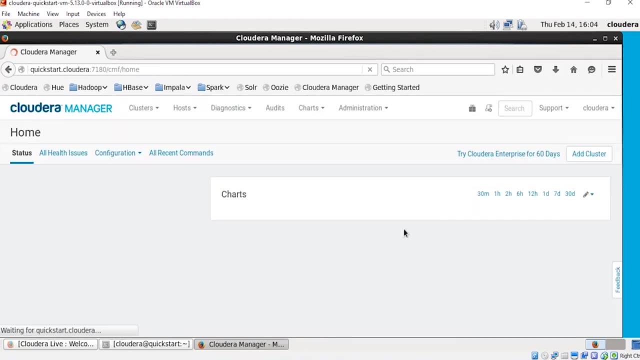 Now, anytime you're removing a particular service, it will only remove the service from the management by clouderamanager. all the role groups under this service will be removed from host templates, so we can click on delete Now. if this service was depending on some other service, it would have prompted me with a message that remove the relevant services on which this particular service depends. 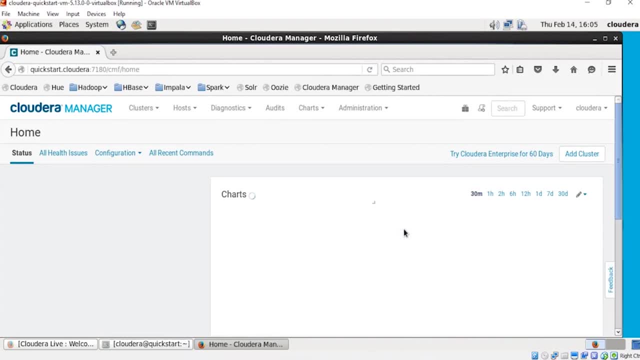 If the service was already running, then it would have given me a message that the service has to be stopped before it can be deleted from the cloudera admin console. Now this is my admin console, which allows you to click on services. look at the different roles and processes which are running for. 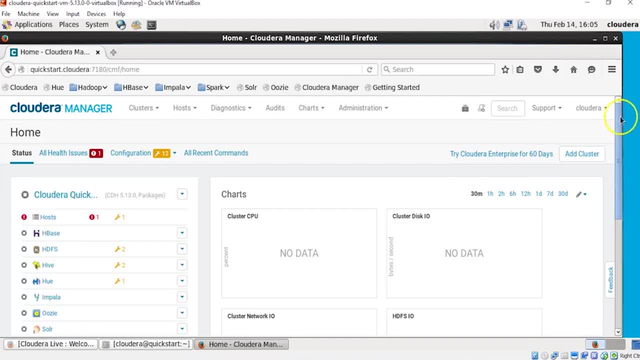 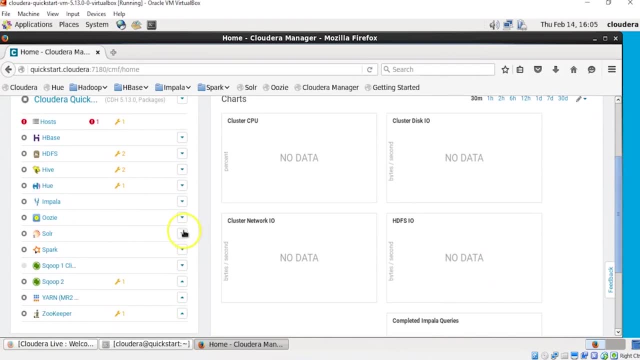 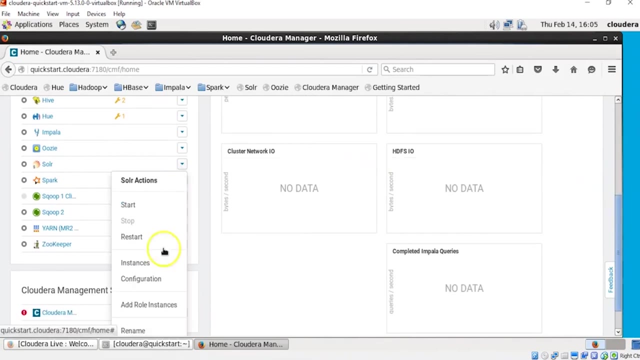 This service. we anyways have access to our cloudera cluster from the terminal using our regular HDFS or YARN or MapRed commands. Now I removed a service. I will also remove Solar, which we will not be using for the beginning, but then it depends on your choice. 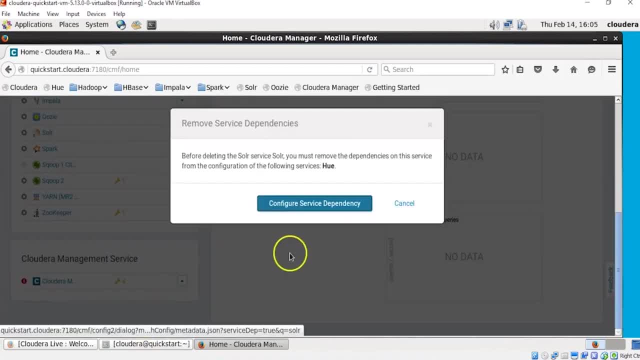 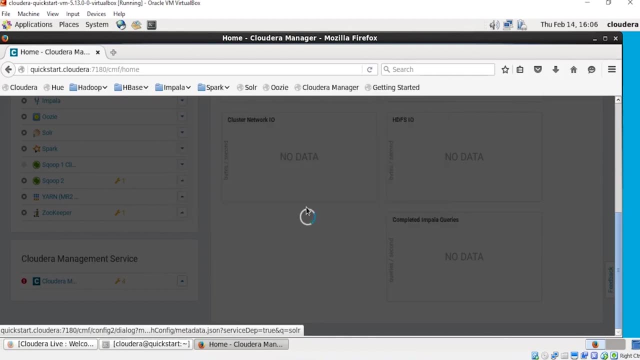 So we can here scroll down to delete it. And that says that before deleting the Solar service, you must remove the dependencies on the service from the configuration of following services. That is Hue Now. Hue is a web interface which allows you to work with your HDFS, and that is depending on this. 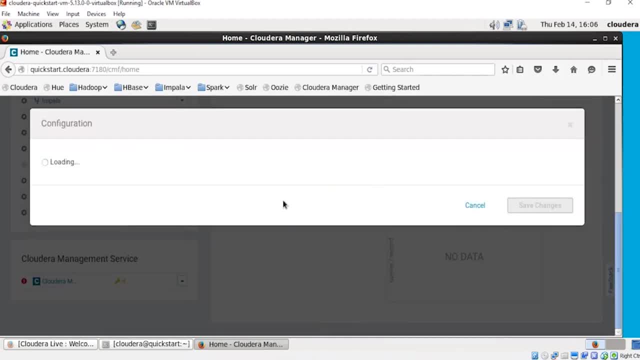 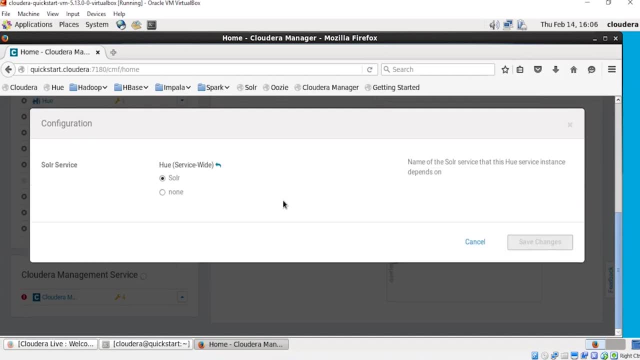 So click on configure service dependency, and here we can make sure that our Hue service does not depend on a particular service we are removing, so that then we can have a clean removal of the service. So I'll click on none and I will say save changes. 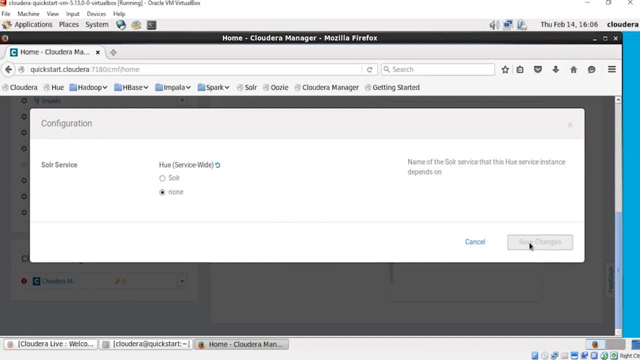 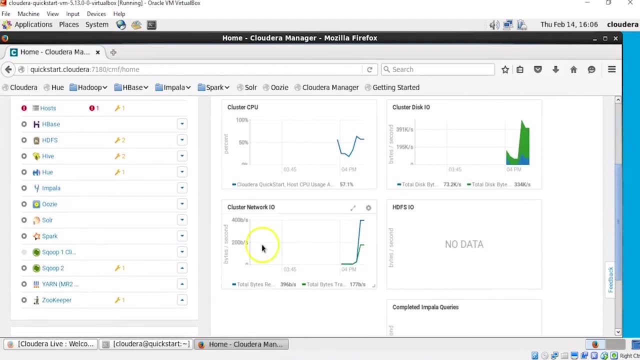 Once this is done, then we can go ahead and try removing the Solar service from our admin console, which will reduce some load On my management console, which will also allow me to work faster on my cluster. Now here we have removed the dependency of Hue on Solar. 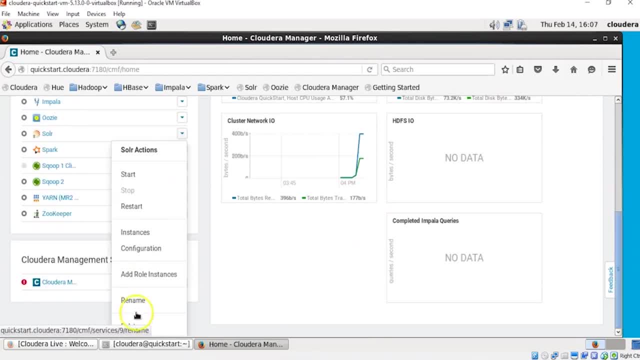 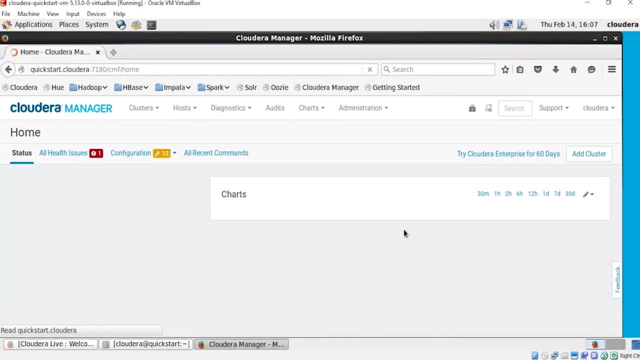 So we can click on this and then we can delete it. Remember, I'm only doing this so that my cluster becomes a little lighter and I can work on my focus services at any point of time. If you want to add more services to your cluster, you can anytime do that. 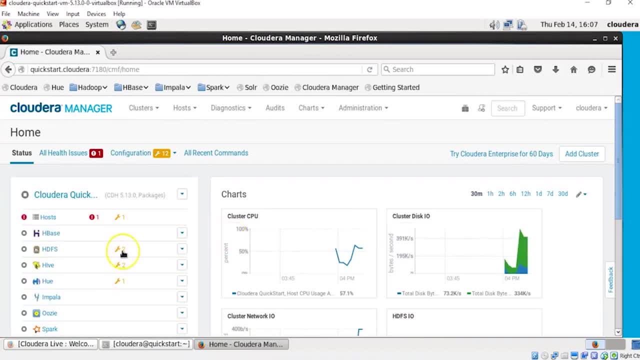 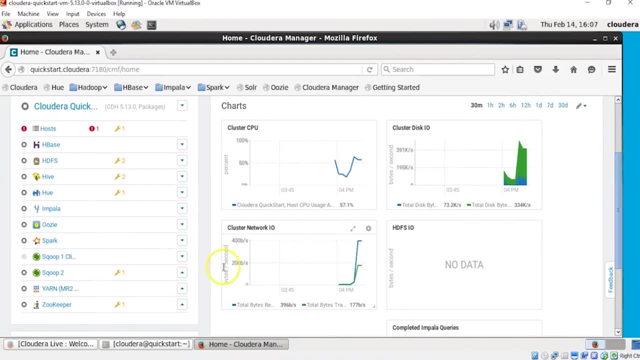 You can fix different configuration issues Like what we see here. We have different warning messages and here we have these services which are already existing. Now, if we don't need any of the service, I can click on the dropdown and click on delete. 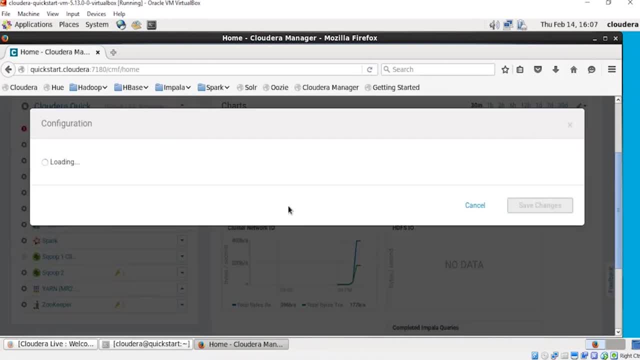 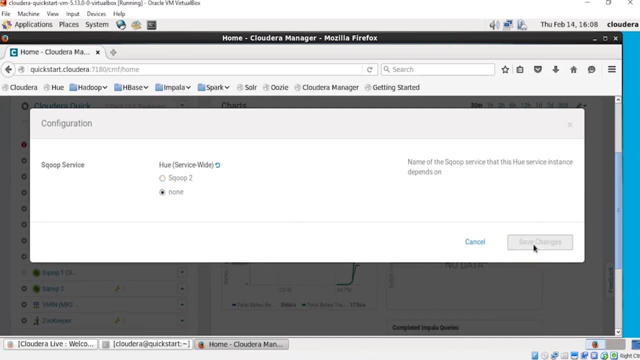 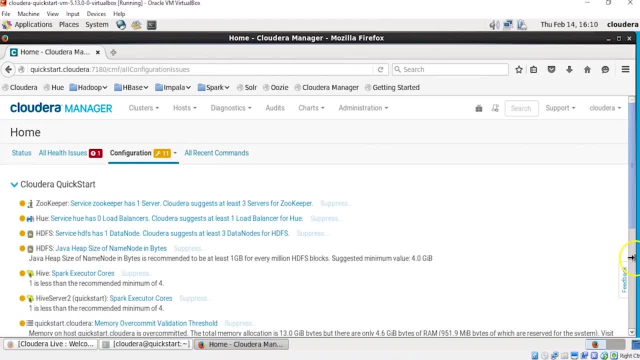 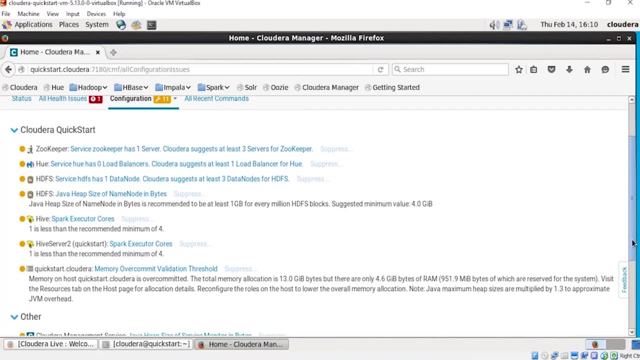 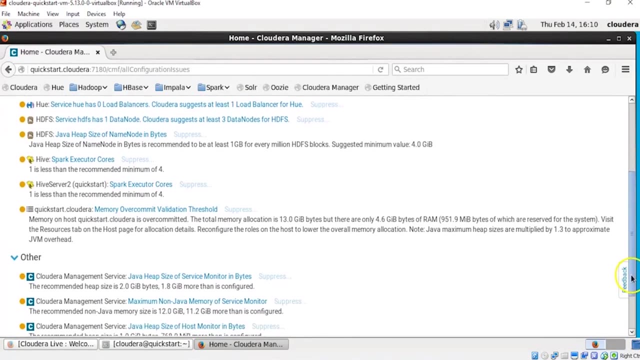 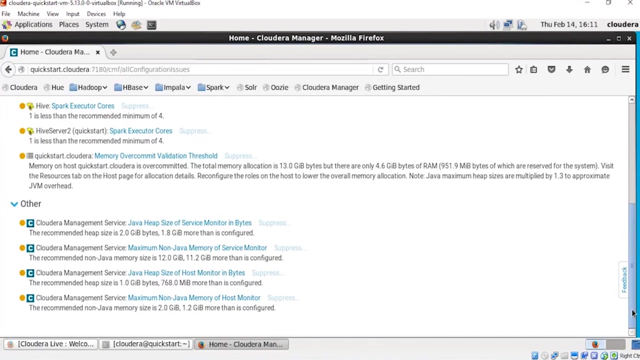 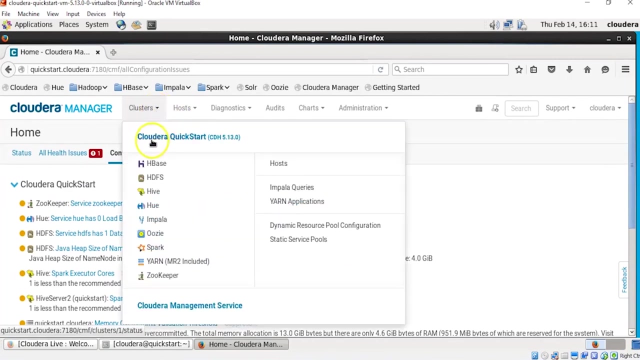 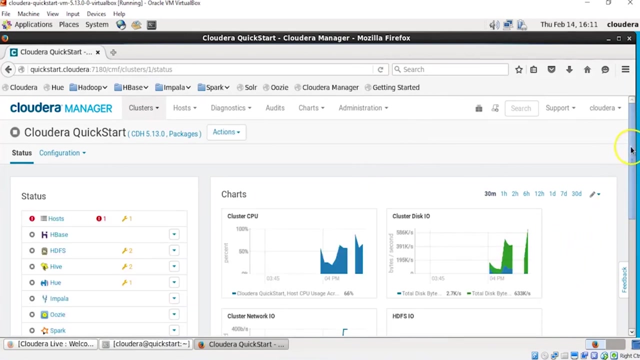 Now this is a cluster to which you can add services. Now, this is a cluster to which you can add services. click on cluster and basically we can look at the services. so we have removed some services which we don't intend to use. now I have also suppressed a offset. 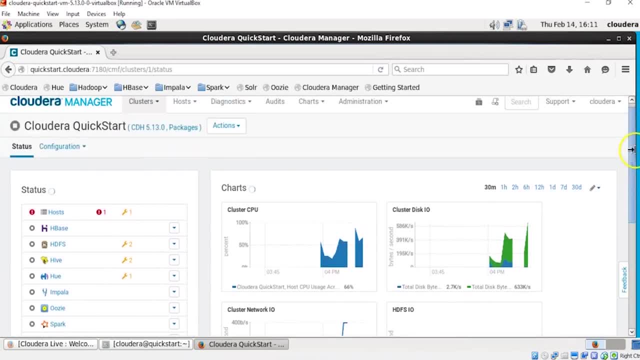 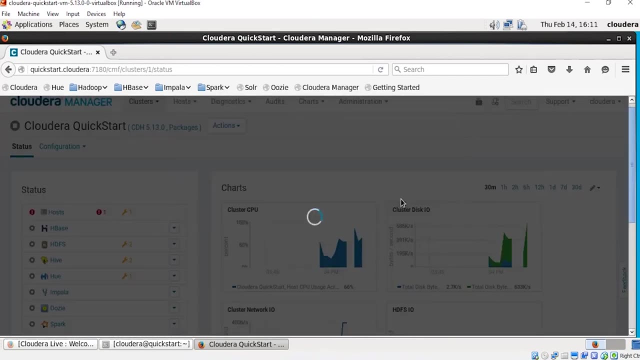 warning, which is not very critical for my use case, and basically I am good to start the cluster at any point of time. as I said, if you would want to add services, this is the actions button which you can use to add service. so we will just say restart my cluster, which will restart all the services one by one. 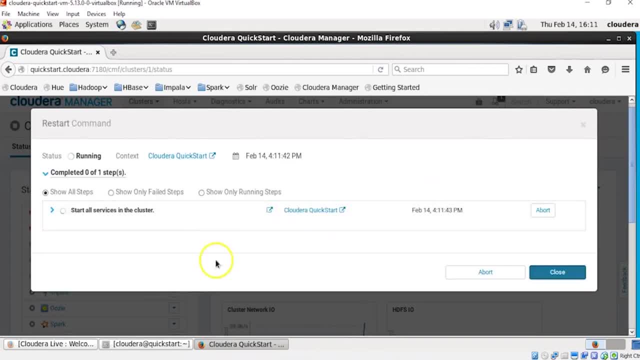 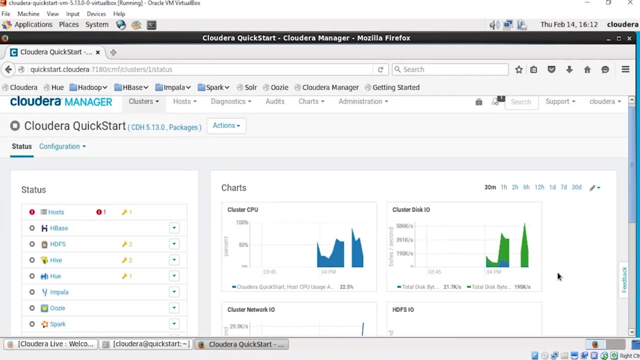 starting from zookeeper as the first service to come up. we can always click on this arrow mark and see what is happening in the services, what services are coming up and in which order. if you have any issues, you can always click on the link next to it, which will take you to the logs, and we can click on close to. 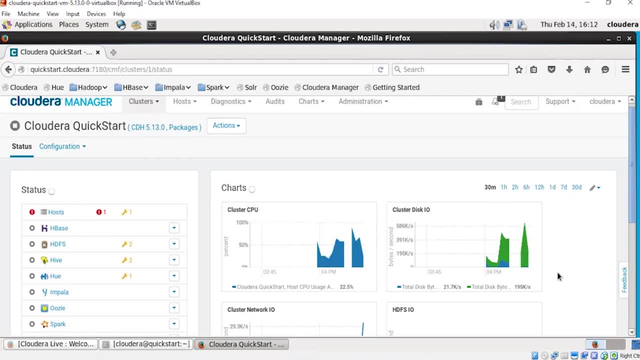 let it happen in the background. so this will basically let my services restart one by one and my cluster will then become completely accessible, either using hue as a web interface or quickstart terminal, which allows you to give your commands. now, while my machines are coming up, you can click on hosts and you can have a look at all the 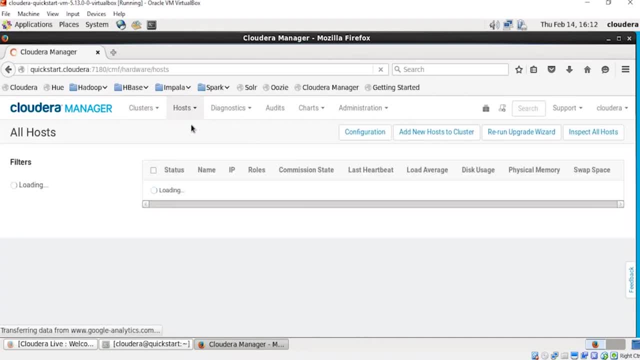 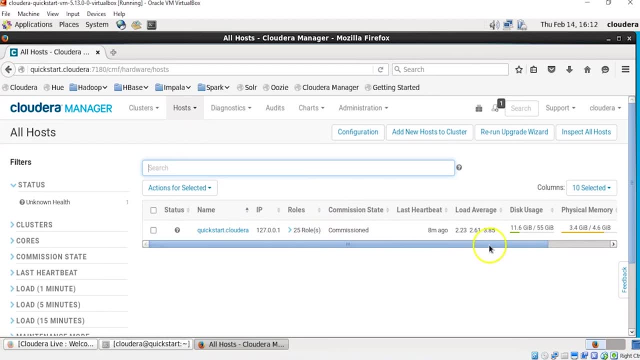 hosts, we have, as of now, only one, which will also tell you how many roles or processes are running on this machine. so that is 25 roles. it tells you what is the disk usage, it tells you what is the physical memory being used and using this host tab, we can add new host to the cluster, we can check the configuration, we 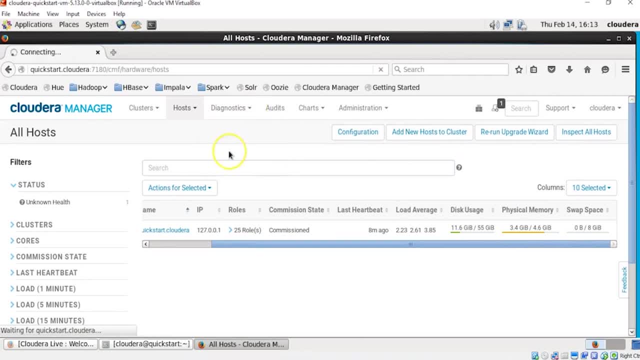 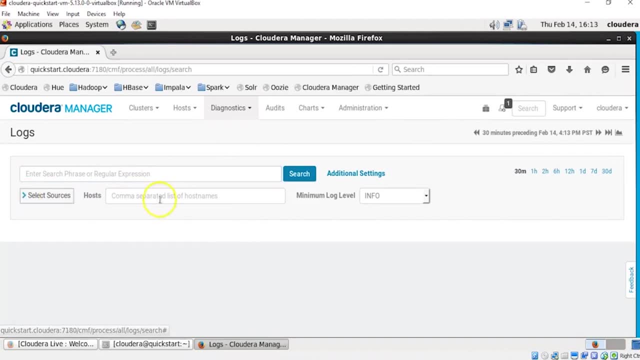 can check all the hosts in Diagnostics. you can look at the logs, which will give you access to all the logs. you can even select the sources from which you would want to have the logs, or you can give the host name. you can click on search. you can build your own charts. you can also do the admin stuff by adding. 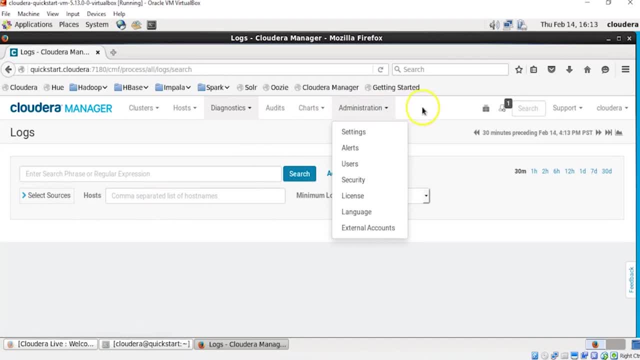 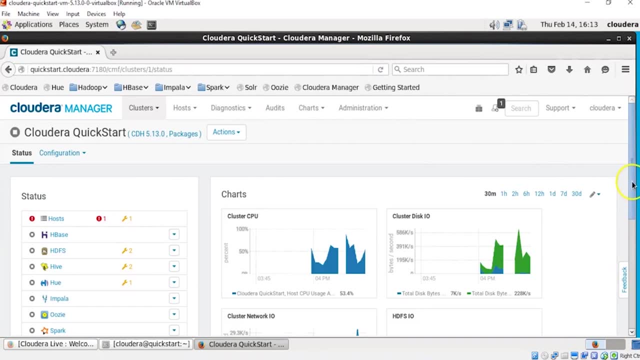 different users or enabling security using the administration tab. so, since we have clicked on restart of a cluster, we will slowly start seeing all the services, one by one, coming up. starting from the start of a cluster, we will slowly start seeing all the services, one by one, coming up. 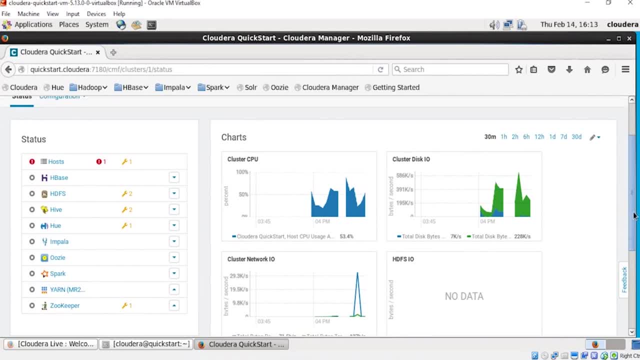 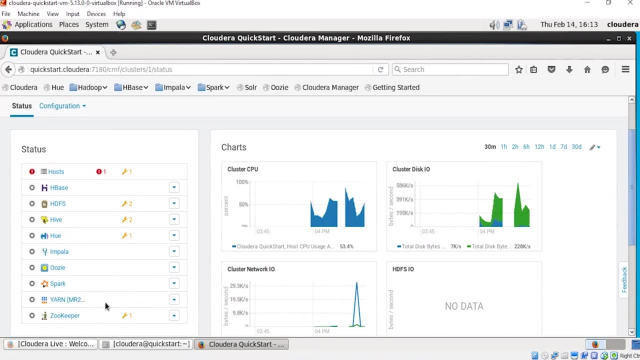 with zookeeper to begin with, and once we have our cluster up and running- whether that is showing all services in green or in a different status- we still should be able to access the service now, as we saw in apache hadoop cluster. even here we can click on sdfs and we can access the web ui once. 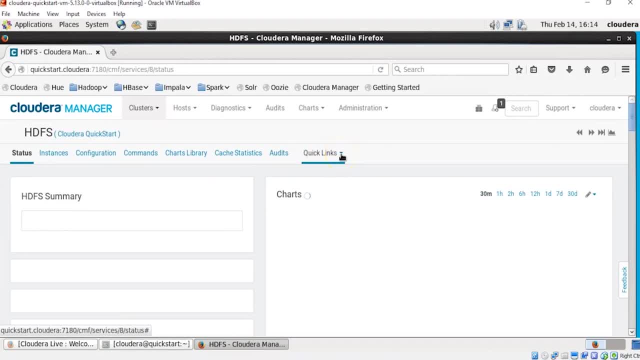 our sdfs service is up by clicking on quick links, so the service is not yet up. once it is up, we should be able to see the web ui link, which will allow you to check things from sdfs web interface. similarly, yarn as a service also has a web interface, so as soon as the service comes up. 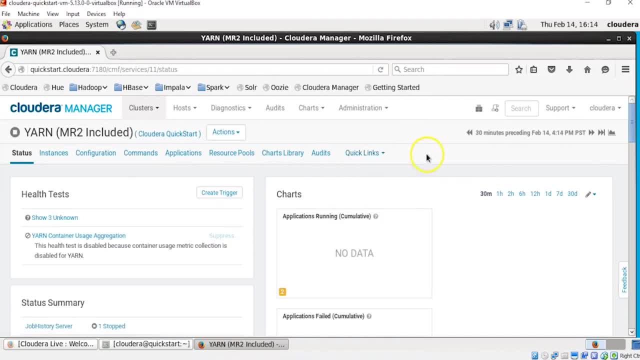 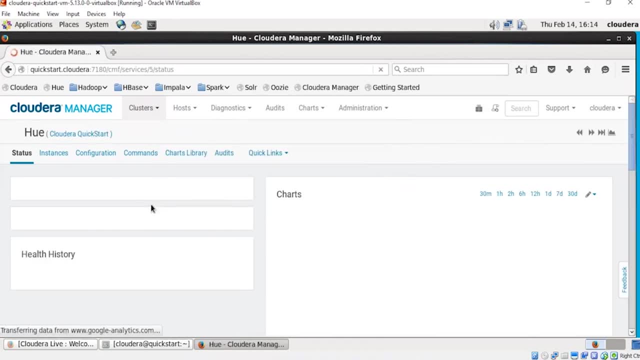 under your quick links, we will have access to the yarn ui and, similarly, once the service comes up, we will have access to hue, which will give you the web interface which allows you to work with your sdfs, which allows you to work with your different sdfs and web hyperlinks. 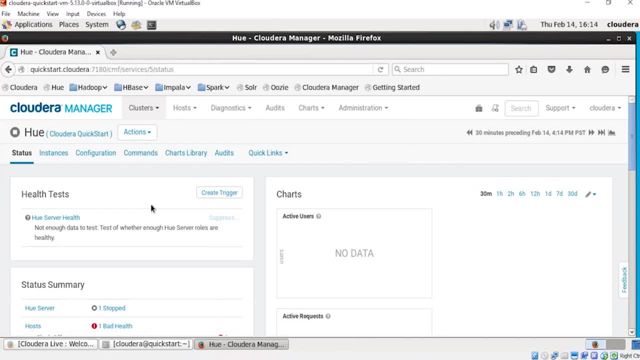 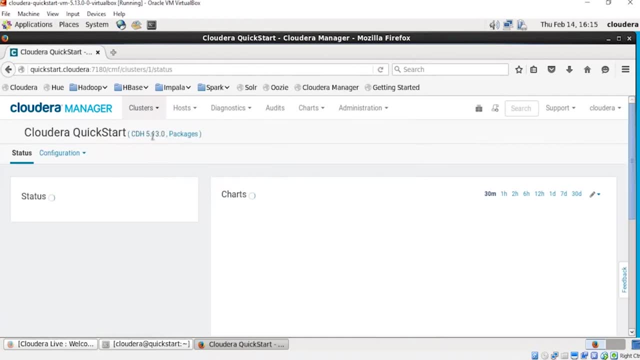 which will easily have access. the web interface which allows you to work with your different only flex to dao fifteen and we'll come back to you in another lesson if we want to do a separate video, other components within the cluster, without even using the command line tools or command line options. so we will have to give it some time while the 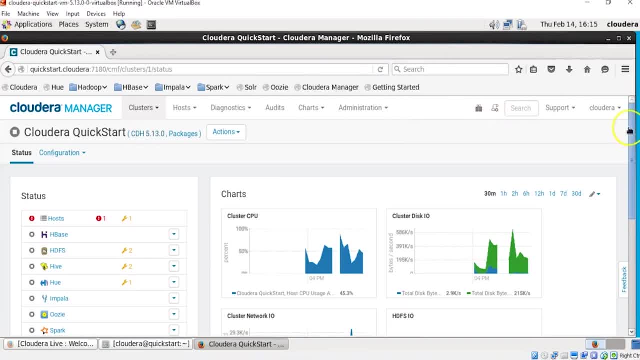 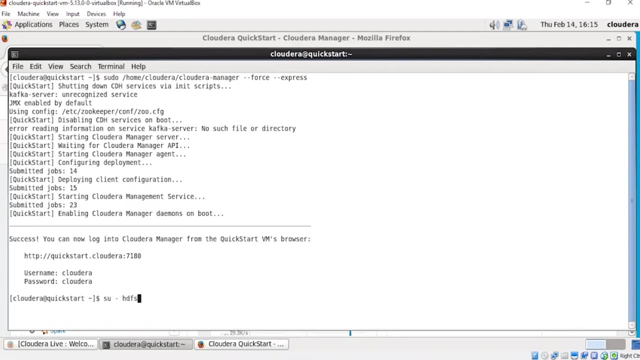 Cloudera SCM agent on every machine will be able to restart the roles which are responsible for your cluster to come up. we can always click here. it tells that there are some running commands in the background which are trying to start my cluster. we can go to the terminal and we can switch as HDFS user. remember HDFS? 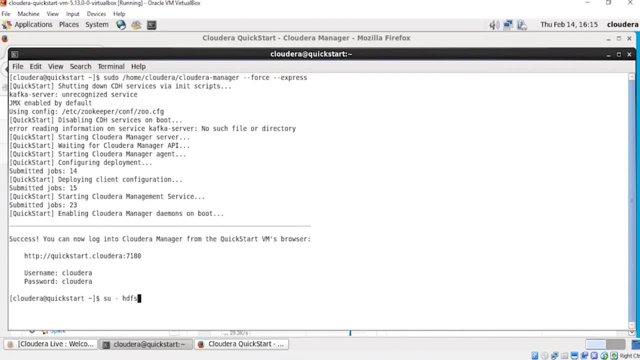 user is the admin user and it does not have a password unless you have set one. so you can just log in as HDFS, which might ask you for a password initially, which we do not have. so the best way to do this is by logging in as root, where 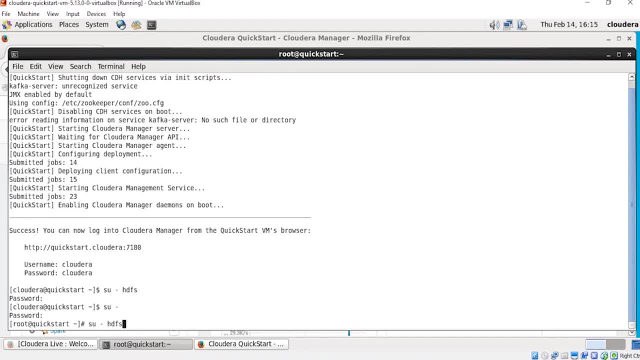 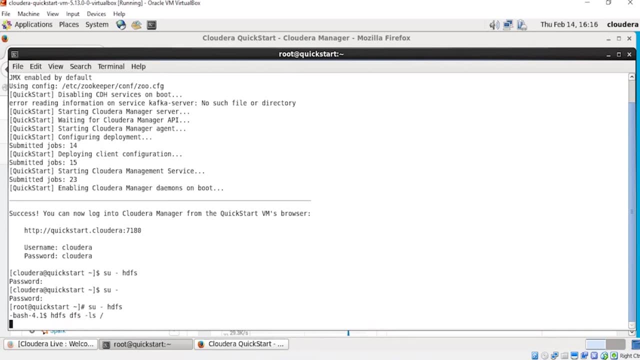 the password is Cloudera and then you can log in as HDFS, so that then onwards you can give your HDFS commands to work with your file system. now, since my services are coming up right now, when I try to give a HDFS, DFS command, it might. 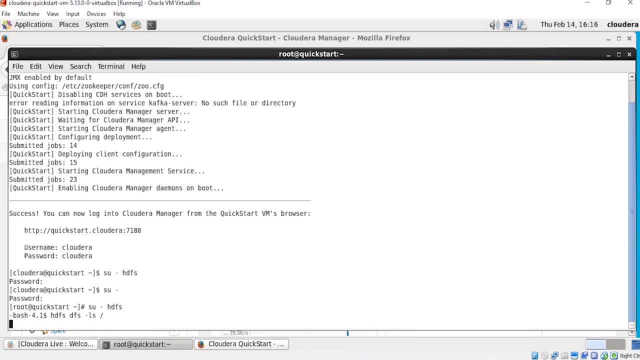 not work, so I have to go back to my cluster and I have to go back to the cluster and I have to go back to my cluster and I have to go back to my work. or it might also say that it is trying to connect to the name node which. 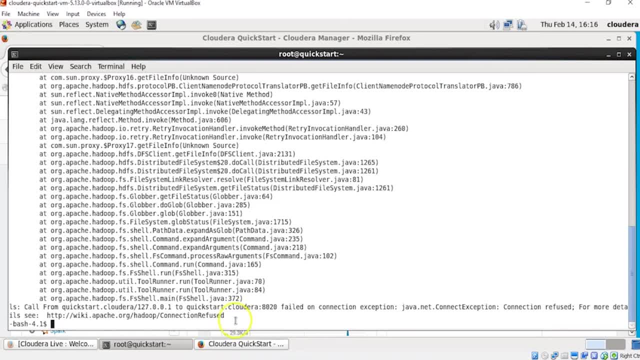 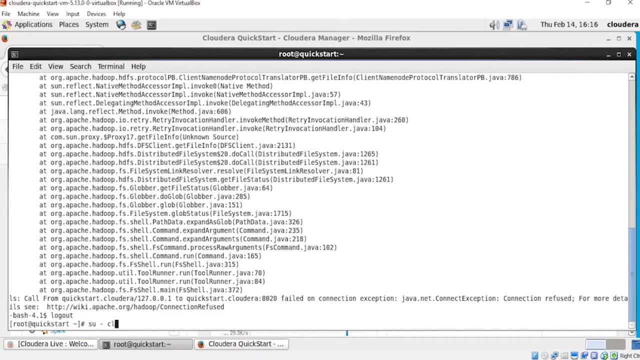 is not up yet, so we will have to give it some time, and only once the name node is up, we will be able to access our HDFS using commands. so this is how you can quickly set up your quick start and then you can be working using the command. 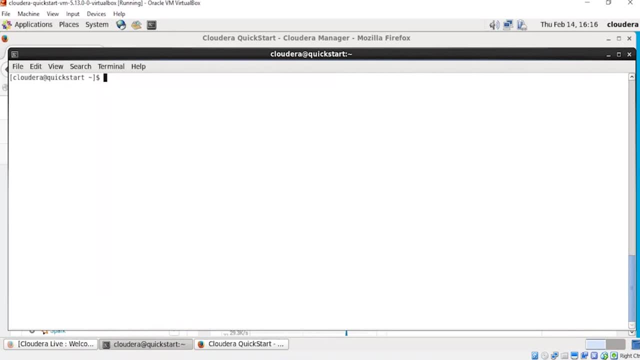 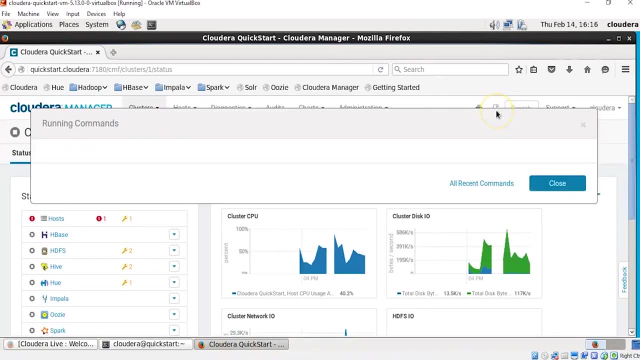 line options from the terminal, like what you would do in a Apache Hadoop cluster. you could use the web interfaces which allow you to work with your cluster. now, if this usually takes more time, so you will have to give it some time before your services are up and running and, for any reason, if you have issues, it might require you to restart your cluster several times in the beginning before it gets accustomed to the settings, what you have given, and it starts up the services at any point of time. if you have any error message then you can always go back and look in logs and see what is happening and try start. 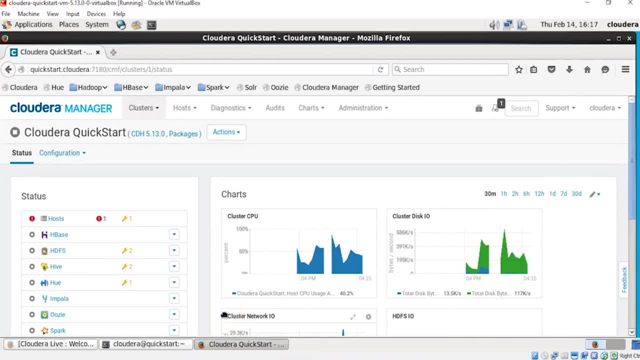 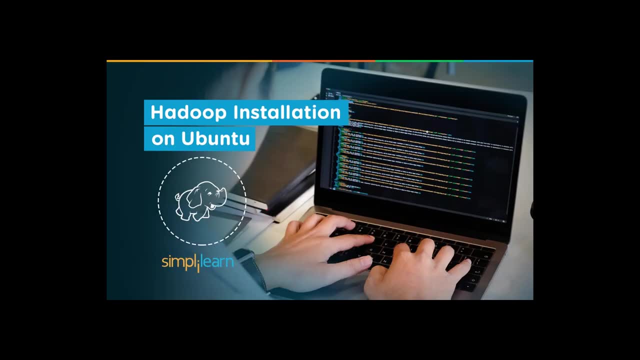 your cluster. so this is how we set up a quick start VM and you can be using this to work with your cloud era cluster. and welcome to the tutorial where we will learn today on setting up a Apache Hadoop cluster. although there are various distributions of Hadoop, as we have already discussed, and you could set 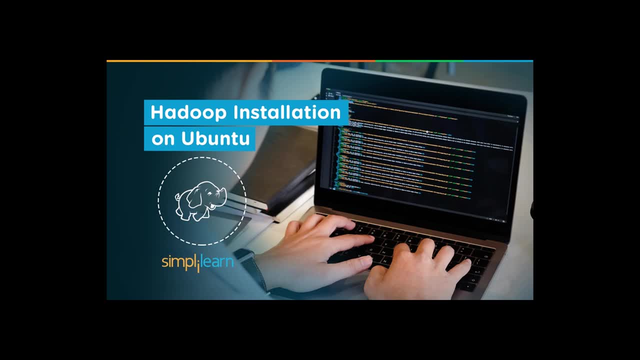 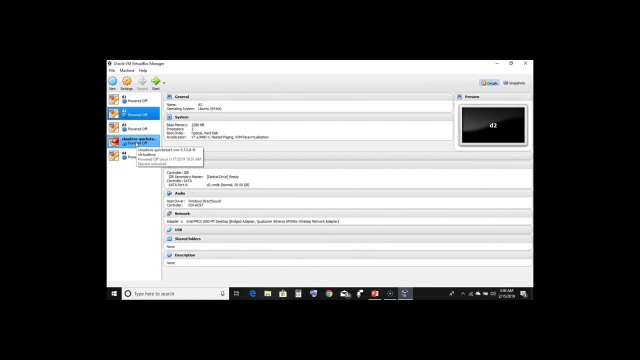 up a Apache Hadoop cluster, which is the core distribution, you could be setting up a cloud era distribution of Hadoop or even a Hortonworks. however, for cloud era you would need machines which are really powerful, at least machines which have 16 GB of RAM and in which you can set up multiple. 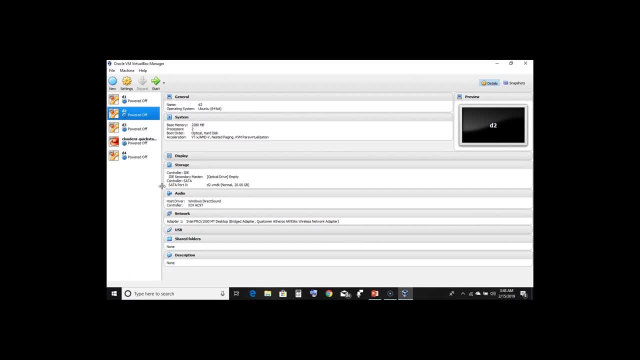 virtual machines, each virtual machine of at least 4 to 5 GB. same thing applies for Hortonworks. or you could always download and set up a cloud era quickstart VM or a Hortonworks sandbox. in this session we will learn how to set up a patchy Hadoop cluster, which is the core distribution. and if one has learned how, 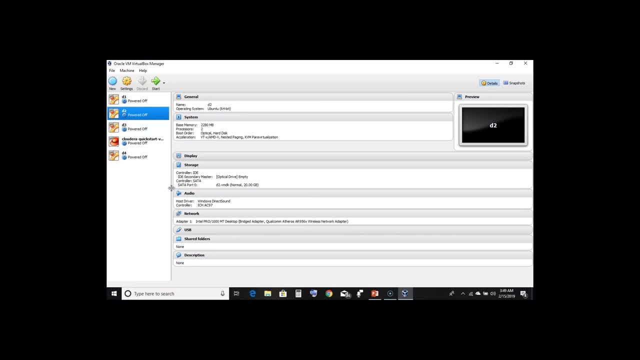 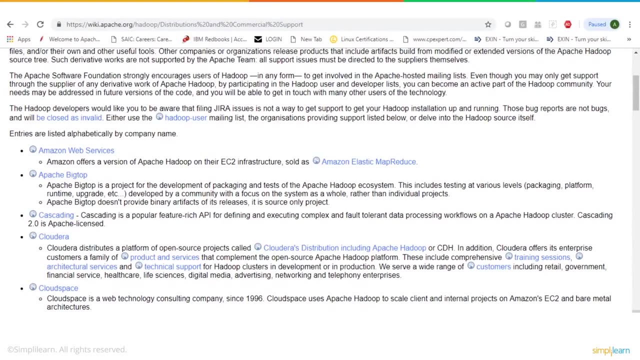 to set up a patchy Hadoop cluster. then they would understand the internals of setting up a cluster: different configuration properties which are needed for your cluster setup. we can say that these are the vendors which take up the Apache Hadoop package it within a cluster management solution so that 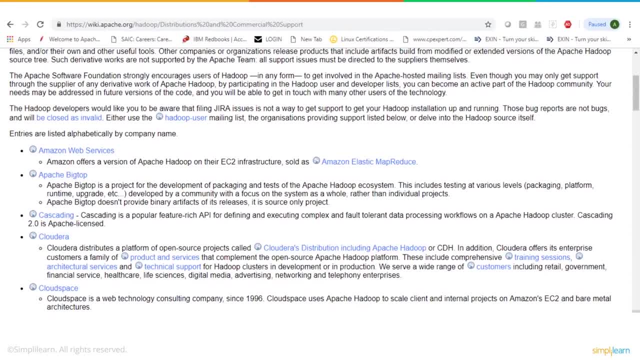 users who intend to use Apache Hadoop would not have difficulties of setting up a cluster, setting up a framework. they could just use a vendor specific distribution with its cluster installation solutions, cluster management solution and easily plan, deploy, install and manage a cluster. so look into this link, which 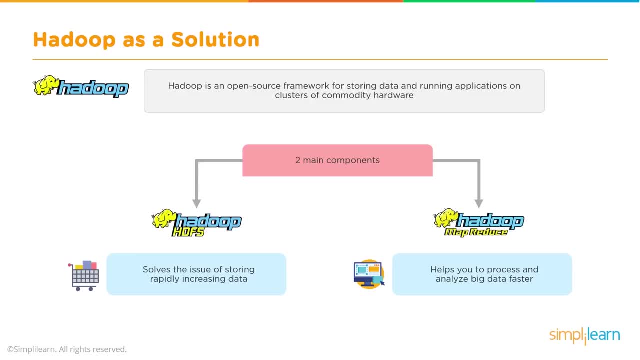 talks about different distributions of Hadoop coming back. what is Hadoop? Hadoop is a open-source framework for storing huge amount of data and processing it. it also depends on commodity machines and it does not have, you know, any kind of- does not need carrier class hardware. Now, when we say commodity machines, we are still talking. 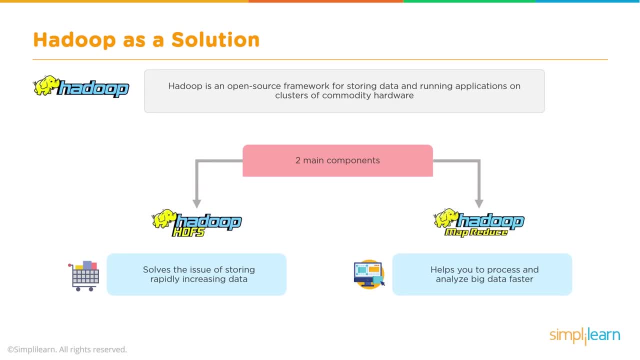 about machines which are higher than a basic laptop or a basic server, but then they are not at the level of a carrier class hardware and costing huge to the organization. Hadoop as a framework has two main components or I would say two processing layers. It has a storage layer. 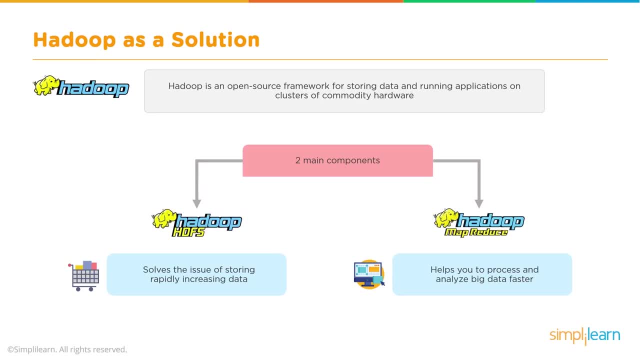 which is called HDFS, Hadoop Distributed File System, and it has a processing layer which is called YARN, which can handle different processing frameworks, in which Hadoop MapReduce is the oldest, most mature and most evolved processing framework. HDFS derives its existence from GFS. 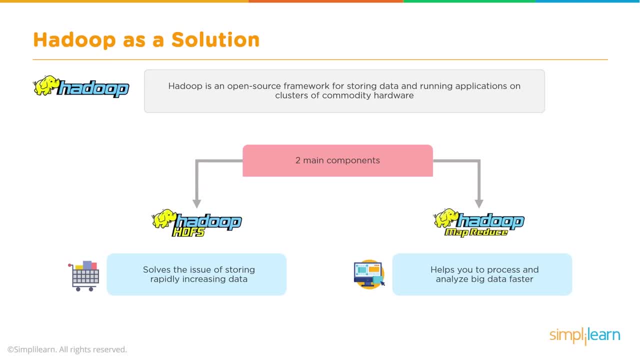 It solves the issue of storing huge amount of data in a distributed fashion, and MapReduce is a programming model which allows to process data which is distributed across a cluster. We will learn on how to use Hadoop Distributed File System and how to use Hadoop Distributed File System. 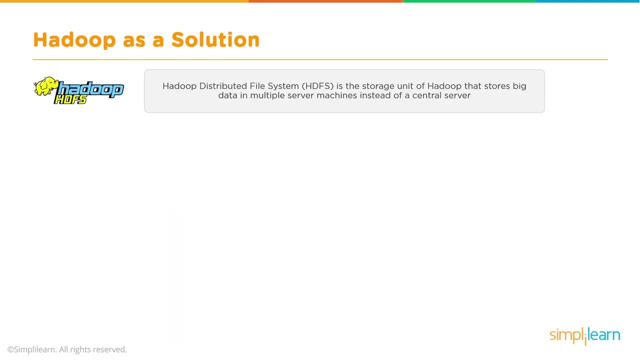 HDFS is a storage layer. Now compare your laptop, compare your desktop. that also has a processing layer and a storage layer. Your disks are your storage layer, Your RAM and CPU core is your processing layer. Similarly, Hadoop, as a solution, has a storage layer, that is, a distributed file. 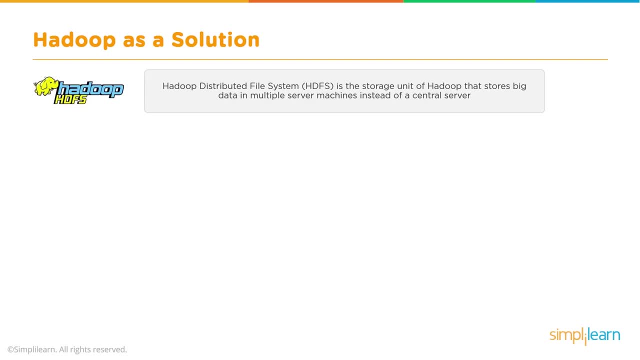 system which can store huge amount of data in multiple machines. Now Hadoop Distributed File System machines instead of a single machine or a single server, which basically makes it highly reliable, highly fault tolerant and distributed for parallel processing. consider a data file of size 1 gigabyte now if that was getting stored in one. 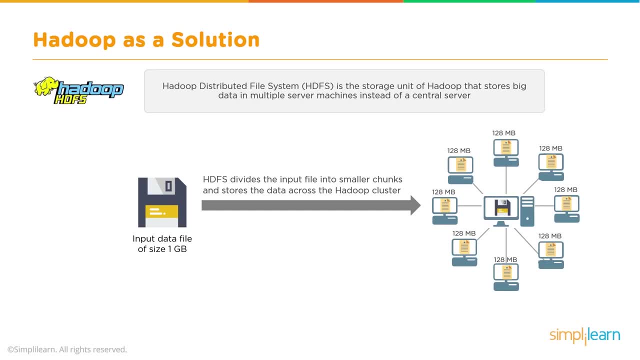 single machine, we would still have the data getting stored in one or multiple disks and if you would try to read the data, the seek time, time taken to read the data, would be very high in comparison to reading it from multiple machines. now HDFS, like your GFS, divides the file into smaller chunks and stores 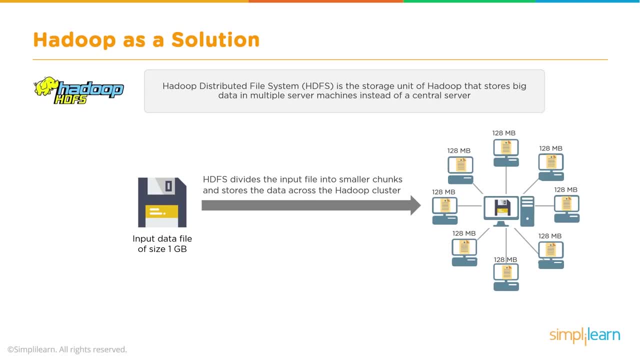 the data across the Hadoop cluster. in previous versions of Hadoop, the default block size was 64 MB. however, from Hadoop version 2 onwards, the block size is 128 MB. now that's customizable depending on the average size of the Hadoop cluster. 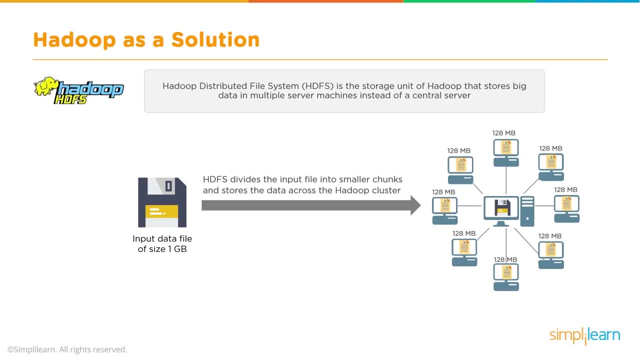 The minimum block size is 128 MB, which basically means that every file which is less than or equal to 128 MB would use one block, and any file which goes beyond the size of block will use multiple blocks, and these blocks would be residing on the underlying slave machines. Files are automatically split. 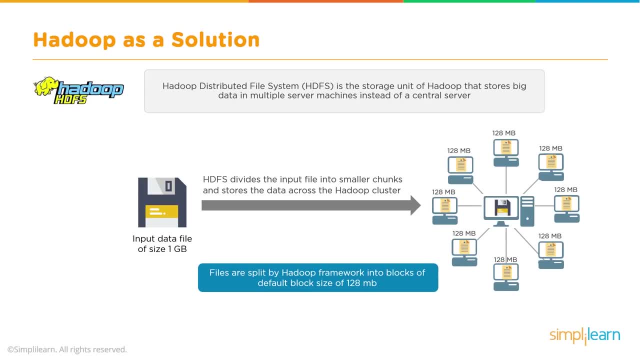 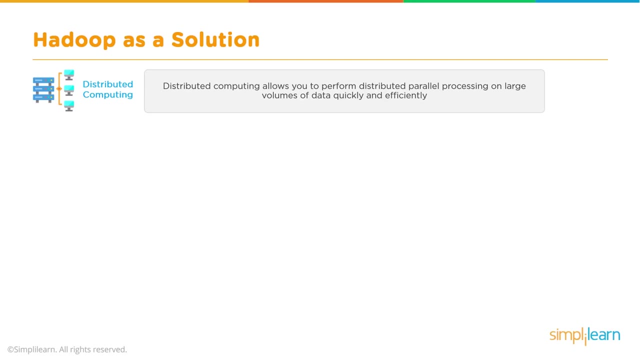 by Hadoop framework into blocks of different sizes. Each node in your hodoo cluster would have a bunch of disks that would be storing these blocks. now, once we have the data stored in a distributed fashion, that also gives us the flexibility of going for distributed computing and when. 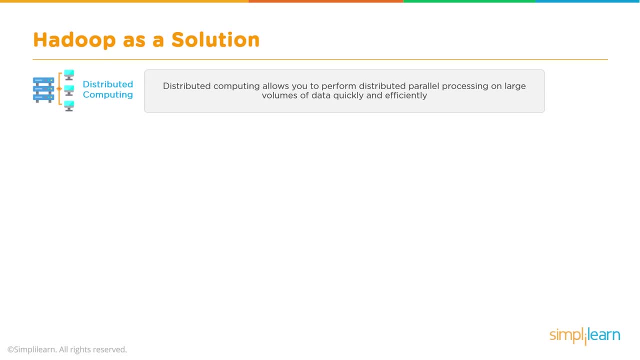 we say distributed computing, we are talking about performing distributed parallel processing on large volumes of data. Take an example where we are talking about one single machine or one in certain classes, and we want to have a lot of data, and we want to have a lot of data and we want to have a lot of data. 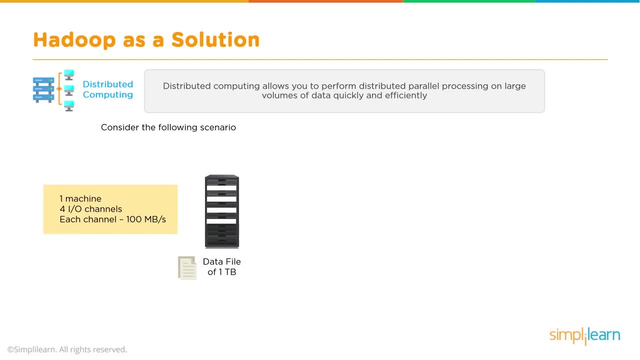 or one huge server which has four IO channels and each input output channel can take care of hundred megabytes of per second. hundred megabytes of data per second. so if we have a data file of one terabyte, it would take approximately 43 minutes for one machine to process one terabyte of data. if you compare that. 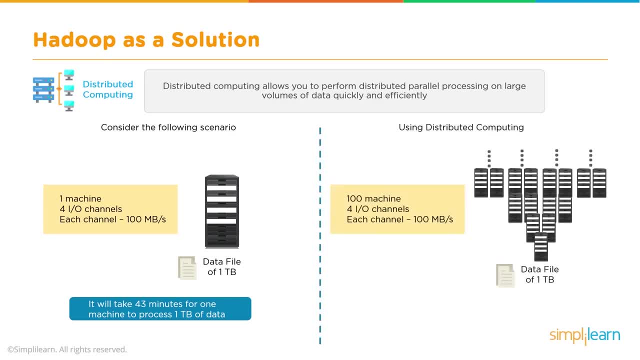 with distributed computing, where we are talking about hundreds of machines, each machine having similar number of input output channels, in each channel having the same capacity to handle hundred megabyte of data per second. if a data file of one terabyte had to be processed in a parallel processing fashion, using 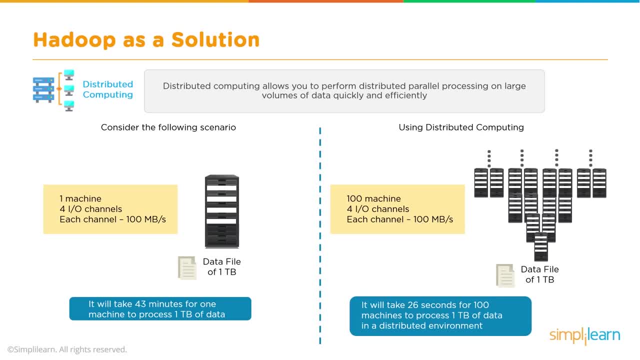 distributed computing. it would take just 26 seconds for hundred machines to process one terabyte of data in this environment. now all of you might be thinking that, yeah, this is right. but then what about the processing logic? that might be complicated, and yes, that would be, but 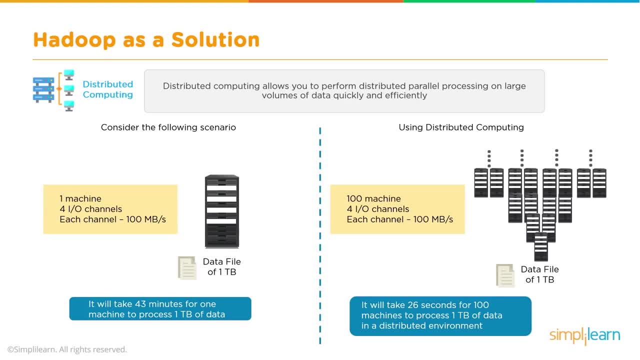 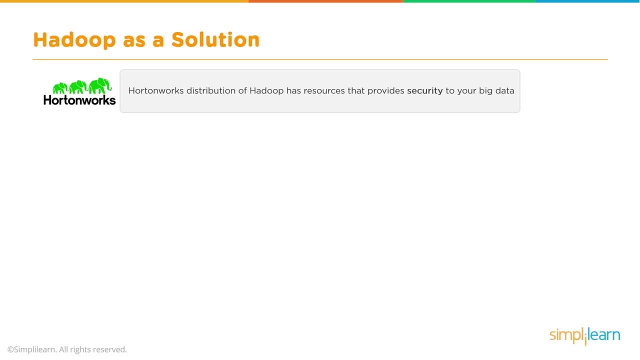 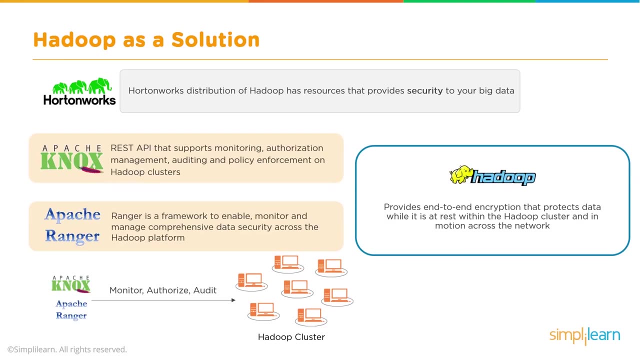 then we have a MapReduce programming model and a processing framework to help us doing that. now, when we look at one of the distributions of Hadoop that is Hortonworks, it also has different resources that provide security to your big data. now, before we start talking on these different services like Apache, 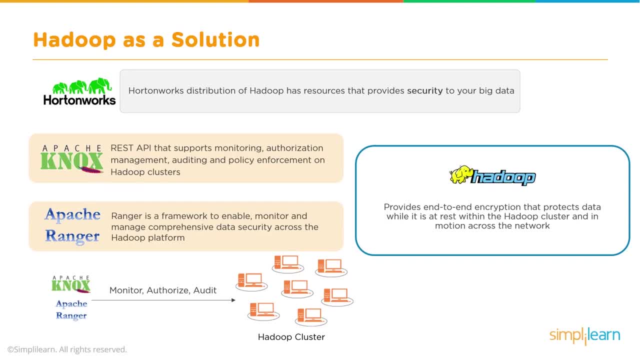 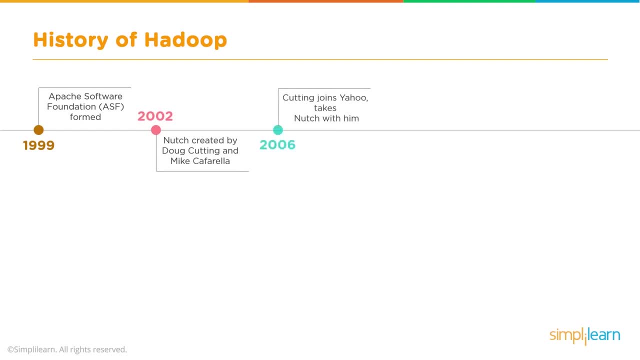 Knox Apache Ranger, which basically allow you to monitor, authorize and audit your Hadoop clusters. let's also look at the history of Hadoop, which started in 1999 with Apache Software Foundation. in 2002 where Nuts created by Doug Cutting and Mike Caffrella. then Doug Cutting joined Hadoop and took Nuts. 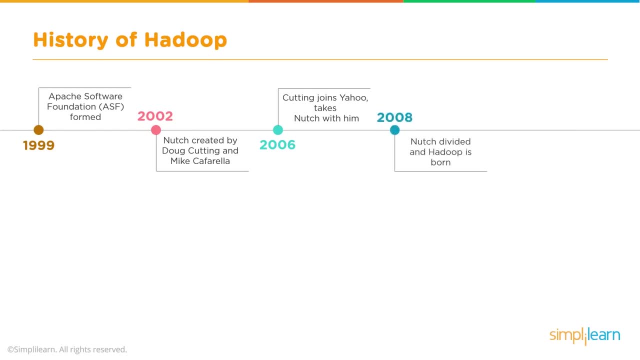 product with him. 2008, Nuts was divided and Hadoop was born. and 2008, Yahoo released Hadoop as an open source project to ASF. in 2008 also, Hadoop based startup Cloudera incorporated Cutting left Yahoo for Cloudera. Yahoo was then coming out with Hortonworks as a commercial Hadoop. 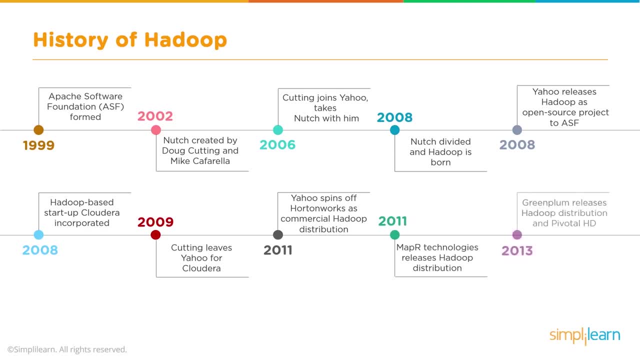 distribution. Mappa technology also released Hadoop distribution. Green Plum released Hadoop distribution and Pivotal HD. so this is a brief on history of Hadoop. you can always read about history of evolution of Hadoop, how it started and today there are more than 10 distributions which are existing in. 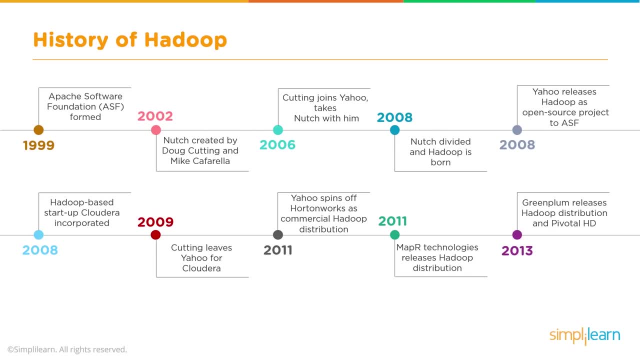 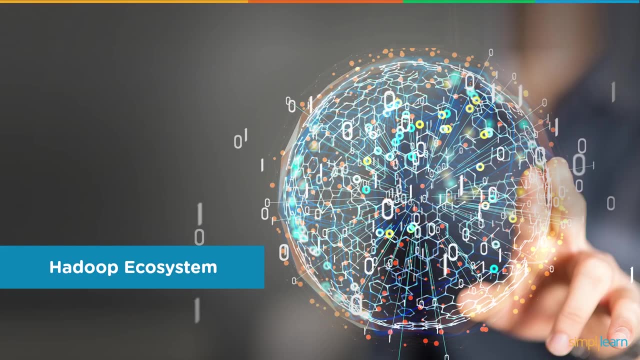 market, however, Cloudera is the dominant one and, as per recent news items, Cloudera and Hortonworks have merged as one entity, which will bring up better solutions to the market. now, here we will want to learn on Hadoop ecosystem. so far, we have learned on big data. so what is big data? we have learned on what are the? 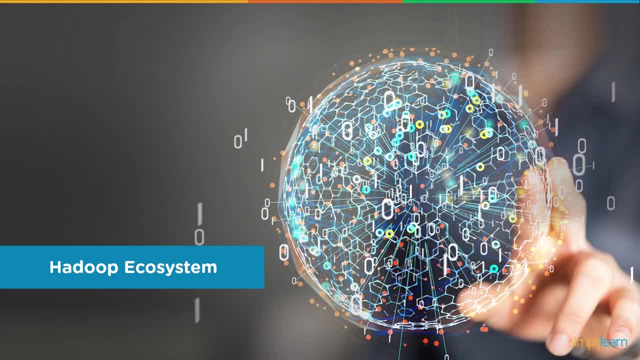 different use cases where big data can be used, different organizations which use big data, and we took an example of Facebook. we also looked at Google file system, which laid the foundation for SDFS, the Hadoop's distributed file system, and we have not yet spoken about the processing. 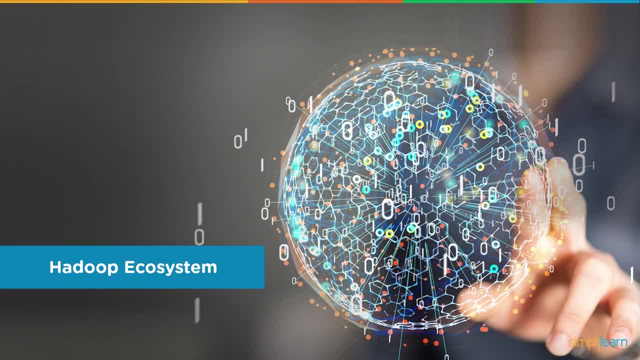 layer, which is yarn, and the processing framework, which is MapReduce, which we will discuss in future slides or further slides. let's spend some time in understanding the Hadoop ecosystem, or you might have heard as ecosphere, which has various products, or you can say tools, or you can say packages, which work. 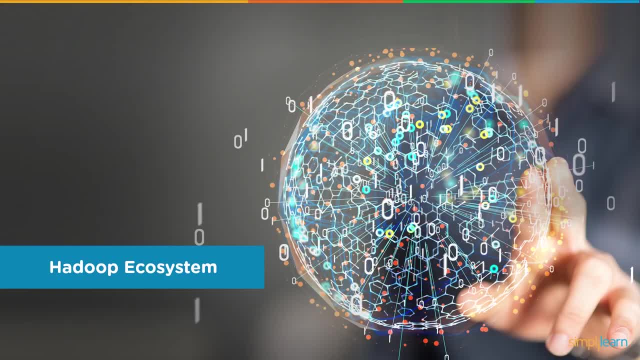 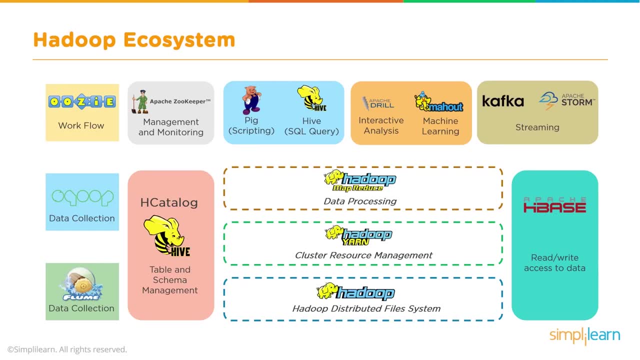 together to comprise your Hadoop cluster. now this picture shows the different components which are used for different requirements to work on your big data, starting from bottom to top, we would look at SDFS, which is Hadoop distributed file system, basically a file system which would use multiple machines to 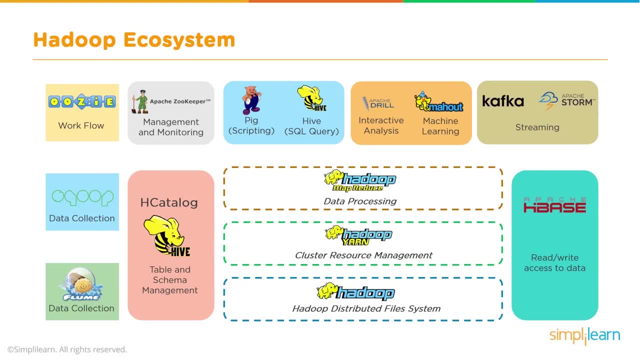 store the data. you have a processing layer that is yarn. we have a programming model that is MapReduce, which could be written in any programming language, primarily in Java, but then that could be also written in Python or Scala or any other programming language. so these are the main components. so you have SDFS and you have yarn. these are the processing. 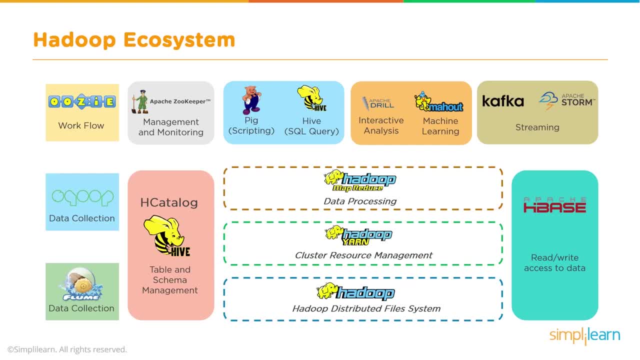 layers and for each processing layer we would have multiple processes which would be running on different machines within a cluster. now, what would a Hadoop cluster do if we did not have any data, and where would that data come from? so there might be a lot of sources where the data is getting generated and that 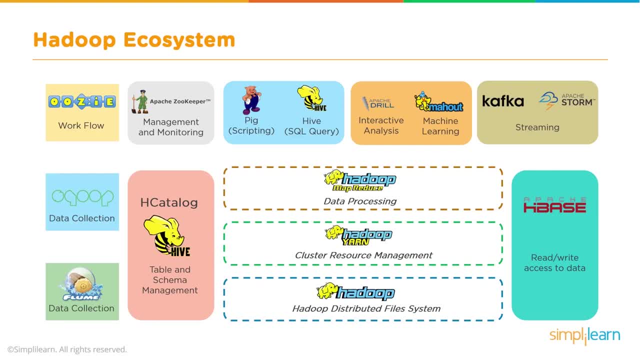 data might already be stored in our DBMS, and if you are interested in bringing in the structured data from your RDBMS layer to your Hadoop ecosystem, then you would use data ingestion tools like scoop. so scoop would be used for data ingestion, transformation and pushing it into SDFS. now that could also be used. 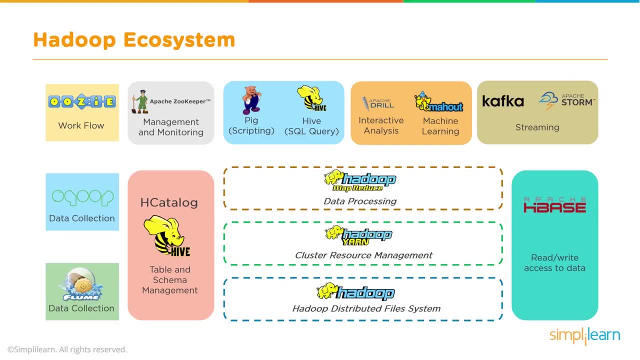 for exporting the data from SDFS back to RDBMS. but scoop mainly is for structured data. now you have other data ingestion tools like flume, which is used for ingestion of streaming or unstructured kind of data. data could directly be ingested into SDFS or it could be going into a data warehousing. 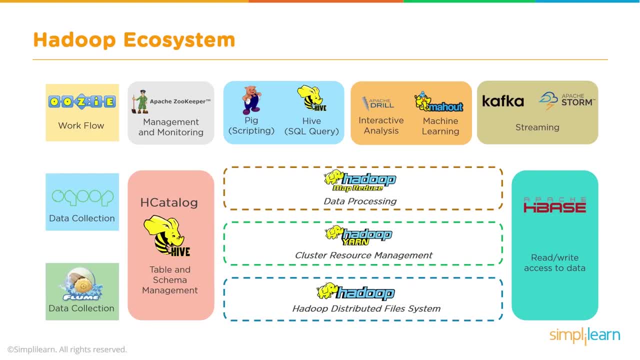 package called Hive. now, Hive is a data warehousing package on top of SDFS where users could write their SQL queries to process the data. they could be creating their tables and databases to store the data and that data would eventually be getting stored in SDFS and then in the underlying systems. Hive could be accessed through. 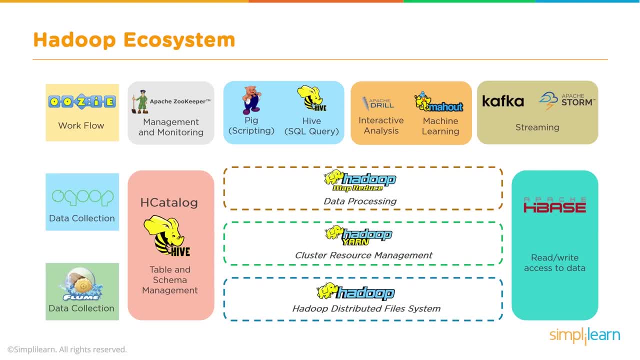 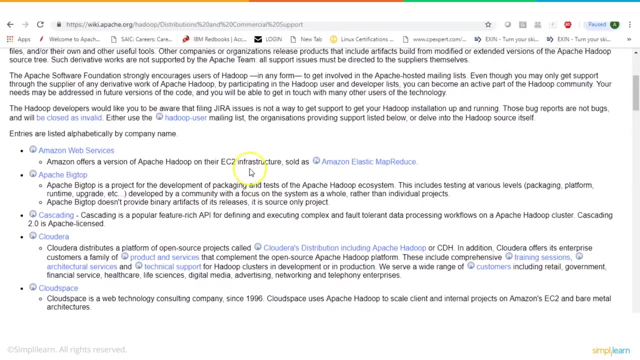 various services and H catalog is one of them. your data which is being ingested could also be stored in a unstructured data store such as Apache HBase. now there are lots of NoSQL databases. there are a lot of data ingestion tools. so if we go to Google and if we search for data injection tools- if I say data, 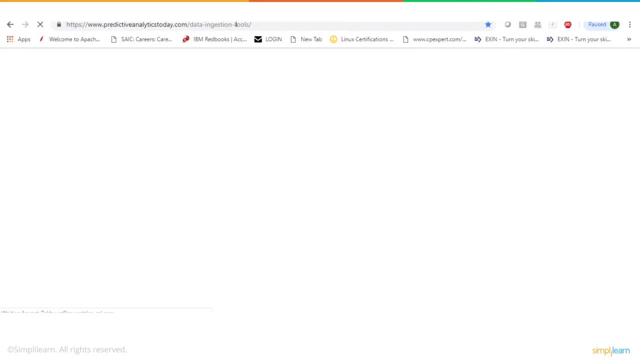 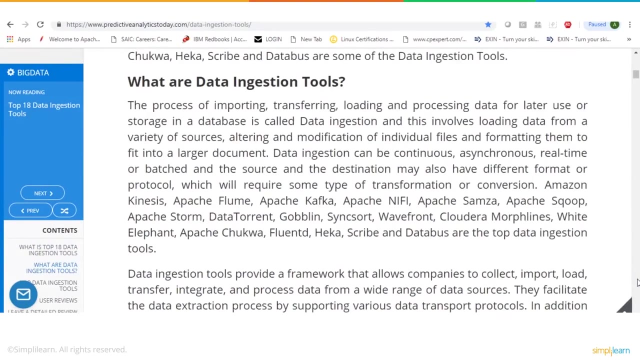 ingestion tools. so you could look at this link which shows around 18 different data ingestion tools which are existing in market. you have these tools for import and export, for transforming, for governance, for even processing the data while the data is being ingested. so you have Apache Kafka, which is a published 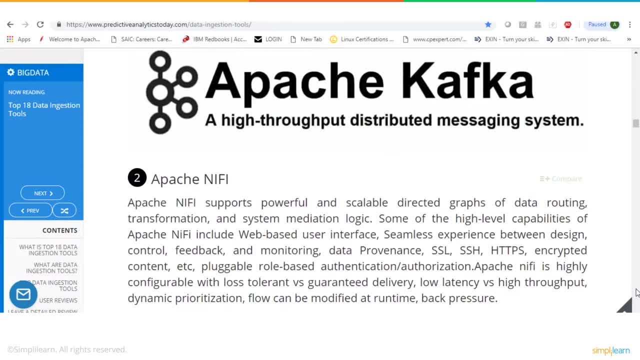 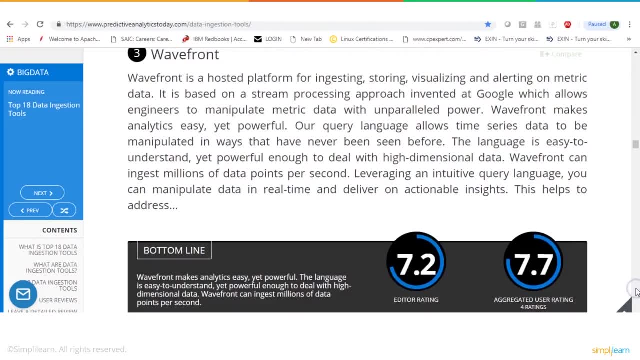 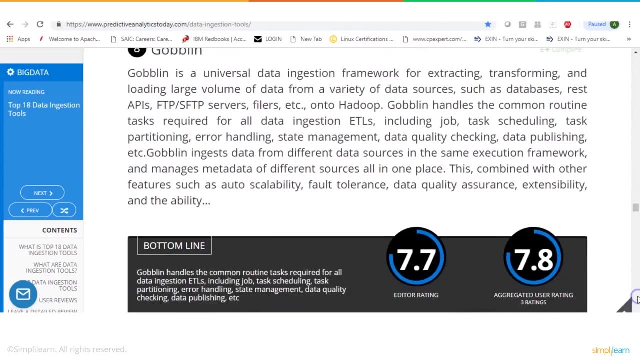 subscribing messaging system. You have Apache NiFi, which is not only for streaming or structured data, but it also helps with governance. You have Wavefront. you have DataTorrent, Amazon's Kinesis, Apache, Storm, Sumza, Syncsort, Goblin. 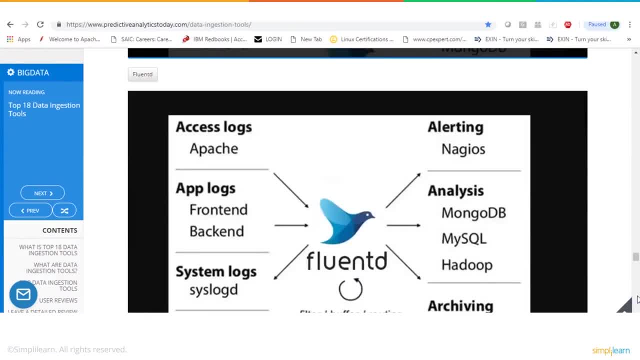 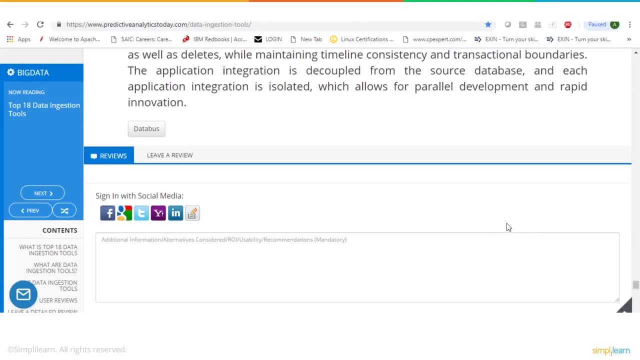 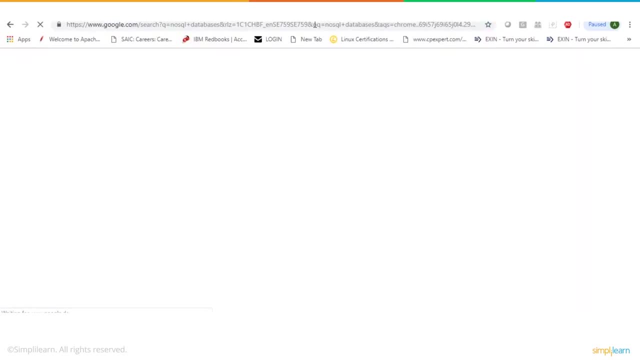 Flume Scoop, Sumza, Fluendi, Moflins, White Elephant, Chukwa, HECA, Scribe, Dataverse and many more. These are some data ingestion tools which can be used. Now we could also look at NoSQL databases and if you just type in: 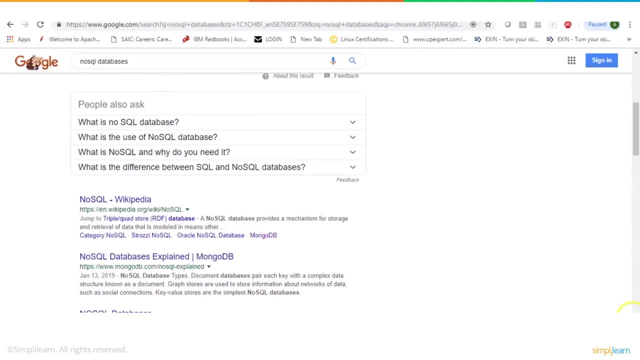 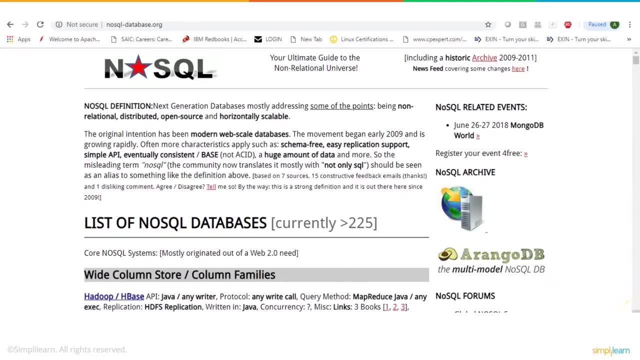 NoSQL databases that can take you to Nosqldborg and that would show you that there are more than 225 NoSQL databases existing in market. NoSQL stands for not only SQL, So these are databases which can be created without age defining any schema. They could be key value stores. They could be document-based databases. 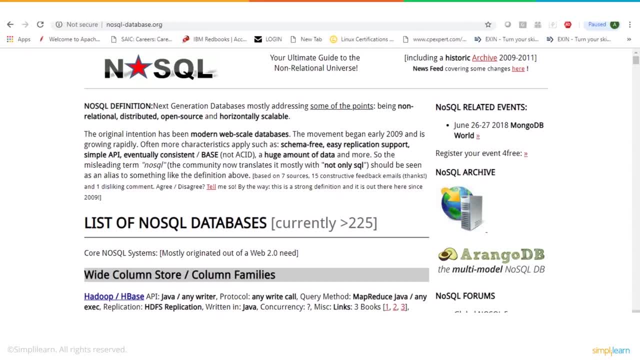 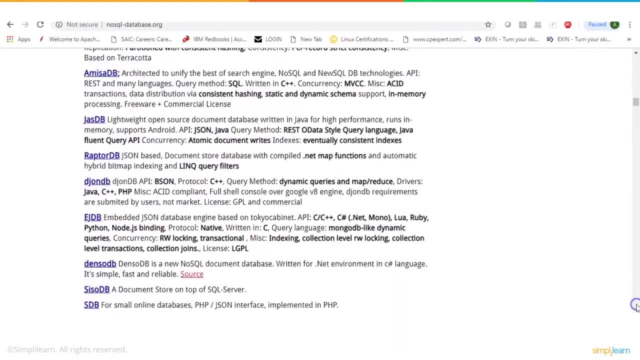 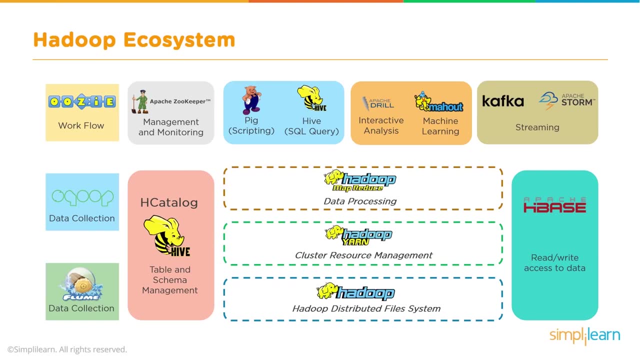 which allow a lot of dynamism, which have different kind of constraints and can allow you to store your structured, unstructured or semi-structured data. So have a look at this exhaustive list of NoSQL databases. So, coming back to your Hadoop ecosystem, your data could be ingested using one. 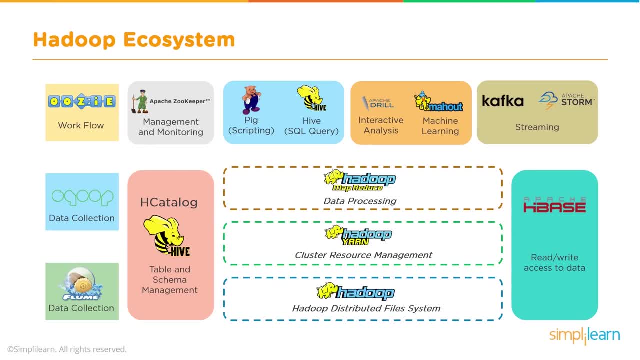 of the data ingestion tools into SDFS or into a Hive table. or into Hive, that would be using SDFS as the underlying layer. Your data could also be imported into a NoSQL databases such as HBase, which is a four-dimensional database. It's a key value store which allows for faster random access. 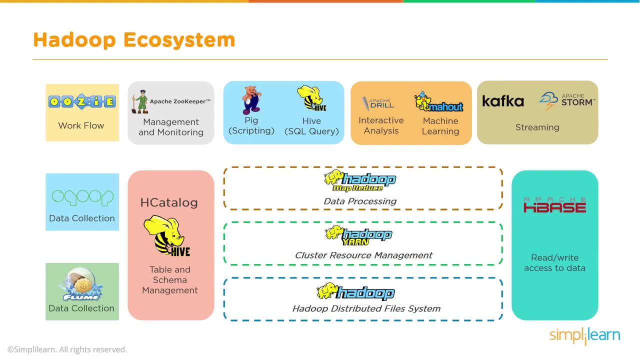 across billions of records. We learn on HBase, on Hive, in other sessions. Now, when you talk about Hadoop ecosystem, you could have a workflow manager such as Uzi. Now there are other workflow managers like Askaban. You have Luji right, which can be used, But Uzi. 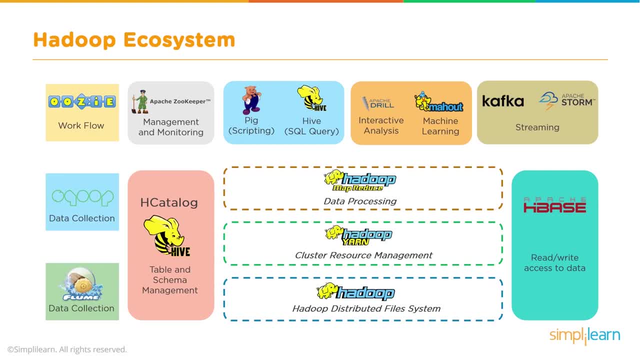 comes with Hadoop Now, not with Apache Hadoop. As I said, Apache Hadoop is an open source And to set up an Apache Hadoop cluster and to set up Hive or HBase or any of these components, we would have to manually download the packages, edit the configs, set up the processes. 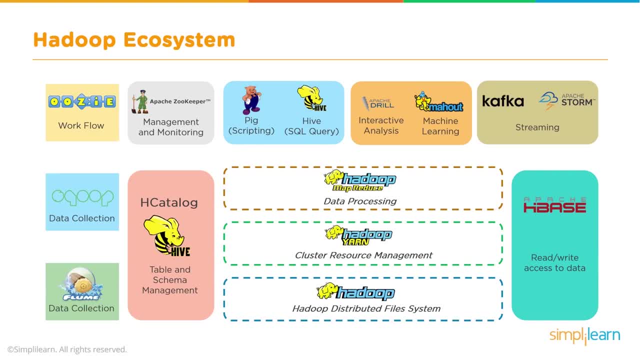 and then we would have to manually download the packages, edit the configs, set up the processes and start the cluster and services. However, if you were using a vendor-specific distribution, many of these packages would come as a packaged solution. So Uzi is a workflow scheduler which 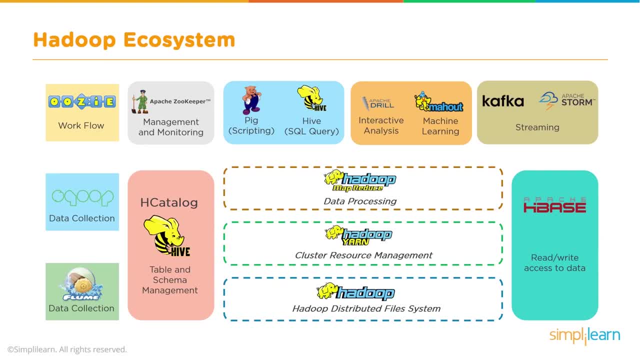 allows you to create a workflow of different jobs which could be run on a Hadoop cluster. You could have a service such as Zookeeper, which is mainly for management and monitoring. So it's a centralized coordination service which especially plays a very important role when it is. 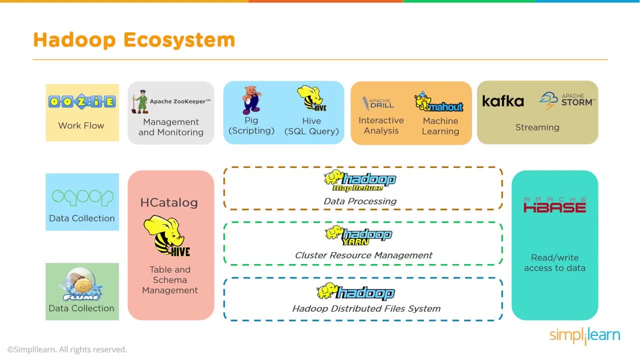 managing a high-availability cluster of Hadoop or HBase. You have PIC scripting, which allows for processing of data in a very concise way. You have Hive querying, which allows users to write their SQL queries to process the data. You could also do interactive analysis using 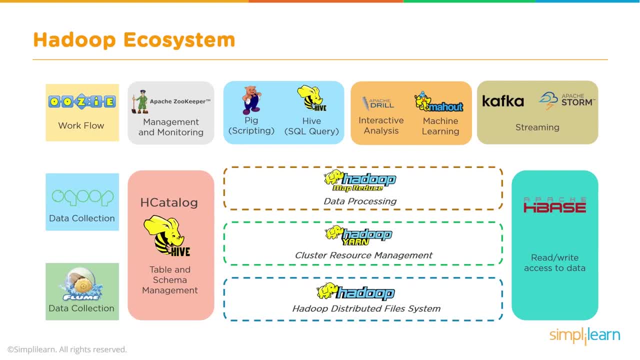 packages like Apache Drill. You have Apache Mahout for machine learning. You have Kafka, Apache Storm and even Spark, which can be used for streaming. Now Spark is a very useful tool. Spark again has different components and it is an in-memory computing framework which allows you. 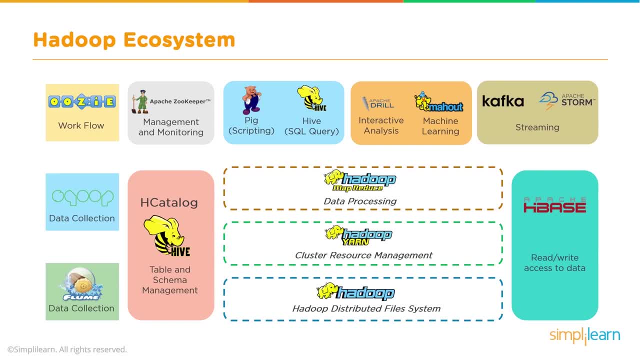 to work on streaming data, structured data, graph-based data and even machine learning algorithms. So Hadoop as such is a solution which allows organizations to work on big data and Hadoop ecosystem and the components which are involved, which can be part of your Hadoop ecosystem. 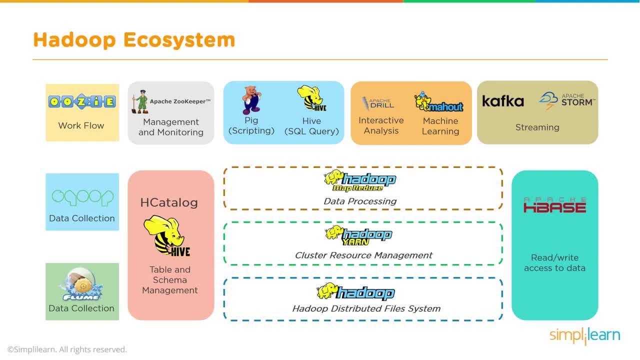 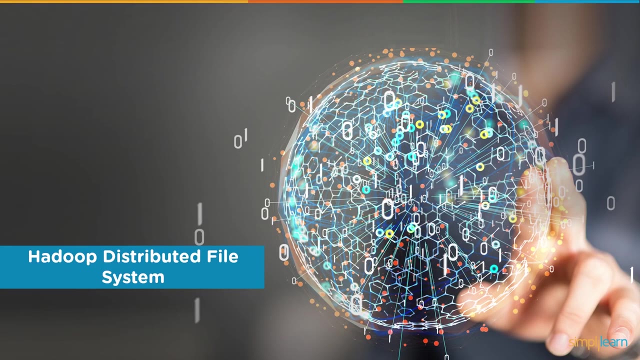 are growing, So there can be lots and lots of other components which can be part of your Hadoop ecosystem, which can be overall used to store, process, capture and analyze big data. This is where we come to a point where we should now start learning on Hadoop distributed file system, which 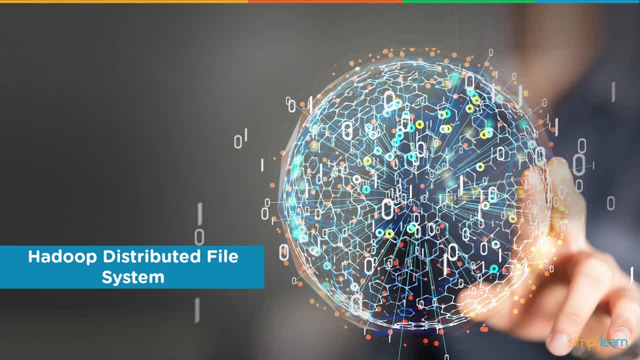 allows you to store data in a distributed fashion. SDFS basically makes it easier for organizations to store huge amount of data. In previous session we were learning on big data: its characteristics. what are organizations interested in when they talk about big data and different use cases? 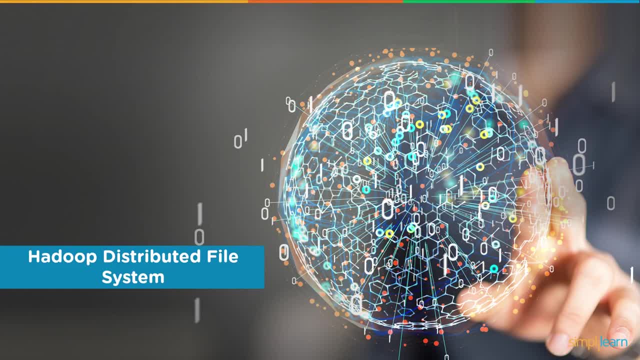 Today we will learn on Hadoop distributed file system, which is basically the logical storage layer for a Hadoop cluster. SDFS is fault tolerant, is reliable and is scalable. So let's understand and learn on the working of SDFS. that is the logical storage layer for a Hadoop cluster: SDFS. 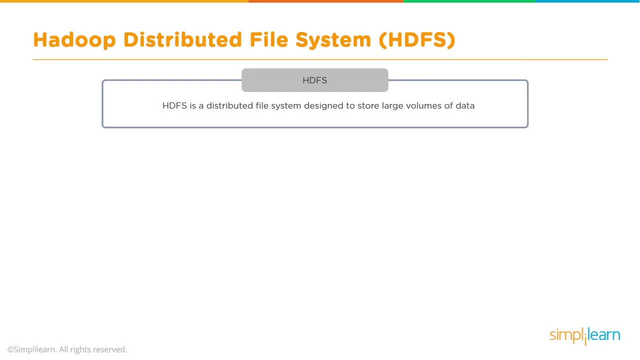 is designed to store large volumes of data on commodity machines. It is designed with a low-cost hardware- and that is what I mean when I say commodity machines- So we could have a cluster of tens and hundreds and thousands of nodes which can still scale and accommodate huge volume of. 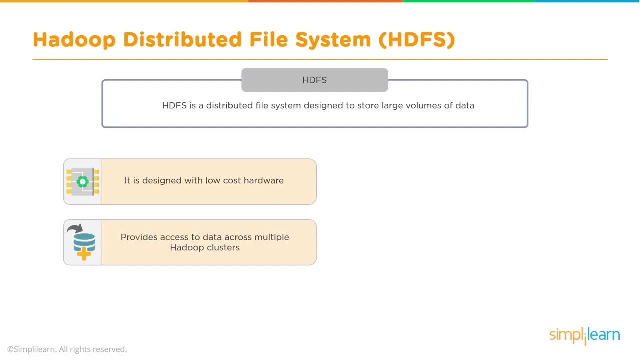 data. It provides access to data across multiple Hadoop clusters. It has a high fault tolerance and throughput, And SDFS stores data on a large volume of data, So it can store large volumes of data in multiple servers instead of a central server. Now, earlier, when we were discussing on 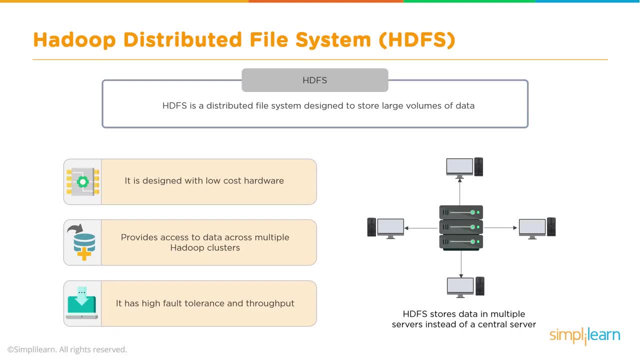 how storing data on a single machine can lead to more read or processing times and basically lead to high seek time. that can be taken care by a distributed file system such as SDFS, which would rely on file systems of multiple machines which form your Hadoop cluster. Now let's understand. 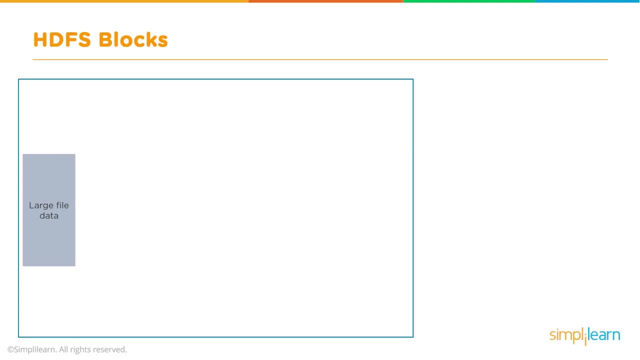 how SDFS works. For example, we have a large number of Hadoop cluster that is based on multiple Hadoop clusters. Now let's understand how SDFS works. For example, we have a large number of Hadoop clusters. Now let's understand how SDFS works. For example, we have a large file which is 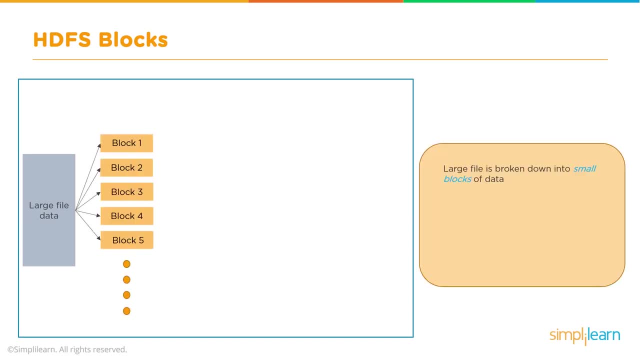 to be stored on SDFS. Now that file would be broken down into blocks and the block size by default is 128 MB. These blocks would then be stored across different slave machines or different nodes which are responsible for storing data. SDFS has a default block size of 128 MB, which can be 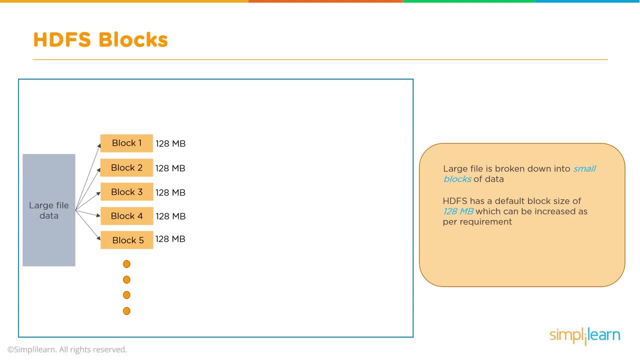 increased as per requirement. Now that could be in megabytes, gigabytes, terabytes or even bigger than that. The default block size is 128 MB from Hadoop version 2 onwards, and your previous versions of Hadoop had the block size of 64 MB. Here the point to be remembered is: block is a. 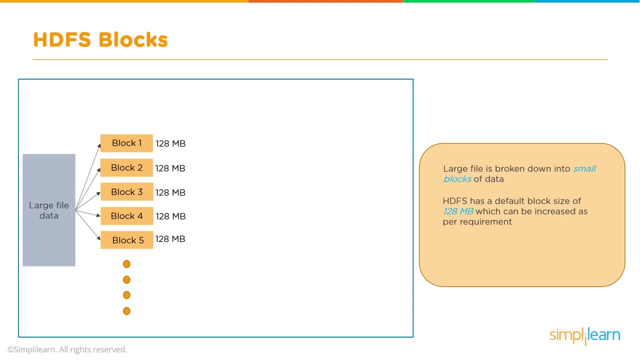 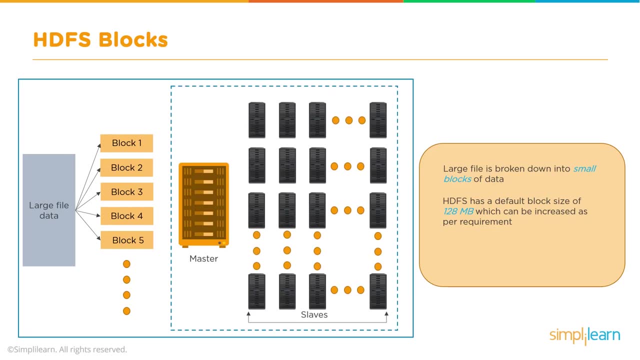 logical entity which basically takes the data and stores it on the underlying machines in their disks. Now this is how it would look in a normal Hadoop cluster. We would have one single master, unless it is a high availability cluster where we could have multiple masters, that is, two masters. 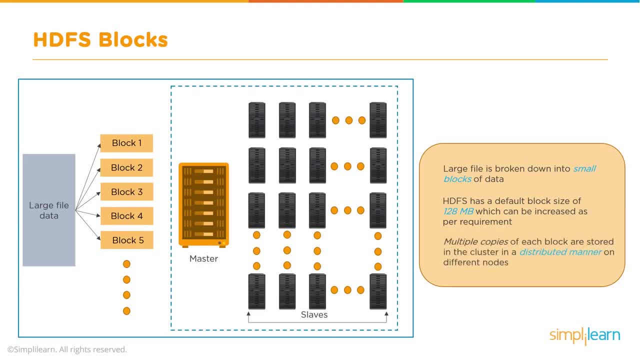 one being active and one being standby. In a normal Hadoop cluster, you would have one master and multiple slave nodes where these data blocks are getting stored. Now, before we understand the map reduce algorithm, let's also understand the working of SDFS and how data gets stored overall. how does 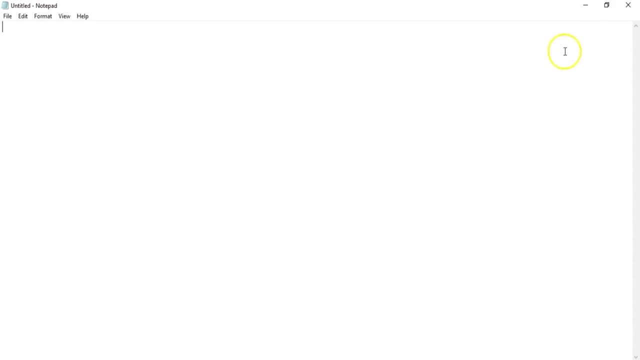 it work. So let me just open up a notepad file and I would explain about SDFS. Now let's imagine that this is. I would like to have, say, five machines which could be forming my cluster. So I would have machine one, machine two. 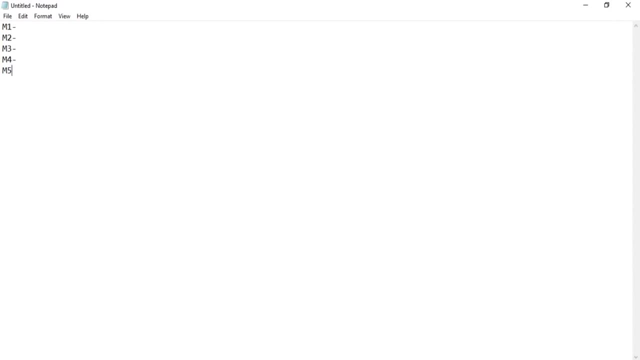 machine three, machine four and machine five. Now, if I say my Hadoop cluster is running on these machines, which could be of a Apache Hadoop core distribution or having a vendor-specific distribution, such as Cloudera or Hortonworks or MapR or 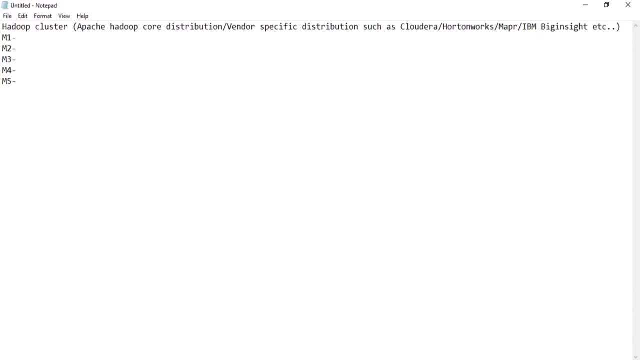 IBM Big Insight, etc. So these are some vendor-specific distributions of a Hadoop cluster. Now here we can discuss later on how or what processes would be running on these machines. Now in case of Apache Hadoop cluster, in case of Apache Hadoop cluster, to have a Hadoop cluster. 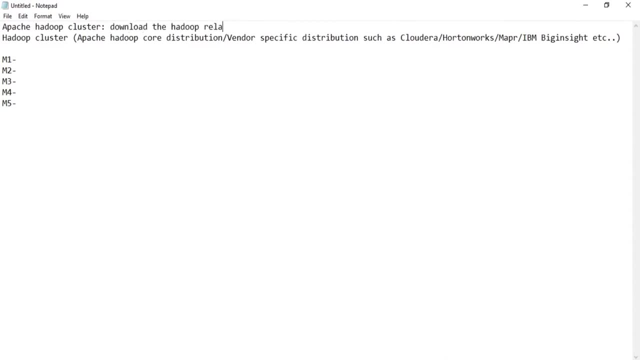 running. we would have to download the Hadoop related packages, We would have to untar, then we would have to edit config files to specify which processes would run on which nodes, and then basically we would be formatting HDFS and then onwards we can go ahead and start our cluster. So it looks. 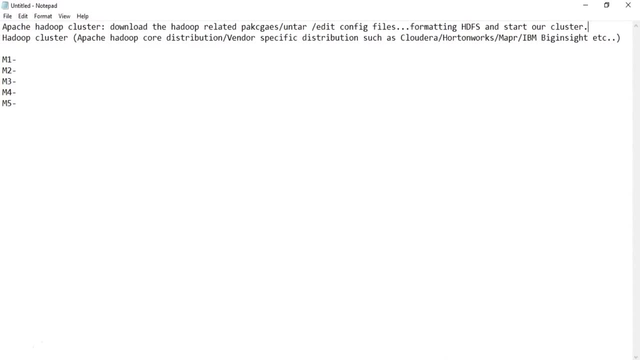 like in Apache Hadoop cluster, we would have to manually do various things, such as downloading the Hadoop related tar file, untarring it, editing the config files, formatting HDFS and then going ahead and starting your cluster. In case of a vendor specific distribution, such as Cloudera or 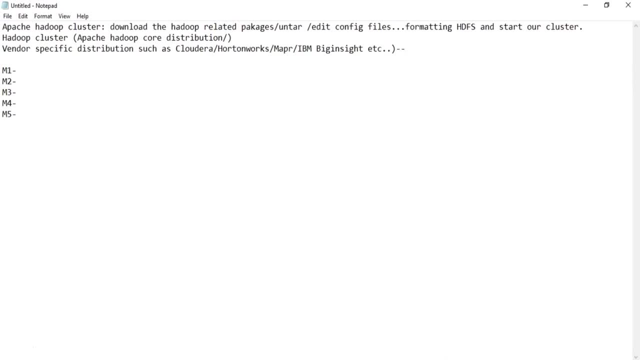 Hortonworks. let me split it here. so you would have basically a cluster management solution that would help you in doing various things to set up your cluster. In case of a Cloudera distribution of Hadoop, you would have a Cloudera installer file and then you would have a Cloudera manager, which. 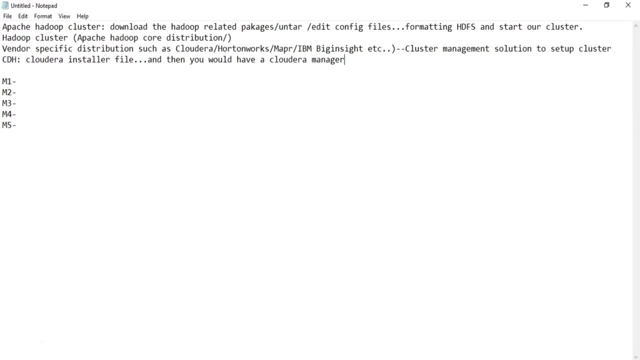 will help in deploying a Cloudera. So downloading Hadoop related parcels or packages, untarring them, editing config files, formatting HDFS and basically starting your cluster would be taken care automatically by Cloudera manager. In case of Hortonworks data platform, it would be Ambari software that would 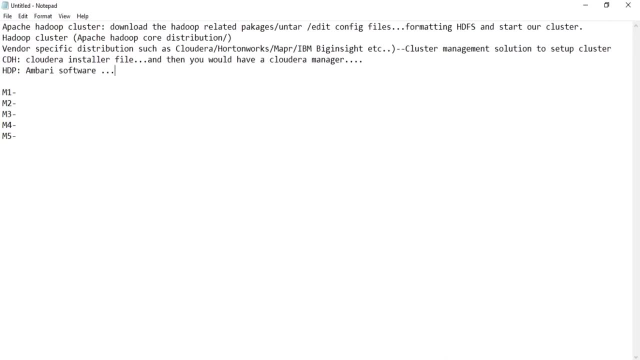 be used for deploying your cluster. Now, no matter which distribution of Hadoop you would be running, you would still have the same roles or processes which would be running. Let me just briefly discuss here about the terminologies. So let me bring up a file here which could explain. 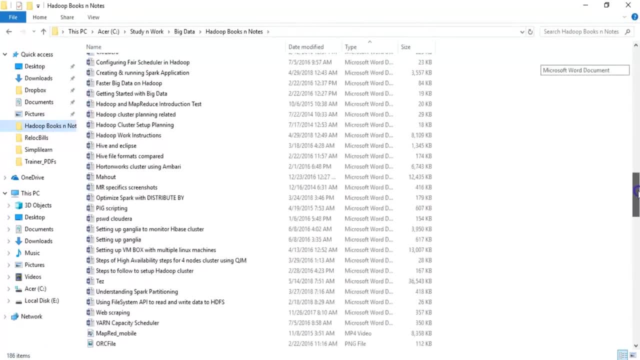 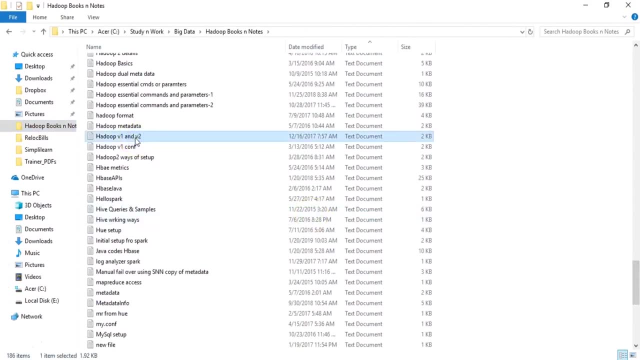 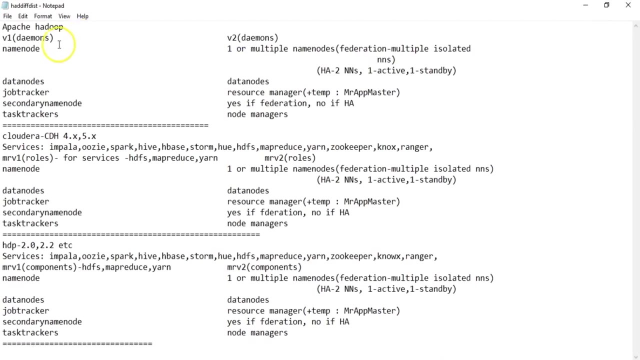 these details. So let's look at this Now. here I have documented how it would look in different distributions of Hadoop. So we have Hadoop version 1 and 2 and let me just look for files. yeah, so this is the one. Now, if you would look in version 1, Apache Hadoop, we would call daemons or processes. 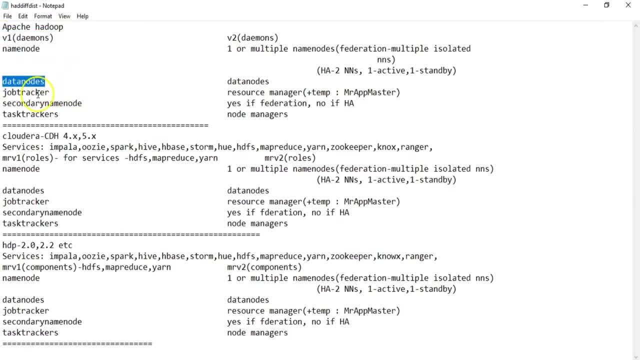 the names. we have the name node, we have data nodes, we have job tracker, we have secondary name node and we have task trackers. in case of version 2, you would still call them demons. you could have one or multiple name nodes. if it was a federation or a high availability kind of setup, you would 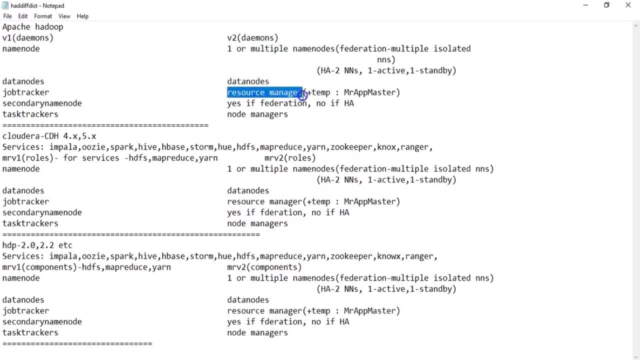 have data nodes. instead of job tracker you would have resource manager and then there is a temporary demand called mr app master. if you had a high availability, then secondary name node would not be allowed, and if there was a federation kind of setup, secondary name node would still be existing. 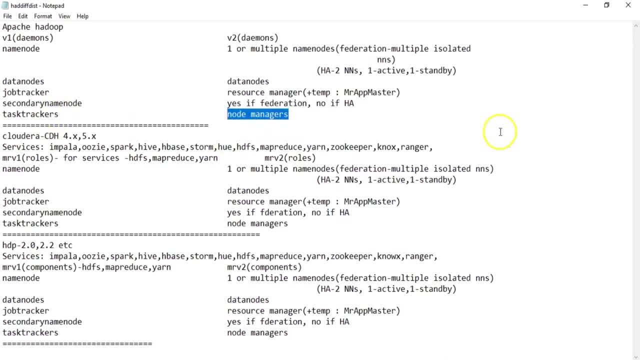 instead of task trackers, you would have node managers. now, in case of vendor specific distributions such as cloud era, whether you are talking about older version or newer version, which is five point something, you would have what we call as roles, so in apache, hadoop, we call them. 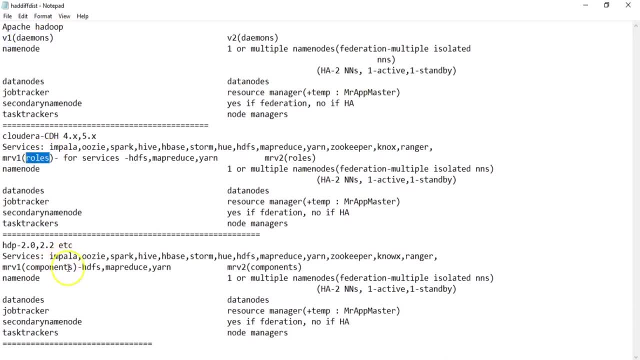 demons in cloud enough, we call them roles. in hotenworks we call them components, but we are talking about the same thing. in case of cloud era, you would have services which would be part of the cluster, such as impala uzi, spark, hive, edge, base, storm, hue, sdfs, map, reduce, yarn and so on. similarly, in cottonworks also, you would have. 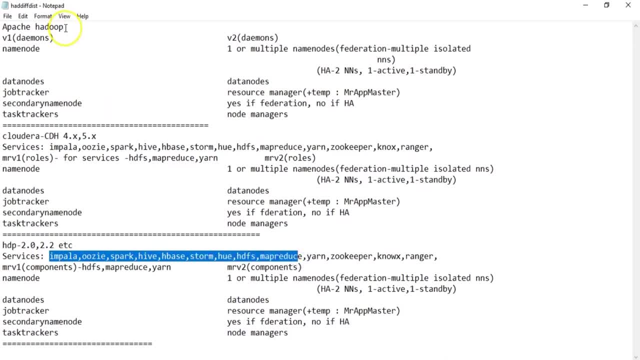 these services which would be running in case of apache hadoop. we would not have so-called services seen, but then the functionality still exists. and how is that? that is depending on these demons. so, basically, if you look in apache hadoop or cloud error or hotenworks, everywhere we have these demons and we have these would be running on one or multiple. 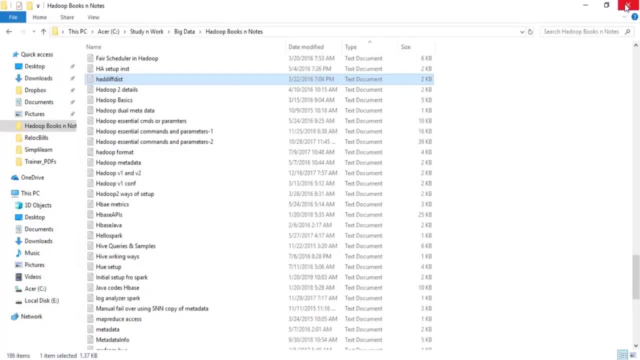 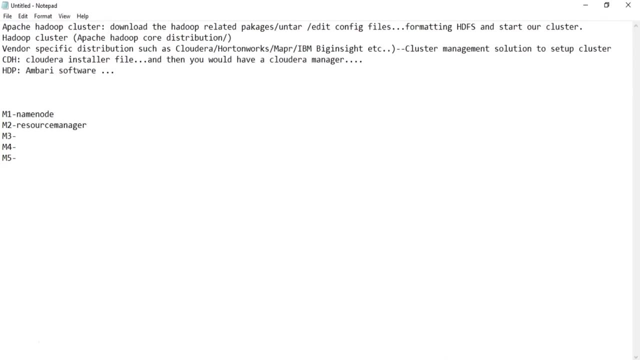 nodes so we could have different kind of setups and just to briefly discuss on that, so we could have a name node running here, a resource manager running here and you could have a secondary name node. now don't go by name, it's not a second name node, we'll discuss. 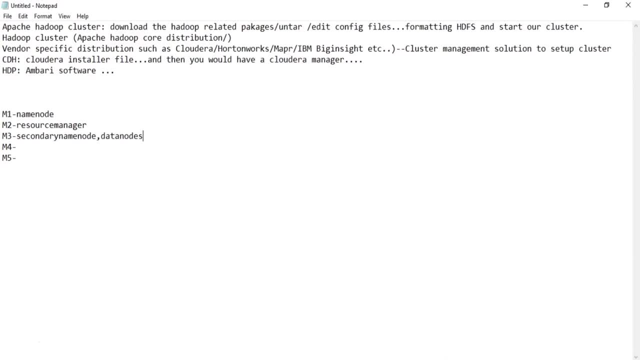 about that later- a secondary name node, and then we could have data nodes running in machines. so this is one kind of setup where i'm talking about data node node manager and here we have a data node node manager and similarly we would have that on one more machine. now, this is one kind of setup. 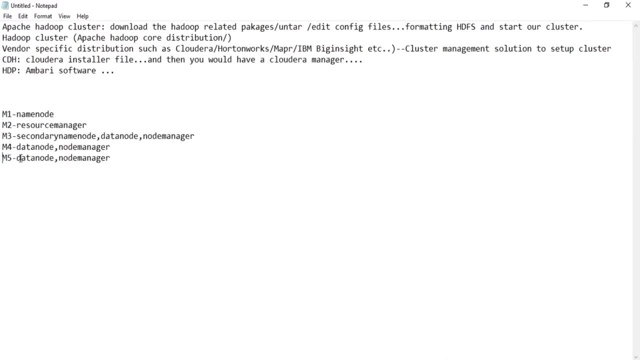 this is not the only setup possible. you could have a different setup where, on the same machines, you could decide to have data node and node manager running on a every node. however, that would not be preferred because you wouldn't want the slaves and the masters to run on the same machine. however, this setup is also possible. you could have 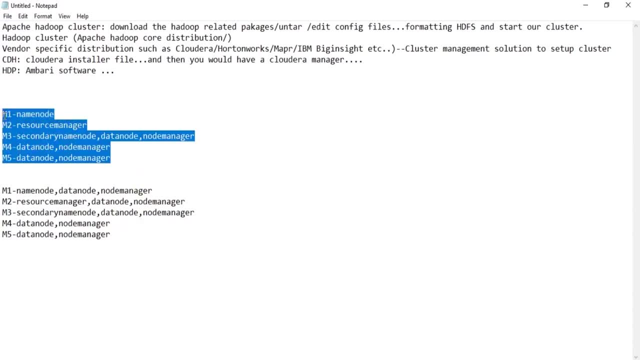 a high availability kind of setup which basically is good for cluster and for an organization, where you could have name node one which would be running here and say we can have a name node two running here, we could have a resource manager two running here and then we could have a resource manager one running here and i could still have my data node and 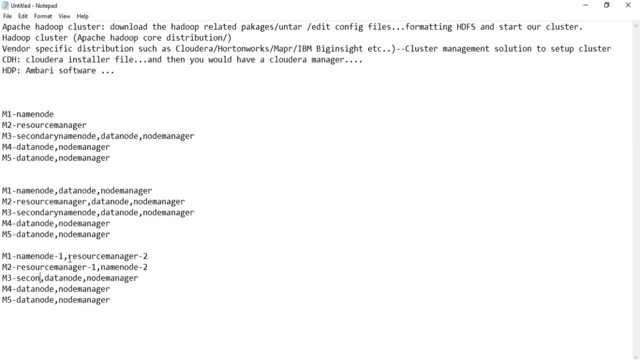 node manager running in the same fashion. now this would not be allowed in a high availability cluster because we have a standby name node. so this is one more setup which is possible and then you could have a single node setup which could be everything having on the same machine. that is name. node resource manager. secondary name: node, data node and node manager. so these are different setups and if somebody asks which is a preferable setup, then i would still go for either this one, which has multiple data nodes and node managers, not this one, or your high availability setup, now a single. 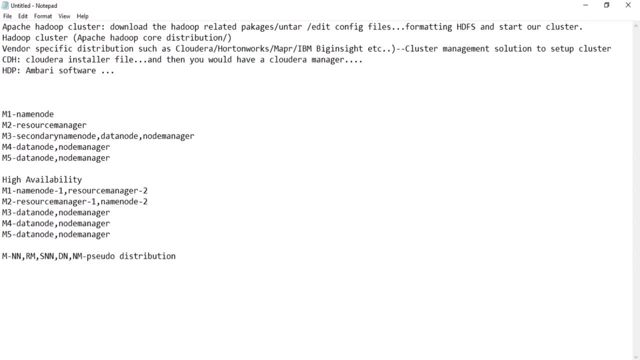 node or a pseudo distributed cluster, is basically good for testing or some development kind of activities. and these are your distributed clusters. now, if we closely see, we basically have the roles or components, demons running on these machines to take care of mainly two functionalities or two services, that is, your hdfs, which is your storage layer, and yarn, which is your processing layer. so in a hadoop, 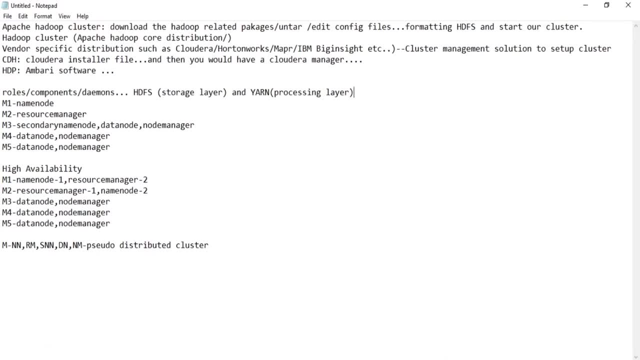 cluster, we have a storage layer and we have a processing layer for storage layer, that is sdfs. you basically have one single master and you have multiple slave processes running. so i could say: for hdfs to work, fine, i should have a name node running, multiple data nodes running and then a. 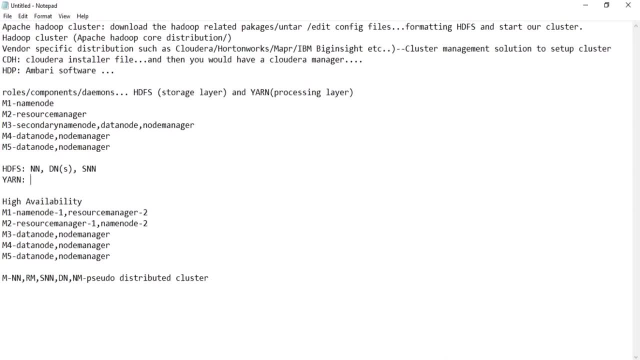 secondary name node running for yarn as a service. that is my processing layer. i would need minimum one resource manager and multiple node managers running on one or multiple machines. so these are the two processing. these are the two layers, one being the storage layer and one being the 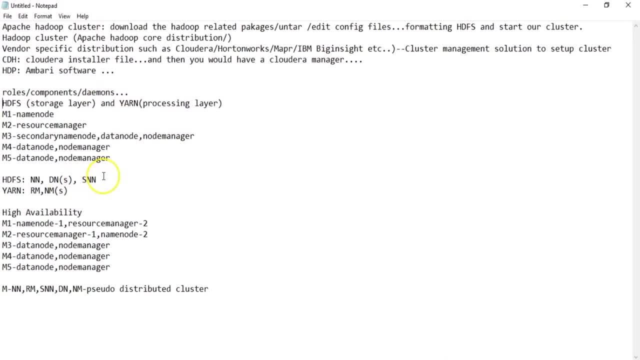 processing layer and for your storage layer. you have these processing layers and you have these processes, wherein your name node is the master and your data nodes and secondary name node can be considered as the slaves. you have your resource manager as the master for your processing layer and node managers are the slaves. now, this is briefly about the setup which could be in a 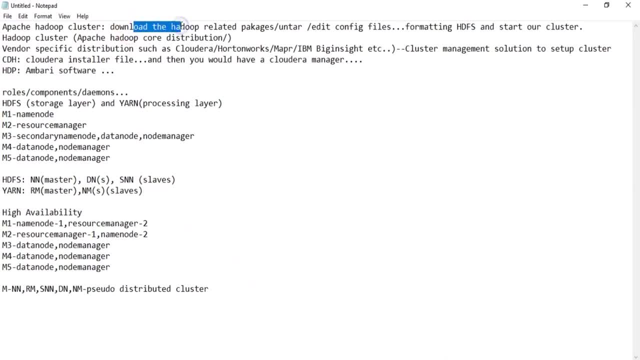 particular environment. now, say, the hadoop related packages or parcels have been downloaded, whether it is a vendor specific distribution or a patch that you Irish should have already installed earlier, which we have done. it could be also a dat, Holly, as you, and load the containervime file in the folder. you could use something else but for like this. hdfs is to be secure, as the system will detect a granular mode as nobody takes control of it, and you could load the containers and there are sites to this and you can do some other work if you are a user and your classics doesn't go under this process. 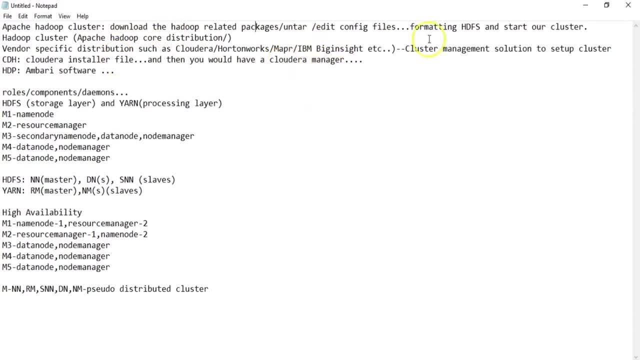 do cluster, say, untiring of that is done, editing of config files is done, formatting is done and your cluster is started. in that case your cluster would be up and running and then we could basically have- and once your cluster is up we would have the sdfs up and running, ready to allow to store data. 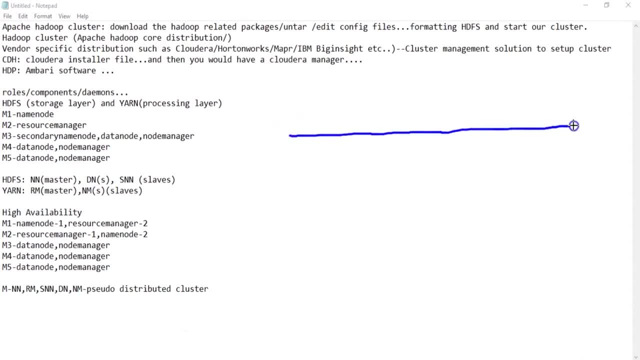 now let's imagine that this is my sdfs, which is up and running, or sdfs as a service is up and running. let's imagine that these are my nodes, which is m1, m2, m3, m4 and m5. now, while the config files were edited for each of these nodes, it would have been defined which processes will run. 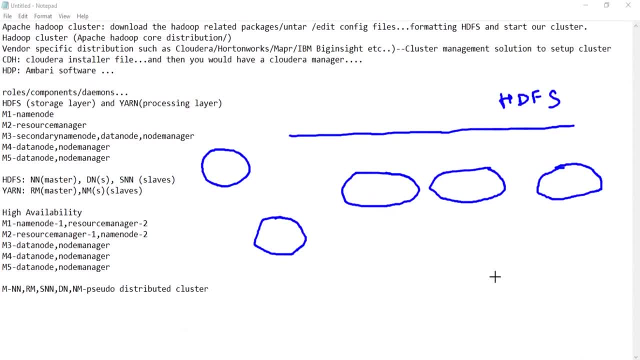 and we would have also given path where these processes will store the data. so let's say that this is my m1, this is m2, m3, m4 and m5. m3, m4 and m5 have data nodes running, so we would have defined a path. let's call it. say abc slash. 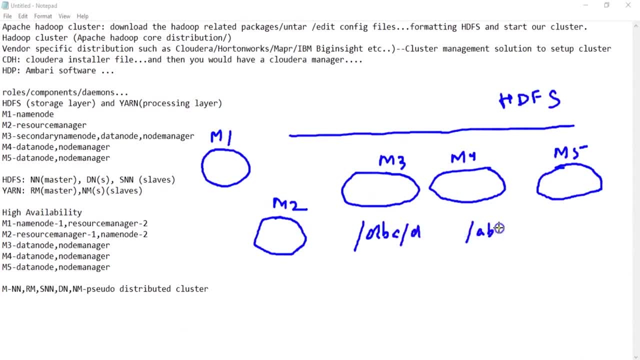 data, abc, slash again data or d and abc. so this is the path which has been defined on every node to store hadoop related data and on m1, where we would have name node running, we would have still defined a path- let's call it abc n- where name node could store its data. so once your cluster is up and running and your sdfs is, 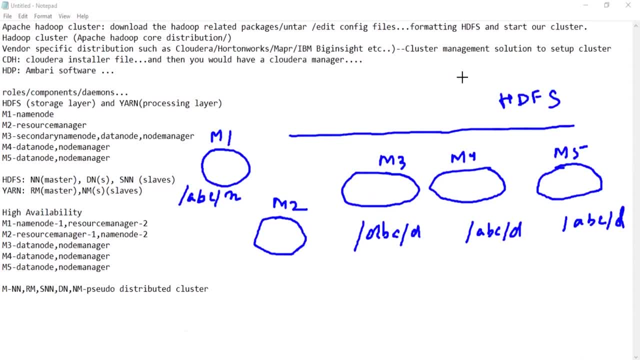 available, we can have our data stored on sdfs. now let's understand how does that work? so any client or an application which would want to write data to the cluster needs to interact with the master to begin with, say, let's say, client machine or an api or an application would be interested in. 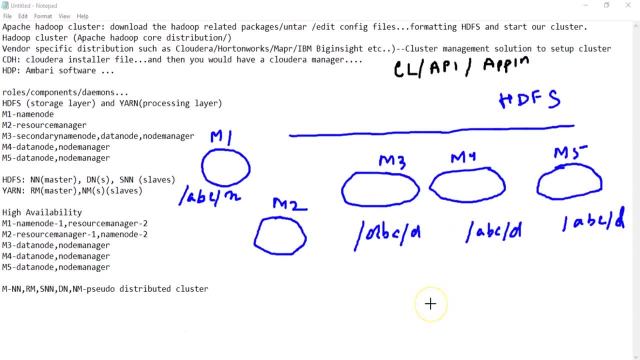 writing the data. now, how would name node know about available data nodes? so as soon as the cluster comes up, the first thing which happens is these data nodes would be sending in their heartbeat to the name node every three seconds. so data nodes send the heartbeat to name node every three seconds to let the name node know. 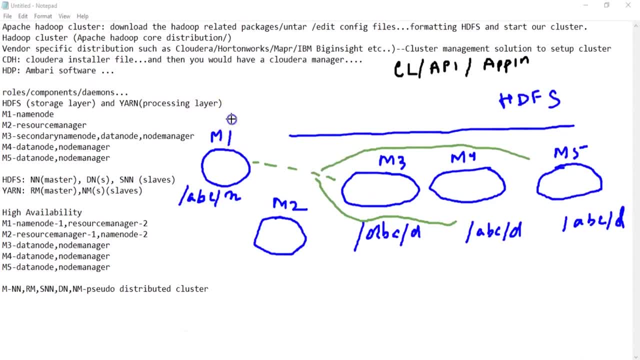 to let the master know that they are available. what does name node do with this? name node is building a metadata in its ram, so it already has some metadata in the name node. so it already has a disk which was created as a result of formatting sdfs, and now we would have metadata in ram which 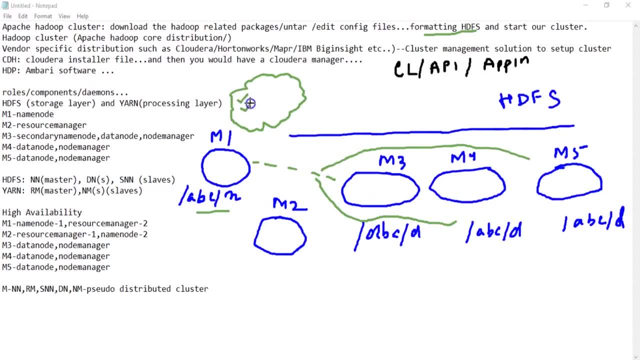 is getting built, so initially name node would have information of which data nodes are available in the cluster. now if a client or an application wants to write data to the cluster, it gets in touch with the name node. inquiring about the slave machines or inquiring about the data nodes where 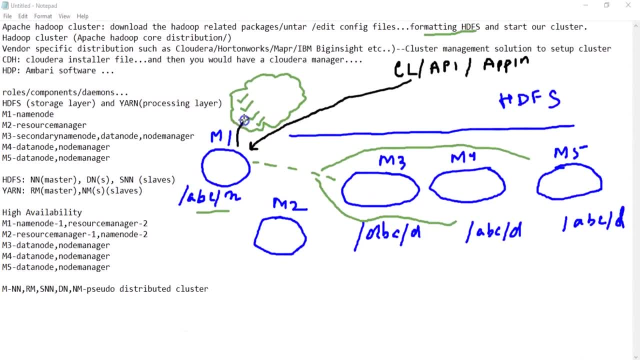 the data can actually be written. your name node refers to metadata collected so far and responds back mentioning the data nodes or the slave machines which are available for data storage. based on this response, your client takes the file to sdfs, intending to write it to the cluster. now in hadoop we basically have two things. one is the default. 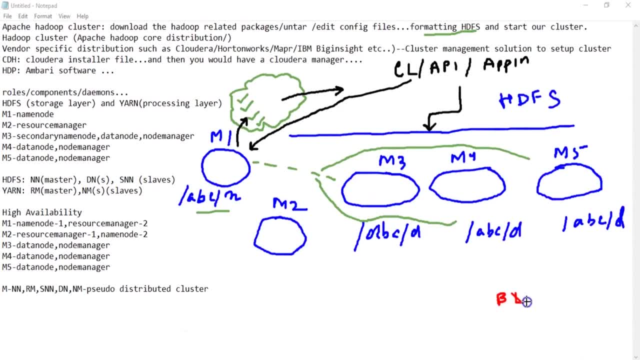 block size, which we discussed earlier, is 128 mb. so you have 128 mb as the default block size, which is customized and that can be changed depending on the average data size, and you have the default replication, which is three. now imagine the application or api or client would want to write a file which is 256 mb. 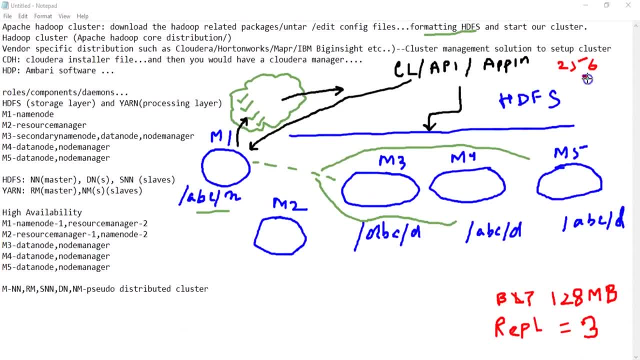 which is bigger than the block size, and this file has to be broken down into what we call as blocks, which are logical entities. so the file is taken to the framework framework will split the file into blocks and the file will be split into blocks, and the file will be split into blocks and the 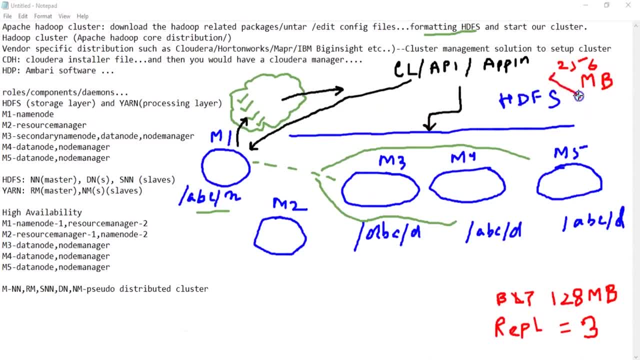 blocks. so let's imagine that this file is 256 mb. it will be broken down into two blocks, b1 and b2, and these blocks will then be randomly distributed to the slave machines, that is, the data nodes. so we would have block one, say, getting stored here now you could also have block one getting stored on. 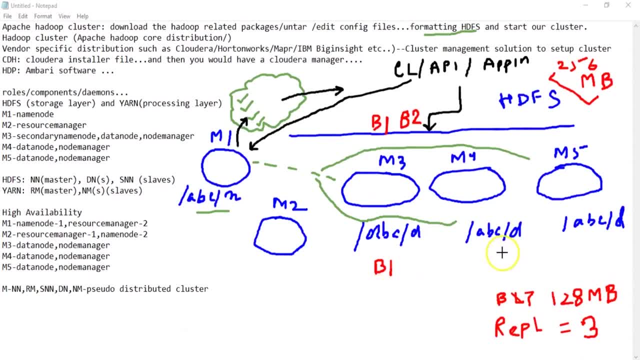 any of these data nodes. so we would have block one, and then we could have block two, which could be written here, and then you would also have the data nodes which are stored on any of these data replicas sitting on the machine. so the rule of replication is: you will never have two identical. 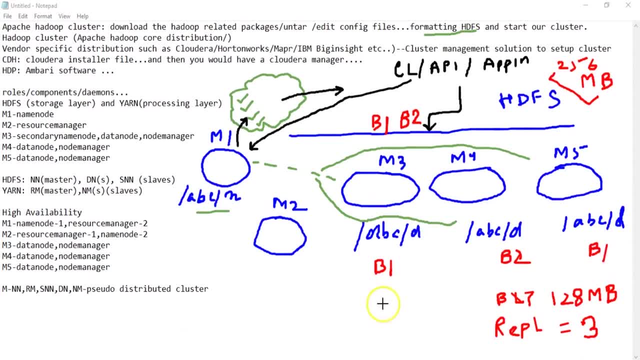 blocks sitting on the same node. so if i have block one here, then i will never have a replica of block one again on the same machine. so we will have a replica of block two here, block one here and you have a replica of block two here. there is no differentiation between which one is the original. 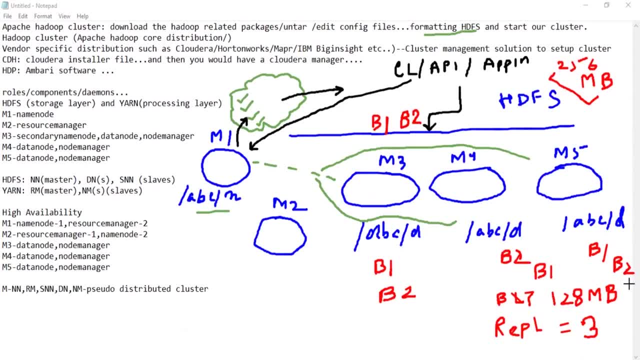 and which one is the replica for the cluster. all the blocks are the same, so we will never have a replica of block two. there is no differentiation between which one is the original block one, and also each block is separate from the an台Why did don't forget Daily. 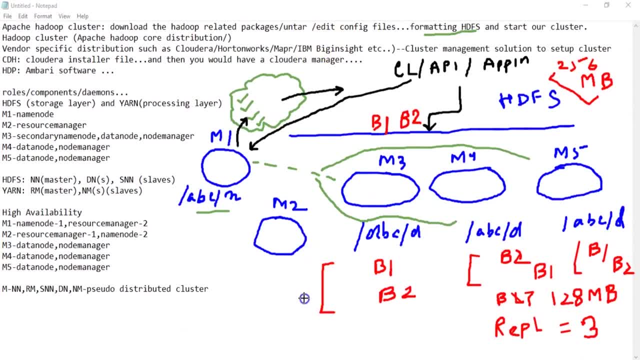 and what also happens is, after the blocks are written, your data nodes are repeatedly sending blog report to name node every 10 seconds and this information is again updated in the name nodes metadata. so now name node will have information. what are the files? the files are broken down and 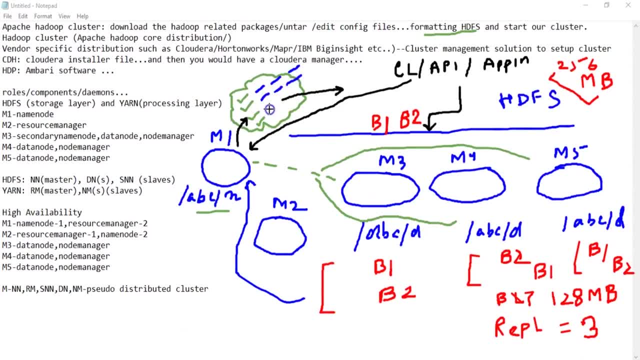 to what blocks the blocks are residing on which data nodes and this metadata is getting built in the name node as data nodes: thenê data. can you change the description? Tabii, criticisms can be changed to regular works. ancer nodes respond with their heartbeats and also every 10 seconds with their block report. now we need to. 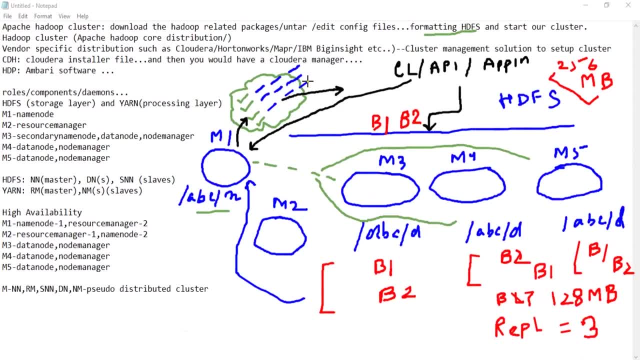 remember one point here: that name node is basically a master and data nodes are the slave. hadoop, as a framework, has been coded in java, which basically means that every directory, every file and file related block is considered as an object which is getting stored and for every object which name. 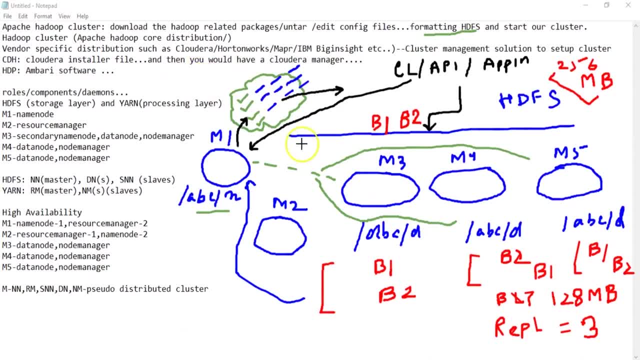 node is tracking 150 bytes of name nodes ram is utilized, which also tells us that if the block sizes were smaller than 128 mb, then for the same file we would have more number of blocks, which would mean that name nodes ram would be over utilized and overload name node. so block size: 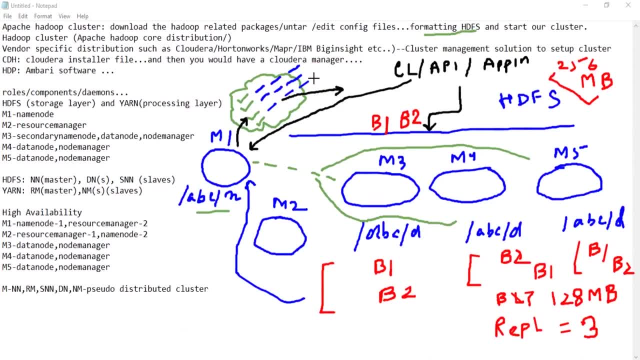 has to be chosen with a lot of consideration on the master's ram and what is the average size of the data. now this is how the data is distributed: in blocks and distributed across the data nodes. thus sdfs is very fault tolerant, because if any of the data nodes fail, then you still have other data nodes which have the replica of data, thus making 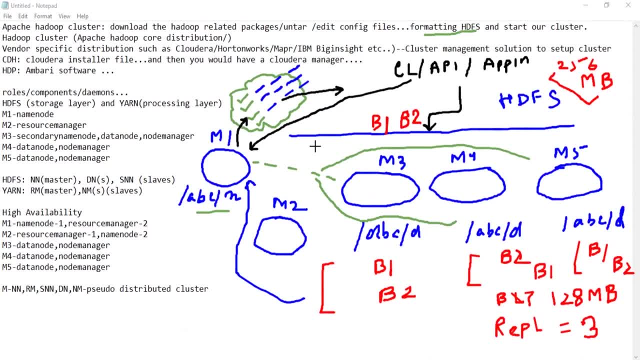 it possible to read the data and access the data even if multiple data nodes go down. now there are other internals. that is, how data nodes are placed in racks or what has rack awareness to do in block placement. we will learn on all that later. so this is how your sdfs works now. there are many other things. 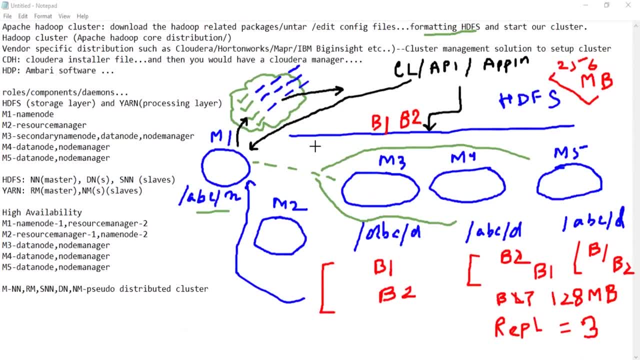 such as the read and write process, which is taken care by your methods, such as open and create, which internally are playing a role when a read or write operation happens. also, facts like replication is a sequential process, but right activity is parallel. so we can learn more functionality of sdfs in later. 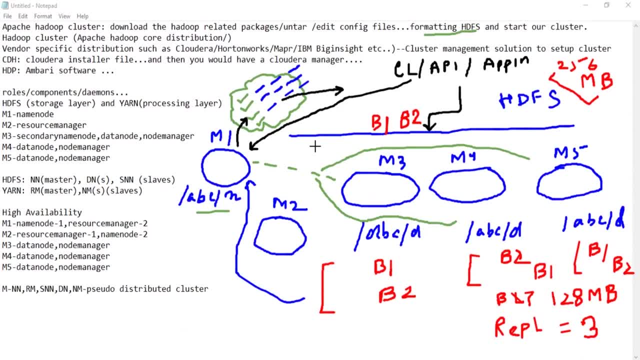 sessions. but this is in brief on how sdfs works, how your file is split into blocks and the blocks are getting stored on the disks. note that the block contains the data. so even if you have a file which is one kilobyte, and if this file is to be stored on sdfs, it will still use a block of 128 mb. 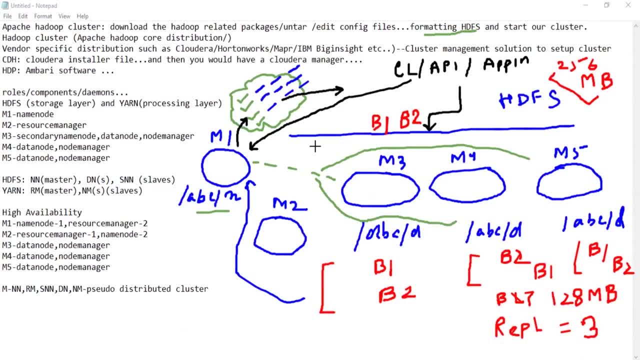 which does not mean that there is a disk space getting wasted. when the block resides on the data node's disk, it will only occupy one kilobyte of space for the data it has, which means that block is a logical entity to take your data to the disk and get it stored on the disk. this is how your sdfs. 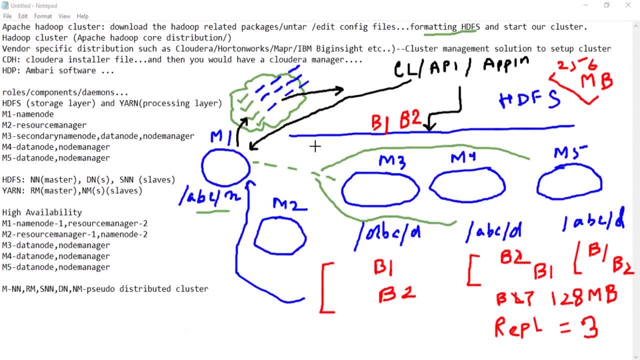 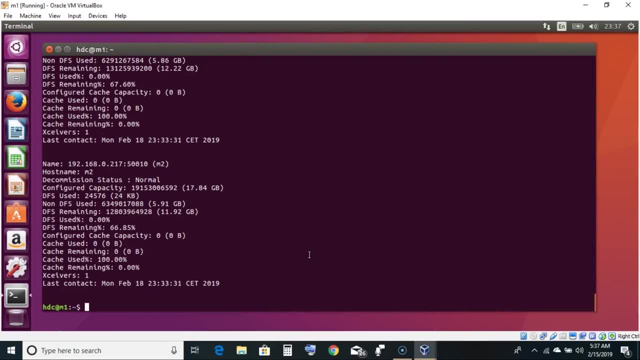 works and basically takes care of reliable data storage across machines in distributed fashion. now that we have set up a two node cluster which has two data nodes, two node managers, one master machine, let's go ahead and see how sdfs works. let's go ahead and see how sdfs works. let's go ahead and. 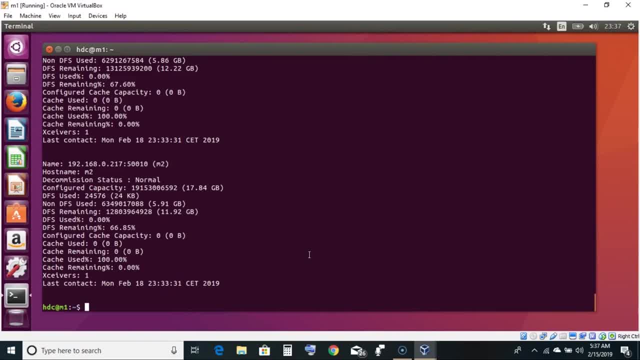 see how sdfs works. let's try working with sdfs. let's look at quick commands which allow you to write data to the cluster. although there are different ways, the first way is using commands, the second is using an ite and where you could write your code to use hadoop's file system api. 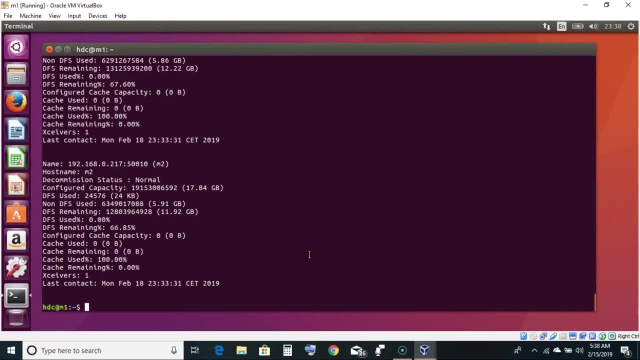 and the third is a graphical user interface called hue, which normally does not come with apache, although it can work with apache. it comes as a service with cloud data and other solutions to work with sdfs. we need some sample data now. there are various websites from where. 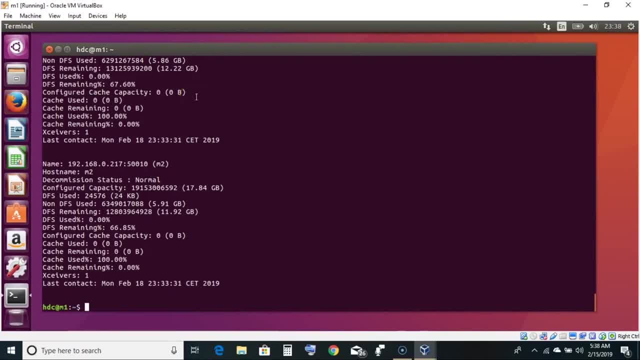 you can get some sample data, so you can open up your browser and let me show you some sample places, or sample data set links from where you can download bigger or smaller files, which then can be used to write data to your sdfs, although you could just pick up a local file or you could 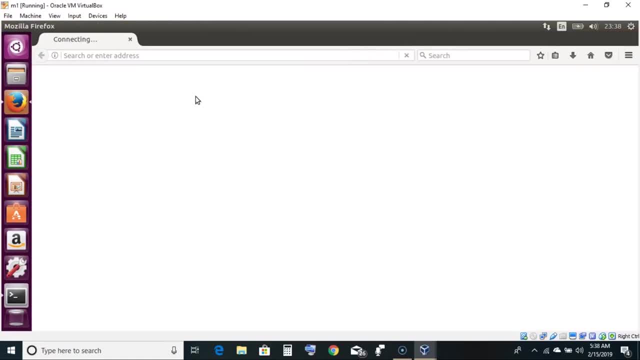 create your own files and write them to sdfs. there are various data set sites which can be used so, for example, you can type in machine learning uci data sets, and this is one link which has more than 200 data sets which can be used for even data science kind of activities. 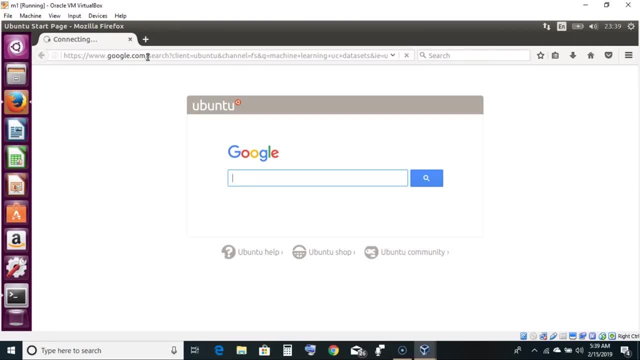 which can be used for testing with your algorithms, and you can download data from here onto your local machine, and then from your local machine we will be writing the data to hdfs, which then, based on the size of the data, splits the data into blocks, and your blocks would get stored on your underlying 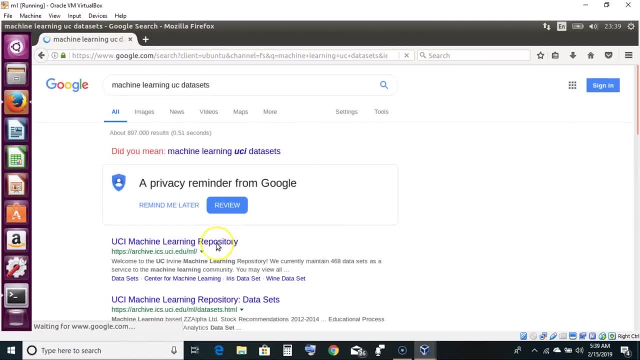 machines wherever data nodes run, so i can click on this uci machine learning repository or even just on data sets. to be very specific, all we need is some sample data sets. you can get kegel data sets. you can get data sets from yelp website, which are bigger data sets zipped, and you can 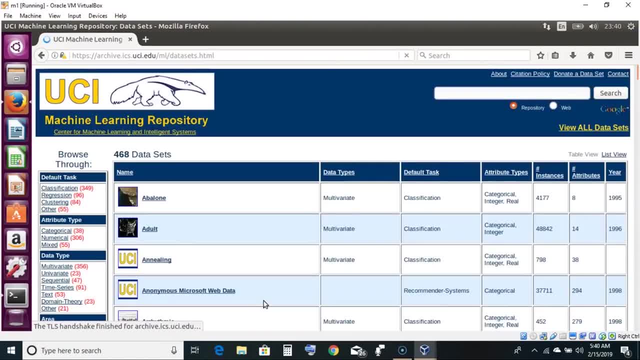 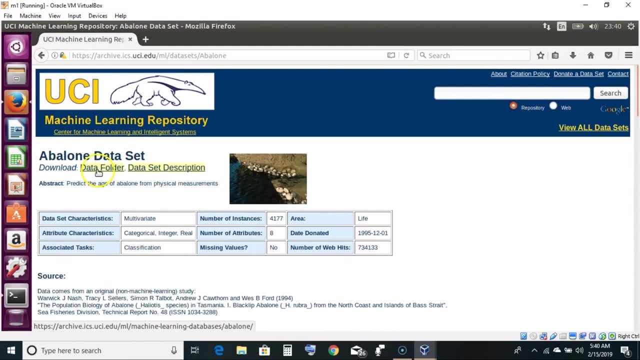 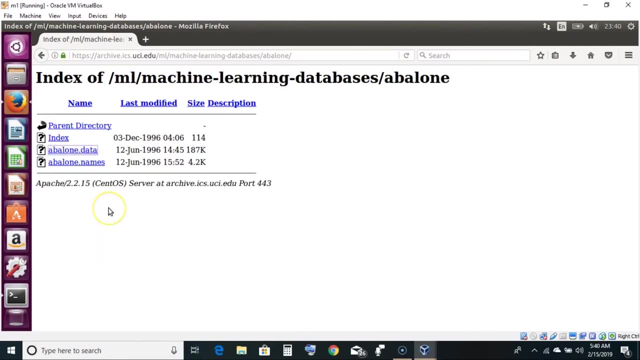 be using them to write data to see how your files split into multiple blocks. now, here we have a lot of data. we can click on any one link to begin with, and here i have the data folder shows me the some file and i can just right click on this save link as and save the file. this. 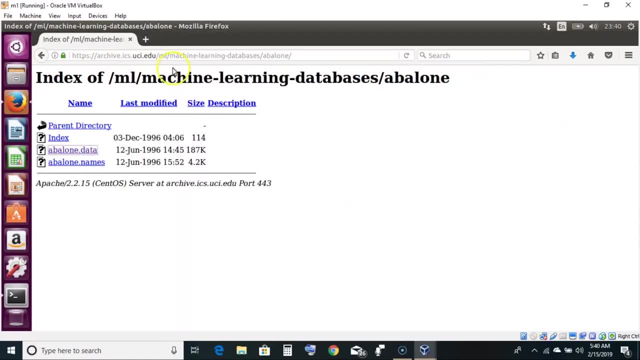 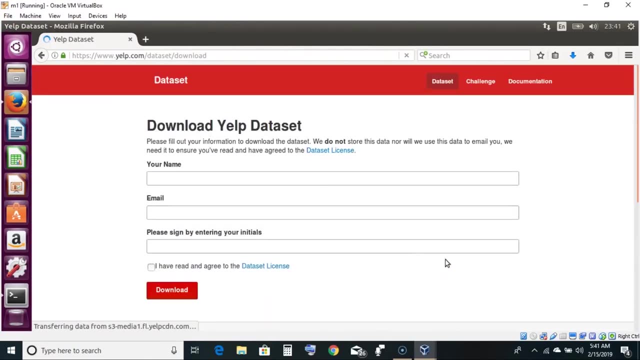 is a simple text file and we can save it and you can get various data sets from here. you can even go to yelp data set challenge and that has bigger files which are zipped and they can be downloaded. so you can click on download data set, although i will not start the downloading. 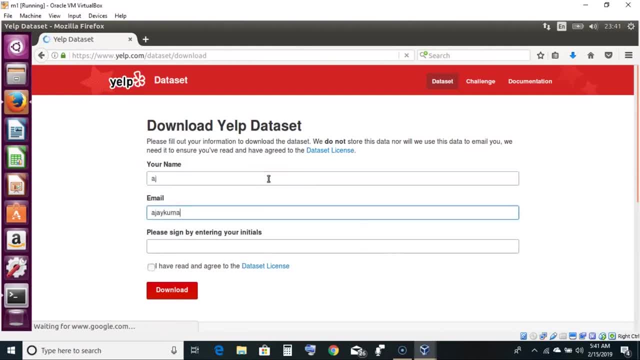 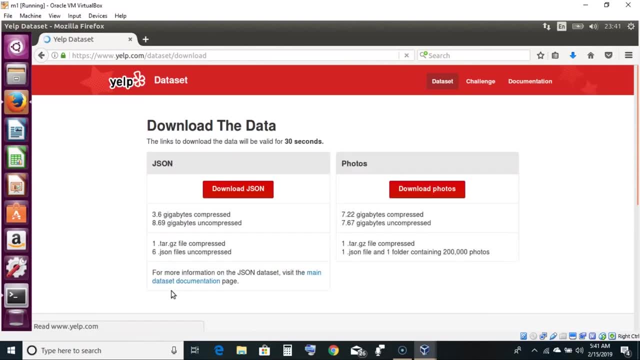 here you can just give in your name here, just some email id, some initials, and you can click on download. so this is one more website where you can download the json data sets, which are 3.6 gigabytes in compressed format, and then you have photos which are in 7.2 gigabytes. you can also say gutenberg. 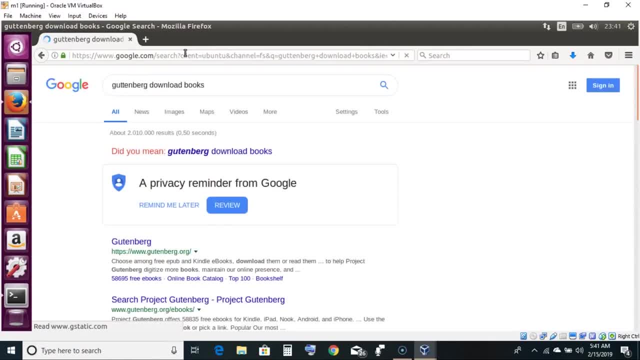 download books, and that is again a website from where you can download free data sets which are not very huge. so try to get some variety of data sets in different formats which then you can write to hdfs. you can even use your sdfs log files, which already exist on your machines and you don't need 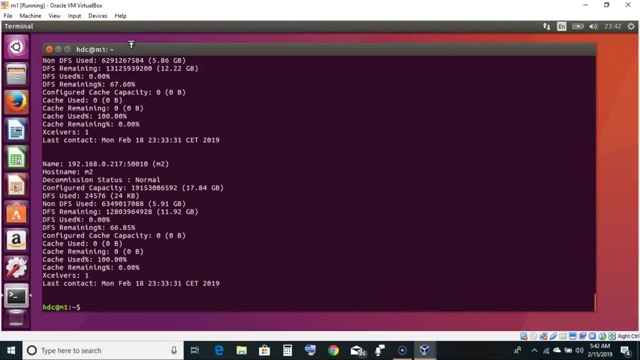 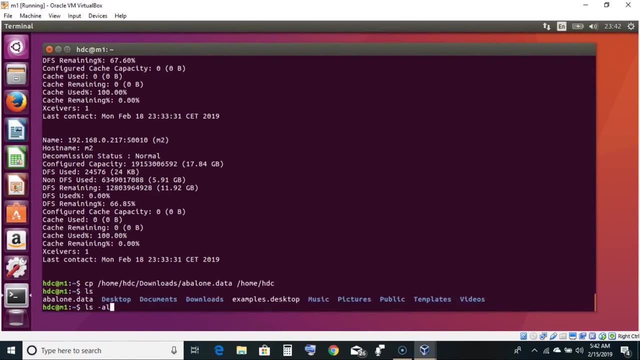 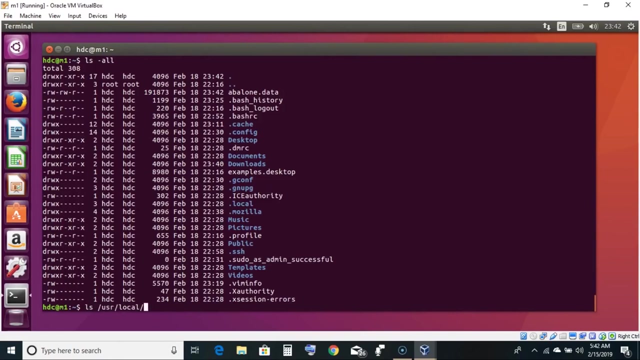 to download anything from internet now. let's close this for now. so i already have some file. let's copy this from home hdc. downloads was my file. let's copy it to home hdc. and here's my file. i can check the permissions. so that's owned by sdc. i can even look into user local hadoop logs and there are some already log. 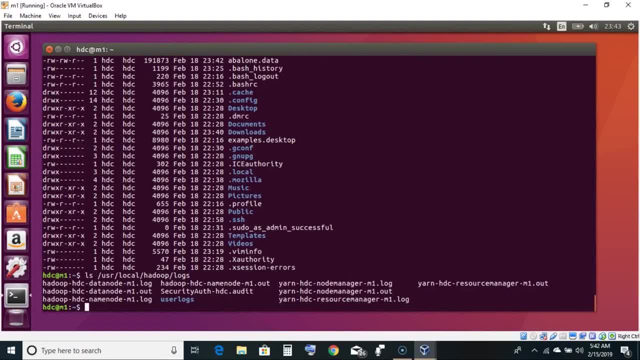 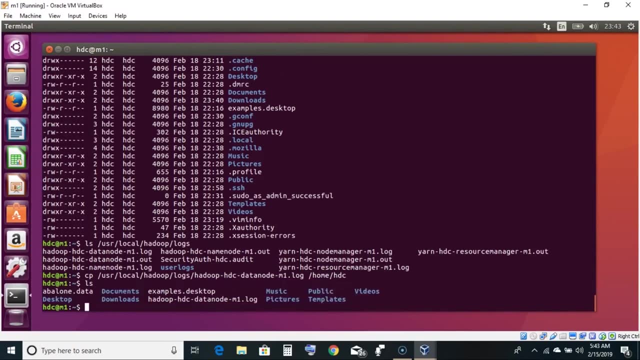 files so you can even copy some of these files using copy user local hadoop logs and let's take hadoop data node related log and let's copy to sdc for our testing. and now we have some other files now to work with sdfs. as i said, you can. 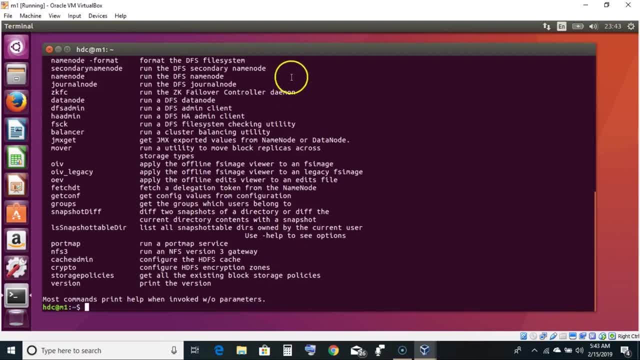 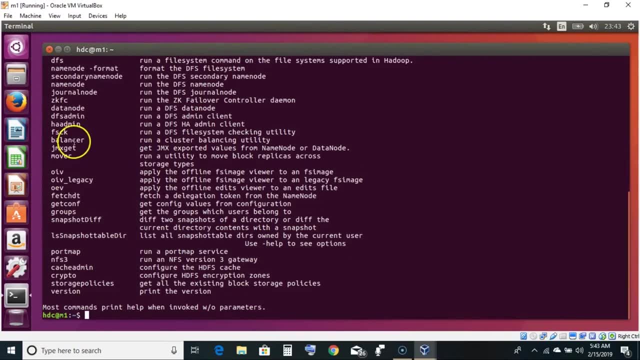 always type in hdfs and that shows you various options. now we already used the first option, which is name, node hyphen format. we also used hd dfs admin to look at how many nodes we have and to work with your sdfs file system. the option is dfs, so you would say hdfs, dfs and then you can. 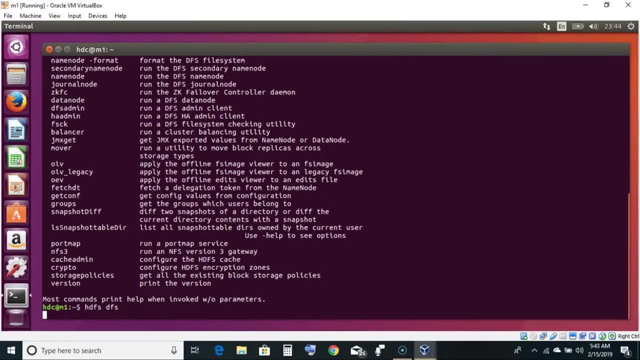 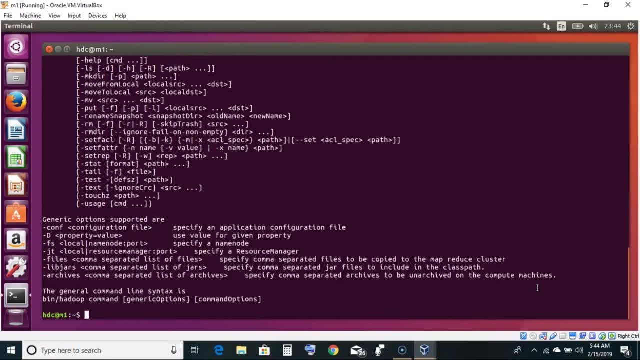 always hit on enter. it shows you various options to work with your distributed file system, like creating a directory, copying some files, getting data from your sdfs to your local machine, changing the permissions, changing the replication and many other options. so here let's click on hdfs, dfs, let's 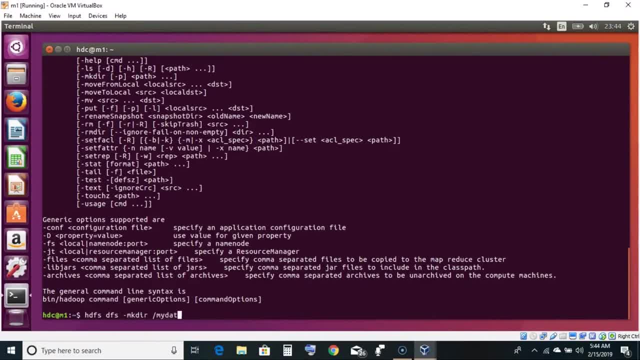 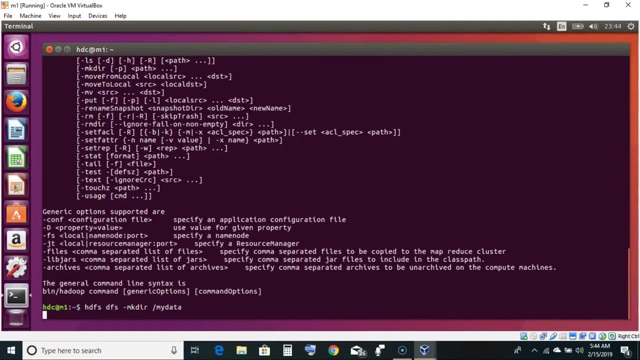 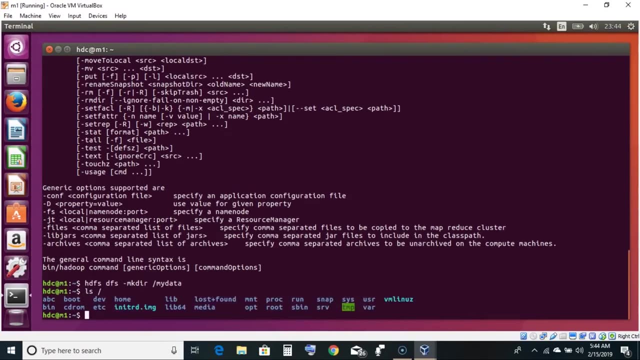 create a directory and let's call it my data. so this is a directory i'm creating on hdfs. remember this directory will not be seen on your local machine. it is a hdfs directory. now, if i look in my root, i don't see my data because that's a sdfs directory which is technically getting created on. 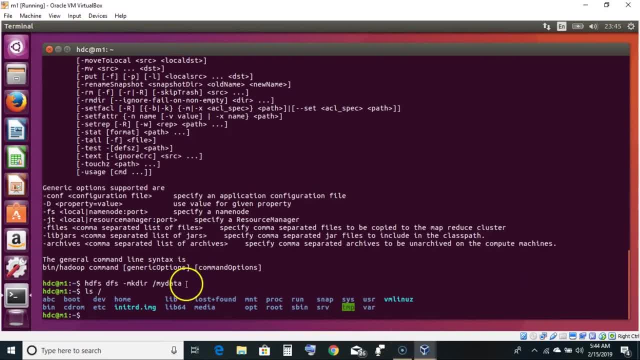 sdfs and once you start writing data to sdfs, the relevant blocks will start getting stored under abc slash data. so as of now, we can always keep a browser open to see as we work with sdfs. how does the data propagate or come to your distributed file system using the web? 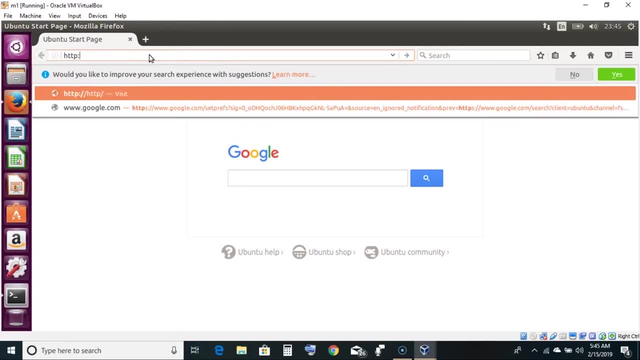 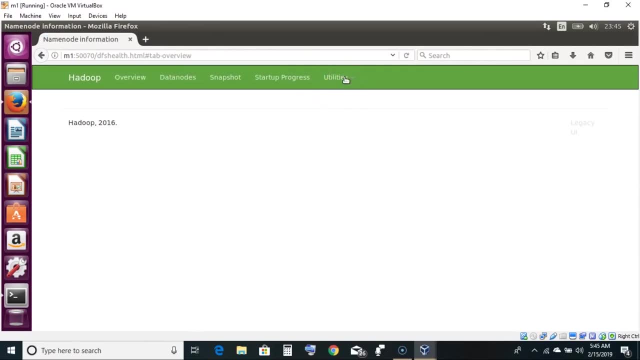 interface. so here let's say: http slash, slash, m1, 5, 0, 0, 7, 0, and that's my browser interface. let's click on utilities and let's click on browse the file system, which will show the directory which we have created, although that does not have any data as of now. 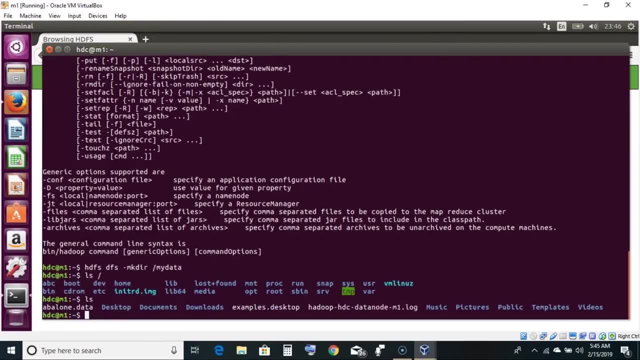 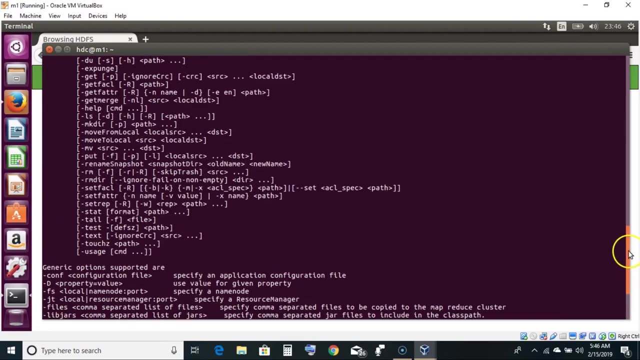 let's go in here. and now we know that we have some files here, so i will say hdfs, dfs, and this has two options: either i can say put or i can say copy from local. both of these do the same thing and both of these you can find here. so we have put and 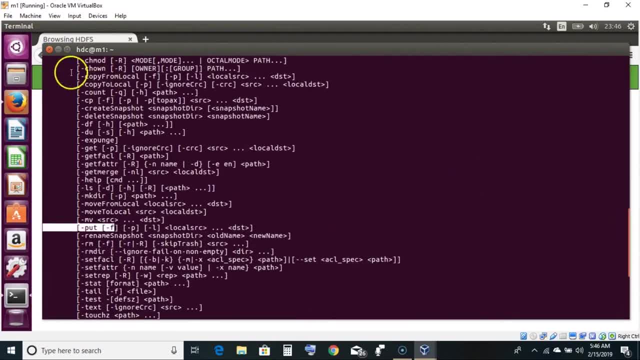 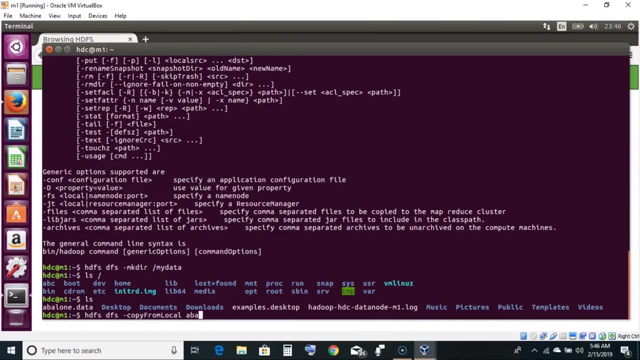 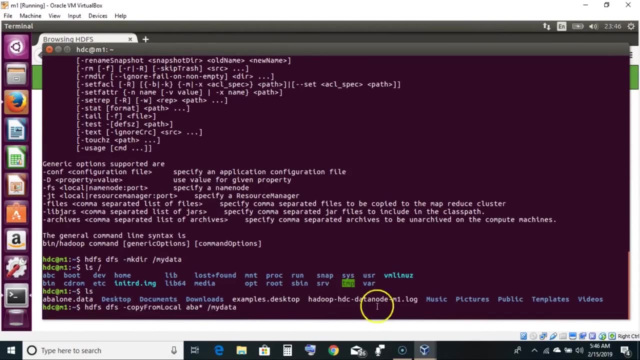 we should have copy from local. that is, you are copying the data from your local machine to your hdfs. so now i will say copy from local. i will say take the aba directory or file and put it in. so now i get my data. so now i'm technically copying a file from my local file system to my hdfs, which is then 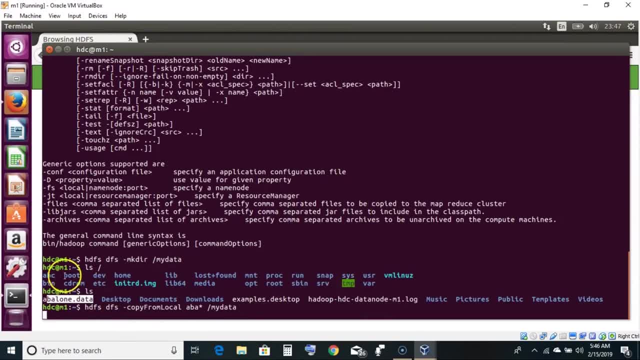 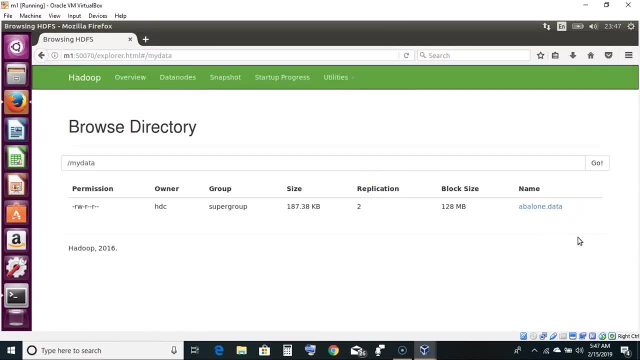 using my local file systems path. so this is done. let's quickly check so by clicking on my data. if my data is written now, if you see, this file is 187 kilobytes. however, this will still use a block of 128 and in my previous sessions i already explained why a Block of 128ates. but when it does remain, it goes into headspace. 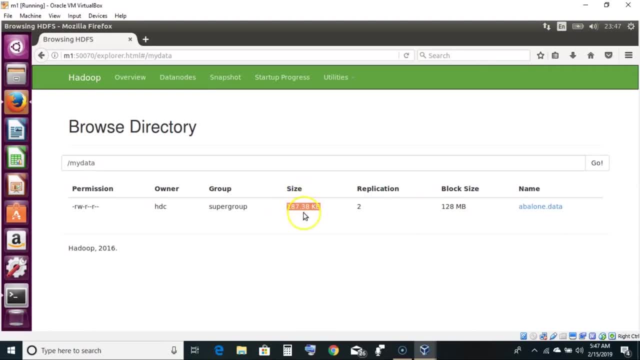 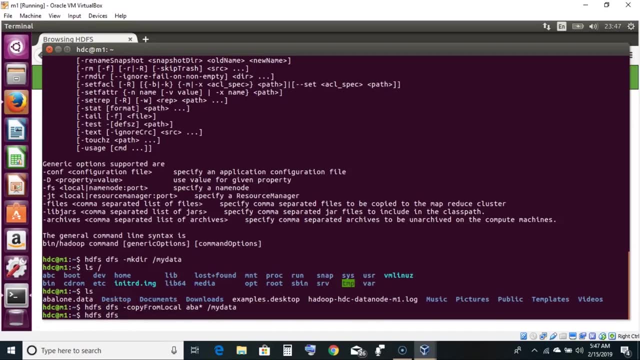 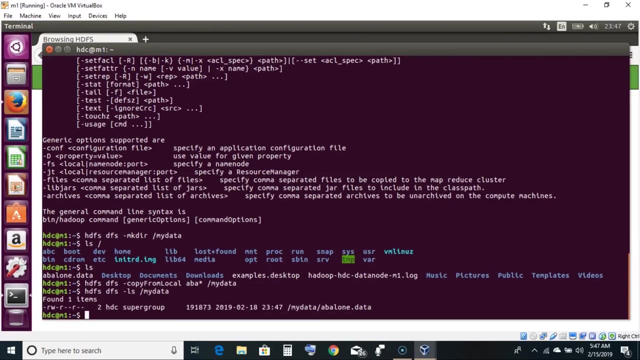 goes to the disk, it will only occupy the space for the data the block has. We can quickly go in here and we can do a HDFS, DFS listing of my directory, which should have my file now, and we can quickly check if my file is replicated either using the web interface which says replication is. 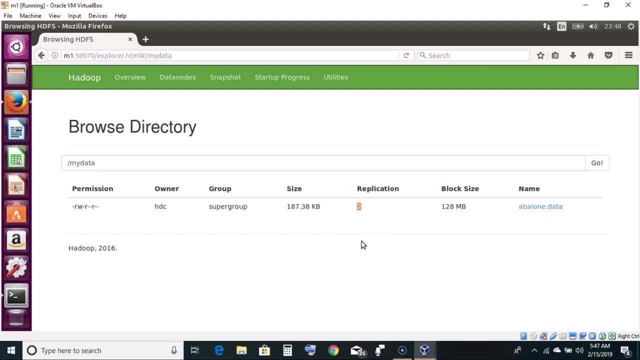 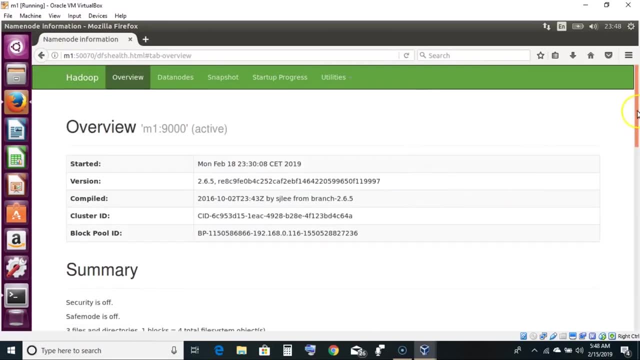 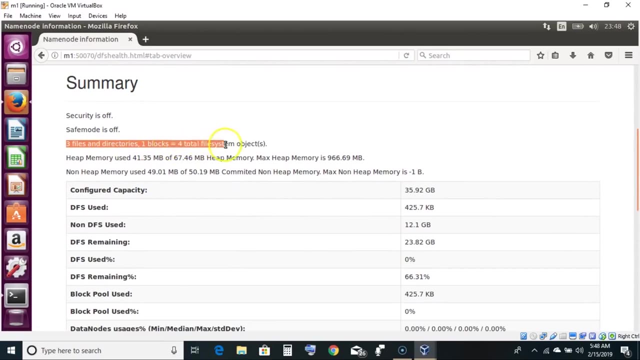 true, That means the file related blocks should be getting stored on the underlying data nodes. We can always click on overview if we would want to browse and scroll down, which says there are three files and a directory. The file has one block, so totally you have four file system objects. 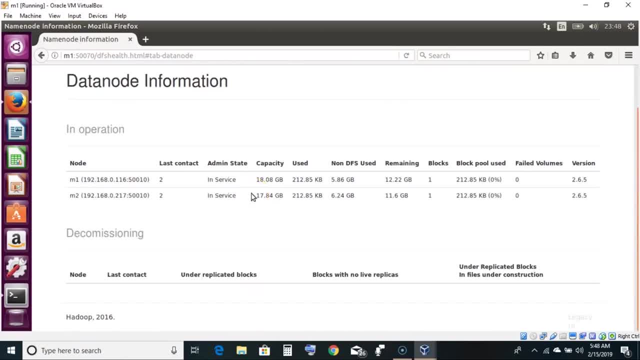 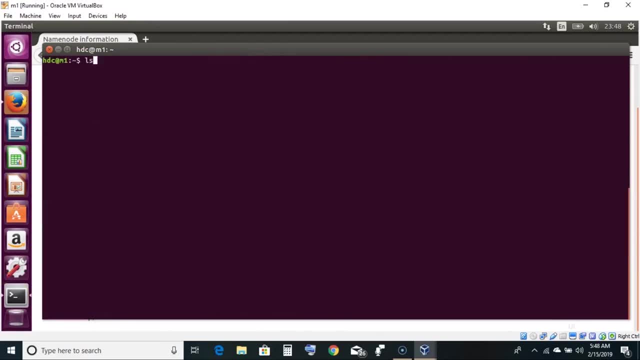 We can scroll down to show or see we have two live nodes and if you see, each node has one block. We can always look from our data path by looking into abc slash, data slash, current that has block. We can also look in the block pool directory that has current, that has finalized, that has sub directory. 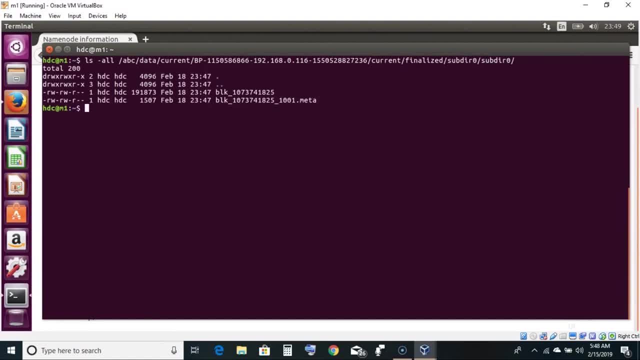 sub directory and the block. Look at the size of the block. it is 191, which relates to the kilobyte size which we are talking about. Similarly, we can check on m2 machine, which also has a data node running, to make sure our file related block is replicated. So look in block pool: current, finalized. 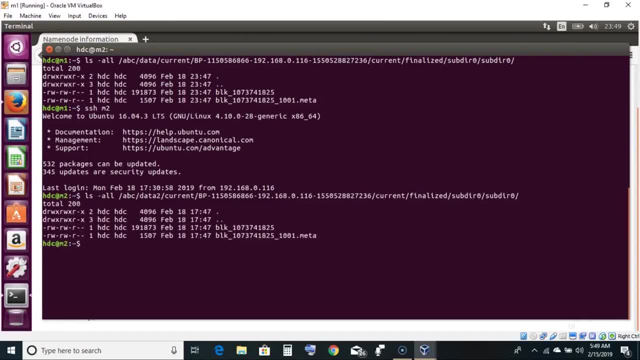 sub directory, sub directory, and that shows me the same block, which is the same block, which is the same block. This ensures that my data is getting replicated as per whatever factor we have set, and my file is written to HDFS. and now I can also do a complete listing. I can just say a recursive listing to: 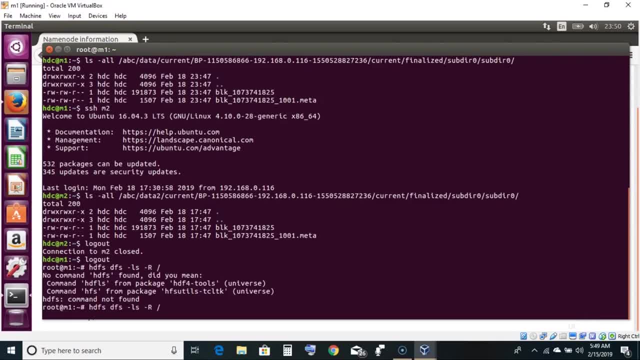 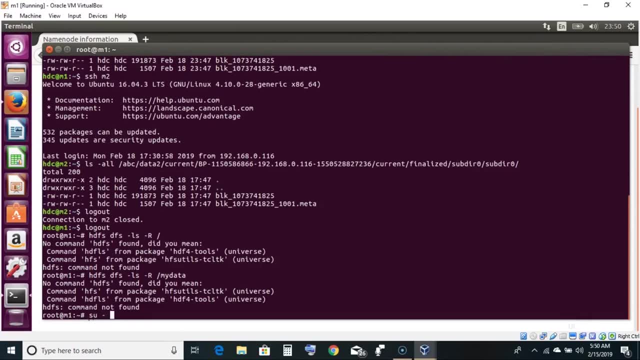 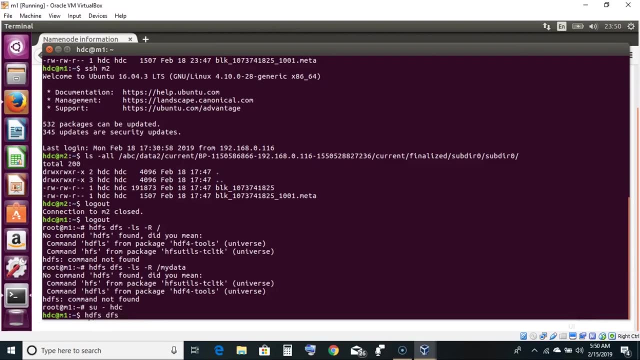 show me all the directories and all the files which I have in my HDFS. I think we are forgetting something. we are logged in as root, which is not right. so we need to be logged in as root And then we can try our commands. that is HDFS, dfs-ls slash, which should show me my directory, but then 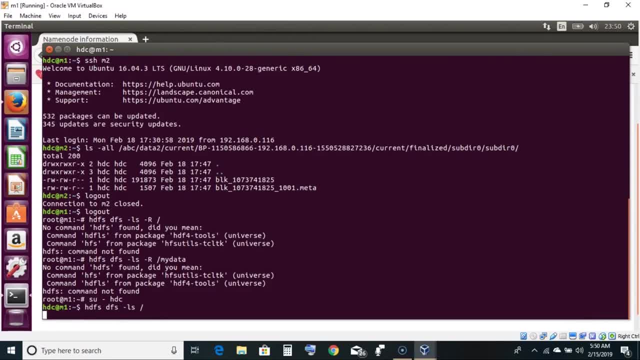 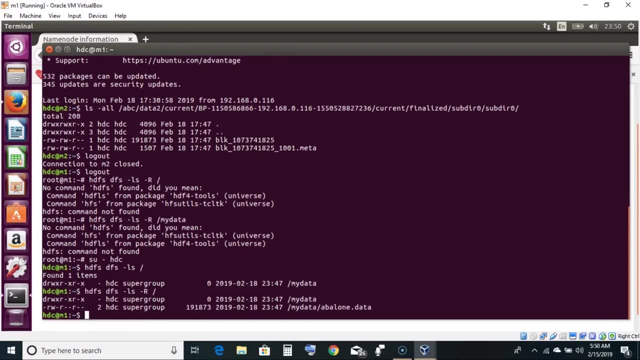 if you would want to do a recursive listing of showing all the directories and files, you can just add hyphen r. So we have written a file to HDFS in my data directory. Similarly, I can write using a put command. Last time we used a copy from local. I will use a put command. I will say: 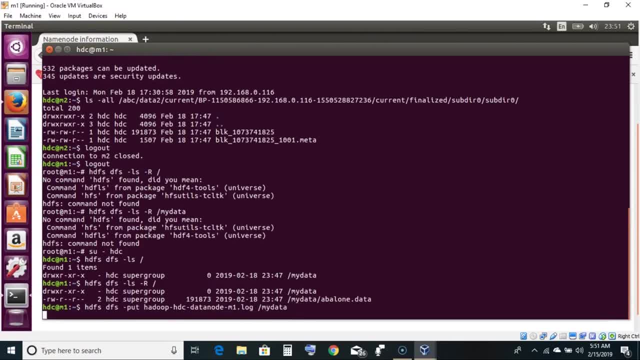 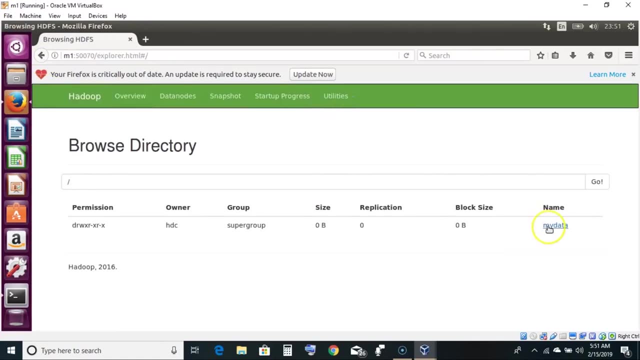 let's take this log file and let us write it to the my data directory instead of copy from local. I'm using a put command which also allows me to write the file to my HDFS. Once this is done, let's go to the web UI and let's go to browse the file system. Let's look in our directory and that. 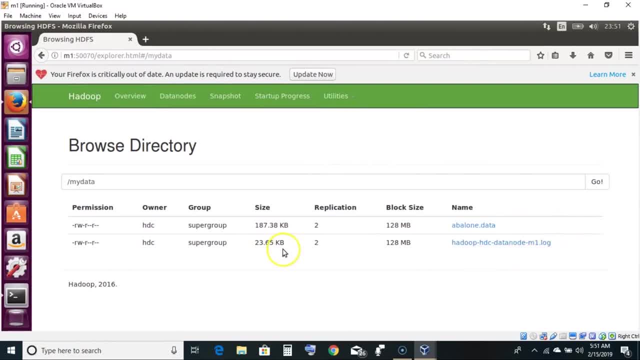 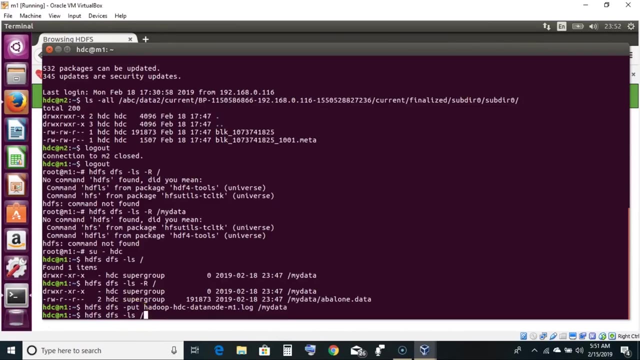 shows me that I have a log file which is even smaller than the first file which we wrote. It is in kilobytes. however, it is replicated. It is using still the block size, It is still using the and we can always go back and look at the terminal to see if, for my new file, I have a new block which. 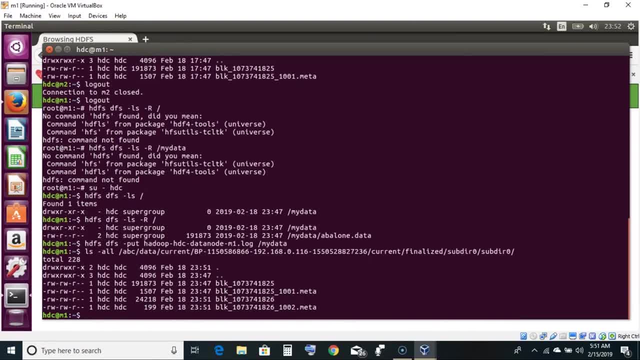 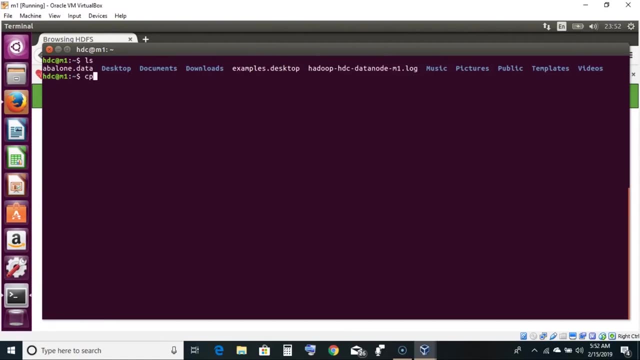 should be in my data path and if you see this, this is my block, which will also have an application on machine 2. so this is how you write one file, or you could write multiple files. you could write multiple files. let's create some files here. so I have these log files. let's say hadoop log and let's 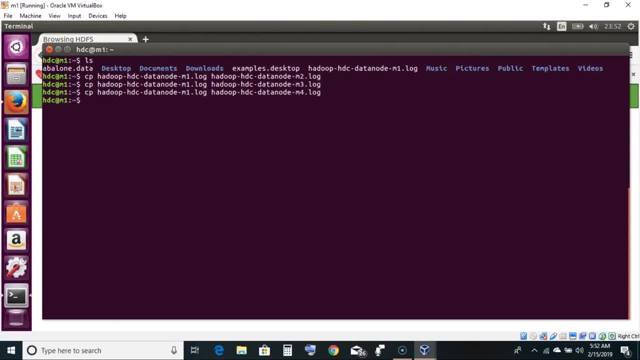 give it a name like this. so now, if you see, I just created multiple files and I can also say sdfs, dfs, make directory, let's say my data 2, so I'm creating a new directory on my sdfs and then I can even copy multiple files or a complete directory. so all I need to do here, 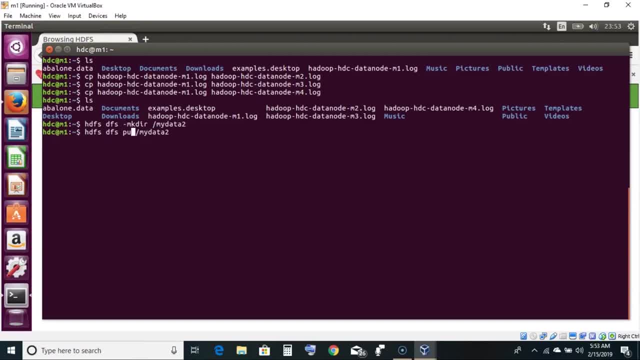 is give a matching pattern or a directory. so I'll say sdfs, dfs, put, and then I can say: take all the directories of files and put it to my data 2. remember this: one file or multiple files are following the replication, what has been set at a cluster level. now, if we 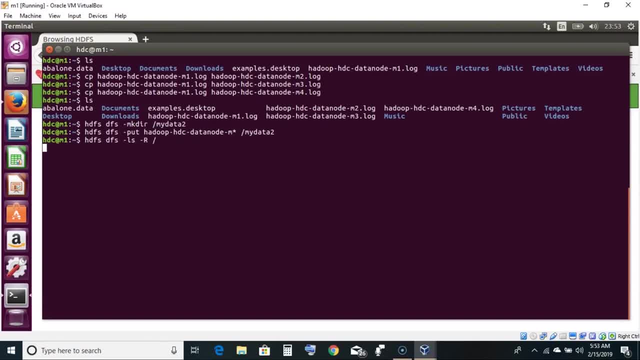 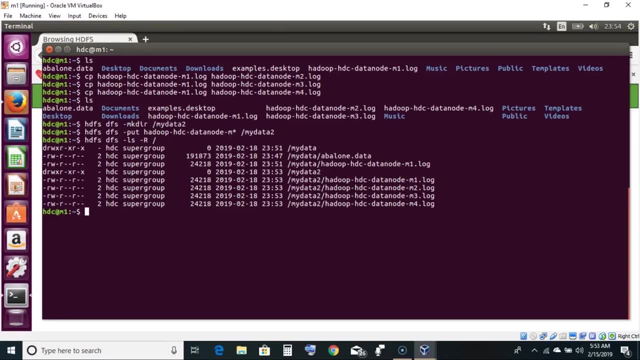 do a recursive listing where I would want to see all the directories and the files which are within my hdfs. I see that I have a my data directory and I also have a my data 2 directory which has multiple files, and all of the files are in my hdfs directory. so I can say: take all the directories. 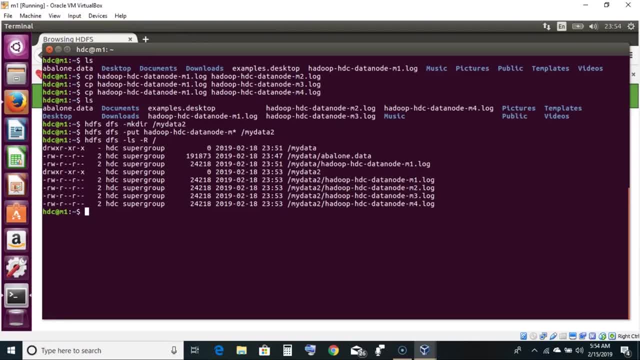 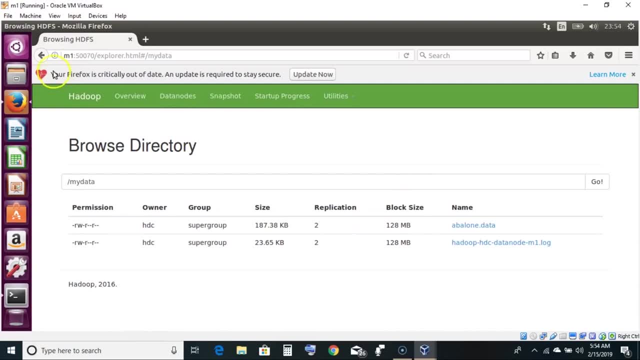 of files within the directory are following the replication set at a cluster level, so all of them are having their blocks replicated twice. we can always go back here. we can just do a back and that shows me what I have in my data 2. everything is replicated twice. what I have in my data is also. 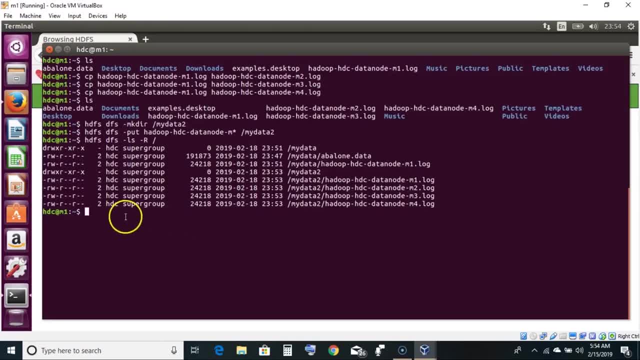 replicated twice. now, sdfs also has a functionality where you can write data with a different replication. so let's create one more directory. and now I'm going to create my data 2 directory. let's write data with a different replication. so the way I write my files. 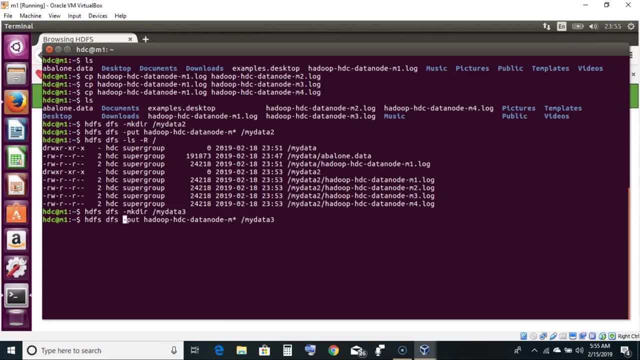 I follow the same thing. however, now I will say hyphen DFS, dot replication and I will specify it as one. so I am passing in as argument and I am specifying that I would want to write data with the replication of just one. so my blocks will not be considered under replicated and I am choosing to write these files. 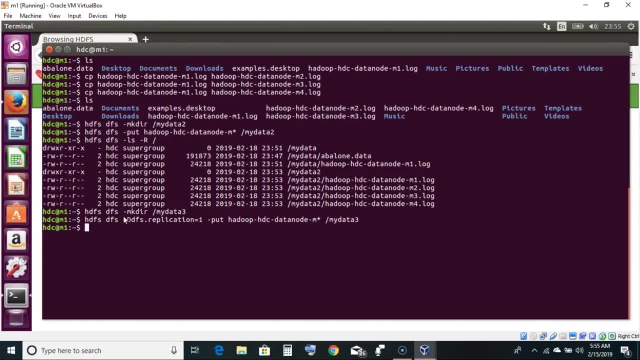 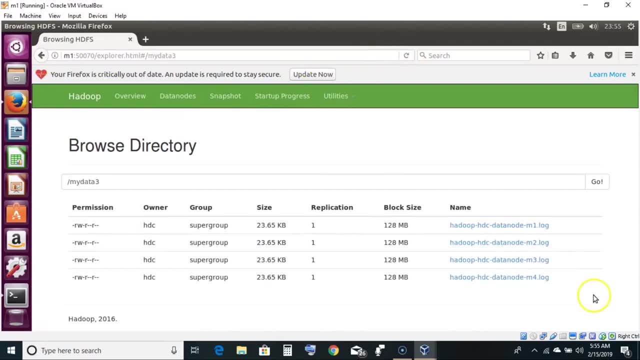 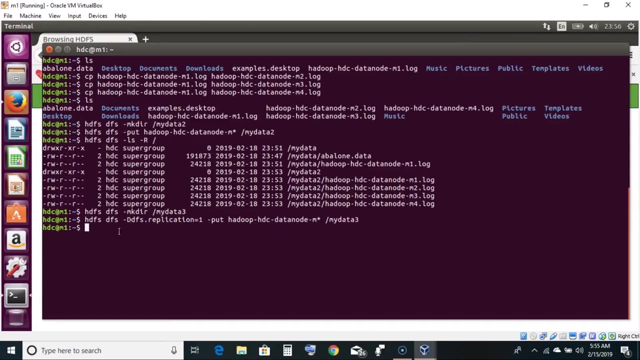 in this directory with an application of one. we can check from our browser interface by just doing a quick refresh, and here, if I click on my data 3, it shows it follows an application of one. there is also a command to check your replication status using HDFS. so we can say: HDFS, fsck, slash files, slash blocks. 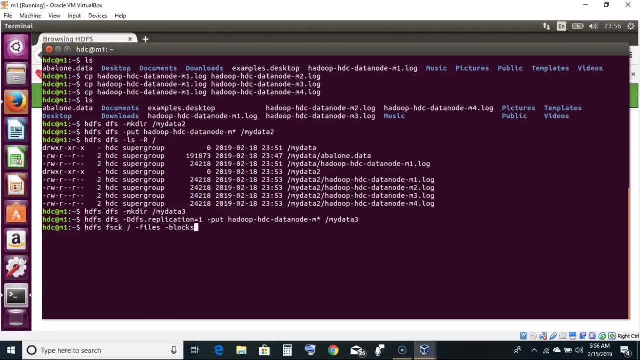 and if I would want to see only blocks or only files, I could just write it as one. so I will say hdfs, fsck, slash files, slash blocks, and if I would want to see only blocks or only files, I could choose one of them. now, here I have, given a complete HDFS file system. I can. 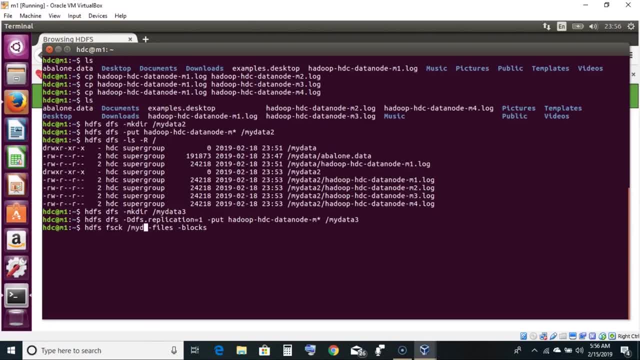 replace that with slash my data, so I can say my data 3. this is what I would want to see, and this will show me within this directory how many files I have, how many blocks does each file use and is it replicated correctly? so my fsck command. 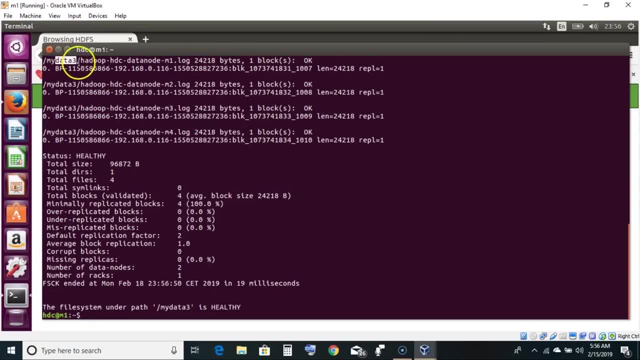 gives me an information that in my data 3 I have one file which is 24 kilobytes- uses one block because it is very smaller than 128 and it is replicated only once. so there is no situation of over under miss replicated blocks. we have our files. 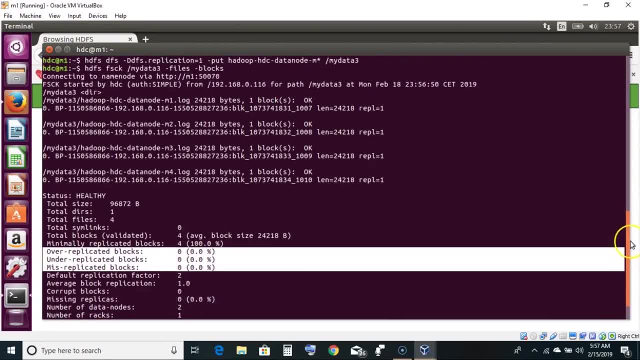 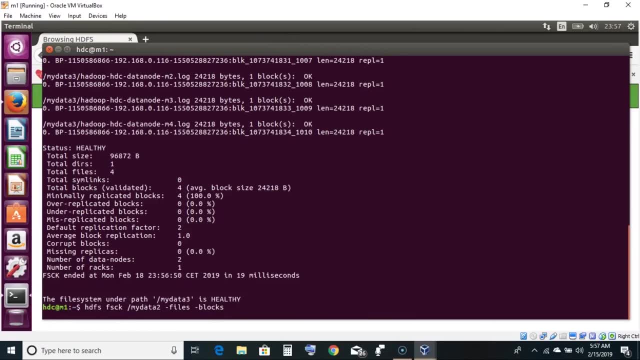 correctly replicated as they were specified while writing. same thing can be seen for other files, say my data 2, and that will tell me that all the files within my data 2 were replicated as per the default replication, which was at a cluster level. and if you see here, everything is. 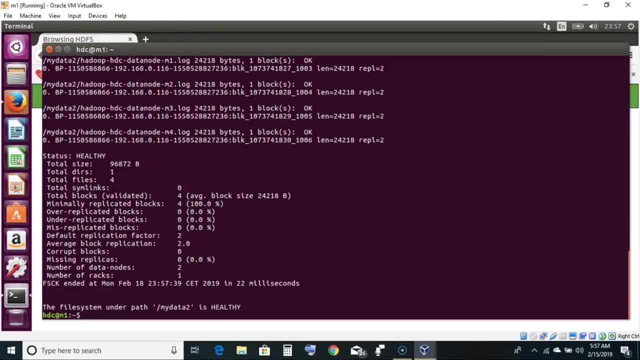 replicated twice. we don't have any over under miss replicated blocks and my file system status is healthy. so this is the HDFS command to make sure that your files are replicated correctly. so we have seen how your files are written with default replication. we have seen how your files follow a dynamic. 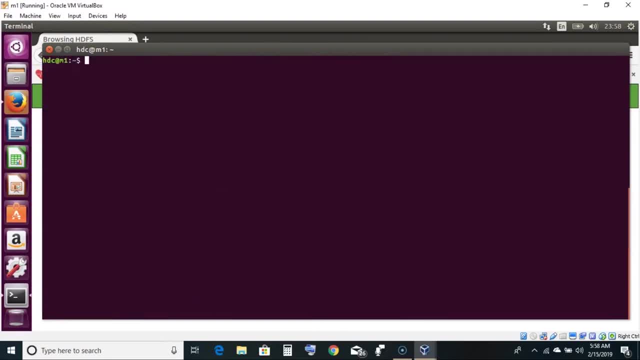 replication what you specify on the command line. now we can also see a command which allows us to change replication after the data has been written, so I can say: hdfs, fsck, slash files, slash blocks. and I can also see a command which allows us to change replication after the data has been written, so I can: 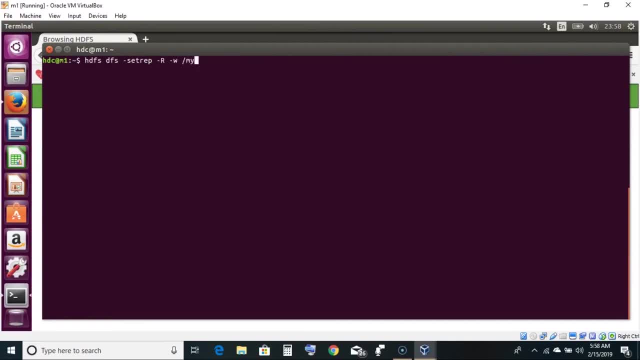 set rep and I can say path. that is my data 3, where I initially had all my file related blocks replicated only once. and now I will say my data 3 and I can specify that this should follow a replication of 2, which basically means that it will look into the directory. it will check all the files which had only 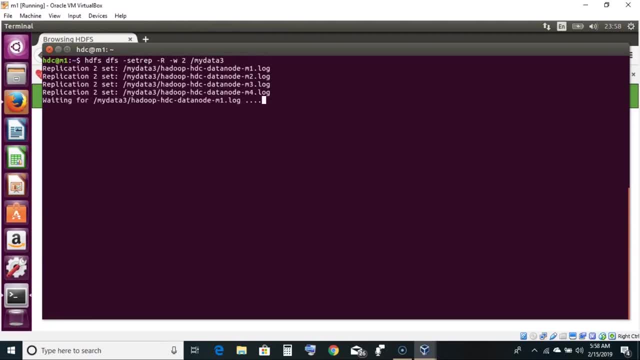 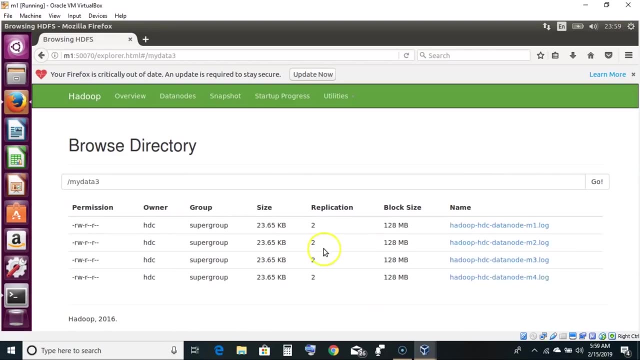 one block and now it will create a replica of those blocks across other data nodes. We can always go back and look into the data node logs to see the replication happening. we can also look from the browser interface, which initially was showing a replication of one and now it shows a replication of two. so this is the 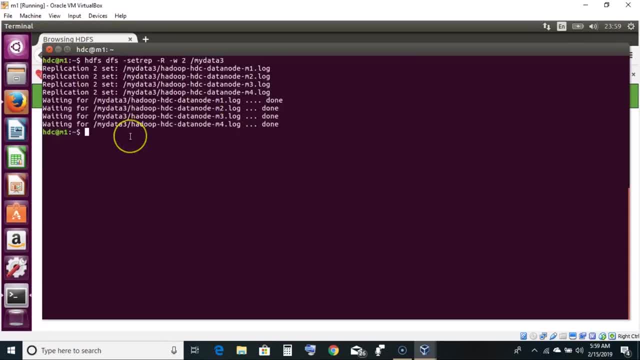 command to change the replication after the data has been written. so our writes can have default replication. we can write files with a different replication. we can change the replication after the data is written. not only that, we can even get the data from our hdfs to my local machine. 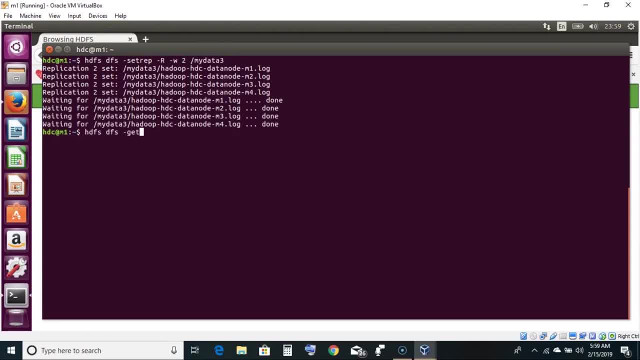 and for that i'll give hdfs get command or copy to local so i can say my data 3 and then i can bring it to my local machine in home hdc using a get command. so this is to get data from your sdfs to your local machine using a hdfs command. now, if you see i should have a. 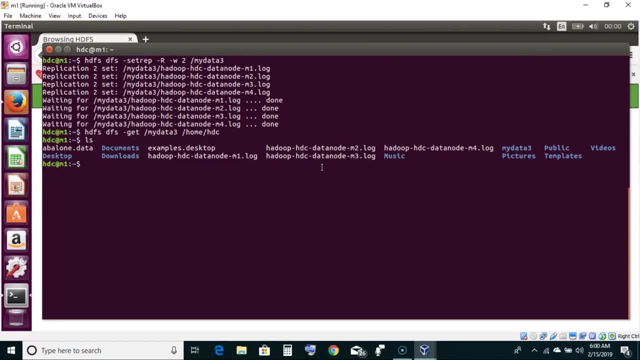 my data 3 directory, which is in my local path and we can look in my data 3, it has all the files which we had on hdfs. so we were not only putting data from our local machine to sdfs, we also successfully brought data from our hdfs to local machine. we have written data. 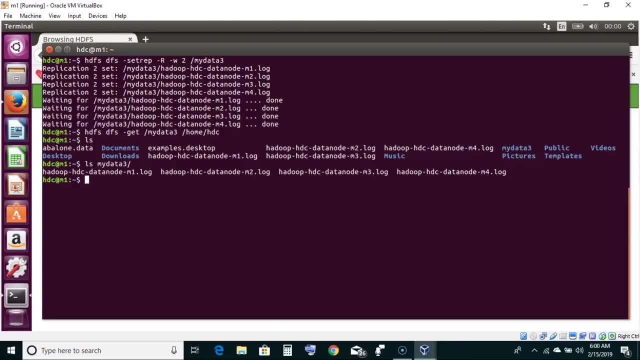 with different replication. we have checked the status of nodes, we have checked the status of blocks and if we would want to delete some data, sdfs also has options for that. so i can say hdfs, dfs, remove, and i could also do a recursive remove to remove everything, including the directory from my data 3, so this will delete. 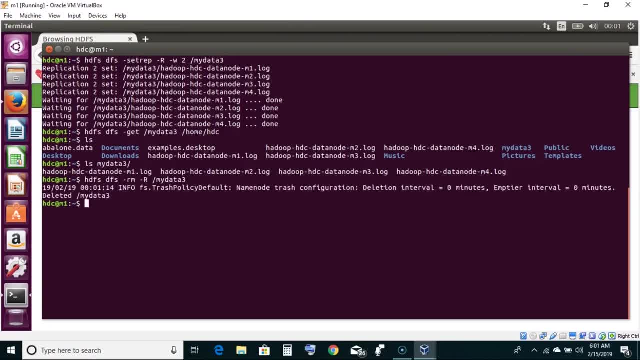 data from my hdfs. however, if thrash is enabled now, thrash basically means recycle bin, which depends on a property in the core hyphen site file. we have not enabled it. if thrash is enabled, then your data will be deleted from hdfs. however, it will not be permanently deleted, it will sit in. 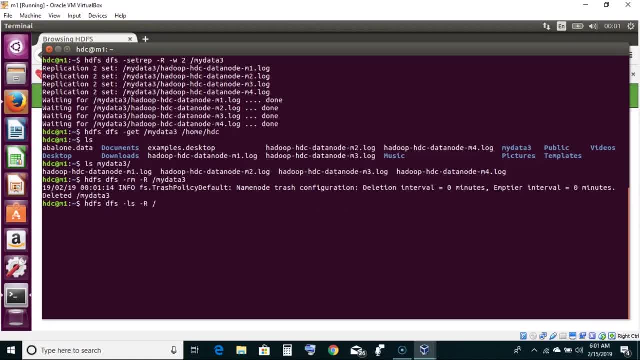 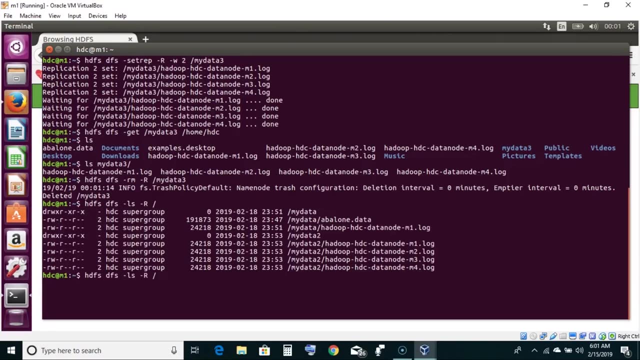 thrash for a time interval, what admin has specified in the configuration file. so right now i deleted thrash and this seems to be gone from sdfs because we have not set up any thrash. however, if a thrash is set up, then either you can decide to have your. 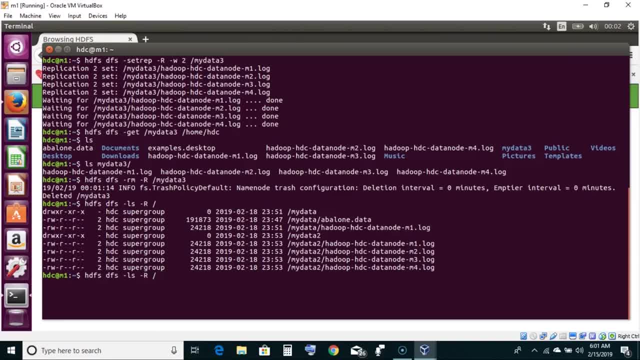 data deleted and still be in thrash so that it could be restored, or you could delete it permanently using a skip thrash option. however, remember this skip thrash option makes more sense if the thrash is enabled in your cluster and you do not want your deleted data to be sitting in thrash. 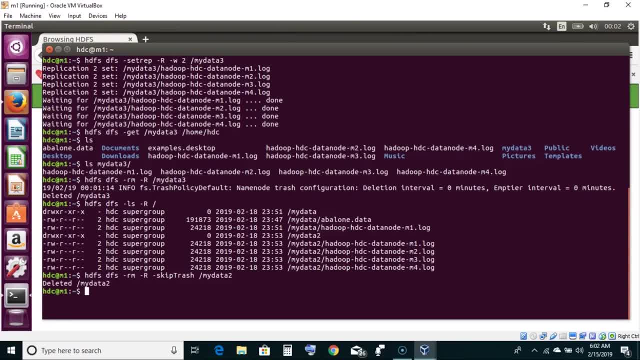 even for whatever time interval has been set, because even if the data sits in thrash and your thrash is a directory structure on hdfs, all the data will still be replicated. so we have seen how you can write data to the cluster, how you can get data from cluster to your local machine, how. 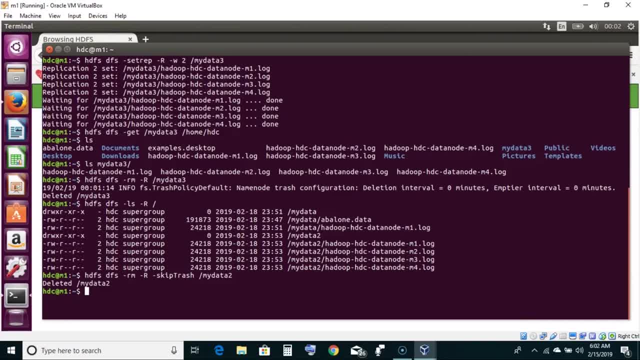 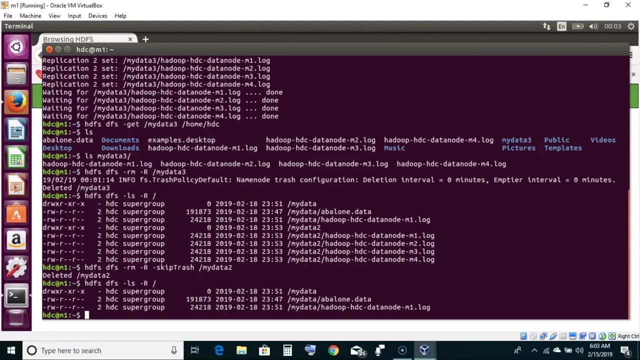 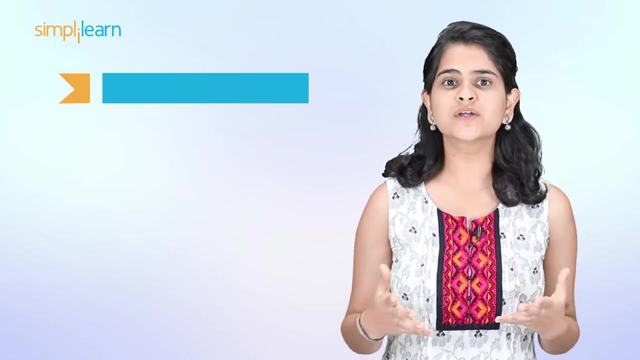 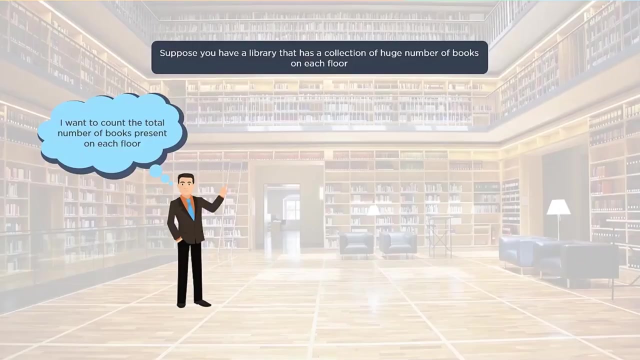 you can write it with different replications, how you can delete it from your cluster and do a simple number of books on each floor and you want to count the total number of books present on each floor. What would be your approach? You could say: I will. 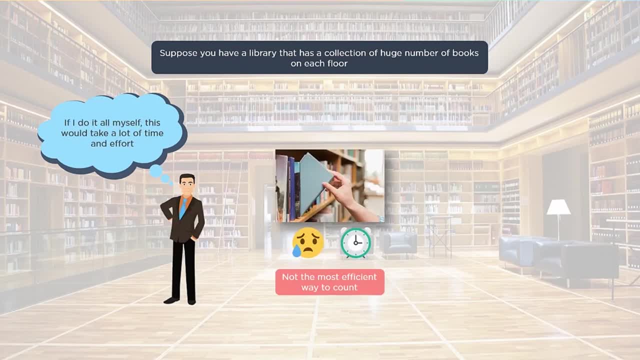 do it myself, but then don't you think that will take a lot of time and that's obviously not an efficient way of counting the number of books in this huge collection on every floor by yourself? Now, there could be a different approach or an alternative to that. You could think of asking. 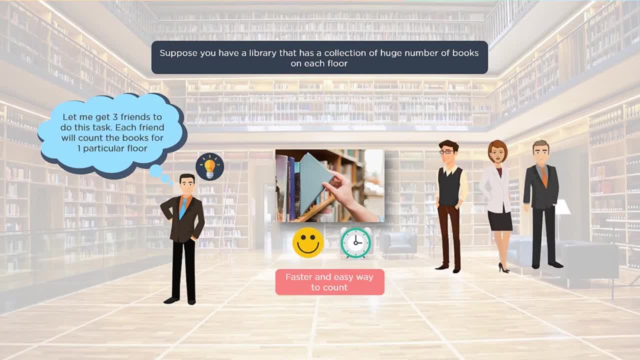 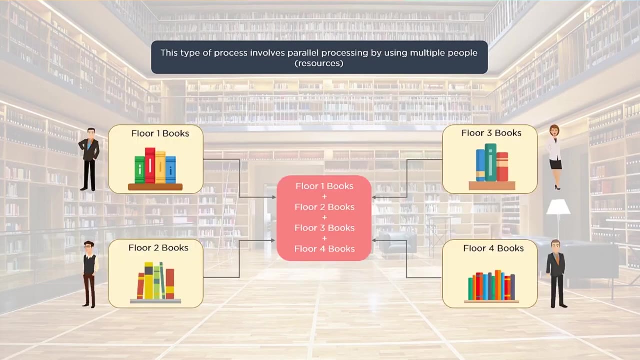 three of your friends or three of your colleagues, and you could then say: if each friend could count the books on every floor, then obviously that would make your work faster and easier. to count the books on every floor. Now this is what we mean by parallel processing. So when you say parallel, 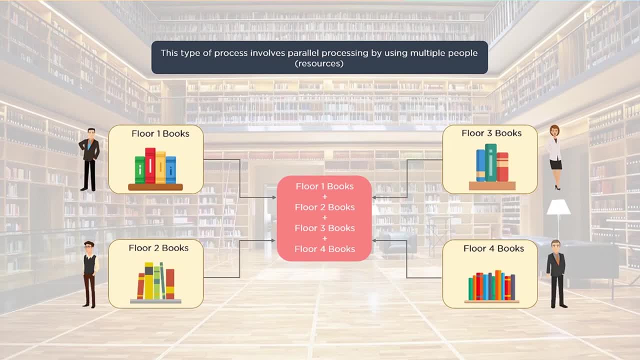 processing. in technical terms, you are talking about using multiple machines, and each machine would be contributing its RAM and CPU cores for processing, and your data would be processed on multiple machines at the same time. Now, this type of process involves parallel processing, in our case, or in our library example, where you would have person 1 who would be taking care of 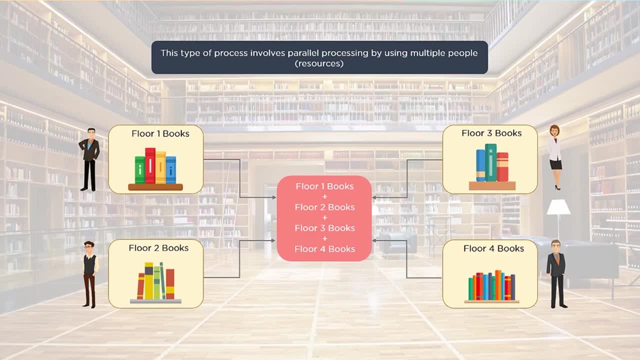 books on floor 1 and counting them Person 2 on floor 2, then you have someone on floor 3 and someone on floor 4.. So every individual would be counting the books on every floor in parallel, so that reduces the time consumed for this activity. and then there should be some mechanism where all 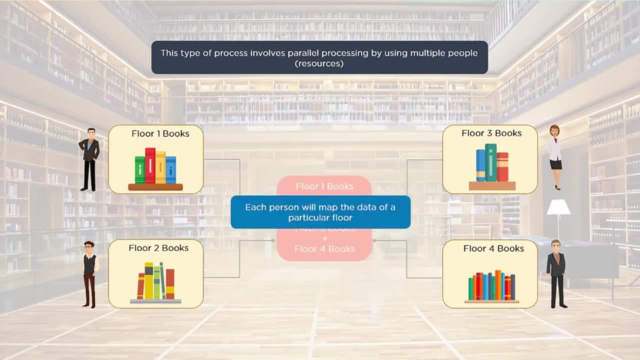 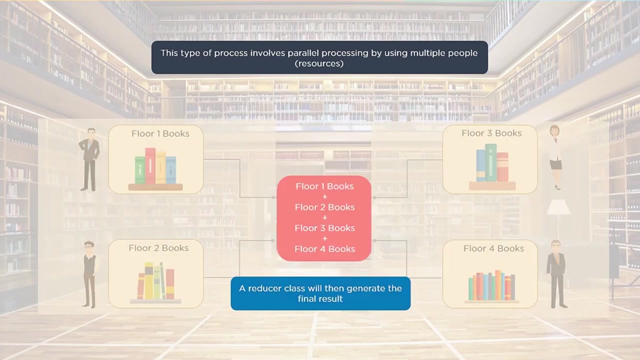 these counts from every floor can be applied, Aggregated. So what is each person doing here? Each person is mapping the data of a particular floor. or you can say each person is doing a kind of activity or basically a task on every floor, and the task is counting the books on every floor. Now then you could have some aggregation mechanism. 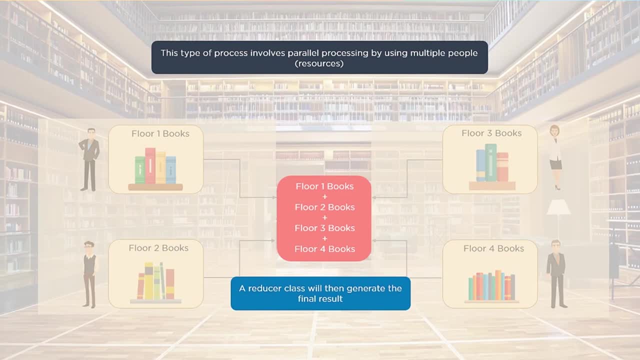 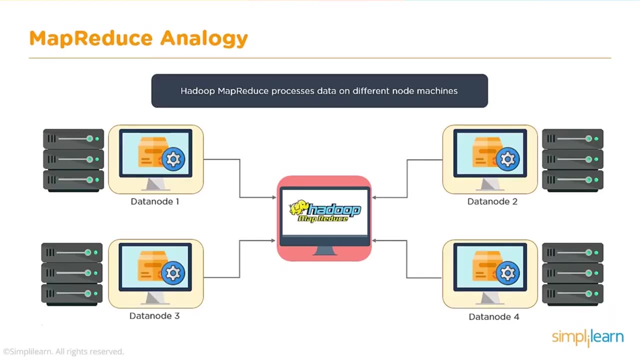 that could basically reduce or summarize this total count and in terms of map reduce, we would say that's the work of regression. So when you talk about Hadoop map reduce, it processes data on different node machines. Now, this is the whole concept of Hadoop framework. right that you not only have your data stored. 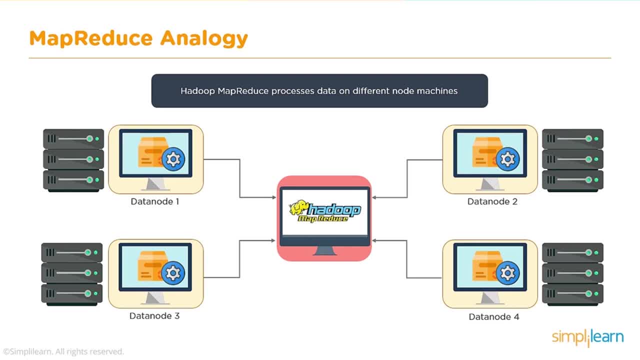 across machines, but you would also want to process the data locally. So instead of transferring the data from one machine to other machine, or bringing all the data together into some central processing unit and then processing it, you would rather have the data processed on the machines, wherever that. 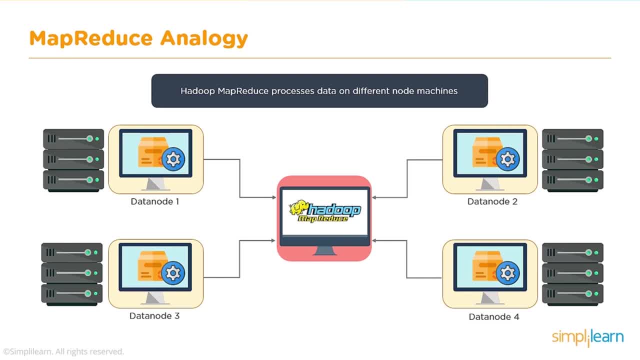 is stored. Now, in case of Hadoop cluster, we would have our data stored on multiple data nodes on their multiple disks, and that is the data which needs to be processed. but the requirement is that we want to process this data as fast as possible, and that could be achieved by using parallel processing. 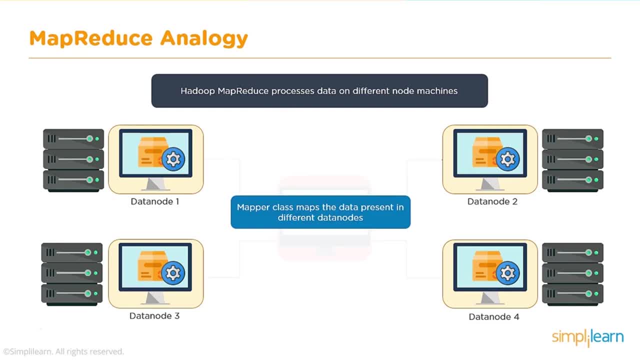 Now, in case of map reduce, we basically have the first phase, which is your mapping phase. So in case of MapReduce programming model, you basically have two phases: one is mapping and one is reducing. Now, who takes care of things in mapping phase? it is a mapper class. 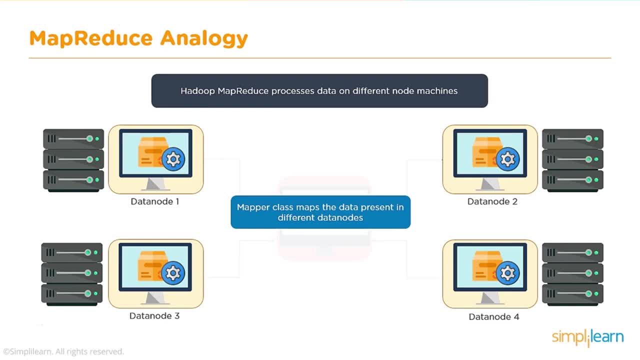 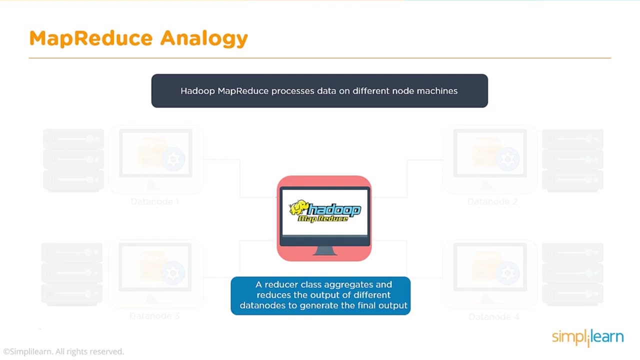 and this mapper class has the function, which is provided by the developer, which takes care of these individual map tasks, which will work on multiple nodes in parallel. Your reducer class belongs to the reducing phase, So a reducing phase basically uses a reducer class which provides a function that will aggregate and reduce the output of different data nodes. 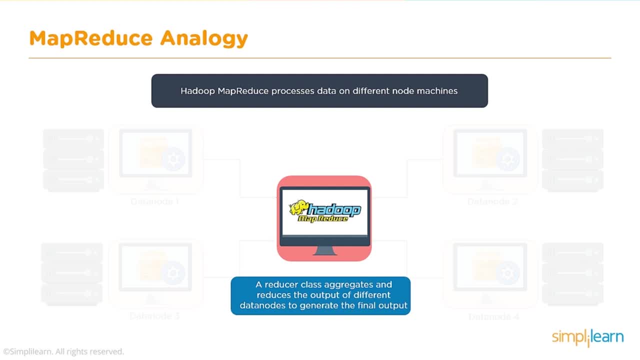 To generate the final output. now that's how your MapReduce works, using mapping and then, obviously, reducing. Now you could have some other kind of jobs which are map only jobs, wherein there is no reducing required. but we are not talking about those. we are talking about our requirement, where 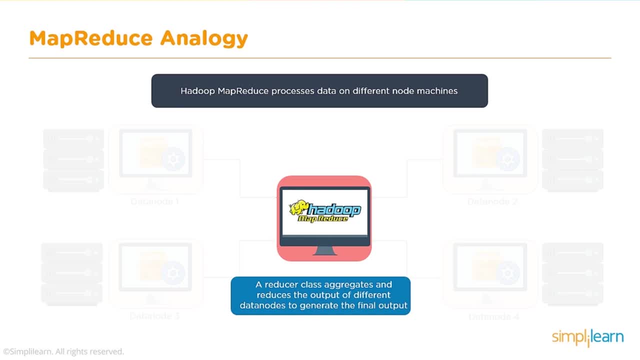 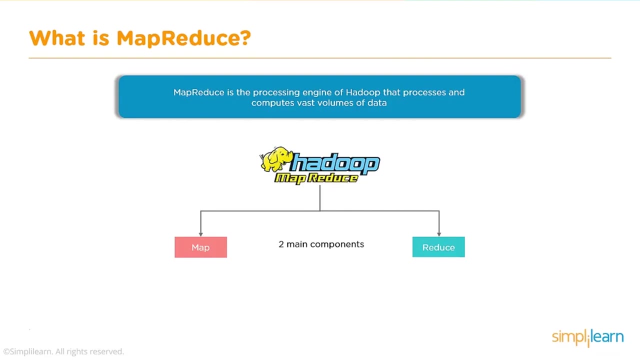 we would want to process the data using mapping and reducing, especially when data is huge, when data is stored across multiple machines and you would want to process the data in parallel. So when you talk about MapReduce, you could say it's a programming model. you could say internally it's a processing engine. 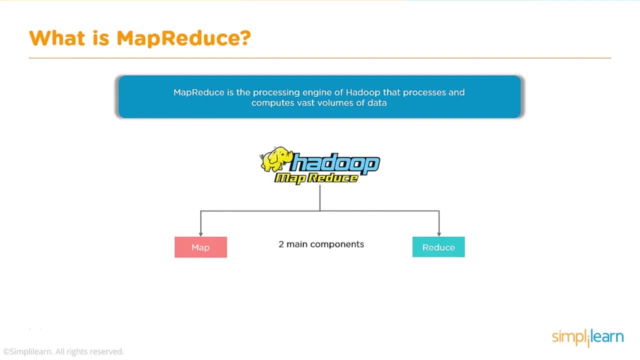 of Hadoop that allows you to process and compute huge volumes of data. and when we say huge volumes of data, we can talk about terabytes, we can talk about petabytes, exabytes and that amount of data which needs to be processed on a huge cluster. We could also use MapReduce programming model and run. 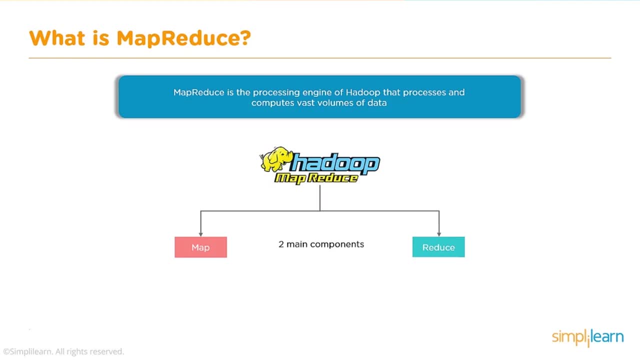 a MapReduce algorithm in a local mode. but what does that mean if you would go for a local mode? it basically means it would do all the mapping and reducing on the same node, using the processing capacity, that is, RAM and CPU cores on the same machine, which is not really efficient. in fact, we 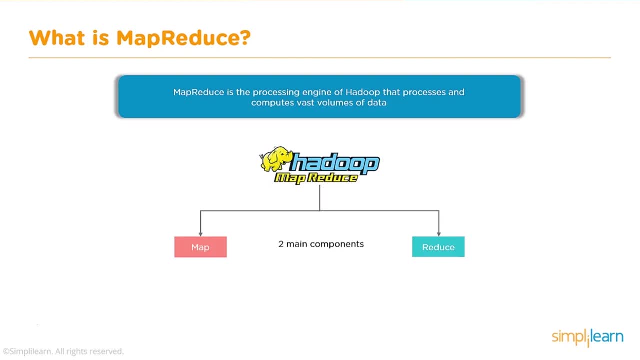 would want to have our MapReduce work on multiple nodes, which would obviously have mapping phase followed by a reducing phase and intermittently there would be data generated. there would be different other phases which help this whole processing. So when you talk about Hadoop MapReduce, you are mainly talking about Hadoop MapReduce. you are mainly 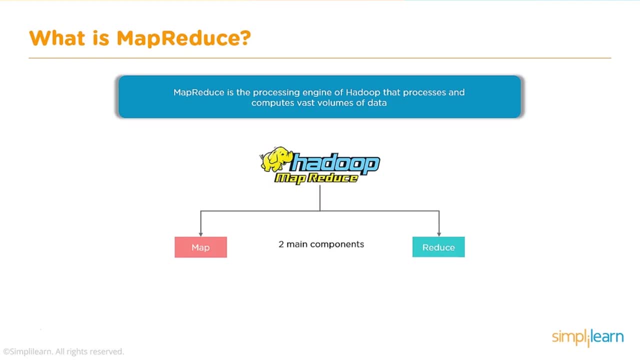 talking about two main components or two main phases, that is, mapping and reducing. mapping, taking care of map tasks. reducing, taking care of reduced tasks, so you would have your data which would be stored on multiple machines. now, when we talk about data, data could be in different formats. we could 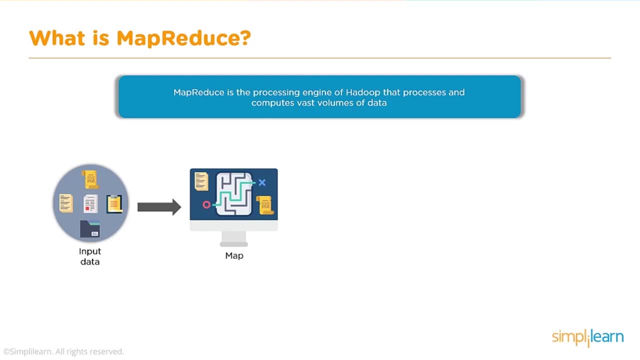 or the developer could specify what is the format which needs to be used to understand the data which is coming in. that data then goes through the mapping internally. there would be some shuffling, sorting and so on, and then reducing, which gives you your final output. so the way we access data from sdfs or the 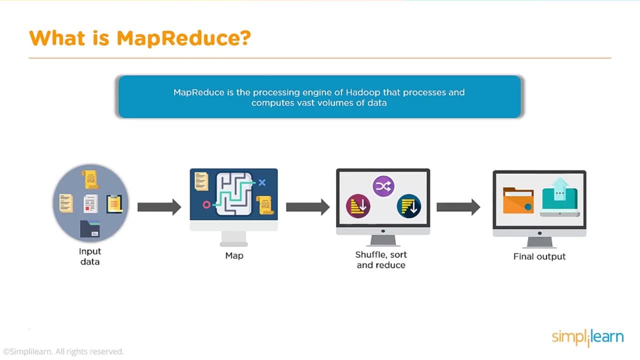 way our data is getting stored on sdfs. we have our input data, which would have one or multiple files and one or multiple directories, and your final output is also stored on sdfs to be accessed, to be looked into and to see if the processing was done correctly. so this is how it looks. 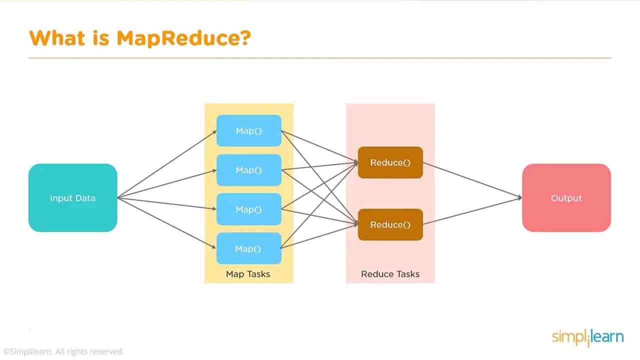 so you have the input data, which would then be worked upon by multiple map tasks. now, how many map tasks? that basically depends on the file. that depends on the input format. so normally we know that in a hadoop cluster you would have a file which is broken down into blocks, depending 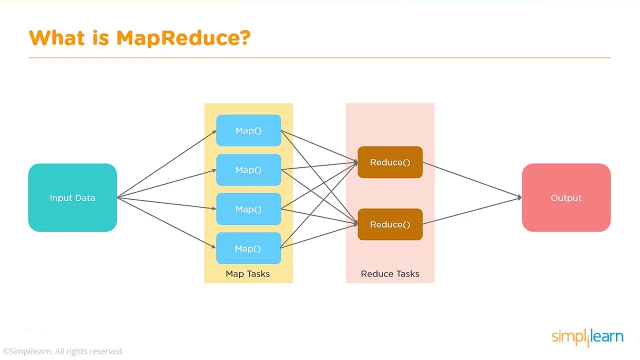 on its size. so the default block size is 128 mb, which can then still be customized based on your average size of data which is getting stored on the cluster. so if i have really huge files which are getting stored on the cluster, i would certainly set a higher block size so that my every 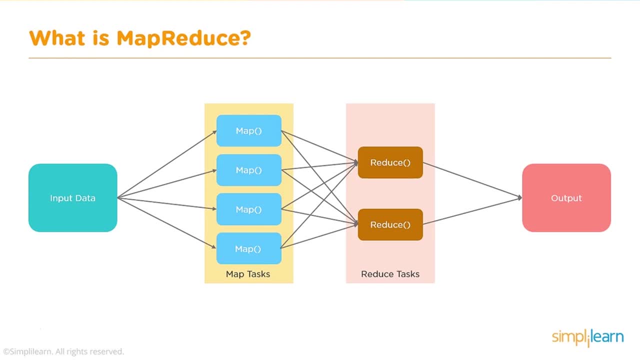 file would be split into multiple blocks, and so it would be a load on name nodes, ram, and so that's tracking the number of elements in your cluster or number of objects in your cluster. so, depending on your file size, your file would be split into multiple chunks, and for every chunk 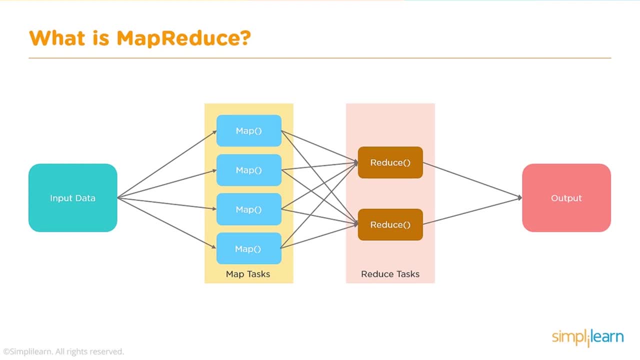 we would have a map task running. now what is this map task doing? that is specified within the mapper class. so within the mapper class you have the mapper function, which basically says what each of task has to do on each of the chunks which has to be processed. This data intermittently is written. 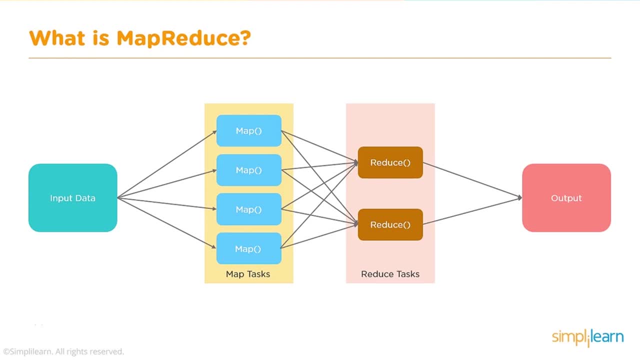 to SDFS, where it is sorted and shuffled, and then you have internal phases, such as partitioner, which decides how many reduced tasks would be used or what data goes to which reducer. You could also have a combiner phase, which is like a mini reducer doing the same reduce operation before it reaches. 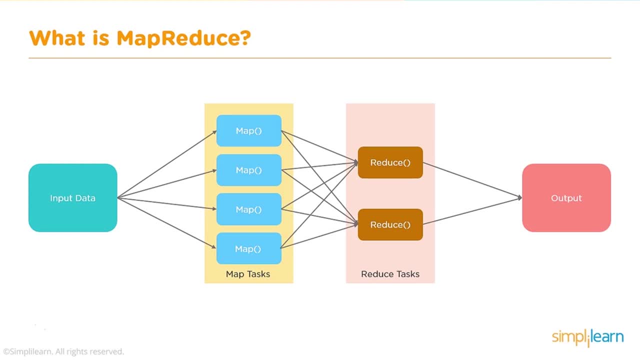 reduce. Then you have your reducing phase, which is taken care by a reducer class, and, internally, the reducer function provided by developer, which would have reduced task running on the data which comes as an output from map tasks. Finally, your output is then generated, which is stored on SDFS. 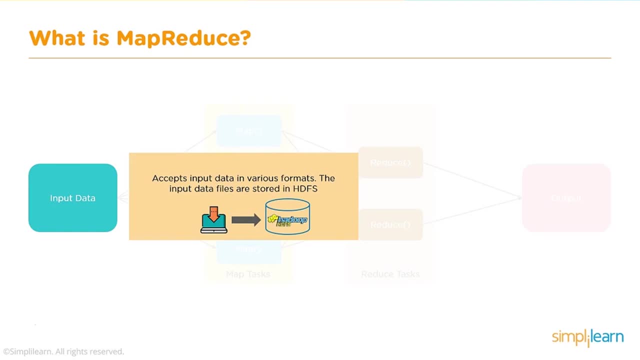 Now, in case of Hadoop, it accepts data in different formats. Your data could be in compressed format. your data could be in parquet. your data could be in abstract. your data could be in abstract format. your data could be in abstract format. your data. 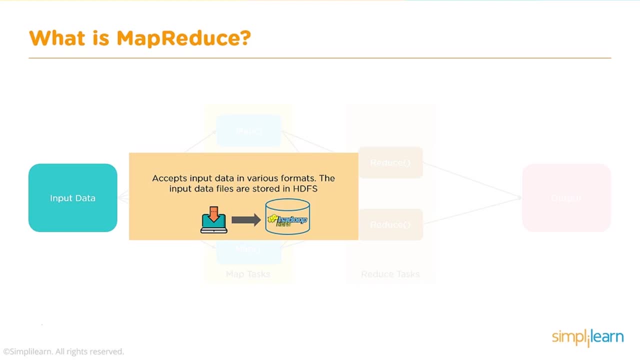 could be in macro text, CSV, TSV, binary format, and all of these formats are supported. However, remember, if you are talking about data being compressed, then you have to also look into what kind of split ability the compression mechanism supports. Otherwise, when MapReduce processing, 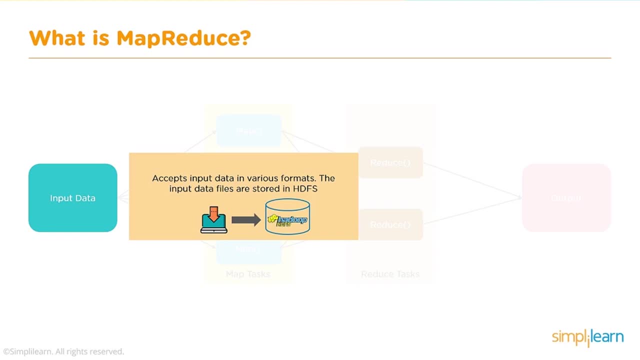 happens, it would take the complete file as one chunk to be processed. So SDFS accepts input data in different formats. This data is stored in SDFS and that is basically our input, which is then passing through the mapping phase. Now what is mapping phase doing? As I said, it reads record by 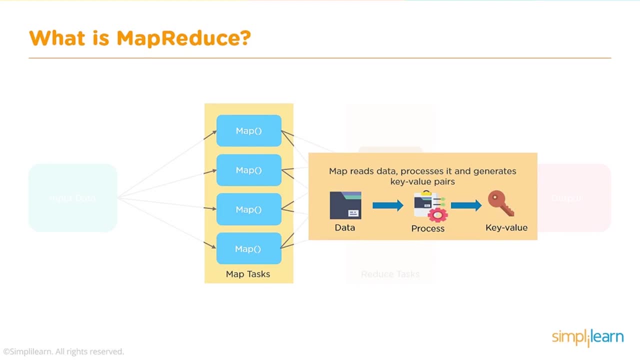 record. depending on the input format it reads the data. So we have multiple map tasks running on multiple chunks. Once this data is being read, this is broken down into individual elements, and when I say individual element, I could say this is my list of key value pairs. So your records based. 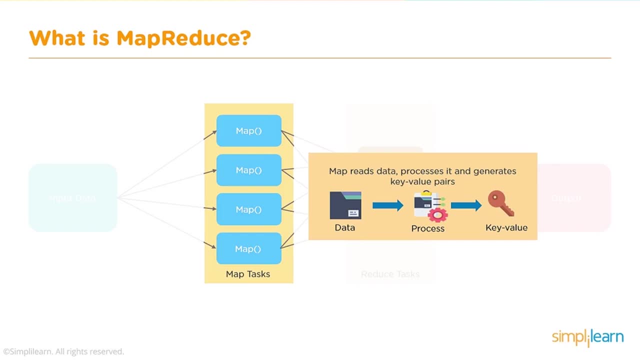 on some kind of delimiter or without delimiter, are broken down into individual elements. So you have a list of elements and thus your map creates key value pairs. Now, these key value pairs are not my final output. These key value pairs are basically a list of elements which will 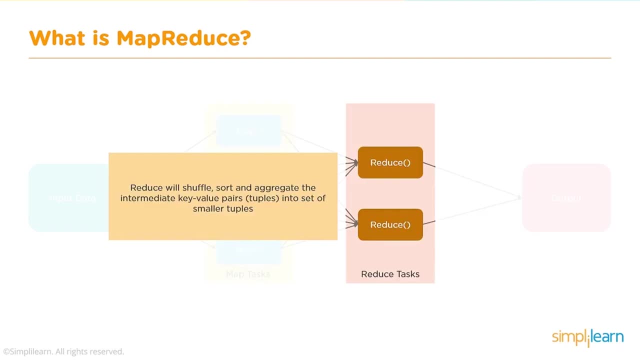 then be subjected to further processing. So you would have internally shuffling and sorting of data so that all the relevant key value pairs are brought together, which basically benefits the processing, and then you have your reducing, which aggregates the key value pairs into set of smaller. 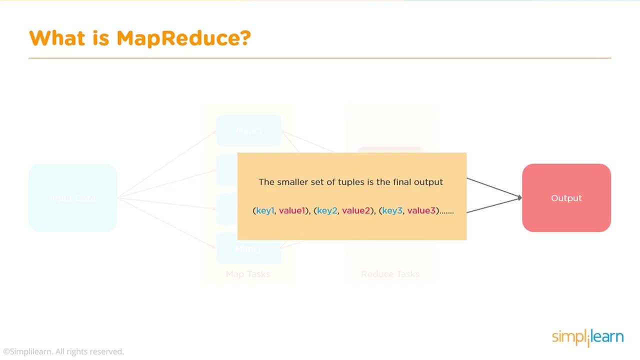 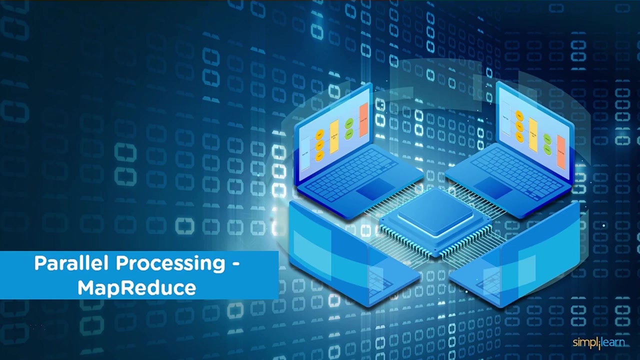 tuples, as you would say. Finally, your output is getting stored in the designated directory as a list of aggregated key value pairs, which gives you your output. So when we talk about MapReduce, one of the key factors here is the parallel processing which it can offer. So we know that. 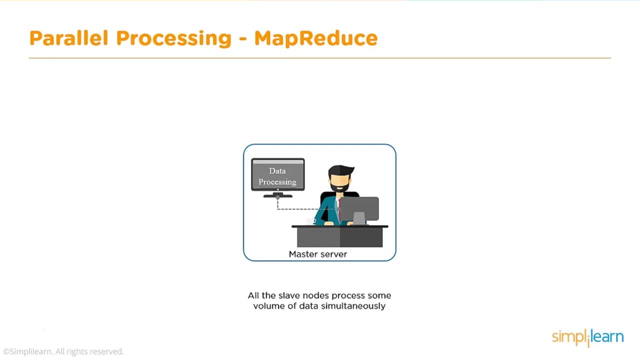 our data is getting stored across multiple data nodes and you would have huge volume of data which is split and randomly distributed across data nodes. So you would have huge volume of data which is split and randomly distributed across data nodes. So you would have huge volume of data which is 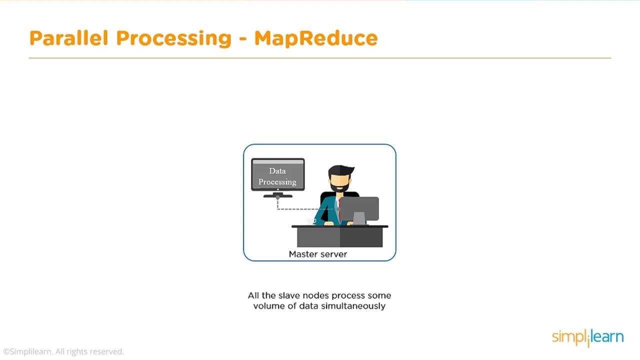 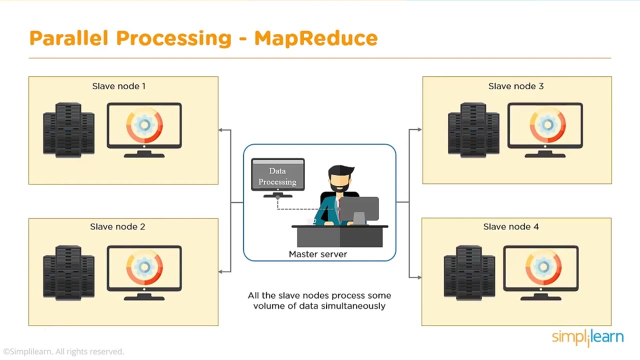 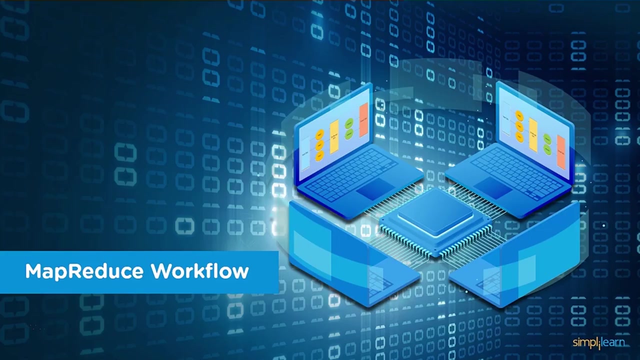 and this is the data which needs to be processed, and the best way would be parallel processing, So you could have your data getting stored on multiple data nodes or multiple slave nodes, and each slave node would have again one or multiple disks To process this data. basically, we have to. 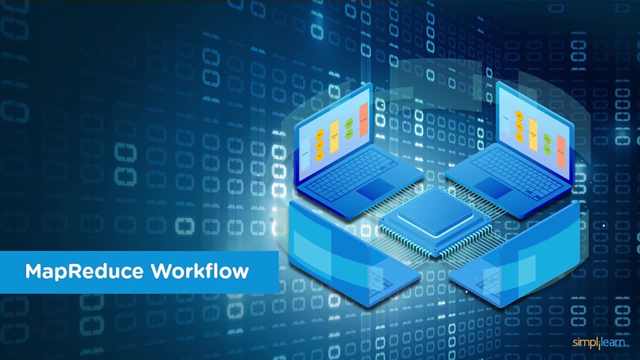 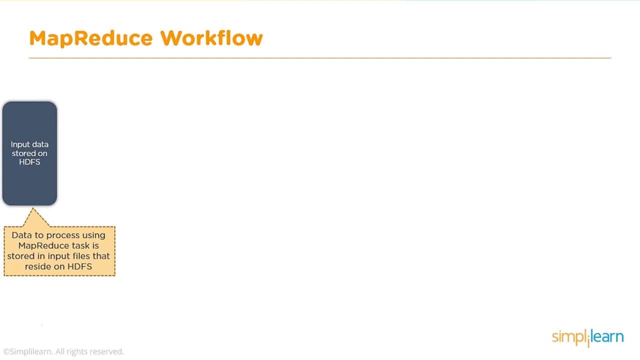 go for parallel processing approach, We have to use the MapReduce. Now let's look at the MapReduce workflow to understand how it works. So, basically, you have your input data stored on SDFS. Now you have the input data which needs to be processed. You can see the data which needs to be processed. 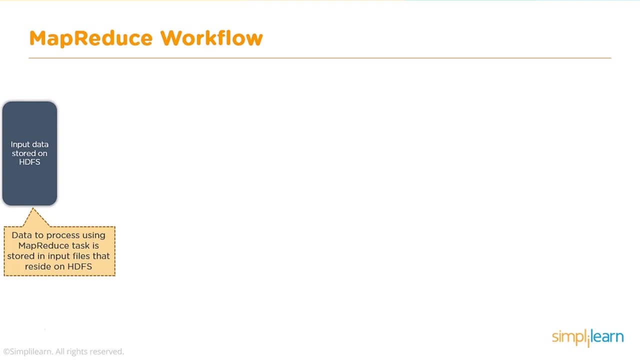 It is stored in input files and the processing which you want can be done on one single file, or it can be done on a directory which has multiple files. You could also later have multiple outputs merged, which we achieve by using something called chaining of mappers. So here you have, your data getting. 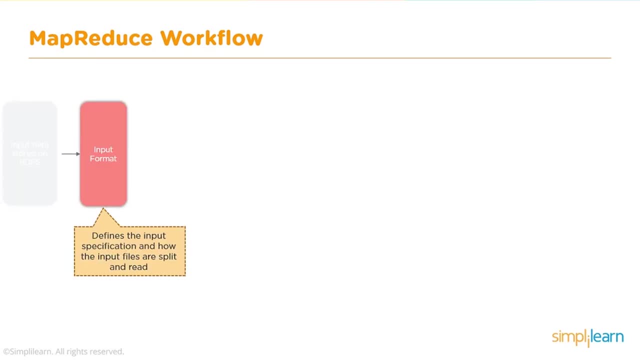 stored on SDFS. Now, input format is basically something to define the input specification and how the input files will be stored. So here we have the input data stored on SDFS. So what we're going to do is to go ahead and be split so there are various input formats. now we can search for that, so we can go to google. 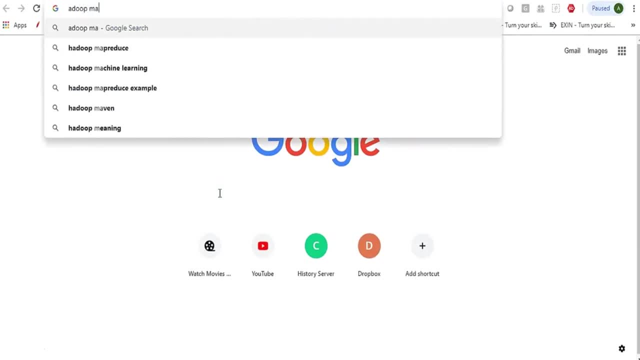 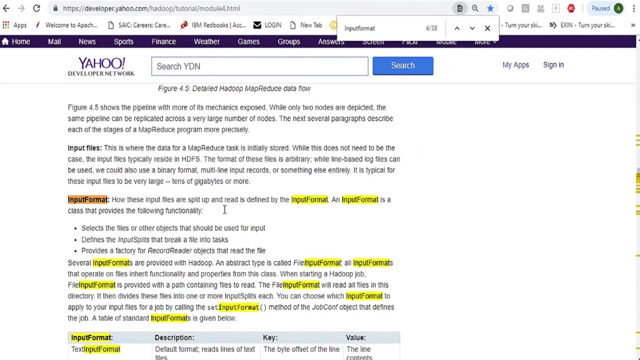 and we can basically search for hadoop map reduce yahoo tutorial. this is one of the good links and if i look into this link, i can search for different input formats and output formats. so let's search for input format. so when we talk about input format, you basically have something. 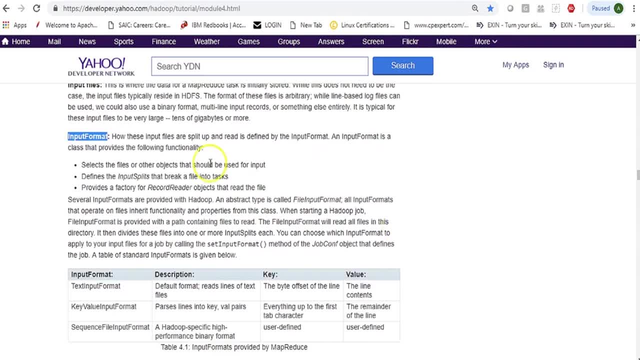 to define how input files are split. so input files are split up and read based on what input format is specified. so this is a class that provides following functionality: it selects the files or other objects that should be used for input. it defines the input split that break a file into. 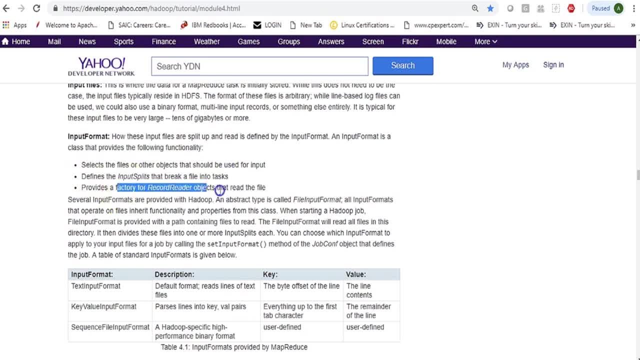 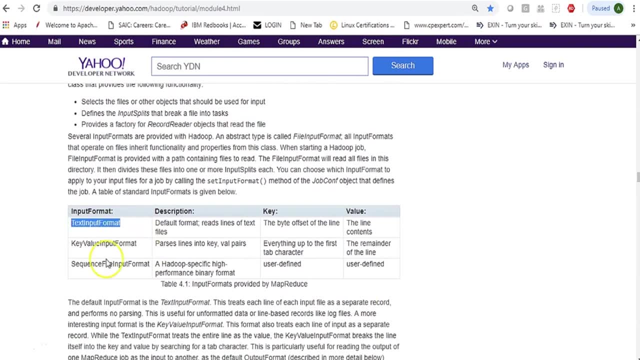 tasks provides a factory for record reader objects that read the file. so there are different formats. if you look in the table here and you can see that the text input format is the default format, which reads lines of a text file and each line is considered as a record. here the key is the byte offset of the line. 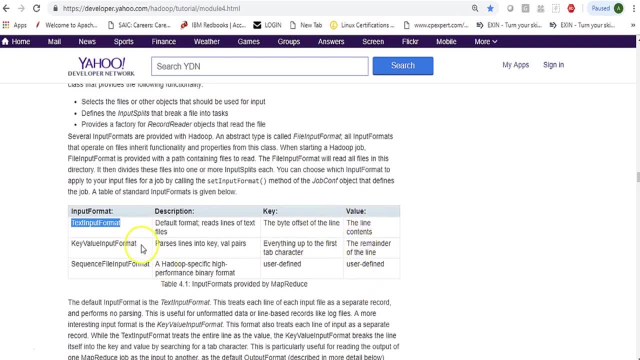 and the value is the line content itself. you can have key value input format which parses lines into key value pairs. everything up to the first tab character is the key and the remainder is the line. you could also have sequence file input format which basically works on binary. 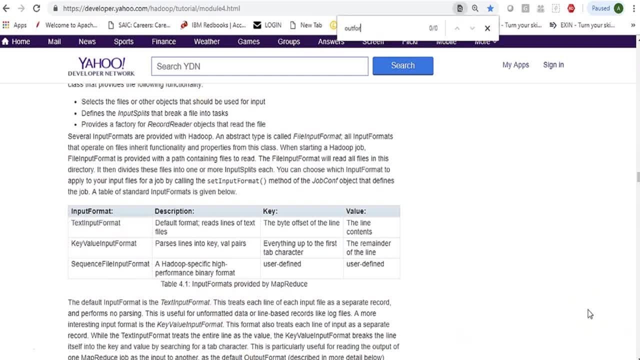 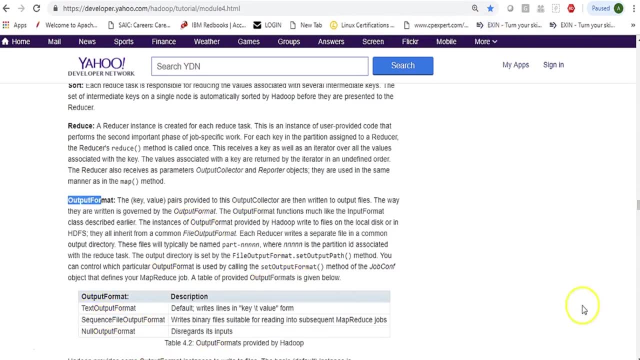 format. so you have input format, and in the same way you can also search for output format, which takes care of how the data is handled after the processing is done. so the key value pairs provided to this output collector are then written to output files the way they are written. 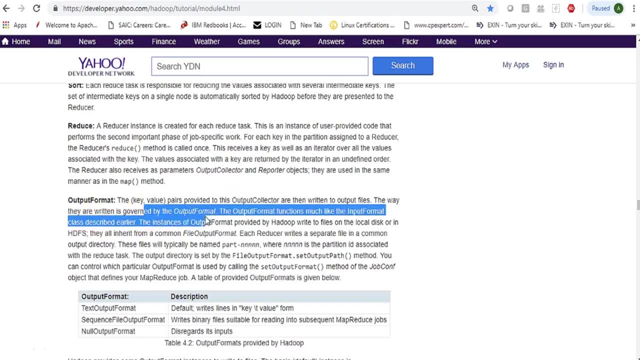 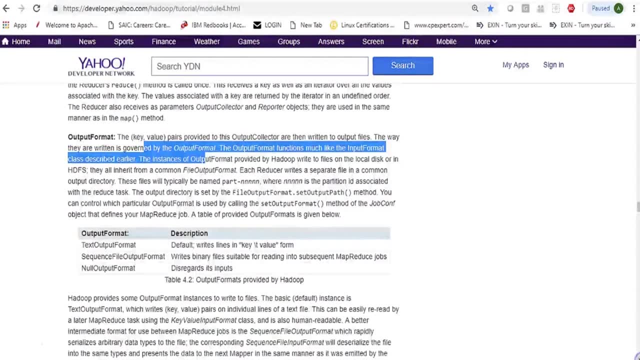 is governed by output format, so it functions pretty much like input format as described in earlier right, so we could set what is the output format to be followed. and again you have text output sequence, file output format, null output format and so on. so these are different classes. 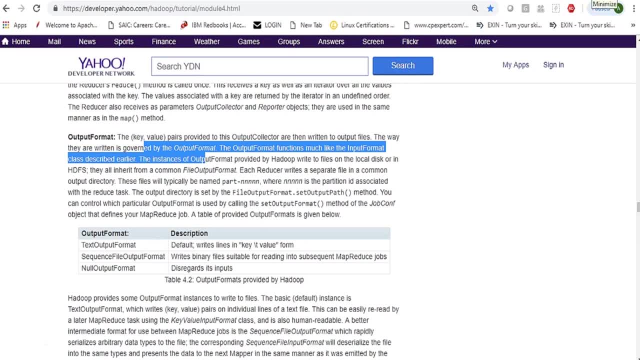 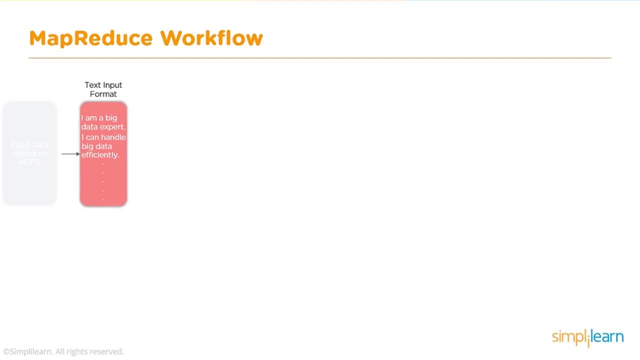 but it is also quite useful if you want to have a data processing module which takes care of how your data is handled when it is being read for processing, or how is the data being written when the processing is done. so, based on the input format, the file is broken down into splits, and this: 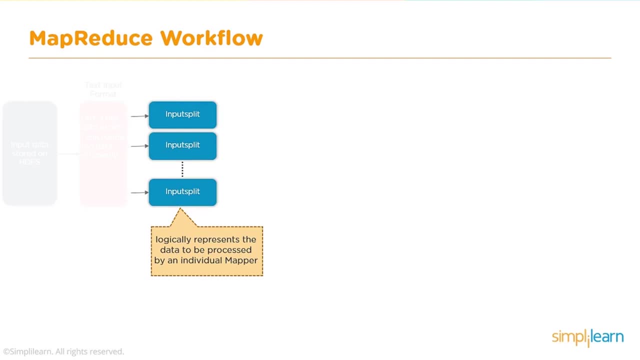 logically represents the data to be processed by individual map tasks, or you could say individual mapper functions, so you could have one or multiple splits which need to be processed, depending on the file size been set. now, once this is done, you have your input splits which are subjected to mapping phase. 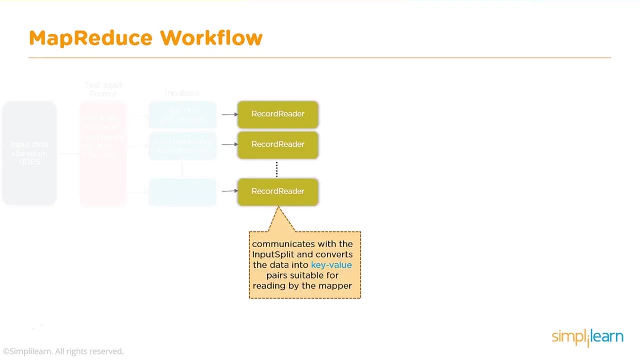 internally, you have a record reader which communicates with the input split and converts the data into key value pairs suitable to be read by mapper. and what is mapper doing? it is basically working on these key value pairs, the map task, giving you an intermittent output which would then be forwarded for further processing. now, once that is done and we have these key value pairs, 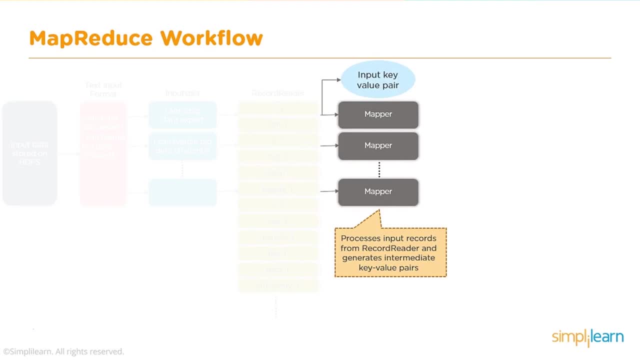 which is being worked upon, my map. your map tasks as a part of your mapper function are generating your key value pairs, which are your intermediate outputs to be processed further. now you could have, as i said, a combiner phase or, internally, a mini reducer phase. now combiner does not have its own. 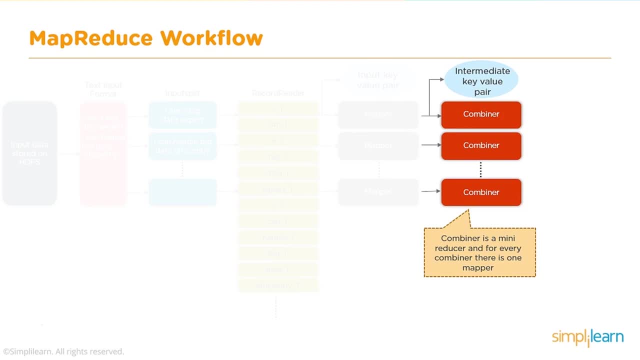 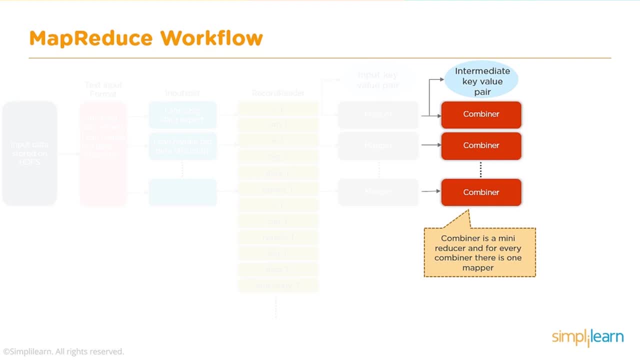 main work is to do some kind of mini aggregation on the key value pairs which were generated by map. so once the data is coming in from the combiner, then we have internally a partitioner phase which decides how outputs from combiners are sent to the reducers. or you could also say: 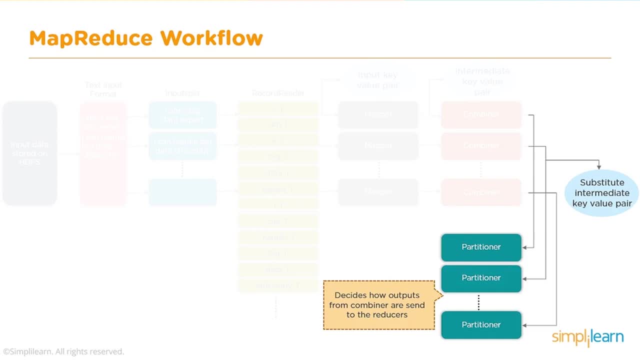 that, even if i did not have a combiner partitioner, would decide, based on the keys and values, based on the type of keys, how many reducers would be required or how many reduced tasks would be required to work on your output which was generated by map task, now, once partitioner. 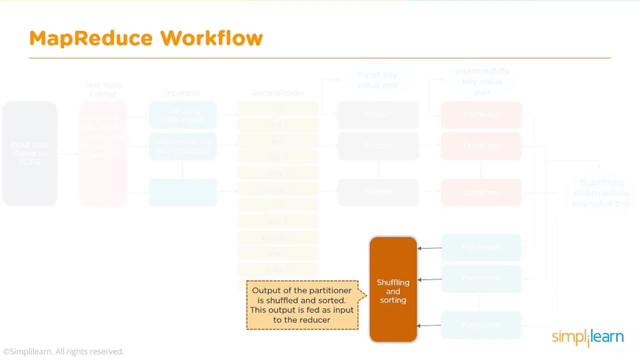 has decided that, then your data would be then sorted and shuffled, which is then fed into the reducer. so when you talk about your reducer, it would basically have one or multiple reduced tasks. now that depends on what or what partitioner decided to do so. now let's talk about the 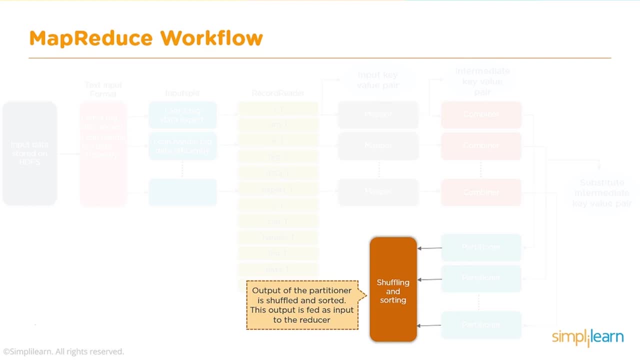 data that is being used to do the reducing or aggregation, and once you have this data, you can see that the data has been decided or determined for your data to be processed. it can also depend on the configuration properties which have been set to decide how many reduced tasks. 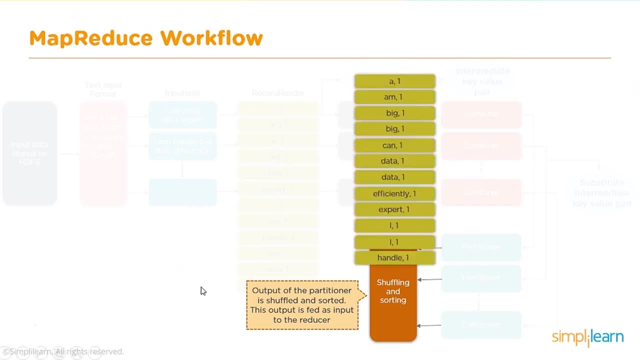 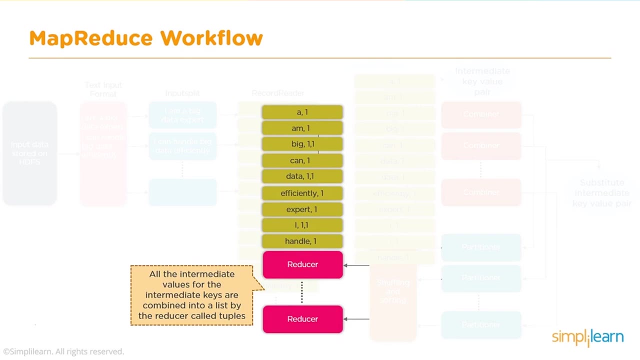 should be used now internally. all this data is obviously going through sorting and shuffling so that your reducing or aggregation becomes an easier task. once we have this done, we basically have the reducer, which is the code for the reducer is provided by the developer, and all the intermediate data has then to be aggregated. 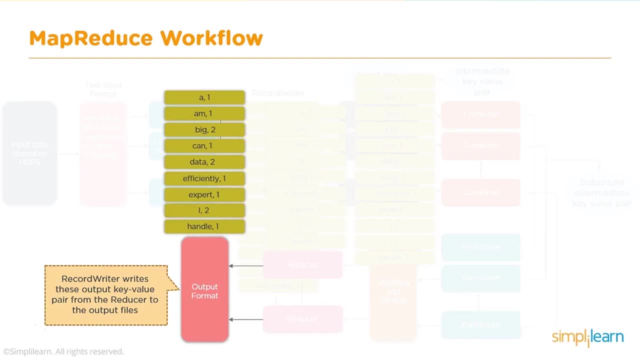 to give you a final output which would then be stored on sdfs. and who does this? you have an internal record writer which writes these output key value pairs from reducer to the output files. now, this is how your map reduce works, wherein the final output data can be not only stored, but then 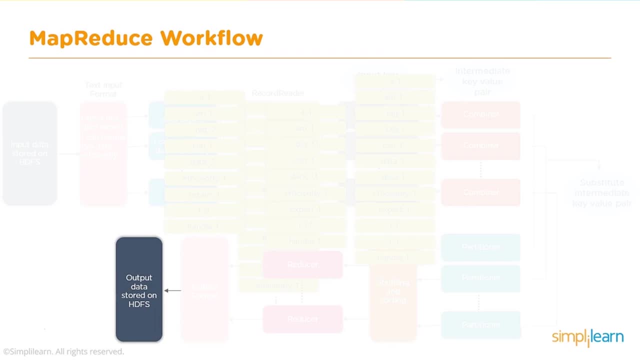 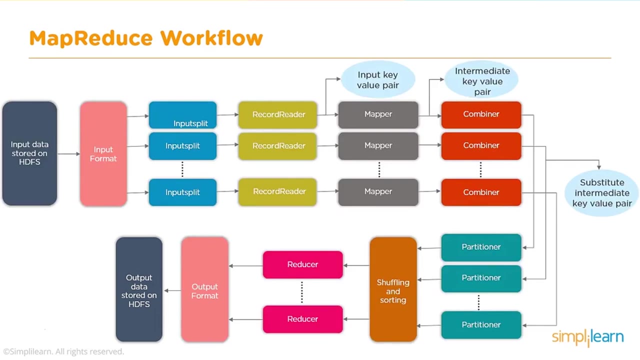 read or accessed from sdfs or even used as an input for further map reduce kind of processing. so this is how it overall looks. so you basically have your data stored on sdfs. based on input format, you have the splits, then you have record reader, which gives your data to the mapping phase, which is then taken care by your mapper function. 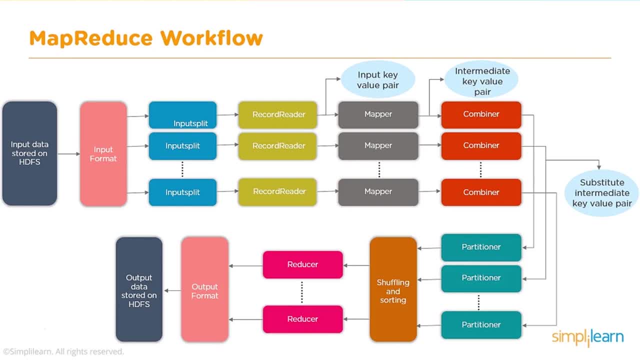 and mapper function basically means one or multiple map tasks working on your chunks of data. you could have a combiner phase, which is optional, which is not mandatory. then you have a partitioner phase, which decides on how many reduced tasks or how many reducers would be used to work on. 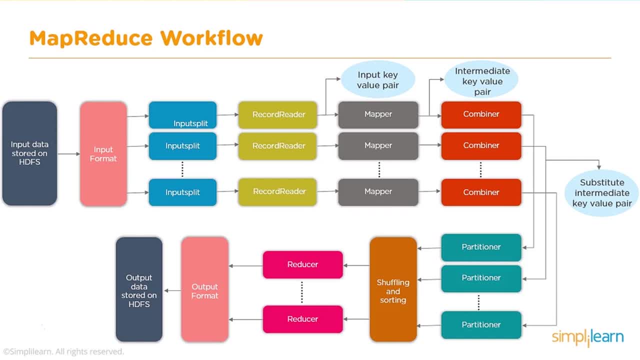 your data. internally, there is sorting and shuffling of data happening and then, basically, based on your output format, your record reader will write the output to sdfs directory. now, internally, you could also remember that data is being processed locally, so you would have the output of each task, which is 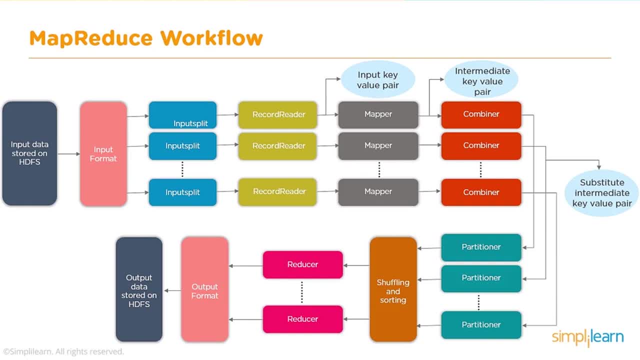 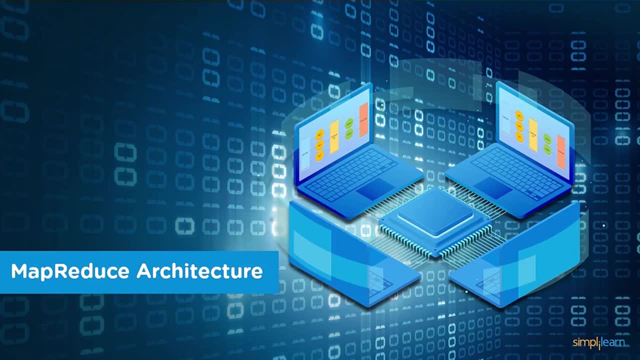 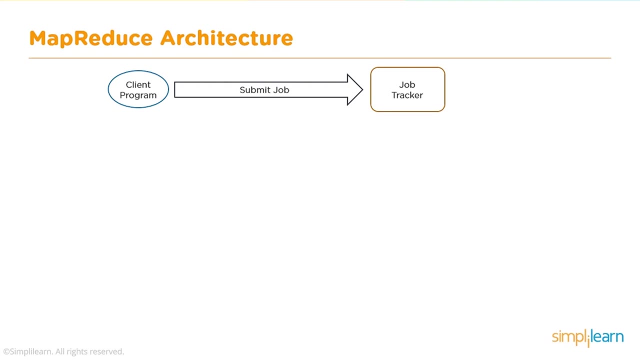 being worked upon stored locally. however, we do not access the data directly from data nodes. we access it from sdfs, so our output is stored on sdfs. so that is your mapreduce workflow. when you talk about mapreduce architecture. now, this is how it would look. so you would have basically a edge node. 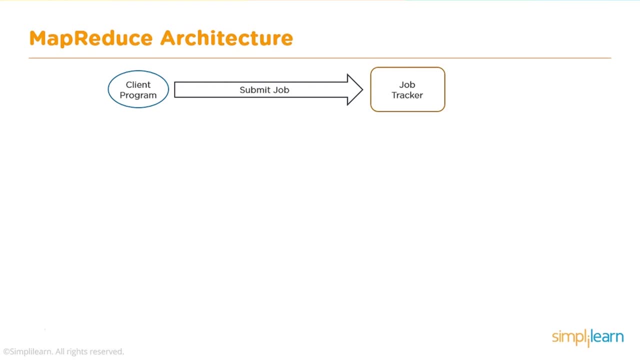 or a client program or an api which intends to process some data, so it submits the job to the job tracker, or you can say resource manager in case of hadoop yarn framework. right now, before this step, we can also say that an interaction with name node will happen in the same way. 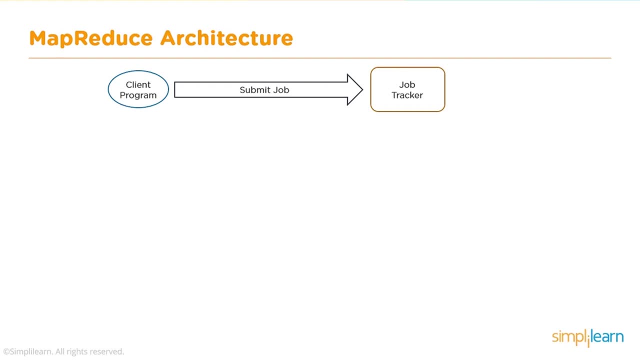 would have already happened, which would have given information of data nodes which have the relevant data stored, then your master processor. so in hadoop version 1 we had job tracker and then the slaves were called task trackers. in hadoop version 2, instead of job tracker you have. 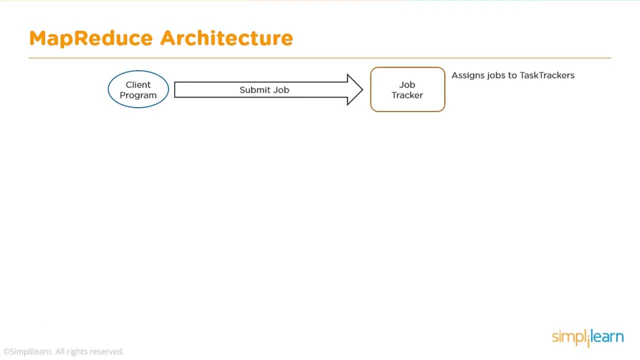 resource manager and instead of task trackers you have node managers. so basically your resource manager has to assign the job to the task trackers or node managers. so your node managers, as we discussed in yarn, are basically taking care of processing, which happens on every node. so internally there is all of this work happening by resource manager, node managers and application. 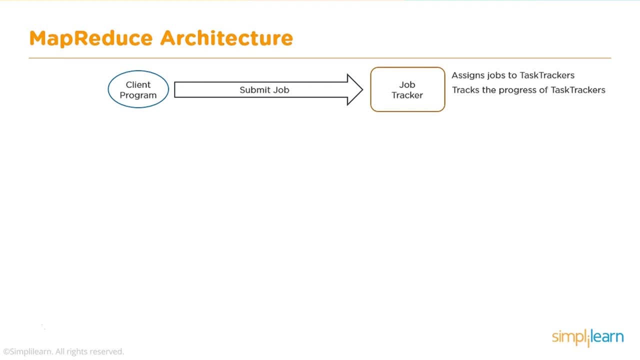 master and you can refer to the yarn based tutorial to understand more about that. so here your processing master is basically breaking down the application into tasks. what it does internally is, once your application is submitted, your application to be run on yarn processing framework is handled by resource manager. now forget about the yarn part as of now. i mean who? 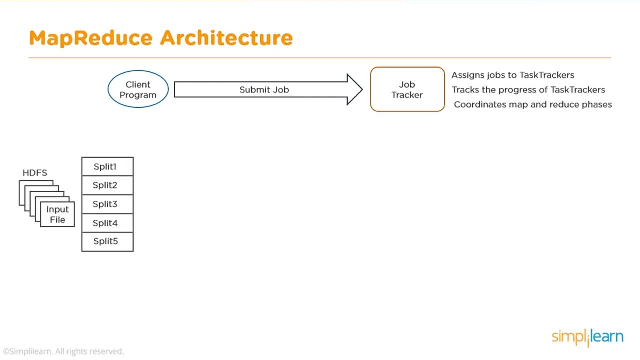 does the negotiating of resources? who allocates them? how does the processing happen? on the nodes right? so that's all to do with how yarn handles the processing request. so you have your data, which is stored in sdfs, broken down into one or multiple splits, depending on the input format. 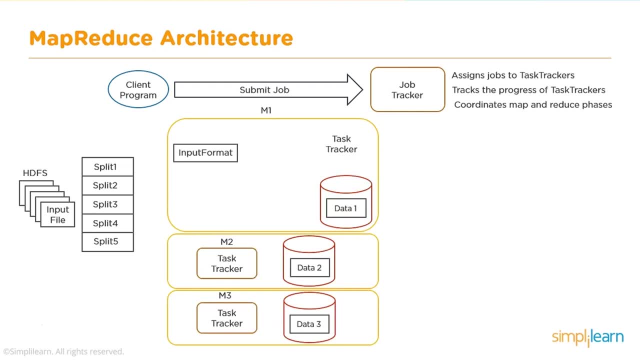 which has been specified by the developer. your input splits are to be worked upon by your resource manager, and the resource manager is responsible for the processing of the task. so you can see here that you have one or multiple map tasks which will be running within the container on the nodes. basically, you have the resources which are being utilized. so for each, 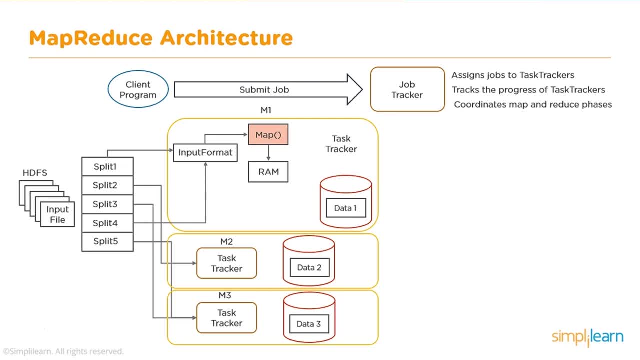 map task, you would have some amount of ram which will be utilized, and then further, the same data which has to go through reducing phase. that is, your reduced task will also be utilizing some ram and cpu cores. now, internally you have these functions which take care of deciding on number of 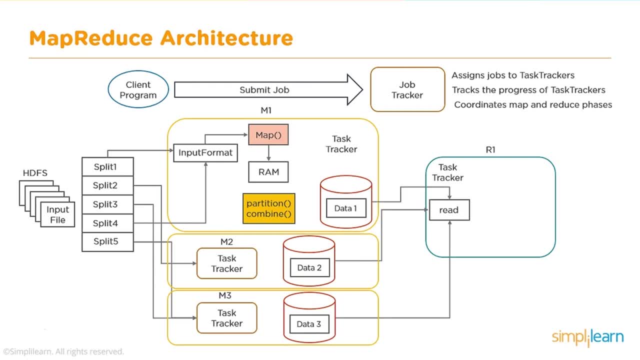 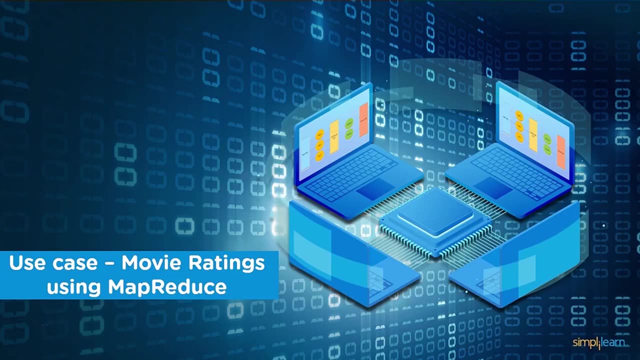 nodes. and then you have the process which is called the map reduce and basically reading and processing the data from multiple data nodes. now this is how your map reduce programming model makes parallel processing work, or processes your data, which is stored across multiple machines. finally, you have your output, which is getting stored on sdfs. 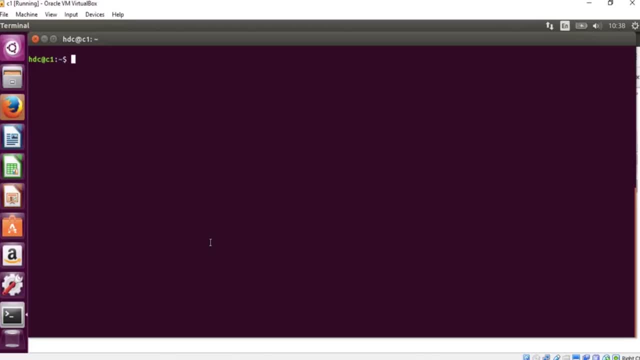 so let's have a quick demo on map reduce and see how it works on a hadoop cluster. now we have discussed briefly about map reduce, which contains mainly two phases, that is, your mapping phase and your reducing phase, and mapping phase is taken care by your mapper function and your reducing. 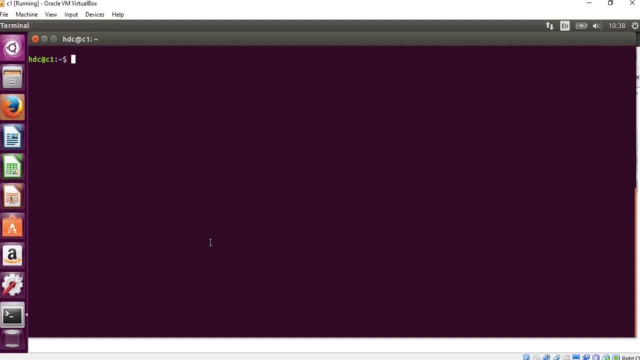 phase is taken care by your reducer function. now, in between we also have sorting and shuffling, and then you have other phases, which are called the mapping phase, and the reducing phase, which consists of other phases, which is partitioner and combiner, and we will discuss about all those. 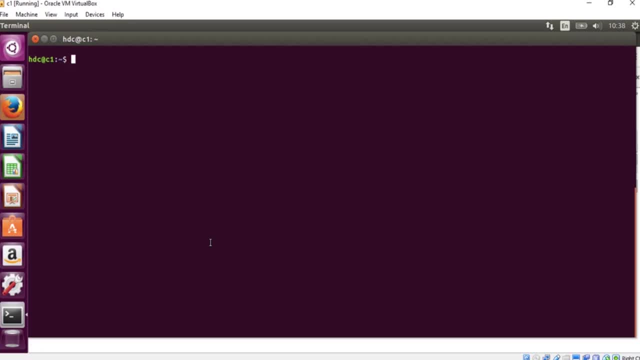 in detail in later sessions, but let's have a quick demo on how we can run a map reduce which is already existing as a package jar file within your apache hadoop cluster or even in your cloud data cluster. now we can build our own map reduce programs. we can package them as jar, transfer them. 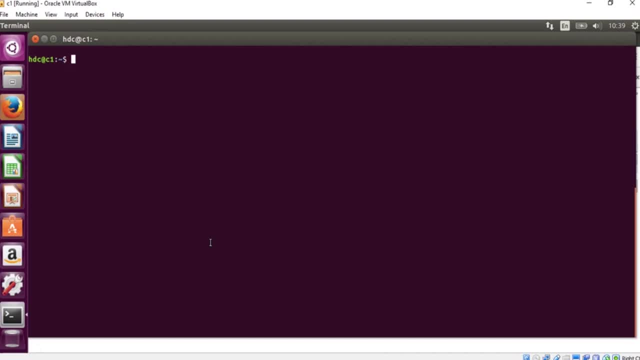 to the cluster and then run it on a hadoop cluster on yarn using already provided default program. so let's see where they are now. these are my two machines which i have brought up and basically this would have my apache hadoop cluster running. now we can. 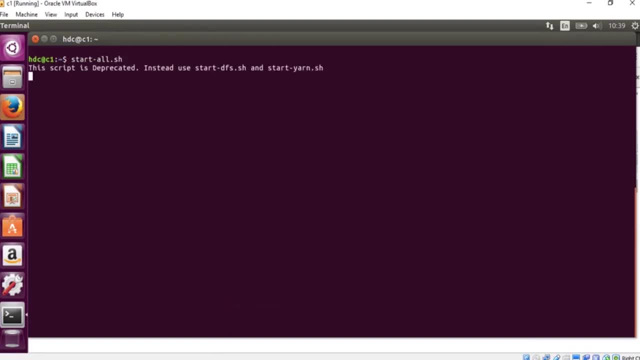 just do a simple start hyphen, all dot sh. now i know that this script is deprecated and it says instead use start dfs and start yarn, but then it will still take care of starting off my cluster on these two nodes where i would have one single name node, two data. 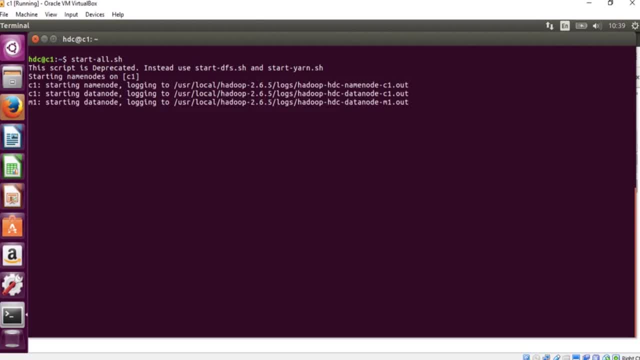 nodes, one secondary name node, one resource manager and two node managers. now, if you have any doubt in how this cluster came up, you can always look at the previous sessions where we had a walkthrough in setting up a cluster on apache, and then you could also have your cluster running using less. 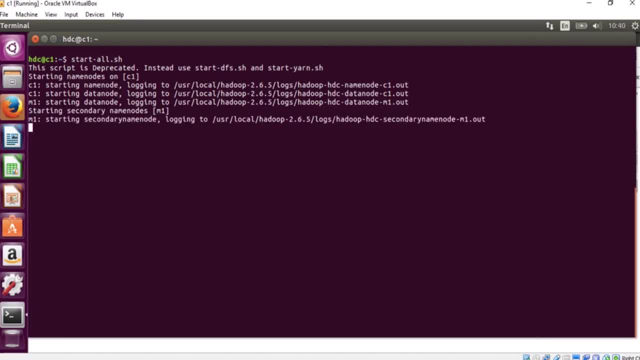 than 3 gb of your total machine ram and you could have apache cluster running on your machine. now, once this cluster comes up, we will also have a look at the web ui, which is available for name node and resource manager. now, based on the settings, what we have given, our uis will show us details of. 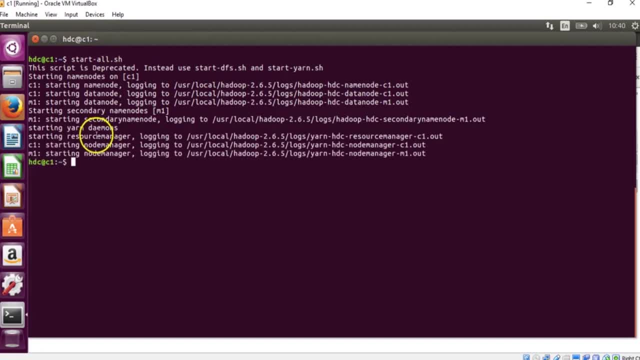 our cluster. but remember, the ui is only to browse. now, here my cluster has come up. i can just do a jps to look at java related processes and that will show me what are the processes which are running on c1, which is your data node, resource manager, node manager and name node, and on my 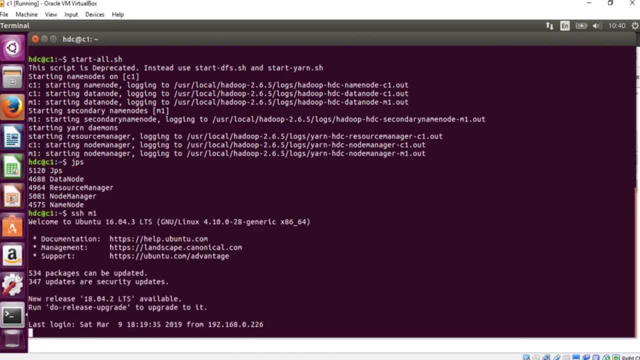 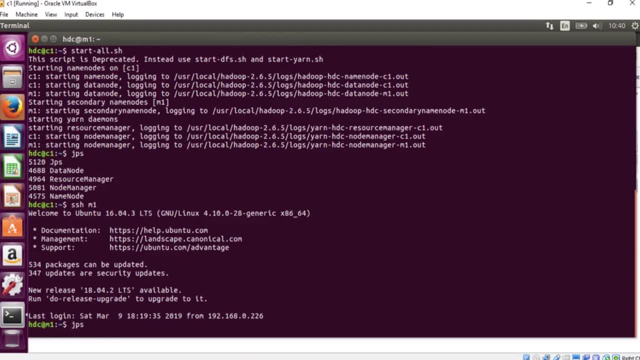 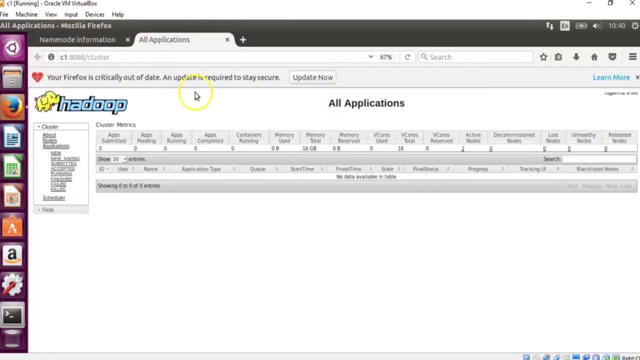 m1 machine, which is my second machine which i have configured. here i can always do a jps and that shows me the processes running. which also means that my cluster is up with two data nodes, with two node managers, and here i can have a look at my web ui so i can just do a refresh and 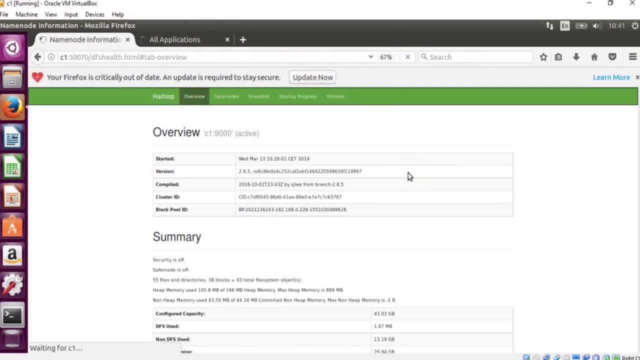 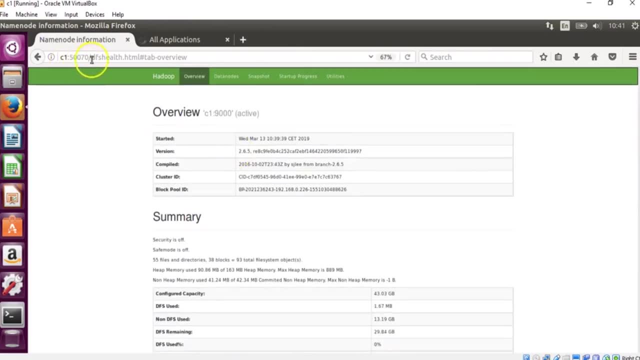 the same thing with this one, just do a refresh. so i had already opened the web pages. so you can always access the web ui using your name, nodes, hostname and 570 port. it tells me what is my cluster id, what is my blockpad, so i can always access the hostname and 570 port. it tells me what is my cluster id, what is my blockpad. 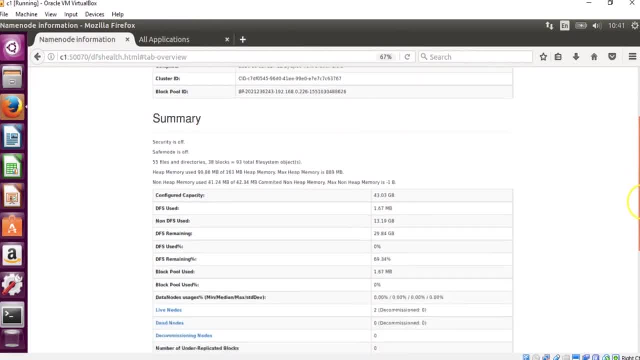 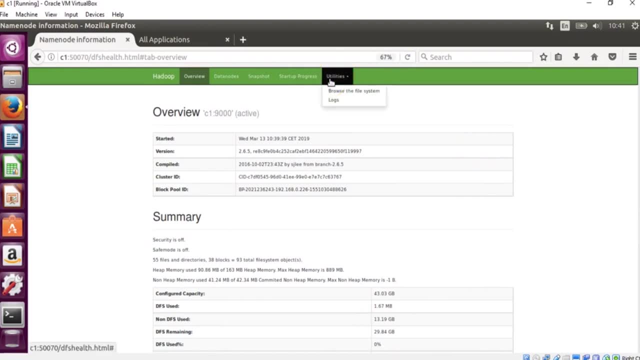 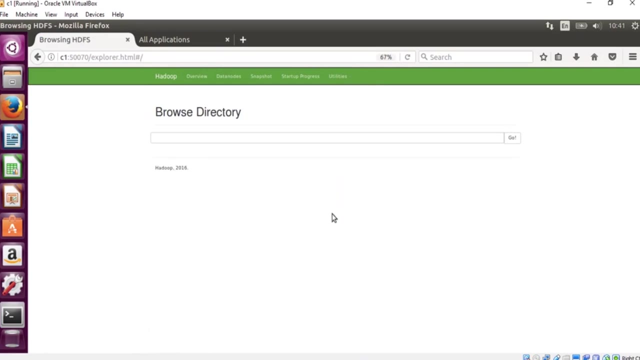 pull id. it gives you information of what is the space usage, how many live notes you have, and you can even browse your file system. so i have put in a lot of data here. i can click on browse the file system and this basically shows me multiple directories and these directories have one or 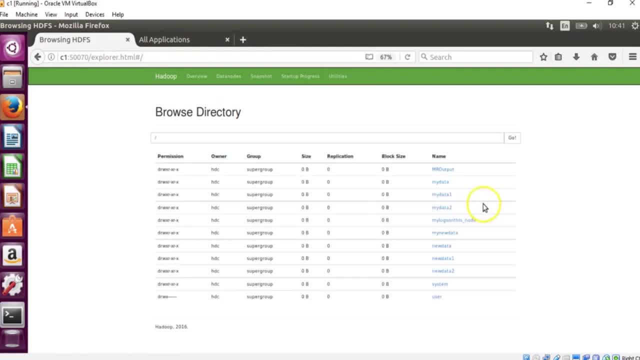 multiple files which we will use for our map reduce example. now, if you see, here these are my directories which have some sample files, although these files are very small, like 8.7 kilobytes, if you look into this directory, if you look into this. i have just pulled in some of my hadoop logs. 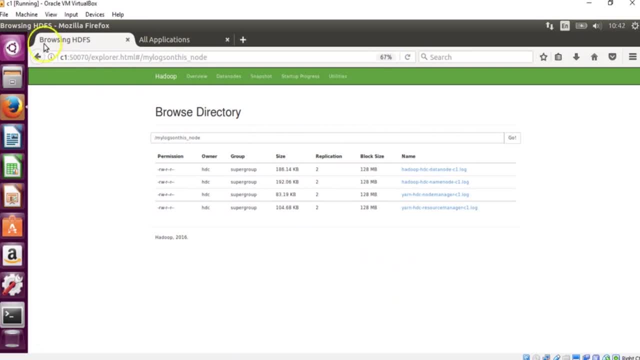 and i have put it on my sdfs. these are a little bigger files, and then we also have some other data which we can see here, and this is data which i have downloaded from web. now we can either run a map, reduce on a single file or in a directory which contains multiple files. let's look at that. 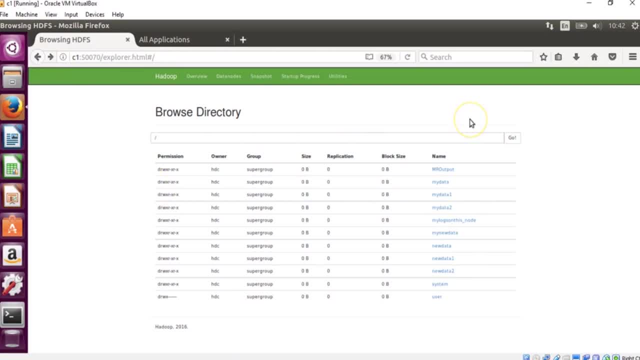 before looking at demo and map reduce, also remember map reduce will create a output directory and we need to have that directory created. plus, we need to have the permissions to run the map reduce job. so by default, since i'm running it using admin id, i should not have any problem. but then, if you, 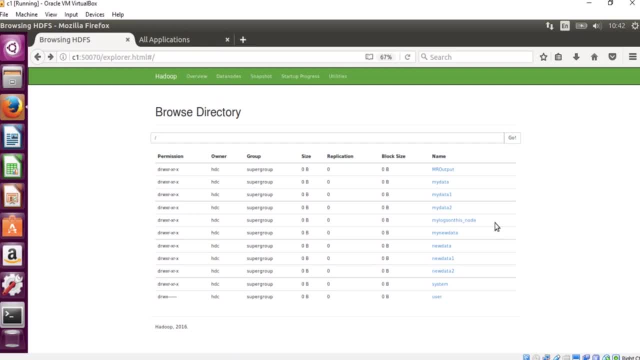 intend to run map reduce with a different user, then obviously you will have to ask the admin or you will have to give the user permission to read and write from sdfs. so this is the directory which i have created, which will contain my output once the map reduce job finishes and 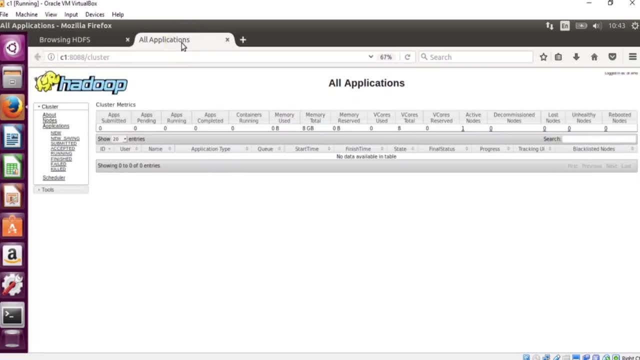 this is my cluster file system. if you look on this ui, this shows me about my yarn, which is available for taking care of any. processing it as of now shows that i have total of 8 gb memory and i have 8 v cores. now that can be depending on what configuration we have set or how many nodes. 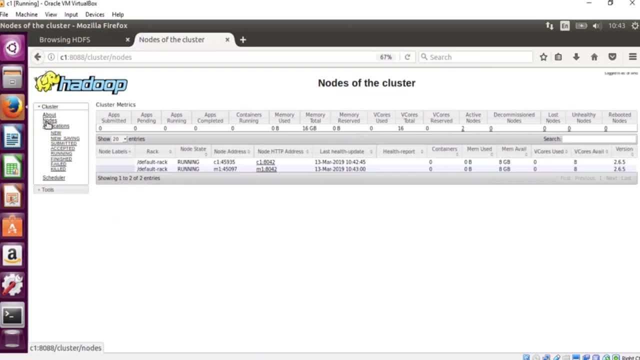 are available. we can look at nodes which are available and that shows me. i have two node managers running, each has 8 gb memory, and i have two node managers running, each has 8 gb memory and 8 v cores. now, that's not true, actually, but then we have not set the configurations for node. 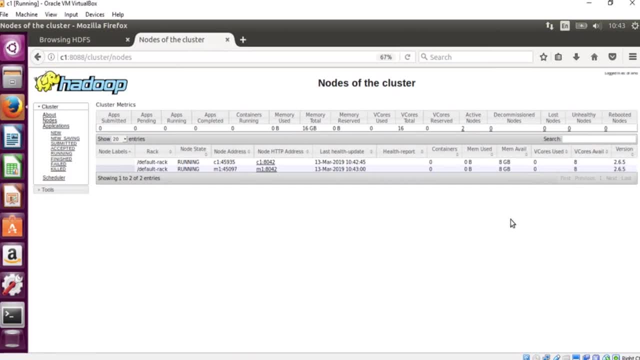 managers and that's why it takes the default properties, that is, 8 gb ram and 8 v cores. now this is my yarn ui. we can also look at scheduler, which basically shows me the different queues, if they have been configured, where you will have to run the jobs. we'll discuss about all these. 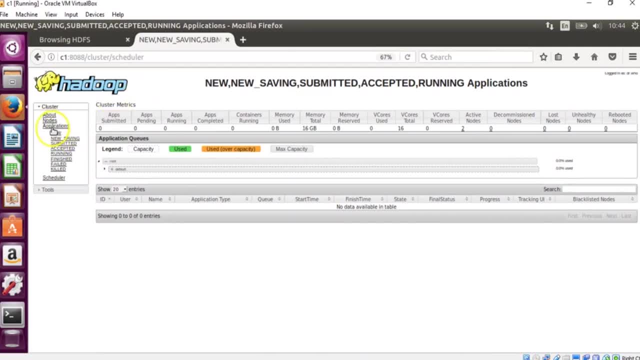 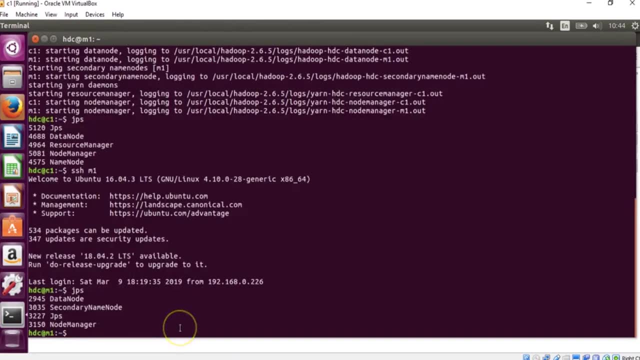 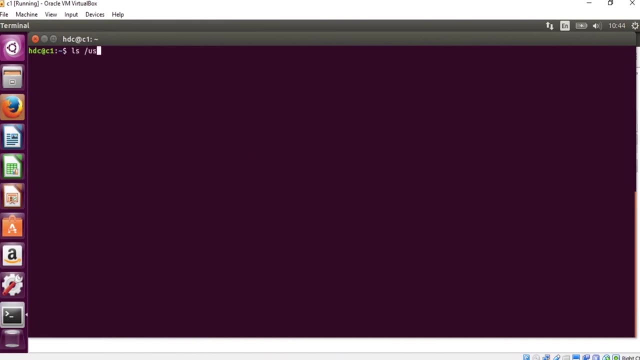 in later in detail. now let's go back to our terminal and let's see where we can find some sample applications which we can run on the cluster. so once i go to the terminal i can well submit the map, produce job from any terminal. now here i know that my hadoop related directory is here and within hadoop you have various directories. 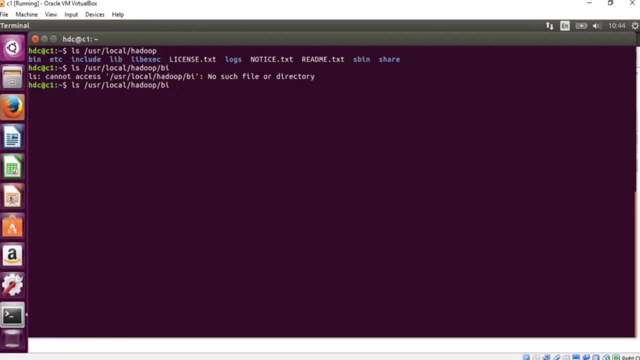 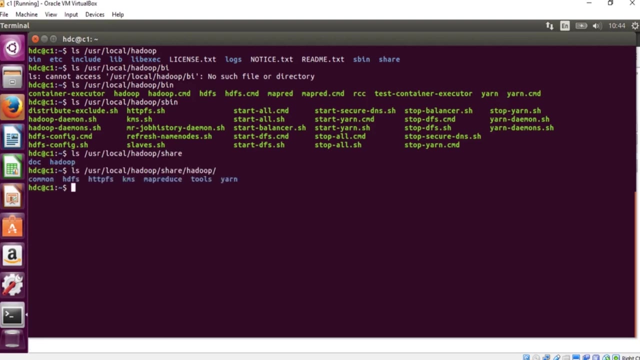 we have discussed that in binaries you have the commands which you can run. in sbin you basically have the startup scripts and here you also notice there is a share directory. in the end, if you look in the shared directory you would find hadoop, and within hadoop you have various sub directories in which we will look for map reduce now this map. 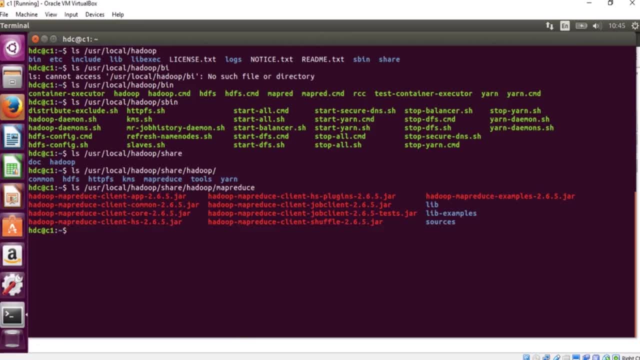 reduce directory has some sample jar files which we can use to run a map reduce on the cluster. similarly, if you are working on a cloud era cluster, you would have to go into opt cloudera parcel cdh lib and in that you would have directories for sdfs map reduce or sdfs yarn. 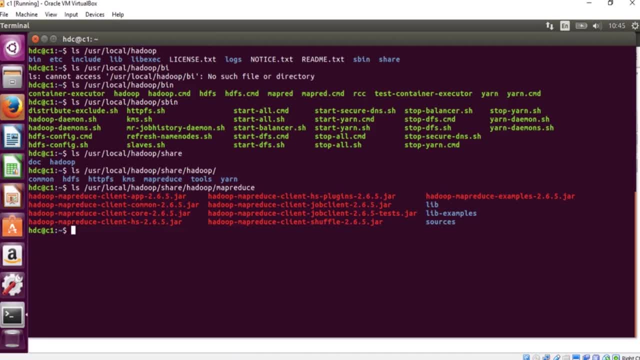 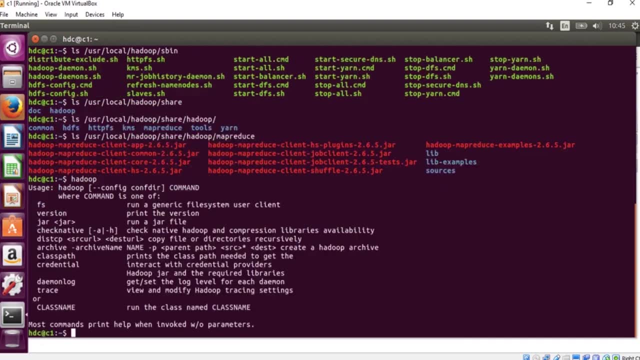 where you can still find the same jars. it is basically a pack which contains your multiple applications. now how do we run a map reduce? we can just type in hadoop and hit enter, and that shows me that i have an option called jar which can be used to run a jar. 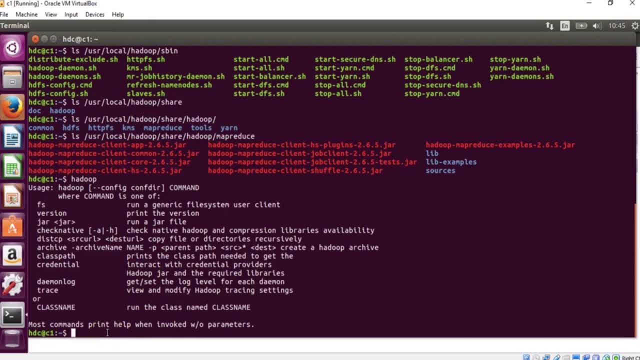 file now, at any point of time. if you would want to see what are the different classes which are available in a particular jar, you could always do a jar minus xvf. for example, i could say jar xvf and i could say user local hadoop share, hadoop map, reduce and then list down your jar file. so i'll say hadoop map. 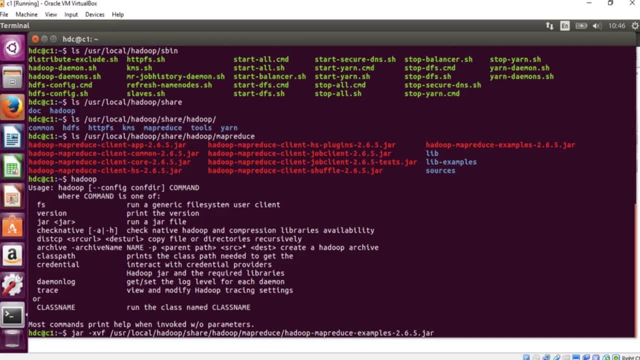 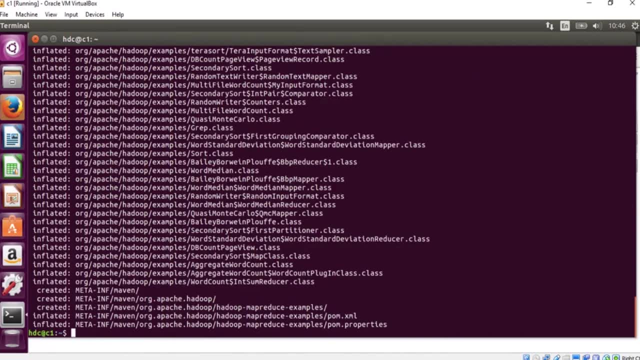 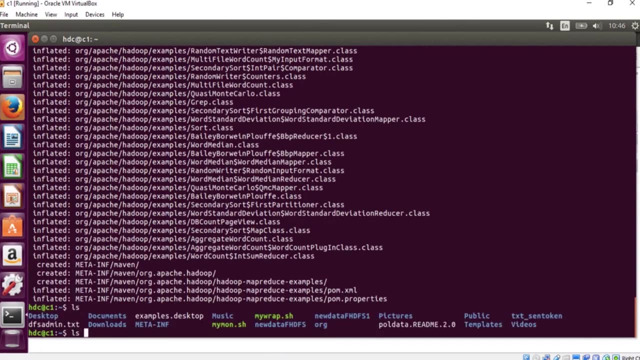 reduce examples and if i do this, this should basically unpack it to show me what classes are available within this particular jar. and it has done this. it has created a meta file and it has created a org directory. we can see that by doing a ls and here if you look in ls org, since i ran 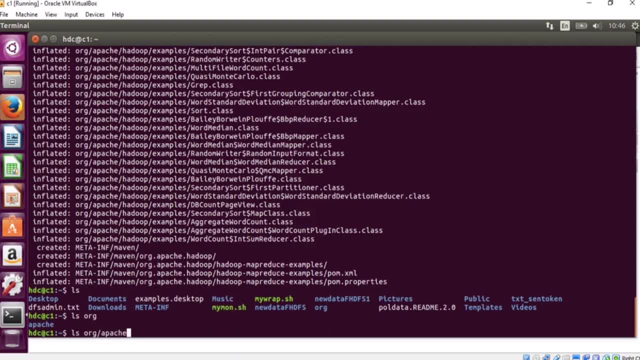 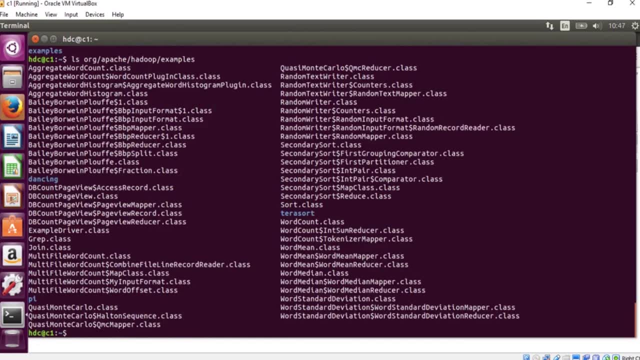 the command from my phone to the computer, i can see that i have a class called hadoop- hadoop share directory. i can look into org patchy hadoop examples which shows me the classes which i have and those classes contain which mapper or reducer classes. so it might not be just mapper and reducer. 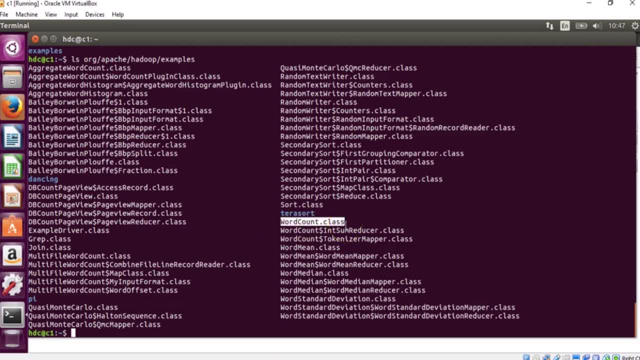 but you can always have a look. so, for example, i am targeting to use word count program which does a word count on files and gives me a list of words and how many times they occur in a particular file or in set of files, and this shows me that what are the classes which belong to word count. so we 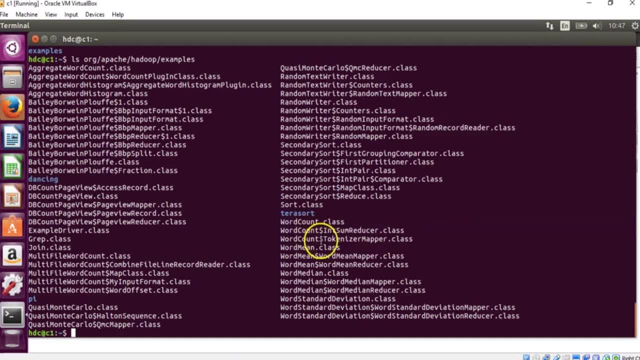 have a int sum reducer, so this is my reducer class. i have tokenizer mapper. that is my mapper class, right, and basically this is what is used. these classes are used if you run a word count. now there are many other programs which are part of this jar file and we can expand and see that. so 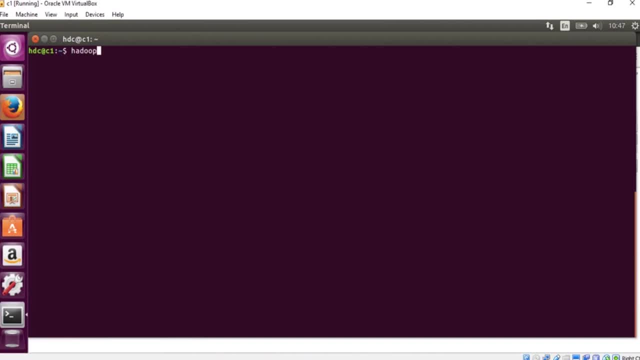 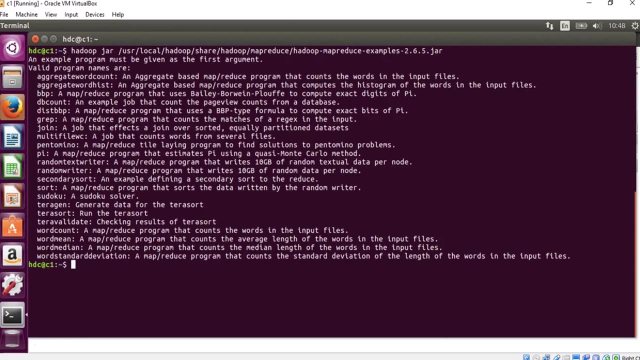 i can say hadoop jar and give your path. so i'll say hadoop jar: user you local hadoop share hadoop map. reduce hadoop map. reduce examples and if i hit on enter, that will show me what are the inbuilt classes which are already available now. these are certain things. 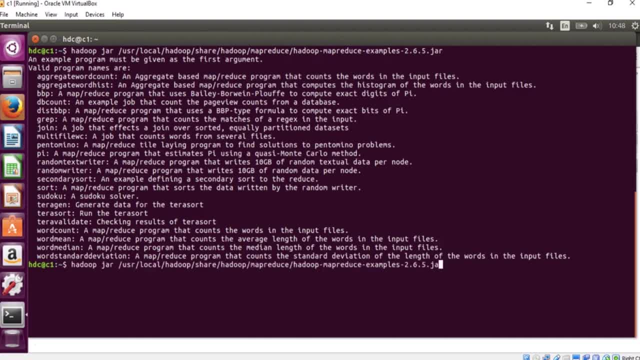 which we can use. now there are other jar files also. for example, i can look at hadoop and here we can look at the jar files which we have in this particular path. so this is one hadoop map examples which you can use. you can always look in other jar files like you can look for hadoop map. reduce client, job client and then. 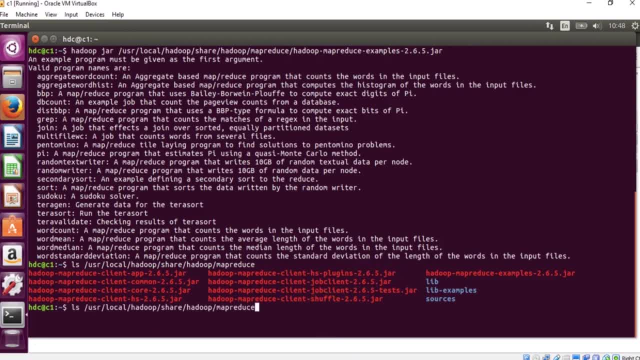 you can look at the test one, so that is also an interesting one. so you can always look into hadoop map: reduce client, job client, and then you have something ending with tests. so if i would have tried this one using my hadoop jar command, so in my previous example, when we did this, it was showing. 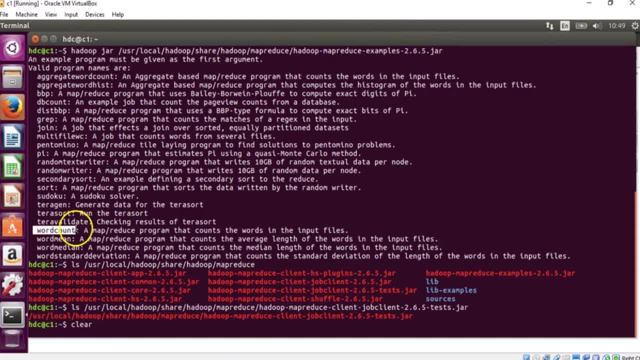 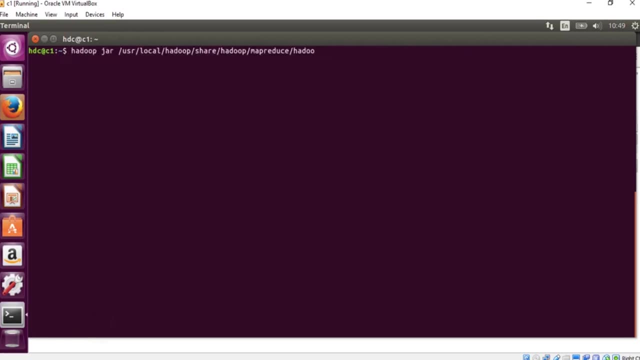 me all the classes which are available, and that already has a word count. now there are other good programs which you can try, like TerraGen to generate dummy data, TerraSort to check your sorting performance and so on, and TerraValidate to validate the results. similarly, we can also do a Hadoop jar, as I said on Hadoop. 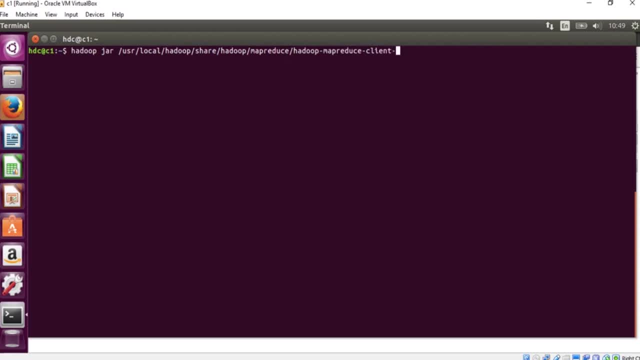 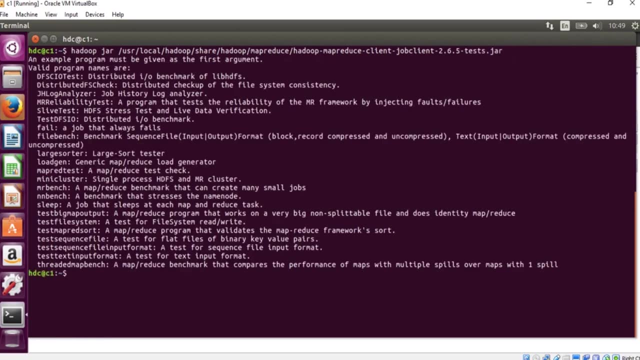 MapReduce- I think that was client- and then we have job client and then test jar. now this has a lot of other classes which can be used, or programs which can be used for doing a stress testing or checking your cluster status and so on. one of them- interesting one, is test EFSIO. but let's not get into all the 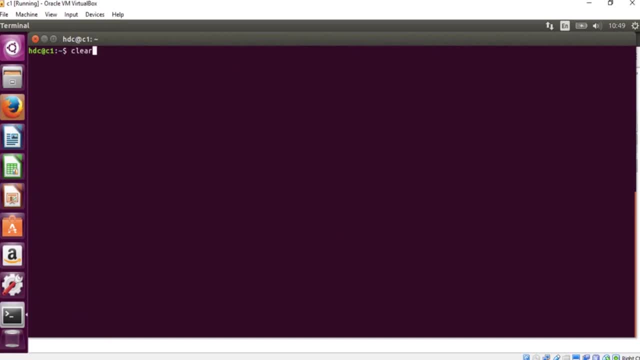 details. in first instance, let's see how we can run a MapReduce. now, if I would want to run a MapReduce, I need to give Hadoop jar and then my jar file, and if I hit on enter it would say it needs the input and output. it needs which class? 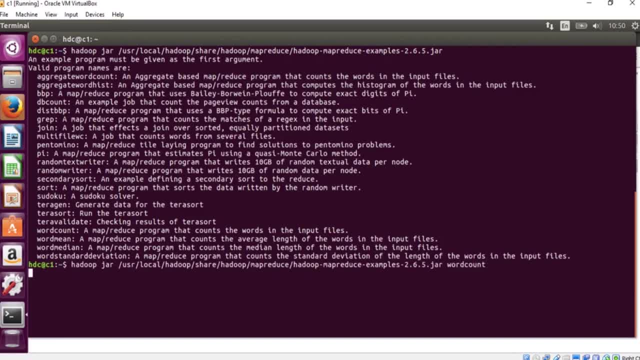 you want to run. so, for example, I would say word count, and again, if i hit on enter it tells me that you need to give me some input and output to process and obviously this processing will be happening on cluster- that is our yarn processing framework, unless and until you would want to run this job in a local mode. so there is a possibility that. 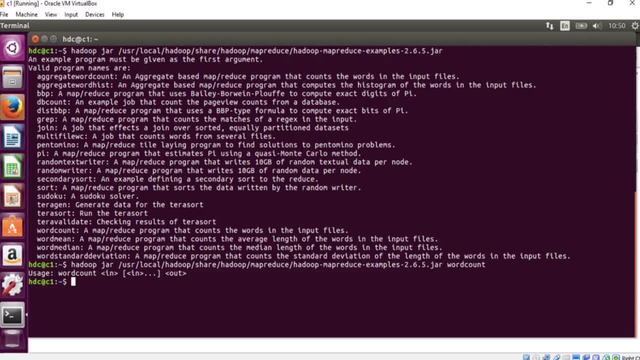 you can run the job in a local mode, but let's first try how it runs on the cluster. so how do we do that? now, here i can do a HDFS ls slash command to see what i have on my HDFS. now, through my UI, i was already showing you that we have set of files and directories which we can use to. 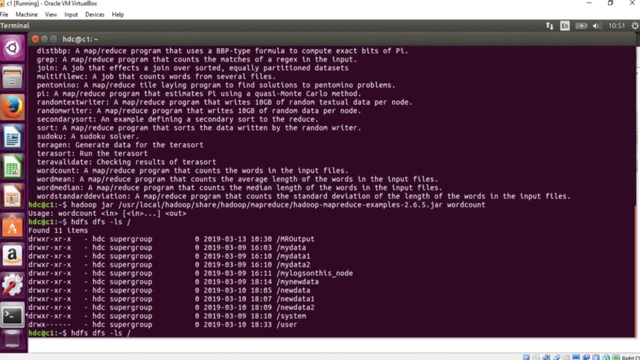 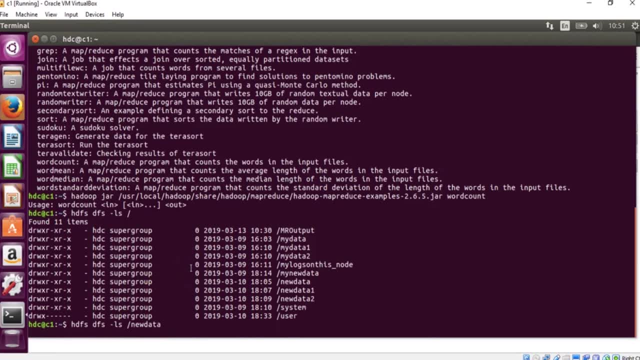 process. now we can take up one single file. so, for example, if i pick up new data and i can look into the files here what we have and we can basically run a MapReduce on a single file or multiple files. so let's take this file, let's run to. basically it took me one single file or one. multiple file, so let's take this file. let's run a MapReduce on a single file or multiple files, so let's take this file. for example, if i pick up new data and the benefits of the concept newly we have localized gets used, so you dream up some data volume access is great. so finally, after I hit the, 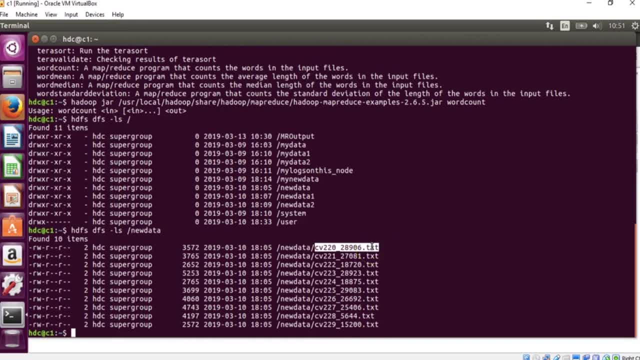 whatever that contains, and I would like to do a word count so that I get a list of words and their occurrence in this file. so let me just copy this now. I also need my output to be written, and that will be written here. so here, if I want. 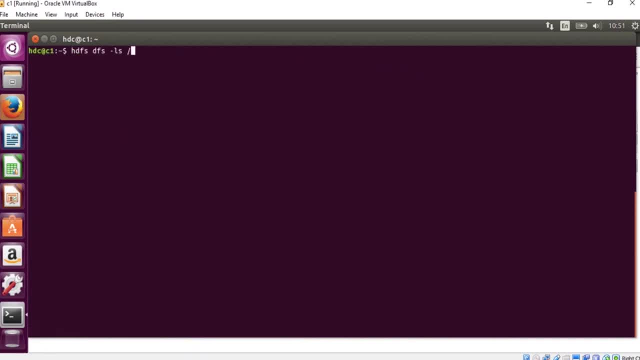 to run a MapReduce. I can say Hadoop, which we can pull out from history, so Hadoop jar word count. now I need to give my input so that will be new data and then I will give this file which we just copied. now I am going to run the word. 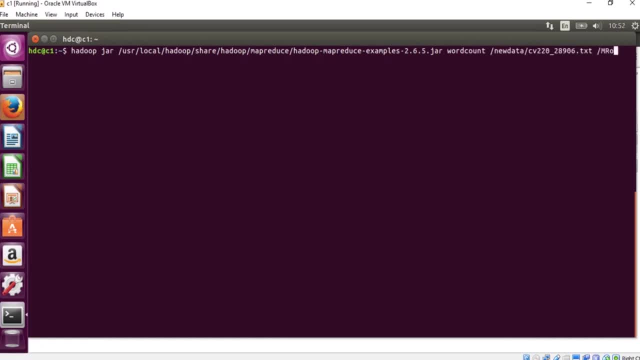 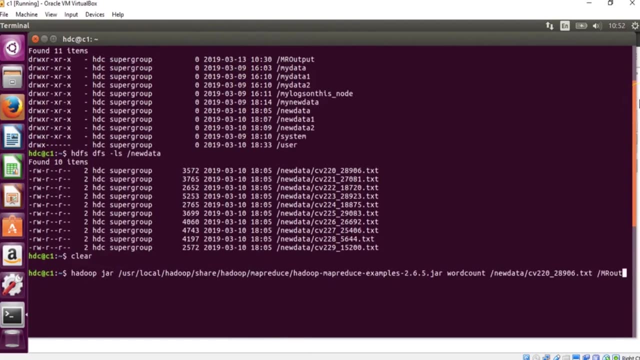 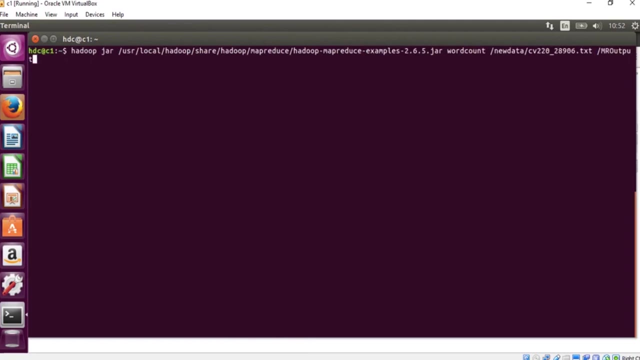 count only on a single file and I will basically have my output, which will be stored in this directory, the directory which I have created already, mr output. so let's do this output, and this is fair enough. now you can give many other properties. you can specify how many map jobs you want to run, how. 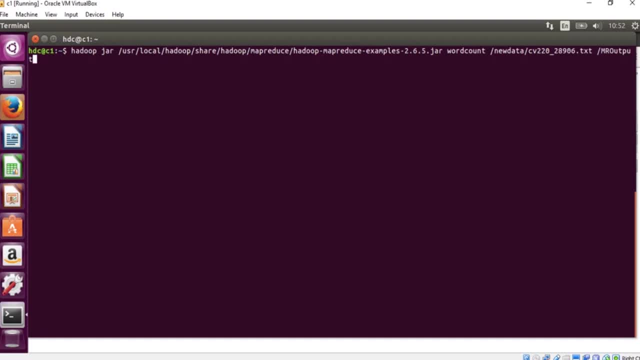 many reduce jobs you want to run, do you want your output to be compressed, do you want your output to be merged, or many other properties can be defined when you are specifying word count, and then you can pass in an argument to pass properties from the command line which will affect your output. now, once I go, 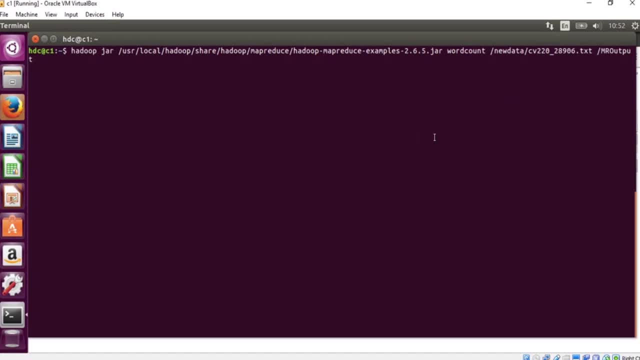 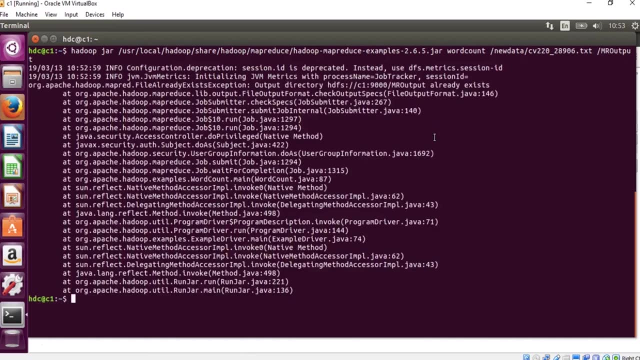 ahead and submit this. this is basically running a simple inbuilt MapReduce job on our Hadoop cluster. now, obviously, internally it will be looking for name node. now we have some issue here and it says the output already exists. what does that mean? so it basically means that Hadoop will create an output. 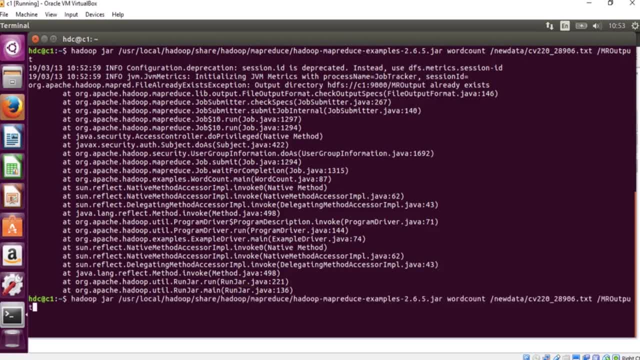 for you. you just need to give a name, but then you don't need to create it. so let's give, let's append the output with number one, and then let's go ahead and run this. so I have submitted this command. now this can also be run in. 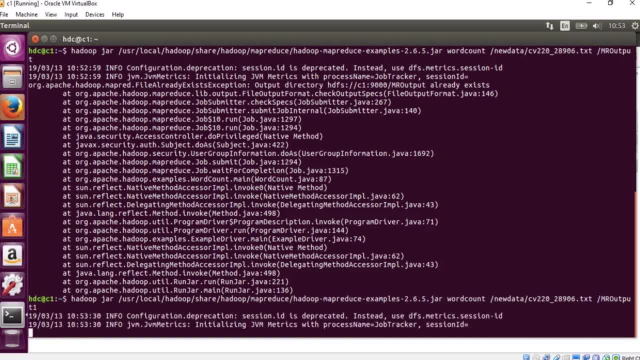 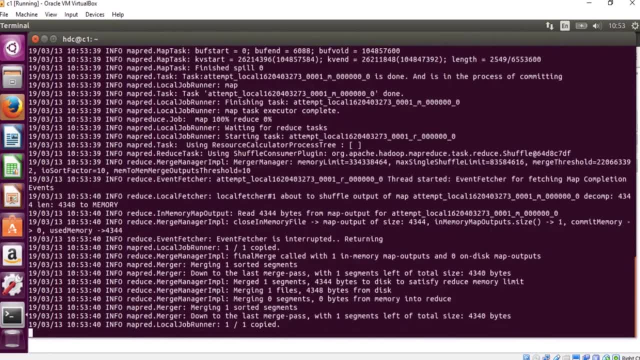 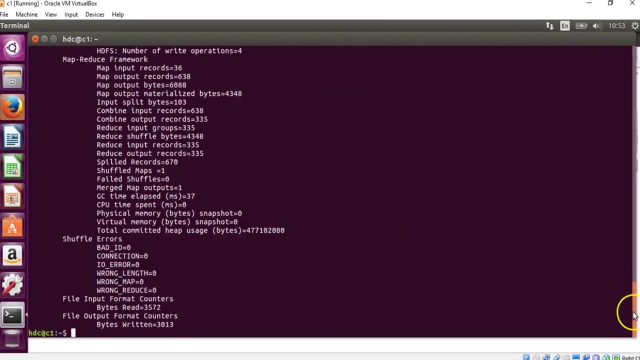 background if you would want to run multiple jobs on your cluster at the same time. so it takes total input paths to processes one. so that is, there is only one split on which your job has to work. now it will internally try to contact your resource manager and basically this is done. so here we can. 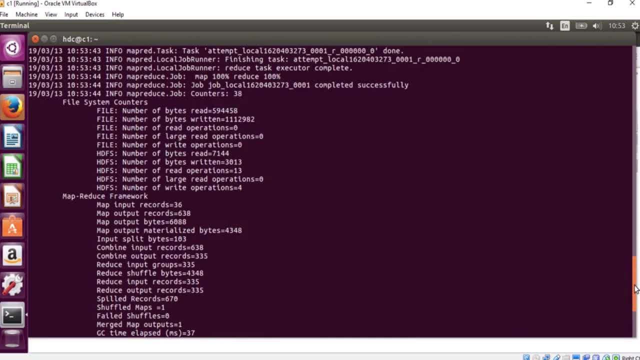 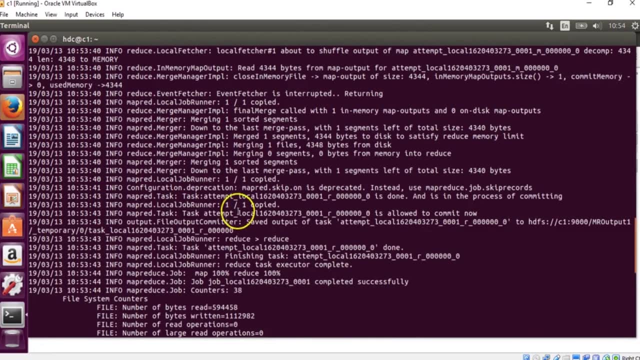 have a look and we can see some counters here. now. what I also see is for some property which it is missing. it has run the job, but it has run in a local mode. it has run in a local mode so, although we have submitted, so this might be. 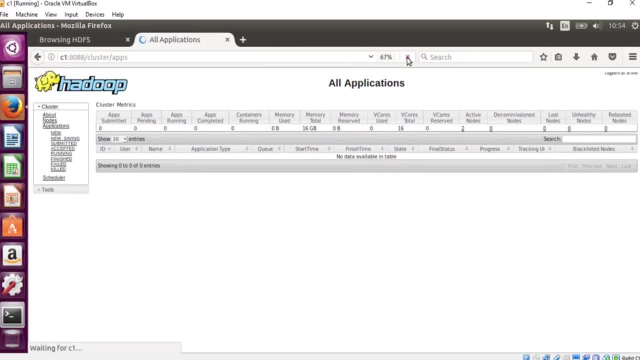 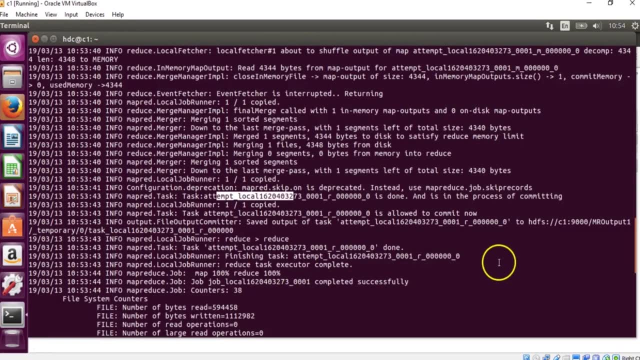 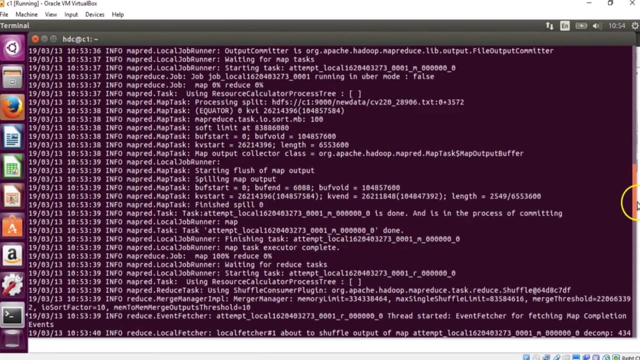 related to my yarn settings and we can check that. so if I do a refresh when I have run my application, it has completed. it would have created an output, but the only thing is it did not interact with your yarn, it did not interact with your resource manager. we can check those properties and here, if we look, 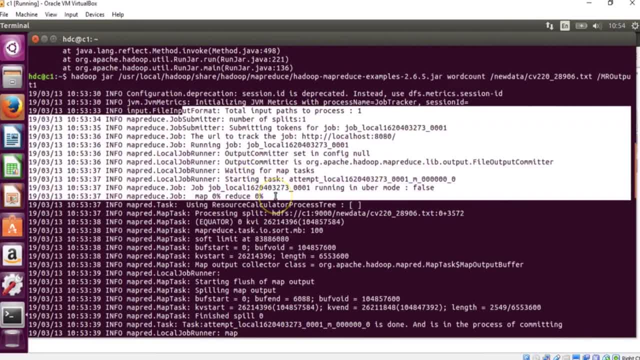 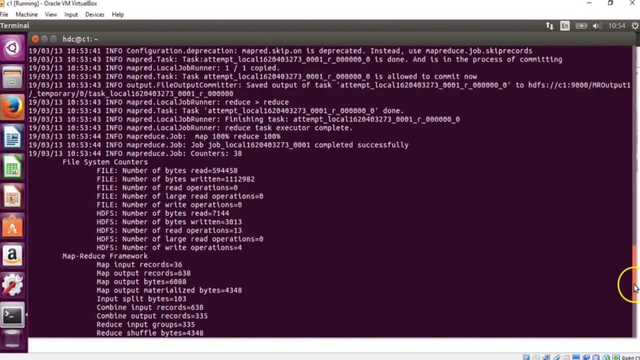 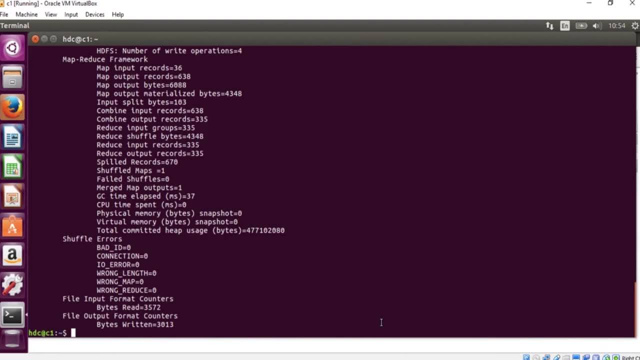 into the job. it basically tells me that it went for mapping and reducing. it would have created an output. it worked on my file, but then it ran in a local mode. it ran in a local mode. so map reduce, remember, is a programming model right now. if you run it on yarn, you get the facilities of running. 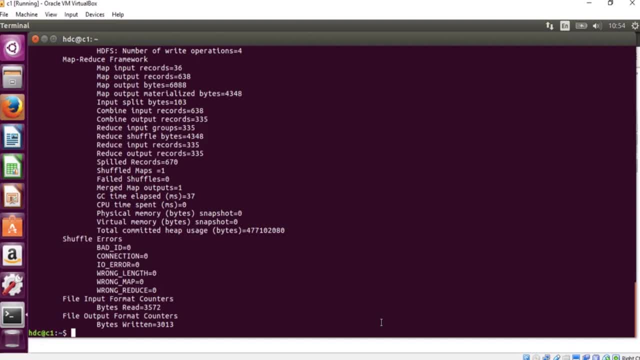 it on a cluster where yarn takes care of resource management. if you don't run it on yarn and run it on a local mode, it will use your machine's ram and cpu cores for processing, but then we can quickly look at the output and then we can also try running this on yarn. so if i look into my hdfs, 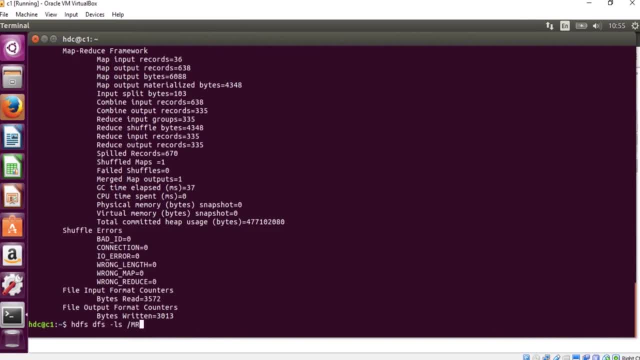 and if i look into my output- mr output, that's the directory which was not used. actually, let's look into the other directory which is ending with one, and that should show me the output created by this map reduce. although it ran in a local mode, it fetched. 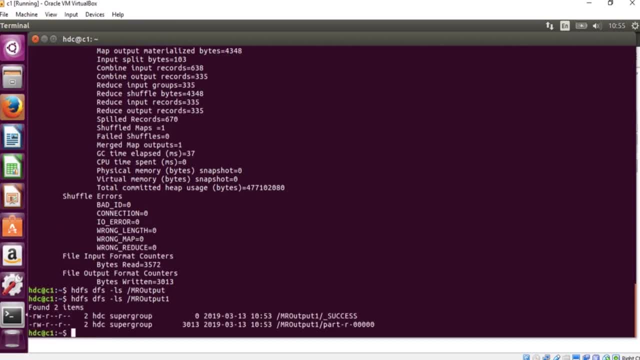 an input file from your sdfs and it would have created output in sdfs. now that's my part file which is created and if you look at part minus r, minus these zeros, if you would have more than one reducer running, then you would have multiple such files created. we can look into this. 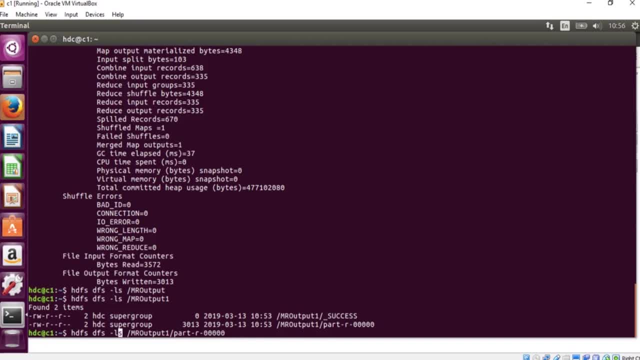 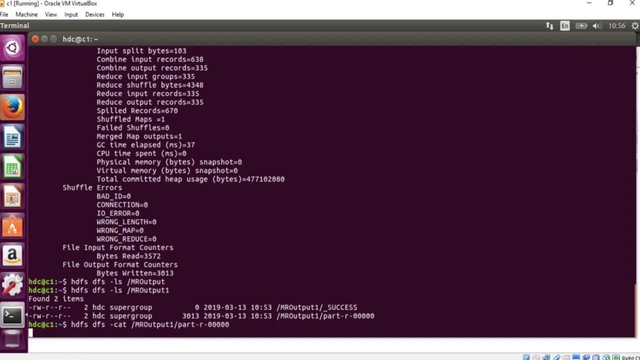 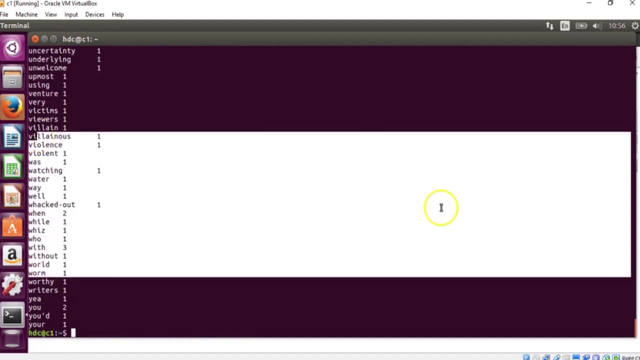 what does this file contain which should have my word count, and here i can say cat, which basically shows me what is the output created by my map reduce? let's have a look into this. so the file which we gave for processing has been broken down and now we have the list of words which occur in. 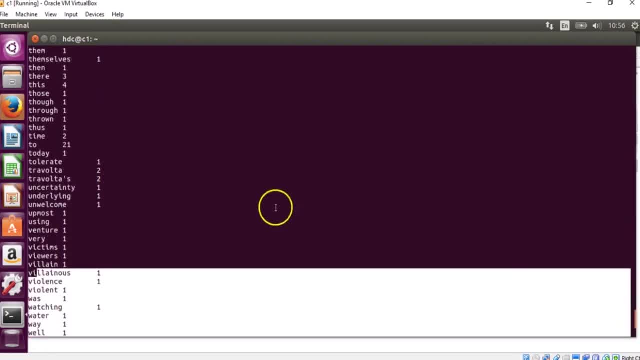 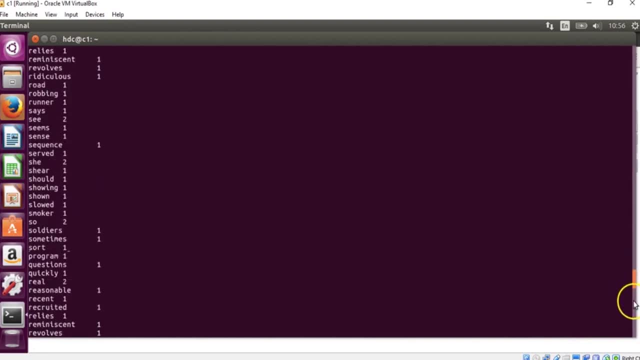 the file plus a count of those words. so if there is some word which is in is more, then it shows me the count. so this is a list of my words and the count for that. so this is how we run a sample map reduce job. i will also show you how we can run it on yarn. now let's 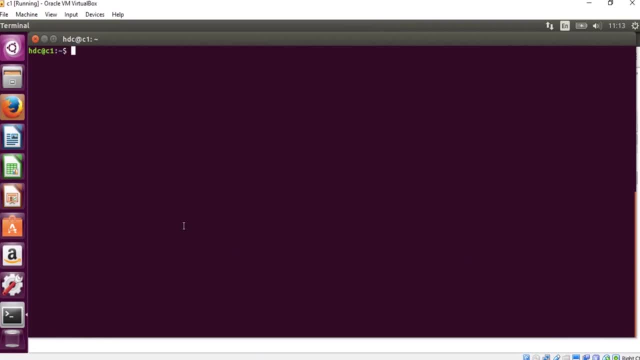 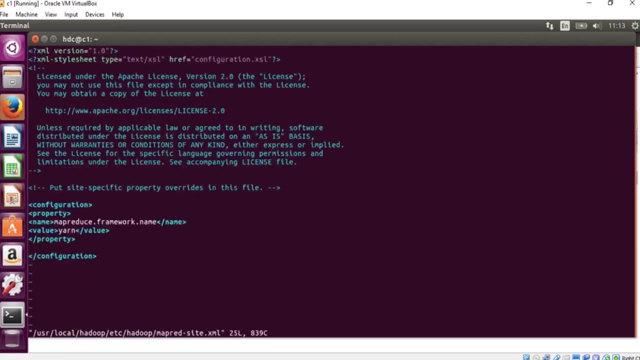 run map reduce on yarn and initially when we tried running a map reduce it did not hit yarn but it ran in a local mode and that was because there was a property which had to be changed in map reduce hyphen site file. so basically, if you look into this file, the error was that i had given. 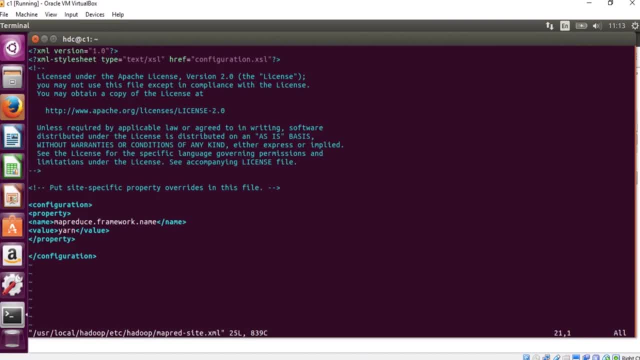 a property which says map red dot framework dot name and that was the property which was not the right property name and it was ignored and that's why it ran in a local mode. so i changed the property to map reduce dot framework dot name, restarted my cluster and everything should be fine. 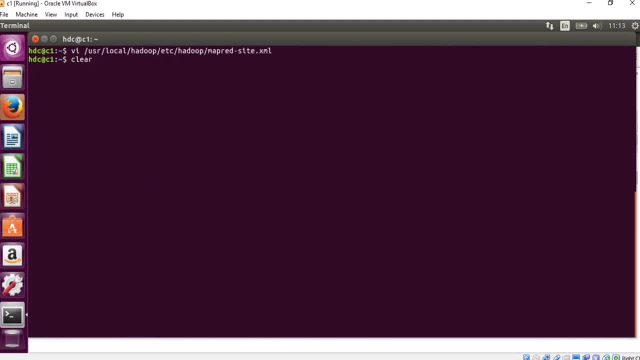 now, and that map red hyphen site file has also been copied across the nodes. now to run a map reduce on a hadoop cluster so that it uses yarn and yarn takes care of resource allocation on one or multiple machines. so i'm just changing the output here and now i will submit this. 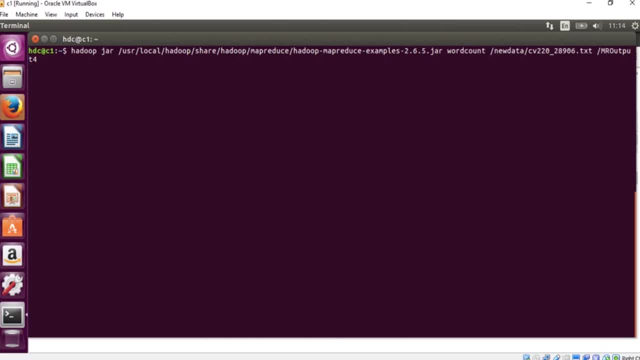 job, which should first connect to the resource manager. and if it connects to the resource manager, that means our job will be run using yarn on the cluster rather than in a local mode. so now we have to wait for this application to internally connect to resource manager and once it starts, 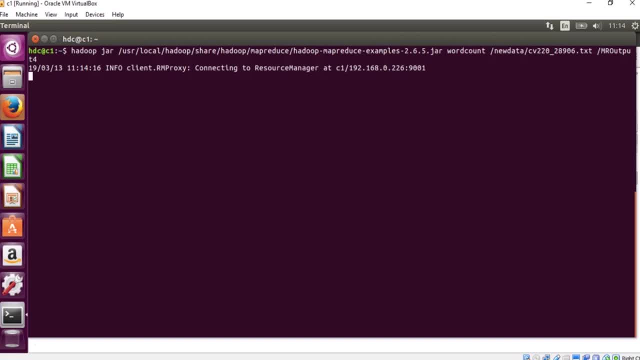 there. we can always go back to the web ui and check if our application has reached yarn. so it shows me that there is one input part to be processed. that's my job id, that's my job name and that's my application id, which you can even monitor status from the command line. now here: 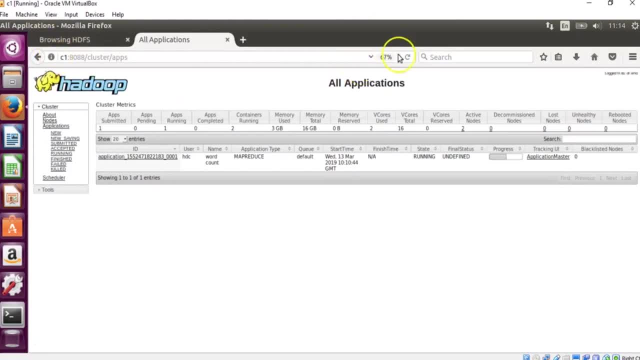 the job has been submitted, so let's go back here and just do a refresh on my yarn ui, which should show me the new application which is submitted. it tells me that it is in accepted state. application master has already started and if you click on this link, it will also give you more details of 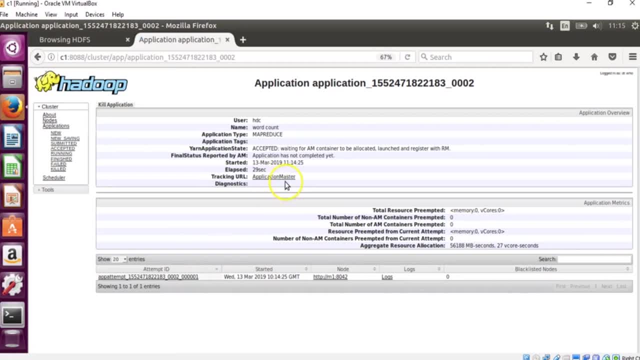 how many map and reduce tasks would run. so, as of now it says the application master is running, it would be using this application master: application master, application master application, this node, which is m1. we can always look into the logs. we can see that there is a one task. 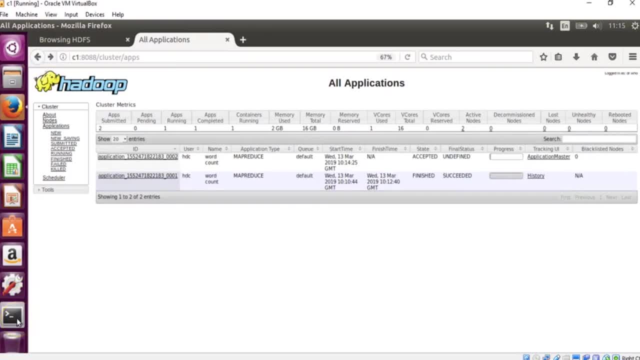 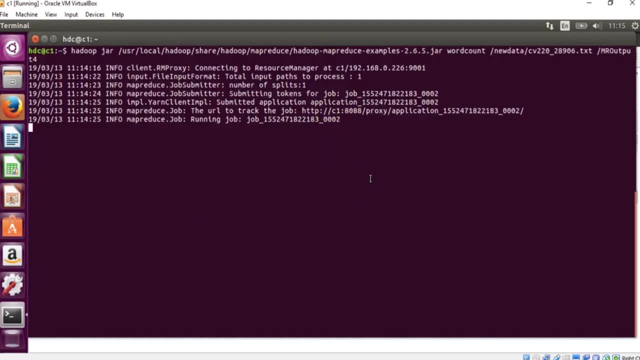 attempt which is being made. and now, if i go back to my terminal, i will see that it is waiting to get some resources from the cluster and once it gets the resources, it will first start with the mapping phase, where the mapper function runs. it does the map tasks one or multiple, depending on. 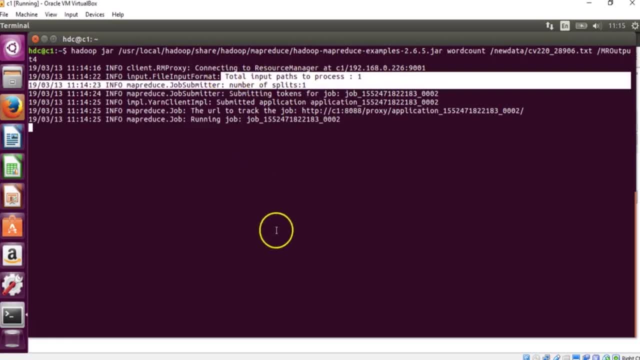 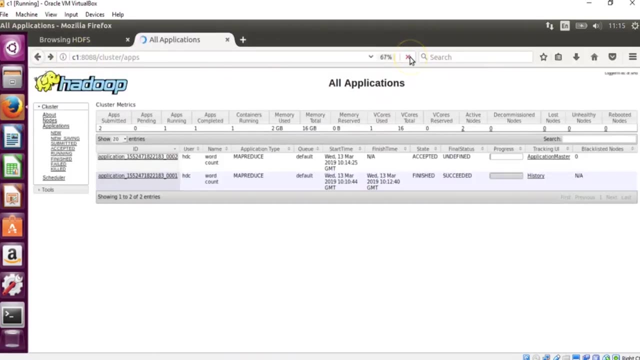 the splits. so right now we have one file and one split, so we will have just one map task running. once the mapping phase completes, then it will get into reducing, which will finally give me my output so we can be toggling through these sessions. so here i can just do a refresh to see what is. 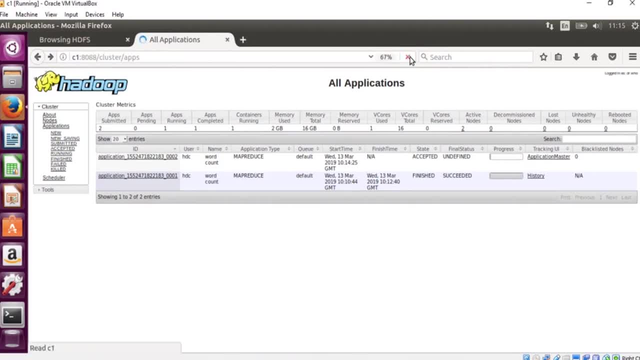 happening with my application? is it proceeding? is it still waiting for resource manager to allocate some resources now? just couple of minutes back i tested this application on yarn and we can see that my first application completed successfully and here we will have to give some more time so that yarn can allocate the resources now, if the resources were used by some. 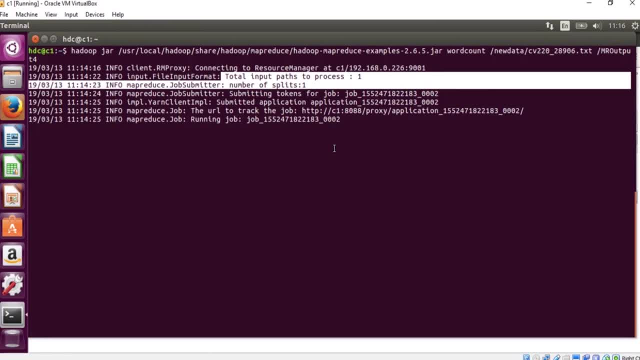 other application, they will have to be freed up now. internally, yarn takes care of all that which we will learn more detail in yarn or you might have already followed the yarn based session. now here we will have to just give it some more time and let's see if my application 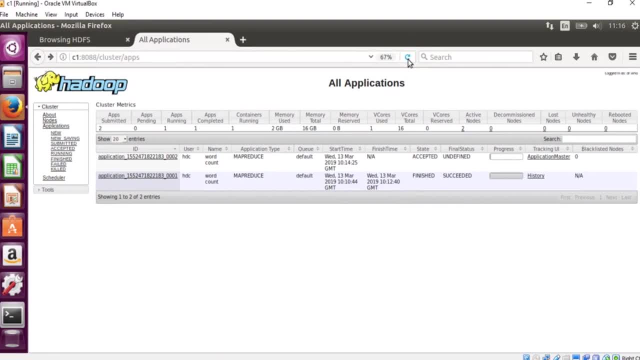 proceeds with the resources what yarn can allocate to it. sometimes you can also see a slowness web ui shows up and that can be related to the amount of memory you have allocated to your nodes. now for apache we can have less amount of memory and we can still run the cluster. and, as i said, 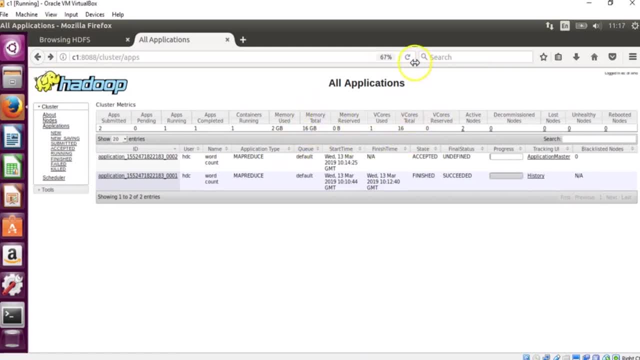 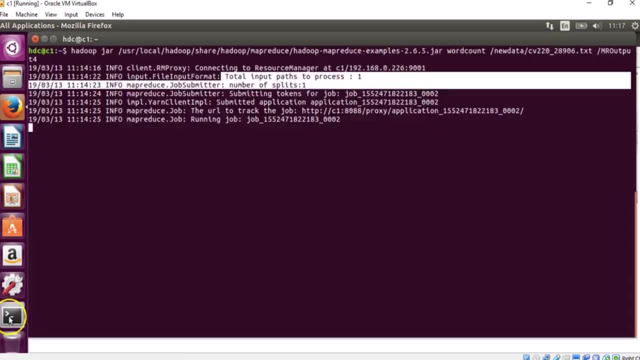 the memory which shows up here- 16 gb and 16 cores- is not the true one. those are the default settings, right? but then my yarn should be able to facilitate running of this application. let's just give it couple of seconds and then let's look into the output. here again, i had to make some 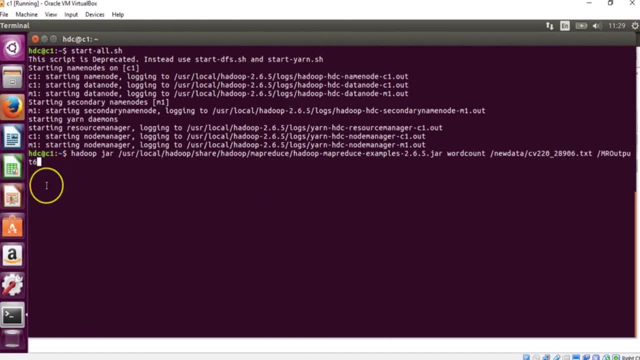 changes in the settings because our application was not getting enough resources and then basically i restarted my cluster. now let's submit the application again to the cluster, which first should contact the resource manager and then basically the map and reduce process should start. so here i've submitted an application, it is connecting to the resource manager, and then 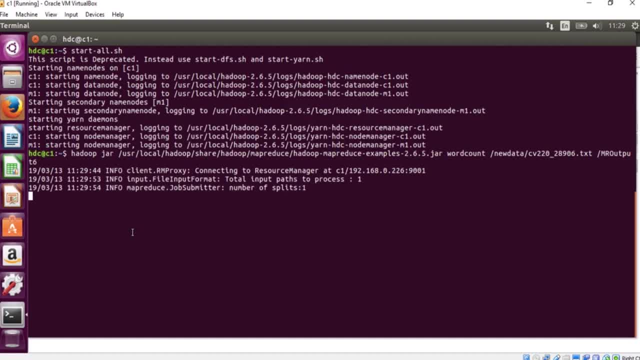 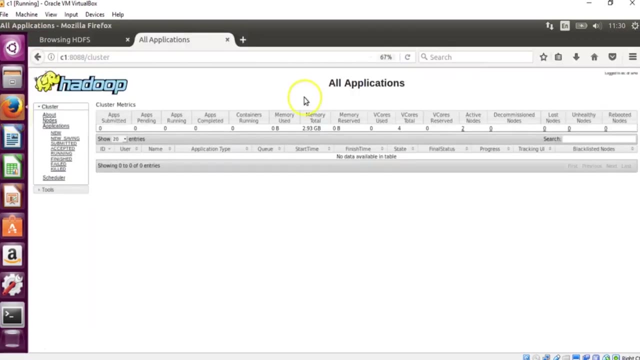 basically, it will start internally an app master. that is application master. it is looking for the number of splits, which is one, it's getting the application id and it basically then starts running the job. it also gives you a tracking url to look at the output, and now we should go back and look at our yarn ui. 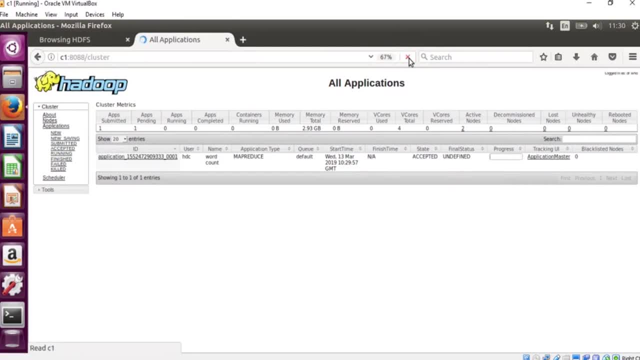 if our application shows up here and we will have to give it a couple of seconds when it can get the final status change to running, and that's where my application will be getting resources. now, if you closely notice here, i have allocated specific amount of memory, that is, 1.5 gb for node manager on every node, and i have basically given two cores each. 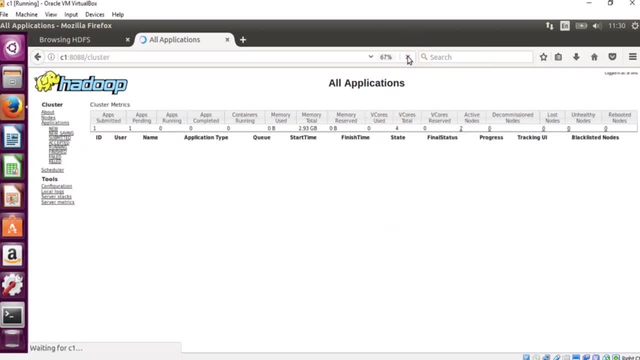 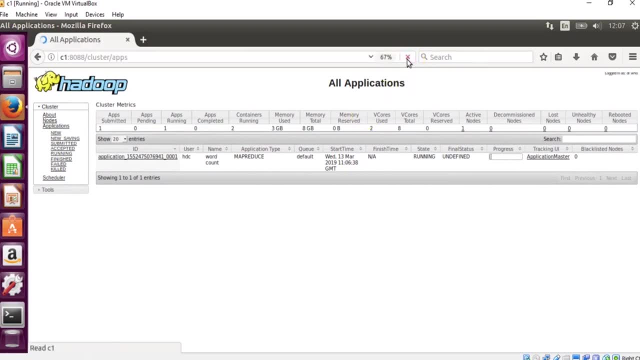 which my machines also have, and my yarn should be utilizing these resources rather than going for default. now the application has started moving and we can see the progress bar here, which basically will show what is happening, and if we go back to the terminal, it will show that. 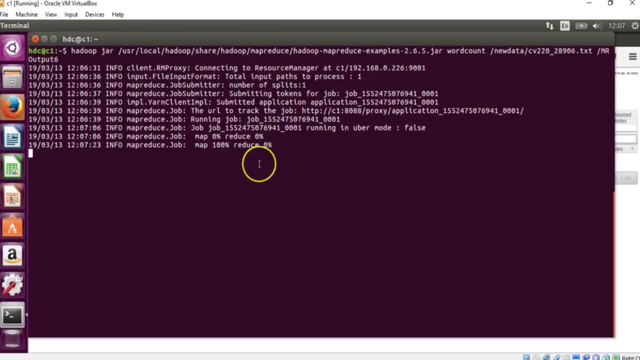 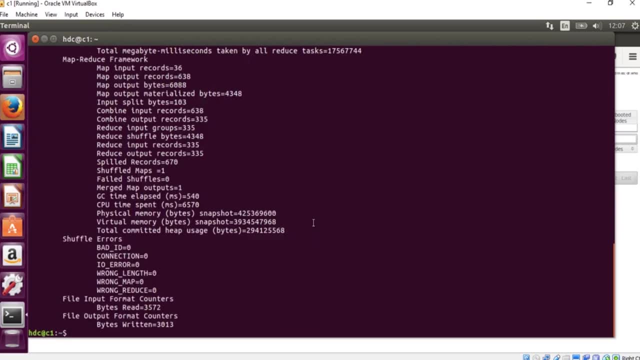 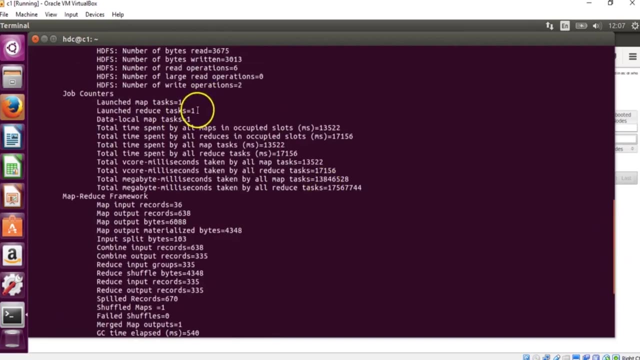 first it went in deciding map and reduce. it goes for map mapping phase completes, then the reducing phase will come into existence. and here my job has completed. so now it has basically used. we can always look at how many map and reduce tasks were run. it shows me that there was one map and one reduced task. now, with the number of map tasks, 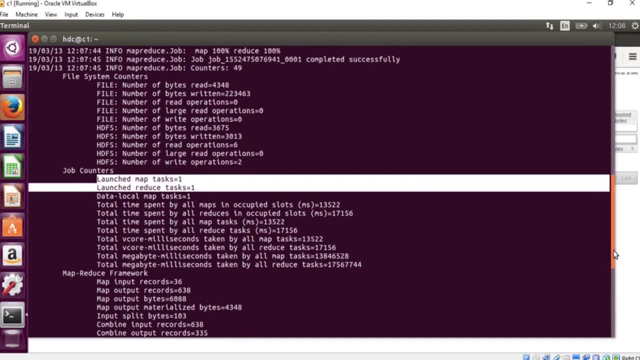 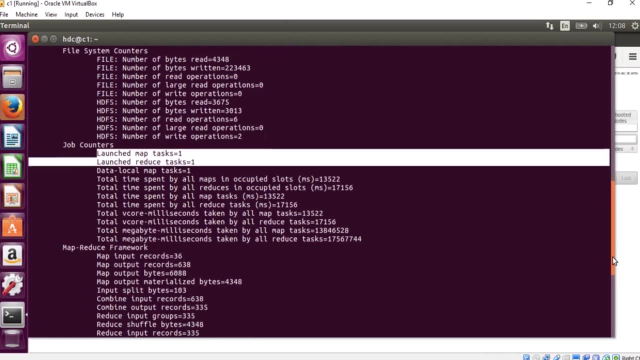 depends on the number of splits, and we had just one file which is less than 128 mb, so that was one split to be processed and reduced. task is internally decided by the reducer or depending on what kind of property has been set in hadoop config files. now it also tells me: 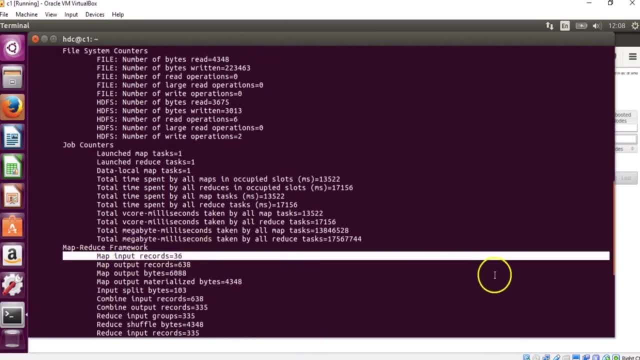 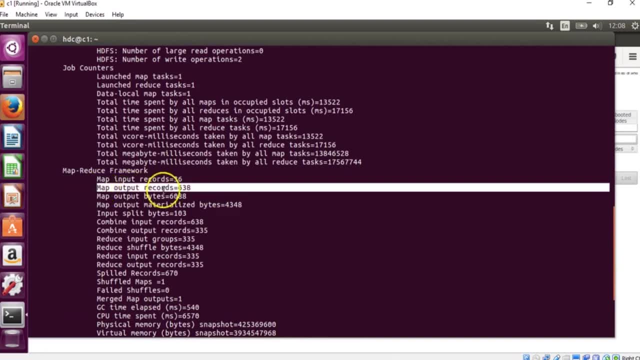 how many input records were read, which basically means these were the number of lines in the file. it tells me output records, which gives me the number of total words in the file- now there might be duplicates- and that which is processed by internal combiner. further processing or forwarding. 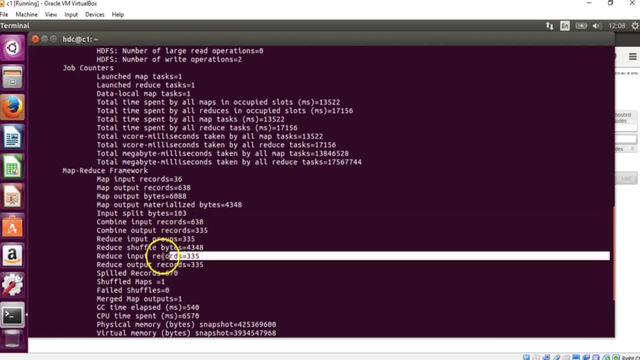 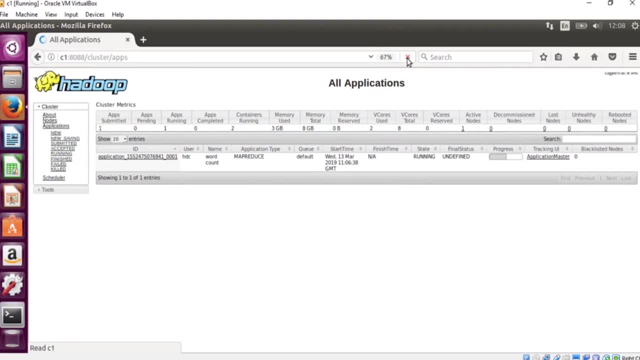 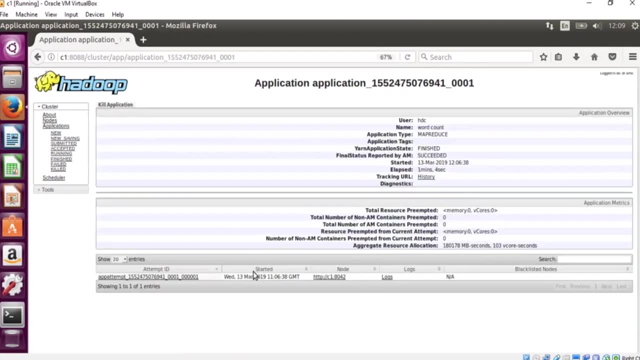 that information to reducer and basically reducer, works on 335 records, which gives us a list of words and their count. now if i do a refresh here, this would obviously show my application is completed. it says succeeded. you can always click on the application to look for more information. it tells me where it ran. now we do not have a history server running as of now. 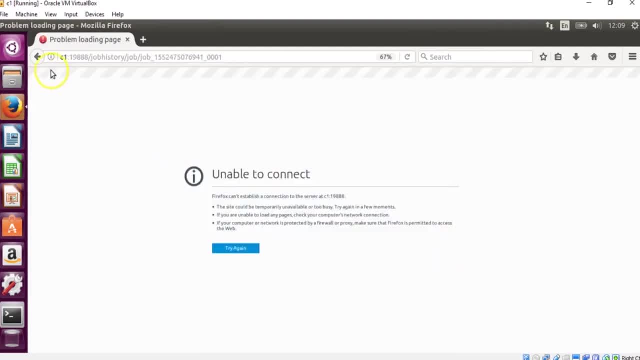 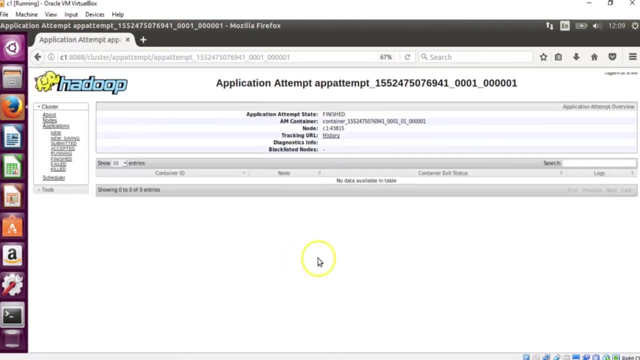 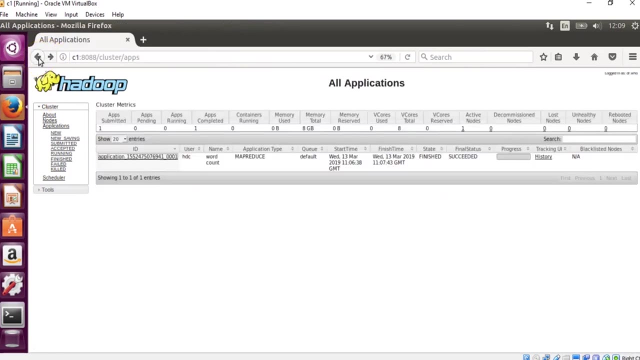 otherwise we can always access more information. so this leads to history server, where all your applications are stored. but i can click on this attempt tasks and this will basically show me history url, or you can always look into the logs. so this is how you can submit a sample application. 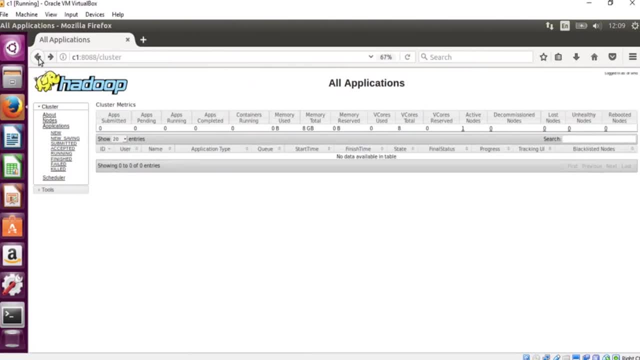 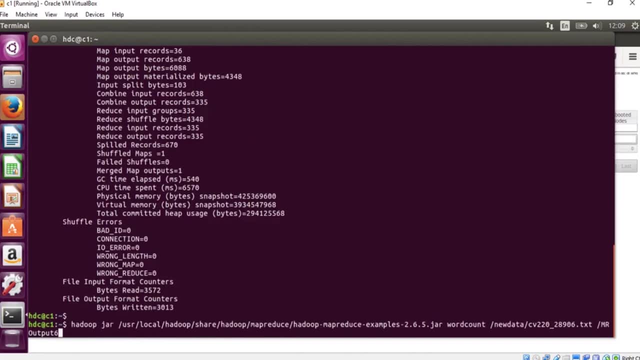 which is inbuilt, which is available in the jar on your hadoop cluster and that will utilize your cluster to run. now you could always, as i said, when you are running a particular job, remember to change the output directory and if you would not want it to be processing a single individual file, 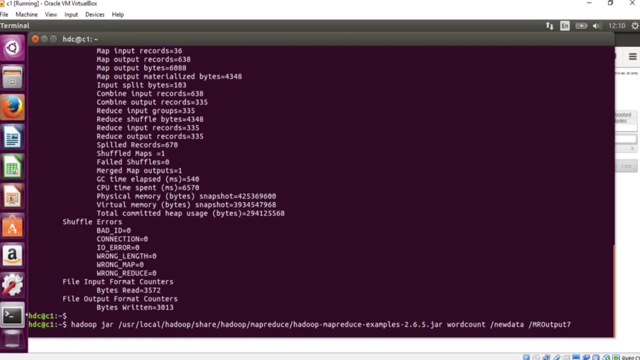 you could also point it to a directory. that basically means it will have multiple files and depending on the file sizes there would be multiple splits and according to that, multiple map tasks will be selected. so if i click on this, this would submit my second application to the. 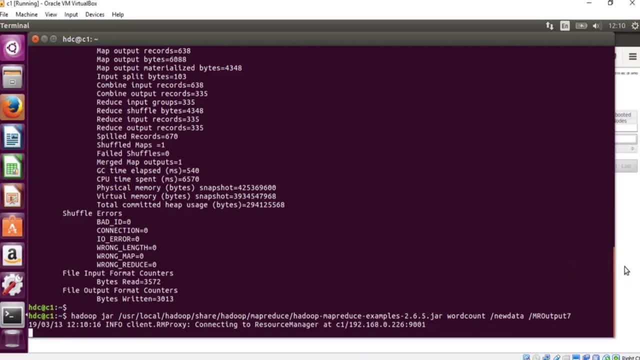 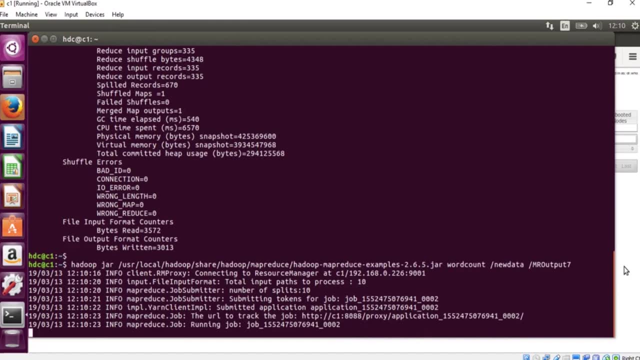 cluster which should first connect to resource manager. then resource manager has to start an application master. now here we are targeting 10 splits. now you have to sometimes give couple of seconds in your machines so that the resources which were used are internally already freed up so that your cluster can pick it up and run it, so that you can run it in the same way you can. 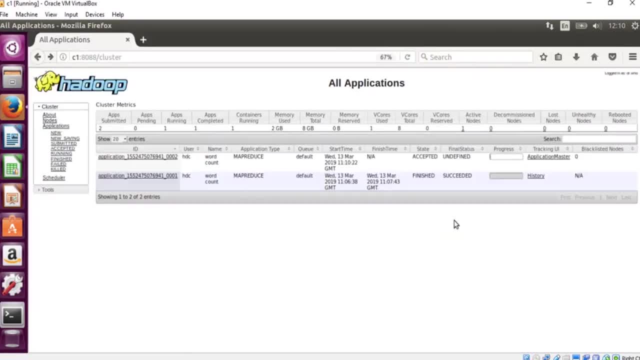 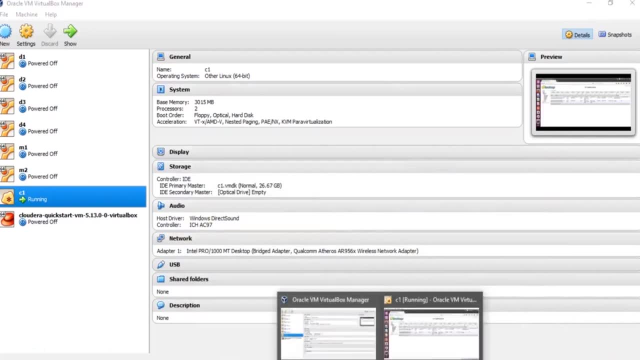 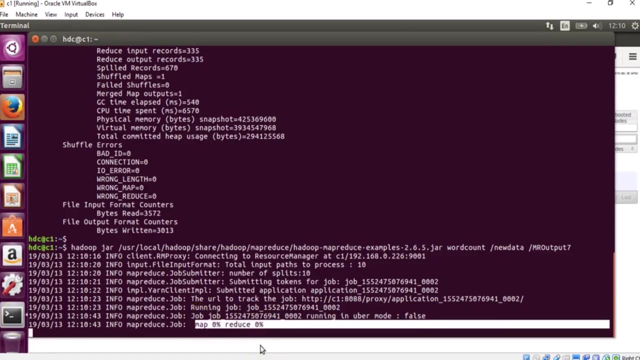 up and then your yarn can take care of resources. so right now my application is in undefined status, but then as soon as my yarn provides it the resources, we will have the application running on our yarn cluster. so it has already started. if you see it is going further, then it would. 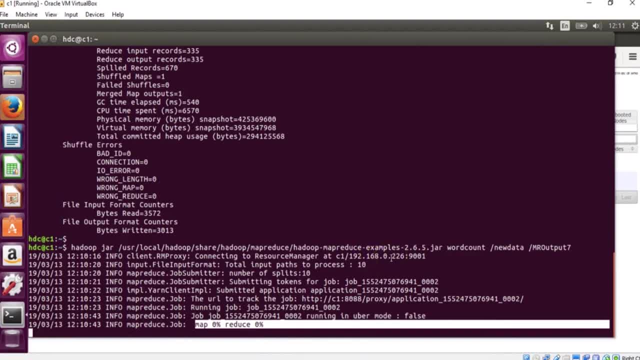 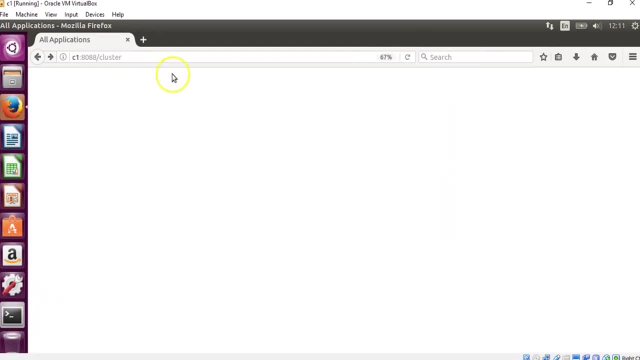 launch 10 map tasks, and it would. the number of reduced tasks would be decided on either the way your data is or based on the properties which have been set at your level. let's just do a quick refresh here on my yarn ui to show me the progress. also, take care. 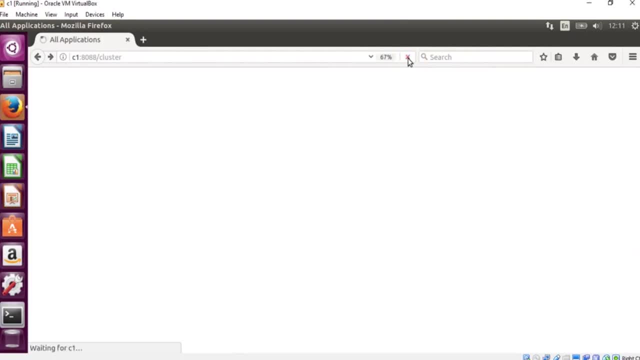 that when you are submitting your application, you need to have the output directory mentioned. however, do not create it. hadoop will create that for you. now, this is how you run a map: reduce without specifying properties, but then you can specify more properties. you can look into what. 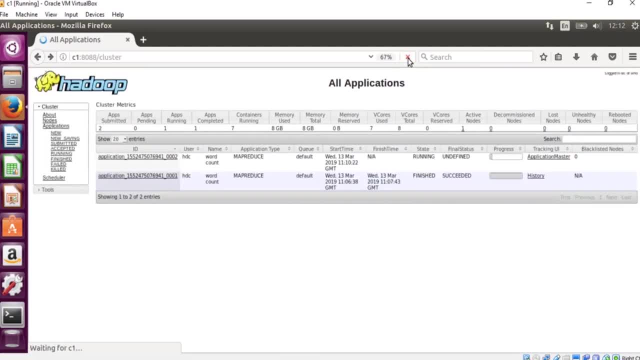 are the things which can be changed for your mapper and reducer, or basically having a combined class which can do a mini reducing, and all those things can be done. so we will learn about that in the later sessions. now we will compare hadoop, version one, that is, with map reduce, version one. 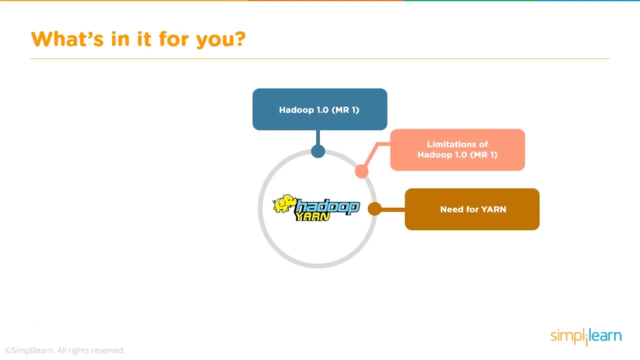 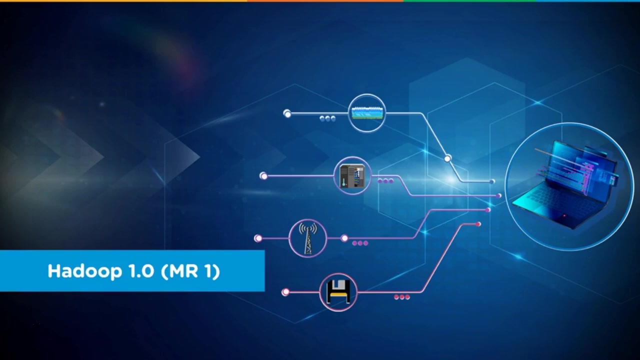 we will understand and learn about the limitations of hadoop version one. what is the need of yarn, what is yarn, what kind of workloads can be running on yarn, what are yarn components, what is yarn architecture? and finally, we will see a demo on yarn. so hadoop version. 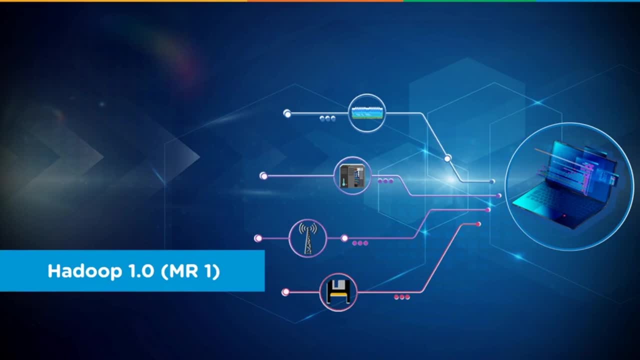 one or map reduce version one. well, that's outdated now and nobody is using hadoop version one, but it would be good to understand what was in hadoop version one and what were the limitations of hadoop version one, which brought in the thought for the future processing layer. that is yarn now when we 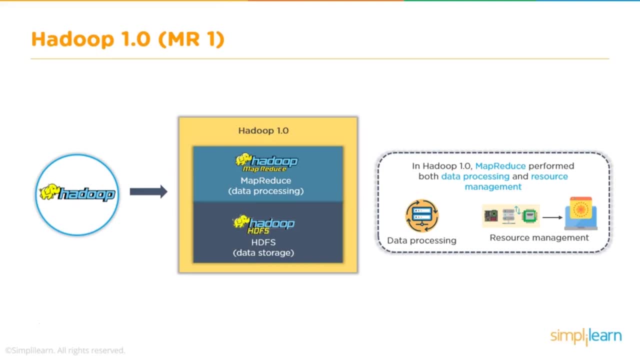 talk about hadoop, we already know that hadoop is a framework and hadoop has two layers. one is your storage layer, that is, your sdfs, and the other one is the storage layer, that is your sdfs, and the other one is the hadoop distributed file system, which allows for distributed storage and processing, which allows 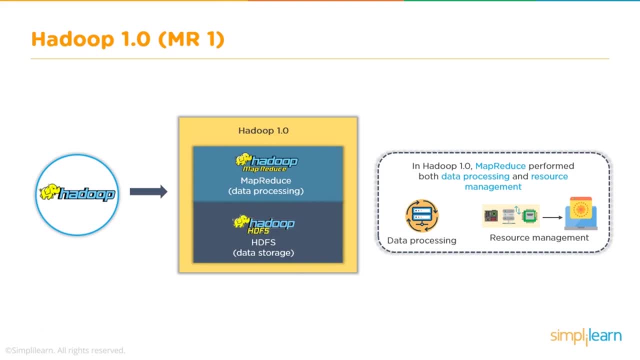 fault tolerance by in-built replication and which basically allows you to store huge amount of data across multiple commodity machines. when we talk about processing, we know that map reduce is the oldest and the most mature processing programming model which basically takes care of your data processing on your distributed file system. so in hadoop version, one map. 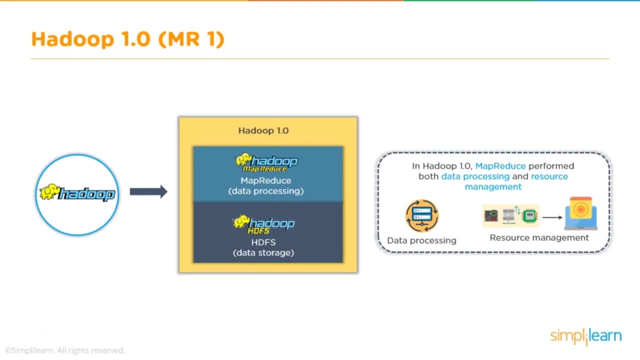 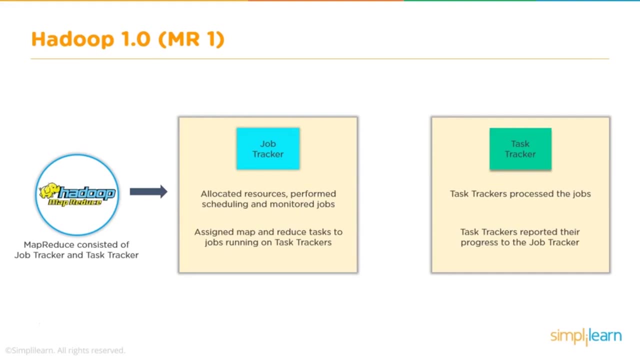 reduce performed both data processing and resource management and that's how it was problematic. in map reduce we had, basically, when we talk about the processing layer, we had the master, which was called job tracker, and then you had the slaves, which were the task trackers. so your job tracker- 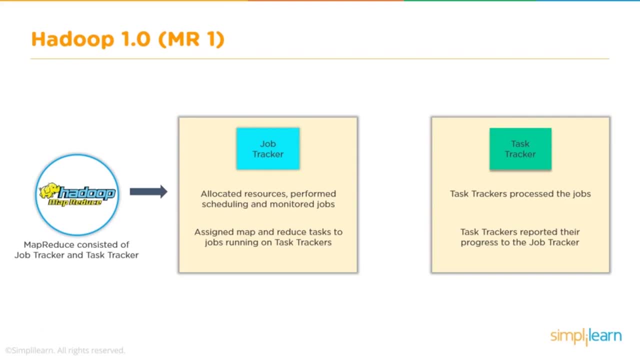 was taking care of allocating resources. it was performing scheduling and even monitoring the jobs. it basically was taking care of assigning, map and reduce tasks to the jobs running on task trackers. and task trackers, which were co-located with data nodes, were responsible for processing the jobs. so task trackers were the slaves for the processing layer which reported their progress to. 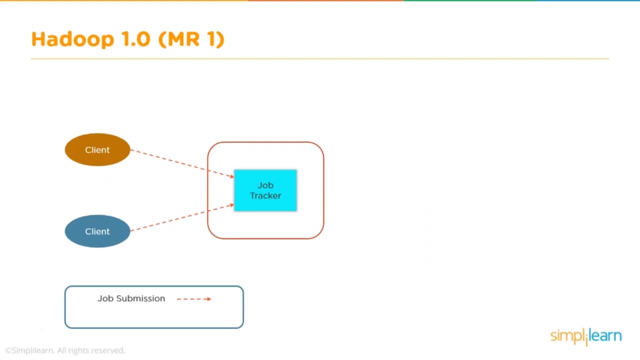 the job tracker. so this is what was happening in Hadoop version 1. now, when we talk about Hadoop version 1, we would have say client machines or an API or an application which basically submits the job to the master. that is job tracker. now, obviously we cannot forget that there would 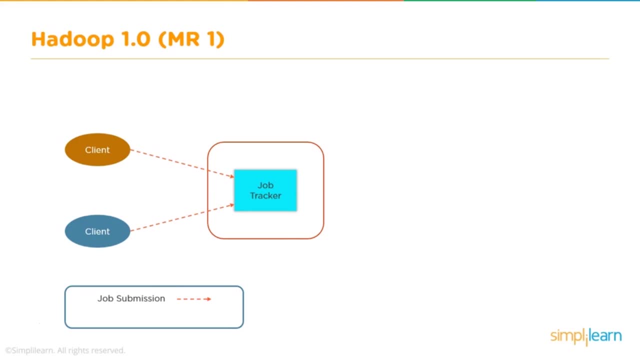 already be an involvement from name node, which basically tells which are the machines or which are the data nodes where the data is already stored. now, once the job submission happens to the job tracker, job tracker being the master daemon for taking care of your processing request and also resource management, job scheduling would then be interacting with your multiple task trackers. 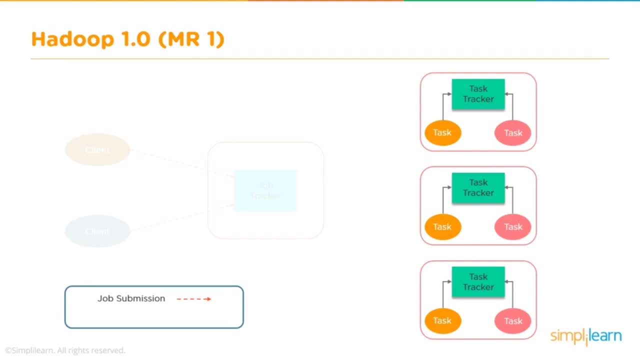 which would then be called task trackers, and these task trackers will be used when doing the job. tracking be running on multiple machines, so each machine would have a task tracker running and that task tracker, which is a processing slave, would be co-located with the data nodes. now we know that. 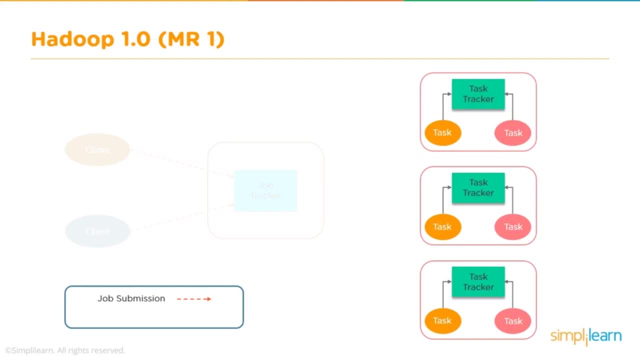 in case of hadoop, you have the concept of moving the processing to wherever the data is stored, rather than moving the data to the processing layer. so we would have task trackers which would be running on multiple machines, and these task trackers would be responsible for handling the 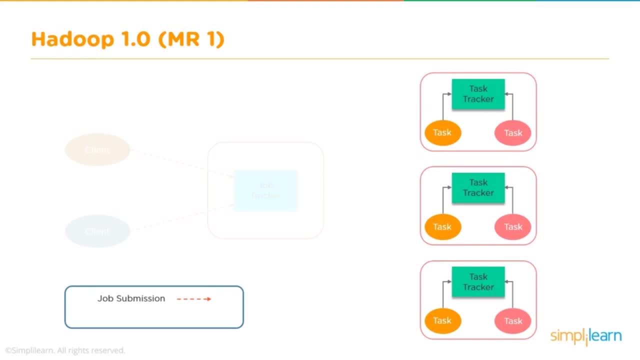 tasks. what are these tasks? these are the application, which is broken down into smaller tasks which would work on the data which is respectively stored on that particular node. now, these were your slave demons, right? so your job tracker was not only tracking the resources, so your task trackers were sending heartbeats, they were sending in packets and information. 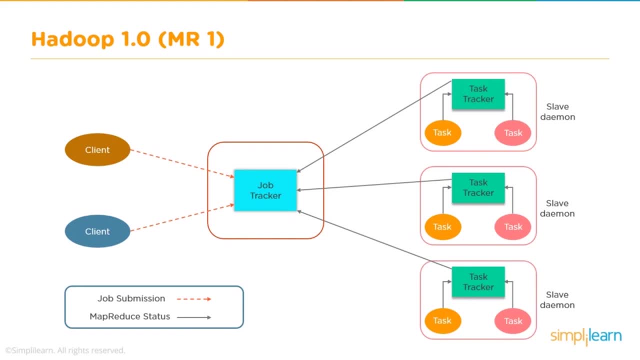 to the job tracker, which would then be knowing how many resources. and when we talk about resources, we are talking about the cpu cores, we are talking about the ram which would be available on every node. so task trackers would be sending in their resource information to job tracker and your job. 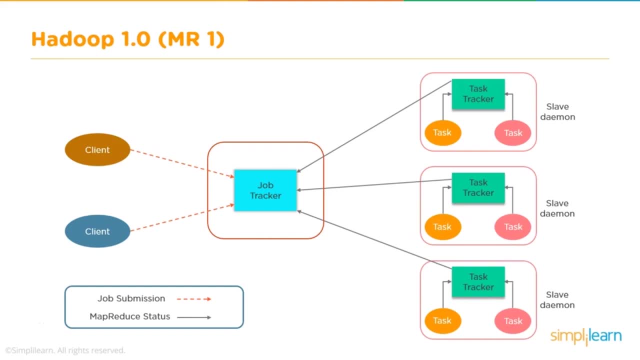 tracker would be already aware of what amount of resources are available on a particular node, how loaded a particular node is, what kind of work could be given to the task tracker. so job tracker was taking care of resource management and it was also breaking the application into tasks and doing the job scheduling part. assign different tasks to these slave demons. 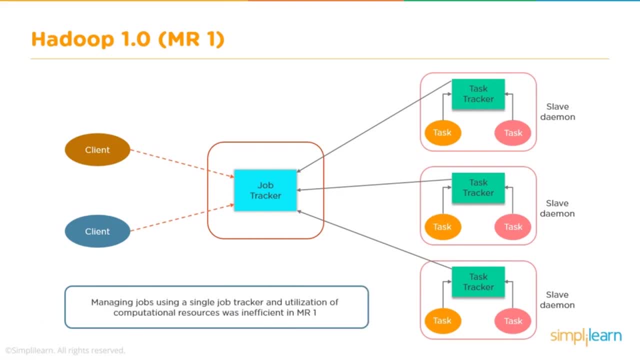 that is, your task trackers. so job tracker was eventually overburdened, right, because it was managing jobs, it was tracking the resources from multiple task trackers and basically it was taking care of job scheduling. so job tracker would be overburdened and in a case of overburdened job, 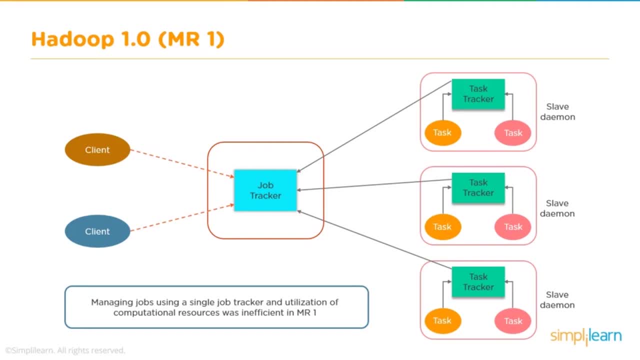 if job tracker would fail, then it would affect the overall processing. so if the master is killed, if the master demand dies, then the processing cannot proceed. now, this was one of the limitations of hadoop version 1.. so when you talk about scalability, that is the capability. 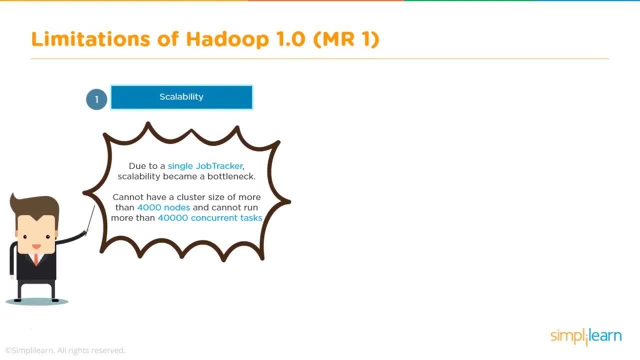 to scale due to a single job tracker, scalability would be hitting a bottleneck. you cannot have a cluster size of more than four thousand nodes and cannot run more than forty thousand concurrent tasks. now, that's just a number. we could always look into the individual resources which each 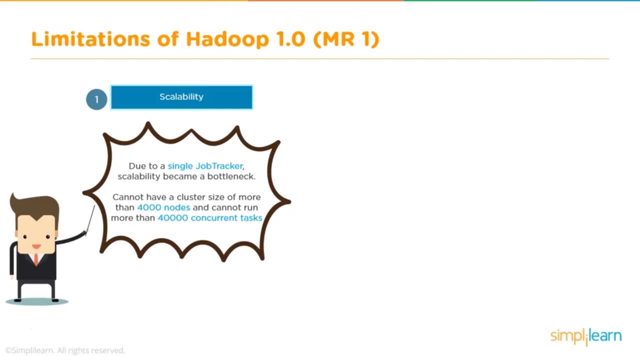 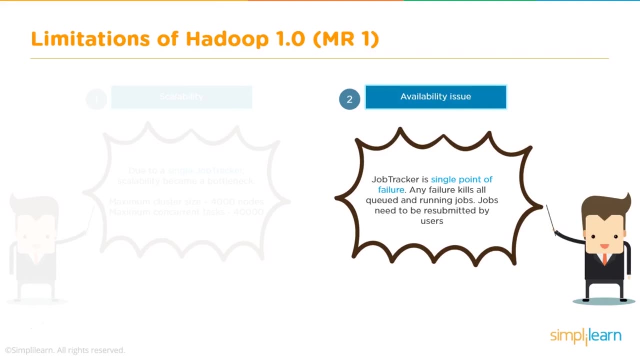 machine was having and then we can come up with an appropriate number. however, with a single job tracker, there was no horizontal scalability for the processing layer because we had single processing master. now, when we talk about availability, job tracker, as i mentioned, would be a single point of failure. now, any failure kills all the queued and running jobs and jobs would. 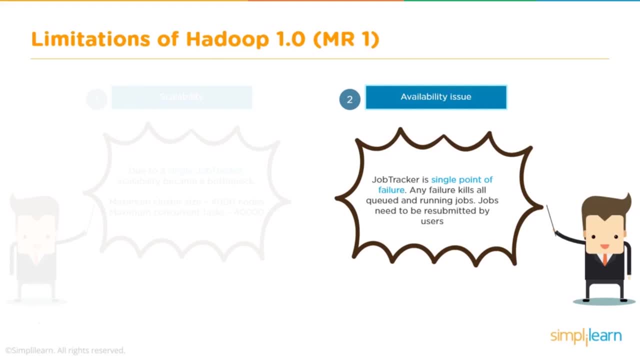 have to be resubmitted. now why would we want that? in a distributed platform, in a cluster which has hundreds and thousands of machines? we would want a processing layer which can handle huge amount of processing, which could be more scalable, which could be more available and could handle different kind of 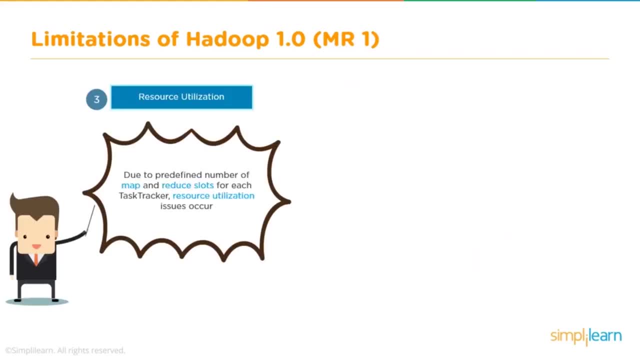 workloads when it comes to resource utilization. now, if you would have a predefined number of map and reduce slots for each task tracker, you would have issues which would relate to resource utilization, and that, again, is putting a burden on the master which is tracking these resources, which has to 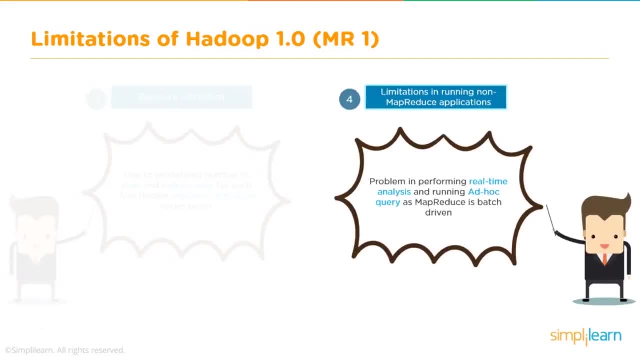 assign jobs which can run on multiple machines in parallel. so limitations in running non-map reduce applications. now that was one more limitation of hadoop version one and map reduce that the only kind of processing you could do is map reduce and map reduce programming model. although it is good, it is oldest, it has matured over a period of time, but then it is. 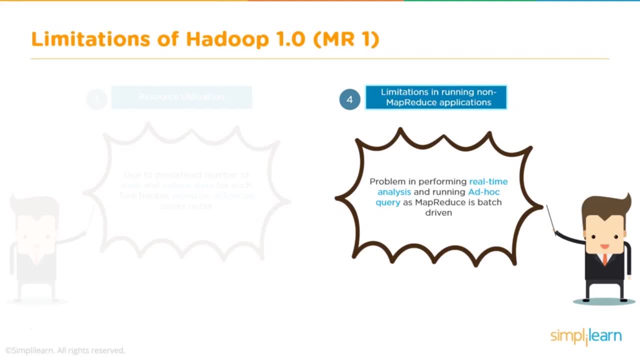 very rigid, you will have to go for mapping and reducing approach, and that was the only kind of processing which could be done in hadoop version one. so when it comes to doing a real-time analysis or doing ad hoc query, or doing a graph based processing or massive parallel processing, 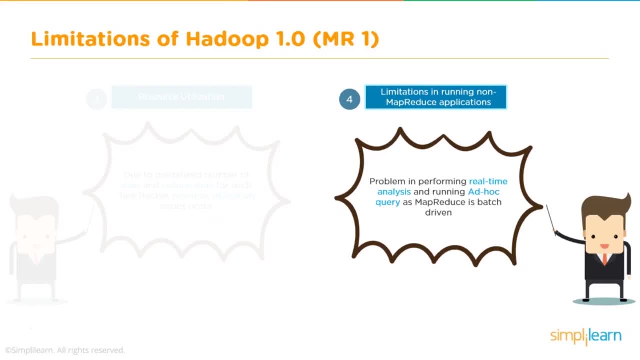 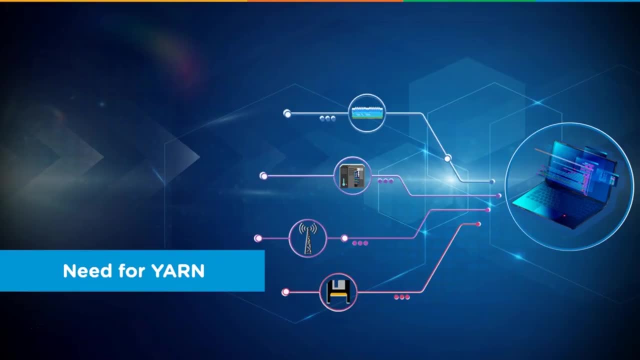 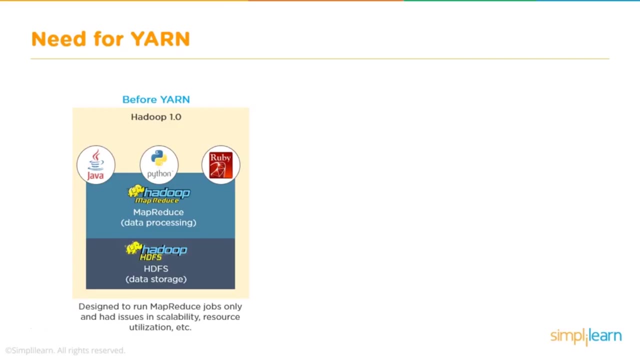 there were limitations because that could not be done in hadoop version one, which was having map reduce version one as the processing component. now that brings us to the need for yarn. so yarn, it stands for yet another resource negotiator. so, as i mentioned before, yarn in hadoop. 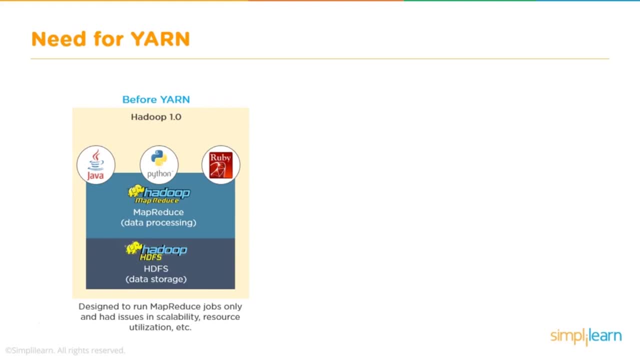 version one. well, you could have applications which could be written in different programming languages, but then the only kind of processing which was possible was map reduce. we had the storage layer, we had the processing, but then kind of limited processing which could be done. now this was one thing which brought in a thought that why shouldn't we have a 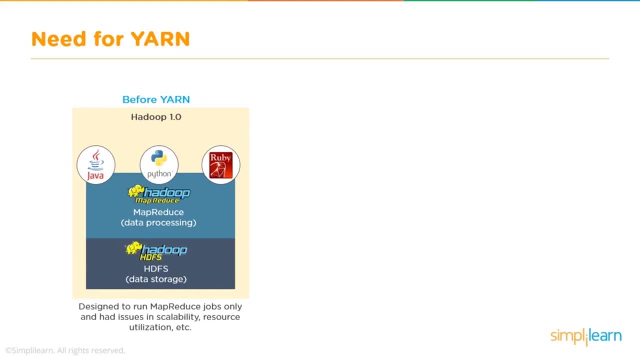 processing layer which can handle different kind of workloads, as i mentioned. might be graph processing, might be real-time processing, might be massive parallel processing or any other kind of processing which would be a requirement of an organization now designed to run map, reduce jobs only and having issues in scalability, resource utilization, job tracking, etc. that led to the need. 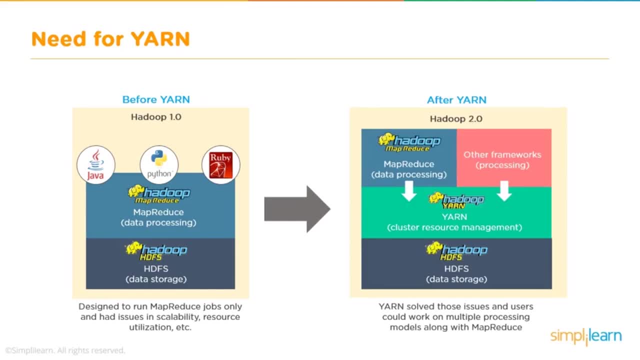 of something what we call as yarn. now, from hadoop version 2 onwards, we have the two main layers have changed a little bit. you have the storage layer, which is intact, that is your sdfs, and then you have the processing layer, which is called yarn- yet another resource. 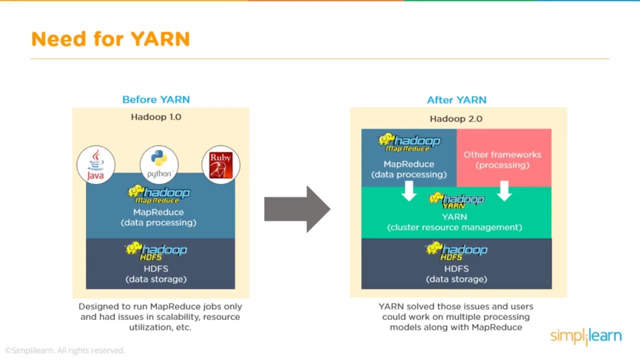 negotiator. now we will understand how yarn works. but then yarn is taking care of your processing layer. it does support map reduce. so map reduce processing can still be done, but then now you can have a support to other processing frameworks. yarn can be used to solve the issues which hadoop version 1 was posing, something like resource management, something like. 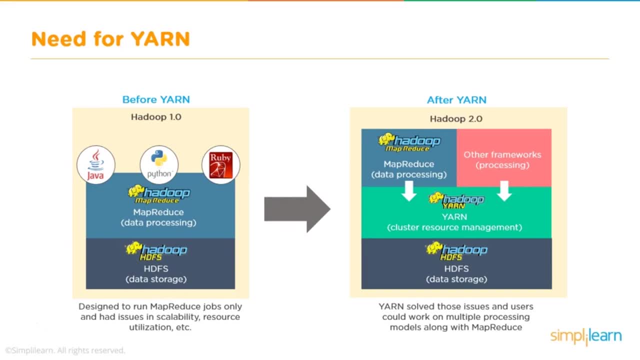 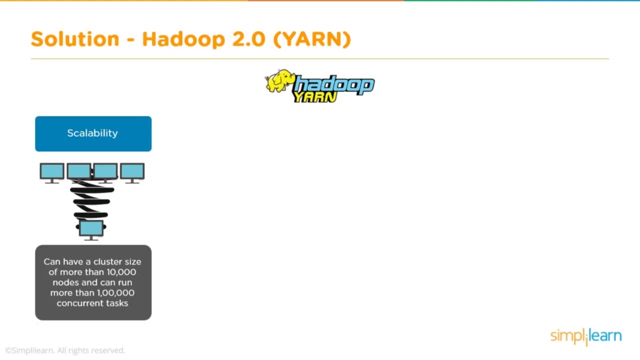 different kind of workload, processing something like scalability, resource utilization. all that is now taken care by yarn. now, when we talk about yarn, we can have now a cluster size of more than 10 000 nodes and can run more than 100 000 concurrent tasks. that's just to take care of. 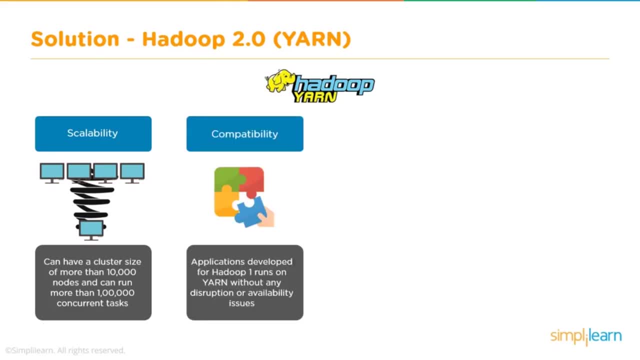 your scalability. when you talk about compatibility applications and which were developed for hadoop version 1, which were primarily map reduced kind of processing, can run on yarn without any disruption or availability issues. when you talk about resource utilization, there is a mechanism which takes care of dynamic allocation of cluster. 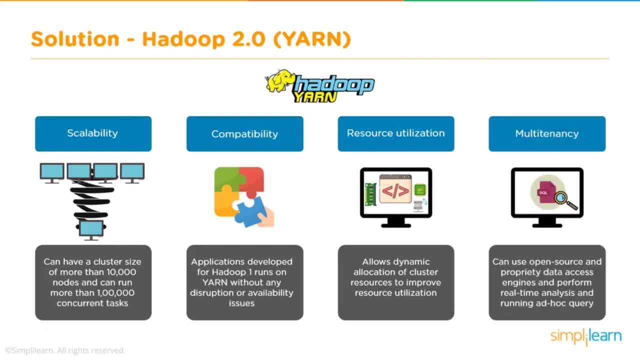 resources and this basically improves the resource utilization when we talk about multi-tenancy. so basically now the cluster can handle different kind of workloads, so you can use open source and proprietary data access engines, you can perform real-time analysis, you can be doing graph processing, you can be doing ad-hoc querying, and this can be supported for multiple workloads. 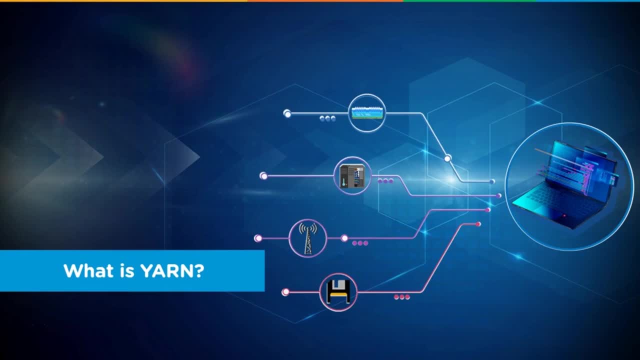 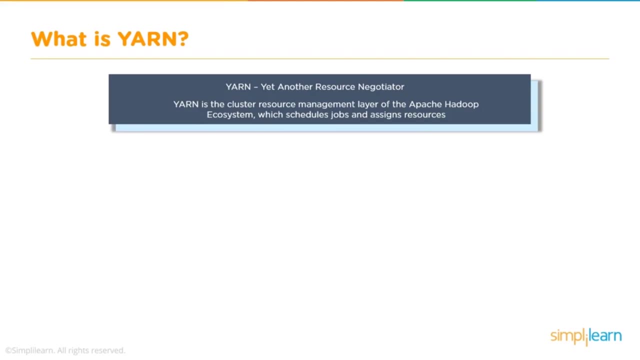 which can run in parallel. so this is what yarn offers. so what is yarn? as i mentioned, yarn stands for yet another resource negotiator, so it is the cluster resource management layer for your apache hadoop ecosystem which takes care of scheduling jobs and assigning resources. now just imagine when you would want to run a particular application. you would basically be: 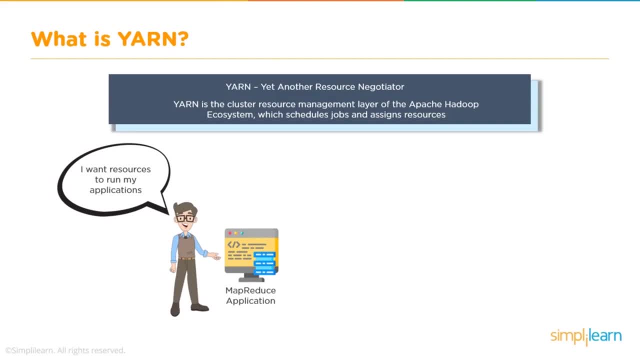 telling the cluster that i would want resources to run my applications. that application might be a map reduce application that might be a hive query which is triggering a map reduce. that might be a pig script which is triggering a map reduce that could be hive, with days as an execution engine. 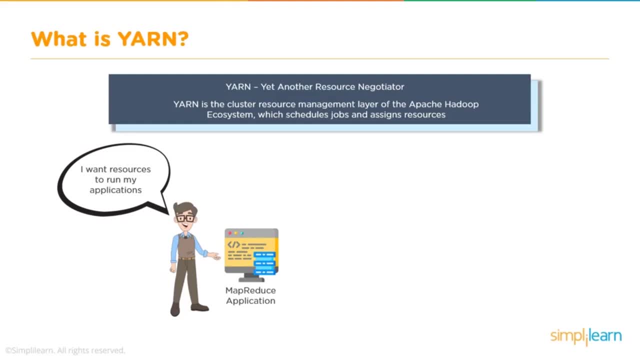 that could be a spark application, that could be a graph processing application. in any of these cases, you would still you as, in in sense, client, or basically an api, or the application would be requesting for resources. yan would take care of that, so yarn would provide the desired resources. 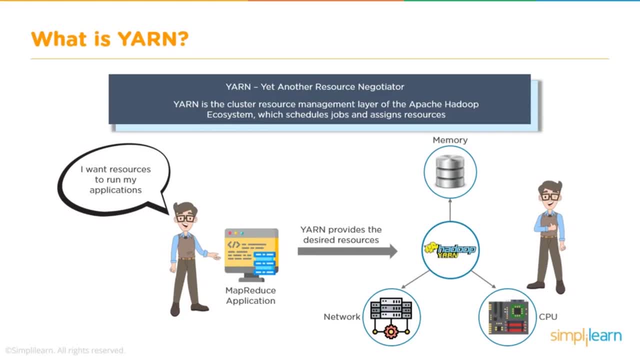 now, when we talk about resources, we are mainly talking about the network related resources. we are talking about the cpu course or, as in terms of yan we say virtual cpu course, we would talk about ram that is in gb or mb. when we talk about a virtual 아니라 application, when we talk about a 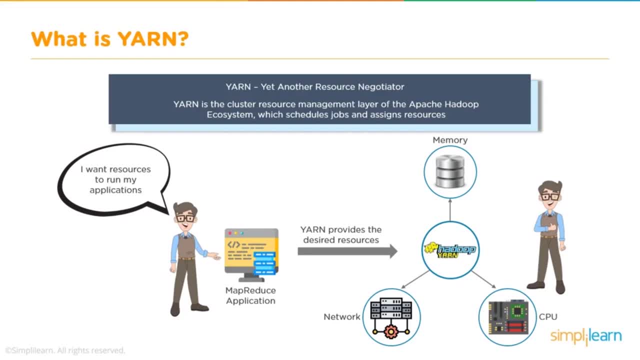 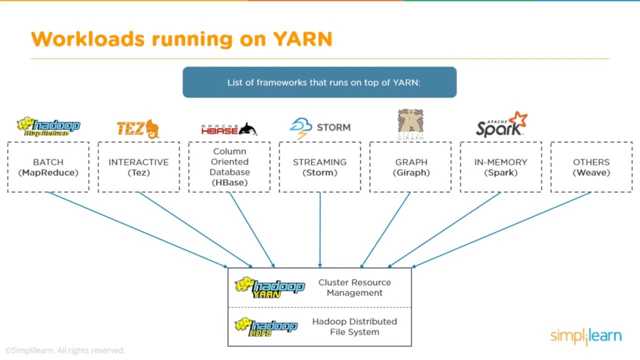 MB or in terabytes, which would be offered from multiple machines, and Yarn would take care of this. So with Yarn you could basically handle different workloads. Now these are some of the workloads which are showing up here. You have the traditional MapReduce, which is mainly batch. 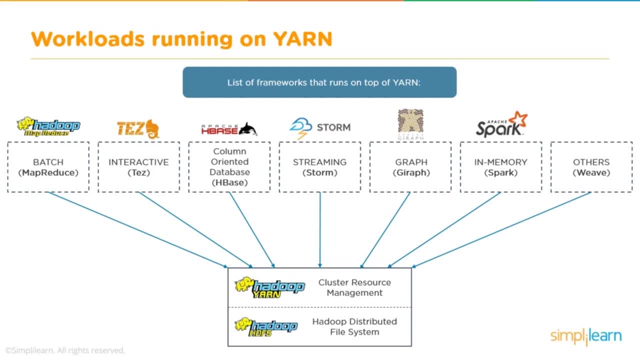 oriented. You could have an interactive execution engine, something as Tase. You could have HBase, which is a column oriented or a four dimensional database, And that would be not only storing data on SDFS but would also need some kind of processing. You could have streaming functionalities. 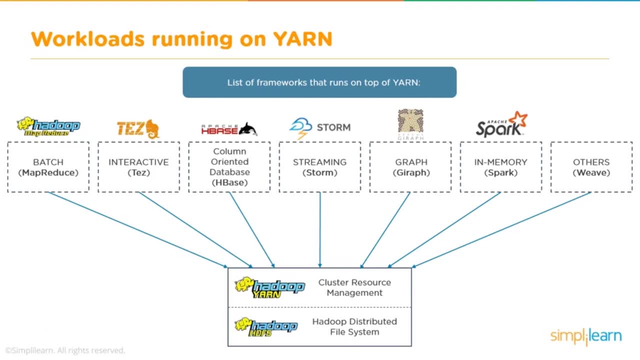 which would be from Storm or Kafka or Spark. You could have graph processing, You could have in-memory processing, such as Spark and its components, and you could have many others. So these are different frameworks which could now run and which can run on top of Yarn. 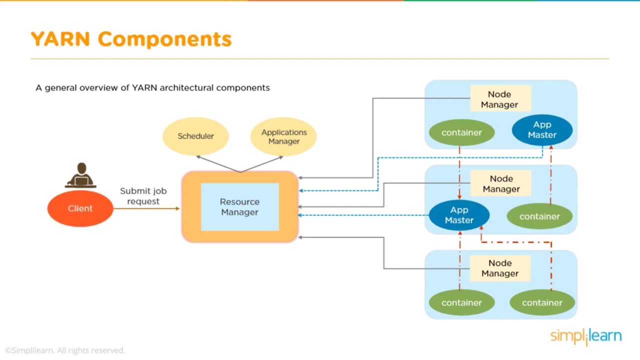 So how does Yarn do that? Now, when we talk about Yarn, this is how a overall Yarn architecture looks. So at one end you have the client. Now client could be basically your edge node, where you have some applications which are running. It could be an API which would want to interact with your cluster. 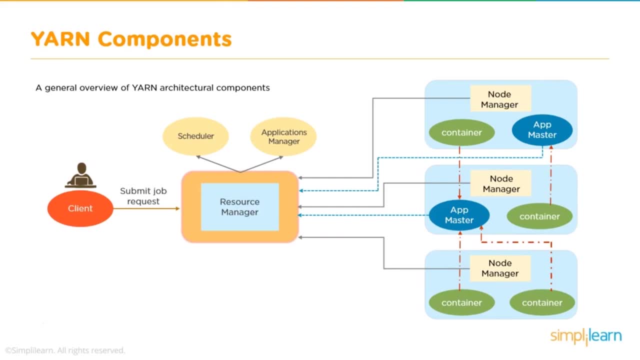 It could be a user triggered application which wants to run some jobs, which are doing some processing, So this client would submit a job request. Now what is the resource manager doing? Resource manager is the master of your processing layer. In Hadoop version one, we basically had job. 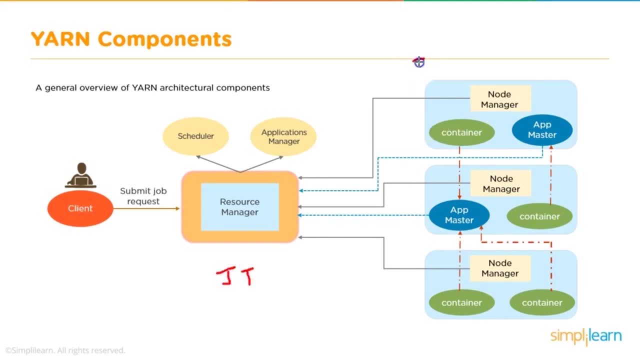 tracker. And then we had task trackers which were running on individual nodes. So your task trackers were sending your heartbeats to the job tracker, Your task trackers were sending it their resource information And job tracker was the one which was tracking the resources and it was doing. 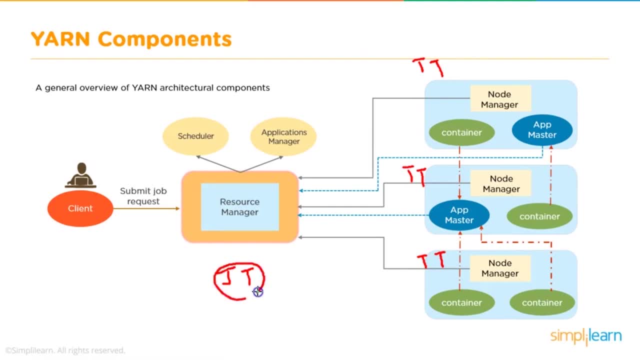 the job scheduling And that's how, as I mentioned earlier, job tracker was overburdened. So job tracker is now replaced by your resource manager, which is the master of your processing layer. Your task trackers are replaced by node managers, which would be then running on every node, And we 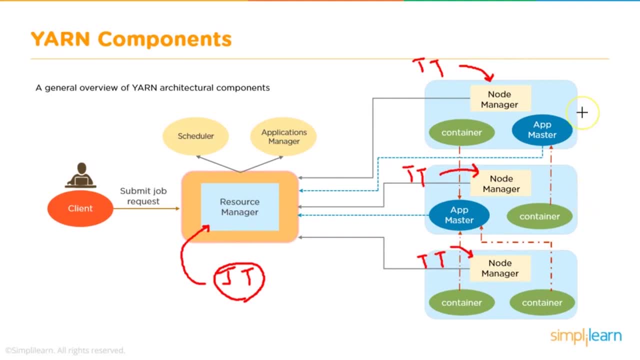 have a temporary daemon, which you see here in blue, and that's your app master. So this is what we mentioned when we say yet another resource negotiator. So app master would be existing in a Hadoop version two. Now, when we talk about your resource manager, resource manager is the master. 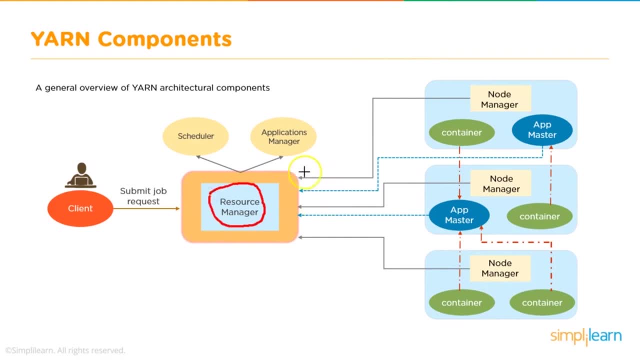 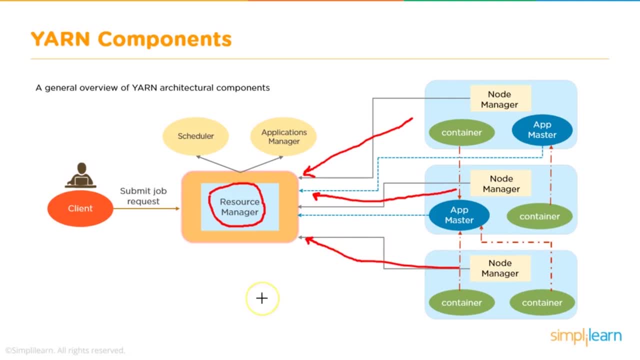 not only updating their status, but they are also giving an information of the amount of resources they have. Now, when we talk about resources, we should understand that if I'm talking about this node manager, then this has been allocated some amount of RAM for processing. 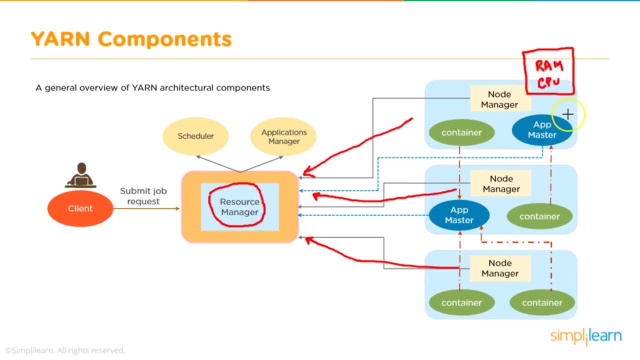 And some amount of CPU cores, And that is just a portion of what the complete node has. So if my node has, say, imagine my node has around 100 GB RAM and I have, say, 60 cores, all of that 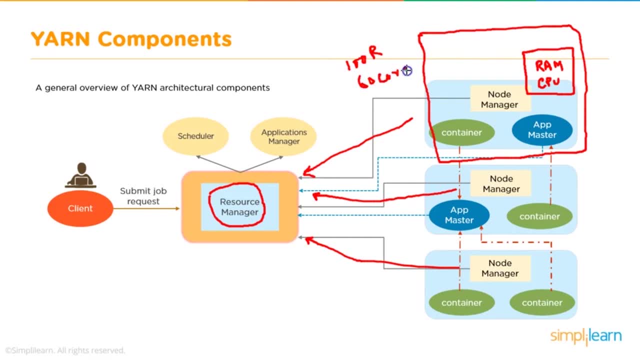 cannot be allocated to node manager. So node manager is just one of the components of Hadoop ecosystem. It is the slave of the processing layer. So we could say, keeping in all the context, such as different services which are running might be Cloudera or Hortonworks-related, 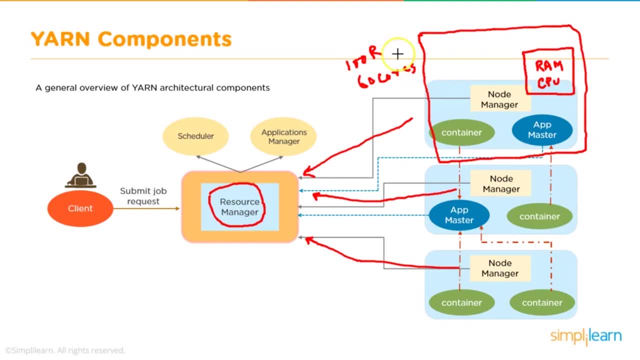 services running system processes running on a particular node. Some portion of this would be assigned to node manager for processing. So we could say, for example, say 60 GB RAM per node and say 40 CPU cores. So this is what is allocated for the node manager on every machine. 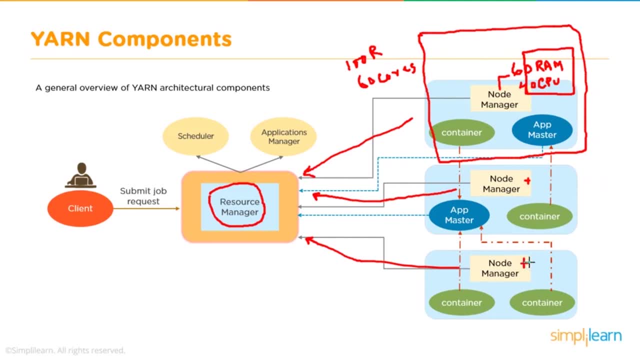 Similarly we would have here. Similarly we would have here. node manager is constantly giving an update to resource manager about the resources, what it has. probably there might be some other applications running and node manager is already occupied, so it gives an update. now we also have a concept of containers which is basically we will, we will talk. 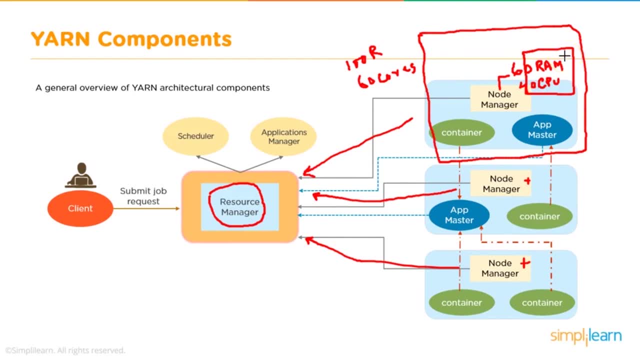 about, which is about these resources being broken down into smaller parts. so resource manager is keeping a track of the resources which every node manager has, and it is also responsible for taking care of the job request. how do these things happen now, as we see here, resource manager at a 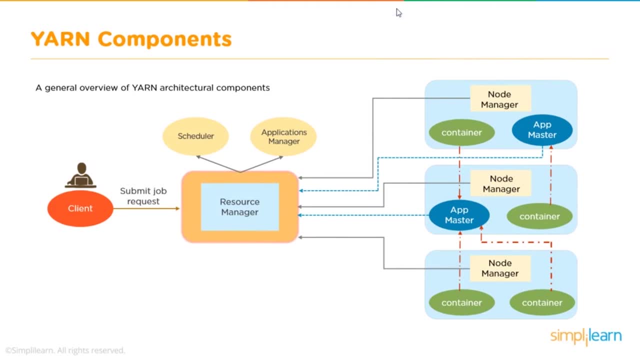 higher level. you can always say: this is the processing master which does everything, but in reality it is not the resource manager which is doing it, but it has internally different services or components which are helping it to do what it is supposed to do. now let's look further. now, as I mentioned, your resource manager has these services or components which 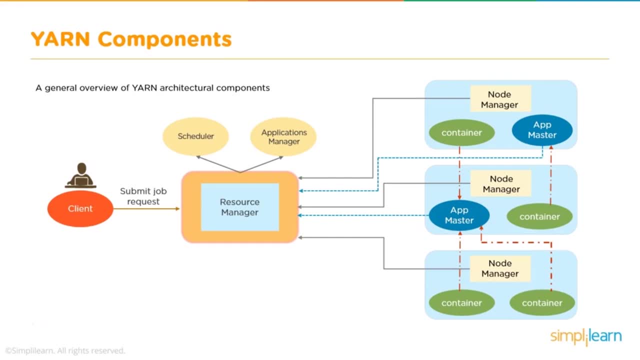 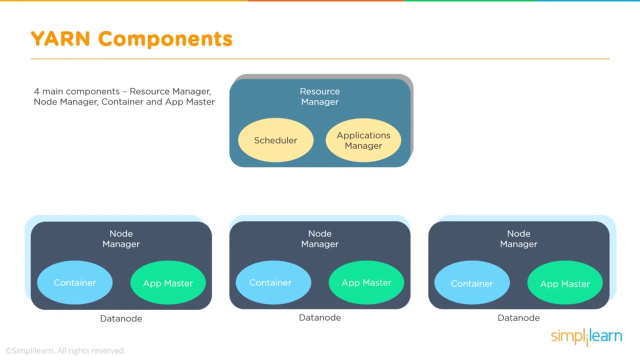 basically helps it to do the things. it is basically a, an architecture where multiple components are working together to achieve what yarn allows. so resource manager has mainly two components, that is, your scheduler and applications manager, and these are, at high level, four main components here. so we talked about resource manager, and resource manager are basically: 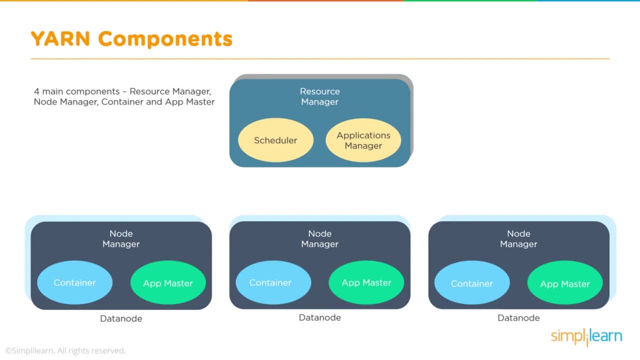 the processing master, which is the processing manager, which is the processing master. you have node managers, which are the processing slaves which are running on every nodes. you have the concept of container and you have the concept of application master. how do all these things work? now let's look. 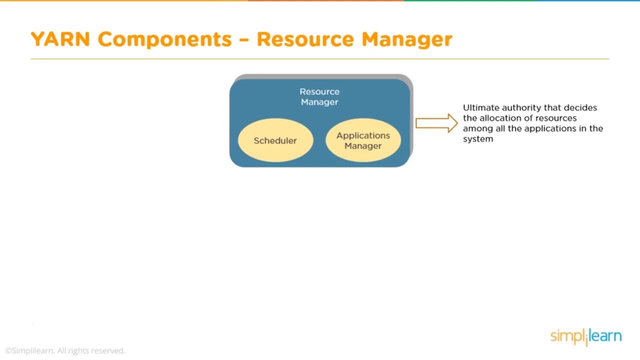 at yarn components. so resource manager basically has two main components, you can say, which assist resource manager in doing what it is capable of. so you have scheduler and applications manager. now there is, when you talk about resources, there is always a requirement for the applications which 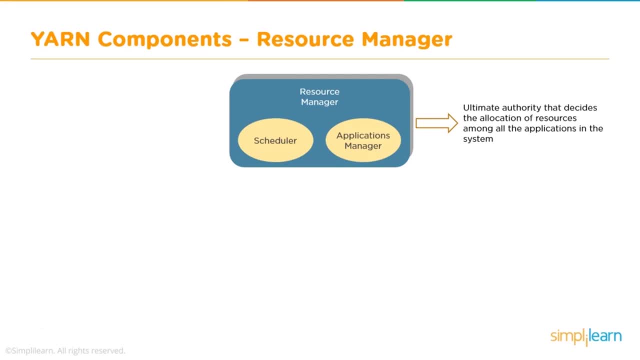 need to run on cluster of resources. So your application, which has to run, which was submitted by client, needs resources And these resources are coming in from multiple machines wherever the relevant data is stored and a node manager is running, So we always know that node manager is. 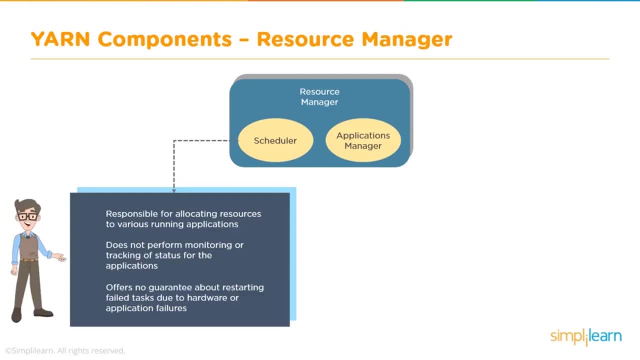 co-located with data nodes. Now, what does the scheduler do? So we have different kind of schedulers here. We have basically a capacity scheduler, we have a fair scheduler or we could have a FIFO scheduler. So there are different schedulers which take care of resource allocation. 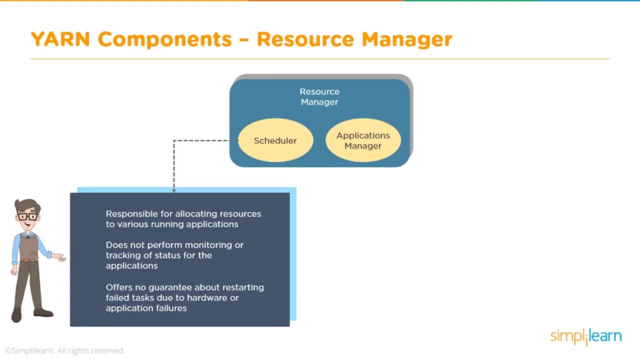 So your scheduler is responsible for allocating resources to various running applications. Now imagine a particular environment where you have different teams or different departments which are working on a particular application. So you have a scheduler which is responsible for allocating resources to various running applications. Now imagine a particular environment where you have 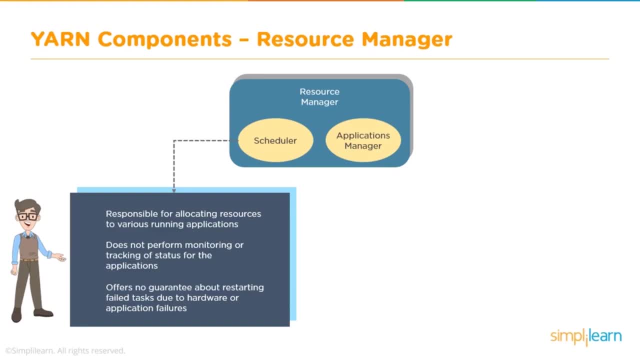 different teams or different departments which are working on the same cluster. So we would call the cluster as a multi-tenant cluster And on the multi-tenant cluster you would have different applications which would want to run simultaneously accessing the resources of the cluster. How is? 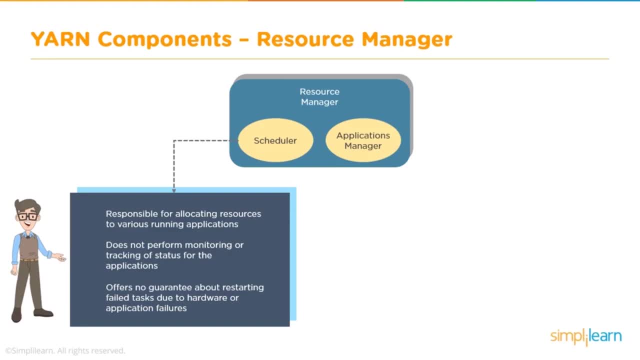 that managed. So there has to be some component which has a concept of pooling or queuing so that different departments or different users can get dedicated resources or can share resources on the cluster. So you have a cluster which is responsible for allocating resources to various running. 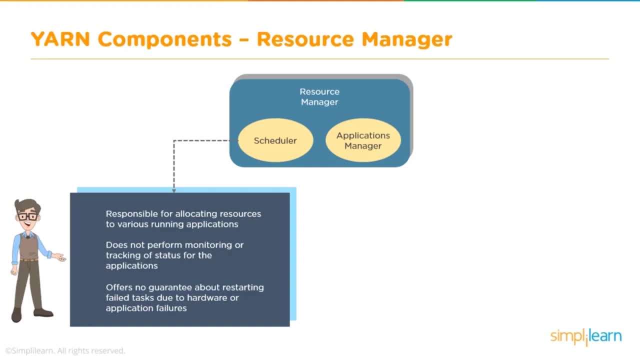 applications. So scheduler is responsible for allocating resources to various running applications. Now it does not perform monitoring or tracking of the status of applications. That's not the part of scheduler. It does not offer any guarantee about restarting the failed tasks due to hardware or network or any other failures. Scheduler is mainly responsible for allocating. 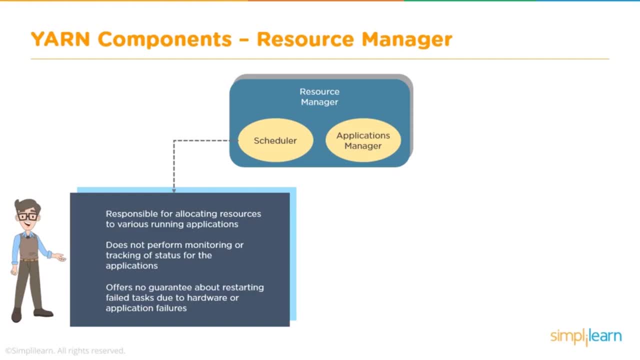 resources. Now, as I mentioned, you could have different kinds of schedulers. You could have a FIFO scheduler, which was mainly in older version of Hadoop, which stands for first in first out. You could have a fair scheduler, which basically means multiple applications could be running in the 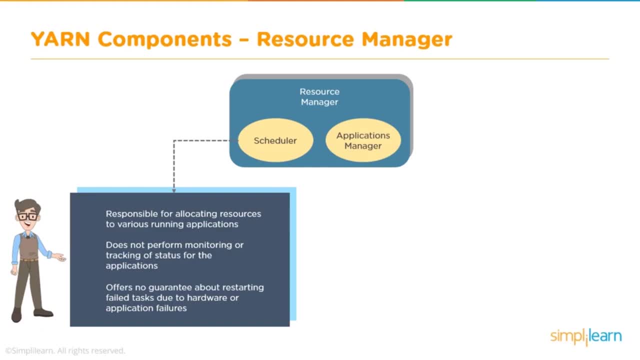 cluster and they would have a fair share of the resources. You could have a capacity scheduler, which would basically have dedicated or fixed amount of resources across the cluster. Now, whichever scheduler is being used, scheduler is mainly responsible for allocating resources. So scheduler is mainly responsible for allocating resources. Then it's your applications manager. 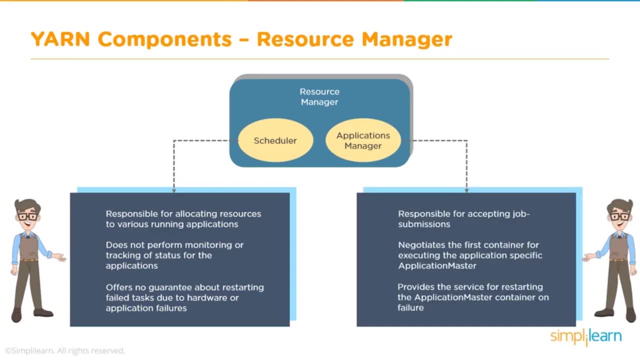 Now this is responsible for accepting job submissions. Now, as I said, at higher level, we could always say: resource manager state doing everything. It is allocating the resources, it is negotiating the resources, it is also taking care of listening to the clients and taking care of job submissions. But who is doing it in real? It is these components. So you have. 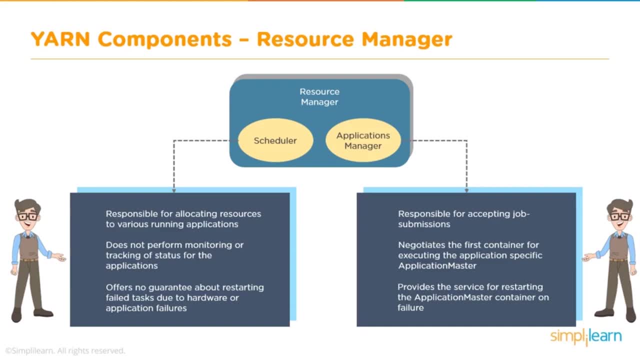 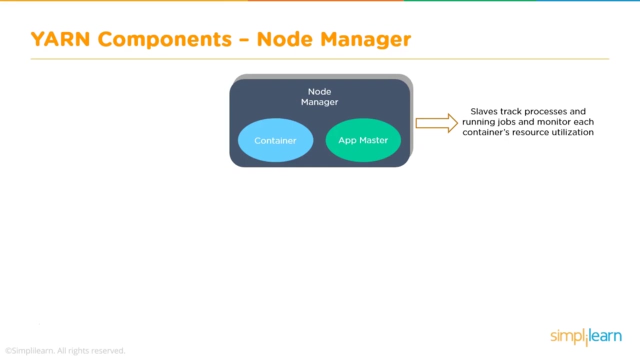 applications manager, which is responsible for accepting job submissions. It negotiates the first container for executing the application, specific application master. It provides the service for restarting the application master. Now, how does this work? How do these things happen in coordination? Now, as I said, your node manager is the slave process which would be running on every 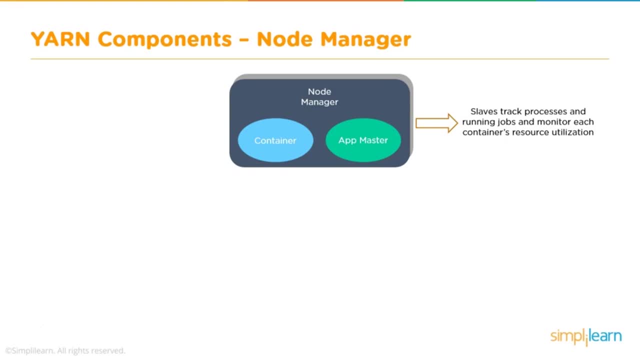 machine Slave is tracking the resources, what it has, it is tracking the processes, it is taking care of running the jobs And basically it is tracking each container resource utilization. So let's understand what is this container So normally when you talk about an application request which comes from a client. so 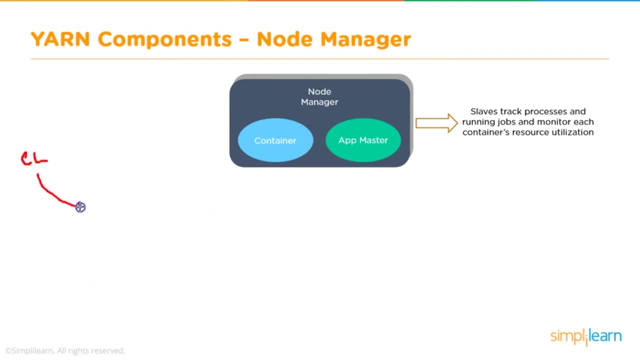 let's say this is my client which is requesting or which is coming up with an application which needs to run on the cluster. Now, this application could be anything. It first contacts your master, That's, your resource manager, which is the master for your processing layer. Now I 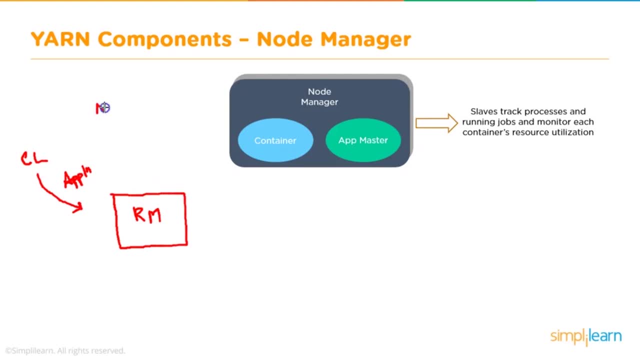 mentioned and as we already know that your name node, which is the master of your cluster, has the metadata in its RAM, which is aware of the data being split into blocks, The blocks when stored on multiple machines and other information. So obviously there was a interaction with the master. 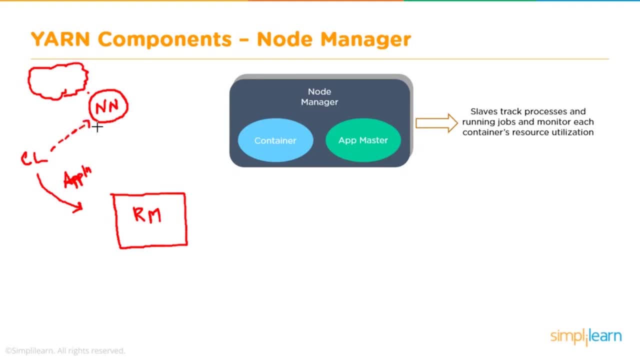 which has given this information of the relevant nodes where the data exists. Now for the processing layer. you need your client, basically the application which needs to run on the cluster, So your resource manager, which basically has the scheduler which takes care of allocating resources, and a 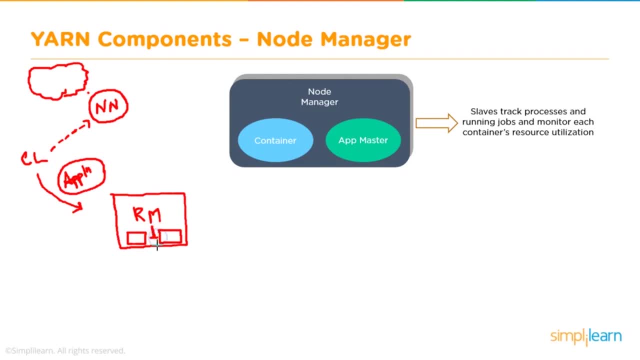 resource manager has mainly these two components which are helping it to do its work. Now for a particular application which might be needing data from multiple machines. Now we know that we would have multiple machines where we would have node manager running. we would have a data node running. 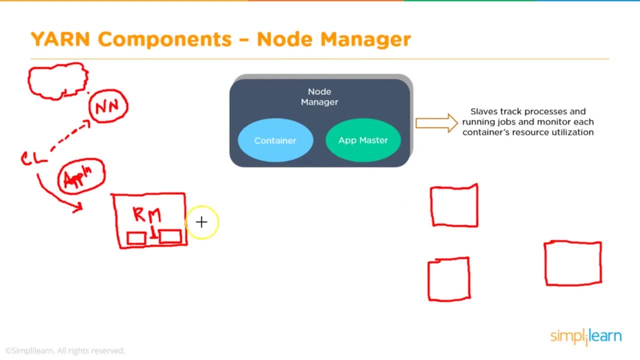 which could then be using that data node for storing the data on disk. The data nodes are responsible for storing the data on disk, So your resource manager has to negotiate the resources. Now, when I say negotiating the resources, it could basically ask each of these node managers for some amount of resources. For example, 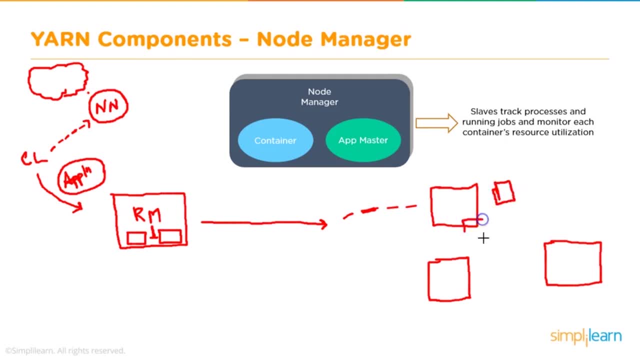 it would be saying: can I have one GB of RAM and one CPU core from you, because there is some data residing on your? have one GB and one CPU core from you. and this is again because some relevant data is stored and this request which resource manager makes of holding the resources, of total resources which 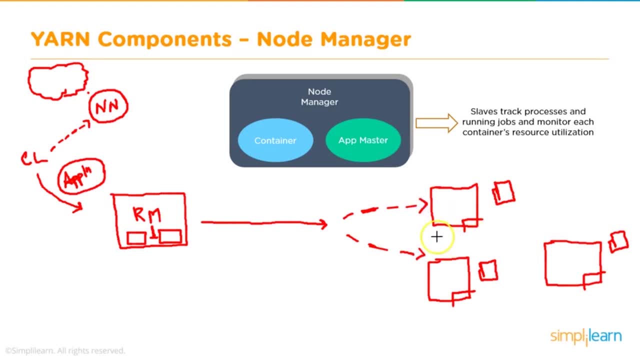 the node manager has. your resource manager is negotiating or is asking for resources from the processing slave, so this request of holding resources can be considered as a container. so resource manager- now we know it is not actually the resource manager, but it is the application manager which is negotiating the resources. so it negotiates the resources which are called. 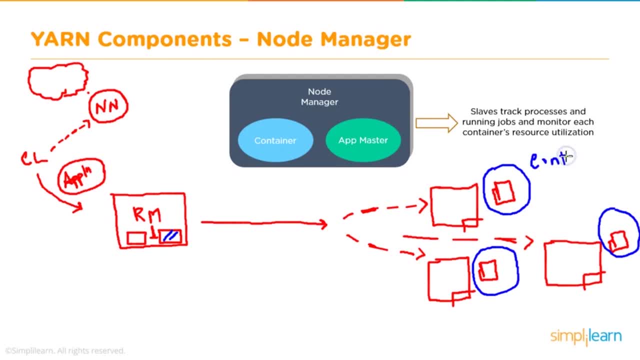 container. so this request of holding resource can be considered as a container. so basically, a container can be of different sizes. we will talk about that in a few minutes. So resource manager negotiates the resources with node manager. now node manager, which is already giving an update of the resources it has, what amount of resources it holds, how much- busy it is. 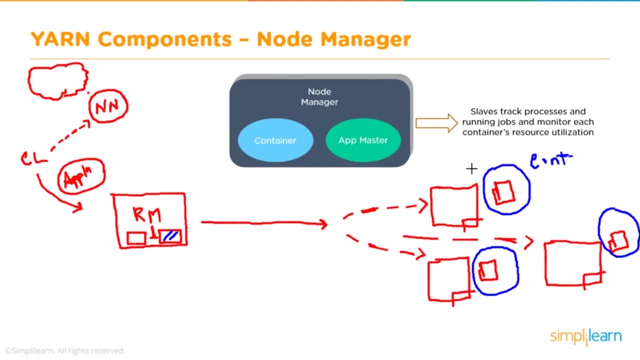 can basically approve or deny this request. so node manager would basically approve in saying yes, I could hold these resources, I could give you this container of this particular size Now, once the container has been approved or allocated- or you can say granted- by your node manager, resource manager now knows: 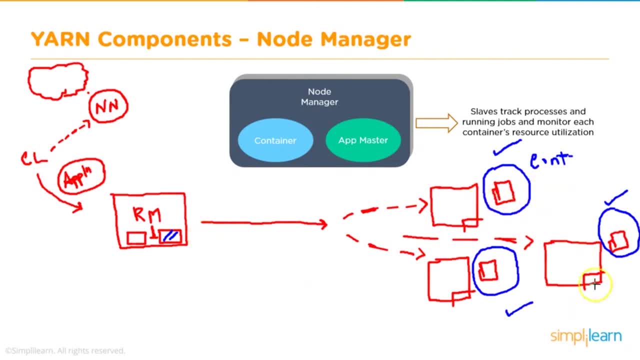 that resources to process the application are available and guaranteed by the node manager. so resource manager starts a temporary daemon called app master. so this is a piece of code which would also be running in one of the containers. it would be running in one of the containers which would then. 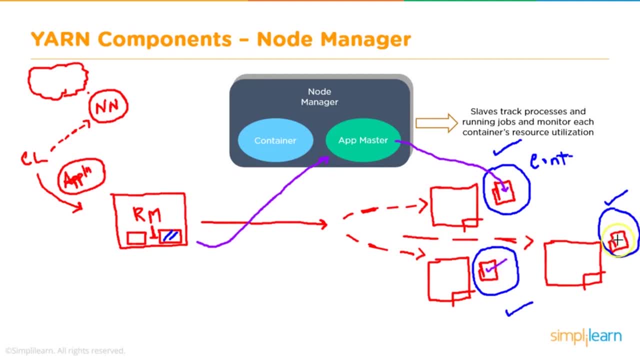 take care of execution of tasks in other containers. So your application master is per application. so I will have 10 different applications coming in from the client. Then we would have 10 app masters, one app master being responsible for per application. now what does this? 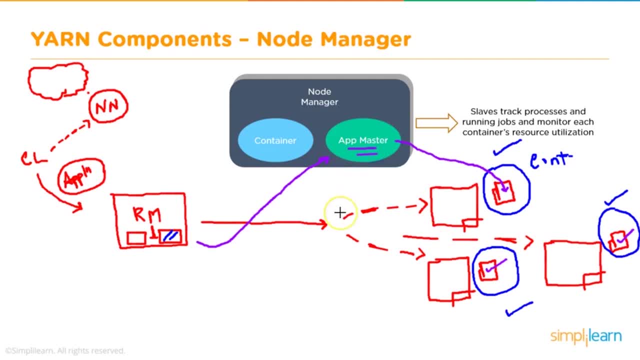 app master do it. basically is a piece of code which is the responsible for execution of the application. so your app master would run in one of the containers and then they wouldn't use the other container. so a container sits in one of responsible for working in a container. an app master will be able to work in the exchanges, so this would be done automatically. related to contents used for your process management, so you can control if you hold a container in any industry. you have others containers and so your application delight from execution of tasks in yource container. 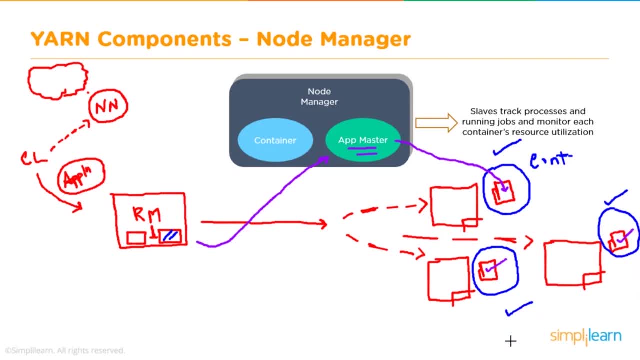 which node manager is guaranteed that it will give when the request application request comes to it. and using these containers, the app master will run the processing tasks within these designated resources. so it is mainly the responsibility of application master to get the execution done and then communicate it to the master. so resource manager is tracking the 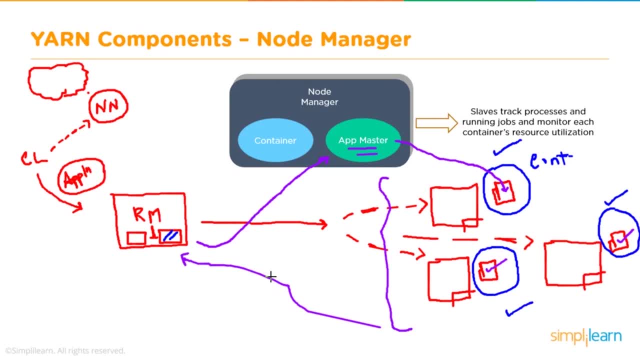 resources. it is negotiating the resources and once the resources have been negotiated, it basically gives the control to application master. application master is then running within one of the containers, on one of the nodes and using the other containers to take care of execution. this is how it looks. so, basically, container, as i said, is a collection of resources. 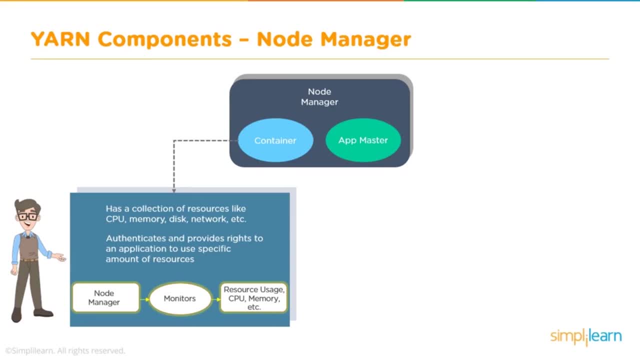 like cpu memory, your disk which would be used or which already has the data and network. so your node manager is basically looking into the request from application master and it basically is granting this request or basically is allocating these containers. now again we could have different sizing of the containers. let's take an example here. 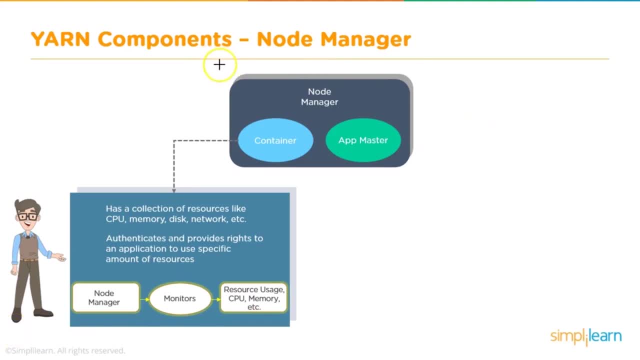 so, as i mentioned, from the total resources which are available for a particular node, some portion of resources are allocated to the node manager. so let's imagine this is my node, where node manager, as a processing slave, is running. so from the total resources which the node has, some portion of ram and cpu cores is basically allocated to the node manager. so i 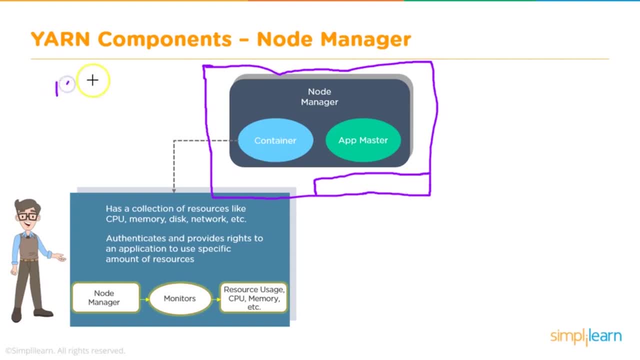 could say, out of total 100 gb ram, we can say around 60 cores which the particular node has. so this is my ram which the node has and these are the cpu cores which the node has, some portion of it, right, so we can say might be 70 percent or 60 percent of the total resources. 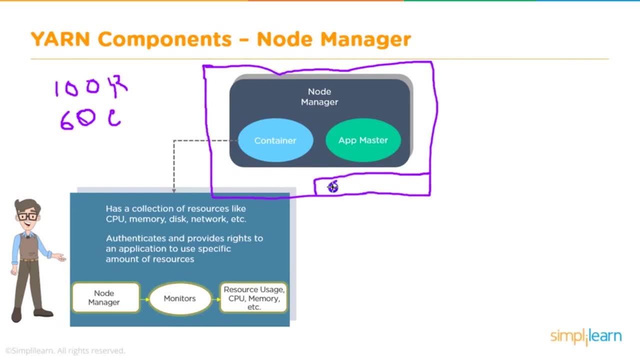 so we could say around 60 gb ram and then we could say around 40 v cores have been allocated to node manager. so there are these settings, which are given in the yarn hyphen site file. now, apart from this allocation, that is, 60 gb ram and 40 v cores, we also have some. 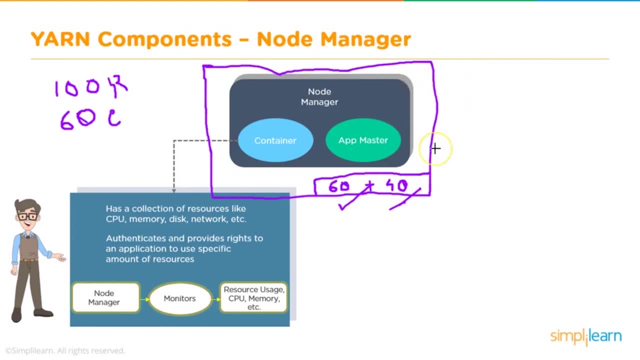 properties which say what will be the container sizes. so, for example, we could have a small container setting which could say: my every container could have 2 gb ram and say, one virtual cpu core. so this is my smallest container. so, based on the total resources you could. 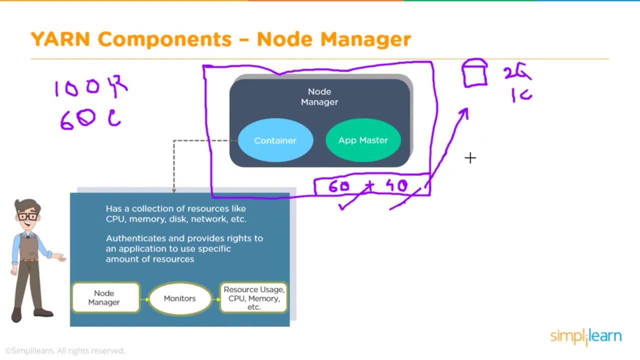 calculate the total resources and then you could calculate the total resources, which is how many such small containers could be running. so if i say 2 gb ram, then i could have around 30 containers, but then i'm talking about one virtual cpu core, so totally i could have around. 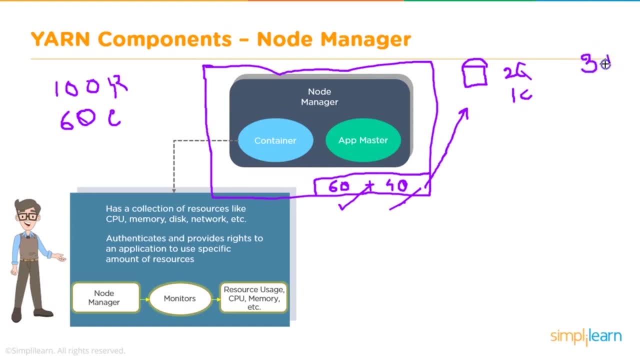 30 small containers which could be running in parallel on a particular node and as of that calculation, you would say 10 cpu cores are not being utilized. you could have a bigger container size which could say i would go for 2 cpu cores and 3 gb ram, and then i could have around. 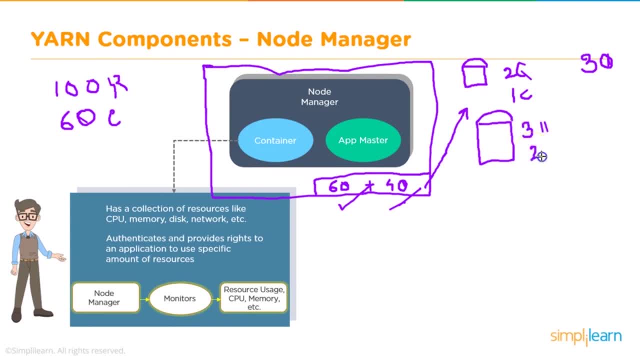 30 gb ram. so 3 gb ram and 2 cpu cores. so that would give me around 20 containers of bigger size. so this is the container sizing which is again defined in the yarn hyphen site file. so what we know is, on a particular node which has this kind of allocation either, we could have 30 small. 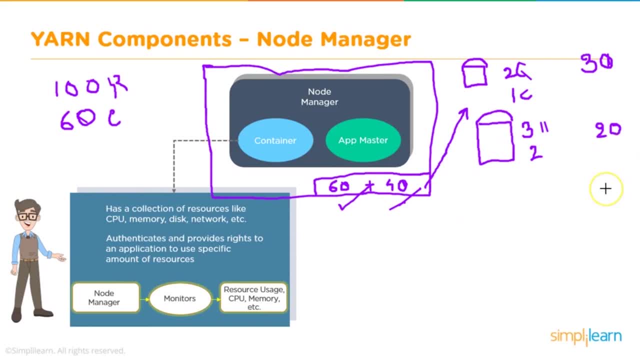 containers running, or we could have 20 big containers running and same would apply to multiple nodes. so node manager based on the request of the container size would be running rather than those kilometers ranging from an activities of maybe differentparameters to different Lithium rigs. so some technology backbone on developers could be running for. 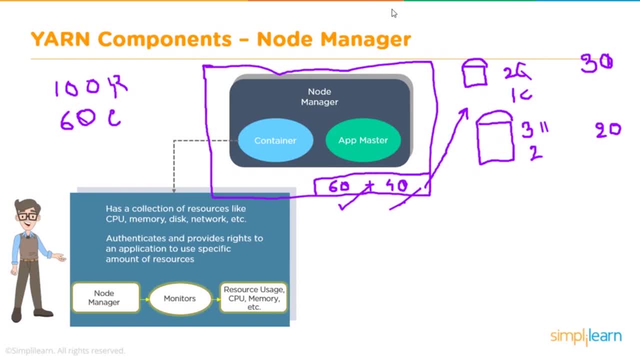 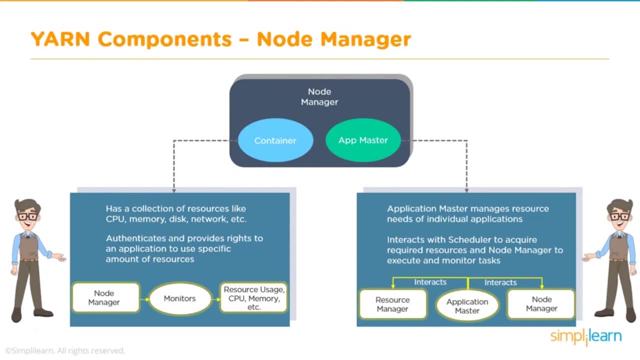 Remember, it is within this, one of these containers you would have an application master running and other containers would be used for your processing requirement. Application master, which is per application, it is the one which uses these resources. It basically manages or uses these resources for individual application. So remember, if we have 10 applications running, 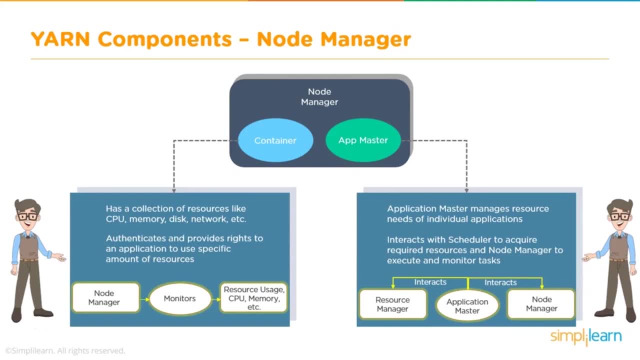 on yarn O rev. Master's one responsible for each application. your application master is the one which also interacts with the scheduler to basically know how much amount of resources could be allocated for one application, and your application master is the one which uses these resources, but it can never negotiate for. 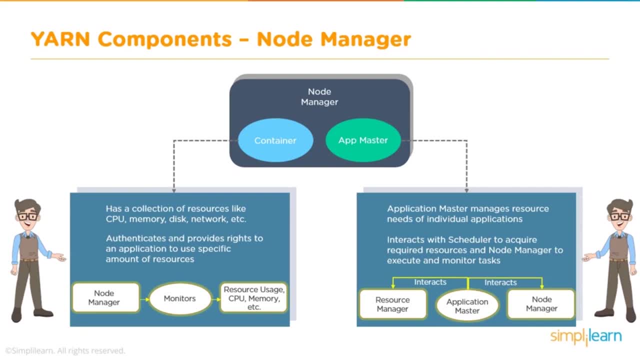 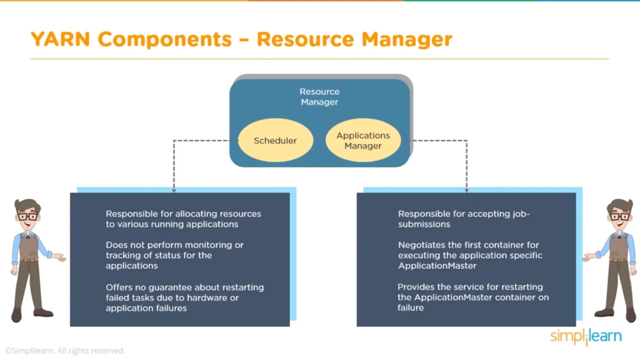 more resources to node manager. application master cannot do that. application master has to always go back to resource manager if it needs more resources. so it is always the resource manager- and internally resource managers- component, that is, application manager, which negotiates the resources at any point of time due to some node failures or due to any other. 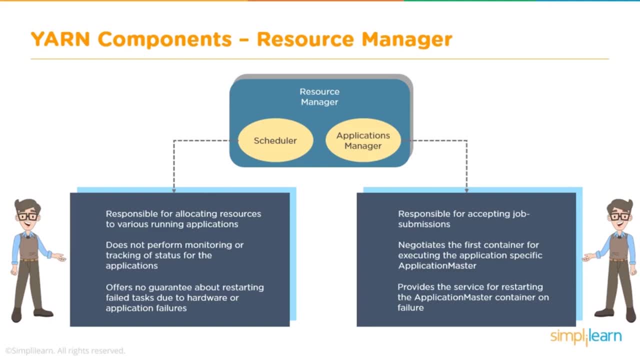 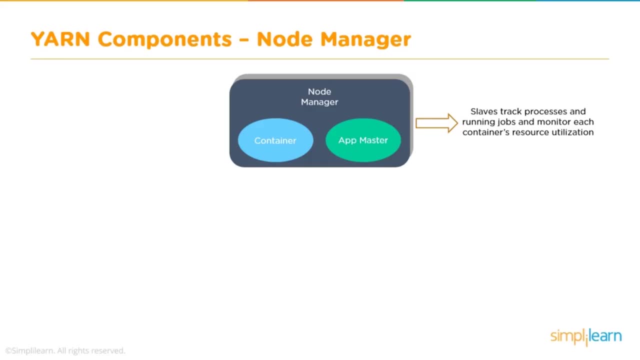 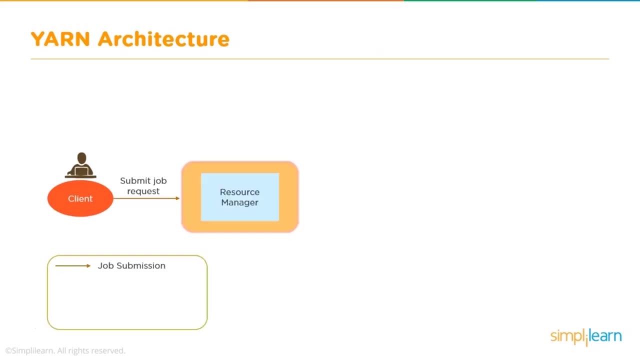 requirements. if application master needs more resources on one or multiple nodes, it will always be contacting the resource manager internally, the applications manager, for more containers. now this is how it looks. so your client submits the job request to resource manager. now we know that resource manager internally has scheduler and applications manager node. 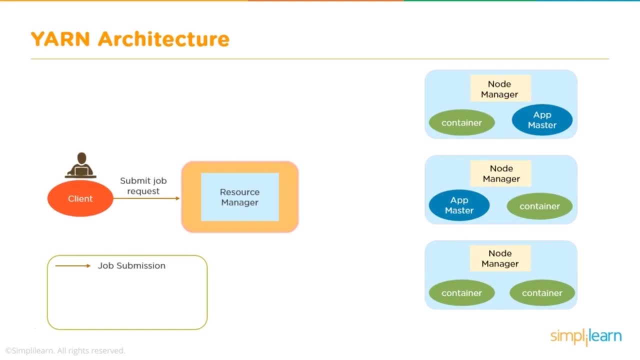 managers which are running on multiple machines are the ones which are tracking their resources, giving this information to resource manager so that resource manager, or I would say it's component applications manager, could request resources from multiple applications, multiple node managers. when i say request resources, it is these containers, so your resource manager. 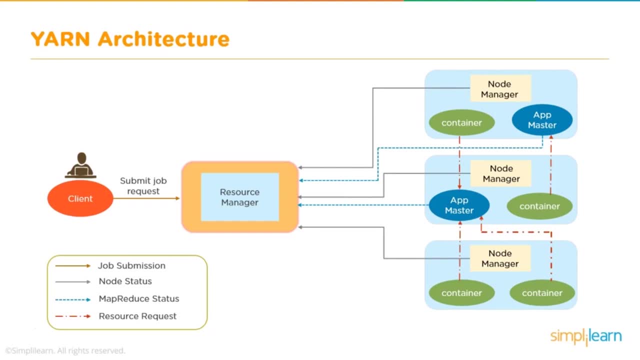 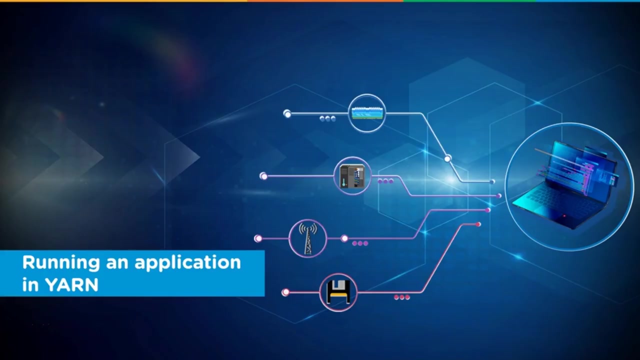 basically will request for the resources on one or multiple nodes. node manager is the one which approves these containers and once the container has been approved, your resource manager triggers a piece of code that is application master, which obviously needs some resources. so it would run in one of the containers and will use other containers to do the execution. so your client. 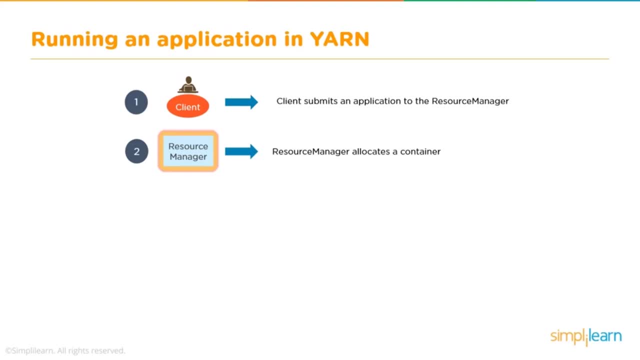 submits an application to resource manager, resource manager allocates a container. or i would say this is at a high level, right. resource manager is negotiating the resources. and internally, who is negotiating the resources? it is your applications manager who is granting this request, it is node manager, and that's how we can say: resource manager allocates a container. application master, basically. 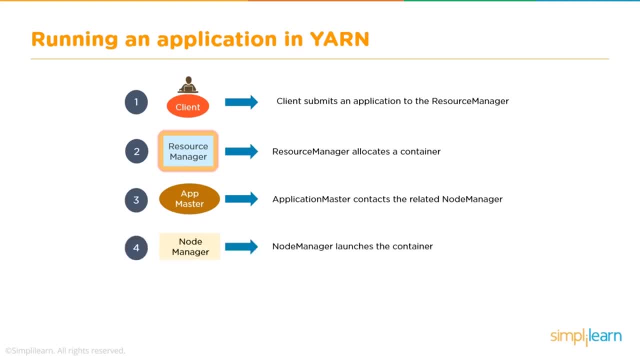 contacts the related node manager because it needs to use the containers. node manager is the one which launches the container or basically gives those resources within which an application can run. an application master itself will then accommodate itself in one of the containers and then use other containers for the processing, and it is within these containers the actual execution happens. 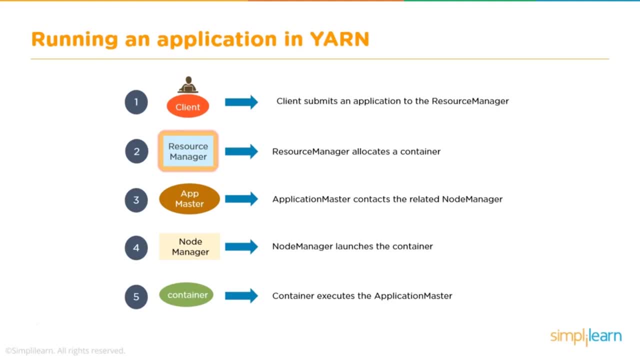 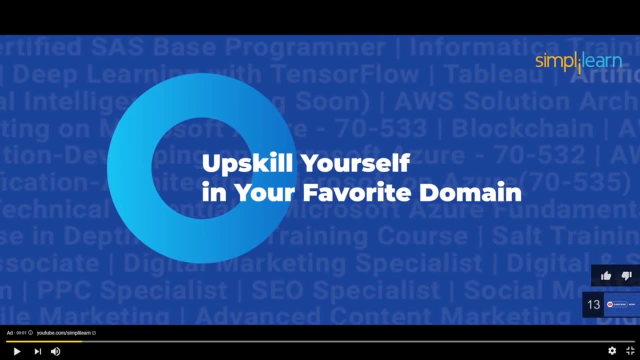 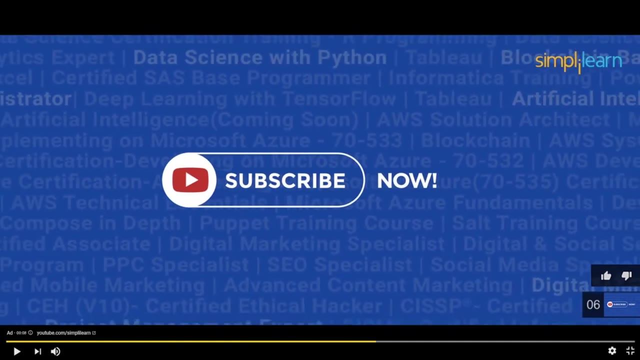 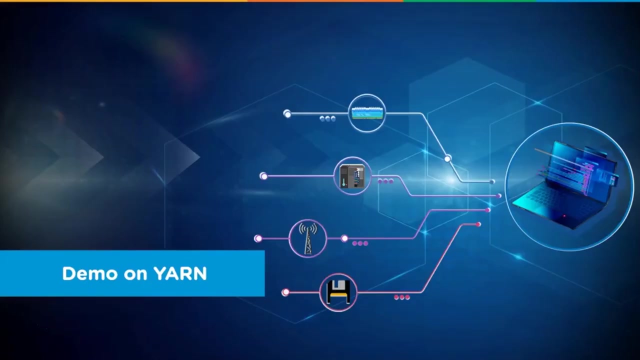 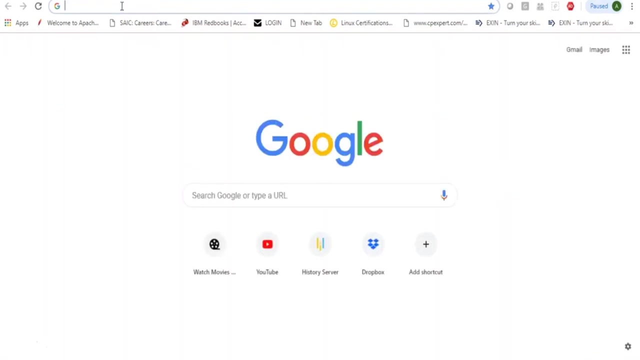 now that could be a map task, that could be a reduced task, that could be a spark executor taking care of spark tasks and many other processing. so before we look into the demo on how yarn works, i would suggest looking into one of the blogs from cloud era so you can just look for yarn untangling and this is: 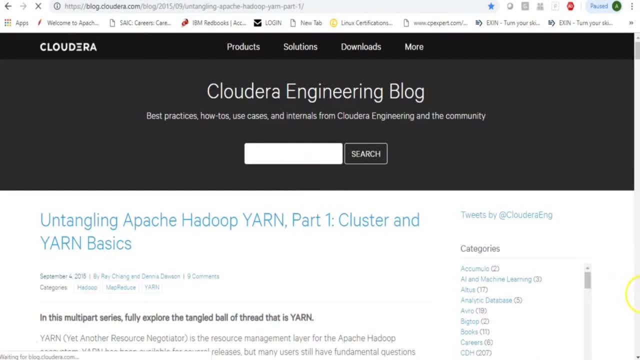 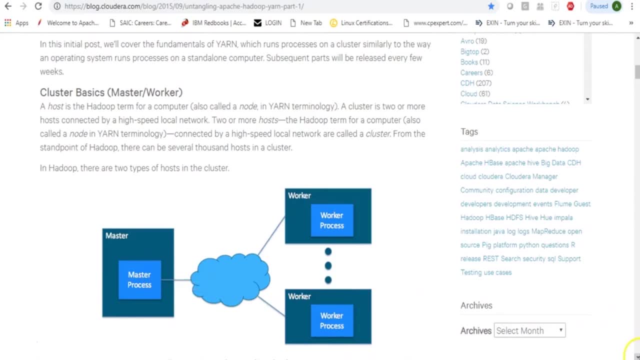 really a good way to get started. so let's get started with the demo. so let's get started with the demo. so this is really a good blog which basically talks about the overall functionality which i explained just now. so, as we mentioned here, so you basically have the master process, you have the 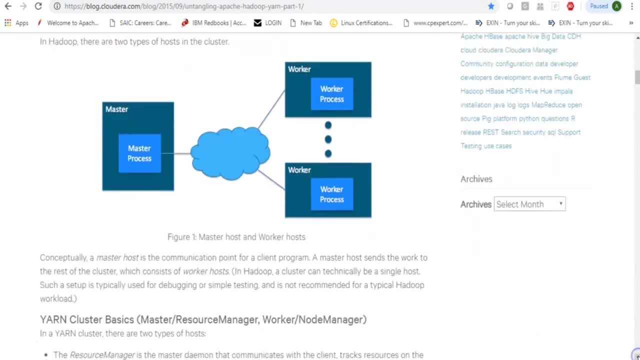 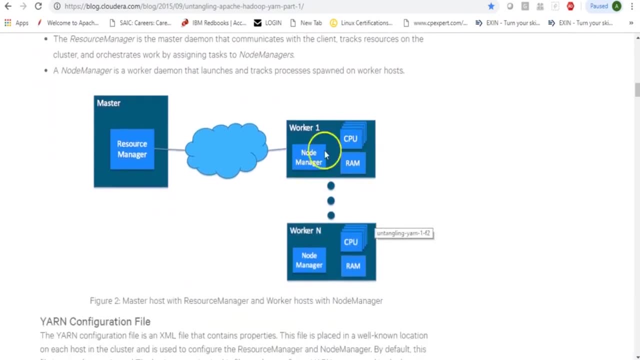 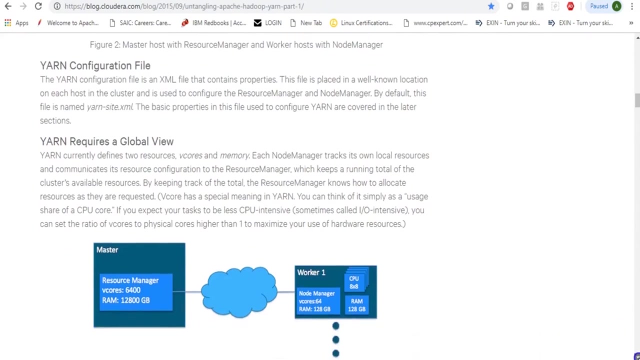 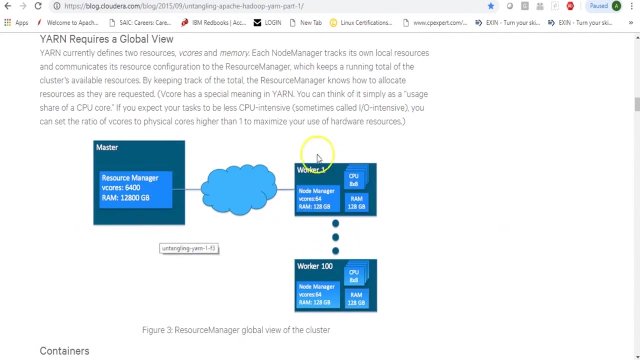 worker process which basically takes care of your processing, your resource manager being the master and node manager being the slave. this also talks about the resources which each node manager has. it talks about the yarn configuration file where you give all these properties. it basically shows you node manager which reports the amount of resources it has to resource manager. now remember: 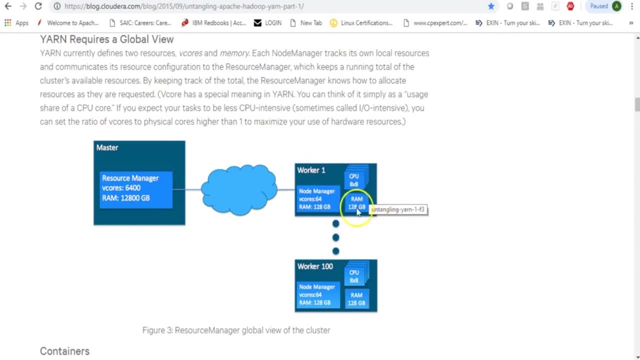 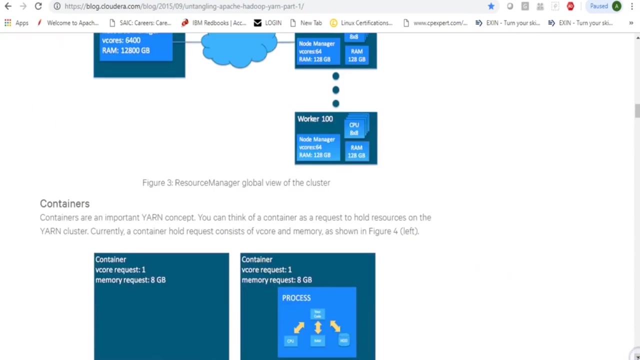 if worker node shows 8 into 8 cpu cores and 128 gb ram and if your node manager says 64 v course and ram 128 gb, then that's not the total capacity of your node. it is some portion of your node which is allocated to node manager. now, once your node manager reports that your 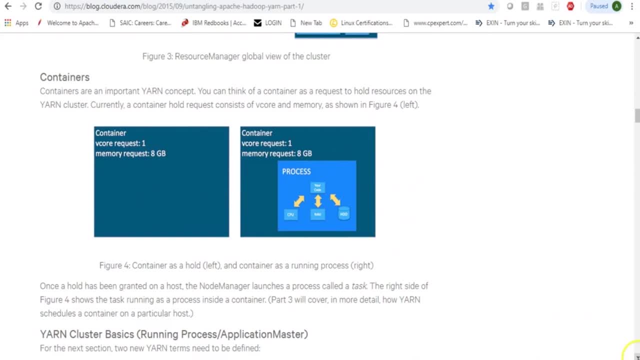 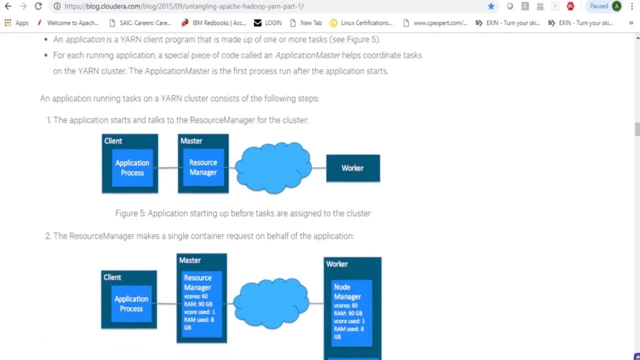 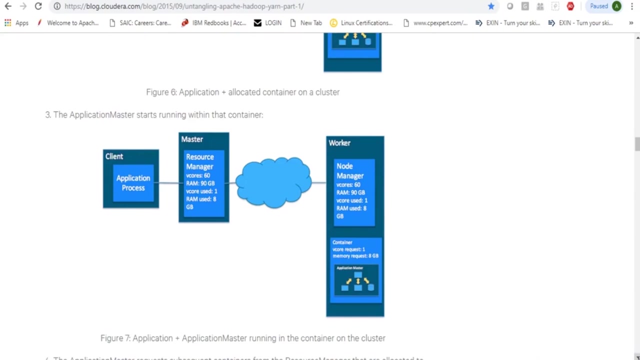 resource manager is requesting for containers based on the application. What is a container? It is basically a logical name given to a combination of vCore and RAM. It is within this container where you would have basically the process running. So once your application starts and once node manager is guaranteed these containers, your application. 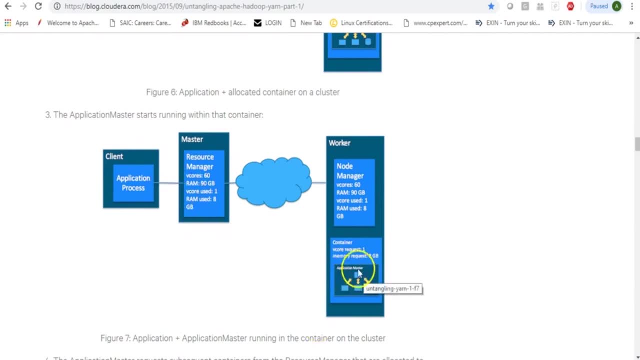 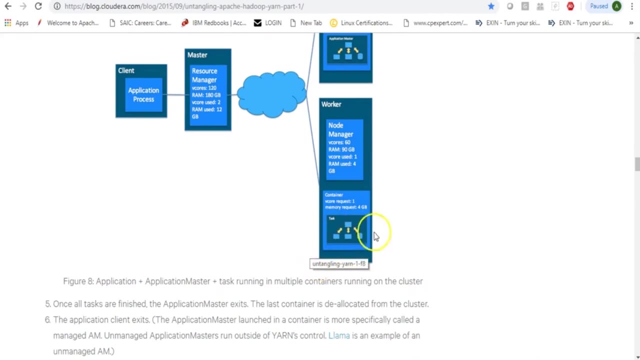 or your resource manager has basically already started an application master within the container, And what does that application master do? It uses the other containers where the tasks would run. So this is a very good blog which you can refer to, and this also talks about MapReduce, If you. 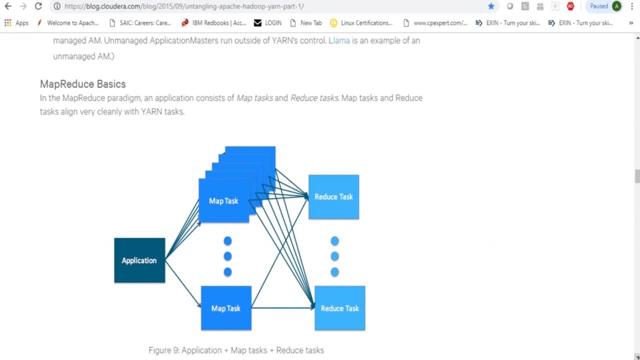 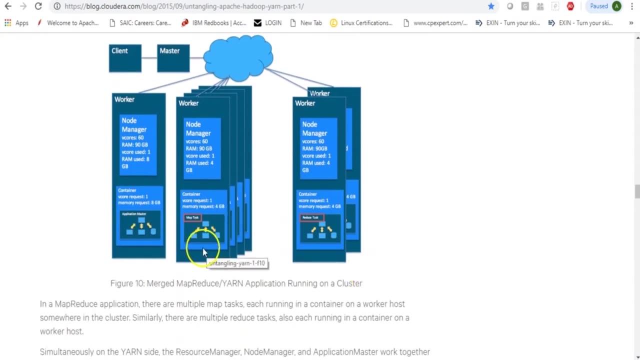 have already followed the MapReduce tutorials in past, then you would know about the different kind of tasks. that is, Map and Reduce, and these Map and Reduce tasks could be running within the container in one or multiple. As I said, it could be MapTask, it could be ReduceTask, it could be a Spark-based. 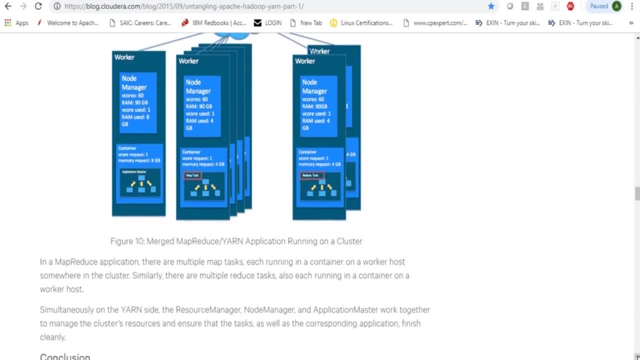 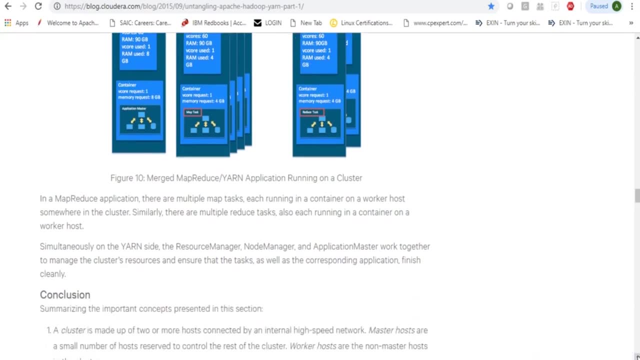 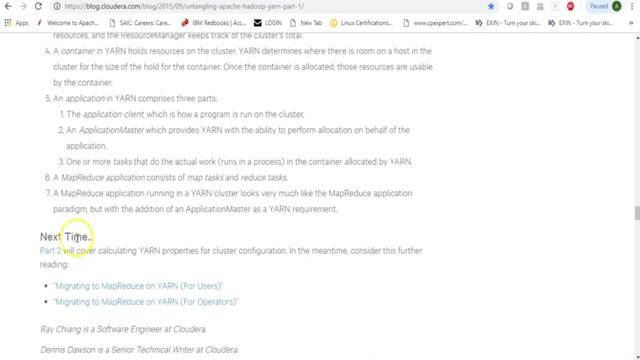 task which would be running within the container. Now, once the task finishes, basically that resources can be freed up, So the container is released and the resources are given back to YARN so that it can take care of further processing. If you'll further look in this blog, you can also look into the part two of it. 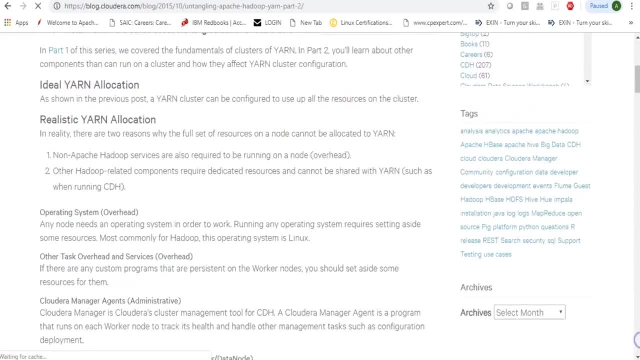 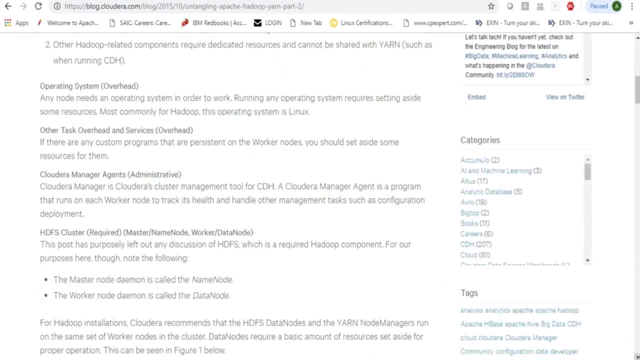 where you talk mainly about configuration settings- You can always look into this- which talks about why and how much resources are allocated to the node manager. It basically talks about your operating system overhead. It talks about other services. It talks about CloudAdr, Hotendworks. 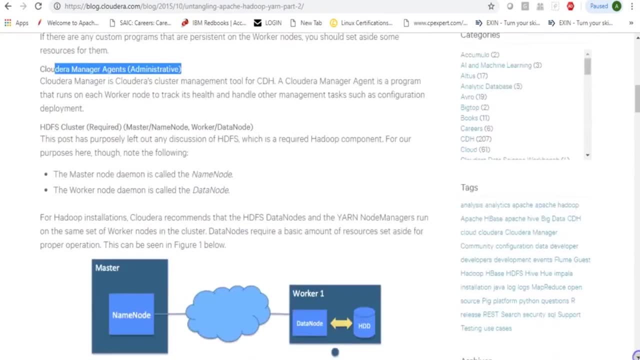 related services running And it talks about the configuration of the container. So the container is released and the resources are given back to YARN so that it can take care of further processing And other processes which might be running And, based on that, some portion of RAM and CPU cores. 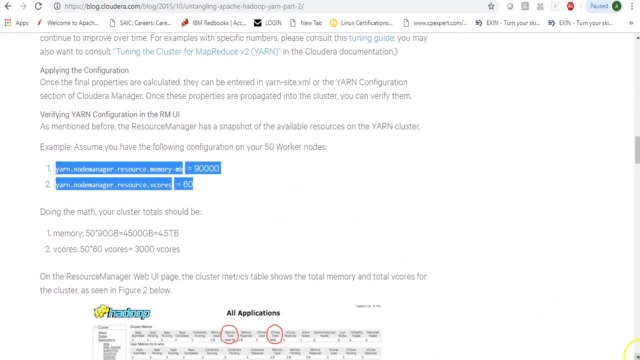 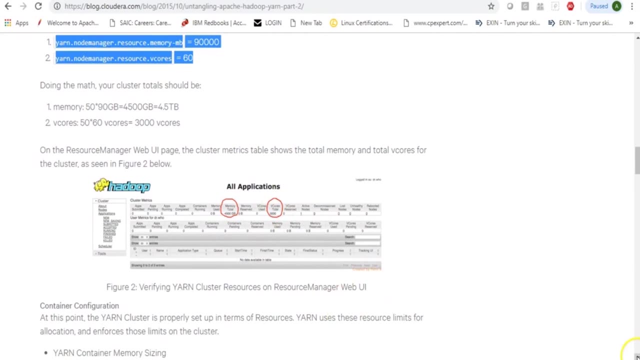 would be allocated to node manager. So that's how it would be done in the YARN hyphen site file and this basically shows you what is the total amount of memory and CPU cores which is allocated to node manager. Then, within every machine where you have a node manager running on, every machine in 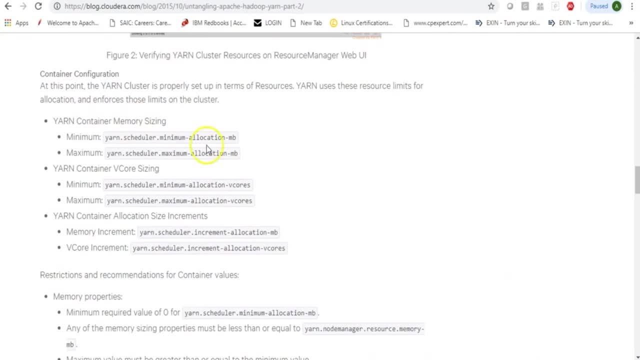 the YARN hyphen site file, you would have such properties, which would say: what is the minimum container size, what is the maximum container size in terms of RAM, what is the minimum for CPU cores, what is the maximum for CPU cores and what is the incremental size in where? 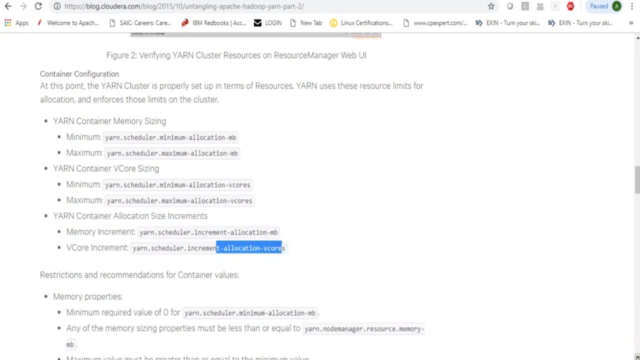 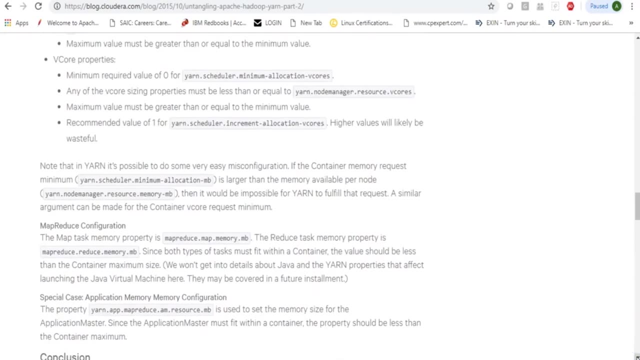 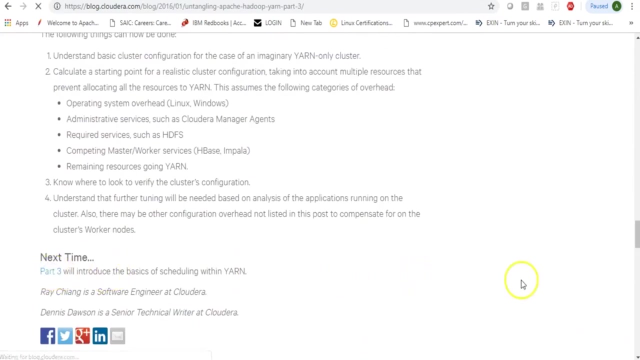 RAM and CPU cores can increment. so these are some of the properties which define how containers are allocated for your application request. so have a look at this and this could be a good information which talks about different properties. now you can look further which talks about scheduling, if you look in this particular blog, which also talks about scheduling, where it talks about 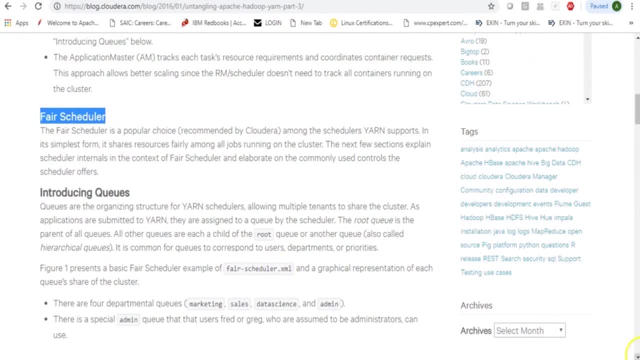 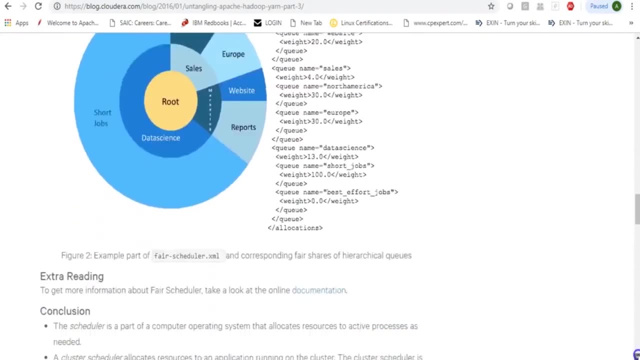 scheduling in yarn, which talks about fair scheduler or you basically having different queues in which allocations can be done. you also have different ways in which queues can be managed and different schedulers can be used. so you can always look at this series of blog. you can also 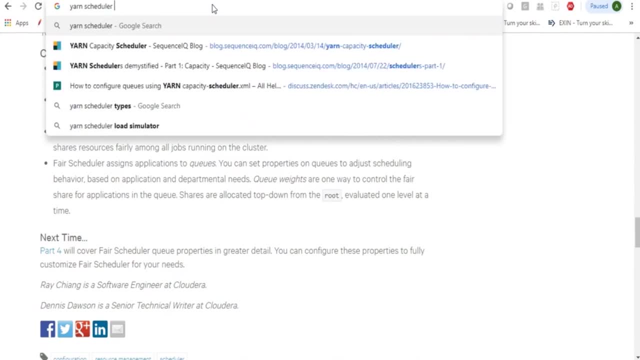 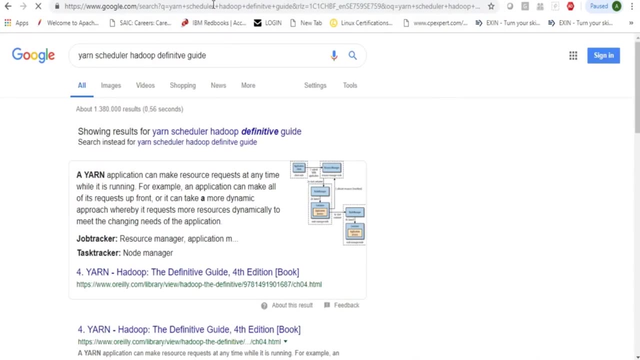 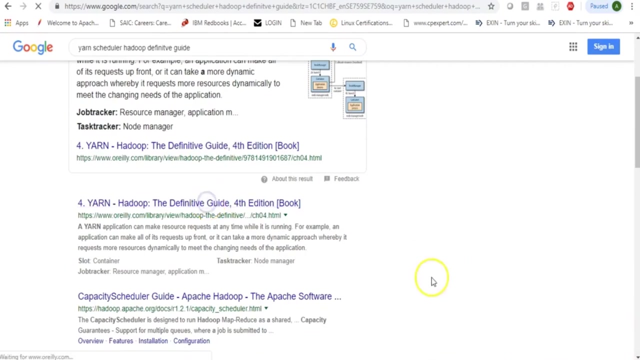 be checking for yarn schedulers and then search for a Hadoop definitive guide, and that could give you some information on how it looks when you look for Hadoop definitive guide. so if you look into this book, which talks about the different resources as I mentioned, so you 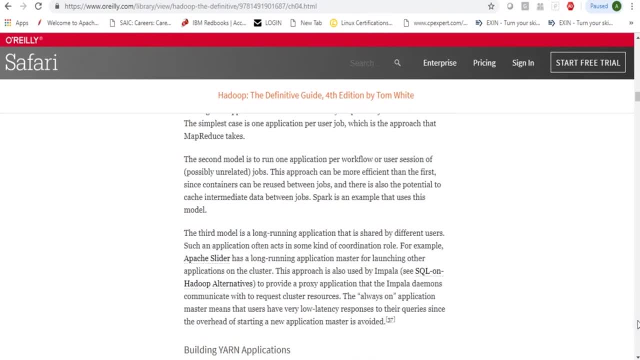 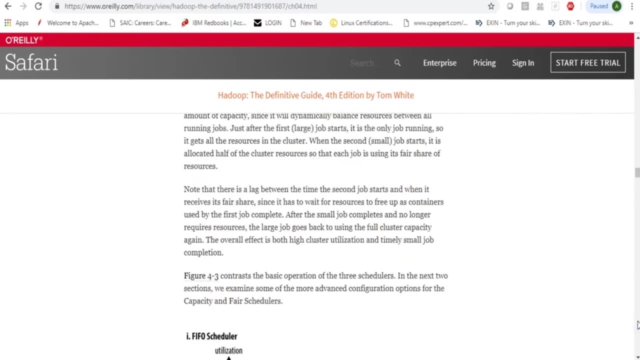 could have a FIFO scheduler that is first in, first out, which basically means if a long running application is submitted to the cluster, all other small running applications will have to wait. there is no other way. but that would not be a preferred option. if you look in FIFO scheduler, if you look 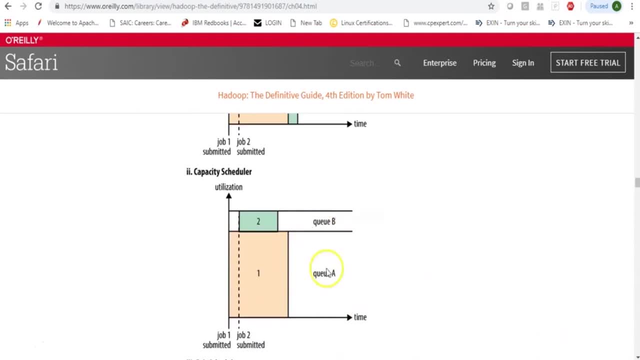 for capacity scheduler. it basically means that you could have different queues created and those queues would have resources allocated. so then you could have a production queue where production jobs are running in a particular queue which has fixed amount of resources allocated. you could have a development queue where development jobs are running and both of them are running in parallel. 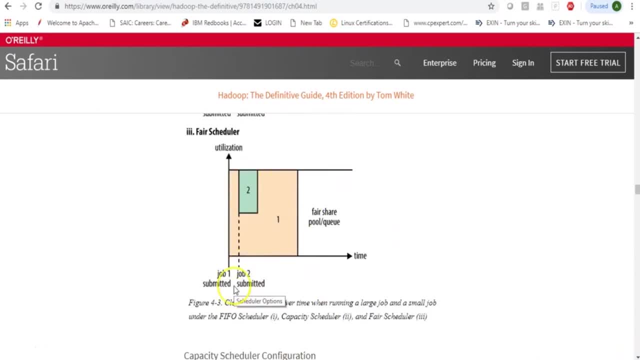 you could then also look into fair scheduler, which basically means, again, multiple applications could be running on the closed. However, they would have a fair share. So when I say fair share in brief, what it means is if I had given 50% of resources to a queue for production and 50% of resources for a queue of development, and if both of them are running in parallel, then they would have access to 50% of cluster resources. 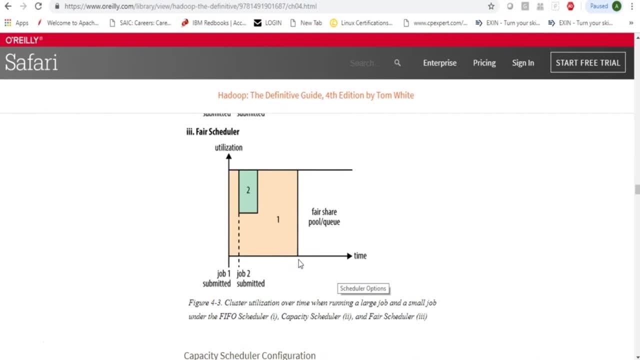 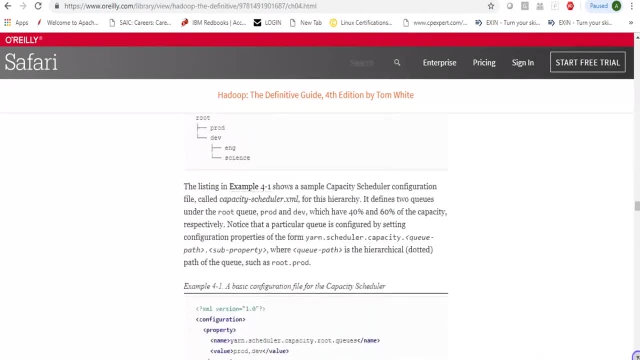 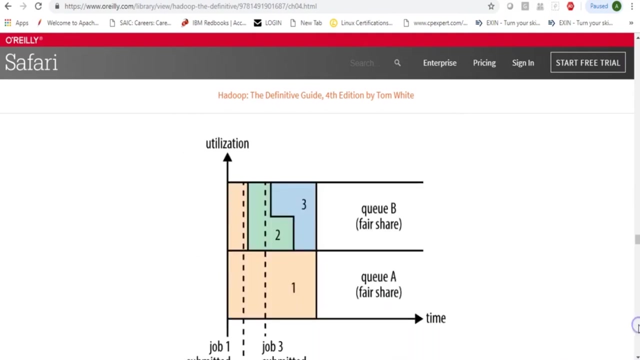 However, if one of the queue is unutilized, then second queue can utilize all cluster resources. So look into the fair scheduling part. It also shows you about how allocations can be given and you can learn more about schedulers and how queues can be used for managing multiple applications. 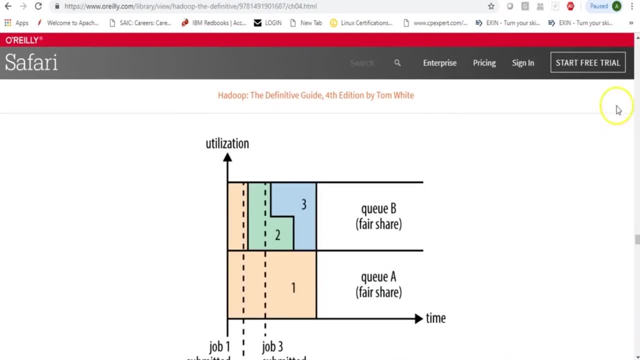 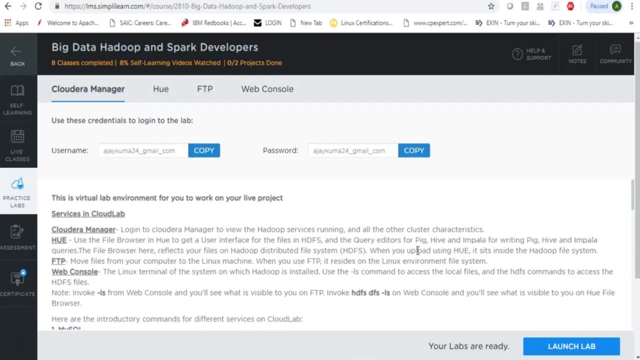 Now we will spend some time in looking into few ways or few quick ways in interacting with yarn in the form of a demo To understand and learn on how yarn works. we can look into a particular cluster. Now here we have a designated cluster which can be used. You could be using the similar kind of commands on your Apache based cluster or a Cloudera quick start VM if you already have, or if you have, a Cloudera or a Hortonworks cluster running. 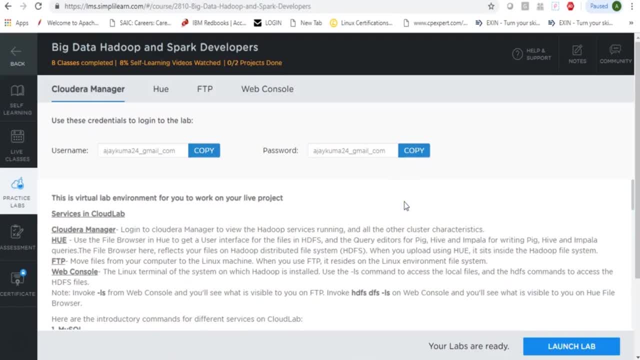 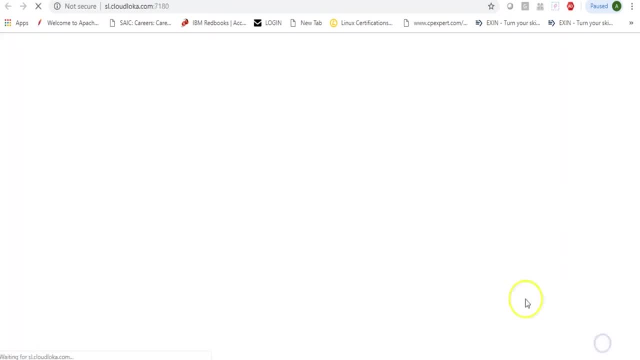 There are different ways in which we can interact with yarn and we can look at the information. One is basically looking into the admin console. So if I would look into Cloudera manager, which is basically an admin console for a Cloudera distribution of a dupe, Similarly you could have a Hortonworks cluster and access to the admin console. 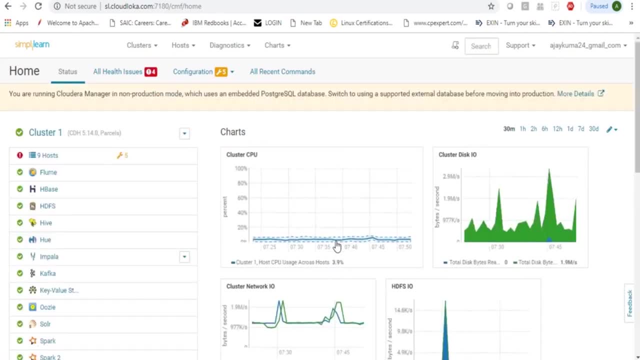 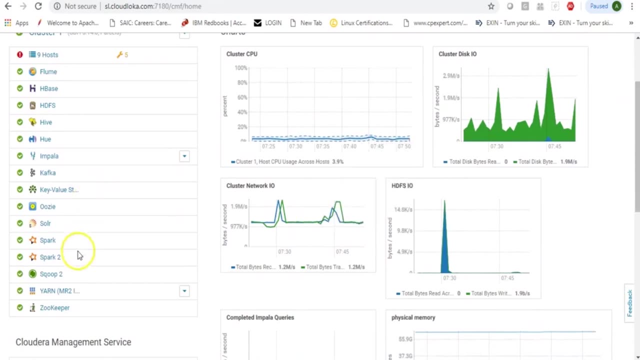 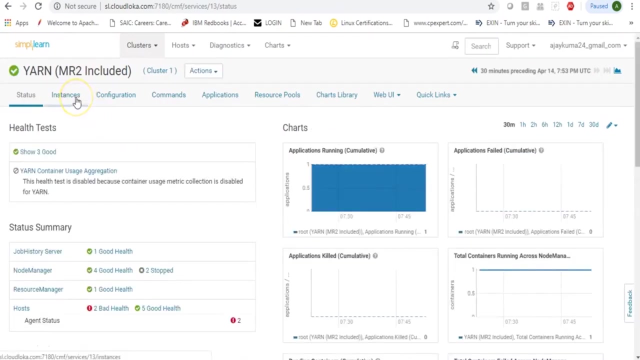 So if you have even read access for your cluster and if you have the admin console, then you can search for yarn as a service, which is running. You can click on yarn as a service and that gives you different tabs. So you have the instances. 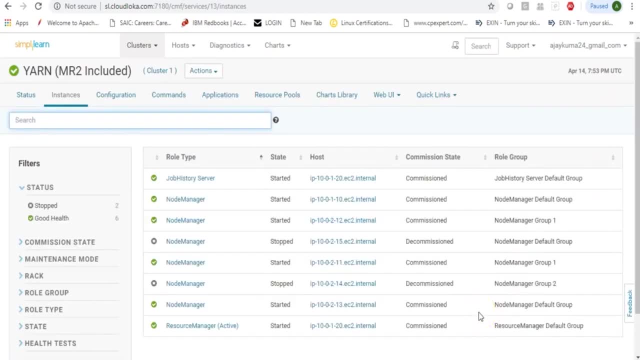 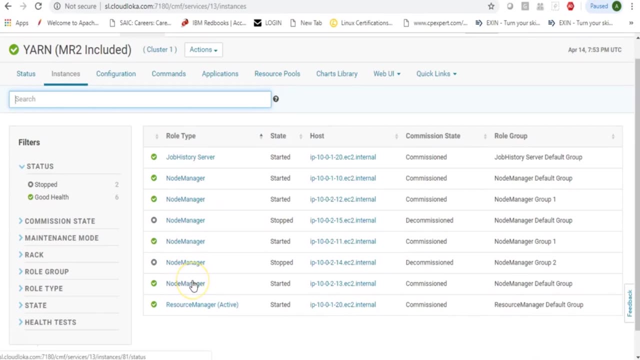 Which tells basically what are the different roles for your yarn service running. So we have here multiple node managers. Now some of them show in stop status, but that's nothing to worry. So we have three and six node managers. We have resource manager, which is one, but then that can also be in a high availability where you can have active and standby. 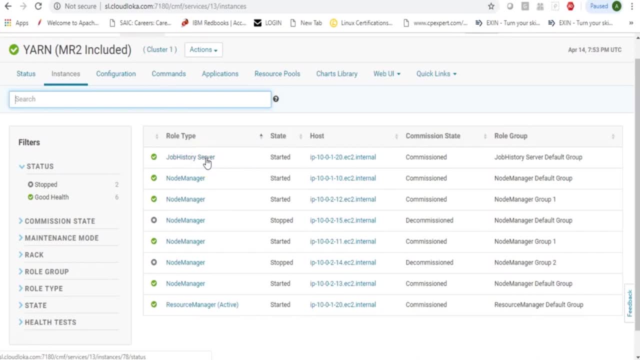 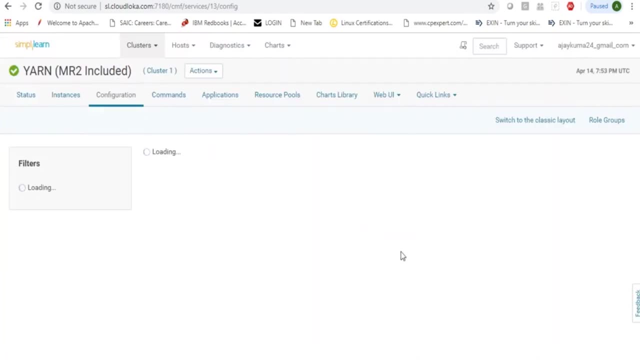 You also have a job history server which would show you the applications once they have completed. Now you can look at the yarn Configurations and, as I was explaining, you can always look for the properties which are related to the allocation. So you can here search, for course, and that should show you the properties which talk about the allocations. 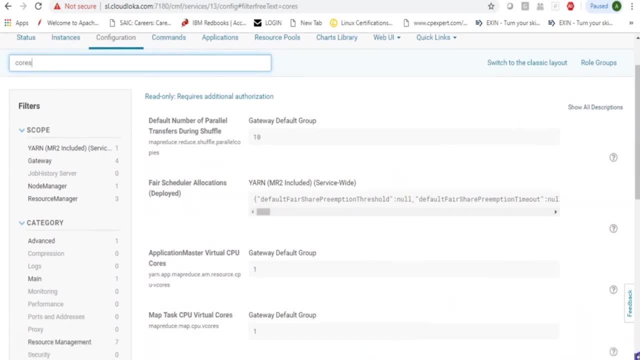 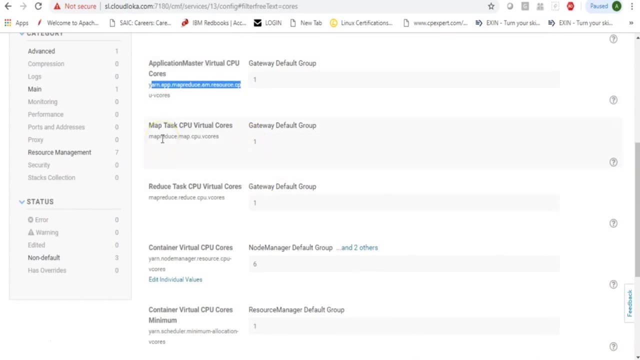 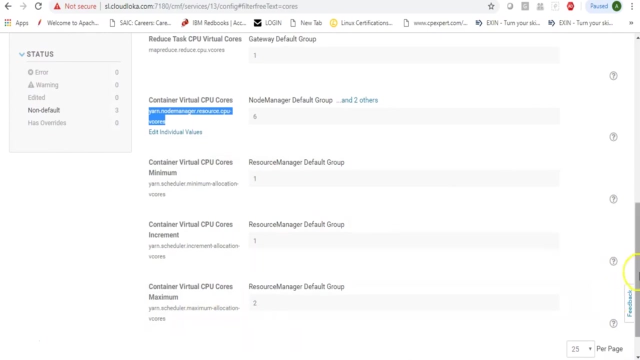 So here, if we see we can be looking for yarn app, map reduce application master resource CPU course. What is the CPU course allocated for? map reduce map task: reduce task. You can be looking at yarn node manager resource CPU course, which basically says every node manager on every node would be allocated with six CPU course and the container sizing is with minimum allocation of one CPU core and the maximum could be two CPU course. 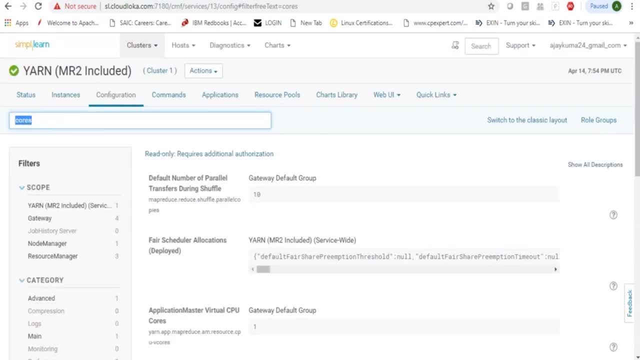 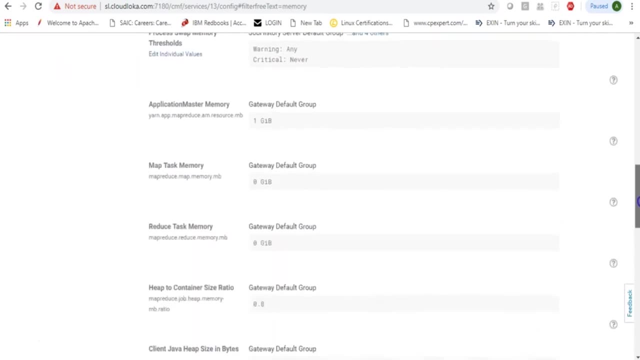 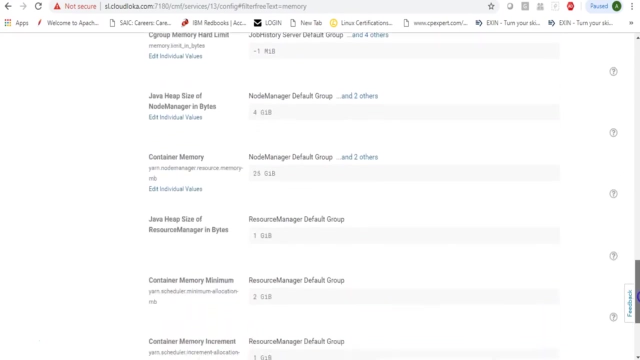 Similarly, you could also be searching for memory allocation and here you could then scroll down to see what kind of memory allocation has been done for the node manager. So if we look further, it should give me information of node manager which basically says here that the container minimum allocation is two GB. 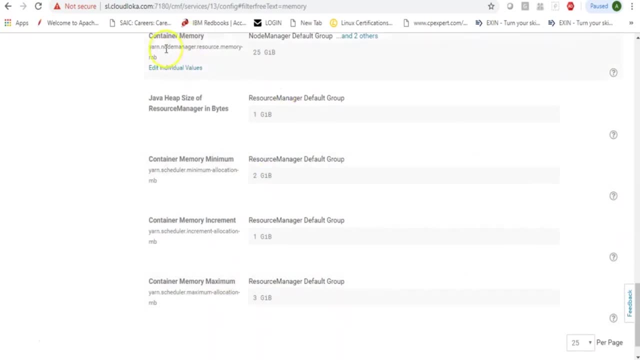 The maximum is three GB and we can look at node manager, which has been given 25 GB per node. So it's a combination of this memory and CPU course, which is the total amount of resources which have been allocated to every node. So that's it. 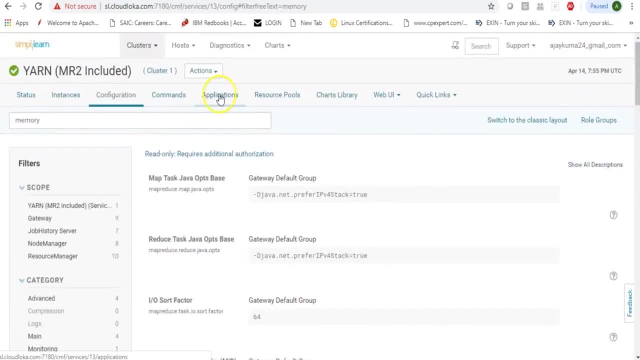 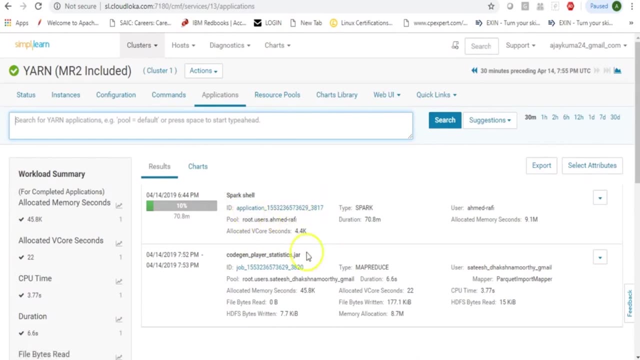 Thank you. Now we can always look into applications tab. that would show us different applications which are submitted on yarn, For example. right now we see there is a spark application running, which is basically a user who is using spark shell which has triggered a application on spark and that is running on yarn. 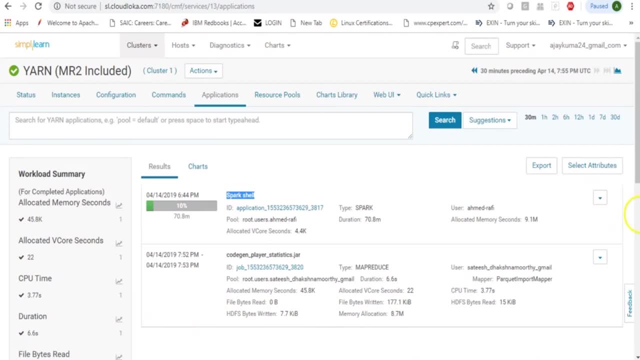 You can look at different applications workload information. You can always do a search based on the number of days, how many applications have run, and so on and so on. you can always go to the web ui and you can be searching for the resource manager web ui. 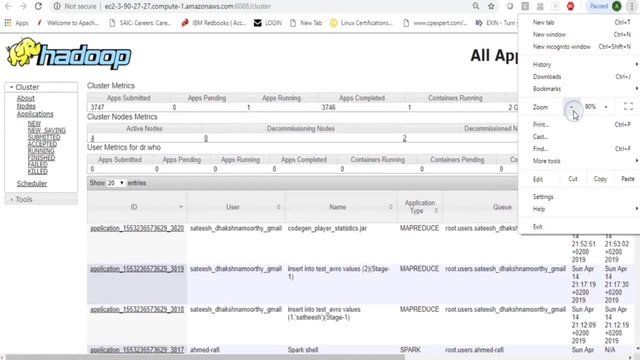 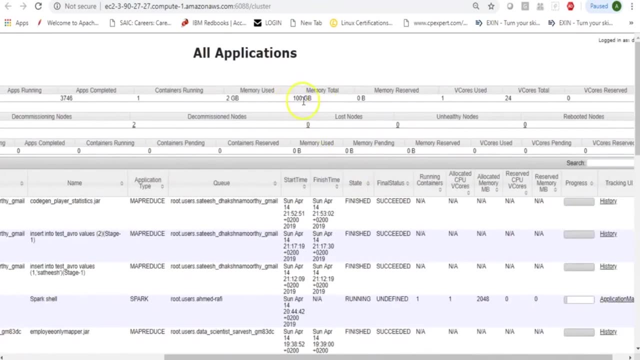 and if you have access to that, it will give you overall information of your cluster. so this basically says that here we have 100 gb memory allocated, so that could be say 25 gb per node, and if we have four node managers running and we have 24 cores, which is six cores per node, if we 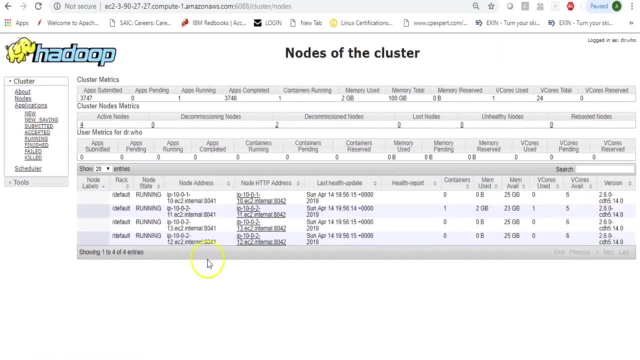 look further here into nodes, I could get more information, so this tells me that I have four node managers running and node managers basically have 25 gb memory allocated per node and six cores out of which some portion is being utilized. we can always look at the scheduler here, which 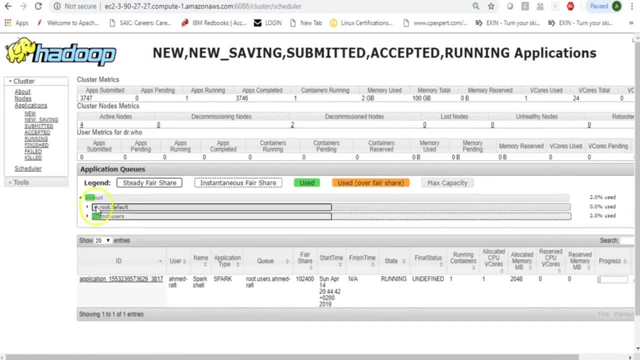 can give us information? what kind of scheduler has been allocated? so we basically see that there is just a root queue and within root you have default queue and you have basically Whoops users queue based on different users. we can always scroll here and that can give us information, if it. 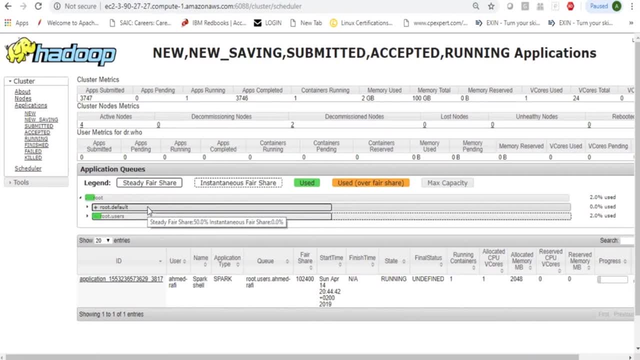 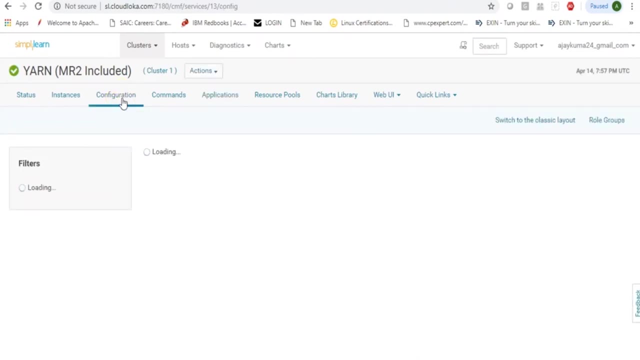 is a fair share. so here we see that my root dot default has 50 percent of resources and the other queue also has 50 percent of resources, which also gives me an idea that a fair scheduler is being used. we can always confirm that if we are using a fair scheduler or a capacity scheduler, which 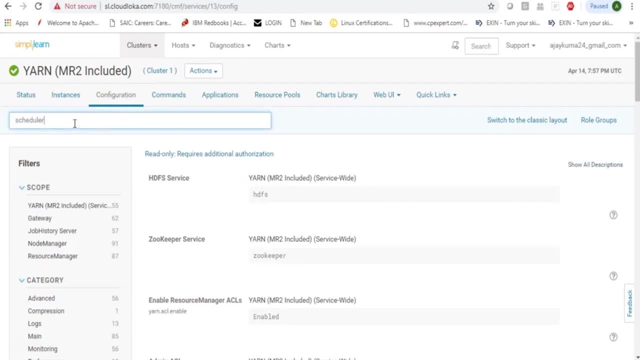 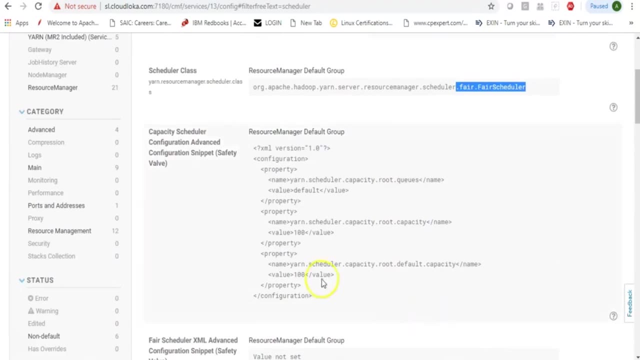 takes care of allocations. so search for scheduler and that should give you some understanding of what kind of scheduler is being used and what are the allocations given for that particular scheduler. so here we have fair scheduler. it shows me you have under root, you have the root queue which has been given 100 percent capacity, and then you have within that. 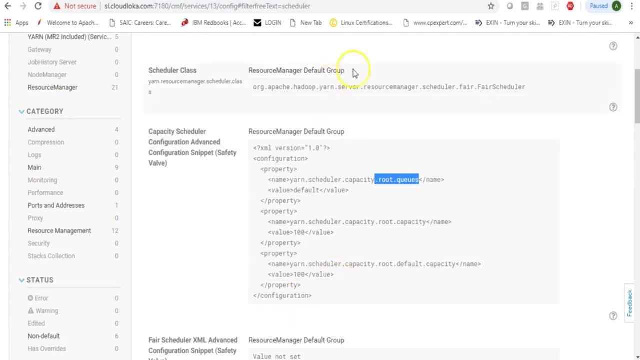 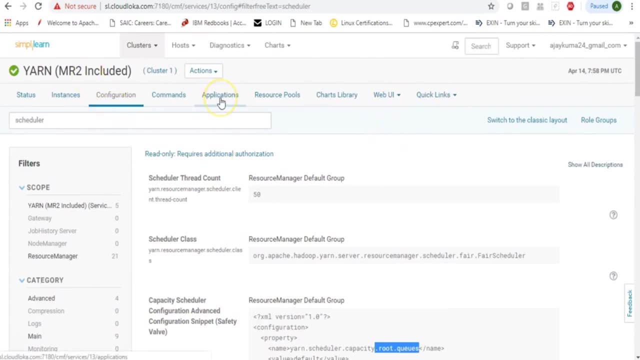 default, which also takes 100 percent. so this is how you can understand about yarn. by looking into the yarn web ui, you can be looking into the configurations. you can look at applications. you can always look at different actions. now, since we do not have admin access, the only information we have is to download. 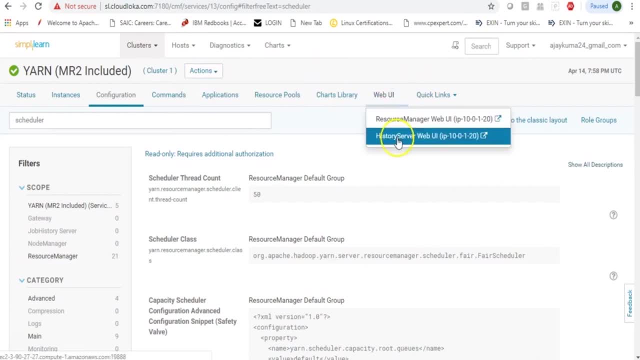 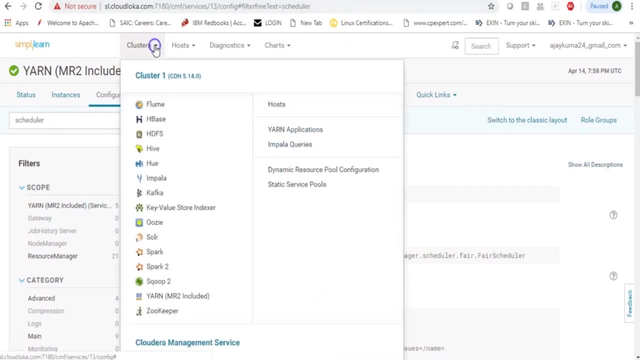 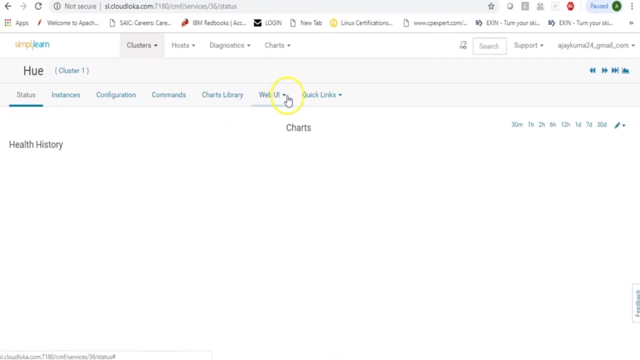 the client configuration, we can always look at the history server, which can give us information of all the applications which have successfully completed. now, this is from your yarn ui. what i can also do is i can be going into hue, which is the web interface, and your web interface also. 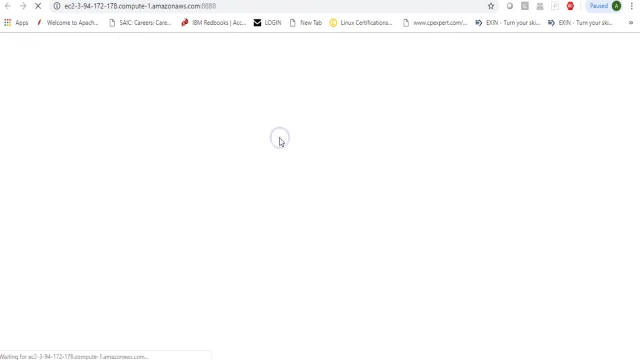 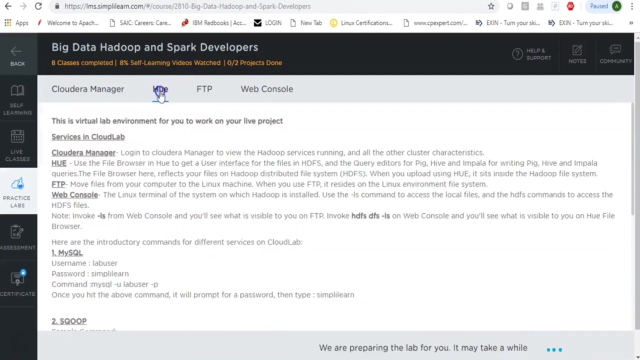 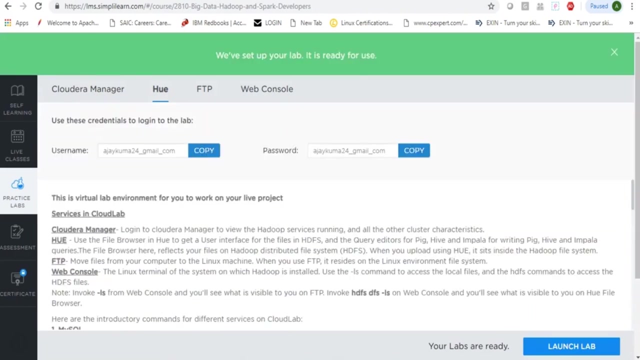 basically allows you to look into the jobs. so you can click on hue web ui and if you have access to that, it should show up or you should have a way to get to your hue, which is a graphical user interface. mainly comes with your cloud era. you can also configure that with apache hot and works. 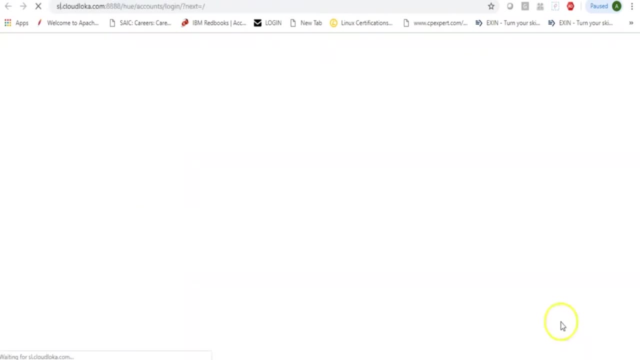 has a different way of giving you the web ui access. you can click and get into the web interface and you can also configure the web ui and you can also configure the web into hue and that is also one way where you can look at yarn, you can look at the jobs. 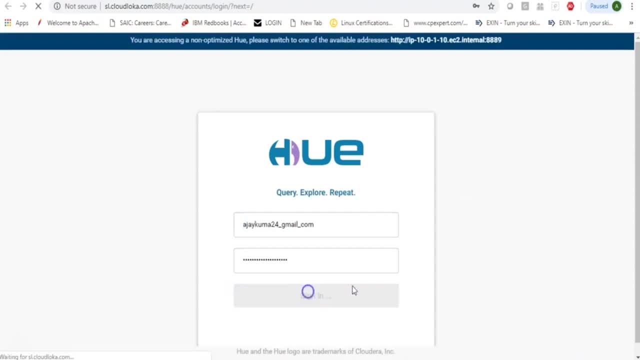 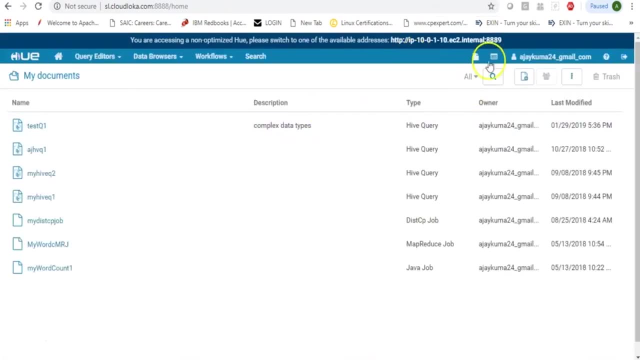 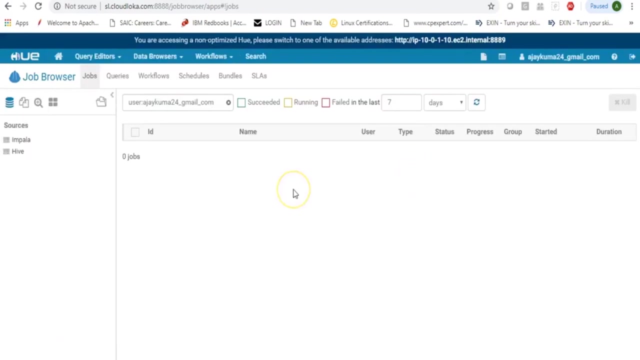 which are running, if there are some issues with it, and these. these are your web interfaces. so either you look from yarn web ui or here in hue you have something called as job browser, which can also give you information of your different applications which might have run. so here i can just remove this one, which should basically give me a list. 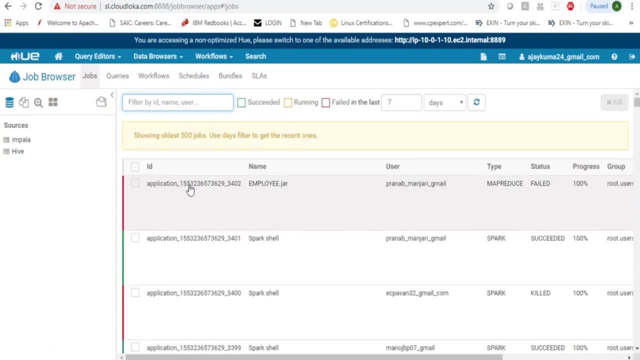 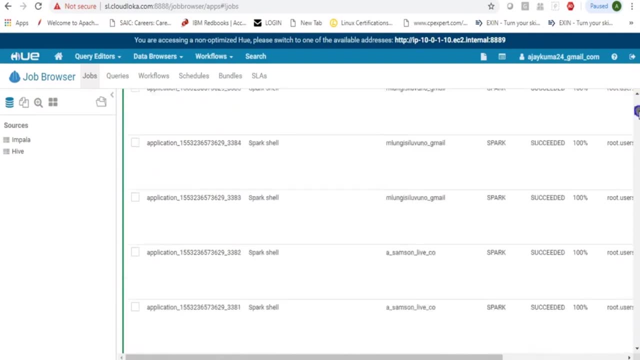 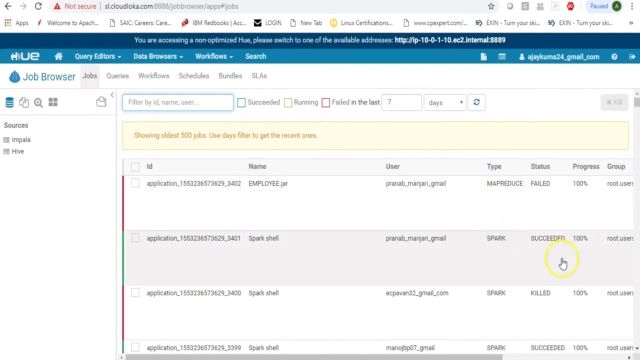 of all the different kind of jobs or workloads which were run. so either it was a spark based application, or it was a map reduce, or it was coming from hive. so here i have list of all the applications and it says: this was a map reduce, this was a spark, something was killed. 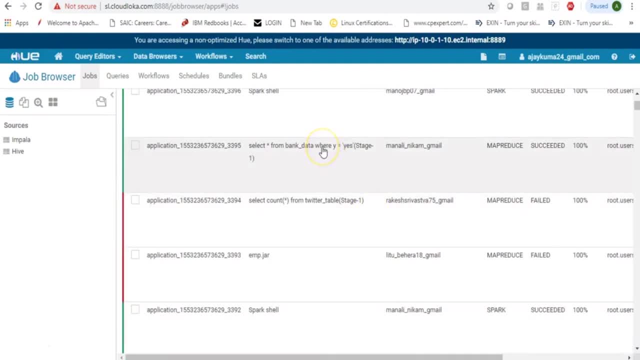 something was successful and this was basically a- probably a hive- query which triggered a map reduce job. you can click on the application and that tells you how many times you have to click on the application. and that tells you how many times you have to click on the application. and. 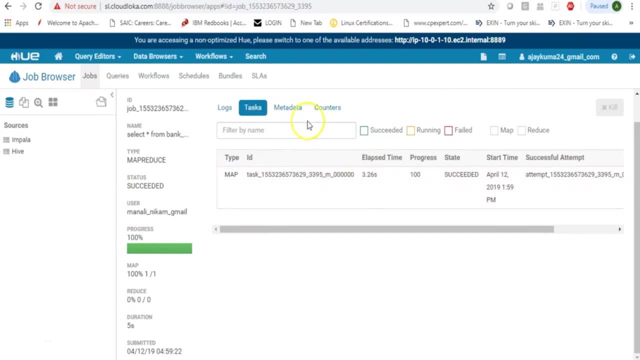 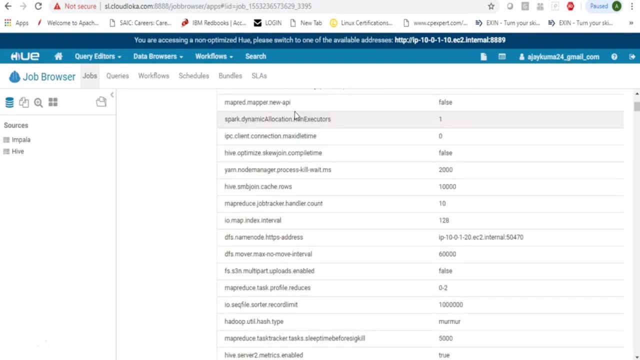 tasks were run for it, so there was a map task which ran for it. you can get into the metadata information which you can. obviously you can also look from the yarn ui to look into your applications which can give you a detailed information of if it was a map, reduce how many map and reduce tasks. 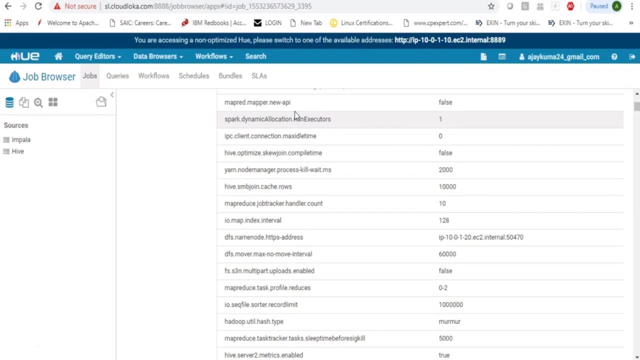 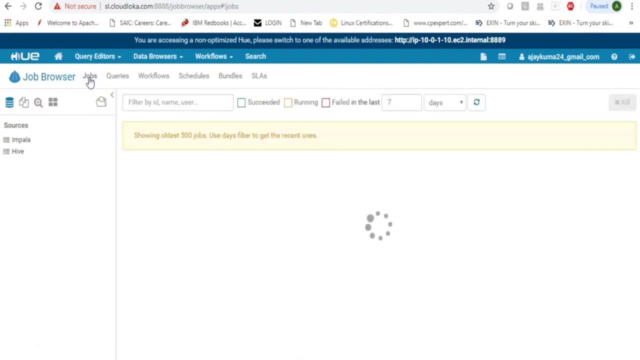 were run. what were the different counters? if it was a spark application, it can let you follow through spark history server or job history server so you can always use the web ui to look into the jobs. you can be finding in a lot of useful information here. you can also be looking at how many resources were used. 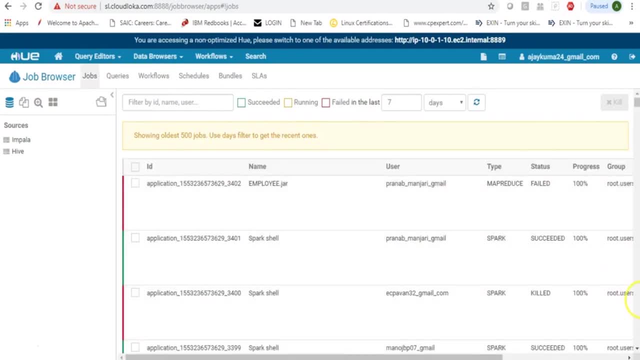 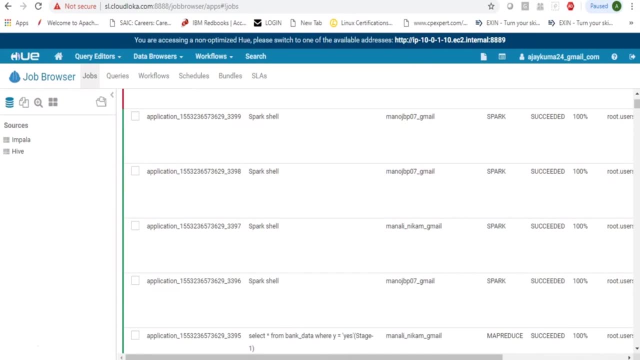 and what happened to the job? was it successful? did it fail? and what was the job status now, apart from web ui, which always you might not have access to. so in a particular cluster, in a production cluster, there might be restrictions and the organization might not have access given to all the users to. 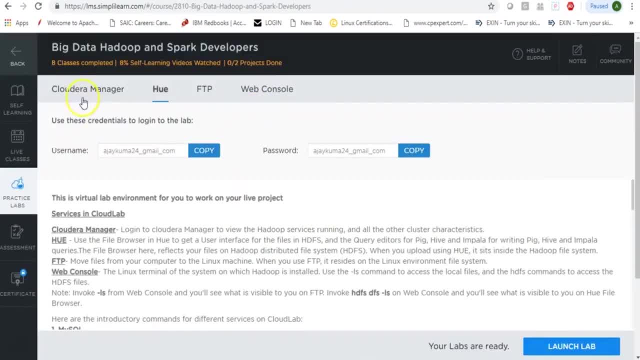 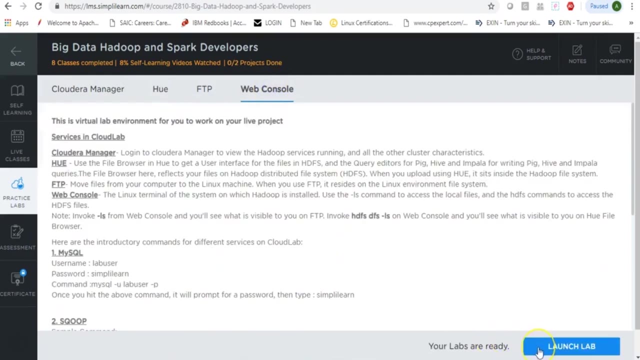 graphical user interface. like you or might be, you would not have access to the cloud data manager or admin console because probably organization is managing multiple clusters using this admin console, so the one way which you would have access is your web console or basically your edge node or client machine, from where you can connect to the cluster. 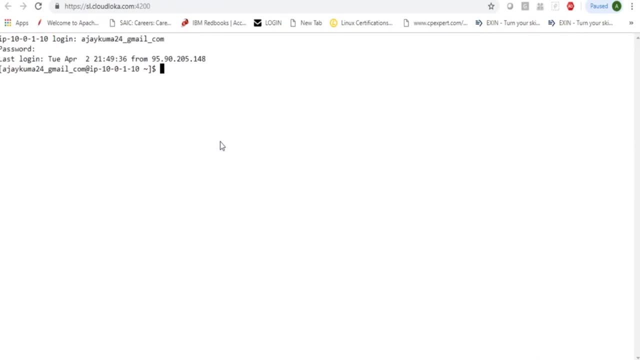 and then you can be working. so let's log in here and now. here we can give different commands. so this is the command line from where you can have access to different details. you can always check by just typing in map read, which gives you different options where you can. 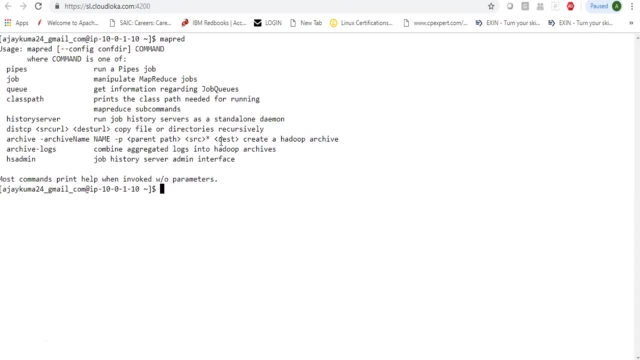 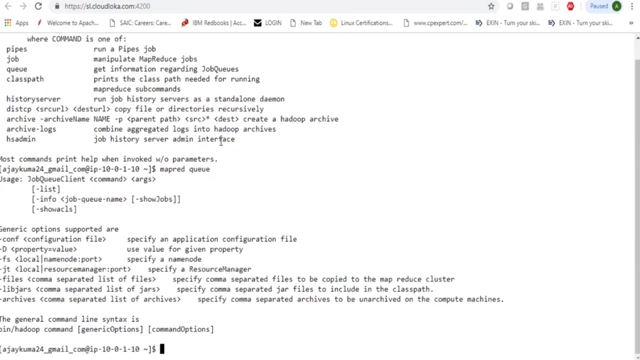 look at the map, reduce related jobs. you can look at different queues- if there are queues configured. you can look at the history server or you can also be doing some admin stuff, provided you have access. so, for example, if i just say map read and queue here, this basically gives me an option. says what? 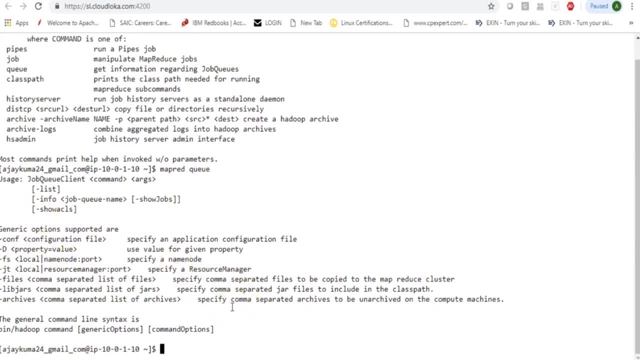 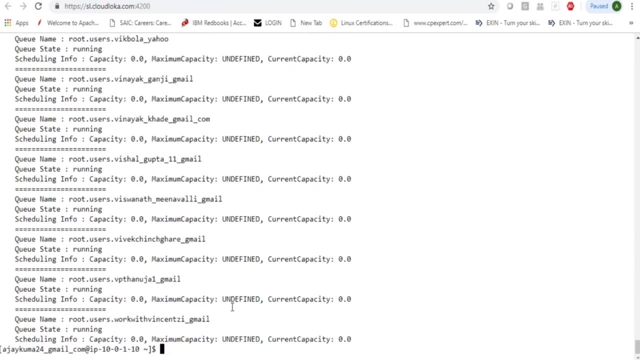 would you want to do? would you want to list all the queues? do you want information on a particular queue? so let's say i want to list all the queues. so let's say i want to list all the queues. so let's try a list, and that should give you different queues which were being used. now, here we know. 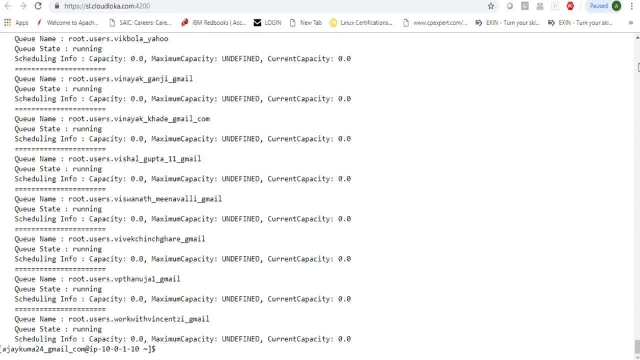 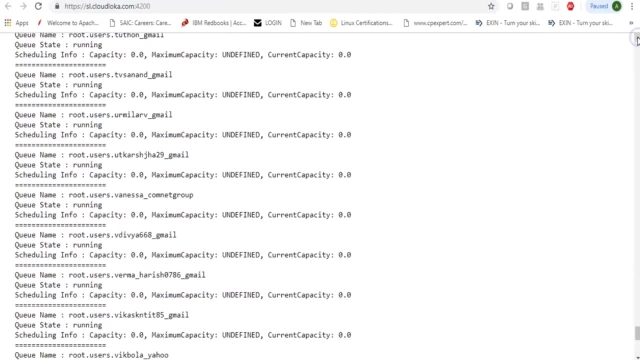 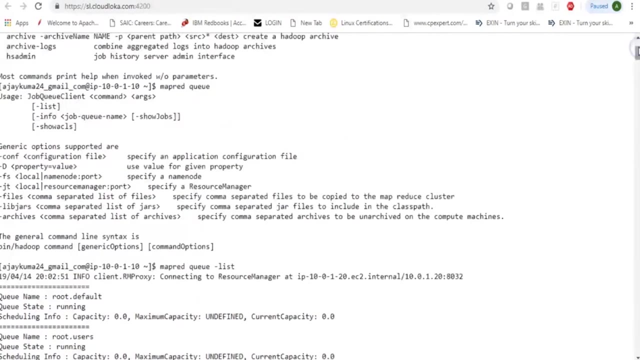 that per user, a queue dynamically gets created which is under root dot users, and that gives me what is the status of the queue, what is the capacity? has there been any kind of maximum capacity or capping done? so we get to see a huge list of queues which dynamically get configured. 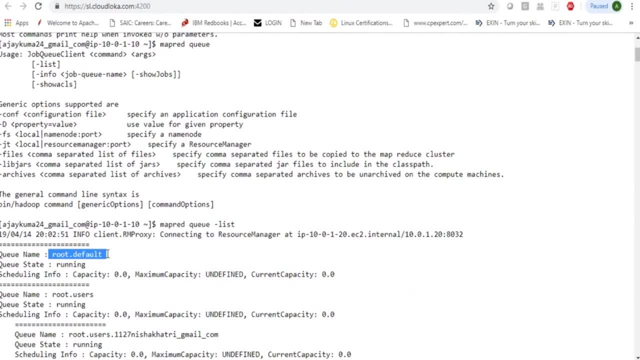 in this environment, and then you also look at your rootdb for it. i could have also picked up one particular queue and i could have said: show me the jobs. so i could do that. now, here we can also give a yarn command. so let me just clear the screen and i will. 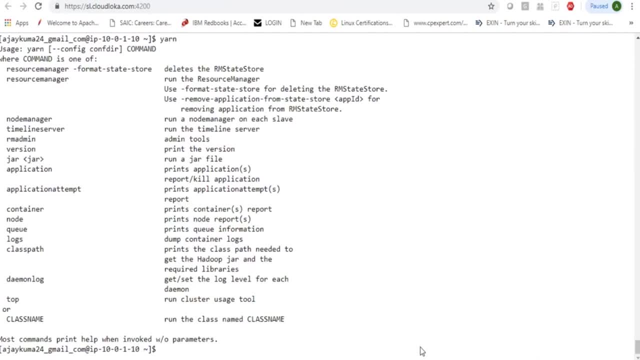 say yarn, and that shows me different options. so apart from your web interface, something like web ui, apart from your yarns web ui, you could also be looking for information using yarn commands here, which we can check. now you can just type in yarn and version if you would want to see the version. 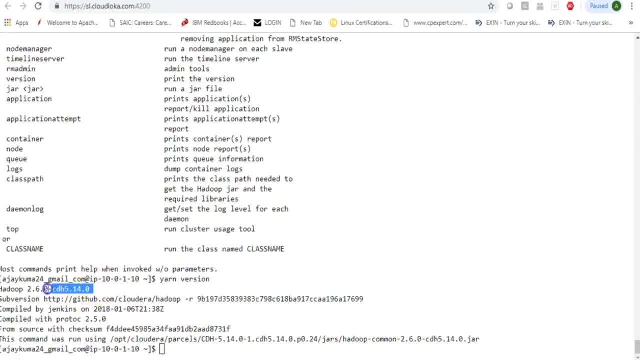 which basically gives you information of what is the hadoop version being used and what is the vendor specific distribution version. so here we see. we are working on cloudera's distribution 5.14, which is internally using hadoop 2.6 now. similarly, you can be doing a yarn application list. 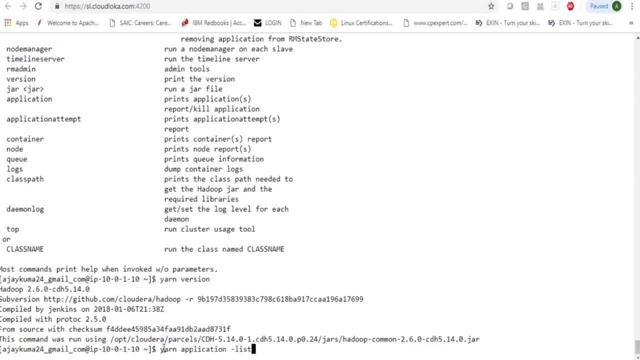 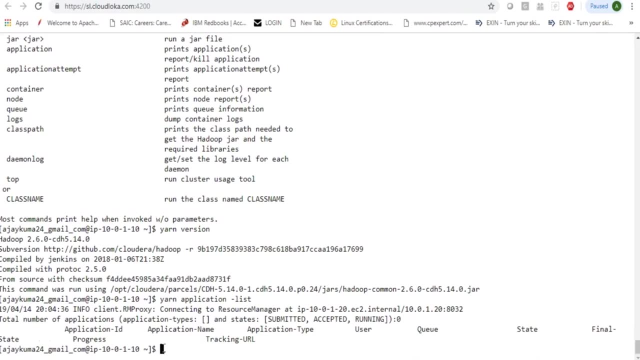 so if you give this, that could be an exhaustive list of all the applications which are running or applications which have completed. so here we don't see any applications because right now probably there are no applications which are running. it also shows you you could be pulling out different status, such as submitted, accepted. 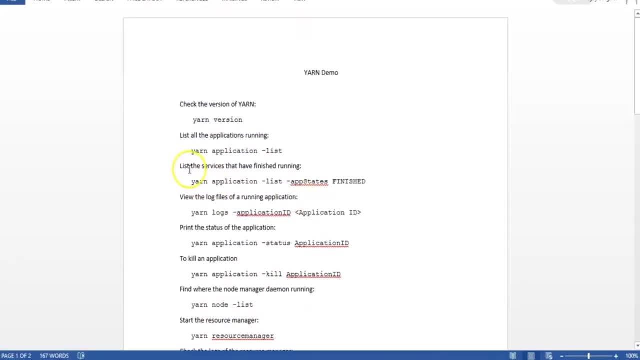 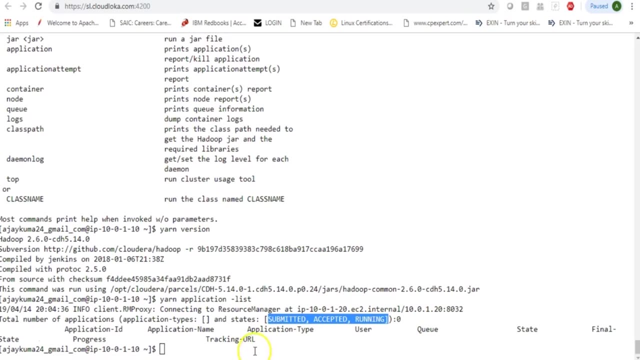 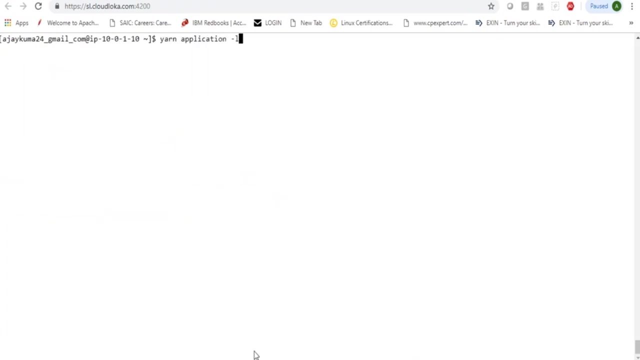 or running now. you could also say: i would want to see the services that have finished running. so i could say yarn application list and app states as finished. so here we could be, using our command, so i could say yarn application list and then i would want to see the app states which gives me. 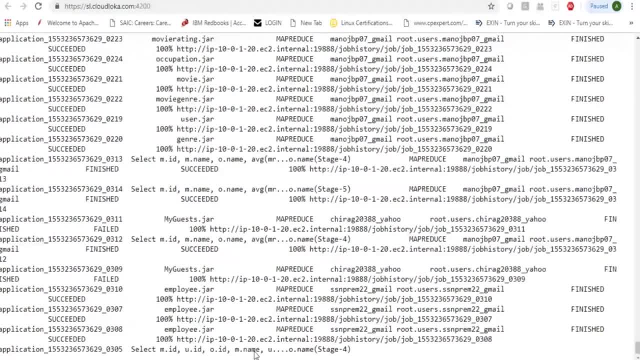 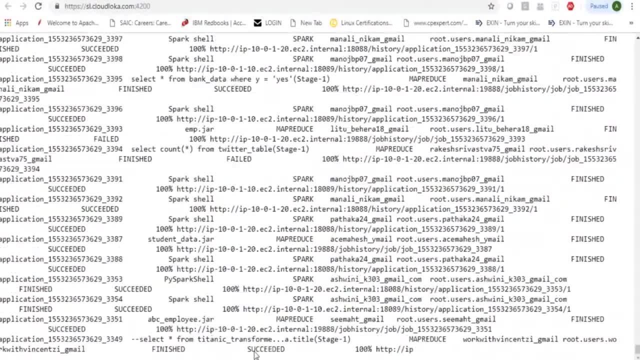 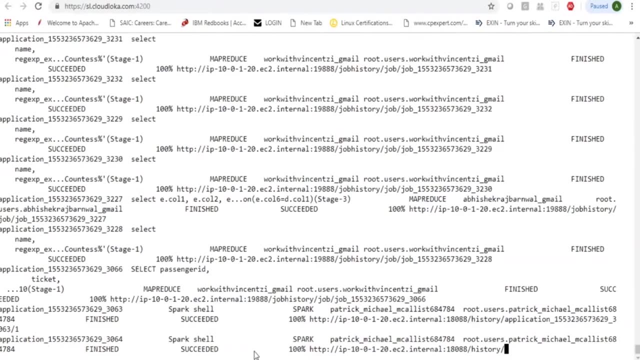 the applications which have finished, and we would want to list all the applications which finished. now, there that might be applications which succeeded right, and there is a huge list of application which is coming in from the history server which is basically showing you the huge list of applications which have completed. so this is one way, and then you could also be searching. 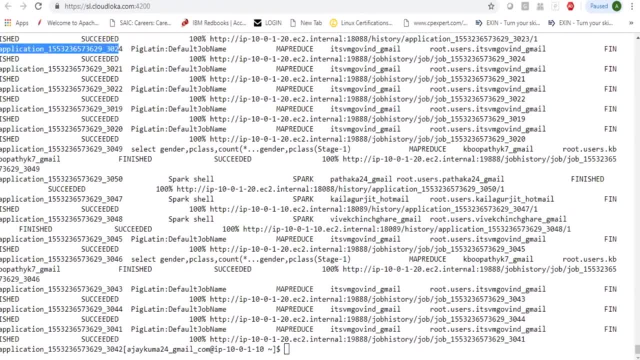 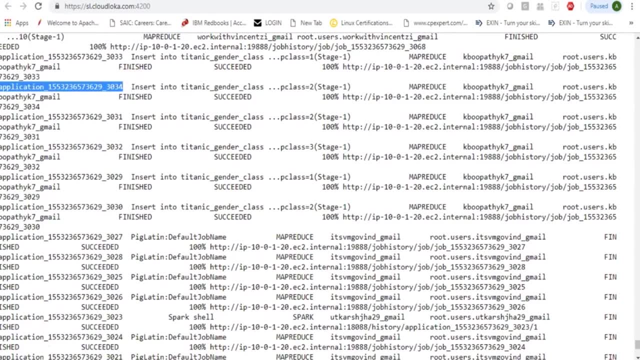 for a particular application. if you would want to search a particular application, if you have the application id, you could always be doing a grip. that's a simple way i could say, basically, let's pick up this one and if i would want to search for this, if i would want more details on this, 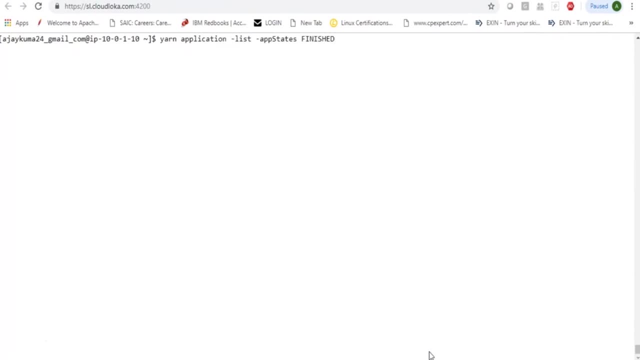 i could obviously do that by calling in my previous command and you could do a grip if that's what you want to do and if you would want to search, is there? any application which is in the list of my applications shows my application. i could pull out more information about my application. 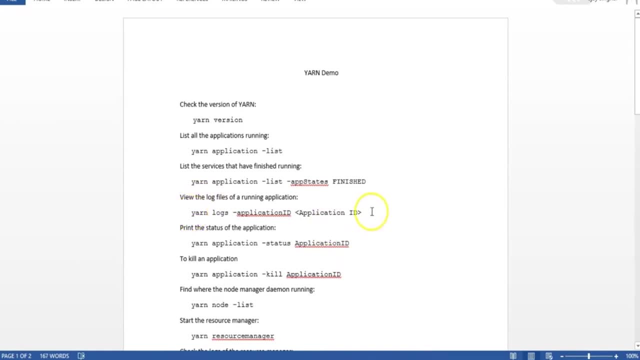 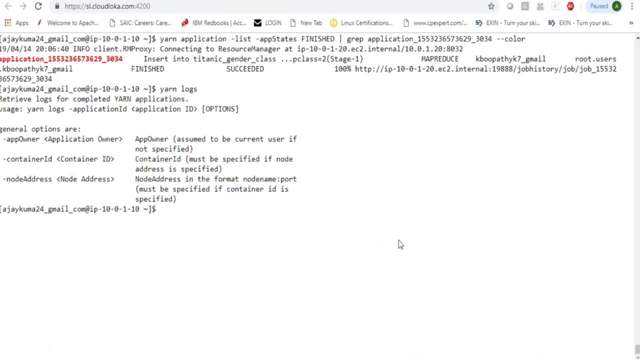 so i could look at the log files for a particular application by giving the application id so i could say yarn logs. now that's an option and every time, anytime you have a doubt, just hit enter. it will always give you options, what you need to give with a particular command so i can say yarn. 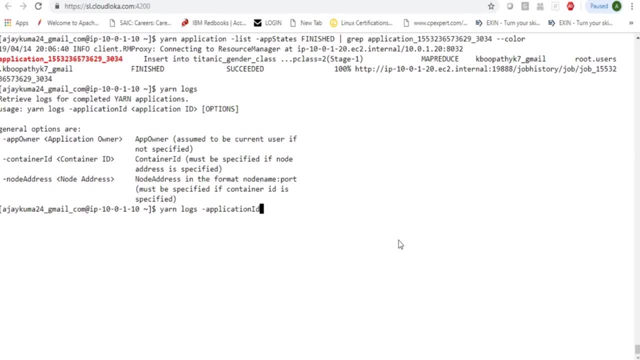 logs- application id. now we copied an application id and we could just give it here. we could give other options, like app owner, or if you would want to get into the container details or if you would want to check on a particular node. now here i'm giving yarn logs and then i'm 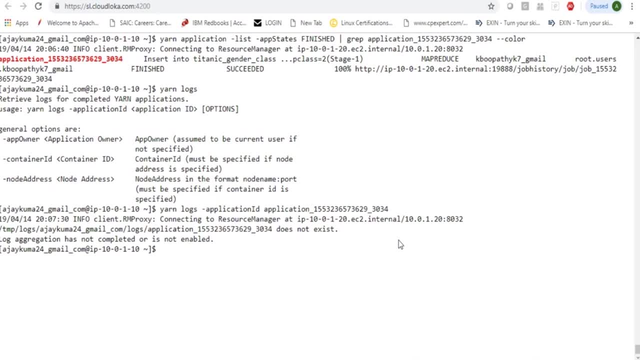 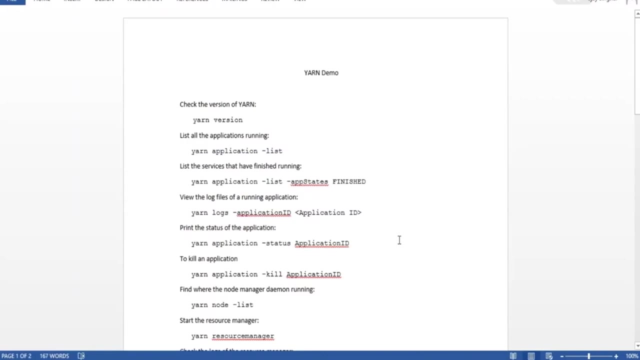 pointing it to an application id and it says the log aggregation has not completed. might be. this was. might be. this was an application which was triggered based on a particular interactive shell or based on a particular query, so there is no log existing for this particular application. you can always look at the status of an application. you can kill an application, so here. 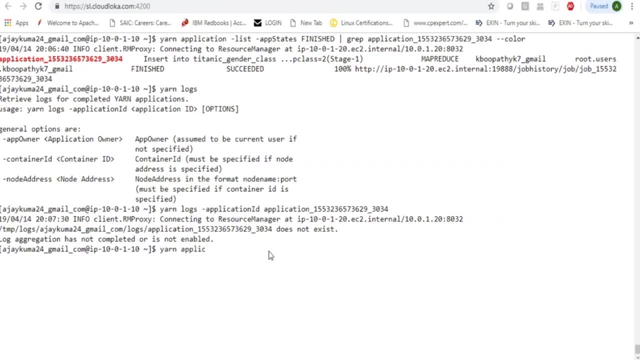 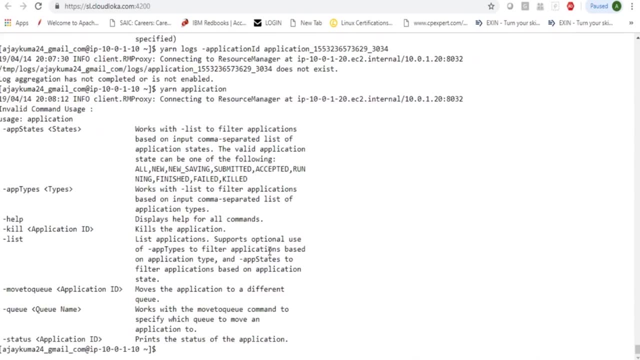 you can be saying yarn, yarn, application. and then what would you want to do with an application? hit and enter. it shows you the different options, so we just tried app states. you could always look at the last one which says status, and then, for my status, i could be giving my application. 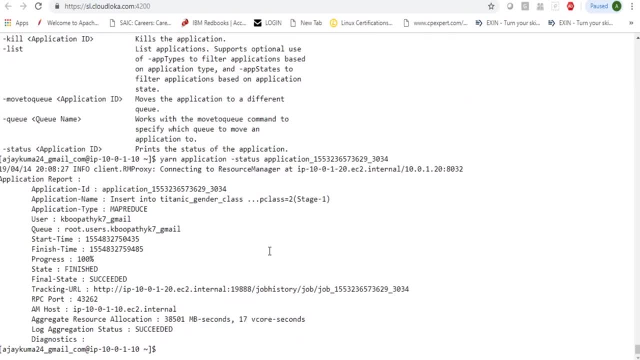 id. so that tells me what is the status of this application. it connects to the resource manager. it tells me what's the application id, what kind of application it was, who ran it, which was the queue where the job was running, what was the start and end time, what is the progress, the status of it. 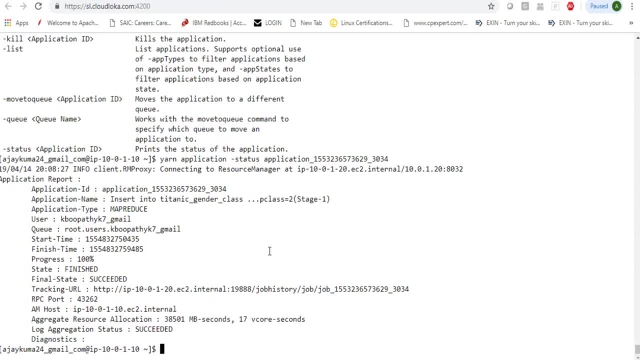 if it is finished or if it has succeeded, and then it basically gives me also an information of where the application master was running. it gives me the information where you can find this job details in history server if you are interested in looking into it. also gives you a aggregate resource. 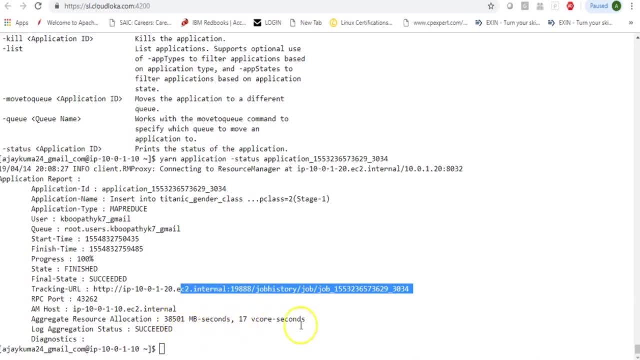 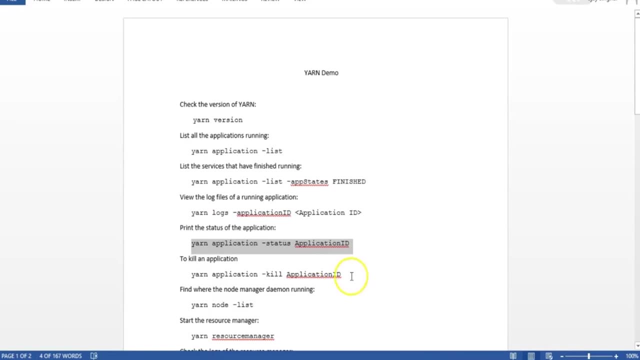 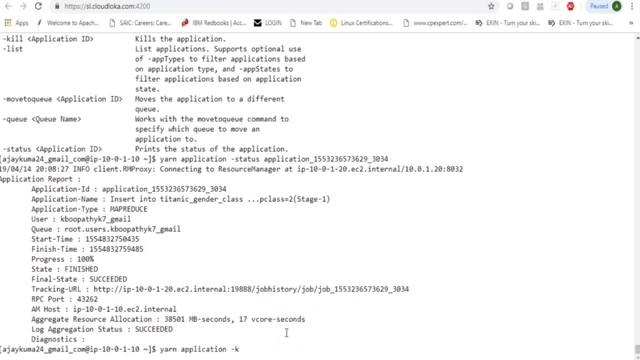 allocation, which tells how much gb memory and how many c core seconds it used. so this is basically looking out at the application details. now i could kill an application if the application was already running. i could always do a yarn: application minus kill, and then i could be giving. 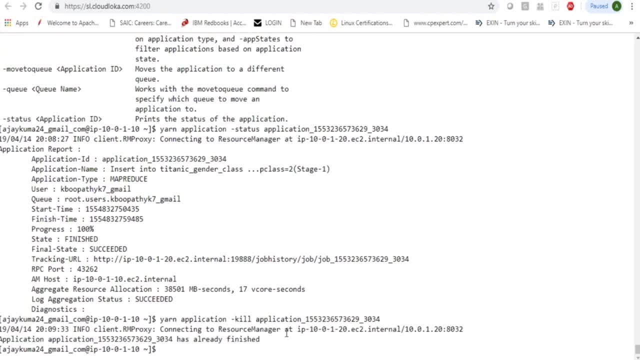 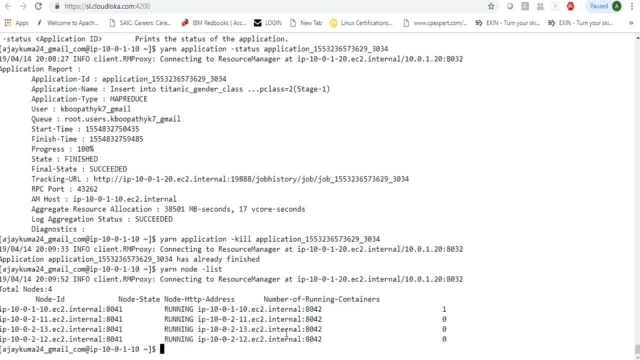 my application. now i could try killing this. however, it would say: the application is already finished. if i had an application running and if my application was already given an application id by source manager, i could just kill it. i can also say: yarn node list, which should give me a list of. 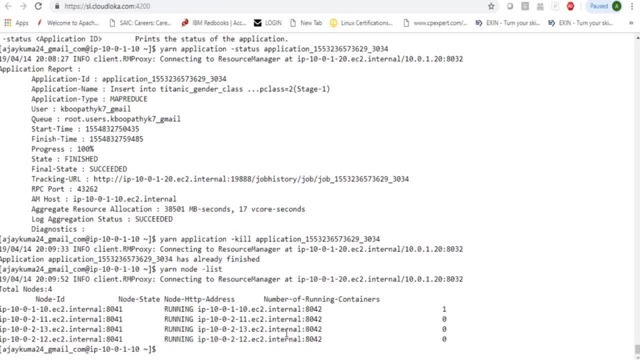 the node managers. now this is what we were looking from the yarn web ui and we were pulling out the information so we can get this and kind of information from your command line. always remember and always try to be well accustomed with the command line so you can do various 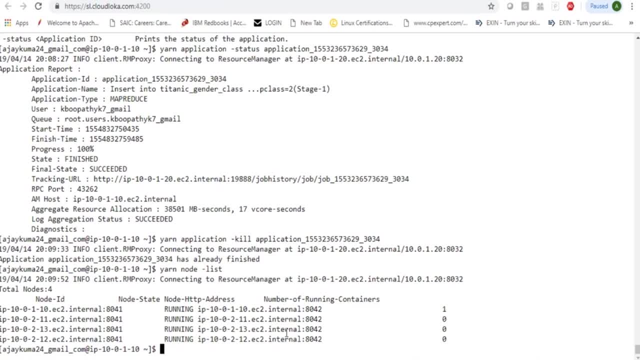 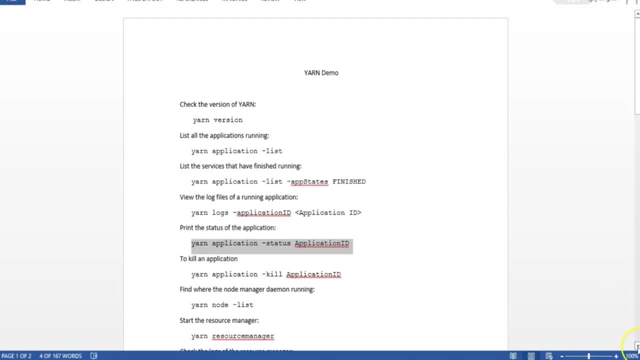 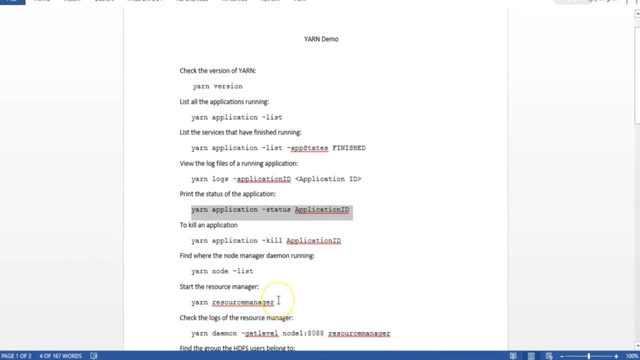 things from the command line, and then obviously you have the web uis, which can help you with a lot of things. now you could be also starting the resource manager, which we would not be doing here because we are already running in a cluster. so you could give a yarn, resource manager, you could. 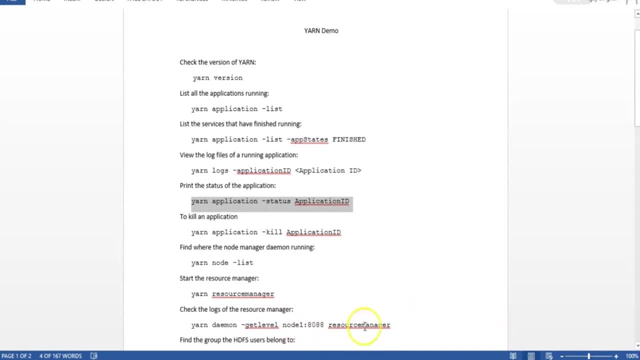 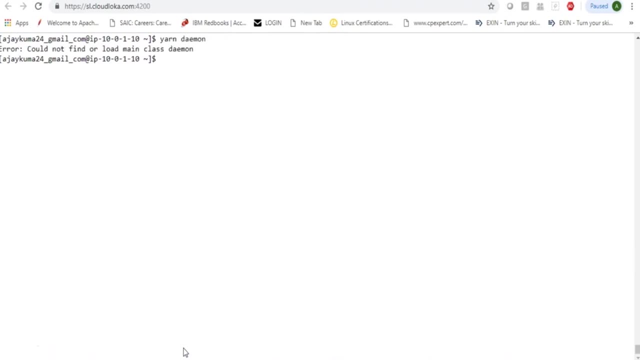 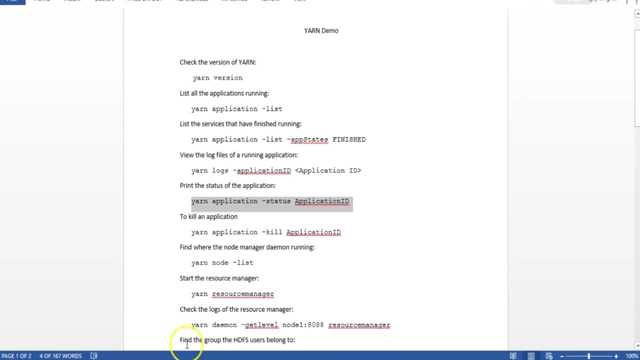 get the logs of resource manager, if you would want, by giving yarn, daemon, so we can try that, so you can say yarn and then daemon, so it says it does not find the daemon. so you can give something like this: get level, and here i will have to give the node and the resource manager and then i will give. 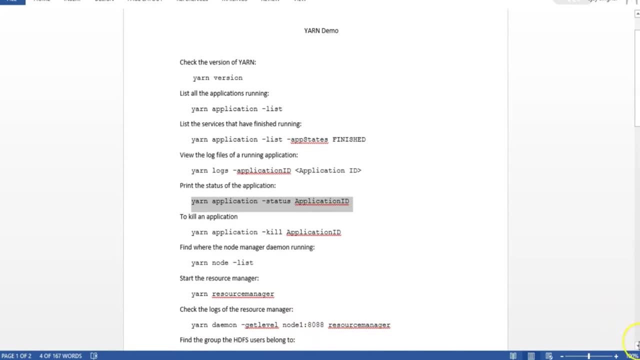 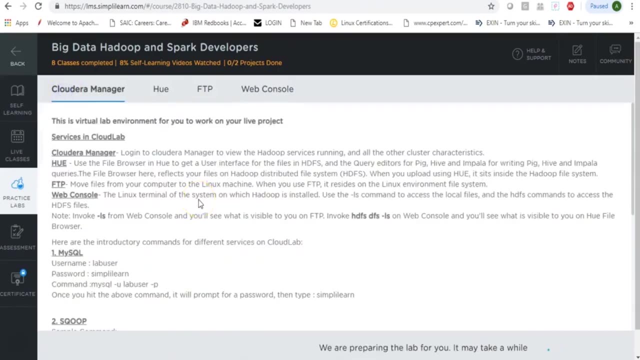 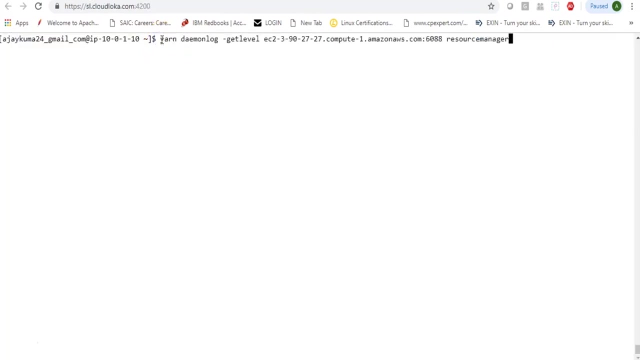 the IP address where you want to check the logs of resource manager. so you could be giving this, for which we will have to then get into cloud data manager to look into the nodes and the ip address. you could be giving a command, something like this, which basically gives you the level of the log. 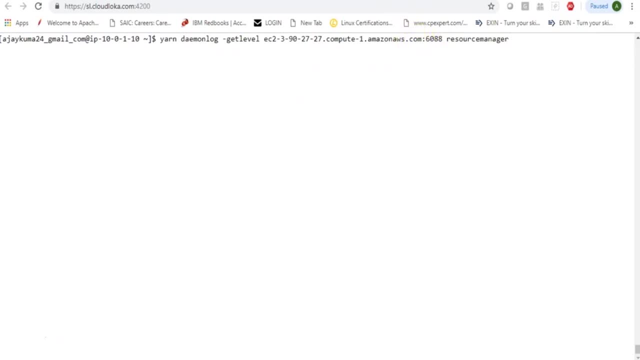 which you have and i got this resource manager address from the web ui. now i can be giving in this command to look into the daemon log and it basically says you would want to look at the resource manager related log and you have the log4j which is being used for logging the kind of level which has been set as info which can again 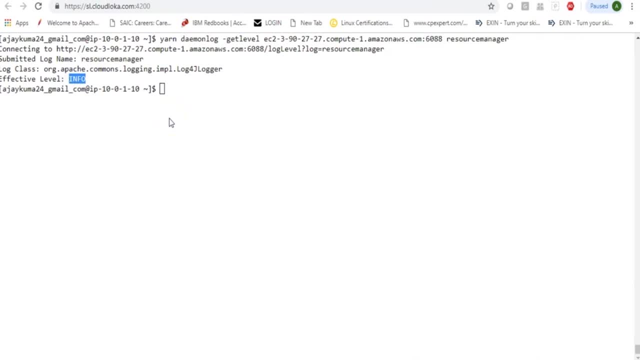 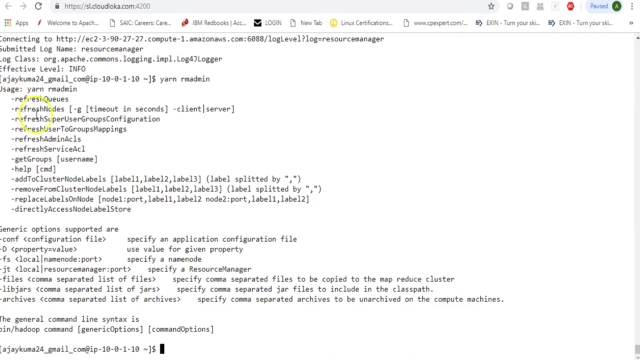 be changed in the way you are logging the information. now you can try any other commands, also from yarn, for example looking at the yarn rm admin, so you can always do a yarn rm admin and this basically gives you a lot of other informations, like you could be searching for a particular user or refreshing the nodes or basically looking at the. 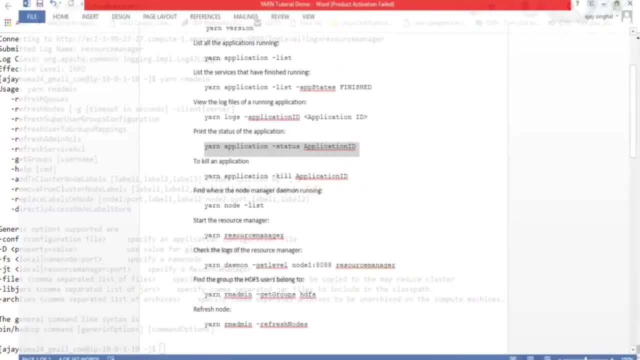 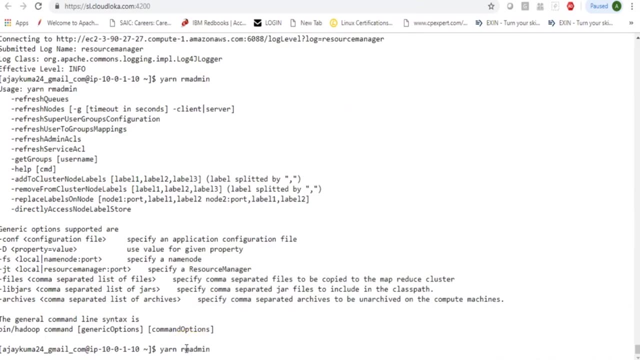 admin, acls or getting groups, so you could always get group names for a particular user. now we could search for a particular user, such as yarn or HDFS itself. so i could just say, here i would want get groups and then i could be searching for, say, username HDFS. so that tells me HDFS belongs to. 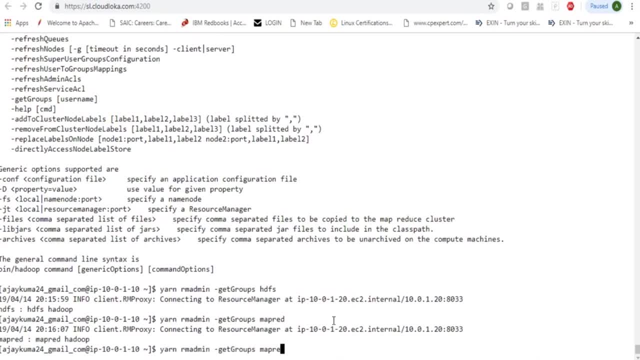 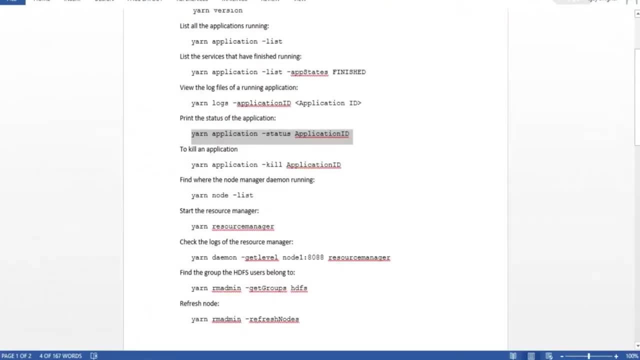 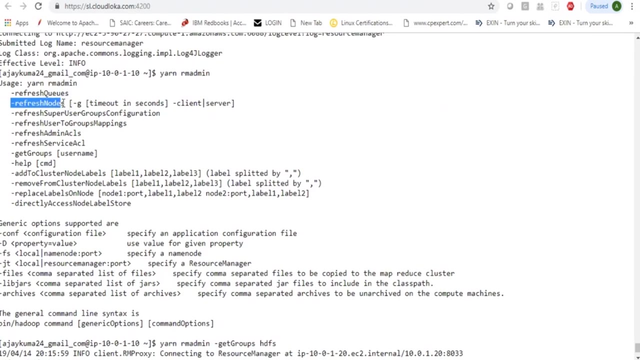 similarly you could search for, say, map read or you could search for yarn. so these are service related users which automatically get created and you can pull out information related to these. you can always do a refresh nodes kind of command and that is mainly done internally. this can be. 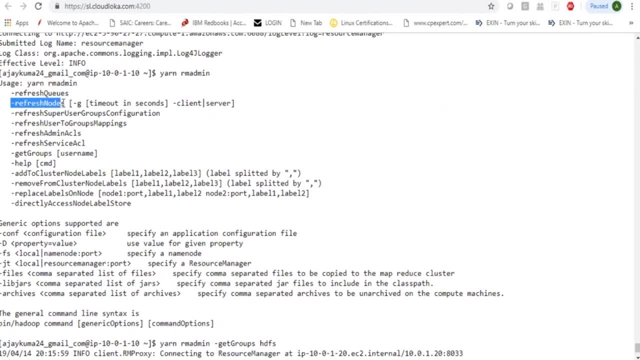 useful when you are doing commissioning decommissioning. but then in case of cloud error or hortonworks kind of cluster, you would not be manually giving this command, because if you are commissioning decommissioning from an admin console and if you are an administrator then you 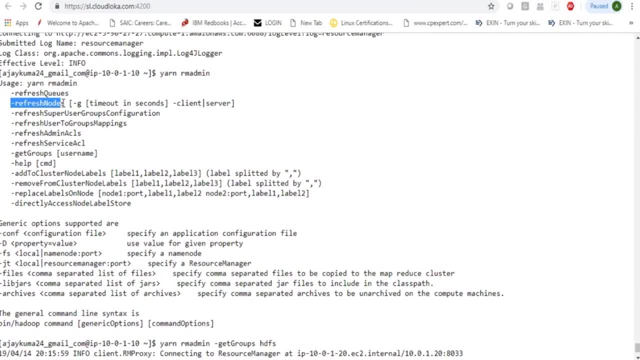 could just restart the services which are affected and that will take care of this. but if you were working in an apache cluster and if you were doing commissioning decommissioning, then you would be using in two commands, refresh nodes and basically that's for refreshing the nodes which should not. 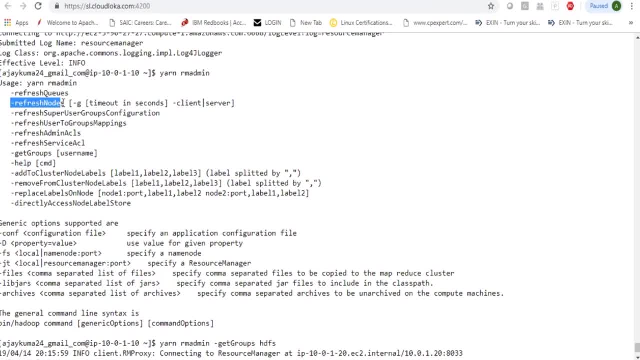 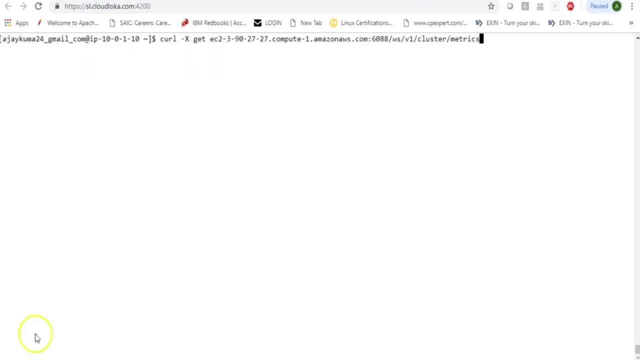 be used for processing, and similarly you could have a command refresh nodes which comes with HDFS. so these are different options which you can use with your yarn on the command line. you could also be using curl commands to get more information about your cluster by giving curl minus x and 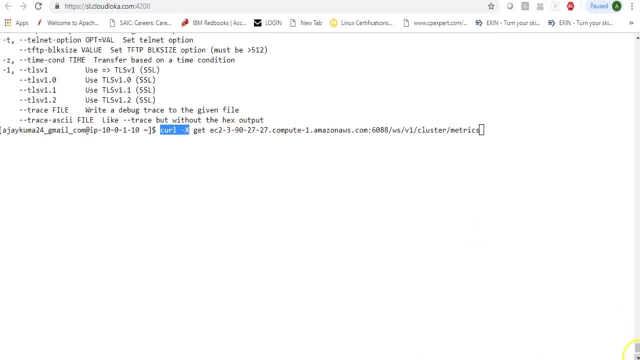 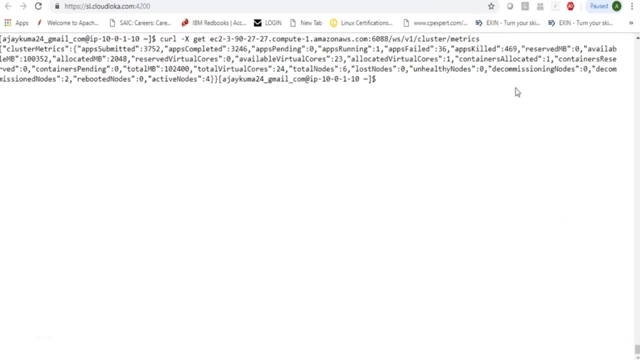 then basically pointing out to your resource manager web ui address. now here i would like to print out the cluster related metrics and i could just simply do this, which basically gives me a high level information of how many applications are there and how many applications are there, and 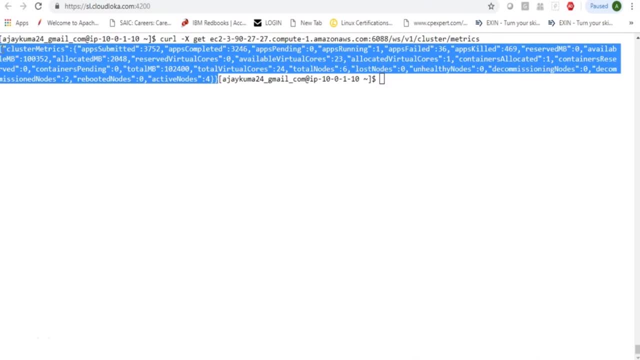 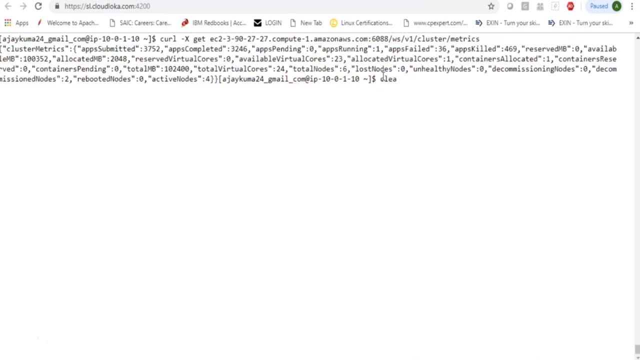 how many applications were submitted, how many are pending, what is the reserved resources, what is the available amount of memory or cpu cores and all the information. similarly, you can be using the same curl commands to get more information like scheduler information, so you would just replace the metrics with scheduler and you could get the information of the different queues. now that's a. 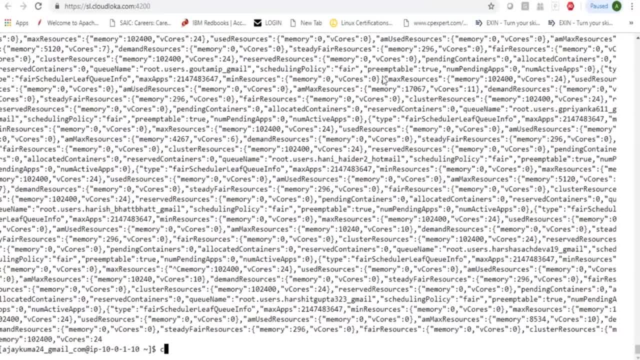 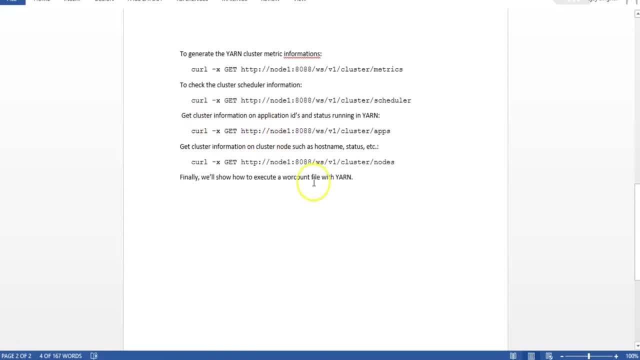 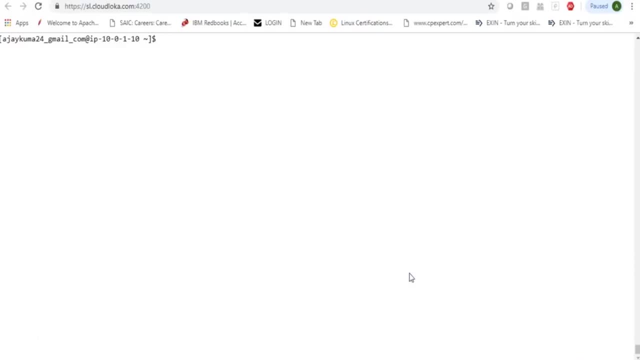 huge list. we can cancel this and that would give me a list of all the queues which are allocated, the resources allocated for each queue. you could also get cluster information on application ids and status running of applications running in yarn. so you would have to replace the last. 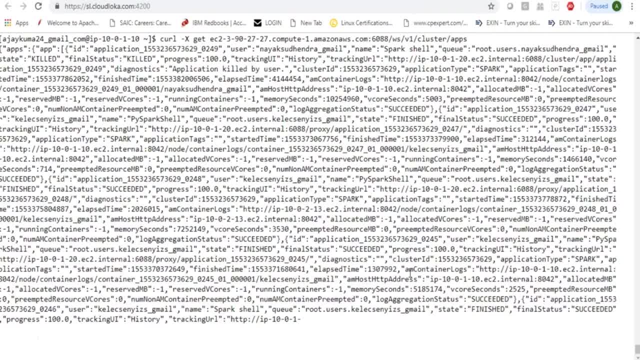 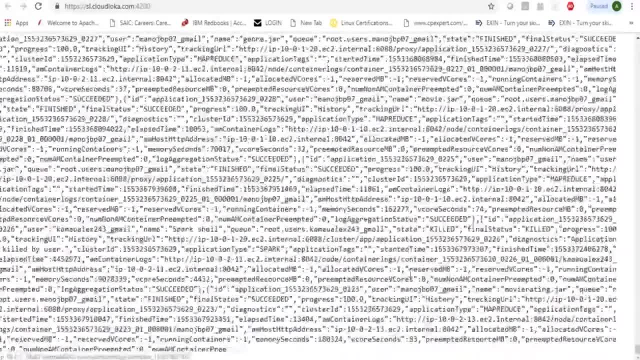 bit of it and you would say i would want to look at the applications and that gives me a huge list of applications. then you can do a grip and you can be filtering out specific application related information. similarly, you can be looking at the nodes, so you can always be. 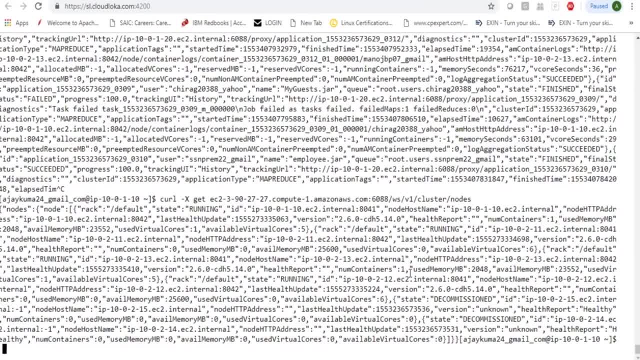 looking at node specific information which gives you how many nodes you have. but this could be mainly used when you have an application which wants to, or a web application which wants to use a curl command and would want to get information about your cluster from an http interface. 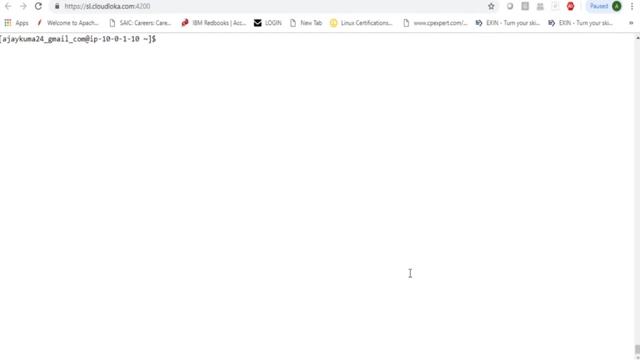 now, when it comes to application, we can basically try running a simple or a sample map, reduced job, which could then be triggered on yarn, and it would use the resources. now i can look at my application here and i can be looking into my specific directory, which is this: 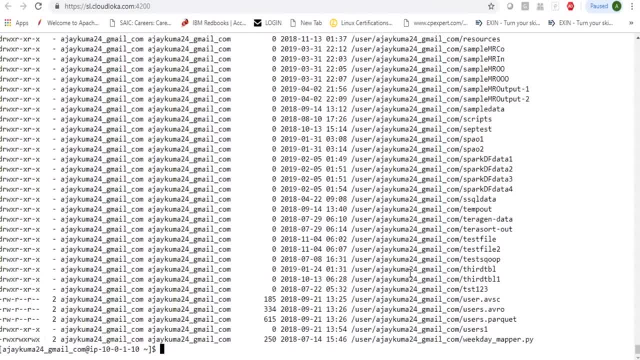 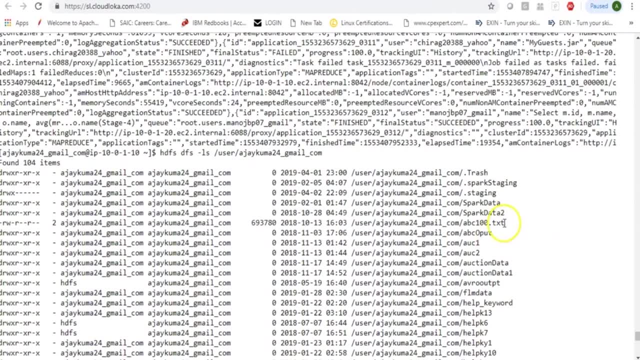 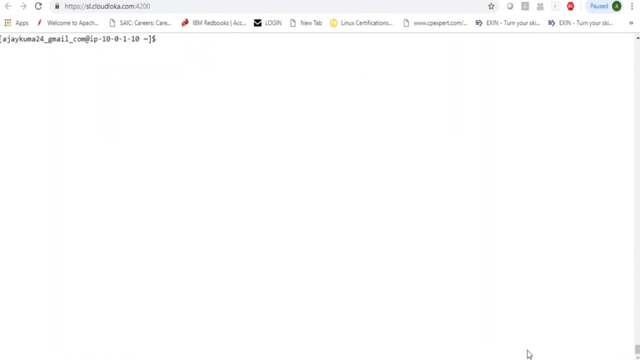 one which should have a lot of files and directories which we have here now. i could pick up one of these and i could be using a simple example to do some processing. let's take up this file, so there is a file and i could run a simple word count or i could be running a hive query. 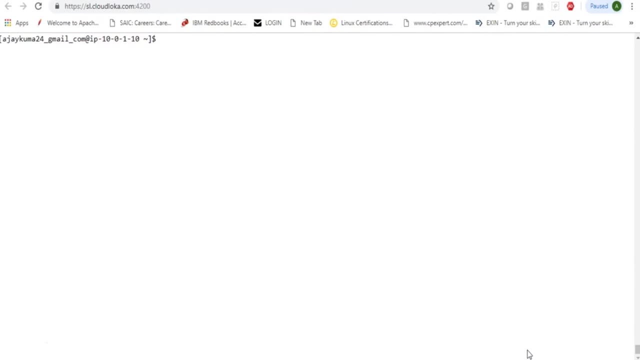 which triggers a map reduce job. i could even run a spark application, which would then show that the application is running on the cluster. so, for example, if i would say spark to shell- now, i know that this is an interactive way of working with spark, but this internally triggers. 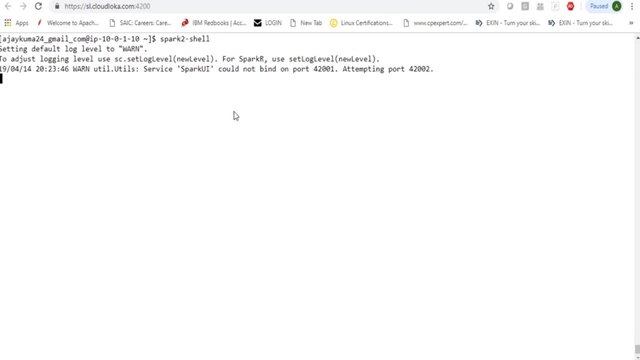 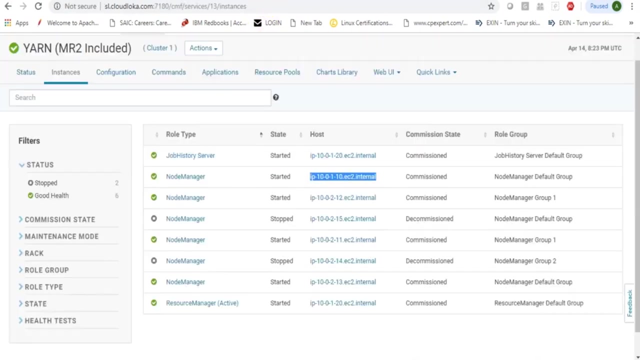 a spark submit and this runs an application. so here, when you do a spark to shell, by default it will contact yarn. so it gets an application id. it is running on yarn, with the master being yarn, and now i have access to the interactive way of working with spark. now, if i go, 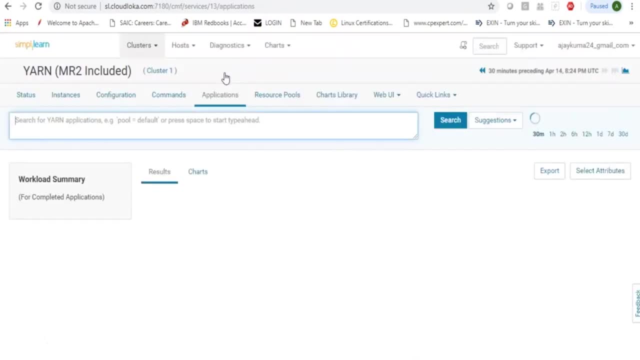 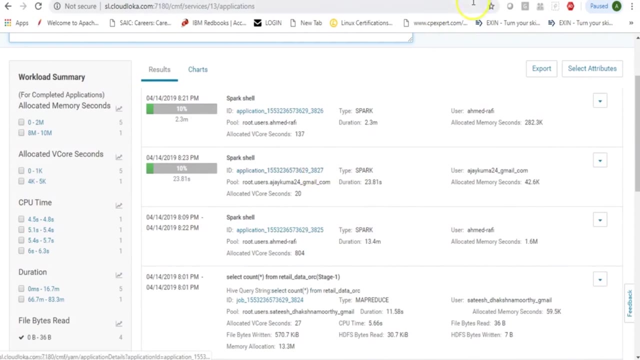 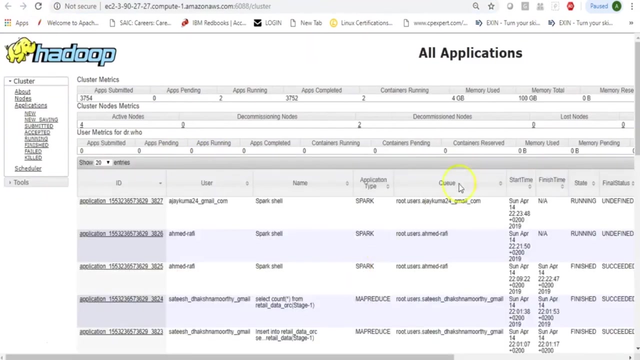 and look into applications, i should be able to see my application which has been started here and it shows up here. so this is my application 3827 which has been started on yarn, and as of now we can also look into the yarn ui, and that shows me the application which has been started, which. 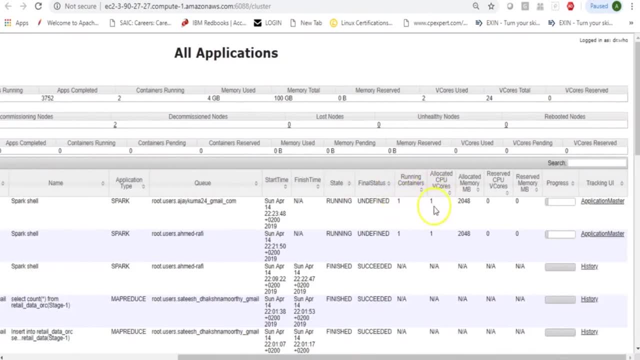 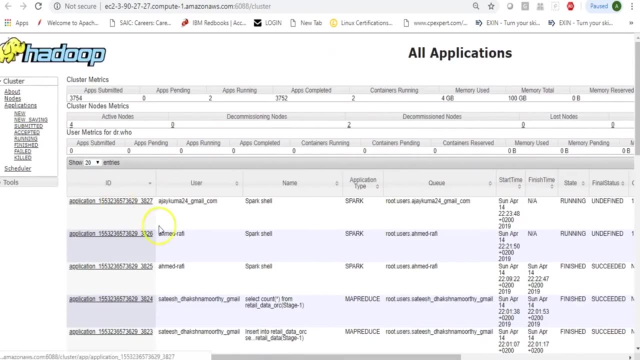 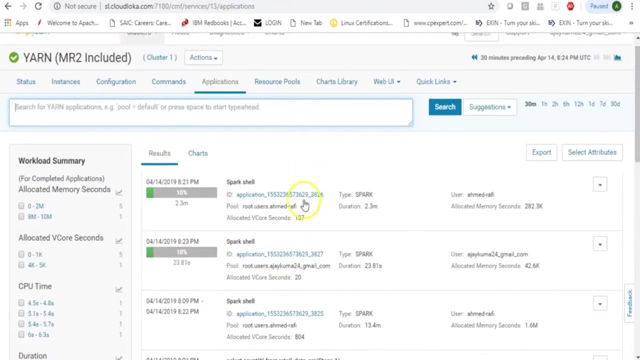 basically has one running container which has one cpu core allocated 2 gb ram, and it's in progress, although we are not doing anything there. so we can always look at our applications from the yarn ui or, as i mentioned, from your applications tab within yarn services, which gives us the information, and you can even click on this. 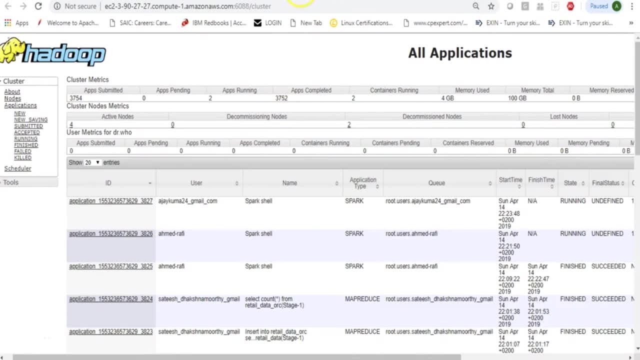 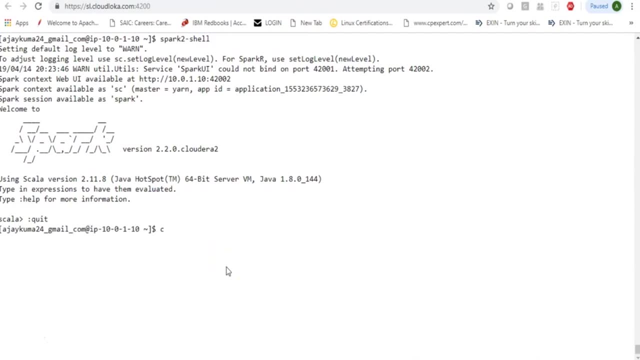 application to follow and see more information, but you should be given access to that now. this is just a simple application which i triggered using spark shell. similarly, i can basically be running a map reduce. now, to run a map reduce, i can say hadoop, jar and that. 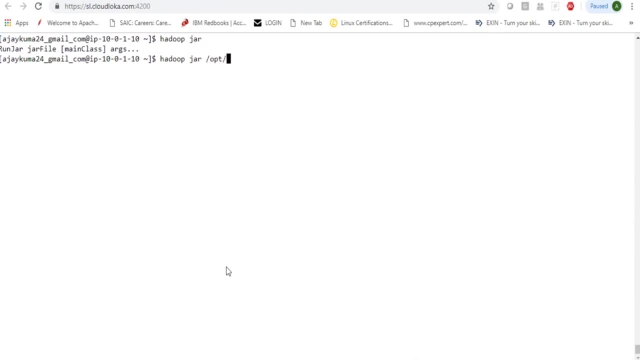 basically needs a class. so we can look for the default path, which is opt, cloud era parcels, cdh, lib, hadoop map reduce. hadoop map reduce examples. and then we can look at this particular jar file and if i hit on enter, it shows me the different classes which are part of this jar. 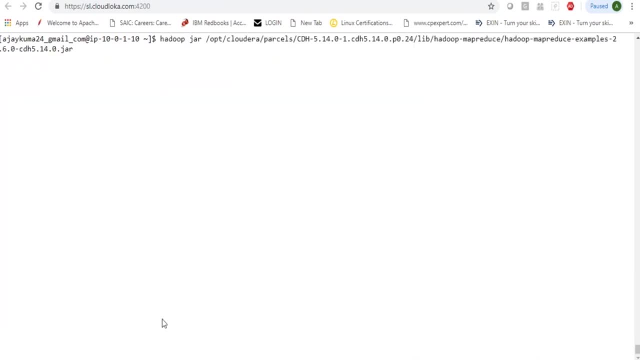 and here i would like to use word count, so i could just give this. i could say word count. now, remember, i could run the job in a particular queue by giving in an argument here. so i could say minus d map, red, dot job, dot, q, dot, name, and then i can point my job to a particular queue. i can even 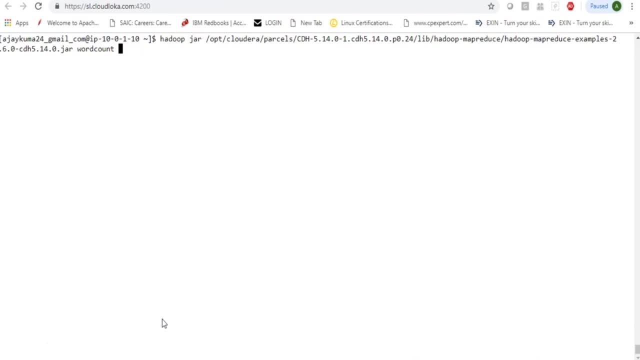 give different arguments in saying i would want my map reduce output to be compressed, or i want it to be stored in a particular directory, and so on. so here i have the word count and then basically what i can be doing is i can be pointing it to a particular input path. 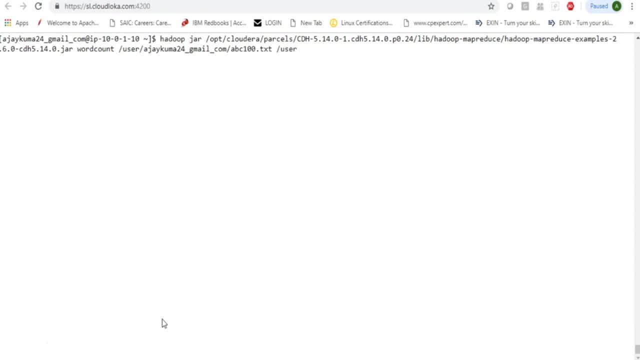 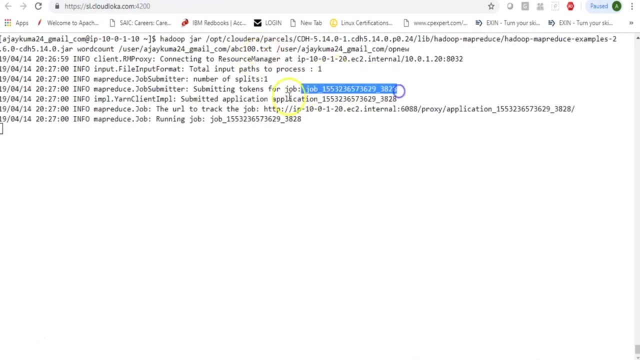 and then i can have my output which can be getting stored here again a directory which we need to choose, and i will say output new and i can submit my job. now, once i have submitted my job, it connects to resource manager. it basically gets a job id, it gets an application id. 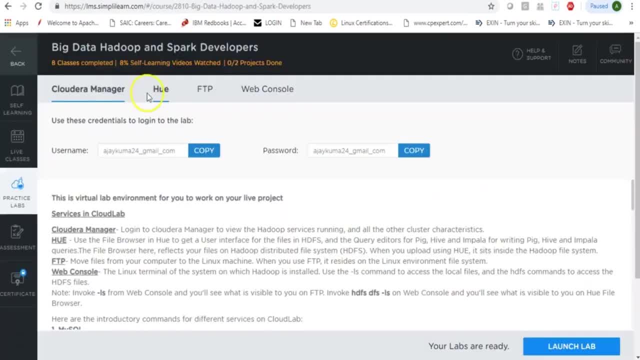 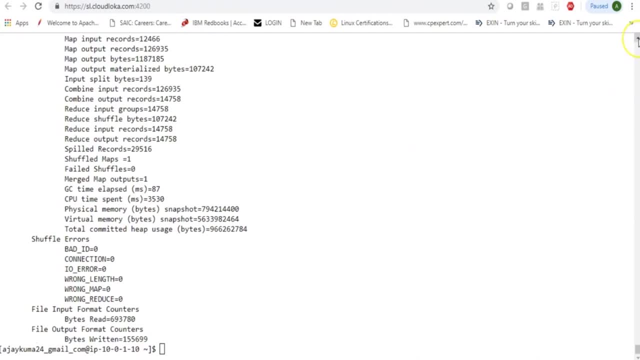 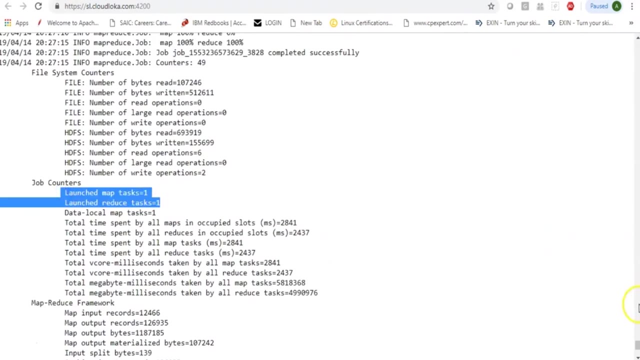 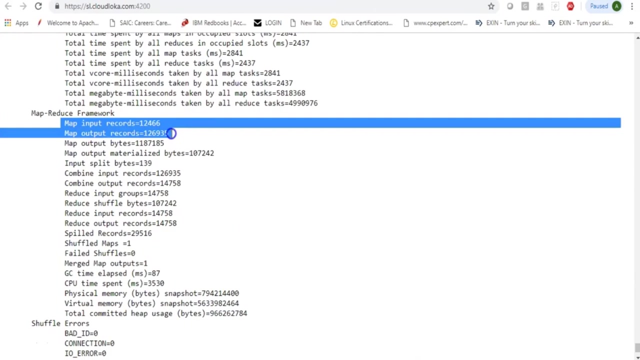 it shows you from where you can track your application. you can always go to the yarn ui and you can be looking at your application and the resources it is using. so my application was not a big one and it has already completed. it triggered one map task, it launched one reduced task. it was working on around 12 466 records, where you have then the 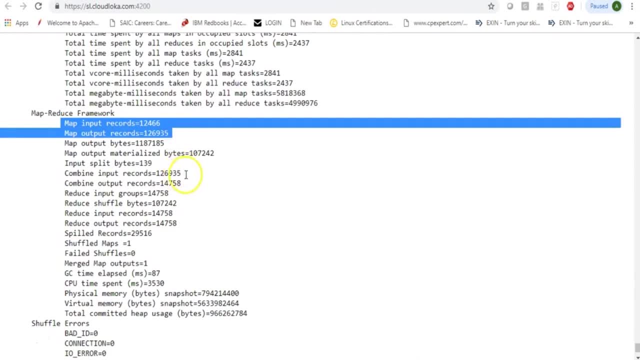 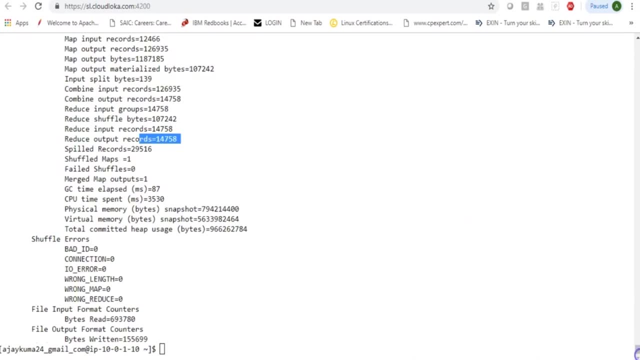 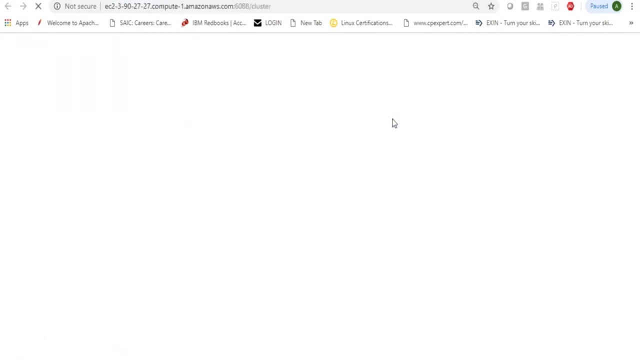 output of map, which is these many number of output records, which was then taken by a combiner and finally by a reducer, which basically gives you the output. so this is my yarn application, which has completed. now i could be looking into the yarn ui and if my job has completed, you might not see your application here. so as of now it shows up. 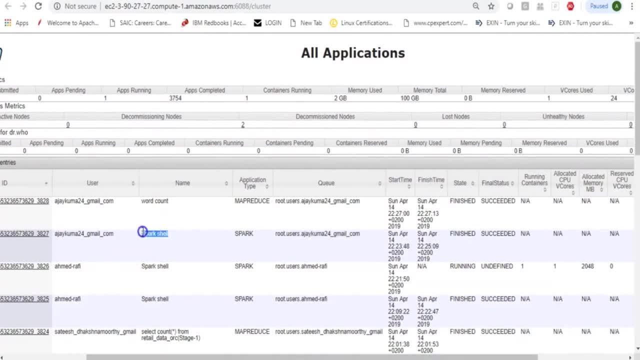 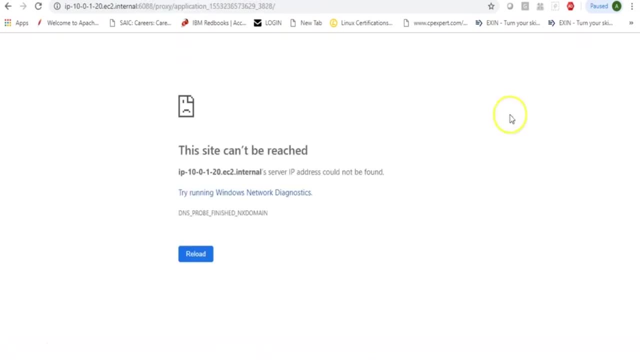 here the word count which i ran. it also shows me my previous spark shell job. it shows me my application is completed and if you would want further information on this, you can click and go to the history server if you have been given access to it, or directly go to the history server. 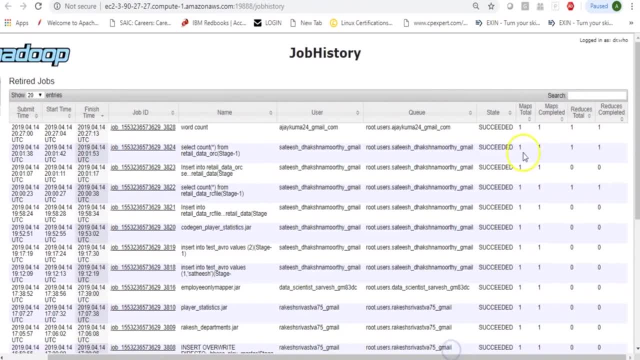 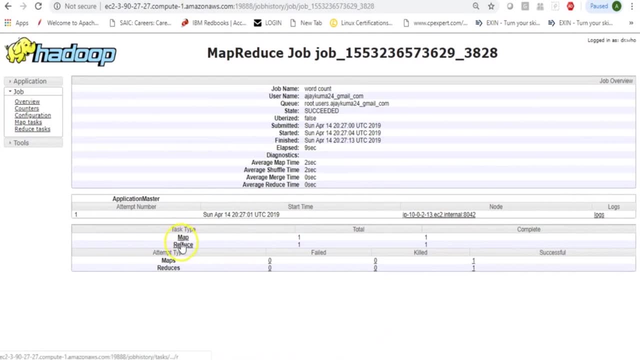 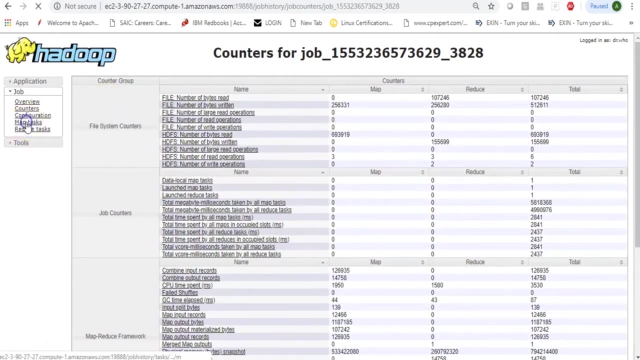 web ui where your application shows up. it shows how many map and reduced tasks it was running. you can click on this particular application which basically gives you information of your map and reduced tasks. you can look at different counters for your application. right, you can always look at map specific tasks. you can always look into one particular task, what it did on which. 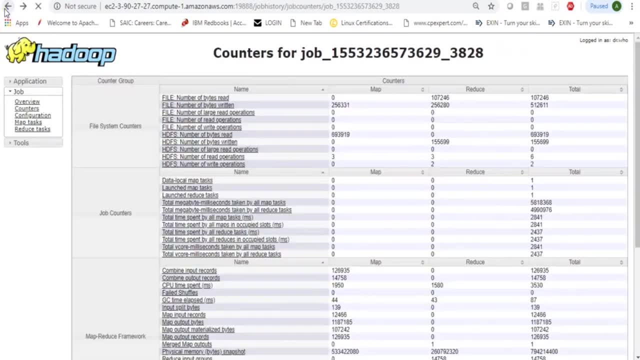 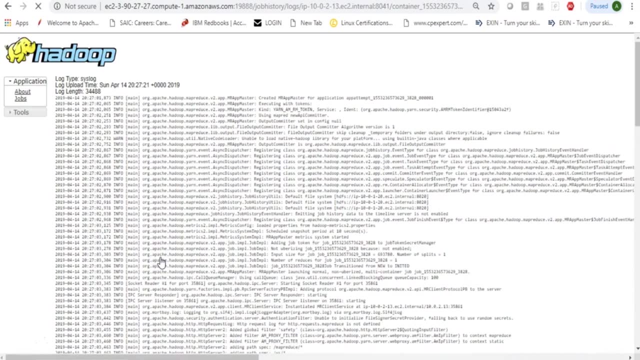 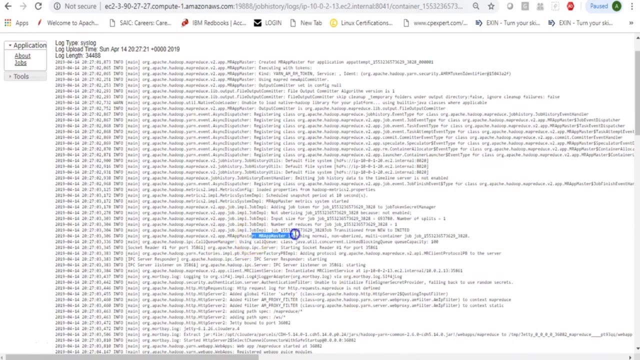 node it was running or you can be looking at the complete application log so you can always click on the logs, and here you have. click here for full log, which gives you the information, and you can look for your application, which can give you information of app master being launched or you. 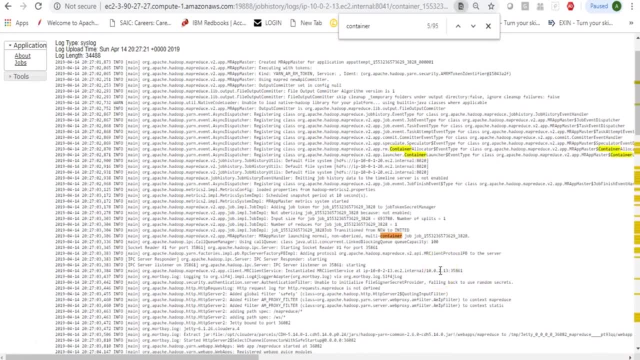 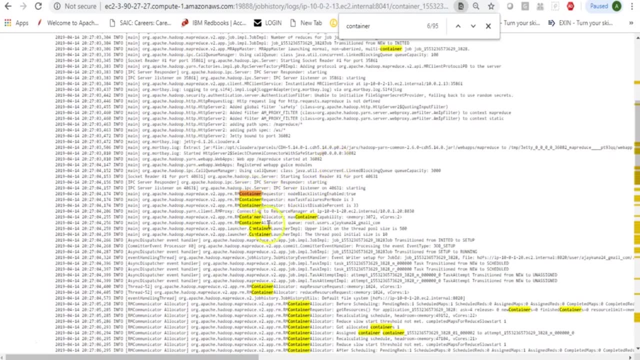 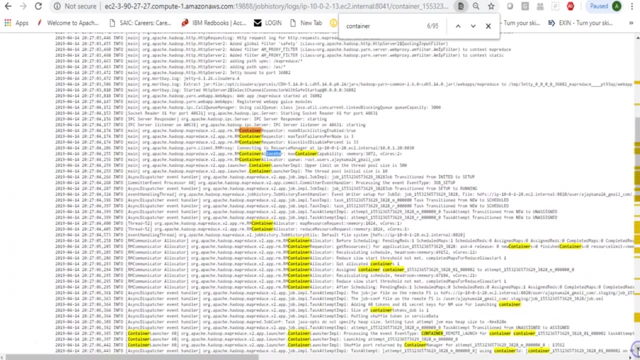 could have search for the word container, so you could see a job which needs one or multiple containers, and then you could say container is being requested, then you could see container is being allocated, then you can see what is the container size and then basically your task moves. 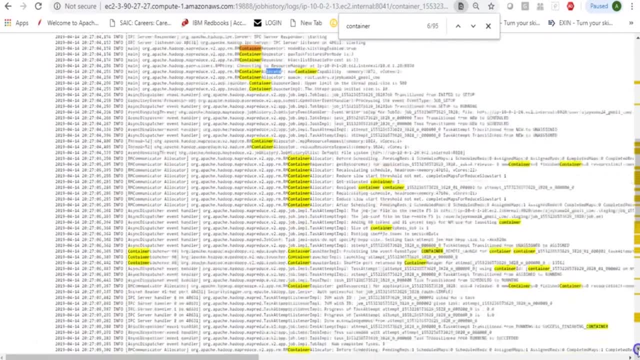 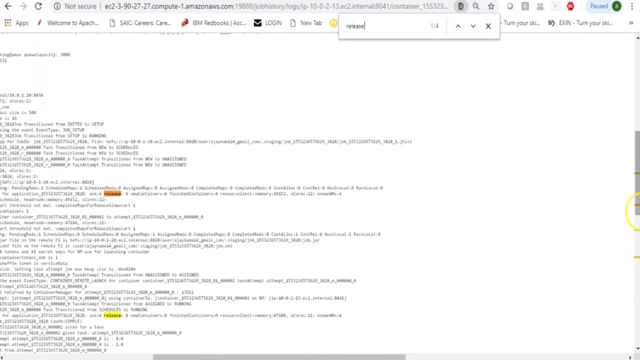 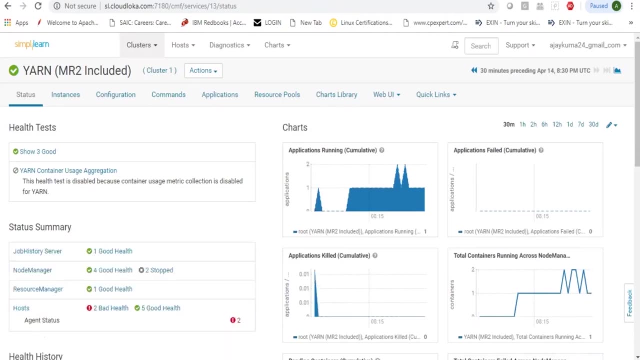 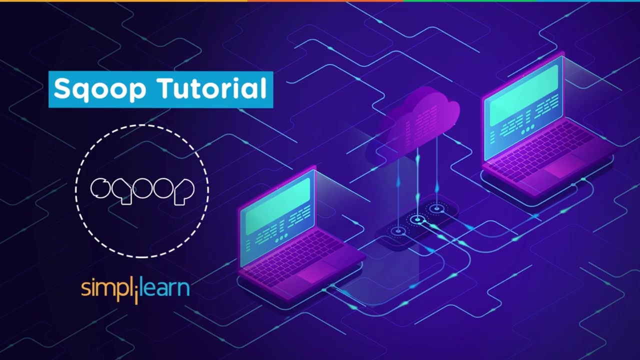 from initializing to running in the container and finally, you can search for release, which will tell you that the container was released, so you can always look into the log for more information. so this is how you can interact with the yarn. this is how you can interact with your command line to look for more information, or using your yarn web ui. my name is. 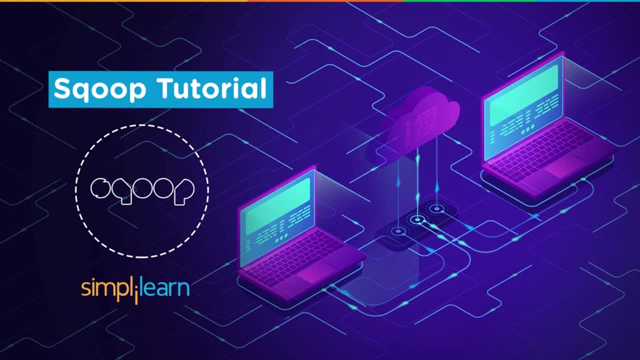 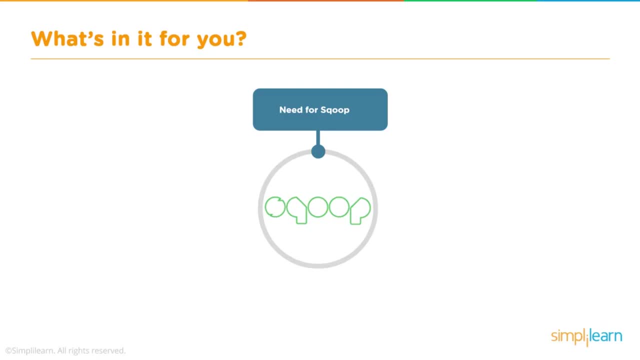 richard kirchner. i am with the simply learn team that's wwwsimplylearncom: get certified, get ahead. today we're going to dive in on scoop, one of the many features that we're going to be talking about. today. we're going to talk about the features of the hadoop ecosystem for the hadoop file system. 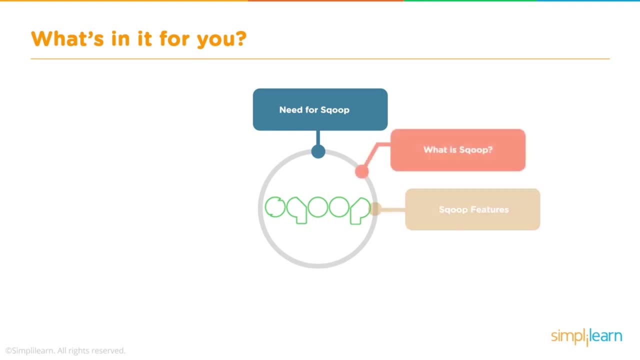 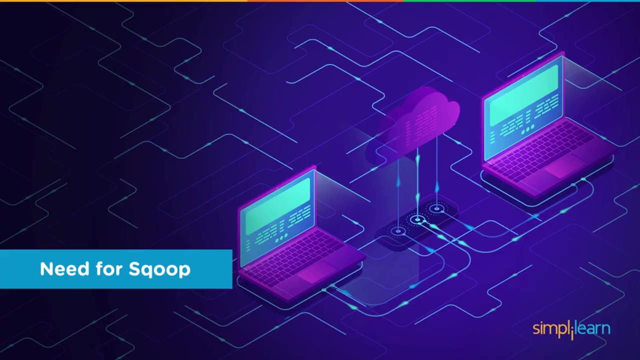 what's in it for you. today, we're going to cover the need for scoop. what is scoop, scoop features, scoop architecture, scoop import, scoop export, scoop processing, and then, finally, we'll have a little hands-on demo on scoops. you can see what it looks like. so where does the need for scoop come in in? 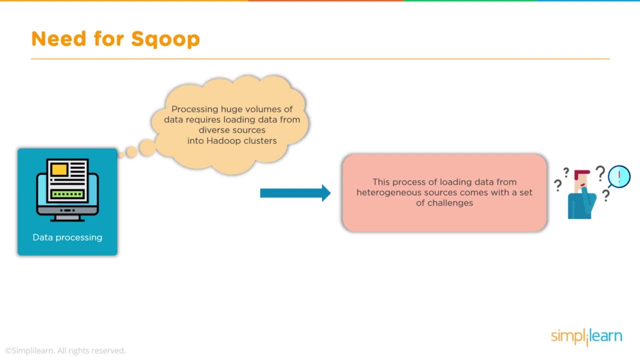 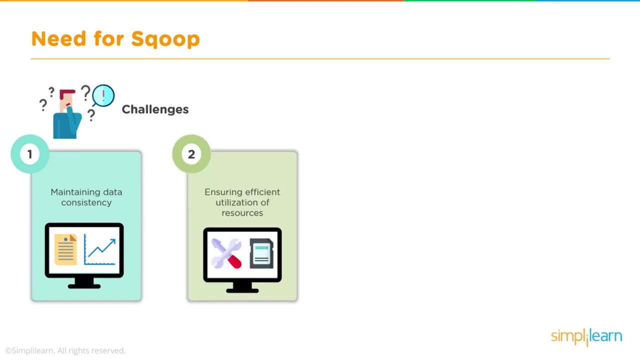 our big data hadoop file system. processing huge volumes of data requires loading data from diverse sources into hadoop cluster. you can see, here we have our data processing. this process of loading data from the heterogeneous sources comes with a set of challenges. so what are the challenges? maintaining data consistency. ensuring efficient utilization of. 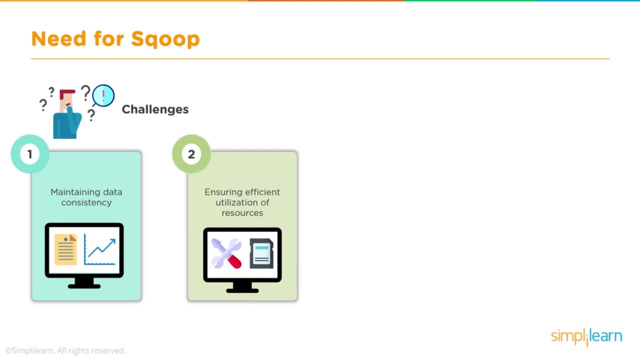 resources, especially when you're talking about big data. we can certainly use up the resources when importing terabytes and petabytes of data over the course of time. loading bulk data to hadoop was not possible. it's one of the big challenges that came up when they first had the 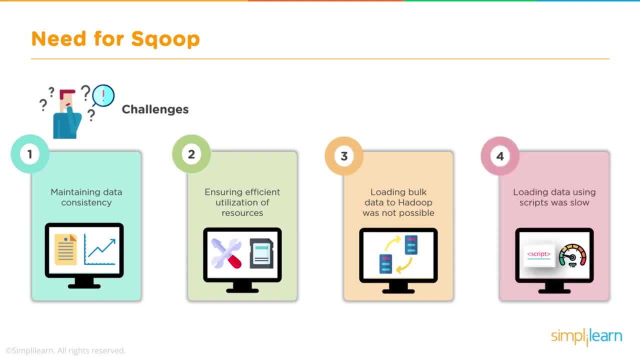 hadoop file system going and loading data using script was very slow. in other words, you'd write a script and whatever load the data was going to have to do with the data that was going to be stored over language you're in and then it would very slowly load each piece and parse it in. so the 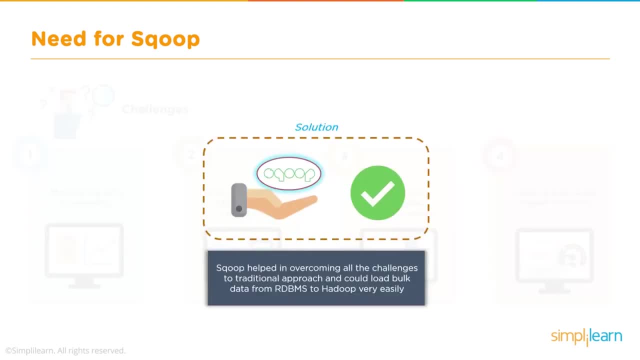 solution scoop. scoop helped in overcoming all the challenges to traditional approach and could lead bulk data from rdbms to hadoop very easily. so think your enterprise server. you want to take the from mysql or your sql and you want to bring that data into your hadoop warehouse. your data filing. 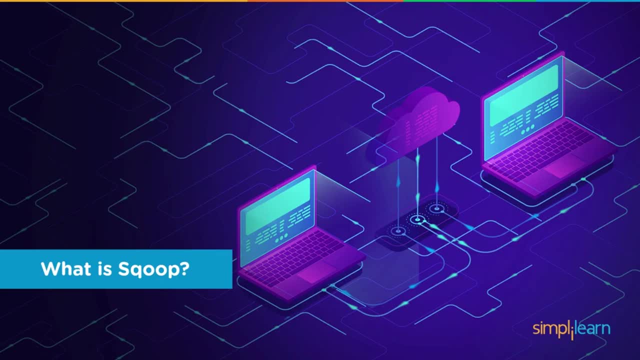 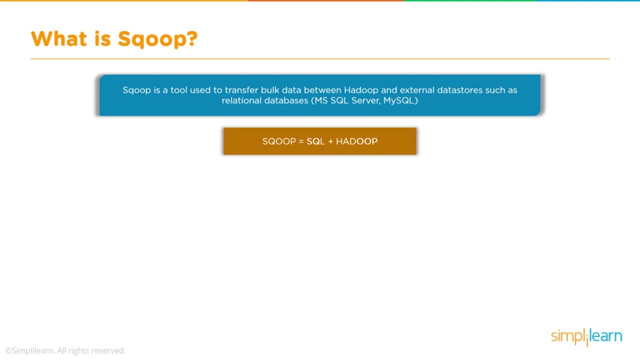 system, and that's where scoop comes in. so what exactly is scoop? scoop is a tool used to transfer data from hadoop and external data storage, such as relational databases and mysql server or the microsoft sql server or mysql server. so scoop equals sql plus hadoop, and you can see here we 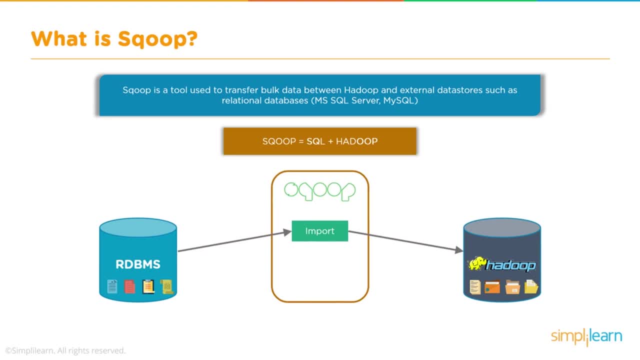 have our rdbms- all the data we have stored on there- and then your scoop is the middle ground and it brings the import into the hadoop file system. it also is one of the features that goes out and grabs the data from hadoop and exports it back out into an rdbms. let's take a look at scoop. 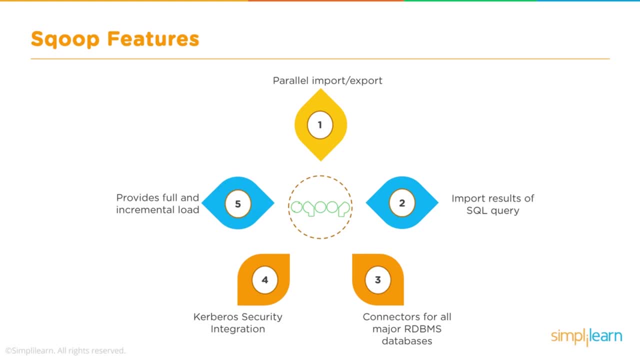 features has parallel import and export. it has import results of sql query connectors for all major rdbms databases. kerberos security integration provides full and incremental load. so we look at parallel import and export. scoop uses yarn, yet another resource negotiator framework, to import and export data. this provides fault tolerance on a top of parallelism. scoop allows us to import. 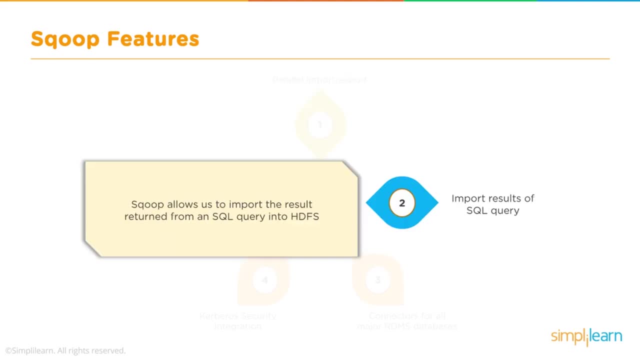 the result return from an sql carry into the hadoop server. so scoop allows us to import the result return from an sql carry into the hadoop server and then import the data into hadoop server. so scoop Duke file system or the HDFS and you can see here where the import results of SQL. 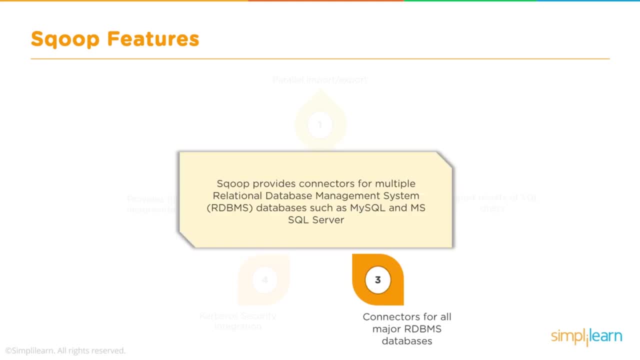 query come in. Scoop provides connectors for multiple relational database management system databases such as MySQL and Microsoft SQL Server, and it has connectors for all major RDBMS databases. Scoop supports Kerberos computer network authentication protocol that allows nodes communicating over a non secure network to prove their identity to one another in a secure. 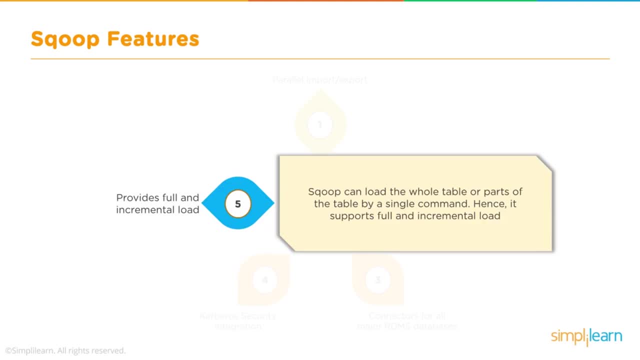 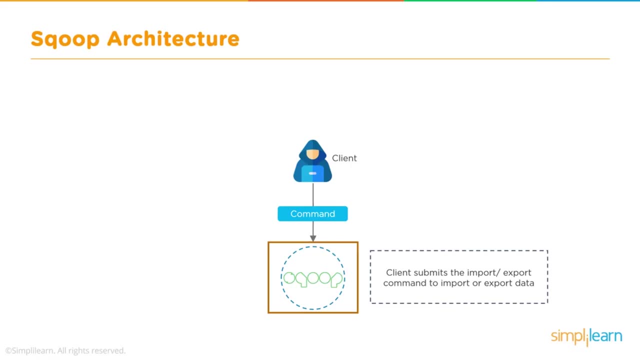 manner. Scoop can load the whole table or parts of the table by a single command. hence it supports full and incremental load. Let's dig a little deeper into the Scoop architecture. We have our client, in this case a hooded wizard- behind his 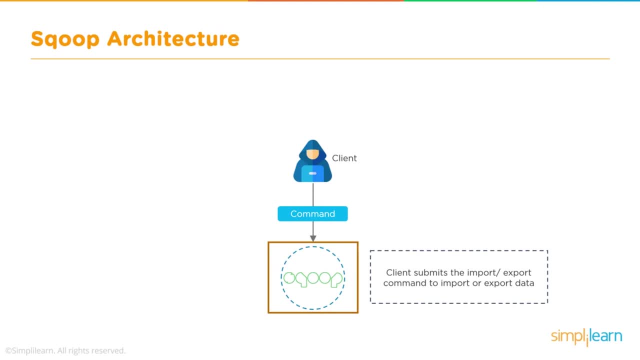 laptop, You never know who's going to be accessing the Hadoop cluster- And the client comes in and sends their command, which goes into Scoop. The client submits the import- export command to import or export data. Data from different databases is fetched by Scoop and so we have. 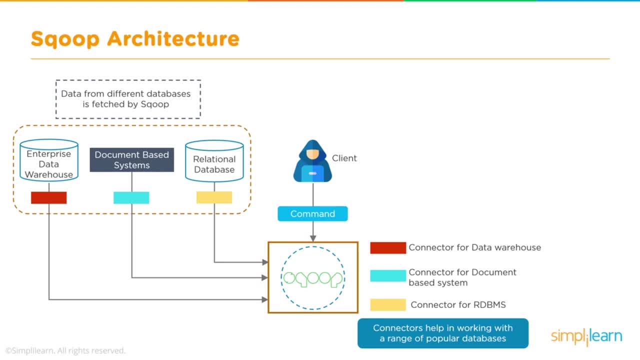 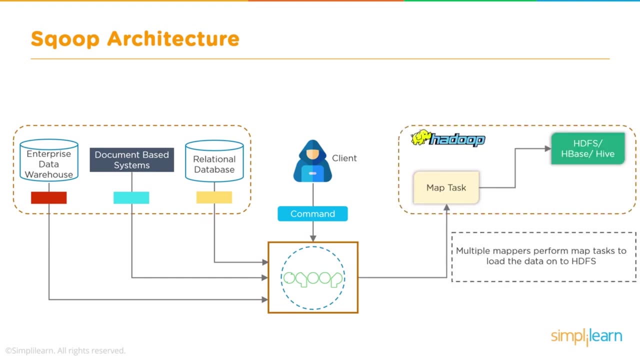 inter- brised data warehouse, document based systems. you have a connector for your data warehouse, a connector for document based systems, which reaches out to those two entities, and we have our connector for the RDBMS. So connectors help in working with a range of popular databases. Multiple mappers perform map. 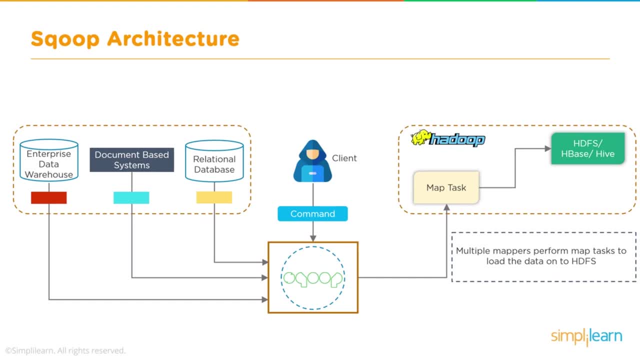 tasks to load the data onto HDFS, the Hadoop file system. You can see, here we have the map task, If you remember from Hadoop. Hadoop is based on MapReduce, Because we're not reducing the data, we're just mapping it over. It only accesses the mappers and it opens up multiple. 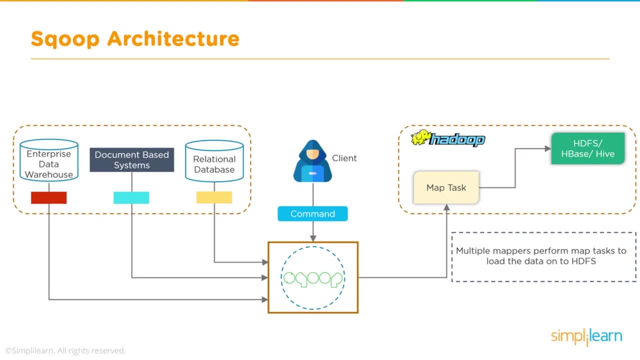 mappers to do parallel processing, And you can see here the HDFS HBase Hive is where the target is for this particular one. Similarly, multiple map tasks will export the data from HDFS on to RDBMS using scoop export command. So just like. 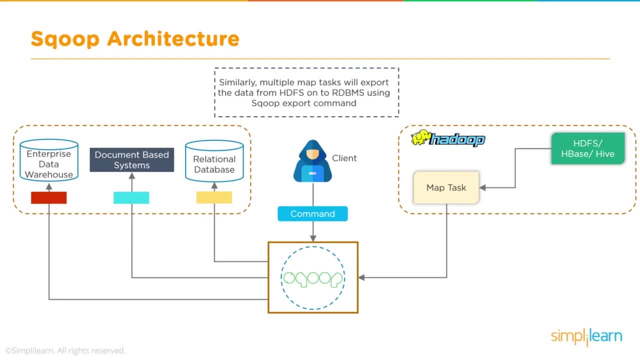 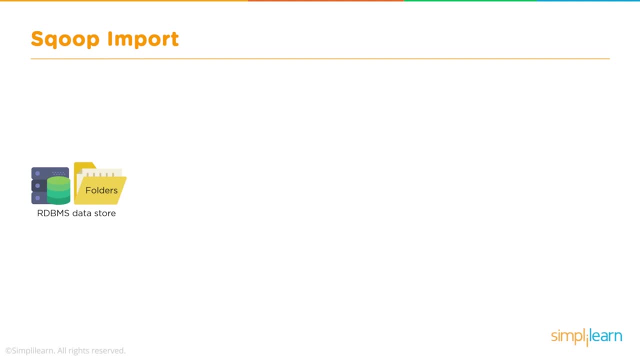 you can import it. you can now export it using the multiple map routines, Scoop import. So here we have RDBMS data store and we have the folders on there. so maybe it's your company's database, maybe it's an archive at Google, with all the searches going on. whatever it is, 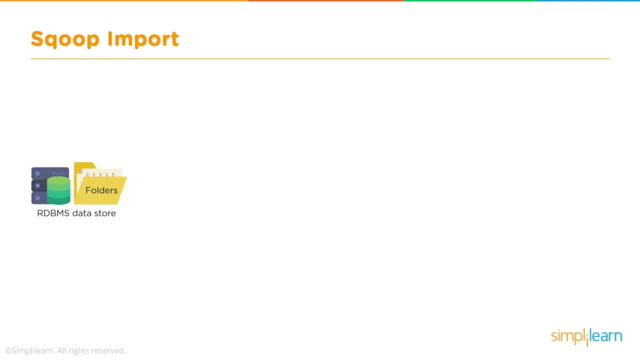 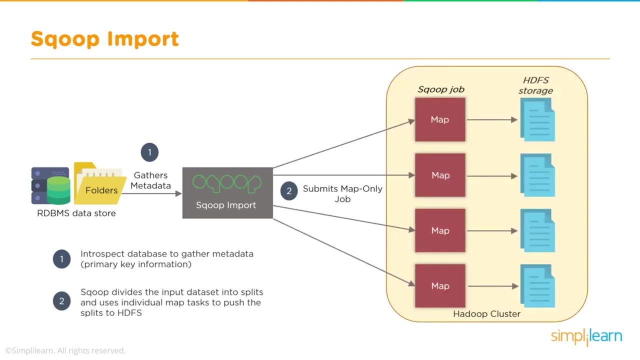 usually you think with scoop, you think SQL, you think my sequel server or Microsoft sequel server, that kind of setup. so it gathers the metadata and you see the scoop, import, so introspect database to gather metadata, primary key information, and then it submits so you can see, submits, map. only job, remember we. 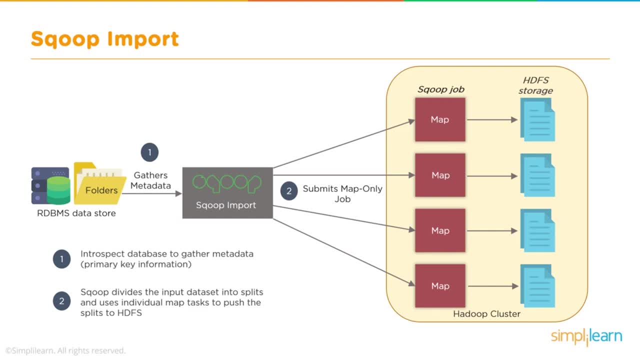 talked about MapReduce. it only needs the map side of it because we're not reducing the data, we're just mapping it over. scoop divides the input data set into splits and uses individual map tests to push the splits into HDFS, so right into the Hadoop file system and you can see down on the right is kind of. 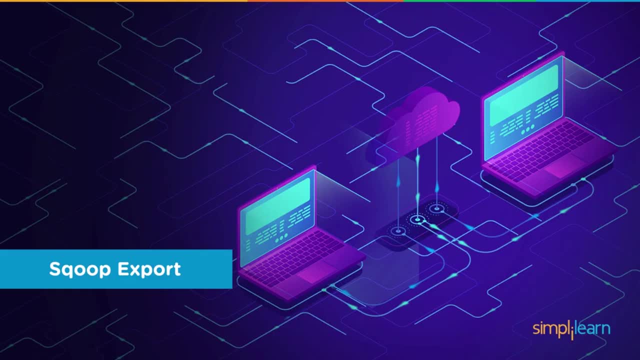 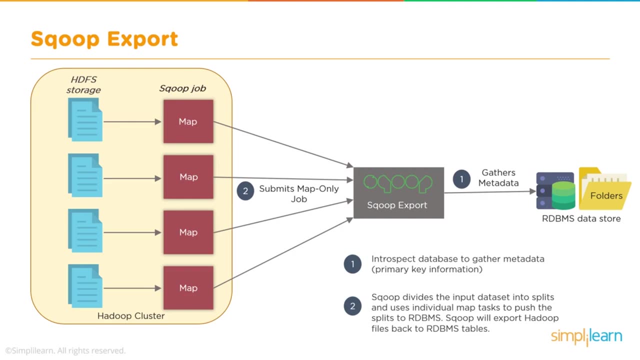 a small depiction of a Hadoop cluster and then you have scoop export. so we're gonna go the other direction. and with the other direction you have your Hadoop file system storage, which is your Hadoop cluster, you have your scoop job and each one of those clusters then gets a map mapper comes out to each one of the 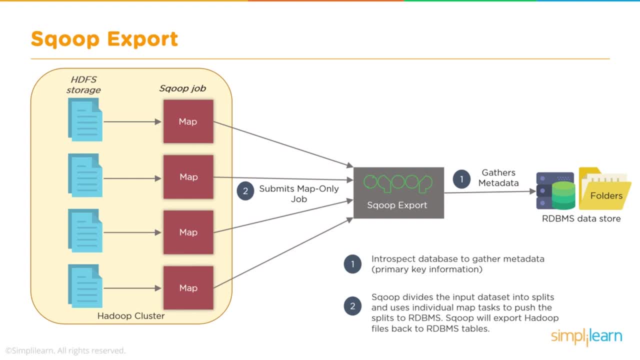 computers. and then you have the Hadoop cluster, and then you have the Hadoop web shooter Kubert форм. you've got the Hadoop cluster. so as a Scikit-learn it's going toividad- the people from devices. and then, while we're making these mapper orders that have 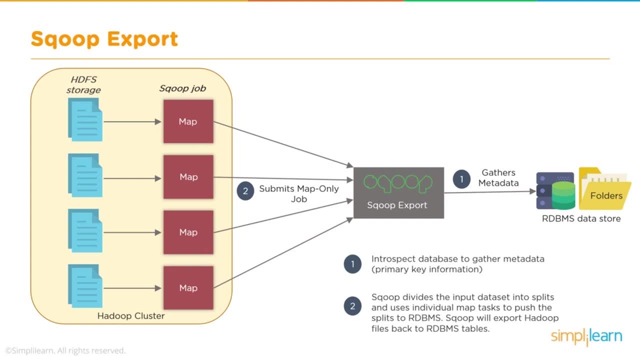 someimana memory. we're taking care of them and you take include. a hard remains- and you're going to have a lot of help with this bakedway- that you need to sort of create a system that has really network computer computers, that has data system into your enterprise machines. There's certainly many others. as far as 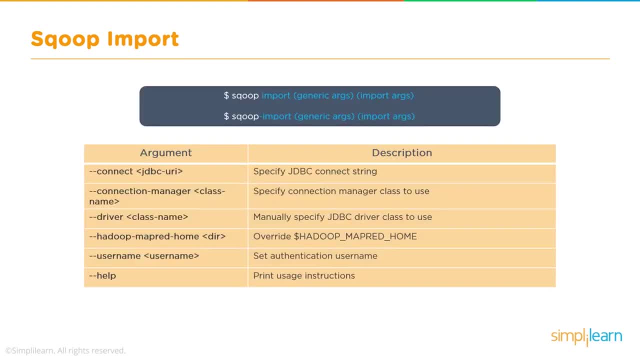 exploring data and data science. So as we dig a little deeper into scoop input, we have our connect, our JDBC and our URL. So specify the JDBC connect string Connecting manager. we specify the connection manager class to use. You can see here driver with the class name. manually specify the JDBC driver class. 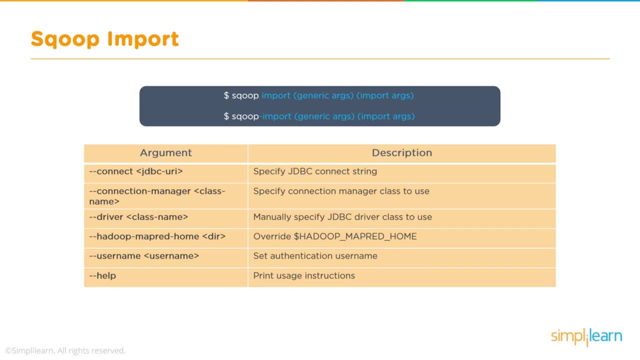 to use Hadoop map. reduce home directory, Override Hadoop mapped home Username, a set authentication username and, of course, help print users instructions. And with the export you'll see that we can specify the JDBC connect string, specify the connection manager class to use manually, specify new JDBC driver class. 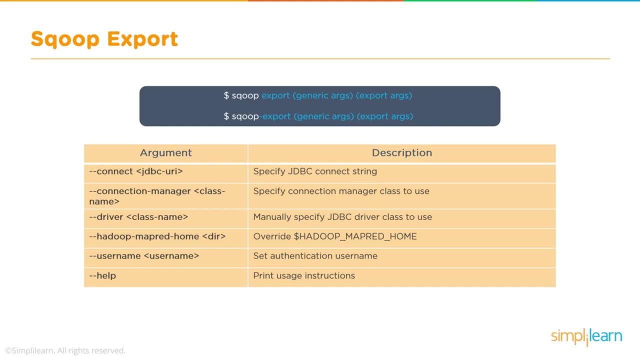 to use. you do have to let it know to override the Hadoop map, reduce home- and that's true on both of these- And set authentication username and finally you can print out all your help set up. So you can see. the format for scoop is pretty straightforward, both import and export. 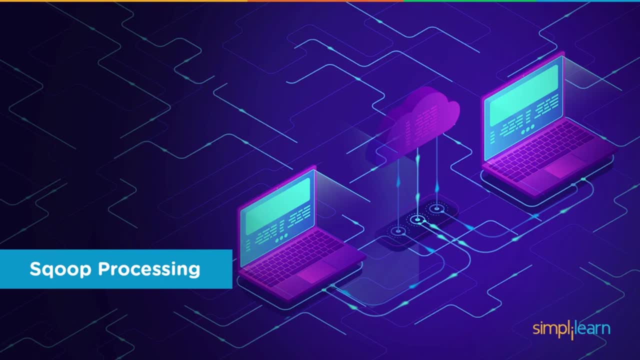 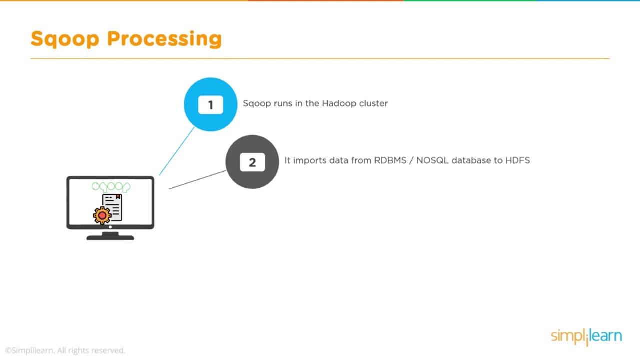 So. So let's continue on our path and look at scoop processing and what the computer goes through for that. And when we talk about scoop processing first, scoop runs in the Hadoop cluster. It imports data from the RDBMS, the NoSQL database, to the Hadoop file system. 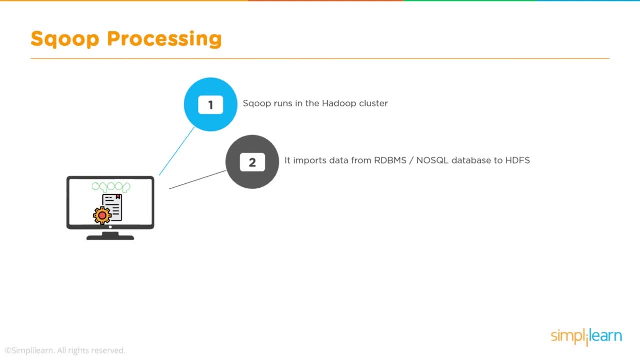 So remember, it might not be importing the data from a RDBMS, it might actually be coming from a NoSQL, and there's many out there. It uses mappers to slice the incoming data into multiple formats and load the data into HDFS. 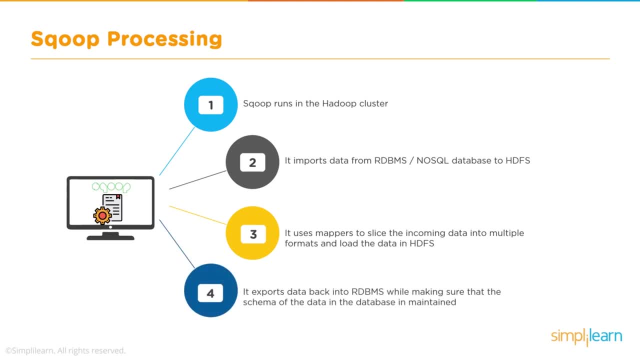 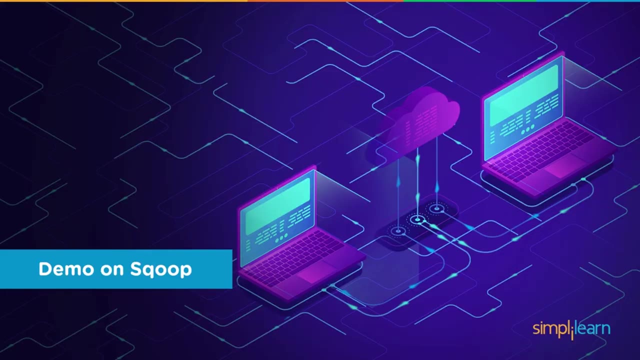 It exports data back into an RDBMS, while making sure that the schema of the data in the database is maintained. So now that we've looked at the basic commands in our scoop and the scoop processing- or at least the basics as far as theory is concerned- let's just jump in and take a look at a demo. 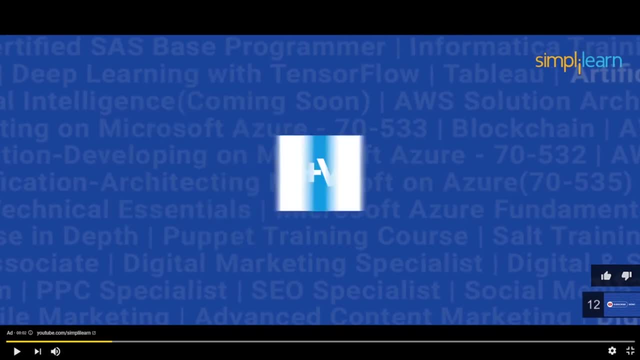 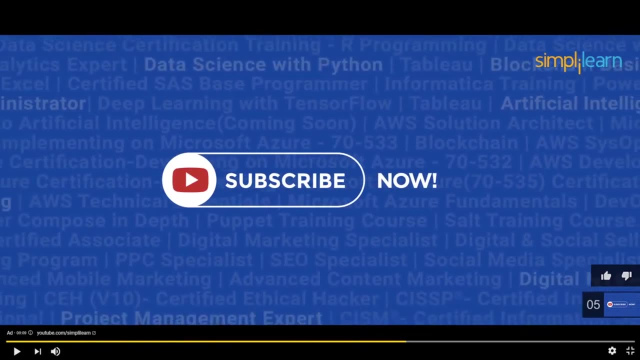 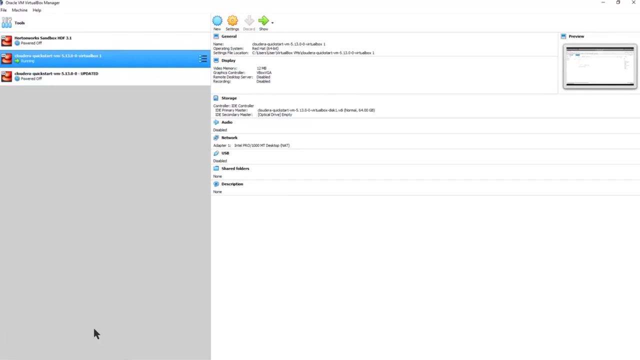 on scoop For this demo. I'm going to use our Cloudera Quickstart. If you've been watching our other demos we've done, you'll see that we've been using that pretty consistently. Certainly this will work in any of your Horton Sandbox, which is also a single-node testing. 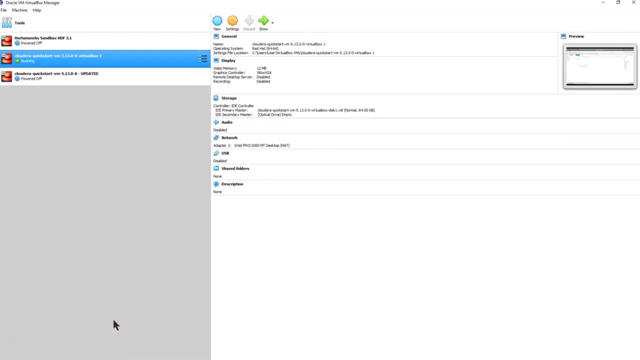 machine. Cloudera is one of them. There's a Docker version instead of VirtualBox and you can also set up your own Hadoop cluster Plan. a little extra time. If you're not an admin, it's actually a pretty significant amount of time. 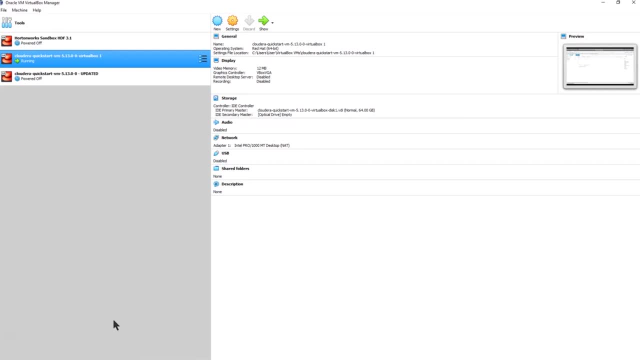 So let's get started. Let's go ahead and start. Cloudera is a pretty significant endeavor For an admin. if you've been adminning Linux machines for a very long time and you know a lot of the commands, I find that for most admins it takes them about two to four hours. 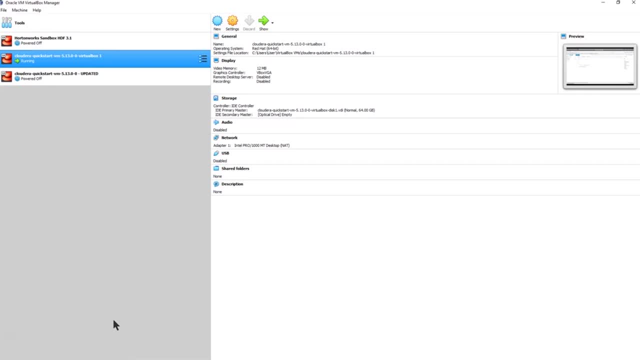 the first time they go in and create a virtual machine and set up their own Hadoop. In this case, though, and you're just learning and getting set up, best to start with Cloudera. Cloudera also includes an installed version of MySQL. 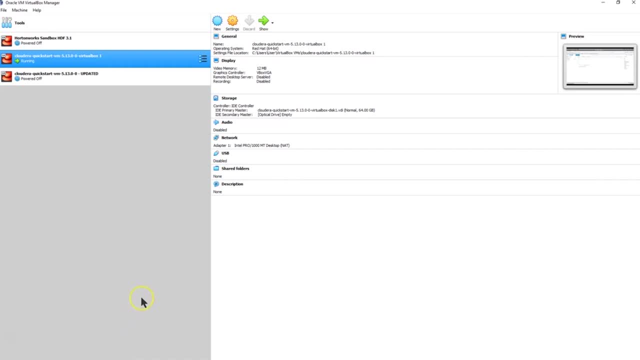 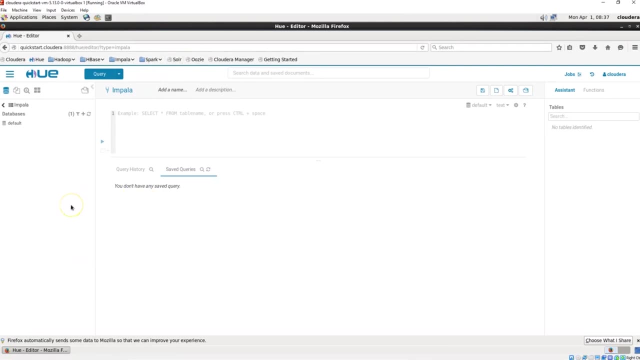 That way you don't have to reinstall the SQL version for importing data from and to. Once you're in the Cloudera Quickstart, you'll see it opens up. It opens a nice CentOS Linux interface and it has a desktop setup on there. 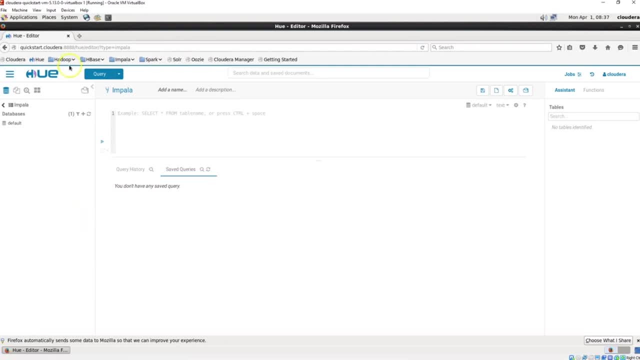 This is really nice for learning, so you're not just looking at command lines, And from in here it should open up by default to Hue. If not, you can click on Hue, Hue's kind of a fun little web-based interface. 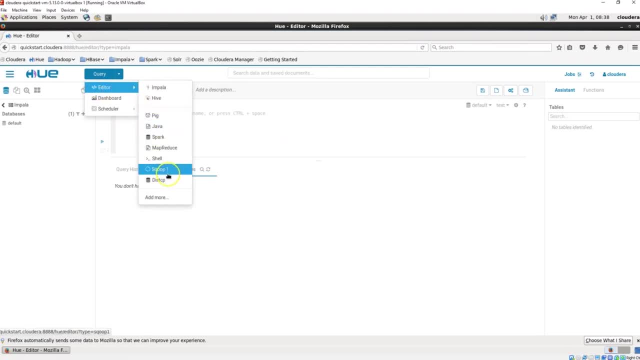 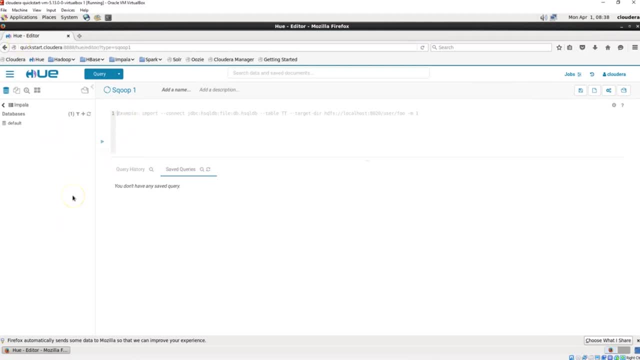 I'm going to go ahead and do that Here. you can see how it's in Hue through the web-based interface. The reason I like to do the command line is specifically on my computer. it runs much quicker, Where if I do the command line here and I run it, it tends to have an extra lag or an. 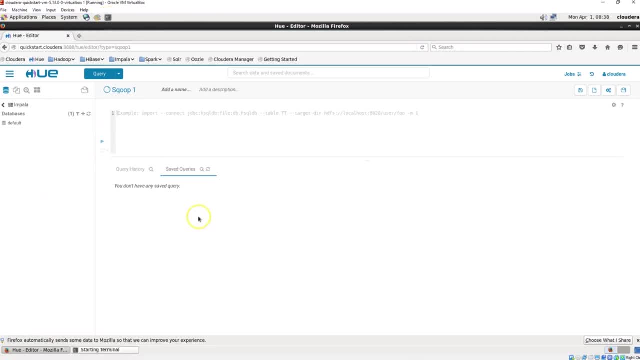 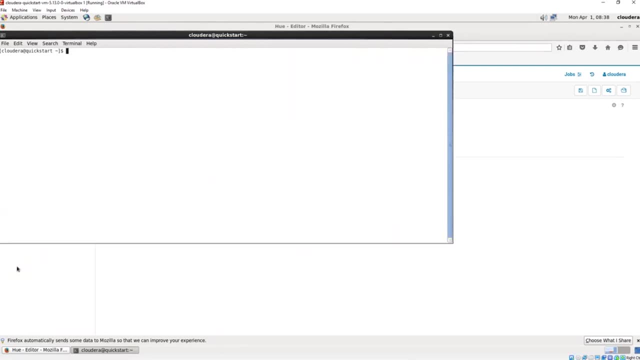 added layer in it. So for this we're going to go ahead and open our command line. The second reason I do this is we're going to need to go ahead and edit our mySQL so we have something to Scoop in. Otherwise I don't have anything going in there. 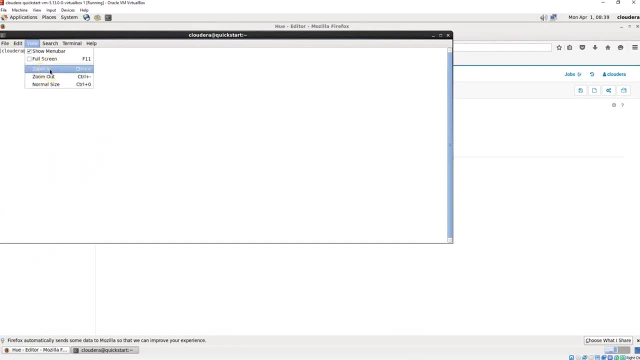 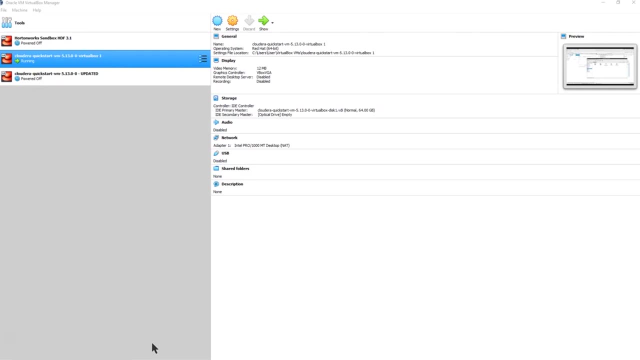 And of course we'll zoom in on this and increase the size of our screen. So for this demo, our hands-on- I'm going to use Oracle Virtual Box Manager and the Cloudera Quick Start. If you're not familiar with this, we do have another tutorial we put out and you can send. 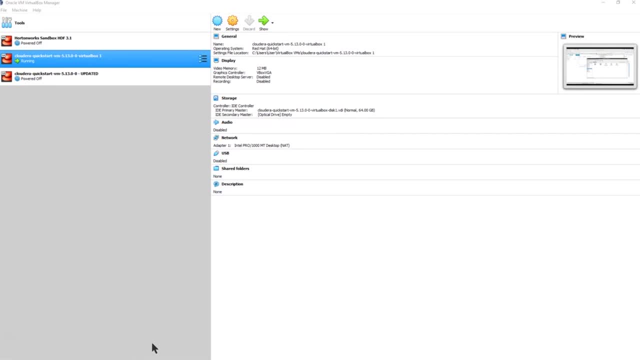 a note in the YouTube video below and let our team know and they'll send you a link. Or come visit wwwsimplylearncom. Now. this creates a Linux box on my Windows computer, So we're going to be in Linux and it'll be the Cloudera version with Scoop. 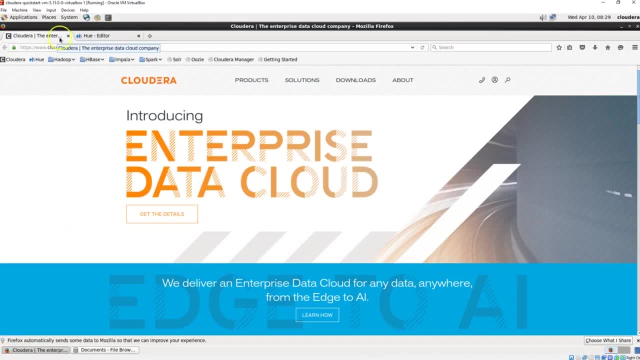 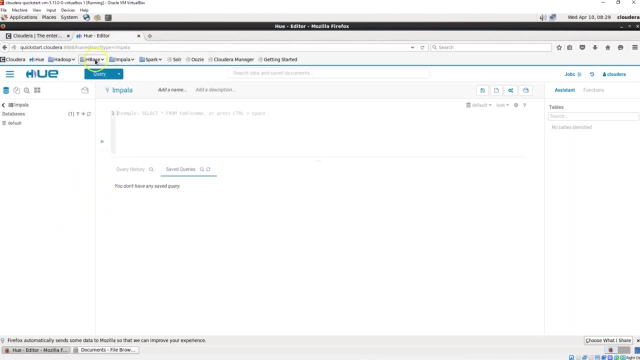 You will also be using MySQL MySQL Server. Once inside the Cloudera Virtual Box, we'll go under the Hue Editor. Now we're going to do everything in Terminal Window, but I just want you to be aware that under the Hue Editor you can go under Query Editor and you'll see as we come down here. 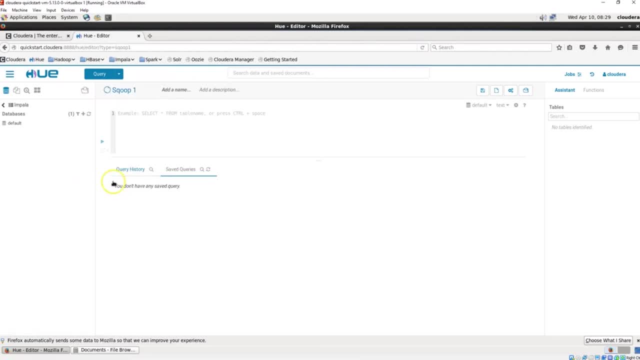 here's our Scoop on this, So you can run your Scoop from in here. Now, before we do this, we have to do a little exploration in MySQL, a MySQL Server. That way we know what data is coming in. So let me go ahead and open up a Terminal Window. 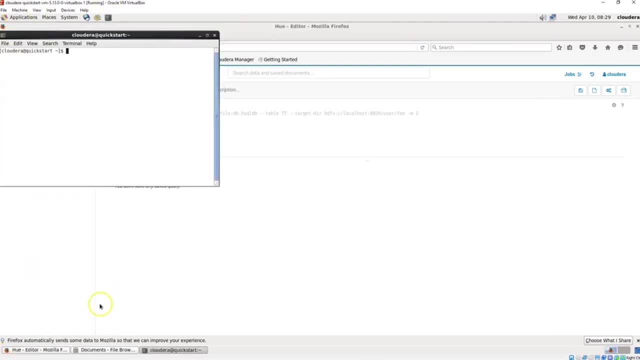 In Cloudera you have a Terminal Window. There's a window at the top here that you can just click on and open it up. And let me just go ahead and zoom in on here. Go View and Zoom In. Now to get into MySQL Server. you typically type in MySQL: 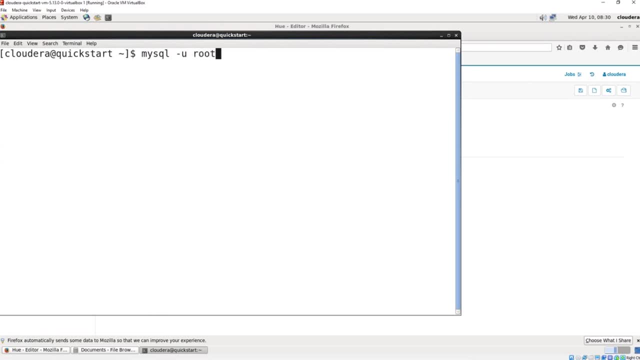 And this part will depend on your setup. Now the Cloudera Quick Start comes up that the username is root and the password is Cloudera. Kind of a strange quirk is that you can put a space between the minus u and the root. 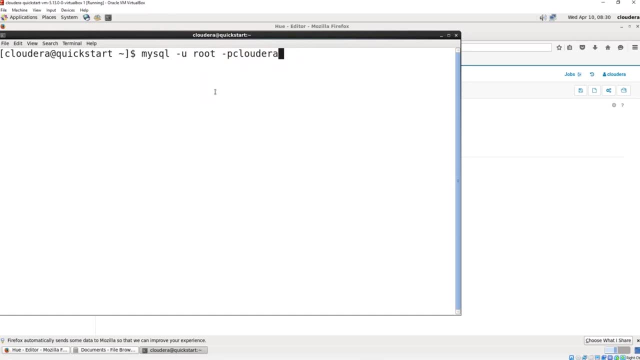 but not between the minus p and the Cloudera. Usually you'd put in a minus capital And then it prompts you for your password on here For this demo. I don't worry too much about you knowing the password on that, So we'll just go right into MySQL Server, since this is the standard password for this Quick. 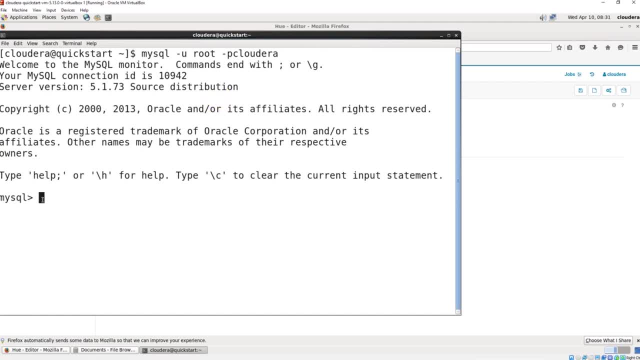 Start And you can see we're now into MySQL And we're going to do just a couple of quick commands. in here There's Show Databases and you follow by the semicolon. That's standard in most of these shell commands, so it knows it's the end of your shell command. 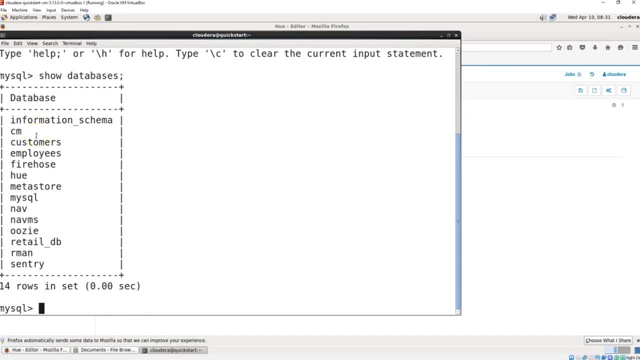 And you'll see in here in the Quick Start- Cloudera, Quick Start- that MySQL comes with a standard set of databases. Some of these have to do with the Uzi, which is the Uzi part of Hadoop, or others of these. 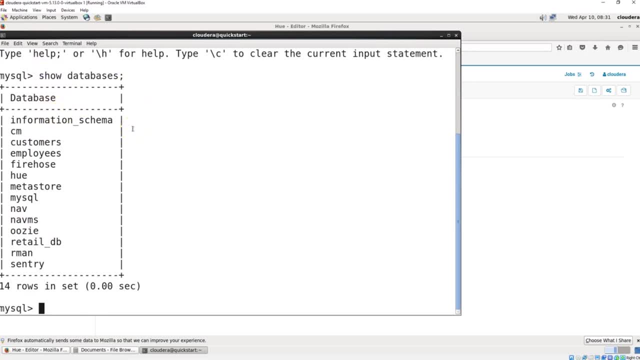 like Customers and Employees and stuff like that. Those are just for demo purposes. They come as a standard setup in there so that people going in for the first time have a database to play with, which is really good for us. so we don't have to recreate those. 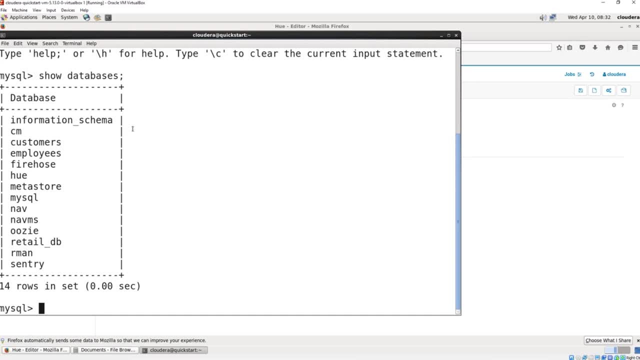 databases, And you will see on the list here we have a retail underscore db And then we can simply do use retail underscore db. So we'll set that as a default in MySQL And then we want to go ahead and show the tables. 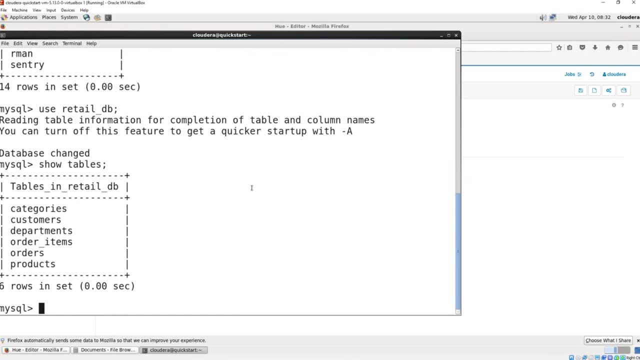 And if we show the tables, you can see under the database- the retail db database- we have categories, customers, departments, order items, orders, products. so there's a number of tables in here And we're going to go ahead and just use a standard SQL command. 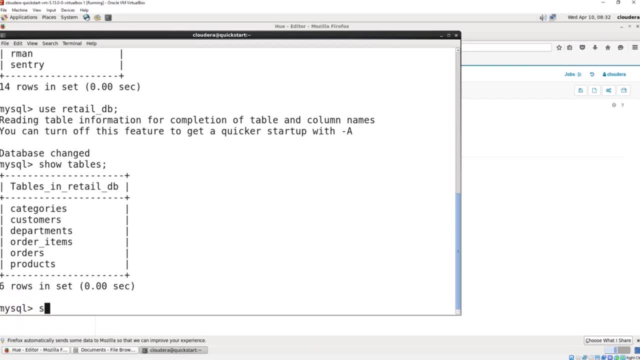 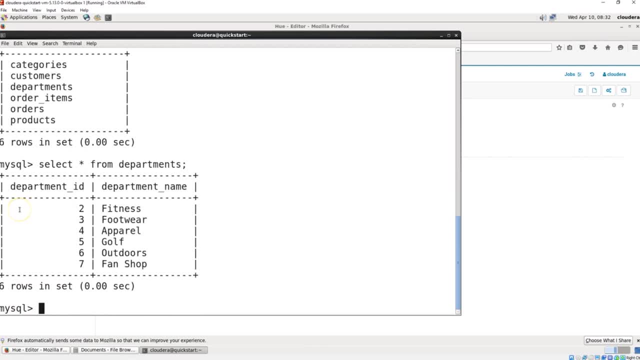 And if you did our Hive language, you'll note, remember it's the same for HQL also on this. So there's our departments table And we're going to list everything on the departments table And you'll see we have about six lines in here. 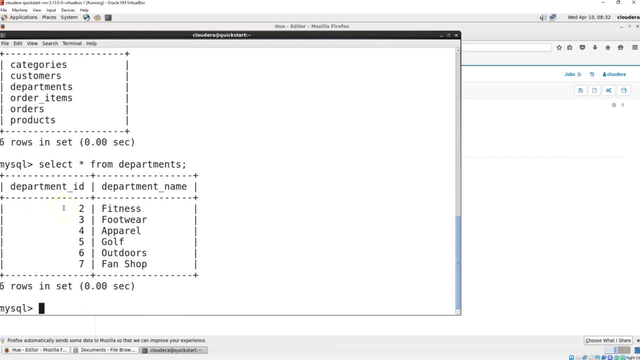 And it has a department ID and a department name: Two for fitness, three for footwear, so on and so forth. Now at this point I can just go ahead and exit, But it's kind of nice to have this data up here so we can look at it and flip back and 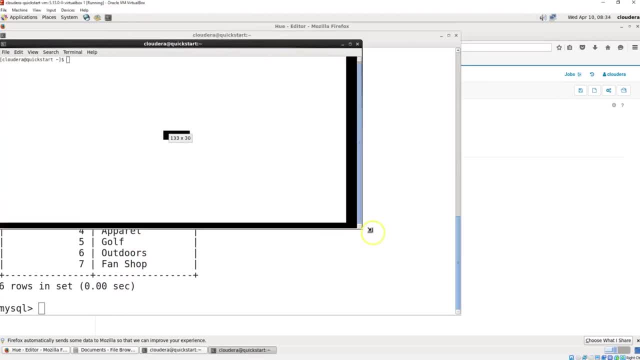 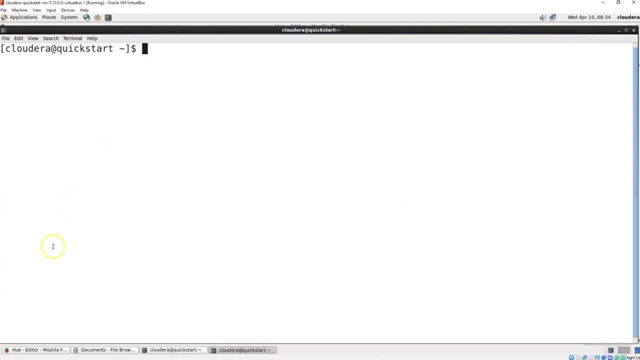 forth between the screens. So I'm going to open up another terminal window And we'll go ahead and zoom in on this also. And it isn't too important for this particular setup, but it's always kind of fun to know what setup you're working with. 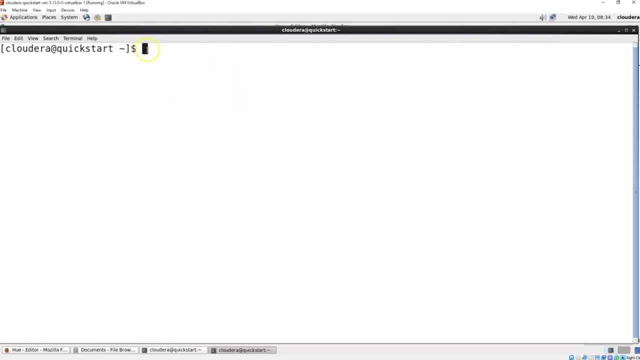 What is your host name, And so we'll go ahead and just type that in. This is a Linux command and it's a host name minus F, And you see we're on Quick Start, Cloudera. No surprise there. Now this next command is going to be a little bit longer because we're going to be doing 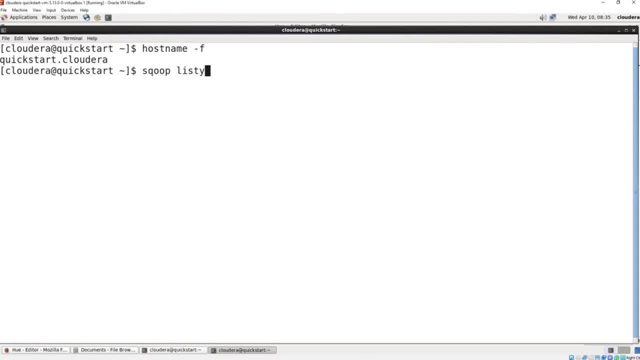 our first scoop command And I'm going to do two of them. We're going to list databases and list tables. This is going to take just a moment to get through this because there's a bunch of stuff going on here. So we have scoop. 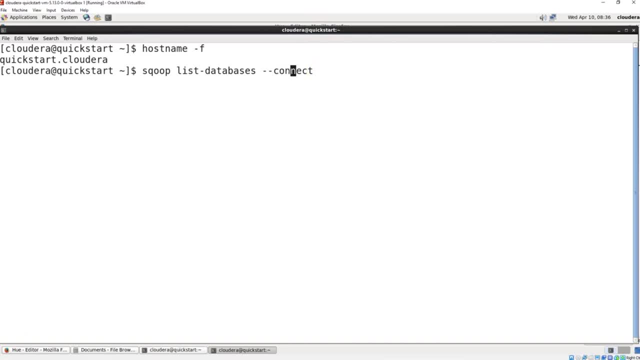 We have list databases, We have connect And under the connect command we need to let it know how we're connecting. We're going to use the JDBC- This is a very standard one- JDBC MySQL. So you'll see that if you're doing an SQL database, that's how you start it off with. 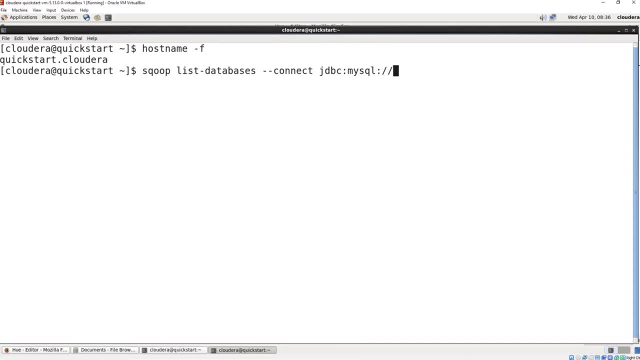 And then the next part. this is where you have to go look it up. It's however it was created. So if your admin created a MySQL server With a certain setup, that's what you have to go by And you'll see that usually they list this as local host. 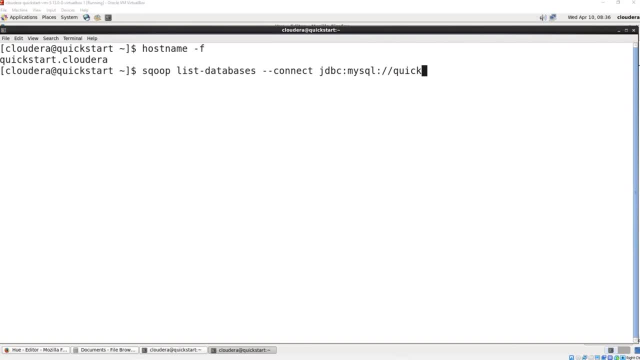 So you'll see something like local host. sometimes There's a lot of different formats, But the most common is either local host or the actual connection. So in this case we want to go ahead and do quick start 3306.. And so quick start is the name of the local host database and how it's hosted on here. 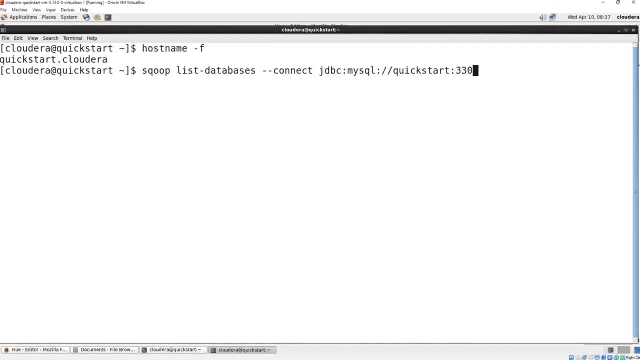 And when you set up the quick start for Hadoop under Cloudera, it's port 3306 is where that's coming in, So that's where all that's coming from, And so there's our path for that, And then we have to put in our password. 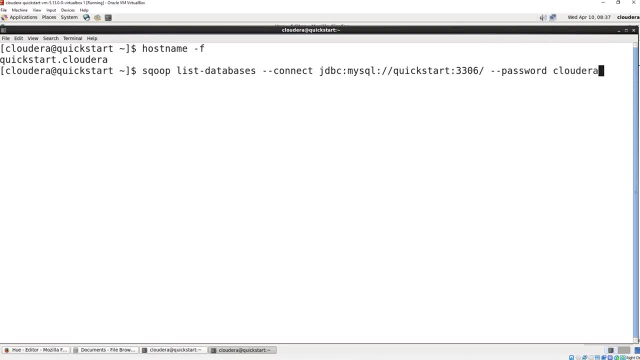 We type in the type password And if you look it up- password on the Cloudera- quick start is Cloudera And we have to also let it know the username. And again, if you're doing this, you'd probably put in a minus capital. 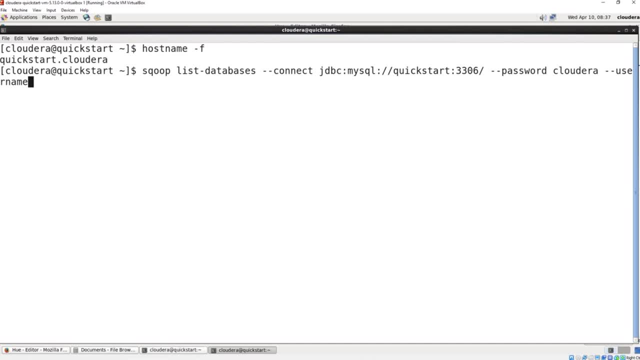 You can actually just do it for a prompt for the password. So if you leave that out it'll prompt you. But for this it doesn't really matter. I don't care if you see my password, It's the default one for Cloudera quick start. 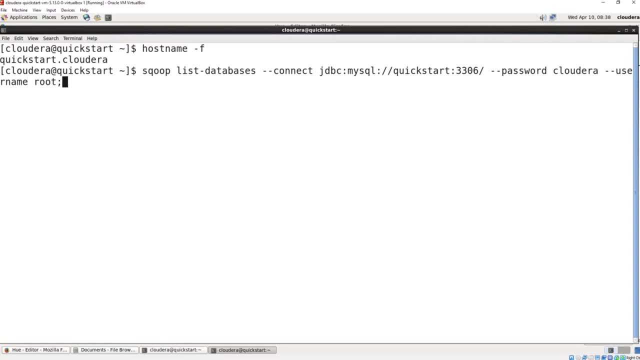 And then the username- on here It's simply root- And then we're going to put our semicolon at the end, And so we have here our full set up and we go ahead and list the databases And you'll see, you might get some warnings on here. 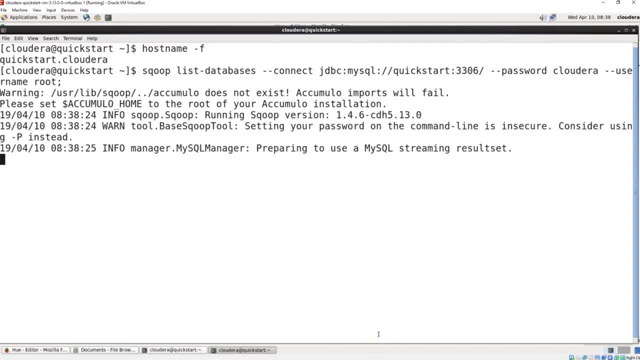 I haven't run the updates on the quick start. I suggest you're not running the updates either, if you're doing this for the first time, because it'll do some reformatting on there And it quickly pops up and you can see here's all of our the tables. we went in there. 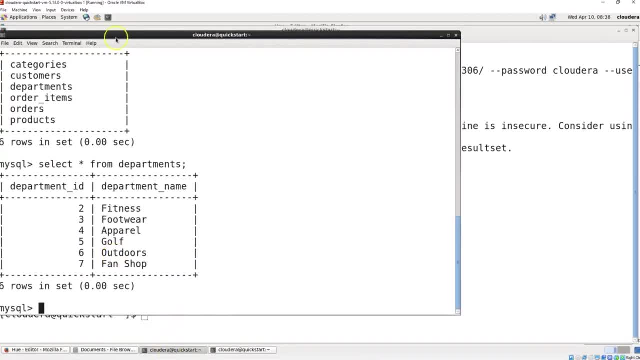 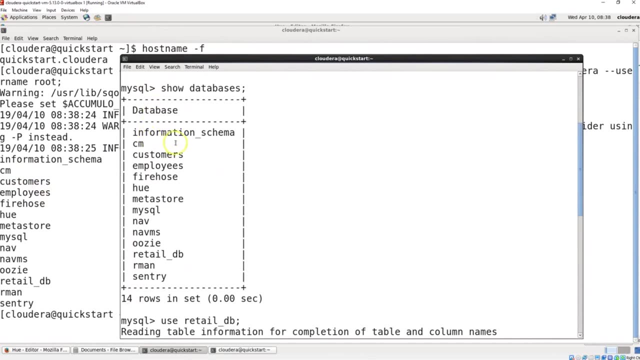 And if we go back to on the previous window, we should see that these tables match. So here we come in And here we have Our databases and you can see back up here where we had the CM, customers, employees and so on. 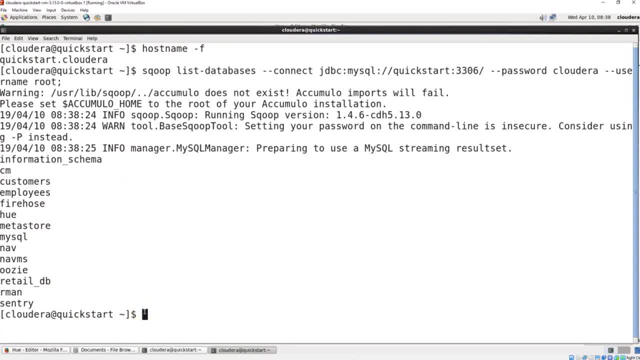 So the databases match. And then we want to go ahead and list the tables for a specific database. So let's go ahead and do that. I'm a very lazy typist So I'll put the up arrow in and you can see here: scoop list databases. 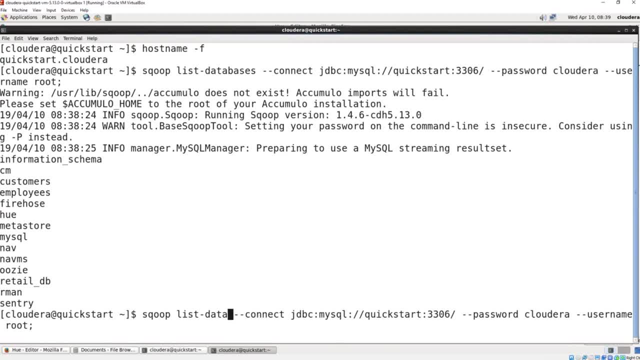 We're just going to go back and change this from databases to list tables, So we want to list the tables in here. Same connection. So most of the connection is the same, Except We want to know which tables we're listing. An interesting fact is you can create a table without being under a database. 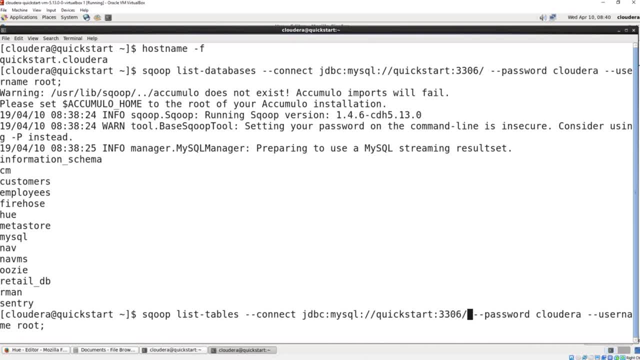 So if you left this blank, it will show the open tables that aren't connected directly to a database or under a database. But what we want to do is right past this last slash on the 3306.. We want to put that retail underscore DB, because that's the database we're going to be working. 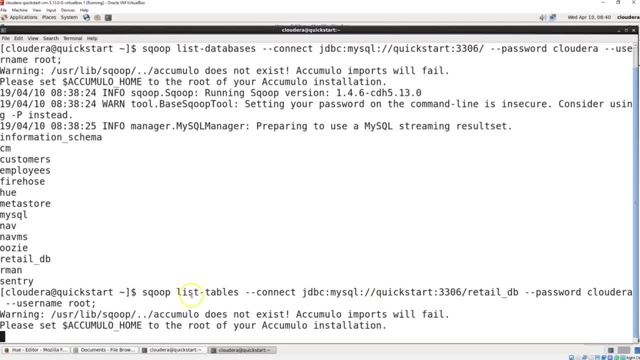 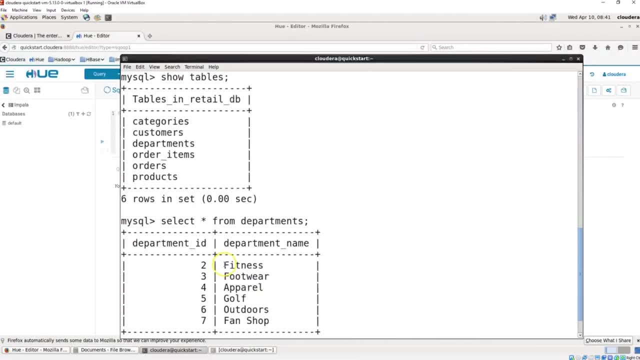 with And this will go in there and show the tables listed under that database. And here we go. We got categories, customers, departments, order items and products. If we flip back here real quick, there it is the same thing we had. 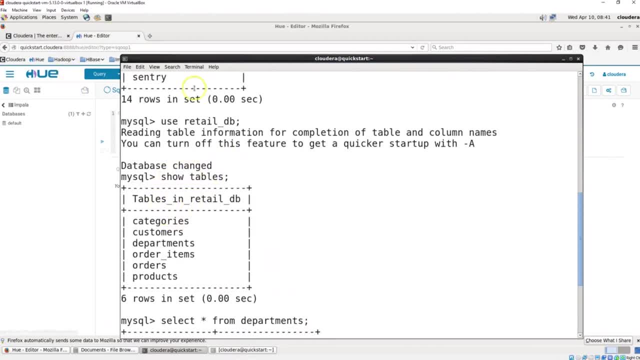 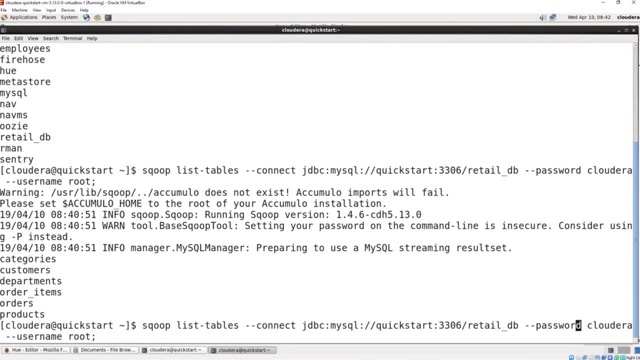 We had categories, customers, departments, order items and so on, And so let's go ahead and run our first import command. And again, I'm that lazy typer. So we're going to do scoop and instead of list tables, we want to go ahead and import. 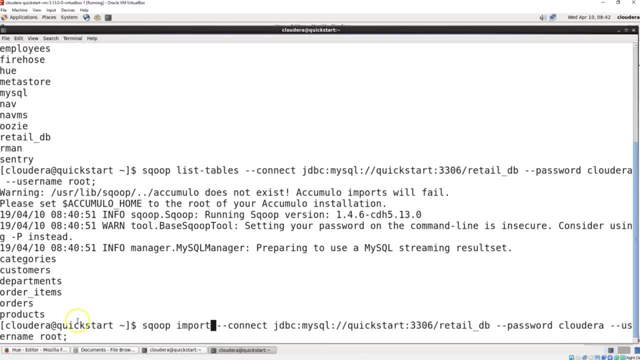 So there's our import command, And so once we have our import command in there, then we need to tell it exactly what we're going to import. So everything else is the same. We're importing from the retail DB, So we keep that. 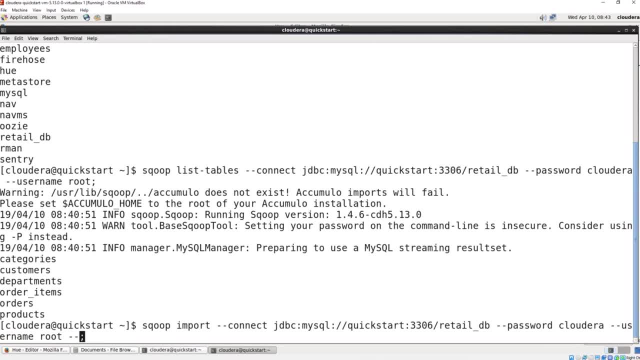 And then at the very end We're going to tag on dash, dash table that tells us we can tell it what table we're importing from And we're going to import departments There we go. So this is pretty straightforward, because what's nice about this is you can see the 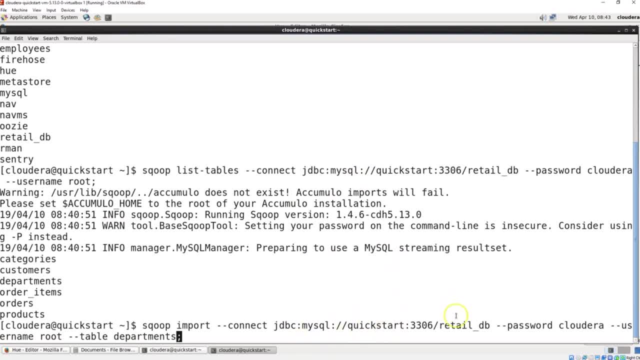 commands are the same. I got the same connection. I change it for the whatever database I'm in. Then I come in here. Our password and the username are going to be the same. That's all under the MySQL server set up, And then we let it know what table we're entering it. 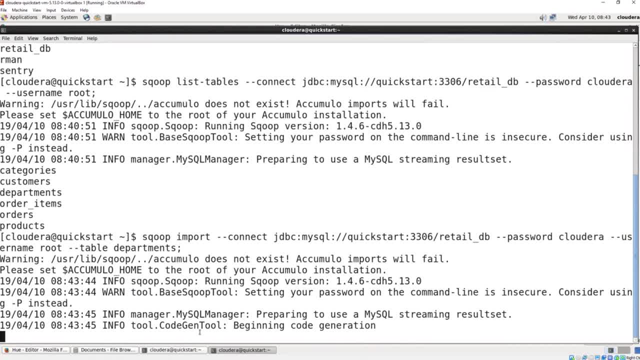 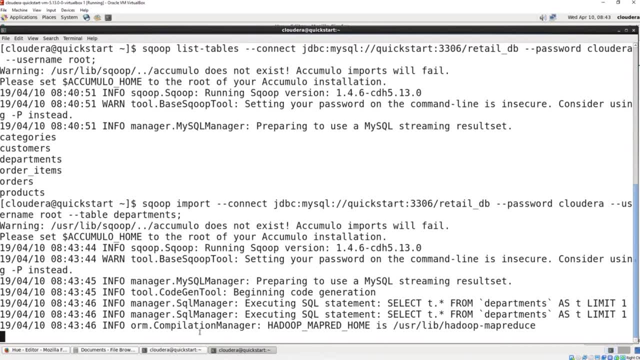 We run this and this is going to actually go through the mapper process in Hadoop. The mapping process: It takes the data and it maps it up to different parts in the setup in Hadoop on there and then saves that data into the Hadoop file system. 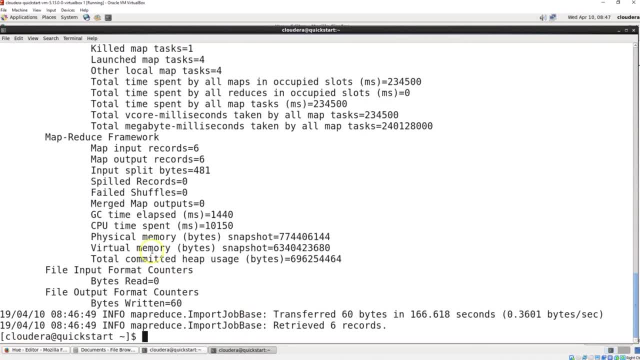 And it does take it a moment to zip through, which I kind of skipped over for you, Since it is running a. you know it's designed to run across the cluster, not on a single node. So when you're running on a single node it's going to run slow, even if you dedicate a couple. 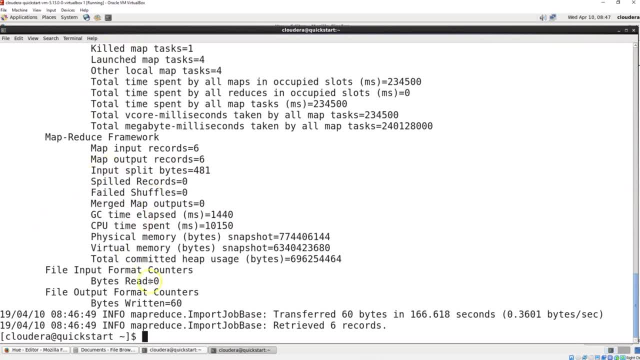 cores to it. I think I put dedicated four cores to this one And so you can see right down here we get to the end is now mapped in that information And then we can go in here We can go under, can flip back to our hue and under hue on the top I have there's databases. 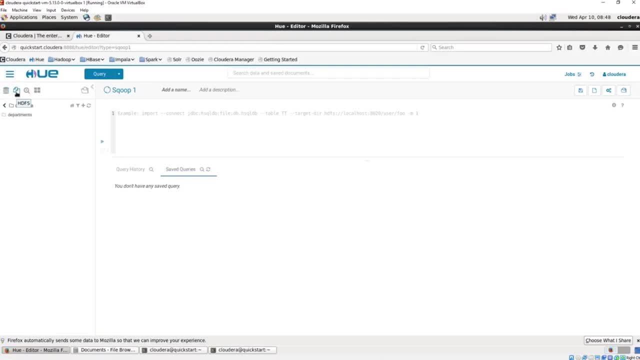 and the second icon over is your Hadoop file system, And we can go in here and look at the Hadoop file system and you'll see it show up underneath our documents. There it is Departments, Cloudera departments, And you can see. there's always a delay when I'm working in hue, which I don't like. 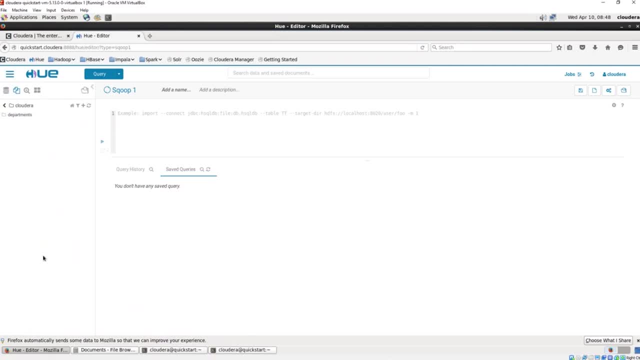 And that's the quick start issue. That's not necessarily running out on a server. when I'm running it on a server you pretty much have to run through some kind of server interface. I still prefer the terminal window. It still runs a lot quicker. 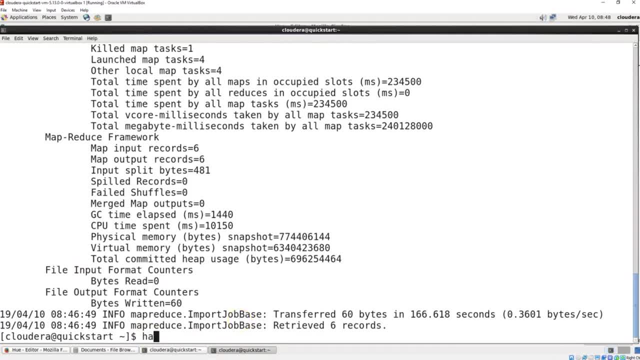 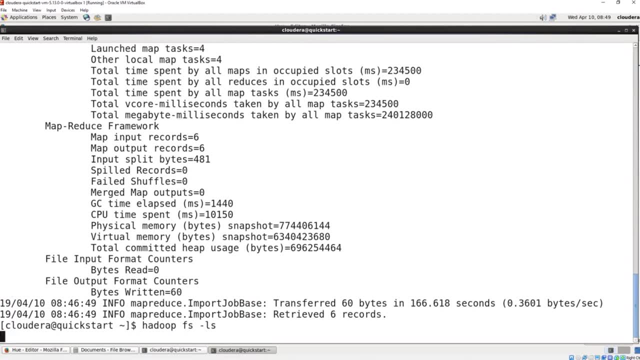 But we'll flip back on over here to the command line and we can do the Hadoop Type in the Hadoop fs and then list minus ls And if we run this you'll see underneath our Hadoop file system there is our departments, which has been added in. 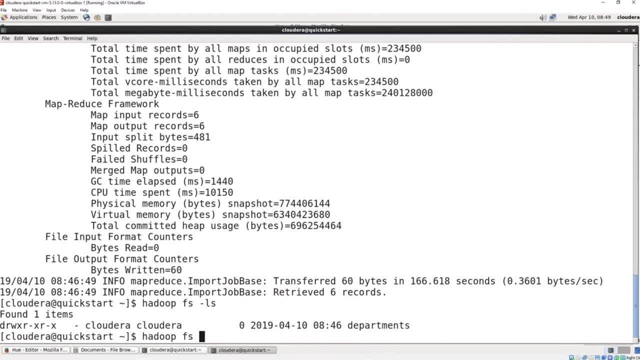 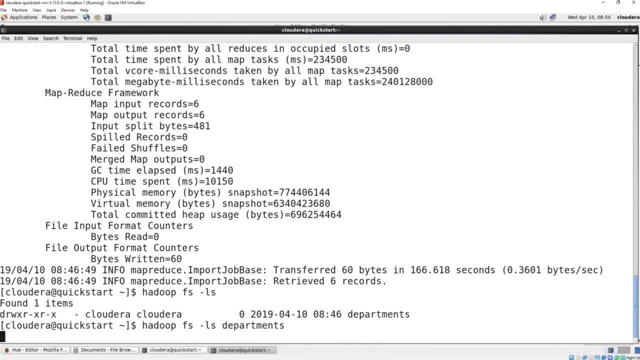 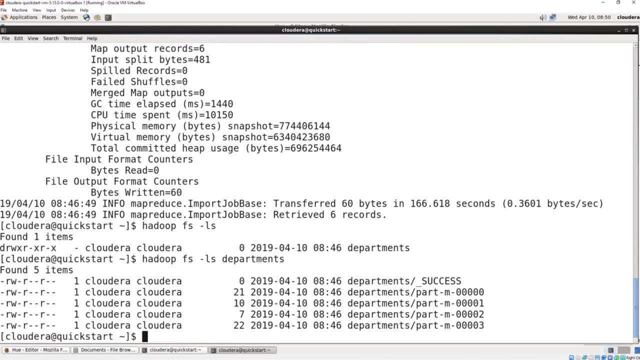 And we can also do Hadoop fs and this is kind of interesting For those who've gone through the Hadoop file system. everything you'll recognize this on here. This is the contents of departments And you'll see underneath departments we have part m000, 001, 002, 003.. 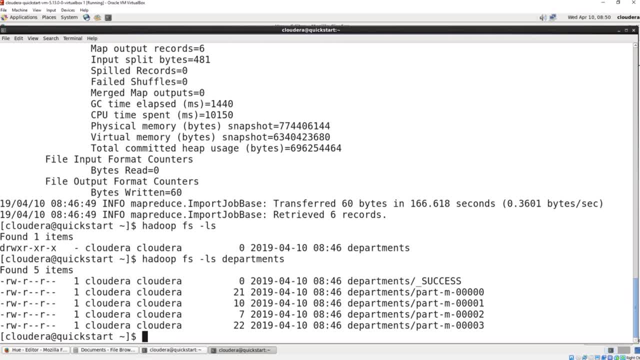 So this is interesting because this is how Hadoop saves these files. This is in the file system. This is not in Hive, So we didn't directly import this into Hive. We put this in the Hadoop file system, Depending on what you're doing. you would then write the schema for Hive to look at the Hadoop. 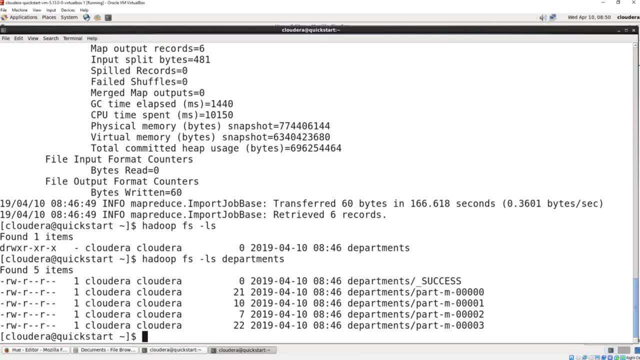 file system. Certainly visit our Hive tutorial for more information on Hive specific. So you can see in here There are different files that it forms, that are part of departments, and we can do something like this. We can look at the contents of one of these files- fs minus ls, or a number of the files. 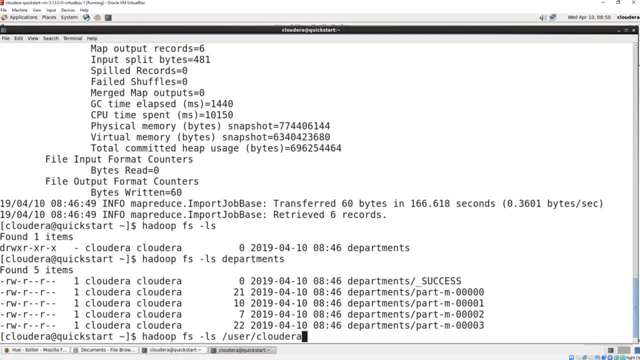 and we'll simply do the full path, which is user Cloudera, and then we already know. the next one is departments, and then, after departments, we're going to put slash, part star, So this is going to say anything that has part in it. So we have part dash, m000, and so on. 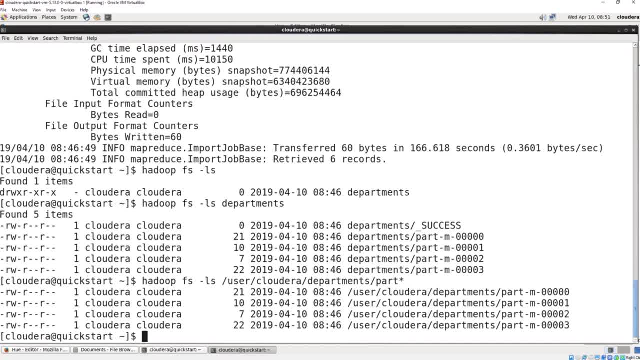 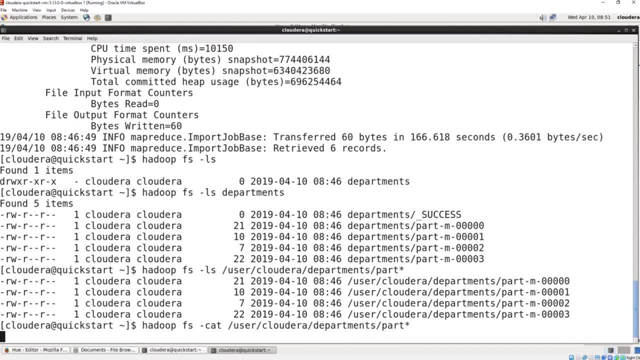 We can go ahead and cat Use that cat command or that list command to bring those up and then we can use the cat command to actually display the contents and that's a Linux command, Hadoop Linux command to cat Catinate, Not to be confused with Catatonic Catastrophic. 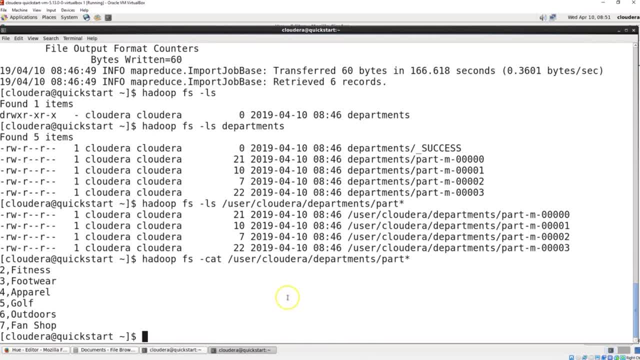 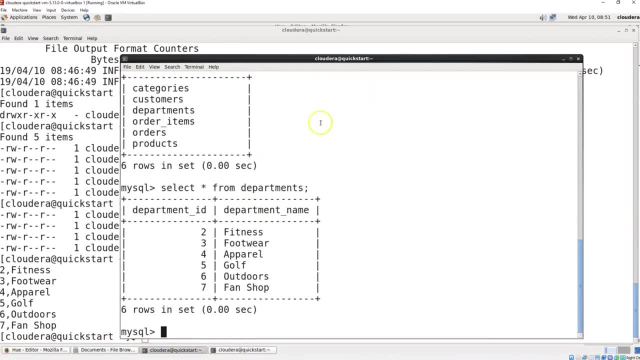 There's a lot of cat got your tongue And we see here fitness footwear apparel. That should look really familiar because that's what we had in our MySQL server When we went in here. we did a select, all on here. There it is. 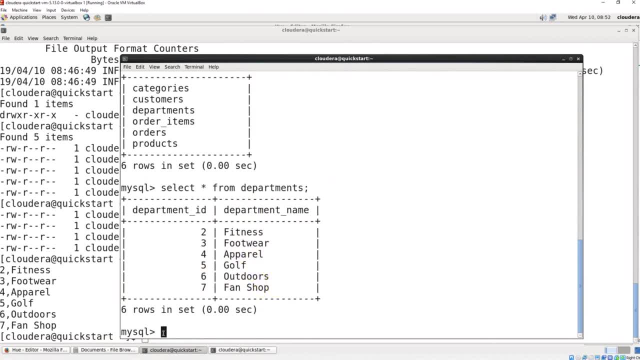 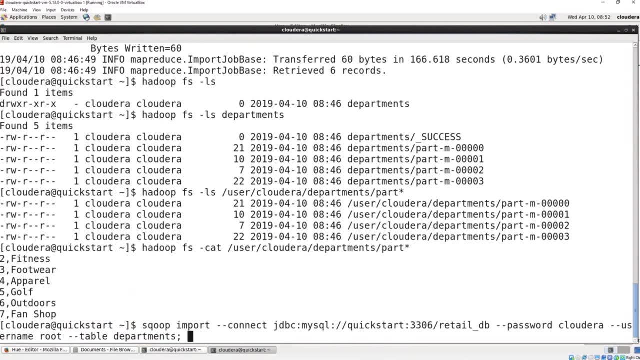 Fitness, footwear, apparel, golf, outdoors and fan shop. And then, Of course, it's really important to be able to tell it where to put the data. So we go back to our import command. So here's our scoop: import, We have our connect. 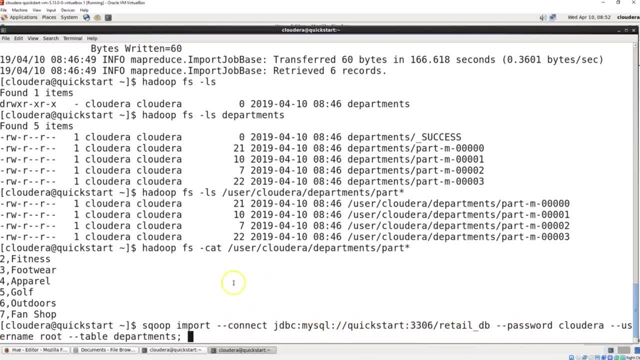 We have the DB underneath our connection, our MySQL server. We have our password, our username, the table going where it's going to, I mean the table where it's coming from, And then we can add a target on here. We can put in target dash directory, and you do have to put the full path. 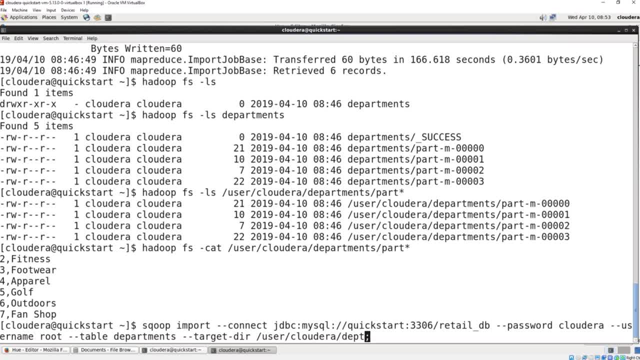 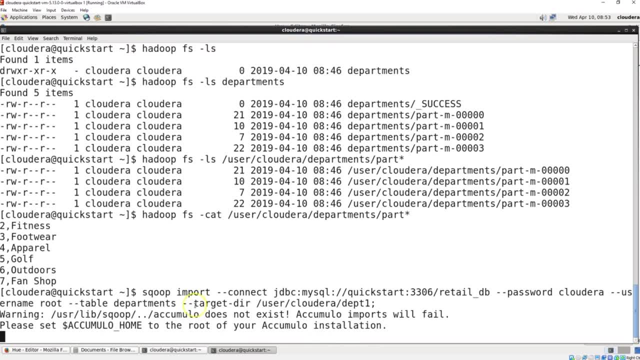 That's a Hadoop thing, It's a good practice And we're going to add it to department. we'll just do department one And so here we now add a target directory in here and user cloud era department one, And this will take just a moment before. 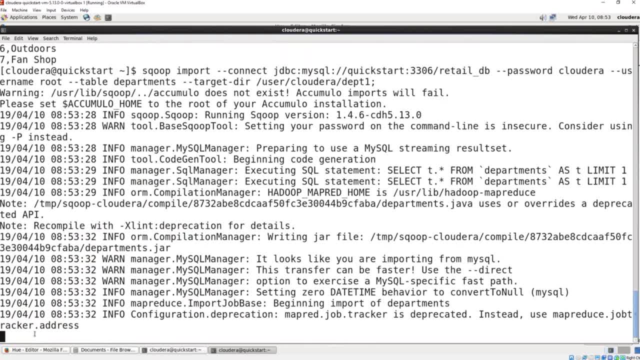 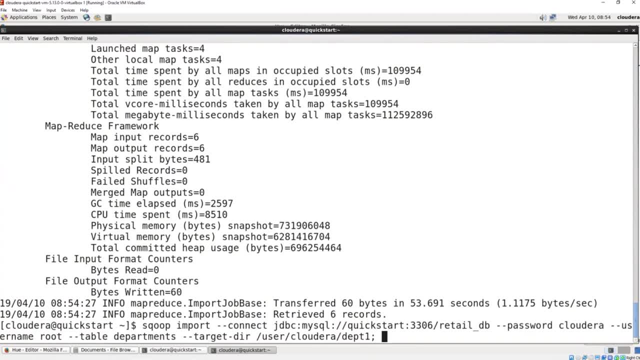 So I'll go ahead and skip over the process, since it's going to run very slowly. It's only running on, like I said, a couple cores and it's also on a single node, And now we can do the Hadoop. let's just do the apparel. 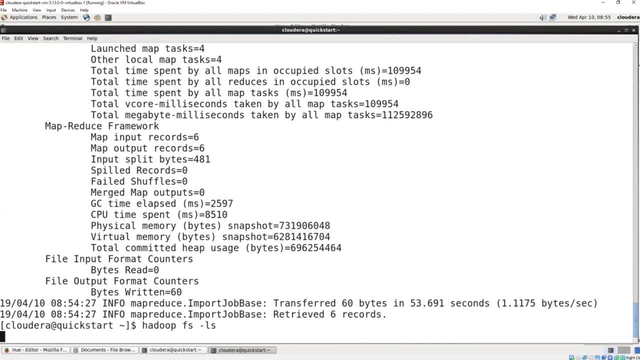 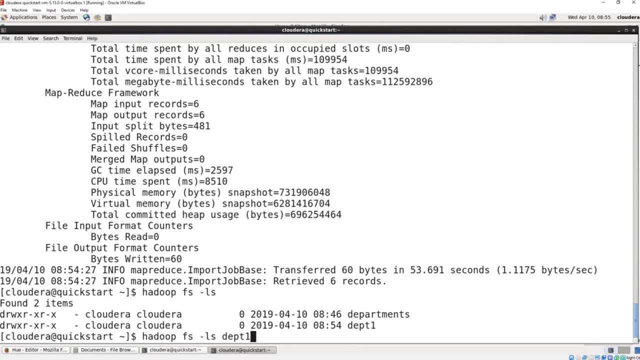 File system list. We want just straight list And when we do the Hadoop file system minus LS or list, you'll see that we now have department one. We can of course do list department one and you can see we have the files inside department. 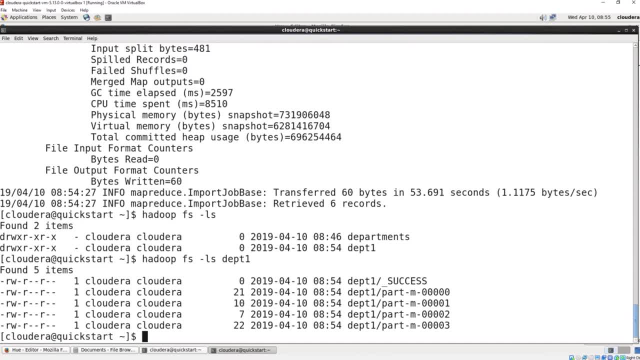 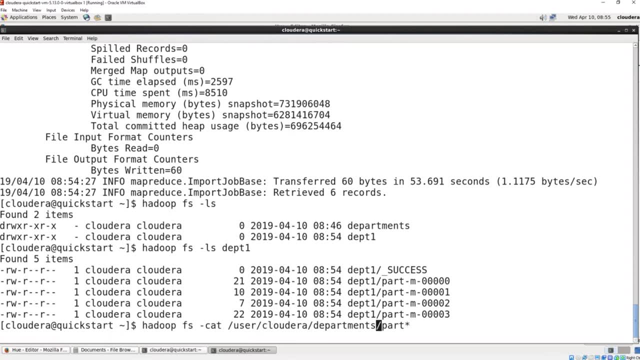 one, And they mirrored what we saw before with the same files in there in the part M-O-0-0 and so on. If we want to look at them, it'd be the same thing we did before with the cat, except instead of departments we'd be department one. 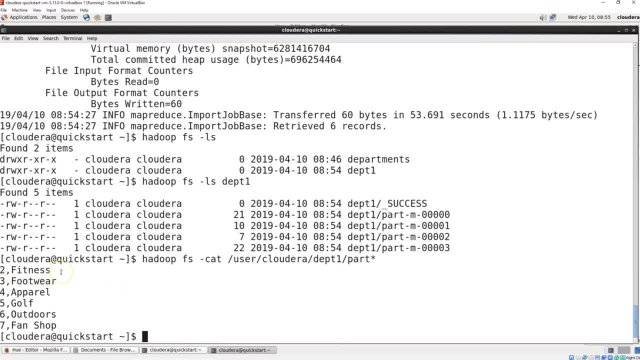 There we go, And then that's going to come up with the same data we had before. Now, one of the important things when you're importing data- and it's always a question to ask- is: do you filter the data? Do we want to filter this data as it comes in, so we're not storing everything in our 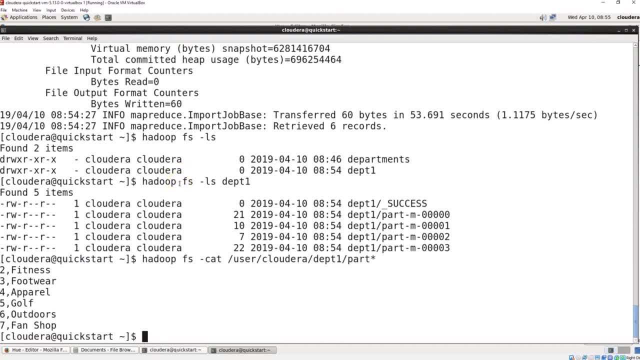 file system. You would think: Hadoop big data, put it all in there. I know from experience that putting it all in there can turn a couple hundred terabytes into a petabyte very rapidly And suddenly you're having to really add on to that data store and you're storing duplicate. 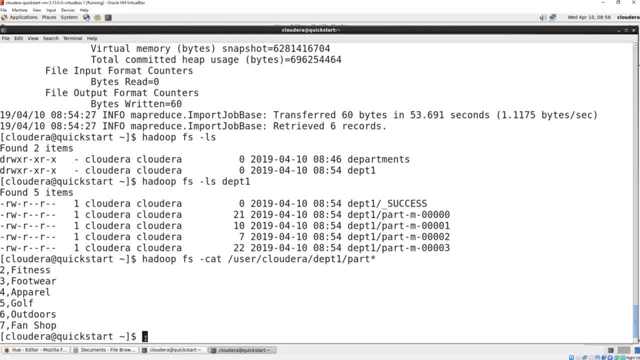 data sometimes. So you really need to be able to filter your data out. And so let's go ahead and use our up arrow to go to our last import. And we're going to go to our last import, Since it's still a lot the same stuff. 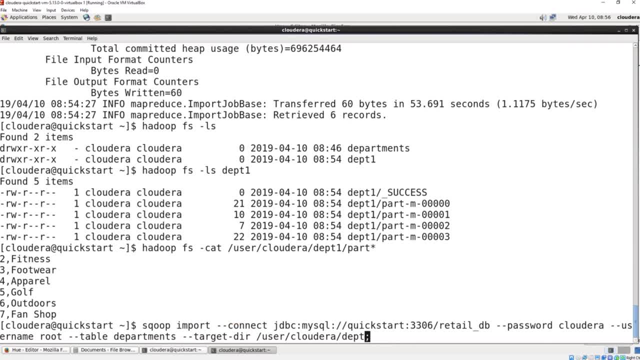 So we have all of our commands under import. We have the target. We're going to change this to department two, So we're going to create a new directory for this one. And then, after departments, there's another command that we didn't really slide in here. 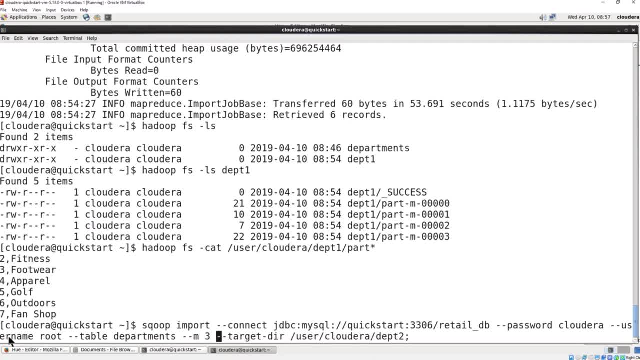 and that's our mapping, And I'll show you what this looks like in a minute. So we're going to put M3 in there. That doesn't have nothing to do with the filtering. I'll show you that in a second, though what that's for. 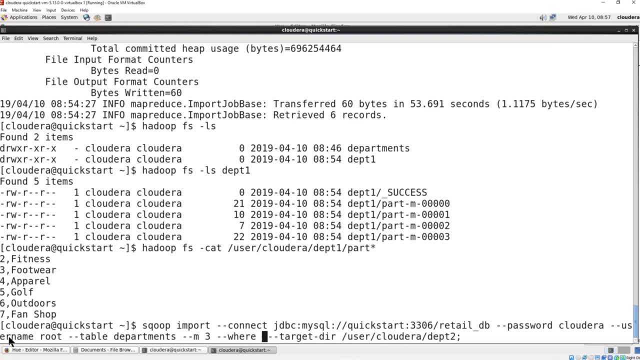 And we just want to put in where. So where and what is the where? In this case? We want to know where department ID and if you want to know where that came from, we can flip back on over here. We have department underscore IDs. 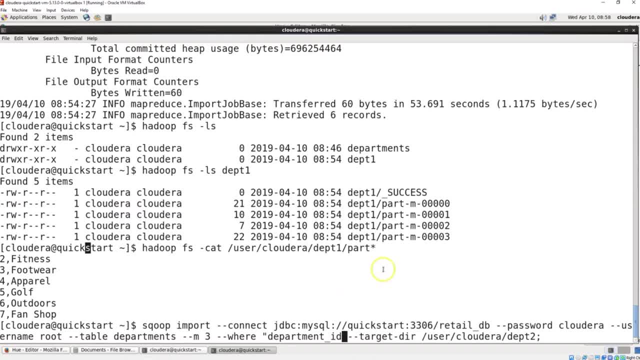 This is where that's coming from. That's just the name of the column on here, And so we come in here to department. ID is greater than four. Simple logic. there You can see where you'd use that for maybe creating buckets for ages. 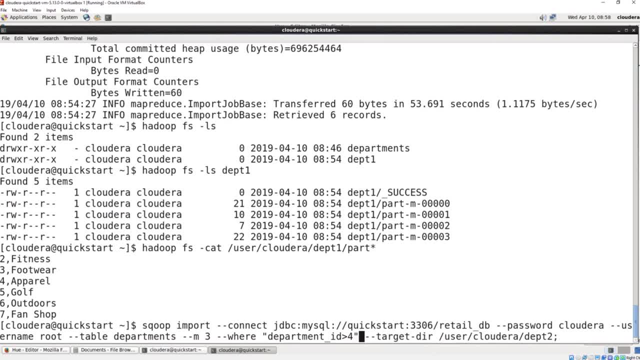 You know age from 10 to 15, 20 to 30. You might be looking for. I mean, there's all kinds of reasons why you could use the where command And then you can also filter information out. Maybe you're doing word counting and you want to know words that are used less than a hundred. 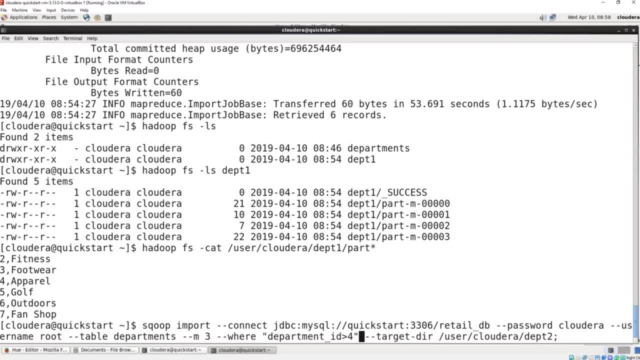 times. You want to get rid of the and is, and, and, and all the stuff that's used over and over again. So we'll go ahead and put the where and then department ID is greater than four, We'll go ahead and hit enter on here. 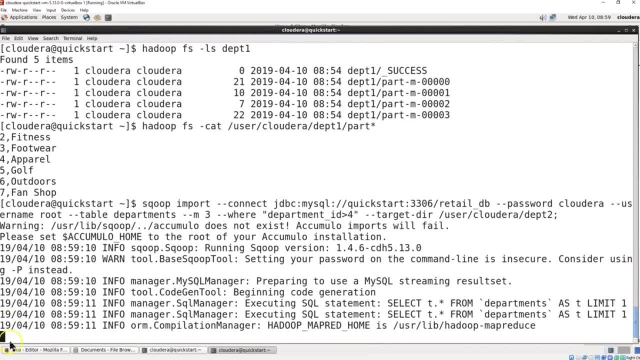 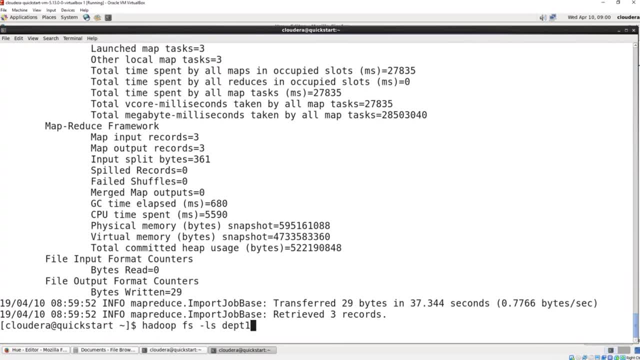 And this will create our department two set up on this, And I'll go ahead and skip over some of the runtime. Again, it runs really slow on a single node. Real quick page through our commands. Let's see, here we go, Here we go. 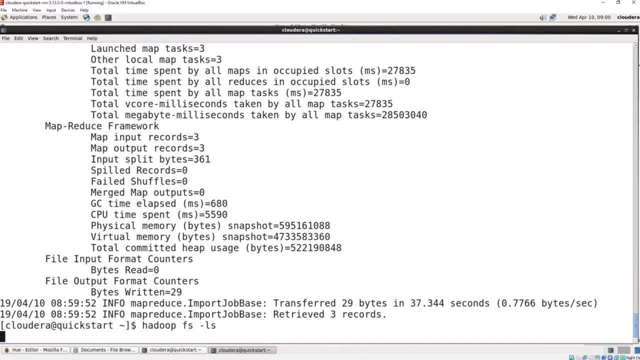 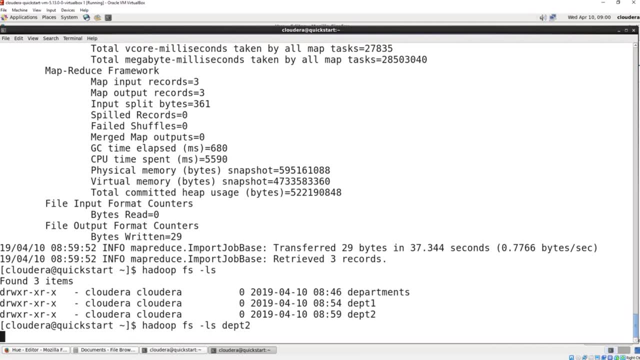 our list and we should see underneath the list the department two on here now and there it is department two, and then i can go ahead and do list department two. you'll see the contents in here and you'll see that there is only three maps and it could be that the data created three maps. but 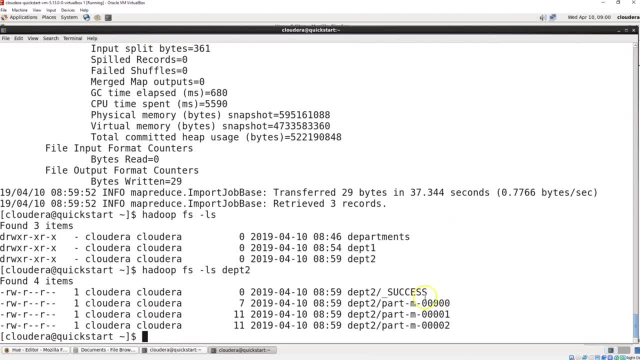 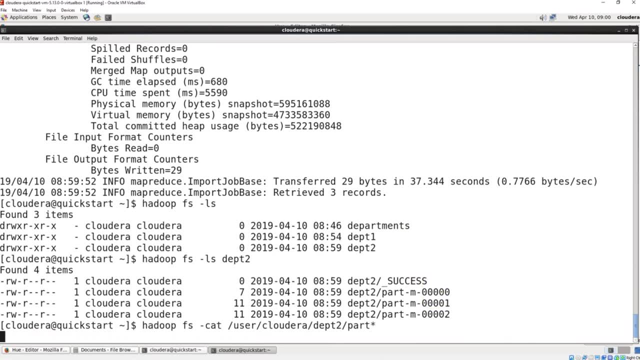 remember i set it up to only use three mappers, so there's zero one and two, and we can go ahead and do a cat on there. remember, this is department two. so we want to look at all the contents of these three different files and there it is. it's greater than four. so we have: golf is five outdoor six. 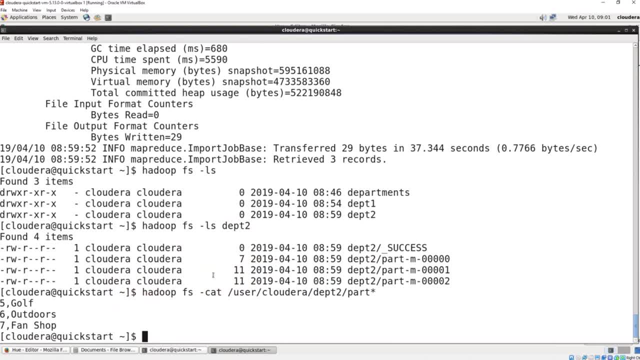 fan shop is seven. so we've effectively filtered out our data and just storing the data we want on our file system. so if you're going to store data on here, the next stage is to export the data. remember, a lot of times you have mysql server and we're continually dumping that data into our 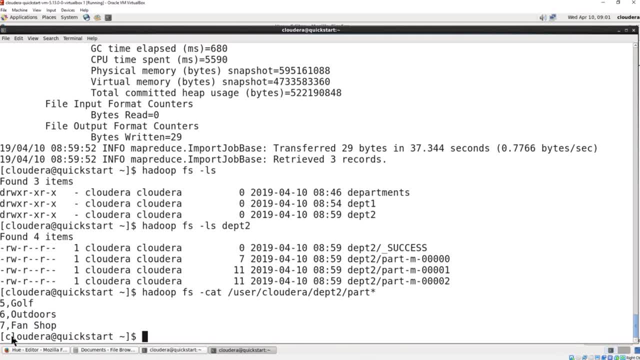 long-term storage and access the hadoop file system. but what happens when you need to pull that data out and you know, restore a database or, uh, maybe you have. uh, you just merged with a new company- a favorite topic, merging companies and merging databases- that's listed under nightmare. and how many different names for company can you have? 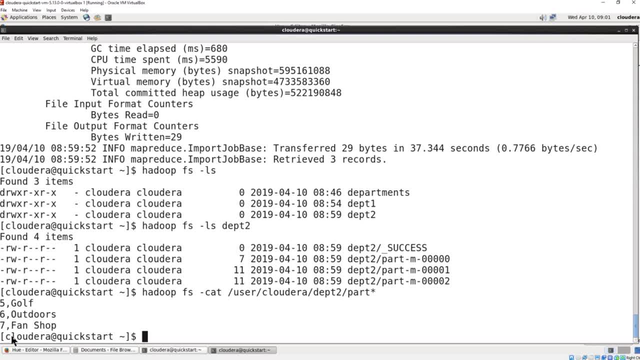 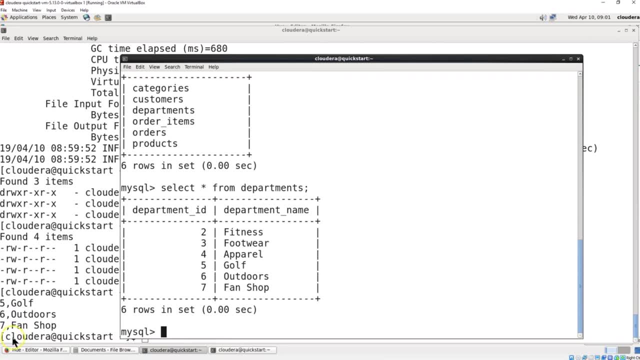 so you can see where uh being able to export is also equally important, and let's go ahead and do that. i'm going to flip back over to mysql server here and we'll need to go ahead and create our database we're going to export into. now i'm not going to go too much in detail on this command. 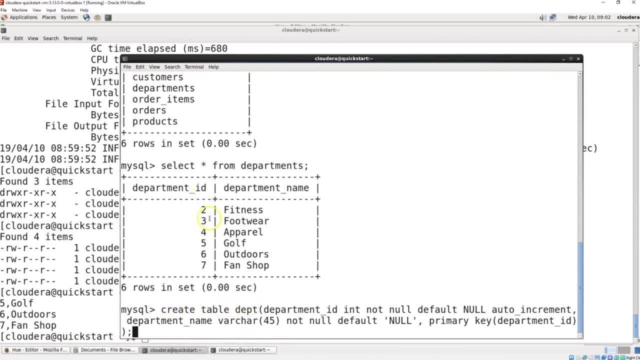 we're simply creating a table and the table is gonna have- uh is pretty much the same table we already have in here from department, but in this case we're going to create a table called d e p t, uh. so it's the same setup, but we're just gong to, we're just giving it a different name, a different. 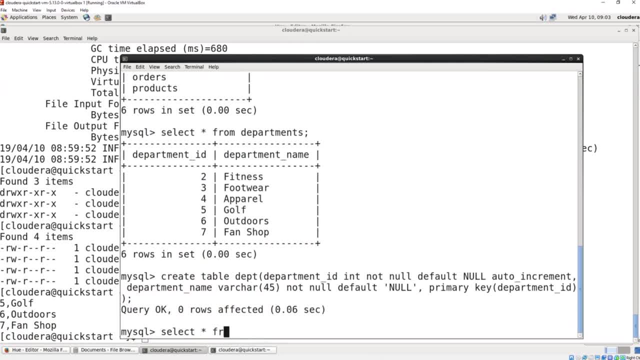 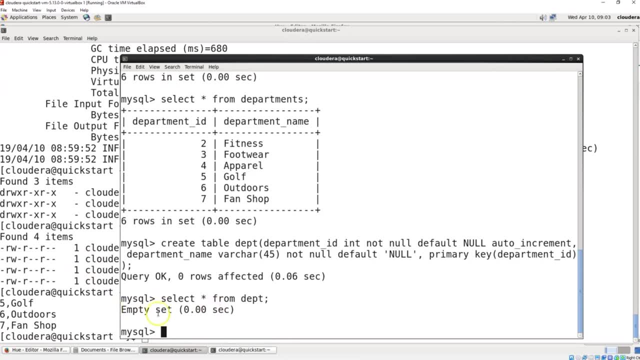 schema, and so we've done that and we'll go ahead and do a select star from d e p t. there we go and it's empty. that's what we expect: a new database, a new data table- and it's empty in there now. so now we need to go ahead and export our data that we just 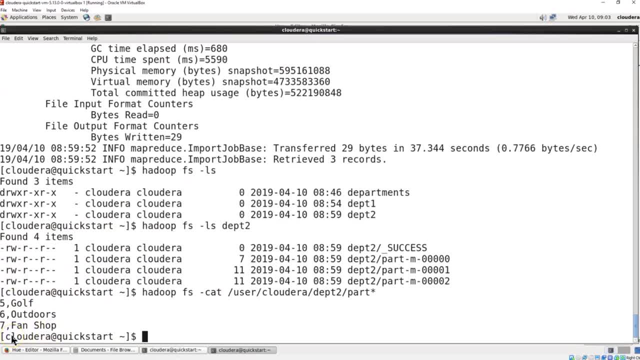 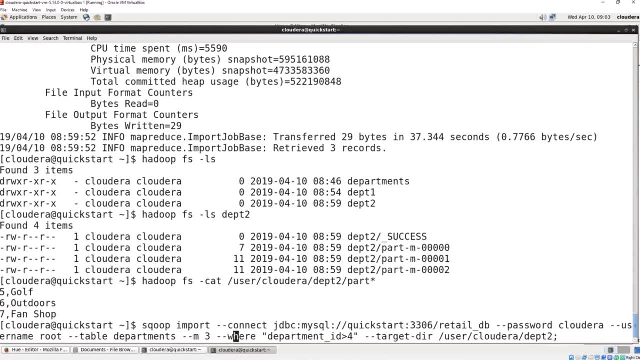 out into there. So let's flip back on over here to our scoop setup, which is just our Linux terminal window, And let's go back up to one of our commands. Here's scoop import. In this case, instead of import, we're going to take the scoop and we're going to export, So we're going to just change. 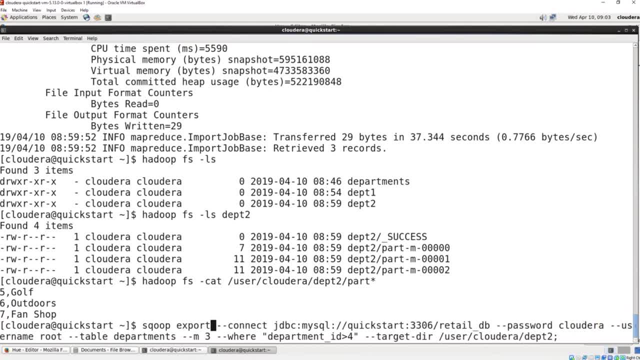 that Export And the connection is going to remain the same. So same connect, same database. We're still doing the retail DB. We have the same password, so none of that changes. The big change here is going to be the table Instead of departments- remember we changed it. 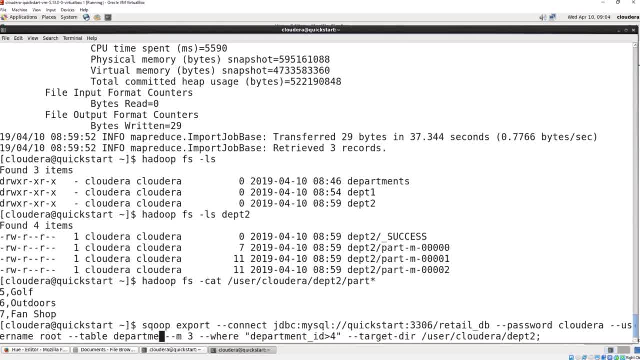 and gave it a new name, And so we want to change it here also: D-E-P-T. So department, We're not going to worry about the mapper count And the where was part of our import. There we go, And then finally, it needs to know where to export from. So instead of target directory, we have 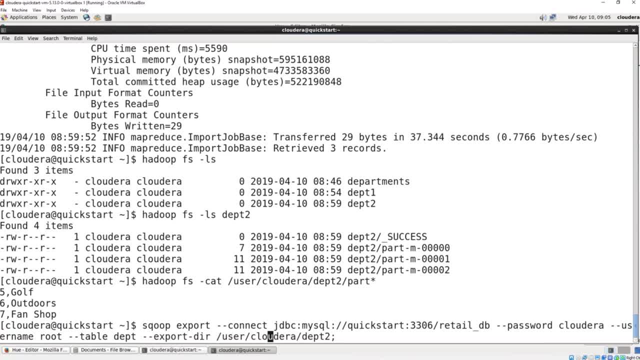 an export directory. That's where it's coming from. Still, user Cloudera And we'll keep it as department 2.. Just so you can see how that data is coming back. that we filtered in And let's go ahead and run. 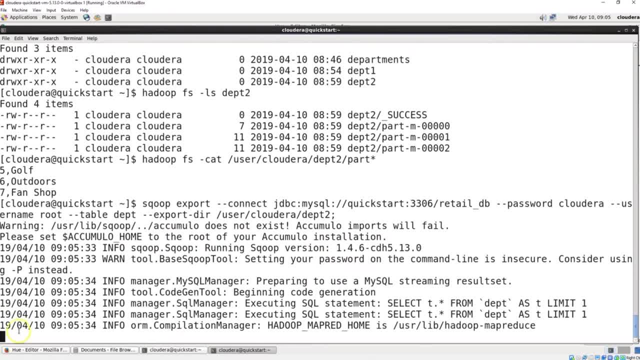 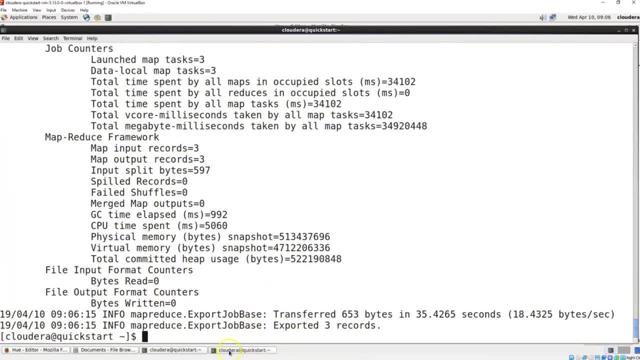 this. It'll take it just a moment to go through its steps And again, because it's slow, I'm just going to go ahead and skip this so you don't have to sit through it. And once we've wrapped up our export, we'll flip back on over here to MySQL. Use the up arrow And this time we're going to. 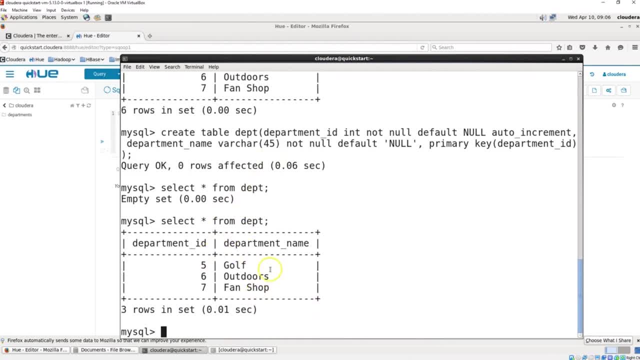 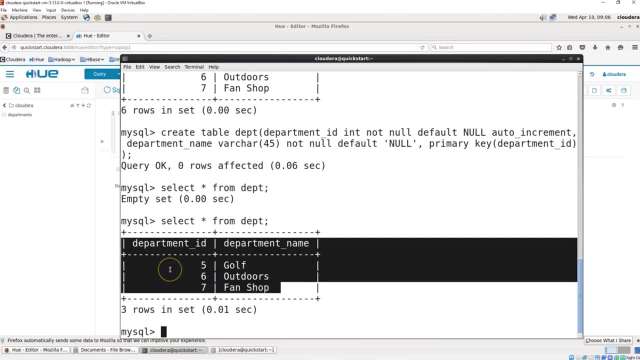 select star from department And we can see that. there it is. It exported the golf outdoors and fan shop, And you can imagine also that you might have to use the where command And in your export also. So there's a lot of mixing. The command line for scoop is pretty. 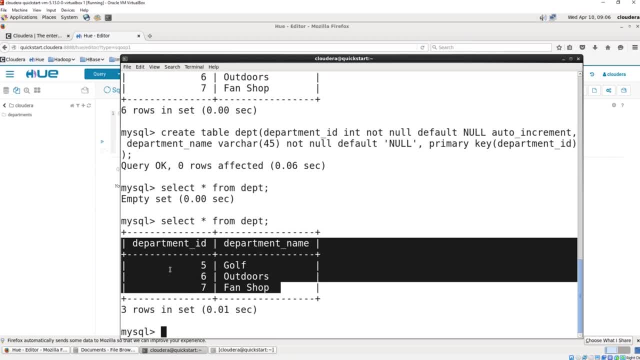 straightforward. You're changing the different variables in there, whether you're creating a table listing a table listing databases. Very powerful tool for bringing your data into the Hadoop file system and exporting it. So now that we've wrapped up our demo on scoop and gone. 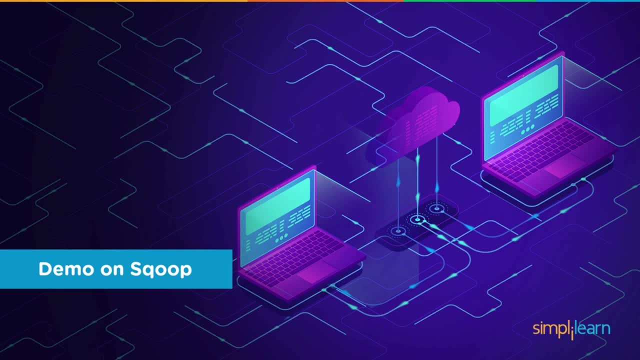 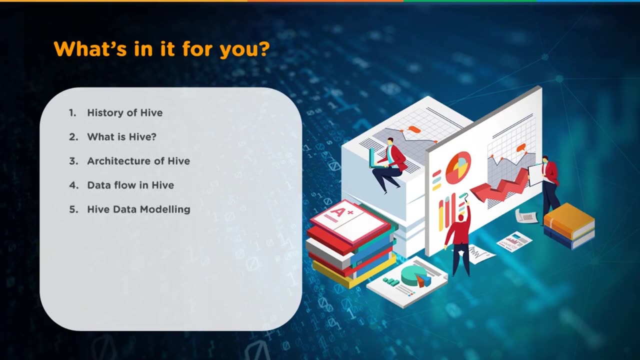 through a lot of basic commands. that wraps it up for us today. First, we're going to start with the history of Hive. What is Hive? Architecture of Hive, Data flow in Hive, Hive data modeling, Hive data types, Different modes of Hive And difference between Hive and 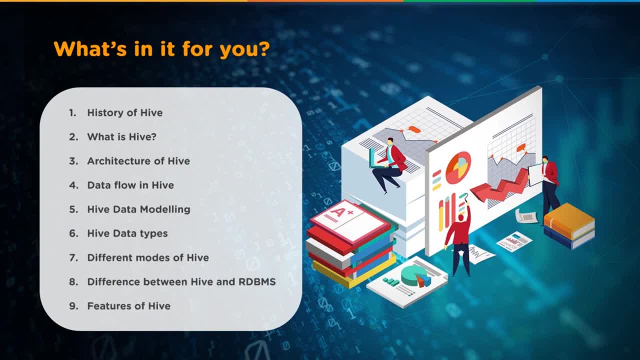 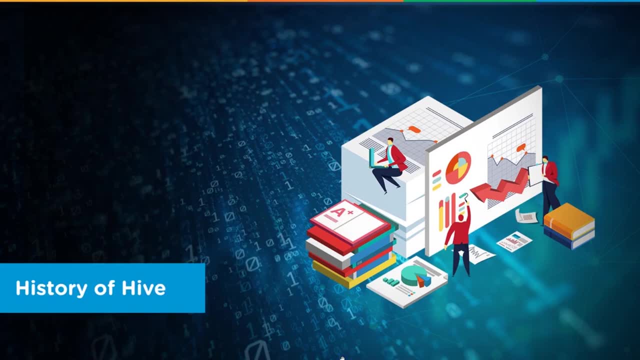 RDBMS. Finally, we're going to look into the features of Hive and do a quick hands-on demo on Hive in the Cloudera Hadoop file system. Let's dive in with a brief history of Hive. So the history of Hive begins with Facebook. Facebook began using Hadoop as a solution to 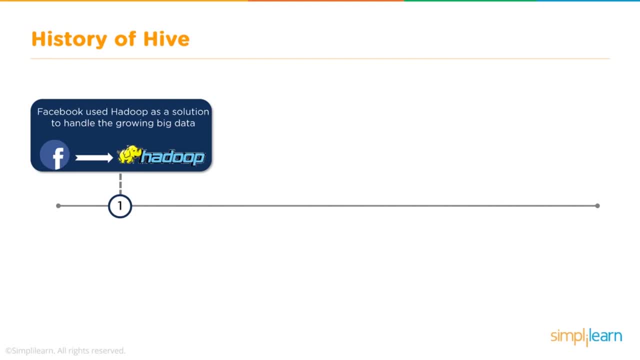 handle the growing big data, And we're not talking about a data that fits on one or two or even five computers. We're talking data that fits on. if you've looked at any of our other Hadoop tutorials, you'll know we're talking about very big data and data pools, And Facebook certainly has a lot of data. it. 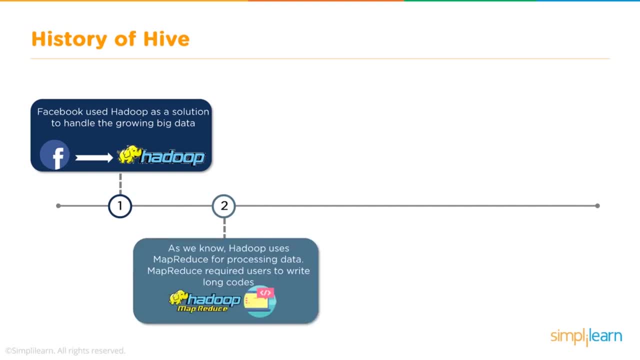 tracks. As we know, the Hadoop uses MapReduce for processing data. MapReduce required users to write long codes, And so you'd have these really extensive Java codes, very complicated for the average person to use. Not all users reversed in Java and other coding languages. This proved to 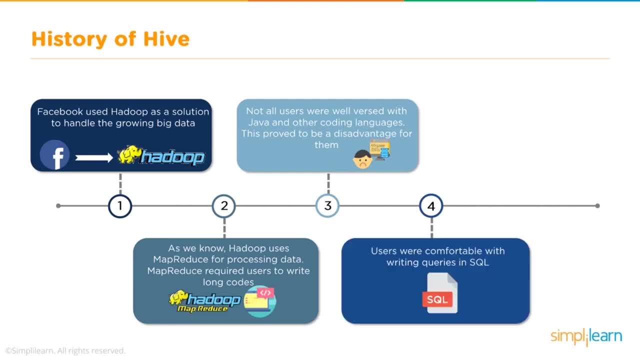 be a disadvantage for them. Users were comfortable with writing- writing queries in SQL. SQL has been around for a long time. the standard SQL query language, Hive, was developed with the vision to incorporate the concepts of tables, columns, just like SQL. 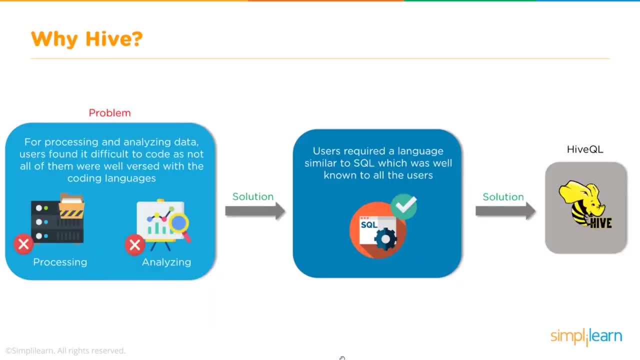 So why Hive? Well, the problem was for processing and analyzing data. users found it difficult to code as not all of them were well versed with the coding languages. You have your processing, you have your analyzing, And so the solution was required: a language similar to SQL, which was well. 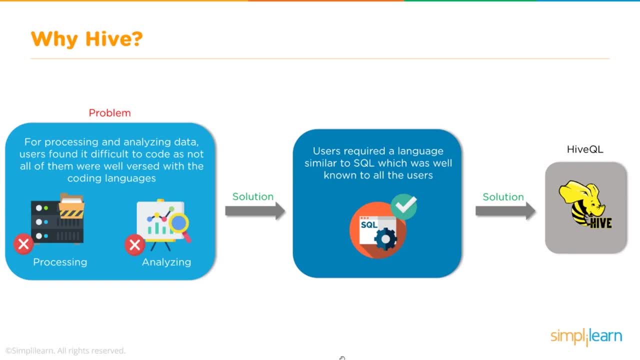 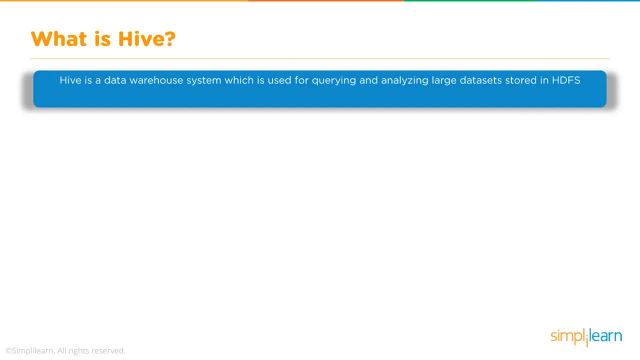 known to all the users And thus the Hive or HQL language evolved. What is Hive? Hive is a data warehouse system which is used for querying and analyzing large data sets stored in the HDFS or the Hadoop file system. Hive uses a query. 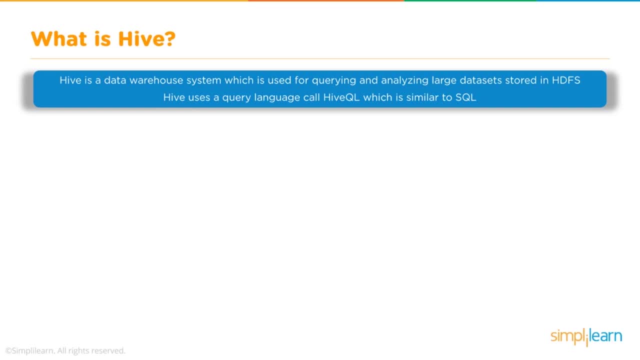 language that we call HiveQL or HQL, which is similar to SQL. So if we take our user, the user sends out their Hive queries and then that is converted into a MapReduce tasks and then accesses the Hadoop MapReduce system. 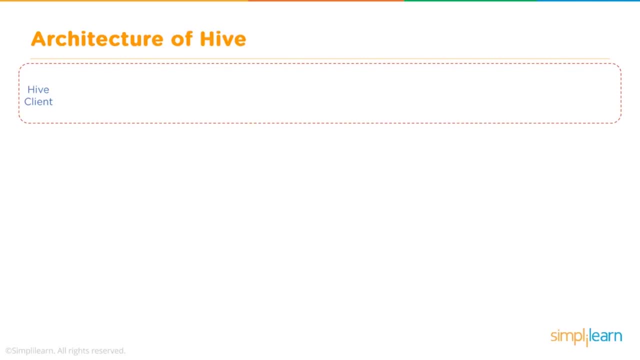 Let's take a look at the architecture of Hive. Architecture of Hive: We have the Hive client, So that could be the programmer, or maybe it's the manager who knows enough SQL to do a basic query to look up the data they need. The Hive client supports different types of client applications in different languages for performing queries. 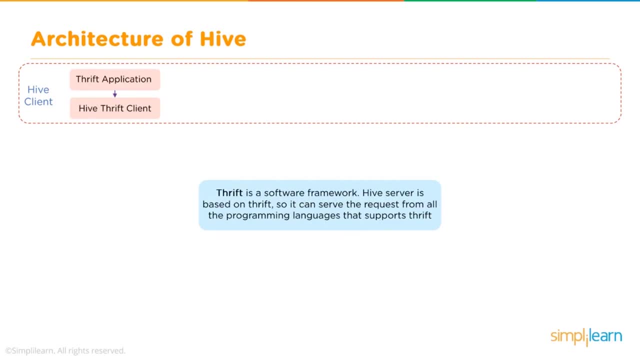 And so we have our Thrift application and the Hive Thrift client. Thrift is a software framework. Hive server is based on Thrift so it can serve the request from all programming languages that support the Hive client. And then we have our JDBC application and the Hive JDBC driver. JDBC- Java Database Connectivity- JDBC application. 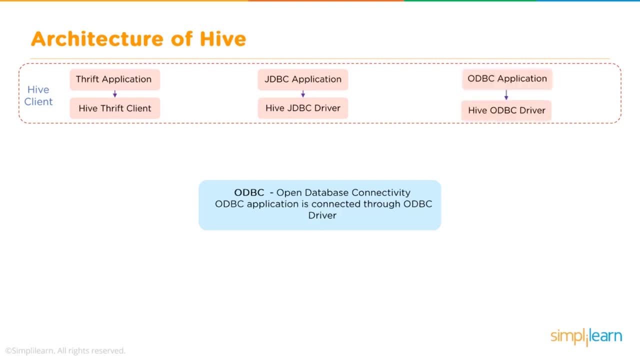 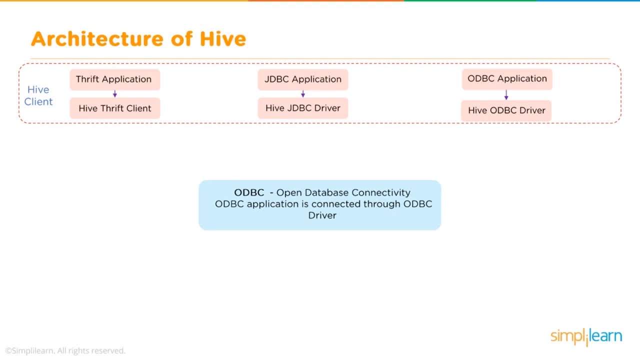 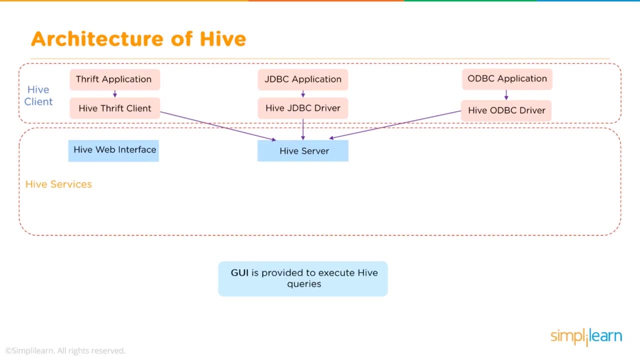 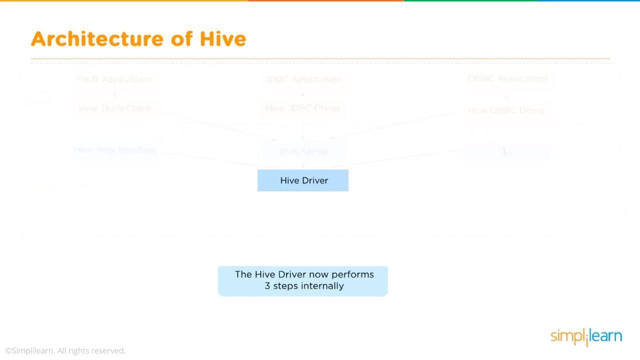 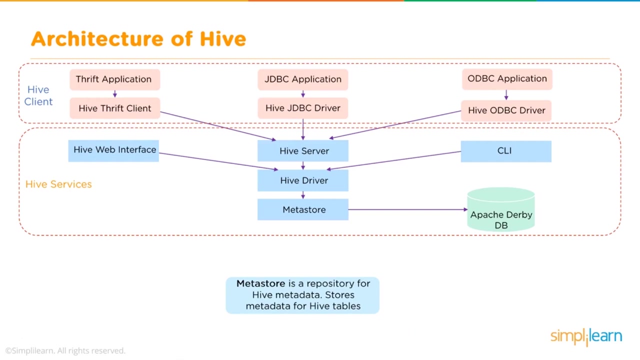 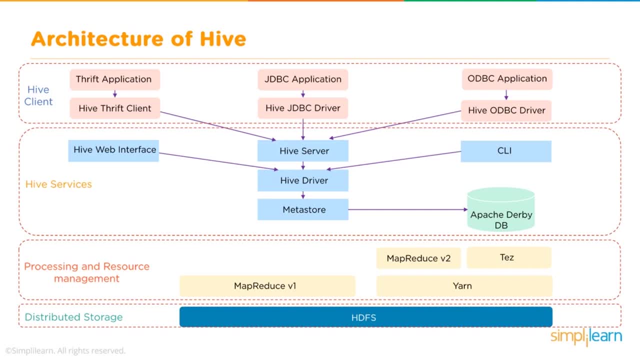 you'll know that these are on commodity machines and are linearly scalable. That means they're very affordable. A lot of time, when you're talking about big data, you're talking about a tenth of the price of storing it on enterprise computers. And then we look at the data flow in Hive. 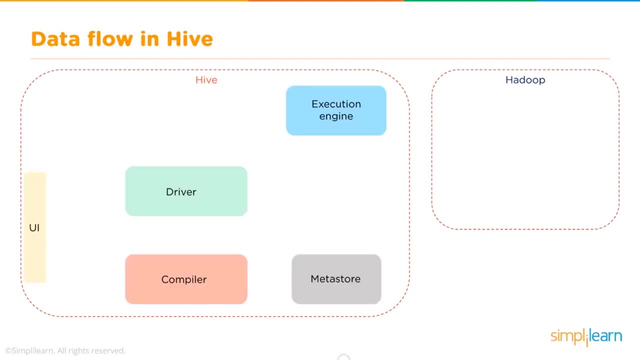 So in our data flow in Hive we have our Hive and the Hadoop system And underneath the user interface or the UI we have our driver, our compiler, our execution engine and our metastore. That all goes into the MapReduce and the Hadoop file system. 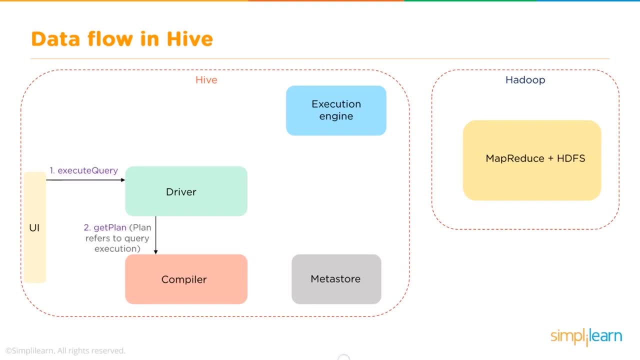 So when we execute a query, you can see it coming in here. It goes into the driver. step one, Step two. we get a plan. What are we going to do? It refers to the query execution. Then we go to the metadata. 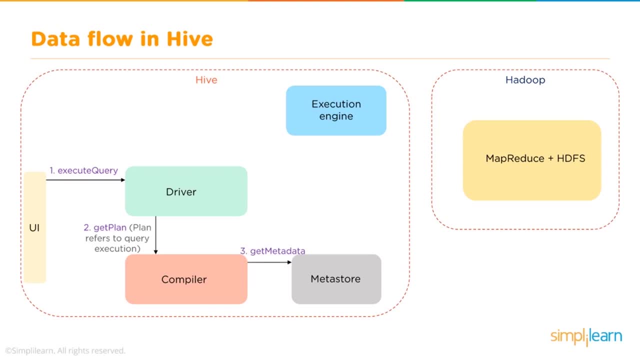 It's like: well, what kind of metadata are we actually looking at? Where is this data located? What is the schema on it? Then it comes back with the metadata into the compiler. Then the compiler takes all that information and the send plan returns it to the driver. 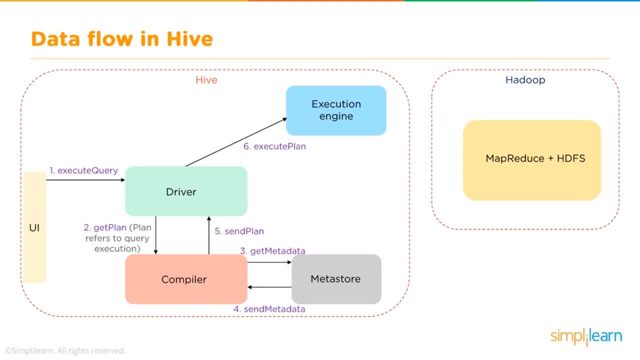 The driver then sends the execute plan to the execution engine. Once it's in the execute, the execution engine acts as a bridge between Hive and Hadoop to process the query And that's going into your MapReduce and your Hadoop file system or your HDFS. 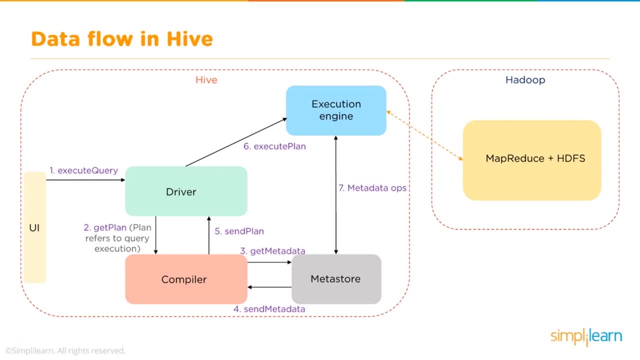 And then we come back with the metadata operations. It goes back into the metastore to update or let it know what's going on, which also goes to the communication between the execution engine and the metastore. Execution engine communications is bidirectionally with the metastore. 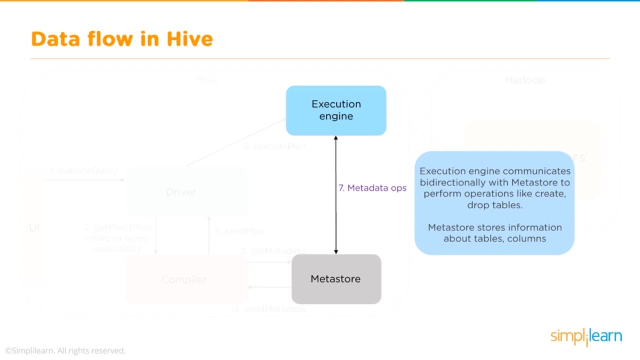 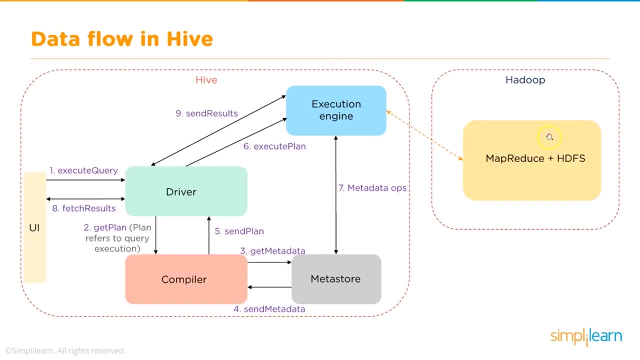 to perform operations like create drop tables. metastore stores information about tables and columns. So again we're talking about the schema of your database And once we have that, we have a bidirectional, a send results communication back into the driver and then we have the fetch results. 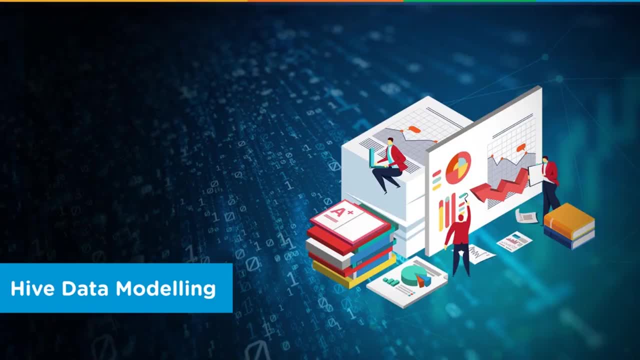 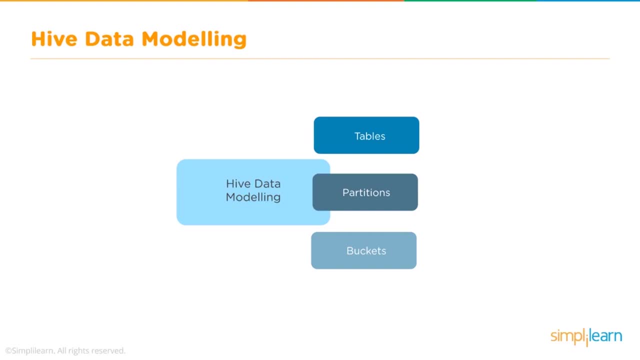 which goes back to the client. So let's take a little bit look at the Hiv data modeling, Hive data modeling. So you have your high data modeling, You have your tables, you have your partitions and you have buckets. The tables in Hive are created the same way. 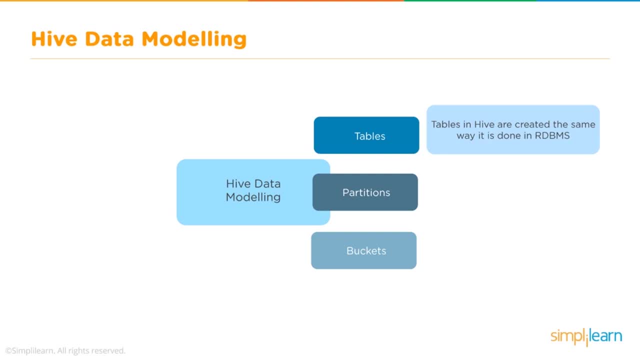 It is done in rdbms. so when you're looking at your traditional sql server or my sql server, where you might have enterprise equipment and a lot of people pulling and removing stuff off of there, the tables are going to look very similar and this makes it very easy to take that information. and, let's say, you. 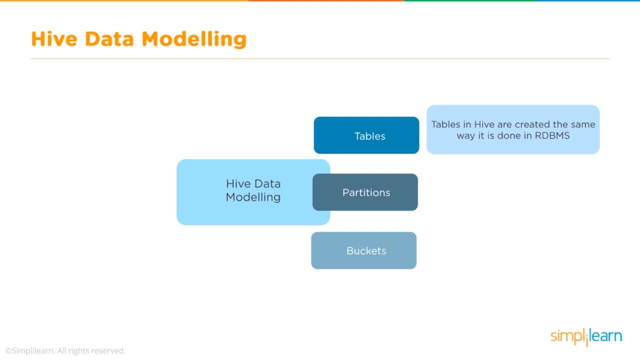 need to keep current information but you need to store all of your years of transactions back into the hadoop hive so you match those. those all kind of look the same, the tables are the same, your databases look very similar and you can easily import them back. you can easily store. 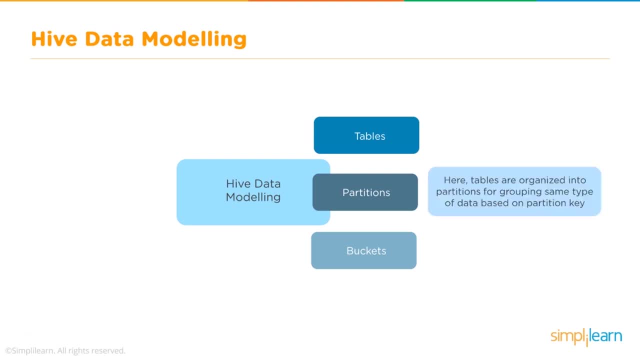 them into the hive system partitions: here tables are organized into partitions for grouping same type of data based on partition key. this can become very important for speeding up the process of doing queries. so if you're looking at dates as far as like your employment dates of employees, if 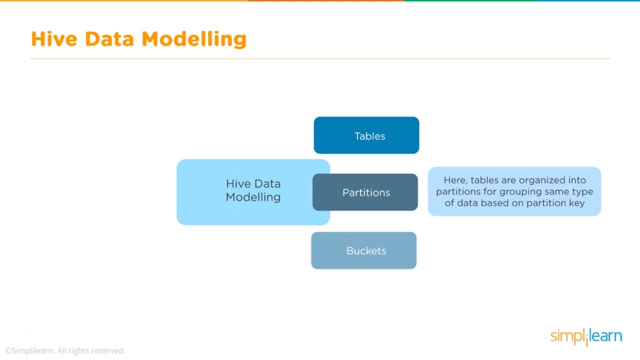 that's what you're tracking. you might add a partition there, because that might be one of the key things that you're always looking up as far as employees are concerned. and finally, we have a little bit more information about what you're looking for in the sql server. so if you're looking 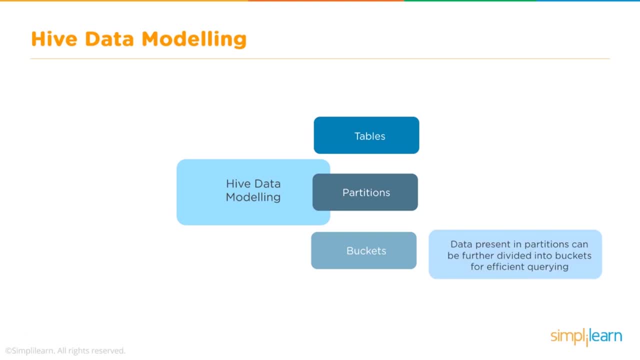 at buckets. data present in partitions can be further divided into buckets for efficient querying. again, there's that efficiency at this level. a lot of times you're taught you're working with the programmer and the admin of your hadoop file system to maximize the efficiency of that. 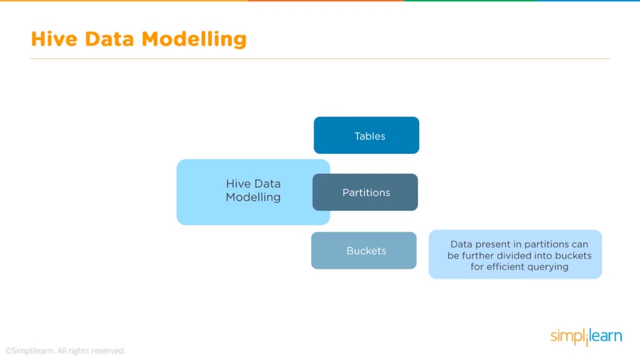 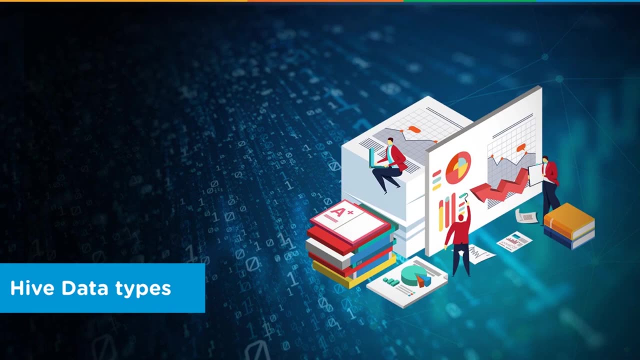 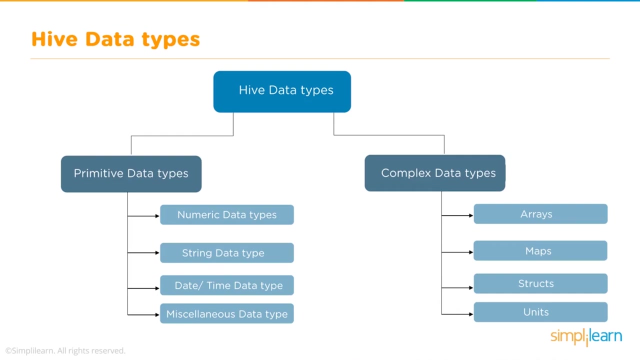 file system, so it's usually a two-person job and we're talking about hive data modeling. you want to make sure that they work together and you're maximizing your resources- hive data types. so we're talking about hive data types. we have our primitive data types and our complex data types. a lot of this will look. 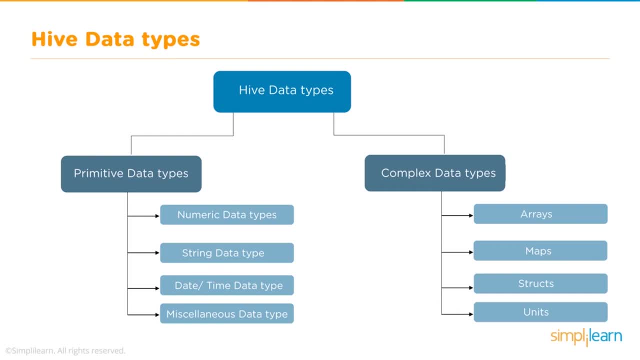 familiar because it mirrors a lot of stuff in sql. in our primitive data types we have the numerical data types, string data type, date time data type and miscellaneous data type, and these should be very, they're kind of self-explanatory. but just in case numerical data is your floats, your integers. 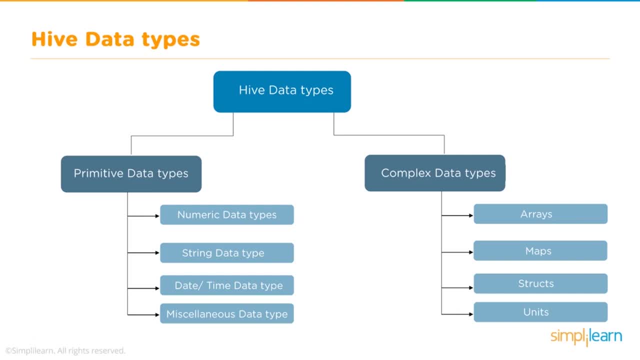 your short integers. all of that numerical data comes in as a number. a string of course is characters in number, and a string of course is characters in number and a string of course is numbers. and then you have your date, time stamp, and then we have kind of a general way of pulling. 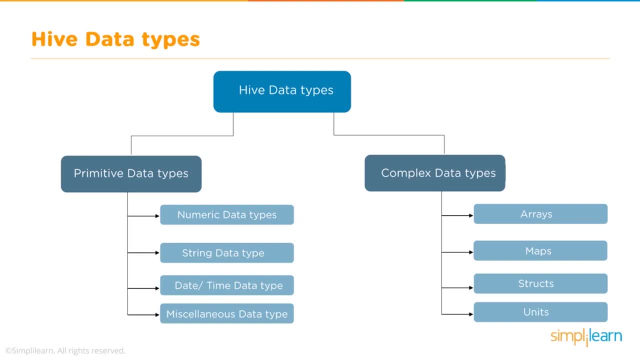 your own created data types in there. that's your miscellaneous data type, and we have complex data types. so you can store arrays, you can store maps, you can store structures and even units in there, as we dig into hive data types and we have the primitive data types and the complex data types. 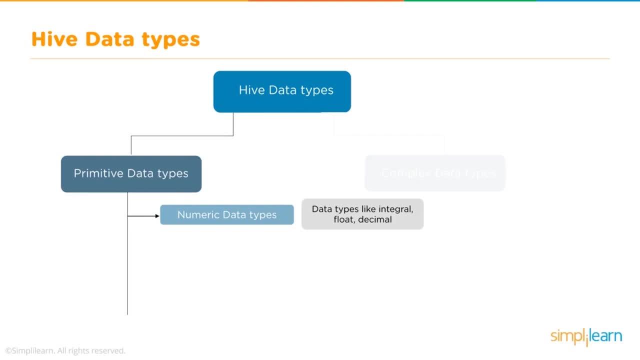 so we look at primitive data types and we're looking at numeric data types, data types like an integer, a float, a decimal. those are all the things that we're going to be looking at in this data type and they're all stored as numbers in the hive data system, a string data type- data types. 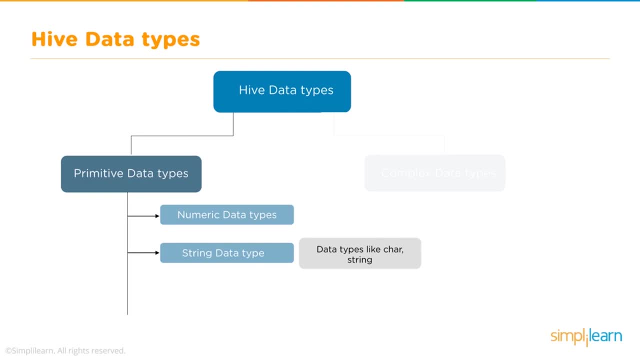 like characters and strings, you store the name of the person you're working with- uh, you know, john doe. the city memphis, the state tennessee, maybe it's uh, boulder, colorado, usa, or maybe it's hyperbad india. that's all going to be string and stored as a string character and, of course, we have our date. 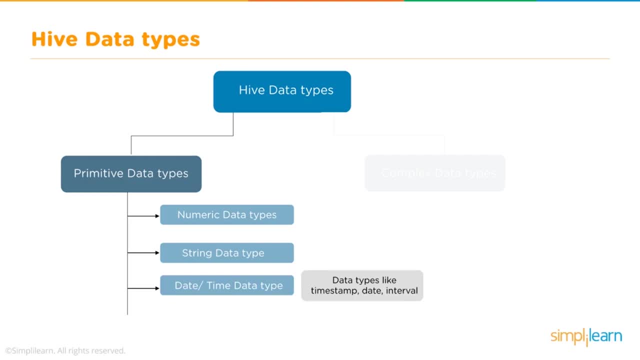 time data type, data types like timestamp, date interval. those are very common, so you can just think if you can type a stamp of time on it. or maybe you're dealing with the race and you want to know the interval. how long did the person take to complete whatever task it was? 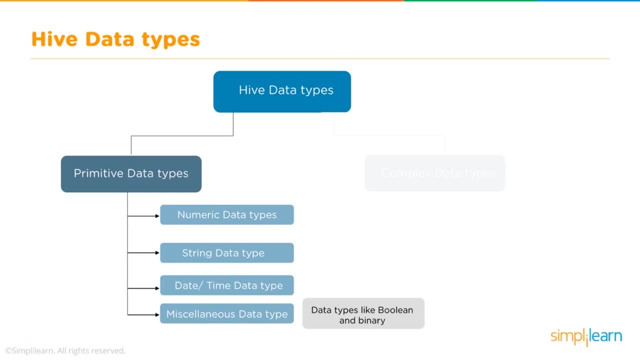 all that is date time data type. and then we talk miscellaneous data type. these are like boolean and binary, and when you get into boolean and binary you can actually almost create anything in there, but your yes knows zero one. now let's take a look at complex data types a little closer. 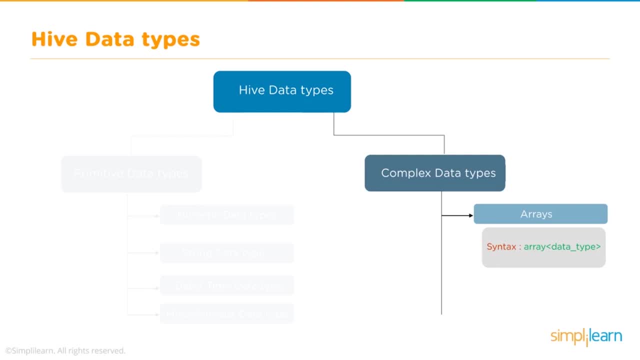 we have arrays, so your syntax is of data type and it's an array and you can just think of a array as a collection of same entities: one, two, three, four, if they're all numbers- and you have maps, this is a collection of key value pairs. so understanding maps is so central to hadoop. 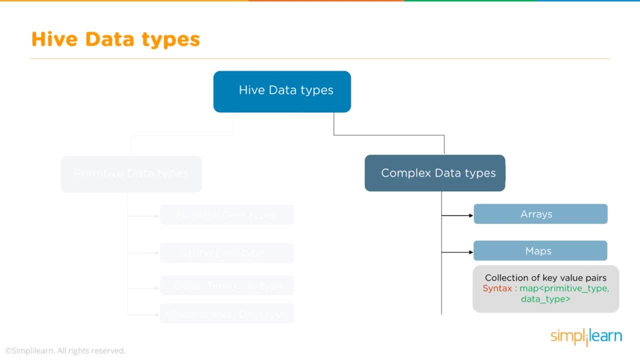 so, when we store maps, you have a key which is a set. you can only have one key per mapped value, and so you, in hadoop, of course, you collect, uh, the same keys and you can add them all up or do something with all the contents of the same key, but this is our map as a primitive type, data type. 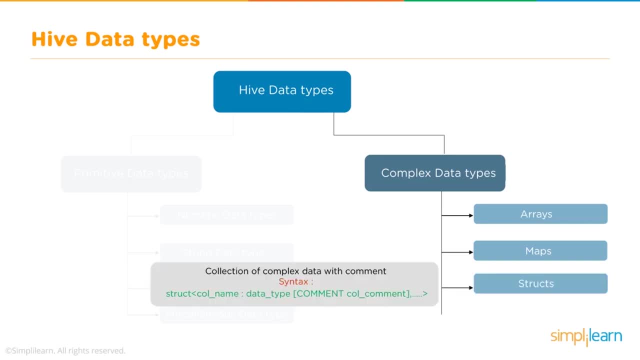 and our collection of key value pairs and then collection of complex data with comment, so we can have a structure where you have, like column name, data type, comment, call a column comment, uh, so you can get very complicated structures in here with your collection of data and your comment and setup. 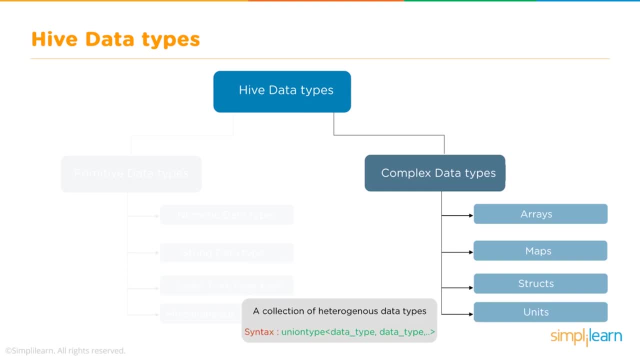 and then we have units, and this is a collection of heterogeneous data types. so the syntax for this is union type, data type, data type and so on. so it's all going to be the same, a little bit different than the arrays where you can actually mix and match different. 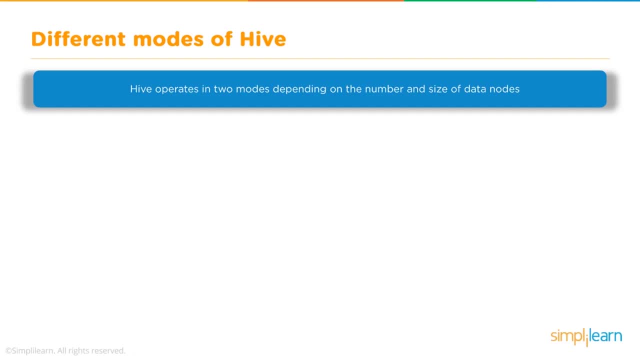 modes of hive. hive operates in two modes depending on the number and size of data nodes. we have our local mode and our map reduce mode. when we talk about the local mode, it is used when hadoop is having one data node and the data is small. processing will be very fast on a smaller data. 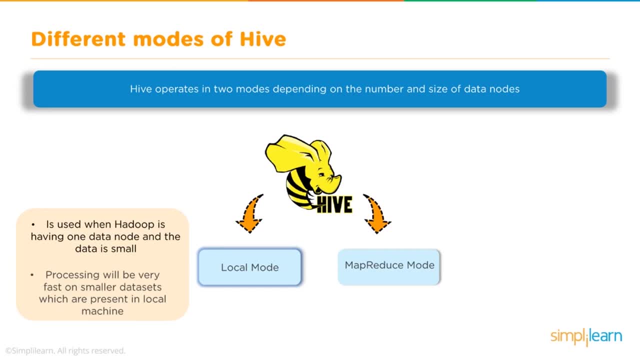 sets which are present in local machine, and this might be that you have a local file stuff you're uploading into the hive and you need to do some processes in there. you can go ahead and run those hive processes and queries on it. usually you don't see much in the way of a single node hadoop system. if you're going to do that, you 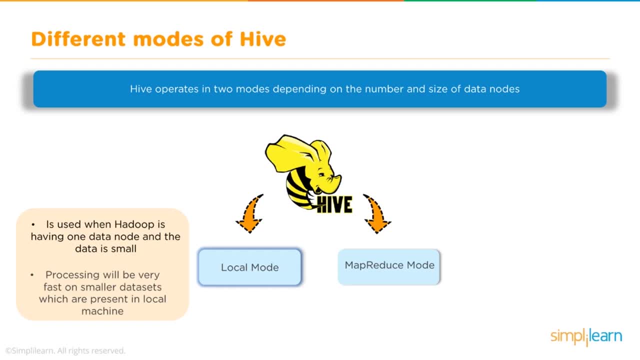 might as well just use like an sql database or even a java sqlite or something. python is sqlite, so you don't really see a lot of single node hadoop databases. but you do see the local mode in hive where you're working with a small amount of data that's going to be integrated into. 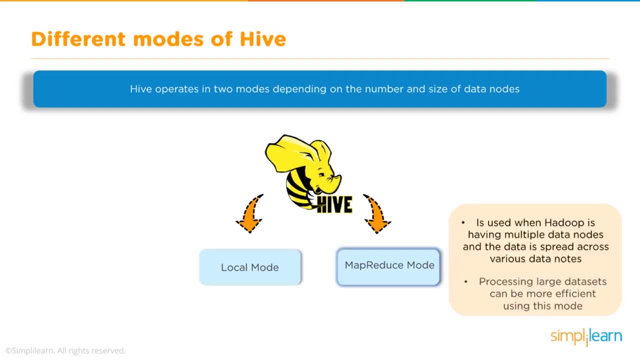 the larger database. and then we have the map reduce mode. this is used when hadoop is having multiple data nodes and the data is spread across various data nodes. processing large data sets can be more efficient using this mode, and this you can think of, instead of it being one, two, three or even five computers, we're usually talking with the hadoop file system. 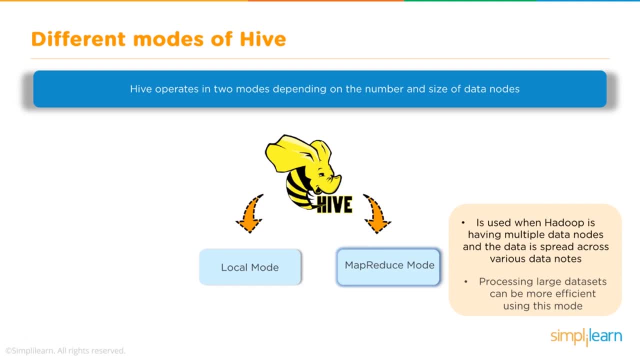 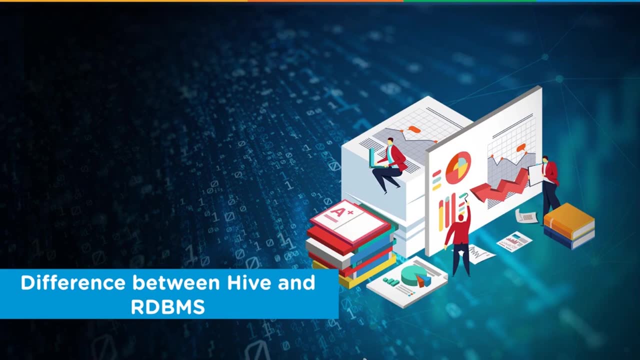 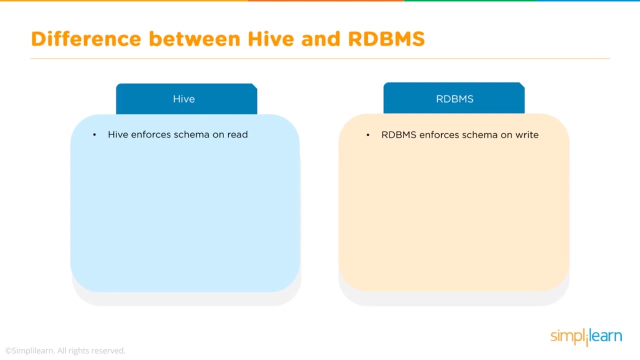 we're looking at 10 computers, 15, 100, where this data is spread across all those different hadoop nodes. difference between hive and rdbms: remember, rdbms stands for the relational database management system. let's take a look at the difference between hive and the rdbms with hive. 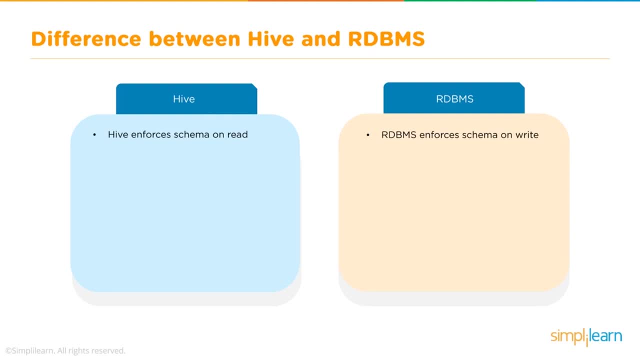 hive enforces schema on read and it's very important that whatever's coming in, that's when hive's looking at it and making sure that it fits the model- the rdbms enforces a schema when it actually writes the data into the database. so it's read the data and then once 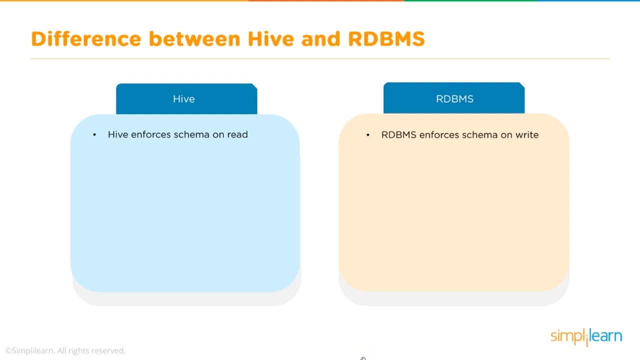 it starts to write it. that's where it's going to give you the error, tell you something's incorrect about your scheme. hive data size is in petabytes. that is hard to imagine. you know. when we're looking at your personal computer on your desk, maybe you have 10 terabytes. if it's. 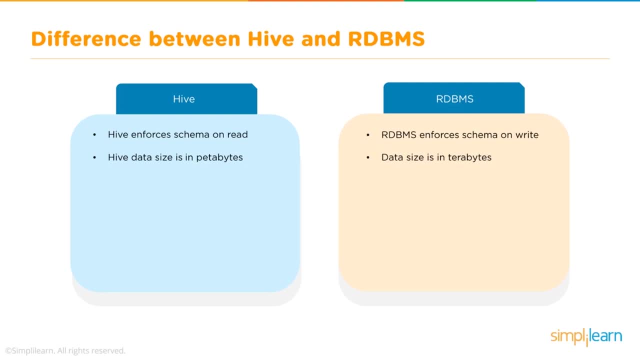 a high-end computer. we're talking petabytes, so that's hundreds of computers grouped together when rdbms data size is in terabytes. very rarely do you see an rdbms system that's spread over more than five computers, and there's a lot of reasons for that. with the rdbms it actually has a high-end. 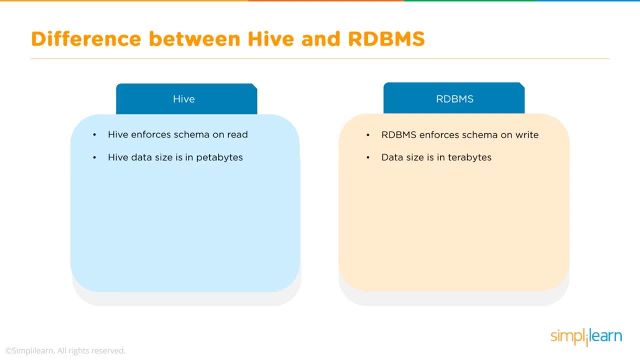 amount of rights to the hard drive. there's a lot more going on there. you're writing and pulling stuff, so you really don't want to get too big with an rdb master. you're going to run into a lot of problems with hive. you can take it as big as you want. you can take it as big as you want. 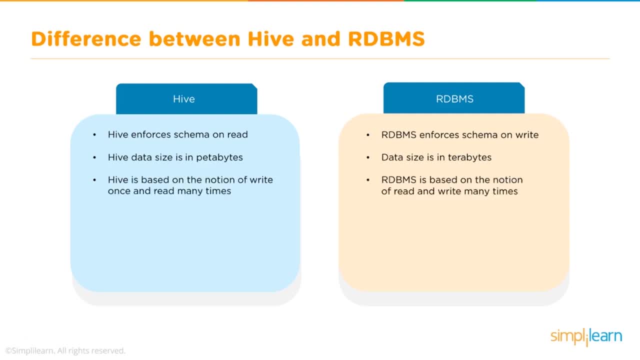 hive is based on the notion of write once and read many times. this is so important. they call it worm, which is right. w once o read r many times m they refer to it as worm, and that's true of any of you. a lot of your hadoop setup it's. it's altered a little bit, but in general we're looking. 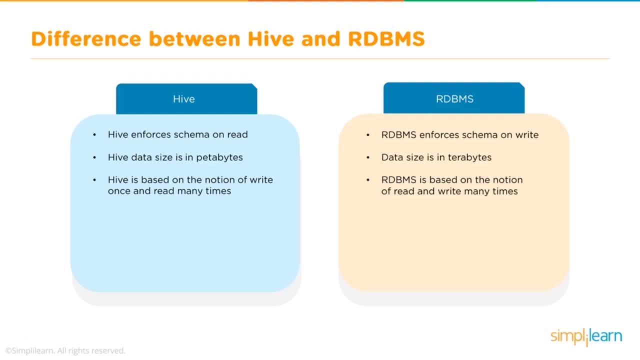 at archiving data that you want to do data analysis on. we're looking at pulling all that stuff off your rdbms from years and years and years of business or whatever your company does, or scientific research, and putting that into a huge data pool so that you can now do queries on it and get that information. 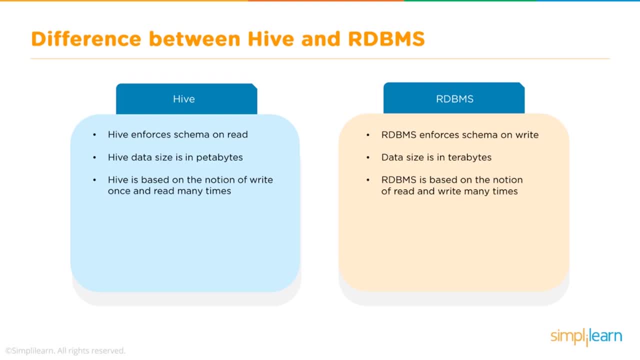 out of it with the rdbms. it's based on the notion of read and write many times. so you're continually updating this database. you're continually bringing up new stuff, new sales. the account changes because they have a different licensing now. whatever software you're selling all that kind of stuff. 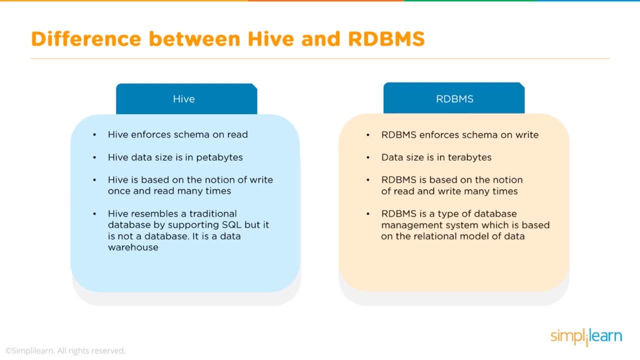 where the data is continually fluctuating, and then hive resembles a traditional database by supporting sql, but it is not a database, it is a data warehouse. this is very important. it goes with all the other stuff we've talked about that we're not looking at a database, but a data warehouse to store the data and still have 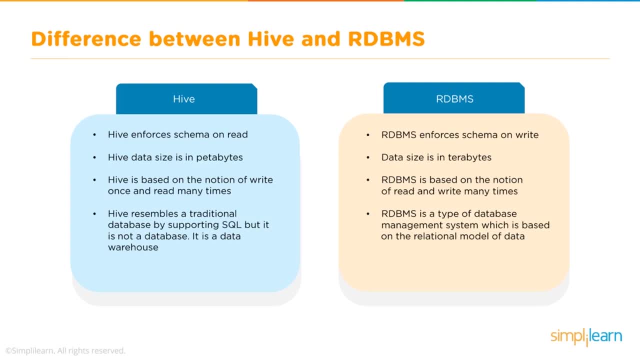 fast and easy access to it for doing queries. you can think of twitter and facebook. they have so many posts that are archived back historically. those posts aren't going to change. they made the post, they're posted, they're there and they're in their database, but they have to store it in. 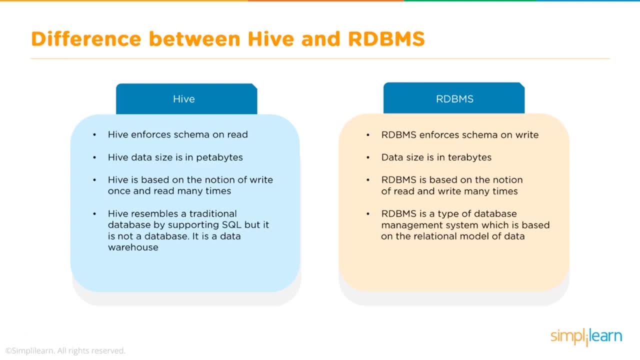 a warehouse in case they want to pull it back up with the rdbms. it's a type of database that's going to be a database management system which is based on the relational model of data and then, with hive, easily scalable at a low cost. again. we're talking maybe a thousand dollars per terabyte. 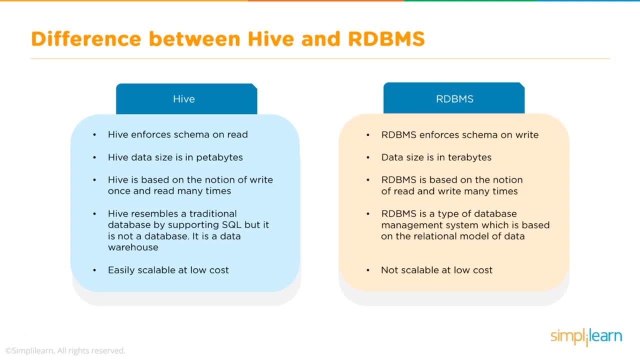 the rdbms is not scalable at a low cost. when you first start on the lower end, you're talking about 10 000 per terabyte of data, including all the backup on the models and all the added necessities to support it. as you scale it up, you have to scale those computers and hardware up so you might start. 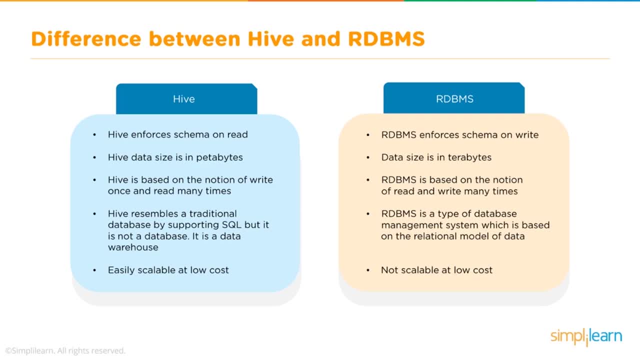 with a basic server and then you upgrade to a sun computer to run it and you spend, you know, tens of thousands of dollars for that hardware upgrade. with hive you just put another computer into your hadoop file system. so let's look at some of the features of hive. when we're looking at the features, 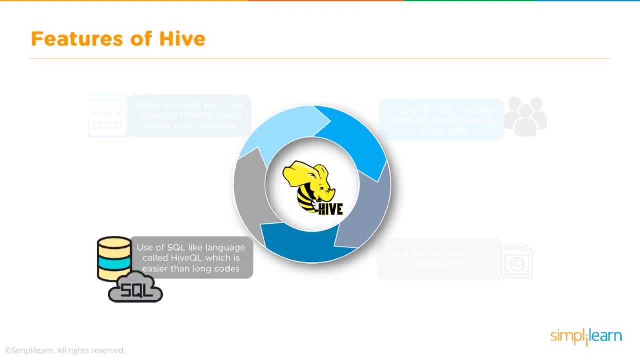 of hive. we're talking about the use of sql like language called hiveql. a lot of times you'll see that as hql, which is easier than long codes. this is nice if you're working with your shareholders. you come to them and you say, hey, you can do a basic sql code, but you're not going to be able to. 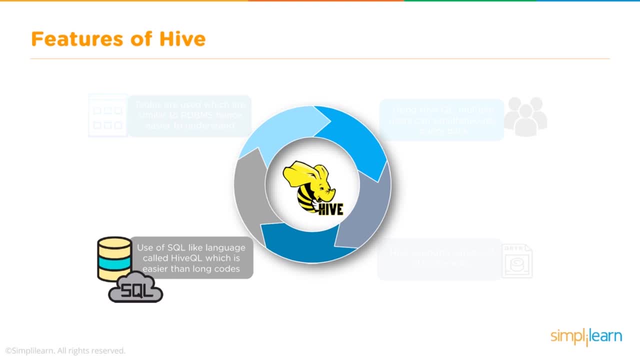 do a basic sql code. but you're going to be able to do a basic sql code, but you're not going to be able to on here and pull up the information you need. this way, you don't have to take off, have your programmers jump in every time they want to look up something in the database. they actually now. 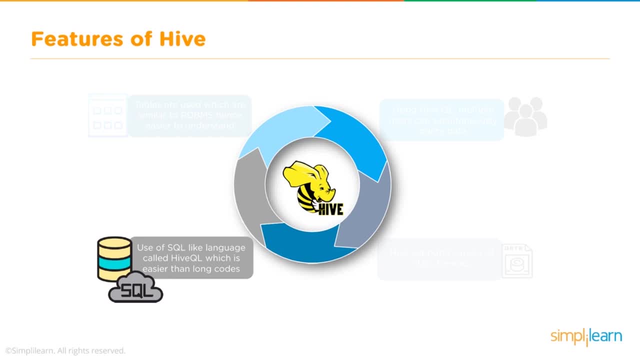 can easily do that if they're not skilled in programming and script writing. tables are used which are similar to the rdbms, hence easier to understand, and one of the things i like about this is when i'm bringing tables in from a mysql server sql server. there's almost a direct 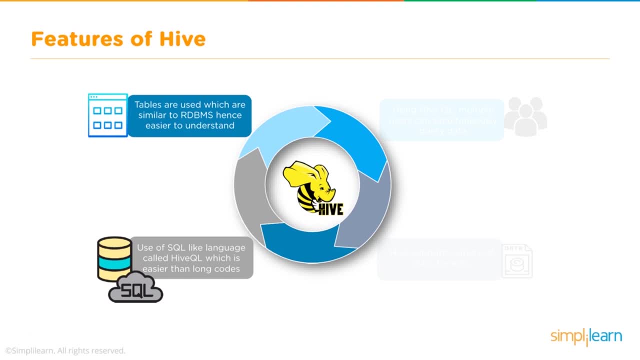 reflection between the two. so when you're looking at one, which is the data which is continually being used in the database, it's not this huge jump where you have to learn a whole new language. you mirror that same schema into the hdfs, into the hive, making it very easy to go between the. 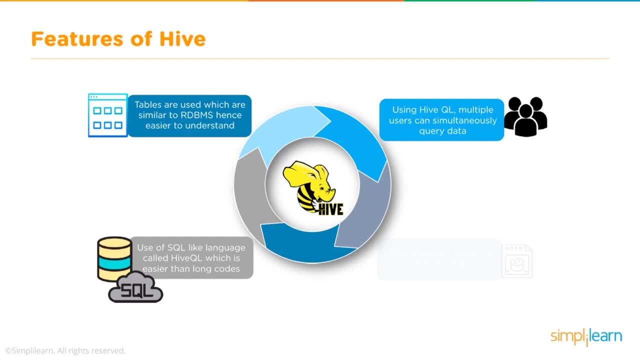 two and then, using hiveql, multiple users can simultaneously query data. so again you have multiple clients in there and they send in their query. that's also true with the rdbms, which kind of queues them up because it's running so fast you don't notice the lag time. well, you get that. 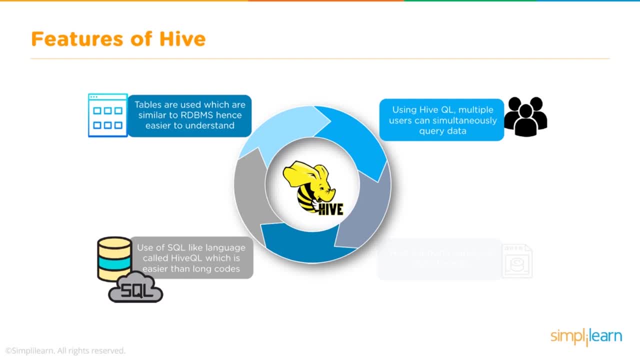 also with the hql. as you add, more computers in the hql server is going to be able to do that query can go very quickly depending on how many computers and how much resources each machine has to pull the information. and hive supports a variety of data types. so with hive it's designed. 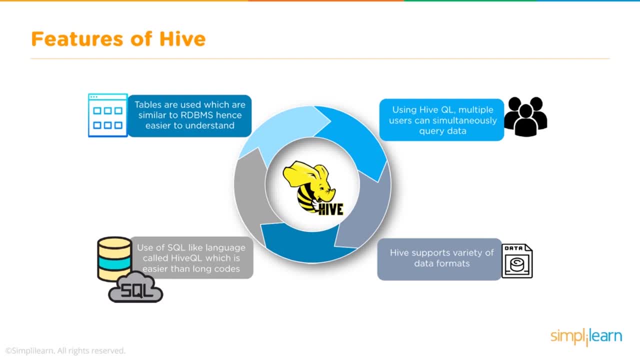 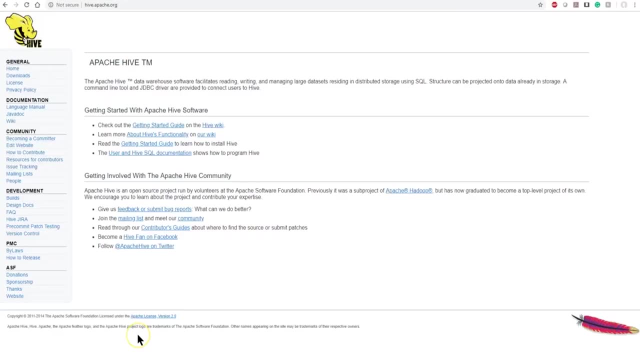 to be on the hadoop system, which you can put almost anything into the hadoop file system. so with all that, let's take a look at a demo on hive ql or hql. before i dive into the hands-on demo, let's take a look at the website hiveapacheorg. 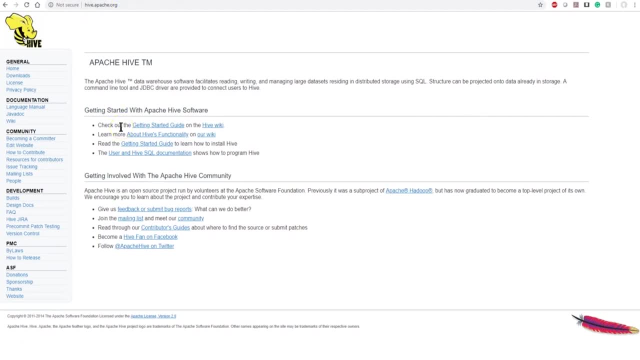 that's the main website, since apache- it's an apache open source software- this is the main software for the main site for the build, and if you go in here you'll see that they're slowly migrating hive into beehive and so if you see beehive versus hive, note the beehive is the new. 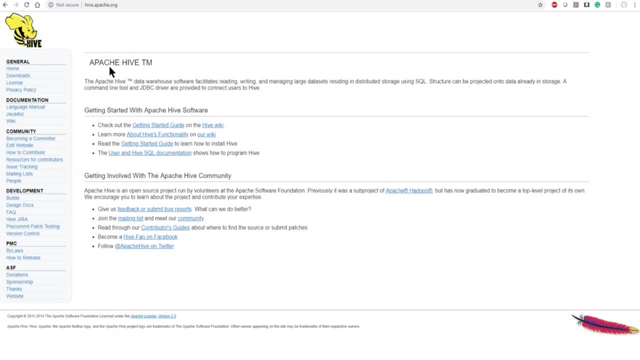 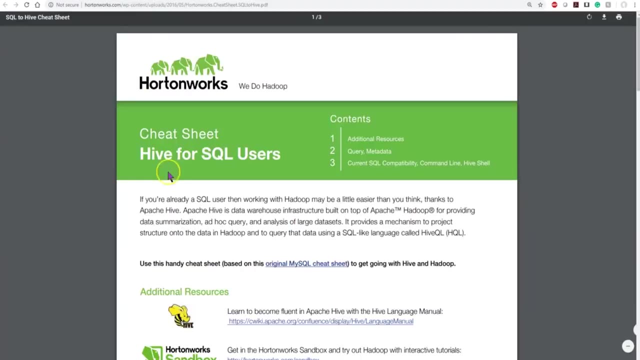 releases coming out. that's all it is. it reflects a lot of the same functionality of hive. it's the same thing. and then we like to pull up some kind of documentation on commands, and for this i'm actually going to go to hortonworkscom hivethivecheatsheet, and that's because hortonworks and cloudera are two of the most common used. 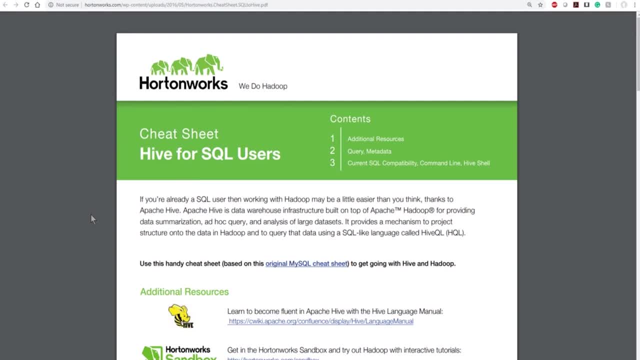 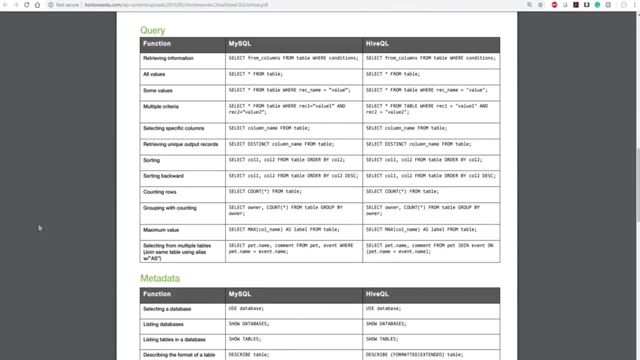 builds for hadoop and for which include hive and all the different tools in there, and so hortonworks has a pretty good pdf. you can download cheat sheet on there. i believe cloudera does too, but we'll go ahead and just look at the horton one, because it's the one that comes up really. 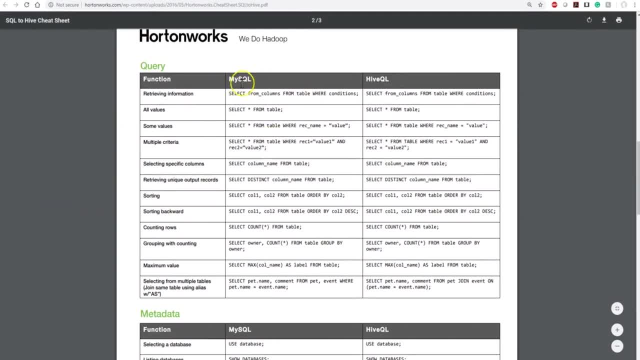 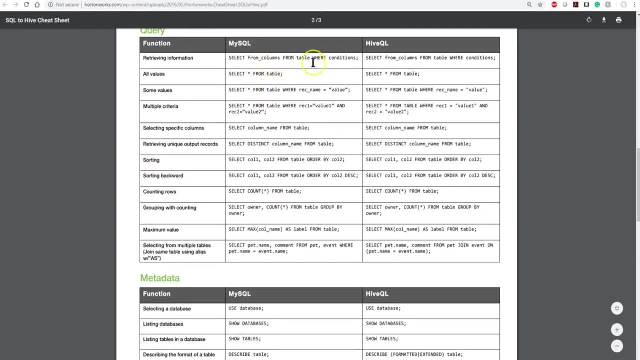 good and you can see when we look at the query language it compares mysql server to hive ql or hql and you can see the basic select. we select from columns, from table where conditions exist. you know most basic command on there and they have different things. you can do with it just like you do with your sql and if you scroll down you'll see. 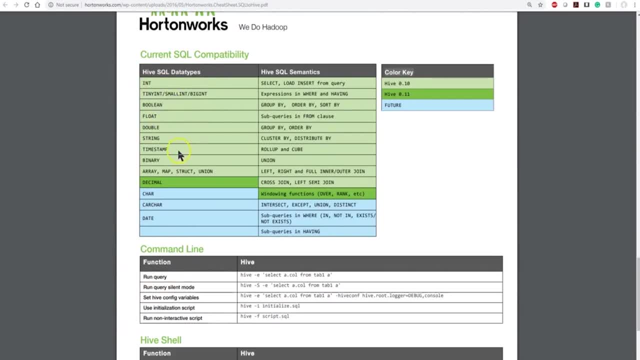 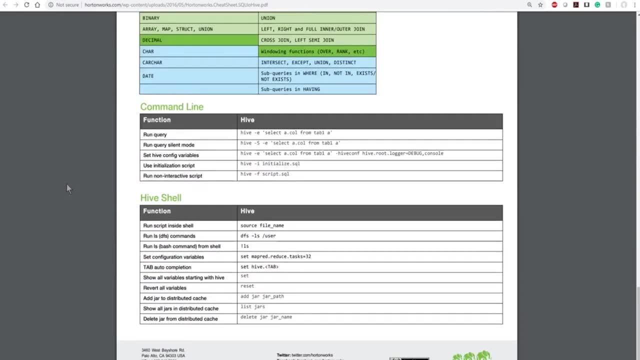 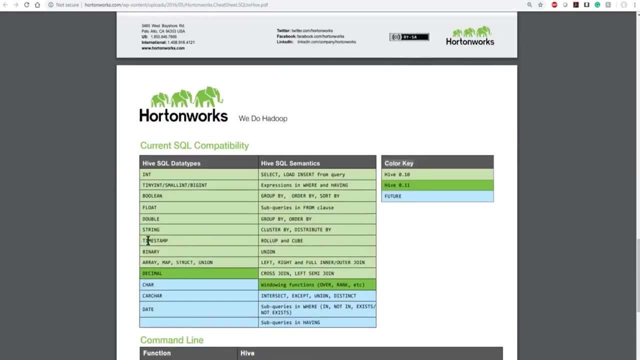 data types. so here's your integer, your flow, your binary double string timestamp and all the different data types. you can use some different semantics, different keys, features, functions for running a hive query, command line setup and, of course, the hive shell setup in here so you can loop through it. it has a lot of your basic stuff and it is. we're basically looking at sql. 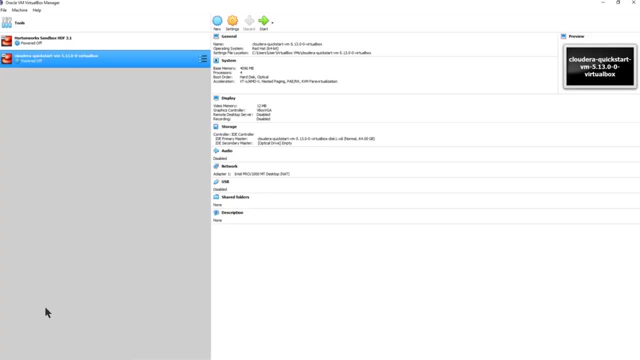 across a horton database. we're going to go ahead and run our hadoop cluster hive demo and i'm going to go ahead and use the cloudera quick start and this is in the virtual box. so again, we have an oracle virtual box, which is open source, and then we have our cloudera quick start, which is the 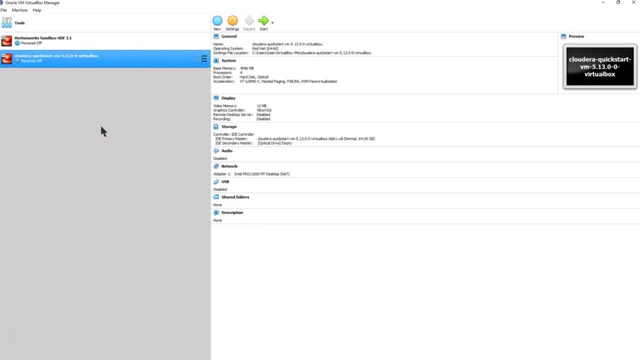 hadoop setup on a single node. now, obviously hadoop and hive are designed to run across a cluster of, and we talk about a single node is for education, testing, that kind of thing, and if you have a chance you can always go back and look at our demo we had on setting up a hadoop system in a 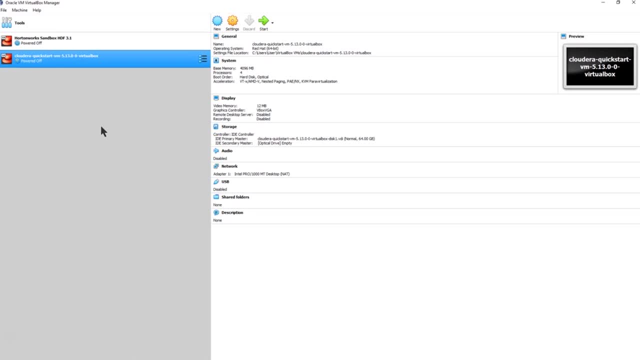 single cluster. just set a note down below in the youtube video and our team will get in contact with you and send you that link if you don't already have it, or you can contact us at the wwwsimplylearncom now in here. it's always important to note that you do need on your 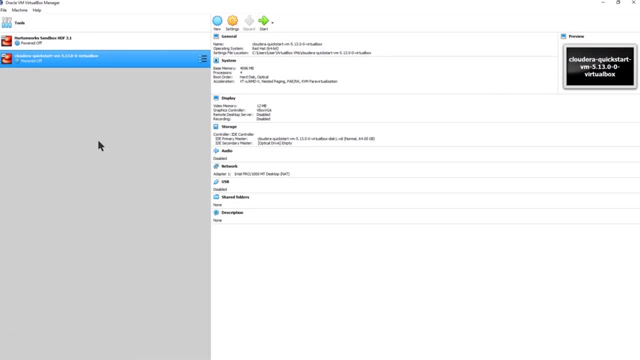 computer. if you're running on windows- because i'm on a windows machine and i'm running on a wikipedia- you're gonna need a probably about 12 gigabytes to actually run. this used to be goodbye with a lot less, but as things have evolved, they take up more and more. 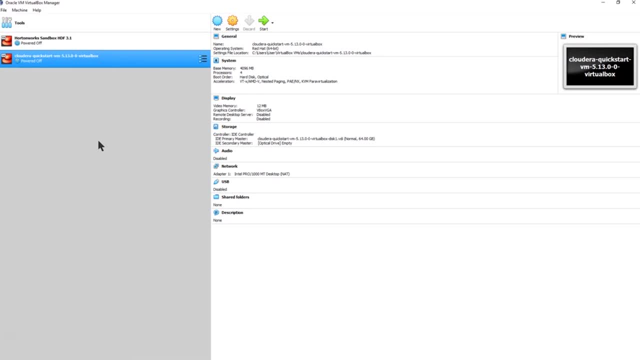 resources and you need the professional version if you have the home version. I was able to get that to run, but boy did it take a lot of extra work to get the home version to. let me use the virtual setup on there and we'll simply click on. 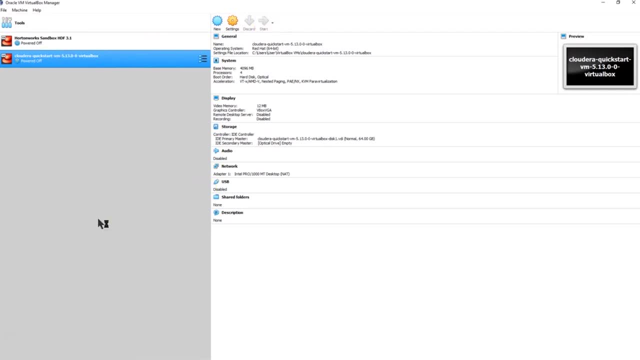 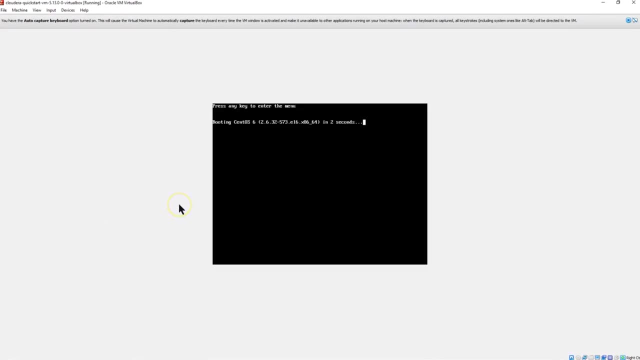 the cloud era, quick start. and I'm gonna go and just start that up. and this is starting up: our Linux. so we have our Windows 10, which is a computer I'm on, and then I have the virtual box, which is gonna have a Linux operating system in. 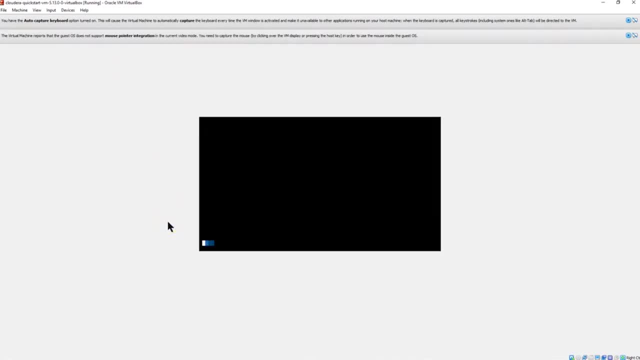 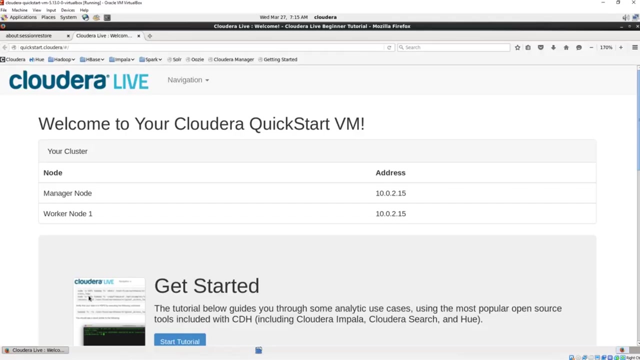 it and we'll skip ahead, so you don't have to watch the whole install. something interesting to know about the cloud era is that it's running on Linux, centos, and, for whatever reason, I've always had to click on it and hit the escape button for it to spin up, and then you'll see the DOS come in here. now that 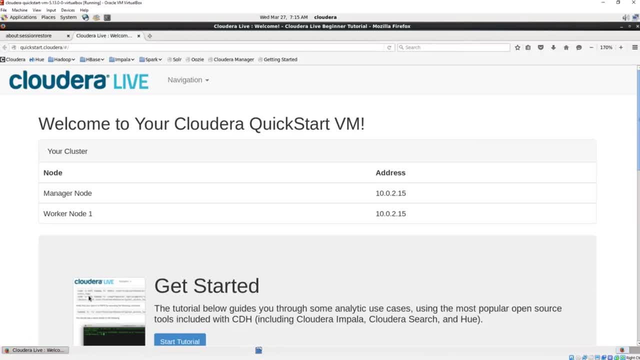 our cloud era is spun up on our virtual machine with the Linux on. we can see here we have our uses. the Thunderbolt browser on here by default and automatically opens up a number of different tabs for us. and a quick note, because I mentioned, like the restrictions on getting set up on your own computer if you have a home edition. 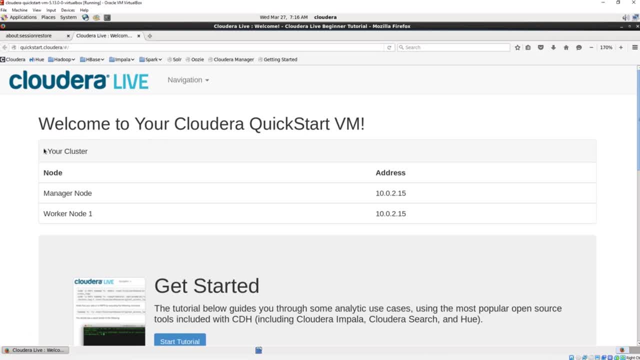 computer and you're worried about setting it up on there. you can also go in there and spin up a one month free service on Amazon web service to play with this. so there's other options. you're not stuck with just doing it on the quick start menu. you can spin this up in many other ways. now the first thing. 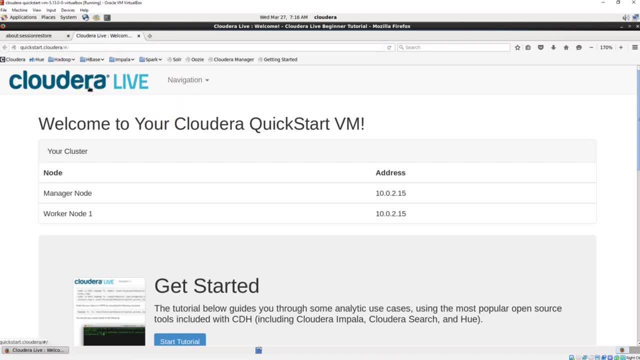 we want to note is that we've come in here into cloud era and i'm going to access this in two ways. the first one is we're going to use hue and i'm going to open a few will take a moment to load from the setup on here. 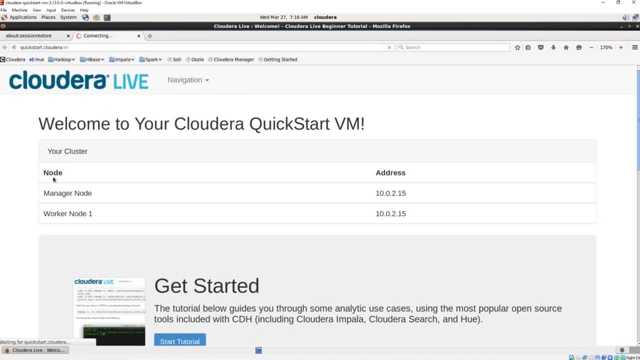 and hue is nice. if I go in and use hue as an editor into hive or into the dupe setup, usually i'm doing it as a from an admin side, because it has a lot more information, a lot of visuals, less to do with, you know, actually diving in there. 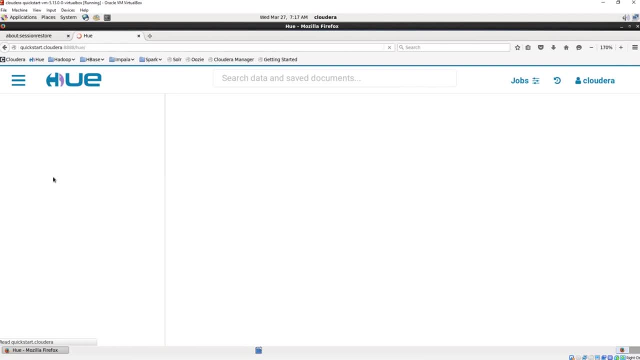 and just executing code, and you can also write this code into files and one file to come out there, that, but it's not called the container, and one example of what that means is just for your mouse to make a PU ever run the load can also write this code into files and scripts, and there's other things you can. 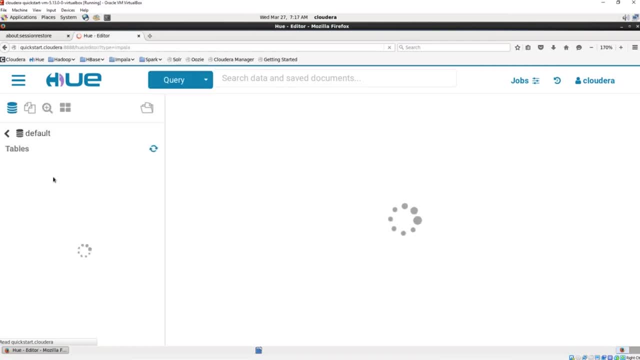 other ways you can upload it into hive. but today we're gonna look at the command lines and we'll upload it into hue and then we'll go into and actually do our work in a terminal window under the hive shell. now in the hue browser window, if you go under query and click on the pull down menu and then you go. 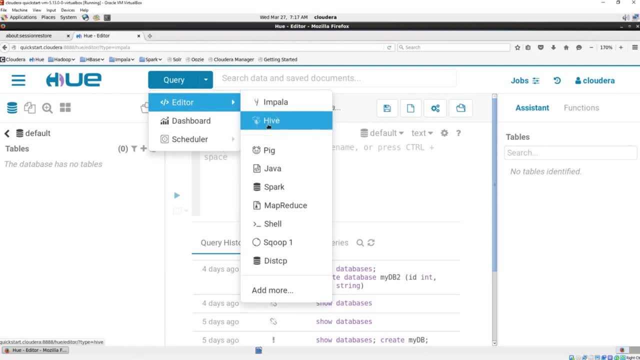 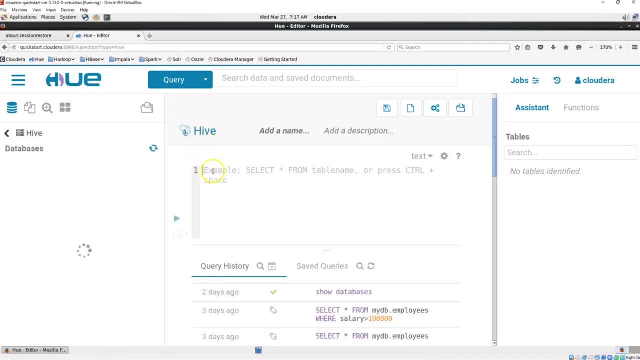 under editor and you'll see hive. there we go, there's our hive setup. I go and click on hive and this will open it up, our query down here, and now it has a nice little B that shows our hive going and we can go something very simple down. 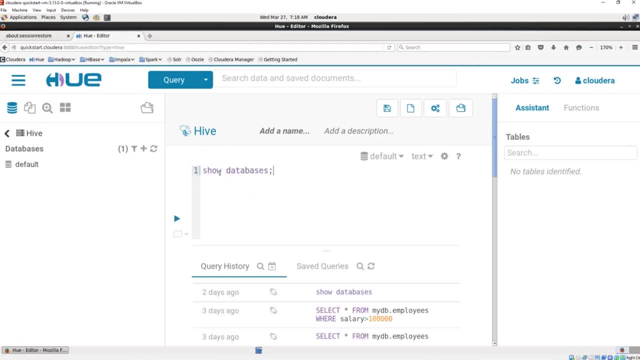 here like show databases, and we follow it with the semicolon and that's the standard in hive, as you always add our punctuation at the end there and I'll go ahead and run this and the query will show up underneath and you'll see down here, since this is a new quick start I just put on here, you'll see it has the. 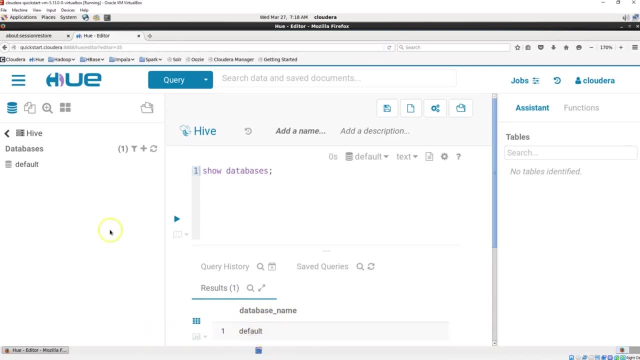 default down here for the databases. that's the database name. I haven't actually created any databases on here- and then there's a lot of other like attributes that we can add here, and then we'll go ahead and create a new assistant function tables your databases up here. there's all kinds of 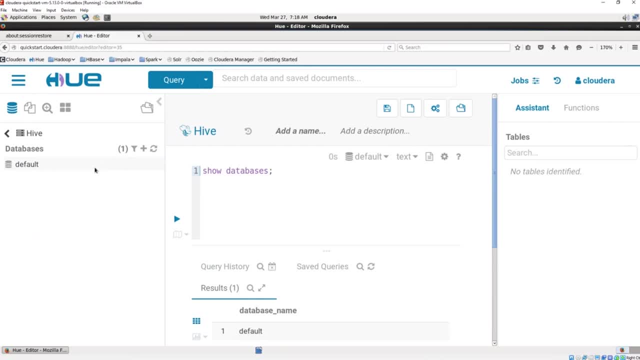 things you can research, you can look at through hue as far as a bigger picture. the downside of this is it always seems to lag for me. whenever I'm doing this, I always seem to run slow. so if you're in Cloudera, you can open up a terminal. 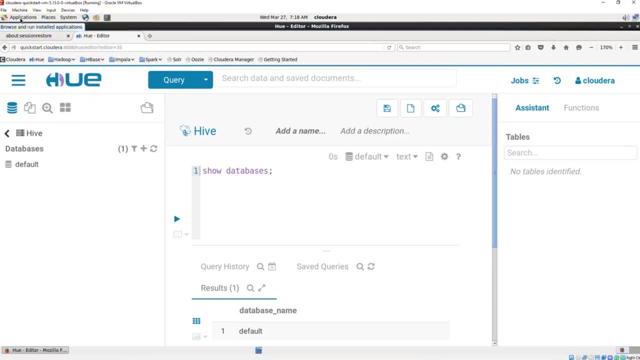 window. they actually have an icon at the top. you can also go under applications and under applications, system tools and terminal. either one will work. it's just a regular terminal window and this terminal window is now running underneath our Linux. so this is a Linux terminal window, or on our virtual machine, which 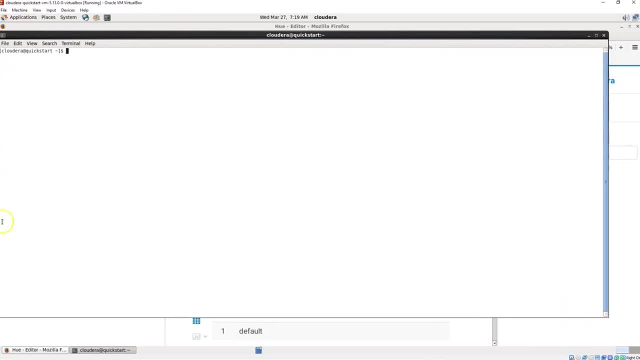 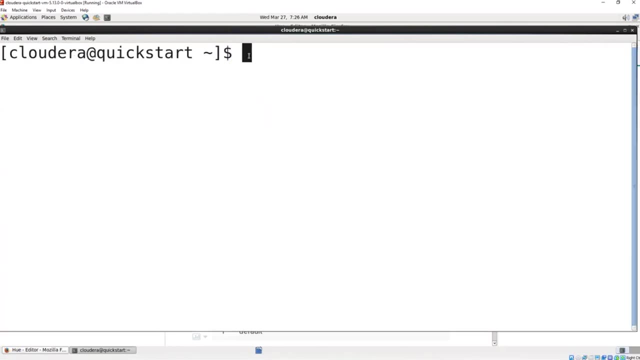 is resting on our regular Windows 10 machine and we'll go ahead and zoom this in so you can see the text better on your own video. I simply just clicked on view and zoom in and then all we have to do is type in hive and this will open up. 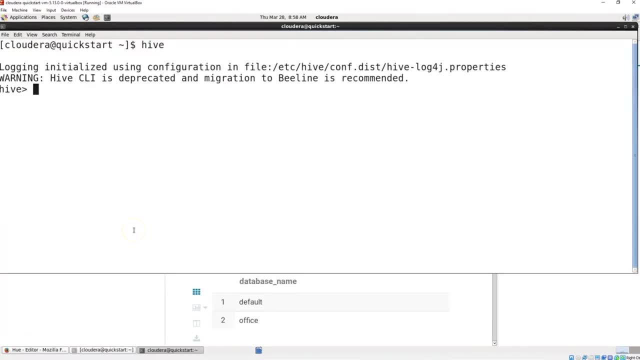 the shell on here and it takes it just a moment to load when starting up hive. I also want to note that, depending on your rights on the computer you're on in your action, you might have to do pseudo hive and put your password and username. most computers are usually set up with the hive login again, it just 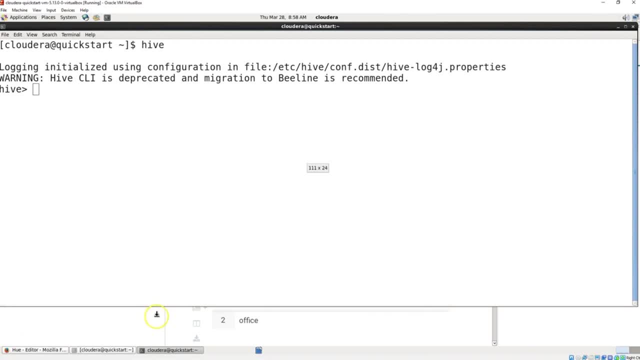 depends on how you're accessing the linux system and the hive shell. once we're in here, we can go ahead and do a simple uh hql command- show databases- and if we do that we'll see here that we don't have any databases. so we can go ahead and create a database and we'll just call it office. 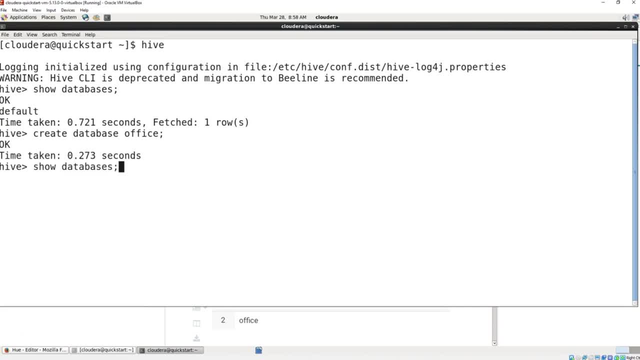 for today, for this moment. now, if i do show, we'll just do the up arrow. up arrow is a hot key that works in both linux and in hive, so i can go back and paste through all the commands i've typed in and we can see. now that i have my, there's of course a default database and then there's the. 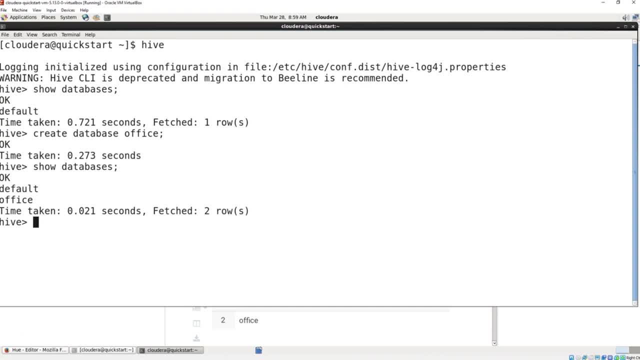 office database. so now we've created a database- it's pretty quick and easy and we go ahead and drop the database. we can do drop database office now. this will work on this database because it's empty. if your database was not empty, you would have to do cascade and that drops all the tables. 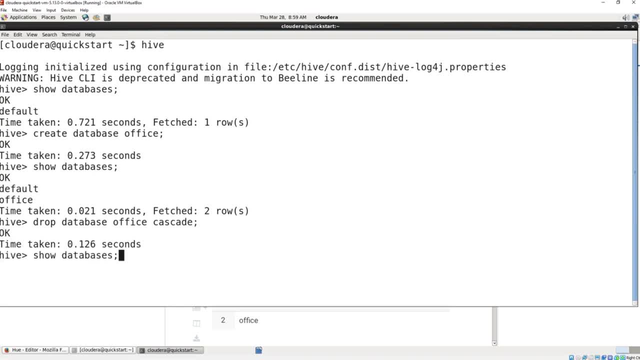 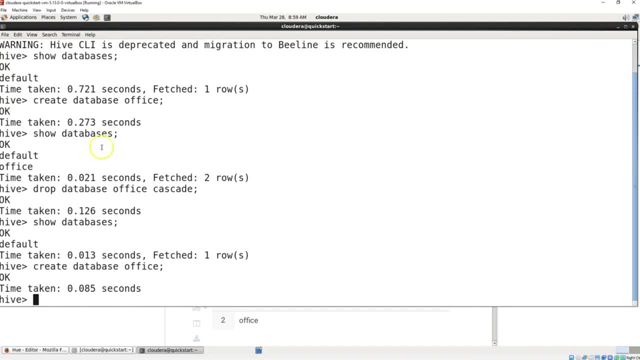 in the database and the database itself. now, if we do show database and we'll go ahead and recreate our database because we're going to use the office database for the rest of this hands-on demo, a really handy command, now set with the sql or hql. 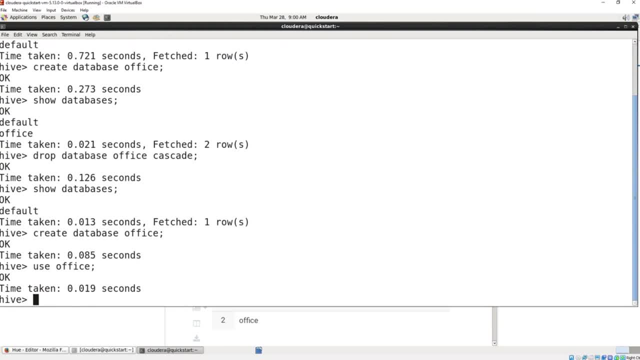 is to use office, and what that does is that sets office as the default database. so, instead of having to reference the database every time we work with a table, it now automatically assumes that's the database being used, whatever tables we're working on. the difference is you put the tedwood faculty shows that in base and predictability, accessibility data until it's every point in front database has defaulted, and so our case, in fact, is log the database with meaning and the data data afterene zehn you when we drag the table out. we've got the tool on the left side here, if you. 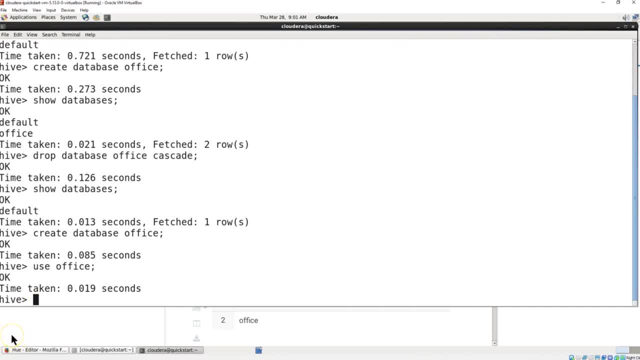 entered a page in page one and then dessert. click on it. once you hit, enter that and then select痒 first name period table, and I'll show you in just a minute what that looks like and how that's different. if we're going to have a table and a database, we should 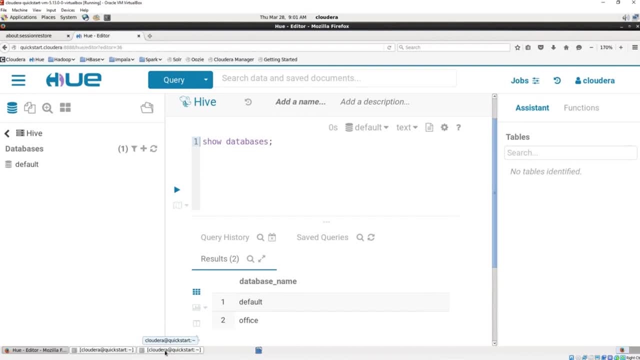 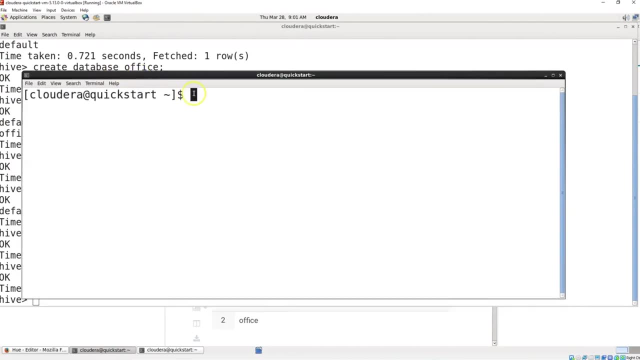 probably load some data into it. so let me go ahead and switch gears here and open up a terminal window. you can just open another terminal window and it'll open up right on top of the one that you have hive shell running in, and when we're in this terminal window first, we're gonna go ahead and just do it list. 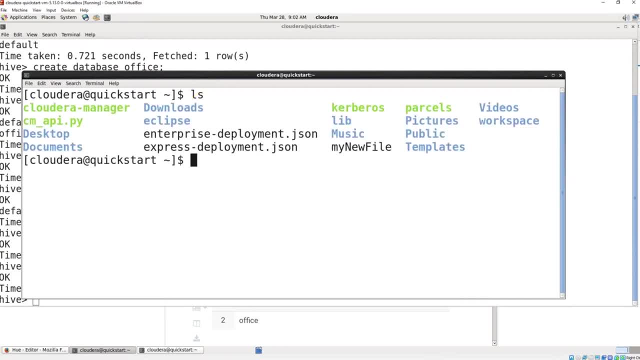 which is, of course, a Linux command. you can see all the files I have in here. this is the default load. we can change directory to documents, we can list in documents- and we're actually going to be looking at employee CSV. a Linux command is the cat. you can use this actually to combine documents. there's all kinds of 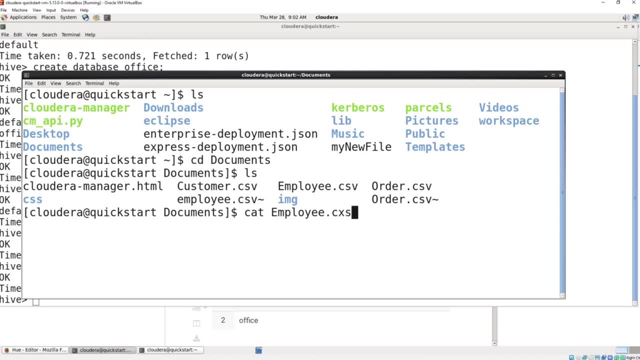 things that cat does. but if we want to just display the contents of our employee CSV file, we can simply do cat employee CSV. and when we're looking at this, we want to know a couple things. one, there's a line at the top, okay, so the very first thing we're going to want to do is we're going to want to do a. 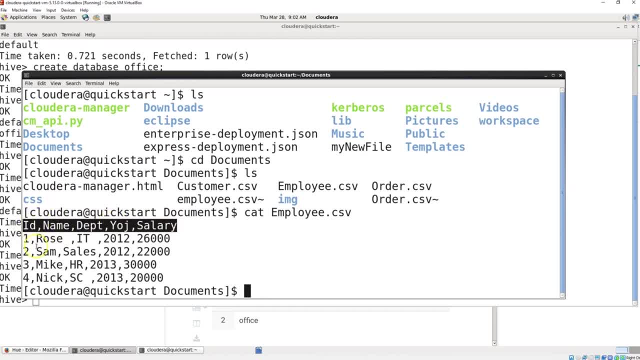 first thing we notice is that we have a header line. the next thing we notice is that the data is comma separated and in this particular case you'll see a space here. generally with these you got to be real careful with spaces. there's all kinds of things you got to watch out for because it can cause issues, these spaces. 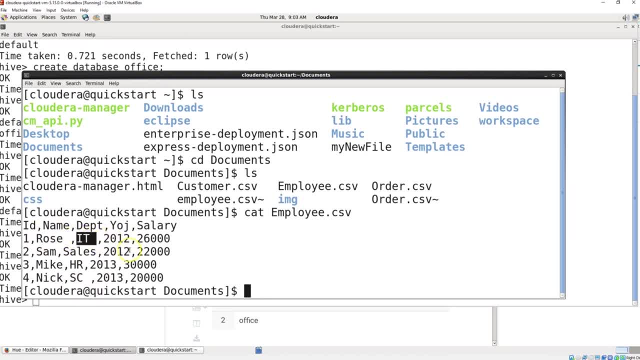 won't, because these are all strings that the space is connected to. if this was a space next to the integer, you would get a null value that comes into the database without doing something extra in there. now with most of Hadoop, that's important to know that you're writing. 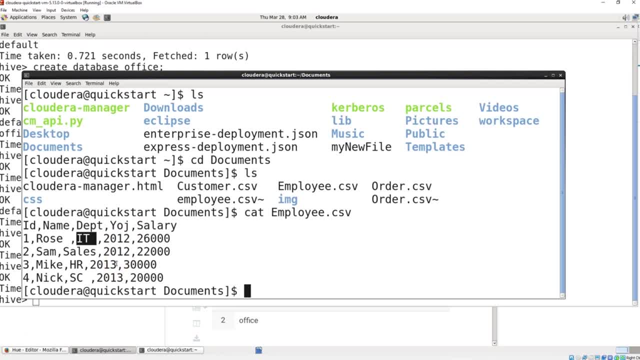 the data once reading it many times, and that's true of almost all your Hadoop things coming in. so you really want to process the data before it gets into the database. and for those who of you have studied data transformation, that's the etl, where you extract transfer form and then load the data. so you really want to. 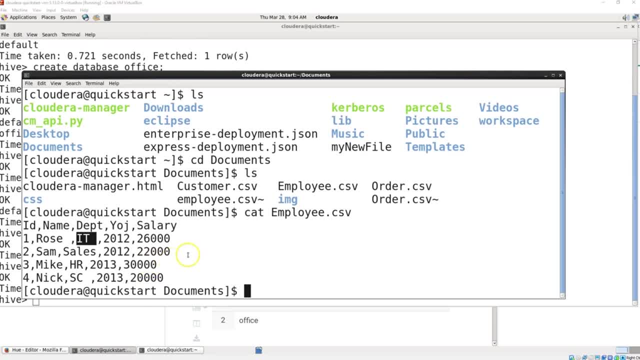 extract and transform before putting it into the hive. then you load it into the hive with the transformed data and of course, we also want to note the schema. we have an integer, string, string, integer, string, string, string, string, string, string, integer, integer. so we kept it pretty simple in here. as far as the way the 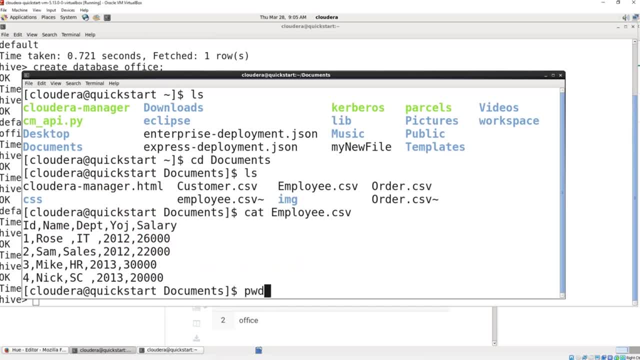 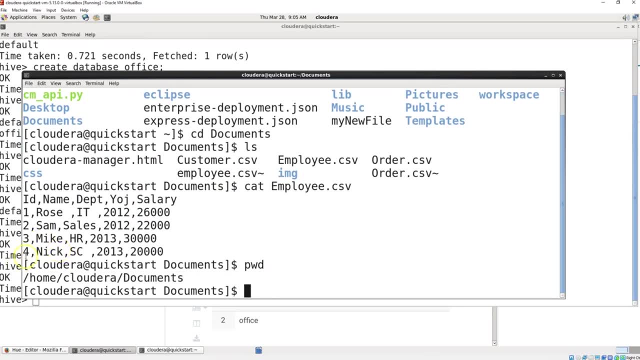 data is set up. the last thing that you're gonna want to look up when your is the source. since we're doing local uploads, we want to know what the path is. we have the whole path. in this case it's home slash, Cloudera slash documents and 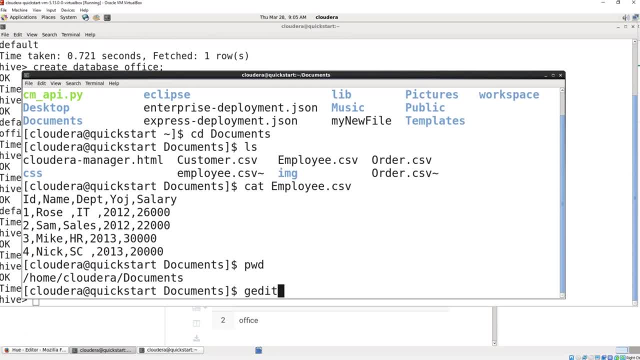 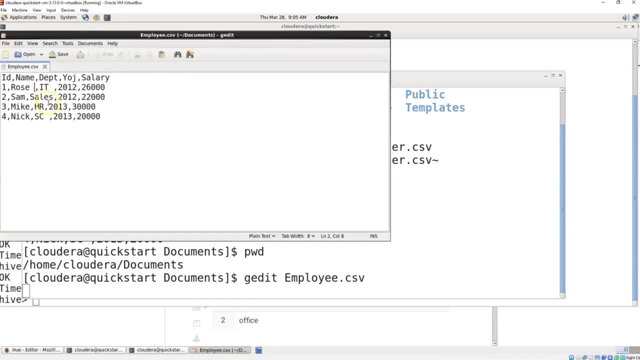 these are just text documents we're working with right now. we're not doing anything fancy, so we can do a simple get edit employee CSV and you'll see it comes up here. it's just a text document so I can easily remove these added spaces. there we go, and then we go ahead, just save it, and so now it has a new. 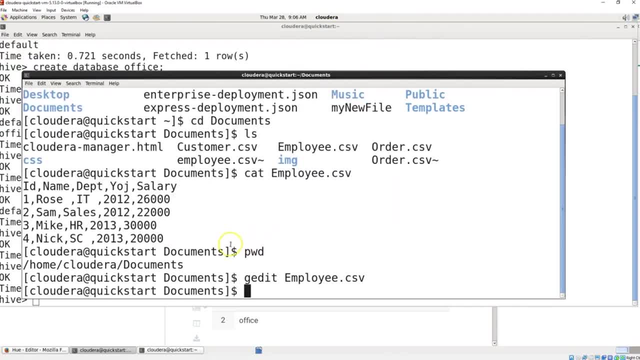 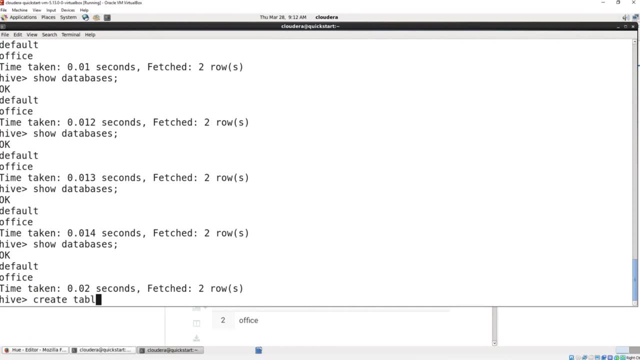 setup in there. we've edited it. the g-edit is usually one of the default that loads into Linux, so any text editor will do back to the hive shell. so let's go ahead and create a table ploy, and what I want you to note here is: I did. 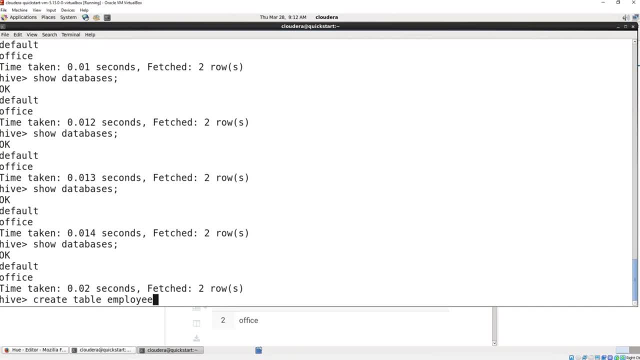 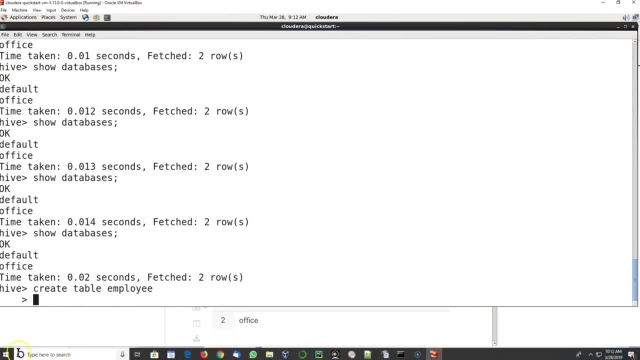 not put the semicolon on the end here. semicolon tells it to execute that line. so this is kind of nice if you're, you can actually just paste it in. if you have it written on another sheet and you can see right here where I have create, 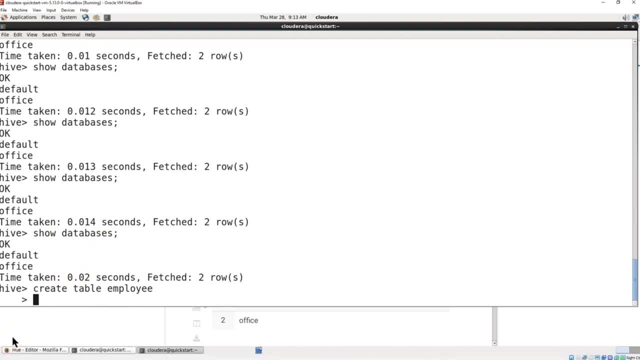 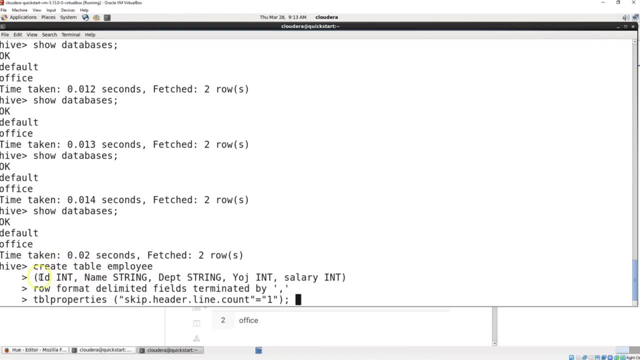 a table ploy and it goes into the next line on there, so I can do all of my commands at once now. just, I don't have any typo errors. I went ahead and just pasted the next three lines in, and the next one is our schema, if you remember. 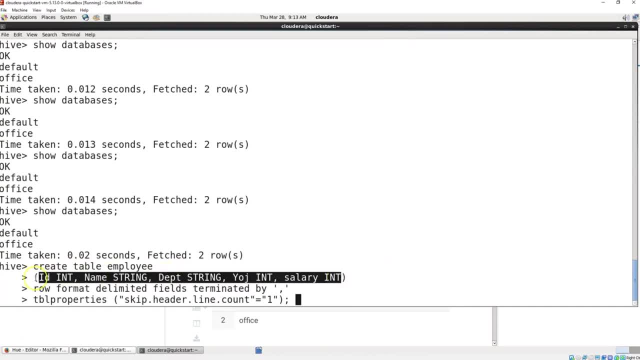 correctly from the other side. we had the different values in here, which was ID name, department, year of joining and salary, and the ID is an integer, name is a string, department string, you're joining energy, salary an integer, and they're in brackets. we put closed black brackets around them. 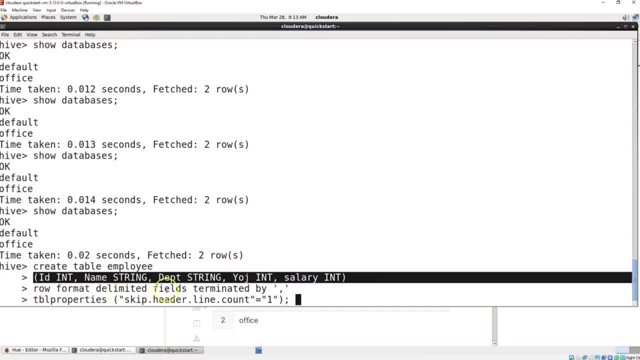 and you could do this all as one line. and then we have row format, delimited fields terminated by comma, and this is important because the default is tabs. so if I do it now, it won't find any terminated fields, so you'll get a bunch of null values loaded into your table and then, finally, our table properties. we 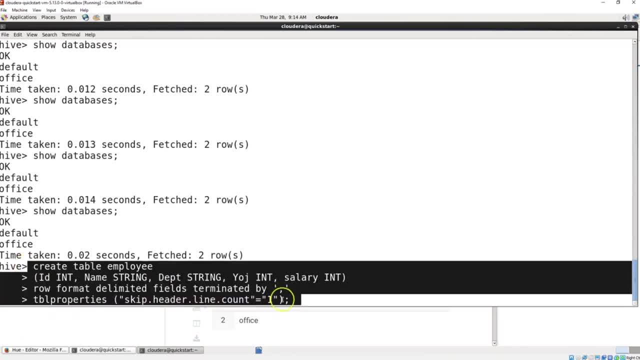 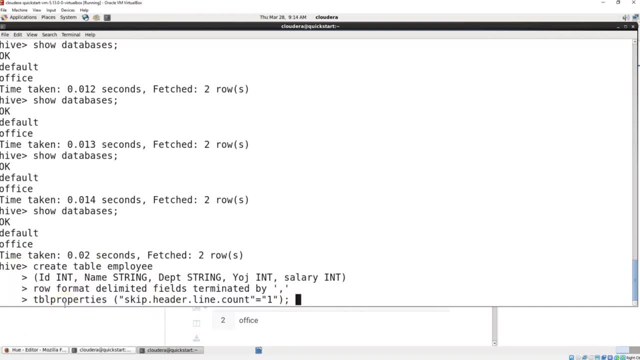 want to skip the header line. count equals one. now this is a lot of work for uploading a single file. it's kind of goofy when you're uploading a single file that you have to put all this in here. but keep in mind hive and Hadoop is designed for writing many files into the database. you write them. 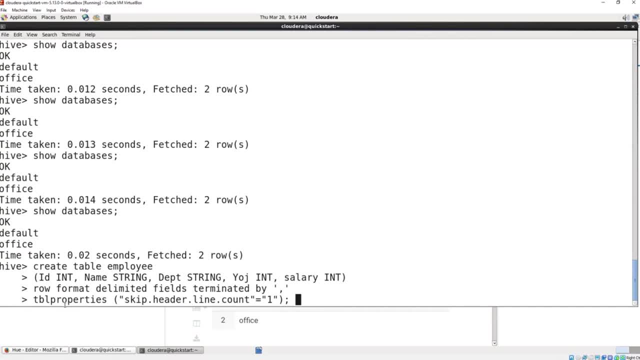 all in there and then you can. they're saved, it's an archive, it's a data warehouse, and then you're able to do all your queries on them. so a lot of times we're not looking at just the one file coming up. we're loading hundreds of. 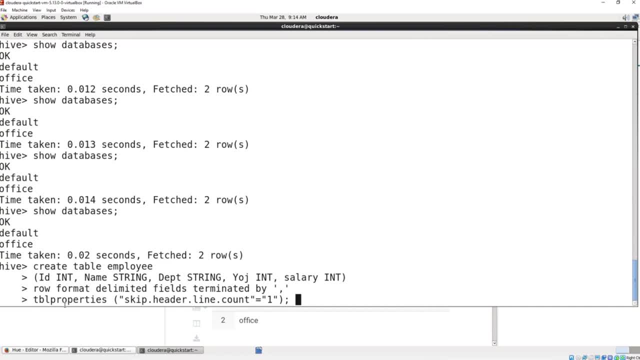 files. you have your reports coming off of your main database, all those reports are being loaded and you have your log files. you have, I mean, all this different data is being dumped into Hadoop and, in this case, hive on top of Hadoop, and so we need to let it know. hey, how do I handle this data and how do I handle it? 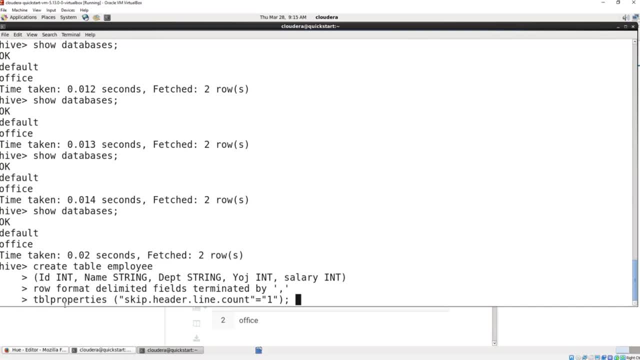 and so we need to let it know. hey, how do I handle this data and how do I handle these files coming in? and then we have the semicolon at the end which lets us know to go ahead and run this line. and so we'll go ahead and run that. and now? 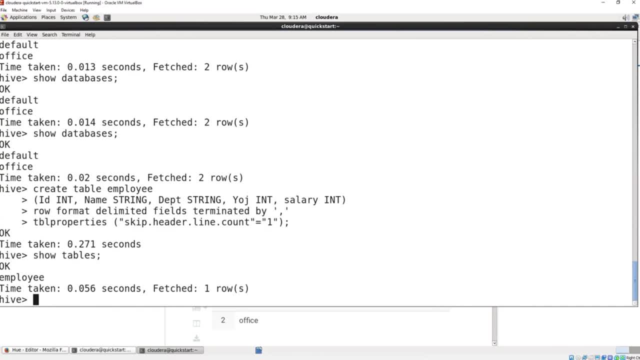 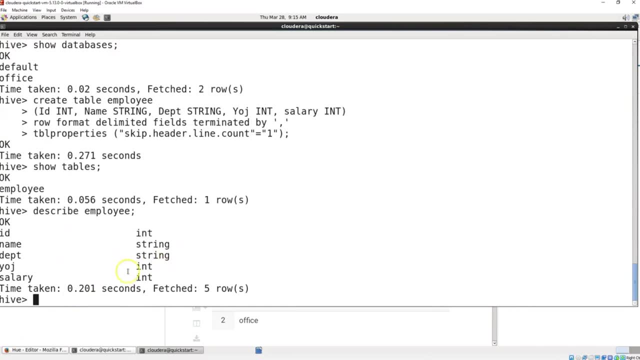 if we do a show tables, you can see there's our employee on there. we can also describe. if we do describe employee, you can see that we have our ID integer, name string, department string, year of joining- integer and salary, integer. and then finally, let's just do a select star employee. very basic SQL and HQL command. 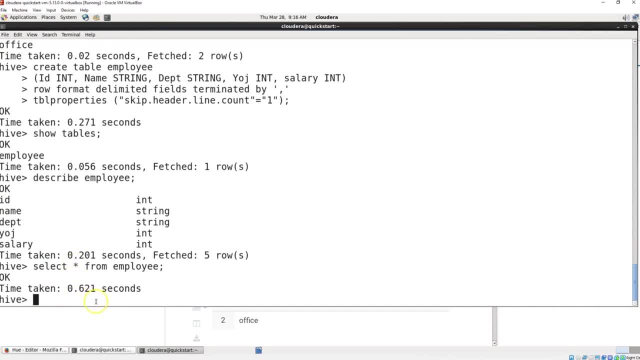 and then finally, let's just do a select star from employee- very basic SQL. and then finally, let's just do a select star- employee- very basic SQL and HQL command selecting data. it's gonna come up and we haven't put anything in it, so as we. 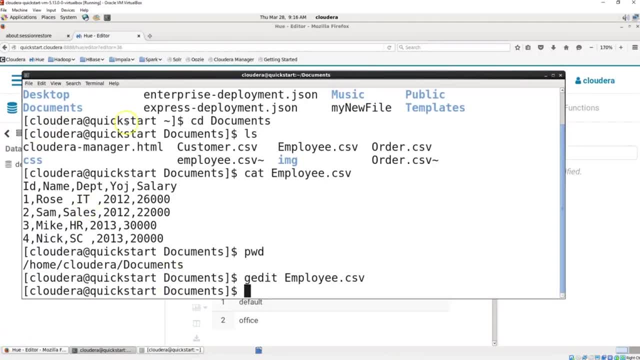 expect. there's no data in it. so if we flip back to our Linux terminal window, you can see where we did the cat employee CSV and you can see all the data we expect to come into it. and we also did our PWD and right here you see. 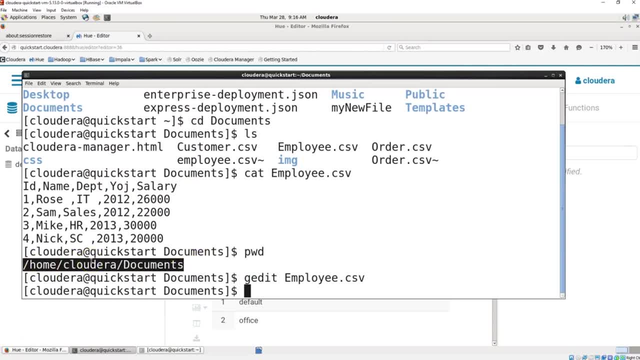 the path. you need that full path. when you are loading data, you know you can do a browse and if I did it right now with just the employee CSV as a name, it will work, work. but that is a really bad habit in general when you're loading data, because 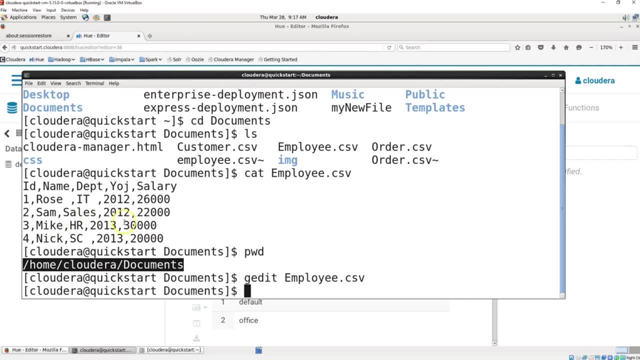 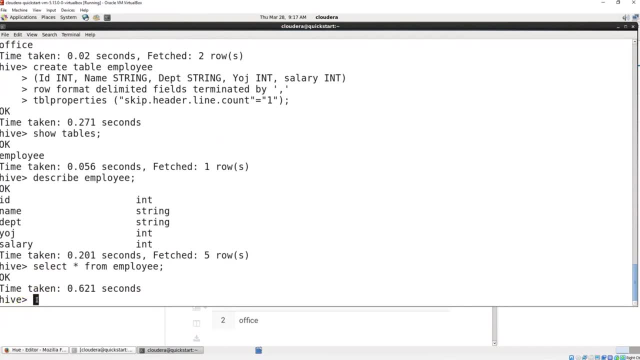 it's. you don't know what else is going on in the computer. you want to do the full path. almost in all your data loads, so let's go ahead and flip back over here to our hive shell. we're working in and the command for this is load data. so 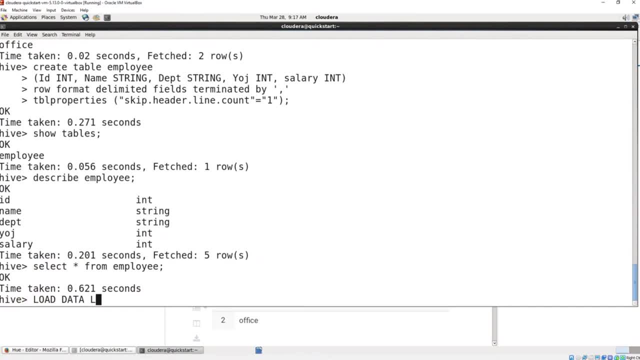 that says: hey, we're loading data, that's a hive command, HQL, and we want local data. so you got to put down local in path. so now it needs to know where the path is. now, to make this more legible, I'm just gonna go ahead and hit enter. 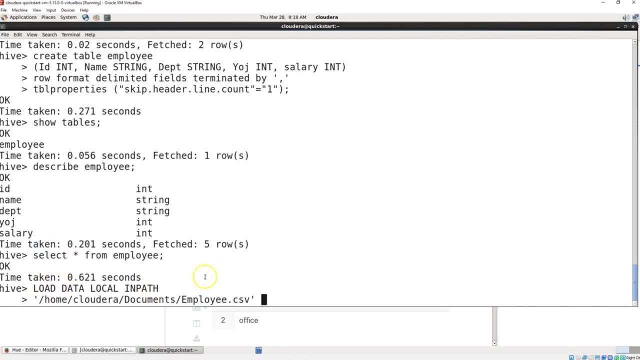 then we'll just paste the full path in there which I have stored over on the side like a good prepared demo, and you'll see, here we have home Cloudera documents- employee CSV. so it's a whole path for this text document in here and we go ahead and hit enter in there and then we have to let it know where the 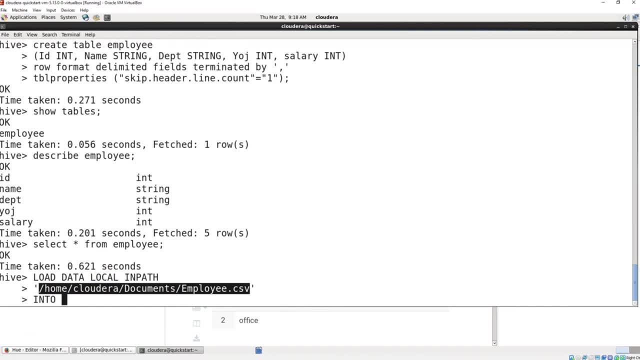 data is going. so now we have a source and we need a destination and it's gonna go into the table and we'll just call it employee. we'll just match the table in there and because I wanted to execute, we put the semicolon on the end. it goes. 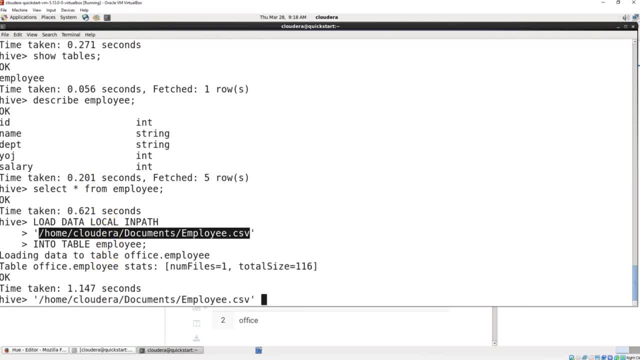 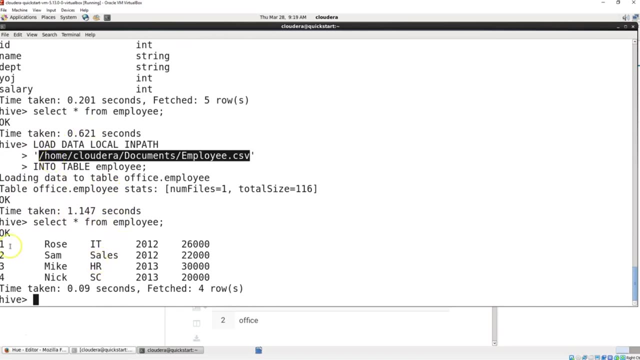 ahead and executes all three lines. now, if we go back, if you remember we did the select star from employee just using the up error to page through my different commands. I've already typed in. you can see right here we have as we expect. we have Rose, Sam, Mike and Nick and we have all their information showing in our 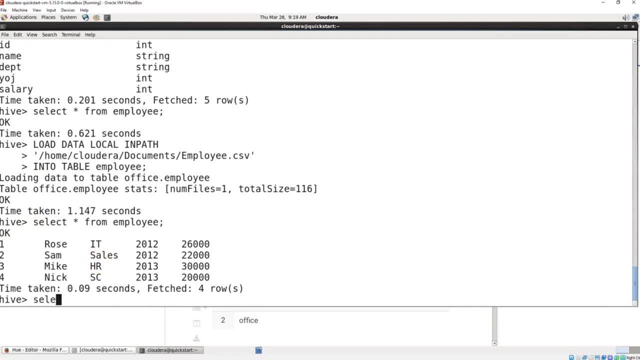 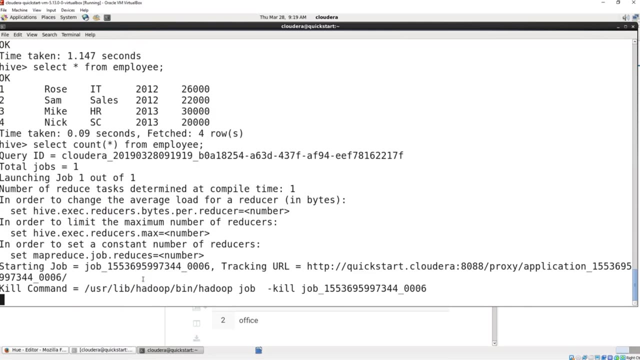 four rows and then let's go ahead and do select and count. we'll just look at a couple of these different select options you can do. we're gonna count everything from employee. now this is kind of interesting because I would say that when I'm doing the count and the 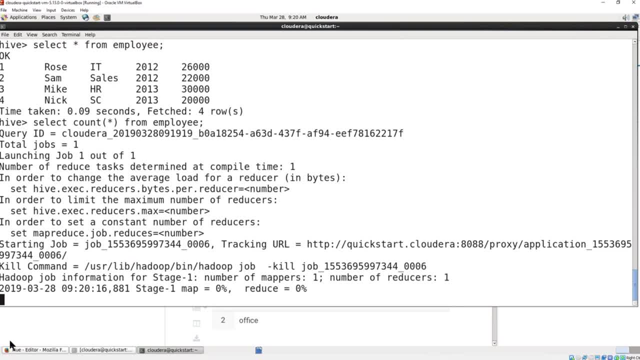 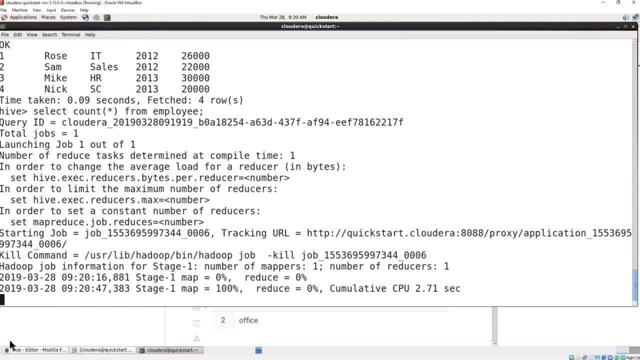 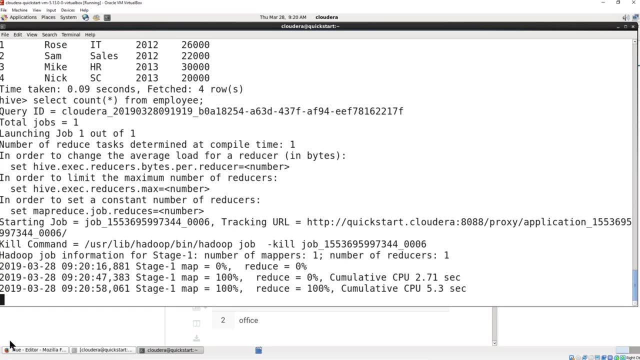 first one just pops up with a basic Select because it doesn't need to go through the full map reduce phase, but when you start doing account it does go through the full map reduce setup in the hive and Hadoop and because I'm doing when you do a single node, as I said earlier, it doesn't do any good as an 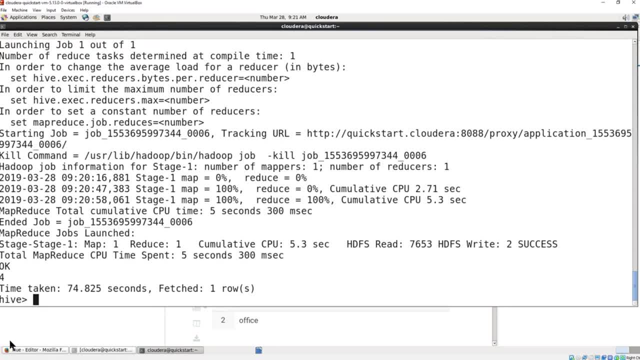 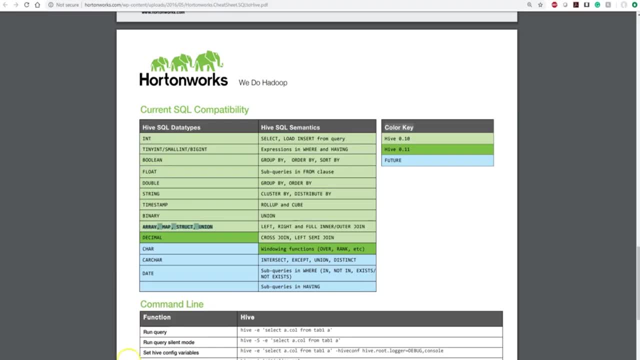 actual distribution, because you're only running it on one computer and then you've added all these different layers to run it and we see it comes up with four, and that's what we expect. we have four rows, we expect four at the end and if you remember from our cheat sheet which we brought up here from Horton's, 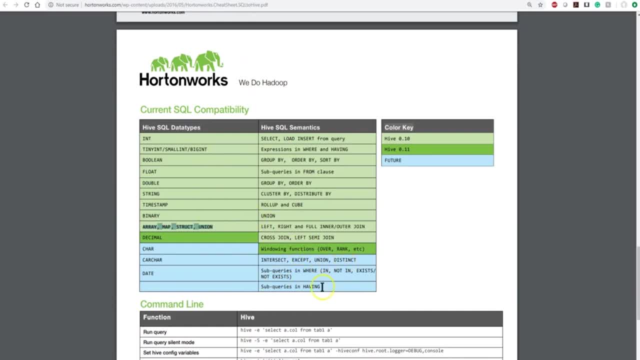 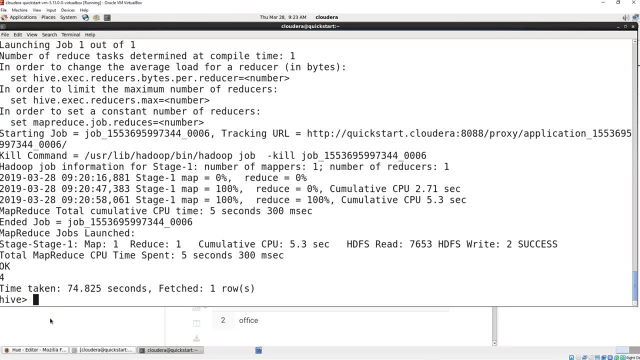 it's a pretty good one. there's all these different commands we can do. we'll look at one more command where we do the what they call sub queries right down here, because that's really common to do a lot of sub queries, and so we'll do. 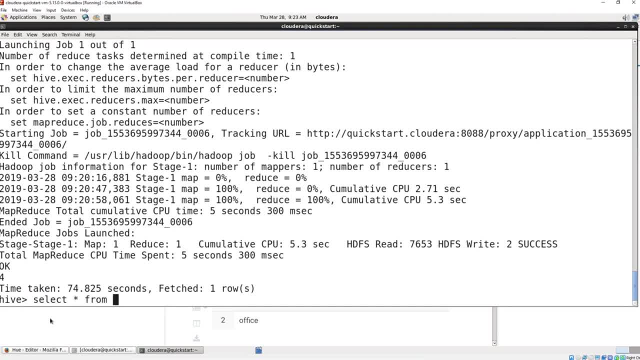 select star or all different columns from employee. now, if we weren't using the office database, it would look like this: from office dot- employee, and either one will work on this particular one because we have office set as a default on there. so, from office employee, and then the command where creates a subset. 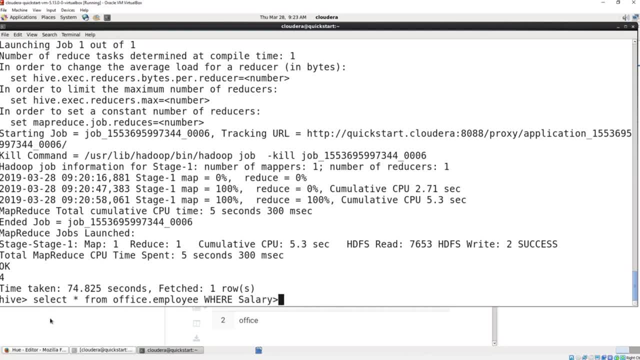 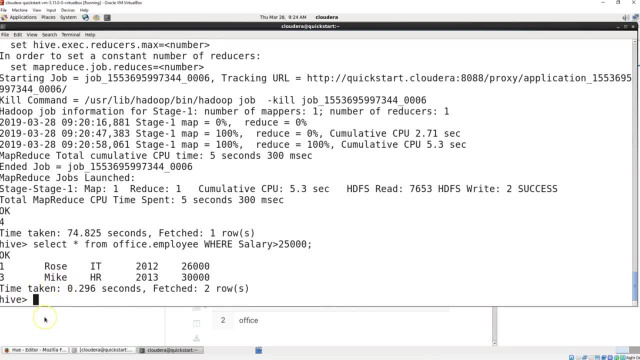 we run this query. you can see it pops up and there's our salaries of people, top earners. we have rows and IT and Mike and HR kudos to them. of course they're fictitional. I don't actually. we don't actually have a rose and a mic in those. 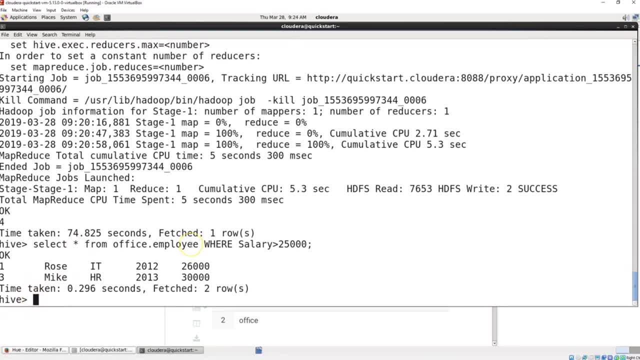 positions, or maybe we do so. finally, we want to go ahead and do is we're done with this table now. remember, you're dealing with a data warehouse, so usually don't do a lot of dropping of tables and databases, but we're gonna go ahead and drop this table here before we drop it. one more quick note is we can change it. 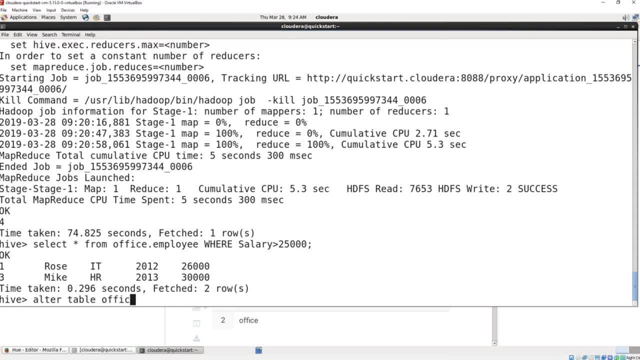 so what we're going to do is we're going to alter table office employee and we want to go ahead and rename it. there's some other commands you can do in here, but rename is pretty common and we're gonna rename it to. it's gonna stay in. 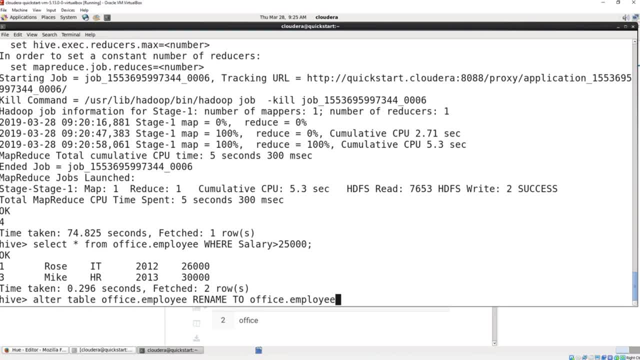 office and turns out one of our shareholders really doesn't like the word employee. he wants employees plural. it's a big deal to him, so let's go ahead and change that name for the table. it's that easy, cuz it's just changing the meta data on there. and now, if we do, 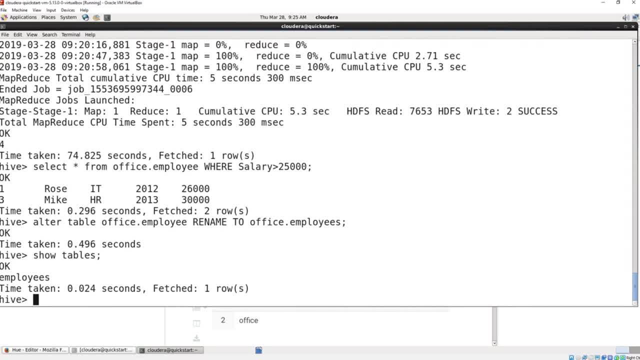 show tables, you'll see we now have employees, not employee. and then at this point maybe we're doing some house cleaning because this is all practice, so we're gonna go ahead and drop table and we'll drop table employees because we changed the name in there. so if we did employee, just give us an error. and now 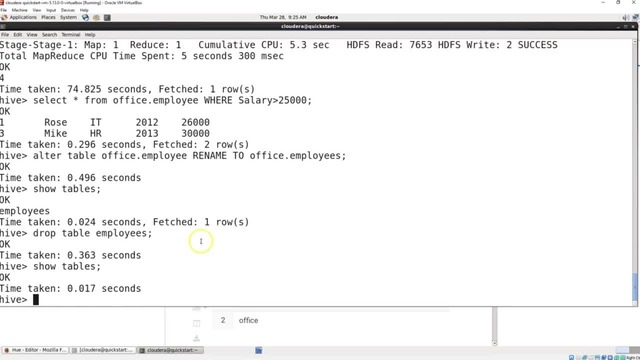 if we do show tables, you'll see all the tables are gone. now the next thing we want to go and take a look at- and we're gonna walk back through the loading of data just real quick, because we're gonna load two tables in here and let me just float back to our terminal window so we 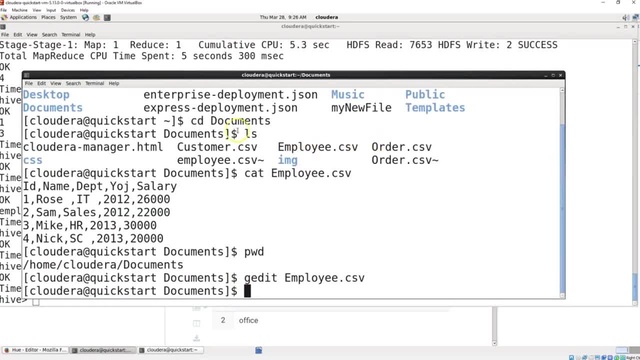 can see what those tables are that were loading and so up here. we have customer, we have a customer file and we have an order file. we want to go ahead and put the customers and the orders in to here. so those the two we're doing and of 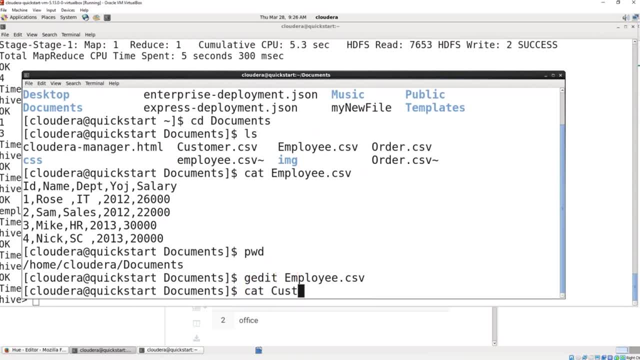 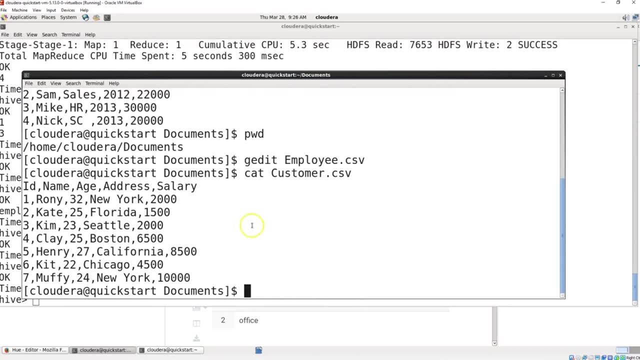 course it's always nice to see what you're working with, so let's do our cat customer CSV. we can always do g edit, but we don't really need to edit these. we just want to take a look at the data in customer, and important in here is again: 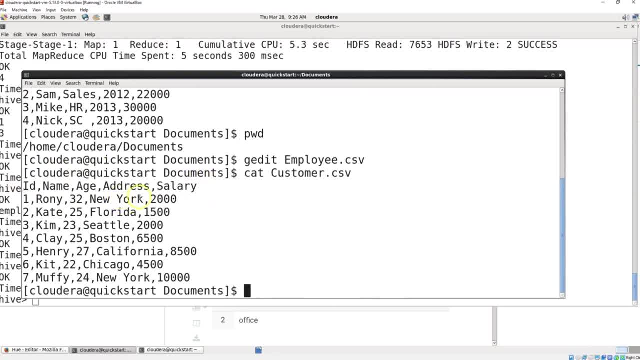 we have a header, so we have to skip a line, comma separated. nothing odd with the data. we have our schema which is integer, string, integer, string, integer. so you know you'd want to take that, note that down or flip back and forth when you're doing it. and then let's go ahead and do cat order dot CSV and we can see. 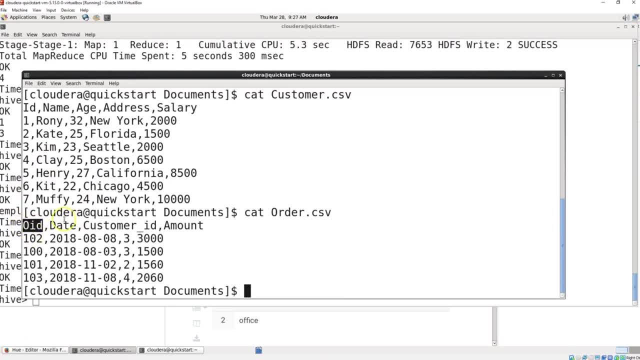 we have o ID, which I'm guessing is the order ID. we have a date up something new. we've done integers and strings, but we haven't done date. when you're importing new and you never worked with the date, dates always one of the more trickier. 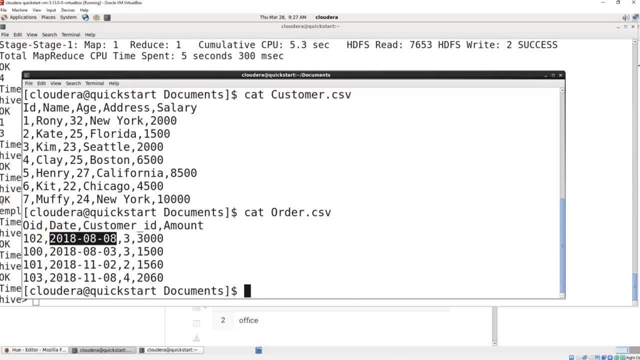 fields to port in, when that's true of just about any scripting language I've worked with. all of them have their own idea of how dates supposed to be formatted, what the default is, this particular format or its year, and it has all four digits. dash month, two digits dash day is the standard import for the 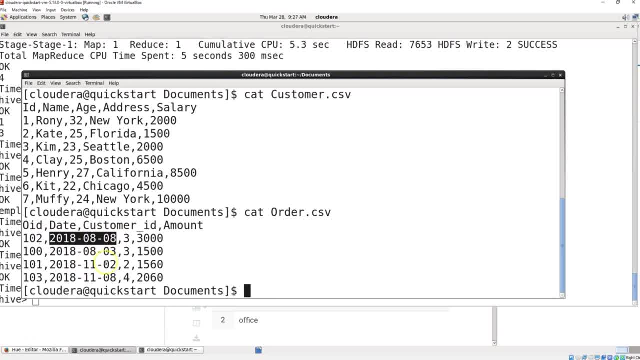 hive. so if you'll have to look up and see what the different formats are, if you're gonna do a different format in there coming in or you're not able to pre-process the data, but this would be a pre-processing of the data thing coming in, if you remember correctly from our adult, which is II. just in case you. 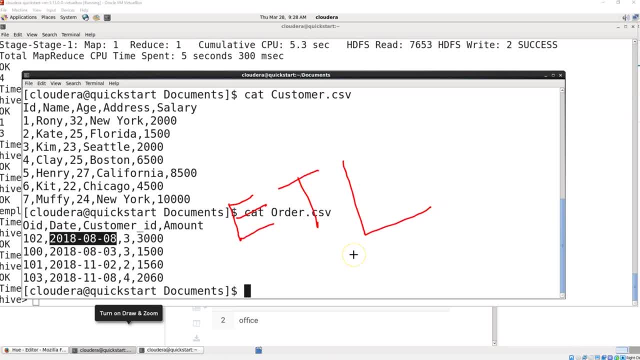 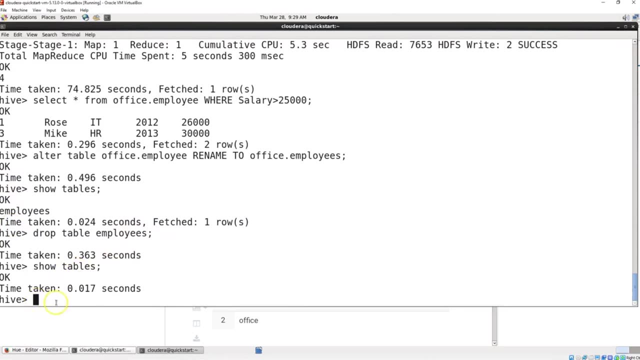 weren't able to hear me last time. ETL, which stands for extract, transform, then load. so you want to make sure you transforming this data before it gets into here, and so we're gonna go ahead and bring both his data in here and really we're doing this so we can show you the basic join there is, if you. 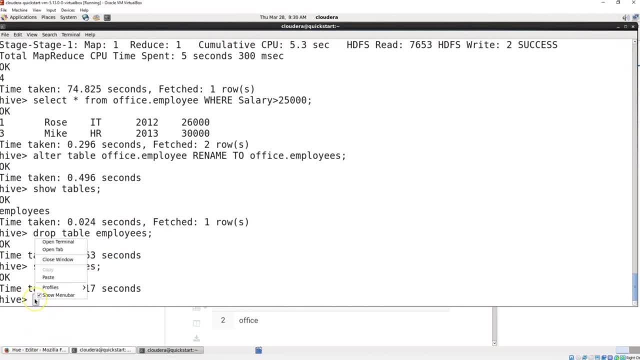 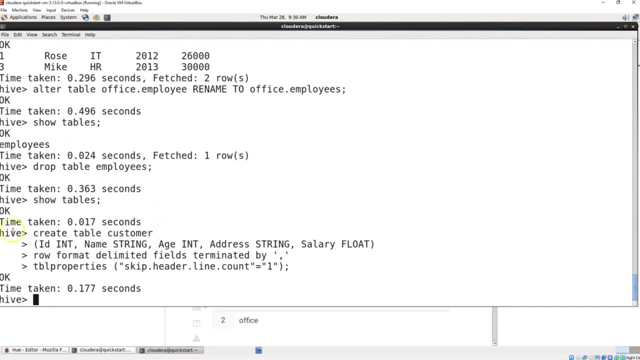 remember from our setup: merge, join- all kinds of different things you can do, and but joining different data sets is so common, so it's really important to know how to do this. we need to go ahead and bring in these two data sets and you can see where I just created a table, customer. here's our schema: the integer. 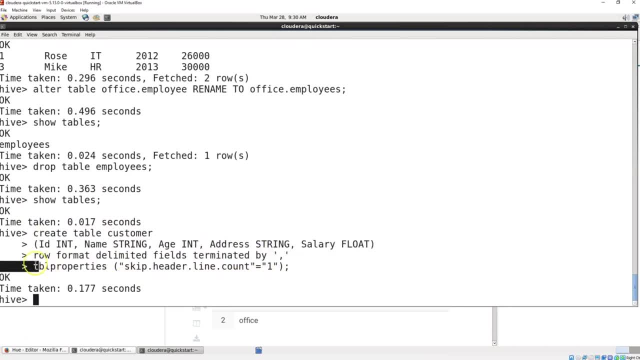 name, age, address, salary. here's our, delimited by commas, and our table properties where we skip a line. well, let's go ahead and load the data first, and then we'll do that with our order, and let's go ahead and put that in here, and I've got it split into three lines so you can see it easily. we got load. 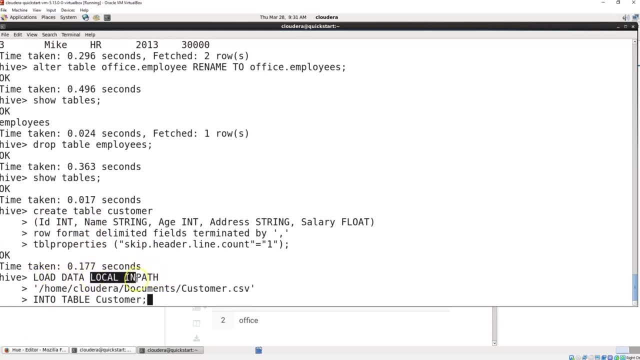 data local in path. so we know we're loading data, we know it's local and we have the path. here's the complete path for oops. this is supposed to be order CSV. grab the wrong one. of course it's gonna give me errors because you can't recreate the same table on there. and here we go. 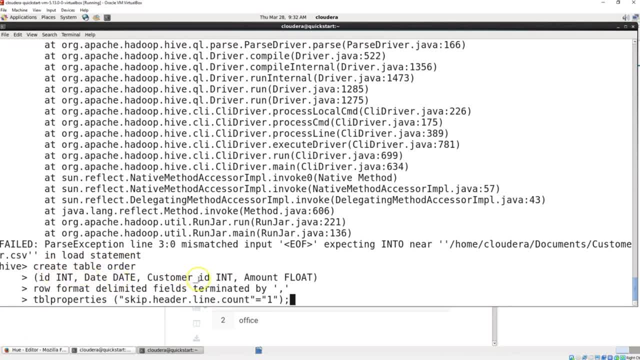 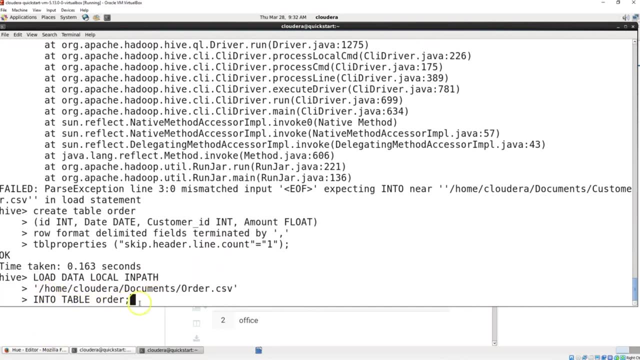 create table. here's our integer date customer, the basic setup that we had coming in here for our schema: row format, commas, table properties. skip header line and then finally, let's load the data into our order table. load data local in path home cloud air order CSV into table order. now, if we did everything right, we should be able. 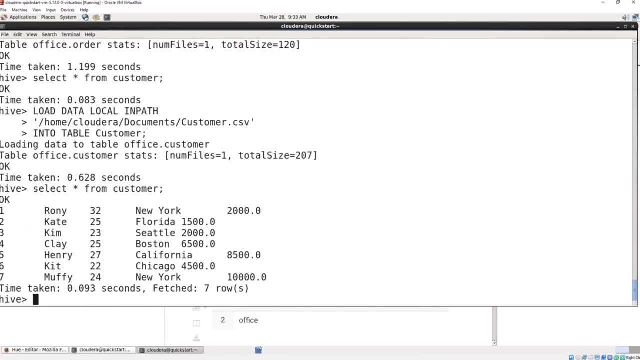 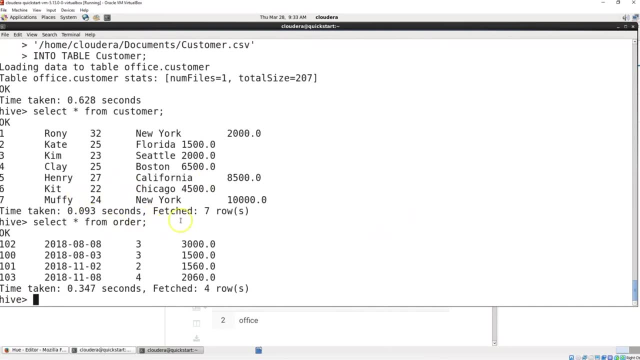 to do select star from customer and you can see we have all seven customers. and then we can do select star from order and we have four orders. so this is just like a quick frame. we have a lot of times when you have your customer databases in business you have thousands of customers from years and years and 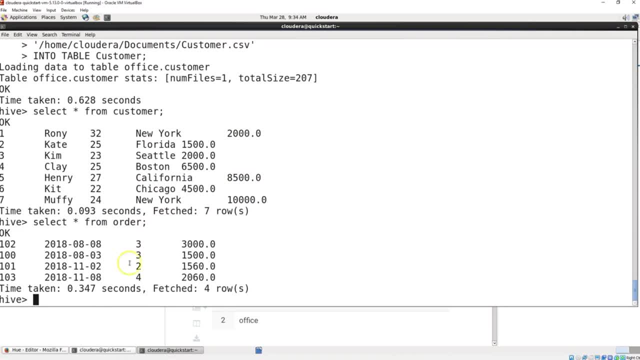 some of them, you know, they move, they close their business, they change names- all kinds of things happen. so we want to do is we want to go ahead and find just the information connected to these orders and who's connected to them. so let's go ahead and do. it's a. 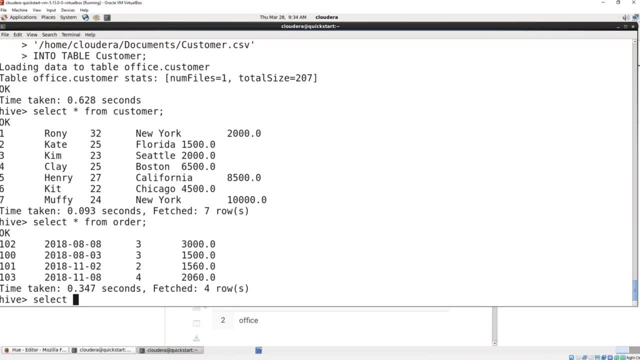 select because we're going to display information. so select and this is kind of interesting. we're going to do cid and I'm going to define C as customers, a customer table. in just a minute we're going to see dot name. again we're going to define the C, C dot age. so this means from the customer, we want to know their. 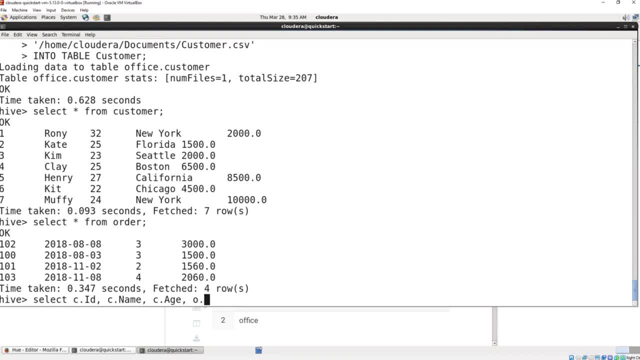 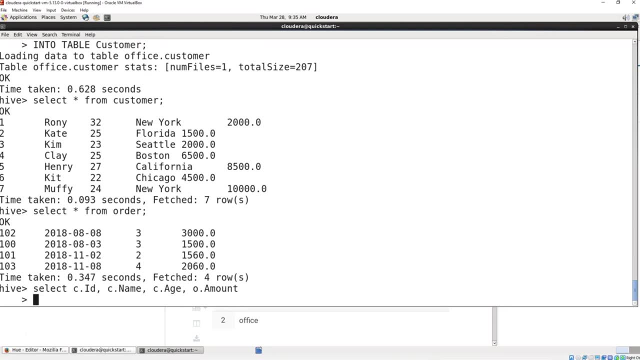 ID, their name, their age, And then you know. I'd also like to know the order amount, So let's do O for dot amount. And then this is where we need to go ahead and define what we're doing, And I'll go ahead and capitalize from customer. 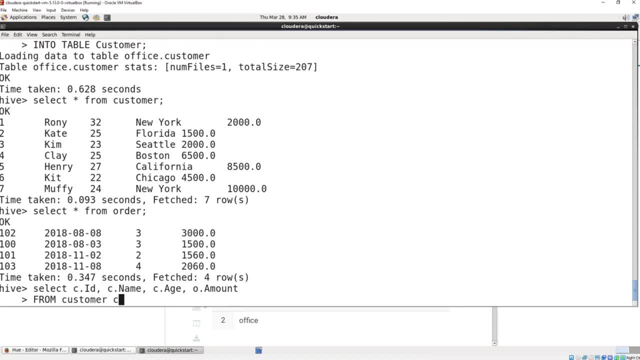 So we're going to take the customer table in here and we're going to name it C. That's where the C comes from. So that's the customer table C, and we want to join order as O. That's where our O comes from. 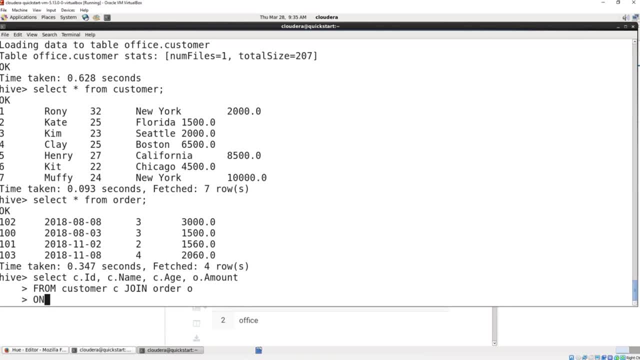 So the O dot amount is what we're joining in there And then we want to do this on. We've got to tell it how to connect the two tables. C dot ID equals O dot- customer underscore ID. So now we know how they're joined. 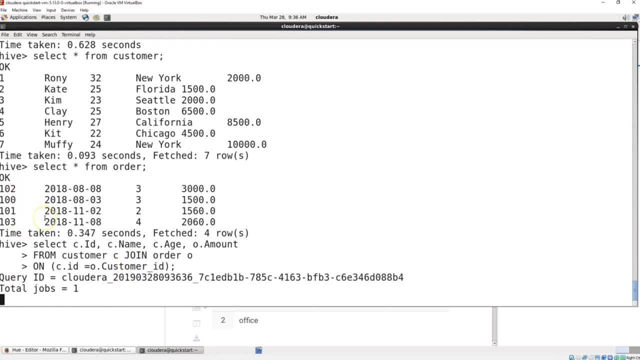 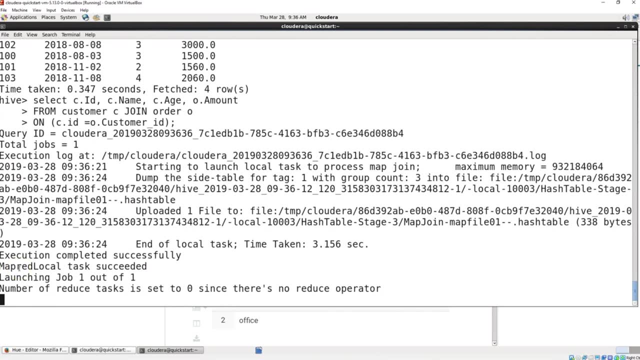 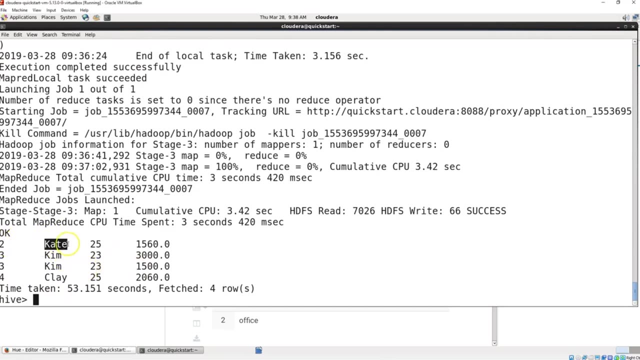 And now remember, we have seven customers in here, We have four orders And, as it processes, we should get a return of four different names joined together. And they're joined based on, of course, the orders on there And once we're done, we now have the order number, the person who made the order. 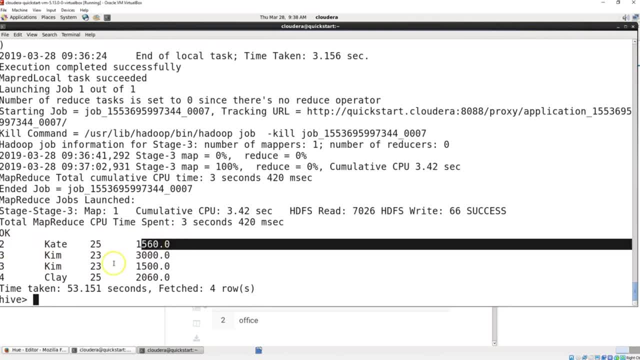 their age and the amount of the order which came from the order table. So you have your different information And you can see how the join works here. Very common use of tables and HQL and SQL. And let's do one more thing with our database. 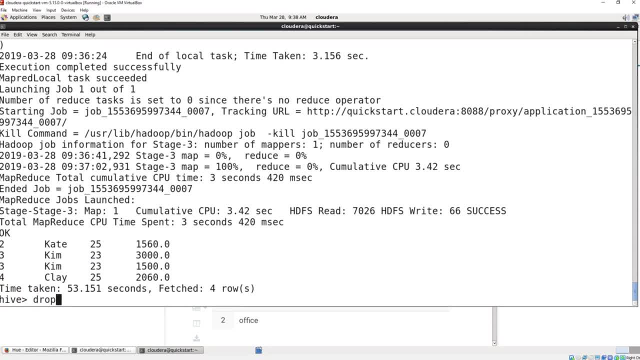 And then I'll show you a couple other Hive commands And let's go ahead and do a drop And we're going to drop database office And if you're looking at this and you remember from earlier, this will give me an error. 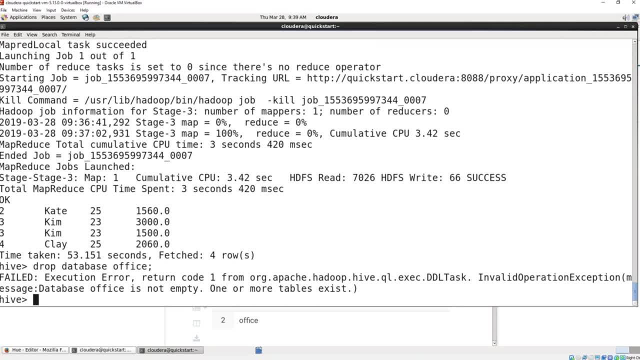 And let's just see what that looks like. It says: failed to execute exception. One or more tables exist. So if you remember from before, you can't just drop a database unless you tell it to cascade. That lets it know. I don't care how many tables are in it. 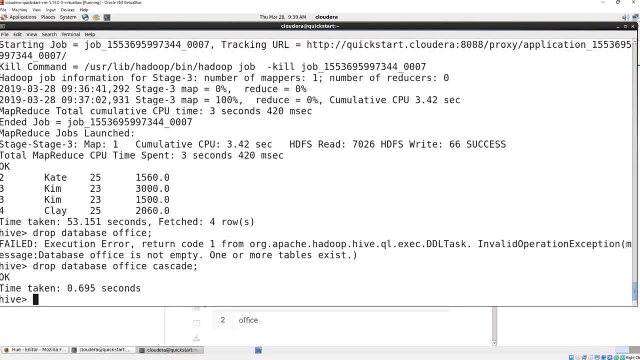 Let's get rid of it. And in Hadoop, since it's a warehouse, a data warehouse, you usually don't do a lot of dropping. Maybe at the beginning, when you're developing the schemas and you realize you messed up, you might drop some stuff. 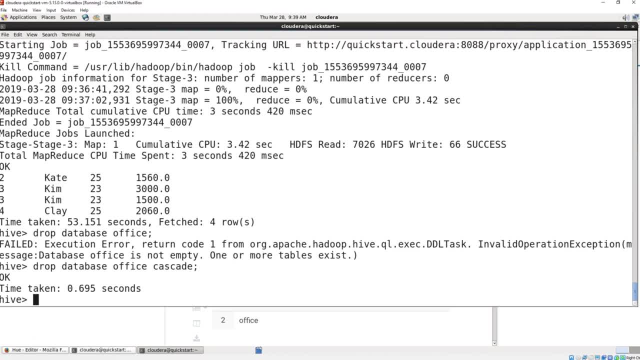 But down the road you're really just adding commodity machines to take up so you can store more stuff on it. So you usually don't do a lot of database dropping And some other fun commands. to know is that you know if you're going to do a drop, you're going to drop a lot of things. And some other fun commands to know is that you know if you're going to do a drop, you're going to drop a lot of things. And some other fun commands to know is that you know if you're going to do a drop, you're going to drop a lot of things. 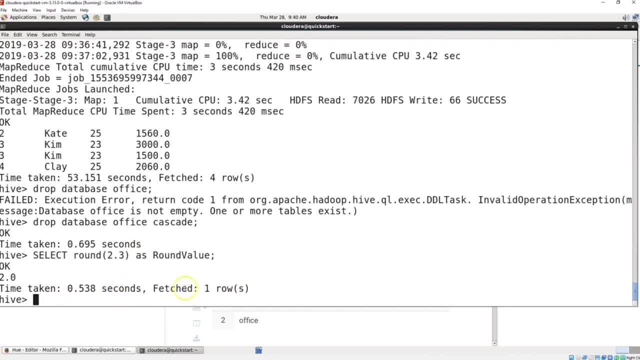 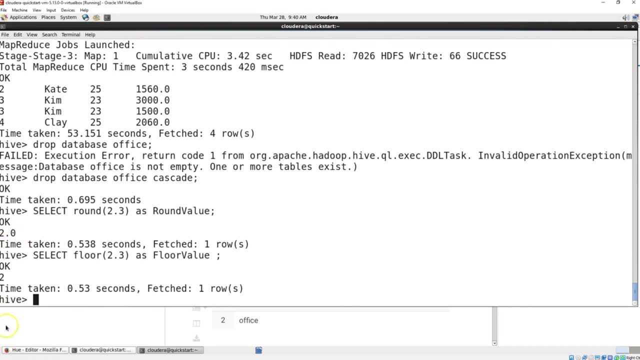 Select round. 2.3 is round value. You can do a round off in Hive. We can do as floor value, which is going to give us a 2.. So it turns it into an integer versus a float. It goes down, you know, basically truncates it. 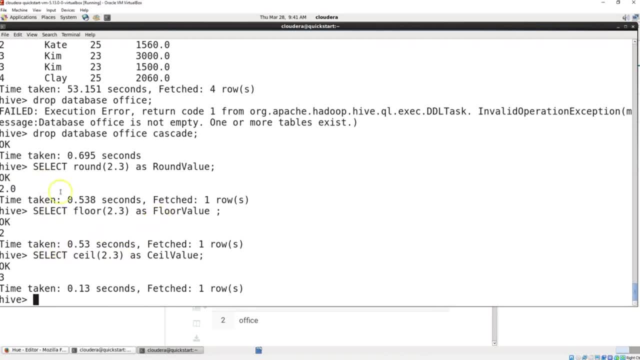 But it goes down and we can also do ceiling, which is going to round it up. So we're looking for the next integer. above There's a few commands we didn't show in here because we're on a single node. It's, as an admin, to help speedy the process. 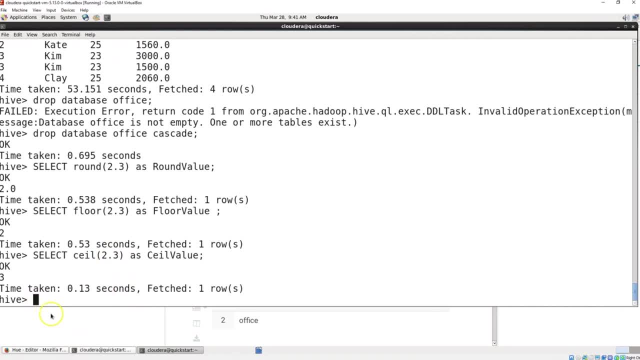 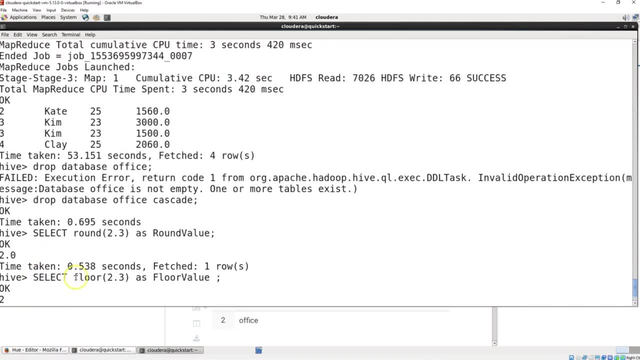 It's as an admin, to help speedy the process. you usually add in partitions for the data and buckets. You can't do that on a single node because when you add a partition, it partitions it across separate nodes. But beyond that you can see that it's very straightforward. 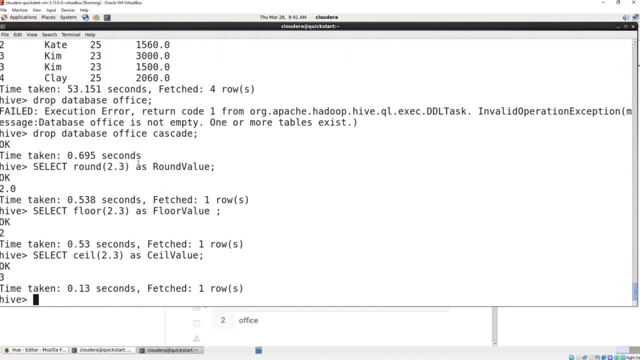 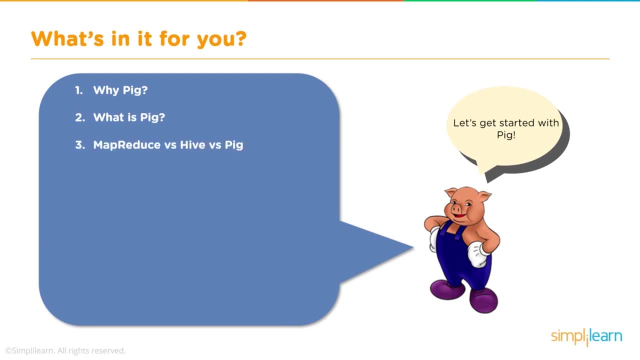 We have SQL coming in and all your basic queries that are in SQL are very similar to HQL. Let's get started with PIG. Why PIG? What is PIG? MapReduce versus Hive versus PIG. Hopefully you've had a chance to do our Hive tutorial. 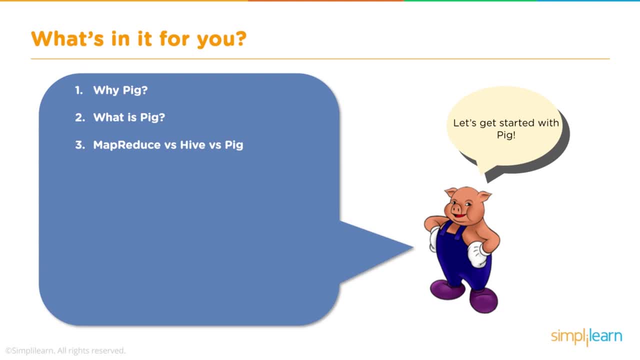 and our MapReduce tutorial. If you haven't, send a note over to SimplyLearn and we'll follow up with a link to you. We'll look at PIG architecture, working of PIG, PIG- Latin data model, PIG execution modes, a use case, Twitter and features of PIG. 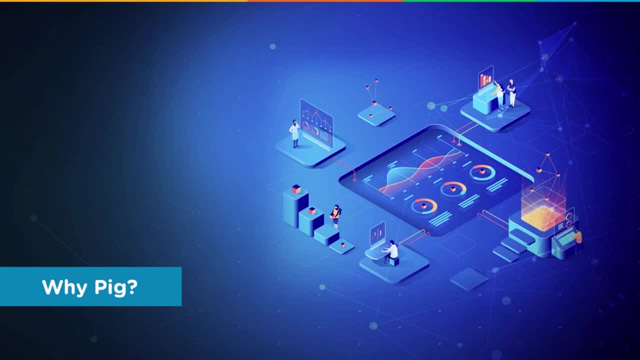 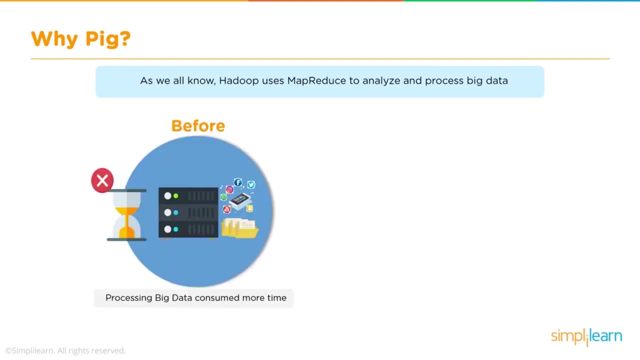 And then we'll tag on a short demo so you can see PIG in action. So why PIG? As we all know, Hadoop uses MapReduce to analyze and process big data. Processing big data consumed more time, So before we had the Hadoop system, 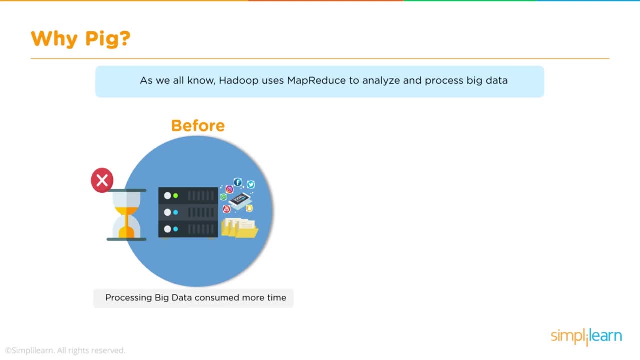 they'd have to spend a lot of money on a huge set of computers and enterprise machines. So we introduced the Hadoop MapReduce, And so afterwards, processing big data was faster using MapReduce. Then what is the problem with MapReduce? 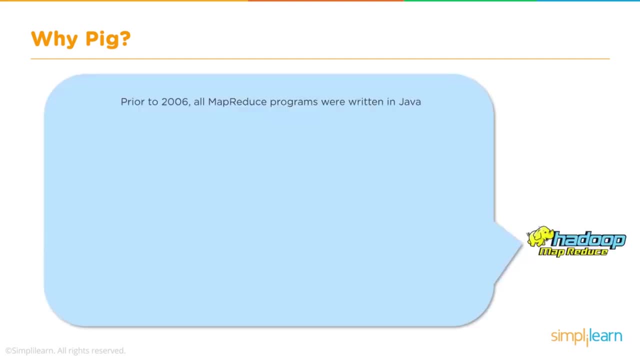 Prior to 2006,, all MapReduce programs were written in Java. Non-programmers found it difficult to write lengthy Java codes. They faced issues in incorporating MapSortReduce to fundamentals of MapReduce while creating a program. You can see here MapPhase, Shuffle and SortReducePhase. 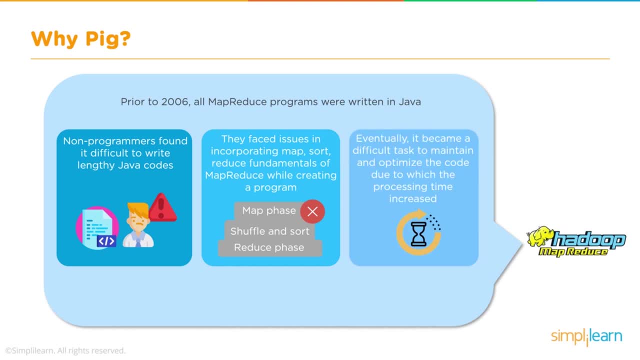 Eventually, it became a difficult task to maintain and optimize a code, due to which the processing time increased. You can imagine a manager trying to go in there and needing a simple query to find out data, and he has to go talk to the programmers anytime he wants anything. 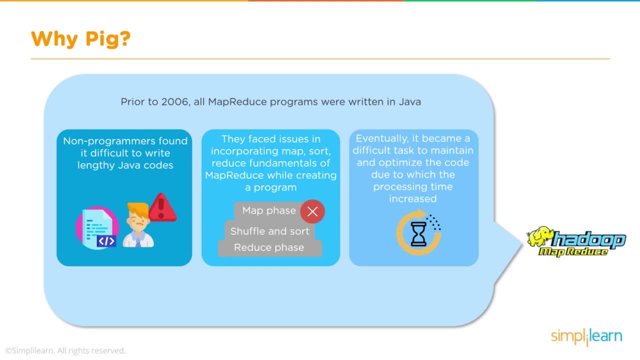 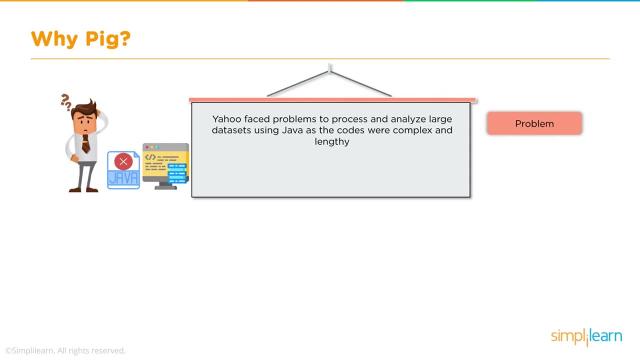 So that was a big problem. Not everybody wants to have a on-call programmer for every manager on their team. Yahoo faced problems to process and analyze large datasets using Java, as the codes were complex and lengthy. There was a necessity to develop an easier way to analyze large datasets without using 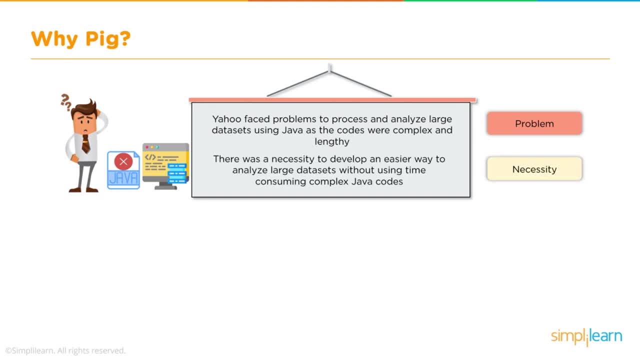 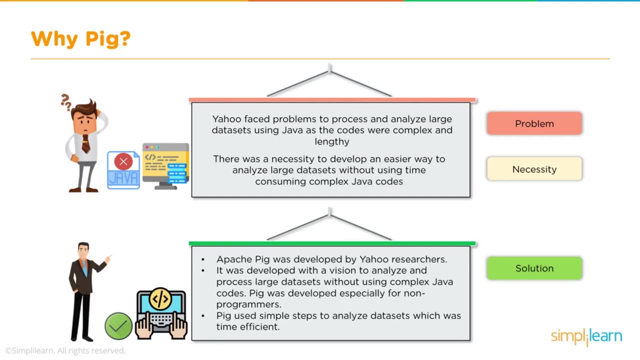 time-consuming, complex Java modes And codes and scripts and all that fun stuff. Apache Pig was developed by Yahoo. It was developed with the vision to analyze and process large datasets without using complex Java codes. Pig was developed especially for non-programmers. Pig used simple steps to analyze datasets, which was time efficient. 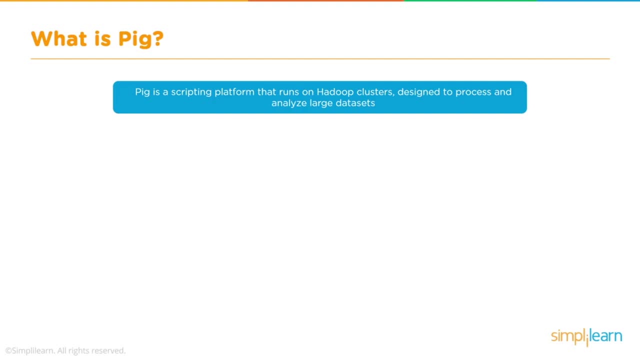 So what exactly is Pig? Pig is a scripting platform that runs on Hadoop clusters, designed to process and analyze large datasets. And so you have your Pig, which uses SQL-like queries- They're definitely not SQL, but some of them resemble SQL queries- And then we use that to analyze our data. 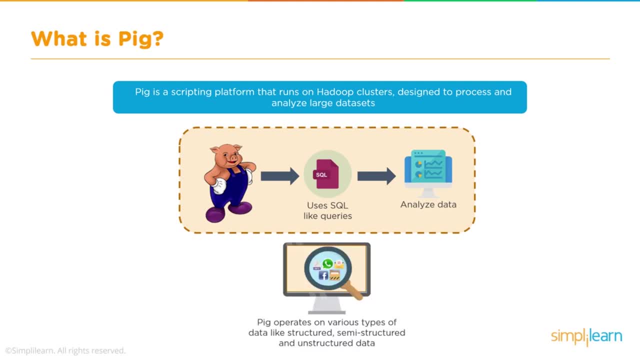 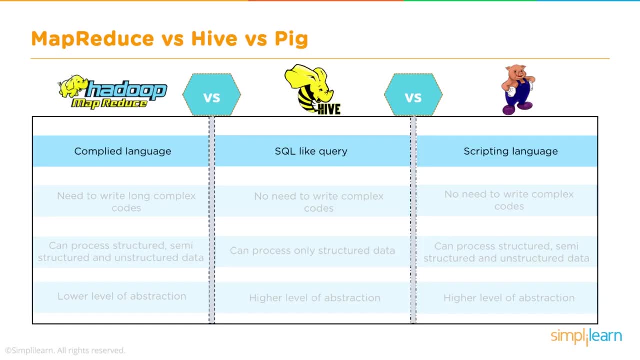 Pig operates on various types of data, like structured, semi-structured and unstructured data. Let's take a closer look at MapReduce versus Hive versus Pig. So we start with a compiled language, your MapReduce, And we have Hive, Which is your SQL-like query. 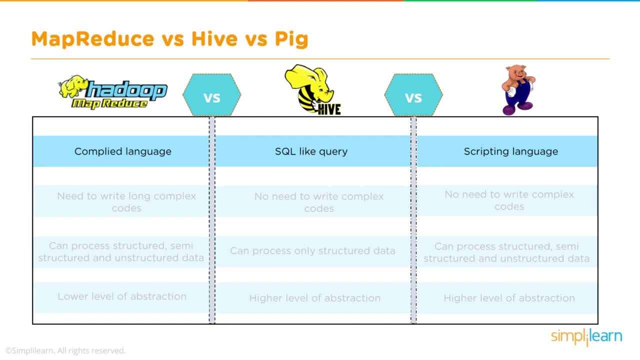 And then we have Pig, which is a scripting language. It has some similarities to SQL, but it has a lot of its own stuff. Remember, SQL-like query, which is what Hive is based off, looks for structured data, And so when we get into scripting languages like Pig now we're dealing more with semi-structured 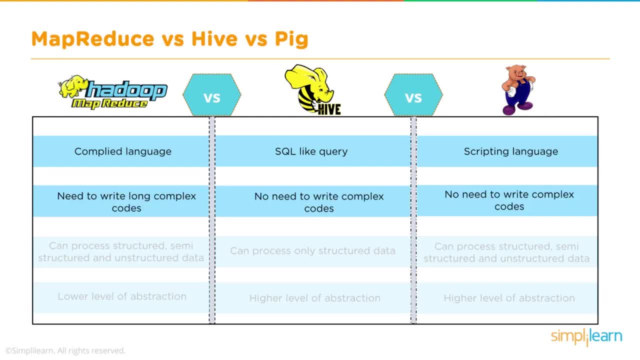 and even unstructured data. With a Hadoop MapReduce, we have a need to write long, complex codes. With Hive, no need to write complex codes. You can just put it in a simple SQL query or HQL, HiveQL, And in Pig, no need to write complex codes as we have Pig Latin. 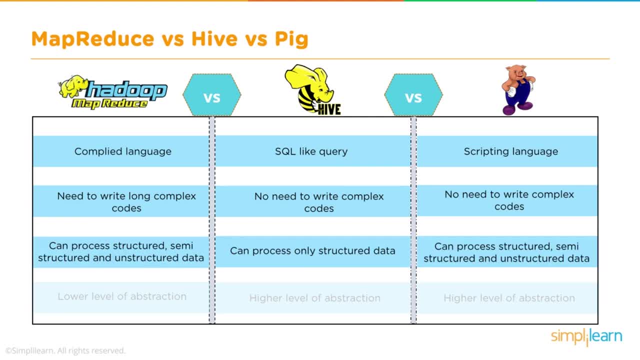 Now, remember, in the MapReduce, it can produce structured, semi-structured and unstructured data And, as I mentioned before, Hive can process only structured data. Think rows and Columns, Where Pig can process structured, semi-structured and unstructured data. 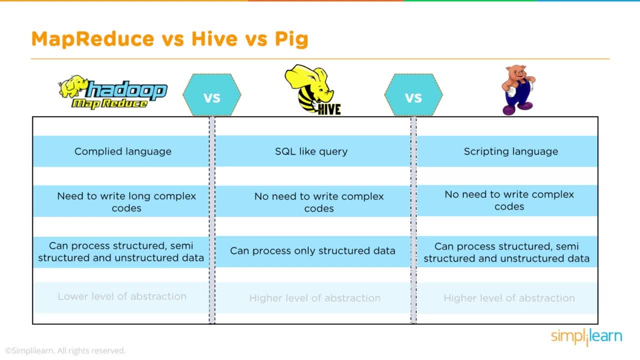 You can think of structured data as rows and columns, semi-structured as your HTML XML documents that you have on your web pages, and unstructured could be anything from groups of documents in written format, Twitter Tweets. any of those things come in as very unstructured. 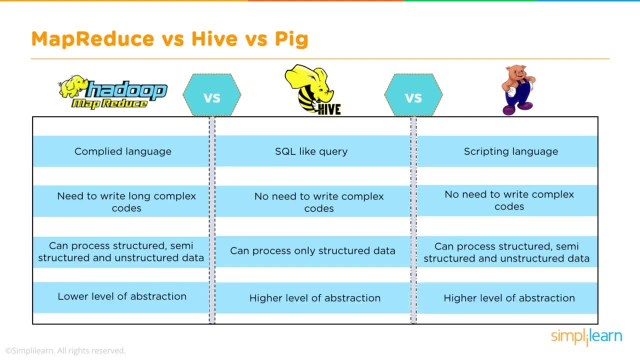 data And with our Hadoop MapReduce we have a lower level of abstraction. With both Hive and Pig we have a higher level of abstraction, So it's much more easy for someone to use without having to dive in deep and write a. 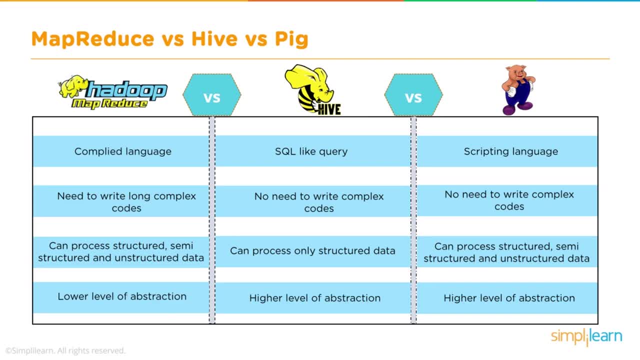 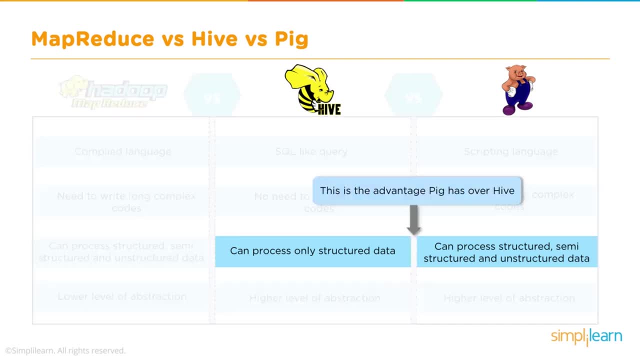 very lengthy MapReduce code And those Map and Reduce codes can take 70, 80 lines of code when you can do the same thing in one or two lines with Hive or Pig. This is the advantage Pig has over Hive. I hope you enjoyed this video. 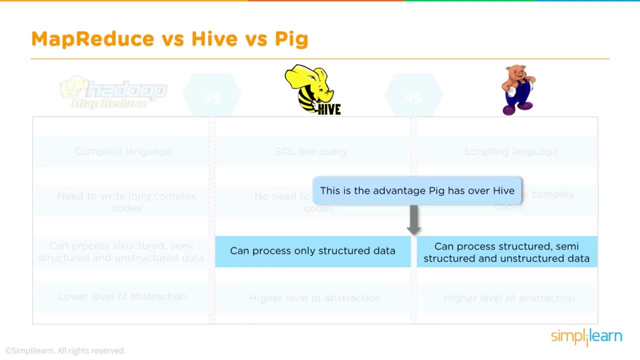 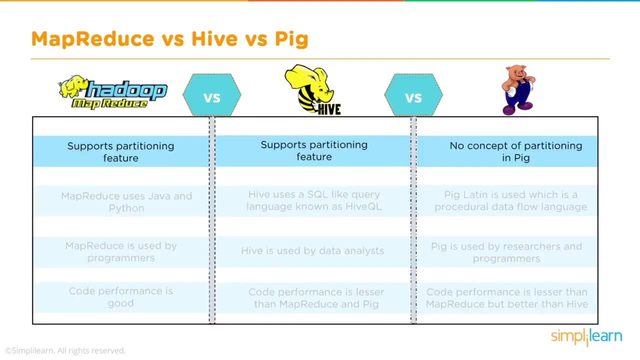 It can process only structured data in Hive, while in Pig it can process structured, semi-structured and unstructured data. Some other features to note that separates the different query languages is when we look at Map and Reduce. MapReduce supports partitioning features, as does Hive. 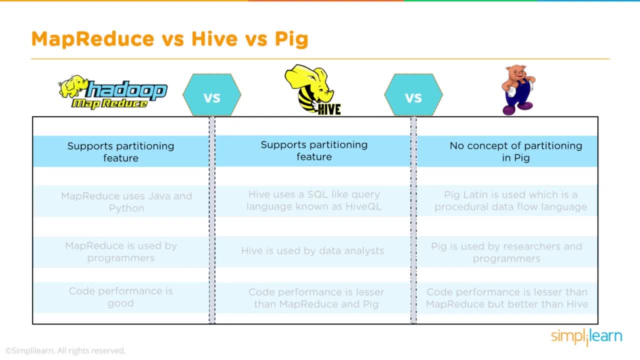 Pig. no concept of partitioning in Pig, So it doesn't support your partitioning feature. Your partitioning features allow you to partition the data in such a way that it can be queried quicker. You're not able to do that in Pig. 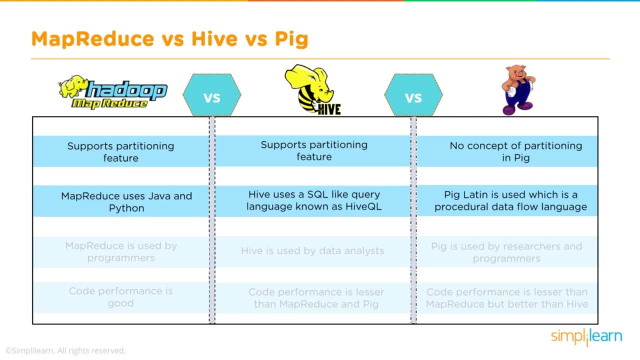 MapReduce uses Java and Python, while Hive uses an SQL-like query language known as HiveQL or HQL. Pig Latin is used, which is a procedural data flow language. MapReduce is used by programmers. pretty much is straightforward on Java. Hive is used by data analysts. 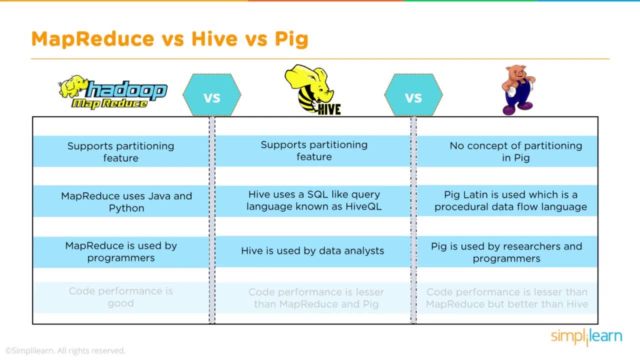 Pig is used by researchers and programmers. Certainly there's a lot of mix between all three. Programmers have been known to go in and use a Hive for a quick query, and anybody's been able to use Pig for a quick query or research. 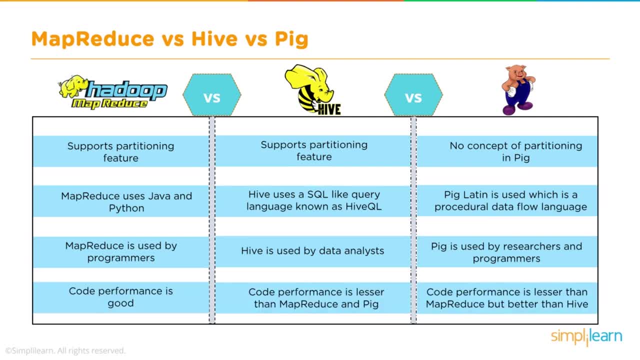 Under Map and Reduce code performance is really good. Under Hive code performance is lesser than Map and Reduce and Pig Under Pig code performance is lesser than MapReduce, but better than Hive. So if we're going to look at speed and time, the MapReduce is going to be the fastest performance. 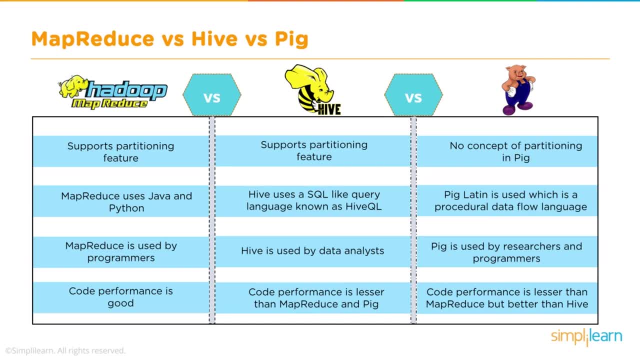 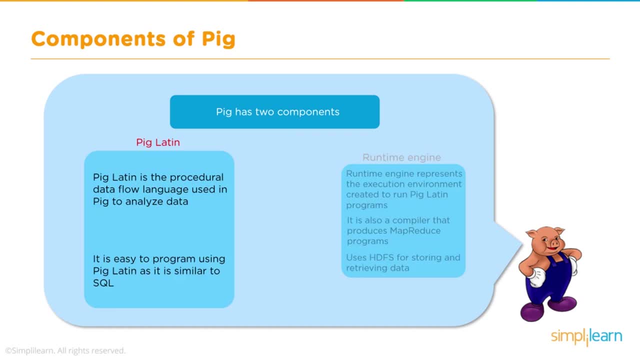 on all of those where Pig will have second and Hive follows in the back. Let's look at components of Pig. Pig has two main components. We have Pig Latin. Pig Latin is the procedural data flow language used in Pig to analyze data. 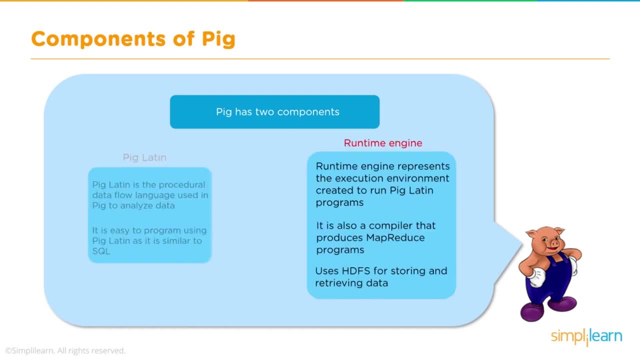 It is easy to program using Pig Latin. it is similar to SQL, And then we have the Runtime Engine. Runtime Engine represents the execution environment created to run Pig Latin programs. It is also a compiler that produces MapReduce programs. uses HDFS or your Hadoop file system. 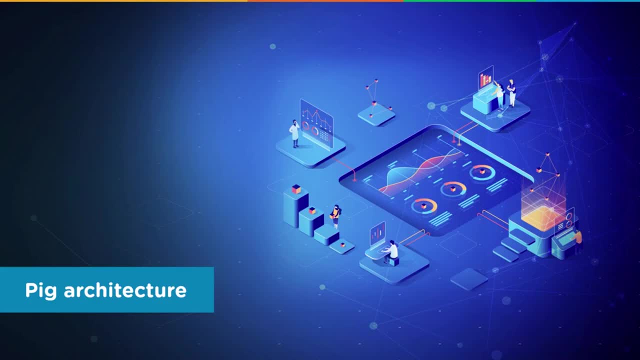 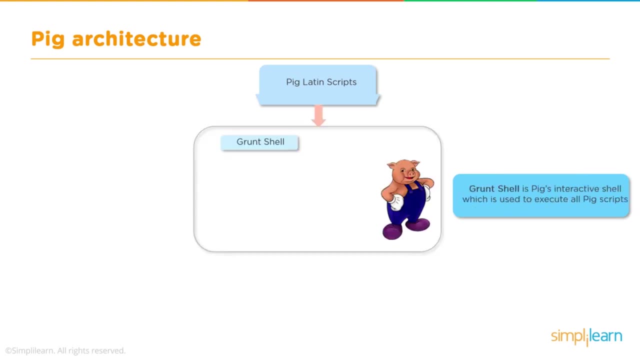 for storing and retrieving data. And as we dig deeper into the Pig architecture, we'll see that we have Pig Latin scripts. Programmers write a script in Pig Latin to analyze data using Pig. Then you have the Grunt shell and it actually says Grunt when we start it up. 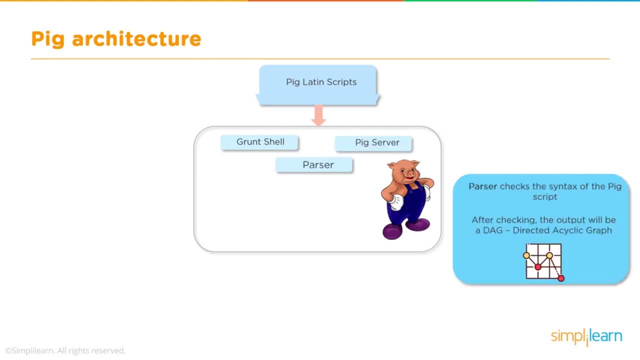 And we'll show you that here in a little bit- Which goes into the Pig server, and this is where we have our parser. Parser checks the syntax of the Pig script. After checking, the output will be a DAG directed acyclic graph. And then we have an optimizer which optimizes after your DAG. your logical plan is passed. 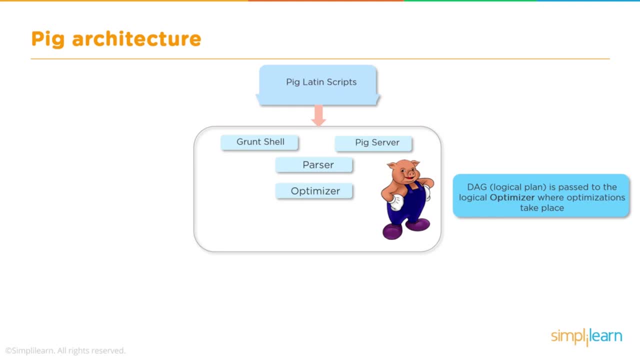 to the logical optimizer where an optimization takes place. Finally, the compiler converts the DAG into MapReduce jobs And then that is executed on the MapReduce under the execution engine. The results are displayed using DumpStack And again we'll show you that. 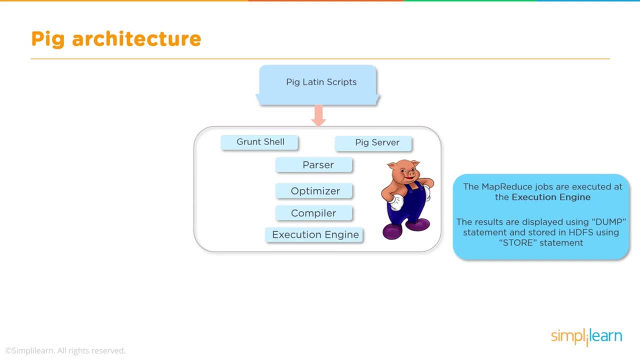 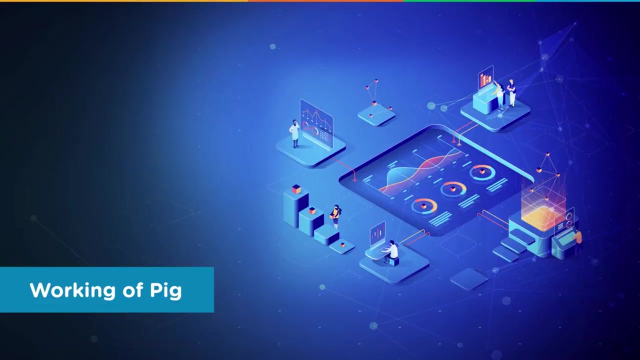 The kind of end you always want to execute everything once you've created it, And so Dump is kind of our execution statement And you can see right here, as we were talking about earlier, once we get to the execution engine and it's coded into MapReduce, then the MapReduce processes it onto the HDFS. 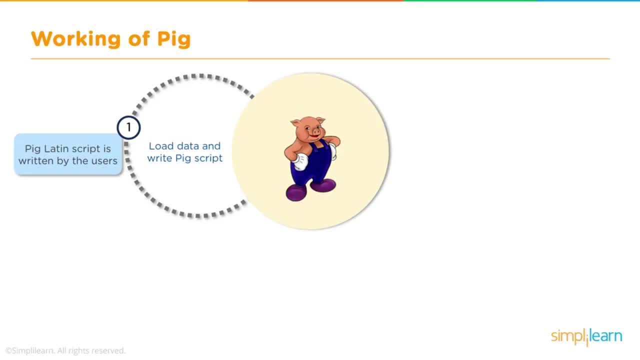 Working of Pig Pig Latin script is written by the users. So you have load data and write Pig script and Pig operations. So when we look at the workings, The working of Pig Pig Latin script is written by the users. There's step one. 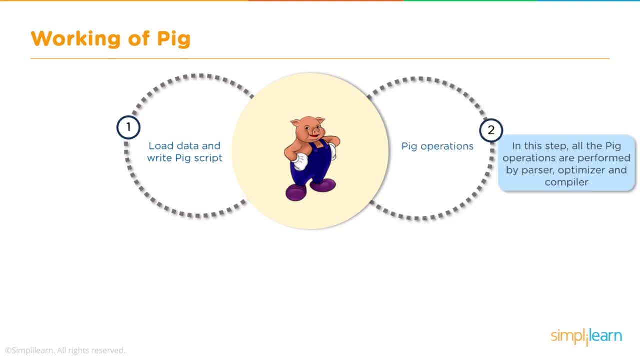 We load data and write Pig script. And step two: in this step all the Pig operations are performed by parser, optimizer and compiler. So we go into the Pig operations And then we get to step three, execution of the plan. 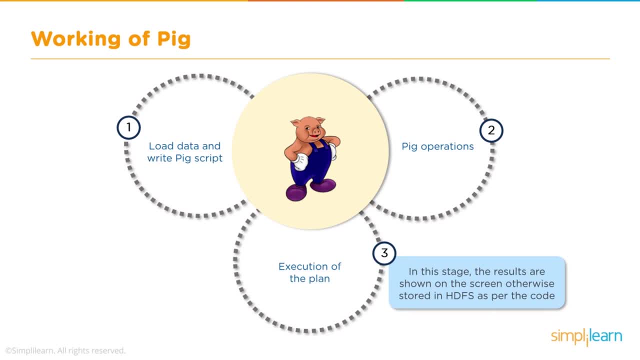 In this stage the results are shown on the screen, otherwise stored in the HDFS as per the code. So it might be of a small amount of data, you're reducing it to and you want to put that on the screen, Or you might be converting a huge amount of data. 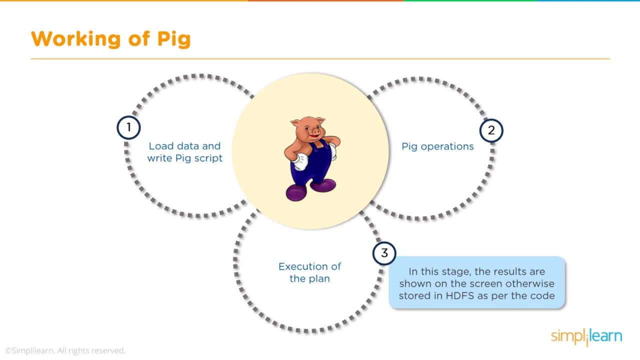 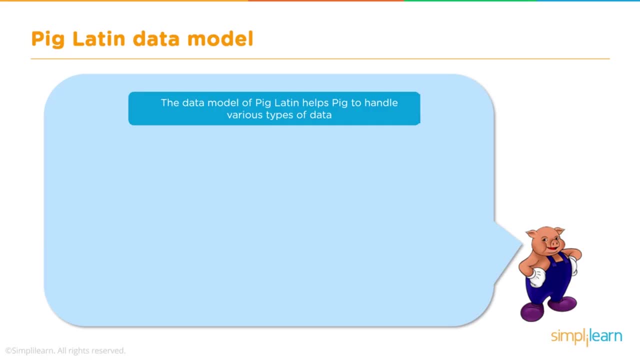 And you want to put that on the screen. So you have a huge amount of data which you want to put back into the Hadoop file system for other use. Let's take a look at the Pig Latin data model. The data model of Pig Latin helps Pig to handle various types of data. 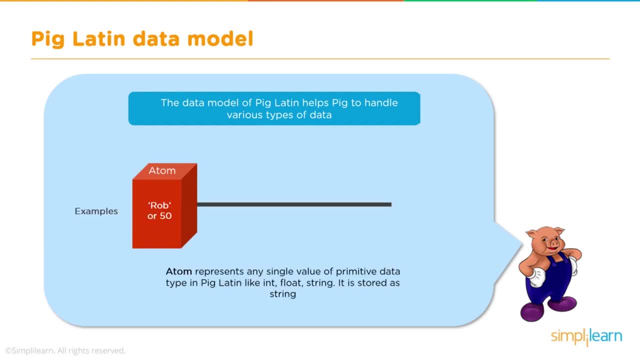 For example, we have atom, rob or 50. Atom represents any single value of primitive data type. in Pig Latin, like integer, float string, It is stored as a string Tuple. so we go from our atom, which are our most basic things. 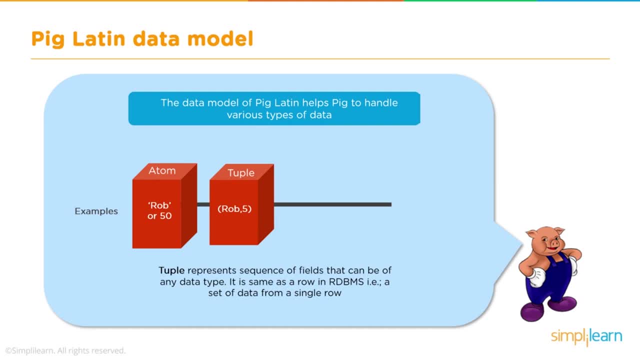 So if you look at just rob or just 50, that's an atom. That's our most basic object we have in Pig Latin. Then you have a tuple. A tuple represents a sequence of fields that can be of any data type. It is the same as a row in RDBMS. 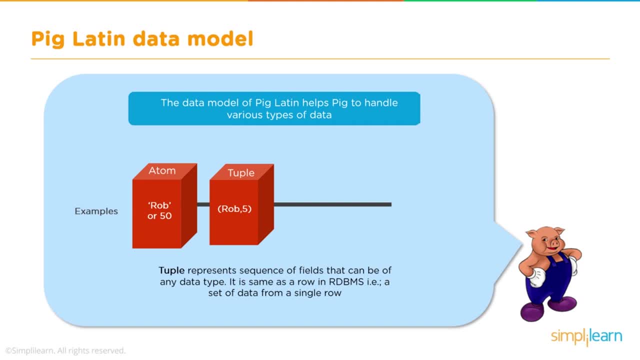 For example, a set of data from a single row. You can see here we have rob, comma five. You can imagine with many of our other examples we've used. you might have the ID number, the name where they live, their age, their date of starting the job. 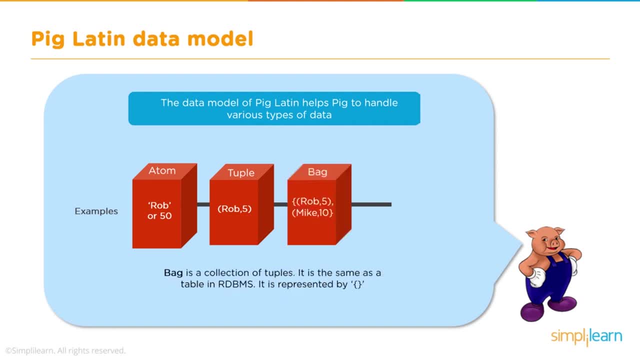 That would all be one row and stored as a tuple, And then we create a bag. A bag is a collection of tuples. It is the same as a table in RDBMS and is represented by brackets. And you can see, here we have our table with rob five, mike ten. 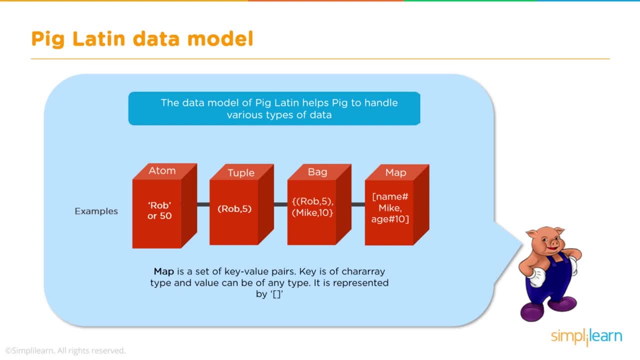 And we also have a map. A map is a set of key value pairs. Key is of character, array, type, and a value can be of any type. It is represented by the brackets, And so we have name and age, where the key value is mike and ten. 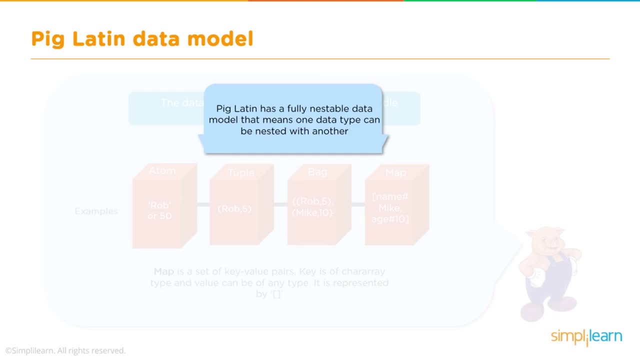 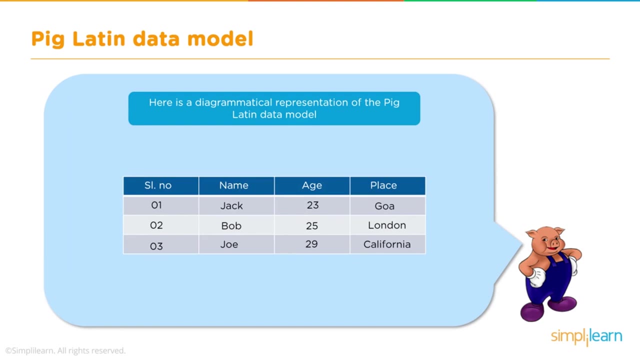 Pig Latin has a fully nestable data model. That means one data type can be nested within another. Here's a diagram, Here's a representation of Pig Latin data model And in this particular example we have basically an ID number, a name, an age and a place. 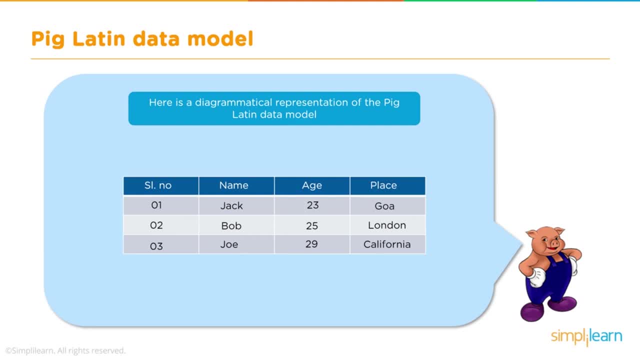 And we break this apart. We look at this model from Pig Latin perspective. We start with our field And, if you can remember, a field contains basically an atom. It is one particular data type And the atom is stored as a string, which then converts it into either an integer or number. 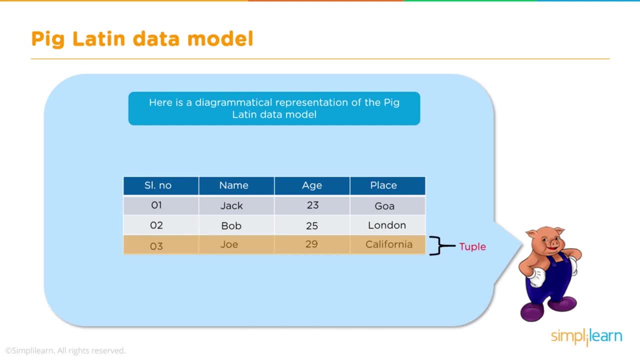 or character string. Next, we have our tuple, And in this case you can see that it represents a row, So our tuple would be a string. And then we have our table: It would be three comma Joe, comma 29 comma, California. And finally, we have our bag, which contains three rows in it, in this particular example, 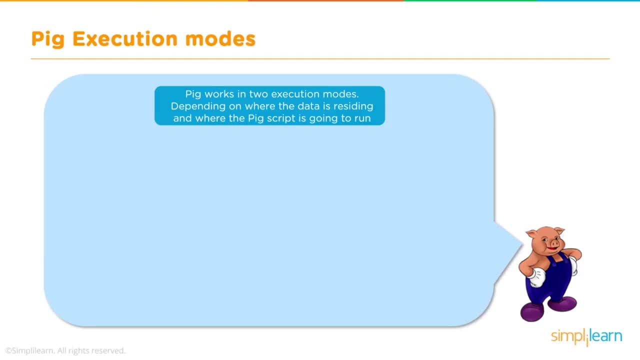 Let's take a quick look at pig execution modes. Pig works in two execution modes, depending on where the data is residing and where the pig script is going to run. We have local mode Here. the pig engine takes input from the Linux file system and the output is stored in the 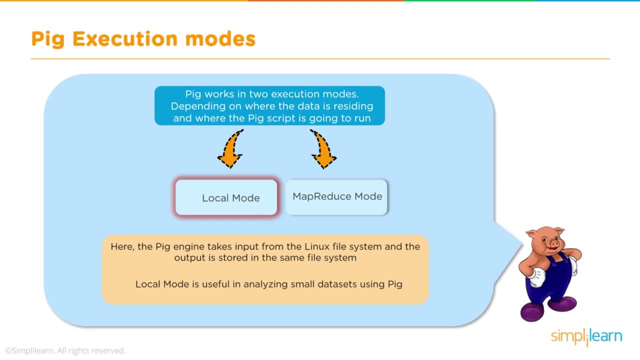 same file system: Local mode. Local mode is useful in analyzing small data sets using pig And we have the MapReduce mode Here the pig engine directly interacts and executes in HDFS and MapReduce. In the MapReduce mode, queries written in pig latin are translated into MapReduce jobs. 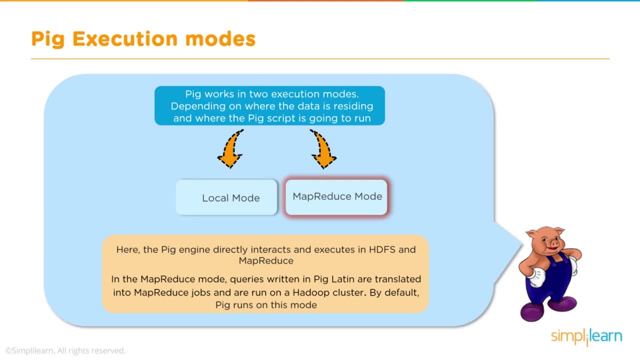 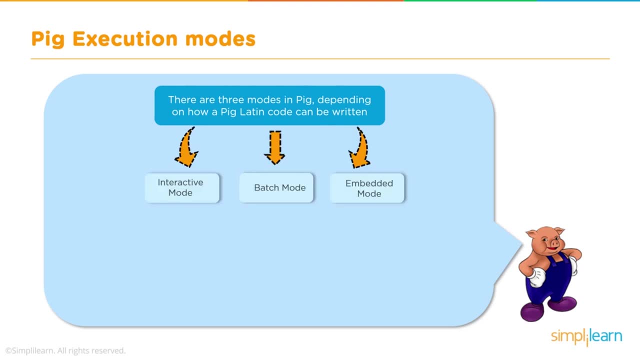 and are run on a Hadoop cluster. By default, pig runs in this mode. There are three modes in pig, depending on how a pig latin code can be written. We have our interactive mode, batch mode and embedded mode. The interactive mode means coding and executing the script line by line. 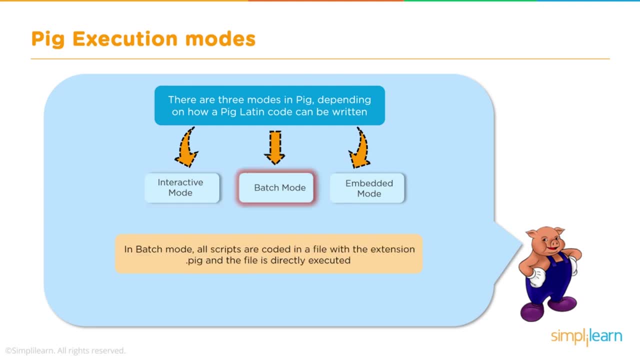 When we do our example, we'll be in the interactive mode. We'll be in the interactive mode In batch mode. all scripts are coded in a file with the extension pig, and the file is directly executed. And then there's embedded mode. 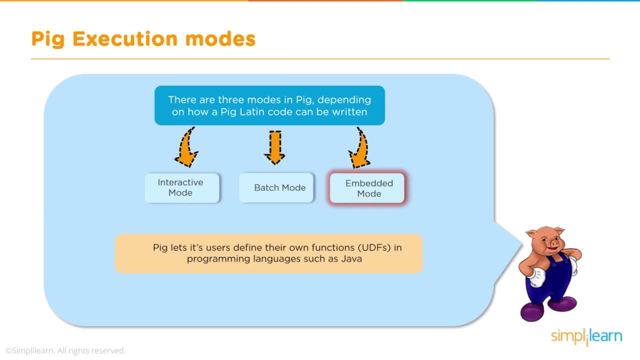 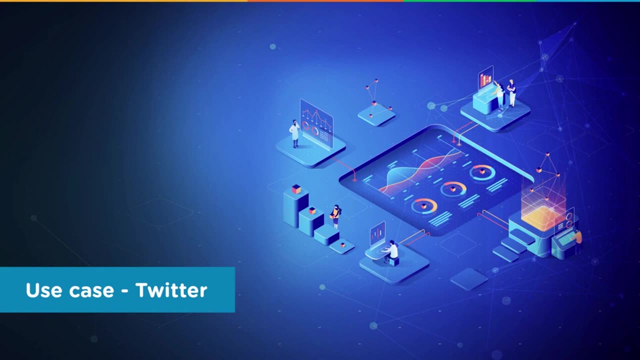 Pig lets its users define their own functions- UDFSs- in a programming language such as Java. So let's take a look and see how this works in a use case. in this case, use case Twitter. Users on Twitter generate about 500 million tweets on a daily basis. 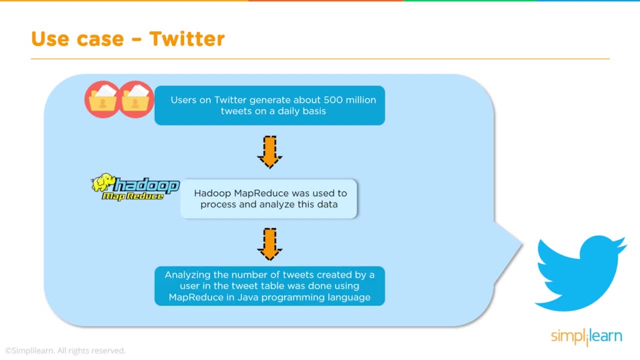 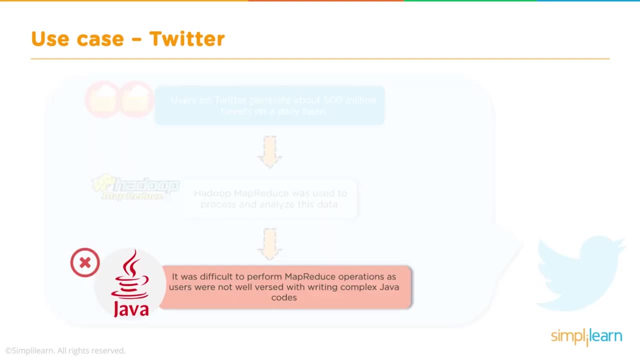 The Hadoop MapReduce was used to process and analyze this data. Analyzing the number of tweets created by the user And the tweet table was done using MapReduce in Java programming language And you can see the problem. It was difficult to perform MapReduce operations as users were not well versed with written. 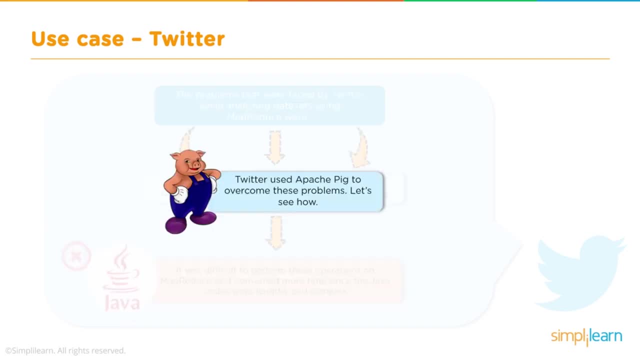 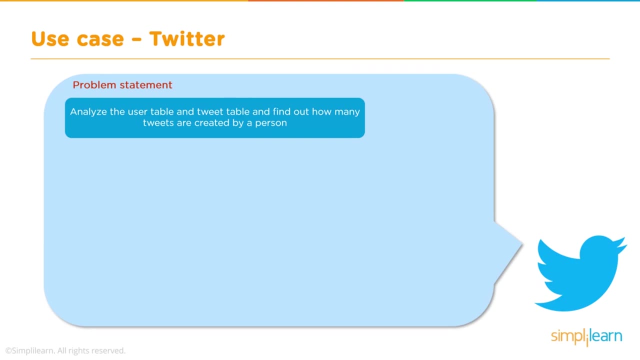 complex Java codes. So Twitter used Apache Pig to overcome these problems. And let's see how. Let's start with the problem statement: Analyze the user table and tweet table and find out how many tweets are created by a person. And here you can see we have a user table. 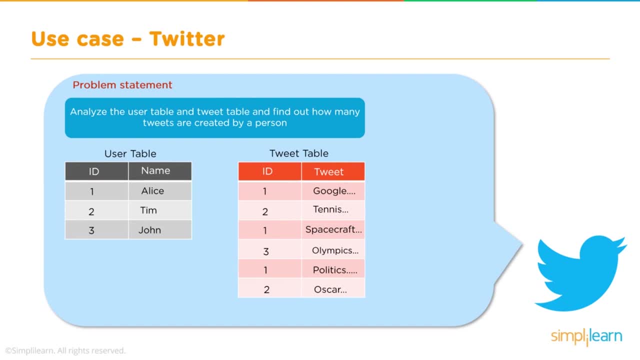 We have Alice, Tim and John with their ID numbers one, two, three, And we have a tweet table. In the tweet table you have the ID of the user and then what they tweeted. Google was a good, whatever it was: tennis, dot dot dot, spacecraft, Olympics, politics. 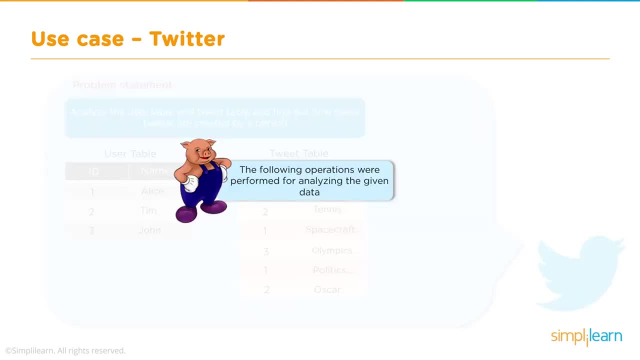 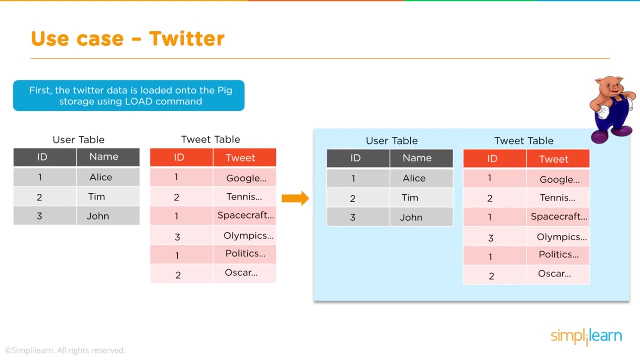 whatever they're tweeting about. The following operations were performed for analyzing given data: First, the Twitter data is loaded into the pig storage using load command And you can see here we have our data coming in and then that's going into pig storage. 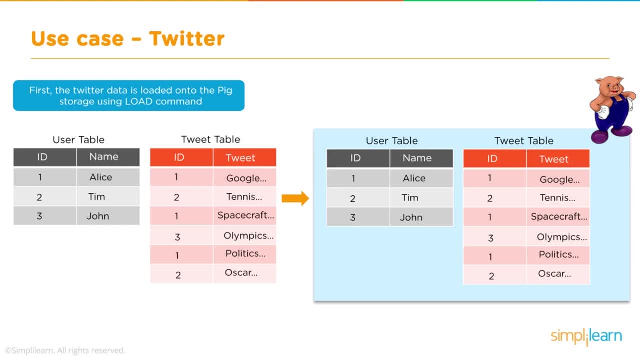 And this data is probably on an enterprise computer, So this is actually active Twitter's going on. And then it goes into Hadoop files. Remember, the Hadoop file system is a data warehouse for storing data, And so the first step is we want to go ahead and load it into the pig storage, into our 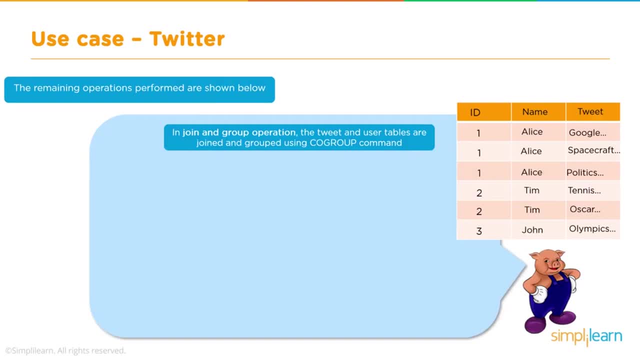 data storage system. The remaining operations performed are shown below. In join and group operation, the tweet and user tables are joined and grouped using co-group command And you can see here where we add a whole column and we go from user names and tweet. 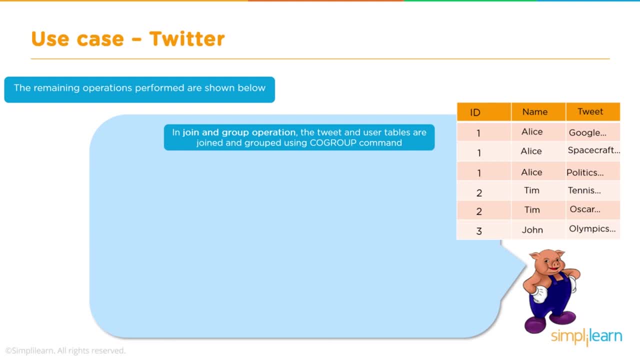 to the ID linked directly to the name. So Alice was user one, Tim was two And John three, And so now they're listed with their actual tweet. The next operation is the aggregation. The tweets are counted according to the names. The command used is count. 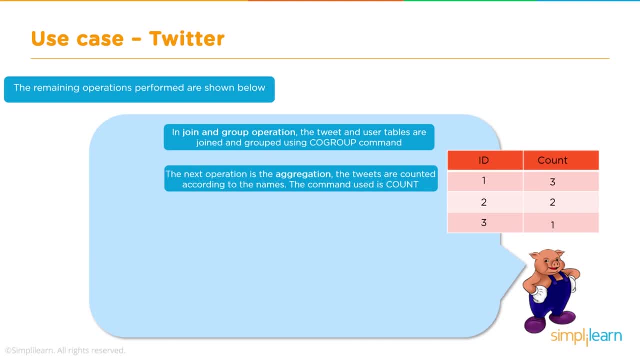 So it's very straightforward. We just want to count how many tweets each user is doing And finally the result after the count operation is joined with the user table to find out the user name, And you can see here where Alice had three, Tim two and John one. 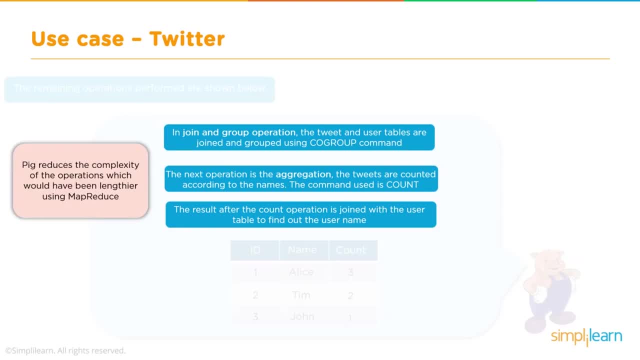 Pig reduces the complexity of the operations, which would have been lengthy, using MapReduce. In join and group operation, the tweet and user tables are joined and grouped using co-group command. The next operation is the aggregation. The tweets are counted according to the names. 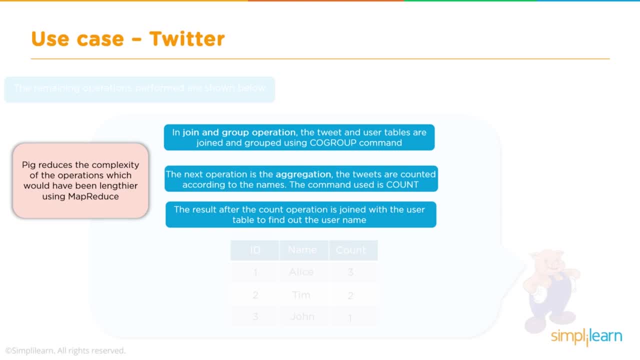 The command used is count. The result after the count operation is joined with the user table to find out the user name, And you can see we're talking about three lines of script versus a MapReduce code of about 80 lines. Finally, we could find out the number of tweets created by a user in a simple way. 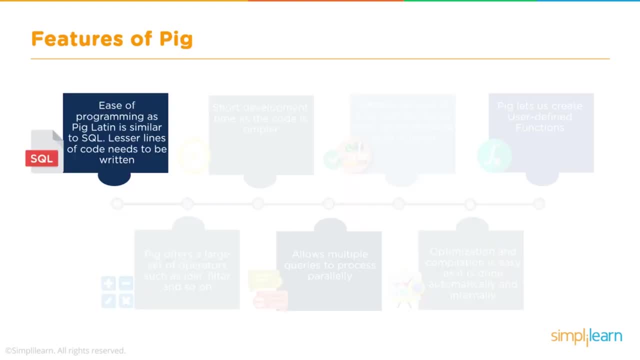 So let's go quickly over some of the features of Pig that we already went through. most of these First, ease of programming, as Pig Latin is similar to SQL. Lesser lines of code need to be written. Short development time, as the code is simpler. 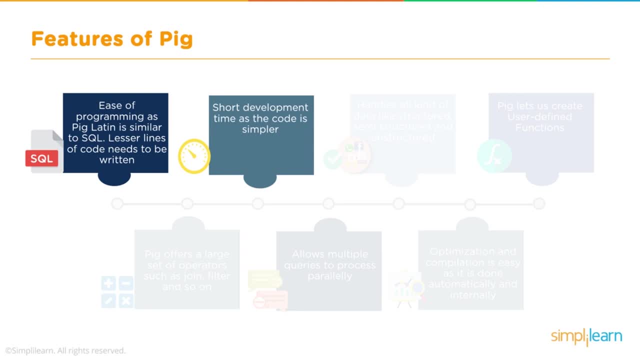 So we can get our queries out rather quickly instead of having to have a programmer spend hours on it. It handles all kinds of data like structured, semi-structured and unstructured. Pig lets us create user defined functions. Pig offers a large set of operators such as join, filter and so on. 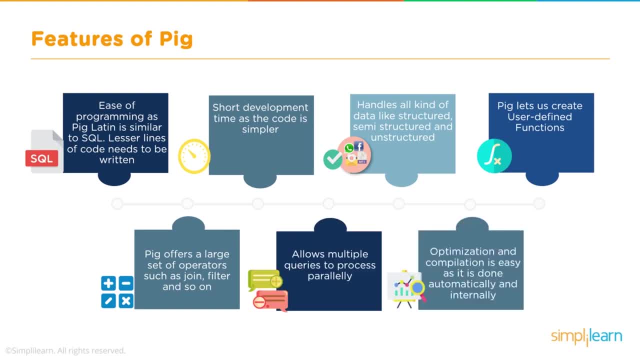 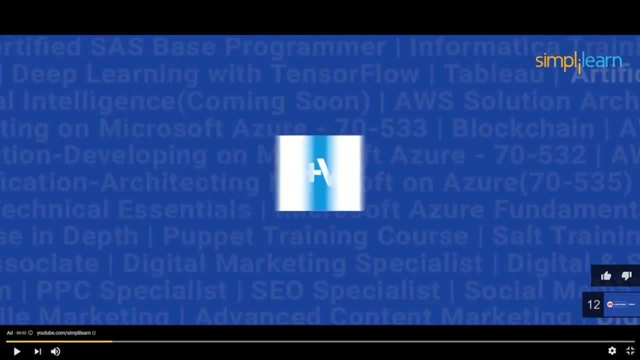 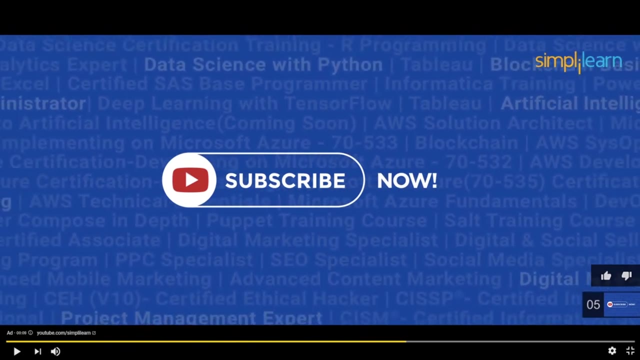 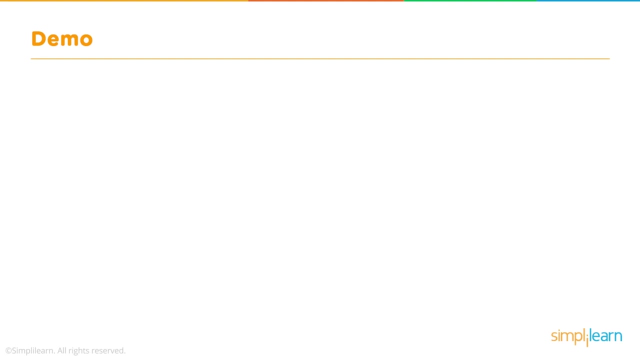 It allows for multiple queries to process unparallel, And optimization and compilation is easy, as it is done automatically and internally. So enough theory, Let's dive in and show you a quick demo on some of the commands you can do and pick Today's setup. 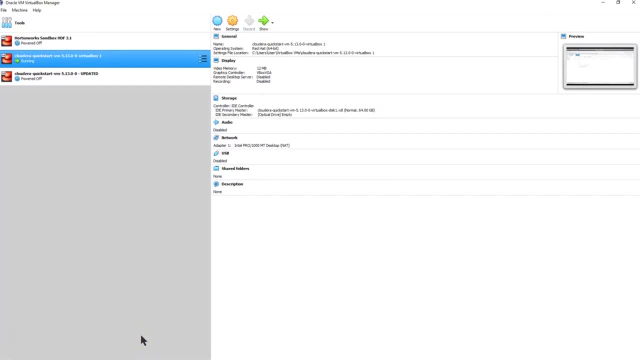 as we have in the last three demos, to go ahead and use Cloudera QuickStart, and we'll be doing this in VirtualBox. We do have a tutorial in setting that up. You can send a note to our Simply Learn team and then get that link to you Once your 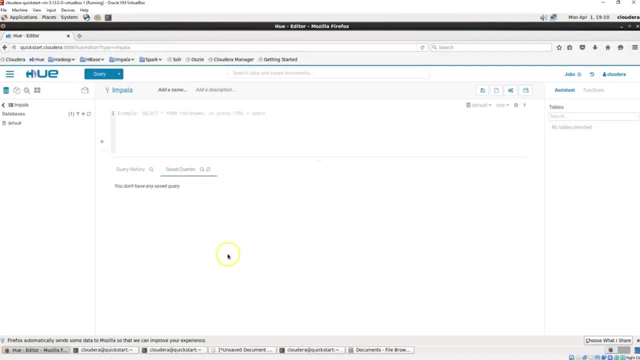 Cloudera QuickStart has spun up and remember, this is VirtualBox. We've created a virtual machine and this virtual machine is CentOS Linux. Once it's spun up, you'll be in a full Linux system here and, as you can see, we have Thunderbird browser, which opens up to the Hadoop basic system browser, and we 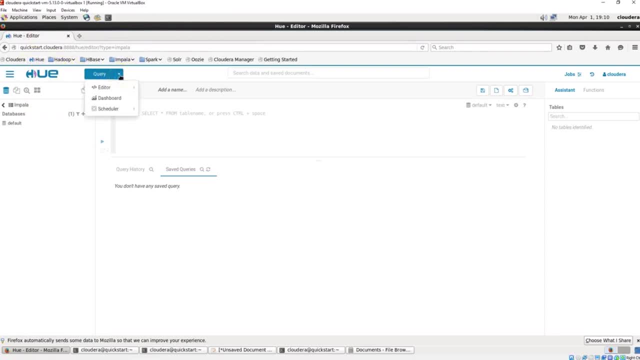 can go underneath the hue, where it comes up by default. If you click on the pull down menu and go under editor, you can see there's our Impala, our Hive PIG, along with a bunch of other query languages you can use. and we're going. 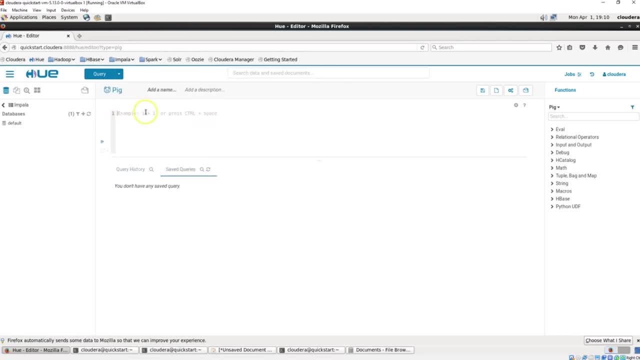 under PIG and then, once you're in PIG, we can go ahead and use our command line here and just click that little blue button to start it up and running. We will actually be working in terminal window, and so, if you were in the cloud, 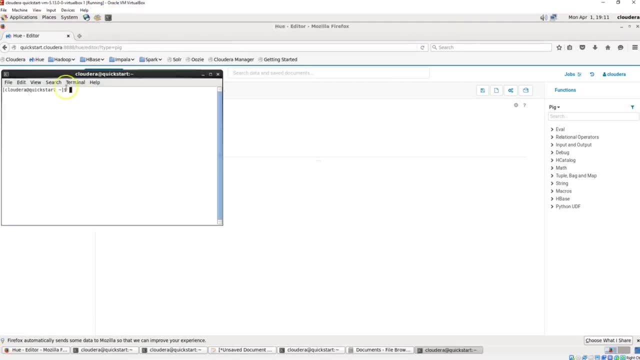 area. you could use that command line here and just click that little blue button to start it up and running. We will actually be working in terminal window and so if you were in the cloud area, you can go ahead and use our. a quick start: you can open up the terminal window up top or, if you're in 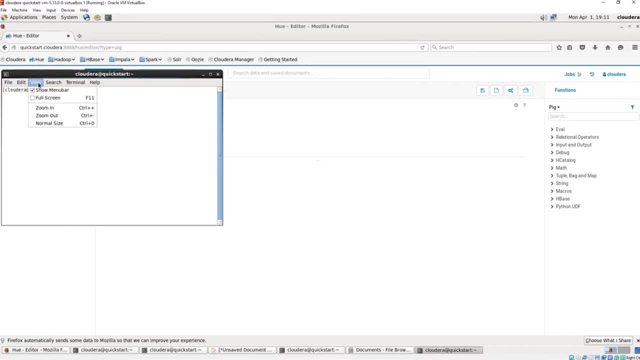 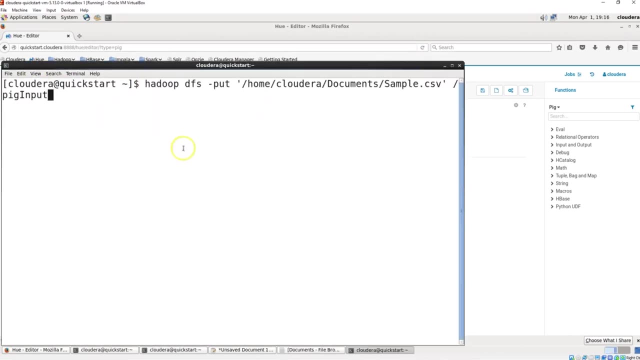 your own setup and you're logged in, you can easily use all of your commands here in terminal window and we'll zoom in. that way you get a nice view of what's going on. There we go Now for our first command. we're going to 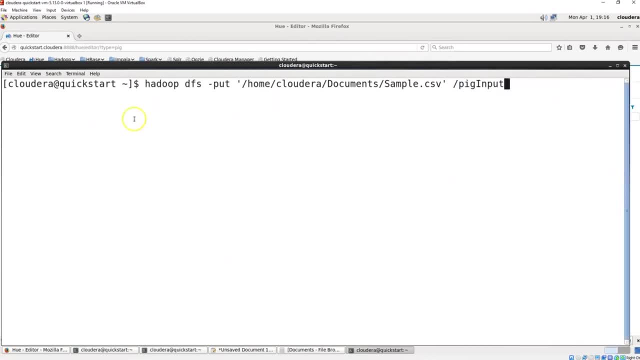 hit and do a Hadoop command and import some data into the Hadoop system, in this case a PIG input. Let's just take a look at this. we have a Hadoop now. let's know it's going to be a Hadoop command DFS. there's actually four variations. 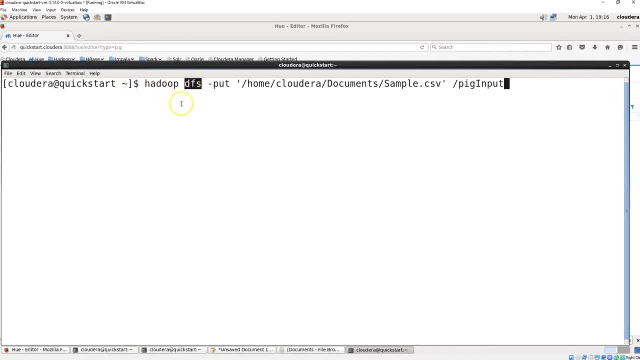 of DFS, if you have HDFS or you know whatever, that's fine. all four of them point used to be different setups underneath different things and now they all do the same thing and we want to put this file, which in this case is under home Cloudera documents and sample, and we just want to take that and put it. 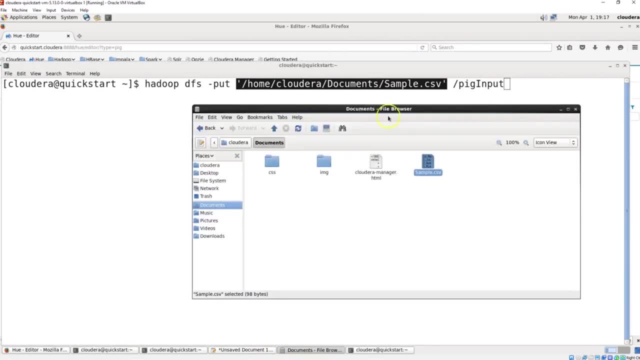 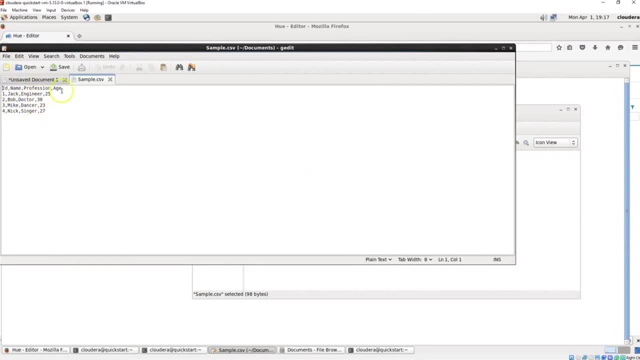 into the PIG input and let's take a look at that file. if I go under my document browsers and open this up, you'll see it's got a simple ID name, profession and age. we have one, Jack engineer, 25, and that was in one of our earlier things we had in there, and so let's go ahead and hit enter. 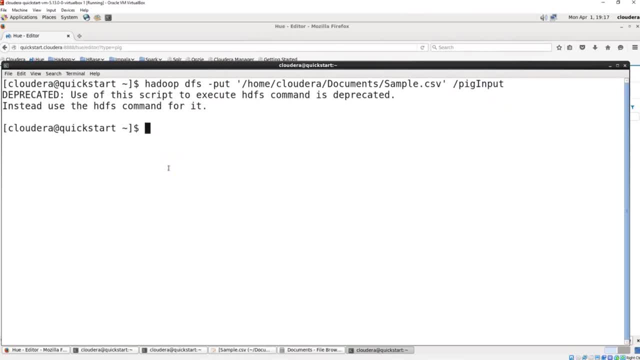 and execute this, and now we've uploaded that data and it's gone into our PIG input. and then a lot of the Hadoop commands mimic the Linux commands and so you'll see we have cat as one of our commands or it has a hyphen before it. so 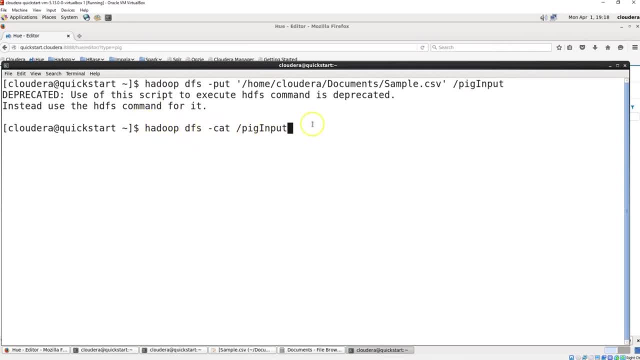 we execute that with Hadoop DFS hyphen cat slash, pig input, because that's what we called it. that's where we put our sample CSV at and we execute this. you can see from our Hadoop system is going to go in and pull that up and sure. 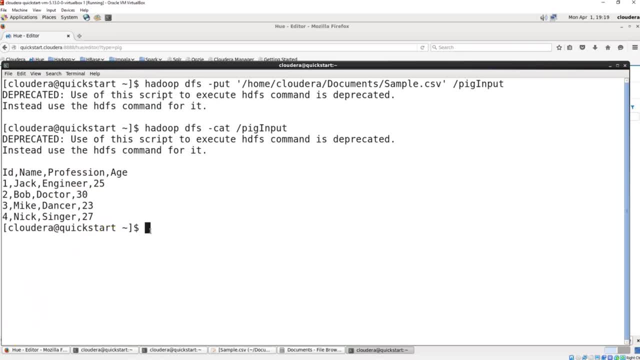 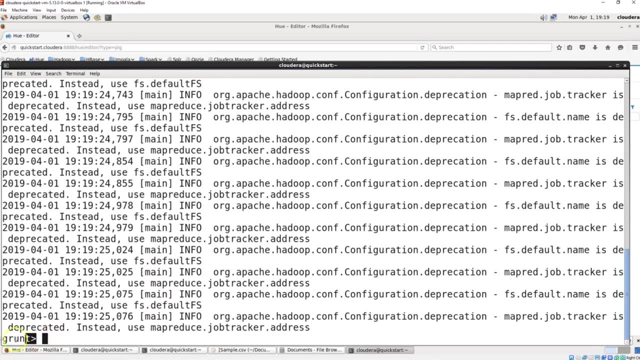 enough. it pulls out the data file we just put in there and then we can simply enter the pig Latin or pig editor mode by typing in pig and we can see here. by our grunt, I told you that's how it was going to tell you you were in pig Latin. 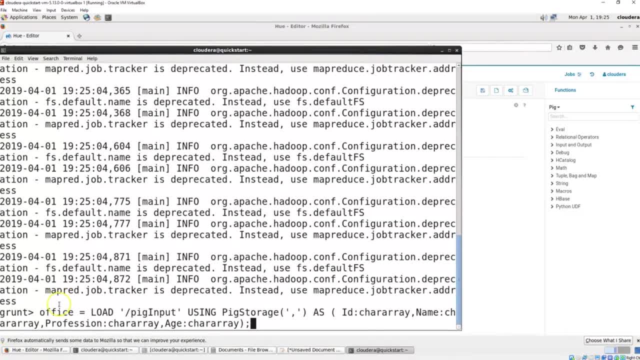 there's our grunt command line. so we are now in the pig shell and then we'll go ahead and put our load command in here, and the way this works is I'm going to have office equals load, and here's my load. in this case it's going to be: 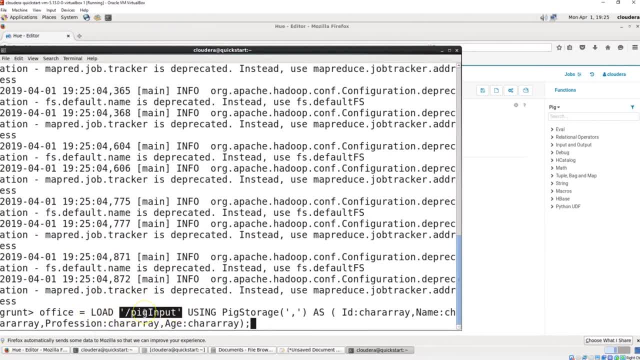 pig input. we have that in single brackets. you remember that's where the data is in the Hadoop file system, where we dumped it into there. we're going to using pig storage. our data was separated, as with a comma, so there's our comma separator and then we have, as in this case we have, an ID character, array name. 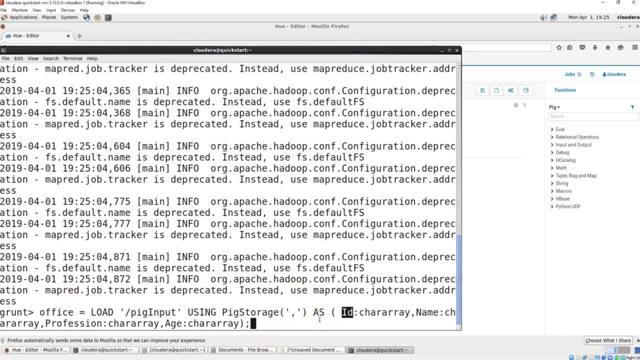 character array, profession character array and age character array, and we're just going to do them all as character arrays just to keep this simple for this one. and then when I hit, put this all in here. you can see that's our full command line going in and we have our semicolon. 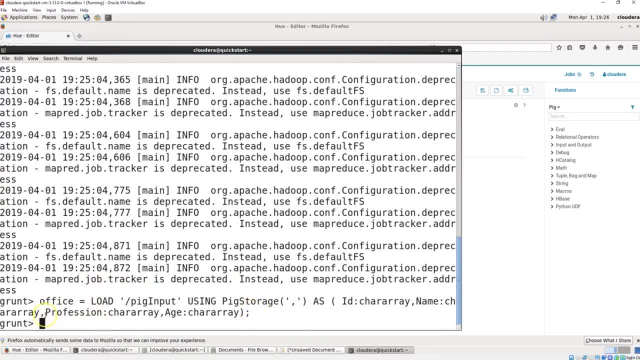 at the end. so when I hit enter it's now set office up, but it hasn't actually done anything yet. it doesn't do anything until we do dump office. so there's our command to execute whatever we've loaded or whatever setup we have in here and we 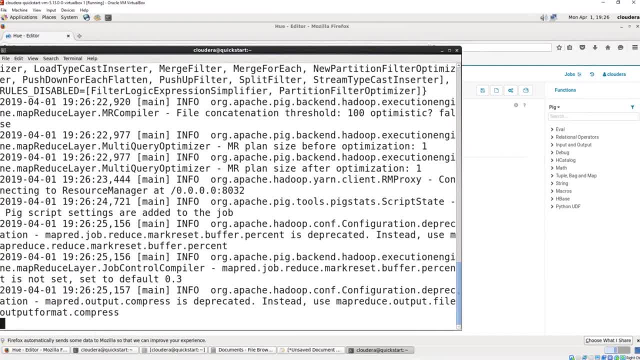 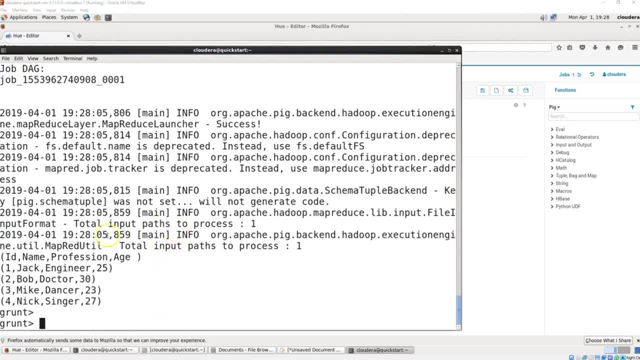 run that you can see it go through the different languages and this is going through the map reduce. remember we're not doing this locally, we're doing this on the Hadoop setup and once we finished our dump you can see we have ID, name, profession, age and all the information that 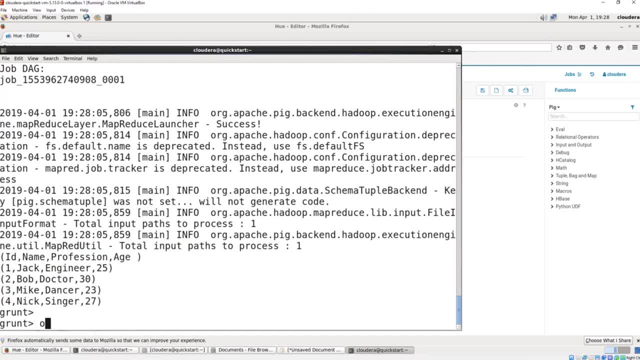 we just dumped into our pig. we can now do. let's say, oh, let's say we have a request, just for- we'll keep it simple in here, but just for the name and age, and so we can go office. we'll call it each as our variable underscore, each. now we'll 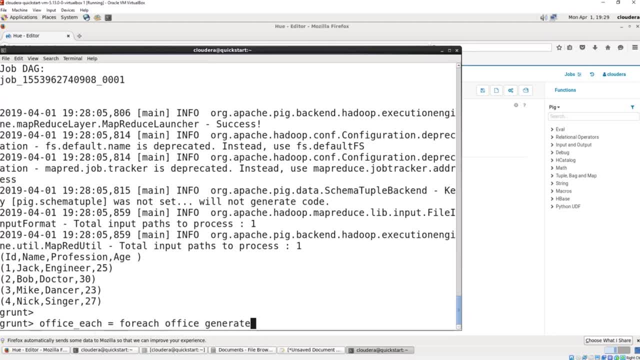 say, for each office, generate name, comma H and for each means that we're going to do this for each row. and if you're thinking map reduce, you know that this is a map function because it's mapping each row and generating name and age on here and of course, we want to go ahead and close it. 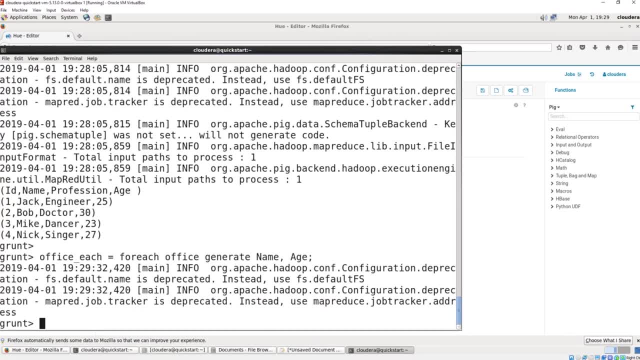 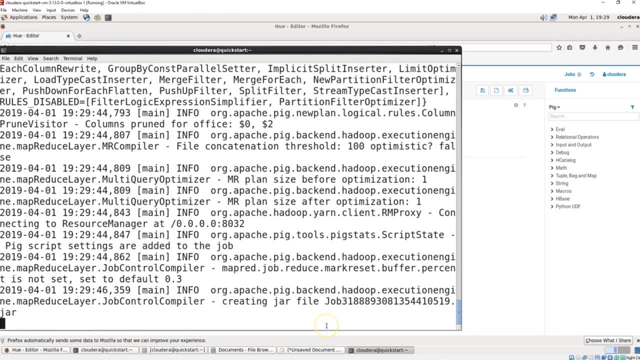 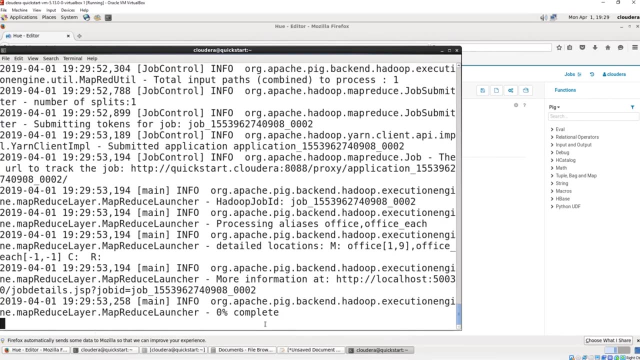 with a semicolon and then, once we've created our query or the command line in here, let's go ahead and dump office underscore each in with our semicolon and this will go through our map reduce setup on here. and if we were on a large cluster, the same processing time would happen. in fact it's really slow because 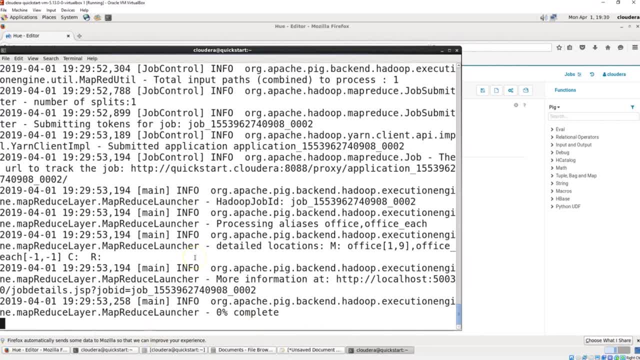 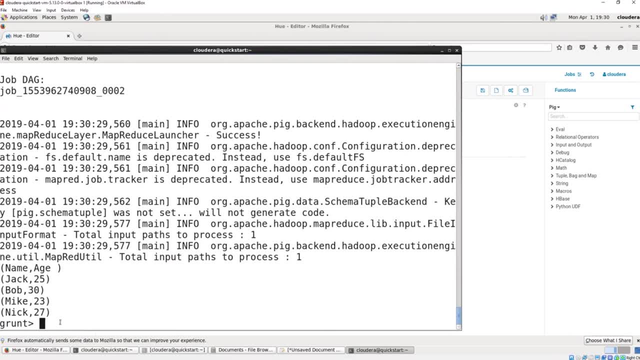 I have multiple things on this computer and this particular virtual box is only using a quarter of my processor. it's only dedicated to this and you can see here. there it is name, and age and it also included the top row, since we did delete that out of there or tell it not. 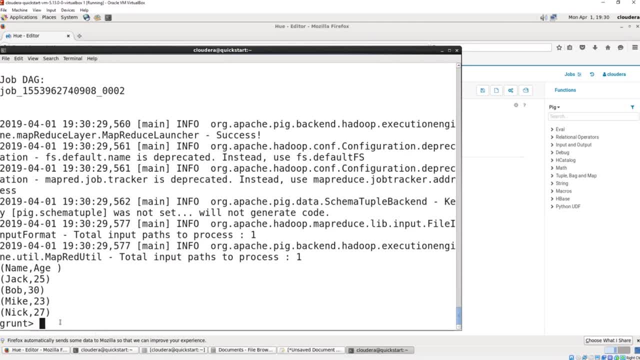 to, and that's fine for this example, but you need to be aware of those things. when you're processing a significantly large amount of data, or any data, then we can also do office and we'll call this DSC for descending. so maybe the boss comes to you and says, hey, can we order office by ID descending and of course, 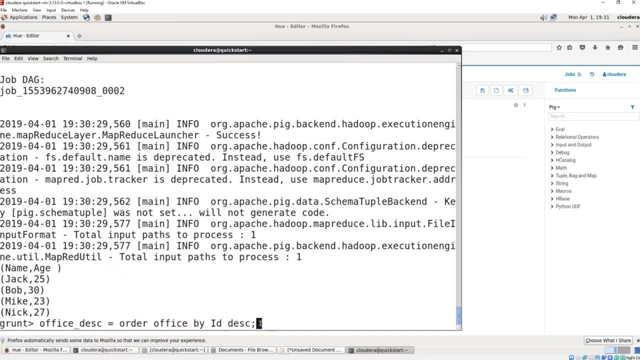 your boss, you've taught them how. to your shareholder- it sounds a little drugatory- say: boss, you've talked to the shareholder and you said: and you've taught them a little bit of pig Latin, and they know that they can now create office description and we can order. 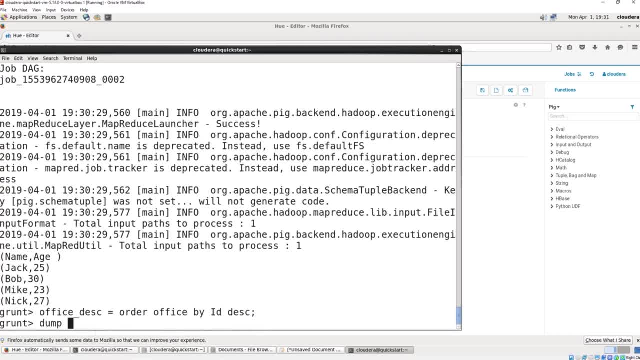 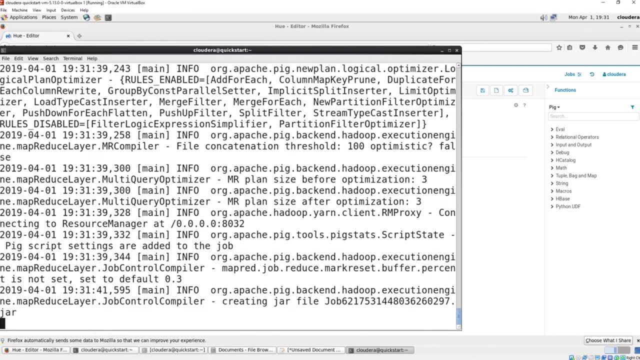 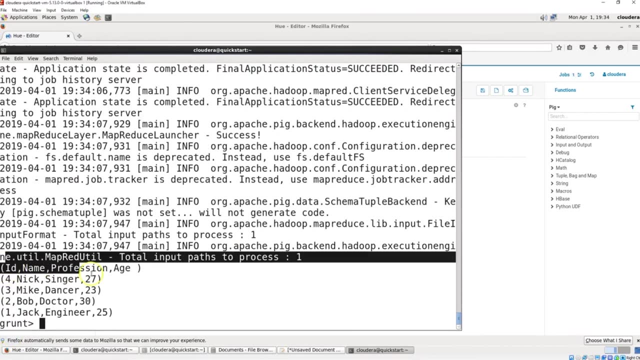 office by ID description and of course once we do that we have to dump office underscore description so that it'll actually execute and there goes into our map reduce. it'll take just a moment for it to come up because again I'm running on only a quarter of my processor and you can see we now have our IDs in. 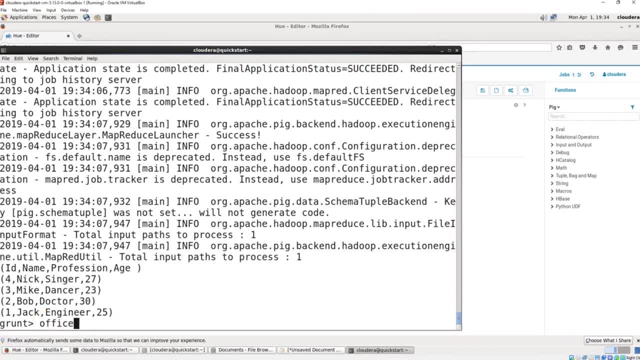 descending order returned. this is so important with any time you're dealing with big data. let's create office with a limit, and you can, of course, do any of this instead of with office. we could do this with office descending so you get just the top two IDs on there. we're gonna limit just to two and, of course, to execute that we 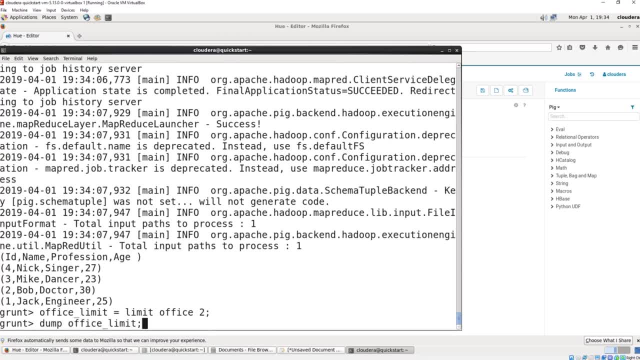 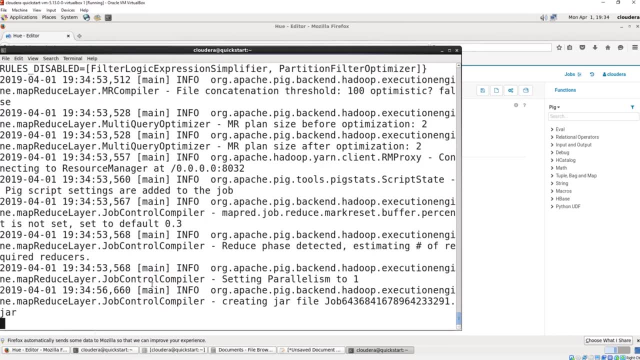 have to dump office underscore limit. you can just think of dumping your garbage into the pig pen for the pig to eat. there we go, dump office limit two and that's going to just limit our office to the top two. and for this example, we're going to limit our office to the top two. and for the 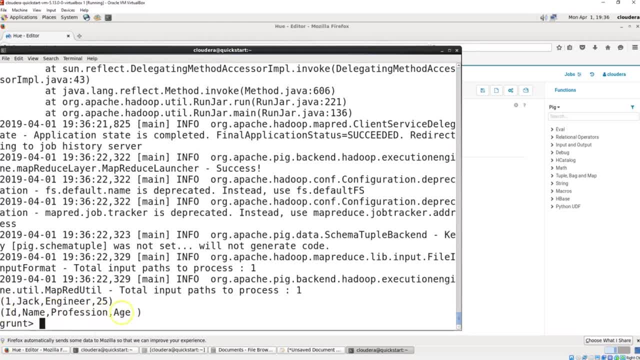 output. we get our first row, which had our ID name, profession and age, and our second row, which is Jack, who's an engineer. let's do one filter. we'll call it office underscore filter. you guessed it equals. filter office by profession equals. and keep note, this is similar to how Python does it with the double equal. 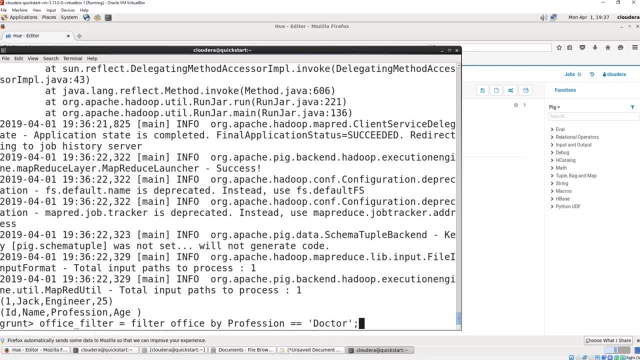 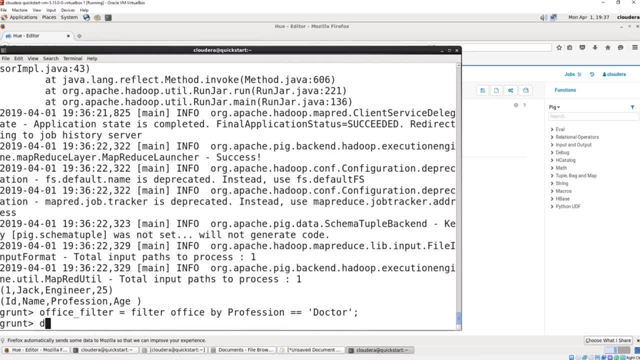 signs for equal for doing a true false statement. so if your logic statement, remember to use two equal signs in pig and we're gonna say it equals doctor. so we want to find a perfect code for the out- how many doctors do we have on our list? And we'll go ahead and do our dump. We're dumping all. 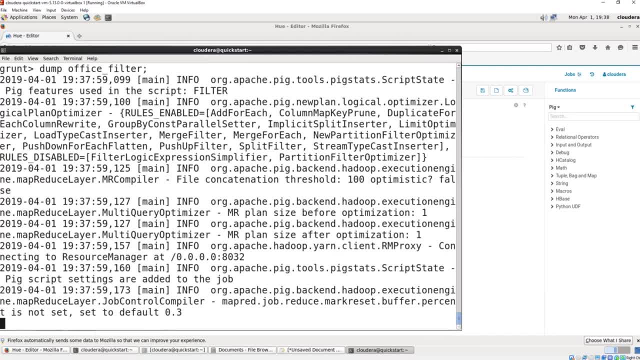 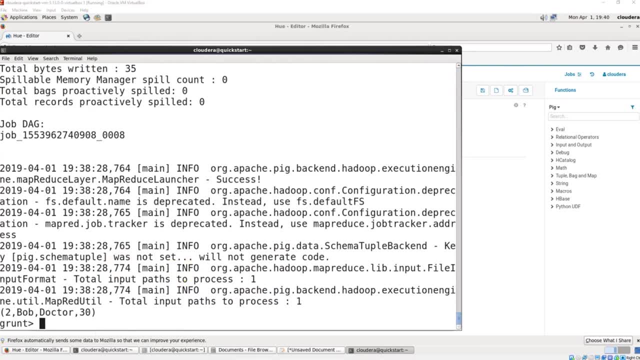 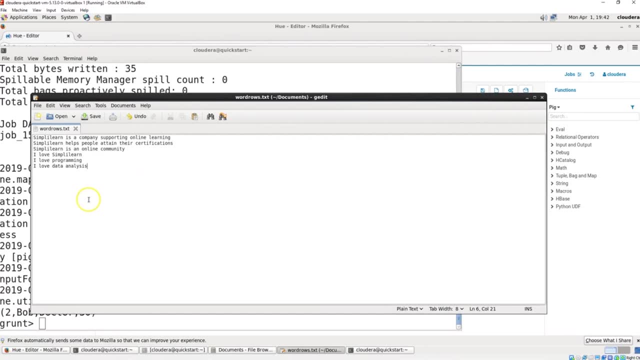 our garbage into the pig pen and we're letting pig take over and see what it can find out. and see who's a doctor on our list And we find employee ID number two: Bob is a doctor, 30 years old. For this next section, we're going to cover something we see a lot nowadays in data analysis. 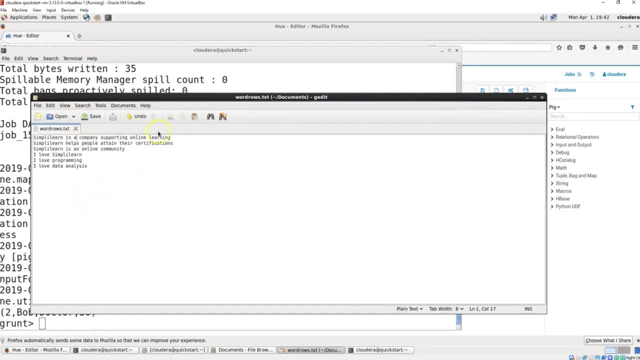 and that's word counting tokenization. That is one of the next big steps as we move forward in our data analysis, where we go from, say, stock market analysis of highs and lows and all the numbers to what are people saying about companies on Twitter. What are they saying on the web pages? 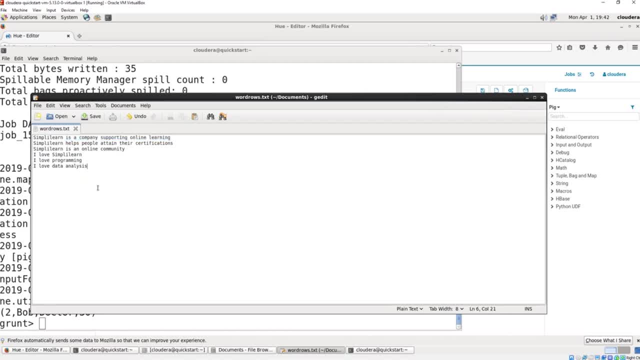 and on Facebook. Suddenly, you need to start counting words and finding out how many words are totaled, how many are in the first part of the document, and so on. We're going to cover a very basic word count example And in this case, I've created a document called wordrowstxt And you 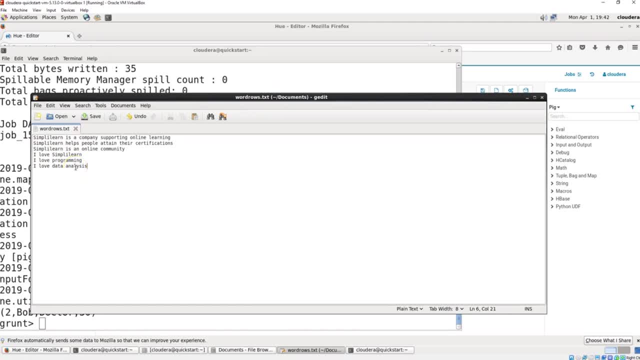 can see here we have. SimpliLearn is a company supporting online learning. SimpliLearn helps people attain their certifications. SimpliLearn is an online community. I love SimpliLearn, I love programming, I love data analysis And I went and saved this into my 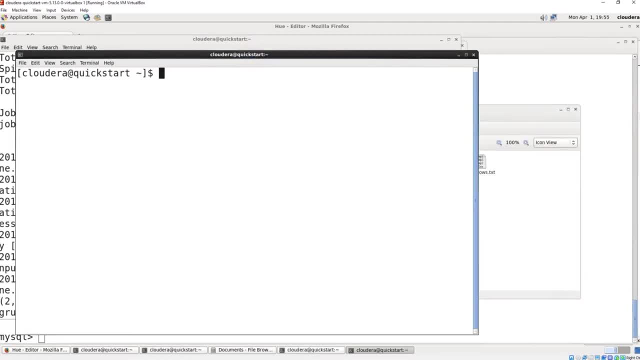 documents folder so we could use it. And let me go ahead and open up a new terminal window for our word count. Let me go and close the old one. So we're going to go in here and, instead of doing this as pig, we're going to do pig minus x local, And what I'm doing is I'm telling the pig to start. 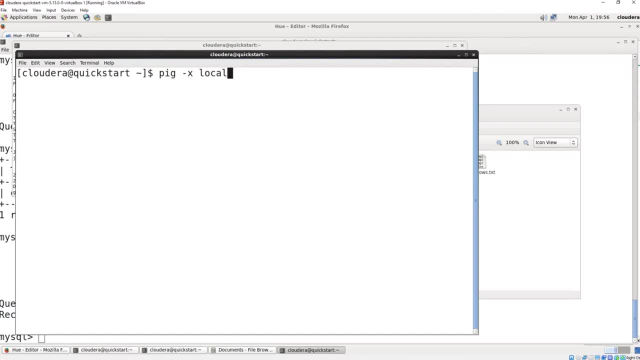 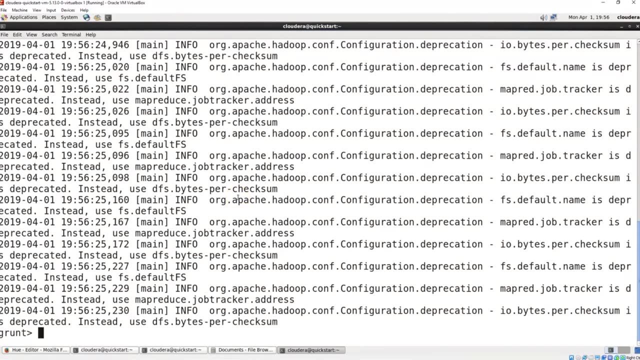 looking at files local to our virtual box or this CentOS machine And let me go ahead and hit enter on there, Just maximize this up, There we go And it'll load pig up And it's going to look just the same as the pig we were doing, which was defaulted to high to our Hadoop system, to our HDFS. This is now. 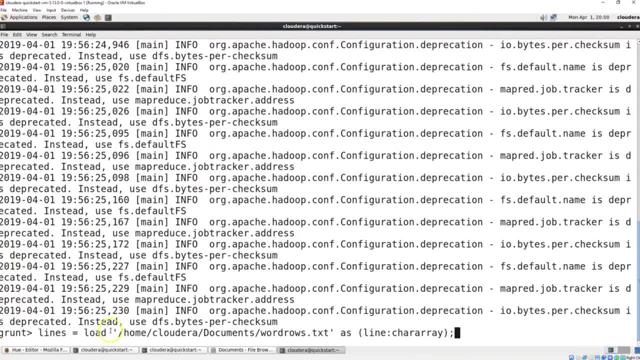 defaulted to the local system And now we're going to create lines. We're going to load it straight from the file. Remember last time we took the HDFS and loaded it into there and then loaded it into pig. So we're going the local, We're just going to run a local script. We have lines equals: load home the. 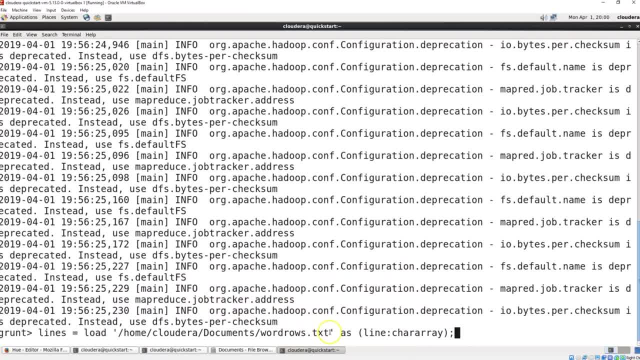 actual full path home Cloudera documents And I called it- word rows, dot text And as line is a character array. so each line- And I've actually you can change this- to read each document, I certainly have done a lot of document analysis- And then you go through and do word counts and 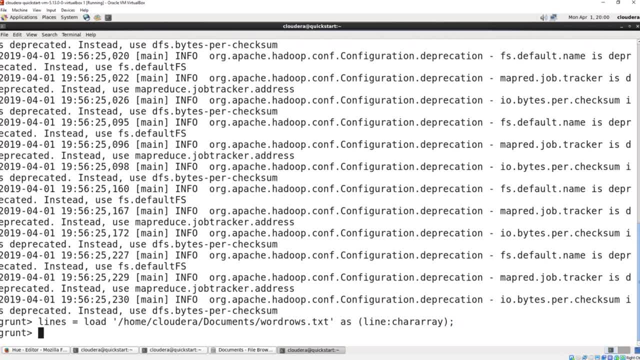 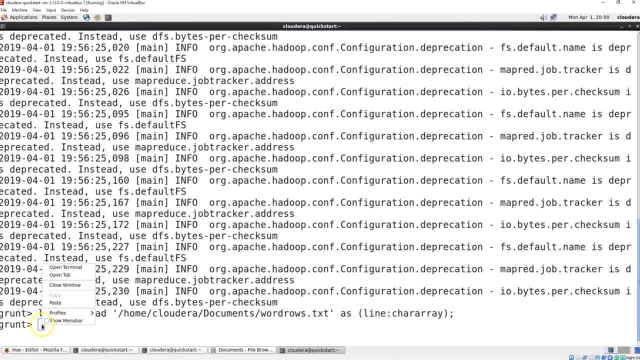 different kind of counts in there. So once we go ahead and create our line, instead of doing the dump, we're going to go ahead and start entering all of our different setups or each of our steps that we want to go through. And let's just take a look at this next one, because the load is 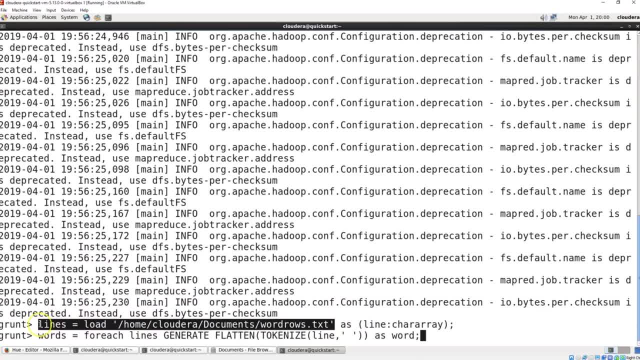 straightforward. We're loading from this particular file- Since we're locals, loading it directly from here instead of going into the Hadoop file system- And it says as: and. then each line is read as a character array. Now we're going to do words equal for each of the lines, generate flat, tokenize. 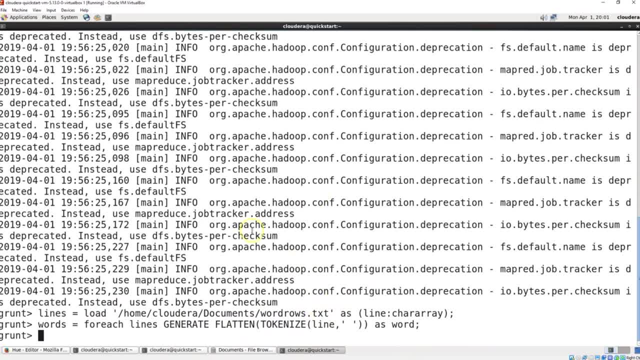 line space as word. Now, there's a lot of ways to do this. This is, if you're a programmer, you're just splitting the line up by spaces. There's actual ways to tokenize it. You got to look for periods, capitalization. There's all kinds of other things you play with. 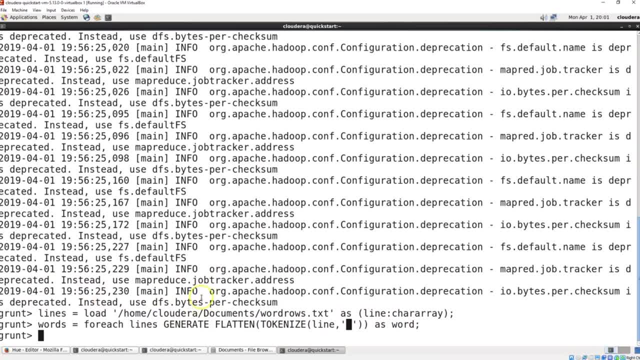 with this, But for the most basic word count, we're just going to separate it by spaces. The flatten takes the line and just creates a. it flattens each of the words out. So this is: we're just going to generate a bunch of words for each line And then each of those words is as a 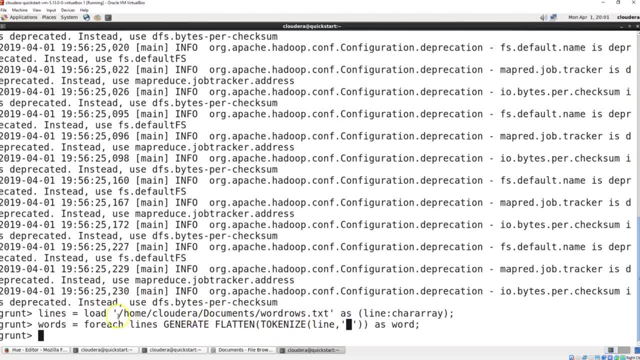 word A little confusing in there, but if you really think about it, we're just going down each line, separating it out and we're generating a list of words. One thing to note is the default for tokenize. you can just do tokenize line without the space in there. If you do that, 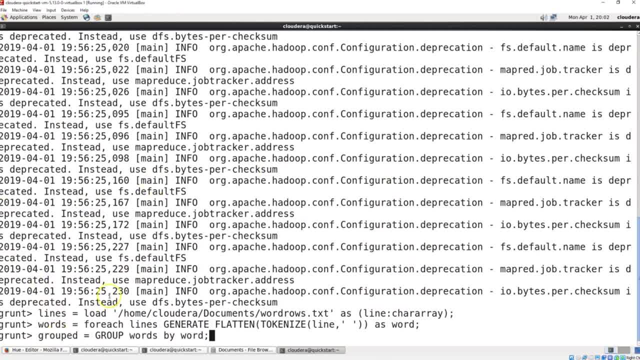 it'll automatically tokenize it by space. You can do either one, And then we're going to do group. We're going to group it by words. So we're going to group words by word. So when we split it up, each token is a word and it's a list of words, And so we're going to grouped equals group words. 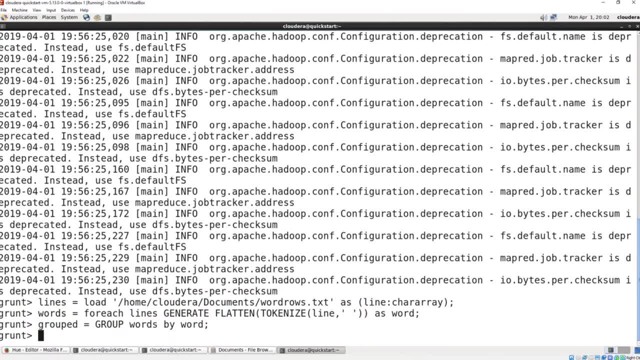 by words. So we're going to group all the same words together. And if we're going to group them, then we want to go ahead and count them. And so, for count, we'll go ahead and create a word count variable, And here's our for each. So for each grouped, grouped is our line. 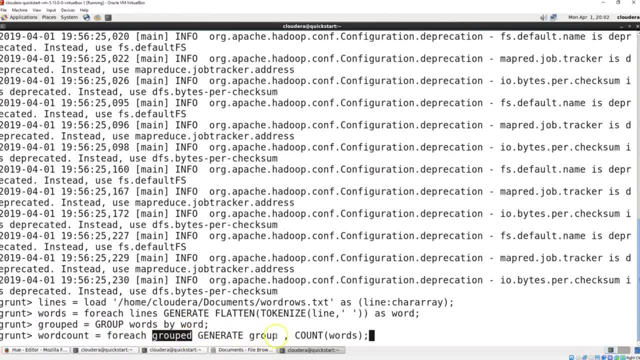 where we group all the words in the line that are similar, We're going to generate a group And then we're going to count the words For each grouped. so for each line where we group the words together, we're going to generate a group and that's going to count the words. 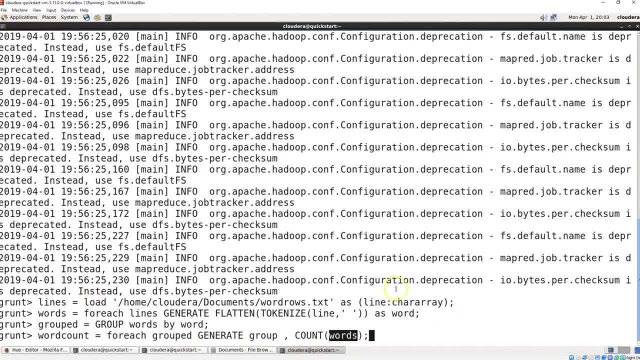 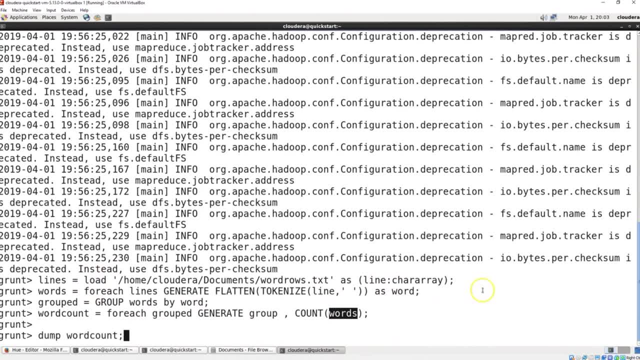 So we want to know the word count in each of those And that comes back in our word count. And finally, we want to take this and we want to go ahead and dump word count. And this is a little bit more what you see when you start looking at Grunt scripts. You'll see right. 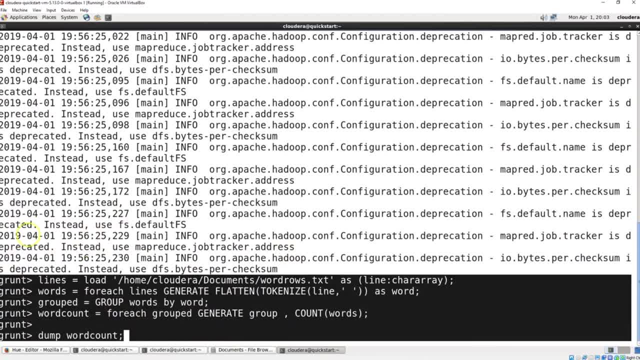 here these lines, right here we have each of the steps you take to get there. So we load our file For each of our lines. we're going to generate and tokenize it into words. Then we're going to take the words and we're going to group them by same words For each grouped. we're going to generate. 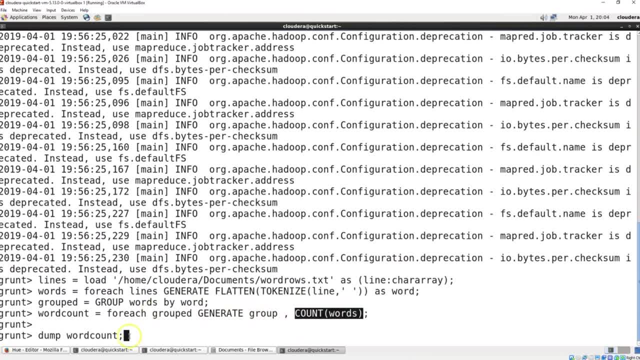 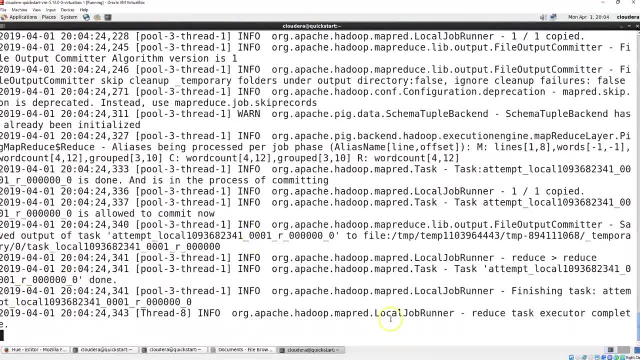 a group and we're just going to count the words. So we're going to summarize all the words in here And let's go ahead and do our dump word count which executes all this, And then we're going to- and it goes through our MapReduce. It's actually a local runner, You'll see down here you start. 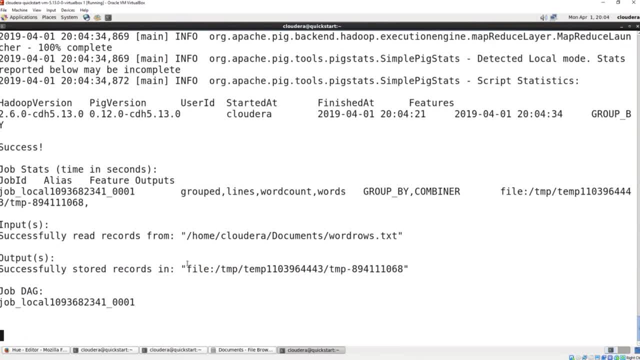 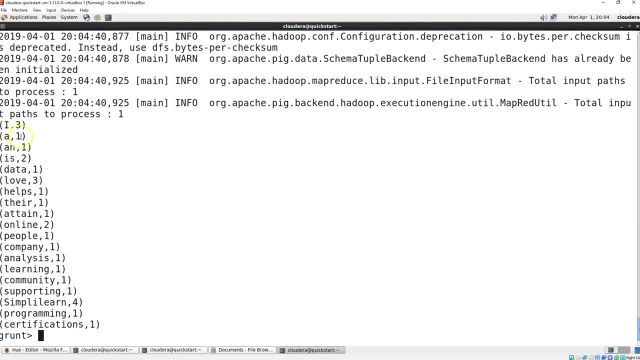 seeing where they still have MapReduce. but it's a special runner. We're mapping it. That's a part of each row being counted and grouped and then when we do the word count, that's a reducer. The reducer creates these keys and you can see I is used three times: A came up once and came up once. 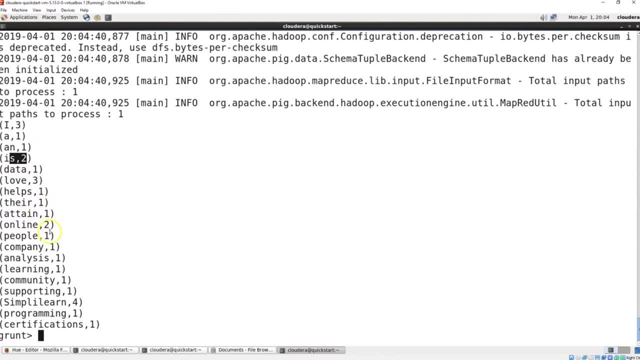 is two. Continue on down here to attain online people company analysis. simply learn. They took the top rating with four certification. so all these things are then counted in the how many words are used In a data analysis. this is probably the very beginnings of data analysis, where you might 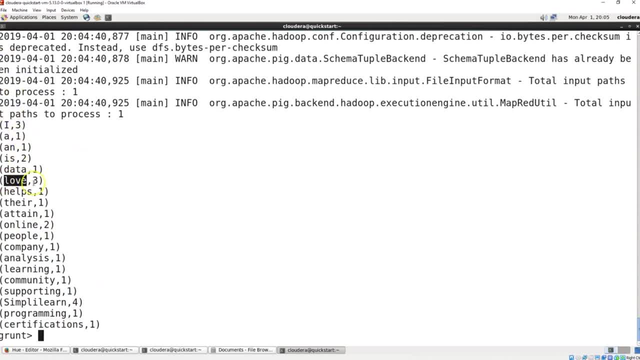 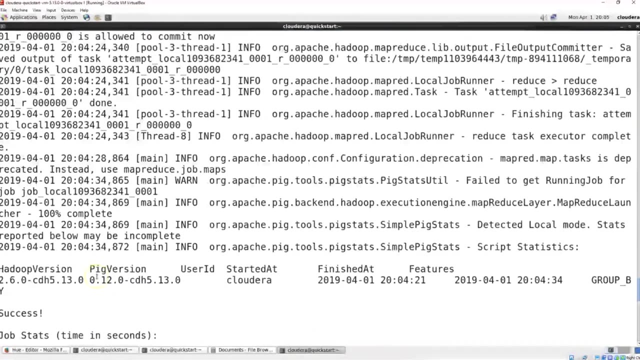 look at it and say, oh, they mentioned love three times. so whatever's going on in this post, it's about love and what do they love. and then you might attach that to the different objects in here, So you can see that Pig Latin is fairly easy to use. There's nothing really, you know it might. 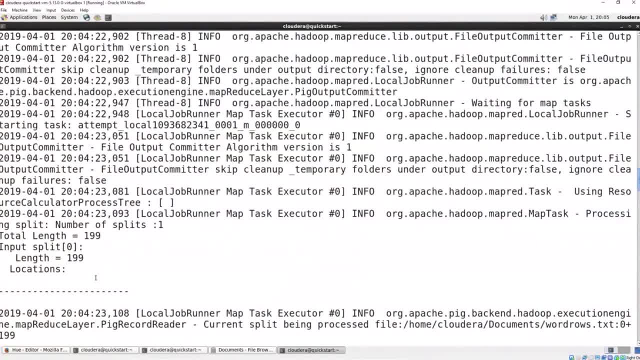 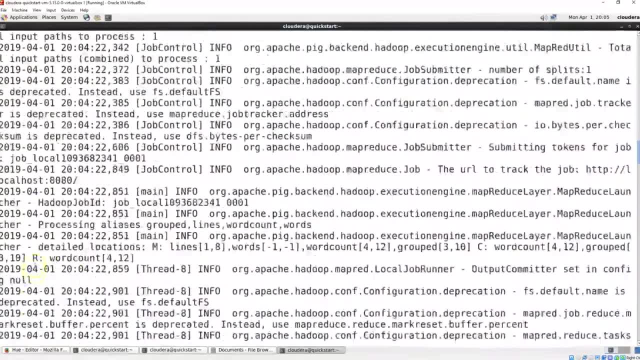 take a little bit to learn the script, depending on how good your memory is. As I get older, my memory leaks a little bit more, so I don't memorize it as much. but that was pretty straightforward. the script we put in there and then it goes through. the full map- reduce, localize, run- comes out and 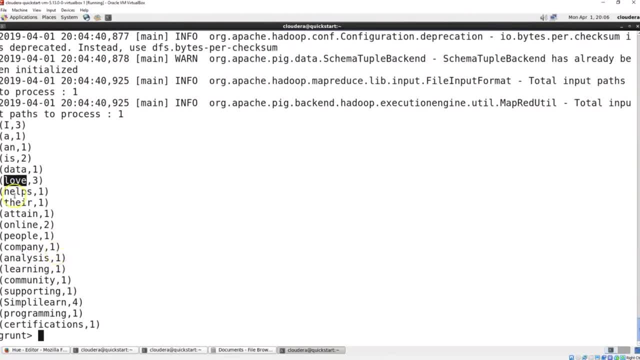 like I said, it's very easy to use. That's why people like Pig Latin is because it's intuitive. One of the things I like about Pig Latin is when I'm troubleshooting, When we're troubleshooting, a lot of times you're working with a small amount of data and you start doing one. 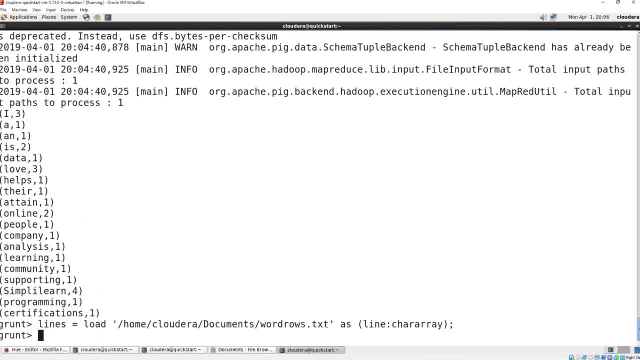 line at a time, and so I can go lines equal load and there's my loaded text and maybe I'll just dump lines and then it's going to run. it's going to show me all the lines that I'm working on in. 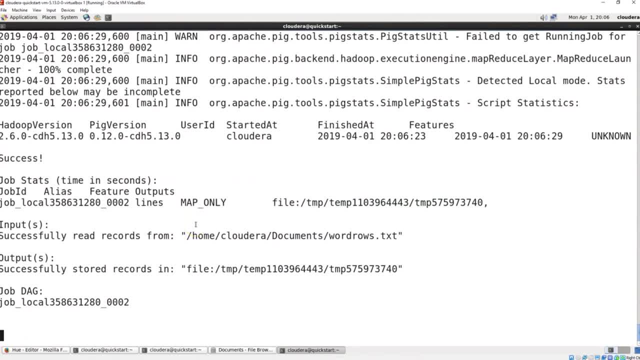 the small amount of data and that way I can test that. If I got an error on there that said, oh, this isn't working, maybe I'll be like, oh my gosh, I'm in map reduce or I'm in the basic. 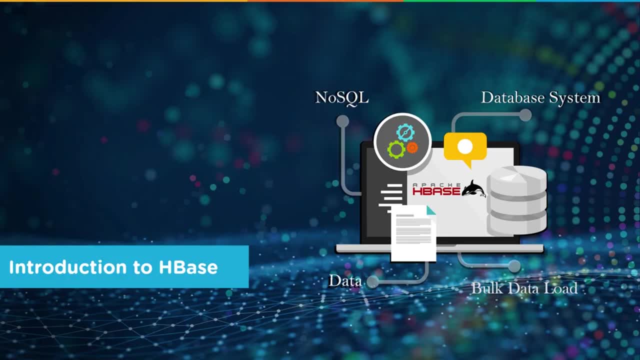 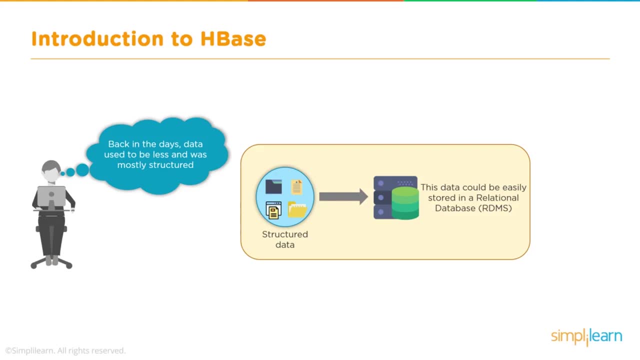 grunt shell instead of the local path grunt. Let's start with an introduction to HBase. Back in the days, data used to be less and was mostly structured. You can see we have structured data here. We usually had it like in a database, where you had every field was exactly the correct. 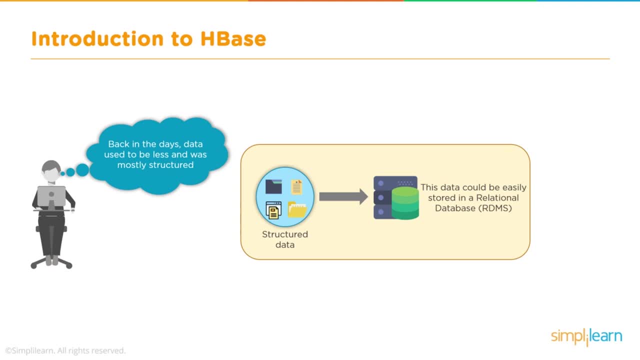 length, so if you had a name field, it was exactly 32 characters. I remember the old access database in Microsoft. The files are small. If we had hundreds of people in one database, that was considered big data. This data could be easily stored in relational database or RDBMS When we 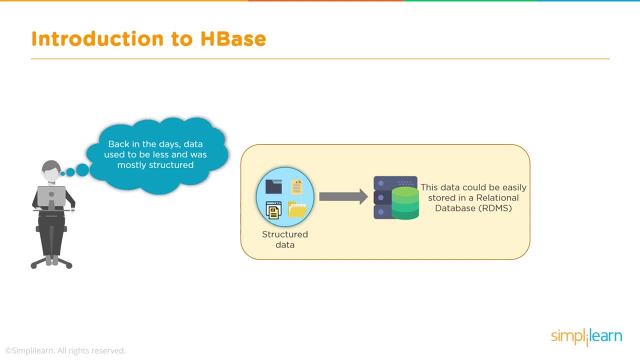 talk about relational database, you might think of Oracle, you might think of SQL, Microsoft, SQL, MySQL. All of these have evolved, even from back then, to do a lot more today than they did, but they still fall short in a lot of ways, and they're all examples of an RDBMS or relationship. 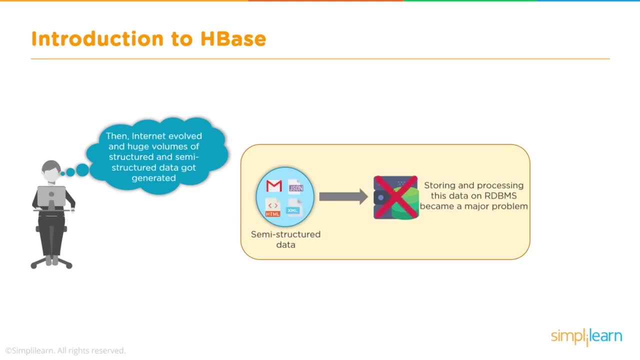 database. Then internet evolved and huge volumes of structured and semi-structured data got generated. You can see here, with the semi-structured data, we have email. If you look at my spam folder you know what we're talking about: All the HTML pages, XML, which a lot of times is. 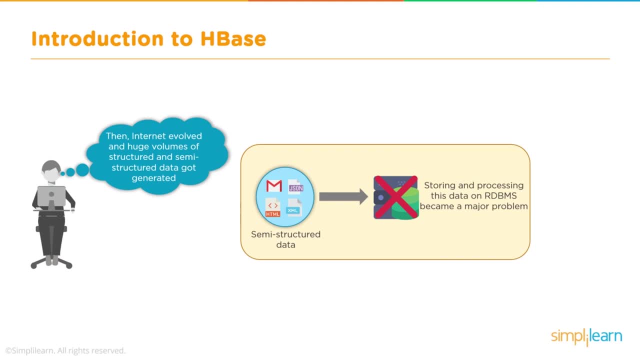 displayed on our HTML and help desk. All of this really has just even in the last. each year it almost doubles from the year before. how much of this is generated. So storing and processing this data on an RDBMS has become a 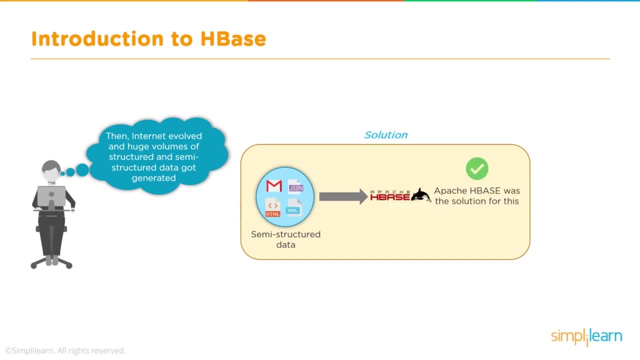 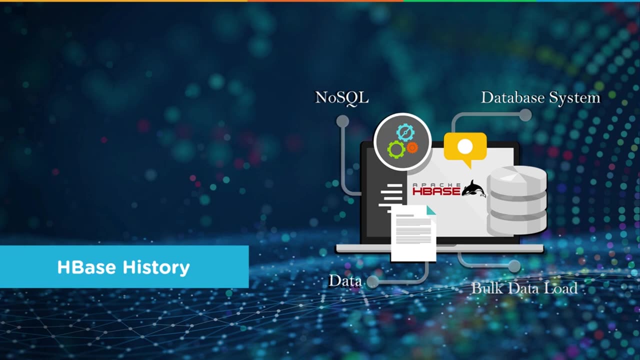 major problem, And so the solution is: we use Apache HBase. Apache HBase was the solution for this. Let's take a look at the history, the HBase history. When we look at the HBase history, we're going to start back in 2006,. November, Google released the paper. 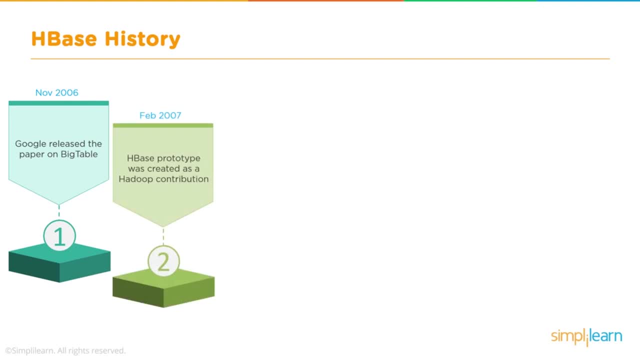 on Bigtable, And then in 2017, just a few months later- HBase prototype was created as a Hadoop contribution. Later on in the year 2007,, in October, first usable HBase along with the Hadoop 0.15 was released, And then in January of 2008,, HBase became 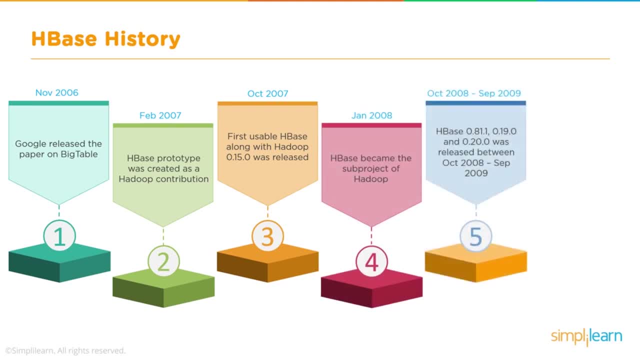 the sub-project of Hadoop. And later on that year, in October, all the way into September the next year, HBase was released, the 0.81 version, the 0.19 version and 0.20.. And for: 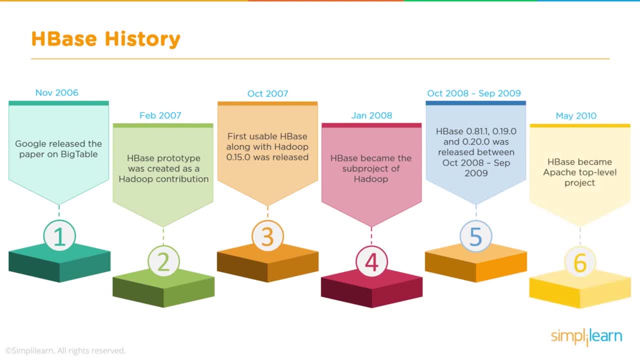 finally, in May of 2010,, HBase became Apache top level project, And so you can see, in the course of about four years, HBase started off as just an idea on paper and has evolved all the way till 2010 as a solid project under the Apache And since 2010, it's continued to evolve and 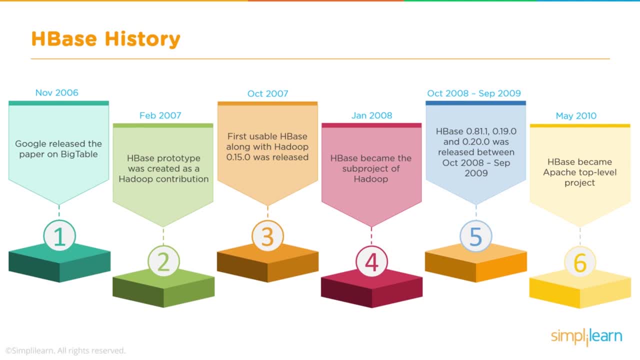 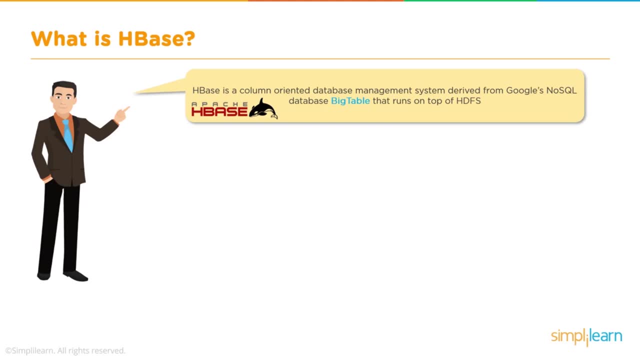 grow as a major source for storing data in semi-structured data. So what is HBase? HBase is a column-oriented database management system. It's derived from Google's NoSQL database, a big table that runs on top of the Hadoop. 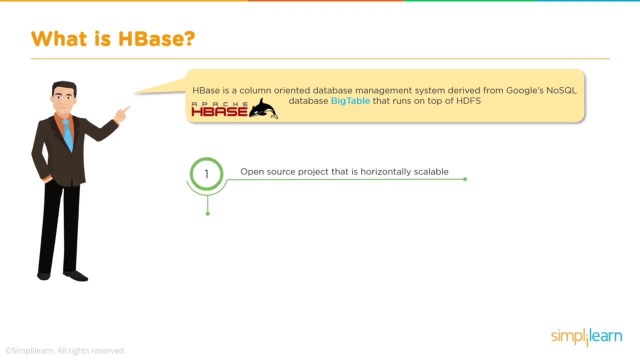 file system or the HDFS. It's an open source project that is horizontally scalable And that's very important to understand, that you don't have to buy a bunch of huge, expensive computers. You're expanding it by continually adding commodity machines And so it's a linear. 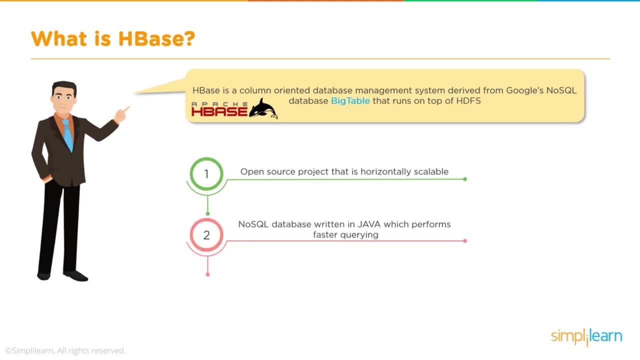 cost expansion as opposed to being exponential NoSQL database written in Java which permits faster querying. So Java is the back-end of the HBase setup And it's well suited for sparse data sets. So it can contain missing or NA values And this doesn't boggle it down like it would another database. 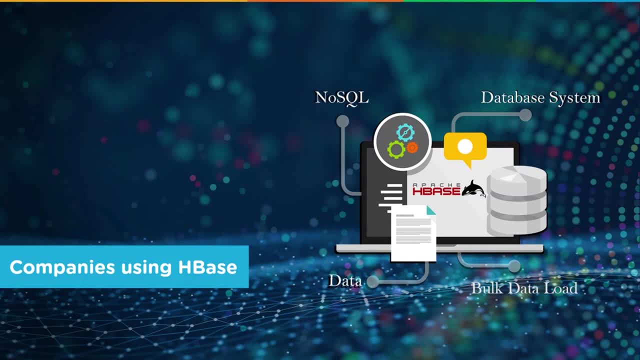 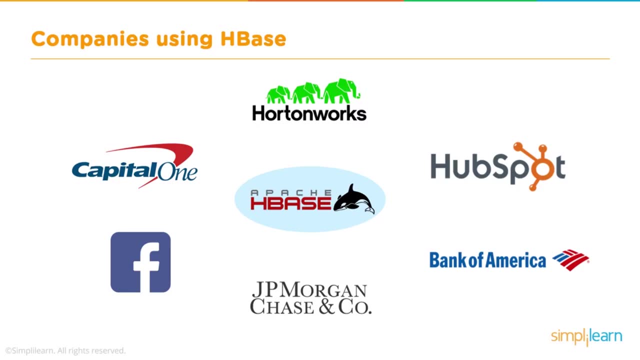 Companies using HBase. So let's take a look and see who is using this NoSQL database for their servers and for storing their data. And we have Hortonworks, which isn't a surprise because they're one of the like Cloudera Hortonworks. They are behind Hadoop and one. 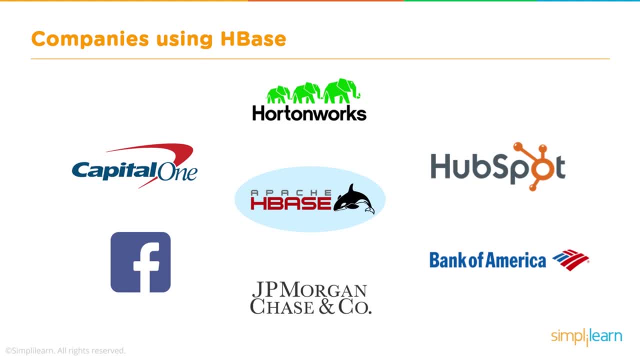 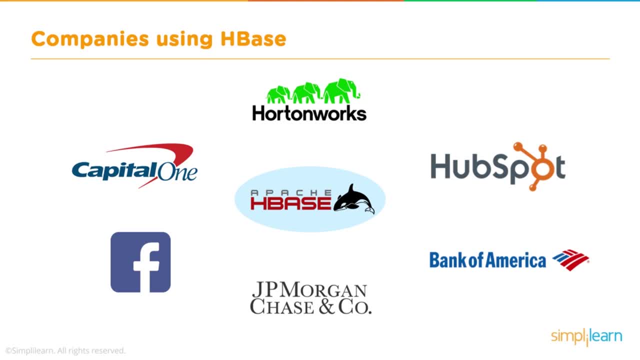 be the same. You have to understand the spread of information. That's the conflict between Japan being a Building HBase. These bloom stops from Japan via Apple22.. And some me guys have been that way too, And that is just your� throw. 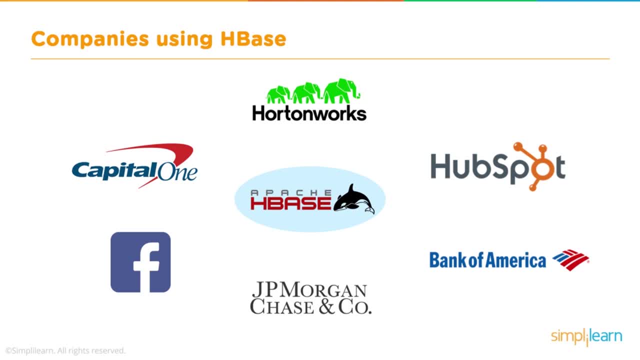 And our business is in Java, but you're looking for something you can find in here€哪 using it. Facebook, certainly, all of your Facebook, Twitter, most of your social medias are using it. and then, of course, there's JP Morgan Chase and company, another bank that uses the H base as their data warehouse for nose SQL. let's 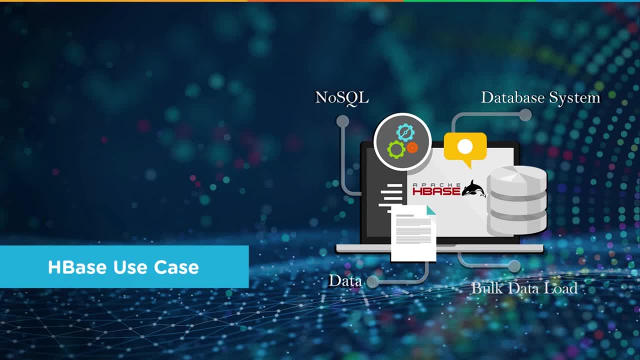 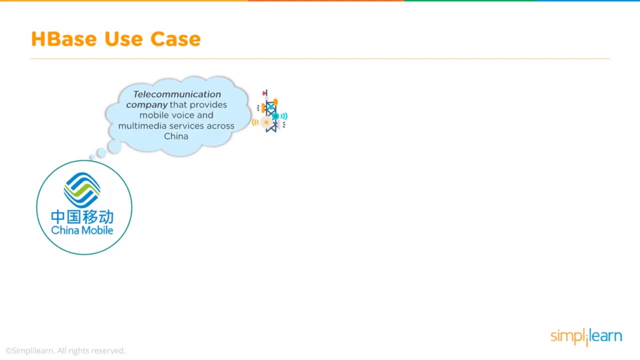 take a look at an H basic use case so we can dig a little bit more into it to see how it functions. telecommunication company that provides mobile voice and multimedia services across China, the China mobile and China mobile. they generate billions of call detailed records, or CDR, and so these CDRs and all 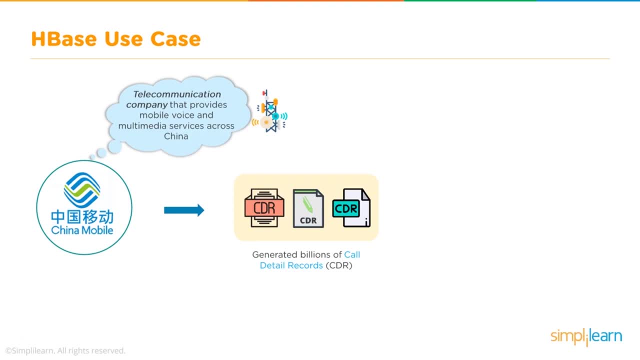 these records of these calls and how long they are, and different aspects of the call, maybe the tower they're broadcasted from. all of that is being recorded so they can track it. a traditional database systems were unable to scale up to the vast volumes of data and provide a cost-effective solution. no. 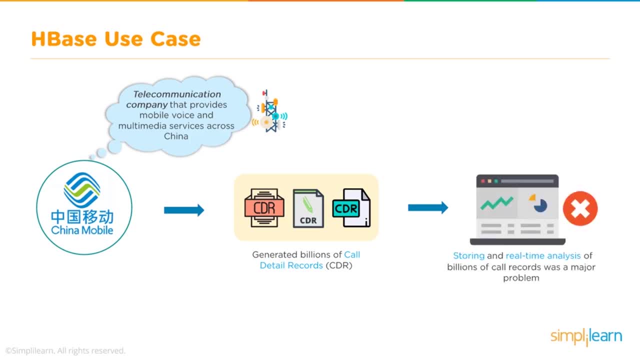 good. so storing in real-time analysis of billions of call records was a major problem for this company. solution: Apache HBase- HBase storage and storage in real-time was a major problem for this company. billions of rows of detailed call records. HBase performs fast processing of records using SQL queries so you can mix your SQL and no SQL queries and 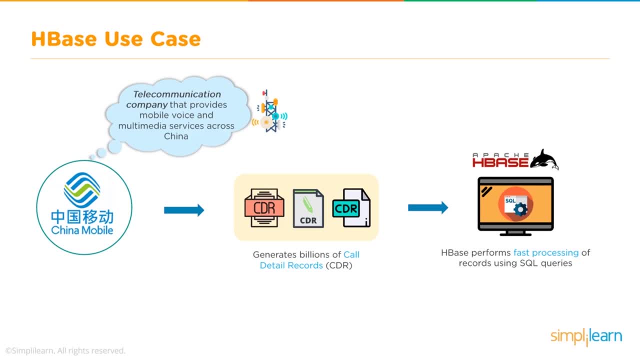 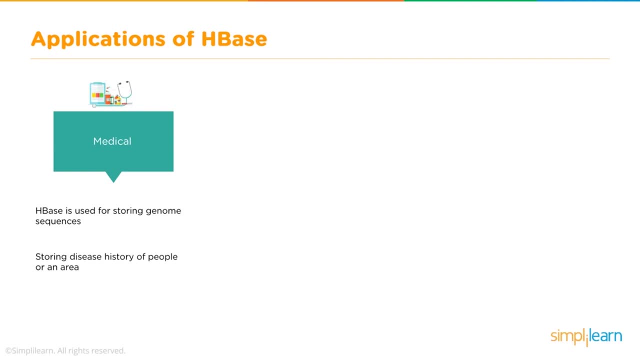 usually just say no SQL queries because of the way the query works. applications of HBase. one of them would be in the medical industry. HBase is used for storing genome sequences, storing disease history of people, of an area, and you can imagine how sparse that is as far as both of those a genome sequence might be. 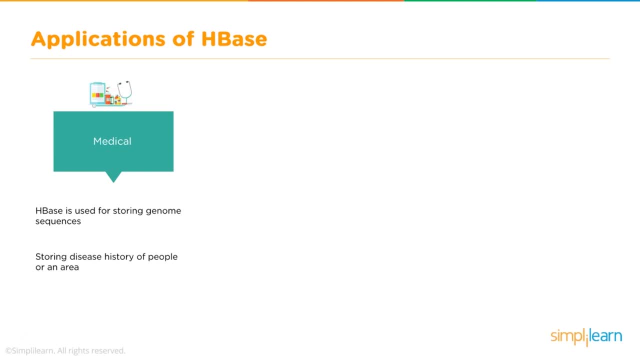 only have pieces to it that each person is unique or is unique to different people, and the same thing with disease. you really don't need a column for every possible disease a person could get. you just want to know what those diseases, those people have had to deal with. in that area, ecommerce HBase is used for. 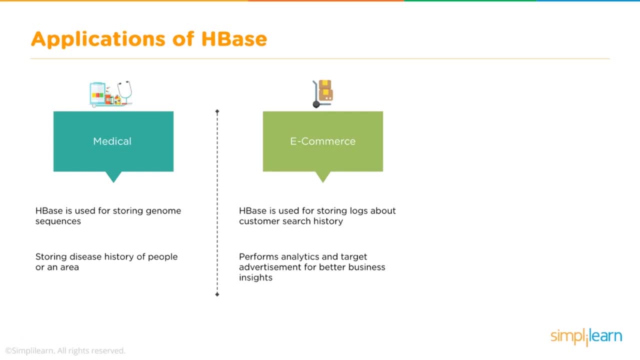 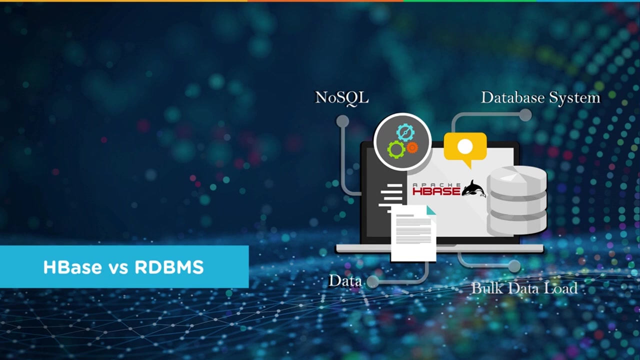 storing logs about customer search history. performs analytics and target advertisement for better business insights. sports HBase stores match details in the history of each match. uses this data for better prediction. so when look at HBase, we all want to know what. what's the difference between HBase versus RDBMS? that is a relational. 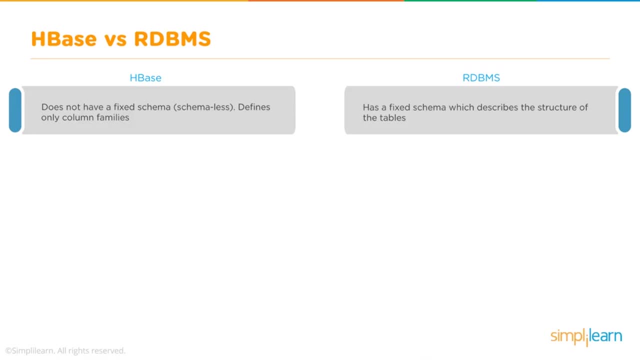 database management system, HBase versus RDBMS. so the HBase does not have a fixed schema, is schemaless, defines only column families, and we'll show you what that means later on. RDBMS has a fixed schema which describes the structure of the tables and you can think of this as you have a row and you have columns and 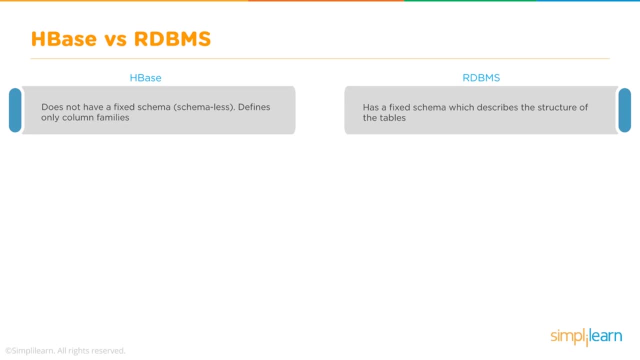 each column is a very specific structure: how much data can go in there and what it does with the HBase. it works like this well with structured and semi structured data. with the RDBMS it works only well with structured data. with the HBase it can have denormalized data. it 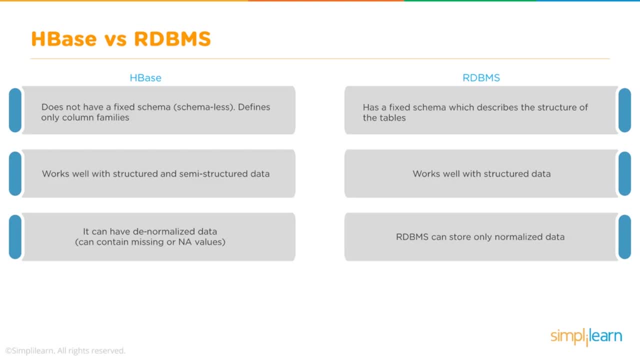 can contain missing or null values. with the RDBMS, it can store only normalized data. now you can still store a null value in the RDBMS, but it still takes up the same space as if you're storing a regular value in many cases, and it also 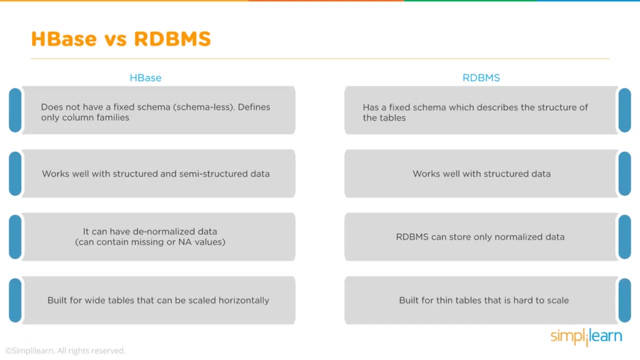 for the HBase is built for wide tables. it can be scaled horizontally. for instance, if you were doing a tokenizer of words and word clusters, you might have 1.4 million different words. you're pulling up and combinations of words, so with an RDBMS spelled for thin tables that are hard to scale. 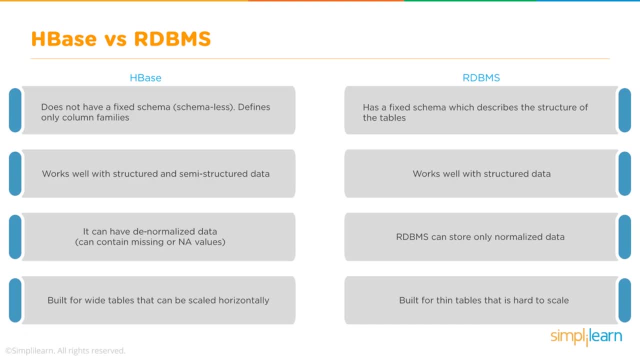 you don't want to store 1.4 million columns in your SQL. it's going to crash. it's going to be very hard to do searches with the HBase. it only stores that data which is part of whatever row you're working on. let's look at some of the features of the HBase. it's scalable. data can be scaled to. 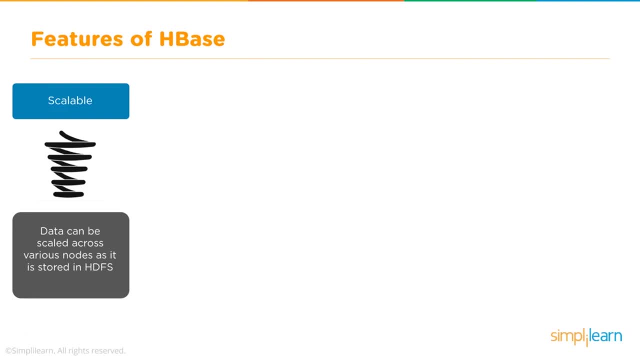 various nodes as it is stored in the HDFS and I always think about this. it's a linear add-on. for each terabyte of data, I'm adding on roughly $1,000 in commodity computing. with an enterprise machine we're looking at about 10,000 at. 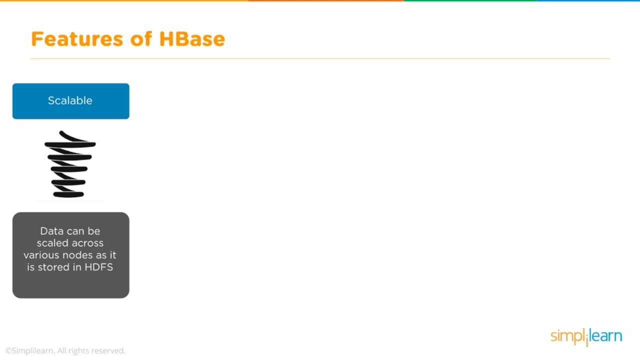 the lower end for each terabyte of data, and that includes all your backup and redundancy, so it's a big difference. it's like a tenth of the cost to store it across the HBase. it has automatic failure support right ahead: log across clusters, which provides automatic support against failure, consistent read. 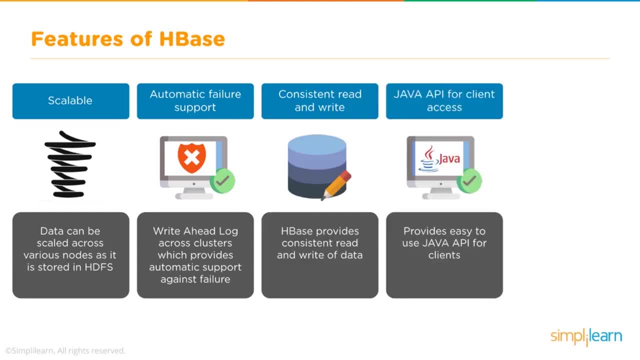 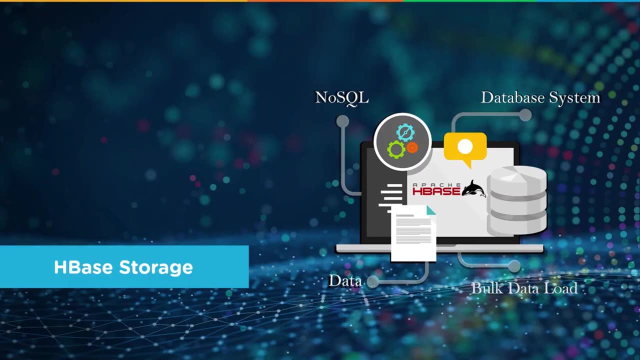 and write HBase provides consistent read and write of the data. it's a Java API for client access. provides easy to use Java API for clients, block cache and bloom filters. so the HBase supports block caching and bloom filters for high volume query optimization. let's dig a little deeper into the HBase storage. 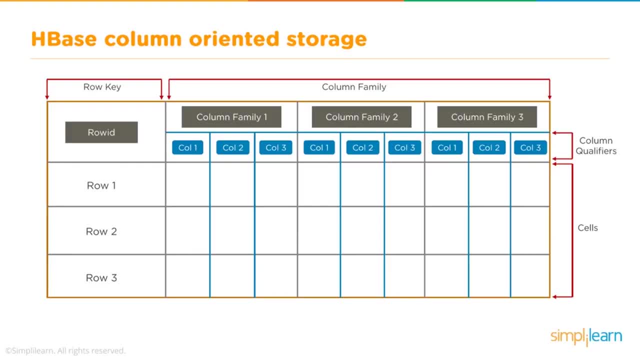 HBase column oriented storage- and I told you we're gonna look into this to see how it stores the data- and here you can see you have a right-hand column oriented storage and here you can see you have a right-hand row key. this is really one of the important references is each row has to. 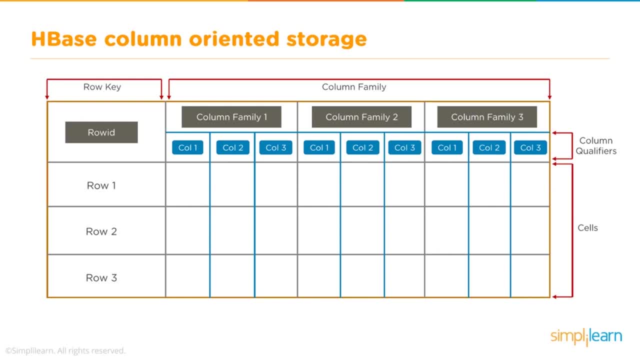 have its own key or your row ID, and then you have your column family and in here you can see we have column family 1, column family 2, column family 3 and you have your column qualifiers. so you can have in column family 1, you can have. 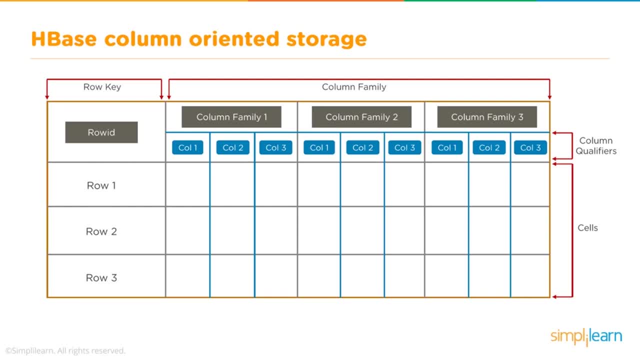 three columns in there and there might not be any data in that. so when you go into column family 1 and do a query for every column that contains a certain thing, that row might not have anything in there and not be queried where. in column family 2 maybe you have column 1. 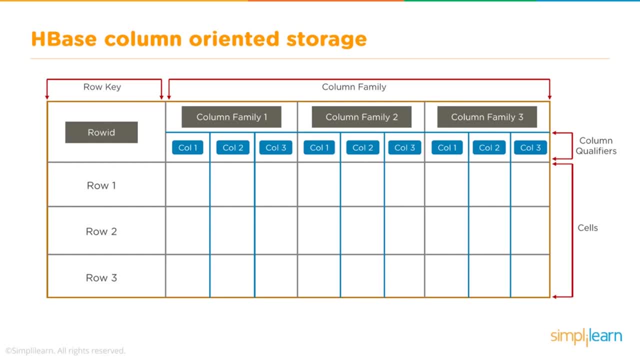 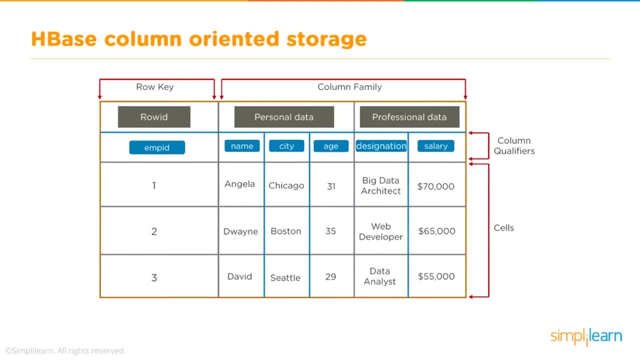 filled out, and column 3 filled out, and so on and so forth, and then each cell is connected to the row where the data is actually stored. let's take a look at this and what it looks like when you fill the data in. so in here we have a. 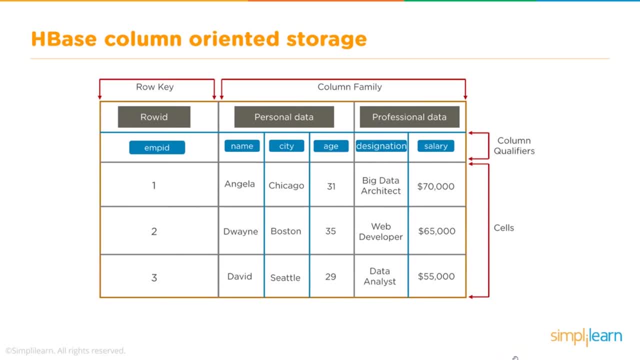 row key with a row ID and we have our employee ID. 1, 2, 3. that's pretty straightforward. you probably would even have that on an SQL server. and then you have your column family. this is where it starts really separating out. your column family might have personal data and under personal data you would have name. 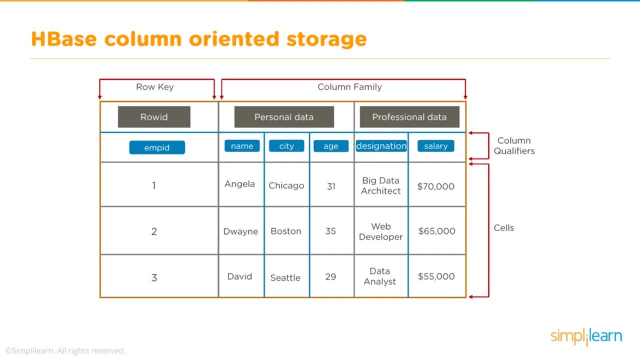 city age. you might have a lot of data in there, and you might have a lot of data in there and under personal data you would have name, city age. you might have a lot more than just that. you might have number of children, you might have degree, all those kinds of different things that go under personal data, and some of them. 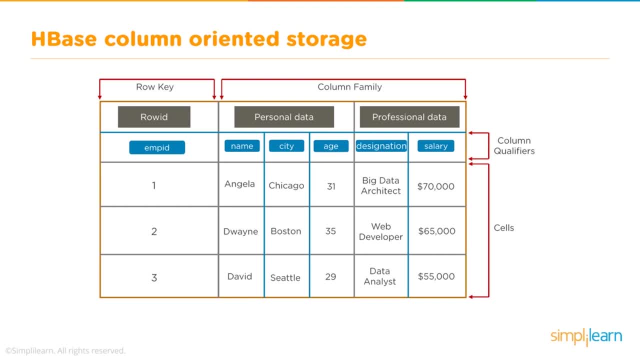 might be missing. you might only have the name and the age of an employee. you might only have the name, the city and how many children, and not the age, and so you can see. with the personal data you can now collect a large variety of data and store it in the age space very easily, and then maybe you have a family. 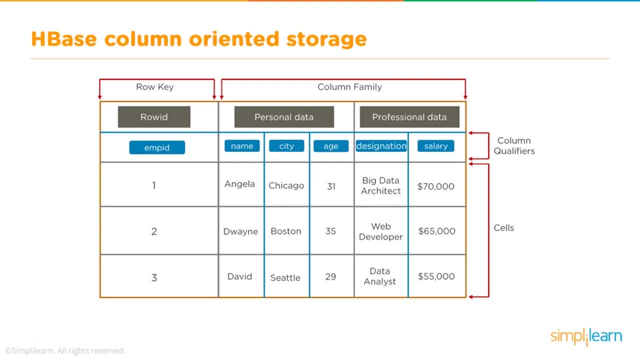 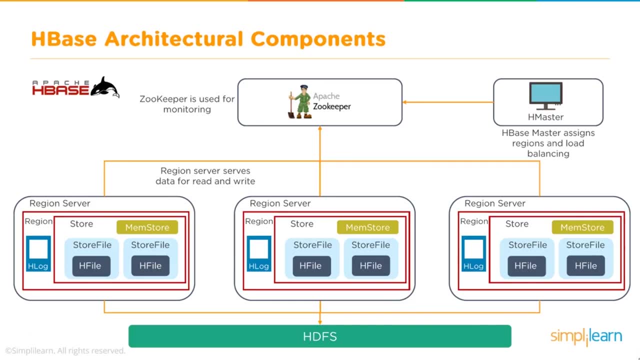 of professional data, your designation, your salary, all the stuff that the employee is doing for you in that company. Let's dig a little deeper into the HBase architecture And so you can see here what looks to be a complicated chart. It's not as complicated as you think. From the Apache HBase we have the 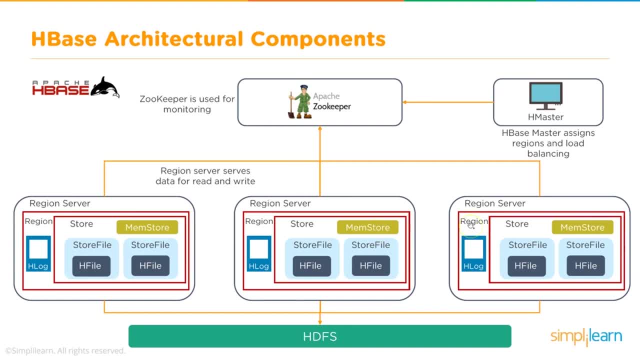 Zookeeper, which is used for monitoring what's going on, And you have your HMaster. This is the HBase master assigns regions and load balancing. And then underneath the region or the HBase master, then under the HMaster or HBase master, you have your ReaderServerServes data for read. 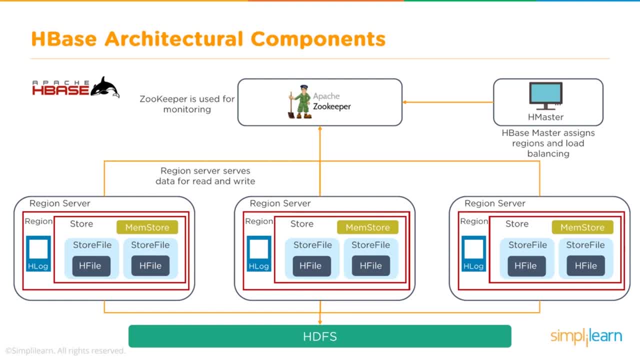 and write And the RegionServer, which is all your different computers you have in your Hadoop cluster. you'll have a region, an HLog, you'll have a store, memory store, and then you have your different files for HFile that are stored on there And those are separated across the. 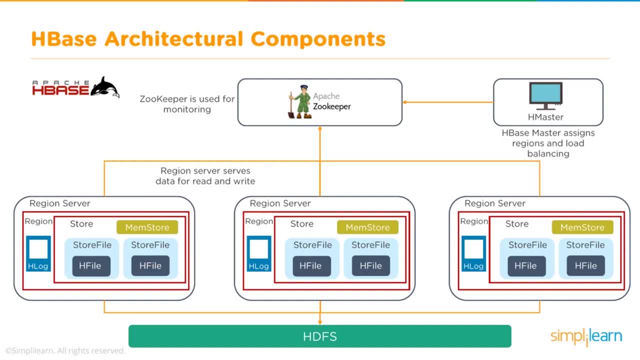 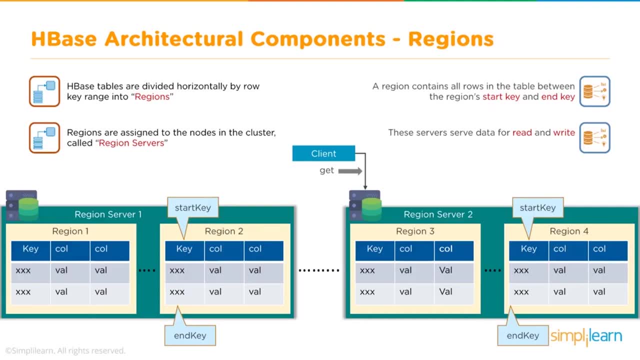 different computers And that's all part of the HDFS storage system. So when we look at the architectural components or regions and we're drilling down a little bit, HBase tables are divided horizontally by a row, So you have a key range into regions. So each of those IDs 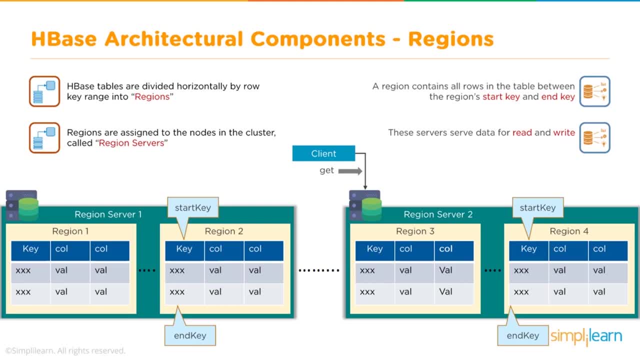 you have a key range into regions. So each of those IDs you have a key range into regions. You might have IDs 1 to 20,, 21 to 50, or whatever they are. Regions are assigned to the nodes in the 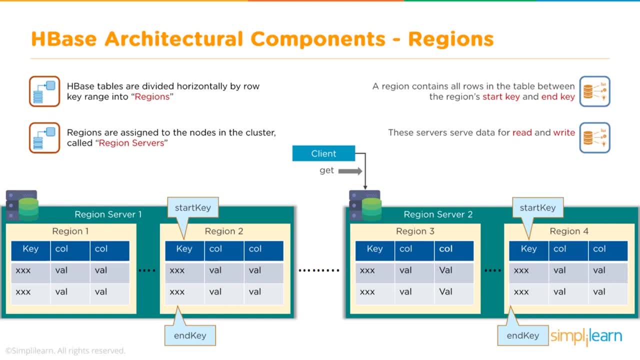 cluster called RegionServers. A region contains all rows in the table between the region's start key and the end key, Again 1 to 10,, 11 to 20, and so forth. These servers serve data for read and write And you can see, here we have the client and the get, and the get sends it out and it finds. 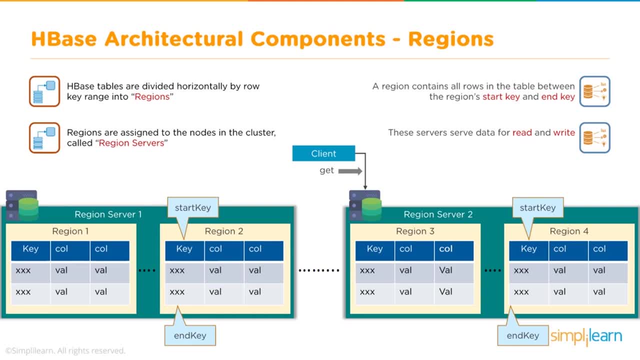 out where that start, if it's between which start keys and end keys, and then it pulls the data from that different region server. And so you can see, here we have the client and the get and the get sends it out and it pulls the data from that different region server. And so you can see, here we 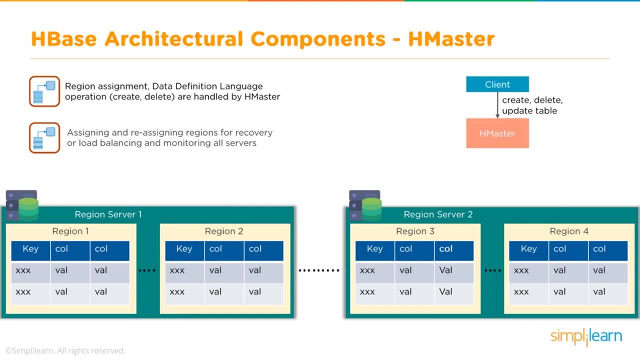 have the client and the get sends it out and it pulls the data from that different region server. So the region sign, data, definition, language operation, create, delete are handled by the HMaster. So the HMaster is telling it: what are we doing with this data? what's going out there? 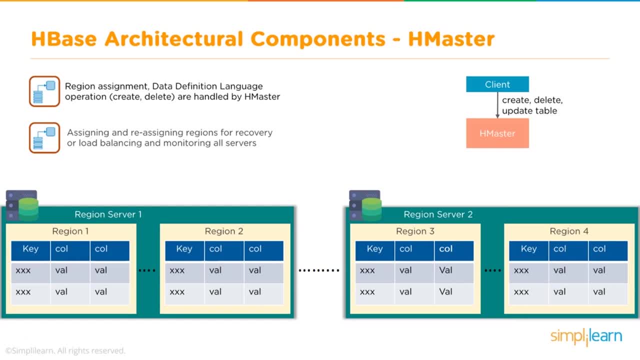 Assigning and reassigning, regions for recovery or load balancing and monitoring all servers. So that's also part of it. So you know if your IDs, if you have 500 IDs across three servers, you're not going to put 400 IDs on server 1 and 100 on server 2 and leave region 3 and region 4. 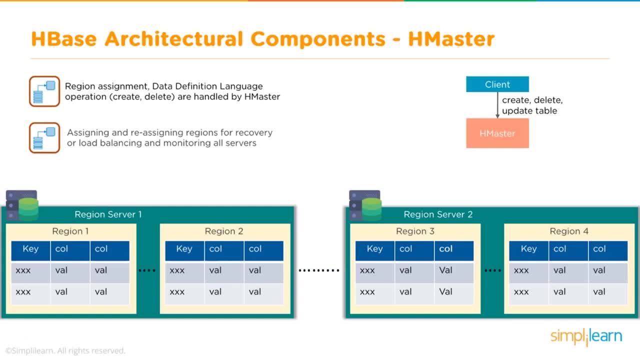 empty. You're going to split that up And that's going to be a lot of work. So you're going to, And you can see here: it monitors region servers, assigns regions to region servers, assigns regions to region servers, and so forth and so forth. HBase has a distributed environment where HMaster. 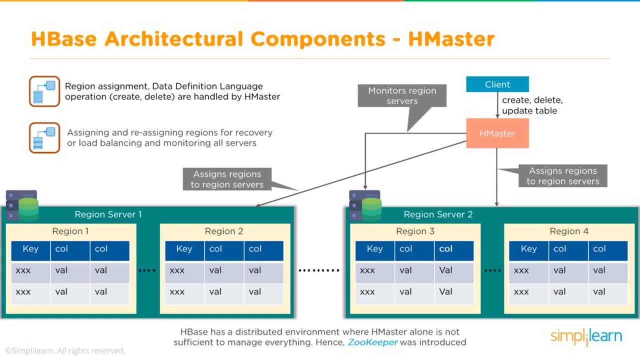 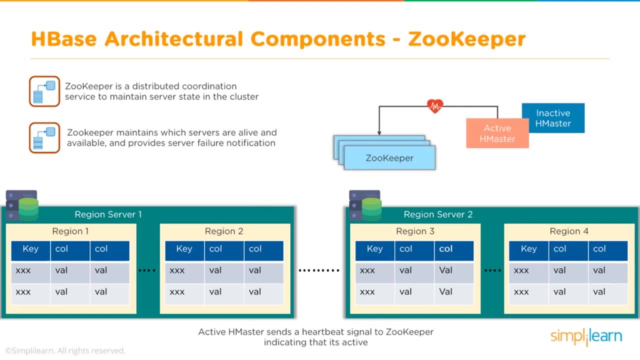 alone is not sufficient to manage everything. Hence ZooKeeper was introduced, It works with HMaster. So you have an active HMaster which sends a heartbeat signal to ZooKeeper indicating that it's active, And the ZooKeeper also has a heartbeat to the region servers, So the region servers send. 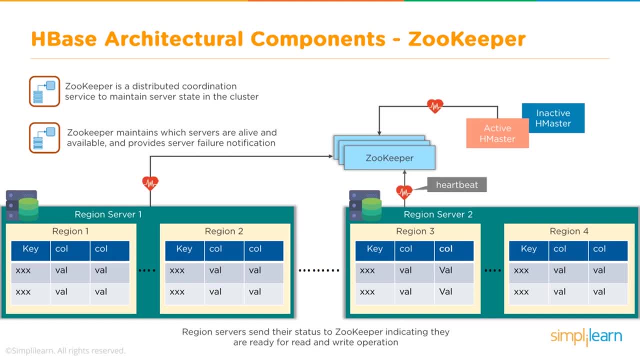 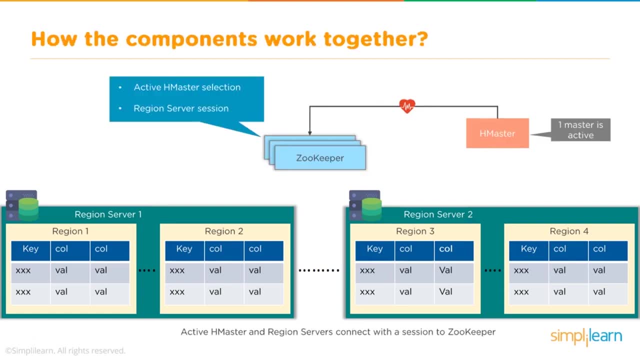 their status to the region servers, And so you can see here it monitors region servers, assigns regions to ZooKeeper, indicating they are ready for read and write operation. Inactive server acts as a backup. If the active HMaster fails, it'll come to the rescue. Active HMaster and region servers. 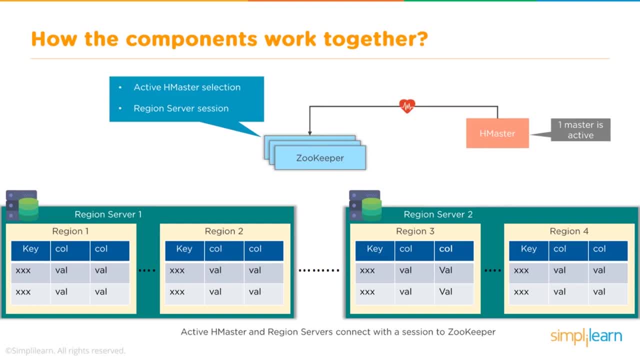 connect with a session to ZooKeeper So you see your active HMaster selection region server session. They're all looking at the ZooKeeper keeping that pulse. An active HMaster and region server connects with a session to the ZooKeeper And you can see here where we have ephemeral nodes. 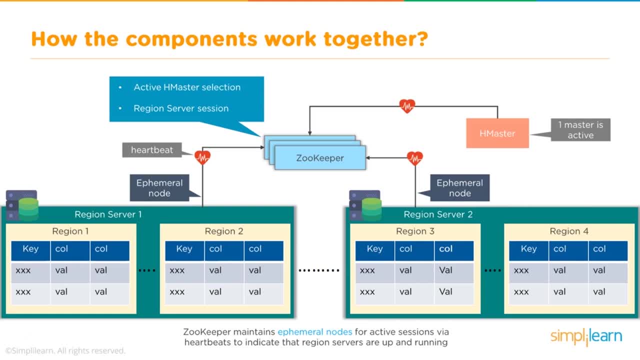 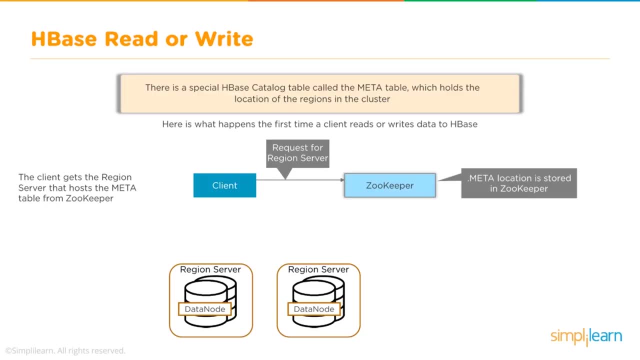 for active sessions via heartbeats to indicate that the region servers are ready for read and write operation. So let's take a look at HBase read or write going on. There's a special HBase catalog table called the meta table, which holds the location of the regions in the cluster. Here's: 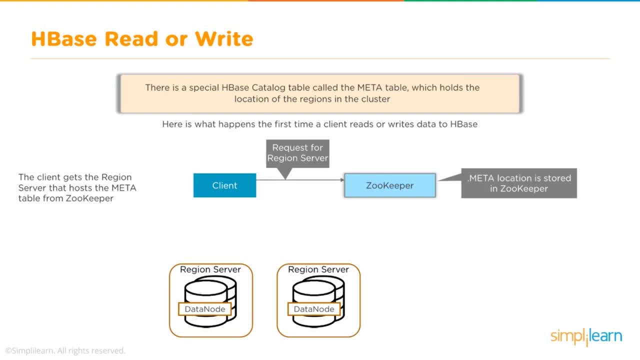 what happens: the first time a client reads or writes data to HBase, The client gets the region server, the host, the meta table from ZooKeeper And you can see right here the client has a request for your region server and goes: hey, ZooKeeper, can you handle this? The ZooKeeper. 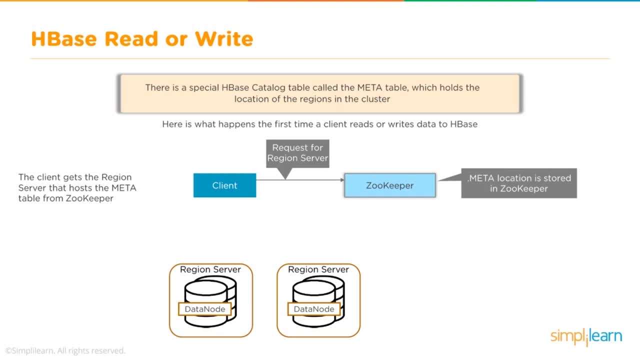 takes a look at it and goes, ah, meta location is stored in ZooKeeper, So it looks at its meta data on there And then the meta data table location is sent back to the client. The client will query the meta server to get the region server corresponding to the row key if it wants to access The client. 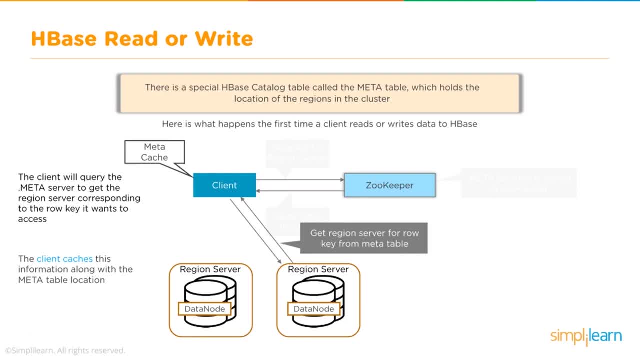 caches this information along with the meta table location, And you can see here the client going back and forth to the region server with the information And it might be going across multiple region servers, depending on what you're querying. So we get the region server for row key from the 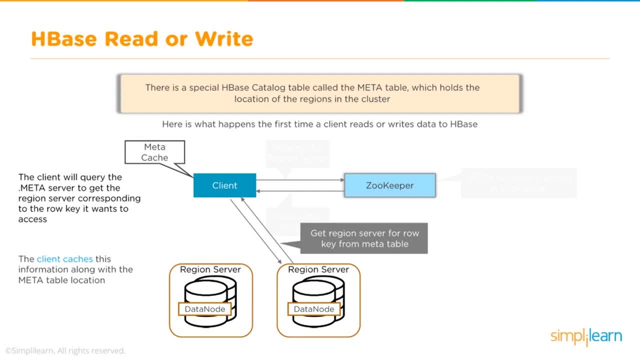 meta table. That's where that row key comes in and says, hey, this is where we're going with this, And so once it gets a row key from the corresponding region server, we can now put row or get row from that region server. Let's take a look at the HBase meta table, special HBase catalog table that 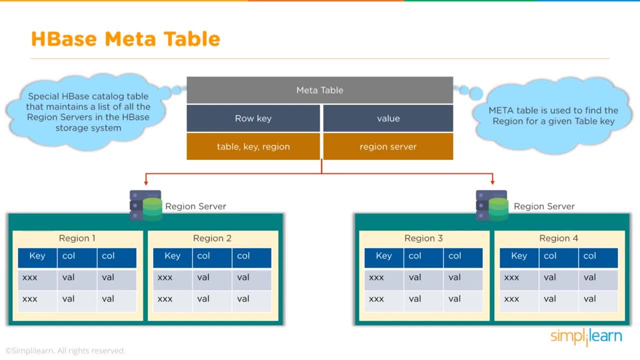 maintains a list of all the region servers in the HBase storage system. So you see, here we have the meta table. We have a row key and a value table key: region region server. So the meta table is used to find the region for the given table key And you can see down here, you know, a meta table. 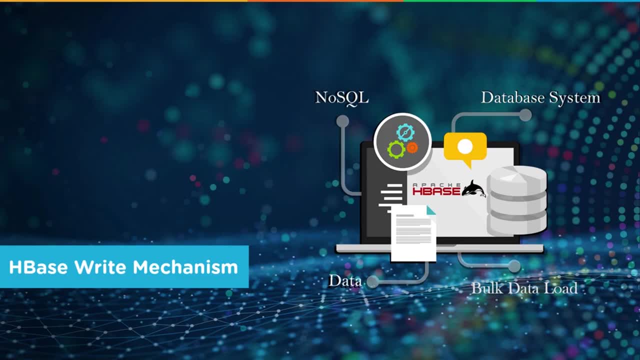 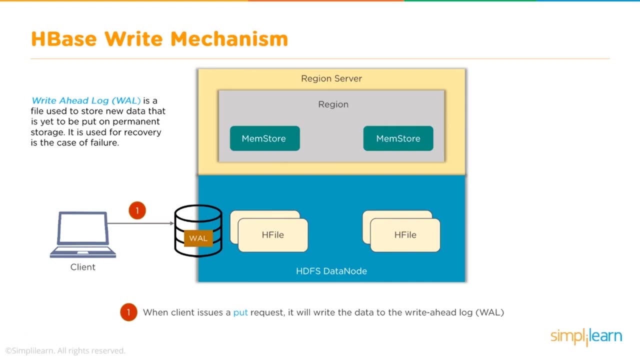 comes in, It's going to figure out where it's going with the region server And we look a little closer at the write mechanism in HBase. We have write ahead log, or wall as you abbreviate it, kind of a way to remember. wall is write ahead log, It's a file. 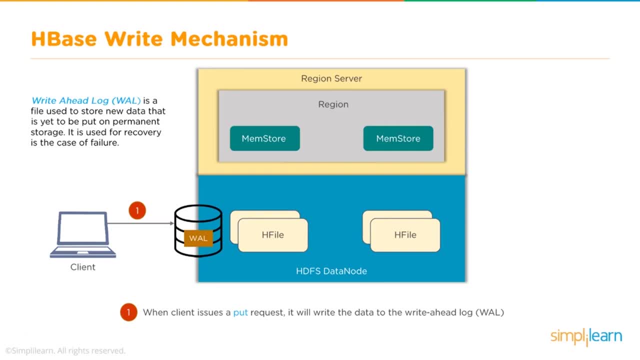 used to store new data that is yet to be put on permanent storage. It is used for recovery in the case of failure, So you can see here where the client comes in and it literally puts the new data coming in into this kind of temporary storage or the wall on there Once it's gone into the wall. 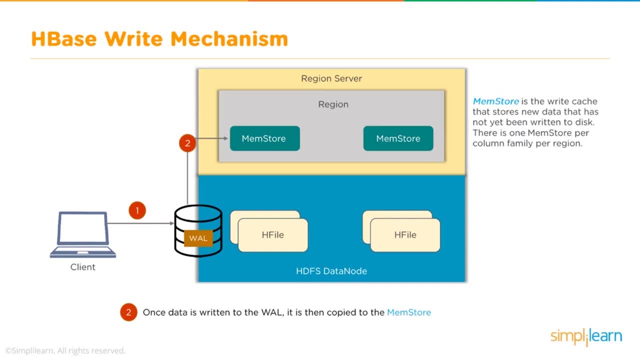 then the memory store. mem store is the write cache. It stores the new data that has not yet been written to disk. There is one mem store per column, family, per region And once we've done that we have three ACK Once the data is placed in mem. 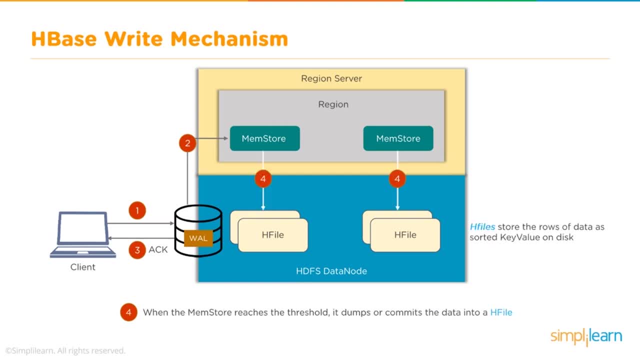 store. the client then receives the acknowledgement. When the mem store reaches the threshold it dumps or commits the data into H file. So you can see, right here we've taken our. it's gone into the wall. The wall then sorts it into the different memory stores And then the memory stores it. 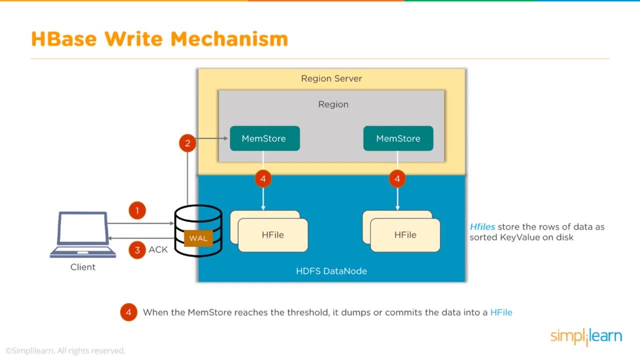 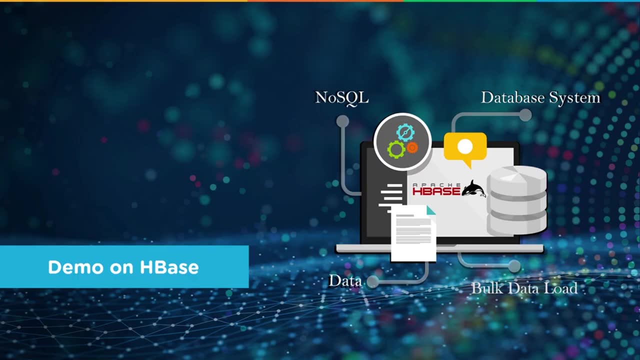 says, hey, we've reached, we're ready to dump that into our H files. And then it moves it into the H file. H files store the rows of data as stored key value on disk. So here we've done a lot of theory. 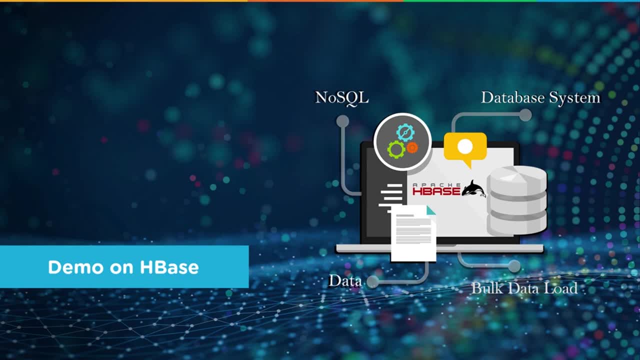 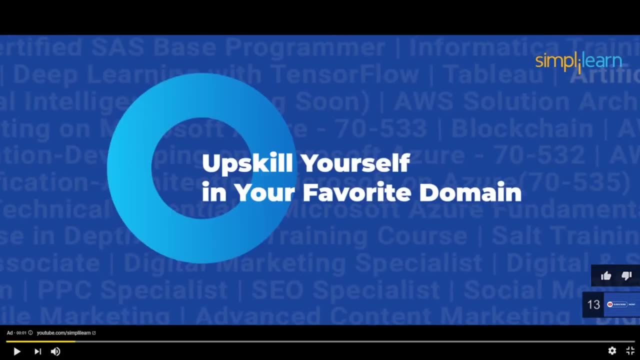 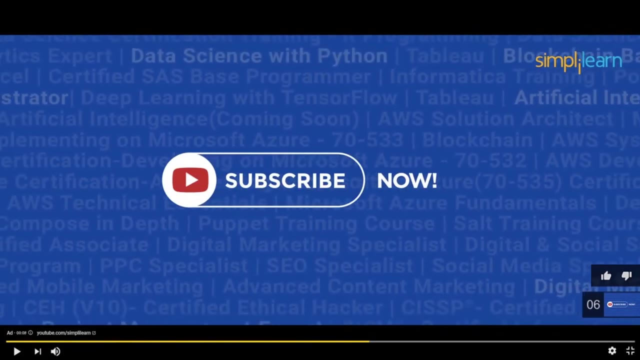 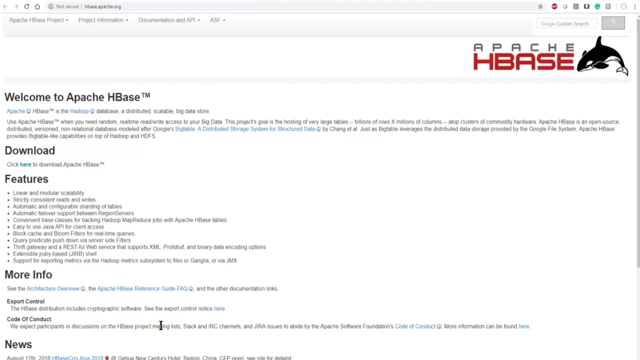 Let's dive in and just take a look and see what some of these commands look like and what happens in our H base when we're manipulating a no SQL setup. So if you're learning a new setup, it's always good to start with. where is this coming from? It's open. 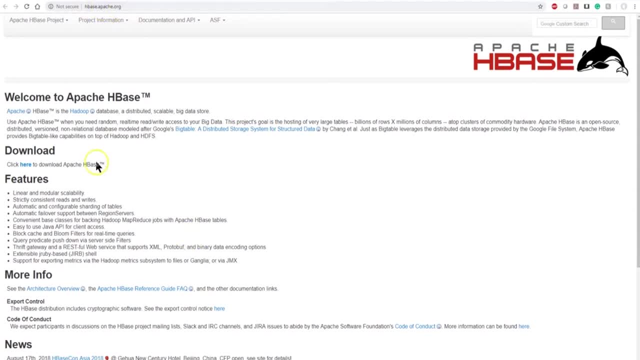 source by Apache And you can go to hbaseapacheorg and you'll see that it has a lot of information. You can actually download the H base separate from the Hadoop, Although most people just install the Hadoop because it's bundled with it And if you go in here you'll find a reference guidance You can. 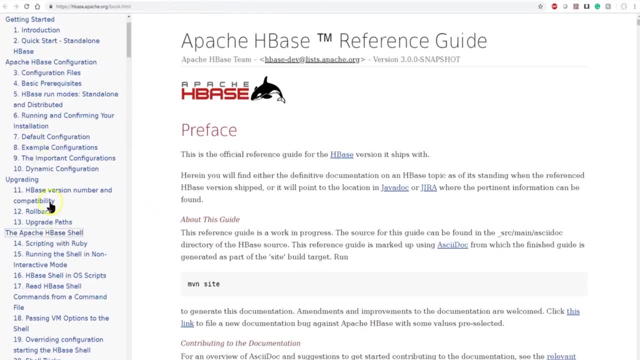 go through the Apache reference guide and there's a number of things to look at, but we're going to be going through Apache H base shell. That's what we're going to be working with And there's a lot of other interfaces on the setup and you can look up a lot of the different commands on. 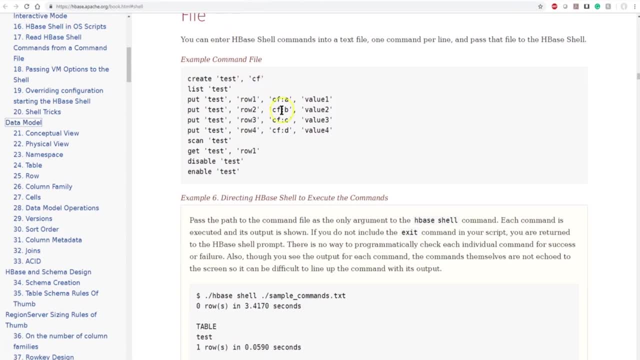 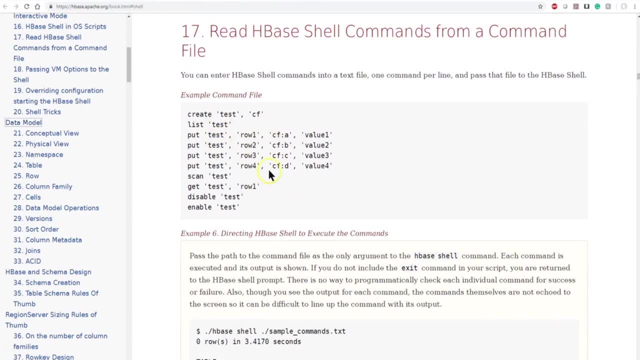 here. so we go into the Apache HBase reference guide. we can go down to read HBase shell commands from a command file. you can see here where it gives you different options of formats for putting the data in and listing the data. certainly can also create files and scripts to do this too, but we're gonna. 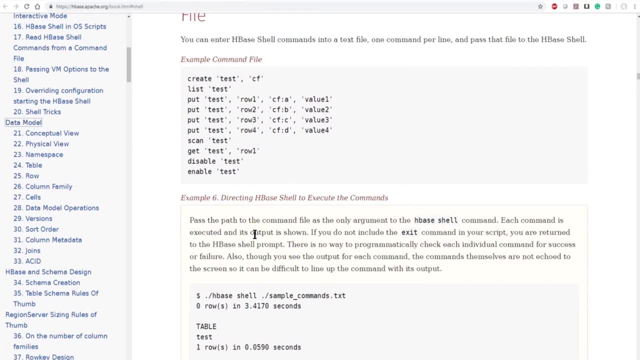 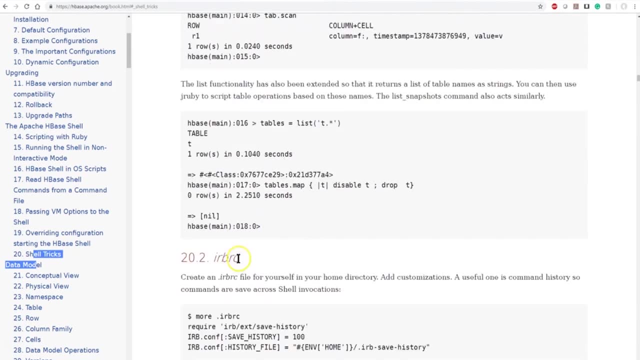 look at the basics. we're gonna go through this on a basic HBase shell, and one last thing to look at is, of course, if you continue down the setup, you can see here where they have more detail as far as how to create and how to get to. 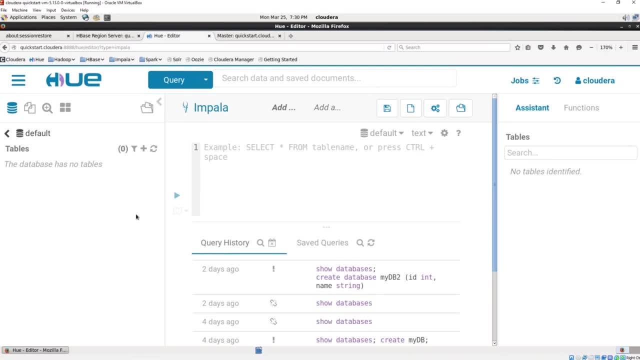 your data on your HBase. now I will be working in a virtual box and this is by Oracle. you can download the Oracle virtual box. you can put a note in below for the YouTube, as we did have a previous session on setting up virtual setup to run your Hadoop system. in there I'm using the Cloudera quickstart. 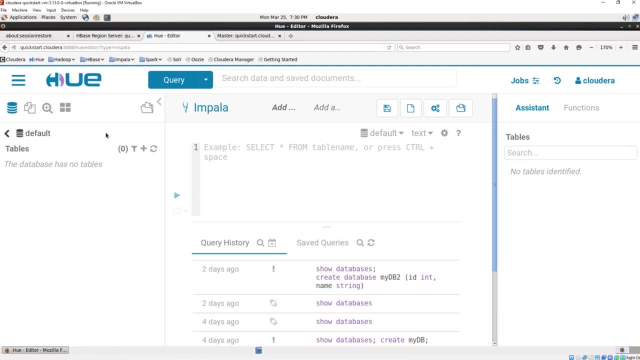 installed in here. there's Horton's. you can also use the Amazon WebService. there's a number of options for trying this out. in this case, we have Cloudera's spiritual land right here, so that would be added next to my cube. and here is the Cloud Area, quikstart, and it's taking out a lot of data and Automata. 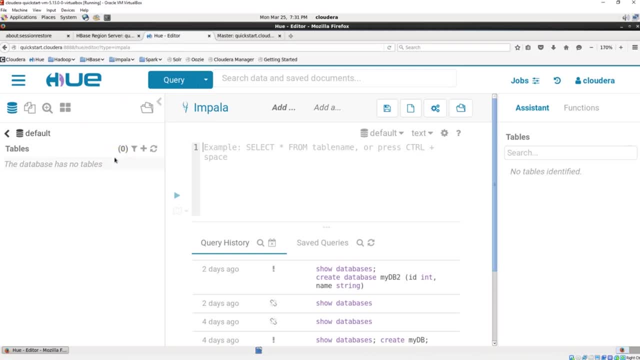 on the Oracle VirtualBox. The VirtualBox has Linux CentOS installed on it and then the Hadoop. It has all the different Hadoop flavors, including HBase, And I bring this up because my computer is a Windows 10.. The operating system of the VirtualBox is Linux and we're looking at the 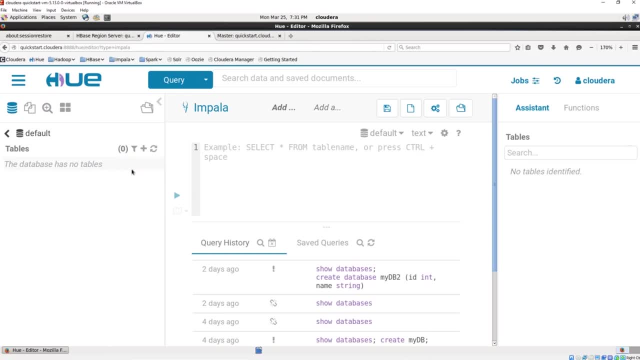 HBase data warehouse And so we have three very different entities all running on my computer And that can be confusing if it's the first time in and working with this kind of setup. Now you'll notice in our Cloudera setup they actually have some HBase monitoring, So I can go. 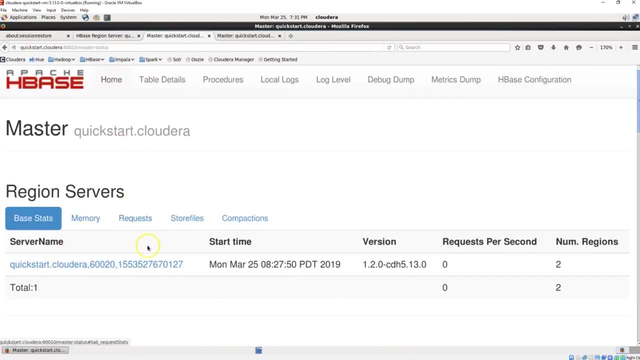 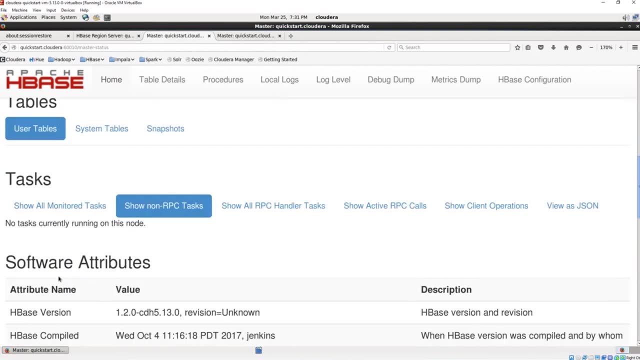 underneath here and click on HBase and master And it'll tell me what's going on with my region servers. It'll tell me what's going on with our backup tables. Right now I don't have any user tables because we haven't created any, And this is only a single node and a single HBase store. 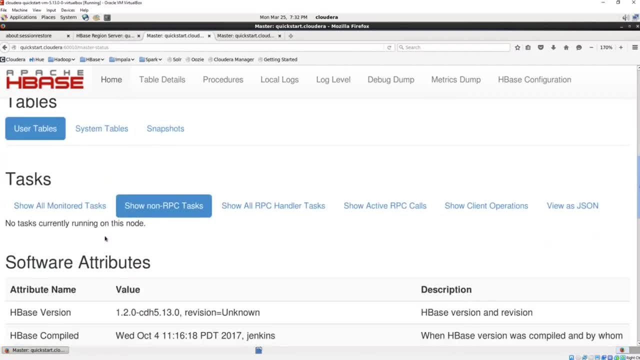 So you're not going to expect anything too extensive in here, since this is for practice and education and perhaps testing out package you're working on. It's not for really you can deploy it. It's not for really you can deploy it. It's not for really you can deploy it. 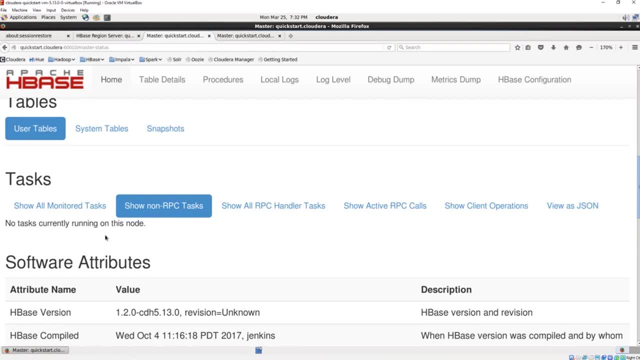 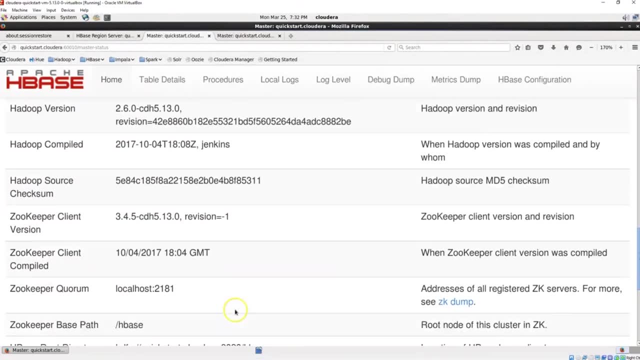 You can deploy Cloudera, of course, But when you talk about a quick start or a single node setup, that's what it's really for. So we can go through all the different HBase and you'll see all kinds of different information with ZooKeeper. If you saw it, flash by down here what version we're. 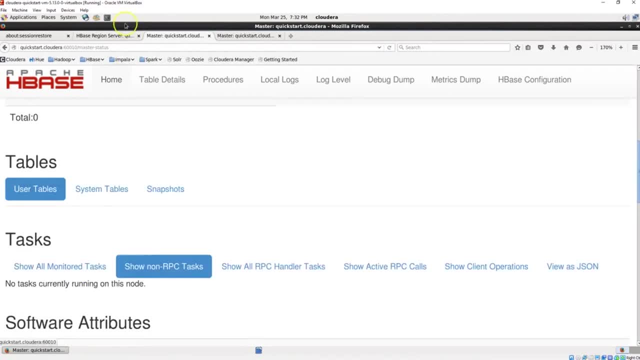 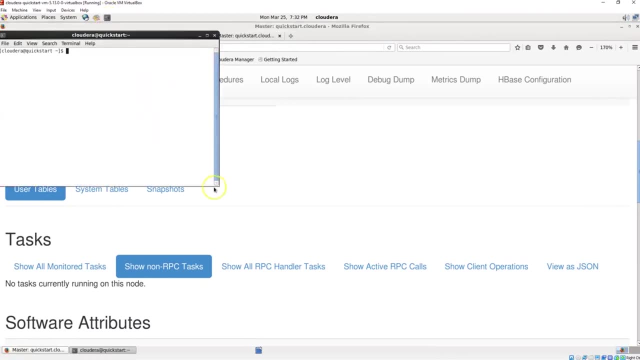 working in, since ZooKeeper is part of the HBase setup. Where we want to go is we want to open up a terminal window, And in Cloudera it happens to be up at the top And when you click on here you'll see your Cloudera terminal window open. And let me just expand this: We have a nice full 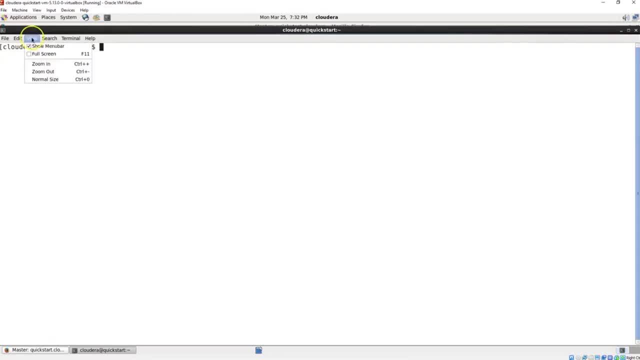 screen And then I'm also going to zoom in. That way I have a nice big picture and you can see what I'm typing and what's going on. And to open up your HBase shell, simply type HBase shell to get in and hit enter And you'll see it takes just a. 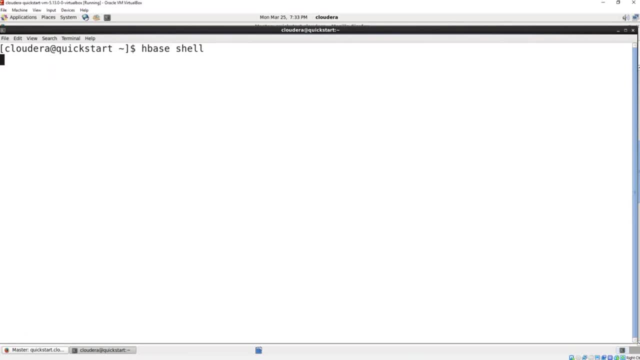 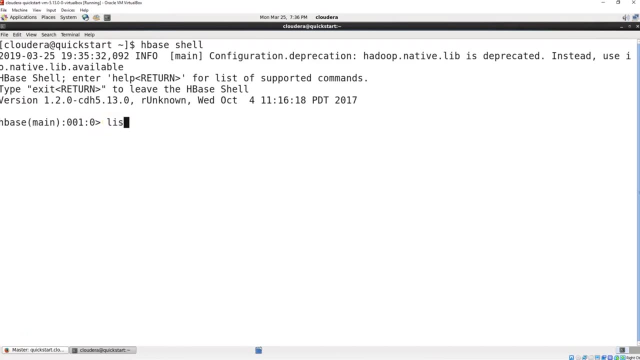 moment to load And we'll be in our HBase shell for doing HBase commands. Once we've gotten into our HBase shell, you'll see you'll have the HBase prompt information ahead of it. We can do something simple like list, And this is going to list whatever tables we have, And it so happens. 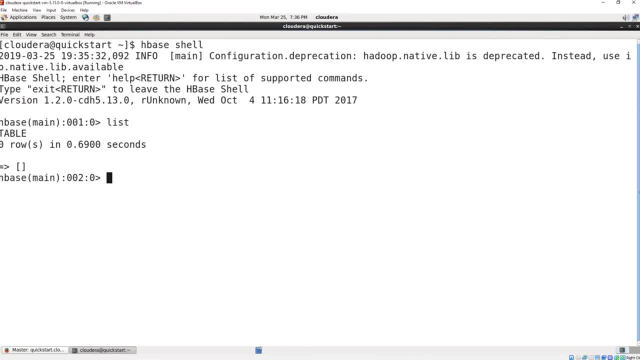 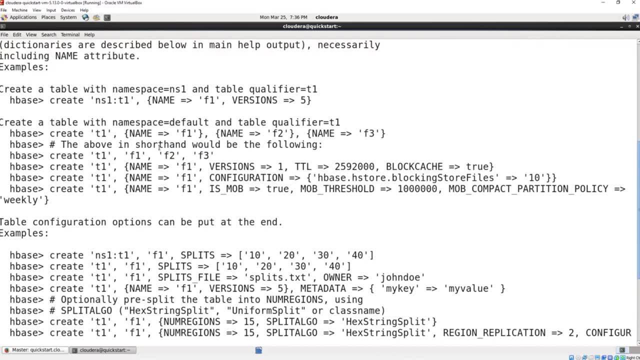 that there's a base table that comes with HBase. Now we can go ahead and create, And I'm going to type in, just create. What's nice about this is it's going to throw me kind of a. it's going to say, hey, there's no, just straight create. But it does come up and tell me all these. 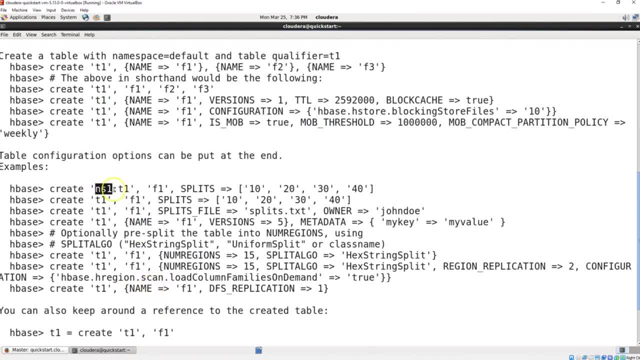 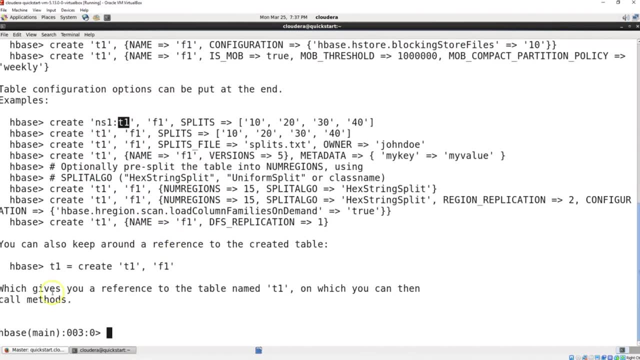 different formats we can use for create. So we can create our table and one of our families. You can add splits, names, versions, all kinds of things you can do with this. But let's just start with a very basic one on here And let's go ahead and create And we'll 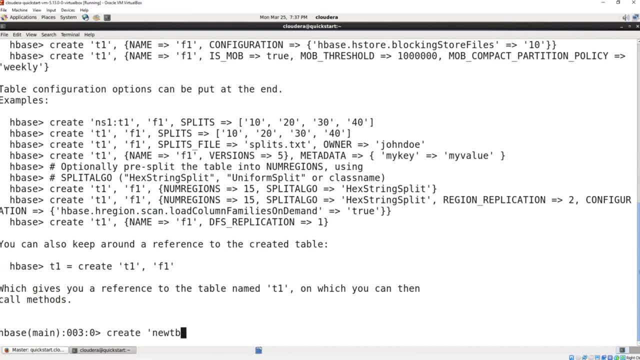 call it new table. Let's just call it new TBL for table, new table. And then we also want to do- let's just take a look at this: I'm creating a new table and it's going to have a family of. 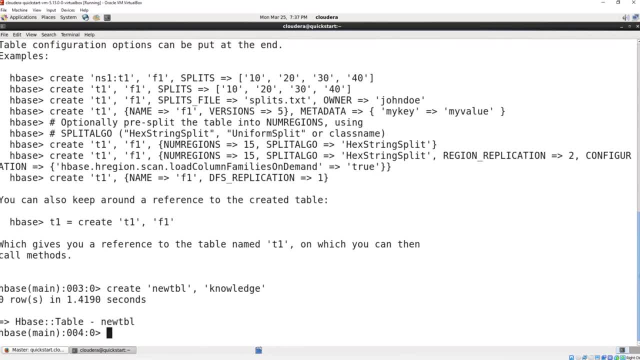 knowledge in it And let me hit enter, It's going to come up. It's going to take it a second to go ahead and create it. Now we have our new table in here, So if I go list, you'll now see table and. 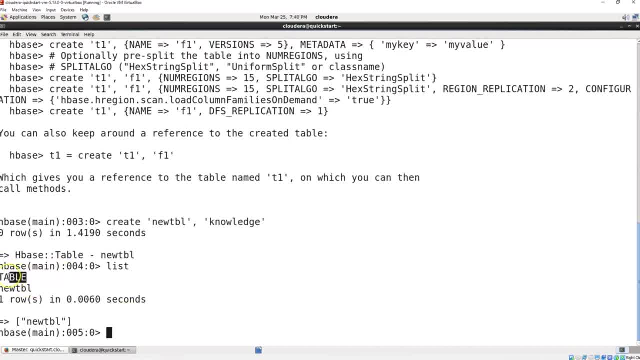 new table. So you can now see that we have the new table and, of course, the default table that's set up in here And we can do something like describe, We can describe, and then we're going to do new TBL And when we describe it it's going to come up. It's going to say: hey name, I have knowledge. 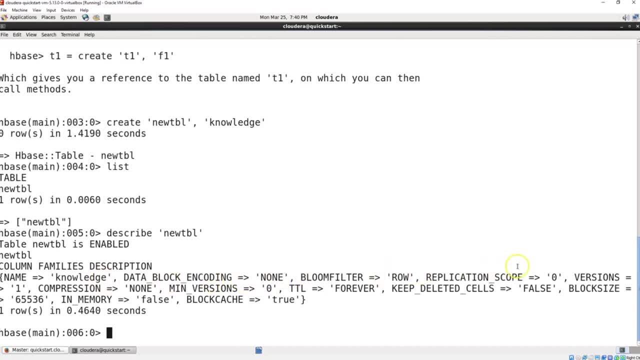 data block encoding none. bloom filter, row replication, scope, version, all the different information you need, New minimum version, zero, forever deleted cells, false block size in memory, And you can look this stuff up on apacheorg to really track it down. 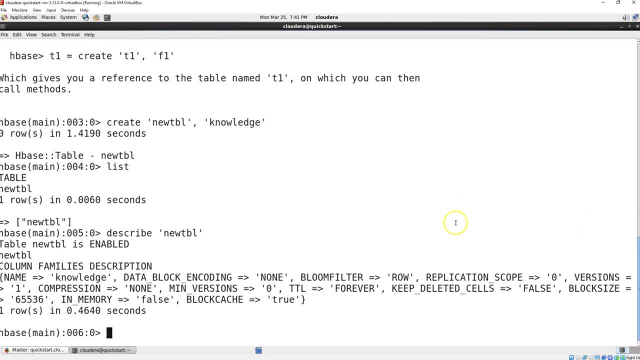 One of the things that's important to note is versions, So you have your different versions of the data that's stored And that's always important to understand that. We might talk about that a little bit later on, And then we have to describe it. We can also do a status. 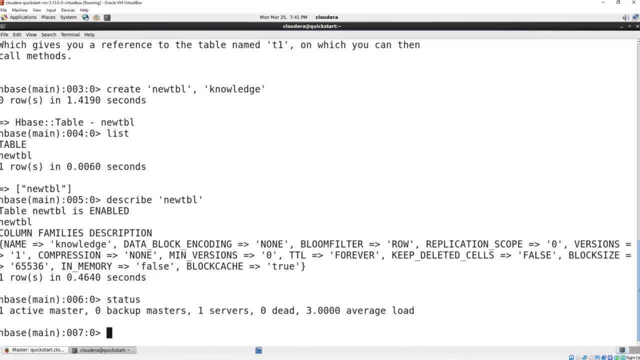 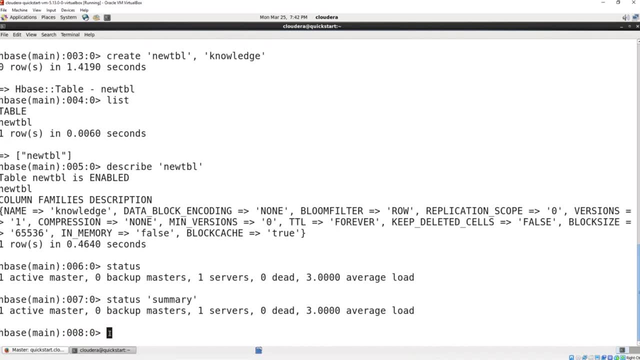 Status says: I have one active master going on. That's our HBase as a whole. We can do status summary. That should do the same thing as status. So we got the same thing coming up And now that we've created it, let's go ahead and put something in it. So we're going to put new TBL And then we 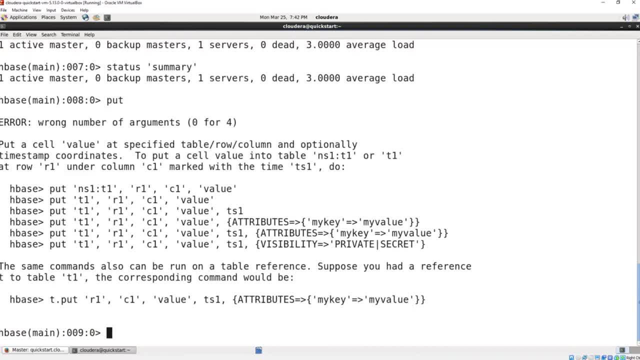 want row one. You know what, Before I even do this, let's just type in put And you can see. when I type in put, it gives us like a lot of different options of how it works and different ways of formatting our data as it goes in, And all of them usually begin with the new table. 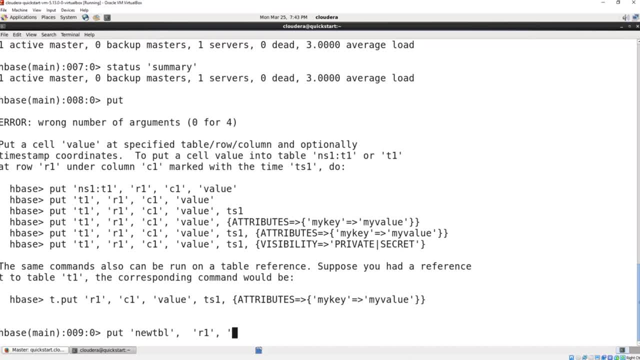 TBL, Then we have- in this case, we'll call it row one, And then we'll have knowledge. If you remember, we created knowledge already And we'll do knowledge sports, And then, in knowledge and sports, we're going to set that equal to cricket. So we're going to put underneath this our knowledge. 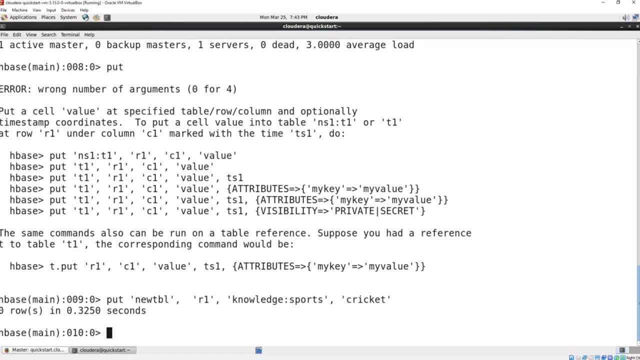 setup. We have a thing called sports in there And we'll see what this looks like in just a second. Let's go ahead and put in. we'll do a couple of these, Let's see. Let's do another row one, And. 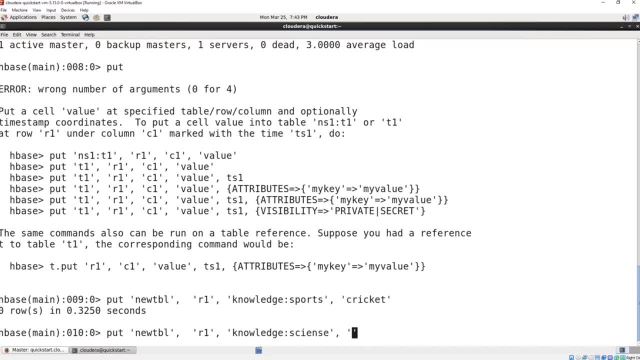 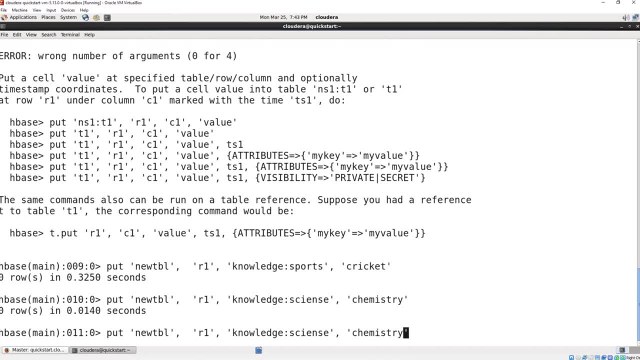 this person not only you know, we have row one which is both knowledgeable in cricket and also in chemistry. So it's a chemist who plays cricket in row one, And let's see if we have, let's do another row one just to keep it going And we'll do science. In this case, let's do physics, Not. 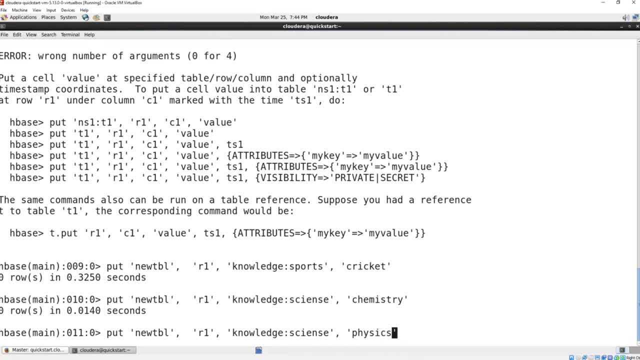 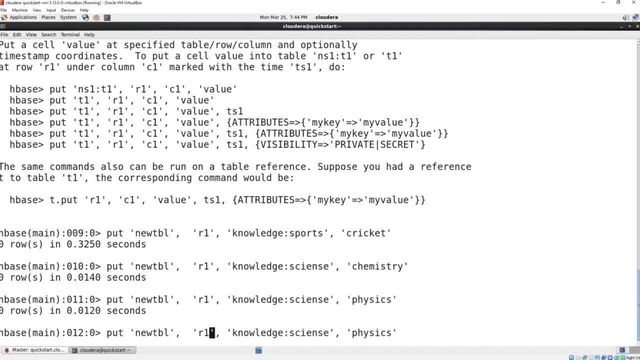 only in chemistry, but also a physicist. I have quite a joy in physics myself. So here we go, We have row one, There we go, And then let's do row two. Let's see what that looks like when we start with the physics. So row two: this person is has knowledge in economics. This is a master of. 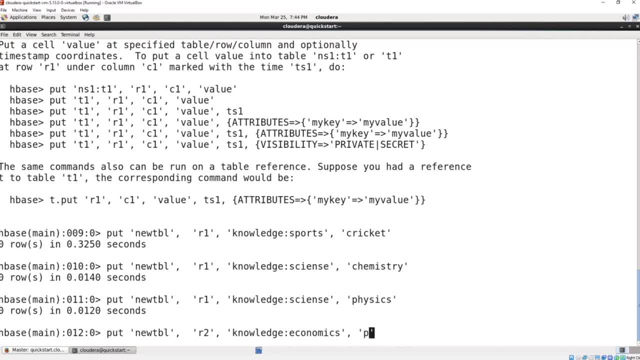 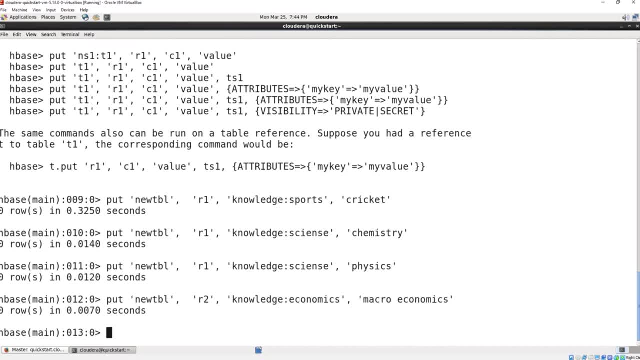 business and how, or maybe it's global economics, Maybe it's just for the business and how it fits in with the country's economics, And we'll call it macroeconomics. So I guess it is for the whole country there. So we have knowledge, economics, macroeconomics, And then let's just do one more. 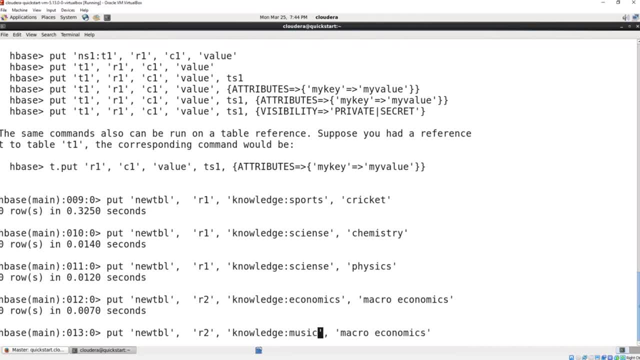 We'll keep it as row two, And this time our economist is also a musician, So we'll put music. And they happen to have knowledge and they enjoy the knowledge, So we'll put music And then we'll enjoy. oh, let's do pop music. They're into the current pop music going on, So we've loaded our. 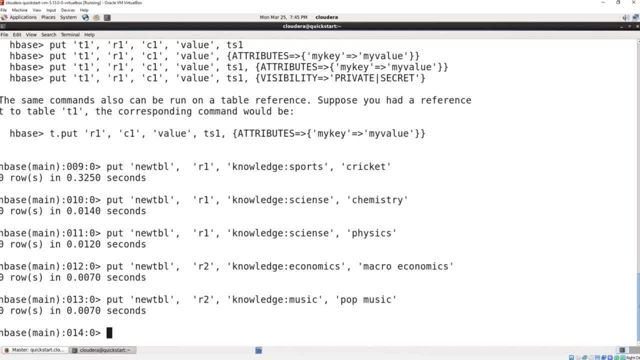 database and you'll see we have two rows, row one and row two, in here, And what we can do is we can list the contents of our database by simply doing scan, Scan and then let's just do scan by itself. So you can see how that looks. You can always just type in there and it tells you all the. 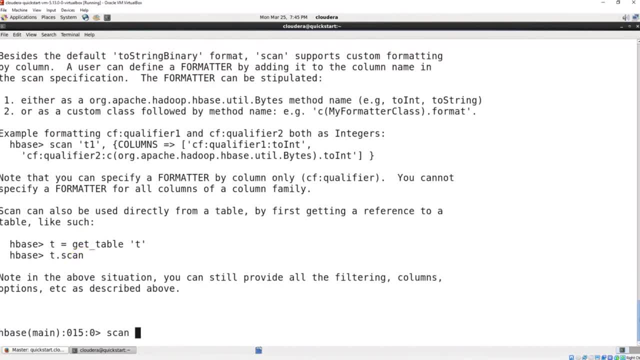 different setups you can do with scan and how it works. In this case we want to do scan new TBL And in our scan new TBL we have row one row one row, two row, two row, three row, four row, five row, six row, seven row eight row nine, row, ten row, ten row. 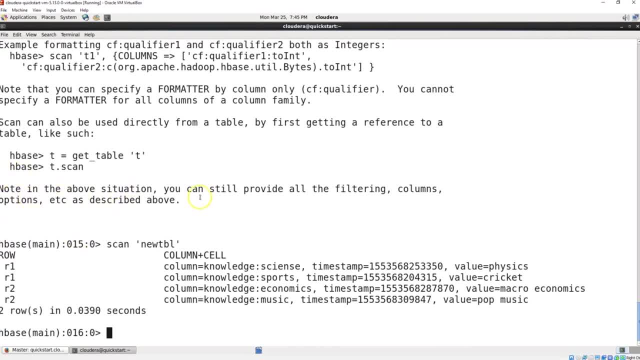 12. And you'll see, row one has a column called knowledge, science, time step, value, crickets, value physics, So it has information as when it was created, when the time stamp is. Row one also has knowledge, sports and a value of cricket. So we have sports and science And this is. 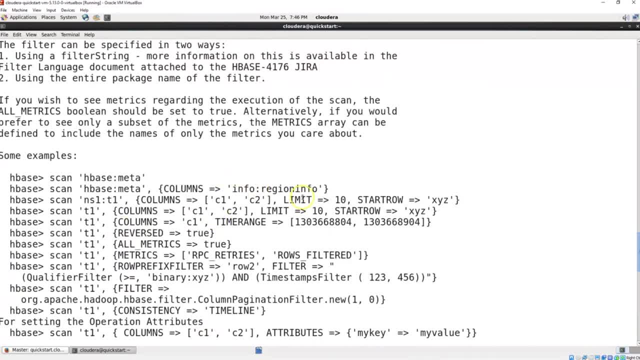 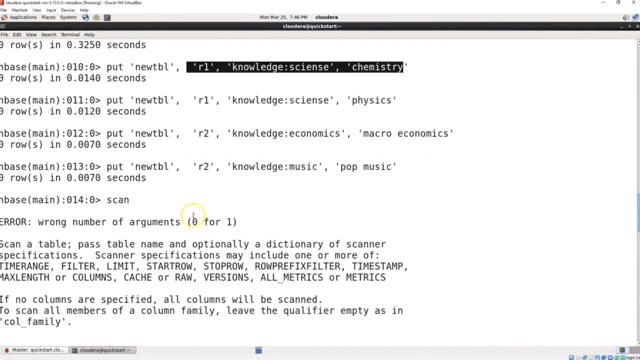 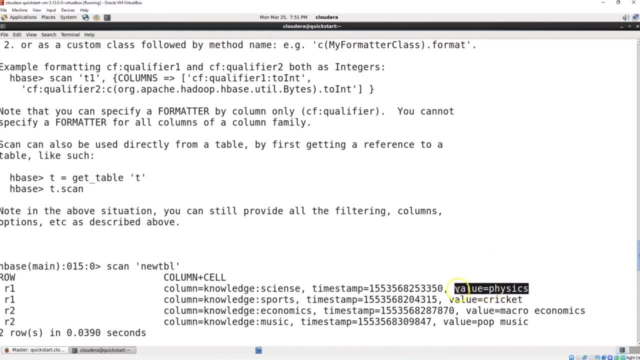 interesting because, if you remember, up here we also gave it originally. we told it to come in here and have chemistry. We had science, chemistry and science, physics. And we come down here. I don't see the chemistry. Why? Because we've now replaced chemistry with physics. So the new value 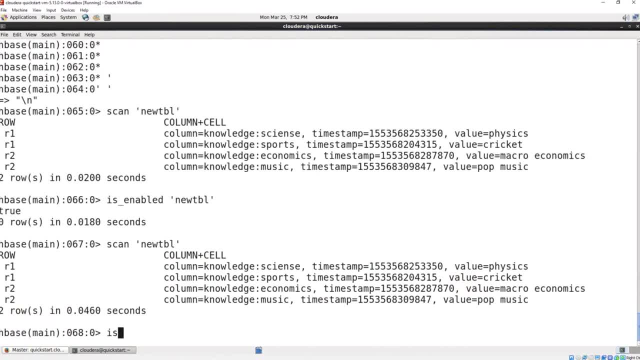 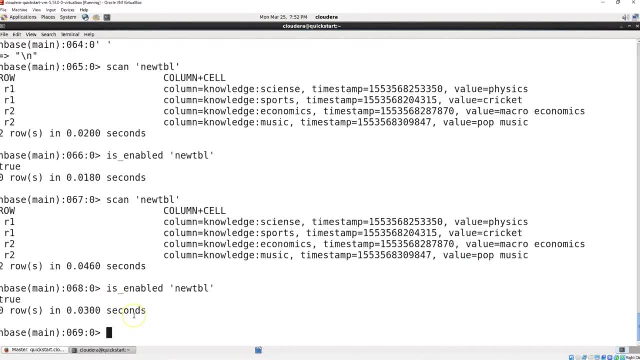 is physics on here. Let me go ahead and clear down a little bit And in this we're going to ask the question: is enabled new table? When I hit enter in here you're going to see it comes out true, And then we'll go ahead and disable it. Let's go ahead and disable new table. Make sure I have. 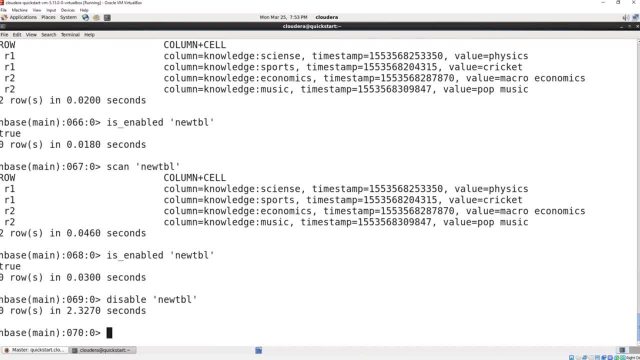 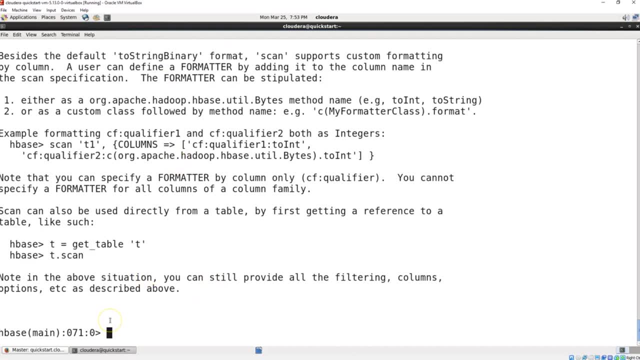 our quotes around it. And now that we've disabled it, what happens when we do the scan? When we do the scan- new table, I hit enter. you're going to see that we get an error coming up. So once it's disabled, you can't do anything with it until we re-enable it. 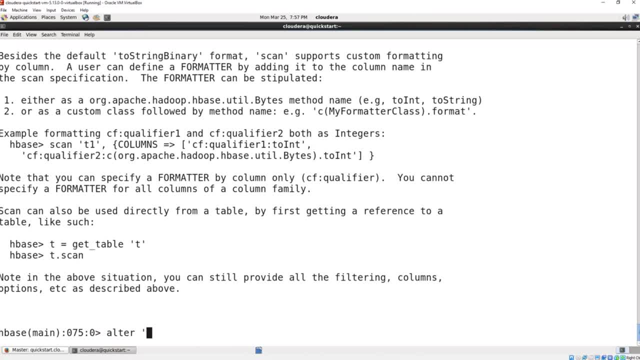 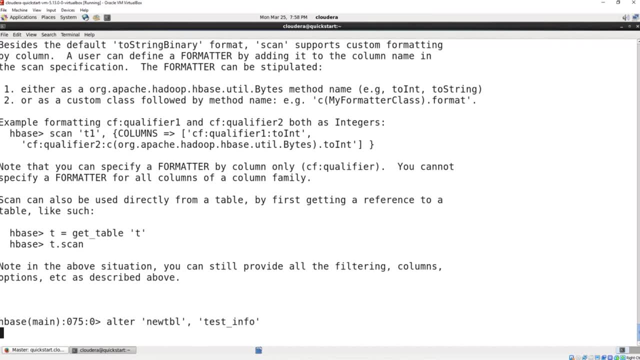 Now, before we enable the table, let's do an alteration on it. And here's our new table, And this should look a little familiar because it's very similar to create. We'll call this test info, We'll hit enter in there, It'll take just a moment for updating And then we want to go. 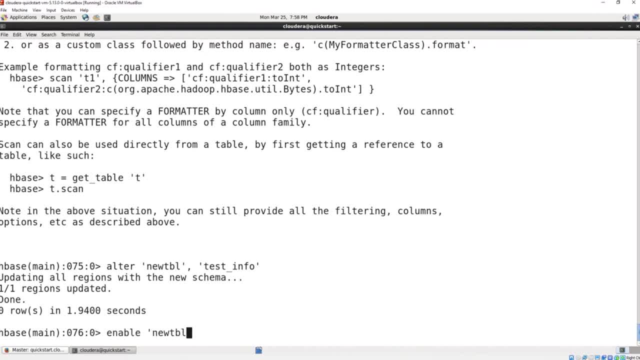 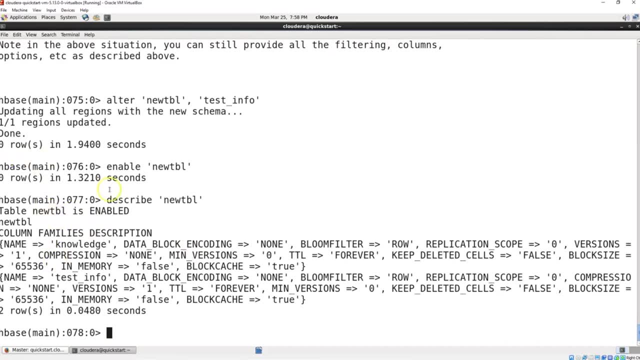 ahead and enable it. So let's go ahead and enable our new table, So it's back up and running. And then we want to describe, Describe new table And we come in here. you'll now see we have name knowledge And under there we have our data encoding and all the information under 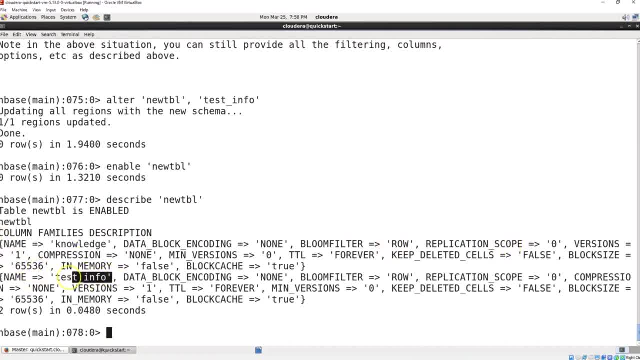 knowledge, And then we also have down below, test info. So now we have the name test info and all the information concerning the test info on here And we'll simply enable it. New table- So now it's enabled. Oops, I already did that. I guess we'll enable it twice, And so let's start looking at. 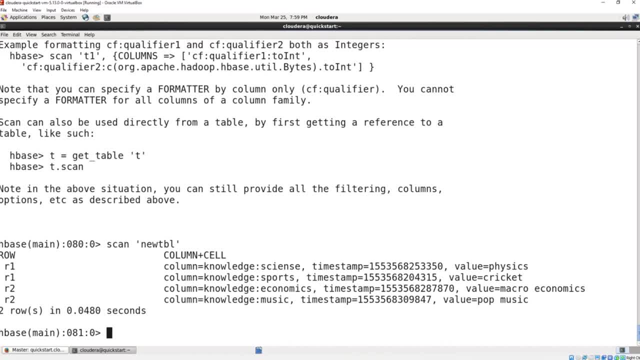 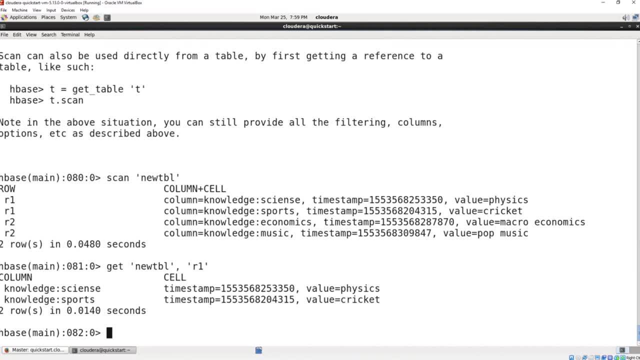 well, we had scan new table And you can see here where it brings up the information like this: But what if we want to go ahead and get a row? So we'll do R1. And when we do HBase R1, you can see we have knowledge, science And it has a timestamp value. 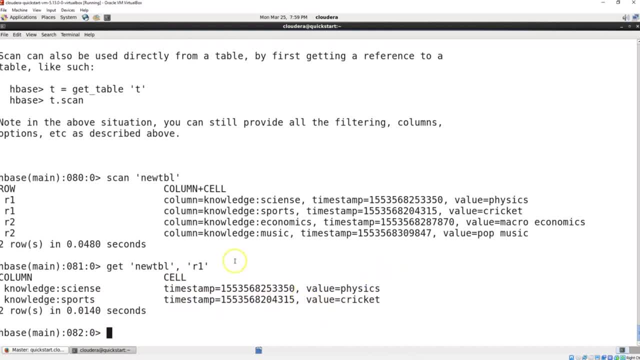 physics, And we have knowledge sports And it has a timestamp on it and value cricket. And then let's see what happens when we put into our new table, And in here we want row one, And if you can guess from earlier because we did something similar, we're going to do knowledge economics. And then 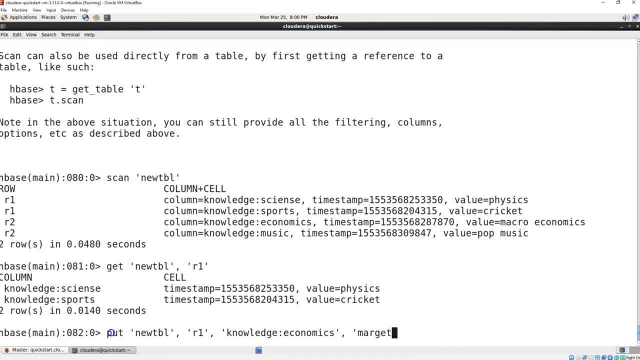 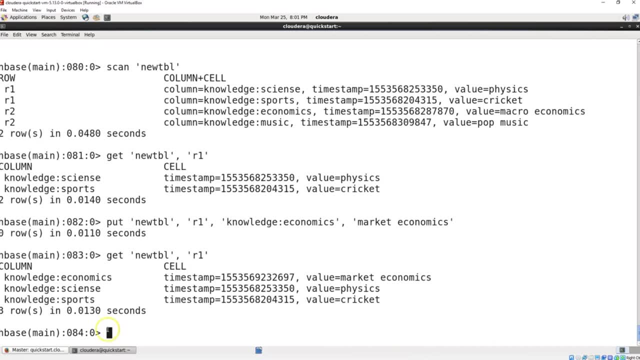 it's going to be a sort of- I think it was what- macroeconomics It's now market economics And we'll go back and do our get command And now see what it looks like And we can see here where we have knowledge. economics- It has a timestamp value: market economics, physics. 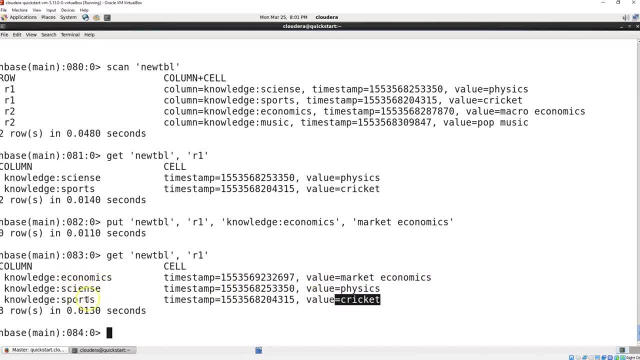 and cricket, And this is because we have economics, science and sports. Those are the three different columns that we have, And then each one has different information in it, And so if you manage to go through all these commands and look at basics on here, you'll now have the ability to 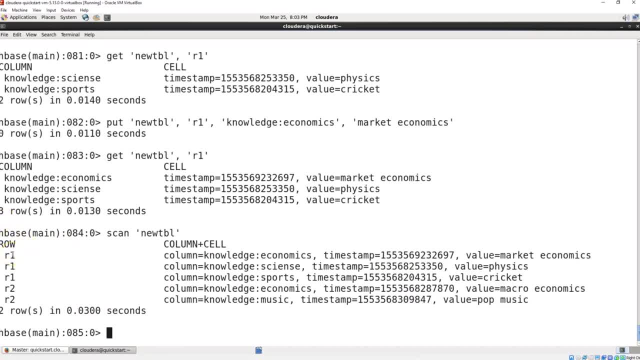 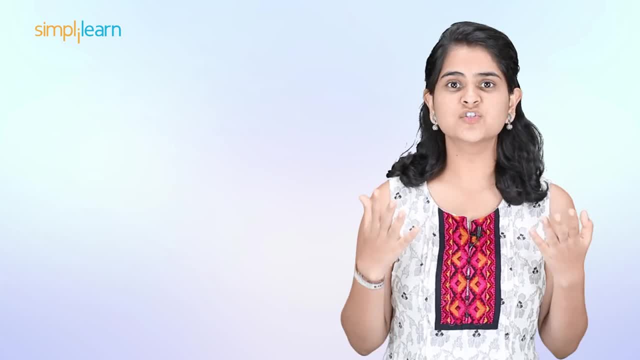 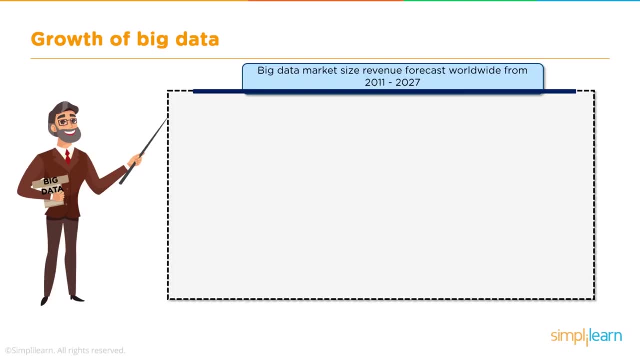 create a very basic HBase. Thank you, guys. Now that we're done with Hadoop ecosystem, we have Shruti, who will take us to big data applications. Before we move on to the applications, let's have a quick look at the big data market revenue. 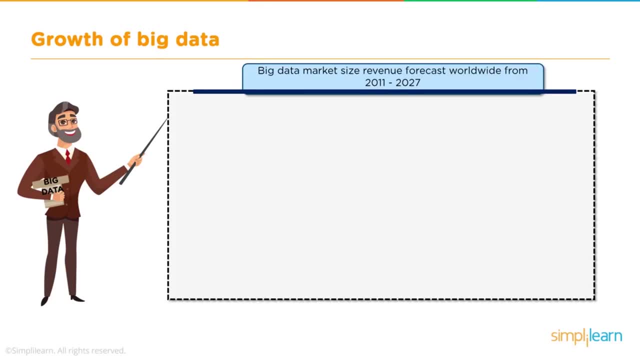 forecast worldwide from 2011 to 2027.. So here's a graph in which the y-axis represents the revenue in billion US dollars and the x-axis represents the years. As it is seen clearly from the graph, the revenue in billion US dollars and the x-axis represents the years. So here's a graph in 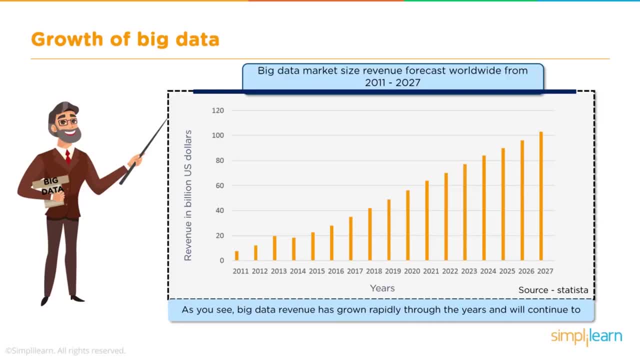 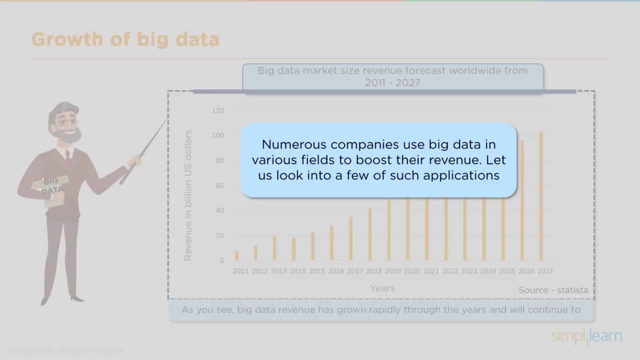 the graph. Big data has grown until 2019 and statistics predict that this growth will continue even in the future. This growth is made possible as numerous companies use big data in various domains to boost their revenue. We will look into a few of such applications. The first: big data. 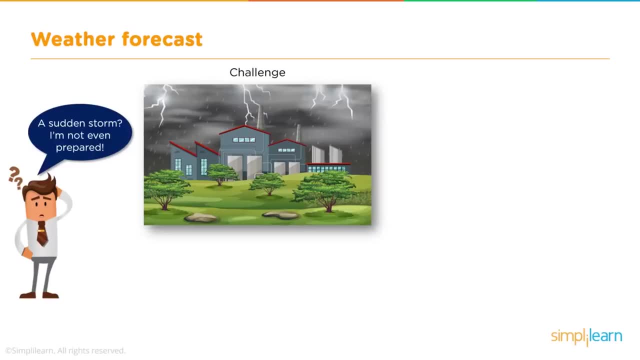 application we will look into is weather forecast. Imagine there is a sudden storm and you're not even prepared. That would be a terrifying situation, isn't it? Dealing with any calamities, such as hurricanes, storms, floods, water, etc. is a very difficult task, So we're going to look into. 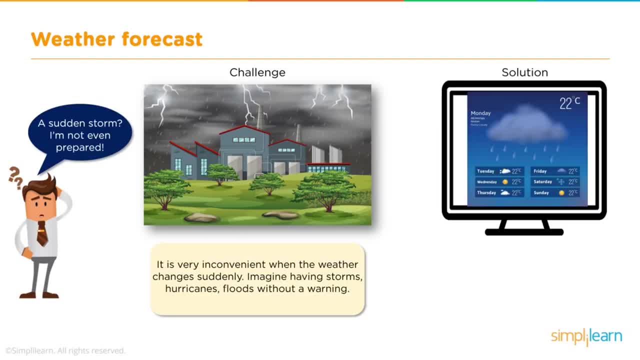 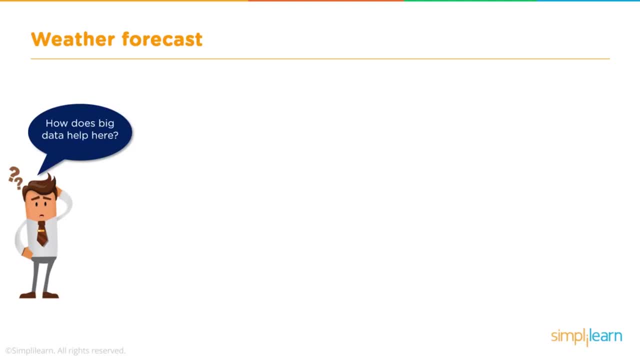 solution is to have a tool that predicts the weather of the coming days well in advance. This tool needs to be accurate, and to make such a tool, big data is used. So how does big data help here? Well, it allows us to gather all the information required to predict the weather Information. 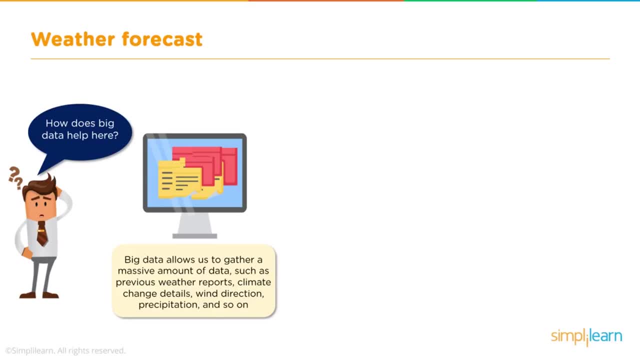 such as the climate change details, wind direction, precipitation, previous weather reports and so on. After all this data is collected, it becomes easier for us to spot a trend, and we can see that and identify what's going to happen next by analysing all of this big data. 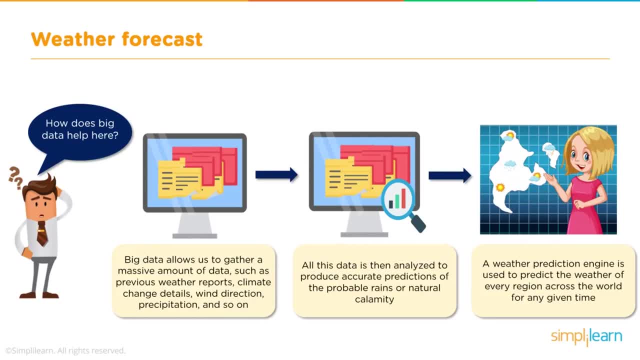 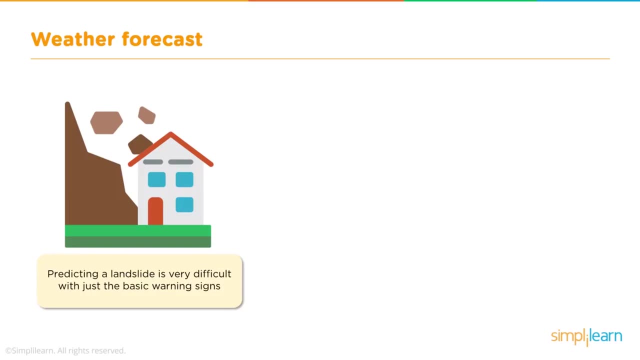 A weather prediction engine works on this analysis. It predicts the weather of every region across the world for any given time. By using such a tool, we can be well prepared to face any climate change or any natural calamity. Let's take an example of a landslide and try to understand how big data is used to tackle such a situation. 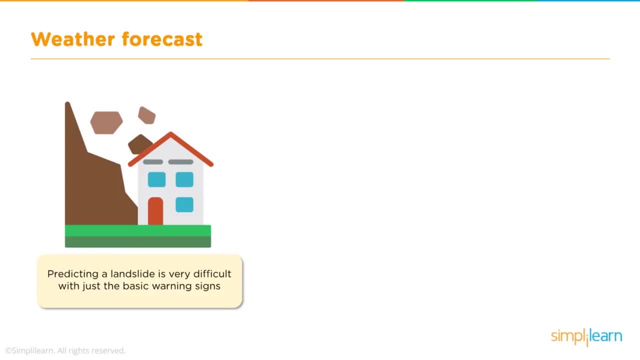 Predicting a landslide is very difficult with just the basic warning signs. Lack of this prediction can cause a huge damage to life and property. This challenge was studied by the University of Melbourne and they developed a tool which is capable of predicting a landslide. This tool predicts the boundary where a landslide is likely to occur two weeks before. 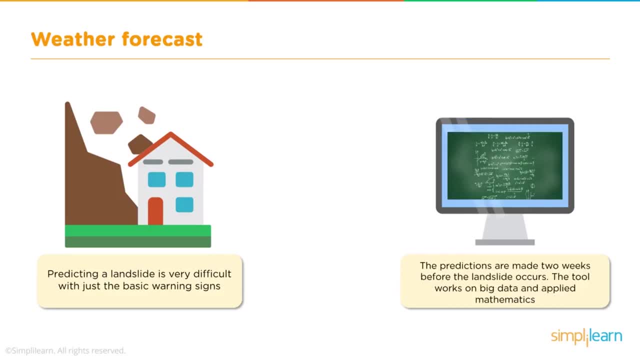 This magical tool works on both big data and applied mathematics. An accurate prediction like this, which is made two weeks before, can save a lot of time. It can save lives and help in relocating people in that particular region. It also gives us an insight into the magnitude of the upcoming destruction. 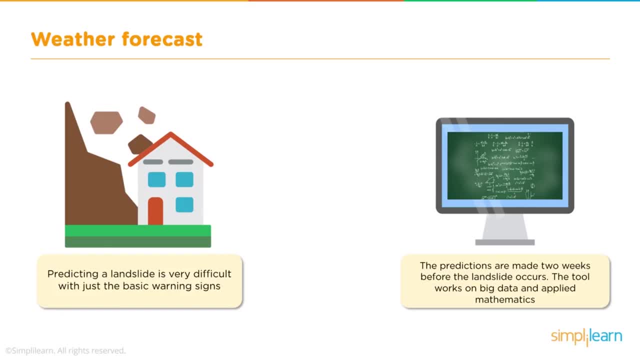 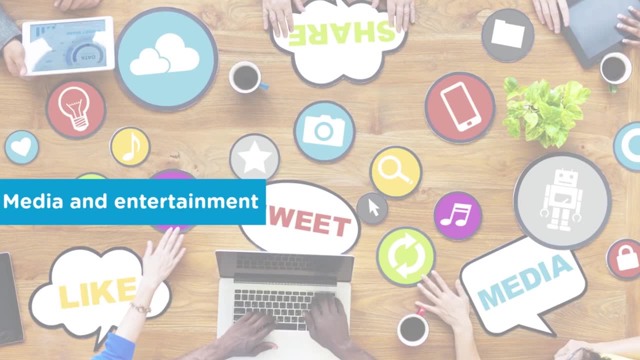 This is how big data is used in weather forecast and in predicting any natural calamities across the world. Let us now move on to our next application, that is, big data application in the field of media and entertainment. The media and the entertainment industry is a massive one. 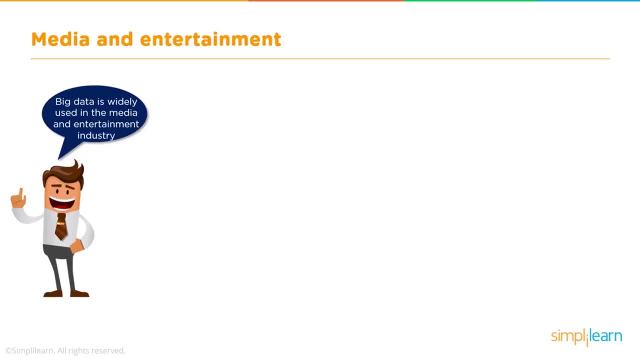 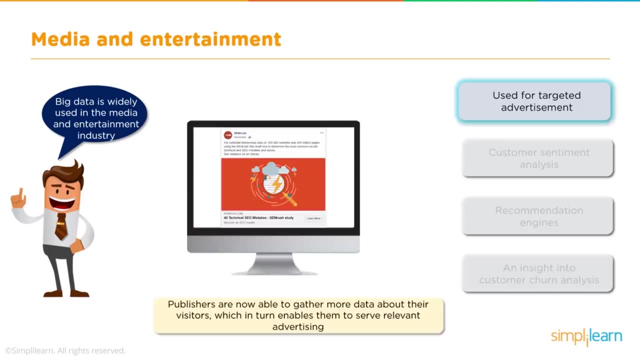 Leveraging big data here can produce sky-high results and boosts the revenue for any company. Let us see the different ways in which big data is used in this industry. Have you ever noticed that you come across relevant advertisements in your social media sites and in your mailboxes? 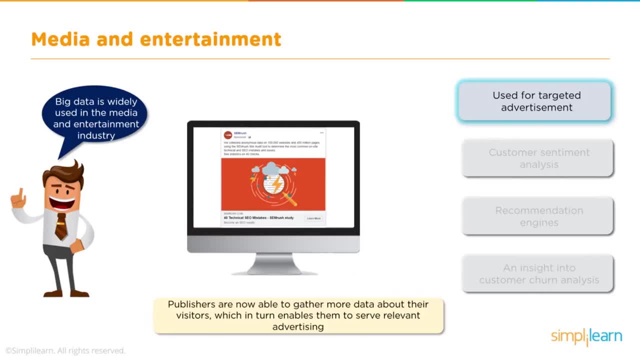 Well, this is done by analysing all your data, such as your previous browsing history and your purchase data. Publishers then display what you like in the form of ads, which will, in turn, catch your interest in looking into it. Next up is customer sentiment analysis. 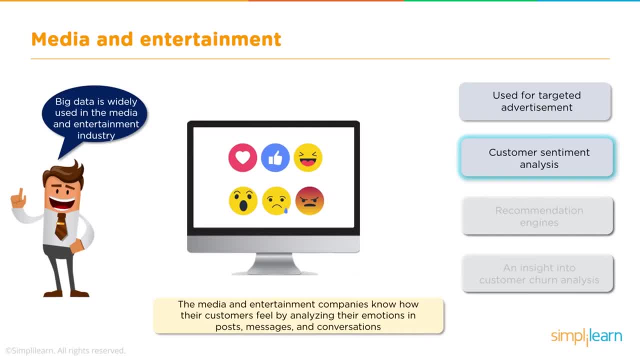 Customers are very important to us. The happier the customer, the greater the company's revenue. Big data helps in gathering all the emotions of a customer through their posts, messages, conversations, etc. These emotions are then analysed to arrive at a conclusion regarding the customer's satisfaction. 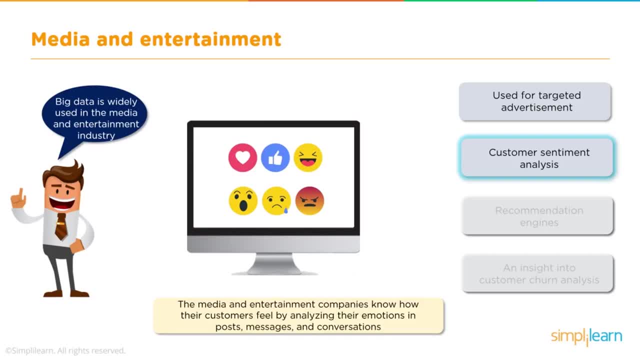 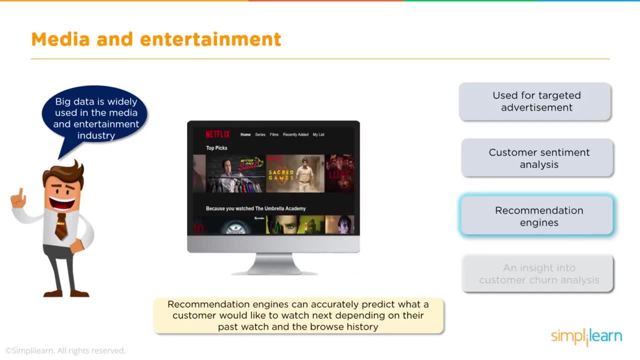 If the customer is unhappy, the company strives to do better the next time and provides their customers a better experience. While purchasing an item from an e-commerce site or while watching videos on an internet, you might have noticed a segment which says Most Recommended List for you. 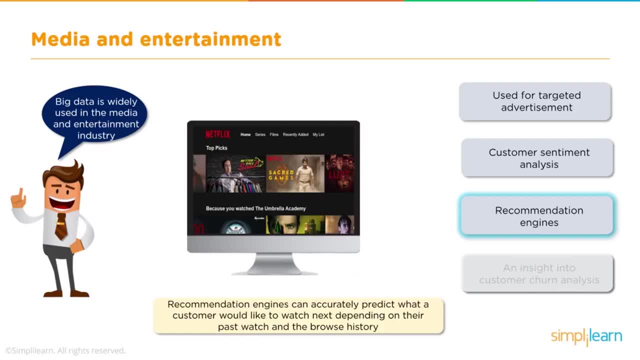 This list is a personalised list, which is made available to you by analysing all the data, such as your previous watch history, your subscriptions, your likes and so on. Recommendation Engine is a tool that filters and analyses all this data and provides you with a list that you would most likely be interested in. 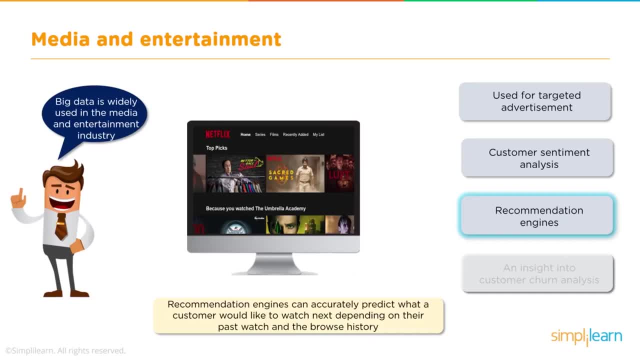 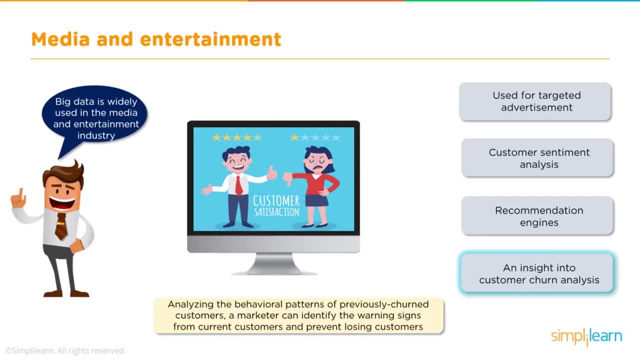 By doing so, the site is able to retain and engage its customer for a longer time. Next is Customer Churn Analysis. In simple words, customer churn happens when a customer stops their subscription with a service. Predicting and preventing this is of paramount importance to any organisation. 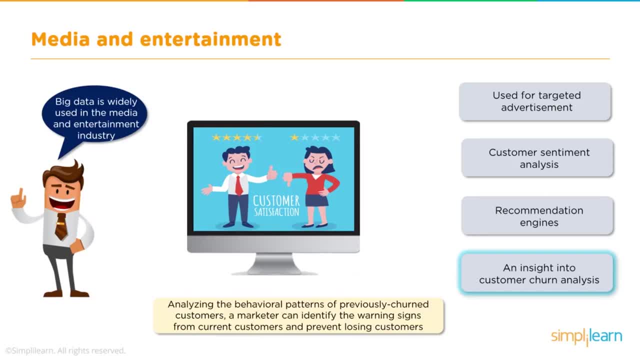 By analysing the behavioural patterns of previously churned customers, an organisation can identify which of their current customers are likely to churn. By analysing all of this data, the organisation can then implement effective churn. This is how the app is used for customer retention. 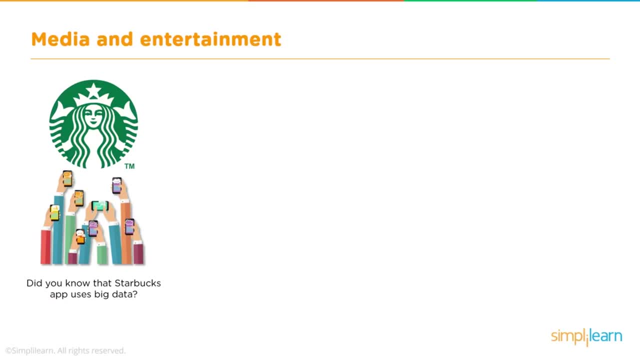 Let us now look into an use case of Starbucks. Big data is effectively used by the Starbucks app. 17 million users use this app and you can imagine how much data they generate- Data in the form of their coffee buying habits, the store they visit and to the time they purchase. 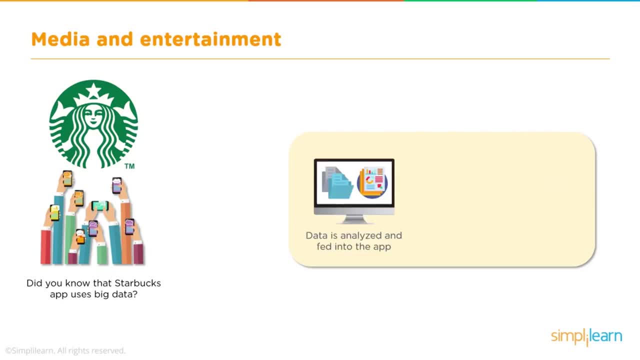 All of this data is fed into the app. So when a customer enters a new Starbucks location, the system analyses all their data and, as a result, they are provided with their preferred order. This app also suggests new products to the customer. In addition to this, they also provide personalised offer. 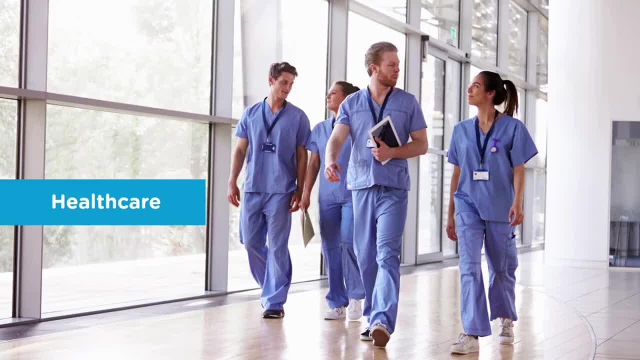 and discounts on special occasions. Moving on to our next sector, which is healthcare, It is one of the most important sectors. Big data is widely used here to save lives. With all the available big data, medical researches are done very effectively. 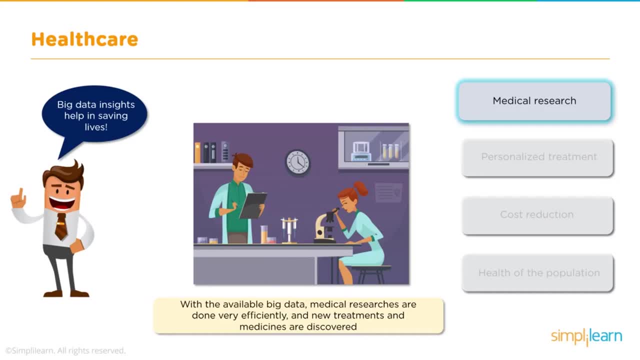 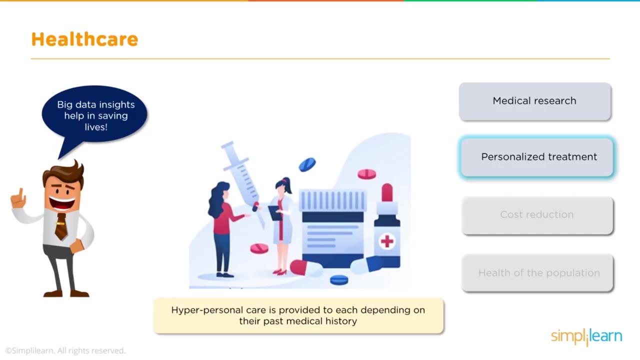 They are performed accurately. by analysing all the pre ounce medical histories, and new treatments and medicines are discovered. Cure can be found out even for few of the incurable diseases. There are cases when one medication need not be effective for every patient, Hence personal care is very important. 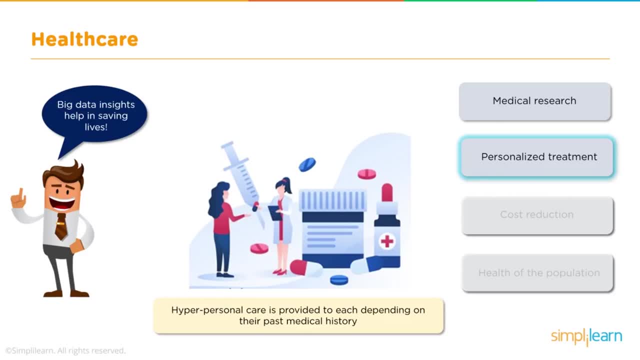 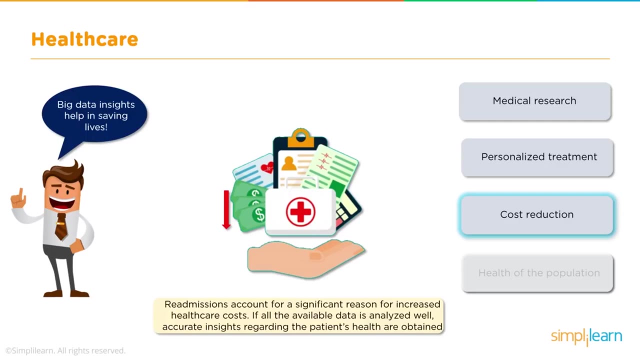 Personal care is provided to each patient depending on their past medical history. An individual's medical history, along with their body parameters, are analysed and personal attention is given to each of them. them. As we all know, medical treatments are not very pocket-friendly. Every time a medical 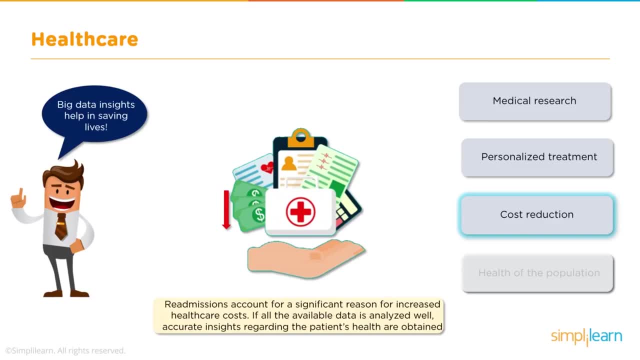 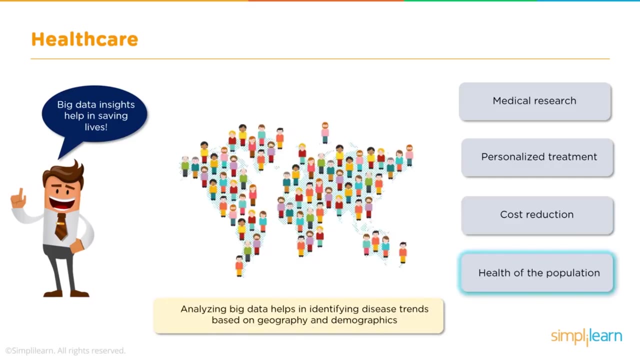 treatment is taken, the amount increases. This can be reduced if readmissions are brought down. Analyzing all the data precisely will deliver a long-term efficient result, which will in turn prevent a patient's readmission. frequently With globalization came an increase in the 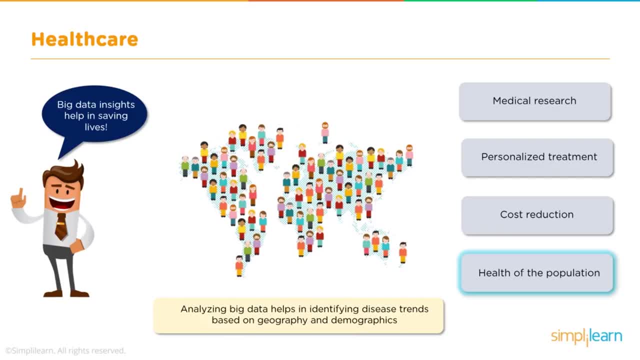 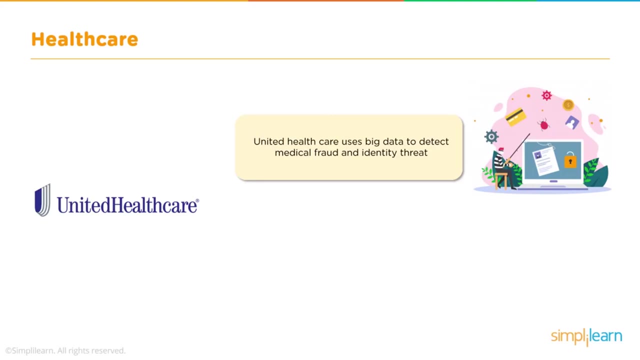 ease for infectious diseases to spread. widely Based on geography and demographics, big data helps in predicting where an outbreak of epidemic viruses are most likely to occur. An American healthcare company, United Healthcare, uses big data to detect any online medical fraud activities, such as payment of unauthorized benefits, intentional misrepresentation of data. 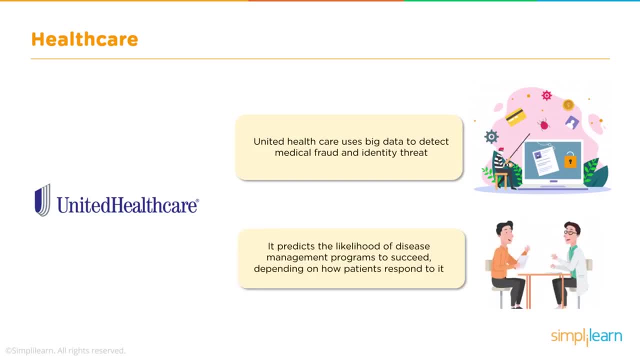 and so on. The healthcare company runs disease management programs. The system is designed to detect and monitor the spread of disease. The success rates of these programs are predicted using big data, depending on how patients respond to it. The next sector we will look into is Logistics. 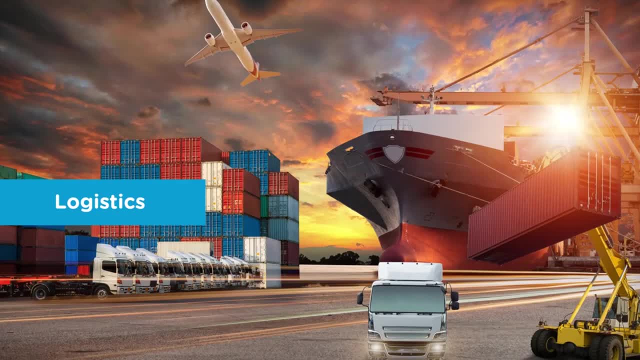 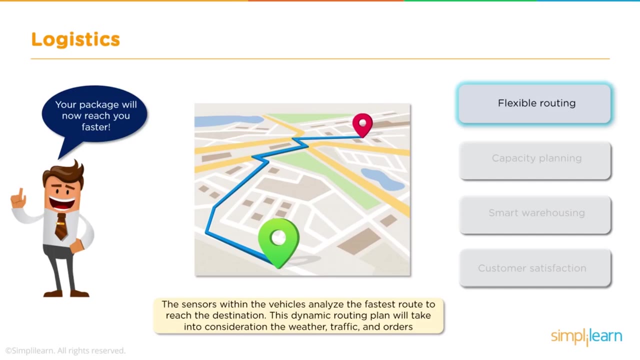 Logistics looks into the process of transportation and storage of goods. The movement of a product from its supplier to a consumer is very important. Big data is used to make this process faster and efficient. The most important factor in logistics is the time taken for the 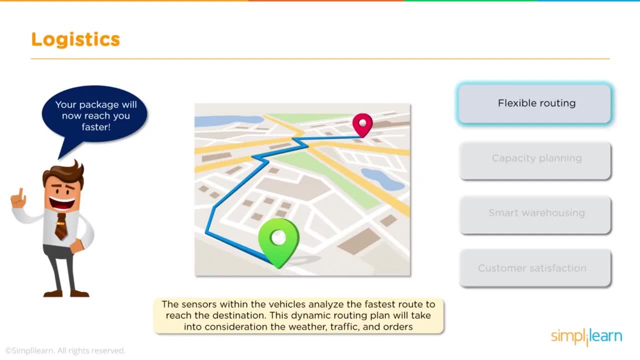 products to reach their destination. To achieve minimum time, sensors within the vehicle analyze the fastest route. This analysis is based on various data, such as the weather, traffic, the list of orders and so on. By doing so, the fastest route is obtained and the delivery 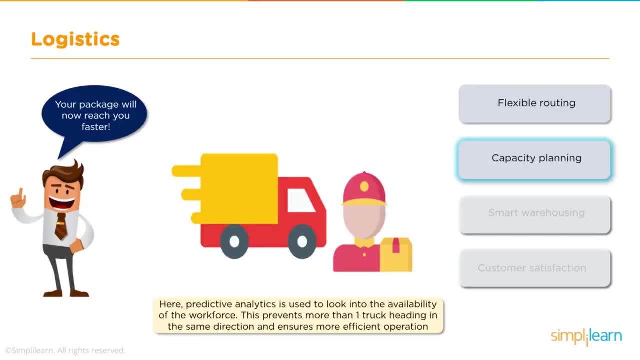 time is reduced. Capacity planning is another factor which needs to be taken into consideration. Details regarding the workforce and the number of vehicles are analyzed thoroughly and are evaluated. Each vehicle is allocated a different route. This is done as there is no need for many trucks to travel in the same direction, which will be pointless Depending on the 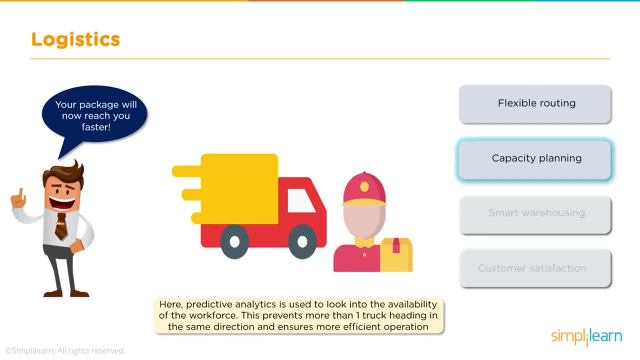 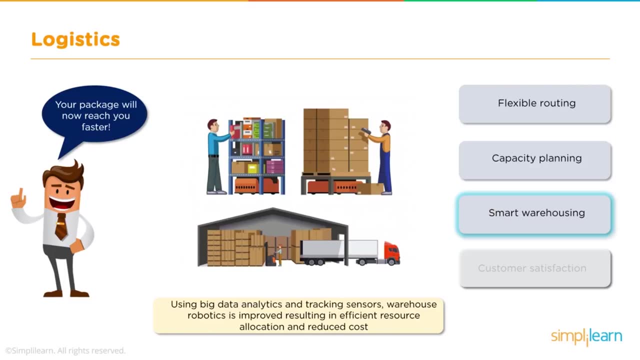 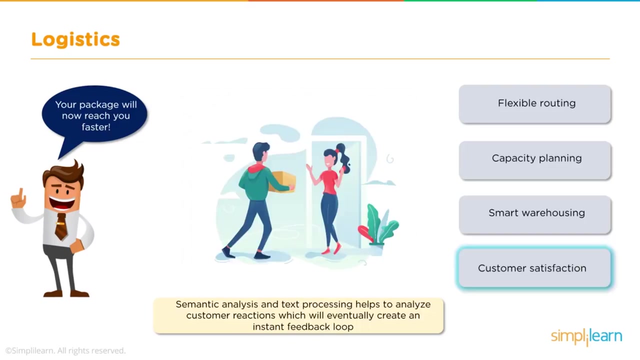 analysis of the available workforce and resources, this decision is taken. Big data analytics also finds its use in managing warehouses efficiently. This analysis, along with tracking sensors, provide information regarding the underutilized space, which results in an efficient resource allocation and eventually reduces the cost. Customer satisfaction is. 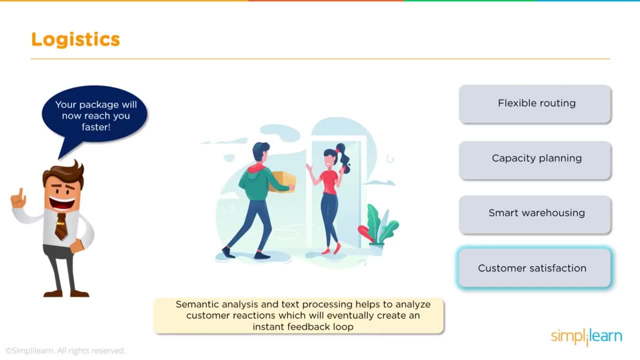 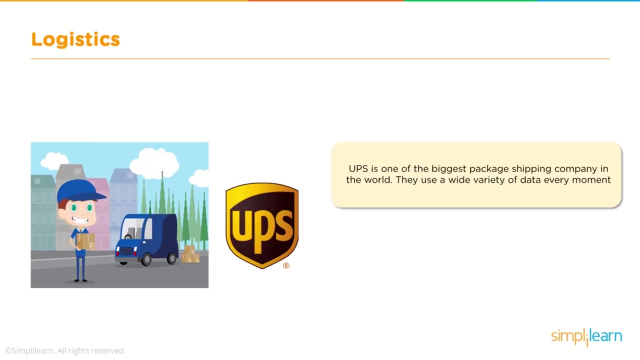 important in logistics just like it is in any other sector. Customer reactions are analyzed from the available data, which will eventually create an instant feedback loop. A happy customer will always help the company gain more customers. Let us now look into a use case of UPS As 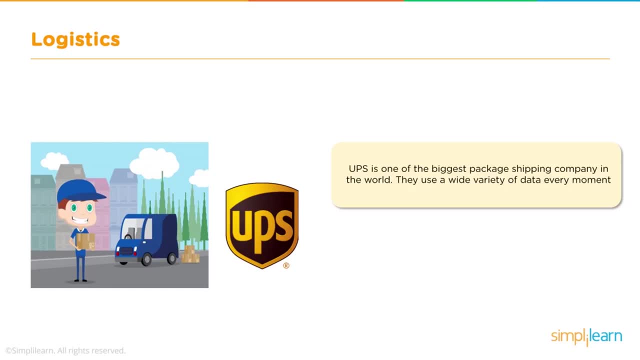 you know, UPS is one of the biggest shipping company in the world. They have a huge customer database and they work on data every minute. UPS uses big data to gather different kinds of data regarding the weather, the traffic jams, the geography, the locations and so. 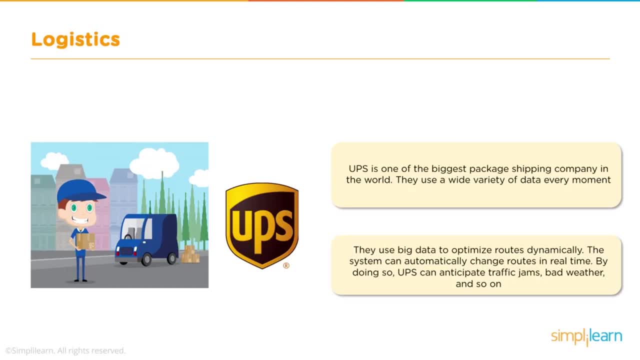 on. After collecting all this data, they analyze it to discover the best and the fastest route to the destination. In addition to this, they also use big data to change the routes in real time. This is how efficiently UPS leverages big data. 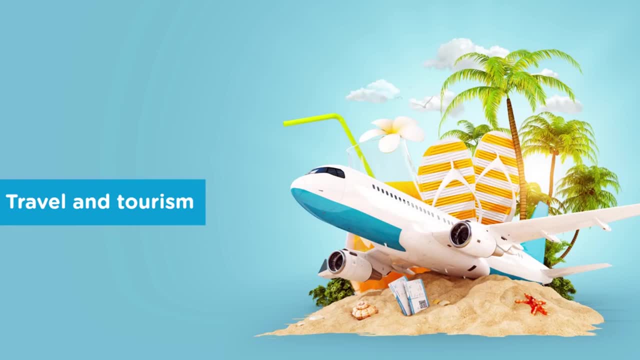 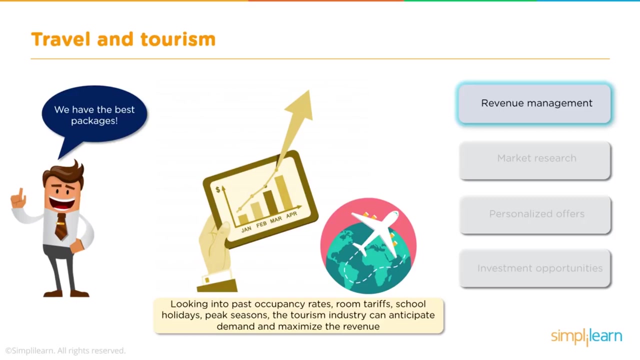 Big data is a very interesting sector, ie the travel and tourism sector. The global tourism market is expected to grow in the near future. Big data is used in various ways in this sector. Let us look into a few of them. Hotels can increase their revenue by adjusting the room tariffs depending on the peak seasons. 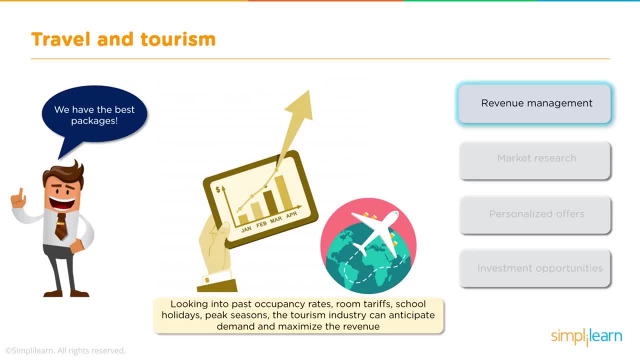 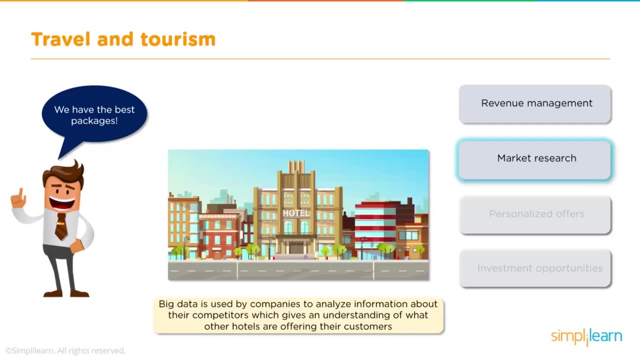 such as holiday seasons, festive seasons and so on. The tourism industry uses all of this data to anticipate the demand and maximize their revenue. Big data is also used to calculate the cost of the room. It is also used by resorts and hotels to analyze various details regarding their competitors. 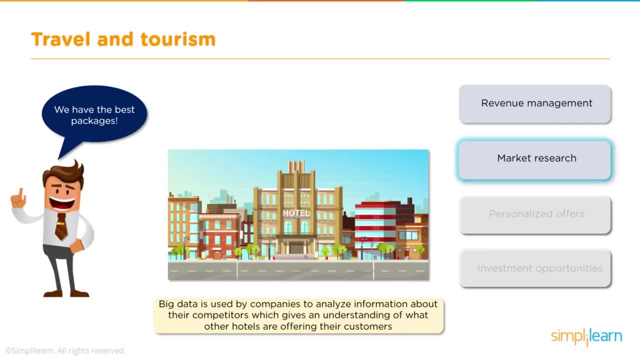 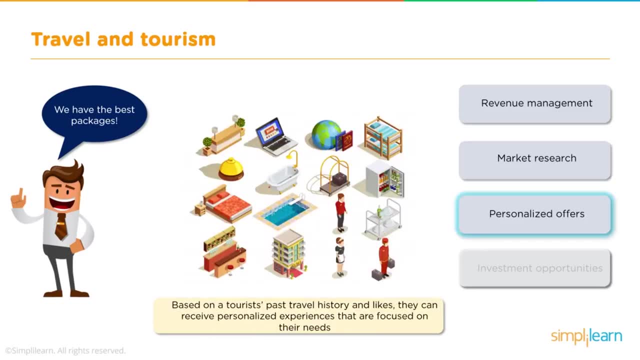 This analysis result helps them to incorporate all the good facilities their competitors are providing, And by doing so, the hotel is able to flourish further. A customer always comes back if they are offered good packages which are more than just the basic ones. Looking into a customer's past travel history, likes and preferences hotels. 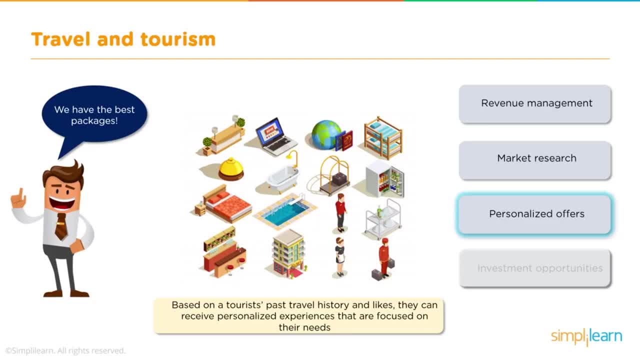 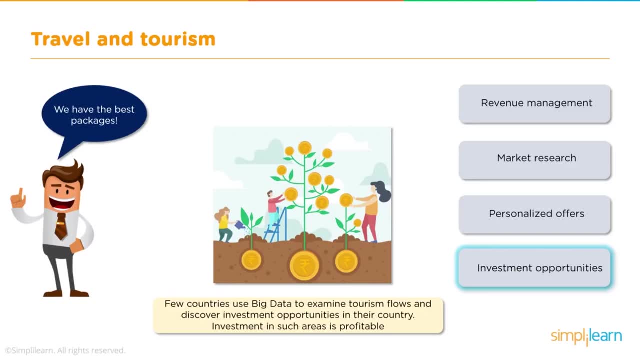 can provide its customers with personalized and personalized hotel facilities. Investing in an area which could be the hub of tourism is very wise. Few countries use big data to examine the tourism activities in their country, and this, in turn, helps them discover new and fruitful investment opportunities. 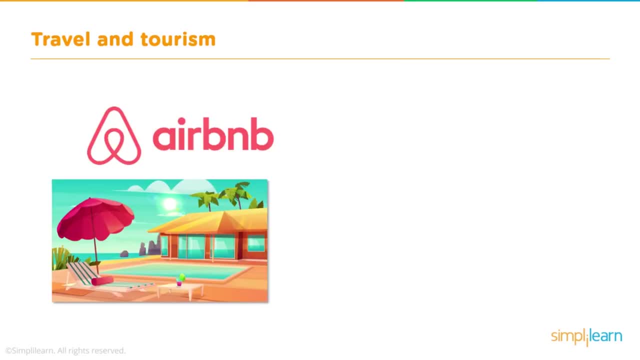 Let us look into one of the best online homestay networks- Airbnb- and see how big data is used by them. Airbnb undoubtedly provides its customers with the best services and services they can offer. Airbnb is one of the best online homestay networks in the world. Airbnb provides its 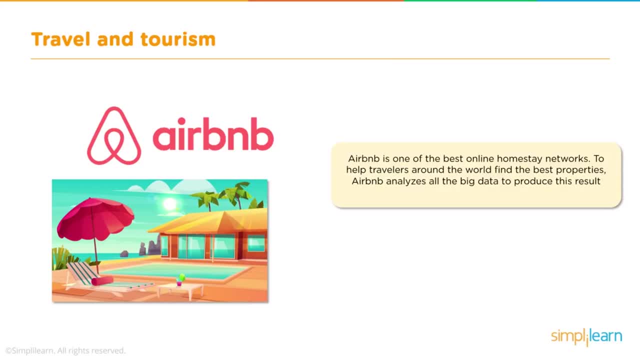 customers with the best services and services they can offer. Airbnb is one of the best online homestay networks in the world. Airbnb provides its customers with the best services and services they can offer. Airbnb provides its customers with the best services and services they can offer. Airbnb provides its consumers with the best space for them to as well. 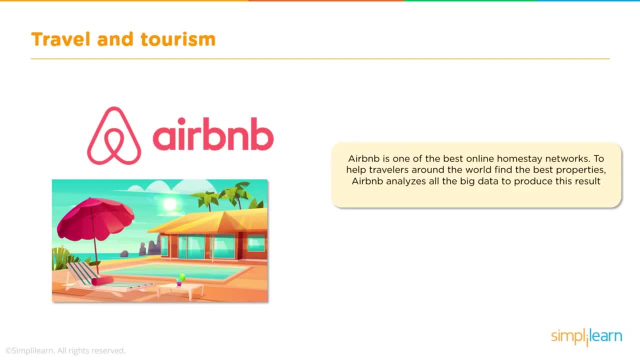 Big data is used by it to analyse the different kinds of available properties Depending on the customer's preferences, the pricing, the keywords, previous customers ratings and experiences. Airbnb filters out the best result. Big data works its magic yet again. Now we will move on to our final sector, which is the government and law enforcement sector. 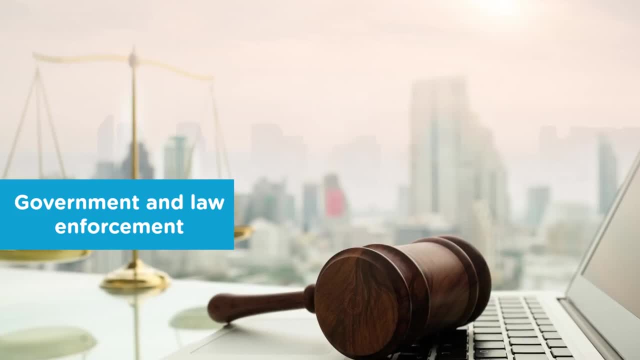 Maintaining law and order is of utmost importance to each customer. The added maravilisatotted law enforcement sector allows business owners to restrict the use of art, advertising and video content. The tips and tricks the company shared with us are ideal and ultimately helpful. 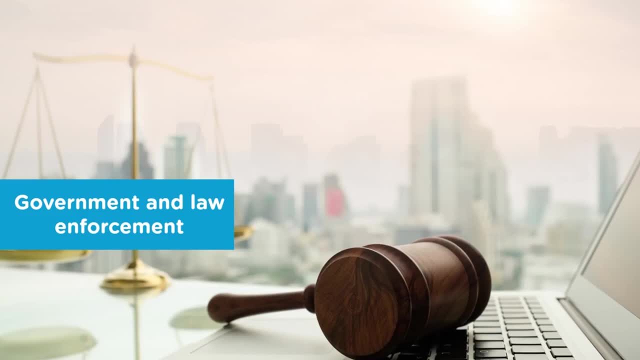 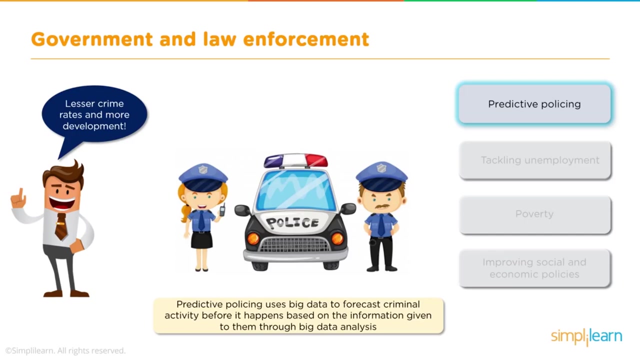 compared to the other companies, any government, It is a huge task by itself. Big data plays an active role here, and in addition to this, it also helps governments bring in new policies and schemes for the welfare of its citizens. The police department is able to predict criminal activities way before it happens by 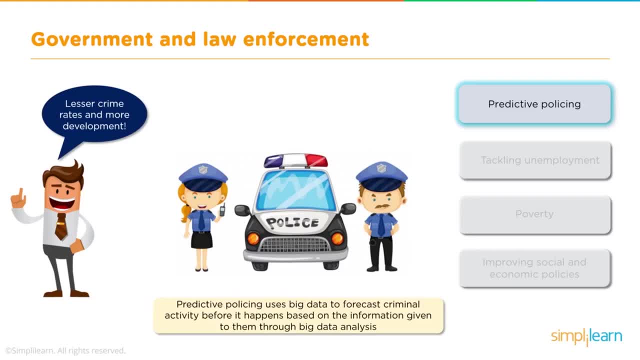 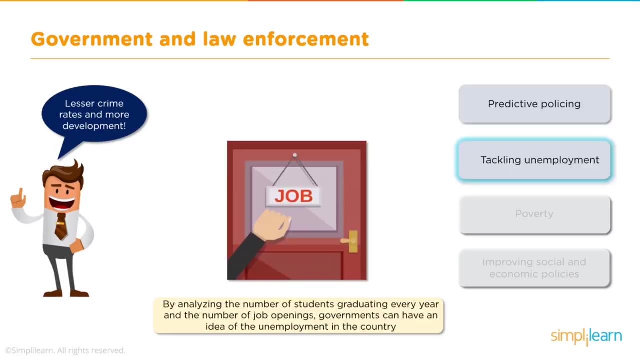 analysing big data information, such as the previous crime records in a particular region, the safety aspect in that region, and so on. By analysing these factors, they are able to predict any activity which breaks the law and order of the region. Governments are able to. 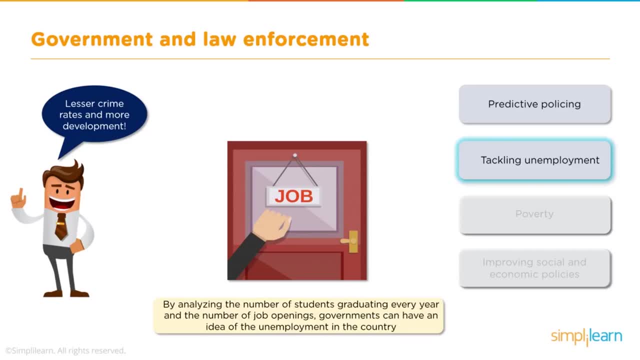 tackle unemployment to a great extent by using big data. By analysing the number of students graduating every year to the number of relevant job openings, the government can have an idea of the unemployment rate in the country and then take necessary measures to tackle it. 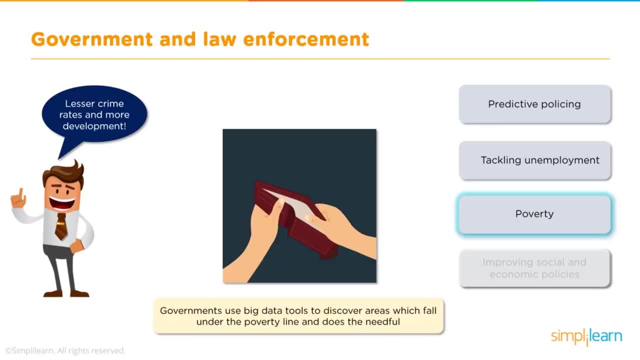 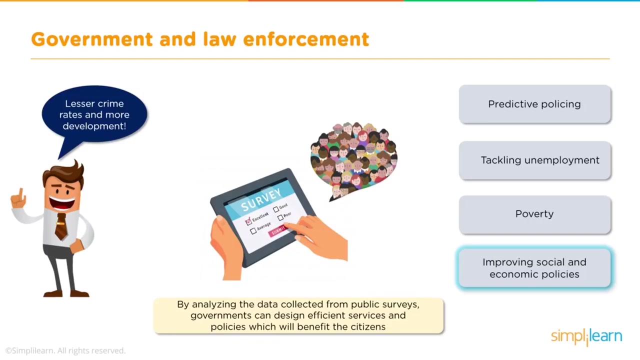 A next factor is poverty. In large countries it is difficult to analyse which area requires attention and development. Big data analytics makes it easier for governments to discover such areas. Poverty gradually decreases once these areas begin to develop. Governments have to always be on the lookout for better development. A public survey voices. 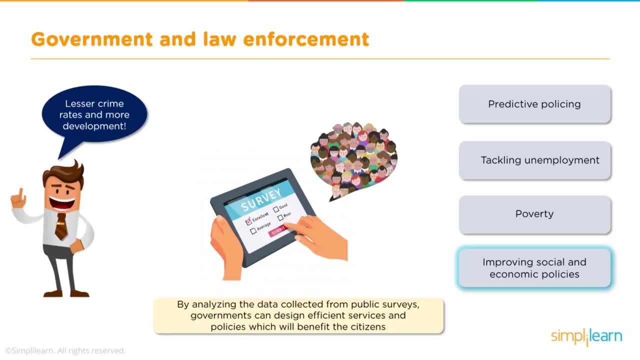 the opinion of a country's citizens. Analysing all the data collected from such surveys, it is easy to see that the number of students graduating every year to the number of students graduating every year is far more than the number of students graduating every year. 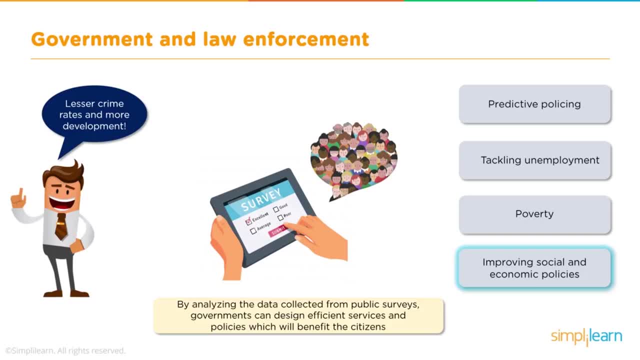 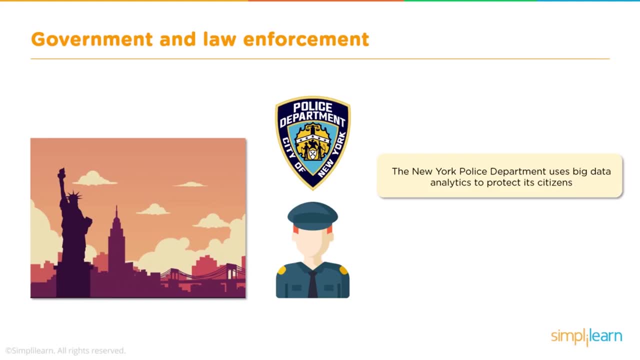 Governments can use big data analytics to help build better policies and services for their citizens. Let us now move on to our use case. Did you know that the New York Police Department uses big data analytics to protect its citizens? The department prevents and identifies crimes by 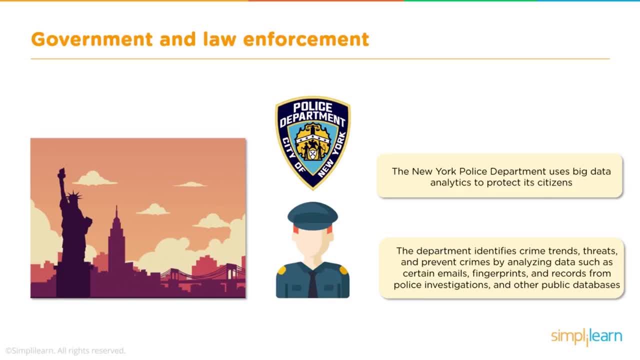 analysing a huge amount of data, which includes fingerprints, certain emails and records from previous police investigations, and so on. After analysing all of this data, the police department will be able to identify crimes, which include fingerprints, certain emails and records from previous police investigations, and so on. After analysing all of this data, 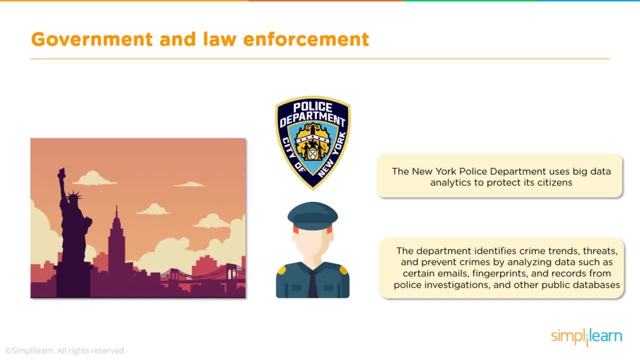 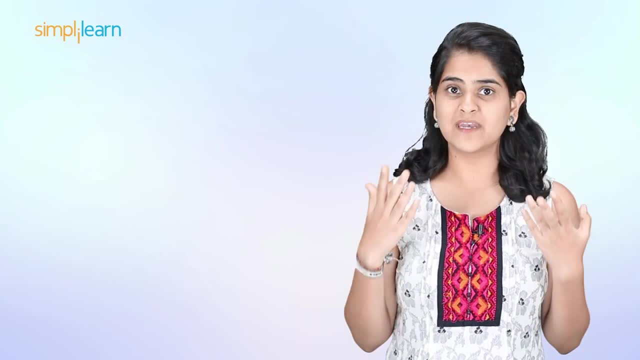 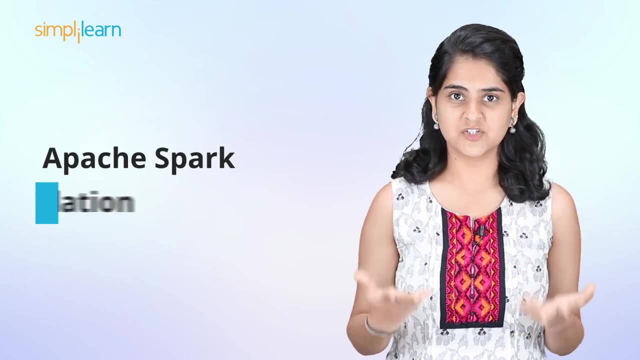 Insights are drawn from it which will help the police in taking the required preventive measures against crimes. Thank you, Shruti. Let us now have a look at the next data processing framework, spark. We have our instructor, Ajay, who will take us through Apache spark, its installation. 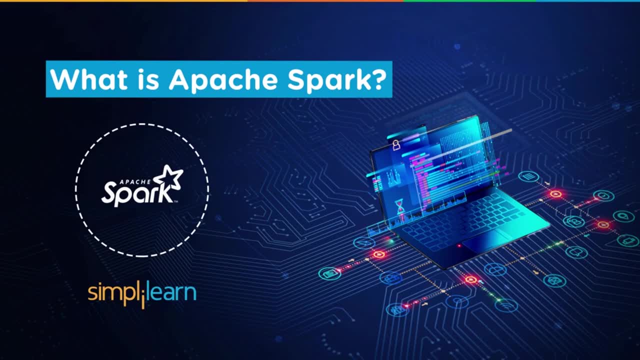 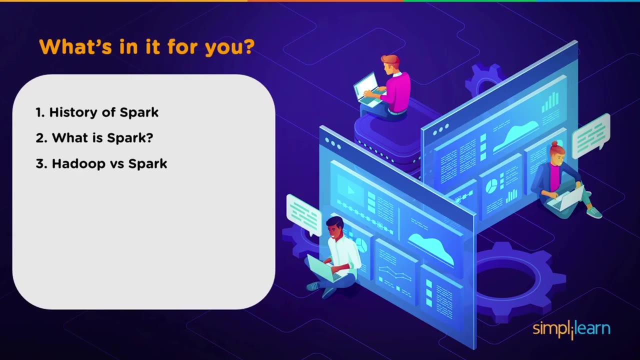 Welcome to this tutorial on Apache spark, one of the most in-demand Technologies and processing frameworks in the big data world, and here we will learn on Apache spark. History of spark. What is spark? Hadoop, which is a framework, again Wes spark components of Apache spark. that is spark core, spark SQL, spark streaming. 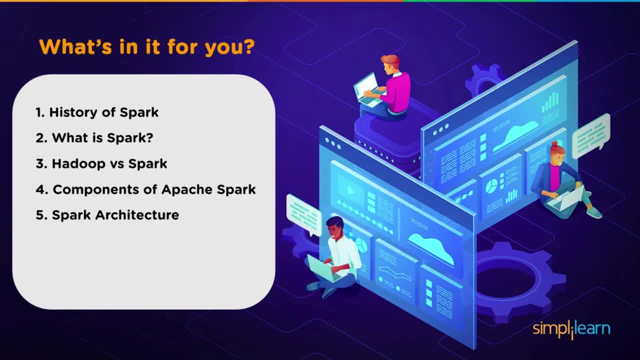 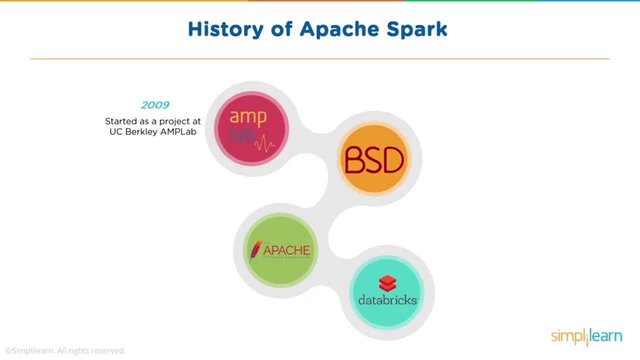 Spark ML lib and graphics. then we will learn on spark architecture, Applications of spark, spark use cases. So let's begin with understanding about history of Apache spark. it all started in 2009 as a project at UC Berkeley amp labs By Mathis area. in 2010 it was open source under a BSD license. in 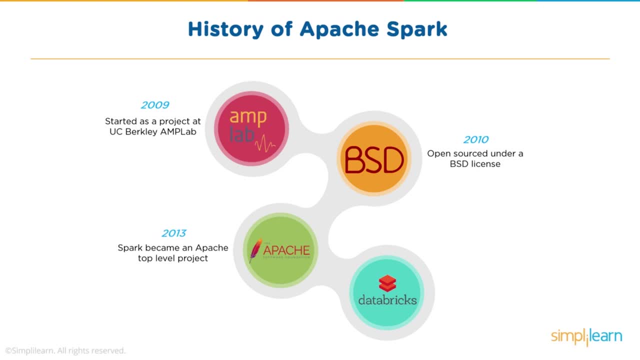 2013, spark became an Apache top-level project and in 2014, used by data bricks to sort large-scale data sets, and it set a new world record. So that's how Apache spark started and today It is one of the most in-demand Processing framework, or I would say, in memory computing framework. 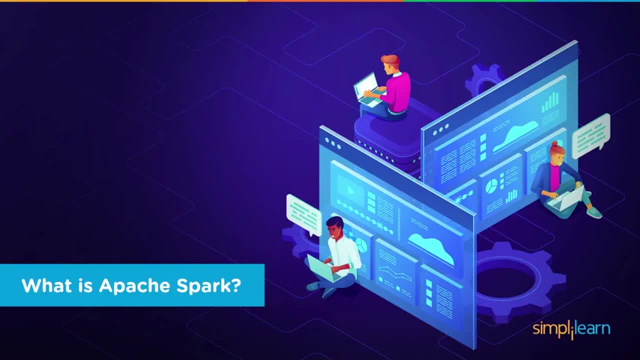 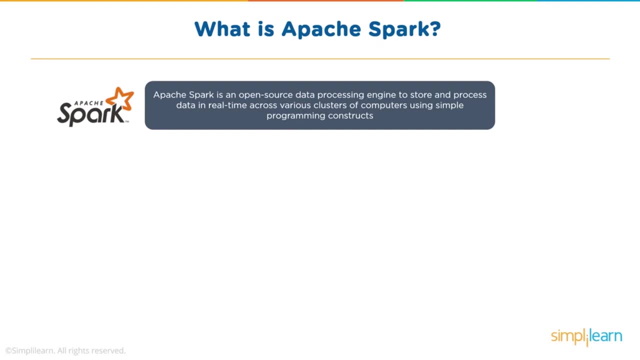 Which is used across The big data industry. so what is Apache spark? let's learn about this. Apache spark is a open source in-memory Computing framework, or you could say data processing engine, Which is used to process data in batch and also in real time across various cluster computers. 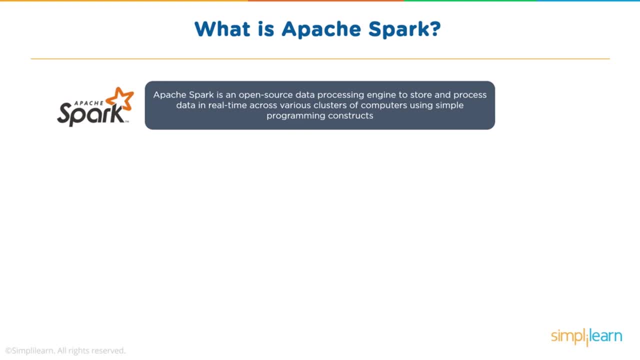 And it has a very simple programming language behind the scenes that is Scala, which is used, although if users would want to Work on spark, they can work with Python, They can work with Scala, they can work with Java and so on, even are, for that matter. So it supports all these programming languages and that's one of the reasons that it is called polyglot. 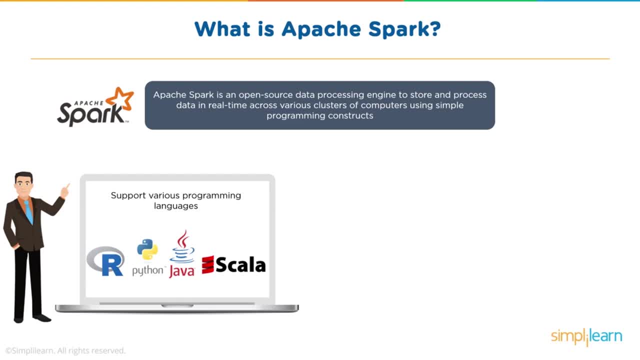 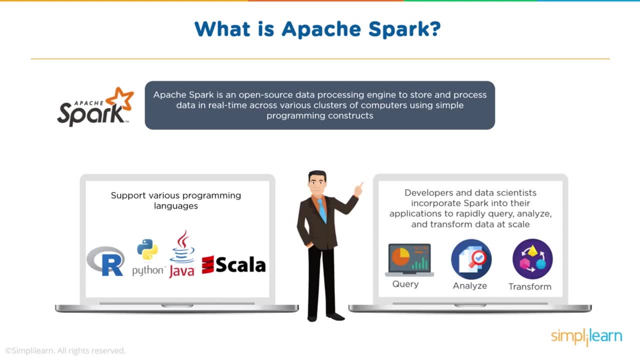 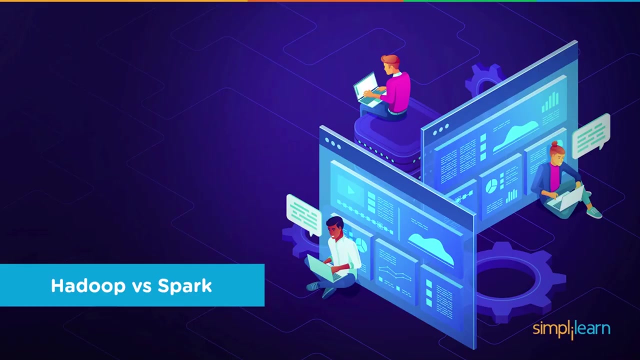 wherein you have good set of libraries and support from all the programming languages, and developers and data scientists incorporate spark into their applications or build spark based applications to process, analyze, query and Transform data at a very large scale. so these are key features of Apache spark. now, if you compare Hadoop, 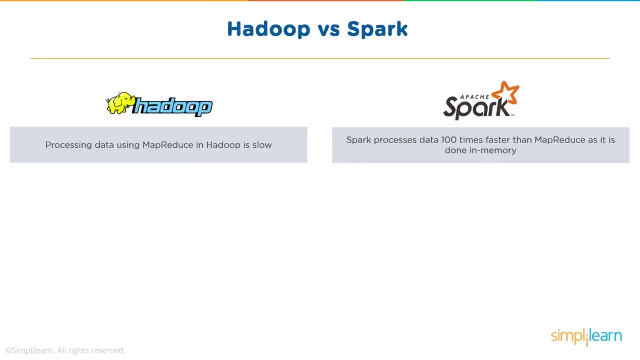 West spark. we know that Hadoop is a Framework and it basically has MapReduce, which comes with Hadoop, for processing data. However, processing data using MapReduce in Hadoop is quite slow because it is a batch oriented operation And it is time-consuming. if you, if you talk about spark, spark can process the same data. 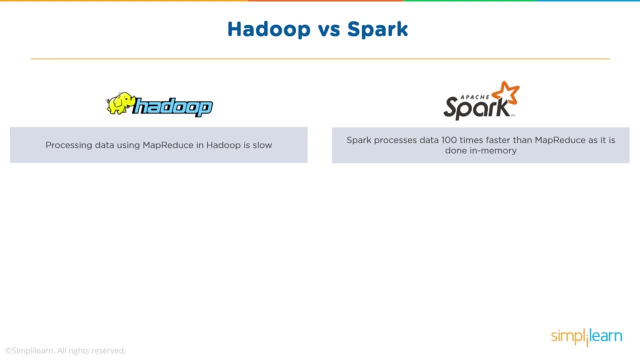 Hundred times faster than MapReduce, as it is a in-memory computing framework. Well, there can always be conflicting ideas saying: what if my spark application is not really efficiently coded and my MapReduce Application has been very efficiently coded? Well then it's a different case. However, 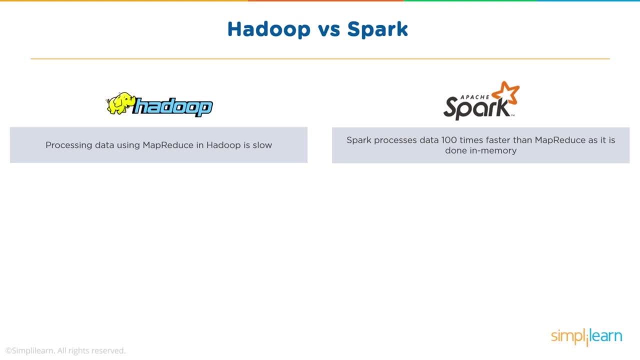 Normally, if you talk about code Which is efficiently written for MapReduce or for spark based processing, spark will win the battle by doing Almost hundred times faster than MapReduce. So, as I mentioned, Hadoop performs batch processing and that is one of the paradigms of MapReduce programming model. 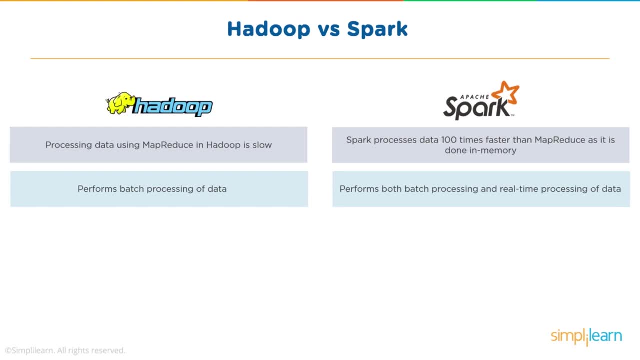 Which involves mapping and reducing, and that's quite rigid. So it performs batch processing. the intermittent data is written to HDFS and written read back from HDFS And that makes Hadoop's MapReduce processing slower. in case of spark it can perform both batch and real-time. 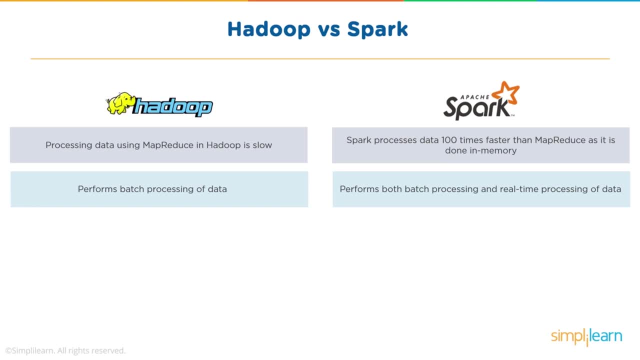 processing. however, a lot of use cases are based on real-time processing. take an example of Macy's, take an example of retail giant Such as Walmart, and there are many use cases who would prefer to do real-time processing or, I would say, near real-time processing. So when we say real-time or near real-time, 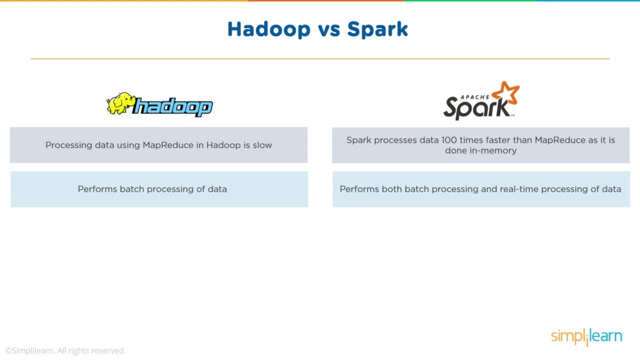 It is about processing the data as it comes in, or you're talking about streaming kind of data. now Hadoop, or Hadoop's MapReduce, obviously was started to be Written in Java. now you could also write it in Scala or in Python. However, if you talk about MapReduce, 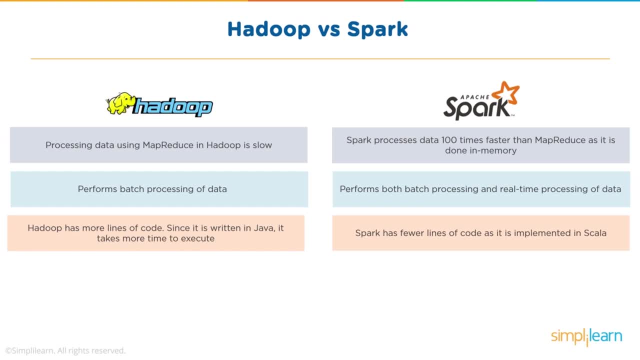 It will have more lines of code, since it is written in Java, and it will take more times to execute. You have to manage the dependencies, You have to do the right declarations, You have to create your mapper and reducer and driver classes. However, if you compare spark, it has few lines of code as it is implemented in Scala and Scala is a statically typed 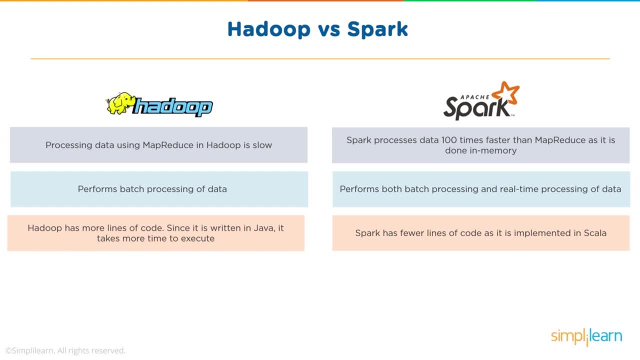 dynamically inferred Language. it's very, very concise and the benefit is it has features from both functional programming and object-oriented Language and in case of Scala, whatever code is written, that is converted into byte codes And then it runs in the JVM. now Hadoop supports Kerberos authentication. 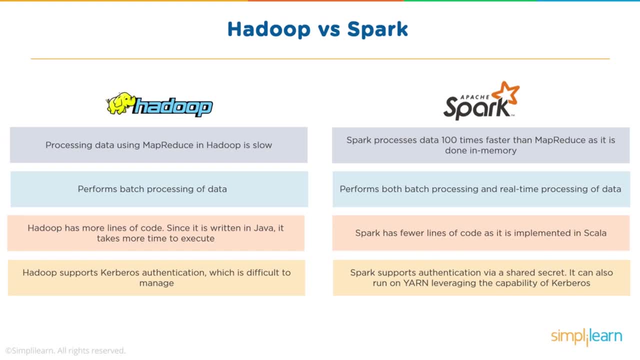 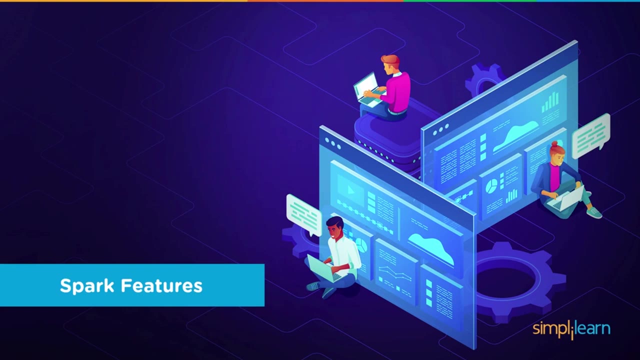 There are different kind of authentication mechanisms. Kerberos is one of the well-known ones and it can really get difficult to manage now. spark supports authentication. We are a shared secret. It can also run on yarn, leveraging the capability of Kerberos. So what are spark features? which really makes it unique or in-demand processing framework? when we talk about spark features, 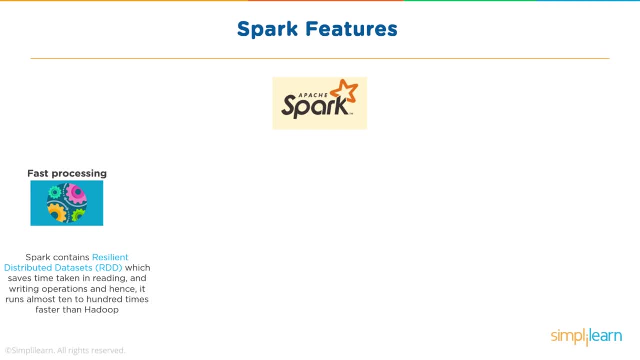 One of the key features is fast processing. So spark contains resilient Distributed datasets. So RDDs are the building blocks for spark and we learn more about RDDs later. So spark contains RDDs, Which saves huge time taken in reading and writing operations. So it can be hundred times, or you can say 10 to 100 times, faster than Hadoop when we say in memory computing. 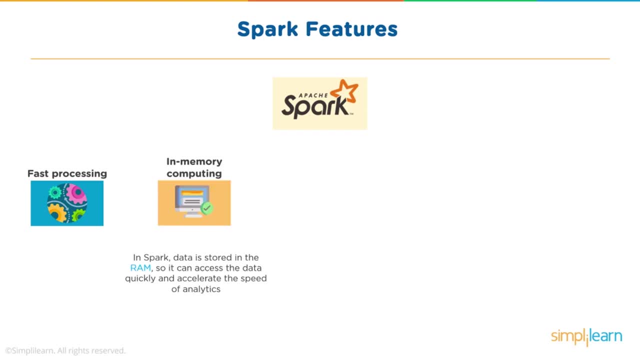 Here I would like to make a note that there is a difference between caching and in memory computing. think about it. Caching is mainly to support read-ahead mechanism, where you have your data Pre-loaded so that it can benefit further queries. However, when we say in-memory computing, 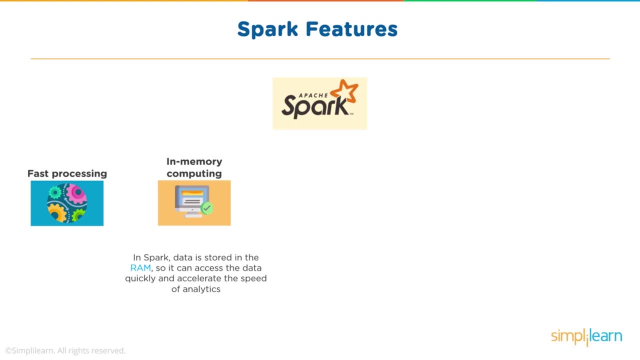 We are talking about lazy evaluation. We are talking about data being loaded into memory only, and only when a specific kind of action is invoked. So data is stored in RAM. so here we can say: RAM is not only used for processing, but it can also be used for storage and 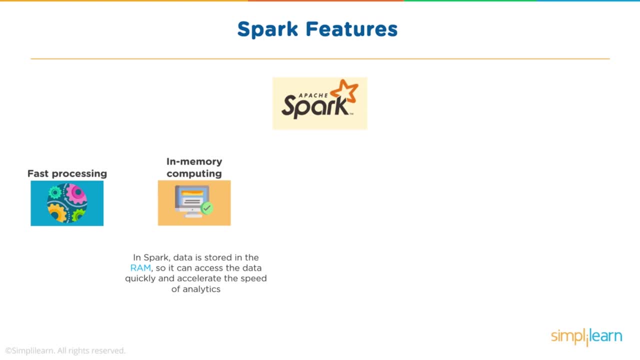 We can again decide whether we would want that RAM to be used for persistence or just for computing, So it can access the data quickly and accelerate the speed of analytics. now, Spark is quite flexible. It supports multiple languages, as I already mentioned, and it allows the developers to write applications in Java, Scala, R or Python. 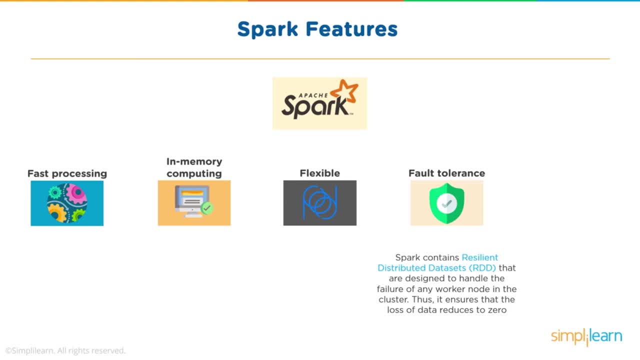 It's quite fault-tolerant. So spark contains these RDDs, or you could say execution logic, or you could say temporary data sets, Which initially do not have any data loaded, and the data will be loaded into RDDs only when execution is happening. So these can be fault-tolerant. 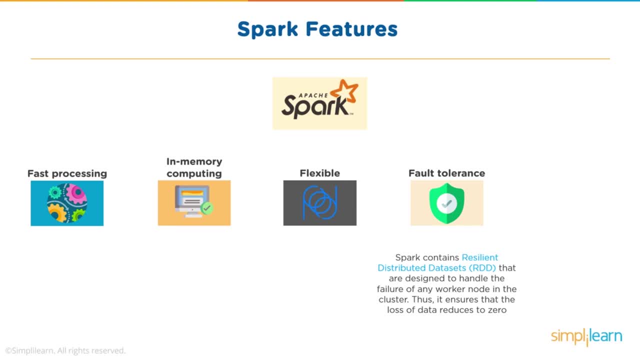 as These RDDs are distributed across multiple nodes, So failure of one worker node in the cluster will really not affect the RDDs because that portion can be Recomputed. so it ensures loss of data. It ensures that there is no data loss and it is absolutely fault tolerant. 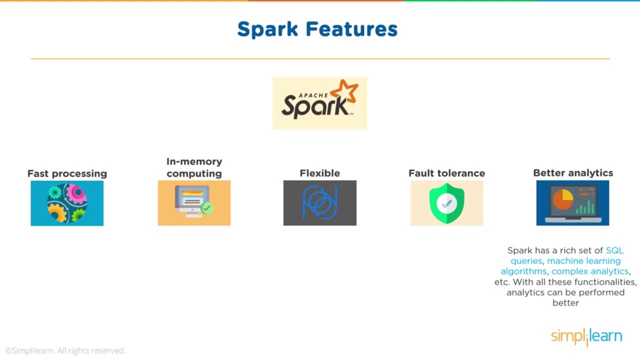 It is for better analytics. So spark has rich set of SQL queries, machine learning algorithms, complex analytics, All of this supported by various spark components which we will learn in coming slides. with all these functionalities, Analytics can be performed better in terms of spark. So these are some of the key features of spark. 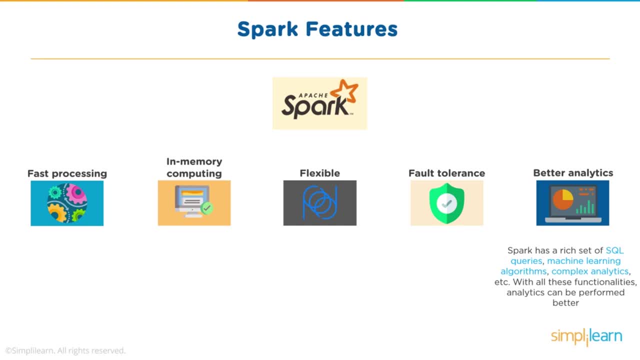 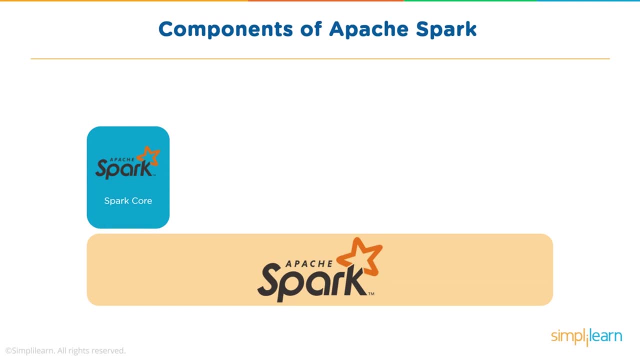 However, there are many more features which are related to different components of spark and we will learn about them. So what are these components of spark which I'm talking about? Spark core, So this is the core component which basically has RDDs, which has a core engine, and 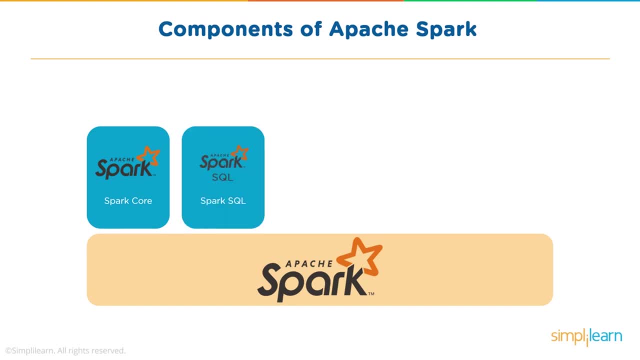 Which takes care of your processing. now You also have spark SQL, so people who would be interested in working on structured data or data Which can be Structurized would want to prefer using spark SQL, and spark SQL internally has a components or Features like data frames and data sets, which can be used to process your structured data in a much, much faster way. 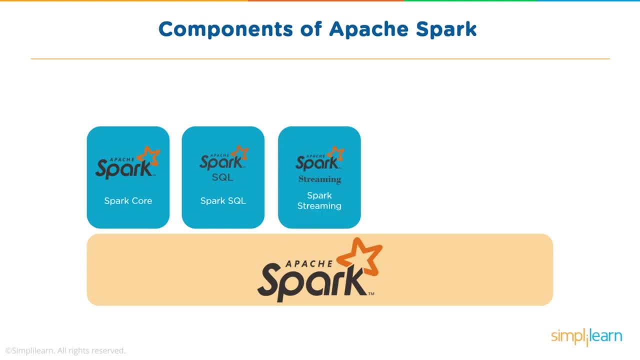 You have spark streaming now. That's again an important component of spark, which allows you to create your Spark streaming applications, which not only works on data Which is being streamed in or data which is constantly getting generated, but you would also, or you could also, Transform the data. you could analyze or process the data as it comes in in smaller chunks. 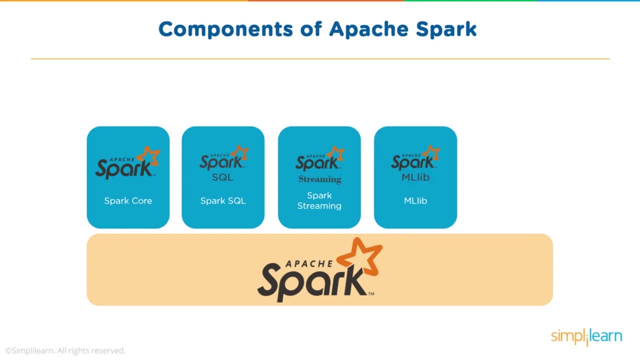 You have sparks ML lib now. This is basically a set of libraries which allows developers or data scientists to build their machine learning algorithms So that they can do predictive analytics or prescriptive, descriptive, Bm-TIV analytics, or they could build their recommendation systems or Bigger, smarter machine learning algorithms using these libraries. and then you have graphics. 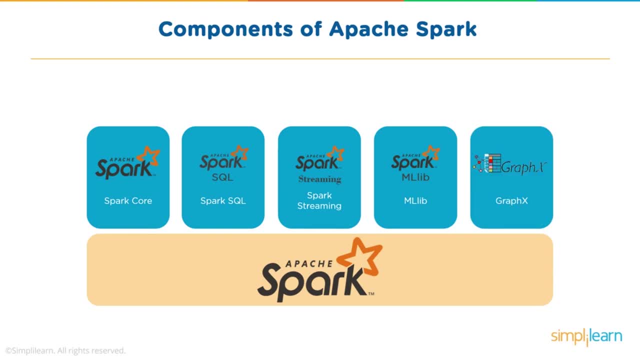 So think about organizations like LinkedIn or, say, Twitter, where you have data Which naturally has a network kind of flow, so data Which could be represented in the form of graphs. now, here, when I talk about graphs, I'm not talking about pie charts or bar charts, But I'm talking about the fact thatuck, I'm talking about some�. 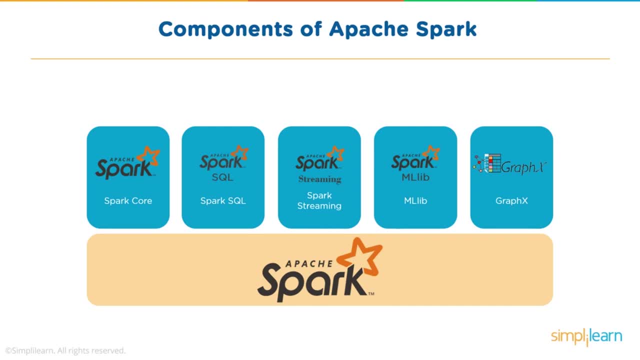 about network-related data, that is, data which can be networked together, which can have some kind of relationship. Think about Facebook, think about LinkedIn, where you have one person connected to other person or one company connected to other company. So if we have our data which can be, 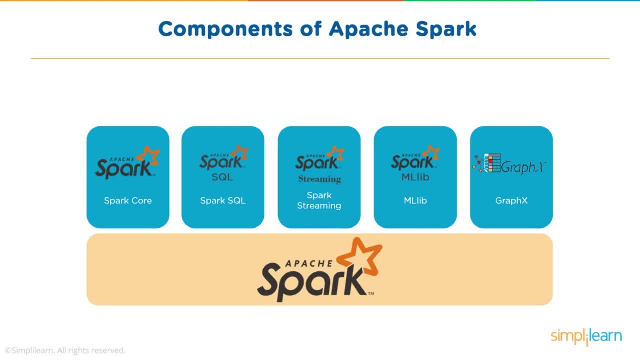 represented in the form of network graphs. then Spark has a component called GraphX which allows you to do graph-based processing. So these are some of the components of Apache, Spark, Spark Core, Spark, SQL, Spark Streaming, Spark, MLlib and GraphX. So to learn more about components of 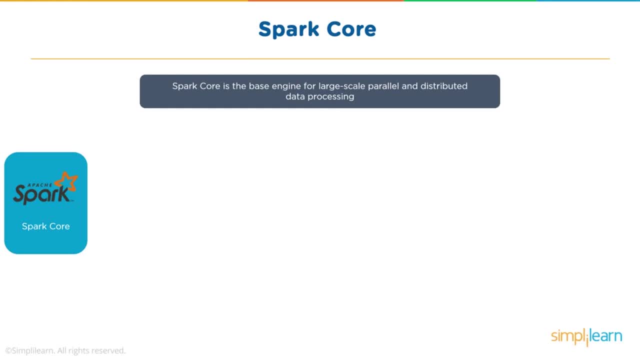 Spark. let's learn here about Spark Core. Now, this is the base engine and this is used for large-scale parallel and distributed data processing. So when you work with Spark, at least- and the minimum you would work with is Spark Core, which has RDDs as the building blocks of your Spark. So it is 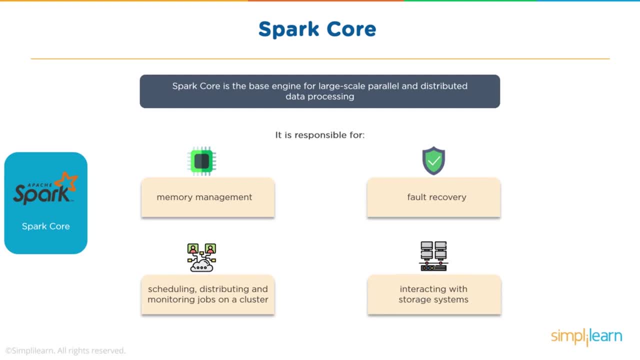 responsible for your memory management, your fault recovery, scheduling, distributing and monitoring jobs on a cluster and interacting with storage systems. So here I would like to make a key point: that Spark by itself does not have its own storage. It relies on storage. Now that 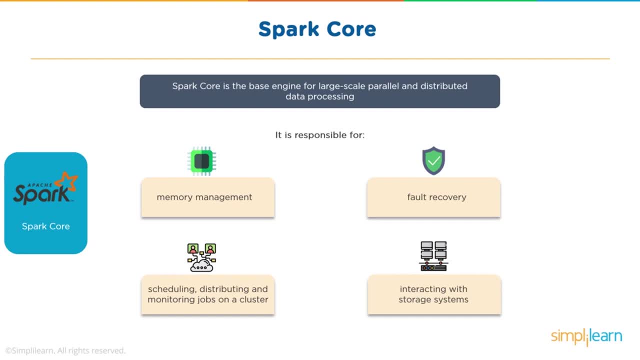 storage could be your SDFS, that is, Hadoop's distributed file system. It could be a database like NoSQL database, such as HBase, or it could be any other database, say RDBMS, from where you could connect your Spark and then fetch the data, extract the data. 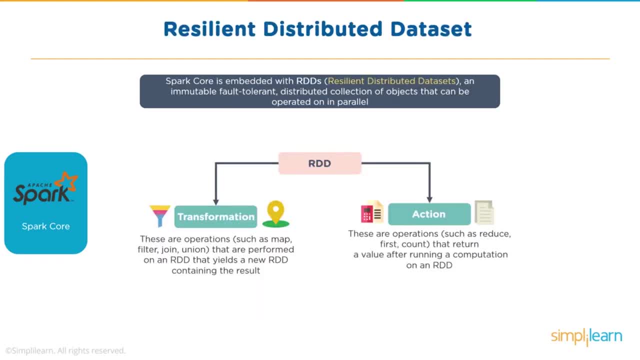 process it, analyze it. So let's learn a little bit about your RDDs, Resilient Distributed Datasets. Now Spark Core, which is the base engine, or the core engine, is embedded with the building blocks of Spark, which is nothing but your Resilient Distributed Datasets. So, as 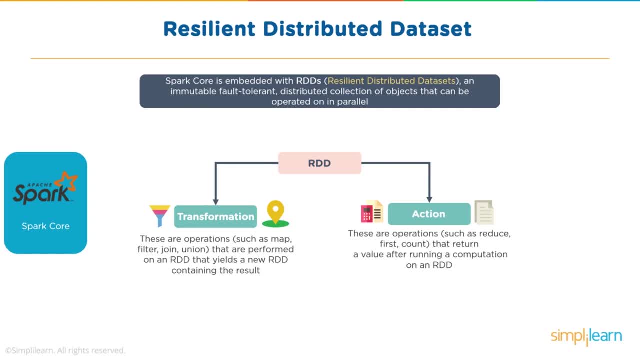 the name says it is resilient, so it is existing For a shorter period of time. distributed, so it is distributed across nodes and it is a dataset where the data will be loaded or where the data will be existing for processing. So it is. 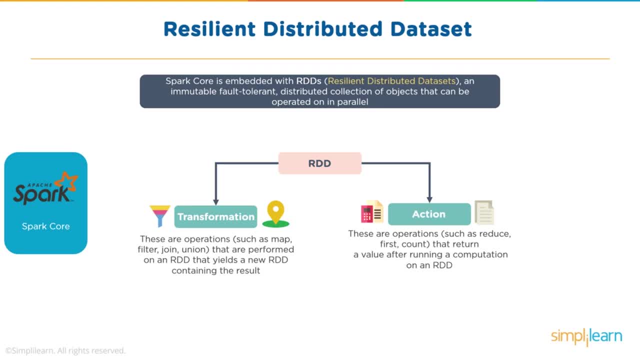 immutable, fault tolerant, distributed collection of objects. So that's what your RDD is, And there are mainly two operations which can be performed on an RDD. Now, to take an example of this, say, I want to process a particular file. Now, here I could write a simple code in Scala and that would basically mean something like this: 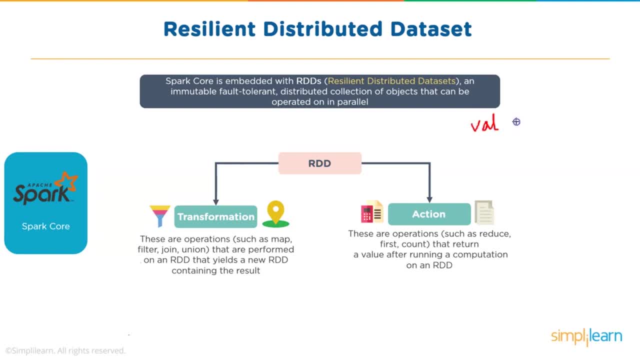 So if I say val, which is to declare a variable, I would say val x, and then I could use what we call a spark context, which is basically the most important entry point of your application. So then I could use a method of spark context- for example, that is text file, and then I could point it to a particular file. 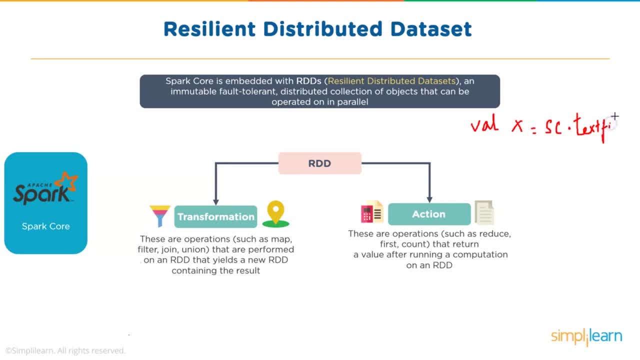 So this is just a method of your spark context, and spark context is the entry point of your application. Now here I could just give a path in this method. So what does this step do? It does not do any valuation. So when I say val x, I am creating an immutable variable and to that variable I am assigning 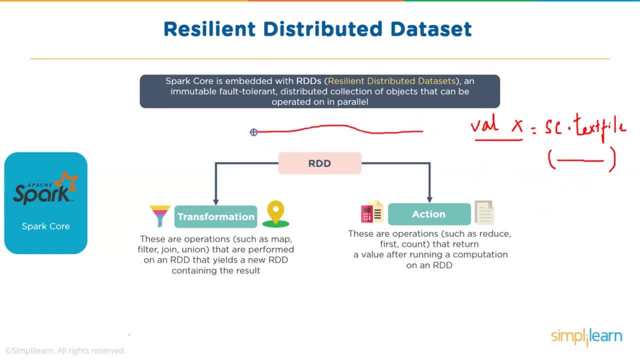 Now what this step does is it actually creates a RDD resilient distributed data set. So we can imagine this as a simple execution logic, a empty data set which is created in memory of your node. So if I would say I have multiple nodes in which my data is split and stored, imagining that your yarn, your spark, is working with Hadoop, 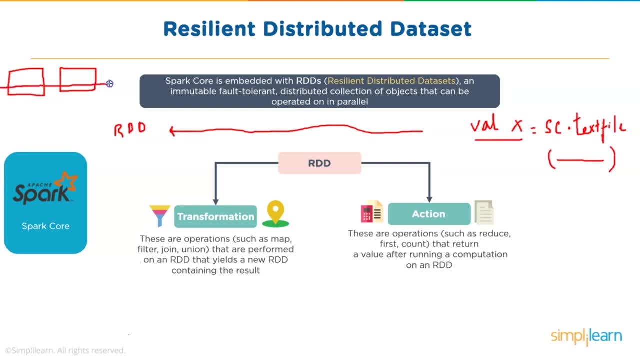 So I have Hadoop which is using, say, two nodes, And this is my distributed file system, HDFS, which basically means my file is written to HDFS and it also means that the file related blocks are stored in the underlying disk of these machines. So when I say val x equals SC dot text file, that is using a method of spark context. 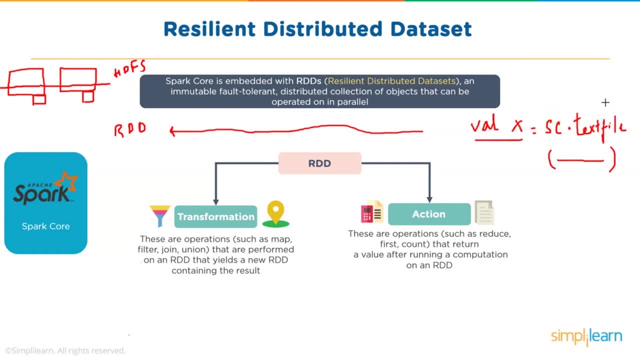 Now there are various other methods, like whole text files, parallelize and so on. This step will create an RDD, So you can imagine this as a Logical data set which is created in memory across these nodes, because these nodes have the data. However, no data is loaded here. 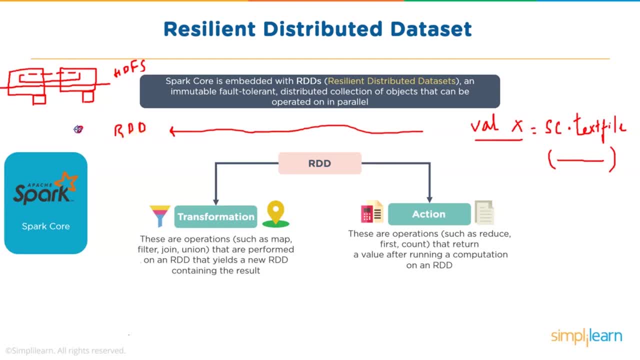 So this is the first RDD and, I can say, first step in what we call as a DAG, A DAG which will have series of steps which will get executed at later stage. Now, later, I could do further processing on this. I could say val y and then I could do something on x. 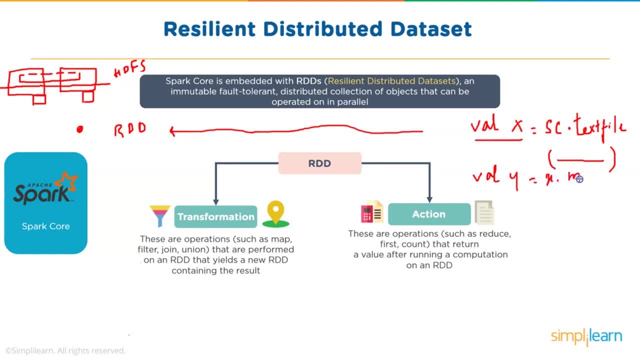 So I could Say x dot map and I would want to apply a function to every record or every element in this file and I could give a logic here: x dot map. Now this second step is again creating an RDD, a resilient distributed data set. 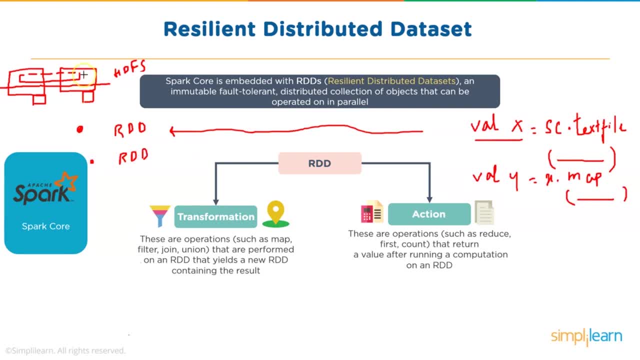 You can say: second step in my DAG, OK, And here you have a external RDD, one more RDD created which depends on the first RDD. So my first RDD Becomes the base RDD or parent RDD, and the resultant RDD becomes the child RDD. 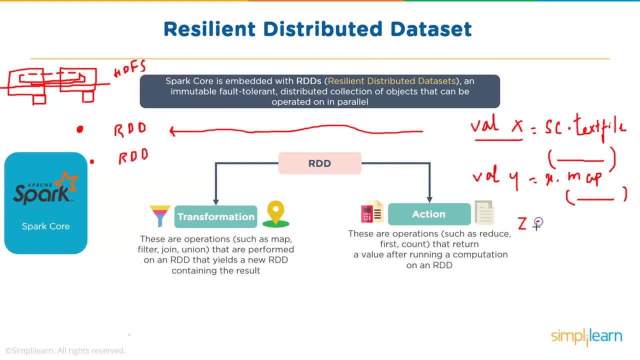 Then we can go further and we could say val z and I would say: OK, Now I would want to do some filter on y. So this filter, which I am doing here and then I could give a logic, might be: I'm searching for a word, I am searching for some pattern. 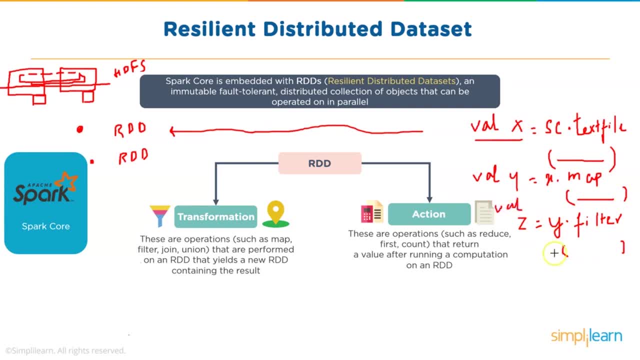 So I could say: val z equals y dot filter, which again creates one more RDD, a resilient distributed data set in memory, and a. you can say: this is nothing but one more step in the DAG. So this is my DAG, which is a series of steps which will be executed. 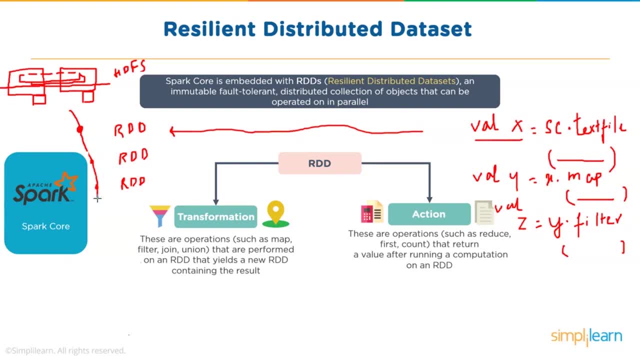 Now here: when does the execution happen? when the data get? when will the data get loaded into these RDDs? So all of this, that is, using a method using a transformation like map, using a transformation like filter or flat map or anything else, These are your transformations. 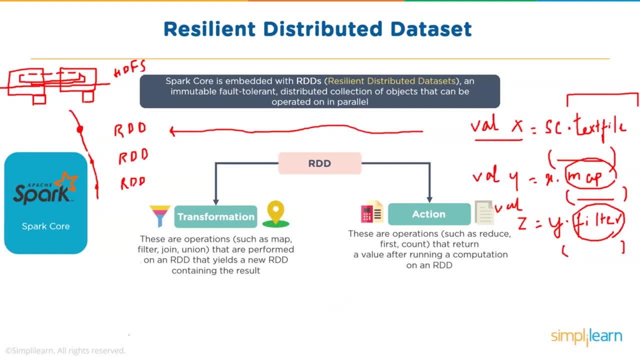 So the operations such as map filter, join, union and many others will only create RDDs, which basically means it is only creating execution logic. No data is evaluated, No operation is happening right now, Only and only when you invoke an action, that is: might be you want to print some result, might be you want to take some. 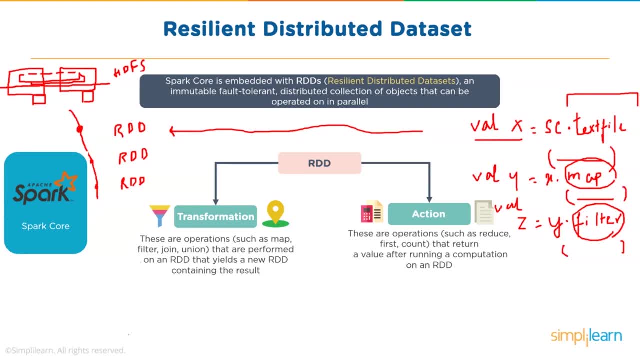 elements and see that might be you want to do a count. So those are actions which will actually trigger the execution of this DAG right from the beginning. So if I here say z dot count, where I would want to just count the number of words which I'm filtering, 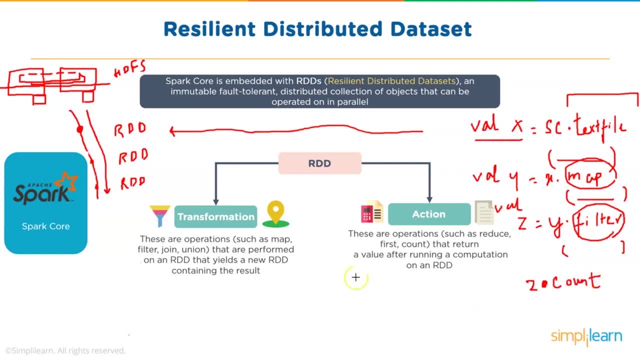 This is an action which is invoked and this will trigger the execution of DAG right from the beginning. So this is what happens in a spark: Spark. Now, if I do a z dot count again, it will start the whole execution of DAG again, right from the beginning. 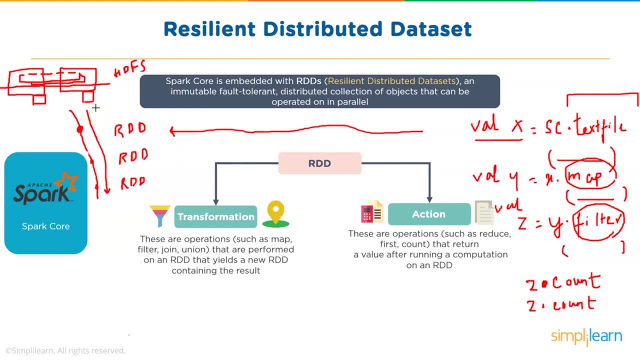 So my z dot count. second time an action is invoked again, The data will be loaded in the first RDD, Then you will have map, then you will have filter and finally you will have result. So this is the core concept of your RDDs and this is how RDD works. 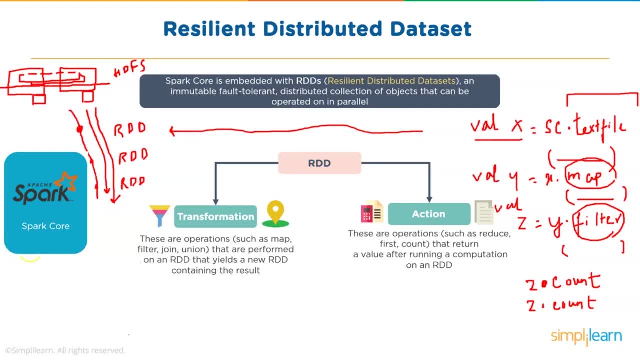 So, mainly in spark, there are two kind of operations. One is your transformations and one is your actions. Transformations, or using a method of spark context, will always and always create an RDD, or, you could say, a step in the DAG. Actions are something which will invoke the execution, which will invoke the execution from the first RDD till the last RDD where you can get your result. 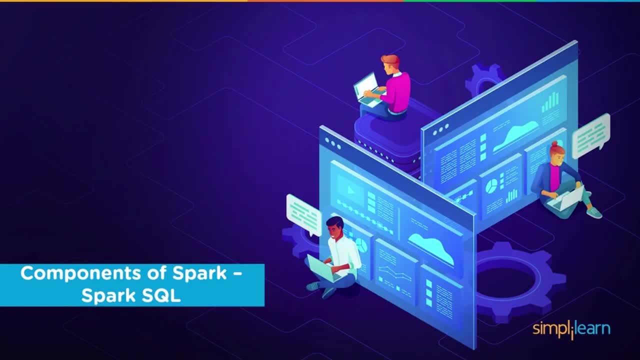 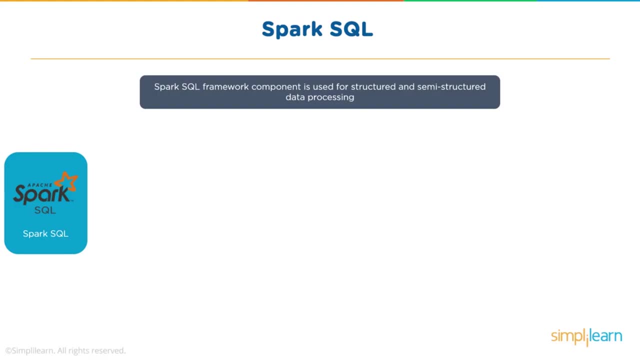 So this is how your RDDs work. Now, If we talk about components of spark, let's learn a little bit about Spark SQL. So Spark SQL is a component type processing framework which is used for structured and semi structured data processing. So usually people might have their structured data stored in RDBMS or in files, where data is structured with particular delimiters and has a pattern. 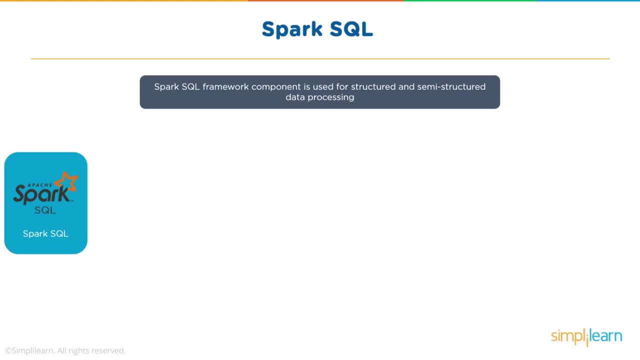 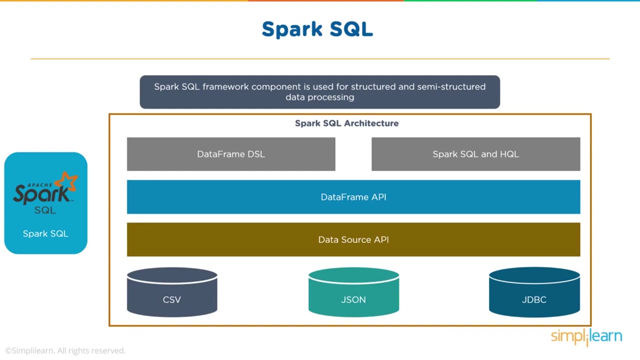 And if one wants to process this structured data, if one wants to use Spark to do in memory processing and work on this structured data, they would prefer to use Spark SQL. So you can work on different data formats, say CSV, JSON. You can even work on smarter formats like Avro Parquet, even your binary files or sequence files. 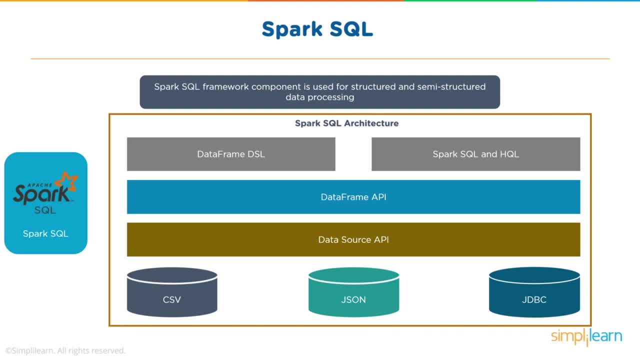 You could have your data coming in from an RDBMS, which can then be extracted using a JDBC connection. So, at the bottom level, when you talk about Spark SQL, it has a data source API Which basically allows you to get the data in whichever format it is. 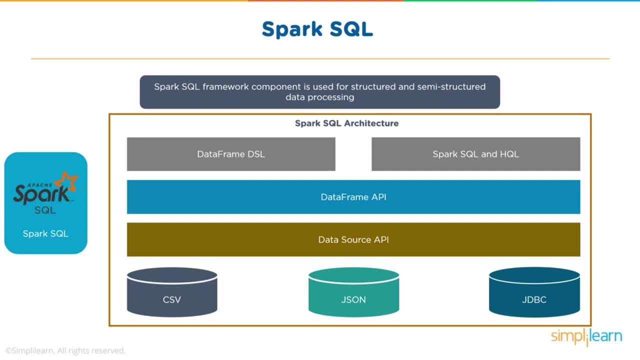 Now Spark SQL has something called as data frame API. So what are data frames? Data frames, in short, you can visualize or imagine as rows and columns, or if your data can be represented in the form of rows and columns with some column headings. So data frame API allows you to create data frames. 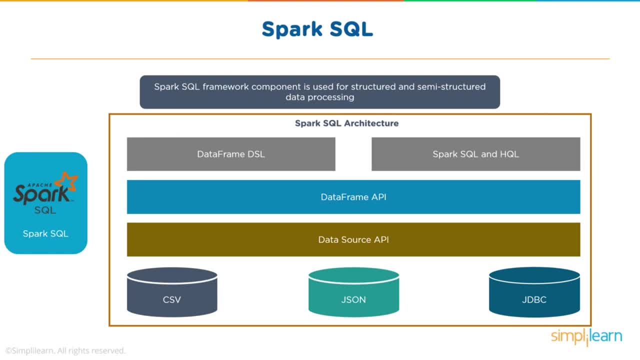 So, like my previous example, when you work on a file, When you want to process it, you would convert that into an RDD using a method of Spark context or by doing some transformations. So, in the similar way, when you use data frames or when you want to use Spark SQL, you would use Sparks context, which is SQL context, or Hive context, or Spark, which allows you to work with data frames. 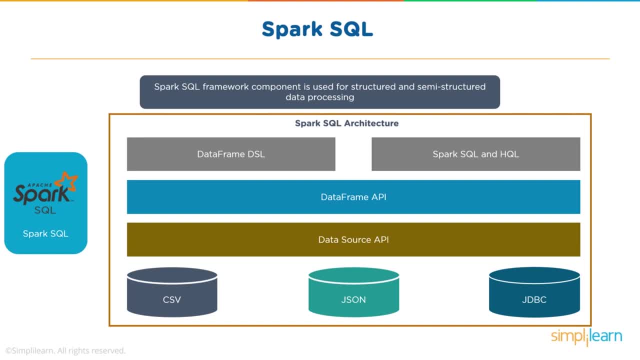 So, like in my earlier example, we were saying: val x equals sctextfile. Now, in case of data frames, instead of sc you would be using, say, Spark dot something. So Spark context is available for your data frames API to be used. In older versions like Spark 1.6 and so on, we were using Hive context or SQL context. 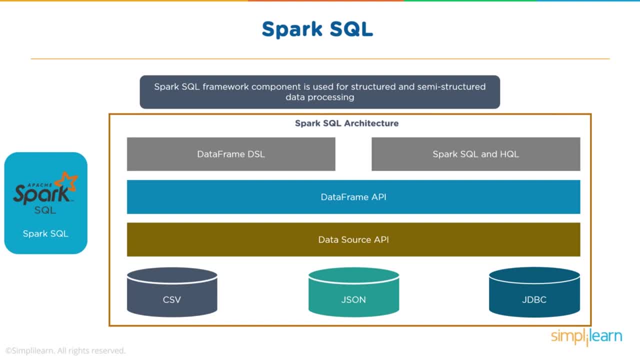 So if you were working with Spark 1.6, you would be saying val x equals SQL context dot. Here we would be using Spark dot. So data frame API basically allows you to create data frames out of your structured data, which also lets Spark know that data is already in a particular structure. 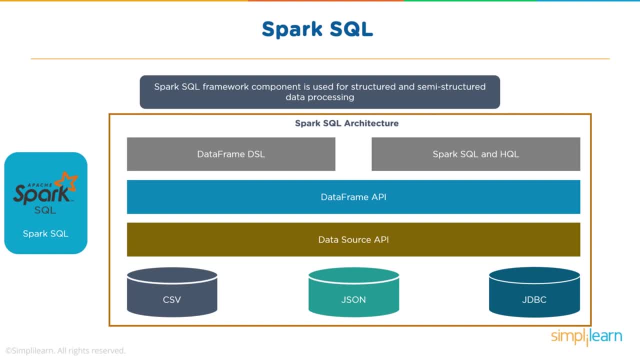 It follows a format and based on that, your Sparks back end DAG scheduler right. So when I say about DAG, I talk about your sequence of steps. So Spark is already aware of what are the different steps involved in your application. So your data frame API basically allows you to create data. 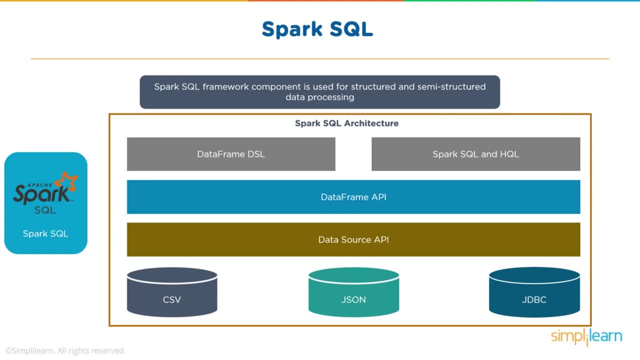 Frames out of your data and data frames. When I say, I'm talking about rows and columns with some headings, and then you have your data frame, DSL language, or you can use Spark SQL or Hive query language. Any of these options can be used to work with your data frames. 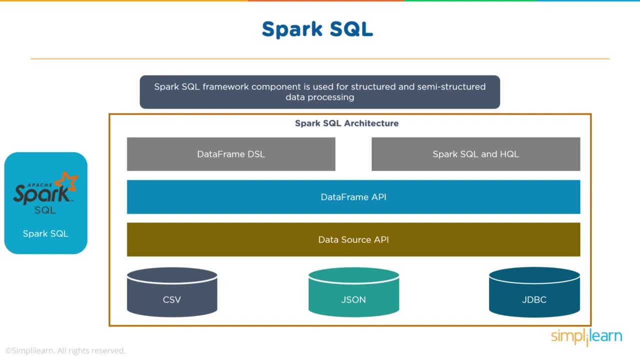 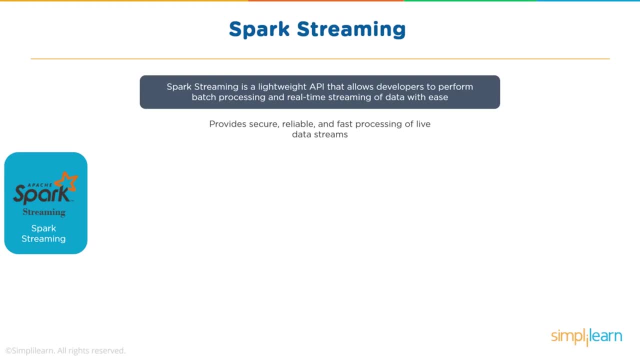 So to learn more about data frames, follow in the next sessions. when you talk about Spark streaming, Now this is very interesting for organizations who want to work on streaming data. Imagine a store like Macy's where they would want to have machine learning algorithms. Now, what would these machine learning algorithms do? 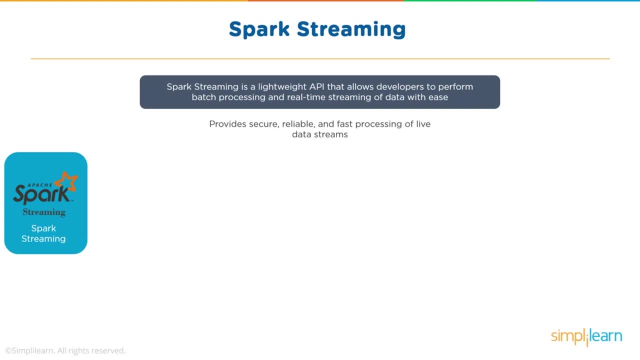 Suppose you have a lot of customers walking in the store and they are searching for a particular product or a particular item, So there could be cameras placed in the store, and this is being already done. There are cameras placed in the store which will keep monitoring in which corner of the store there are more customers. 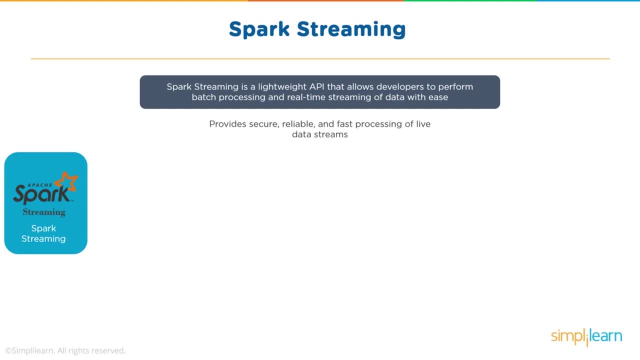 Now, once Camera captures this information, this information can be streamed in to be processed by algorithms, and those algorithms will see which product or which series of product customers might be interested in And if this algorithm, in real time, can process based on the number of customers, based on the available product in the store, it can come up with a attractive alternative price so that which the price can be displayed on the screen and 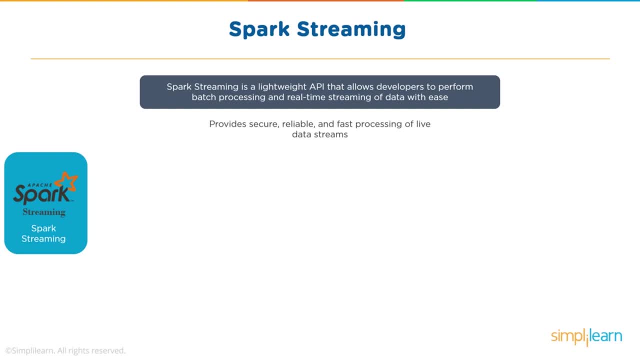 And probably customers would buy the product. Now, this is a real time processing, where the data comes in, algorithms work on it, do some computation and give out some result, and which can then result in customers buying a particular product. So the whole essence of this machine learning and real time processing will really hold good if and when customers are in the store. or this could relate to even an online shopping portal where there might be machine learning algorithms. 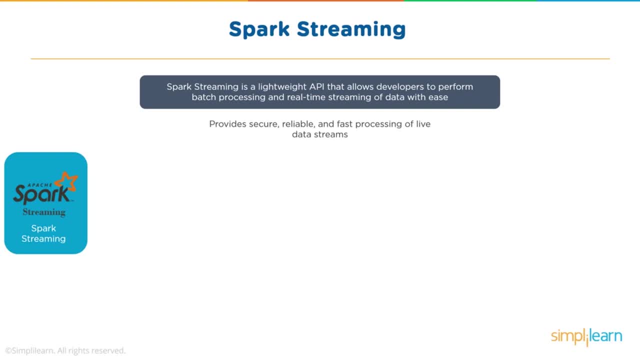 Which might be doing real time processing based on the clicks which customer is doing. based on the clicks, based on customer history, based on customer behavior, algorithms can come up with recommendation of products or, better, altered price so that the sale happens. now, in this case, we would be seeing the essence of real time processing only in a fixed or in a particular duration of time. 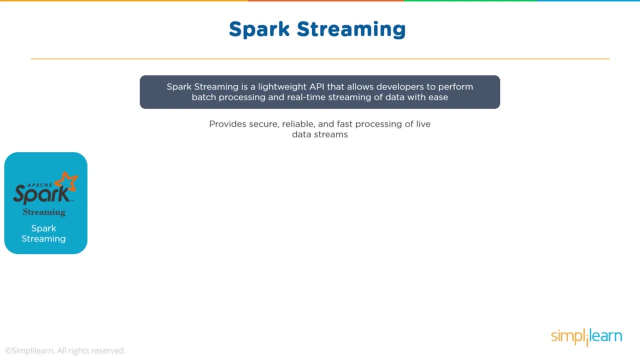 And this also means that you should have Something which can process the data as it comes in. so spark streaming is a lightweight API that allows developers to perform batch processing and also real time streaming and processing of data, so it provides secure, reliable, fast processing of live data streams. 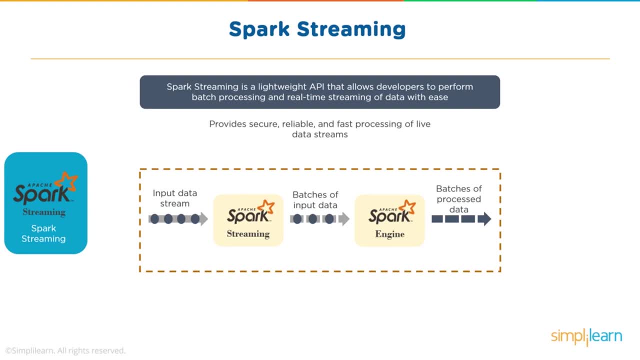 So what happens here in spark streaming? in brief, so you have a input data stream. now that data stream could be a file which is constantly getting upended. it could be some kind of metrics, it could be some kind of Even Events, based on the clicks which customers are doing or based on the products which they are choosing in a store. this input data stream is then pushed in through a spark streaming application. now spark streaming application will broke, break this content into smaller streams, what we call as this criticize streams or batches of smaller data on which processing can happen in frames. so you could say: process my file every five seconds for the latest data which has come in. now there are 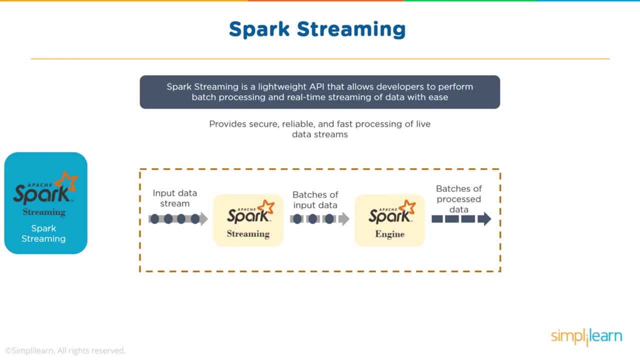 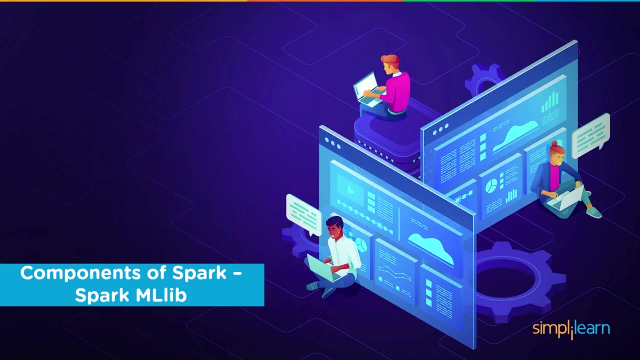 Also some windows based Options like when I say windows, I mean a window of fast three events, window of past three events, each event being of five seconds. so your batches of smaller data is processed by spark engine and this process data can then be stored or can be used for further processing. so that's what spark streaming does. when you talk about ml live, it's a low level machine learning library that is simple to use. 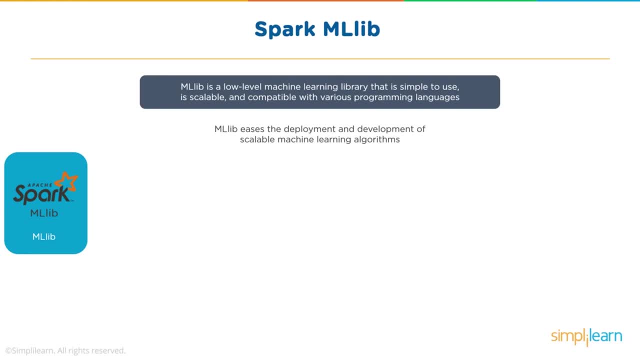 Scalable and compatible with various programming languages. now, hadoop also has some libraries. like you have a patchy mahout which can be used for machine learning algorithms. however, in terms of spark, we are talking about machine learning algorithms which can be built using ml libs libraries and then spark can be used for processing. so ml libs eases the deployment and development of scalable machine learning algorithms. I mean think about your clustering techniques. 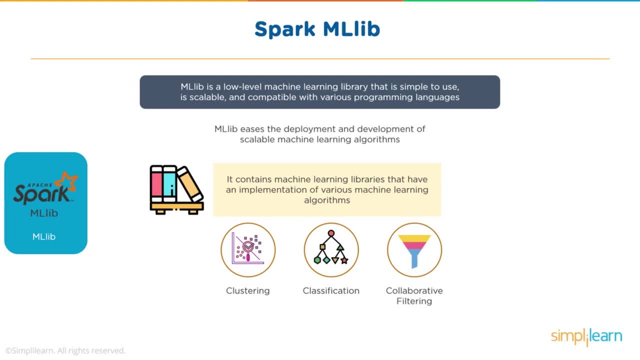 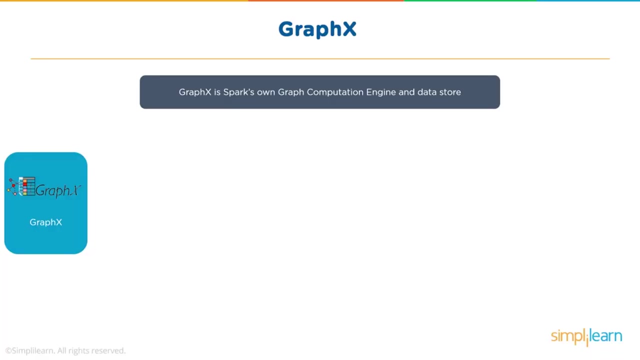 Think about Facebook, think about LinkedIn, where you can have your data which can be stored, and that data has some kind of network connections or you could say it is well networked. 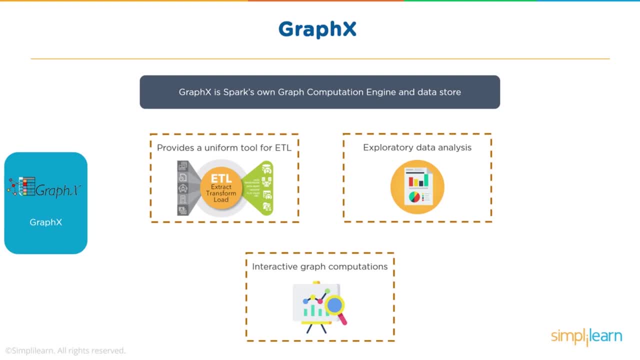 being connected and the connection between these are called edges. So I could say A is friend to B, So A and B are vertices and friend, a relation between them, is the edge. Now, if I have my data which can be represented in the form of graphs, if I would want to do a processing in such way, 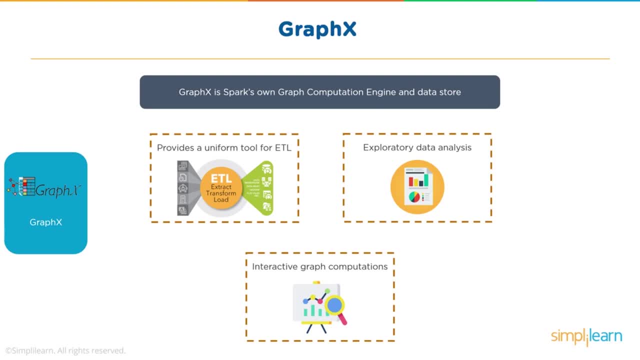 this could be not only for social media. it could be for your network devices, it could be a cloud platform, it could be about different applications which are connected in a particular environment. So if you have data which can be represented in the form of graph, then graphics can be used to. 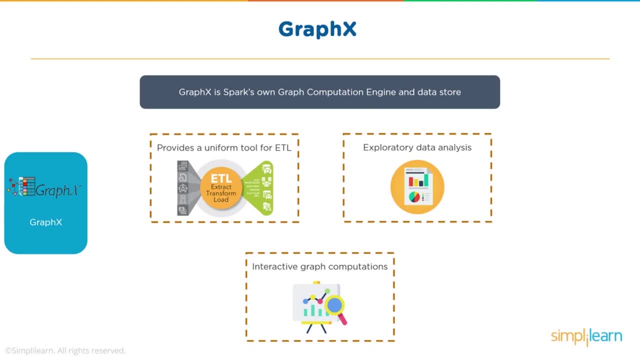 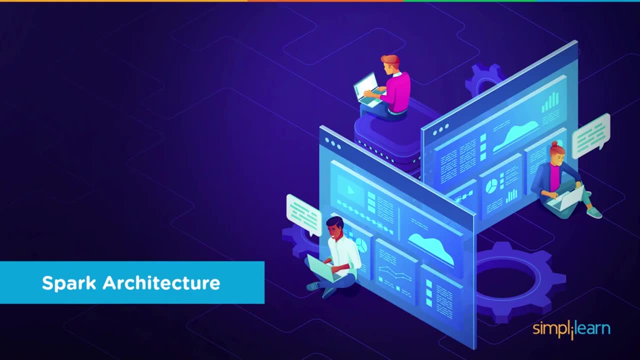 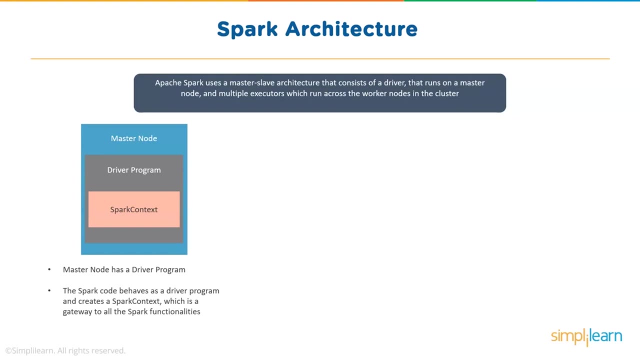 do ETL, that is, extraction, transformation load to do your data analysis and also do interactive graph computation. So graphics is quite powerful. Now, when you talk about Spark, your Spark can work with your different clustering technologies. So it can work with a. 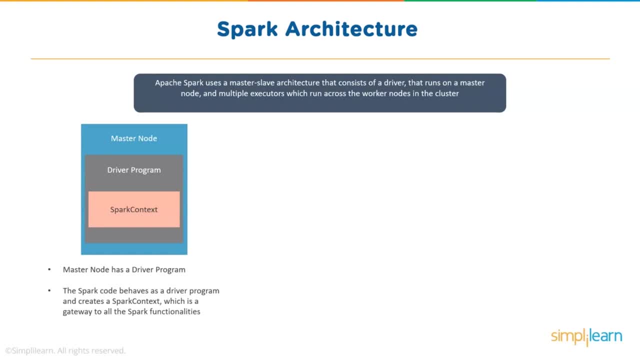 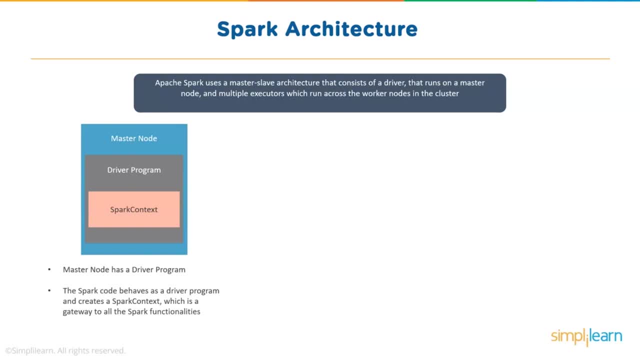 Mesos. Spark can work with YARN, which is usually you will see in different working environments. Spark can also work as standalone, that means without Hadoop. Spark can have its own setup with master and worker processes. So usually, or you can say technically, Spark uses a master. 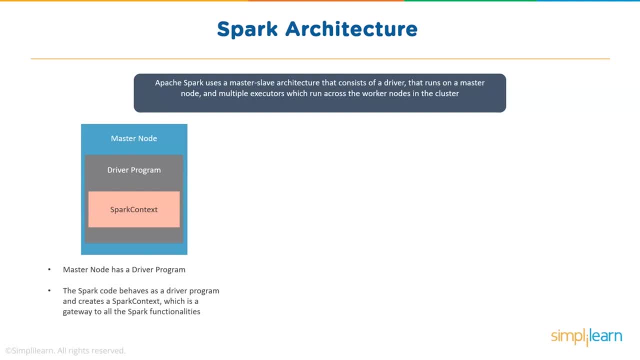 slave architecture. Now, that consists of a driver program that can run on a master node. It can also run on a client node, It depends on how you have configured or what your application is. and then you have multiple executors which can run on worker nodes. So your master node- 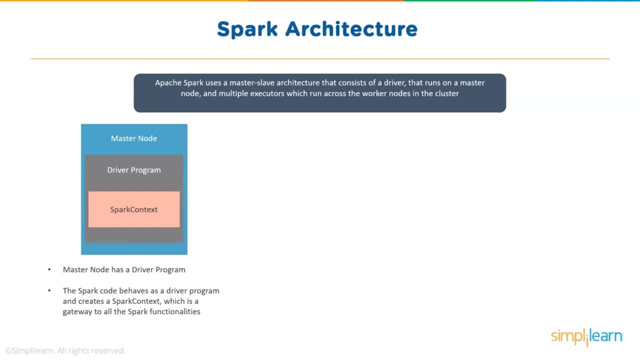 has a driver program and this driver program internally has the spark context. So your spark, every spark application, will have a driver program and that driver program has a inbuilt or internally use spark context, which is basically your entry point of application for any spark functionality. 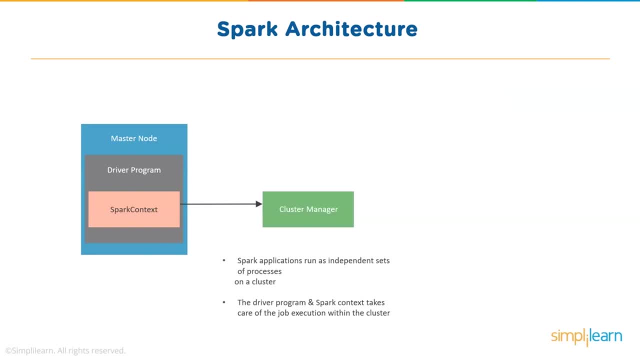 So your driver or your driver program interacts with your cluster manager. Now, when I say interacts with cluster manager, so you have your spark context, which is the entry point that takes your application request to the cluster manager. Now, as I said, your cluster manager could be say: 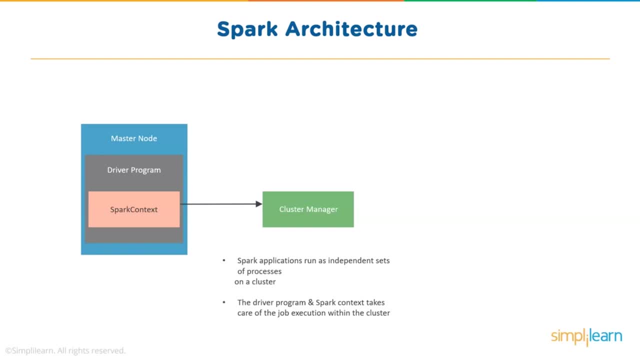 Apache mesos, it could be yarn, it could be spark standard loan master itself. So your cluster manager, in terms of yarn, is your resource manager. So your spark application internally runs as series or set of tasks and processes. Your driver program, wherever that is run, will have a spark context and spark context will take care of your application. 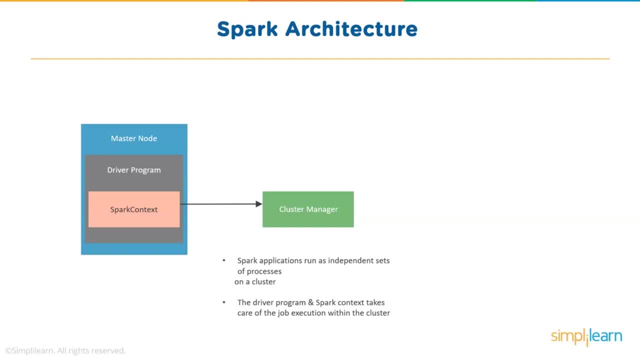 execution. How does that do it? Spark context will talk to cluster manager. So your cluster manager could be yarn and in terms of access to that data, you can call your Yoioscope dot org application. So terms of when i say cluster manager for yarn would be resource manager. so at high level we can say: 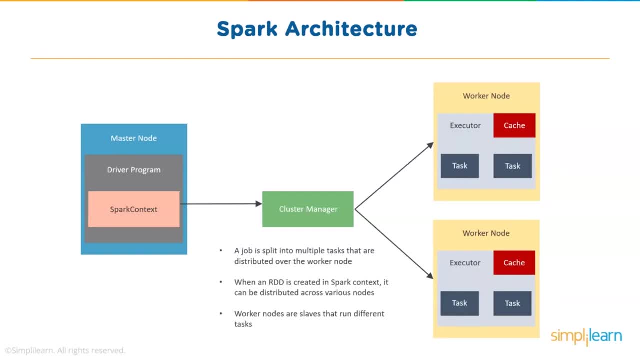 a job is split into multiple tasks and those tasks will be distributed over the slave nodes or worker nodes. so whenever you do some kind of transformation or you use a method of spark, context and rdd is created and this rdd is distributed across multiple nodes, as i explained earlier. worker. 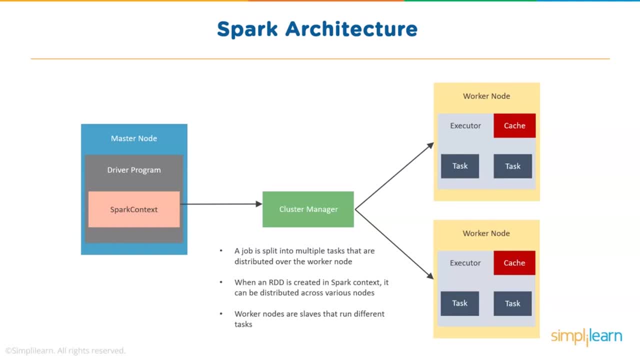 nodes are the slaves that run different tasks. so this is how a spark architecture looks like. now we can learn more about spark architecture and its interaction with yarn. so usually what happens when your spark context interacts with the cluster manager? so in terms of yarn, i could say resource manager. now we already know about yarn, so you would have say node managers running. 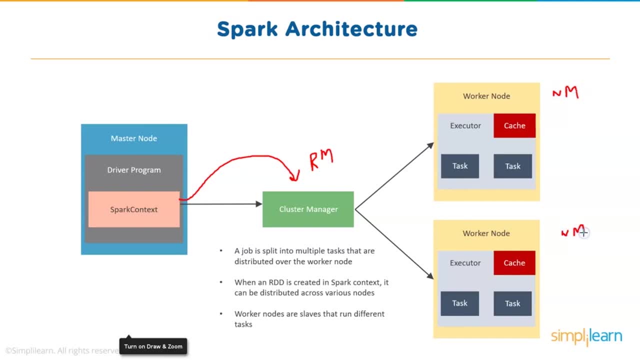 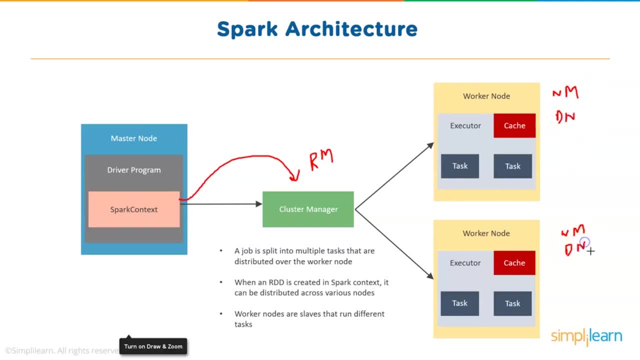 which obviously are there to have the hadoop related data. so whenever the application wants to process the data, your application, via spark context, contacts the cluster managers. that is resource manager. now what does resource manager do? resource manager makes a request, so resource manager makes request to the node manager of the machines wherever the relevant data resides. ask: 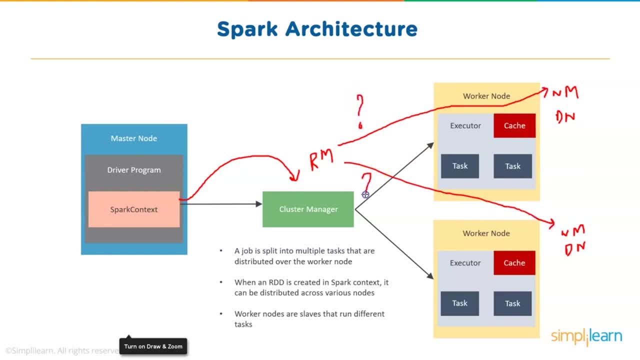 for containers. so your resource manager is negotiating or asking for containers from node manager saying, hey, can i have a container of one gb ram and one cpu core? can i have a container of one gb ram and one cpu core? and your node manager, based on the kind of processing it is doing, will. 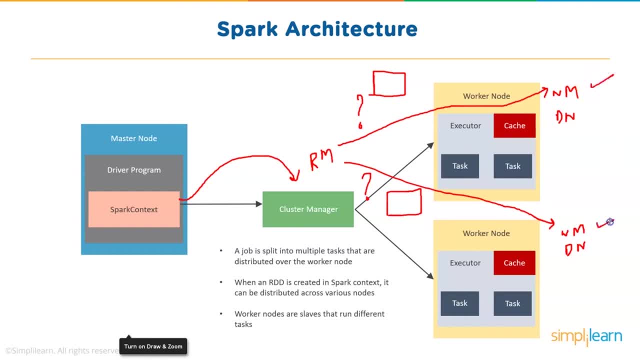 approve or deny it. so node manager would say: fine, i can give you the container. and once this container is allocated or approved by node manager, resource manager will basically give you the container and basically start an extra piece of code called app master. so app master is responsible. 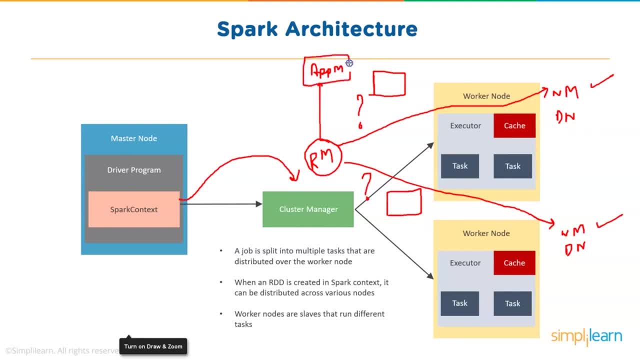 for execution of your applications, whether those are spark applications or map reduce. so your application master, which is a piece of code, will run in one of the containers, that is, it will use the ram and cpu core and then it will use the other containers which were allocated by node. 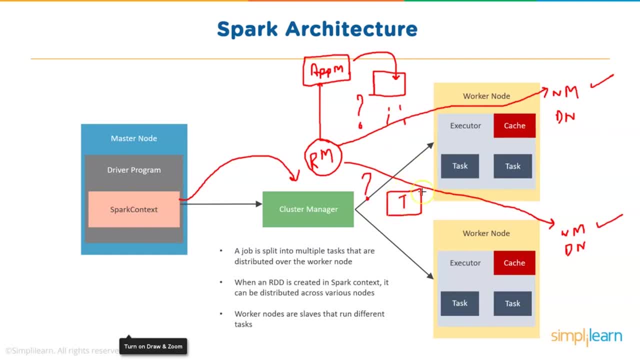 manager to run the tasks, so it is within this container which can take care of execution. so what is a container? combination of ram and cpu core? so it is within this container. we will have a executor process which would run and this executor process is taking care of your application related tasks. 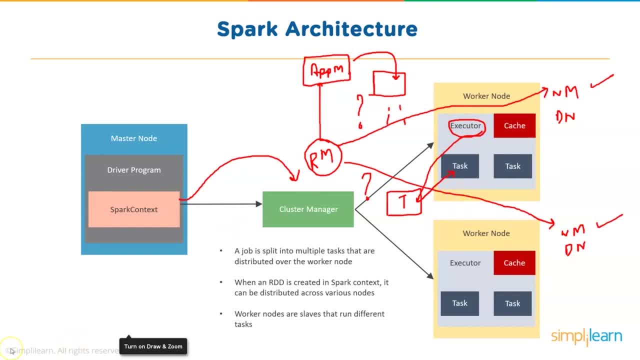 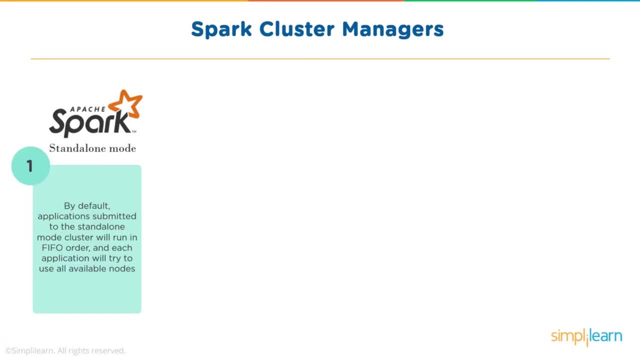 so that's how overall spark works in integration with yarn. now let's learn about this spark cluster managers. as i said, spark can work in a standalone mode, so that is without hadoop. so, by default, application submitted to spark standalone node cluster will run in fifo order and each application will try to use all the available. 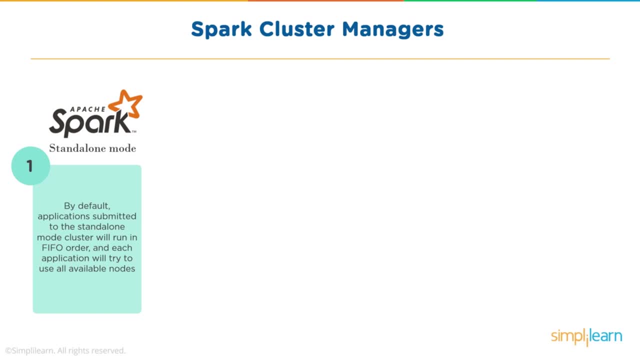 nodes. so you could have a spark standalone cluster, which basically means you could have multiple nodes. on one of the nodes you would have the master process running, and on the other nodes you would have the spark worker processes running. so here we would not have any distributed file. 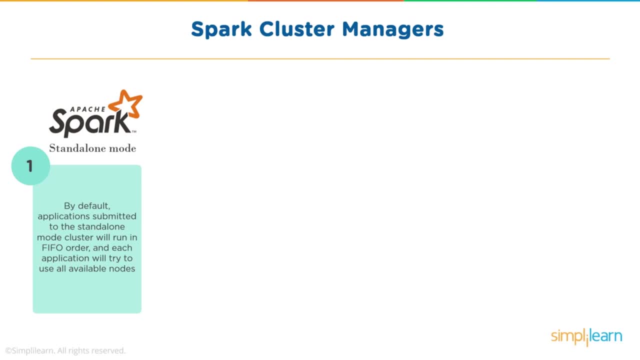 system because spark is standalone and it will rely on an external storage to get the data or probably the file system of the node to run both cases. so first knob means we will be running fivo on another node, first node distinctly, just for this Beati in the node to load on the node and if nothing else, you can save the apps. if you have any spec, jusqu. fox or type in directly to at the top and then if anything else, we do not have an extra location. so work that out. so that will actually be leveled up for you because you need only you know that for each of them, not a runout. 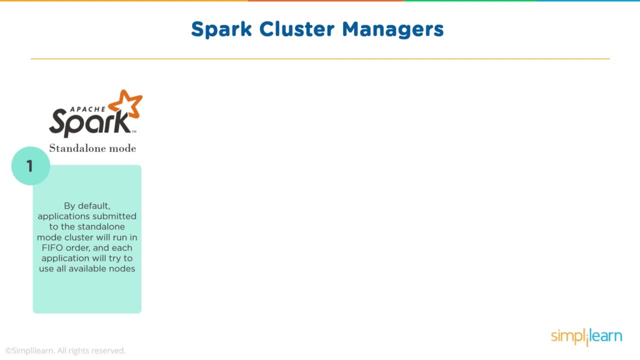 nodes where the data is stored, and processing will happen across the nodes where your worker processes are running. You could have Spark working with Apache Mesos. Now, as I said, Apache Mesos is an open source project to manage your computer clusters and can also run Hadoop. 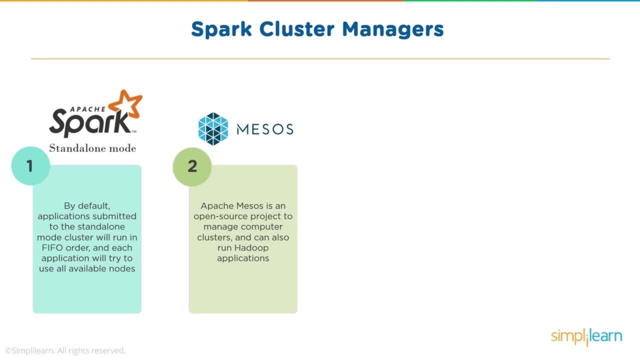 applications. Apache Mesos was introduced earlier and Spark came in and has existence. to prove the credibility of Apache Mesos, You can have Spark working with Hadoop's YARN. This is something which widely, you will see in different working environments. So YARN, which takes care of your. 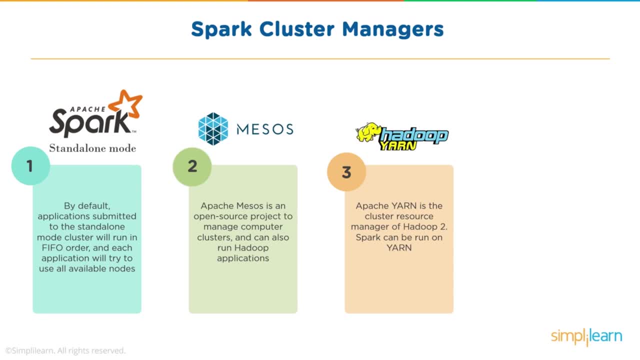 processing and can take care of different processing frameworks. also supports Spark. You could have Kubernetes Now. that is something which is making a lot of news in today's world. It is an open source system for automating deployment, scaling and management of containerized 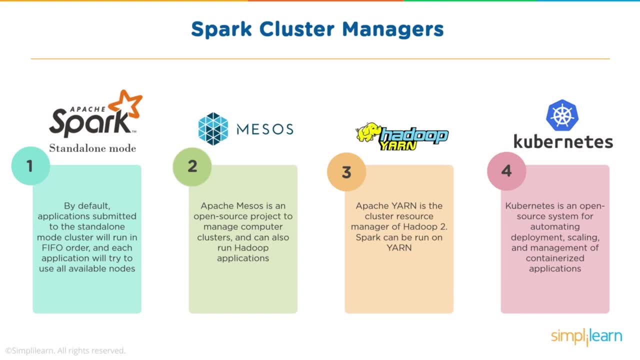 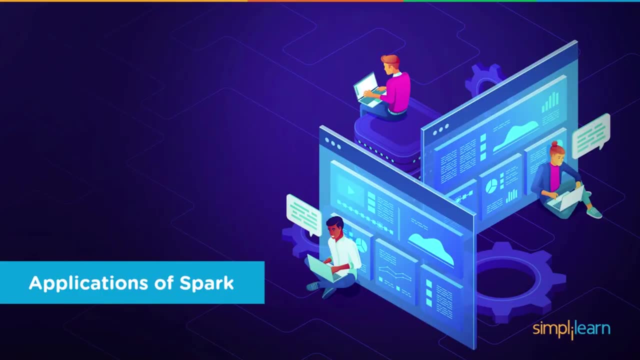 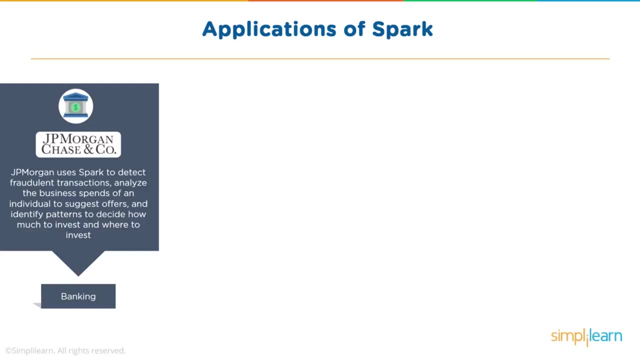 applications. So where you could have multiple Docker based images which can be connecting to each other. So Spark also works with Kubernetes. Now let's look at some applications of Spark. So JPMorgan Chase and company uses Spark to detect fraudulent transactions, analyze the business spends of an individual, to suggest offers and identify patterns to decide. 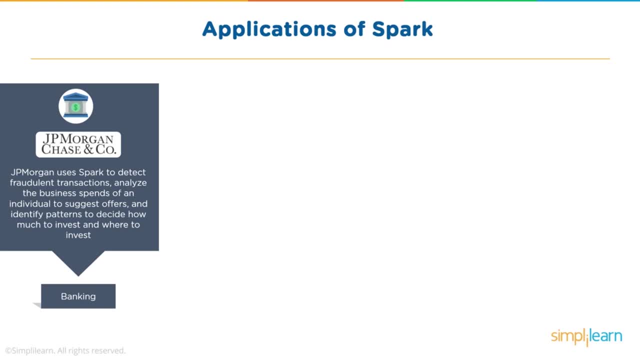 how much to invest and where to invest. So this is one of the examples of banking. A lot of banking is using Spark to detect fraudulent transactions, So this is one of the examples of banking. A lot of banking is using Spark to detect fraudulent transactions, So this is one of 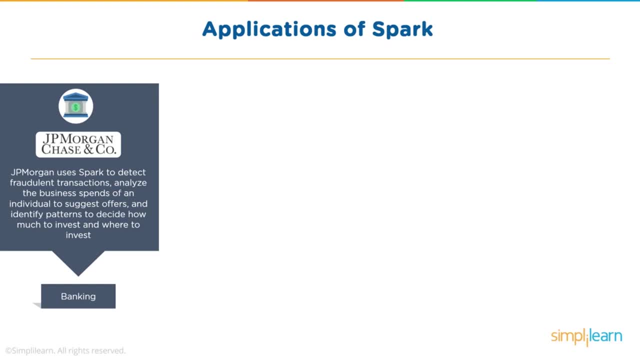 banking environments are using Spark due to its real-time processing capabilities and in-memory faster processing, where they could be working on fraud detection or credit analysis or pattern identification and many other use cases. Alibaba group that uses also Spark to analyze large data sets of data, such as real-time transaction details. Now that might be based online or in the. 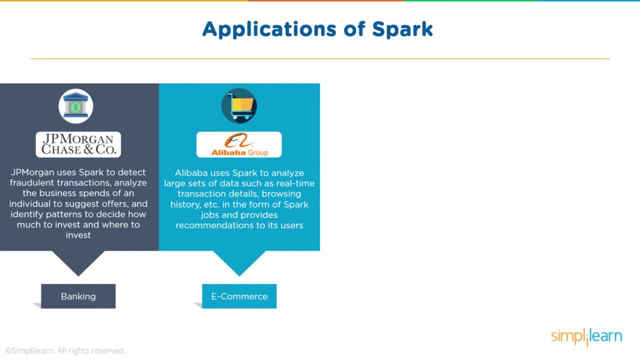 stores Looking at the browsing history in the form of Spark jobs, and then provides recommendations to its users. So Alibaba group is using Spark in its e-commerce domain. You have IQ Now. this is a leading healthcare company that uses Spark to analyze patients' data, identify possible health issues and diagnose it based on. 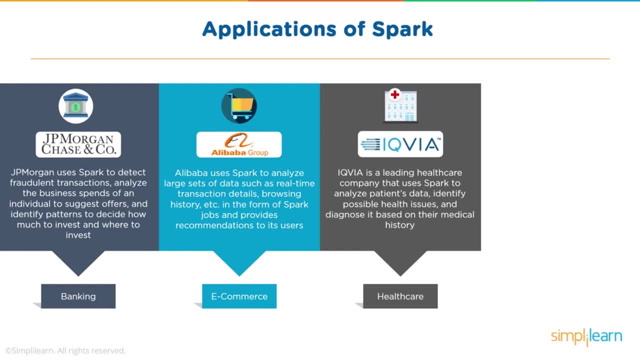 their medical history. So there is a lot of work happening in healthcare industry, where real-time processing is finding a lot of importance. and real-time processing is finding a lot of importance, So real-time and faster processing is what is required. So healthcare industry and IQ. 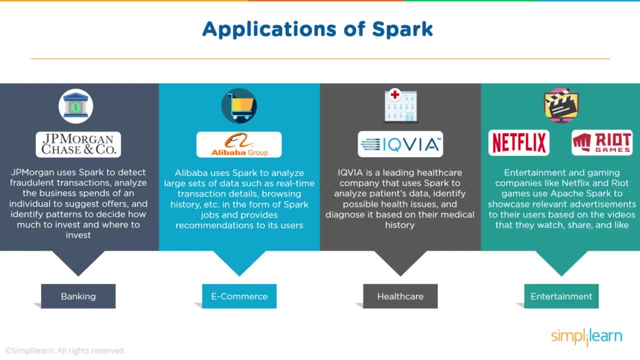 is also using Spark. You have Netflix, which is known, and you have Riot Games. So entertainment and gaming companies like Netflix and Riot Games use Apache Spark to showcase relevant advertisements to their users based on the videos that they have watched, shared or liked. So these are few domains which find use cases of Spark. that is, bank. 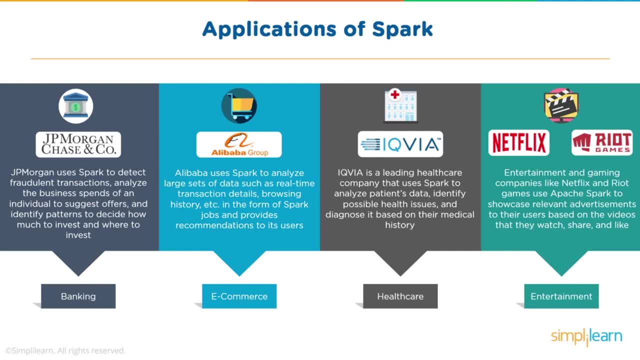 banking, e-commerce, healthcare, entertainment, and then there are many more which are using Spark in their day-to-day activities for real-time, in-memory, faster processing. Now let's discuss about Spark's use case, and let's talk about Conviva, which is world's 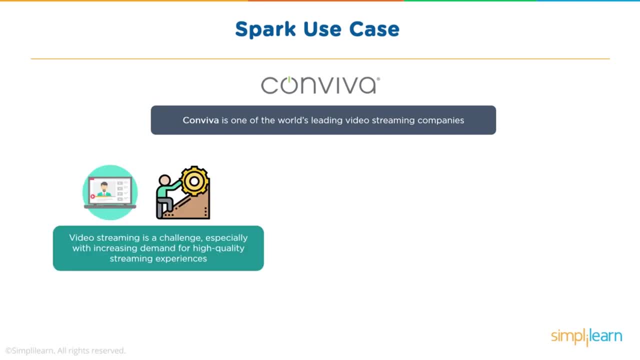 leading video streaming companies, So video streaming is a challenge. Now, if you talk about YouTube, which has data, you could always read about it. So YouTube has data which is worth watching 10 years. So there is huge amount of data where people are uploading their videos. 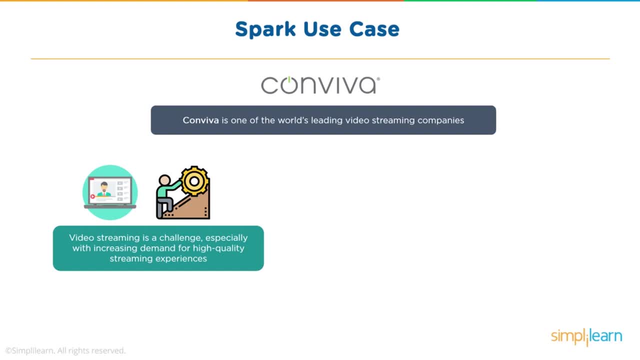 or companies are doing advertisements, and these videos are streamed in or can be watched by users. So video streaming is a challenge, and especially with increasing demand for high quality streaming experiences. Conviva collects data about video streaming quality to give their customers visibility into the end user experience they are delivering Now. 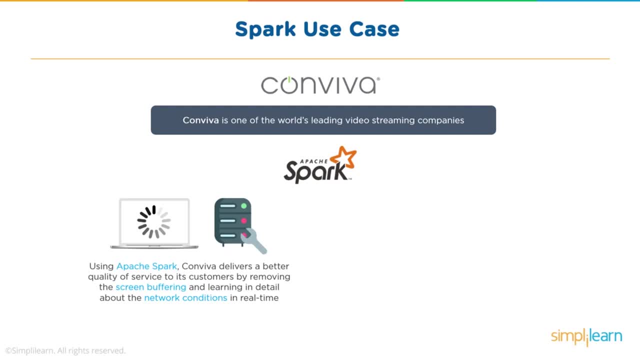 how do they do it? Apache Spark Again. using Apache Spark, Conviva delivers a better quality of service to its customers by removing the screen buffering and learning in detail about network condition in real time. This information is then stored in the video player to manage. 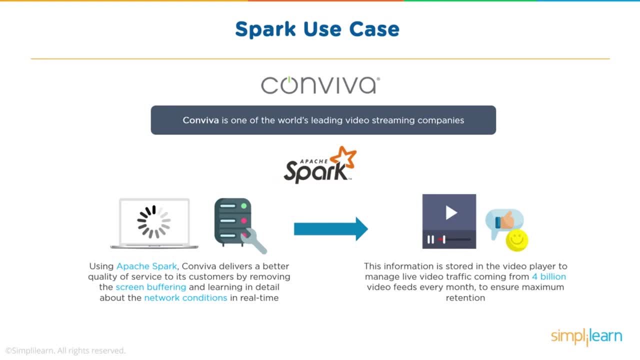 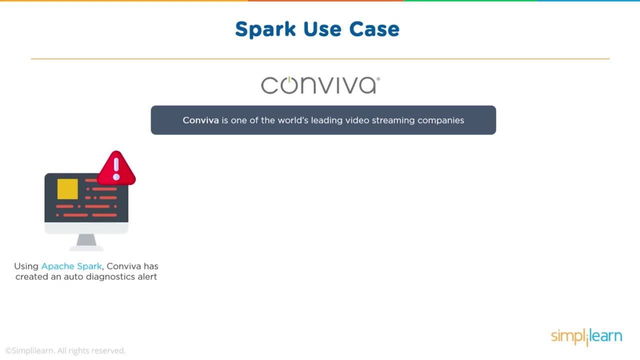 live video traffic coming in from 4 billion video feeds every month to ensure maximum retention. Now, using Apache Spark, Conviva has been able to reduce the risk of a bad connection to the Internet. The best way to do this is by investing the most money you. 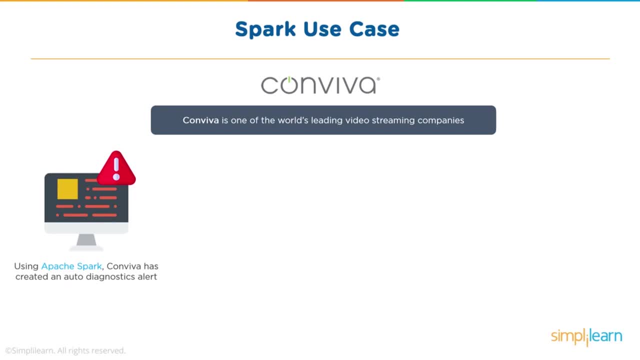 has created an auto-diagnostics alert. It automatically detects anomalies along the video streaming pipeline and diagnoses the root cause of the issue. Now this really makes it one of the leading video streaming companies. based on auto-diagnostic alerts, It reduces waiting time before the video starts, It avoids buffering and recovers the video from a technical 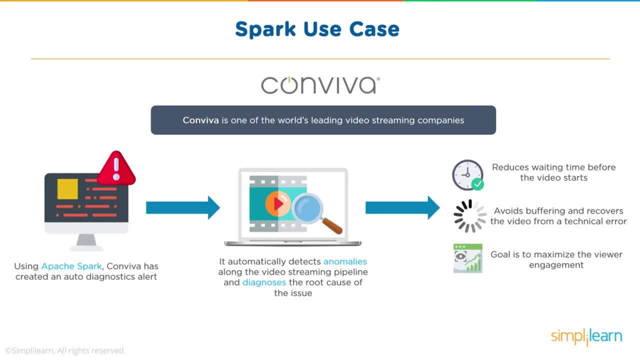 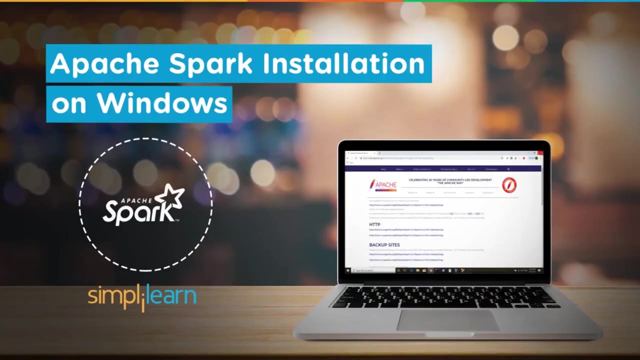 error and the whole goal is to maximize the viewer engagement. So this is Spark's use case, where Conviva is using Spark in different ways to stay ahead in video streaming-related deliveries. So let's have a quick demo on setting up Spark on Windows and trying out the Spark's interactive. 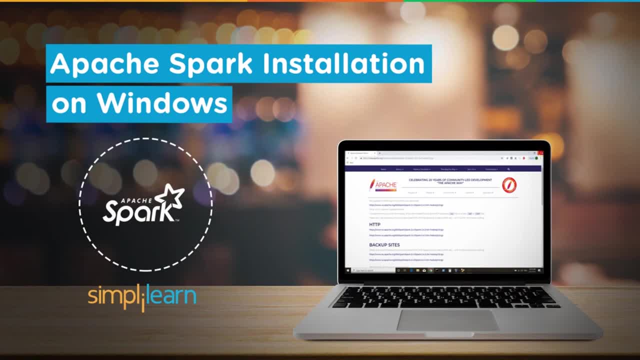 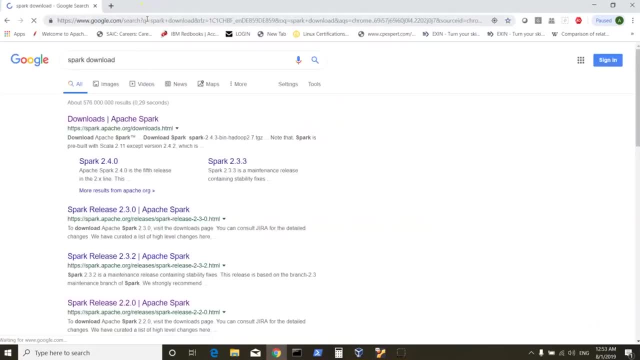 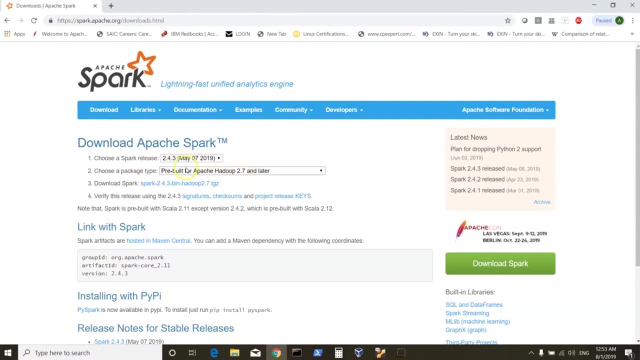 way of working For this. first thing is you will have to download Spark. Now you can just go to Google and type Spark download and once you click on this link it shows you a Spark release, a package type which says pre-built. So we will have to get. 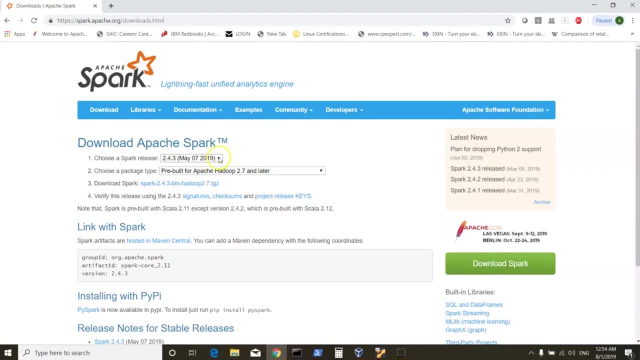 a pre-built Apache Hadoop-related Spark. So here I will choose, say, Spark 2.4.3, and I will choose pre-built for Apache 2.6, and then I can just click and download on the Spark 2.4.3.. 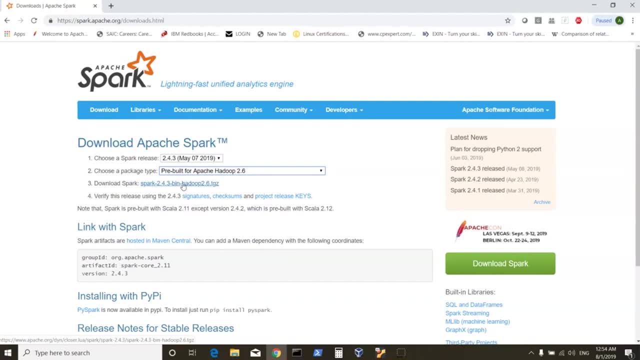 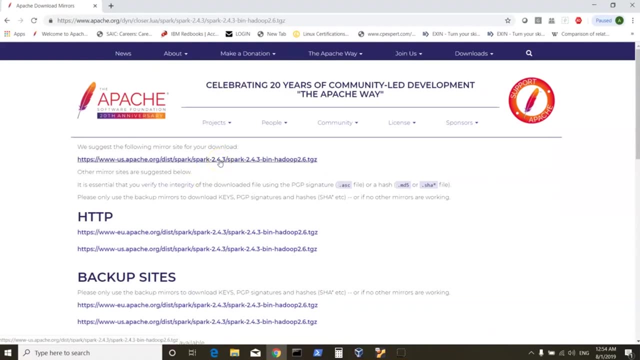 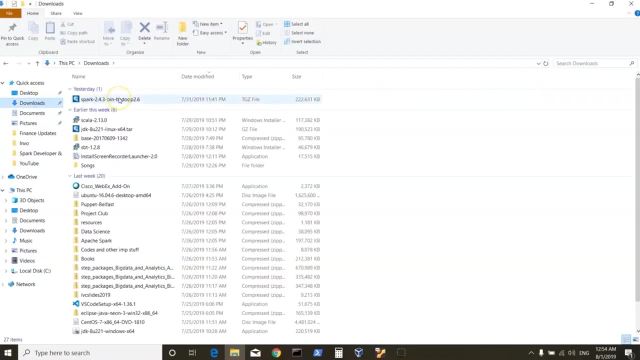 Once you click on this link, it takes you to the mirror site and you can just click on this link and download Spark 2.4.3.. Once this is done, which I have already downloaded here, I can go to my downloads and it shows that I have a tar file. Now we will have 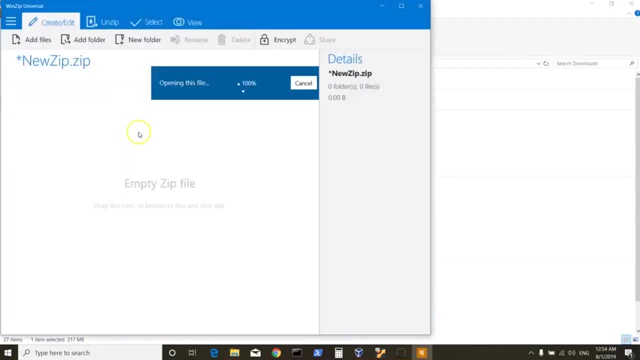 to untar it or unzip it. So I can click on this link and I already have WinZip which allows me to unzip Spark 2.4.3.. I can just click on this link and I already have WinZip which allows me to unzip Spark. 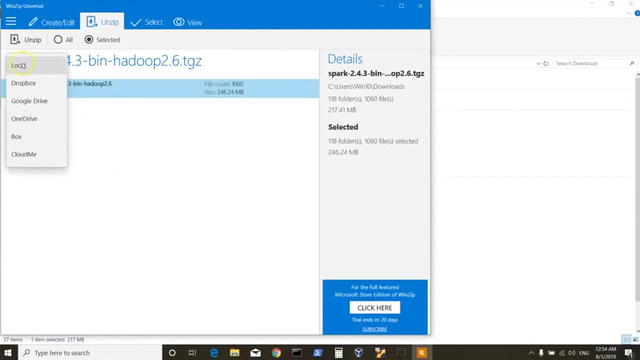 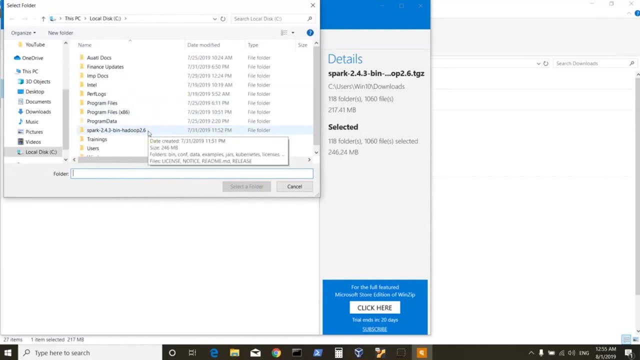 2.4.3.. I can choose a location. So I can say unzip, click on unzip, choose local, and then I can choose one of my folders. So I have already unzipped it here and that's how my Spark. 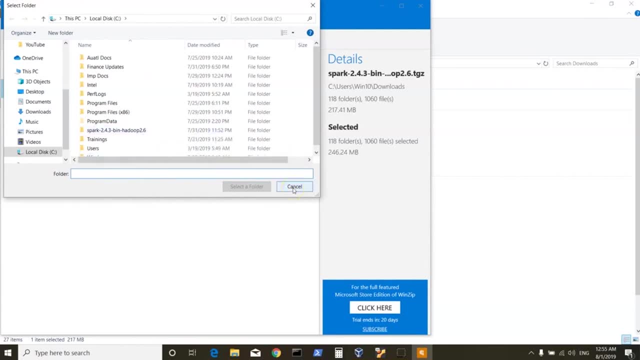 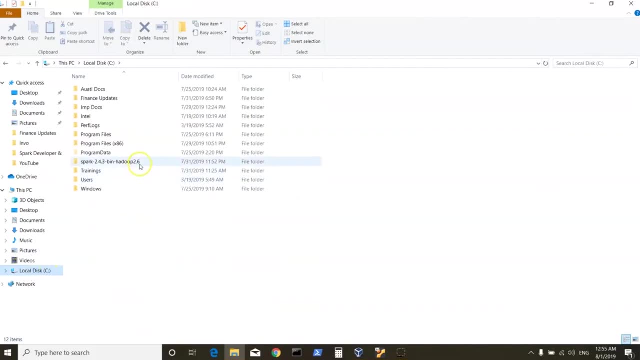 2.4.4 directory exists here: 2.4.3,. I'm sorry. Now let's go and look into this directory and what it contains. So I can click on C drive and then Spark 2.4.3, and this has the folders which are required for us to use. 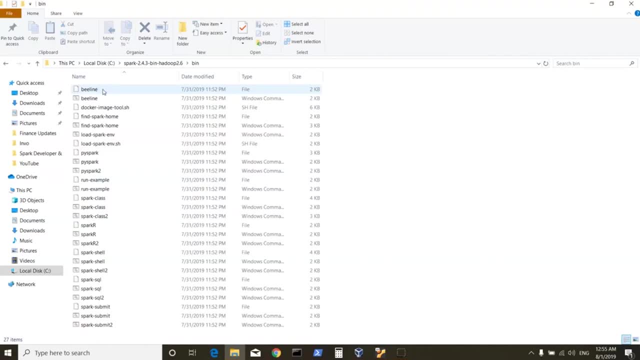 Spark. If you look in bin, we have Spark 2.4.3.. If you look in bin, we have Spark 2.4.3.. If you look in bin, we have Spark 2.4.3.. We have different applications and commands which we can use. and if you also see, I would 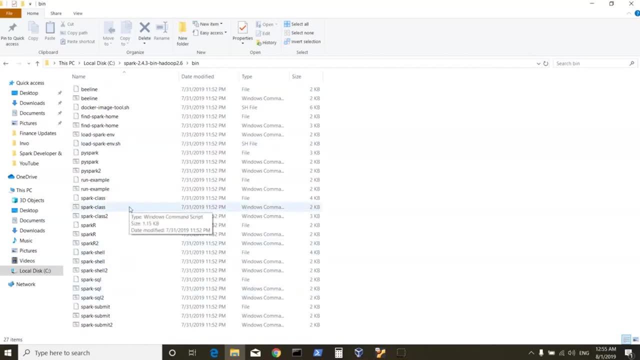 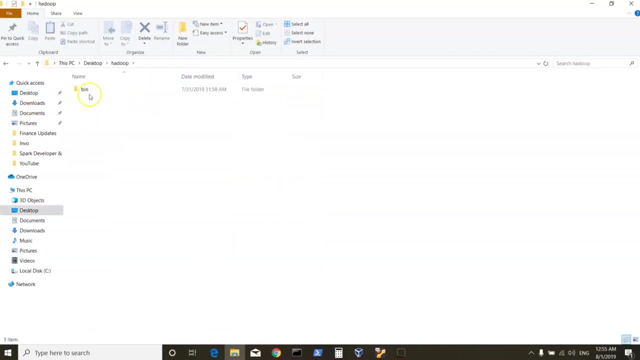 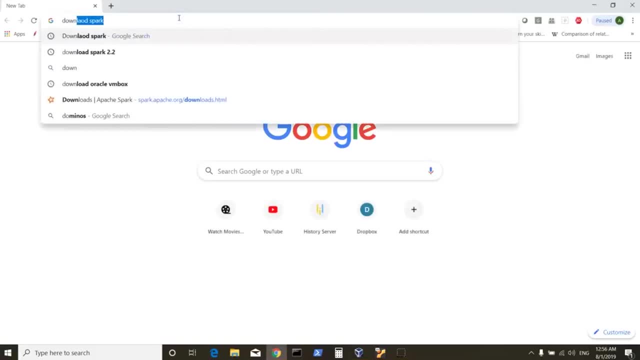 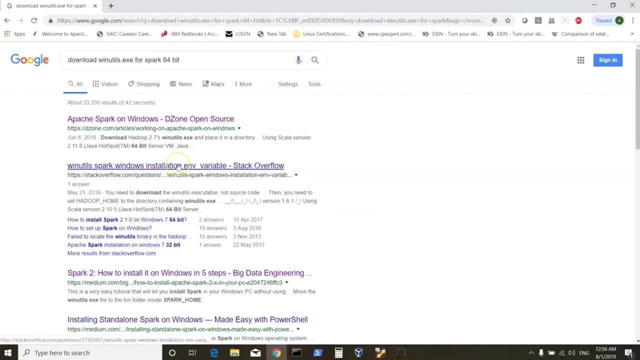 So I have a WinUtils executable and here I have downloaded a WinUtils executable file, which you can always search on internet and you can say: download WinUtilsexe for Spark 64-bit and then you can find the link from where you can download this, For example. 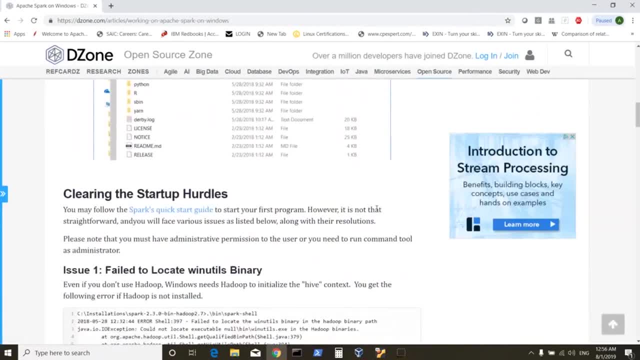 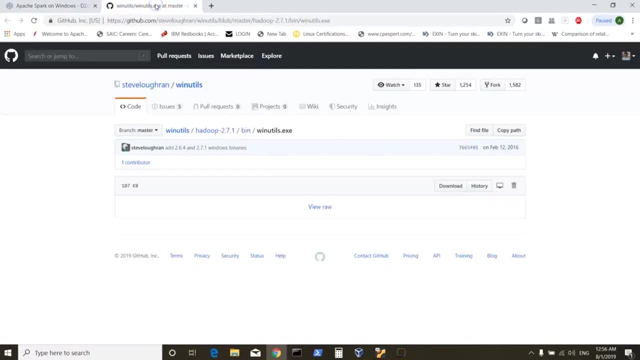 we can click on this and here we can search for WinUtils. So here we have the link. I can open this link in a different tab and this basically shows me WinUtils for Hadoop 2.7.1.. Similarly, you can search for Hadoop 2.6, and you can download. However, 2.7 will. 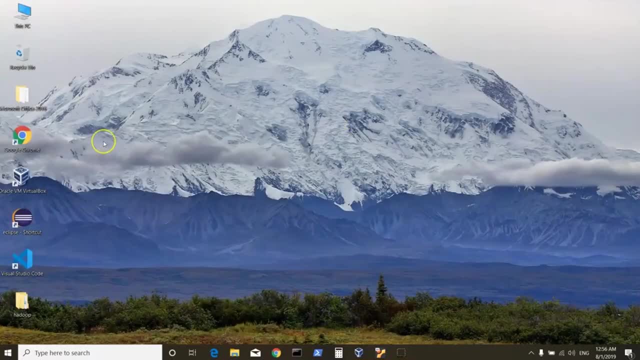 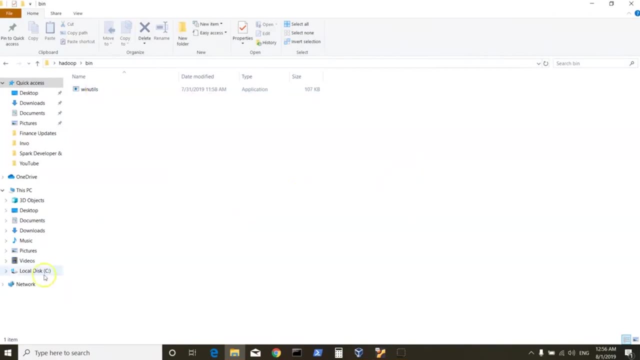 also work fine. Now I have downloaded WinUtilsexe and that's in this Hadoop folder Within bin. I have this, So we need two things here. One is Spark, which is untarred and in a particular location, and then your Hadoop, which has bin, and this has WinUtils. Now, once you 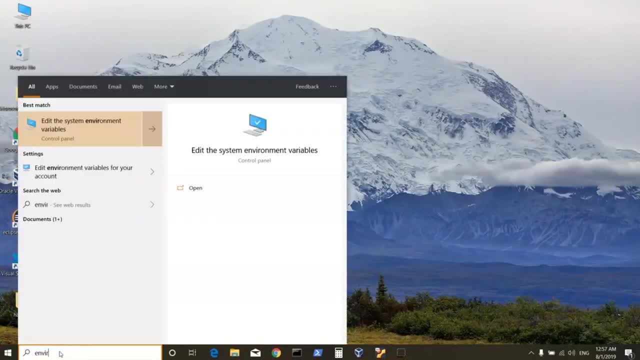 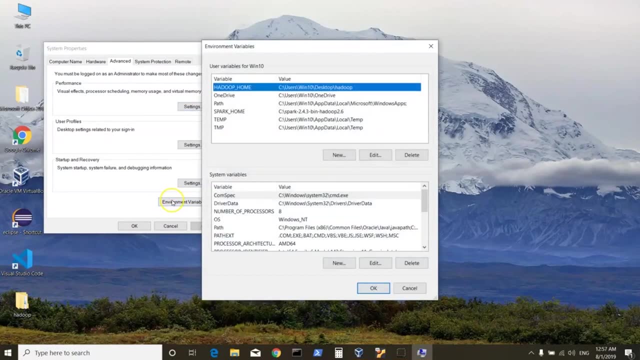 have these things. you can set your environment variables by just type in envir. go to your edit system, environment variables, click on environment variables and here, if you see, I have added two variables So you can just click on new and then you can give your variable name as Hadoop, underscore home and 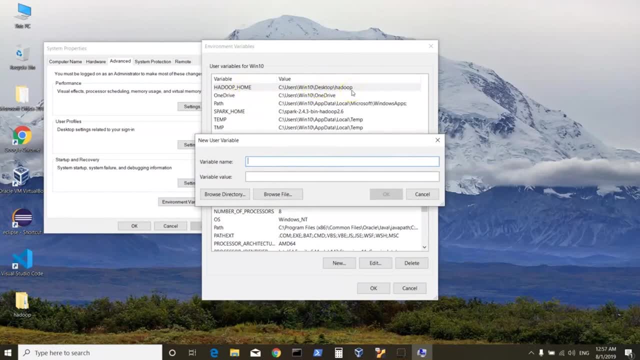 then you can give the path where you have your Hadoop directory that contains bin and that contains WinUtilsexe. I also have added Spark home, which points to my Spark directory. Now, once you have this, you can add the new Hadoop directory. Now, once you have this, 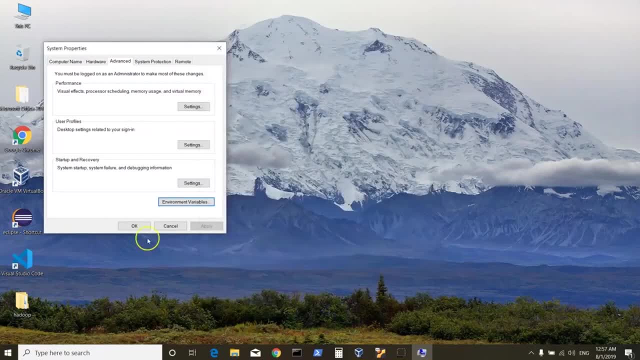 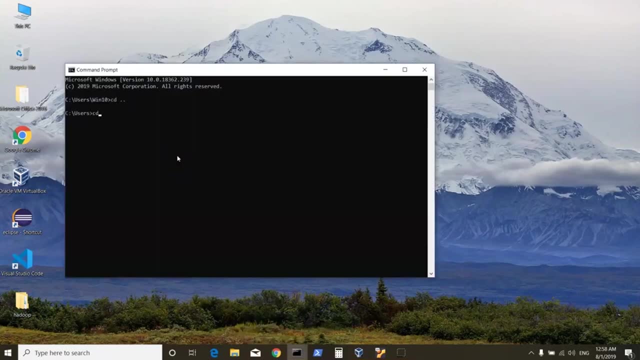 you are ready to use your Spark on Windows in local mode. Once this is done, I can open up my command prompt, and here I need to go to my Spark directory. I can just say cd, spark 2.4.3, and then I can do a dir slash p which shows me the folders where we have. 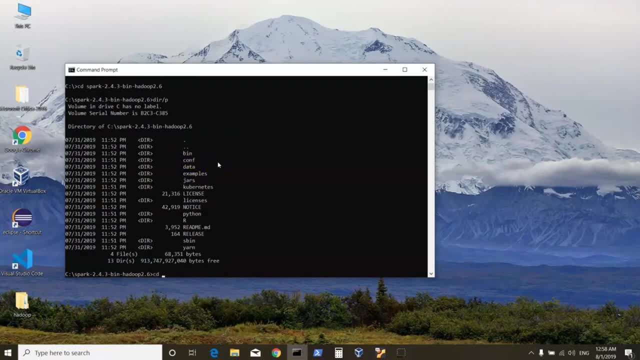 bin So to execute Spark, we can look into what our bin has and it has different programs, and then I can use this to 할게요. So in this case you have Spark shell to work with Scala and an interactive way of working with Spark. You can also use PySpark, which 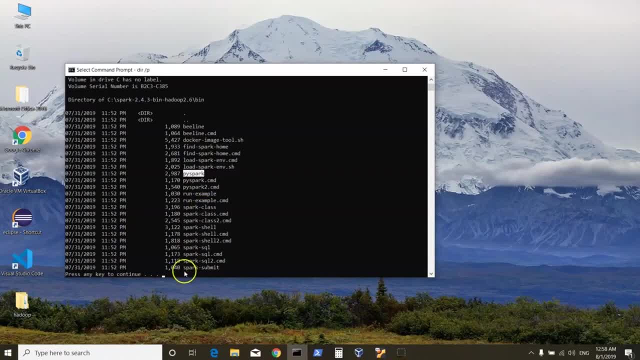 allows you to use Python to work with Spark and you also have Spark submit if you have packaged your application in a jar file to submit it on a cluster. So in this case we would be using Spark in a local mode. So let's use Spark shell and test it. So I can just say Spark shell in this way to: 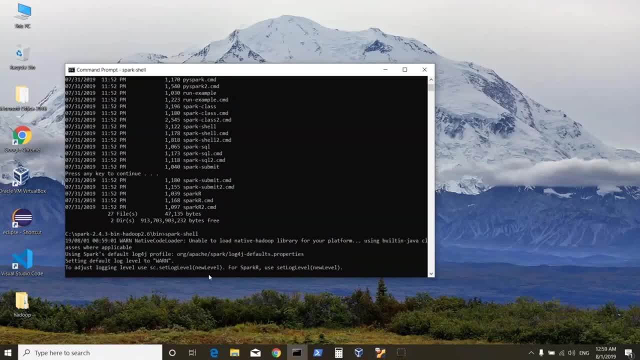 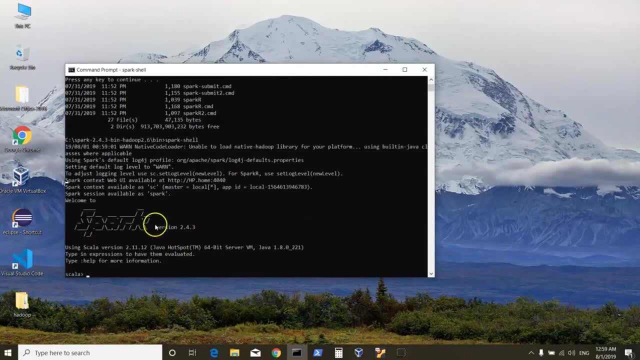 start my Spark in a local mode interactive way. Now, based on the path which you have set for your winutilsexe and Spark shell, you should be able to use Spark. So it says welcome to Spark version 2.4.3.. It also shows that Spark context, which is the entry. 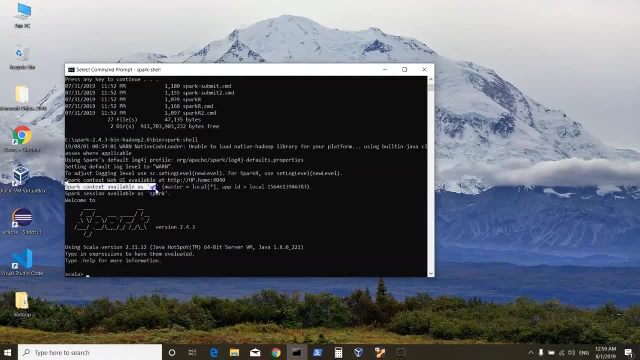 point of your application is available as SC, wherein it is connecting to master as local and it has an application ID. It also shows you a Spark UI which you can look at and it says Spark session is available as Spark. So if you are interested in working with Spark core, that is, with RDDs, we would 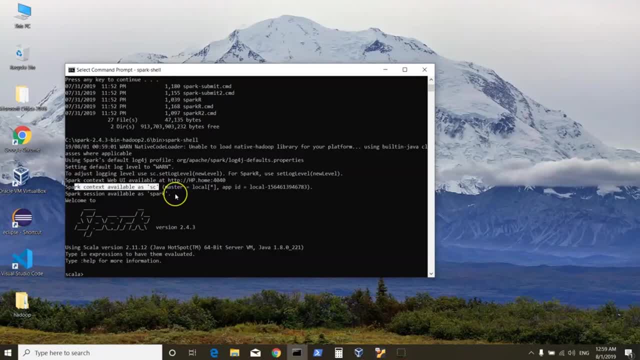 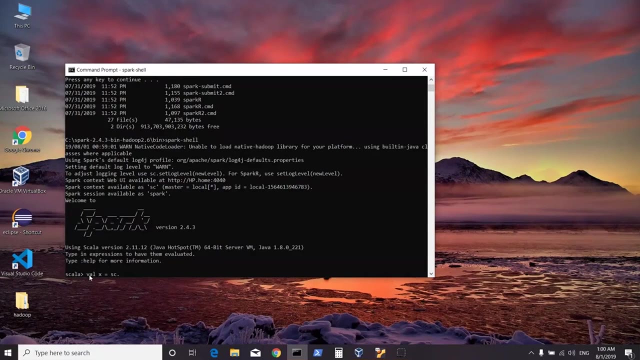 be using Spark context, and if you are interested in working with Spark SQL, that is, data frames and data sets- then we can be using Spark session. So let's try it out, So we can declare a variable that is a immutable variable. and now I will use Spark context with a method of Spark. 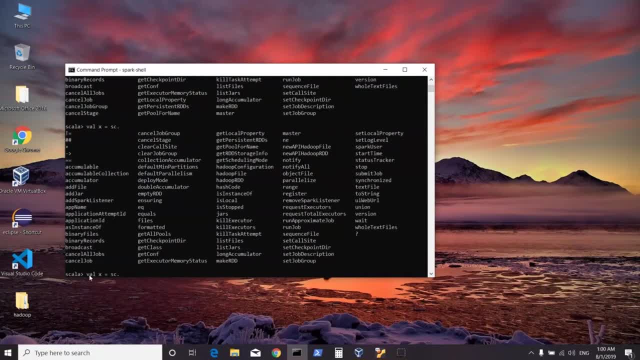 context. So I could just do a tab to see what are the available options within your Spark context and here we can use one of them to read a file. So I will use sctxt file and then I need to point to a file. So I already know that in. 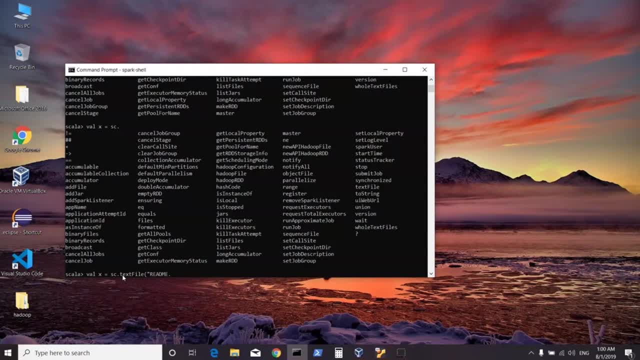 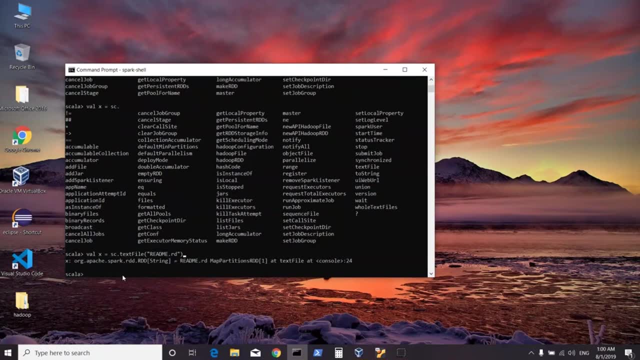 my Spark directory I have a file called readmerd and this is the method of Spark context. If I enter, it will create a RDD. Now, as I've explained about RDDs, these are resilient, distributed data sets. There is no evaluation happening right now, So, even if this file does not exist, I would 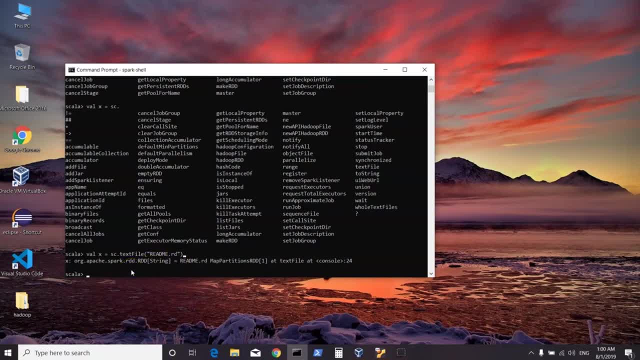 still have an RDD created. Now I can go further and do some more transformations on this. So I could say val y and then I could say take X. I would like to do a map transformation on it and I would use to uppercase: Now this is a inbuilt. 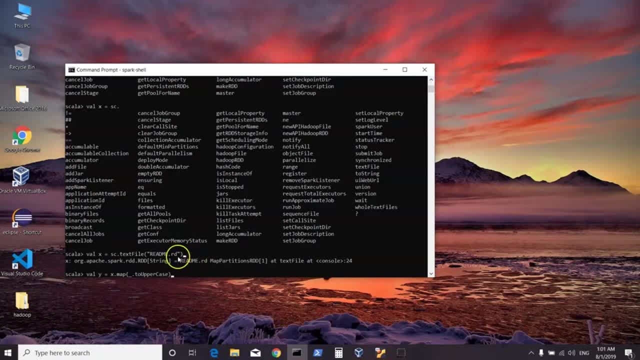 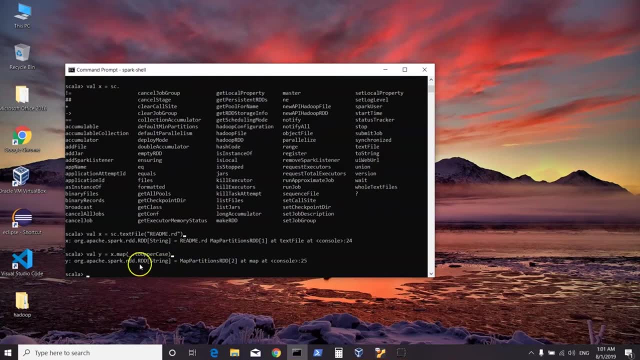 function where I would want to convert the content of this file into uppercase. When I hit on enter, it again creates an RDD, and this RDD is basically a child RDD of the parent RDD created by text file. Remember, here we don't have any evaluation happening or any execution. 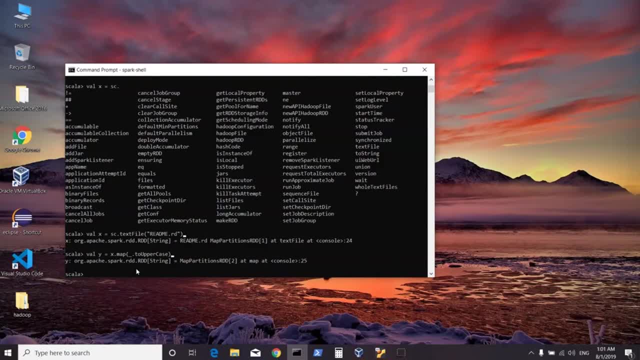 happening. It has just transformations which will lead to creation of further RDDs. Now we can invoke an action to see the result, and whenever you invoke an action, it will create a new RDD. Now we can invoke an action to see the result, and whenever you invoke an action, it will. 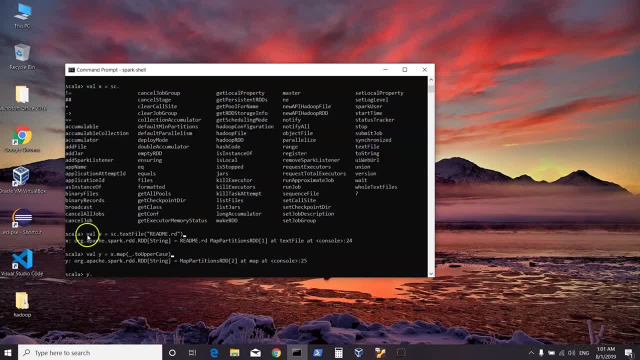 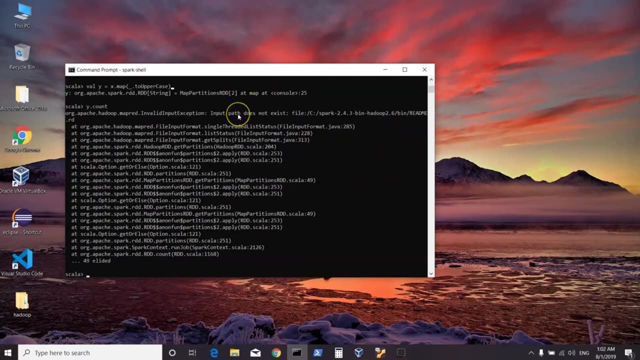 trigger the execution of your DAG, starting from your first RDD till the last transformation you did before invoking an action. So I could just say count to see how many lines it has. and once I do this it says input path does not exist. it is not able to find a file in this location. So this clearly. 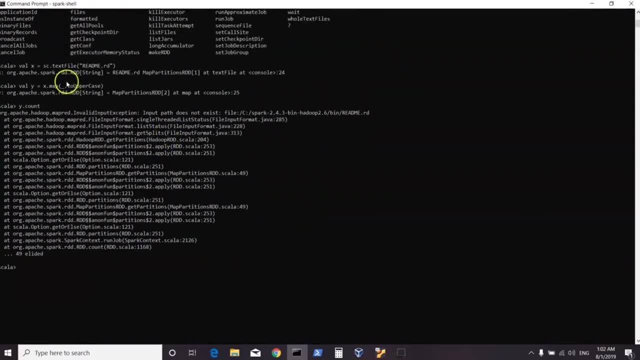 explains that there was no evaluation happening when we did this, when we tried to read a file, and neither when we did a map transformation only, and only when we invoked an action. it tried to search for file in this location. so let's quit this and check if the file exists. to quit, you can just do. 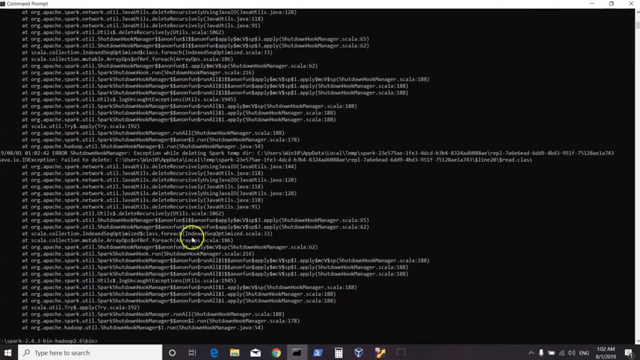 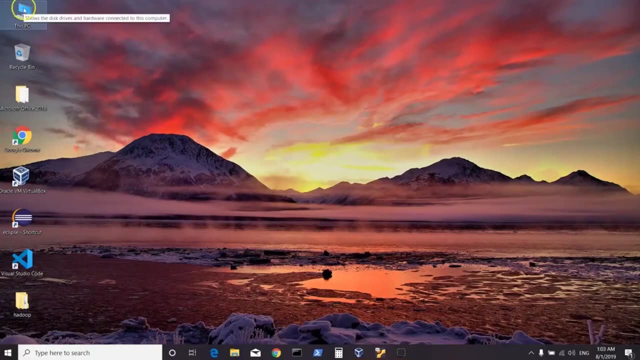 a control d or you could do a colon quit now here if you see some messages like this, which says unable to delete temporary file. so that's a known issue. we can fix that. but my spark is working fine. now let's go and check if the file exists. so i will go in here and then i will look in my spark. 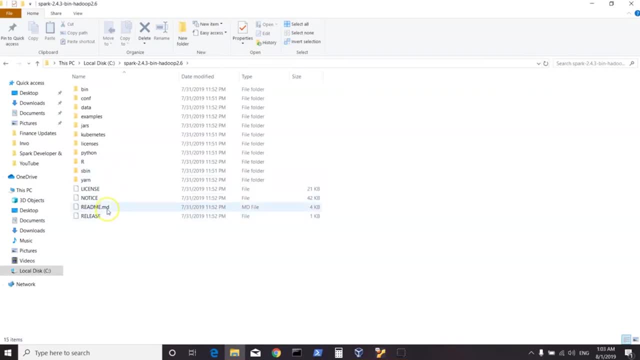 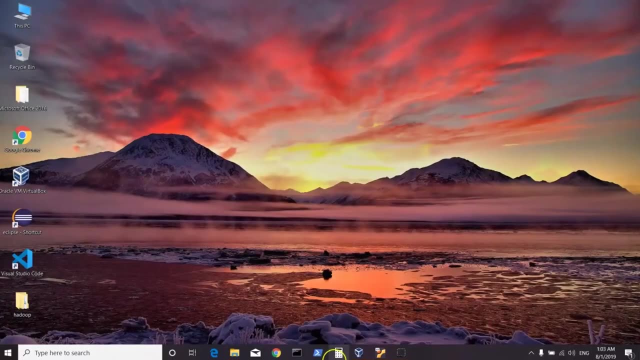 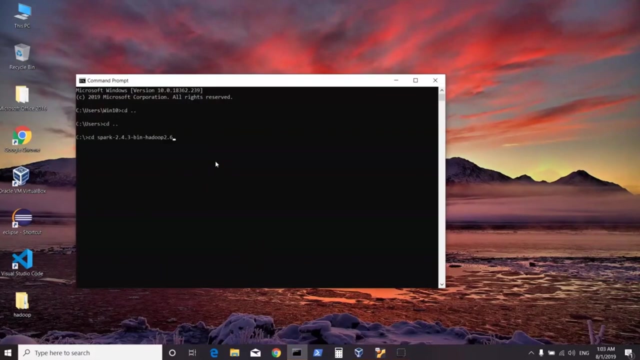 directory to see if the file exists. so this is the file: readmemd. however, i had done readmerd, so let's do it again and let's test if our spark shell works. fine, so we can go into the spark directory by just doing this and then either i could be going into bin directory and then start. 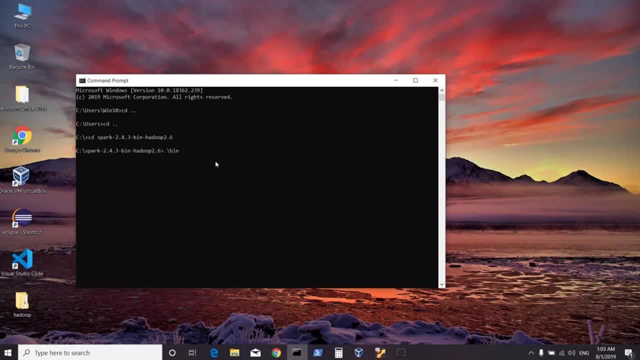 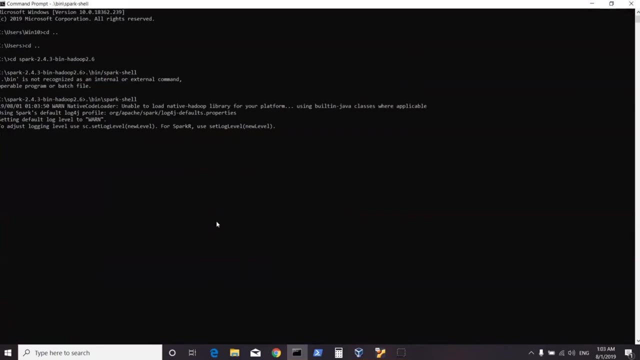 spark shell, or some people prefer to do it this way, wherein you can say: bin spark shell and that should start your spark shell. but there was an error in the in the slash, so let's do it this way and this will start your spark shell. an interactive way of working with your spark and using spark context. 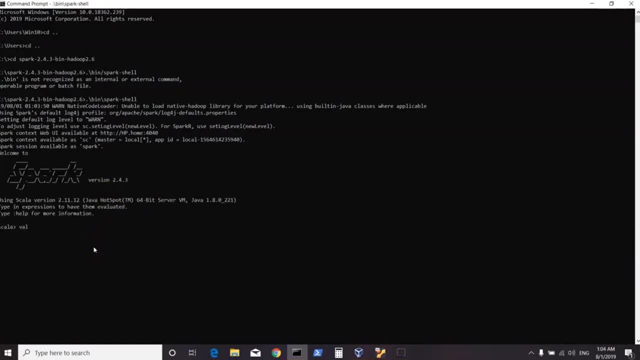 or spark. now, once we have done this, i can again say val x and i can say sc, which is spark, context, which is already initialized when you start your spark shell. i can say text file, and i would want to read a file which is readmemd. now we know that this. 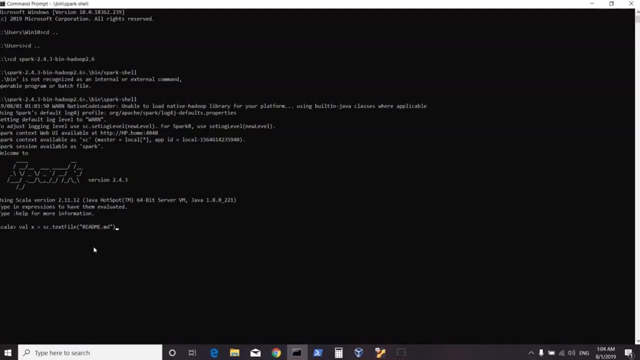 file exists. however, the checking of the file existing or not- that means an evaluation- does not happen when you do a transformation or when you use a method of spark context. it just creates an rdd. click on this and this has created an rdd of string. now we can do further transformation. 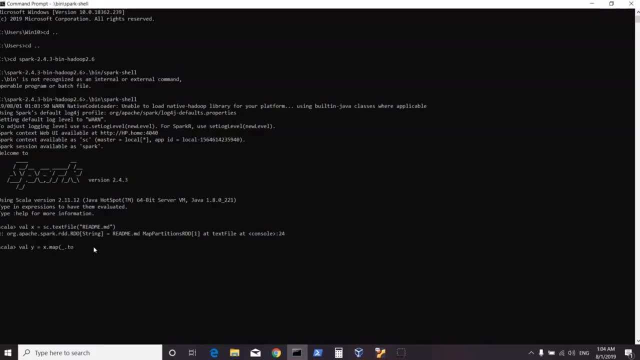 on x by saying map, and then we can do further transformation on x by saying map, and then we can say: i would want to convert the content into uppercase, and that's also done now. finally, let's invoke an action which will trigger the execution of my tag which contains these rdds, so i could: 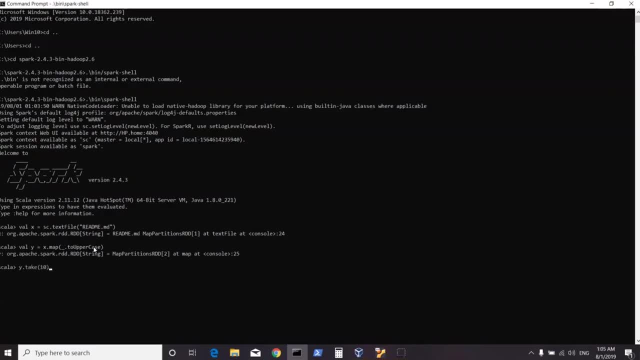 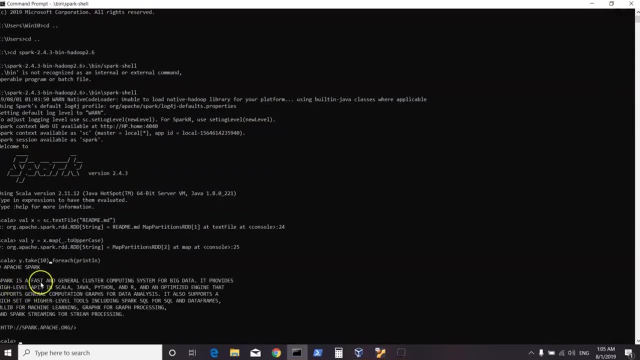 just say y and i could say take 10, and i could say for each print, ln, and this should be able to invoke an action and it shows me the result from the file which is converted into uppercase. remember, if i do a y dot count, which is another action, it will trigger the execution of dag right from the. 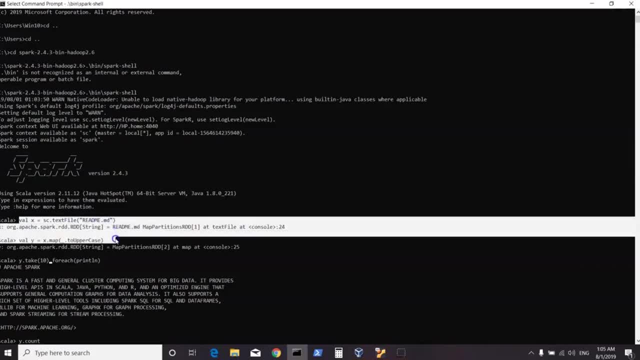 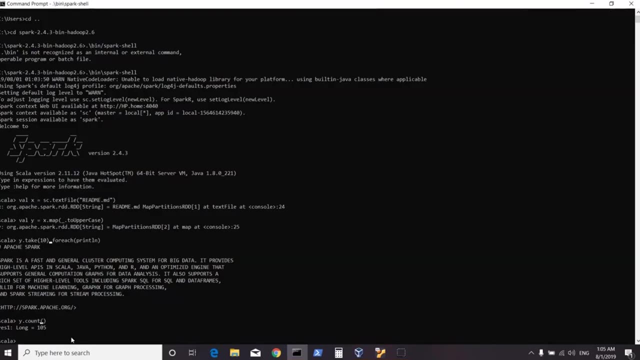 beginning, where the first rdd was created, the transformation will be done and then it will show me the count of lines which exist as a result of this. so we can do this, and this says me that there are 105 lines. this is a simple example of using spark shell and using spark in an interactive way. 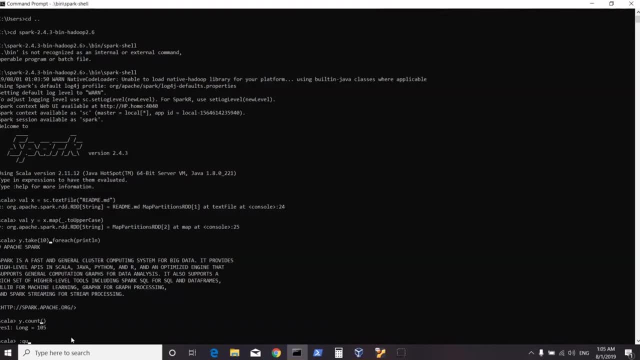 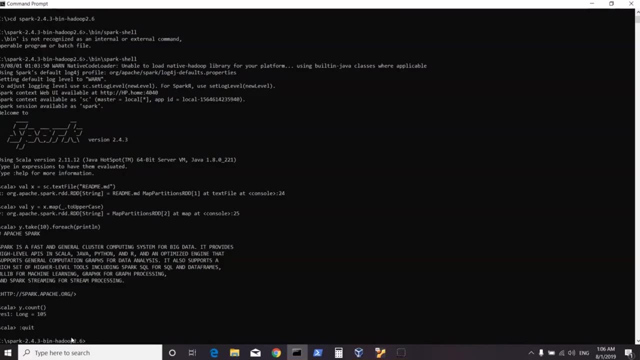 on your web browser. so let's see what happens. if i do a y dot count, which is another action, it will project a manual on my windows machine. now to quit. we can always do a colon quit, or we could do a ctrl d and that basically takes you out of your spark shell. similarly, we can work on py spark by: 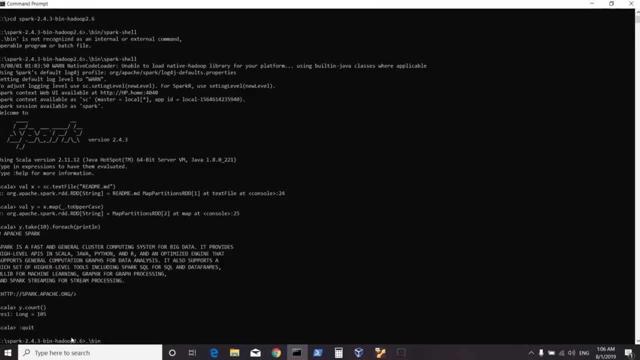 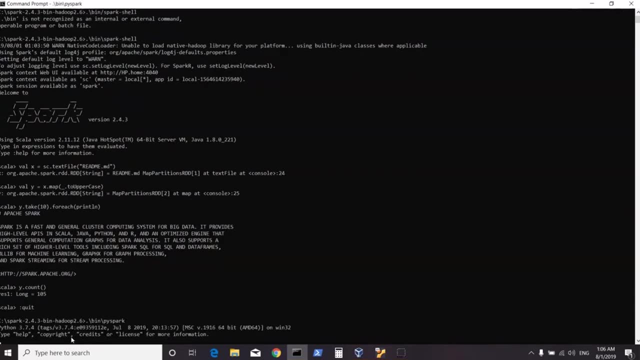 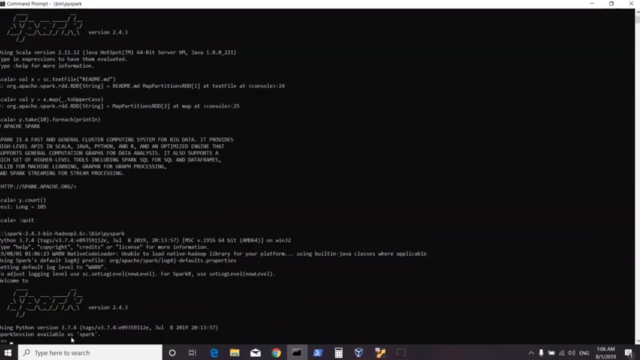 just saying dot, slash, bin, slash, py, spark, and that's python's way of working with spark, which brings your python shell. it starts the spark context which is available as sc, and if you are interested in working on data frames or data sets using spark sql, then we would. 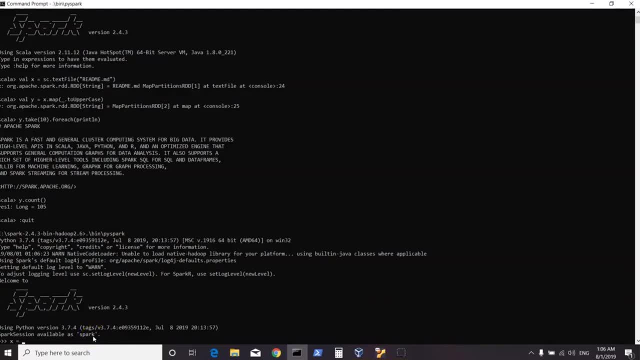 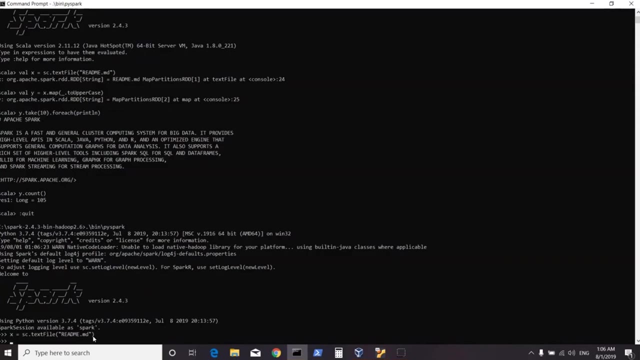 be using spark. now here i can just declare a variable x and i can just do sc dot text file, like what we did using scala. we can be referring to the same file, readme dot md- and this has created an rdd. you can just type in x and that shows the rdd which was created. you can then 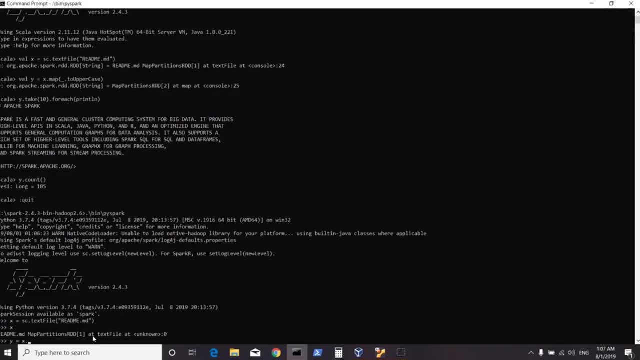 further, do some transformation on it using x dot map, and then i could say i would want to convert this to uppercase. now, in case of python, you would normally use lambda if you would want to do any kind of transformation. so i would say lambda x and then i would want to convert this to uppercase. 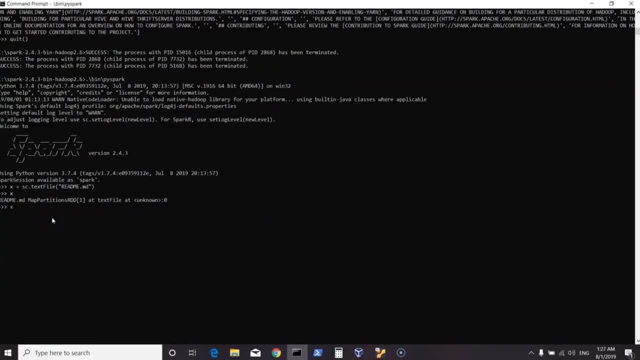 so here we can check if my rdd was correctly created and, as i was saying, i would want to convert this to uppercase. and then i would want to convert this to uppercase. we can then do some transformation on it so i can say again: y equals. and then i would want to do: 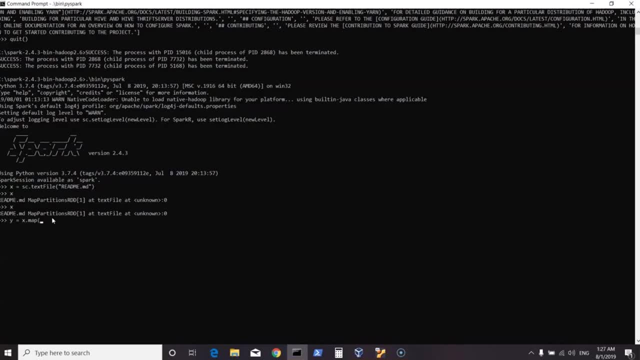 some transformation. on x i would say x dot map. so in case of python, as i explained, whenever we want to use an anonymous function or we want to do some transformation, then we can pass in the function to the transformation. so here i can say lambda and then i can just say line, or i could say x or 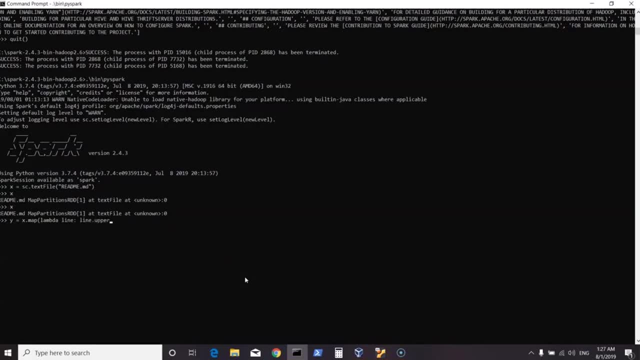 a, whatever that is, and i could say line, i would use a inbuilt function that is upper, which should convert the content of x to uppercase. now remember, we are just doing some transformations here. so if i click on y again and enter- sorry, if i enter y- it will show me that that has created an rdd to. 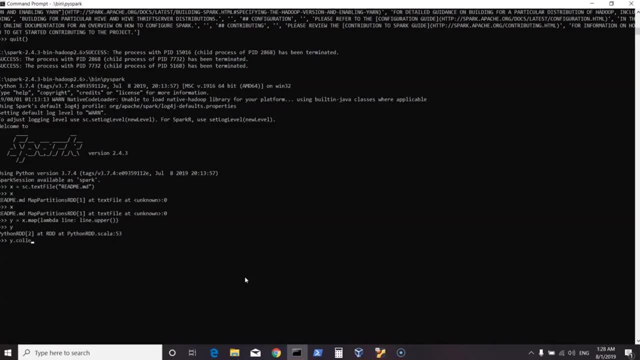 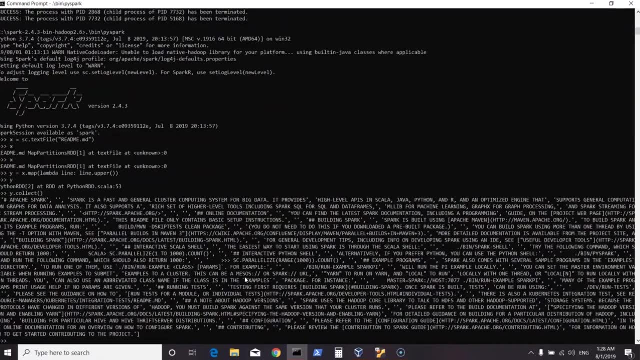 see the content. i can just say y dot collect, and that should show me the content of first few lines which is converted in uppercase. so this clearly shows that we can even use python to work with spark by using pi spark. now to quit this, we can just say quit and that should take you out of your 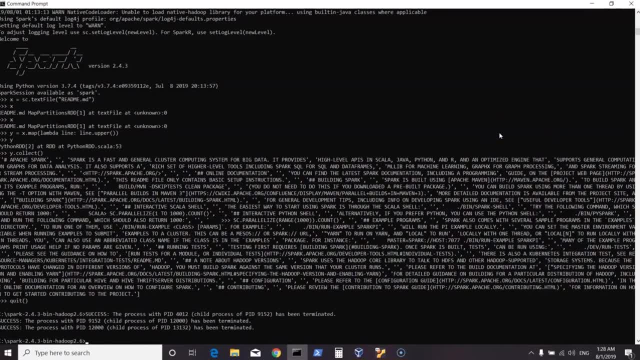 pi spark shell. so this is how you work on spark shell or pi spark on your windows machine. so this has a local spark setup, or basically spark running in a local mode, and you could be using the interactive way of working with spark. now, if we have a local spark setup, we can just say quit and 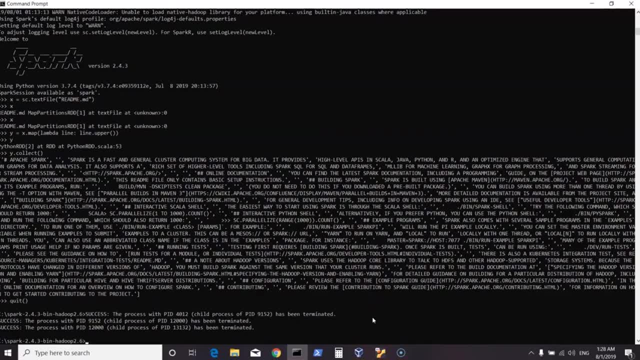 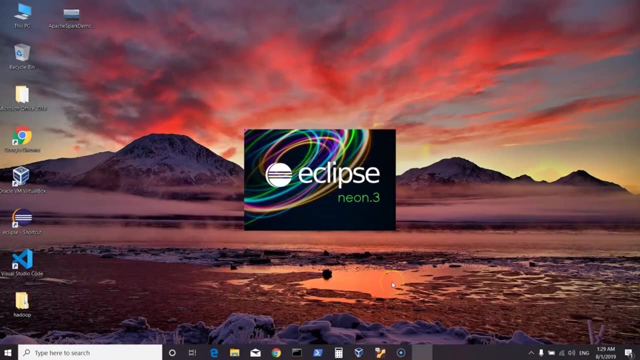 have packaged our application in a jar file. then i could be using spark submit to submit my application. how do we do that? for this we can basically bring up one of our ids. so in my case i'm using eclipse and i can get into my eclipse. now there are two options here. one we can be: 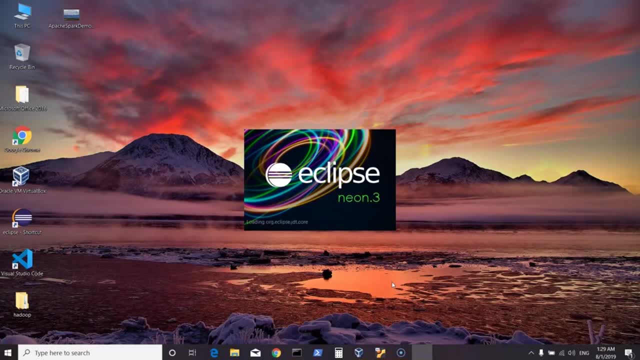 writing code in your ide. that is eclipse. we can be compiling the code based on the spark related jars, and then we can also compile the code based on the spark related jars, and then we can also we can run our application from ide which would interact with your spark. that's one way. the second: 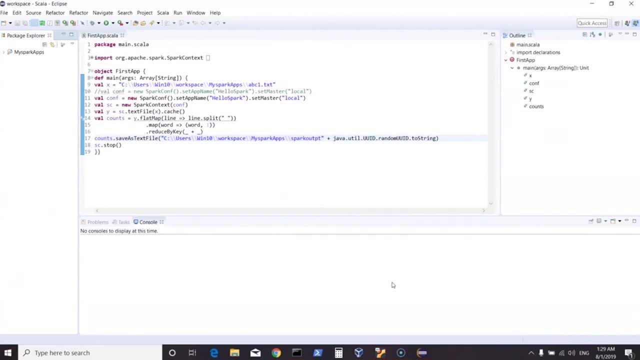 way is: we can use packaging tools like sbt to package our application as jar and then push the jar to your local spark or a hadoop based spark and then run it using spark. submit now. this is a simple sample application for which i have set up certain things here. the first thing is: 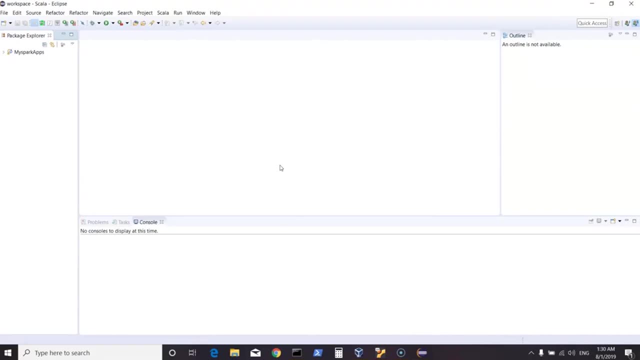 when you have downloaded eclipse for all the people who are new, they might have to add the scala plugin. now. if you see here in my eclipse, it shows up java perspective and it shows scala perspective. now how did i get this? you can click on help and you can say install new software and 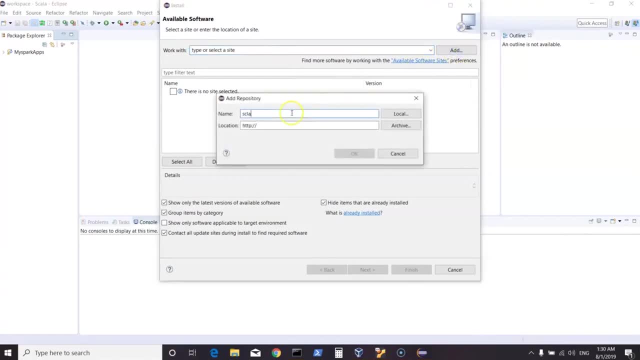 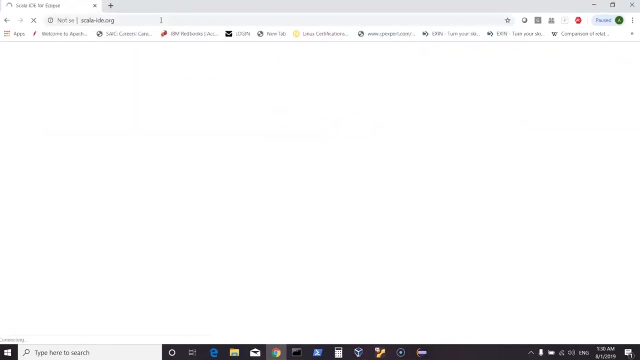 here you can say add, you can say scala ide, and then you will have to give a link from where you can get the scala ide. how do i get that? go to my browser and I can say Scala IDE dot org, and once you go to this link, 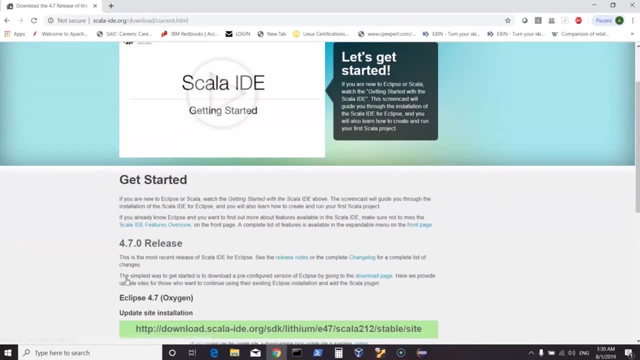 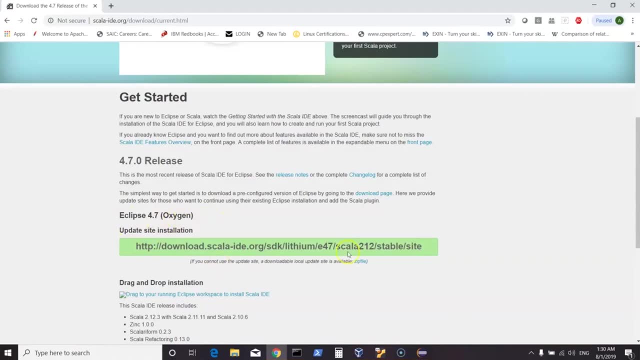 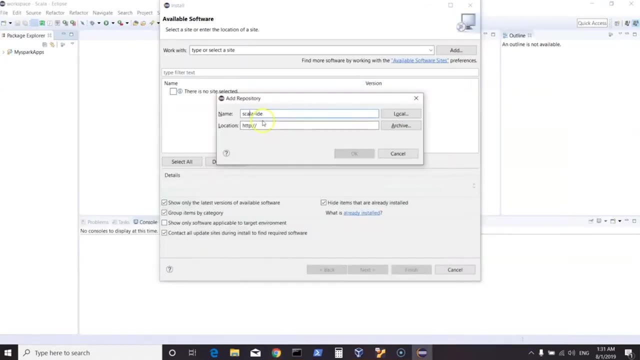 just scroll down, click on stable, and that shows you different releases for your different IDEs. now for Eclipse, although this shows for oxygen and I have Eclipse neon. but that works fine. you can just copy this link and here, once you have copied the link, give the location here and you can say: ok, now. 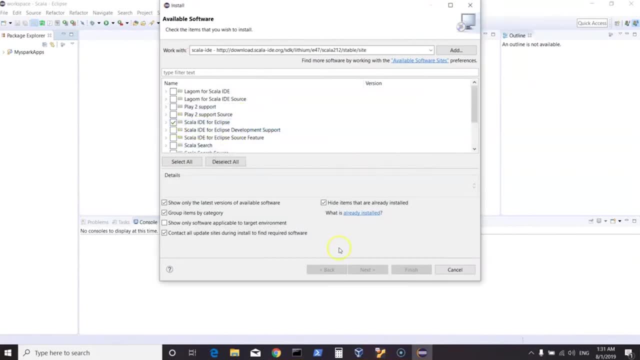 once you do that, it shows you different options from where you can choose Scala IDE for Eclipse. now, in my case, it is already installed, so these options don't show up. however, if you do not have this option, for example, let's choose something else, say, I will say Scala search and once I do this, next gets: 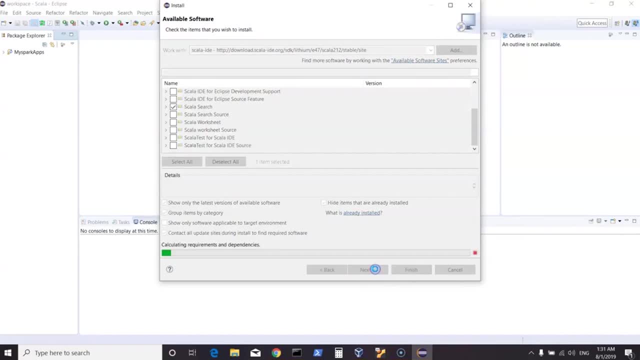 activated, so Scala IDE is already installed in my case, so I can click on next, and this should basically get Scala search plugin also, which can be added to my Eclipse now. once this is done, you will be prompted to restart your Eclipse and then you should have your Scala perspective. so for now I'll just cancel. 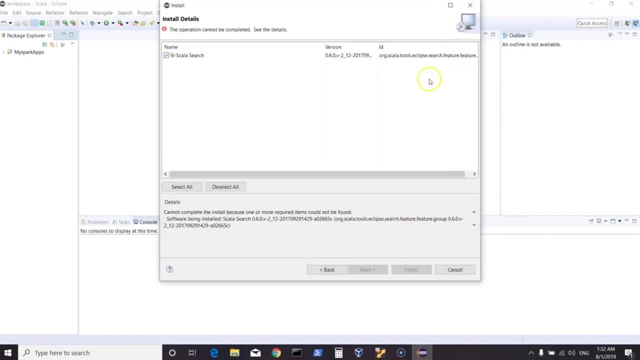 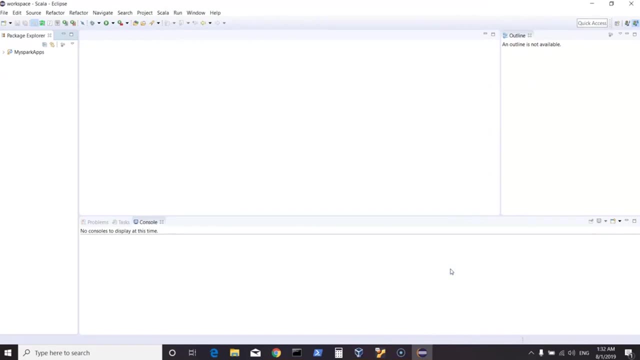 this because I already have my Scala IDE dot Eclipse, so this is done. I'll just do a cancel here now. once you have your Scala IDE or Scala plugin added to your IDE, you can always click on this icon here and here you can just click double click on Scala. that will open up Scala IDE. 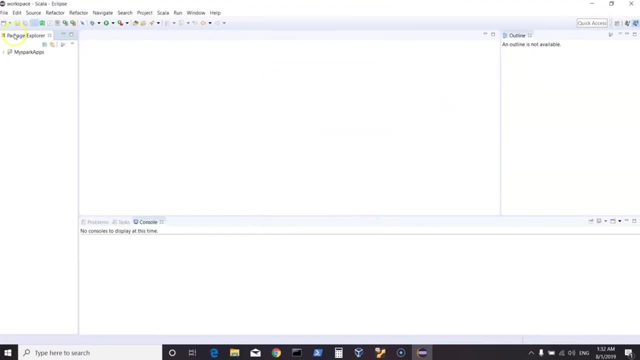 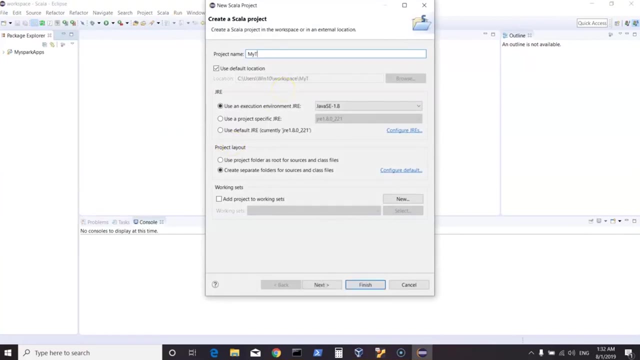 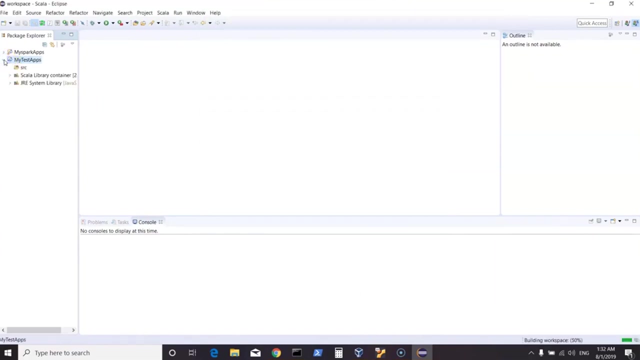 up Scala perspective. so that's the first thing. then you can always click on file new and create a Scala project. for example, I could say my test apps, and then I can just say finish, so it has added a project. now what we need to do is we need to make sure that our setup is fine. so first thing, 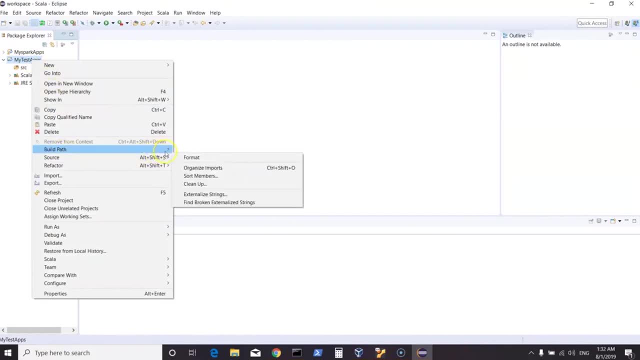 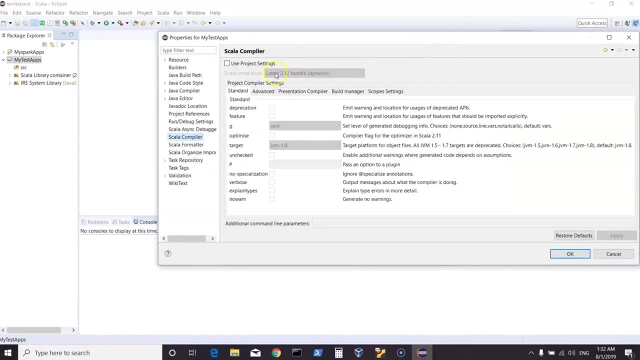 I would suggest is: click on this, go to your build path and here click on configure build path. so where it says Scala compiler, it would be good to choose for your project settings: instead of 2.12, go for 2.11. so sometimes you might have problems with Scala 2.12, which might not be able to compile. 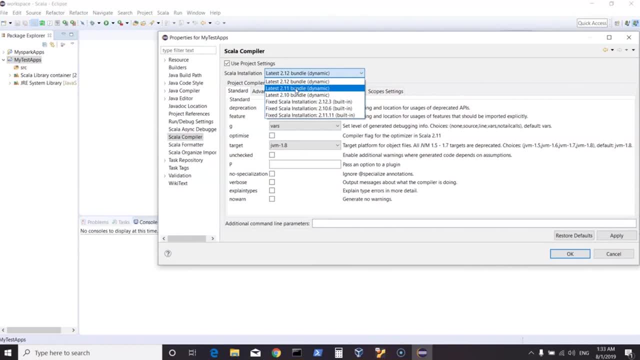 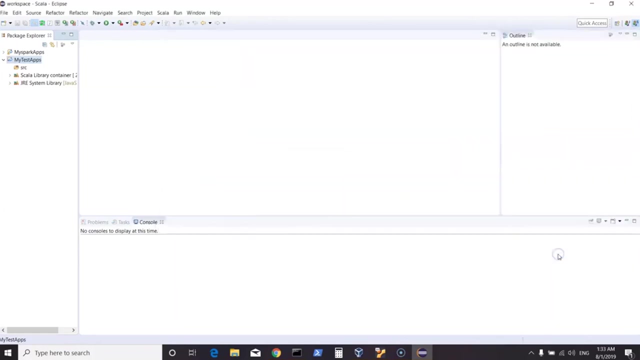 for your Scala 2.11. so use latest 2.11 bundle and then you can say apply. it says compiler settings have changed. a full rebuild is required for changes to take effect. shall all projects be clean Now? we can say okay and we can say okay. so this will build your workspace to use Scala 2.11 bundle. 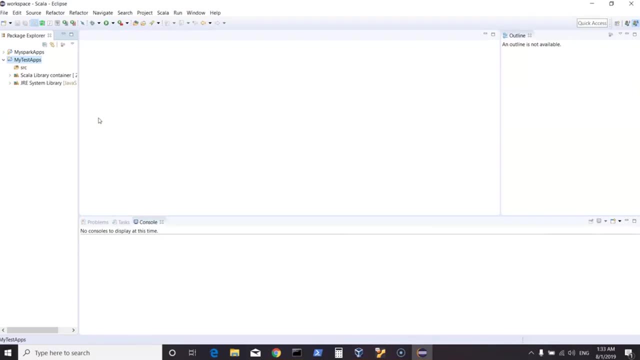 now, once that is done. second thing, what we need is we would want to write our code and we would want our code to compile for that, as I said, if we want to write our code using an IDE and then run it from our IDE rather than using a build tool like Meven or SVT, I can just add the spark related. 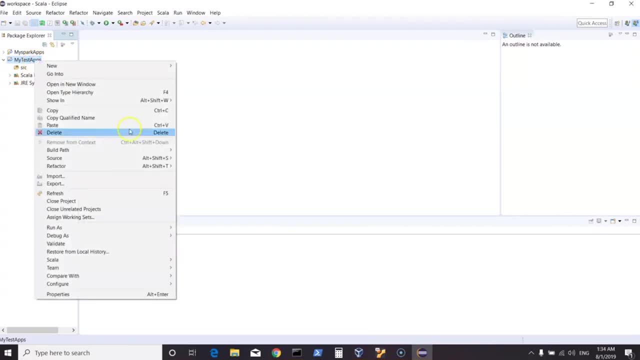 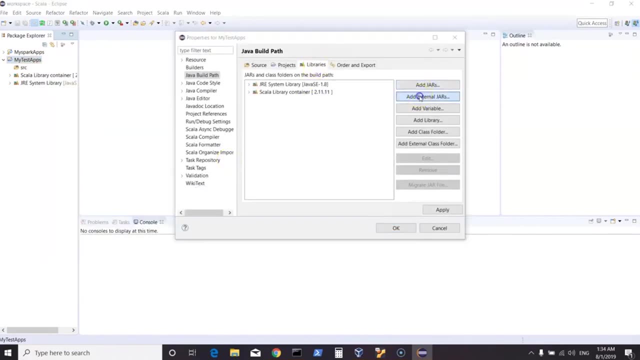 jars to my Scala 2.11 bundle and then I can just compile it. and then I can just compile it and my build path, so I can right click here, I can say build path and I can click on configure build path and here, where it says libraries, I can say add external jars. now this needs my spark related jars. 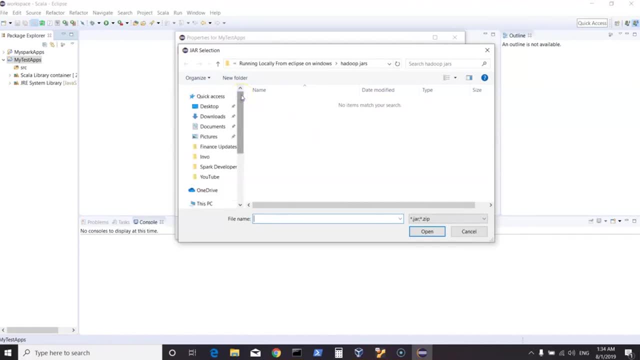 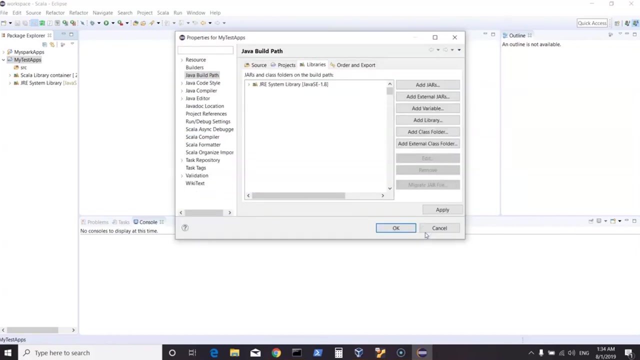 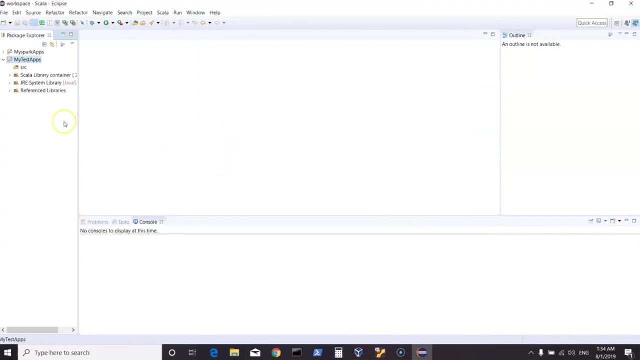 now, where do I find it? so remember, we have downloaded spark so you can even find it there, so you can click on wherever your spark is, and then you can click for jars, which shows you all spark related jars. So once this is done, you have already added the spark related jars which might be good enough for. 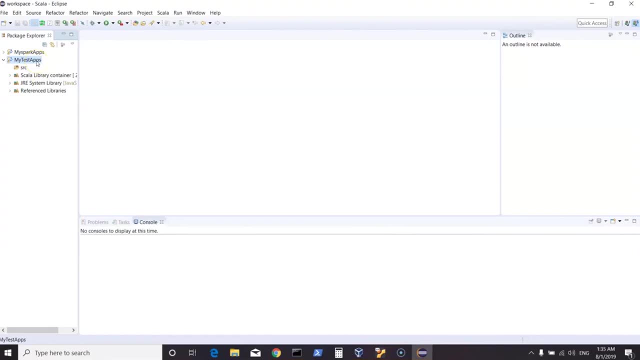 you to write an application. once this is done, we need to basically go ahead and write our code. now how do I do that? I can just click on source and I can say new, and then I can say package, and here you can say main dot Scala. click on finish and that has created main dot Scala. so that would 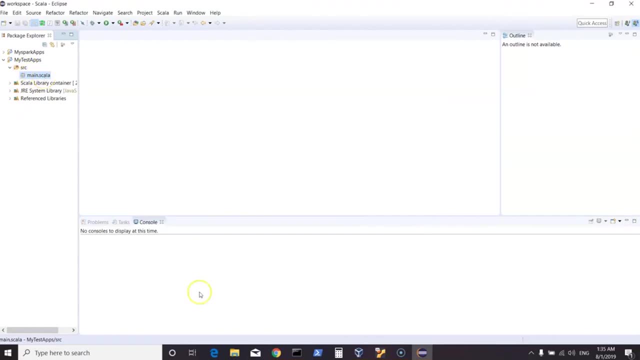 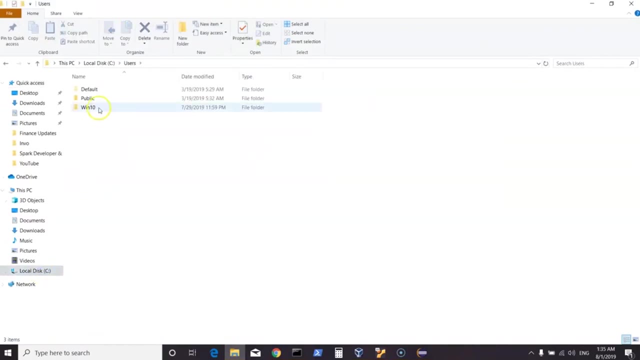 be source, slash main, slash Scala in the folders. we can always check that. so I can go to C drive, I can look in users, Wintan, and then look in my workspace for my project and if you see, in source we have main and we have Scala. now this is where we will be writing our code. 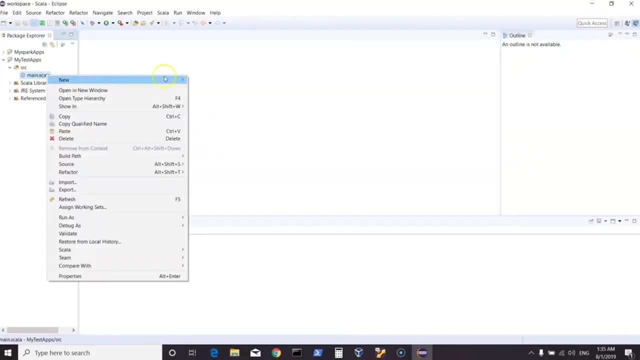 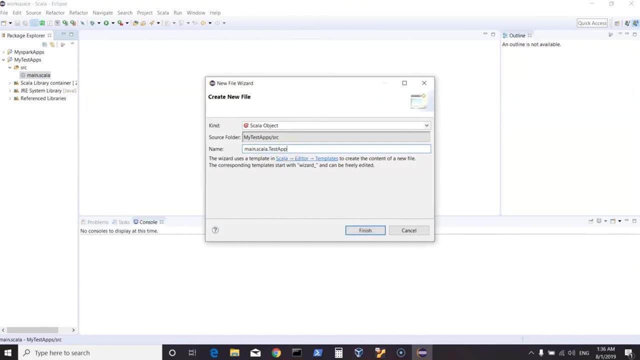 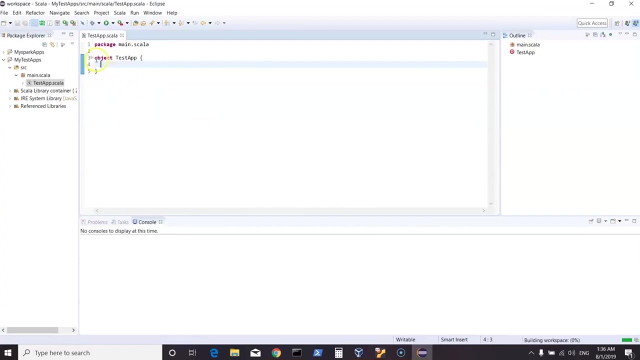 So for this then I can just right click and I can say new and I can just create an object and I can give it a name. so we can say test app and then we can say finish. so in case of Scala and spark, we need to create an object and then we need to define main class here. once that is done, we also 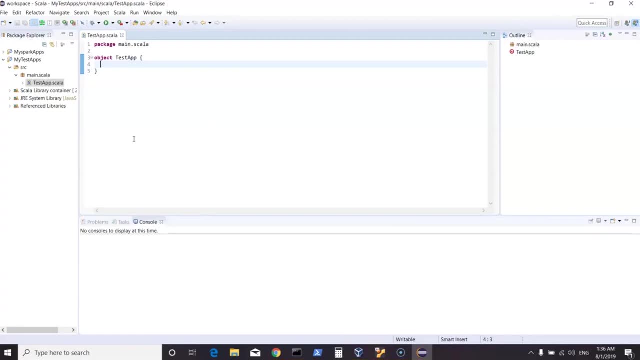 need to import some packages and we need to initialize the spark context now for that. you can take an example here. so I have already written the code and I can look in source main Scala and I have created an app called first app dot Scala. now here we have the package name we are importing. 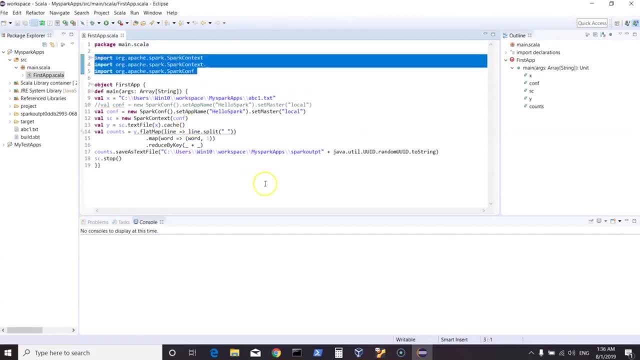 some packages which are required for us to initialize spark context and spark configuration. so it is spark context, spark conf, and here is my object, and for a particular project, at least one of your object or one of your application to be the main. so we define the main here by saying def, main, args and array of string. then we 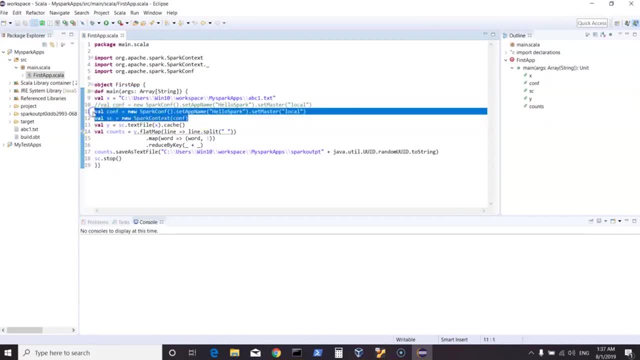 need to basically define our spark context. so I'm creating a configuration object here and then I say new spark conf. I am setting my application name to hello spark and then- this is very important- if you intend to run your spark application, either using spark submit or from your ID, you need to. 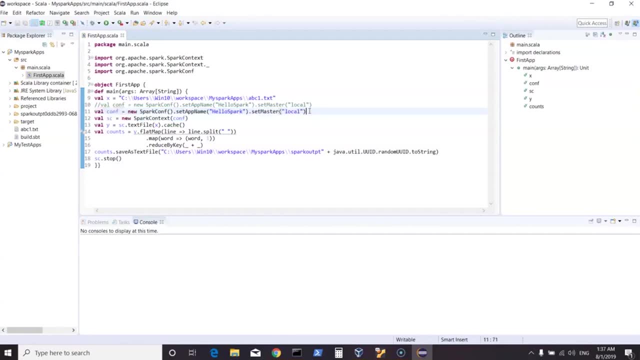 specify the name of your application. and then you need to specify the name of your application and then you need to specify your master as local. now that could be given with one thread or multiple threads. so this is my configuration, and then I initialize my spark context pointing to my 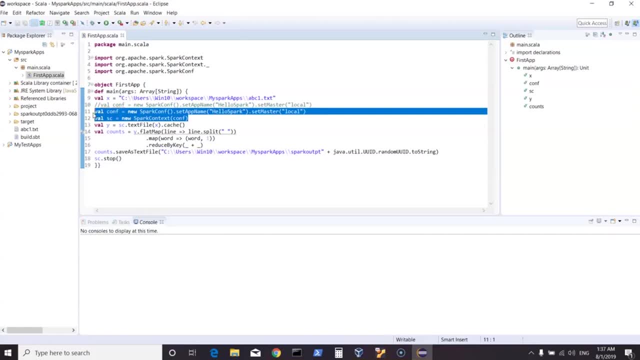 configuration. so this is the most important part here. now. if you see, this is something which I showed you in the command line. so I'm doing a val x and I'm pointing it to a file in my project directory which is abc1.txt. so this is just to. 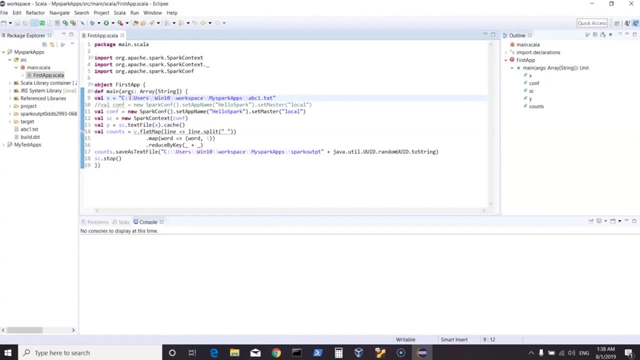 make sure that you are giving a windows path and you are giving the right escape characters. now, if it would be, if you intend to run this application on a hadoop based cluster, then you will have to give the path of the file accordingly, which we can see later. so here I have val x. I am pointing 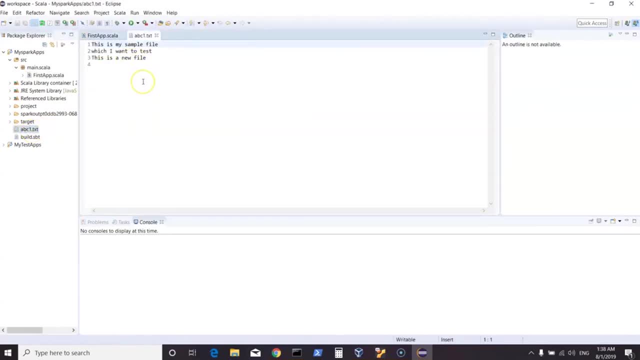 it to a file which I have created here, and this just contains three lines. this is my sample file which I want to test. this is a new file now. here I have created a variable called x. further I would say val y and I would use spark context method text file, like what we did in. 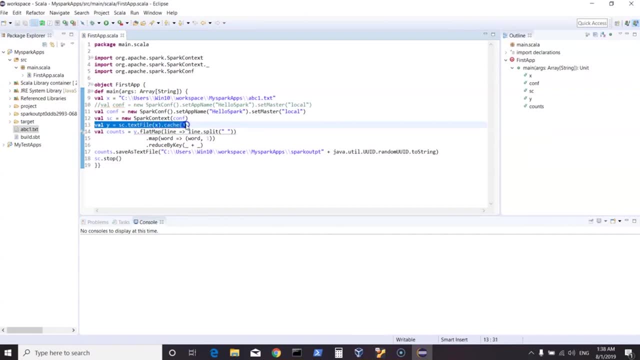 interactive way and I'm pointing it to x. I'm also using some extra features like caching, so that I can cache the RDD which gets created further. I create a variable called counts and then I do a flat map transformation on y, where I would split the content based on space. I would do a map. 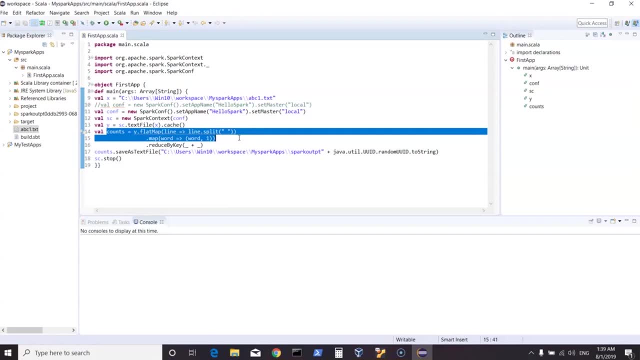 transformation, where I would get every word from the file and map it with number one, and finally, I do a reduce by key operation. once this is done, I do a saves as text file. now I could do a collect, I could do a take, I could do a count and I could also do a save as text file where I would want my output to be saved. 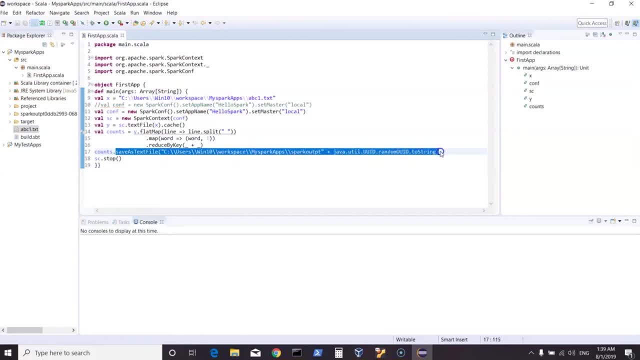 in this location. plus, I'm using a java utility to append a random number to my output directory. finally, I do a spark context stop. so this is my application and if you see, here my application completely compiles because I have already added the relevant jar files in the. 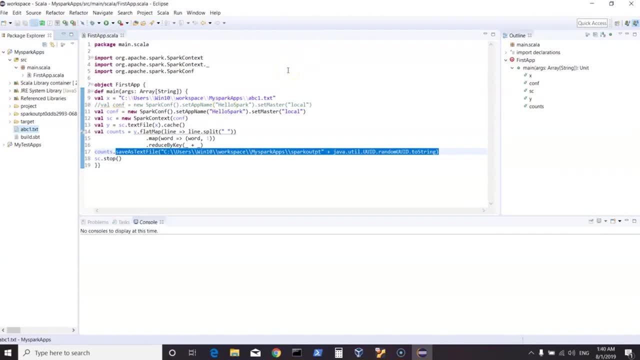 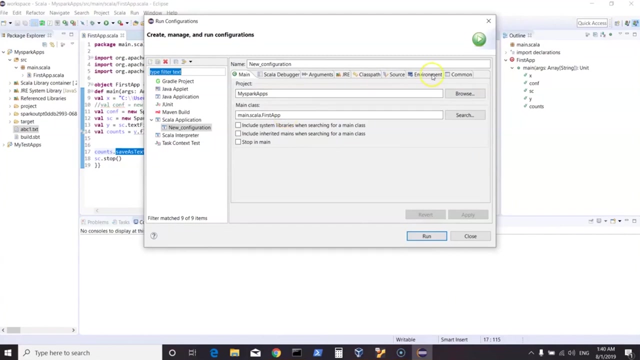 build path. now, once this application is done, we need to run this. but before doing that, we need to look into our run configurations. so you can click on run configurations, and here I'm giving my project name. I am specifying my main class, which is first app. then you can straight away. 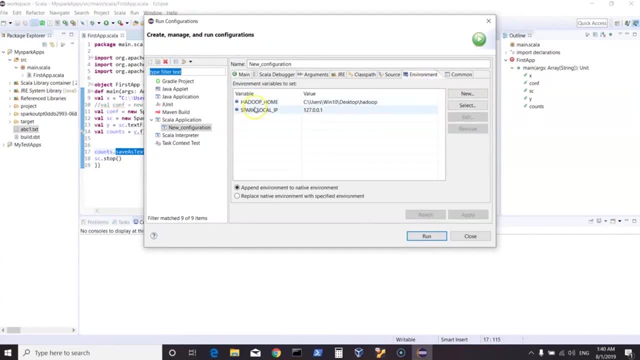 go to environment, and here I have added two variables. one is spark underscore- local, underscore IP, which points to this machine's local host. and then I have said Hadoop underscore home, because spark, even when you are running locally, would want if Hadoop is existing. so we can just set Hadoop underscore home- and I am pointing it to my desktop: Hadoop. 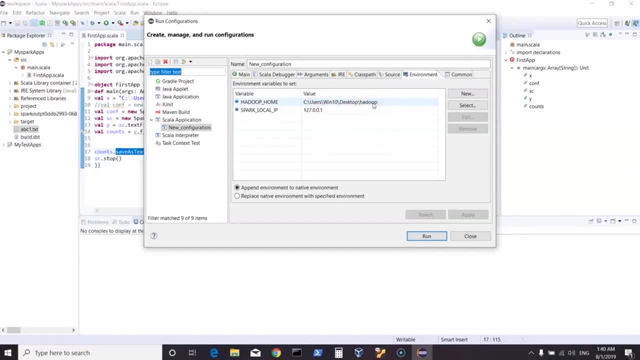 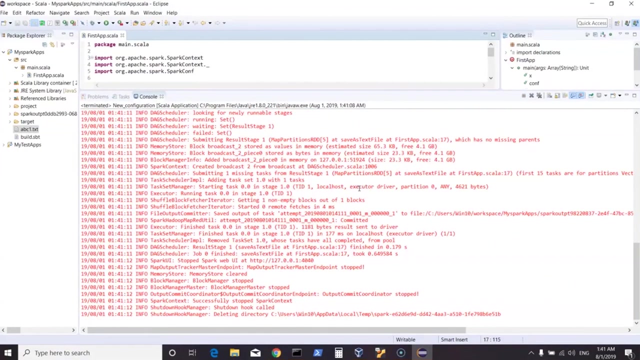 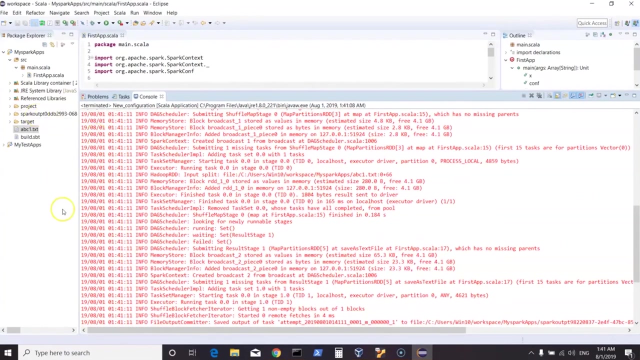 directory which contains bin folder, and that bin folder contains a winutilsexe. once this is done, we are fine, and then I can test my application. by just clicking on. now this should trigger my application on my Windows machine using my IDE. I didn't have to package this as jar, and here my application is completed, which should have created one. 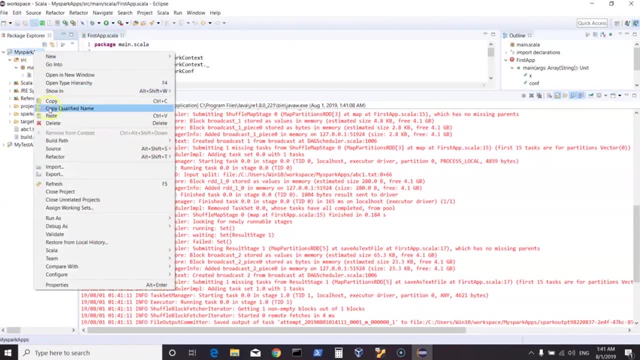 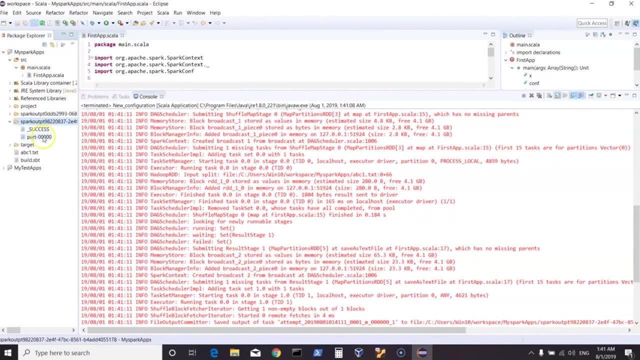 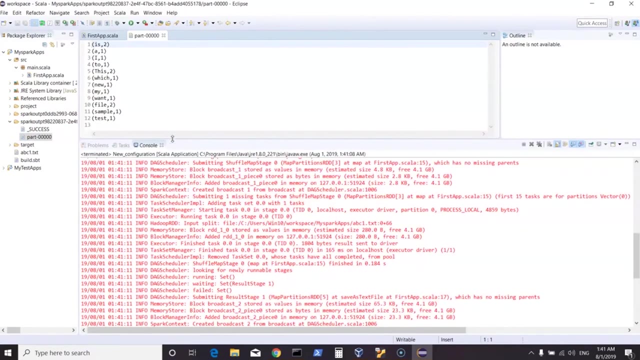 additional directory here so I can click on this, I can right click and I can try doing a refresh and here you see, a new output is created. we can look into this. it has a part file which shows my word count. so this is a simple example of setting up your IDE. 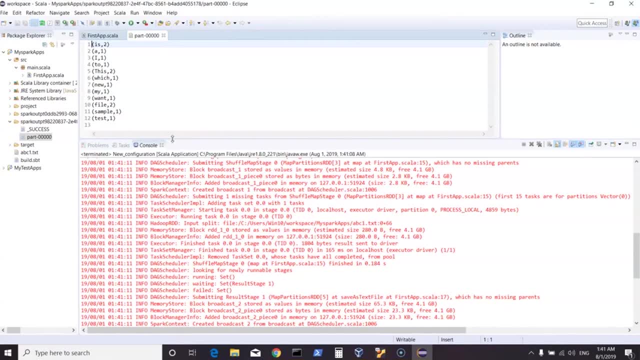 and running your applications from IDE on a local spark. now, what you also see is a build file here. what is that for? so, in case you would want to create a project and you would want to package the application as a jar file and then run it on the cluster using spark, submit now in that. 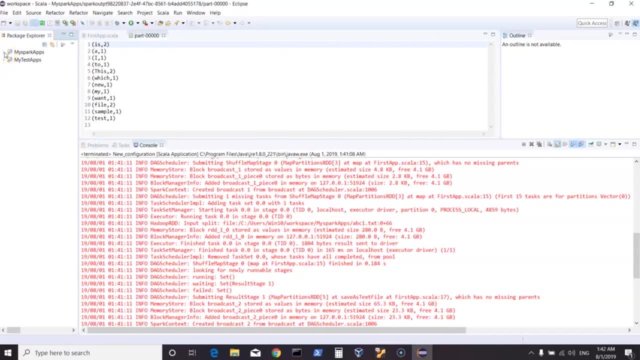 case, we can avoid adding the jars to my build path. but what I would need is I would need build dot SBT file within my project folder. remember, if you intend to package your application as a jar and then run it on a cluster or on a local setup, you would not need the build related jars. however, 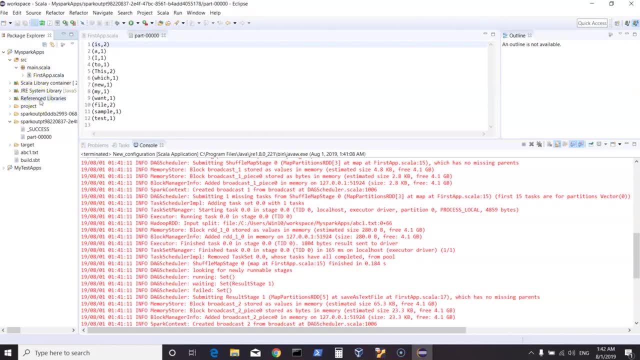 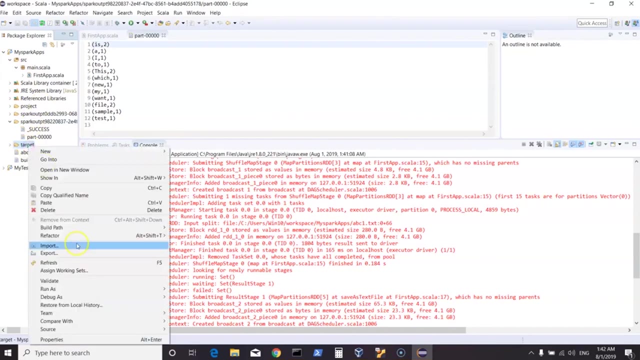 if the build related jars which are already here will not cause any harm, let them be there now. we have a build dot SBT file also, which is existing in my project folder. now, just for this run, I can in fact delete this target directory. it will be anyways recreated and if you would want we can. 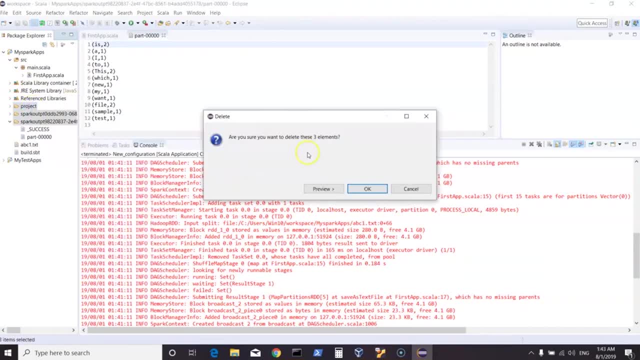 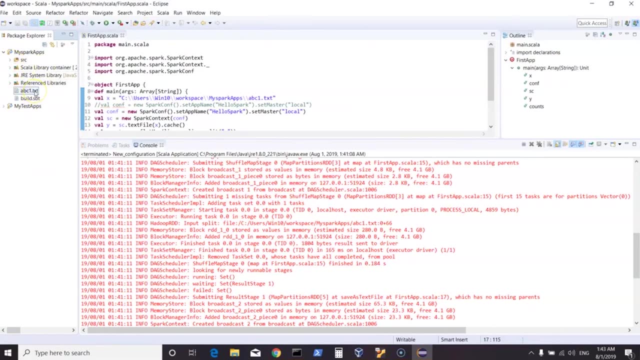 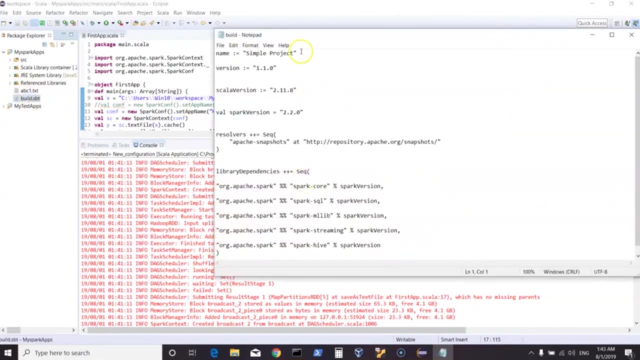 also clean up these. just to avoid the confusion, I will delete these now. I just have my project folder and I have the libraries, I have abc1.txt and I have a build dot SBT file. what does that contain? so this basically has a name. I'm giving a version which will be appended to my jar. I'm 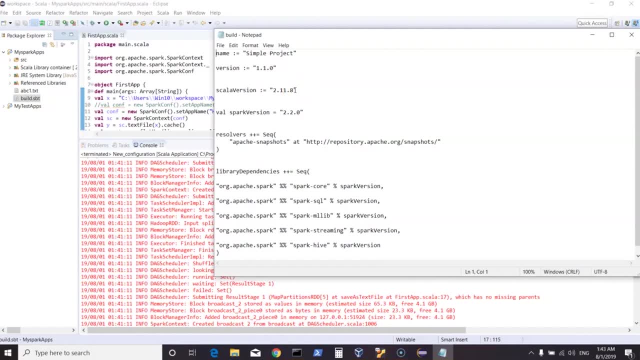 saying the Scala version which I'm using, which is 2.11.8, and I'm saying spark version, which is 2.2.0. you can replace these with the version which you intend to use. other than that, we are pointing to the different spark components and the relevant dependency related jars which your SBT can get for. 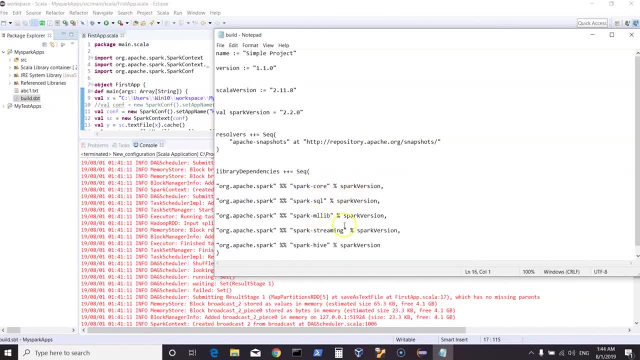 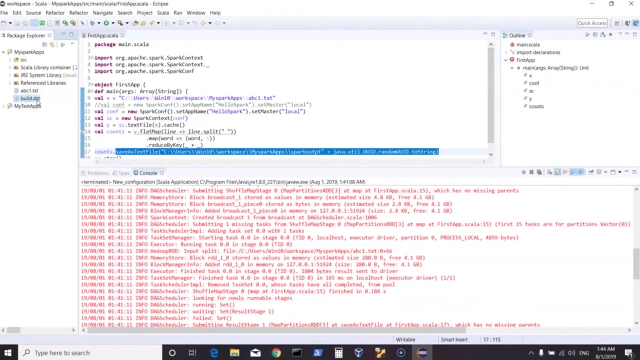 you. so I have given spark core, spark SQL mlib, spark streaming and spark hive, which will be then fetched from the repository. so this is my build dot SBT file, which exists in my project folder. we have our code written. we have our build dot SBT file, which is already existing in my project folder. my code is already fine. now we 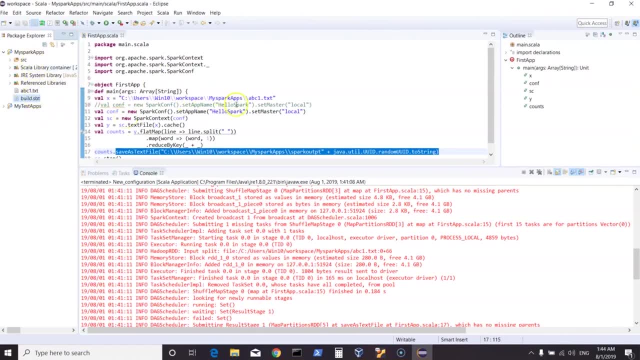 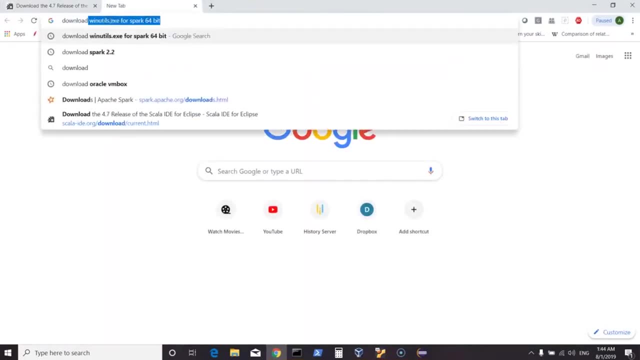 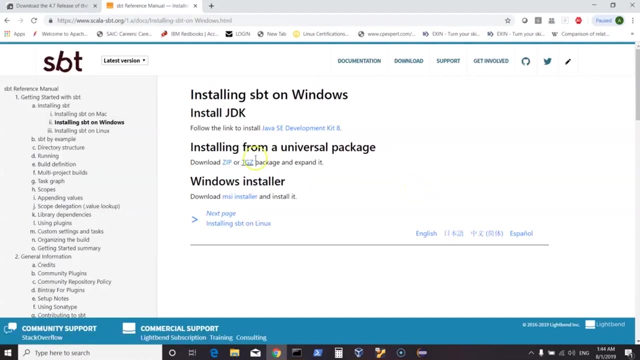 need to use SBT to package my applications into jar, for which you will have to download SBT. so you can just say: download SBT windows and that should take you to the installing SBT on Windows page. now, here you can just download the msi installer and run through. 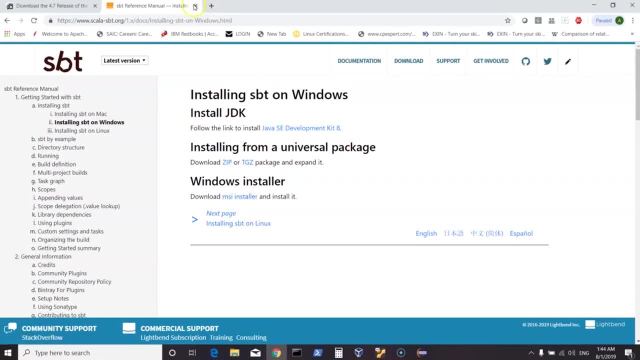 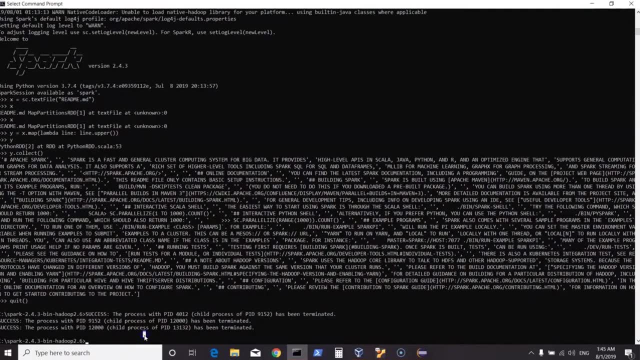 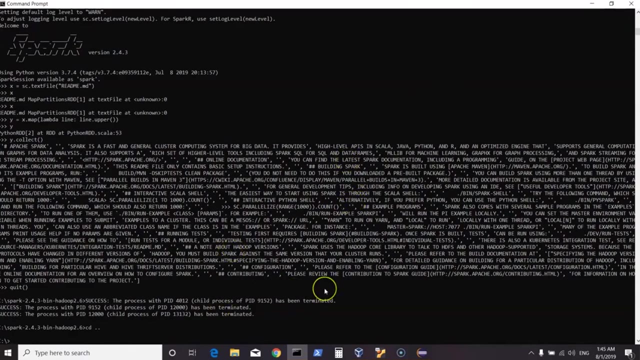 the installer, which will basically install SBT on your machine. now I have already done that, so my build file is ready, my code is ready. all I need to do is now use SBT. so what I can do is, from my command line, I can just say CD and I will go into users, I'll go into win 10 and I'll go into my. 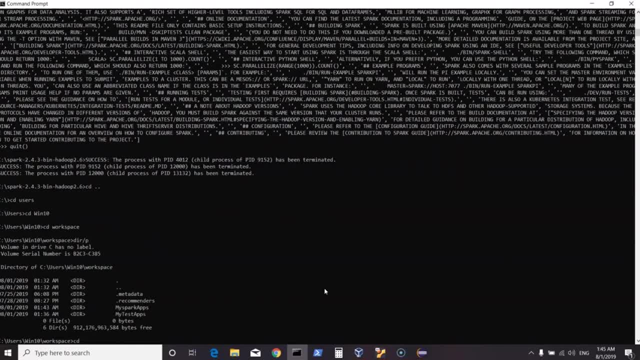 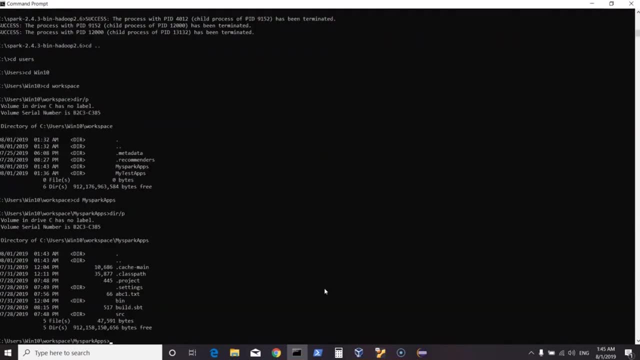 projects. now here I can see for my projects and I can go into my spark apps. now, once I'm in my project folder, we can double check that it has a build dot SBT, which is fine. SBT is already installed on this machine and I can just say SBT. if you would want to check, you can always do SBT. 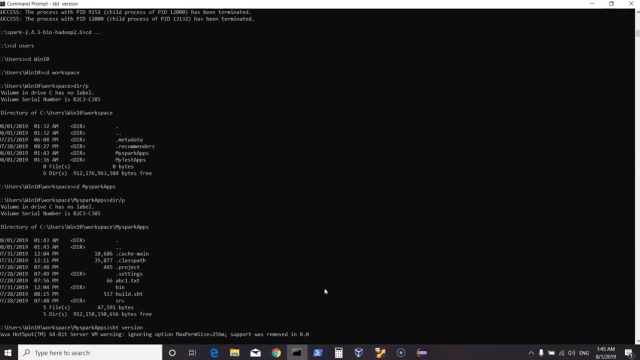 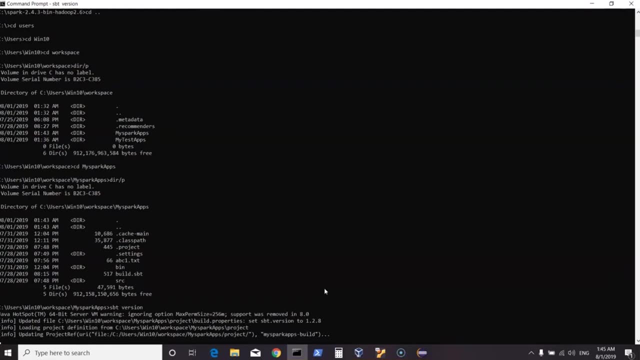 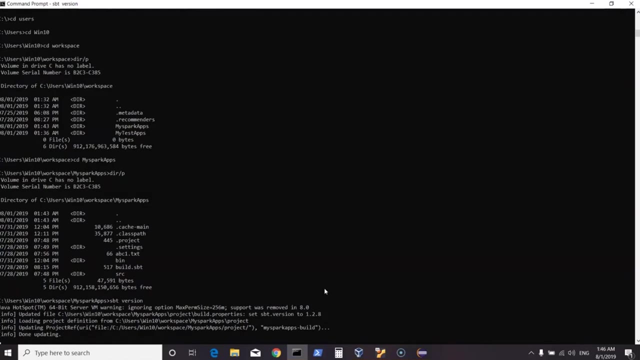 version to check if you have SBT. and this command is also done once you install SBT for the first time you can always do SBT version and before displaying it was displaying SBT's version. it will try to fix all your dependencies. it will try to get all the relevant dependencies. so this is just to check that SBT is installed on. 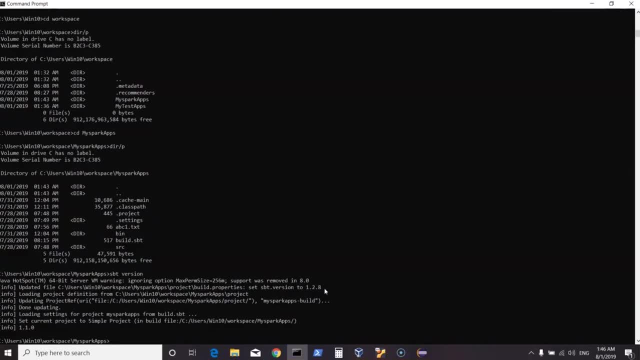 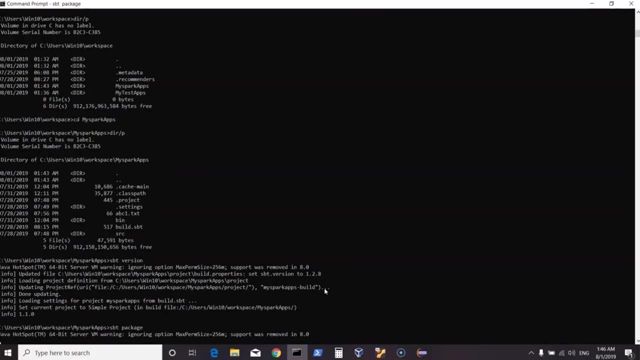 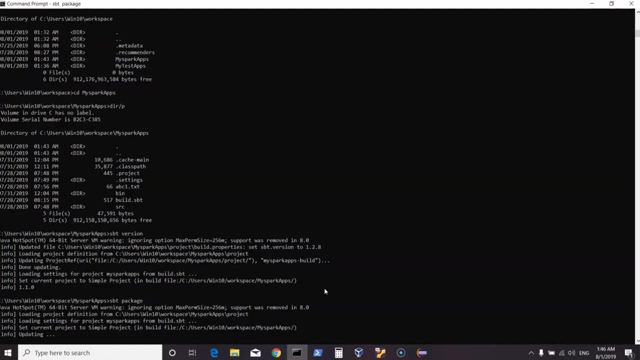 my machine. as I said, my code is already ready. I have a buildsbt file and I can just say: SBT package, which then will refer to buildsbt, will look for your code in source main Scala and then, if everything is fine, it will package it as jar and it will create folders within your project folder. we. 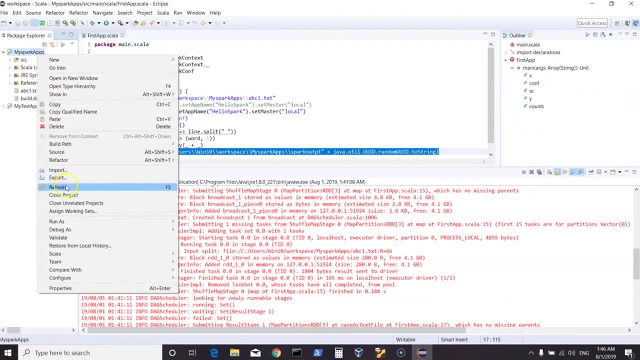 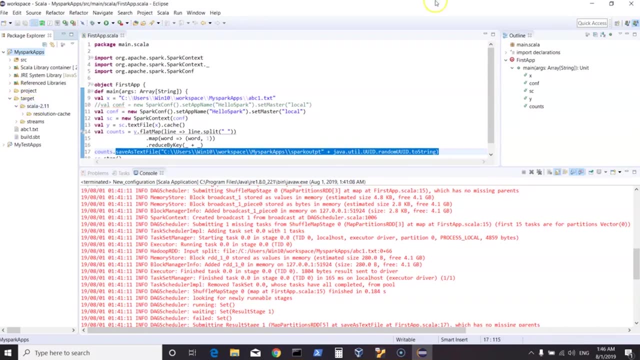 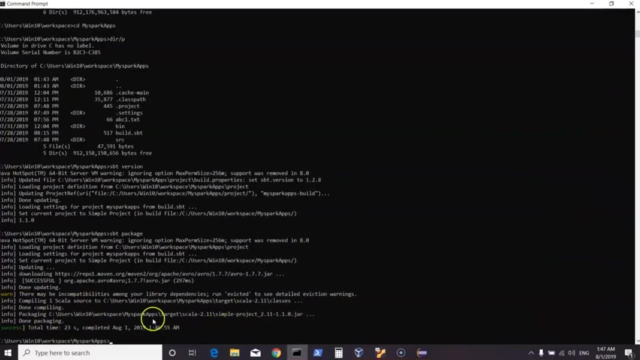 can click on this. we can try doing a refresh to see now. if you see, here the project was again created. a target folder is created within Scala 2.11. I will have my jar created so we can see that my SBT was fine. it has packaged the code and it has created a jar file as simple. project 2.11. 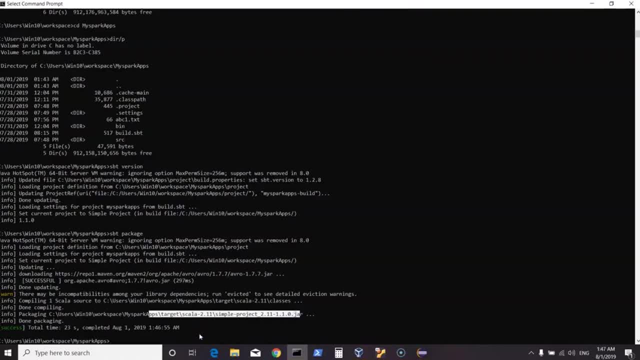 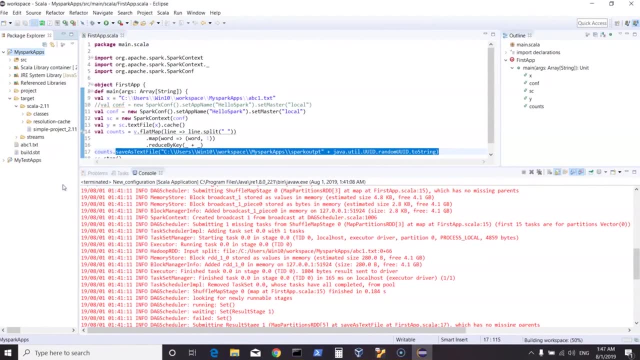 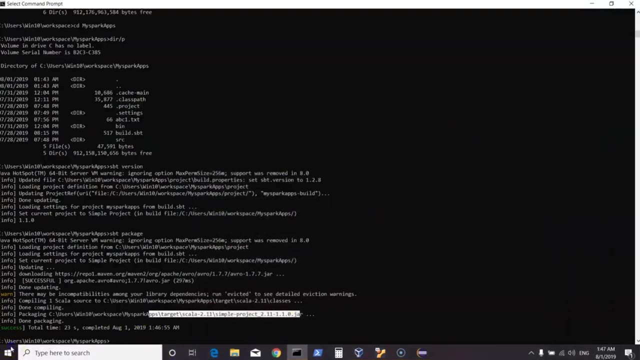 which can be used to run on the cluster or in a local mode. let's check in Eclipse. I'll click on this and I'll just do a refresh, and I see my jar is already existing, which basically means then we can do a spark submit. so this is where we see that I am already running a spark submit. 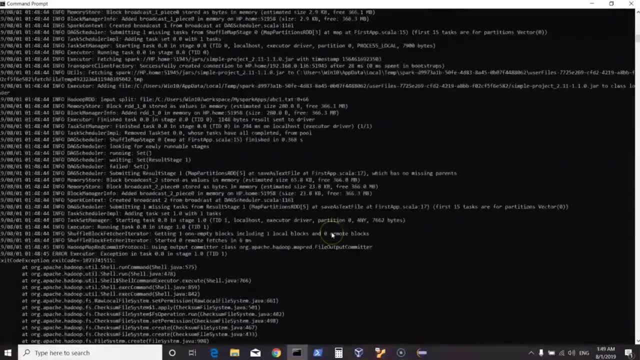 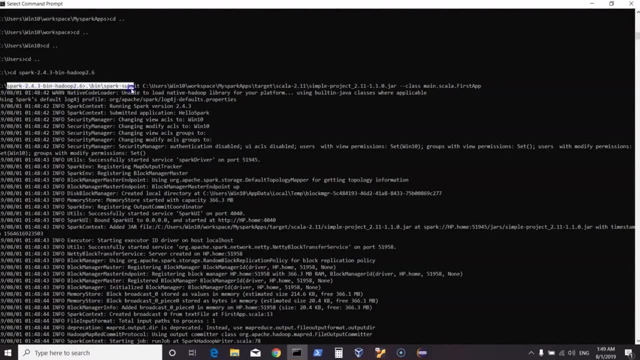 command. now this might show up some error messages, but we can see how we did this. so if you see here the packaging was done. I went into my spark folder, I did a bin slash, spark submit, I mentioned my jar file and then I said: my class main dot, Scala dot, first step. so this is my app and this is how I'm. 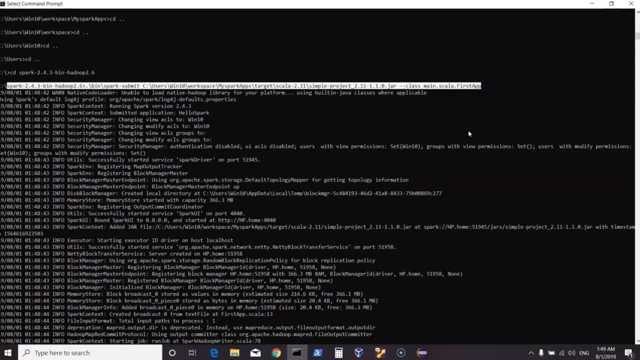 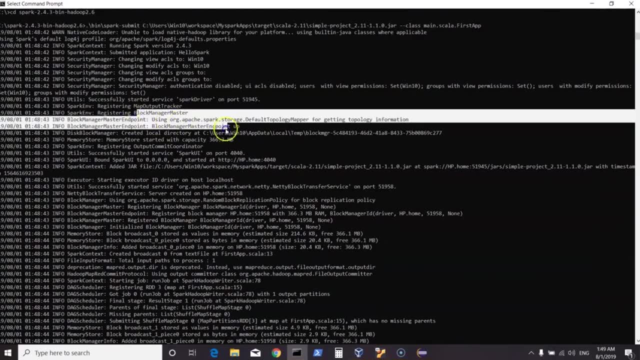 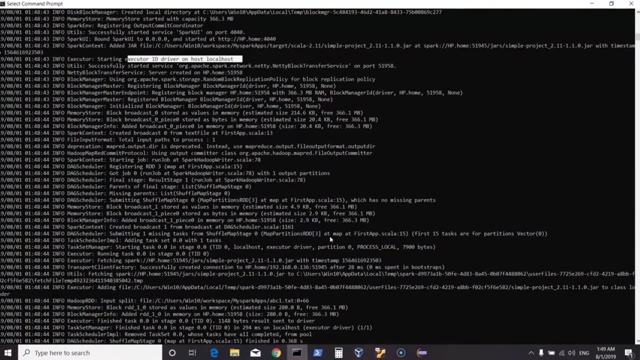 using spark submit to submit an application which is running in local mode so we can see further. if it starts processing, so here it says created local directory, then it's starts an executor on local host, it goes for execution and then, if we see further, we could also see it. 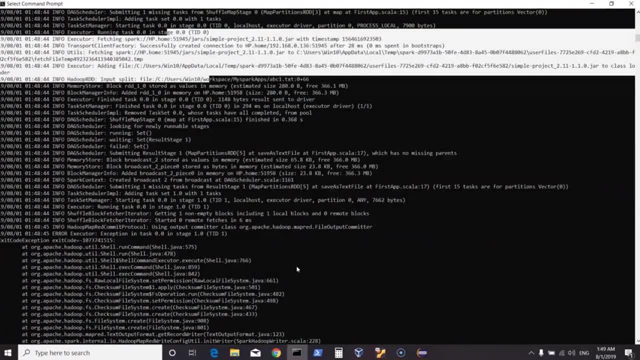 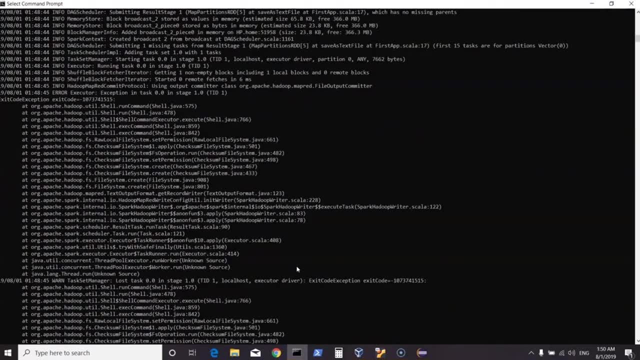 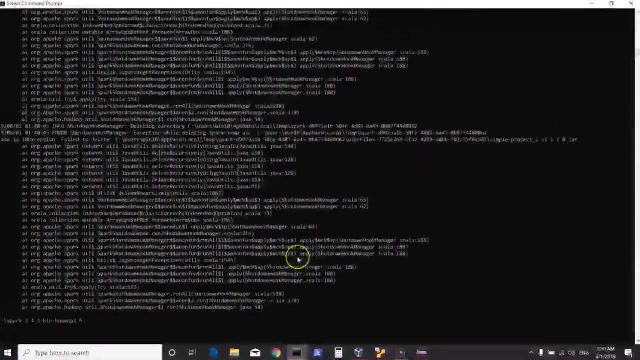 will add our jar to the class path and then, finally, it should be doing the execution now if there is any error message that might be related to your file not being deleted or if there is any problem with executor, so we can basically come back and check here if there was any specific. 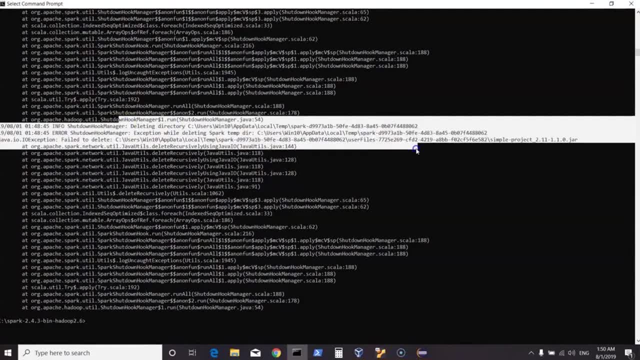 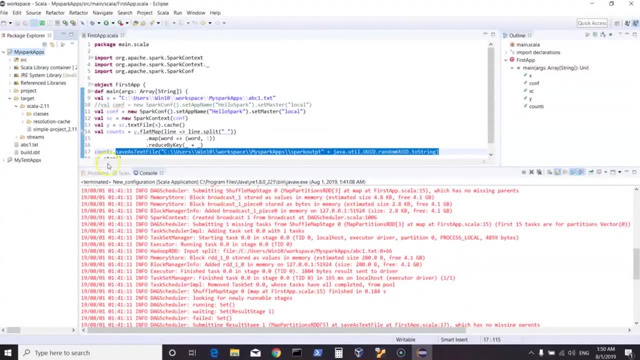 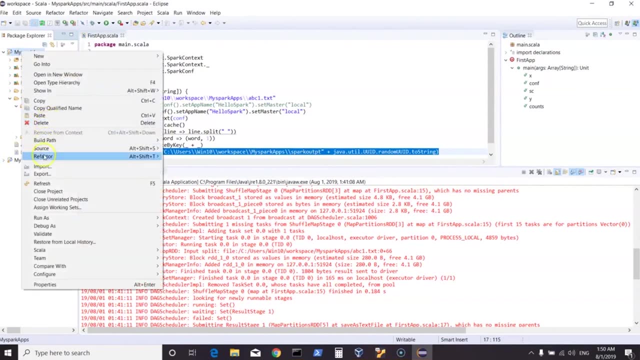 error. so it the error was that it tries to delete a temp directory but it does not have the permission. so we have not done that. but as per my application, it should be creating a output in this folder as Spark out. so let's click on this and see. I'll do a refresh right and if you see, a new Spark output has been. 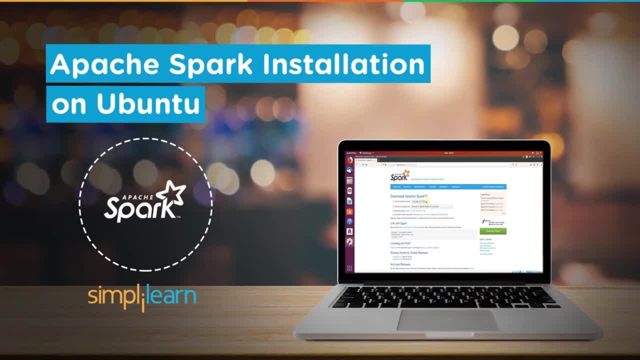 created previous sessions, we have seen how we can set up Spark on Windows or set up our Spark related on our applications on Windows. now here we have a quick demo on setting up Spark as a standalone cluster on Ubuntu machines and then trying out Spark way of working, for which we need at least 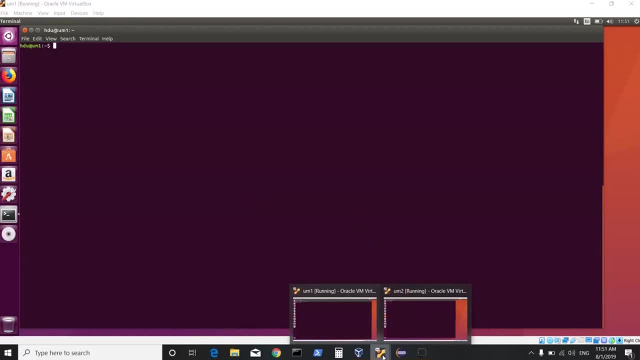 two machines, and here I have Ubuntu machines set up, um1 and um2, just to give insights on how my machines look. so if I look in my etc. host I have the IP address of multiple machines so I can ping one machine to other machine by just doing a ping um2 and that. 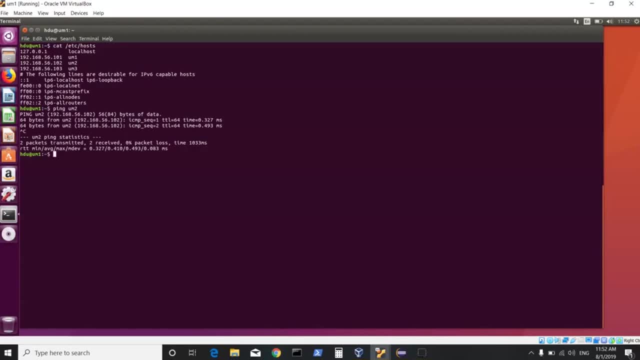 should work fine. similarly, I have also set up ssh access for these machines. both of the machines have HDU as the user and I can just do a ssh, um2 and that logs me into the second machine without a password. similarly, I can check the same thing from my second machine by doing a ssh. 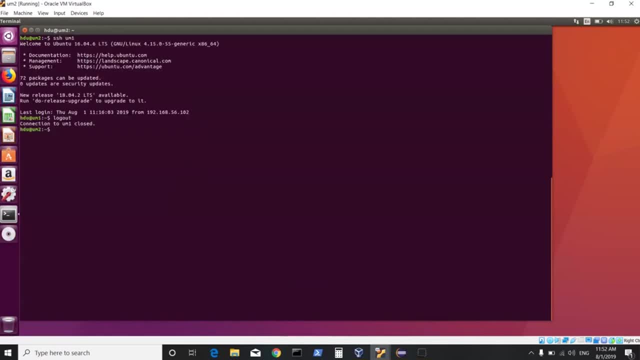 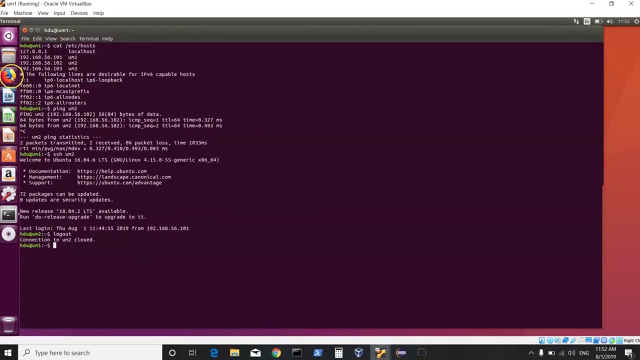 um1, and that works fine too. so we need two machines which can ping each other, firewall disabled, able to ssh each other, so that we can set up a standalone cluster of Spark. how do we do it? so? first thing is we will have to download the Spark related tarp file. now I can just go to Google and I can type: 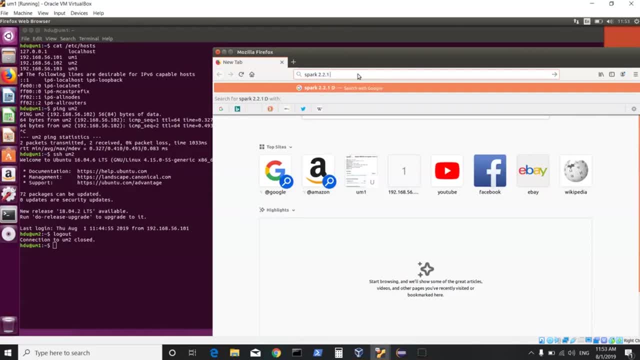 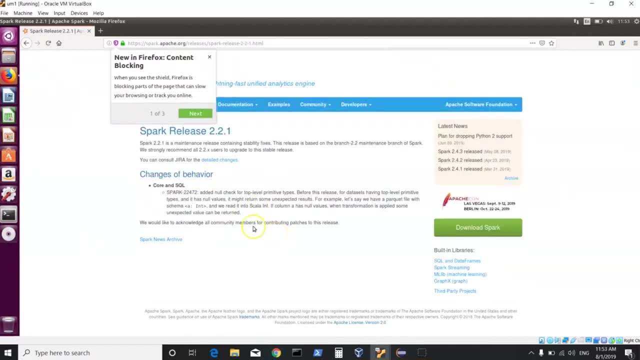 in Spark 2.2.1 download. now, that's what I'm interested in, and this takes you to Spark release 2.2.1. however, here it shows you the latest release is 2.4 and then 2.4.2. so what we can. 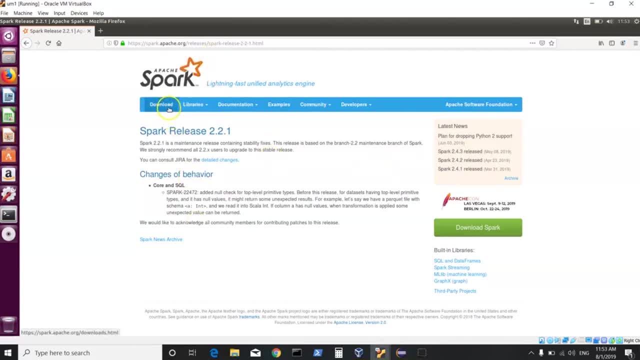 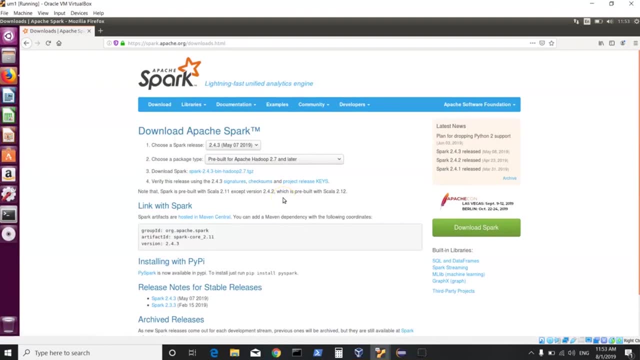 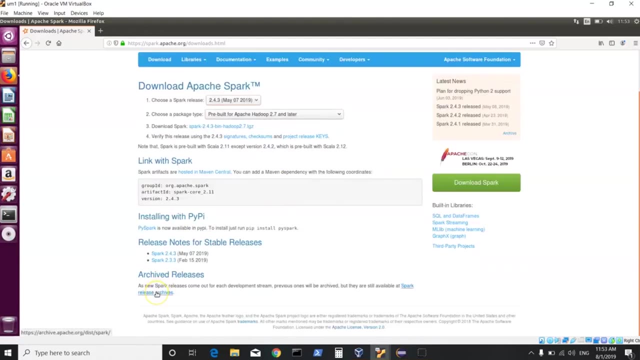 do is we can go to archives, so I can basically look at existing versions. now here I can click on download and this shows me a Spark release and also pre-built for Apache Hadoop. now what we can also do is we can go to release archives for an older, stable version. I 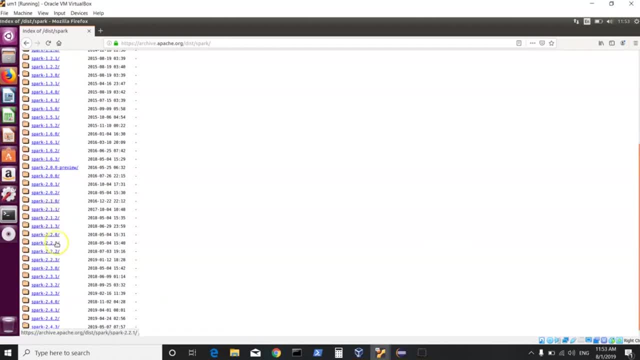 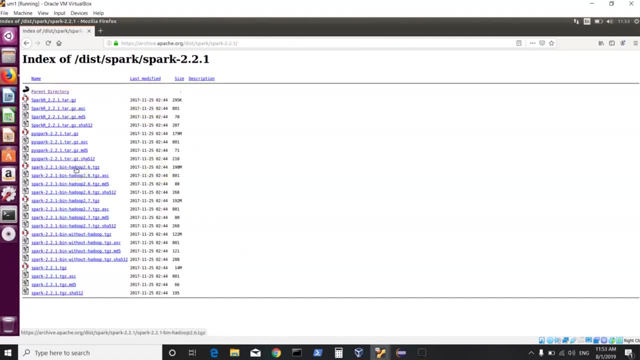 can click on this, and here I have Spark 2.2.1. now I can click on this and we can either install something which is not already built or we can download this one, which is Spark 2.2.1. bin Hadoop 2.6 point T, G, Z, so you click on this link and then save this file, which I have already done. 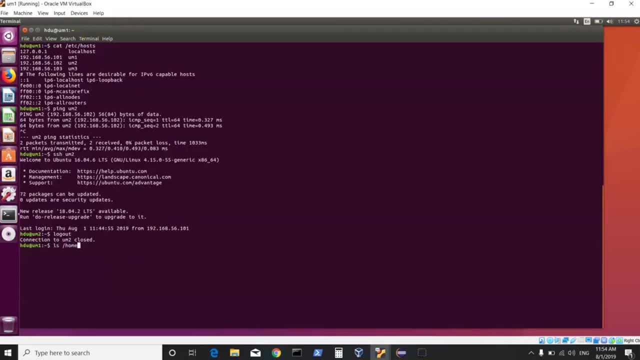 and here, if you see, in my machine, I have home HDU downloads which has my current packages which I have downloaded. also, if you notice, I have downloaded JDK 8, so you can check on my machines. so, apart from machines being able to ping each other and being able to do a SSH, 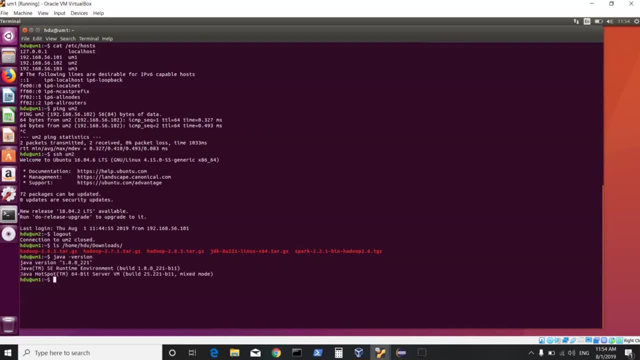 we also need machines to have Java which is already installed. once this is done- now I have my Spark related package, so I go into user local directory and then you can give a command here that is sudo, CF, home, SDU downloads and then give your Spark package. now, once you do this, this will untar the 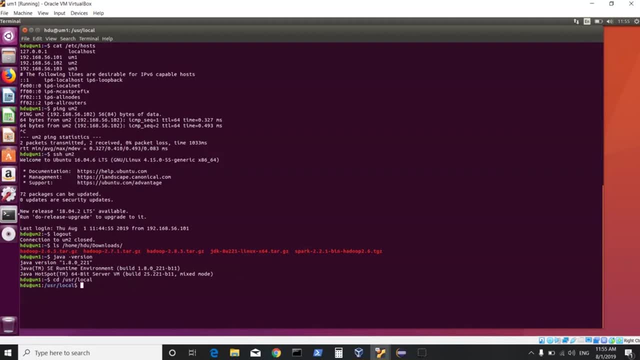 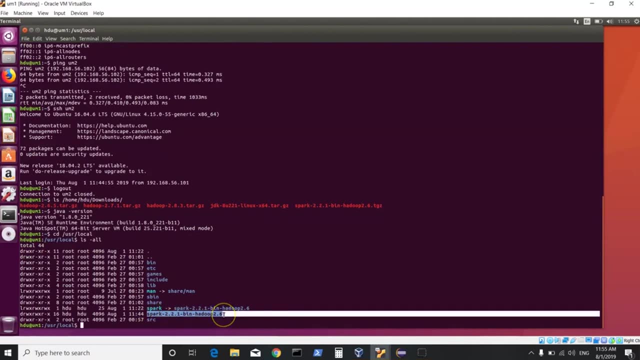 Spark directory and create a directory in my user local location. if you see here, this is the directory which is created, but you also see that there is a Spark link which is pointing to Spark. now that is because if you would want to work on a newer version of Spark, you could just do. 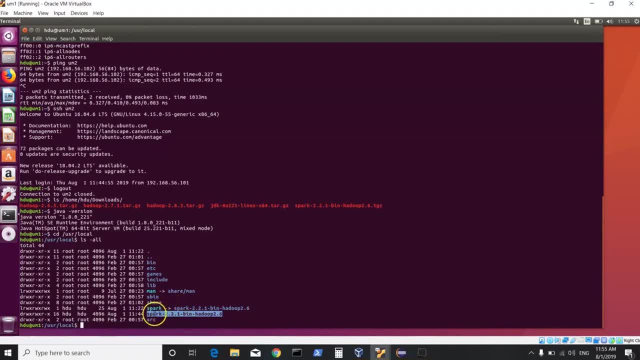 the same thing for newer version and then make your link pointing to the newer version of spark. how do you create a link? you can just say: sudo ln minus s. you can give your spark directory and then you can create a link. so i've already created a link and my spark 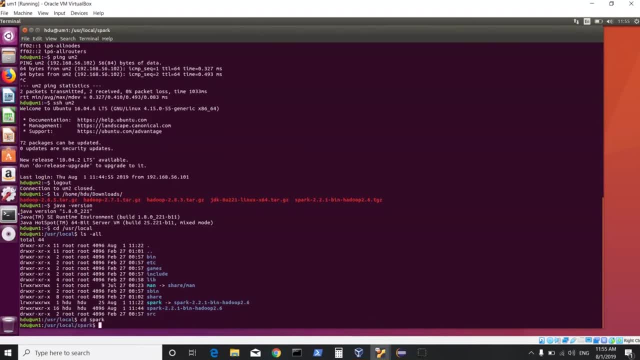 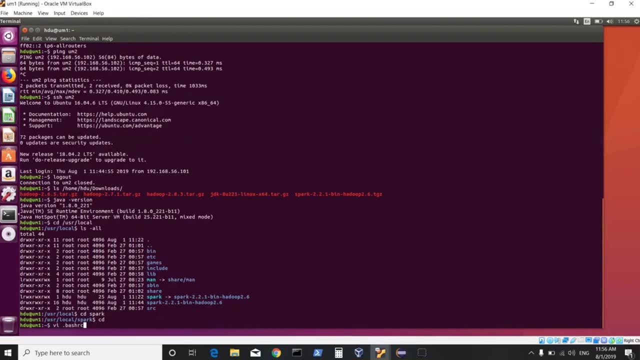 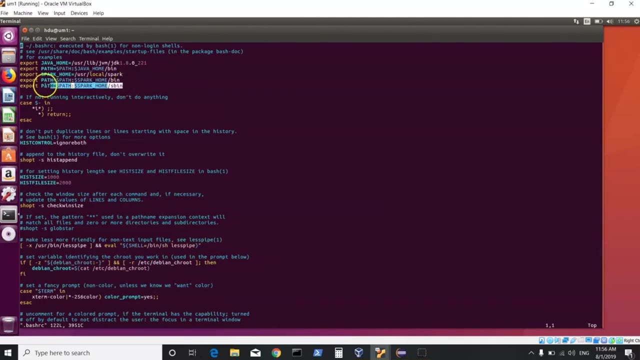 path will then become this: now, what do we do with this? once we have done this, once we have created a link, we can go into the bash file of my user and, if you carefully see here, i have given my java path so that i can execute java related commands, and i have also added my spark related path here, which 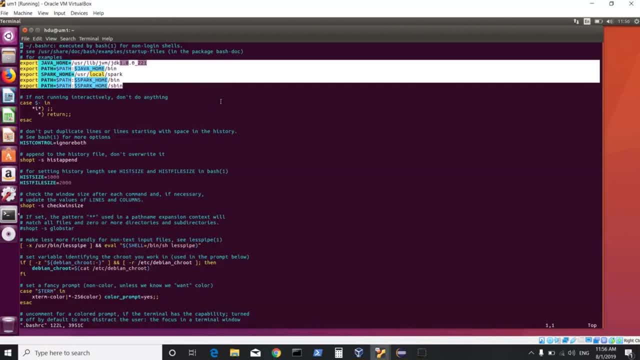 says user local spark. so in case you would be changing your spark version to a latest one, you will not have to change things in your bash file. only thing you will have to do is unlink the existing spark link and create a new link to your newer version. so this is done on this machine. 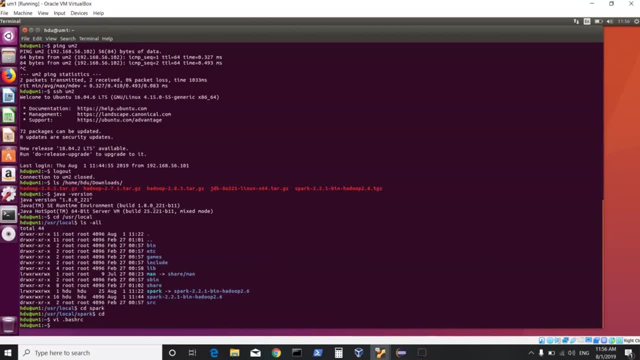 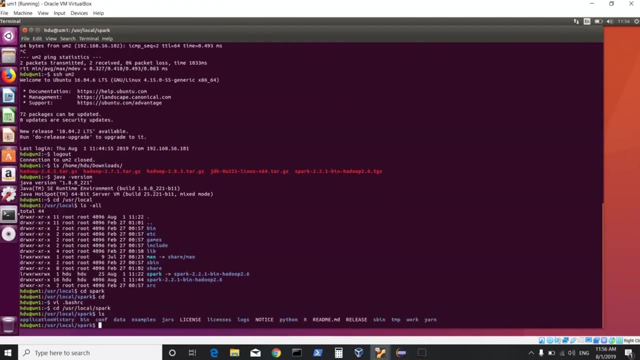 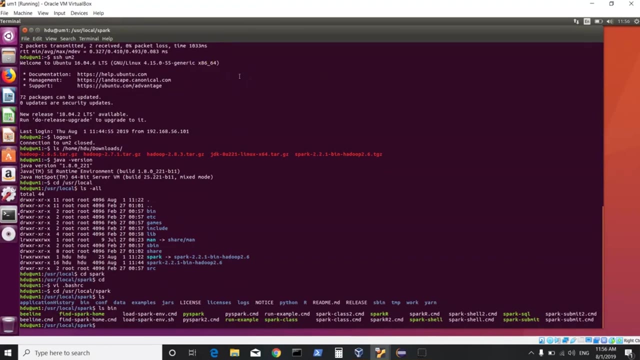 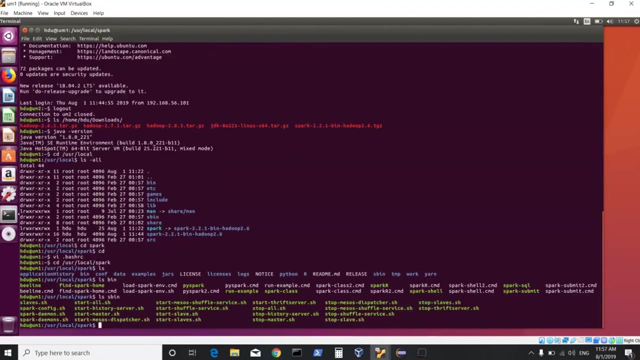 and now i can basically be using spark. now, before doing that, we can go into user local spark and this has different directories. so if you look in bin, these has the binaries programs like your pi spark, your spark shell, spark sql and spark submit, which we will see how we can use here. if you look in sbin, it has other startup scripts to start your. 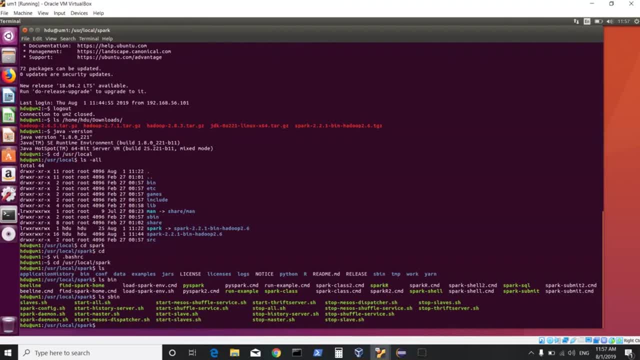 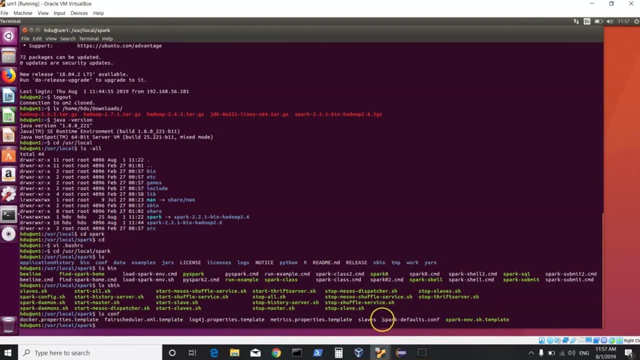 history server or to start your master or worker processes. if you look in conf, this has your config here by default. you might see spark minus default dot conf- dot template. i have renamed that to dot conf. slaves template has been renamed to slaves, so let's look into this so i can go into conf. 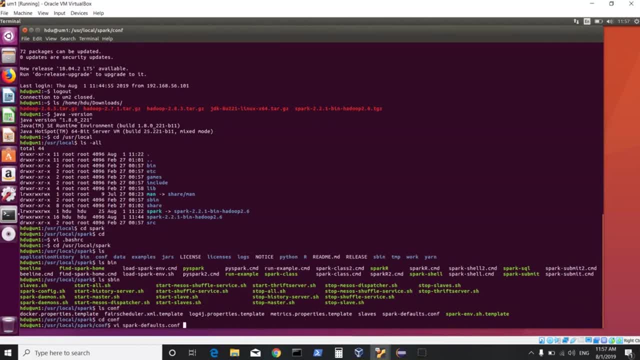 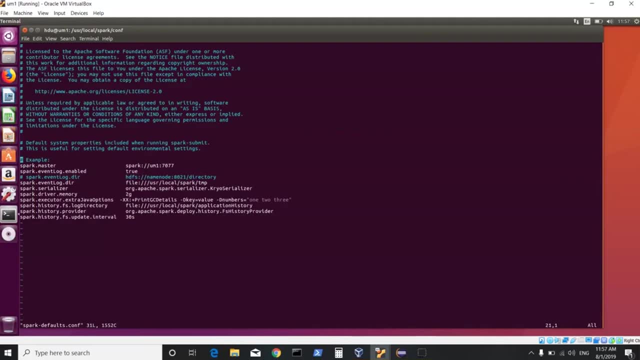 and then i will look in spark default conf now here based on our setup now here we intend to set up a spark standalone cluster that is without hadoop, but i would want to have a spark standalone distributed cluster. i have uncommented this property. it says spark dot master and i say spark and i also mentioned 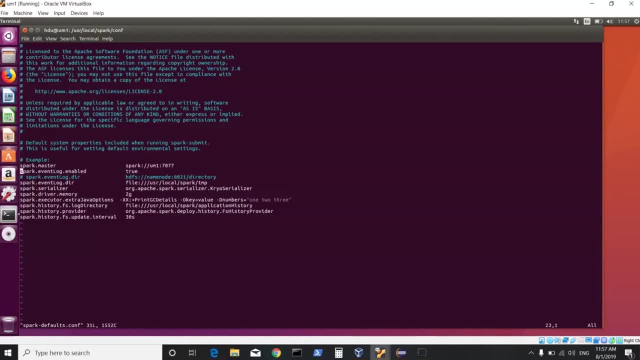 that my master will run on this machine, which is um1 spark event log dot enabled, is true because we would want to track the events. i have mentioned a directory, so this is a local directory in user local spark and we will have to create it. it talks about the default serializer. it talks about the 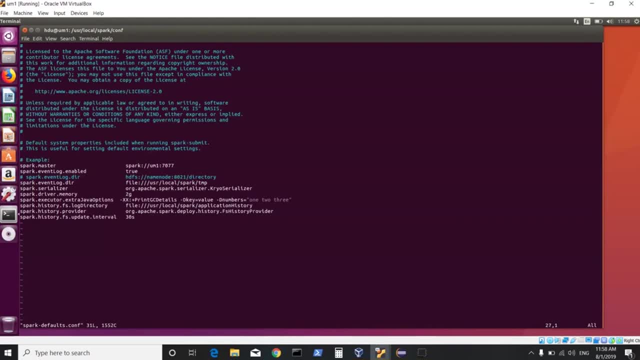 driver memory, which was by default 5 gigabyte. i have reduced it to 2 gigabyte based on my machine configuration. you have java options and then, if you intend to run a history server so that whenever your spark applications complete, you will have your application stored in history. 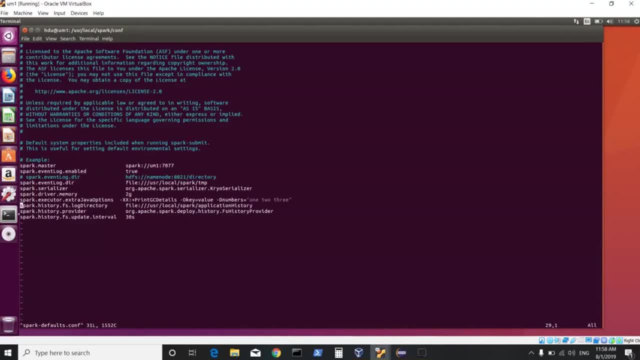 server. i have given the log directory which is user, local, spark and then application history, and this also needs to be created. we have spark history provider for the class which takes care of history server and the update interval of looking for your applications. so this is what we 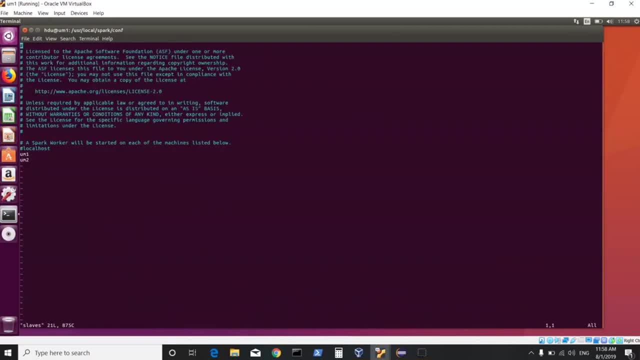 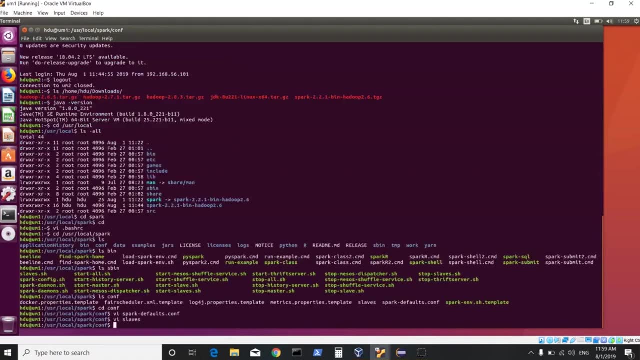 are going to do in our spark default and if you look in slaves, i have given the machines where i would want my worker processes to run. so that is um1 and um2. now, once you have made your changes in your spark default, conf and slaves file, what you can simply do is scp, assuming that, whatever. 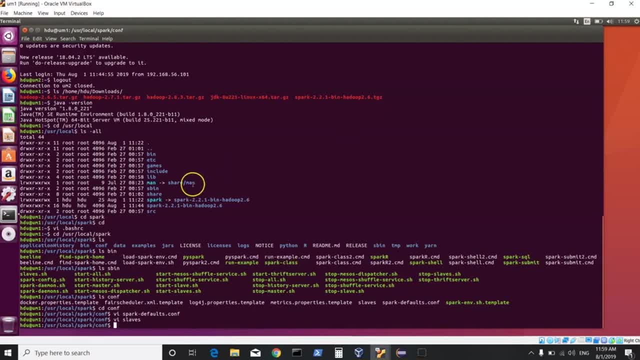 was done on this machine, that is, untying your spark directory, creating a link, updating your bash rc and untying your spark directory, creating a link, updating your dash rc and renaming your config files. same steps need to be done on the second machine and your second machine. 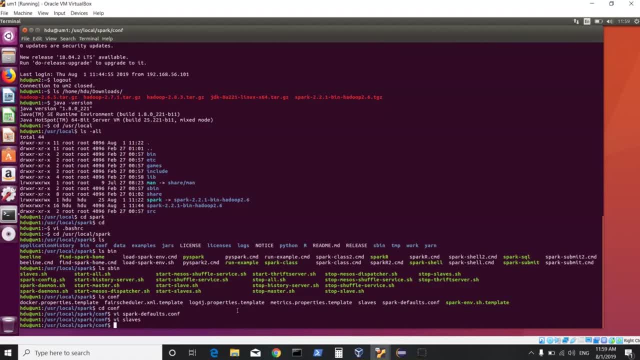 would also be prepared to be used for your spark cluster. so once you have both the machines, which can ping each other, which can ssh each other, both of the machines have java, both of the machines have the same spark version downloaded and the basic setup done, i can just easily copy the spark. 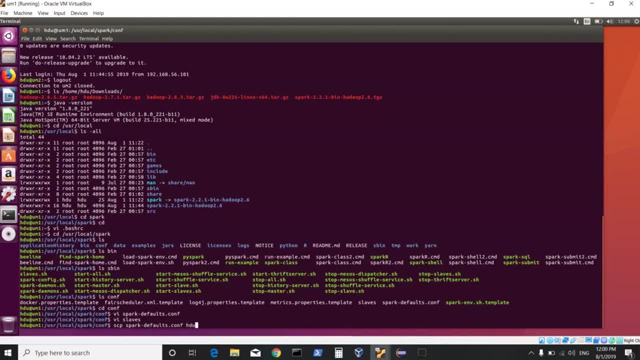 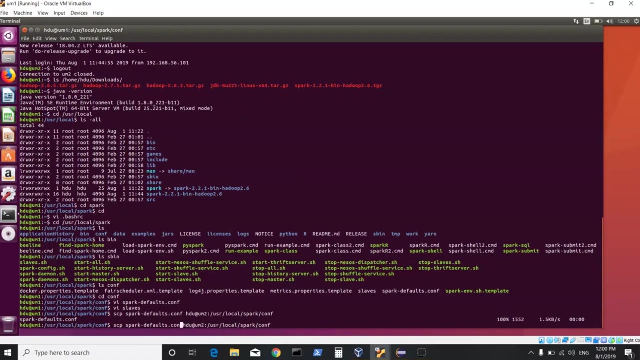 related config from here into my other machine, that is sdu um2, and then i can give a path which is user local spark conf, and in this way i don't need to edit my config files again, and similarly i can even copy the slaves file. this is: 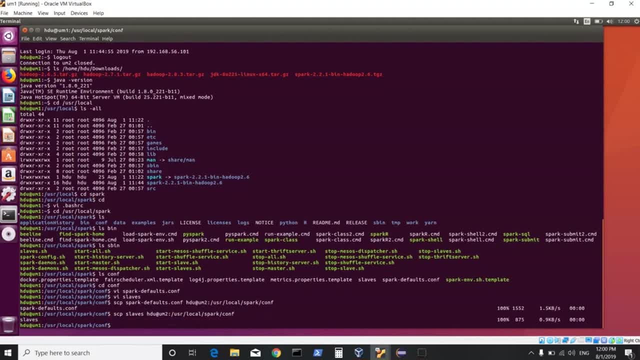 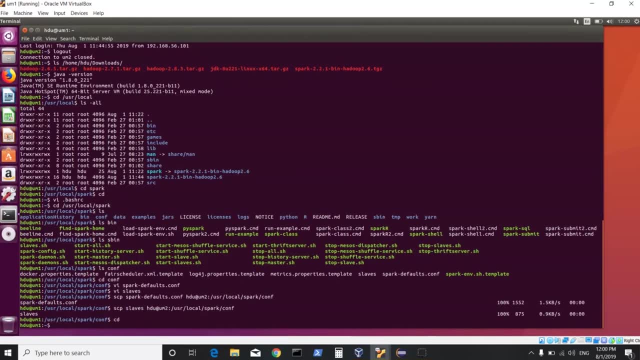 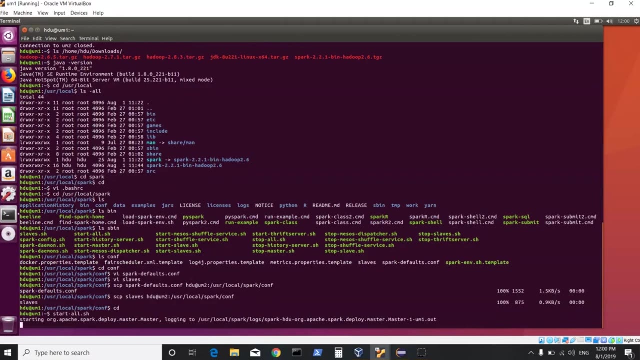 all we need to basically have our spark standalone cluster. now, since we have updated our bash rc, we can give our spark command from anywhere. we have set up our config files, so i can just do a start dot sh and that, based on my config files, based on the directories which are mentioned, it will 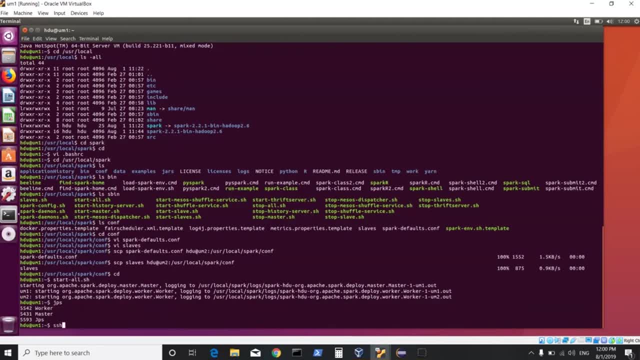 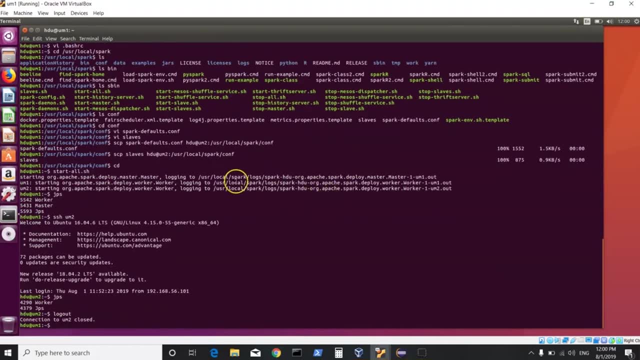 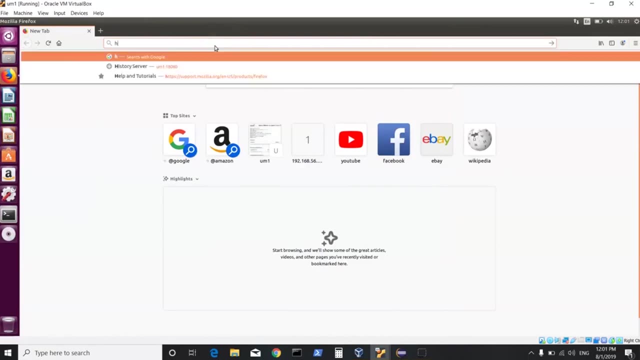 start my master process and my worker process on both the machines. so here we have a spark standalone cluster which has two workers and one master. now we can always go to the browser interface and we can check for the spark ui, which should be available, by typing in http: slash my master and 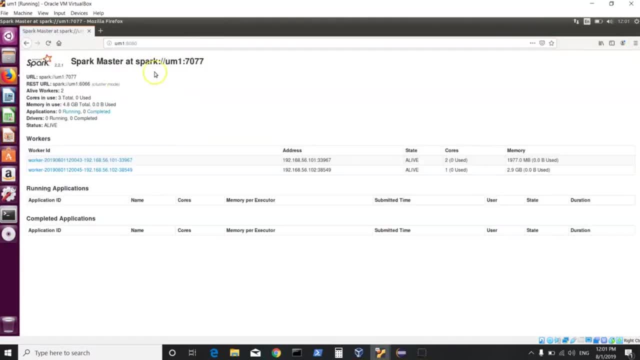 then the port is 8080, so this shows that i have a spark master running. i have two worker processes. right now there are no applications which are running, but my spark ui is already available. when we start using spark, either by spark shell or pi spark or even spark submit, we will see our applications. 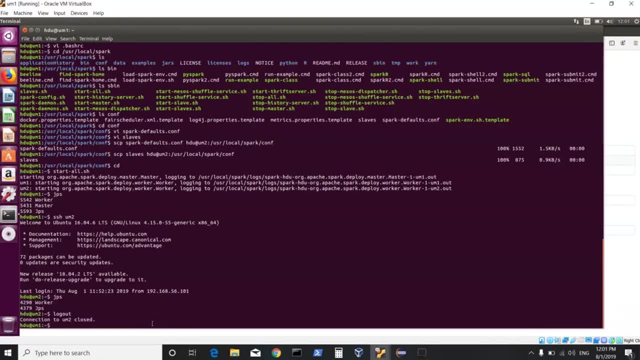 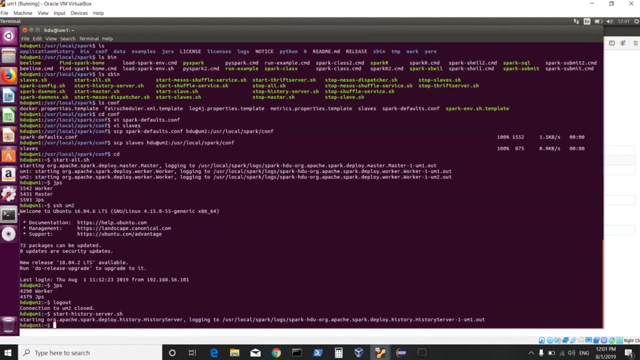 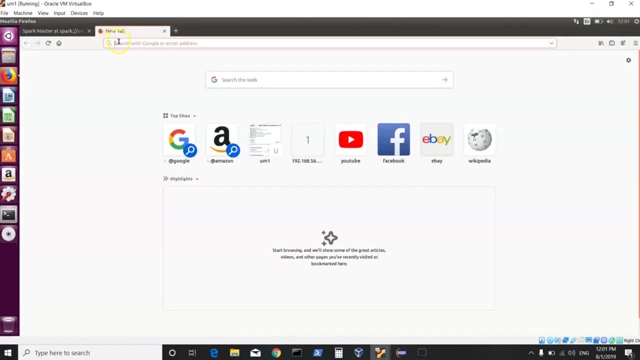 getting populated here. additionally, we can also start the start history server by just saying start history server dot sh and that will start my history server. once this is done, we have a history server also running and we can go back. and then we can again pull out the history server user interface by giving in the port, which is default, 18080. 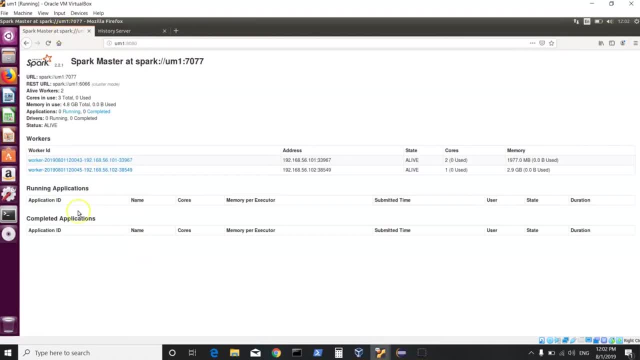 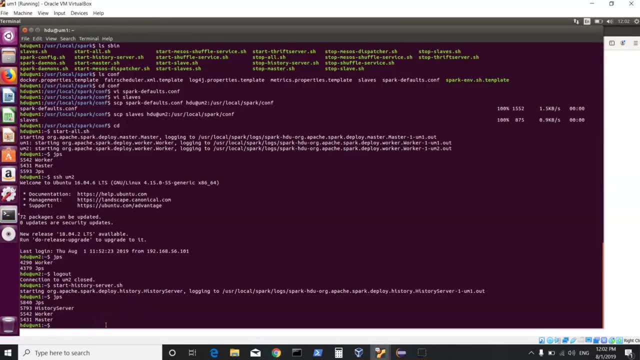 so i have a spark standalone cluster with one master, two workers and also a history server which is running. once we have this, we can try working with spark, either with spark shell or by spark, or if you have packaged your application as a jar using sbt or mevin, you could also use. 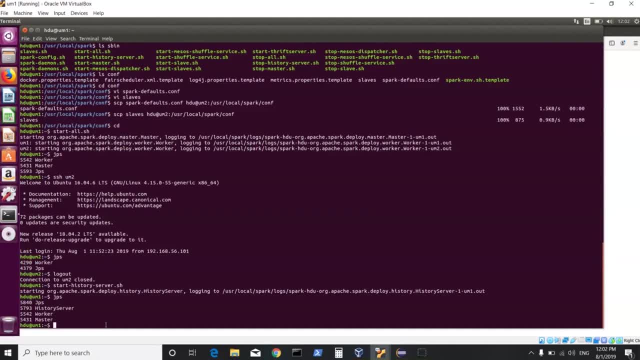 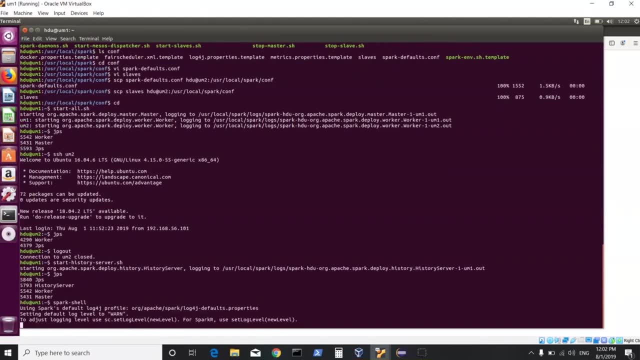 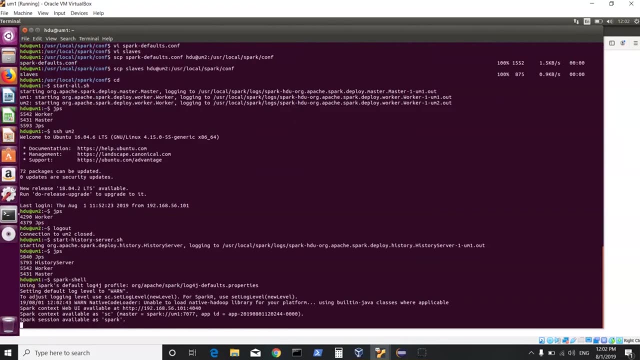 spark submit. additionally, you could also use spark sql. so to work with spark, i would just say spark shell on one of my machines, both my machines, which have worker processes running. we can start our spark shell on any of these machines. remember here, our spark will rely on the storage of these. 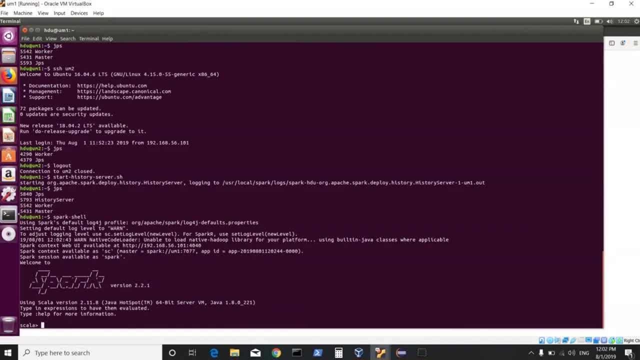 machines. that is the file system, because it does not have any hadoop or distributed file system. we have started our spark shell and that shows spark context, which is available as sc. spark session is available as spark, so to work with spark core and rdds we would be using spark context and if you intend to work with spark sql. 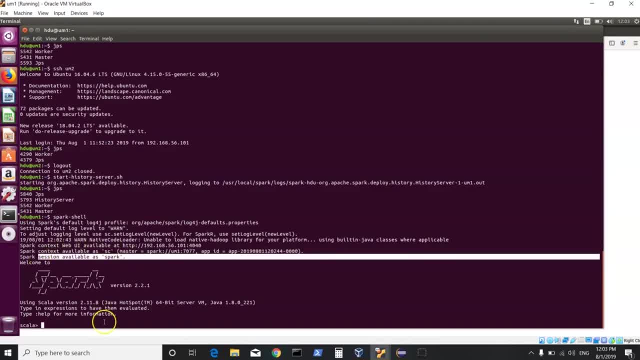 that is, data frames and data sets. you can be using spark. let's try a quick, simple example. so i'll say val x- sc dot text file. and now i would want to point it to the file, so i will say the complete path. remember, i am giving the spark command from my home directory. 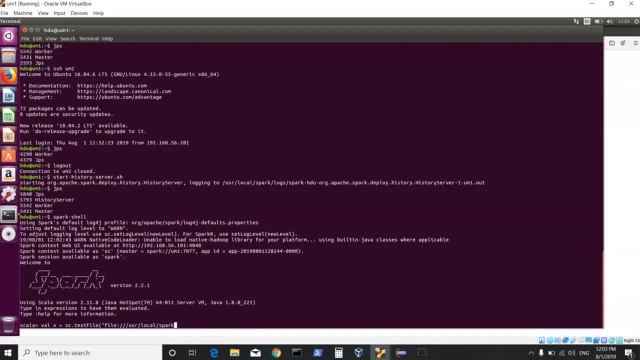 so i will have to say user local spark and then i can point to a file which is existing here and this is what i would want to use to do some processing. we are using the first step here, wherein we are using a method of spark context which will not relate in any evaluation, and it 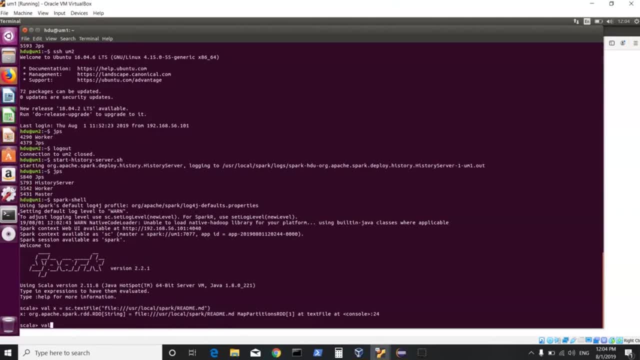 will just create an rdt. now we are using the scalars way, so let's create one more variable and then we can do some transformation on it by saying: to upper case. i would just want to convert the content into upper case, and this is again a. 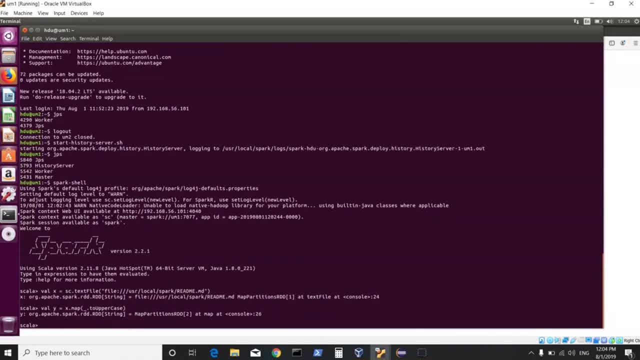 transformation, so that will just create an rdt. once this is done, we can invoke an action to basically see some results. so i could just simply do a collect, which is an action, and this action will trigger the execution of dag, which starts from the farthest rdd. 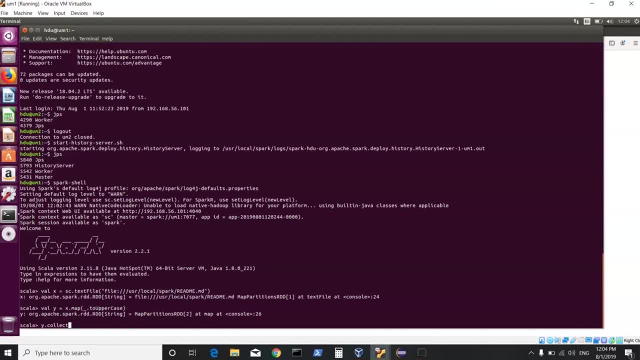 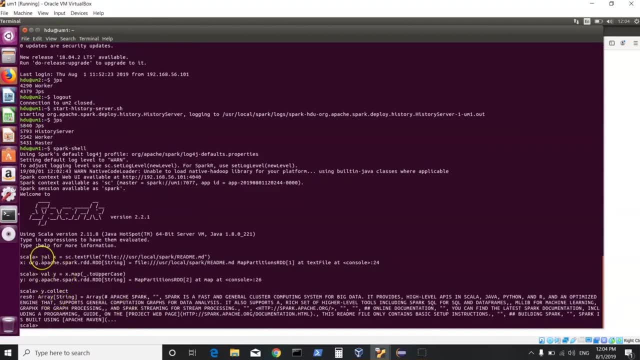 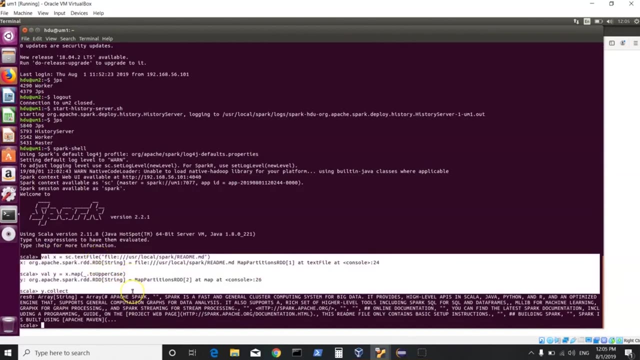 that is the first step, where your file is loaded into rdt. now, once we do this, we should be able to see our result, and that, basically, is execution of dag. so, from the time we have used a text file, which is a method of spark context, to, we did a transformation and till we invoked an action. 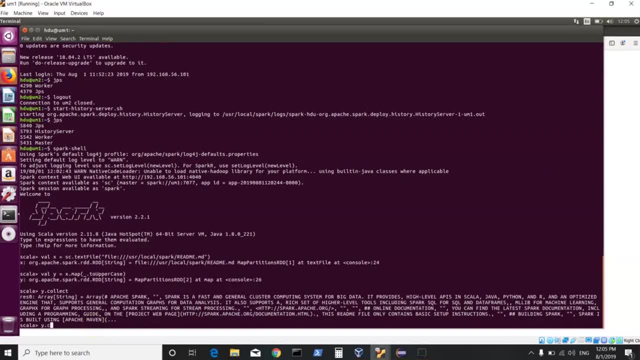 becomes my one job now. if i would do y dot count, which is again a different action, this will trigger the execution of tag right from the beginning, that is sc dot text file, where the data will again be loaded in rdd, a map transformation will happen and then you will have a count. now we can always see this in the spark ui by just going in here. 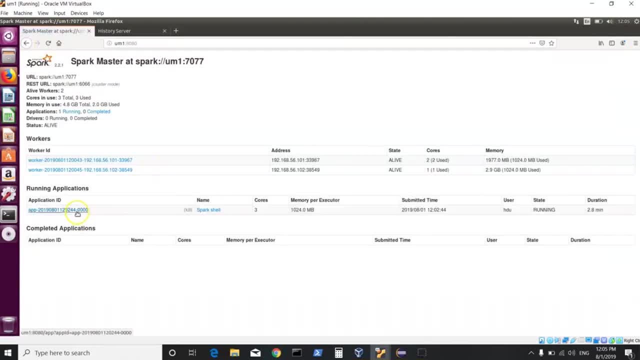 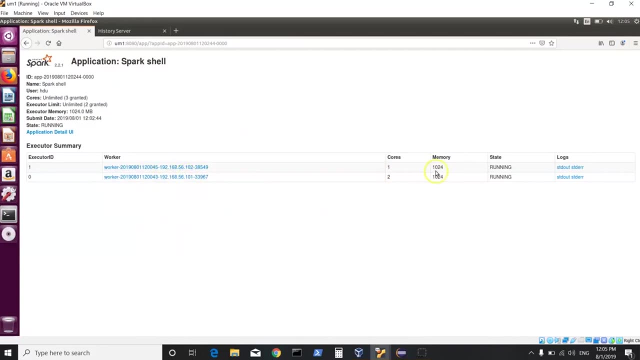 and just doing a refresh. so that will show me that there is an application which is running via spark shell. it has utilized three cores, it has utilized memory per executor- one gigabyte and we can click on this application which shows that it used both the workers- one core and one gb- on this worker and two cores and memory on this worker. i can click. 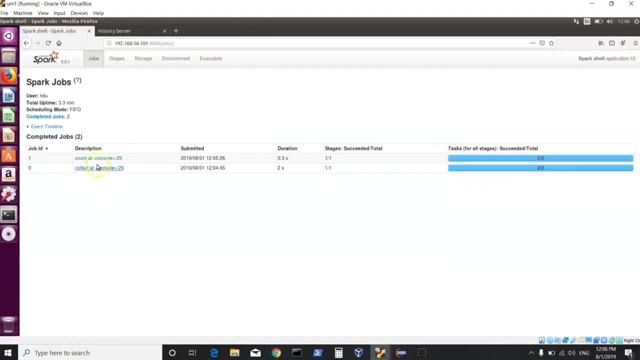 on application detail ui, wherein i can see what are the actions i invoked. we also see the number of tasks which are run, and that is because every rdd which is created by default is having two partitions and for each partition you would have one task. well, we can change the 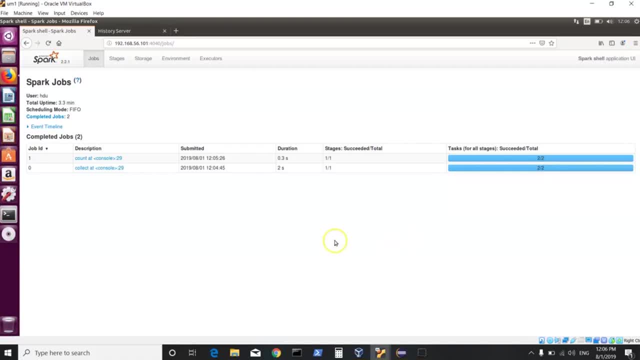 partitions and many more things can be done, but that you can learn in later sessions. here we have two jobs: one ended with collect and one ended with count. now i can click on collect and i can see the tag visualization which tells me we started a text file, we did a map and finally we 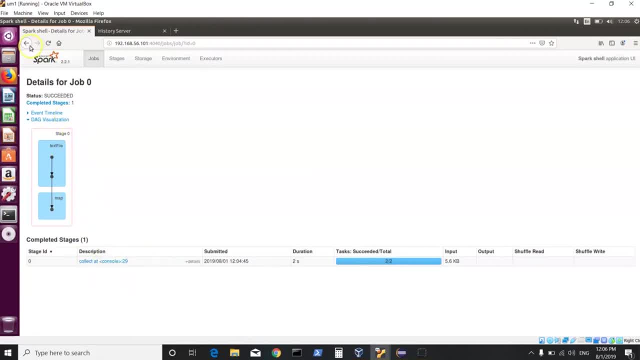 did a collect. it shows that everything was done in state 0. that is just one stage. i can click on count and that again shows me the tag visualization, which is a different stage, a different job id, which started with text file map, and then we did a count. if you would want to see, 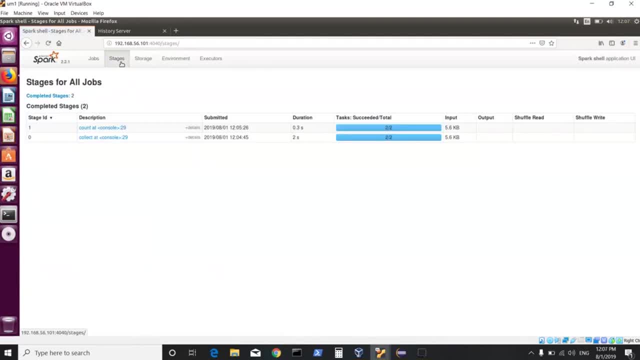 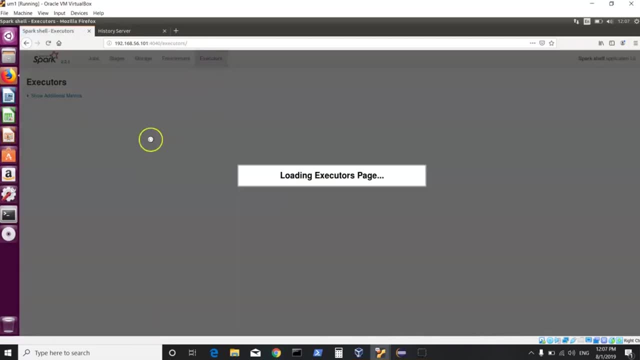 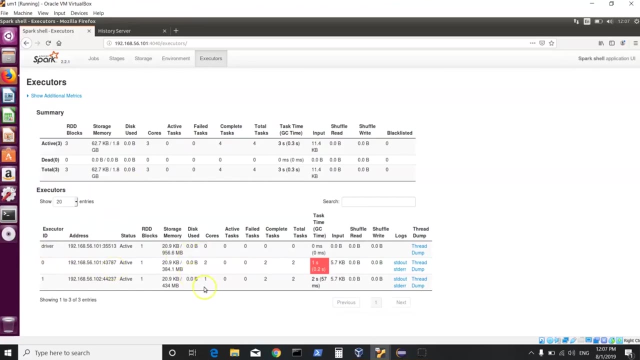 more details. you can always use these tabs to look at different stages within your application. if you were doing some caching, looking at environment variables, and also to see how many executors were used, including the one for the driver, on which nodes these executors ran, how many cores, how many tasks were run, was there any shuffling involved, and so on. so this is how. 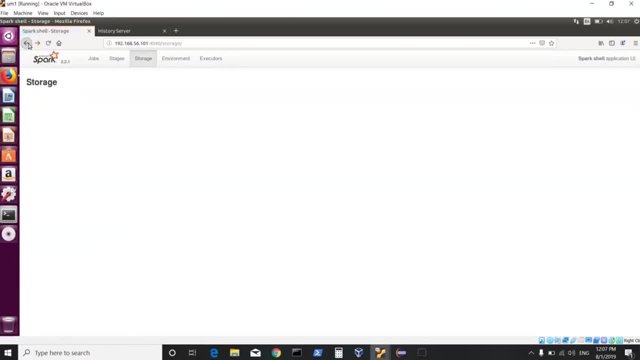 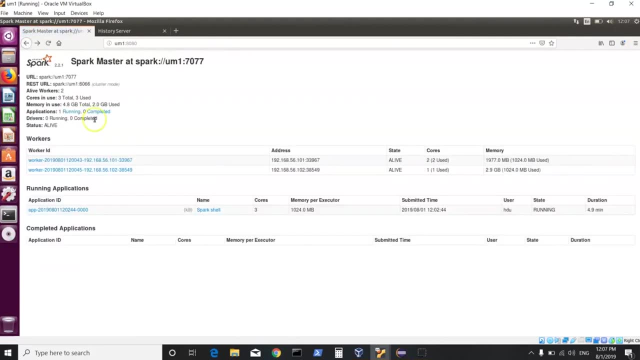 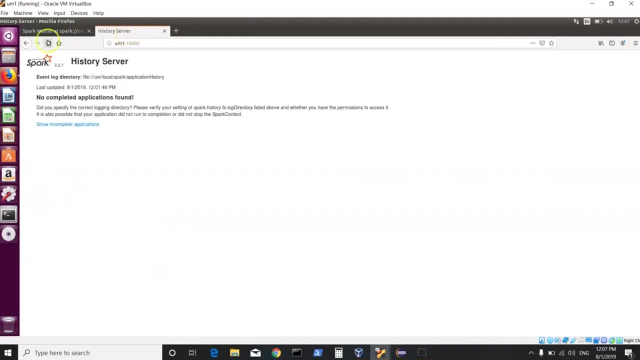 i have used spark shell. that is an interactive way of running my application and, since we have a spark ui, we can always look at applications when they have run and we can always drill down. and no more details. now, since my application is completed, i can do a refresh on history server. 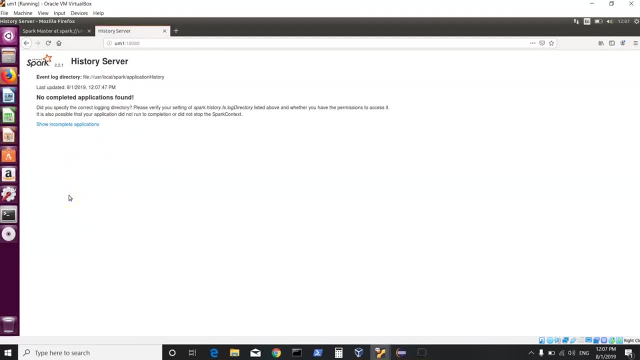 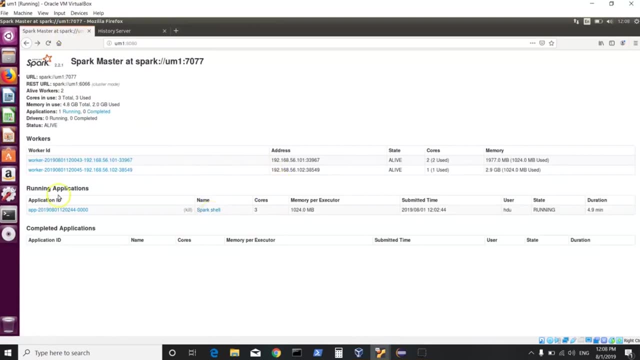 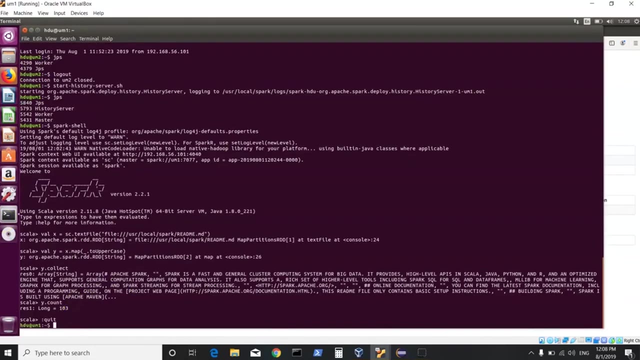 but that does not show anything, because when we started a spark shell, it started an application and that application is still in running status, if you see here under running applications. so this is how we use spark shell on a standalone spark cluster. now we can just do a colon quit and that takes me out of spark shell. similarly, if i would want to, 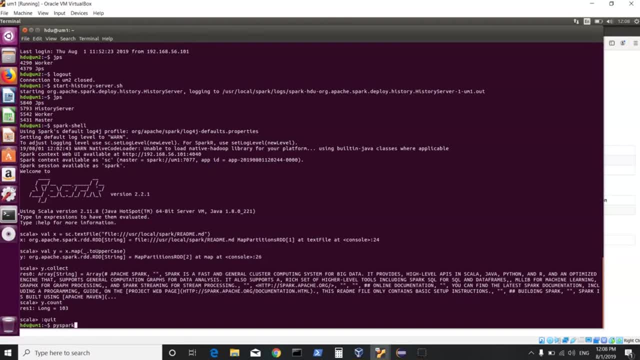 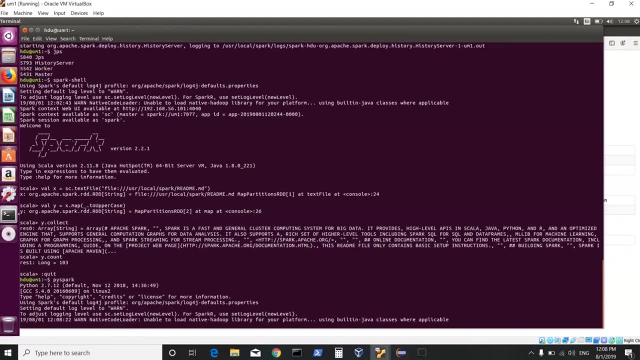 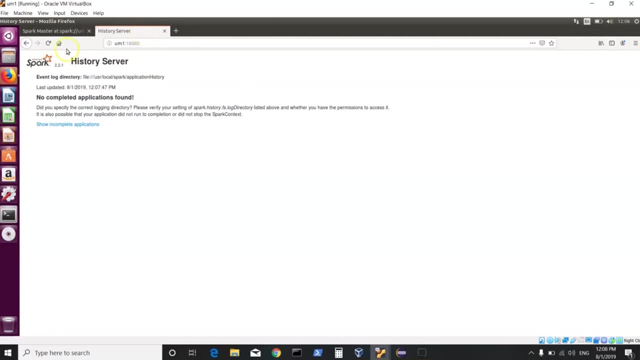 work on pi spark. that is python's way of working with spark. i can just type in pi spark, which should bring my python shell, and then i can continue working with spark and again go back and look at my ui while my pi spark comes up. i can go here, since i quit my spark shell, i can. 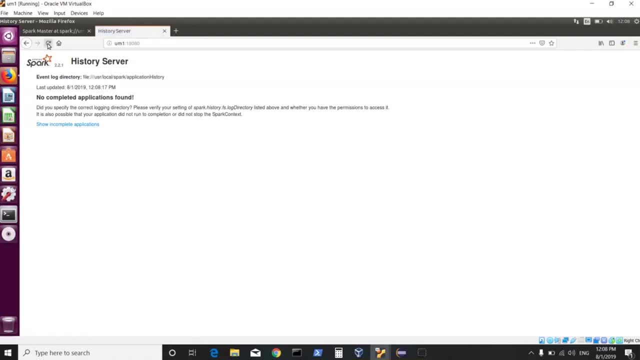 just do a refresh to see if my application is yet coming up in history server. it might take some time and you can always go back and look at incomplete applications or wait till your application is populated in history server. now, if i do a refresh here on spark ui. 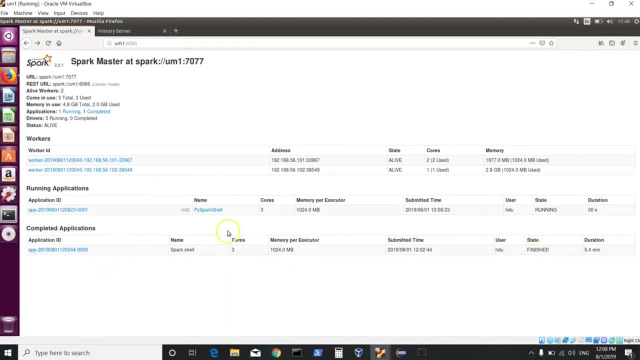 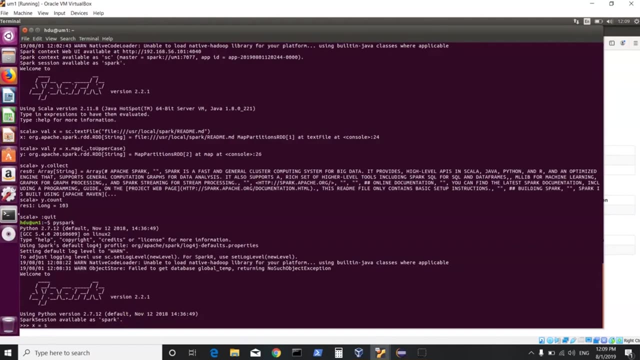 it says this application was completed. it says finished. and then now we have started pi spark. so it has started a new application, pi spark shell, and that is in running status. we can come back here, and now we have our python's way so i can do the same thing which i did in scala using sc dot. 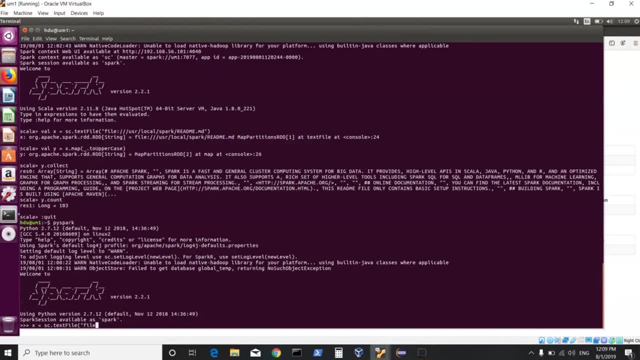 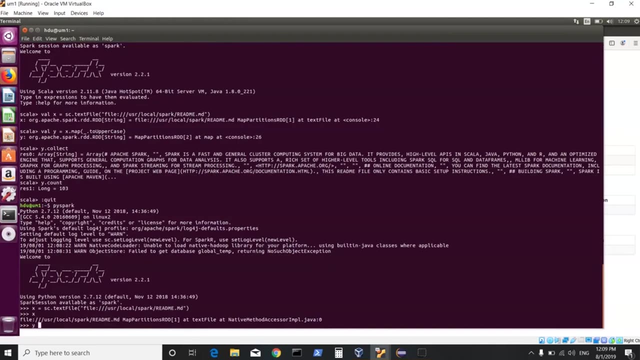 text file. i will point it to a file which exists in user local spark. read me dot md. so that's the file which i'm interested in now. this would have created an rdt which we can confirm by just typing in x. now i can create a different variable and i can say i would want to do a transformation. 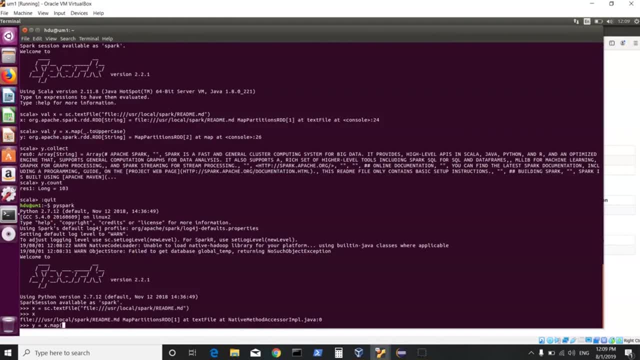 of map. now, in case of python, when you use anonymous functions or when you want to apply some functions to your transformations, you use lambda functions. so we can say we say lambda line and then i would say what i want to do to the line. i will say i will use a. 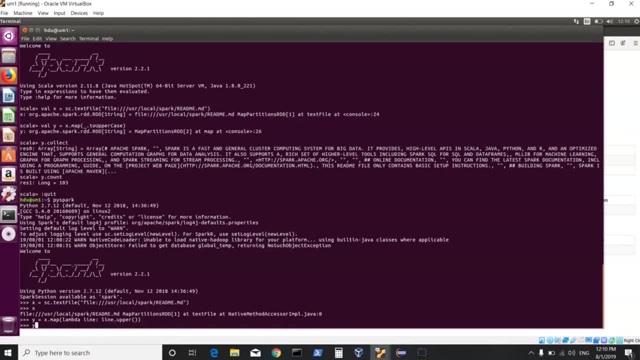 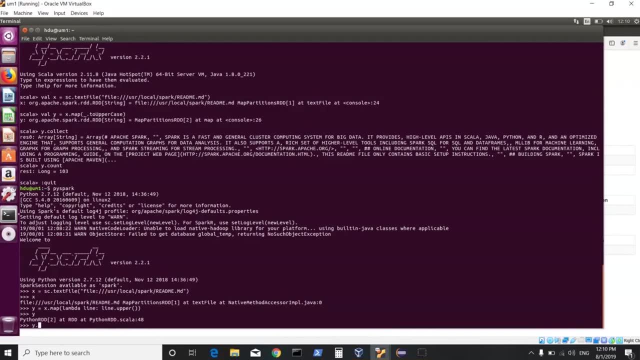 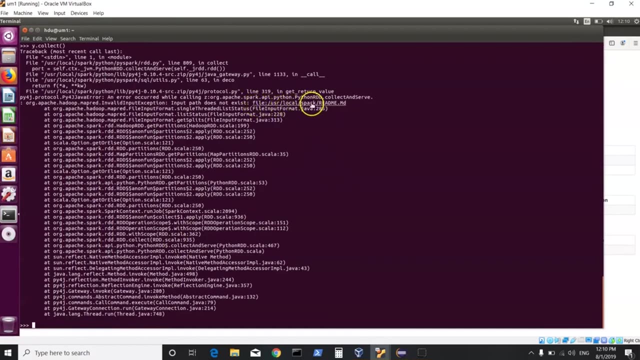 inbuilt uppercase upper function which should convert my content into uppercase, but as of now this is a transformation, so it only creates an rdt to see the result. i can do a y dot collect and that should bring up my result. now in case, if it says the file does not exist, that is because 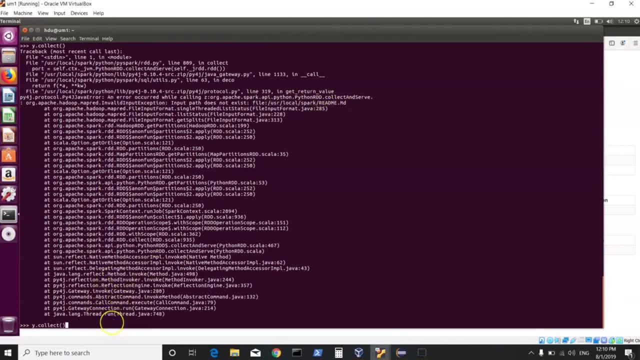 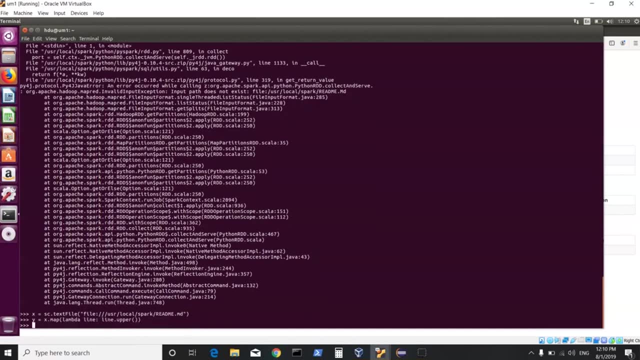 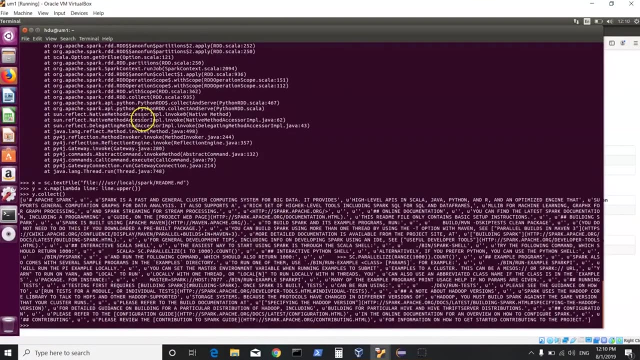 there was a typo here and we can repeat this step. so let's say we want to do the same thing here. so let's bring up here again x and i can give the right name of the file, i can do a transformation and finally i can see the result. so this is using pi spark on a standalone spark cluster. 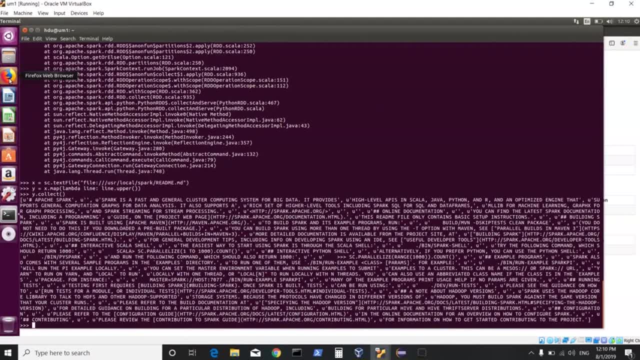 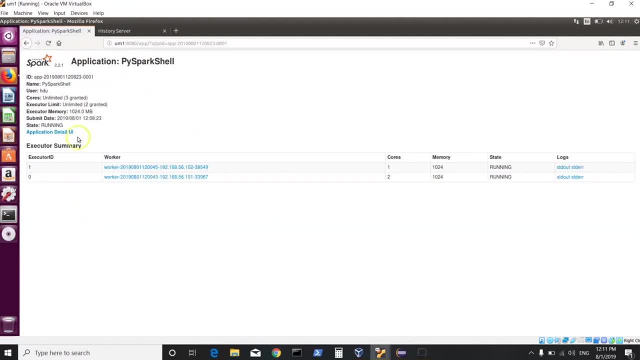 which is working without hadoop, which has two worker nodes and one master node. we can always come and do a refresh here to look at more details. so we have our application. we can click on this again similarly, like we did for scala application in ui. i see my application ended at collect. it ran two tasks and i can look at my tag. so this is how. 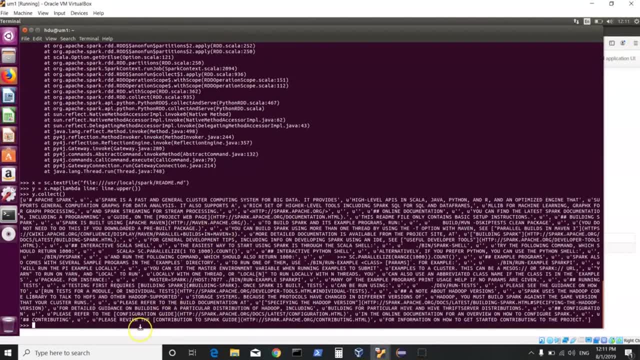 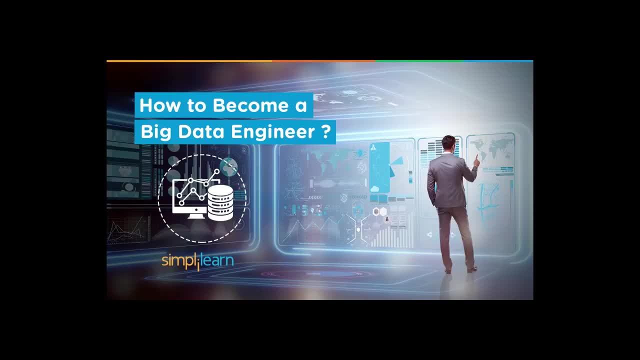 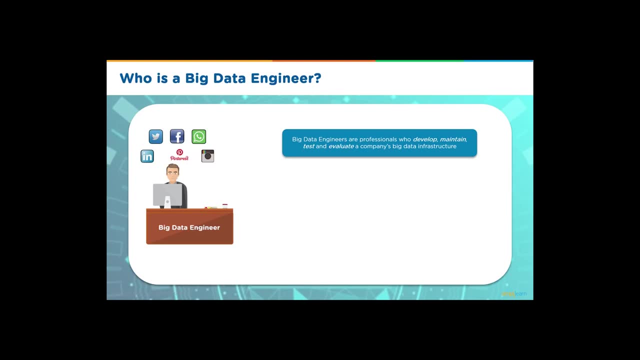 we can use spark shell or pi spark. thank you, ajay. now we have rahul, who will tell us how to become a big data engineer. now let's find out who is a big data engineer. a big data engineer is a professional who develops, maintains, tests and evaluates the company's big data infrastructure. 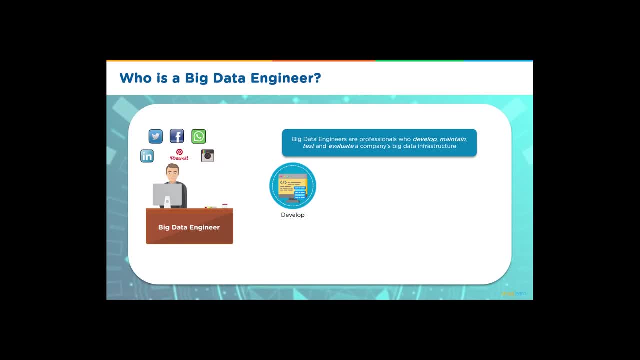 in other words, develop big data solutions based on a company's requirements. they maintain these solutions, they test out these solutions as to the company's requirements, they integrate this solution with the various tools and systems of the organization and, finally, they evaluate how well the solution is working to fulfill the 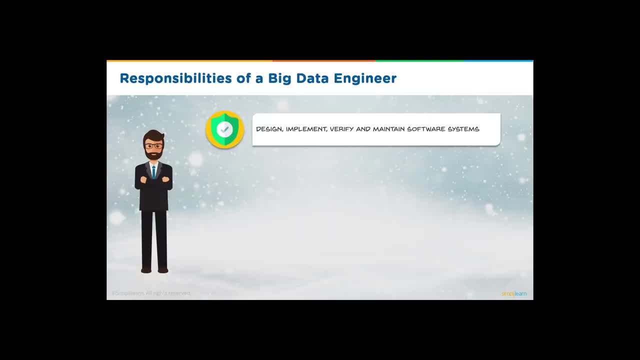 company's requirements. next up, let's have a look at the responsibilities of a big data engineer now. they need to be able to design, implement, verify and maintain software systems now for the process of ingesting data as well as processing it. they need to be able to build highly scalable. 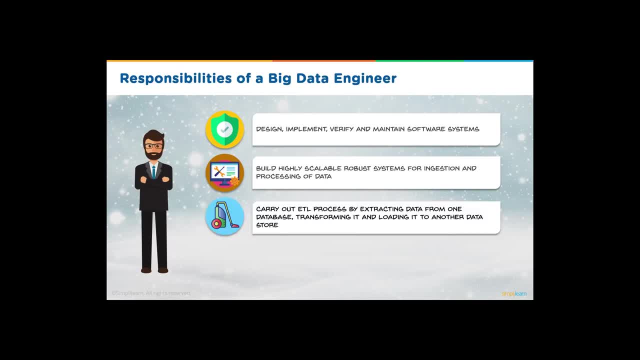 as well as robust systems. they need to be able to extract data from one database, transform it, as well as load it into another data store with the process of etl or the extract transform load process, and they need to research as well as propose new ways to acquire data, improve the 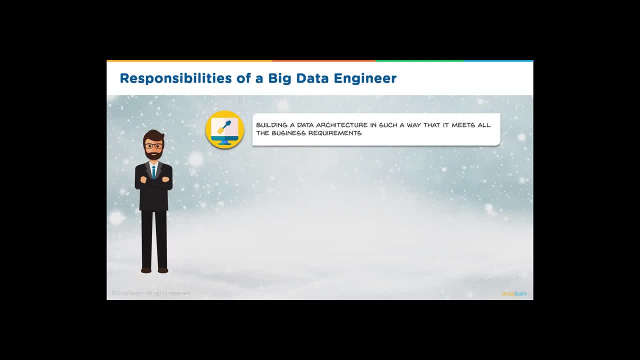 overall data quality and the efficiency of the system. now, to ensure that all the business requirements are met, they need to build a suitable data architecture. they need to be able to integrate several programming languages and tools together so that they can generate a structured solution. they need to build models that reduce the overall complexity. 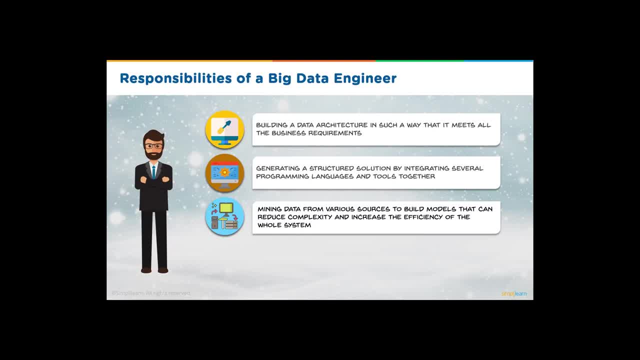 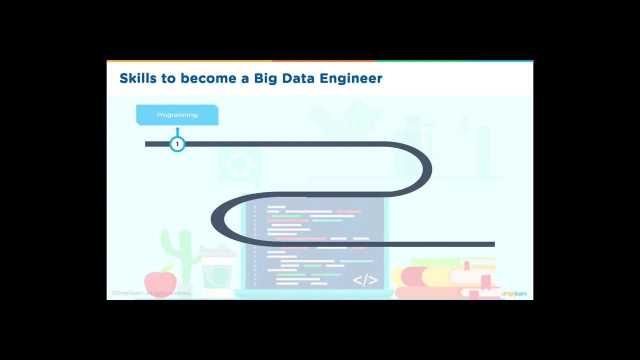 and increase the efficiency of the whole system by mining data from various sources. and, finally, they need to work well with other teams, ones that include data architects, data analysts and data scientists. next up, let's have a look at the skills required to become a big data engineer. the first step is to have programming knowledge, one of the most important skills. 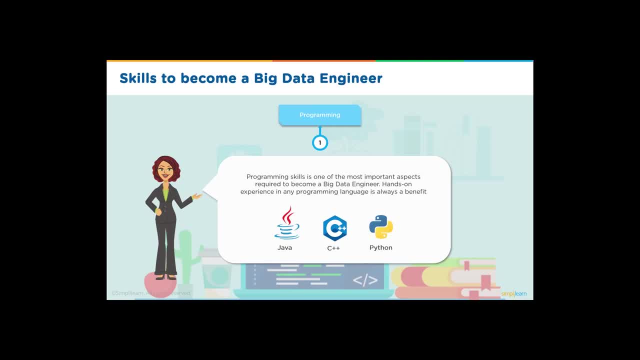 required to become a big data engineer is that of experience with programming languages, especially hands-on experience. now, the big data solutions that organizations would want you to create will not be possible without experience in programming languages. i can even tell you an easy way through which you can get experience with programming languages: practice, practice and more practice. 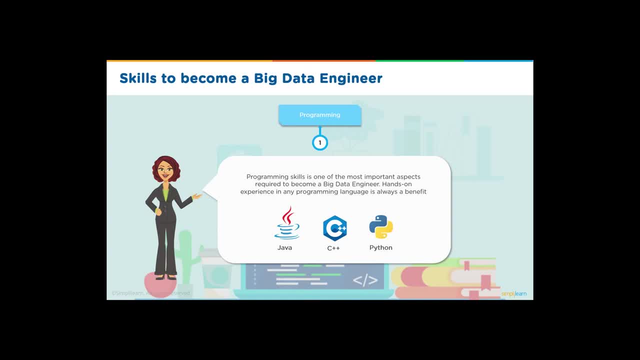 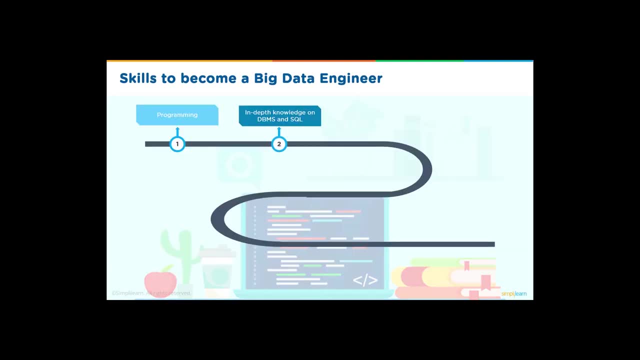 some of the most commonly used programming languages used for big data engineering are python, java and c plus plus. the second skill that you require is to have in-depth knowledge about dbms and sql. you need to know how data is maintained as well as managed in a database. you 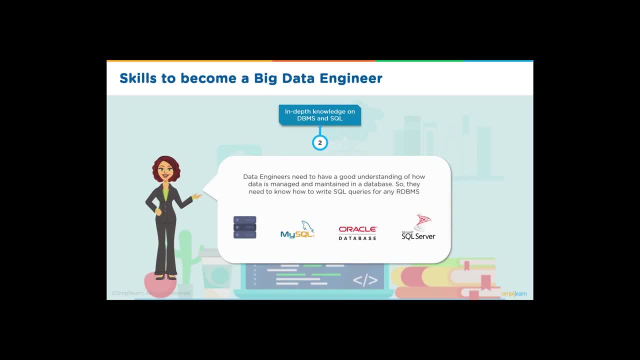 know how sql can be used to transform as well as perform actions on a database and, by extension, know how to write sql queries for any relational database management systems. some of the commonly used database management systems for big data engineering: mysql, racl database and the microsoft sql server. the third skill that you require is to have experience working with etl and warehousing. 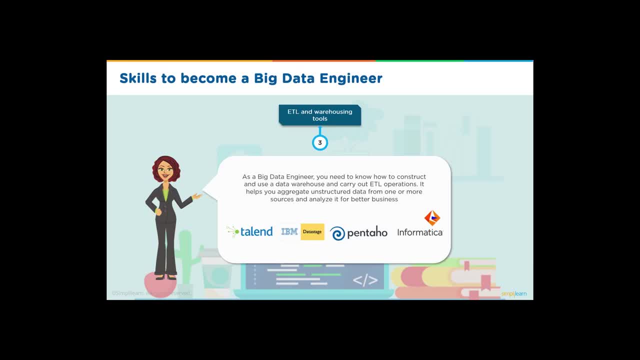 tools. now you need to know how to construct, as well as use, a data warehouse so that you can extract, transform and load operations. now, as a big data engineer, you'll be constantly tasked with extracting unstructured data from a number of different sources, transforming it into meaningful 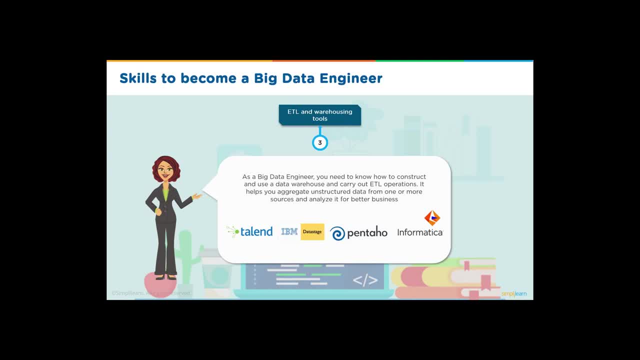 information and loading it into other data storages, databases or data warehouses. now, what this is is basically aggregating unstructured data from multiple sources, analyzing it so that you can take better business decisions. some of the tools used for this purpose are talent, ibm, data stage. 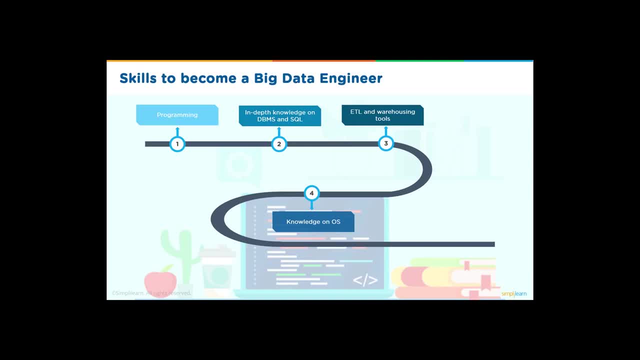 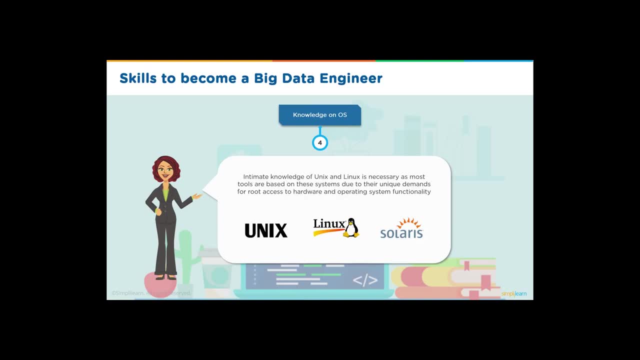 pentejo and informatica. next up we have the fourth skill that you require, which is knowledge about operating systems. now, since most big data tools have unique demands, such as root access to operating system functionality, as well as hardware, having a strong understanding of operating systems like linux and unix is absolutely mandatory. some of 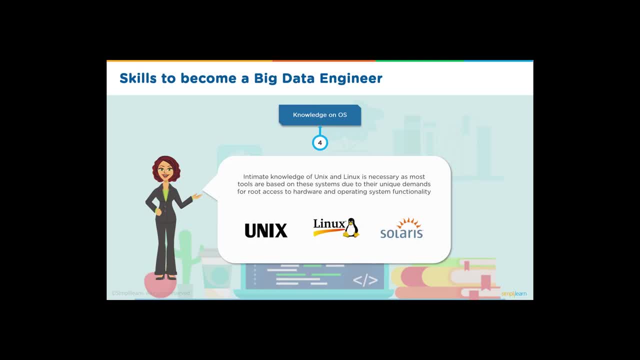 the operating systems used by big data engineers are unix, linux and solaris. now, the fifth skill that you require: to have experience with hadoop based analytics. since hadoop is one of the most commonly used tools when it comes to big data engineering, it's understood that you need to have experience with apache, hadoop based technologies, technologies. 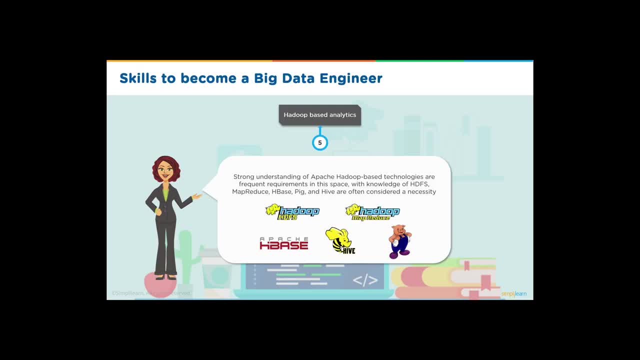 like hdfs, hadoop, map, produce, apache, edgebase, hive and pig. the sixth skill that you require is to have worked with real-time processing frameworks like apache, spark. now, as a big data engineer, you'll have to deal with vast volumes of data, so for this data, you need an analytics engine like spark, which 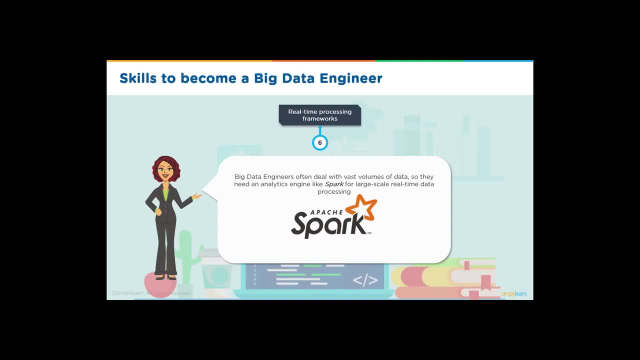 can be used for large-scale real-time data processing. now, spark can process live streaming data from a number of different sources like facebook, instagram, twitter and so on. it can also perform interactive analysis and data integration. and now we're at our final skill requirement, which is to have experience with 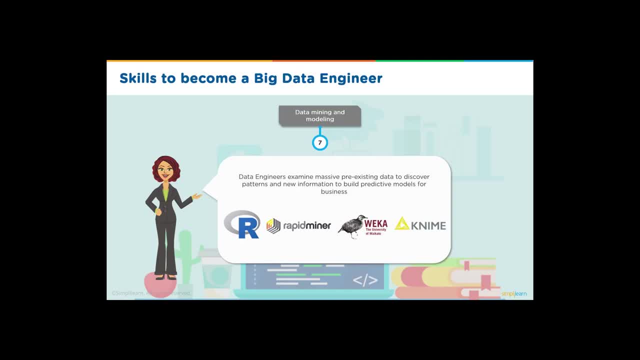 data mining and modeling. so, as a data engineer, you'll have to examine massive pre-existing data so that you can discover patterns as well as new information. with this, you'll create predictive models for your business so that you can make better informed decisions. some of the tools used: 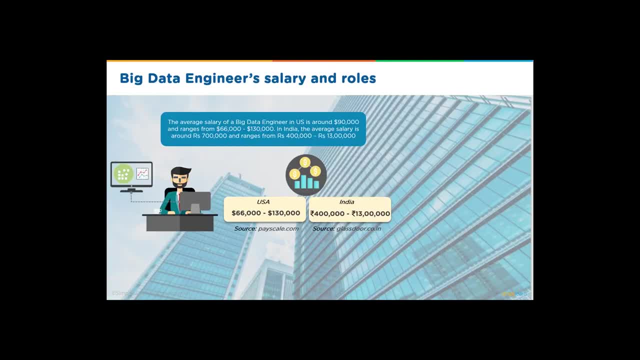 for this are our rapid miner, veca and name. now let's talk about the next skill that you need to know, about the next skill that you need to know, about the next skill that you need to know, about a big data engineer's salary, as well as other roles they can look forward to. now, the average salary of 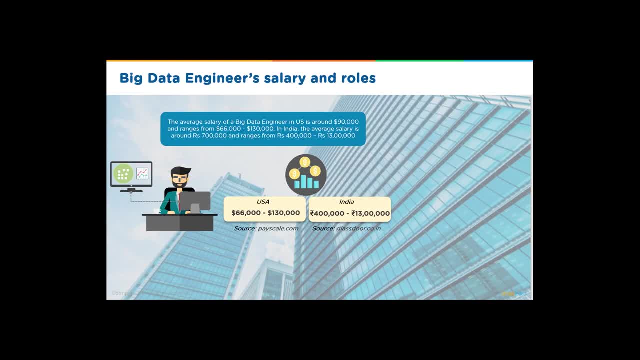 a big data engineer in the united states is approximately ninety thousand dollars per year. now this ranges from sixty six thousand dollars all the way to hundred and thirty thousand dollars per annum. in india, the average salary is around seven lakh rupees and ranges from four lakhs to 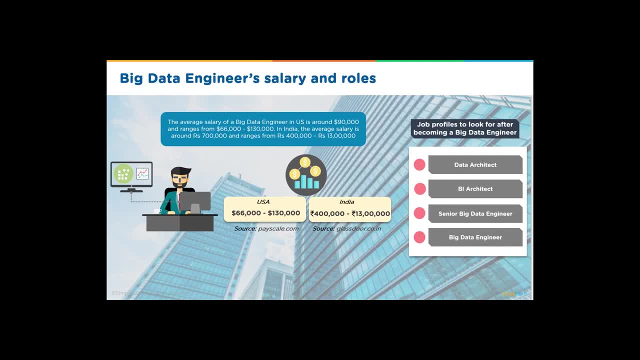 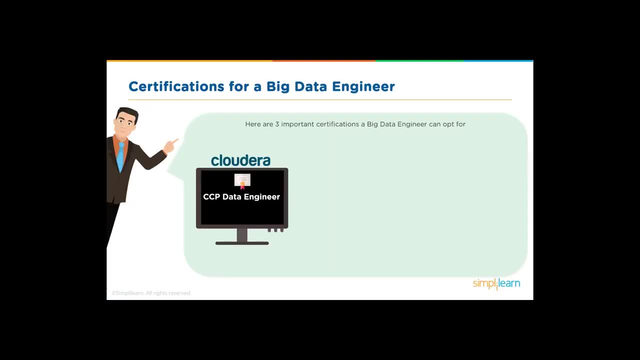 thirteen lakhs per annum. after you've become a big data engineer, some of the job roles that you can look forward to are that of a senior big data engineer, a business intelligence architect and a architect. now let's talk about certifications that a big data engineer can opt for. first off, 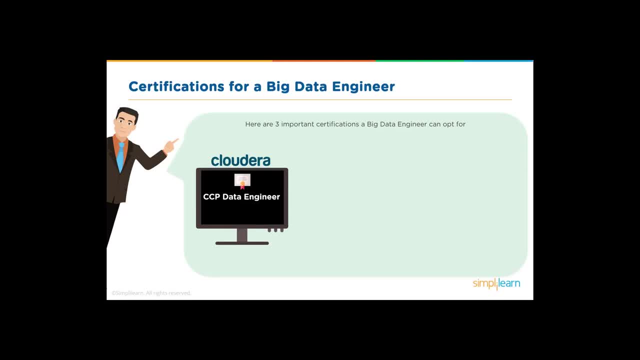 we have the cloudera ccp data engineer. a cloudera certified professional data engineer possesses the skills to develop reliable and scalable data pipelines that result in optimized data sets for a variety of workloads. it is one of the industry's most demanding performance-based certification. ccp evaluates and recognizes a candidate's mastery of the technical skills. 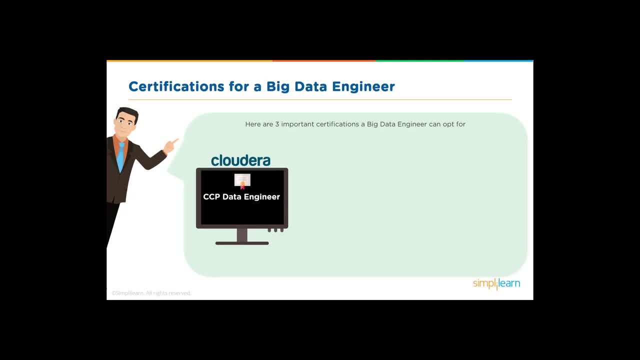 most sought after by employers. the time limit for this exam is 40 minutes and it costs 400. next we have the ibm certified data architect big data certification. an ibm certified big data architect understands the complexity of data and can design systems and models to handle different data variety, including structured, semi-structured, unstructured volume. 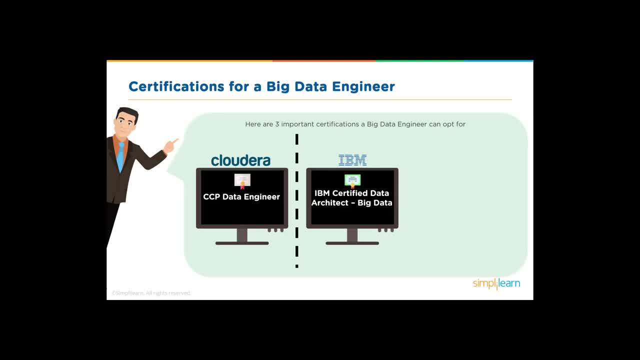 velocity, veracity and so on. a big data architect is also able to effectively address information governance and security challenges associated with the system. this exam is 75 minutes long. we have the google cloud certified data engineer. a google certified data engineer enables data-driven decision making by collecting, transforming and publishing data. they should also 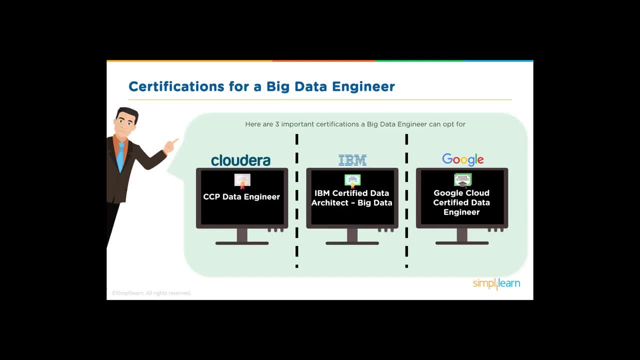 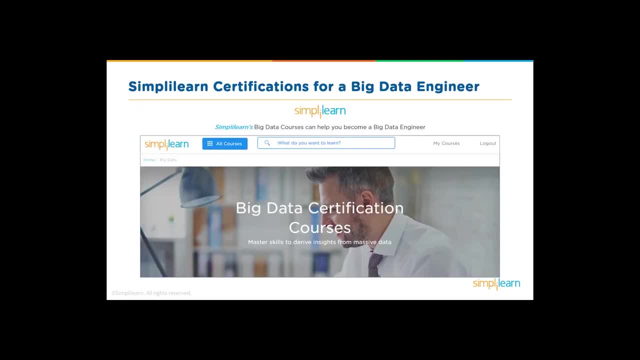 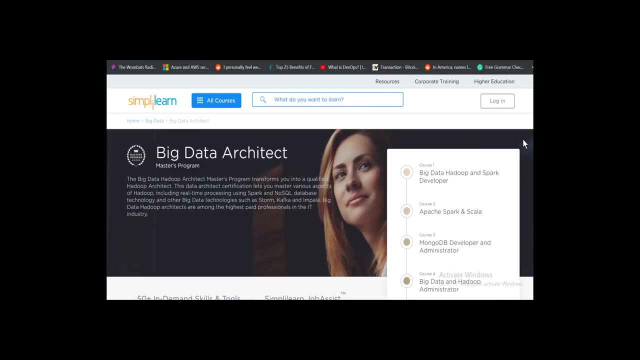 be able to leverage, deploy and continuously train pre-existing machine learning models. the length of the certification exam is two hours and its registration fee is two hundred dollars. now let's have a look at how simply learn can help you become a big data engineer. simply learn provides the big data architect master's program. this includes a number of different courses like 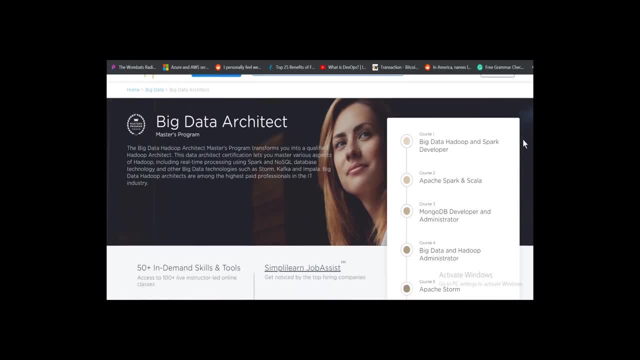 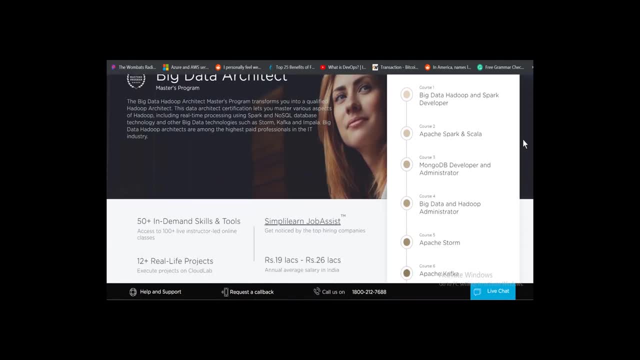 data, hadoop and spark developer, apache, spark in scala, mongodb developer and administrator, big data and hadoop administrator, and so much more. this course goes through 50 plus in-demand skills and tools, 12 plus real life projects and the possibility of an annual average salary of 19. to 26 lakh rupees per annum. it will also help you get noticed by the top hiring companies. this course will also go through some major tools like kafka, apache, spark flume, edgebase, mongodb, big map, produce, java, scala and much more. now why don't you head over to simplylearncom? 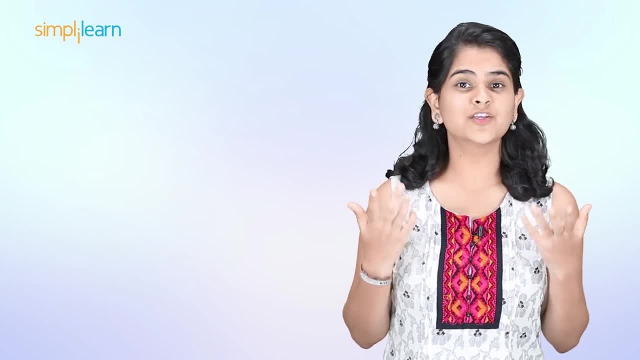 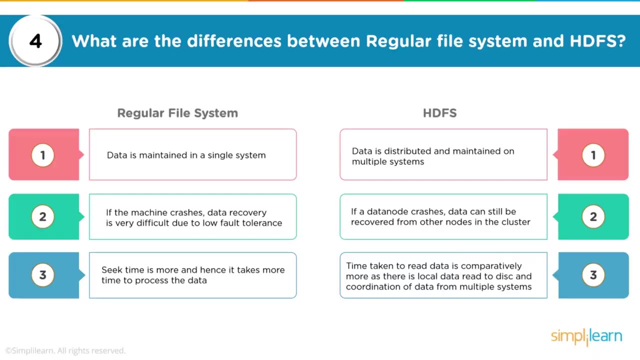 and get started on your journey to get certified and get. thank you, rahul. now we will have a look at the hadoop interview questions and answers. our instructor ajay will guide us through it. one single machine with huge amount of disks and huge amount of ram, but then the time taken to read. 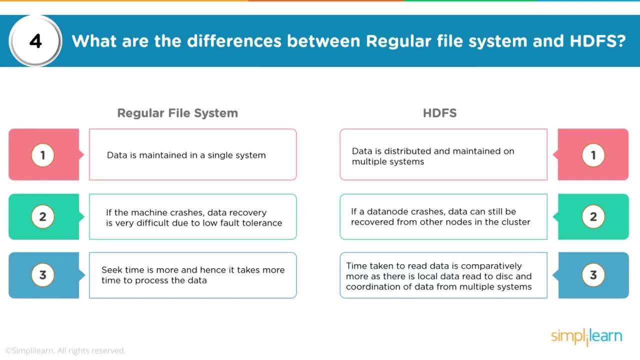 that data, when all the data is stored in one machine, would be very high and that would be with least fault tolerance. if you talk about sdfs, your data is distributed, so sdfs stands for hadoop- distributed file system. so here your data is distributed and maintained on multiple systems. 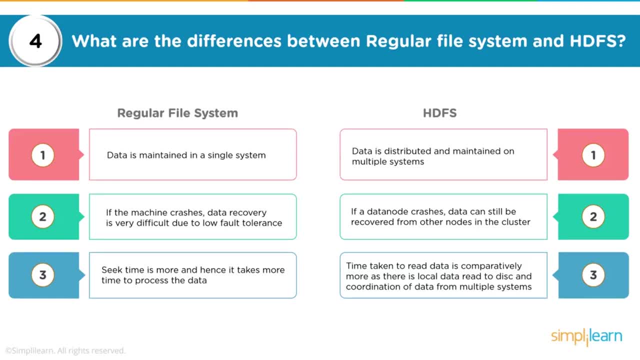 so it is never one single machine. it is also supporting reliability. so whatever is stored in sdfs, say, a file being stored depending on its size is split into blocks, and those blocks will be spread out to multiple nodes. not only that, every block which is stored on a node will have its replicas. 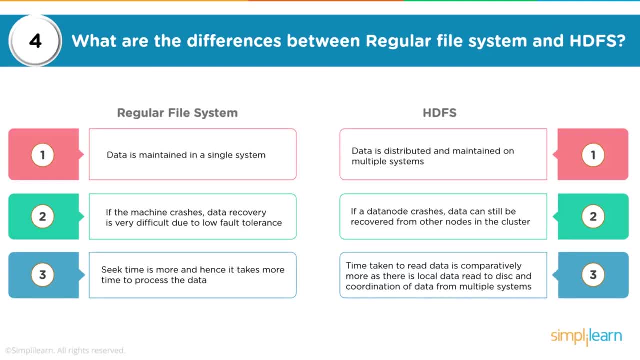 stored on other nodes. replication factor depends, but this makes sdfs more reliable in cases of your slave nodes or data nodes crashing. you will rarely have data loss because of auto replication feature. now, time taken to read the data is comparatively more, as you might have situations where your data is 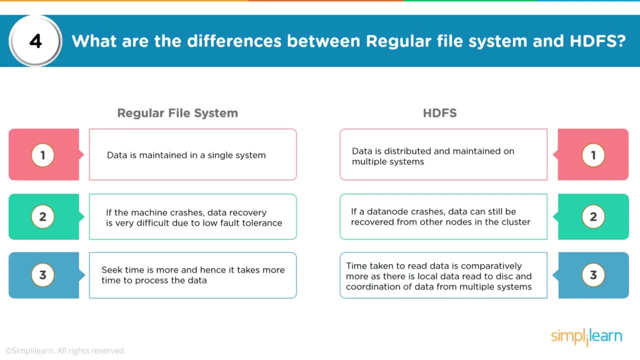 distributed across the nodes and even if you are doing a parallel read, your data read might take more time because it needs coordination from multiple machines. however, if you are working with huge data which is getting stored, it will still be beneficial in comparison to reading from a single machine, so you should always think about its reliability through auto replication feature. 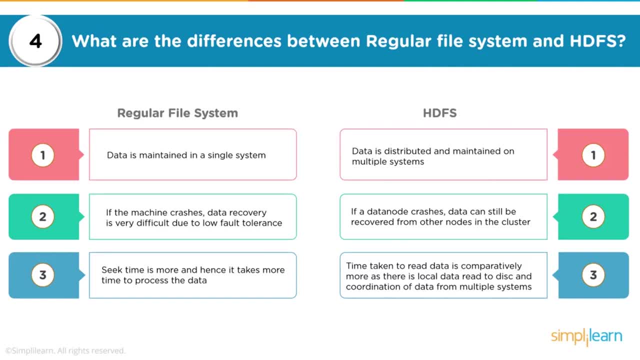 its fault tolerance- because of your data getting stored across multiple machines- and its capability to scale. so when you talk about sdfs, we are talking about horizontal scalability, or scaling out. when you talk about regular file system, you are talking about vertical scalability, which is scaling up. now let's look at some specific sdfs questions. what is this? why is? 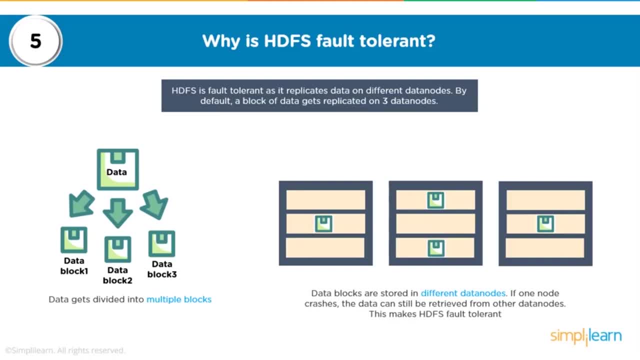 sdfs fault tolerant. now, as i just explained in previous slides, your sdfs is fault tolerant as it replicates data on different data nodes. so you have a master node and you have multiple slave nodes or data nodes where actually the data is getting stored. now we also have a default block size of 128 mb. that's the minimum since hadoop version 2.. so 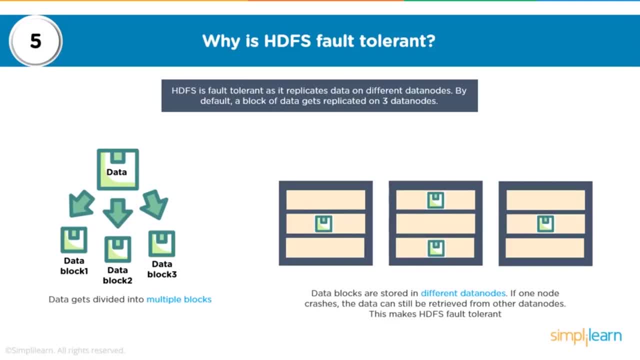 any file which is up to 128 mb would be using one logical block, and if the file size is bigger than 128 mb, then it will be split into blocks and those blocks will be stored across multiple machines. now, if these blocks are stored across multiple machines, it makes it more fault tolerant, because 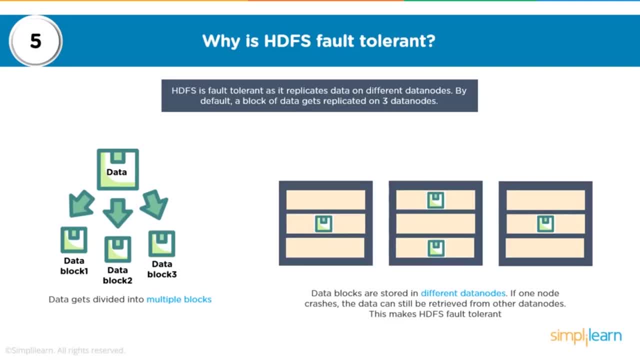 even if your machines fail, you would still have a copy of your block existing on some other machine. now there are two aspects here. one: we talk about the first rule of replication, which basically means you will never have two identical blocks sitting on the same machine, and the second rule. 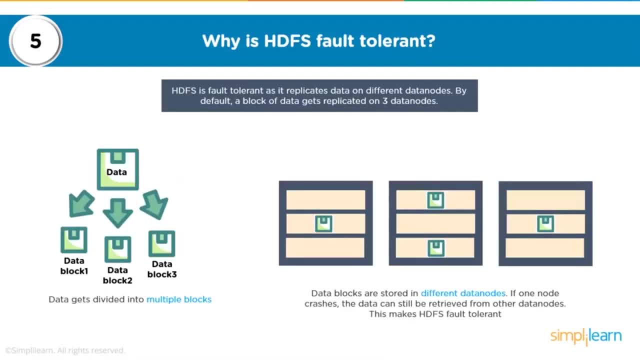 of replication is in terms of rack awareness. so if your machines are placed on the same machine in racks, as we see in the right image, you will never have all the replicas placed on the same rack, even if they are on different machines. so it has to be fault tolerant and it has to 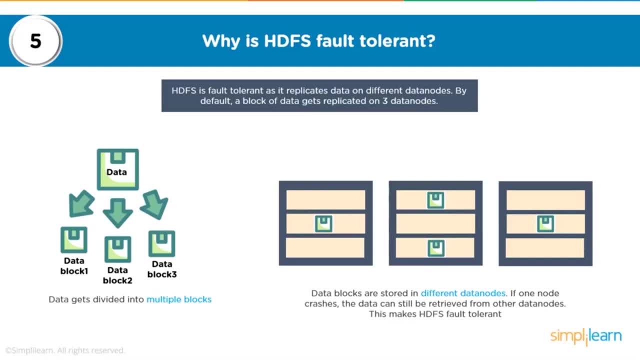 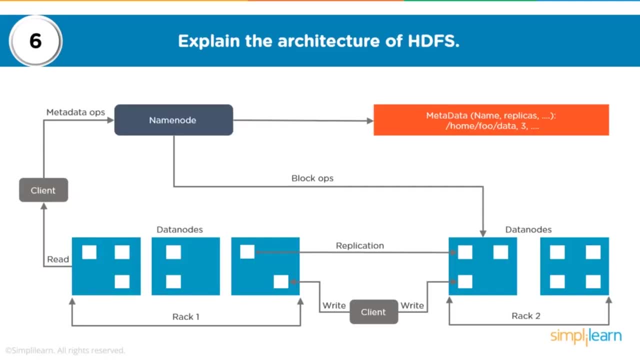 maintain redundancy. so at least one replica will be placed on some other node, on some other rack. that's how sdfs is fault tolerant. now here let's understand the architecture of sdfs. now, as i mentioned earlier, you would in a hadoop cluster. the main service is your hdfs. so for your sdfs service you would have a name node which is your. 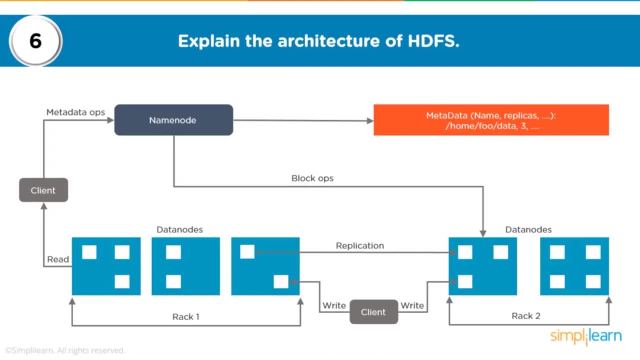 master process running on one of the machines and you would have data nodes, which are your slave machines getting stored across or getting, or the processes running across multiple machines. each one of these processes has an important role to play when you talk about sdfs, whatever data is. 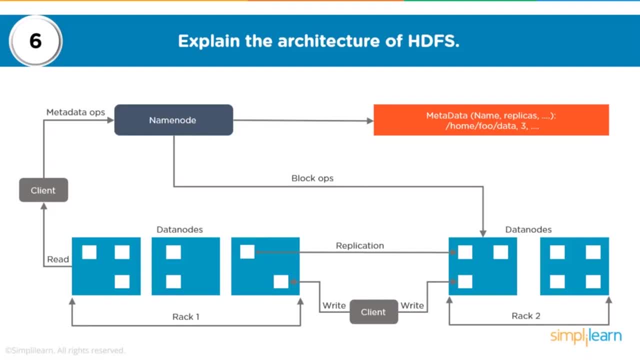 written to hdfs, that data is stored on the same machine and that data is stored on the same machine. so you can see here that the data nodes are split into blocks depending on its size, and the blocks are randomly distributed across nodes with auto replication feature. these blocks are also 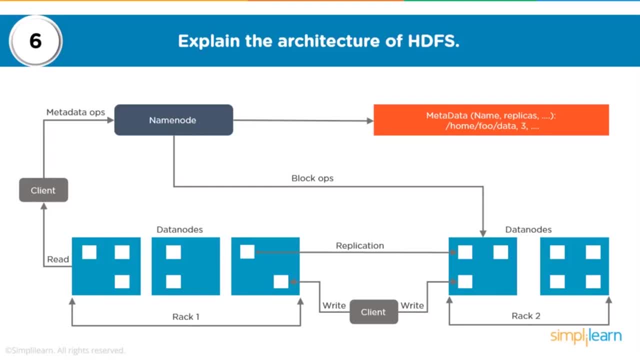 auto replicated across multiple machines, with the first condition that no two identical blocks will sit on the same machine. now, as soon as the cluster comes up, your data nodes, which are part of the cluster and based on config files, would start sending their heartbeat to the name node and this 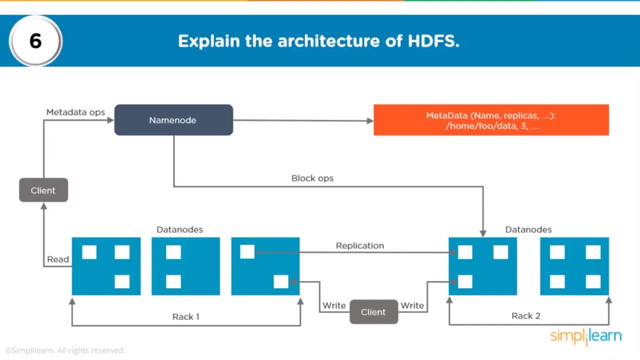 data node will send a block report every three seconds. what does name node do with that? name node will store this information in its ram. so name node starts building a metadata in its ram and that metadata has information of what are the data nodes which are available in the beginning. 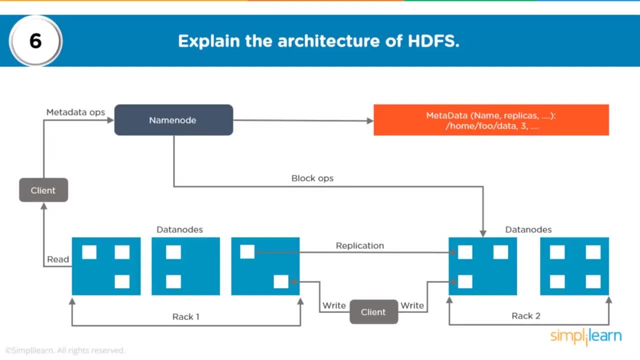 now, when a data writing activity starts and the blocks are distributed across data nodes, data nodes every 10 seconds will also send a block report to name node. so name node is again adding up this information in its ram or the metadata in ram, which earlier had only data. 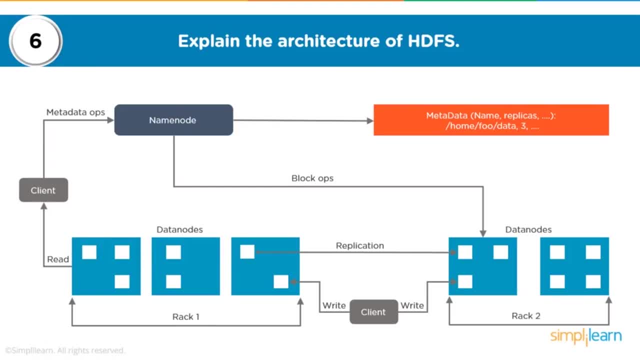 node information. now. name node will also have information about what are the files, the files are split in which blocks, the blocks are stored on which machines and what are the file permissions. now, while name node is maintaining this metadata in ram, name node is also maintaining metadata in 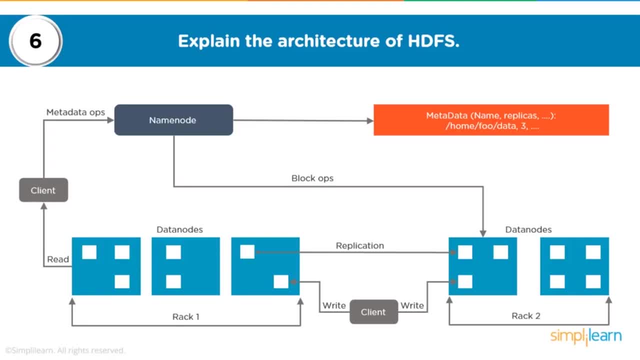 disk- now that is what we see in the red box, which basically has information of whatever information was written to hdfs. so, to summarize: your name node has metadata in ram and metadata in disk. your data nodes are the machines where your blocks or data is actually getting stored. and then there is a auto replication feature which is always existing unless and until. 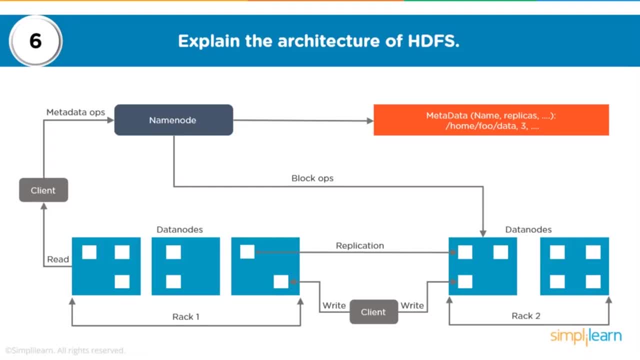 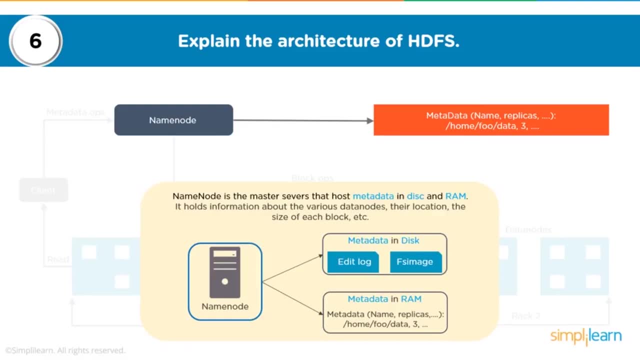 you have disabled it and your read and write activity is a parallel activity. however, replication is a sequential activity. now, this is what i mentioned about when you talk about name node, which is the master process hosting metadata in disk and ram. so when we talk about disk, it basically has a edit log, which is 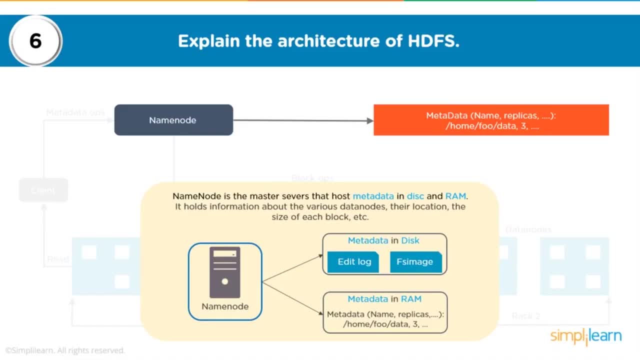 your transaction log and your fs image, which is your file system image. right from the time the cluster was started, this metadata in disk was existing and this gets appended every time read, write or any other operations happen on sdfs. metadata in ram is dynamically built every time the cluster comes up. 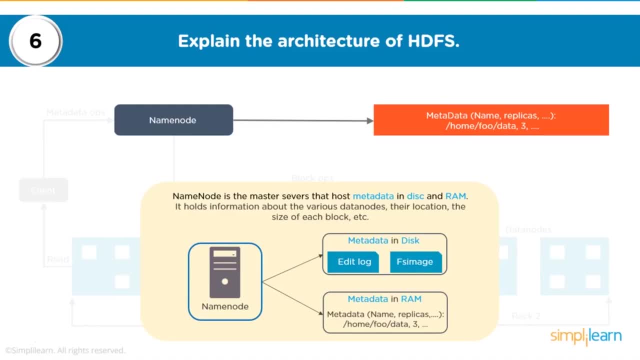 which basically means that if your cluster is coming up, name node in the initial few seconds or few minutes would be in a safe mode, which basically means it is busy registering the information from data nodes. so name node is one of the most critical processes. if name node is down, 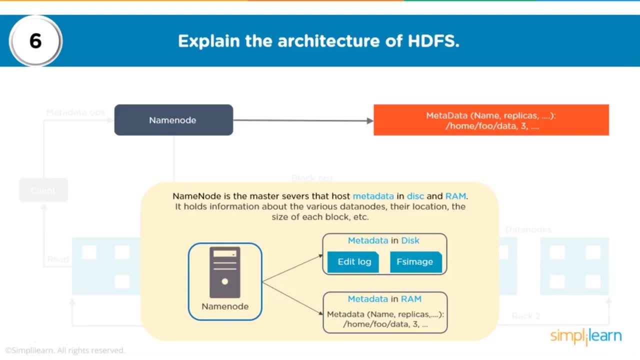 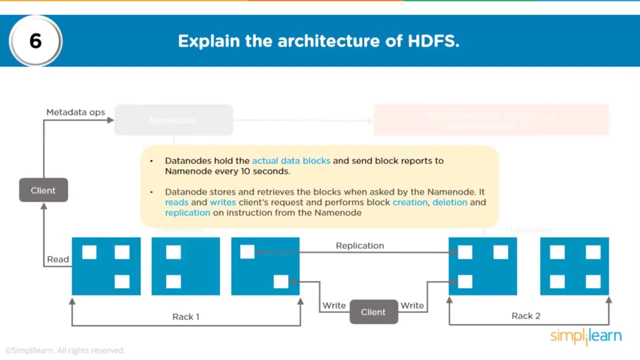 and if all other processes are running, you will not be able to access the cluster name nodes. metadata in disk is very important for name node to come up and maintain the cluster name nodes. metadata in ram is basically for all or satisfying all your client requests. now when we look at data nodes, as i mentioned, data nodes hold the actual data blocks. 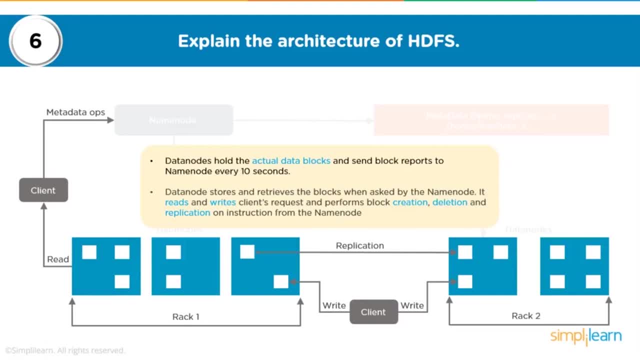 and they are sending these block reports every 10 seconds. so the metadata in name nodes, ram, is constantly getting updated and metadata in disk is also constantly getting updated based on any kind of write activity happening on the cluster. now data node which is storing the block will also help in any kind of read activity whenever a client requests. so whenever a client 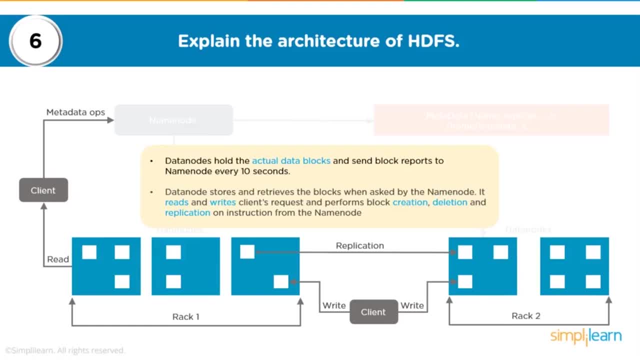 or an application or an api would want to read the data, it would first drop to name node. name node would look into its metadata on ram and confirm to the client which machines could be reached to get to that data. that's where your client would try to read the data from sdf. 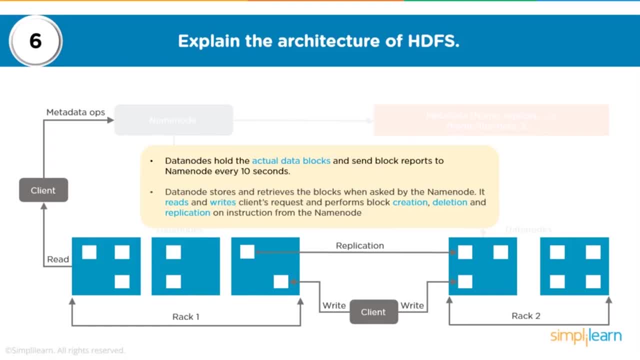 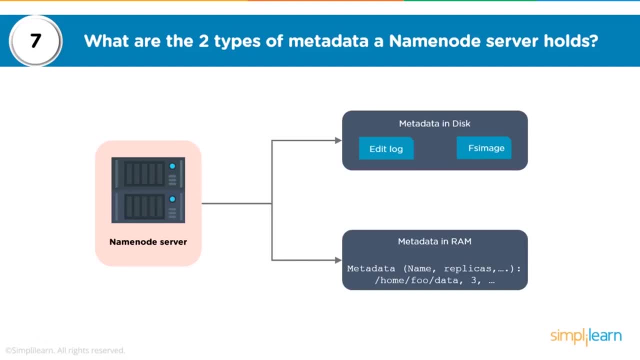 s, which is actually getting the data from data nodes, and that's how your read write requests are satisfied. now what are the two types of metadata in name node? server holds, as i mentioned earlier, metadata in disk- very important to remember- edit, log, nfs, image. metadata in ram, which is 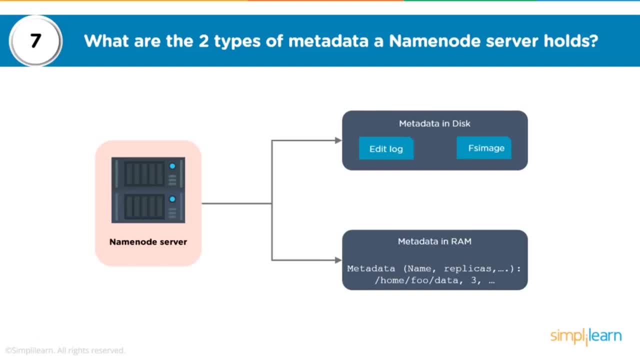 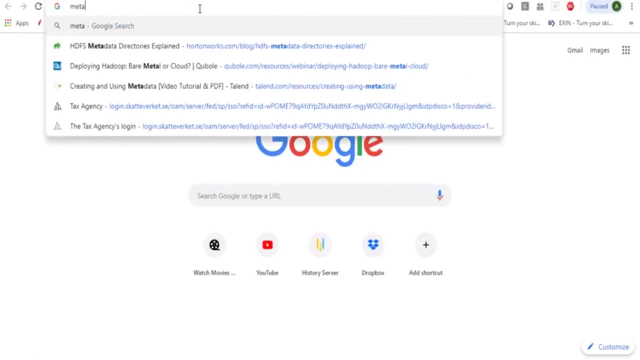 information about your data nodes, files, files being split into blocks, blocks residing on data nodes and file permissions. so i will share a very good link on this and you can always look for more detailed information about your metadata so you can search for sdfs metadata directories explained now. this is from hortonworks, however. 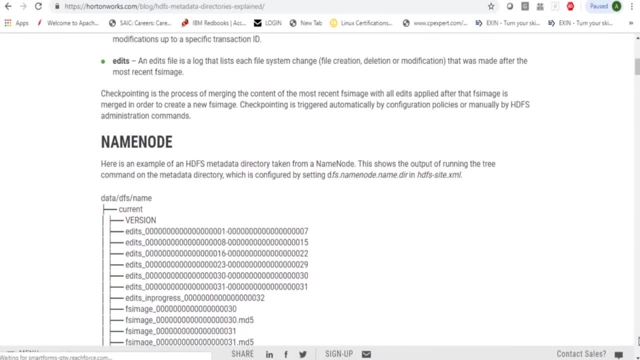 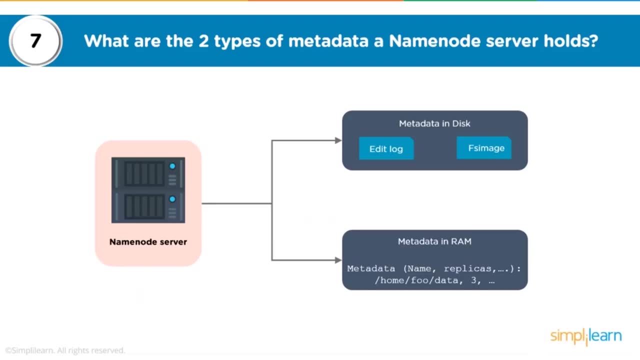 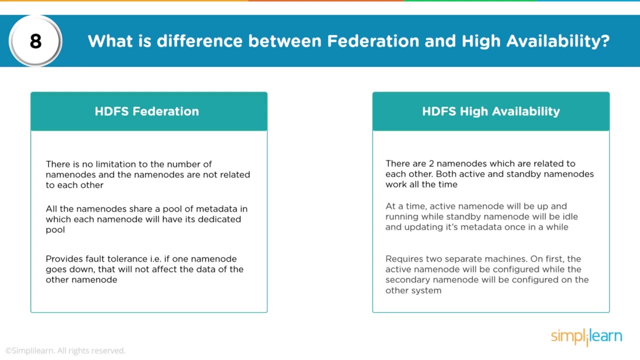 it talks about the metadata in disk which name node manages and details about this. so have a look at this link if you are more interested in learning about metadata on disk. coming back, let's look at the next question: what is the difference between federation and high availability? now, these are the features which were introduced in hadoop version 2.. both of 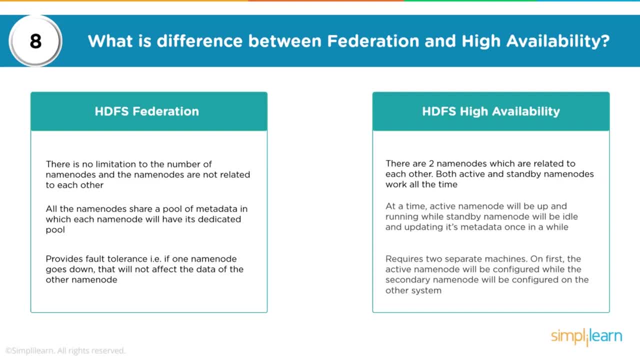 these features are about horizontal scalability of name node. so prior to version 2, the only possibility was that you could have one single master, which basically means means that your cluster could become unavailable if name node would crash, so hadoop. version 2 introduced two new features: federation and high availability. however, high availability- 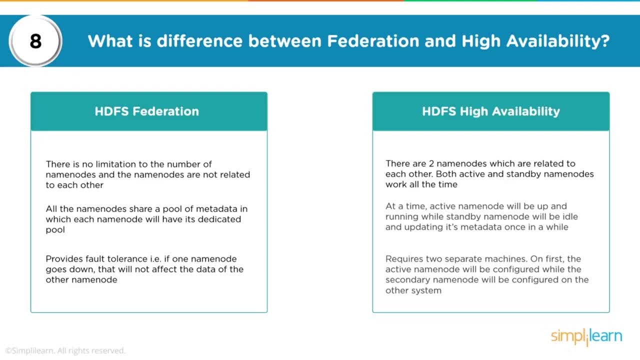 is a popular one. so when you talk about federation, it basically means any number of name nodes, so there is no limitation to the number of name nodes. your name nodes are in a federated cluster, which basically means name nodes still belong to the same cluster, but they are not. 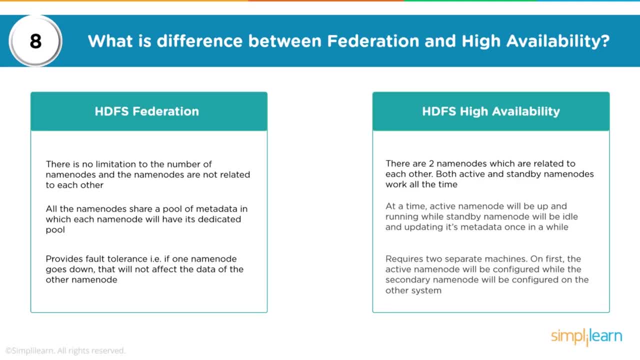 coordinating with each other. so whenever a write request comes in, one of the name node picks up that request and it guides that request for the blocks to be written on data nodes. but for this your name node does not have to coordinate with other name node to find out if the block id which 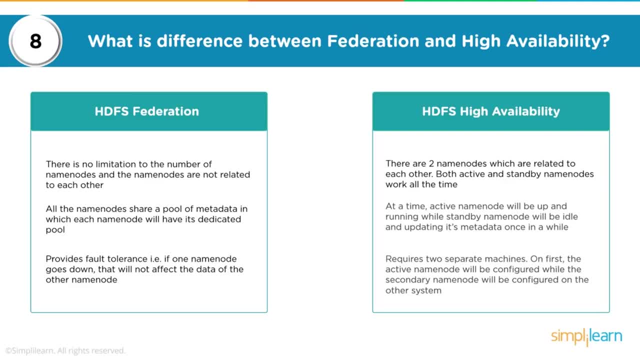 was being assigned was the same one as assigned by other name node, so all of them belong to a federated cluster. they are linked via a cluster id. so whenever an application or an api is trying to talk to cluster, it is always going via an cluster id and one of the name. 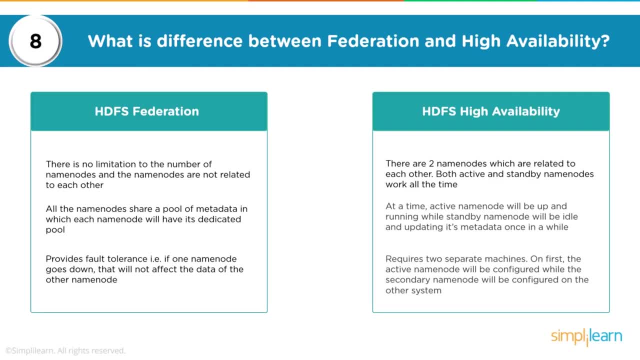 node would pick up the read activity or write activity or processing activity. so all the name nodes are sharing a pool of metadata in which each name node will have its own dedicated pool, and we can remember that by a term called namespace or name service. so this also provides. 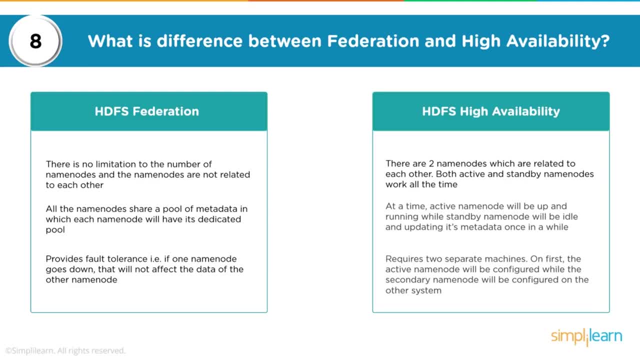 high fault tolerance. suppose your one name node goes down, it will not affect or make your cluster unavailable. you will still have your cluster reachable because there are other name nodes running and they are available now. when it comes to heartbeats, all your data nodes are sending their heartbeats to all the name nodes and all the name nodes are aware of. 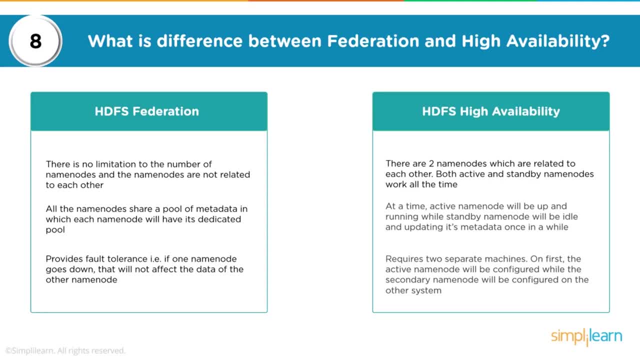 all the data nodes. when you talk about high availability, this is where you would only have two name nodes, so you would have an active and you would have a standby. now, normally in any environment, you would see a high availability setup with zookeeper. so zookeeper is a centralized 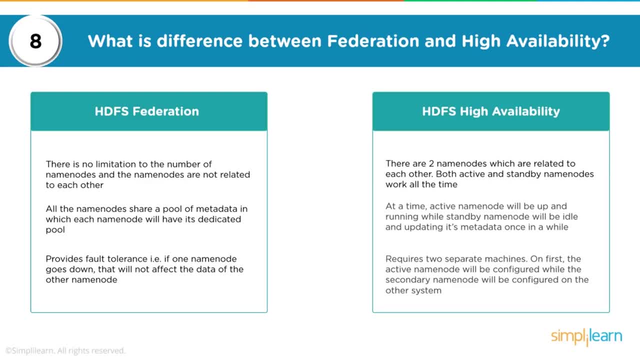 coordination service. so when you talk about your active and standby name nodes, election of node to be made as active and taking care of a automatic failover is done by your zookeeper. high availability can be set up without zookeeper but that would mean that the admins intervention would. 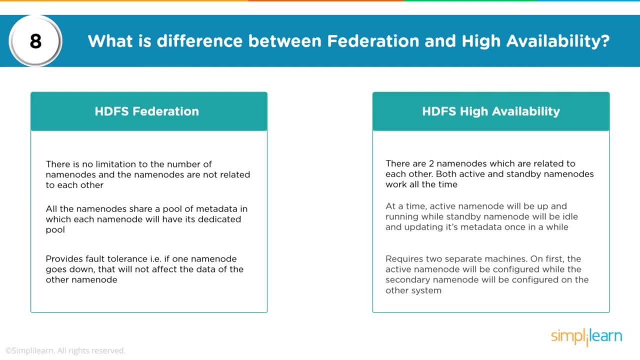 be required to make a name node as active from standby or also to take care of failover. now, at any point of time in high availability, a active name node would be taking care of storing the edits about whatever updates the name node is going to be taking care of. so this is where you 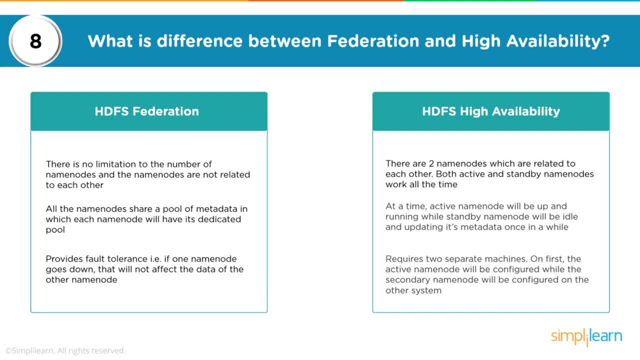 would see, the updates are happening on sdfs and it is also writing these edits to a shared location. standby name node is the one which is constantly looking for these latest updates and applying to its metadata, which is actually a copy of whatever your active name node has. 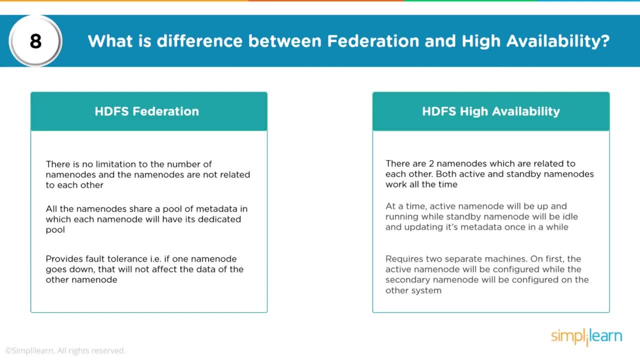 so in this way, your standby name node is always in sync with the active name node and if, for any reason, active name node fails, your standby name node will take over and become the active. remember, zookeeper plays a very important role here. it's a centralized coordination service. 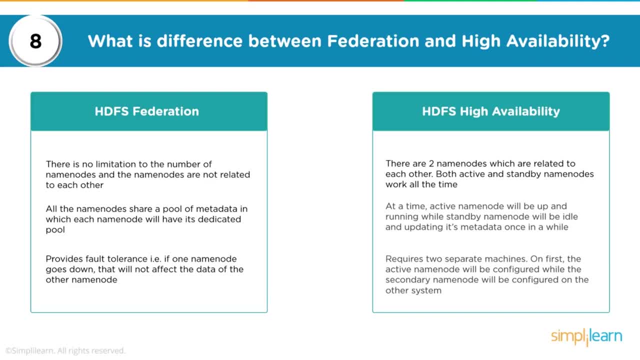 one more thing to remember here is that in your high availability, secondary name node will not be allowed. so you would have an active name node and then you will have a standby name node which will be configured on a separate machine, and both of these will be having access to a shared 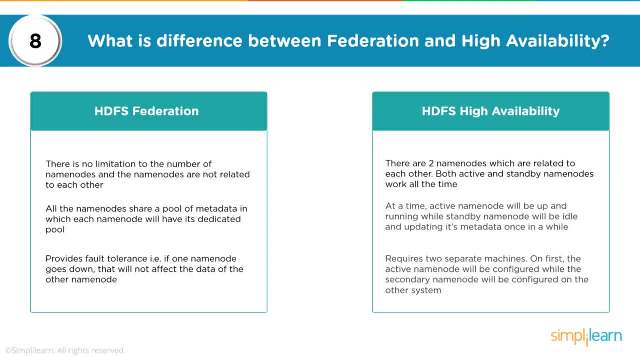 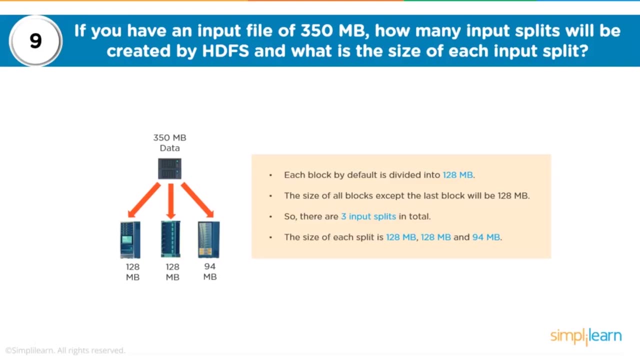 location. now that shared location could be nfs or it could be a quorum of general nodes. so for more information, refer to the tutorial where i have explained about sdfs, high availability and federation. now let's look at some logical question here. so if you have a input file of 350, 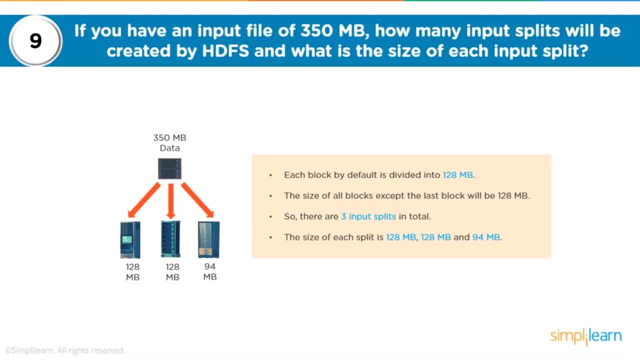 mb, which is obviously bigger than 128 mb, how many input splits would be created by sdfs and what would be the size of each input split? so for this, you need to remember that by default, the minimum block size is 128 mb. now, that's customizable. 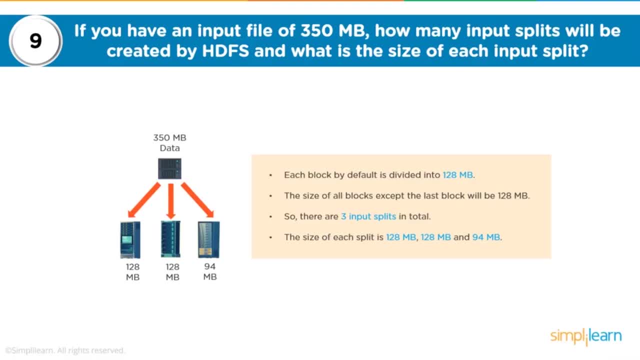 if your environment has more number of larger files written on an average, then obviously you have to go for a bigger block size. if your environment has a lot of files being written but these files are of smaller size, you could be okay with 128 mb. remember in hadoop, every entity. 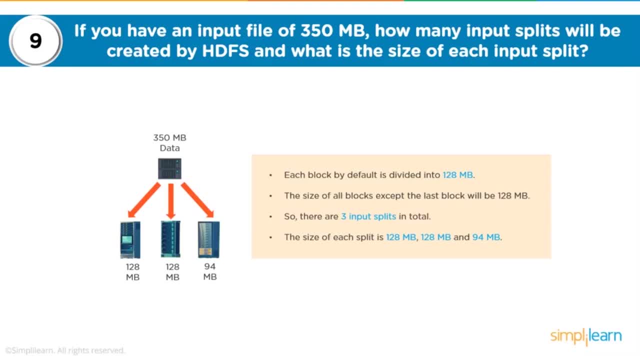 that is, your directory on sdfs file on sdfs and a file having multiple blocks. each of these are considered as objects and for each object, name nodes ram, 150 bytes is utilized. so if your block size is very small, then you would have more number of blocks which would directly affect the name nodes ram. if you keep a block size very high. 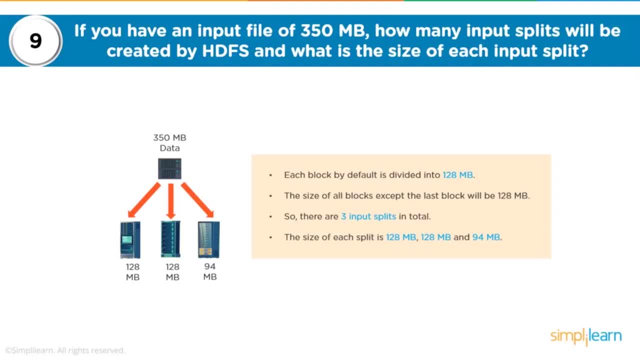 that will reduce the number of blocks, but remember that might affect in processing because processing also depends on splits. more number of splits, more the parallel processing. so setting of block size has to be done with consideration about your parallel ism requirement and your name, nodes ram, which is available. now coming to the question, if you have, 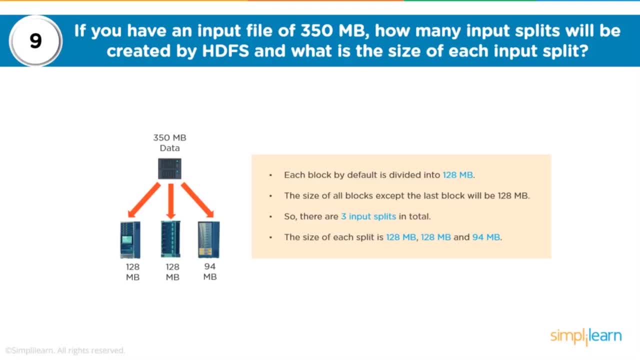 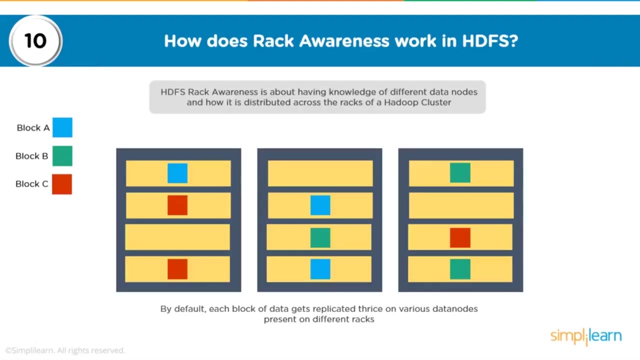 a file of 350 mb. that would be split into three blocks, and here two blocks would have 128 mb data and the third block, although the block size would still be 128, it would have only 94 mb of data. so this would be the split of this particular file. now let's understand about rack awareness: how 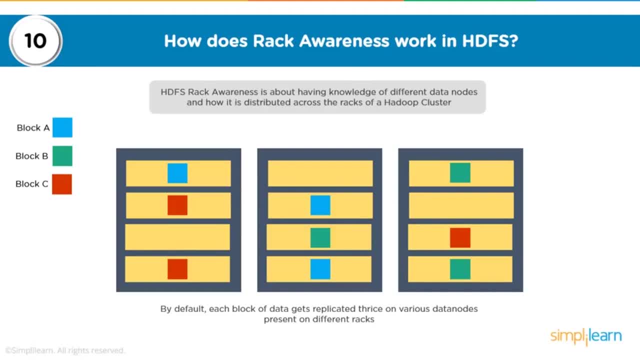 does rack awareness work or why do we even have racks? so organizations always would want to place their nodes or machines in a systematic way. there can be different approaches. you could have a rack which would have machines running on the master processes and the intention would be that this. 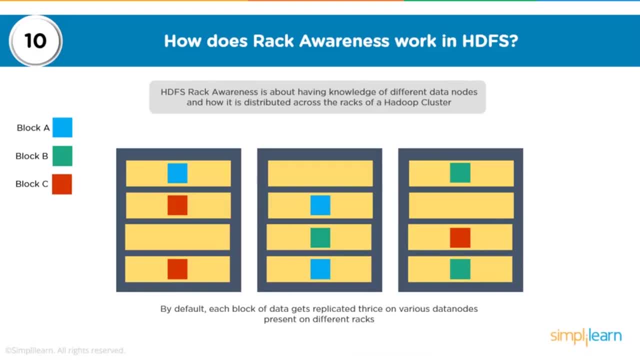 particular rack could have higher bandwidth, more cooling, dedicated power supply, top of rack switch, and so on. the second approach could be that you could have one master process running on one machine of every rack and then you could have other slave processes running. now, when you talk about your rack awareness, one thing to understand is that if your machines are placed within racks, 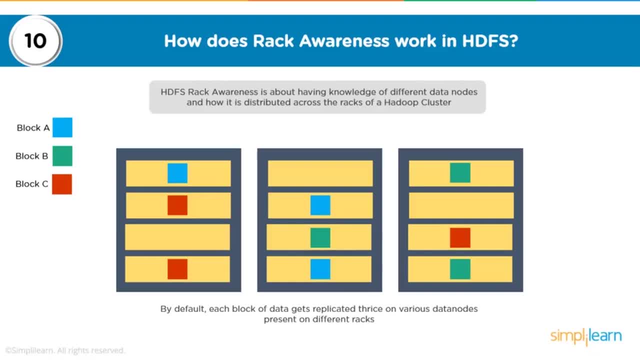 and we are aware that adobe follows auto replication. the rule of replication in a rack aware cluster would be that you would never have all the replicas placed on the same rack. so if we look at this, if we have block a in blue color, you will never have all the three blue boxes in the same rack, even if they are on. 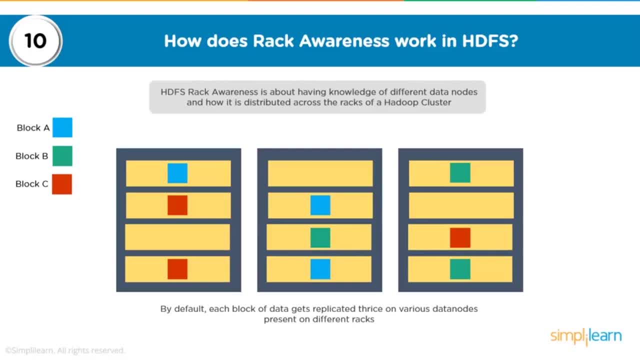 different nodes, because that makes us- that makes it- less fault tolerant. so you would have at least one copy of block which would be stored on a different rack, on a different node. now let's look at this. so basically, here we are talking about replicas being placed in such a way. now, 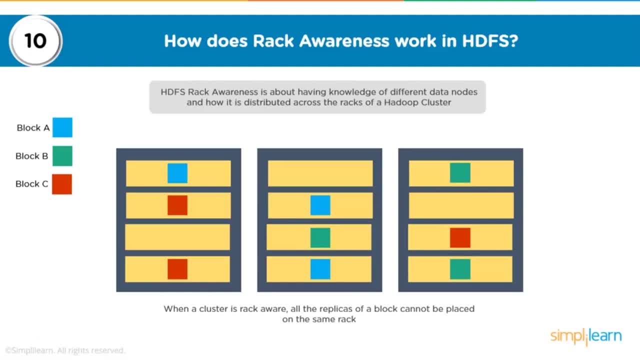 somebody could ask a question. can i have my block and its replica is spread across three racks? and yes, you can do that, but then, in order to make it more redundant, you are increasing your bandwidth requirement. so the better approach would be two blocks on the same rack on different machines and one copy on a different rack. now let's proceed. how can you? 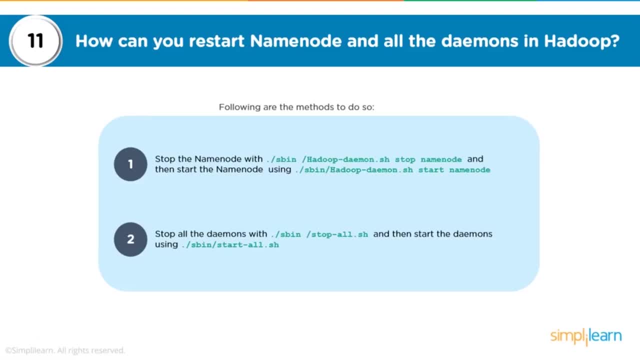 restart name node and all daemons in hadoop. so if you were working on a apache hadoop cluster then you could be doing a start and stop using hadoop and you could also use the open mocking finance Hadoop daemon scripts. So there are these Hadoop daemon scripts which would be used to start and 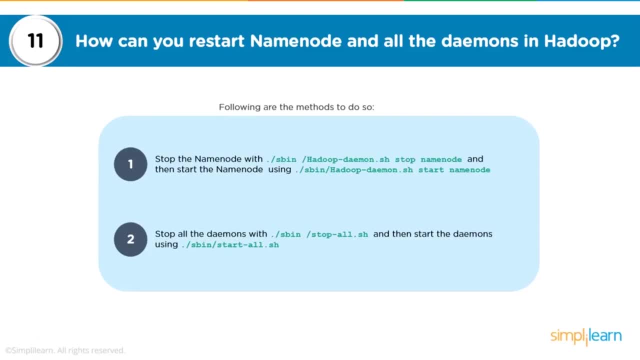 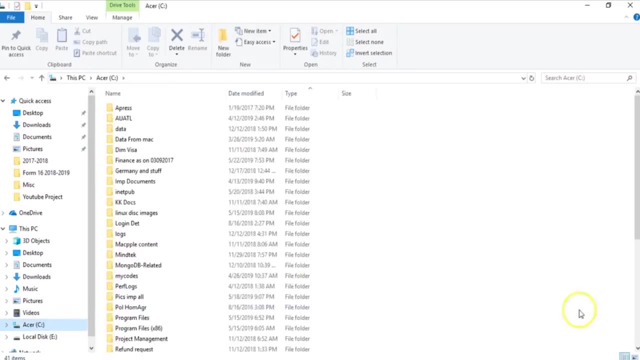 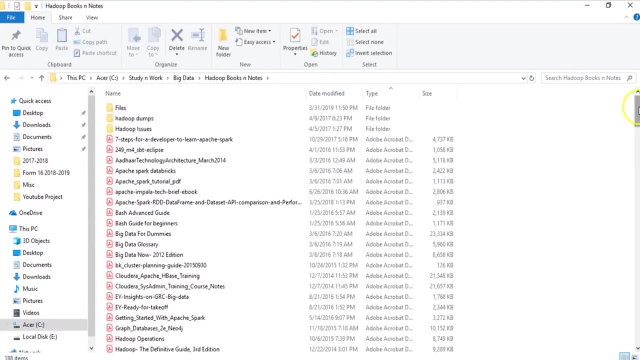 stop your Hadoop, And this is when you talk about your Apache Hadoop. So let's look at one particular file which I would like to show you more information here, And this talks about your different clusters. So let's look into this. And so let's look at the start and stop, And here I have a file, Let's look. 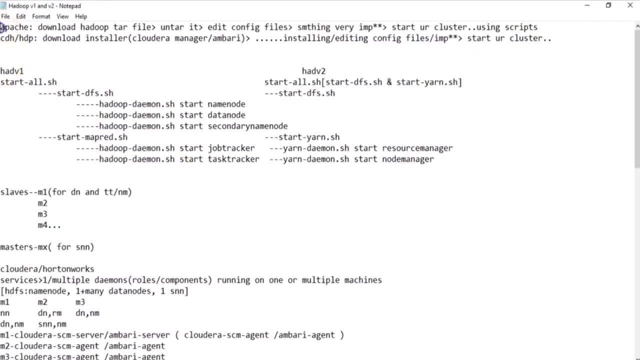 at this one, And this gives you highlights. So if you talk about Apache Hadoop, this is how the setup would be done. So you would have it, download the Hadoop tarp file, You would have to untar it, edit the config files, You would have to do formatting and then start your cluster. And here I have said using scripts. So this is in case of Apache Hadoop. you could be using a start all script that internally triggers start DFS and start yarn, And these scripts start DFS internally would run Hadoop daemon multiple times based on your configs, to start your different processes. Then your start. 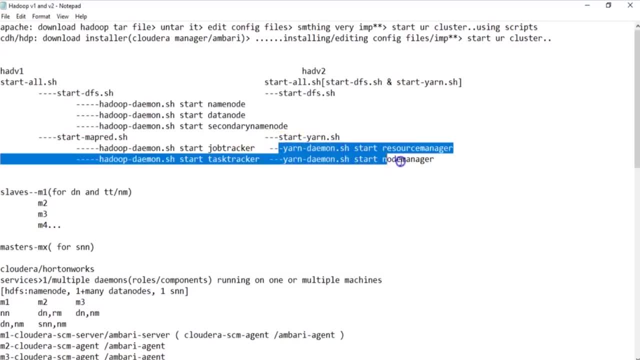 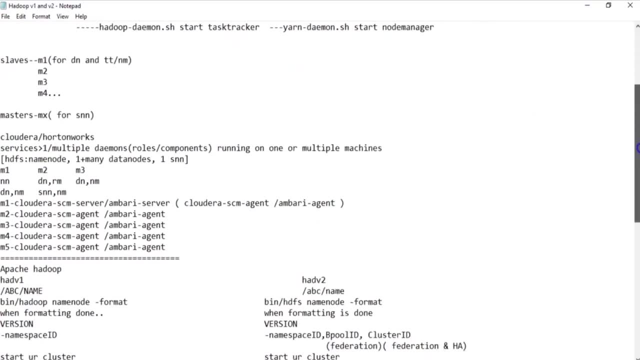 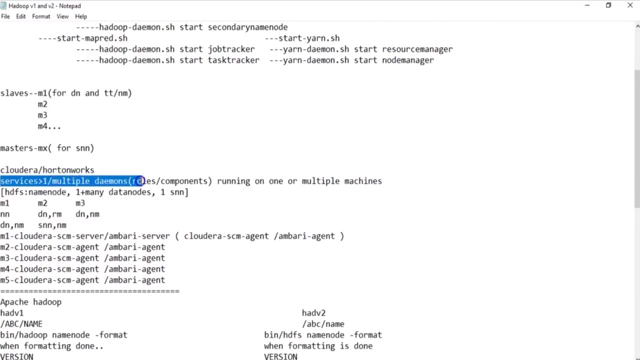 yarn would run yarn daemon script to start your processing related processes. So this is how it happens in Apache Hadoop. Now in case of Cloudera or Hortonworks, which is basically a vendor specific distribution, you would have say multiple services, which would have one or multiple. 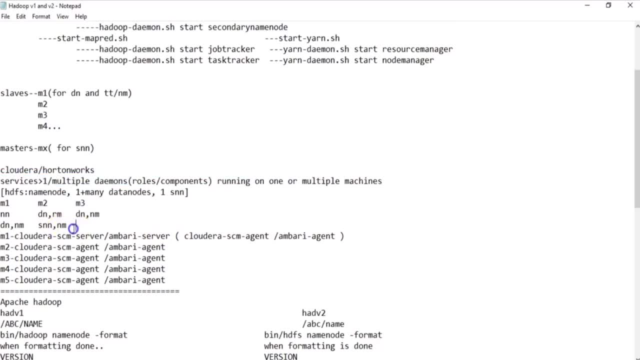 daemons running across the machines. Let's take an example here that you would have machine one, machine two And machine three, with your processes spread across. However, in case of Cloudera and Hortonworks, these are cluster management solutions, So you would never be involved in running a script. 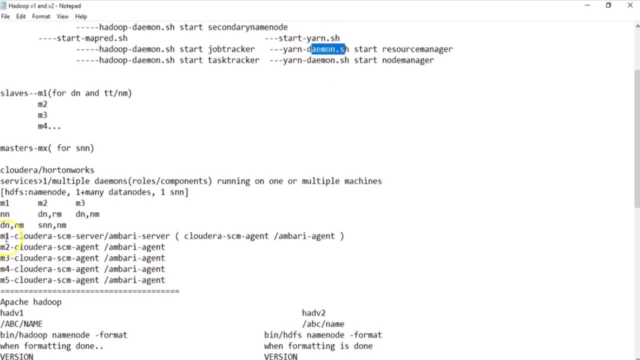 individually to start and stop your processes. In fact, in case of Cloudera, you would have a Cloudera SCM server running on one of the machines and then Cloudera SCM agents running on every machine. If you talk about Hortonworks, you would have Ambari server and Ambari agent running. So 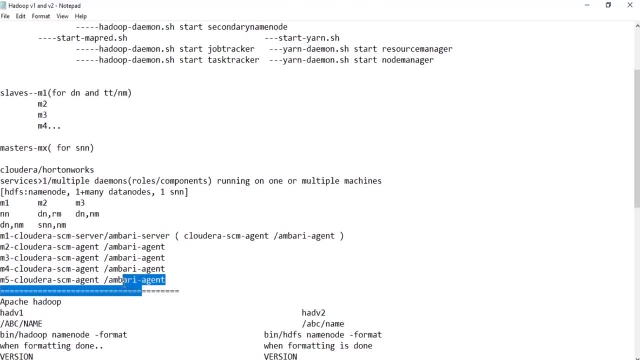 your agents, which are running on every machine, are responsible to monitor the processes. send also their heartbeat to the master. that is your server. And your server is the one, or a service, which basically will give instructions to the agents. So in case of vendor specific distribution, 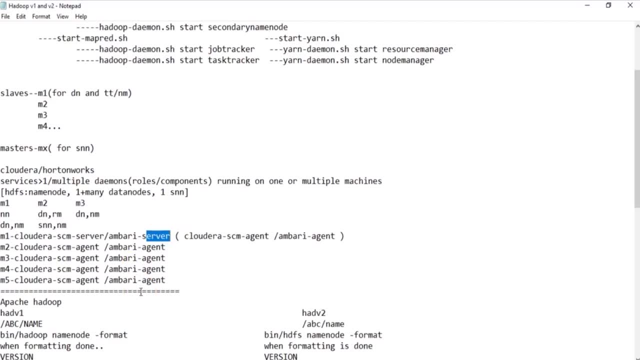 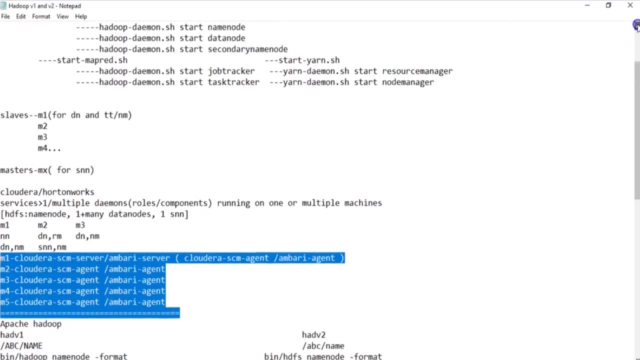 your start and stop of processes is automatically taken care by these underlying services, And these services internally are still running on the same machine, So you would have a server running on every machine, However only in Apache Hadoop. you have to manually follow these to start and stop. 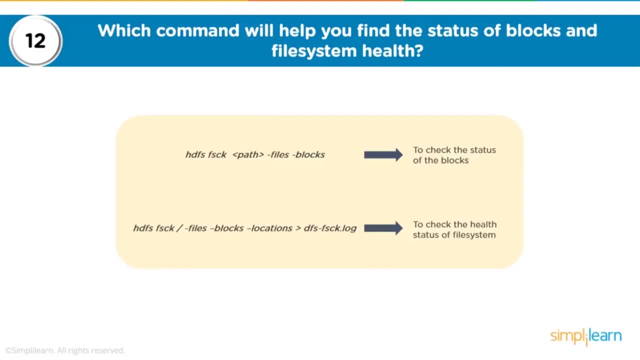 Coming back we can look into some command related questions. So which command will help you find the status of blocks and file system health? So you can always go for a file system check command Now that can show you the files for a particular HDFS path. It can show you the blocks. 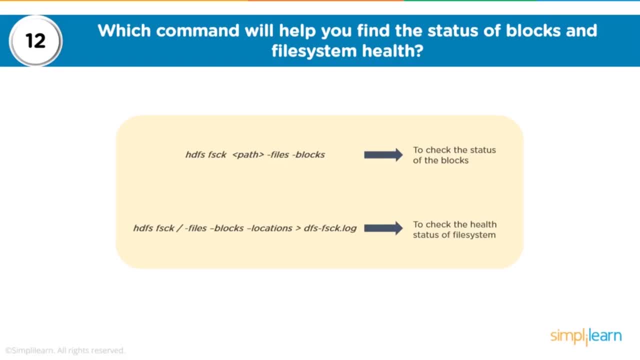 and it can also give you information on status, such as under-replicating, over-replicating, over-replicating, mis-replicating and so on. So this file system check utility does not repair if there is any problem with the blocks. 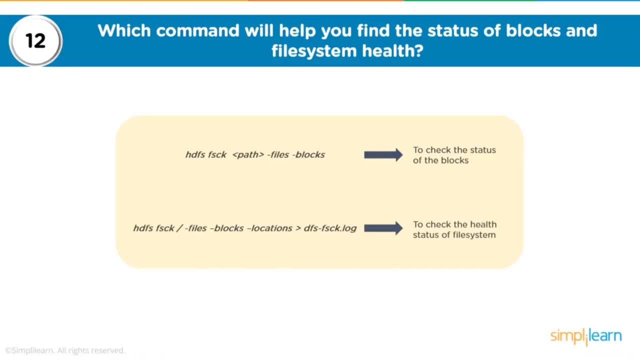 but it can give you information of blocks related to the files, on which machines they are stored, if they are replicated as per the replication factor or if there is any problem with any particular replica. What would happen if you store too many small files in a cluster? 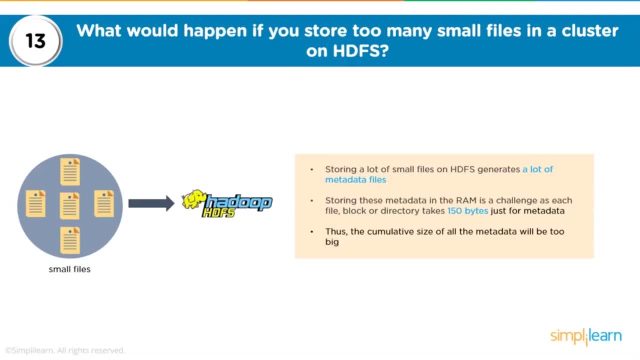 relates to the block information which I gave some time back. So remember, Hadoop is coded in Java, So here every directory, every file and file related block is considered as an object, And for every object within your Hadoop cluster. 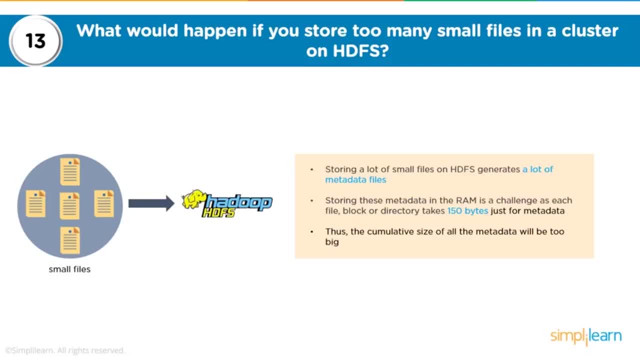 name-nodes-ram gets utilized, So more number of blocks you have, more would be usage of name-nodes-ram And if you're storing too many small files, it would not affect your disk, It would directly affect your name-nodes-ram. That's why, in production, 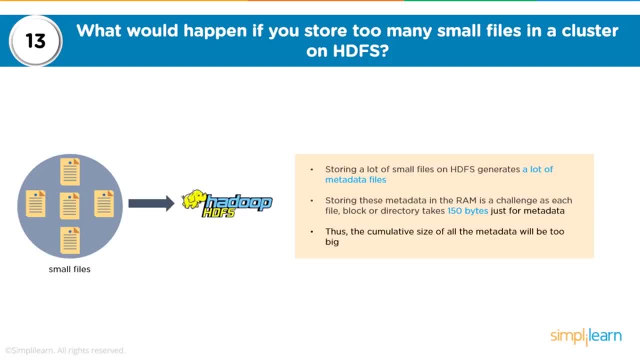 clusters admin guys or infrastructure specialists will take care that everyone who is writing data to HDFS follows a quota system, so that you could be controlled in the amount of data you write plus the count of data an individual writes on HDFS. Now how do you copy data from local system onto HDFS? 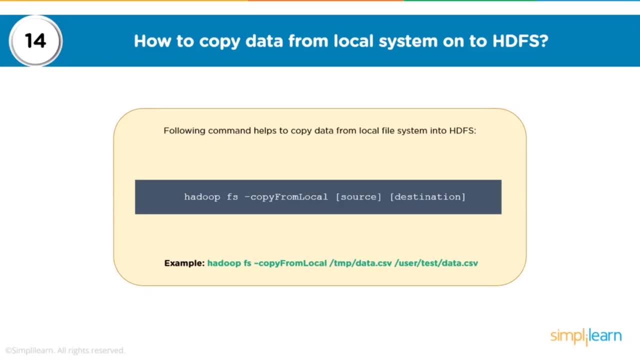 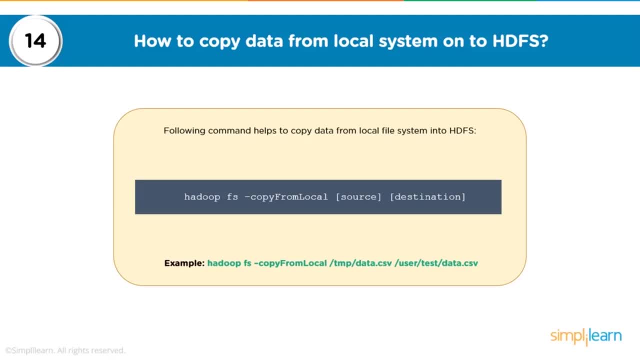 your HDFS path. Remember you can always do a copy from local using a minus F option. That's a flag option And that also helps you in writing the same file or a new file to HDFS. So with your minus F you have a chance of overwriting or rewriting the data. 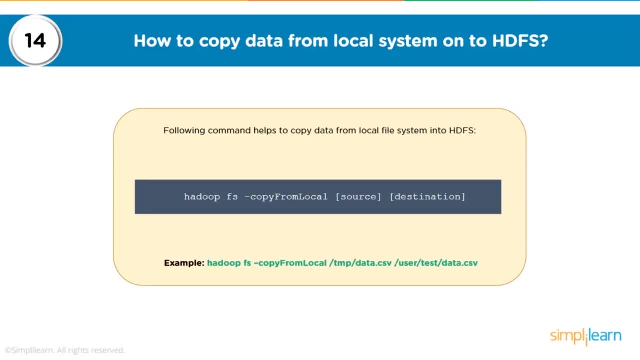 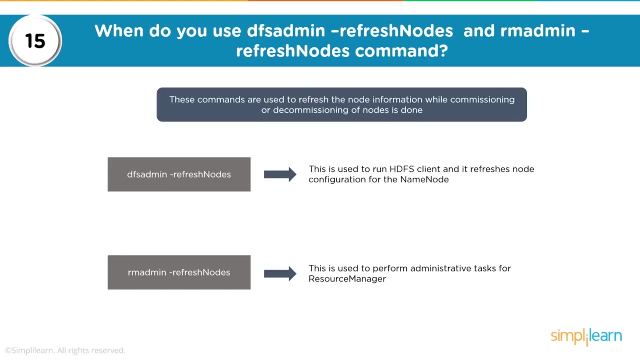 which is existing on HDFS. So copy from local or minus put. both of them do the same thing And you can also pass an argument when you're copying to control your replication or other aspects of your file. Now, when do you use DFS admin refresh nodes or the RM admin refresh? 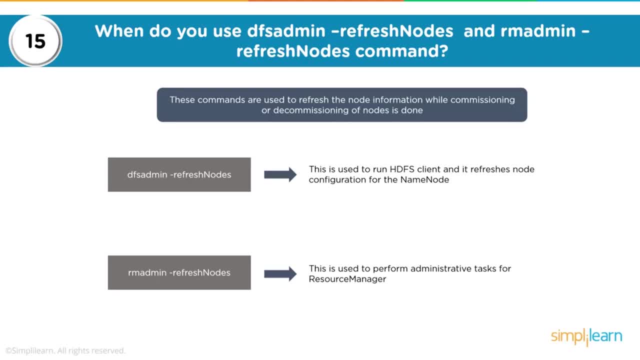 nodes. So, as the command says, this is basically to do with refreshing the node information. So your refresh nodes is mainly used when, say, a commissioning or decommissioning is done, So when a node is added into the cluster or when a node is removed from the cluster, 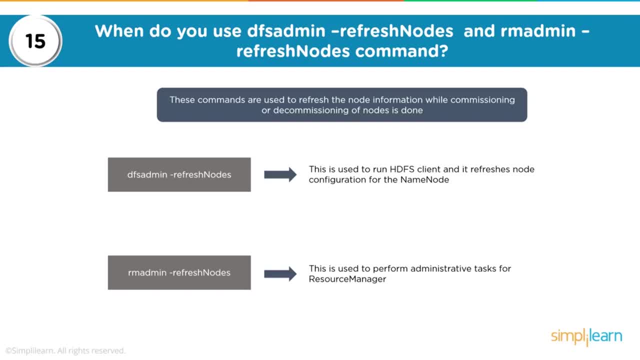 you are actually informing Hadoop master that this particular node would not be used for storage and would not be used for processing. I mean that case you would be. once you are done with the process of commissioning or decommissioning, you would be giving these. 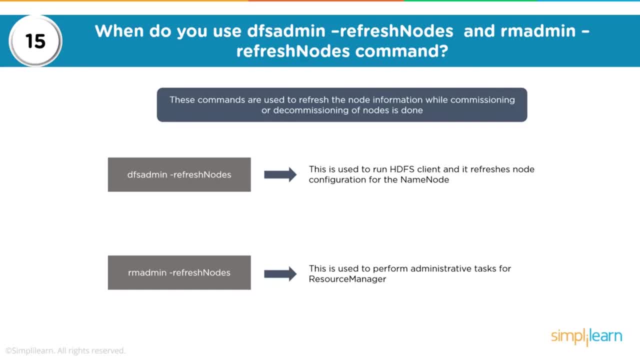 commands, That is, refresh nodes and RM admin refresh nodes. So you can use that as the command and that's it. See you in the next class. Bye, admin, refresh notes. so internally, when you talk about commissioning, decommissioning, there are: 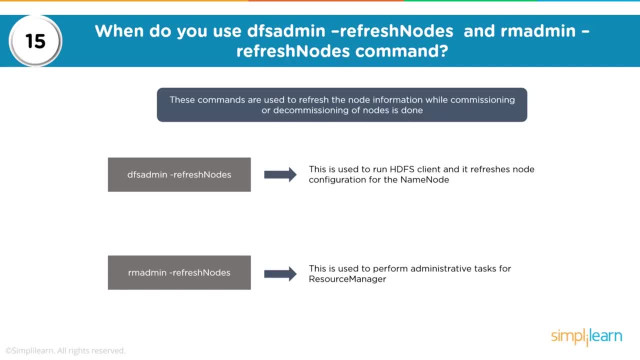 include and exclude files which are updated, and these include and exclude files will have entry of machines which are being added to the cluster or machines which are being removed from the cluster. and while this is being done, the cluster is still running, so you do not have to restart. 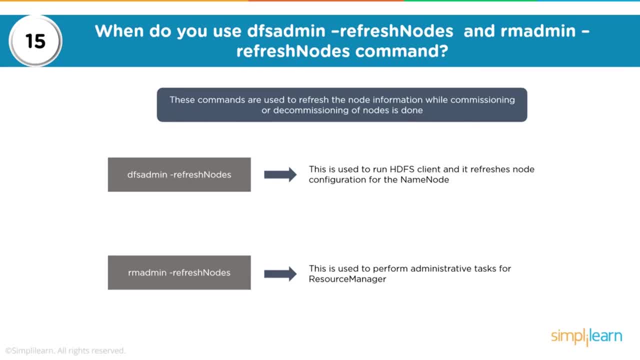 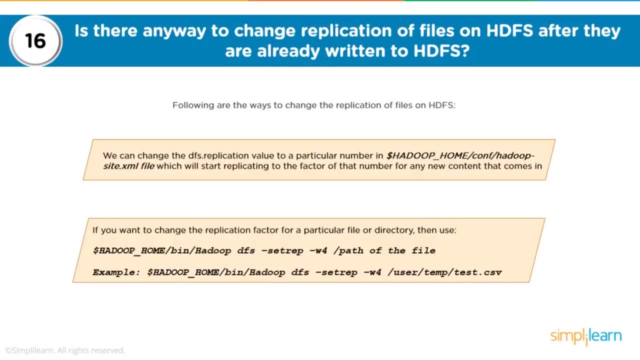 your master process. however, you can just use these refresh commands to take care of your commissioning decommissioning activities. now, is there any way to change replication of files on sdfs after they are already written? and the answer is, of course, yes. so if you would want to, 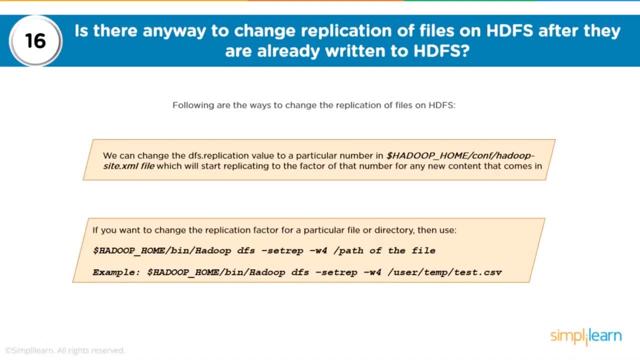 set a replication factor at a cluster level and if you have admin access, then you could edit your sdfs hyphen site file or you could say hadoop hyphen site file, and that would take care of replication factor being set at a cluster level. however, if you would want to change the 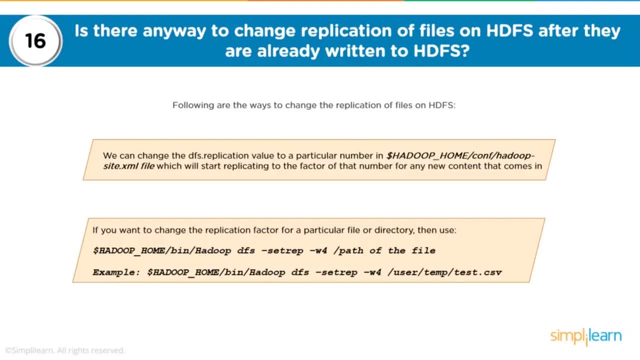 rep application. after the data has been written, you could always use a set rep command. so set rep command is basically to change the replication after the data is written. you could also write the data with a different replication and for that you could use a minus, d dfs dot replication. 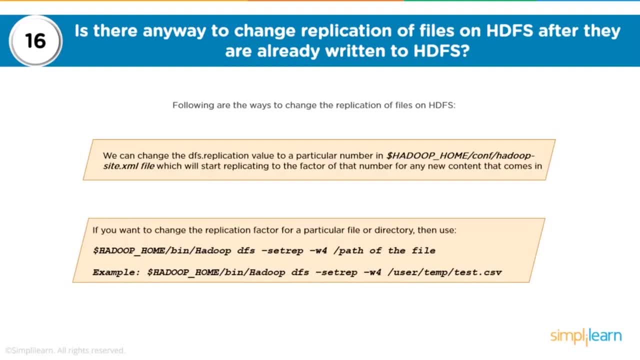 and give you a replication factor when you are writing data to the cluster. so in hadoop you can let your data be replicated as per the property set in the config file. you could write the data with a different replication. you could change the replication after the data is written. so all these options are available now. 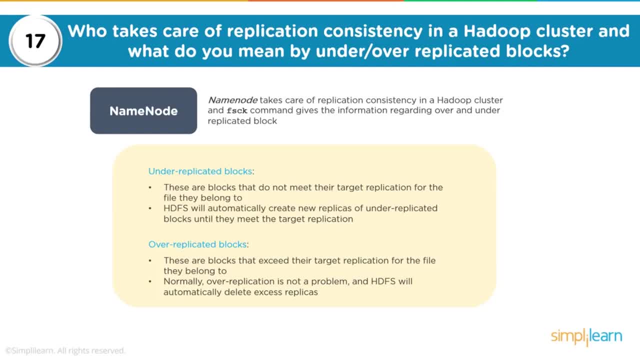 who takes care of replication consistency in a hadoop cluster and what do you mean by under over replicated blocks? now, as i mentioned, your fsck command can give you information of over or under replicated blocks. now in a cluster, it is always and always named node and it is always a name node. 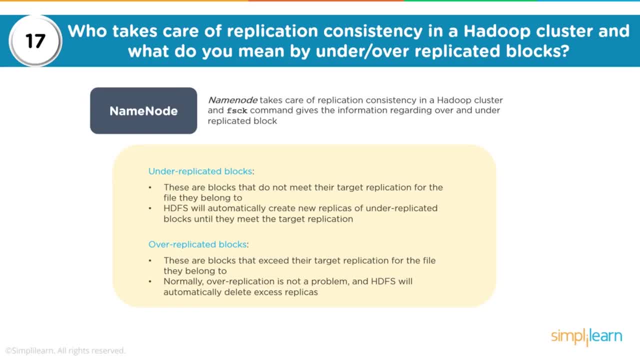 which takes care of replication consistency. so, for example, if you have set up a replication of three and since we know the first rule of replication, which basically means that you cannot have two replicas residing on the same node, it would mean that if your replication is three, you would need at least three data notes available. now say, for example, you had a cluster with three. 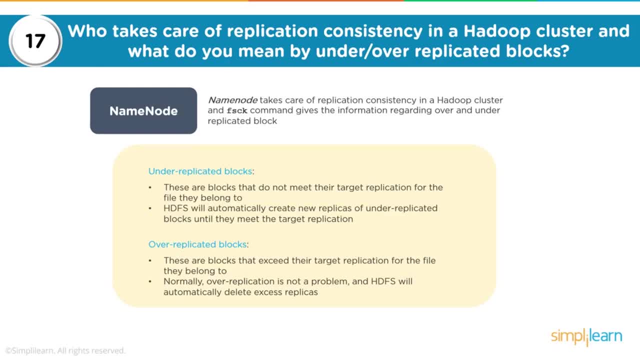 nodes and replication was set to three. now, if we apply this, the first rule, it gives you this series of three data nodes and replication need to create each on three records that protecting or outside of all prepositions, andけれ three: At one point of time one of your name node crashed And if that happens, your blocks. 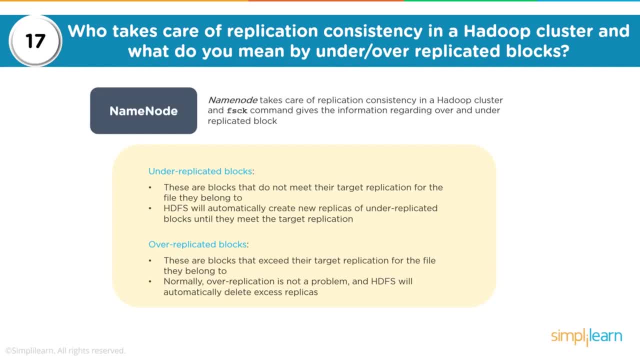 would be under replicated. That means there was a replication factor set, but now your blocks are not replicated or there are not enough replicas as per the replication factor set. This is not a problem. Your master process or name node will wait for some time before it will start. 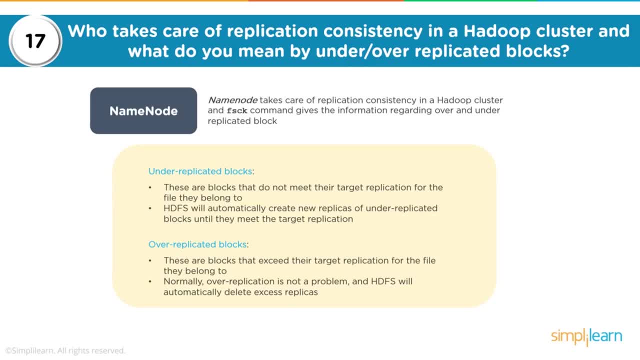 the replication of data again. So if a data road is not responding or if a disk has crashed and if name node does not get information of a replica, name node will wait for some time and then it will start re-replication of those missing blocks from the available nodes. However, while name node is, 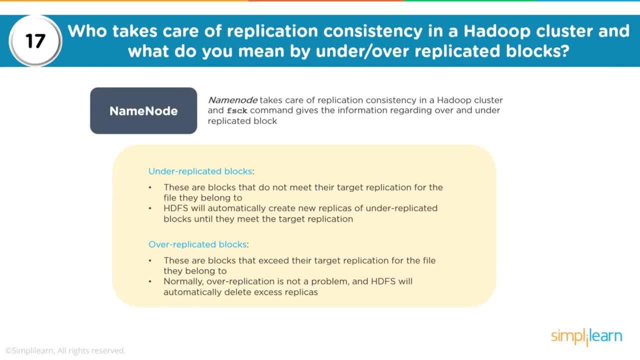 doing it. the blocks are in under replicated situation. Now, when you talk about over replicated, this is a situation where name node realizes that there are extra copies of block. Now this might be the case that you had three nodes running with a replication of three. One of the node went down due to a network failure or some other issue. 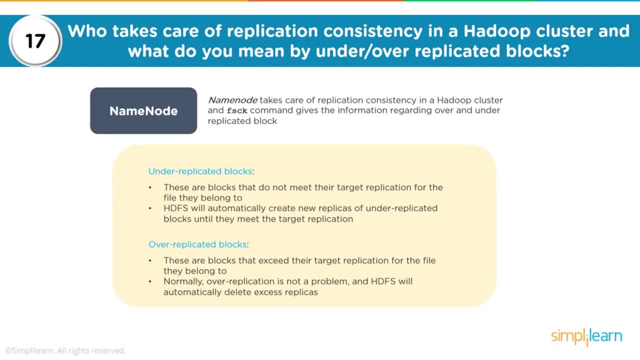 Within a few minutes, name node re-replicated the data and then the failed node is back with its set of blocks Again. name node is smart enough to understand that this is an over replication situation and it will delete set of blocks from one of the nodes. It might be the 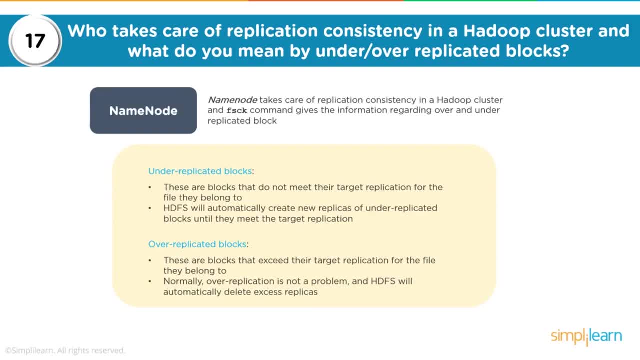 node that is running with a replication of three. Now, if you have a replication of three, it might be the node which has been recently added, It might be your old node which has joined your cluster again, or any node That depends on the load on a particular node. Now we discussed about Hadoop. 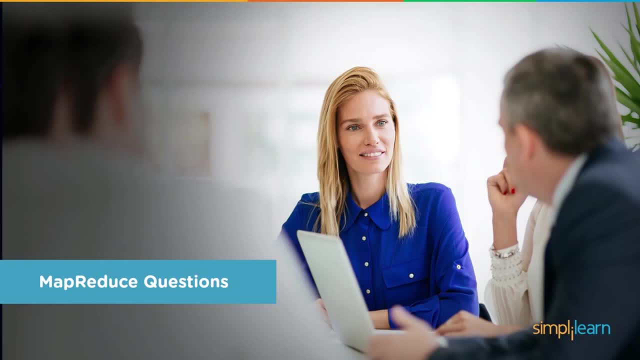 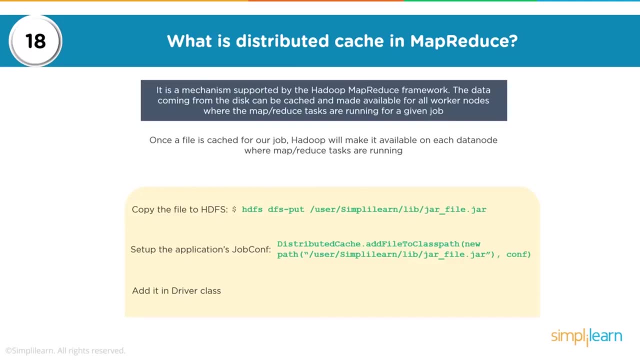 We discussed about SDFS. Now we will discuss about MapReduce, which is the programming model and, you can say, processing framework, What is distributed cache in MapReduce? Now we know that when we talk about MapReduce, the data which has to be produced by the data is the data which 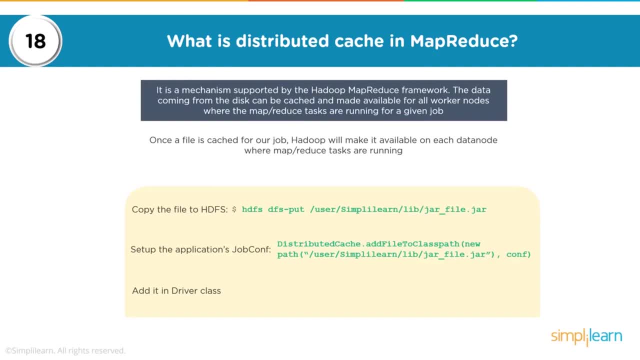 processed might be existing on multiple nodes. So when you would have your MapReduce program running, it would basically read the data from the underlying disks. Now this could be a costly operation if every time the data has to be read from disk. So distributed cache is a mechanism. 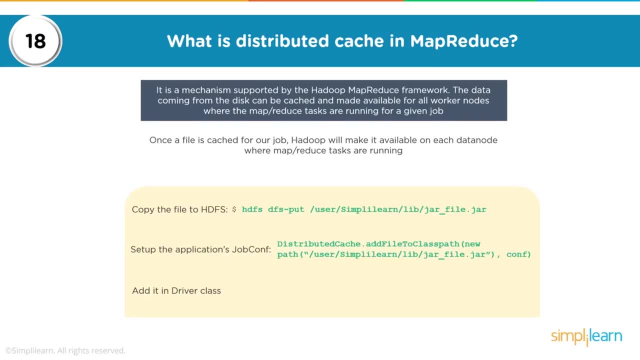 wherein data set or data which is coming from the disk can be cached and available for all nodes. Now how will this benefit? So, when a MapReduce is running, instead of every time reading the data from disk, it would pick up the data from. 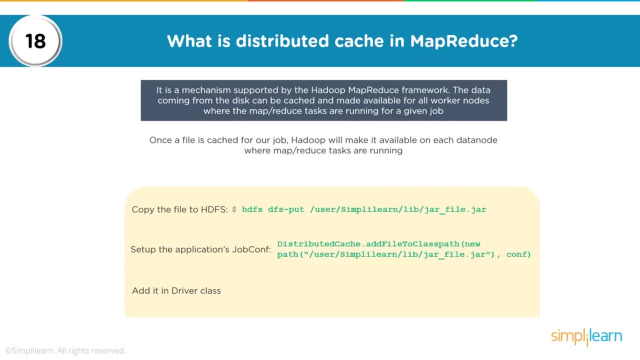 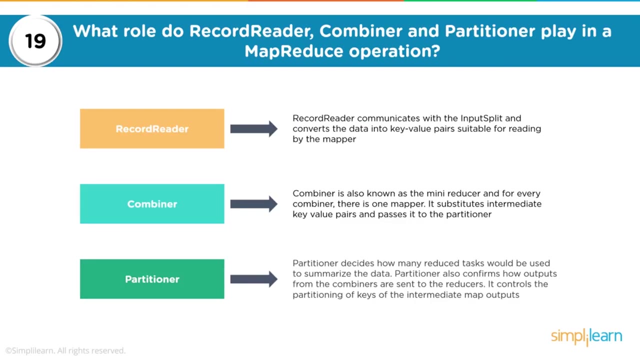 distributed cache and this will benefit your MapReduce processing. So distributed cache can be set in your job conf, where you can specify that a file should be picked up from distributed cache. Now let's understand about these roles. So what is a record reader? What is a combiner? What is a? 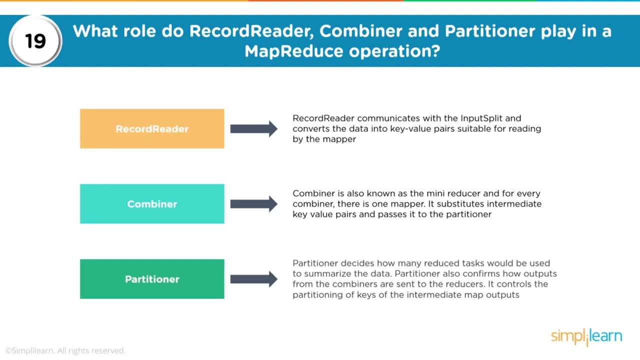 partitioner And what kind of data is being collected from distributed cache. Now let's understand. what kind of roles do they play in a MapReduce processing paradigm or MapReduce operation? So record reader communicates with the input split and it basically converts the data. 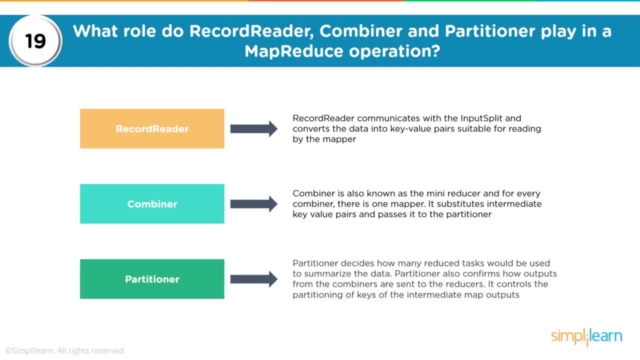 into key-value pairs, And these key-value pairs are the ones which will be worked upon by the mapper. Your combiner is an optional phase. It's like a mini-reduce. So combiner does not have its own class, It relies on the reducer class. 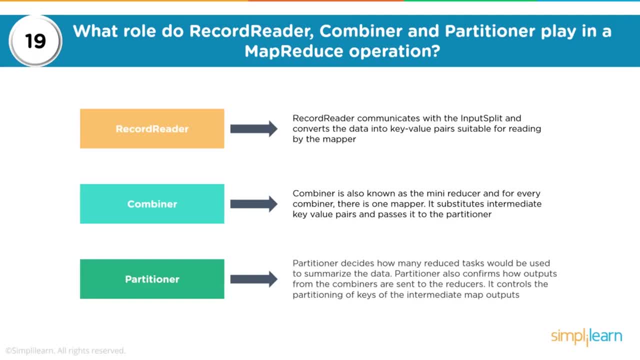 Basically, your combiner would receive the data from your map tasks which would have completed works on it, based on whatever reducer class mentions, and then passes its output to the reducer phase. Partitioner is basically a phase which decides how many reduced tasks would be. 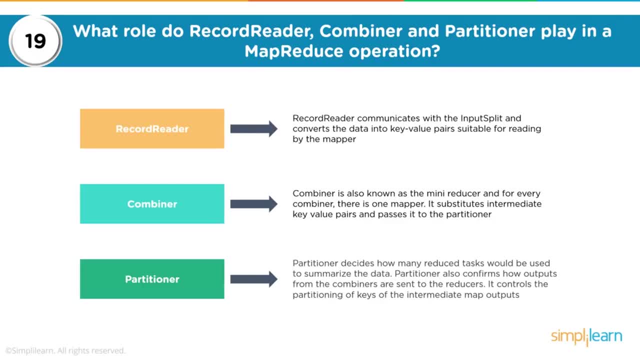 used to aggregate or summarize your data. So partitioner is a phase which would decide. based on the number of keys, based on the number of map tasks, your partitioner would decide if one or multiple reduced tasks would be used to take care of processing. So either it could be partitioner, 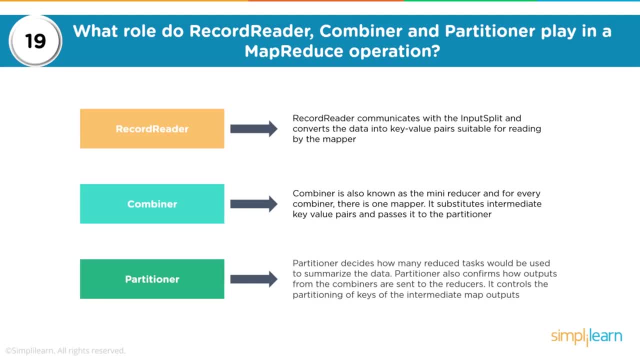 which decides on how many reduced tasks would run, or it could be based on the properties which we have set within the cluster, which will take care of the number of reduced tasks which would be used. Always remember, your partitioner decides how outputs from combiner are sent to reducer and to. 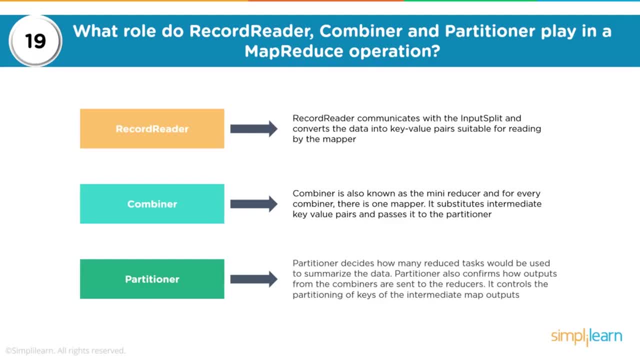 how many reducers. It controls the partitioning of keys of your intermediate map outputs. So map phase, whatever output it generates, is an intermediate output and that has to be taken by your partitioner or by a combiner and then partitioner to be sent to one or multiple reduced tasks. 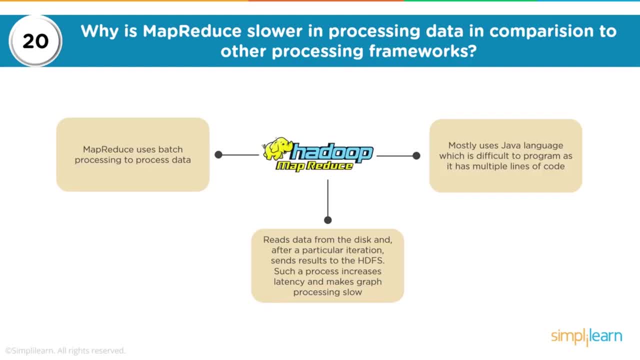 This is one of the common questions which you might face. Why is MapReduce slower in processing? So we know MapReduce goes for parallel processing. We know we can have multiple map tasks running on multiple nodes at the same time. We also know that multiple reduced tasks 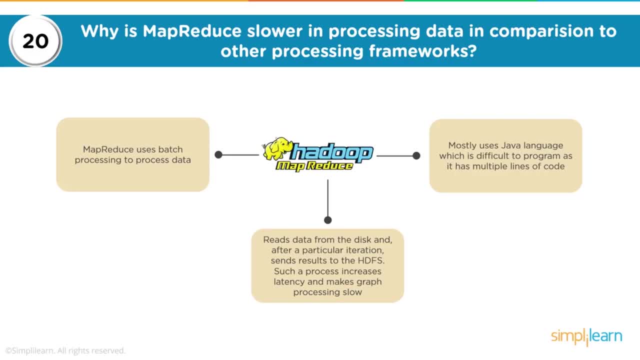 could be running. Now why does then MapReduce become a slower approach? First of all, your MapReduce is a batch-oriented operation. Now, MapReduce is very rigid and it strictly uses mapping and reducing phases. So, no matter what kind of processing you would want to do, you would have to still provide. 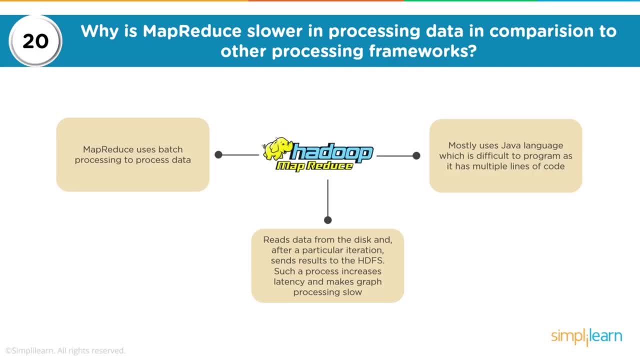 the mapper function And the reducer function to work on data. Not only this: whenever your map phase completes, the output of your map phase, which is an intermittent output, would be written to HDFS and thereafter underlying disks, And this data would then be shuffled and sorted and picked up for reducing phase. So every 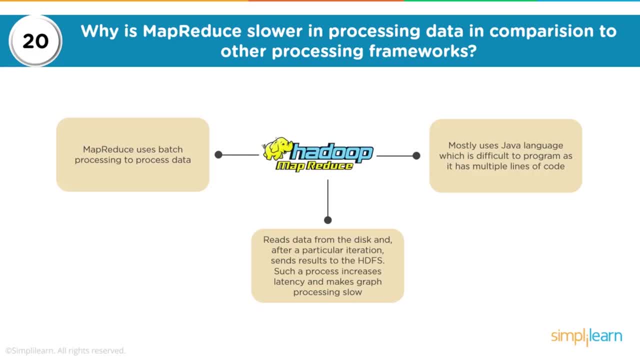 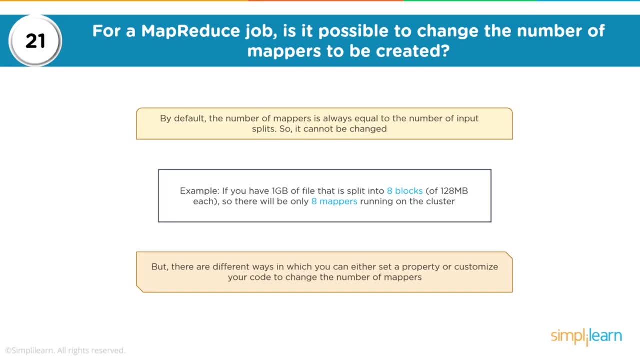 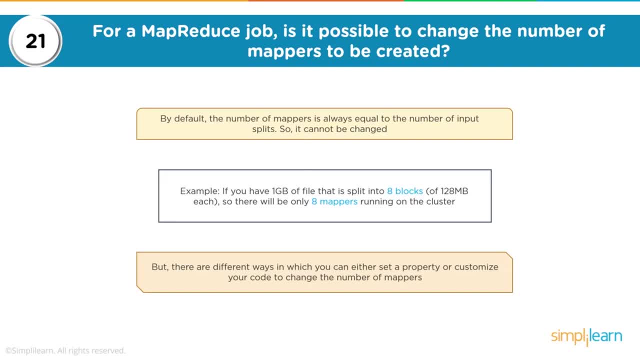 Now, by default, you cannot change the number of map tasks, because number of map tasks depends on the input splits. However, there are different ways in which you can either set a property to have more number of map tasks which can be used, or you can customize your code or make it use a different. 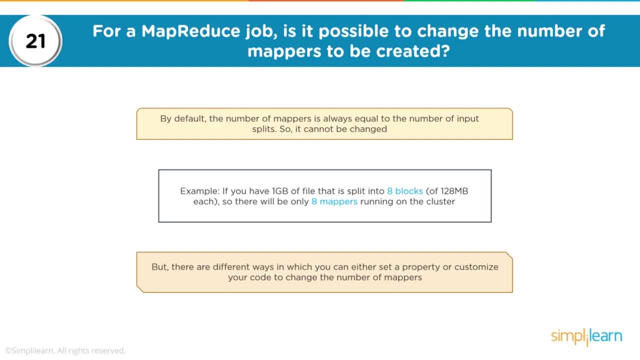 format Which can then control the number of map tasks. By default, number of map tasks are equal to the number of splits of file you are processing. So if you have a 1GB of file that is split into eight blocks of 128 MB, there would be eight map tasks running on the clusters. 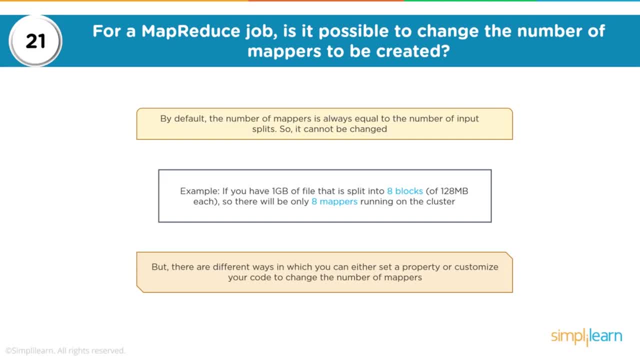 These map tasks are basically running your mapper function. If you have hard-coded properties in your MapRed-Site file, your test machine will not be able to do the operation And you will not be able to be able to do all the operation. So if you do not have a hard-coded properties in your MapRed-Site file, this is just an example for you to think about before you start working on your mapers. If you have hard-coded properties in your MapRed-Site file, if you do not have a hard-coded properties in your map, 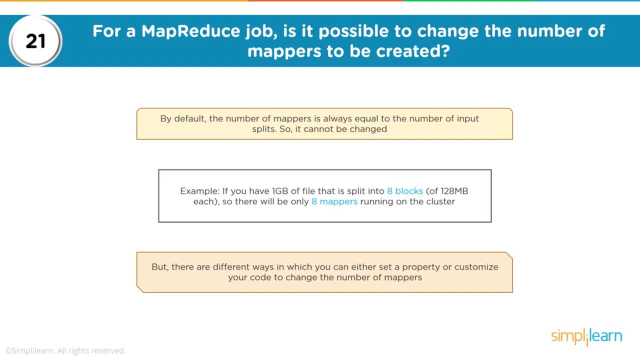 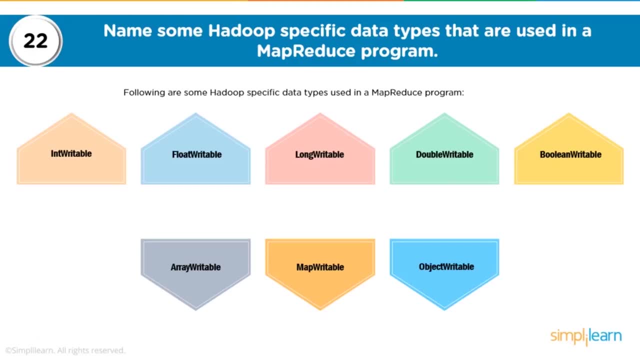 file to specify more number of map tasks. then you could control the number of map tasks. let's also talk about some data types. so when you prepare for hadoop, when you want to get into big data field, you should start learning about different data formats. now there are different data formats, such 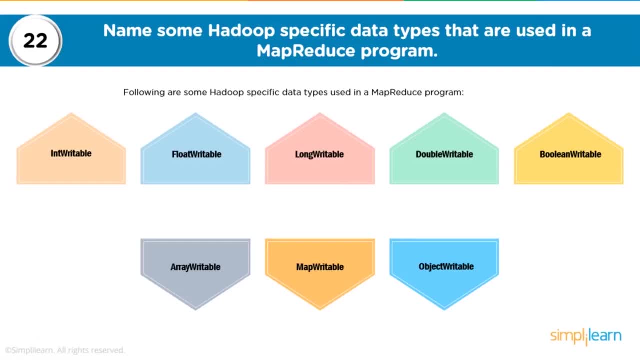 as avro parquet, you have sequence file or binary format, and these are different formats which are used now. when you talk about your data types in Hadoop, these are implementation of your writable and writable comparable interfaces. so for every data type in Java, you have a equivalent in Hadoop. 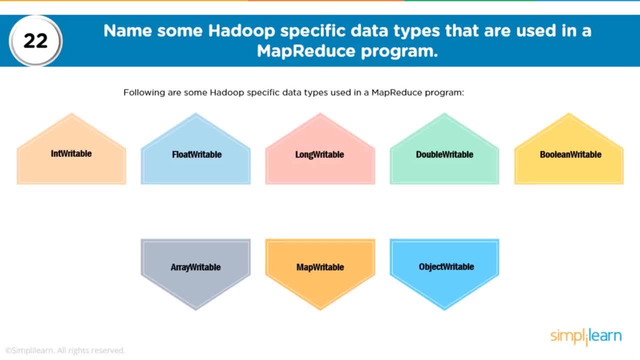 so int in Java would be int writable. in Hadoop, float would be float writable, long would be long writable, double writable, boolean writable, array writable, map writable and object writable. so these are your different data types that could be used in Hadoop within your MapReduce program and these are implementation of writable and writable. 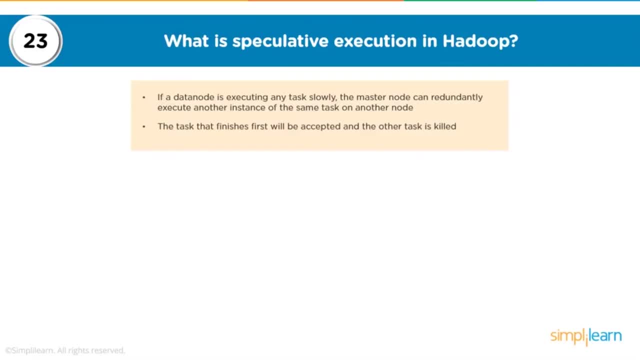 comparable interfaces. what is speculative execution? now imagine you have a cluster which has huge number of nodes and your data is spread across multiple slave machines or multiple nodes. now, at a point of time, due to a disk degrade or network issues, or machine heating up or more load being on, 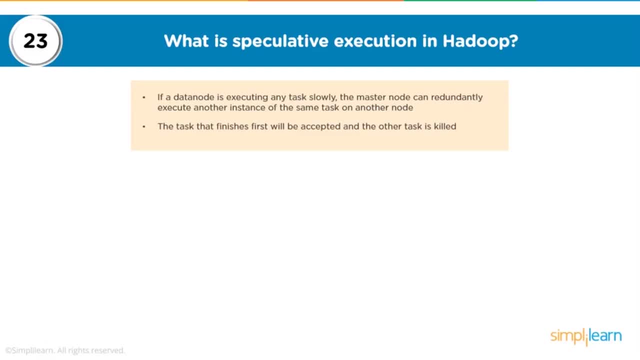 there can be a situation where your data node will execute tasks in a slower manner. now, in this case, if speculative execution is turned on, there would be a shadow task or a another similar task running on some other node for the same processing. so whichever task finishes first, 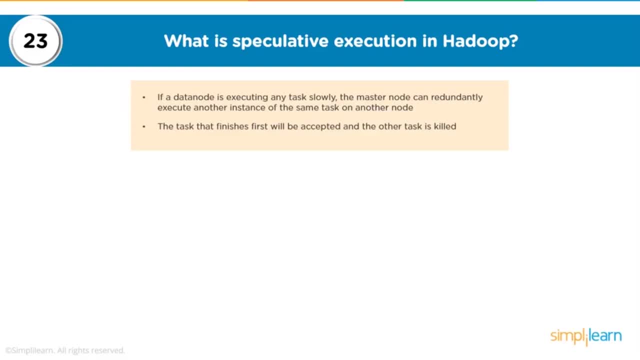 will be accepted and the other task would be killed. so speculative execution could be good if you are working in an intensive workload kind of environment where if a particular node is slower, you could benefit from a unoccupied or a node which has less load to take care of your 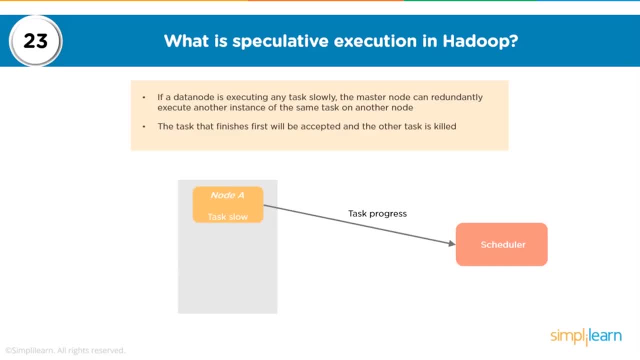 processing going further. this is how we can understand. so node A, which might be having a slower task, you would have a scheduler which is maintaining or having knowledge of what are the resources available. so if speculative execution properties turned on, then the task which was running slow, a copy of that task. or you can say: 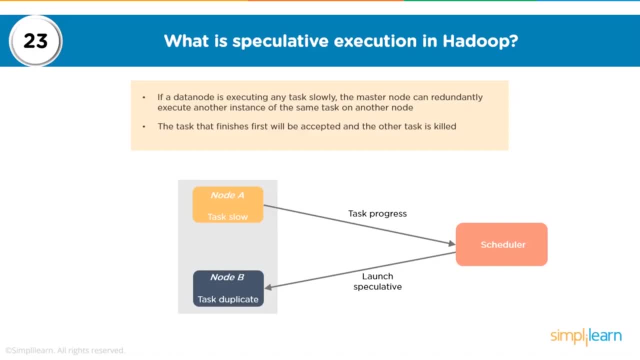 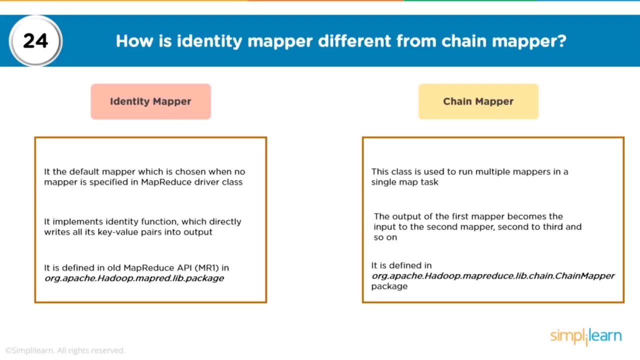 a shadow task would run on some other node, and whichever task completes first will be considered. this is what happens in your speculative execution. now, how is identity mapper different from chain mapper? now, this is where we are getting deeper into MapReduce concepts. so when you talk about 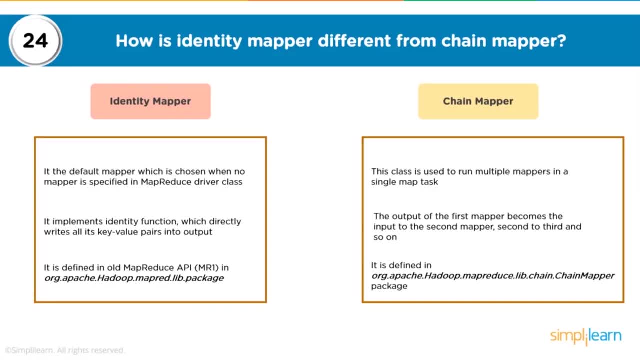 mapper identity mapper is the default mapper which is chosen when no mapper is specified in MapReduce driver class. so for every MapReduce program you would have a map class which is taking care of your mapping phase, which basically has a mapper function and which would run one or multiple map tasks. right, your programming, your program would. 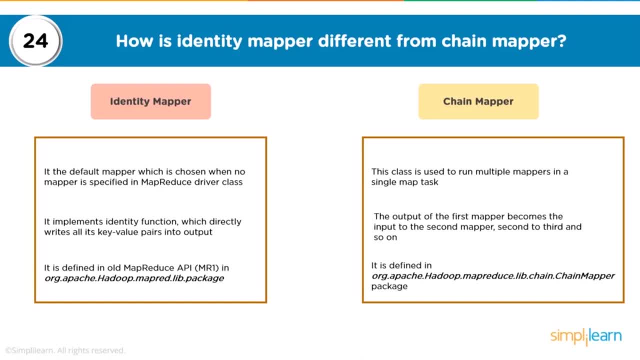 also have a reduce class, which would be running a reducer function which takes care of reduced tasks running on multiple nodes. now, if a mapper is not specified within your driver class, so driver class is something which has all information about your flow. what's your map class? what is your reduced class? what's your input format? what's. 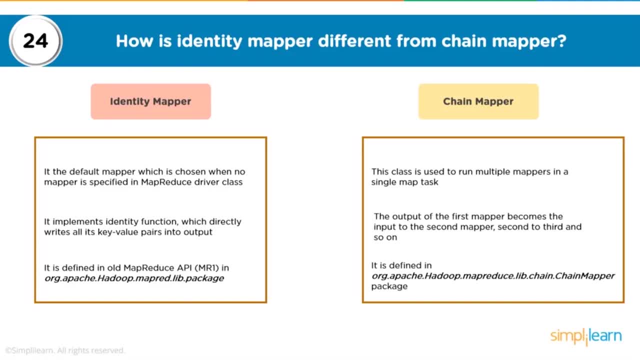 your output format, what are the job configurations and so on. so identity mapper is the default mapper which is chosen when no mapper class is mentioned in your driver class. it basically implements an identity function which directly writes all its key pairs into output and it was defined in old MapReduce API in this particular package. but when you talk about 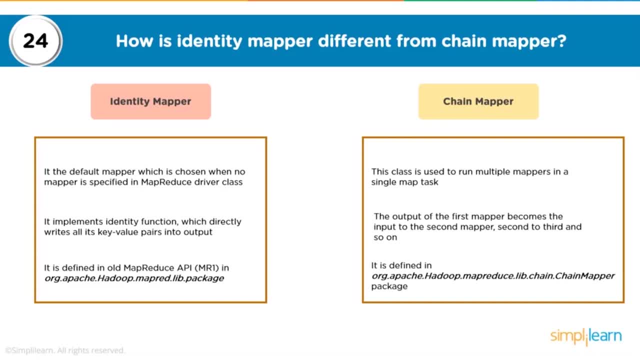 chaining mappers or chain mapper. this is basically a class to run multiple mappers in a single map task. or basically you could say multiple map tasks would run as a part of your processing. the output of first mapper would become as an input to second mapper and so on, and this can be defined in the 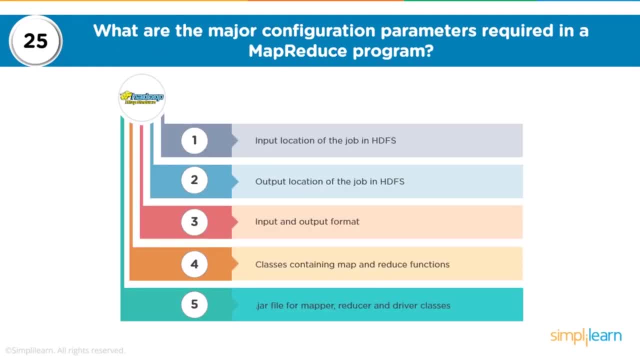 mapper or package. what are the major configuration parameters required in a MapReduce program? obviously we need to have the input location. we need to have the output location. so input location is where the files will be picked up from, and this would preferably on HDFS directory. output location is the path where your job output would be written by your MapReduce program. you. 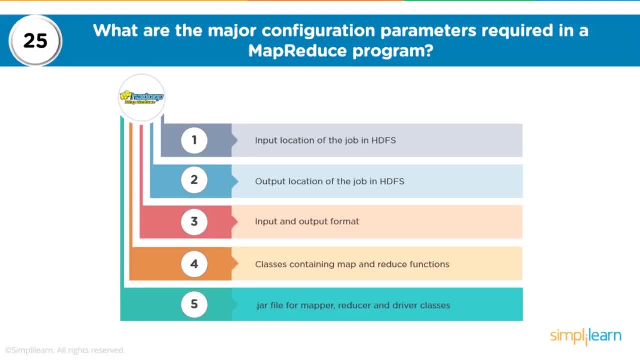 also need to specify input and output formats. if you don't specify, the defaults are considered. then we need to also have the classes which have your map and reduce functions. and if you intend to run the code on a cluster, you need to package your class in a jar file, export it to your cluster and 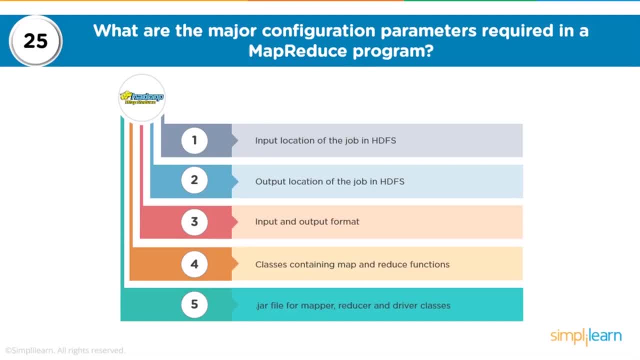 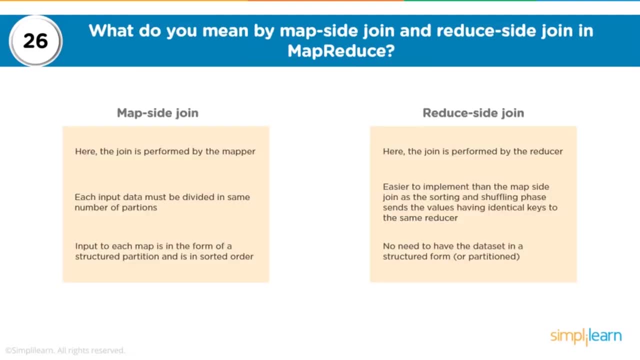 then this jar file would have your mapper reducer and driver classes. so these are important configuration parameters which you need to consider for a MapReduce program. now what is the difference or map site join and reduce site join. map site join is basically when the join is performed at the 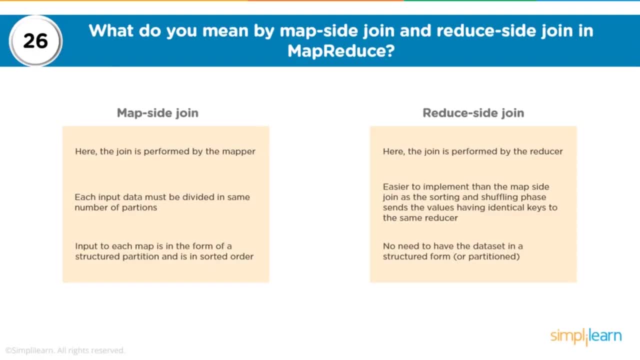 mapping level, or at the mapping phase, or is performed by the mapper. so each input data which is being worked upon has to be divided into same number of partitions. input to each map is in the form of a structured partition and is in sorted order. so map site join. you can understand it in a 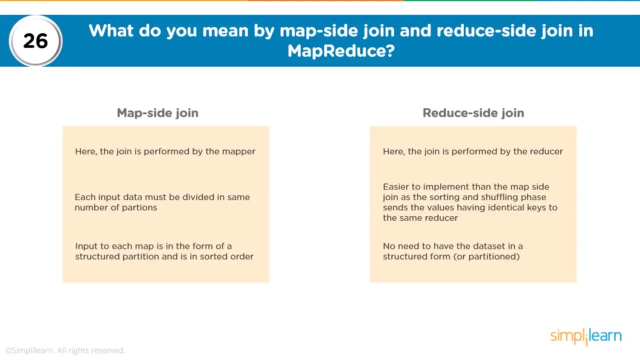 way that, if you compare it with rdbms concepts, where you had two tables which were being joined, it will always be advisable to give your bigger table as the left side table or the first table for your join condition, and it would be your smaller table on the left side and your bigger. 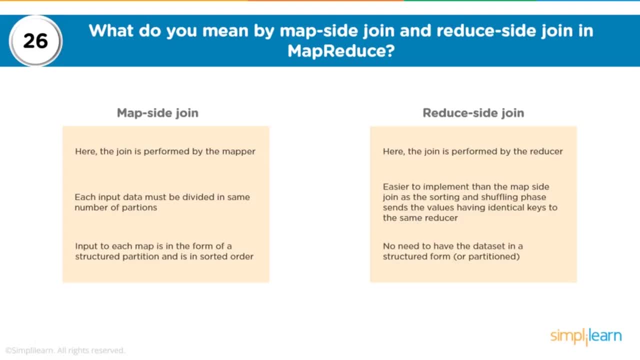 table on the right side, which basically means the smaller table could be loaded in memory and could be loaded in memory as well. so map site join is a kind of mechanism where input data is divided into same number of partitions. when you talk about reduce site join, here the join is performed by 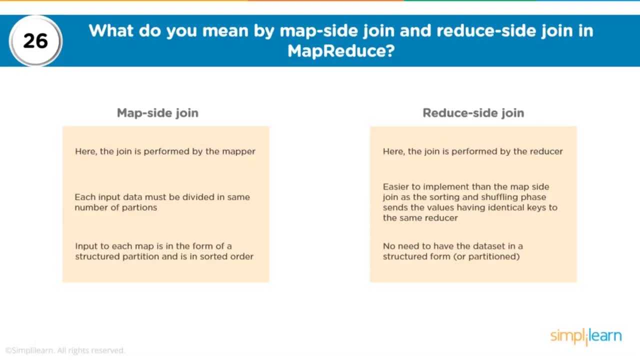 the reducer, so it is easier to implement than map site join, as all the sorting and shuffling will send the values, or send all the values having identical keys to the same reducer. so you don't need to have your data set in a structured form. so look into your map site join or reduce site join. 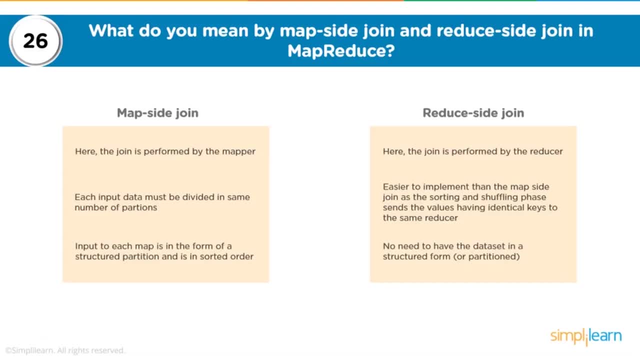 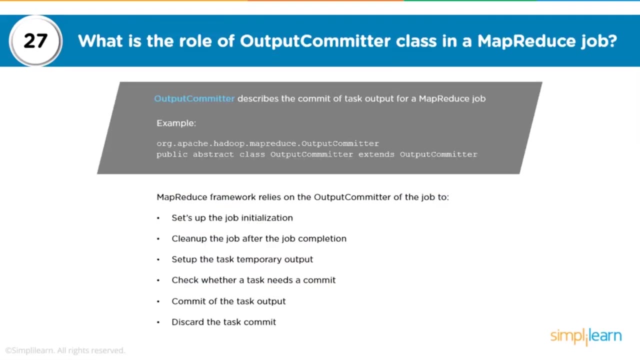 just to understand how MapReduce works. however, I would suggest not to focus more on this, because MapReduce is still being used for processing, but the amount of MapReduce based processing has decreased overall or across the industry. now, what is the role of output committer class in a 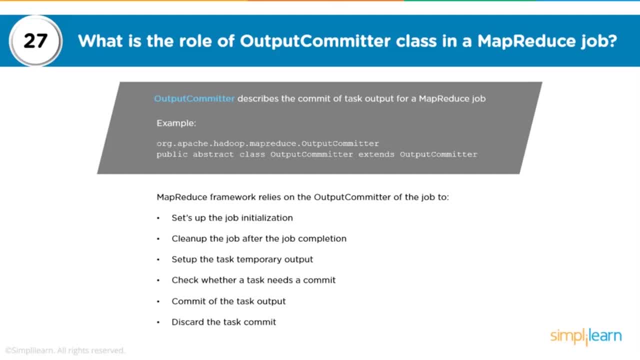 MapReduce job. so output committer, as the name says, describes the commit of task output for a MapReduce job. so we could have this as mentioned, or the Apache Hadoop MapReduce output committer. you could have a class which extends your output committer class. 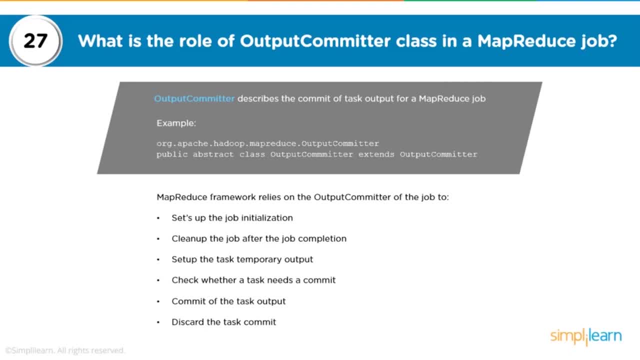 so MapReduce relies on this. MapReduce relies on the output committer of the job to set up the job initialization, cleaning up the job after the job completion. that means all the resources which were being used by a particular job: setting up the task, temporary output, checking whether a task 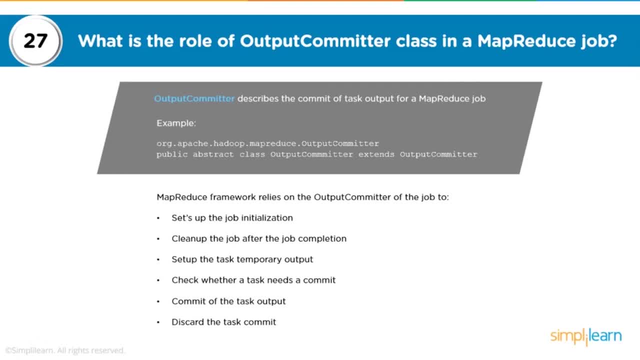 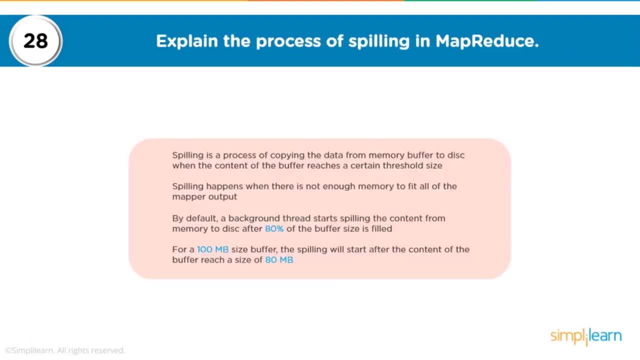 needs a commit committing the task output and discarding the task output. so this is the way. this is a very important class and can be used within your MapReduce job. what is the process of spilling in MapReduce? what does that mean? so spilling is basically a process of copying the 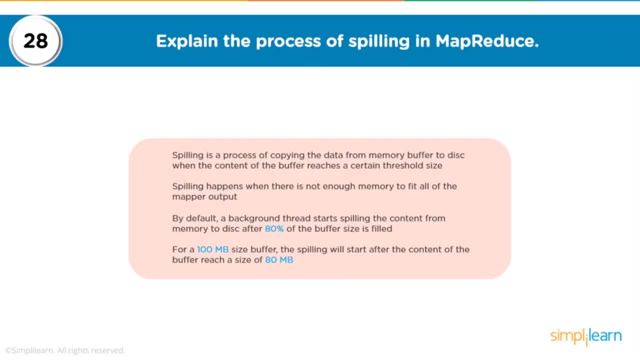 data from memory buffer to disk when, obviously, the buffer usage reaches a certain threshold. so if there is not enough memory in your buffer, in your memory, then the content which is stored in buffer or memory has to be flushed out. so this is a very important class and can be used within your MapReduce job. 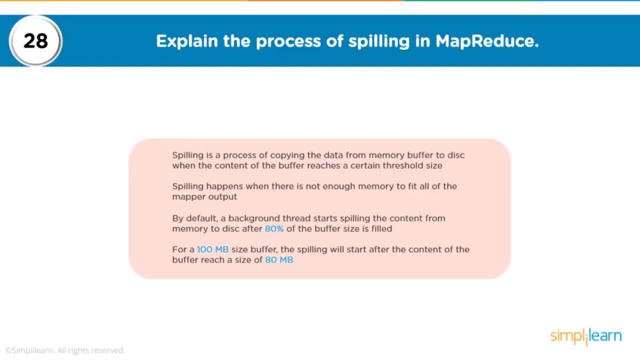 so, by default, a background thread starts spilling the content from memory to disk after 80 percent of buffer size is filled. now, when is the buffer being used? so when your MapReduce processing is happening, the data from data is being read from the disk loaded into the buffer. and then some 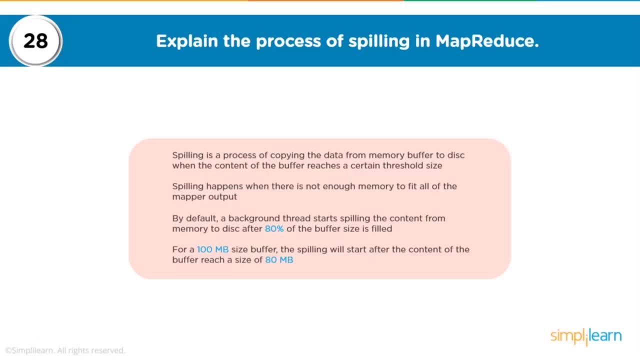 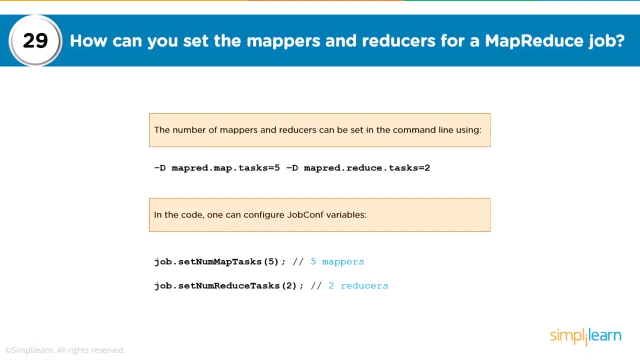 processing happens. same thing also happens when you are writing data to the cluster. so you can imagine: for a 100 megabyte size buffer, the spilling will start after the content of buffer reaches 80 megabytes. this is customizable. how can you set the mappers and reducers for a MapReduce job? so 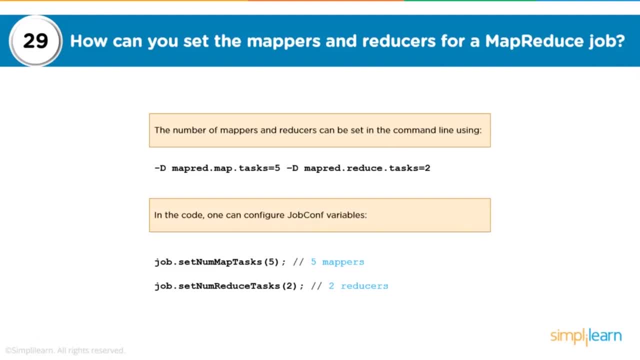 these are the properties. so number of mappers and reducers, as I mentioned earlier, can be customized. so by default, your number of map tasks depends on the split and number of reduced tasks depends on the partitioning phase which decides number of reduced tasks which would be used, depending on 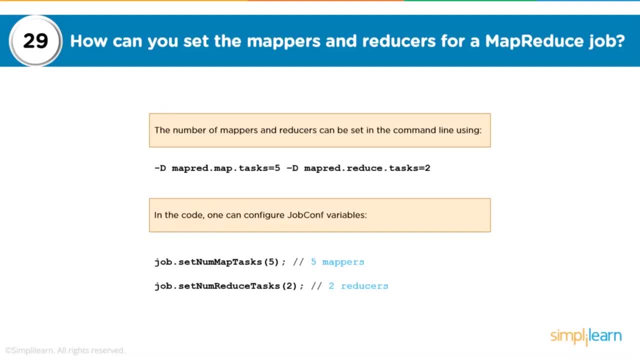 the keys. however, we can set these properties either in the config files or provide them on the command line, or also make them part of our code, and this can control the number of map tasks or reduced tasks which would be run for a particular job. let's look at one more interesting question: what happens when a node running a map task fails? 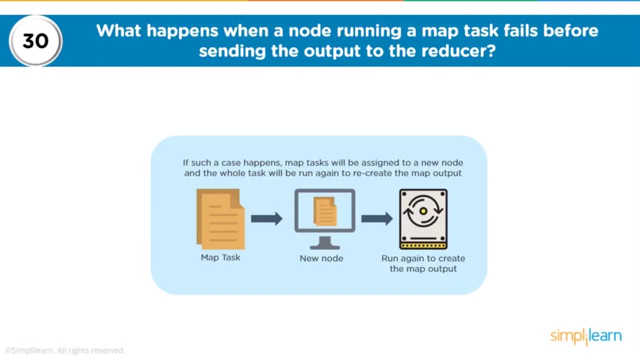 before sending the output to the reducer. so there was a node which was running a map task and we know that there could be one or multiple map tasks running on one or multiple notes and all the map tasks have to be completed before the further stages, that such as combiner or reducer. 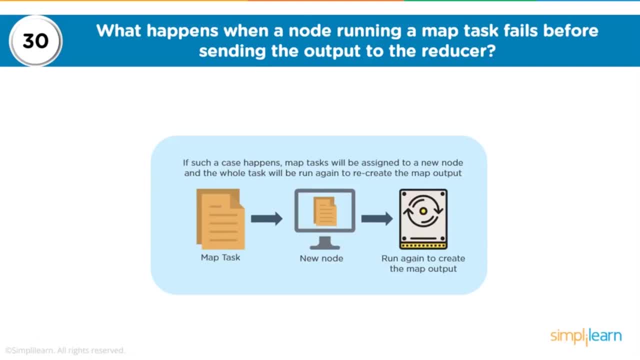 come into existence. so in a case if a node crashes where a map task was assigned to it, the whole task will have to be run again on some other node. so in Hadoop, version 2, yarn framework has a temporary Daven called application master. so your application master is taking care of. 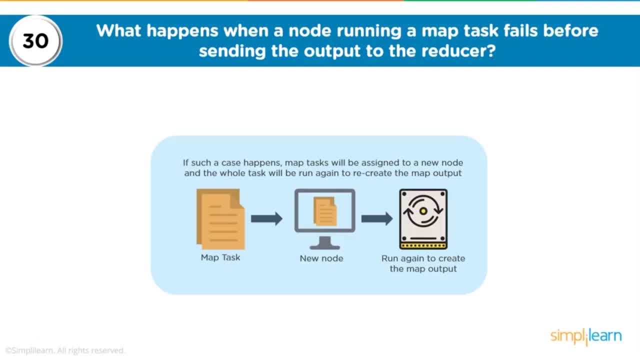 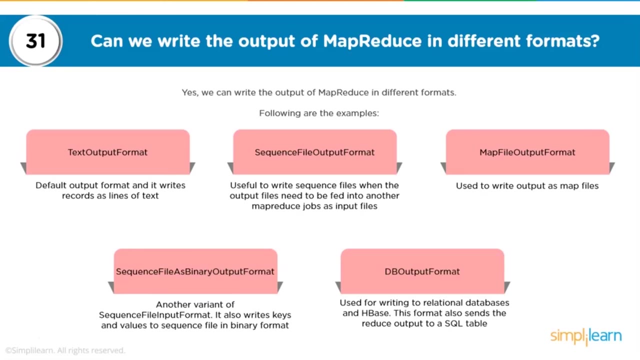 the execution of your application. and if a particular task on a particular node failed due to unavailability of note, it is the role of application master to have this task scheduled on some other node. now can we write the output of map, reduce in different formats? of course we can. 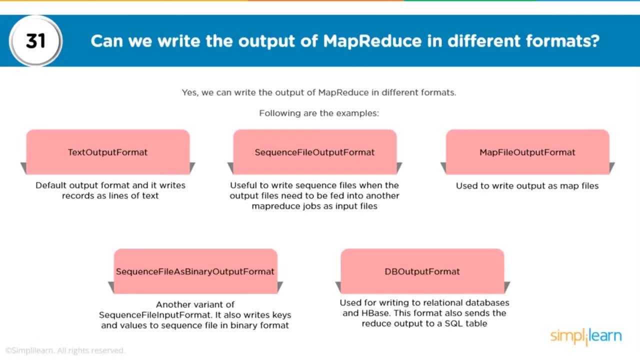 so Hadoop supports various input and output formats so you can write the output of map reduce in different formats so you could have the default format, that is, text output format, wherein records are written as line of text. you could have sequence file, which is basically to write sequence files, or your binary format files, where your output files need to be fed. 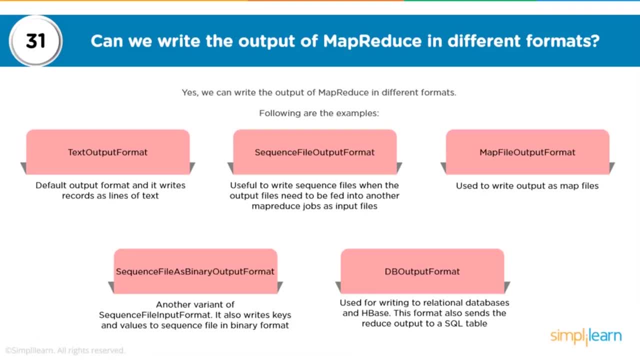 into another map, reduce jobs. you could go for a map file output format to write output as map files. you could go for a sequence file as a binary output format. so that's again a variant of your sequence file input format. it basically writes keys and values to a. 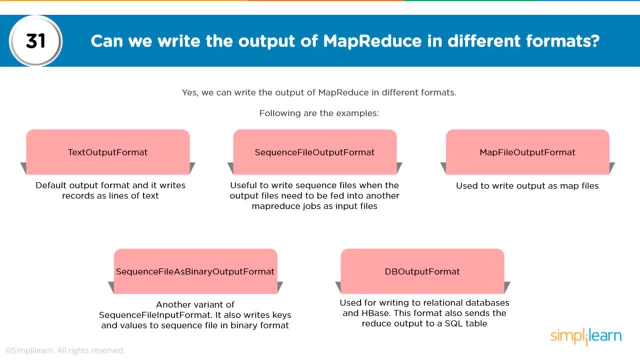 sequence file. so when we talk about binary format, we are talking about a non-human readable format, DV output format. now, this is basically used when you would want to write data, to say relational databases or say no SQL databases such as HBase. so this format also sends the reduce output to a 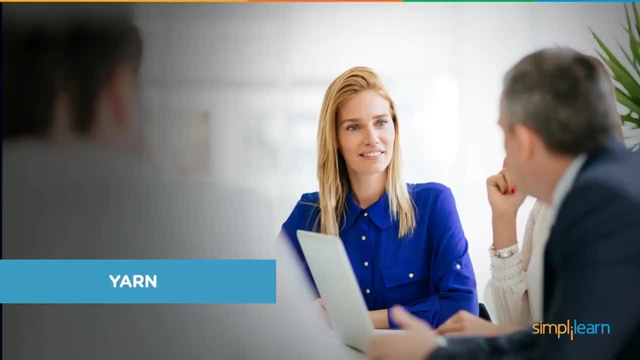 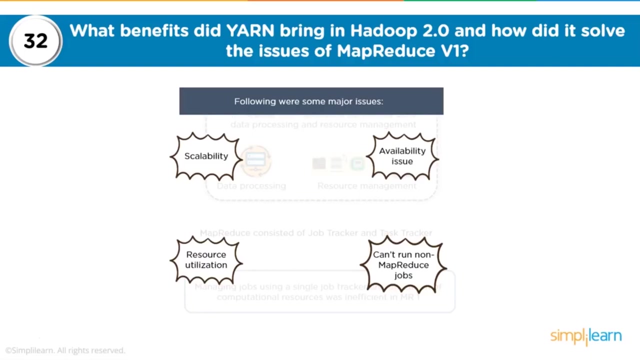 SQL table. now let's learn a little bit about yarn. yarn, which stands for yet another resource, it's the processing framework. so what benefits did yarn bring in Hadoop version 2 and how did it solve the issues of MapReduce version 1? so MapReduce version 1 had major issues when it 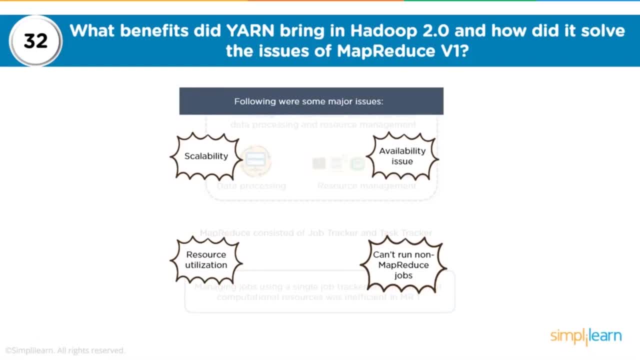 comes to scalability or availability because, sorry, in Hadoop version 1 you had only one master process for processing layer and that is your job tracker. so your job tracker was listening to all the task trackers which were running on multiple machines, so your job tracker was responsible for resource tracking and job scheduling. in yarn you still have a processing. 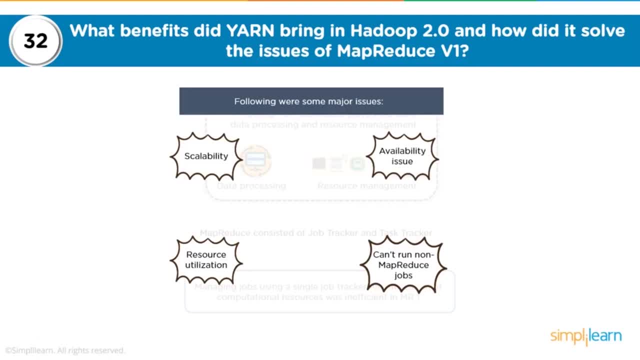 master, but that's called resource manager instead of job tracker. and now with Hadoop version 2, you could even have resource manager running in high availability mode. you have node managers which would be running on multiple machines, and then you have a temporary daemon called application master. 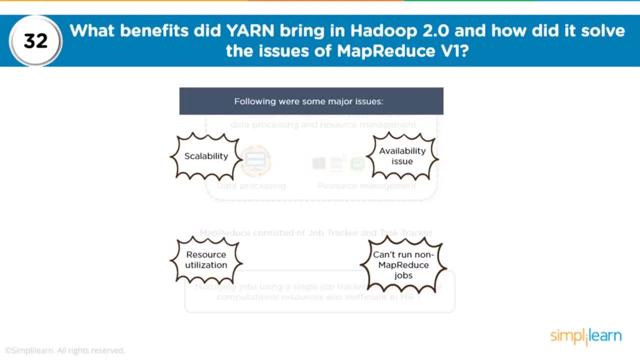 so in case of Hadoop version 2, your resource manager or master is only handling the client connections and taking care of tracking the resources. the jobs scheduling or basically taking care of execution across multiple nodes is controlled by application master till the application completes. so in yarn you can have different. 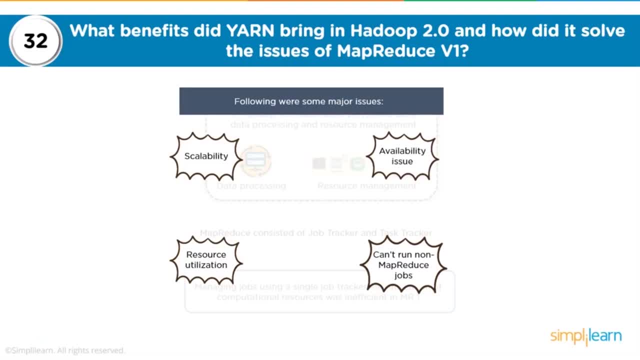 kind of resource allocations that could be done and there is a concept of container. so container is basically a combination of RAM and CPU cores. yarn can run different kind of workloads, so it is not just MapReduce kind of workload which can be run on Hadoop version 2, but you could have graph processing, massive parallel processing you. 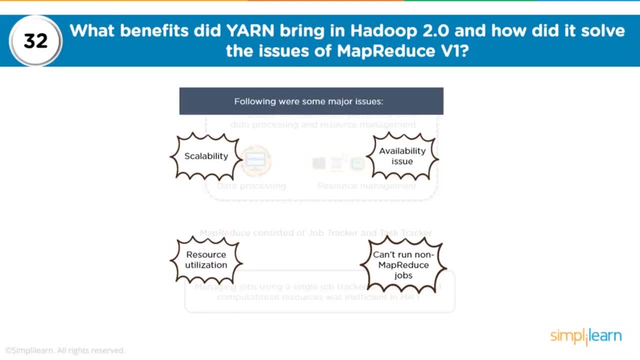 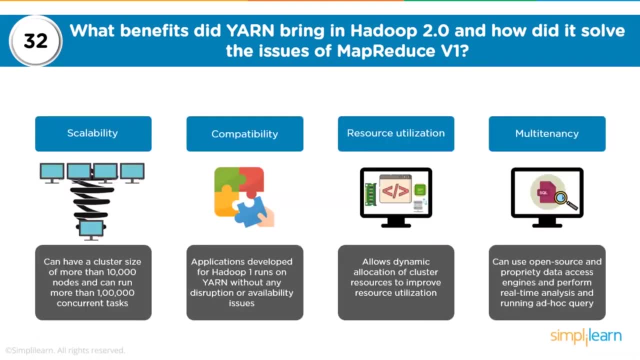 could have a real-time processing and huge processing applications could run on a cluster based on yarn. so when we talk about scalability, in case of your Hadoop version 2, you can have a cluster size of more than ten thousand nodes and can run more than hundred thousand concurrent tasks. and this is because, for every 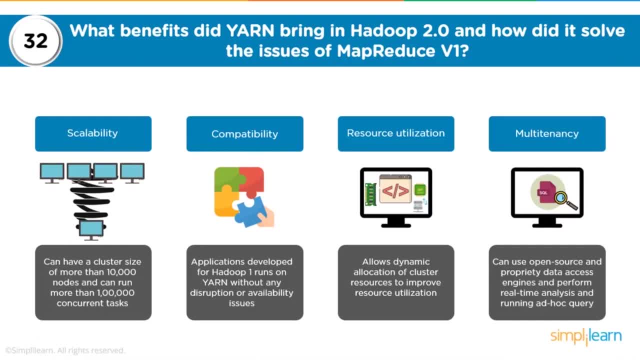 application which is launched, you have this temporary daemon called application master. so if I would have 10 applications running, I would have 10 app masters running taking care of execution of these applications across multiple nodes. compatibility: so Hadoop version 2 is fully compatible with whatever was developed as per Hadoop version 1 and all your processing needs. 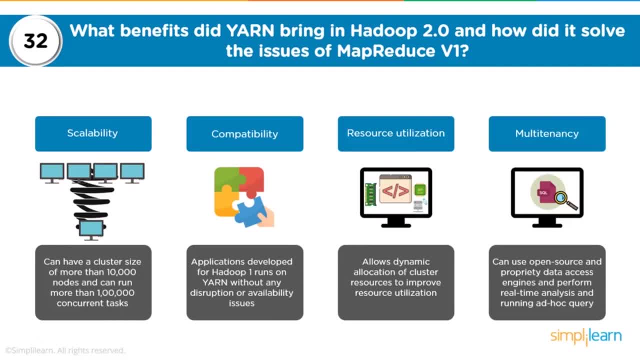 would be taken care by yarn. so dynamic allocation of cluster resources, taking care of different workloads, allocating resources across multiple machines and using them for execution- all that is taken care by yarn. multi-tenancy, which basically means you could have multiple users or multiple teams, you could have open source and proprietary data access engines, and all of these could be. 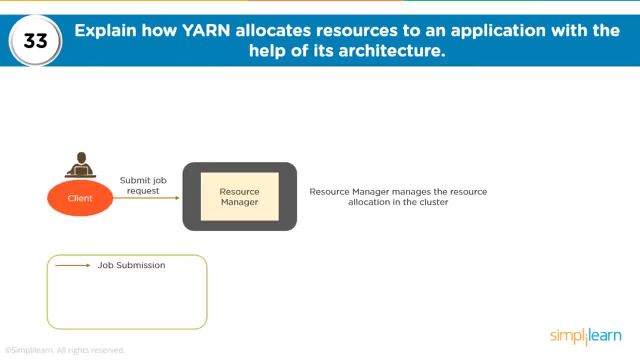 basically hosted in the same cluster. now, how does yarn allocate resources to an application with the help of its architecture? so, basically, you have a client or an application or an API which talks to resource manager. resource manager is, as I mentioned, managing the resource allocation in the cluster when you 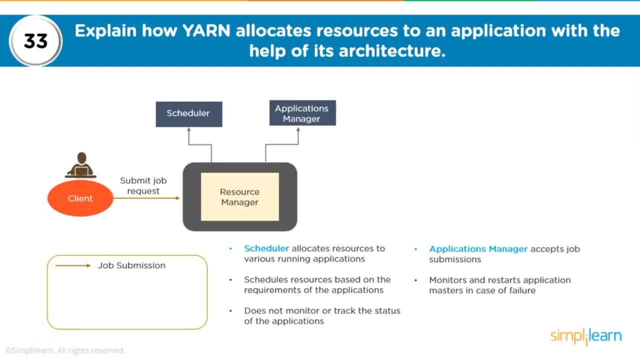 talk about resource manager, you have its internal two components: one is your scheduler and one is your applications manager. so when we say resource manager, being the master is tracking the resources, resource manager is the one which is negotiating the resources with slave. it is not actually resource manager who is doing it, but these. 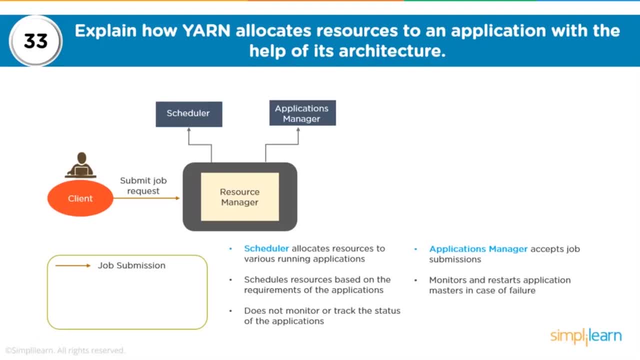 internal components. so you have a scheduler which allocates resources to various running applications. so scheduler is not bothered about tracking your resources or basically tracking your applications. so we can have different kind of schedulers, such as FIFO, which is first in, first out. you could have a fair scheduler or you could have a capacity scheduler and these schedulers basically. 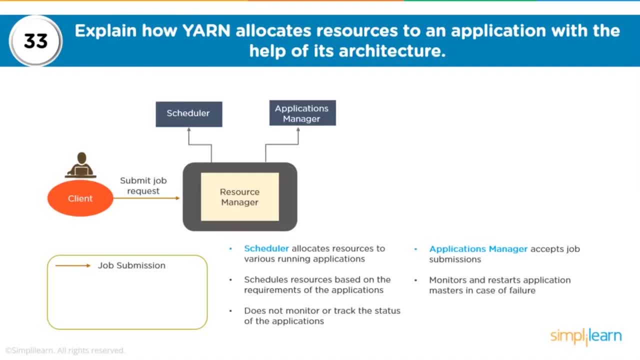 control how resources are allocated to multiple applications when they are running in parallel. so there is a queue mechanism. so scheduler will schedule resources based on requirements of application, but it is not monitoring or tracking the status of applications. your applications manager is the one which is accepting the job. 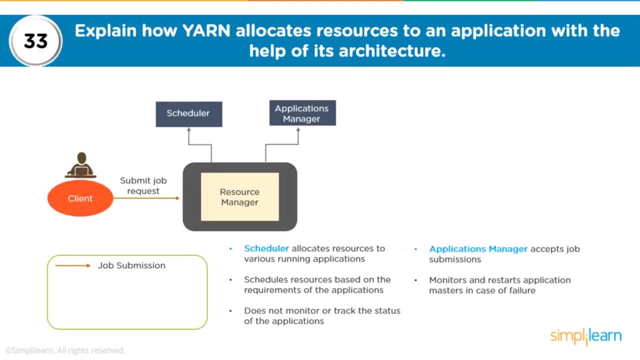 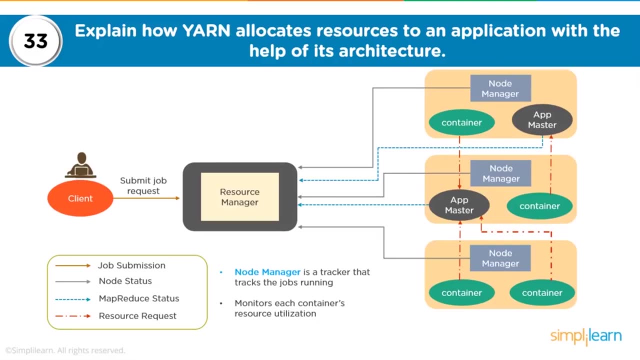 submissions, it is monitoring and restarting the application Masters, so it's application manager which is basically then launching a application master which is responsible for an application. so this is how it looks. so whenever a job submission happens, we already know that resource manager is aware of the resources which are available with every node manager. so on every node which has 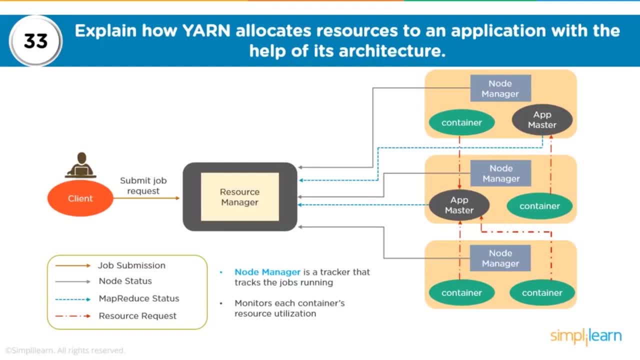 fixed amount of RAM and CPU course. some portion of resources, that is, your RAM and CPU course, are allocated to node manager. now resource manager is already aware of how much resources are available across nodes. so whenever a client request comes in, resource manager will make a request to node manager. it will basically request: 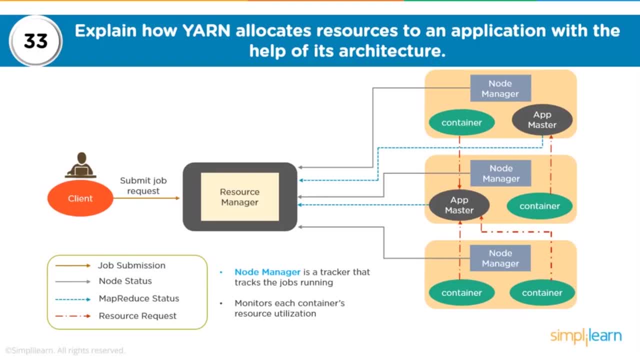 node manager to hold some resources for processing. node manager would basically approve or disapprove this request of holding resources and these resources, that is, a combination of RAM and CPU cores, are nothing but containers. we can allocate containers of different sizes within yarn hyphen site file, so your node manager, based on a request from resource manager, guarantees the container. 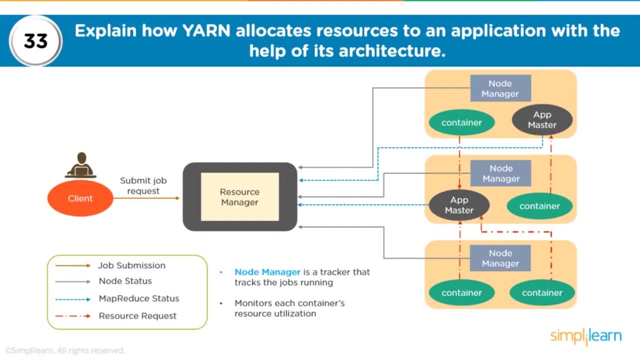 which would be available for processing. that's when your resource manager starts a temporary ится, a temporary demand called application master, to take over this process. that's when your resource manager starts a temporary demand called application master, to take over this process, care of your execution. so your app master, which was launched by resource manager. or we can say: 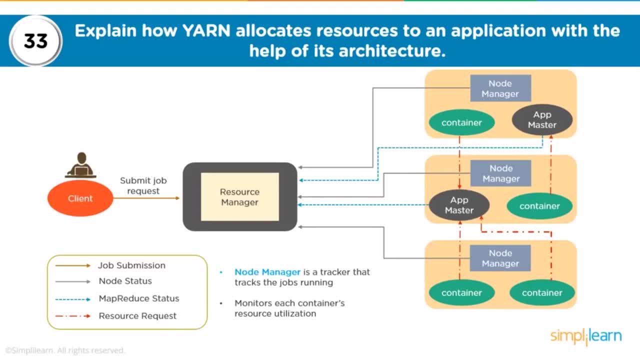 internally by applications manager will run in one of the containers, because application master is also a piece of code, so it will run in one of the containers and then other containers will be utilized for execution. this is how yarn is basically taking care of your allocation. your application master is managing resource needs. it is the one which is interacting with scheduler. 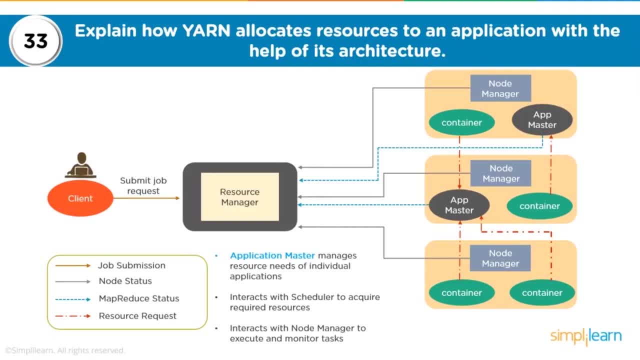 and if a particular node crashes, it is the responsibility of app master to go back to the master, which is resource manager, and negotiate for more resources. so your app master will never, ever negotiate resources with node manager directly. it will always talk to resource manager and resource manager is the one which negotiates. 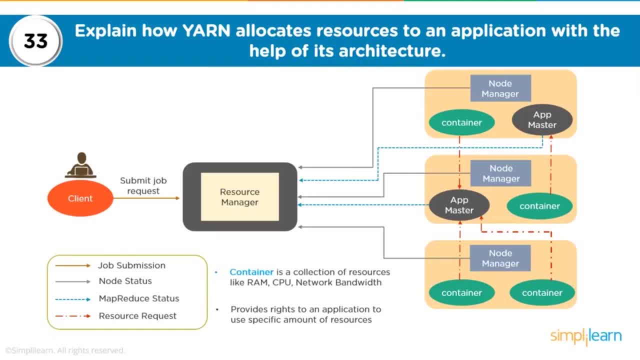 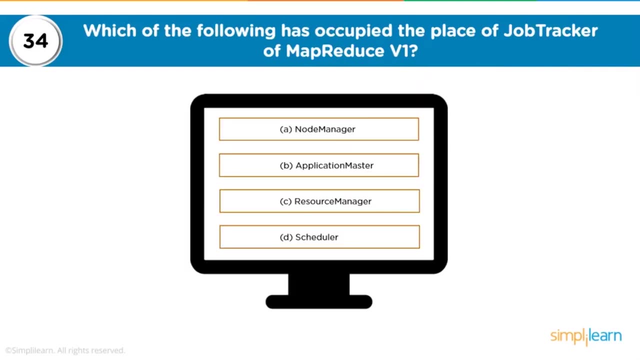 the resources container, as I said, is a collection of resources like your RAM, CPU, network bandwidth, and your container is allocated based on the availability of resources on a particular node. so which of the following has occupied the place of a job tracker of MapReduce? so it is your. 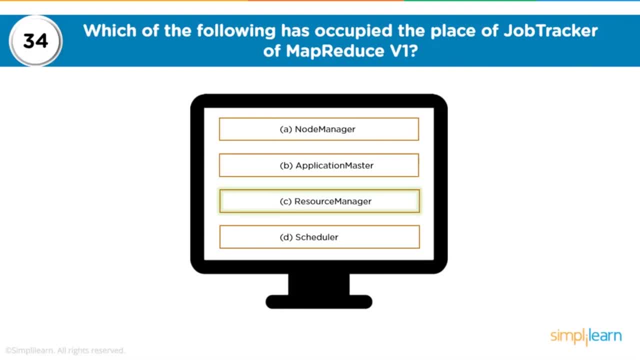 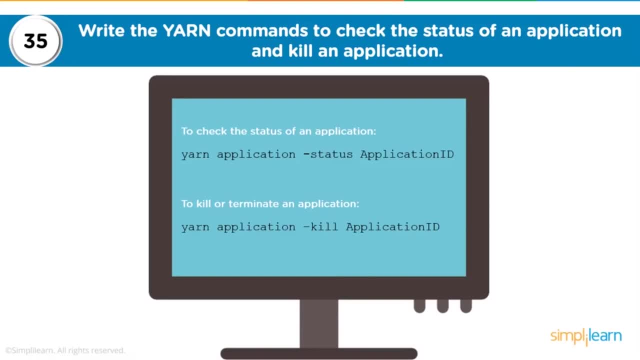 resource manager. so resource manager is the name of the master process in Hadoop version 2. now if you would have a question, please ask me in the comment section below and I will answer it in the next class. so we have to write yarn commands to check the status of an application, so we could. 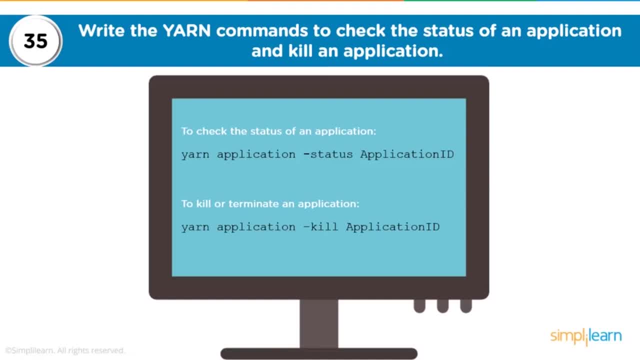 just say yarn, application minus status, and then the application ID and you could kill it also from the command line. remember your yarn has a UI and you can even look at your applications from the UI. you can even kill your applications from the UI, however, knowing the command line commands would. 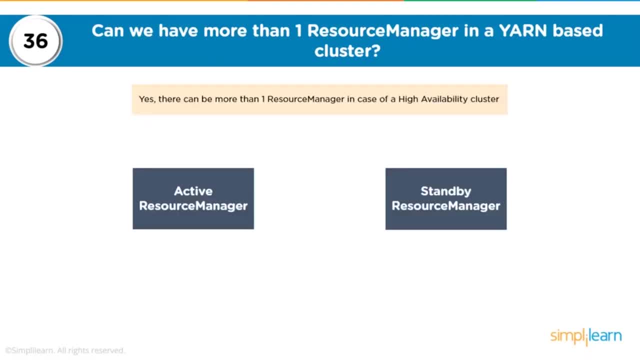 be very useful. can we have more than one resource manager in a yarn based cluster? yes, we can. that is what Hadoop version 2 allows us to have, So you can have a high availability yarn cluster where you have an active and standby and the coordination is taken care by your zookeeper At a particular 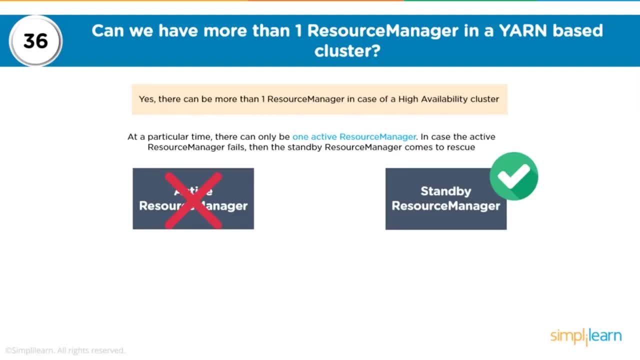 time. there can only be one active resource manager and if active resource manager fails, your standby resource manager comes and becomes active. However, zookeeper is playing a very important role. Remember, zookeeper is the one which is coordinating the server state and it is doing the election of active to standby failover. What are the different schedulers? 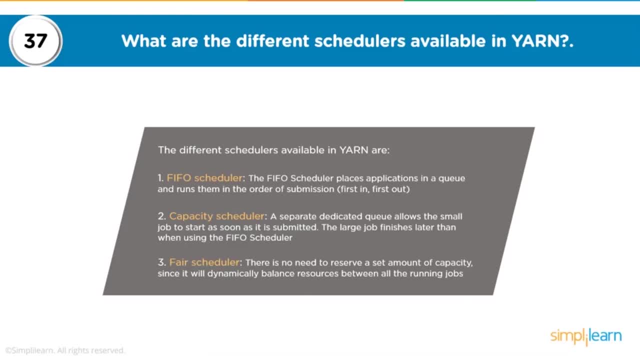 available in yarn. So you have a FIFO scheduler that is first in, first out, and this is not a desirable option because in this case a longer running application might block all other small running applications. Your capacity scheduler is basically a scheduler where dedicated queues are created and they have fixed amount of resources, So you can. 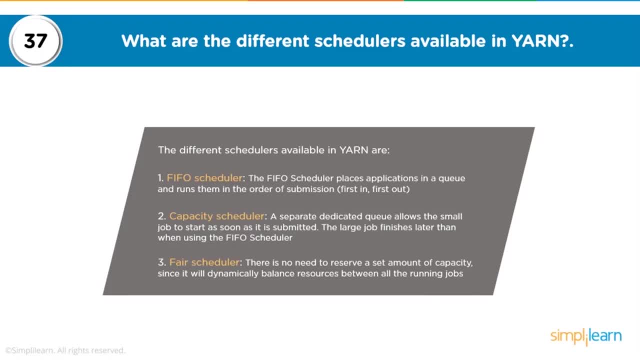 have multiple applications accessing the cluster at the same time and they would be using their own queues and the resources allocated to them. If you talk about fair scheduler, you don't need to have a fixed amount of resources. you can just have a percentage and you could. 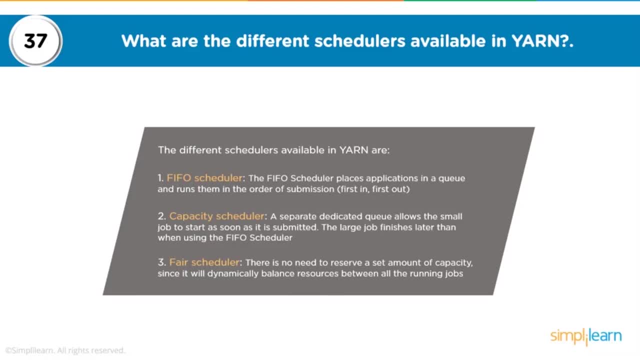 decide what kind of fairness is to be followed, which basically means that if you were allocated 20 gigabytes of memory, however, the cluster has 100 gigabytes and the other team was assigned 80 gigabytes of memory, then you have 20 percent access to 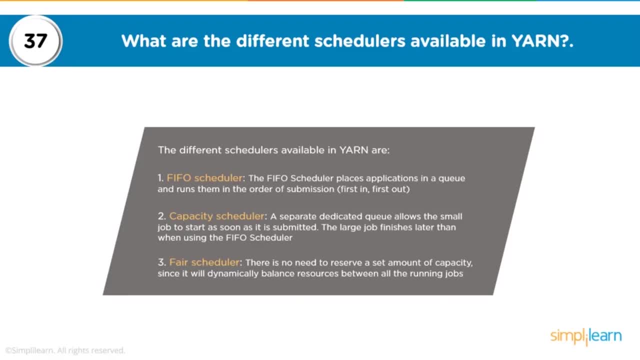 the cluster and other team has 80 percent. However, if the other team does not come up or does not use the cluster, in a fair scheduler you can go up to maximum of 100 percent of your cluster. To find out more information about your schedulers, you could either look: 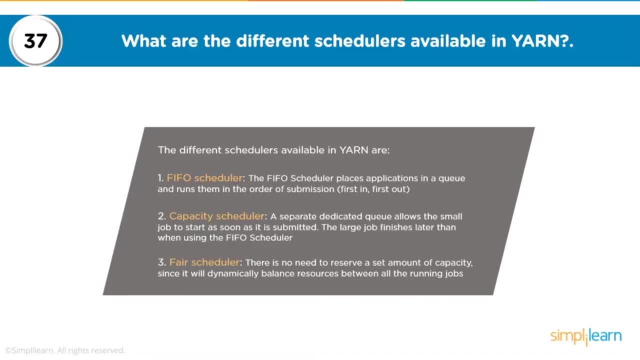 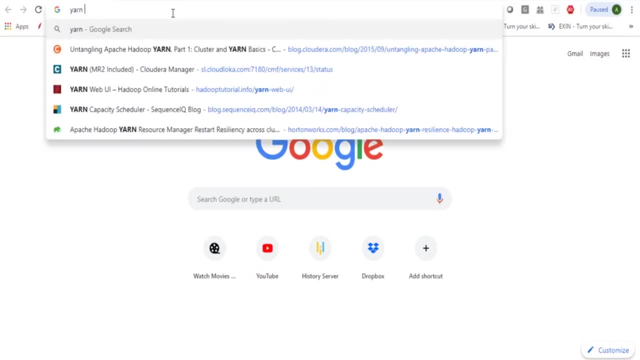 in Hadoop definitively, or you could look in Hadoop Hadoop definitive guide. or what you could do is you could just go to Google and you could type, for example, yarn scheduler- let's search for yarn scheduler- and then you can look in Hadoop definitive guide. and so this is your Hadoop definitive guide, and it beautifully. 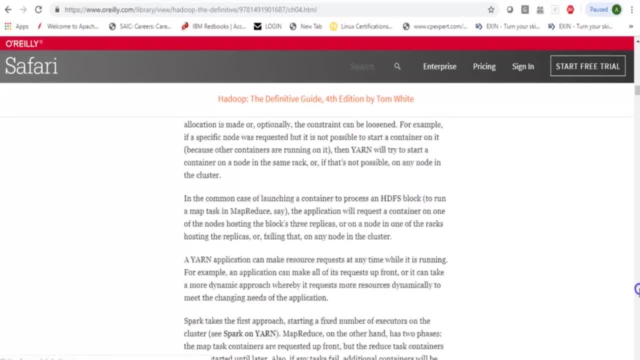 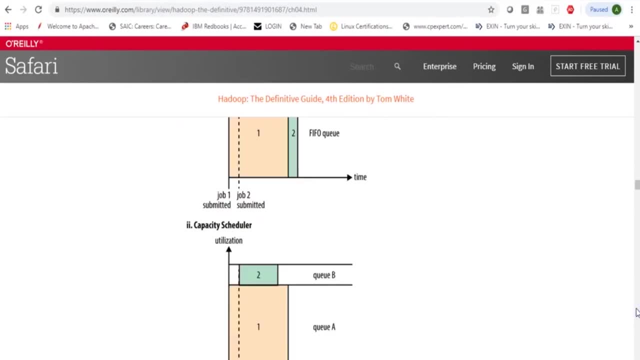 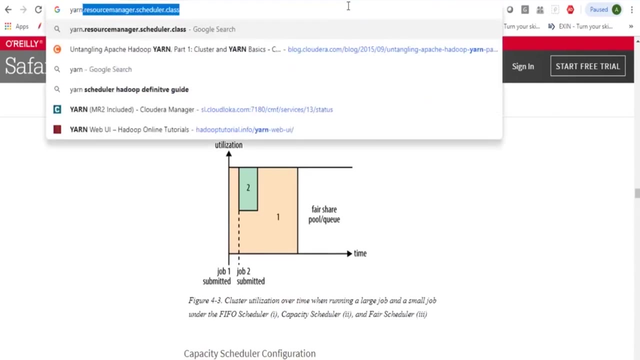 explains about your different schedulers. how do multiple applications run, and that could be in your FIFO kind of scheduling, It could be in capacity scheduler or it could be in a fair scheduling. So have a look at this link. it's a very good link. you can also search for yarn untangling and this is a blog. 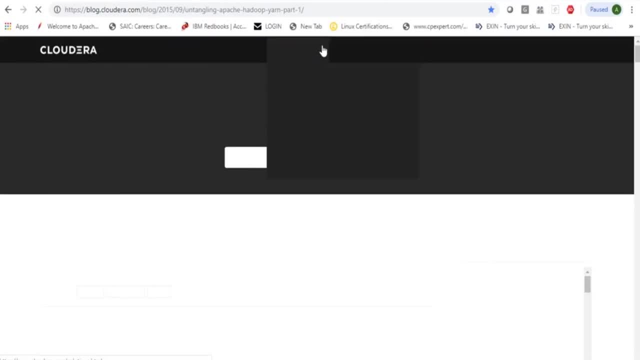 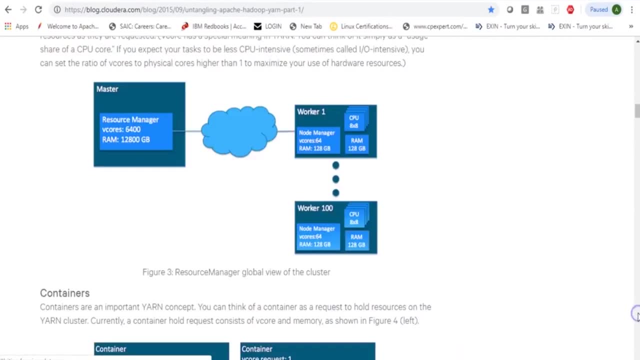 of four, or this is a series of four blogs where it's beautifully explained about your yarn, how it works, how the resource allocation happens, what is a container and what runs within the container, so you can scroll down, you can be reading through this and you can then also search for part two of it for your Hadoop definitive guide. 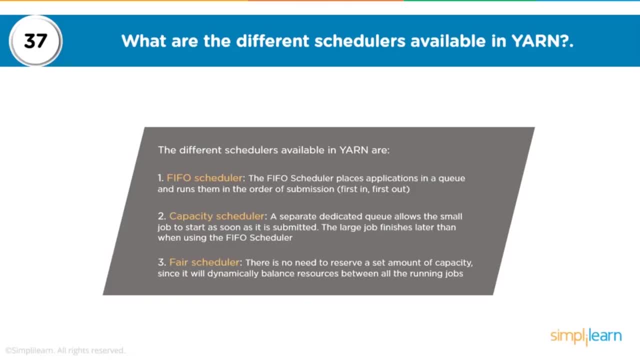 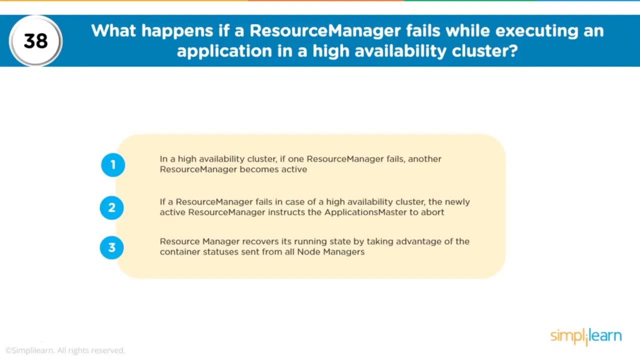 Which talks about allocation and so on. so, coming back, we basically have these schedulers. what happens if a resource manager fails while executing an application in a high availability cluster? so, in a high availability cluster, we know that we would have two resource managers: one being active, one being standby, and zookeeper which is keeping a track of the server states. 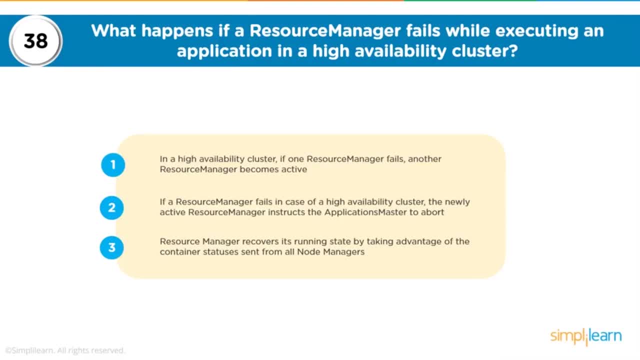 so if a rm fails, in case of high availability, the standby will not be able to run because the server will be elected as active and then basically, your resource manager or the standby would become the active one, and this one would instruct the application master to abort in. 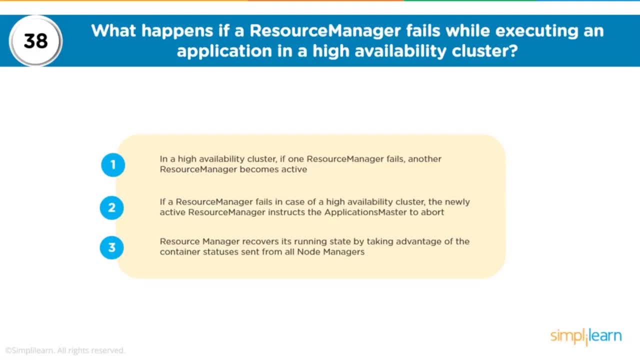 the beginning. then your resource manager recovers its running state. so there is something called as RM State store where all the applications which are running their status is stored. so resource manager recovers its running state by looking at your state store, by taking a advantage of container statuses, and then continues to take care of your processing, Now in a cluster. 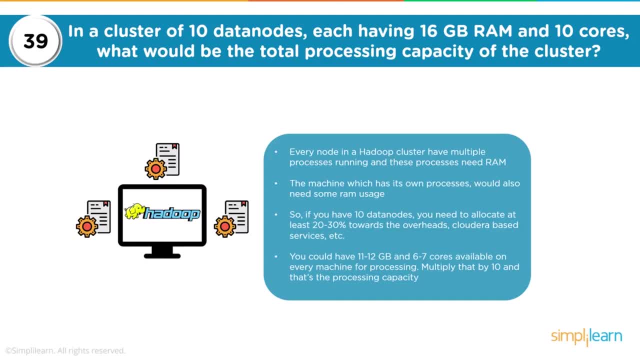 of 10 data nodes, each having 16 GB and 10 cores, what would be total processing capacity of the cluster? Take a minute to think: 10 data nodes, 16 GB RAM per node, 10 cores. So if you mention, 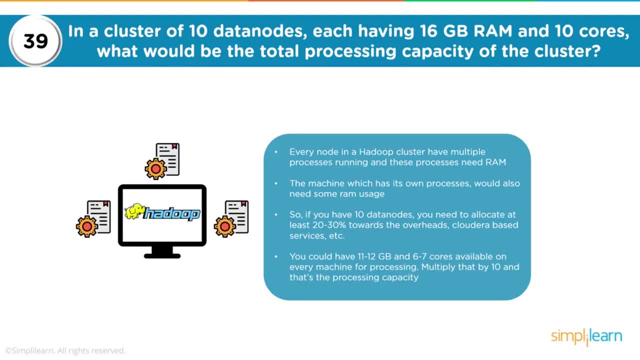 the answer as 160 GB RAM and 100 cores, then you went wrong. Now think of a cluster which has 10 data nodes, each having 16 GB RAM and 10 cores. Remember, on every node in a Hadoop cluster you 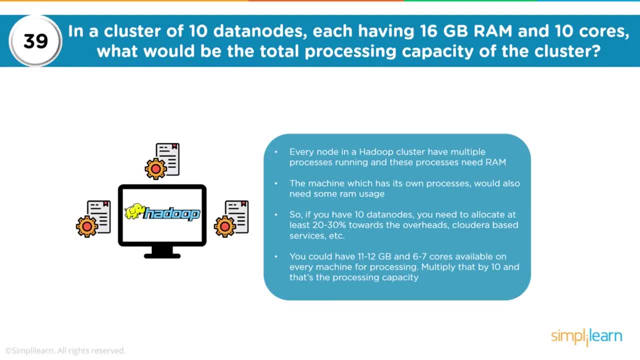 would have one or multiple processes running. Those processes would need RAM. The machine itself, which has a Linux file system, would have its own processes. So that would also be having some RAM usage, which basically would have 16 GB RAM per node. So if you think of a cluster of 10 data nodes, 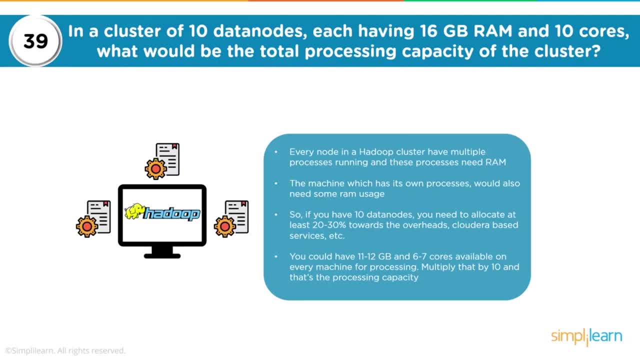 it basically means that if you talk about 10 data nodes, you should deduct at least 20 to 30 percent towards the overheads, towards the cloud database services, towards the other processes which are running, And in that case I could say that you could have 11 or 12 GB available on every. 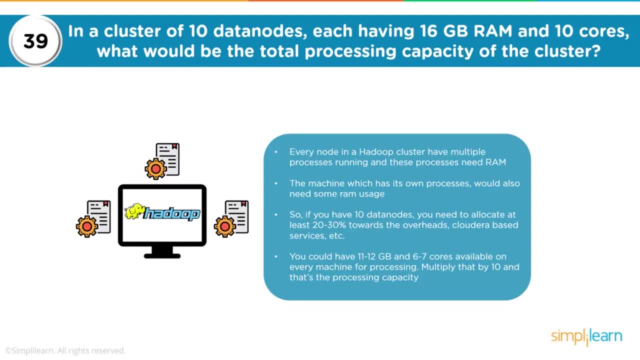 machine for processing and say 6 or 7 cores, Multiply that by 10 and that's your processing capacity. Remember, the same thing applies to the disk usage also. So if somebody asks you, in a 10 data node cluster where each machine has 20 TB of disks, what is my total storage capacity? 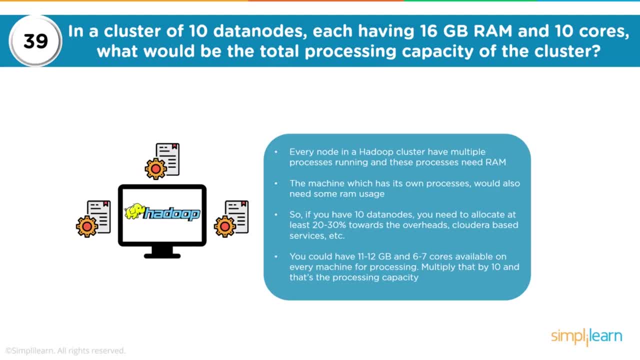 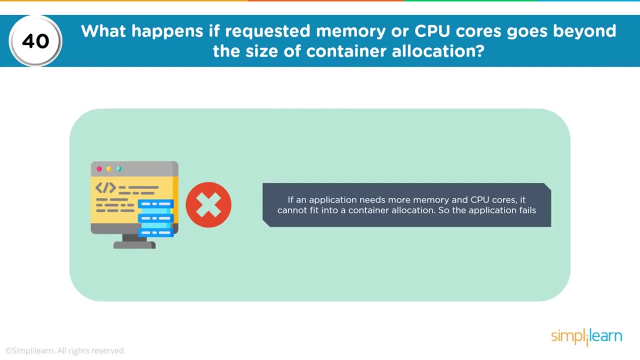 available for HDFS. So the answer would not be 200.. You have to consider the overheads And this is basically which gives you your processing capacity. Now let's look at one more question. So what happens if requested memory or CPU cores beyond, or goes beyond the size of container? Now 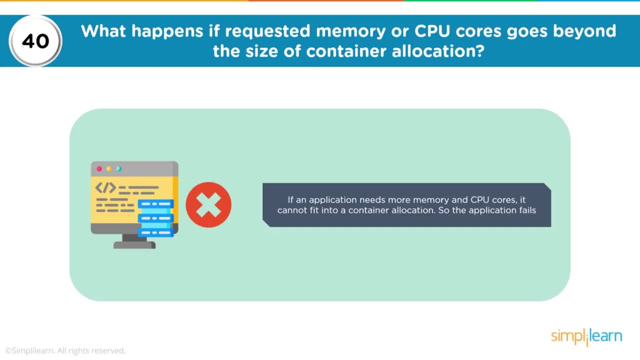 you can have your configurations which can say that in a particular data node which has 100 GB RAM, I could allocate, say, 50 GB for the processing Out of 100 cores. I could say 50 cores for processing. So if you have 100 GB RAM and 100 cores, you could ideally allocate 100 for. 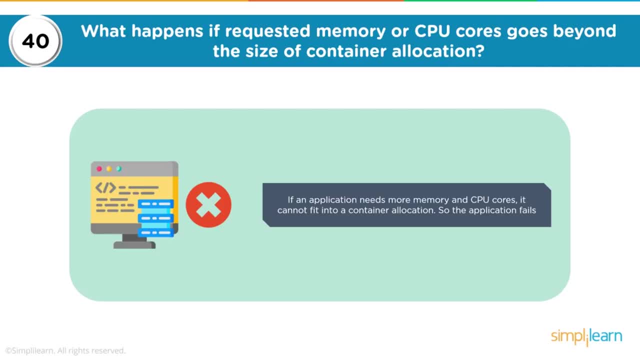 processing. but that's not ideally possible. So if you have 100 GB RAM, you would go for 50 GB, And if you have 100 cores, you would go for 50 cores. Now, within this RAM and CPU cores, you have the concept of containers. So container is a combination. 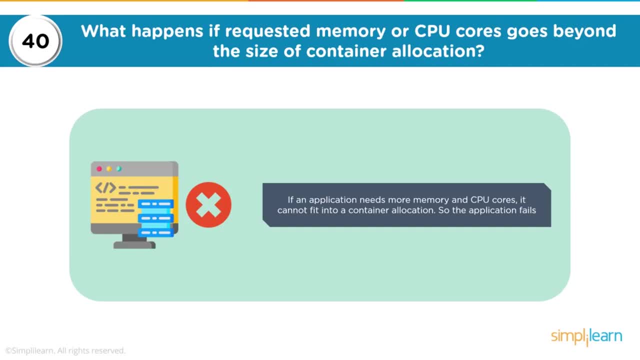 of RAM and CPU cores So you could have a minimum size container and maximum size container Now, at any point of time. if your application starts demanding more memory or more CPU cores and this cannot fit into a container location, your application will fail. Your application will fail. 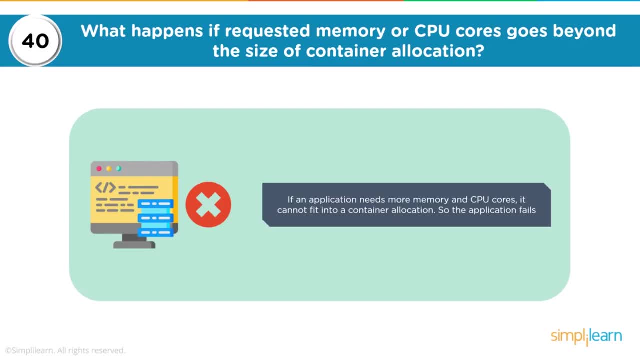 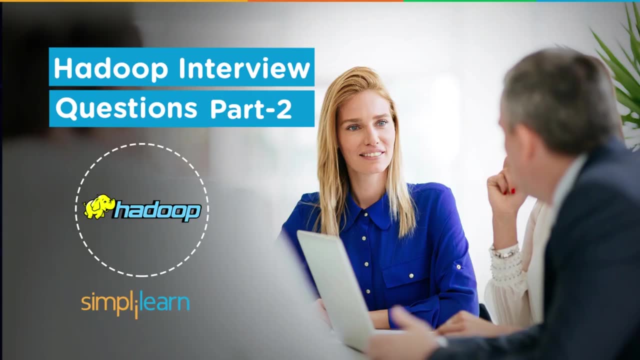 because you have requested for a memory or a combination of memory and CPU cores which is more than the maximum container size. Now here we will discuss on Hive, PEG, HBase and these components of Hadoop which are being used in the industry for various use cases. 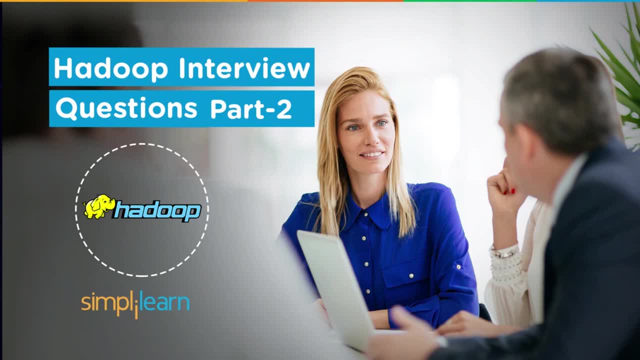 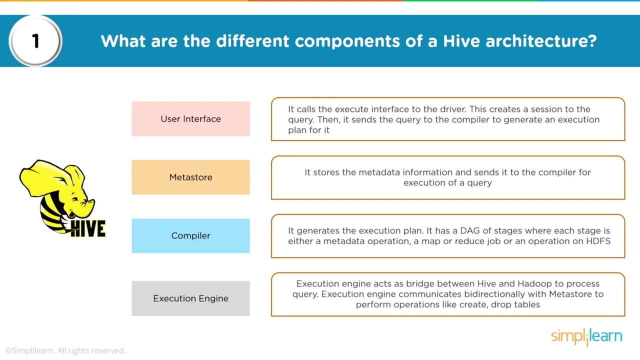 Let's look at some questions here and let's look how you should prepare for them. So first of all, we will learn on Hive, which is a data warehousing package. So the question is: what are the different components of Hadoop? 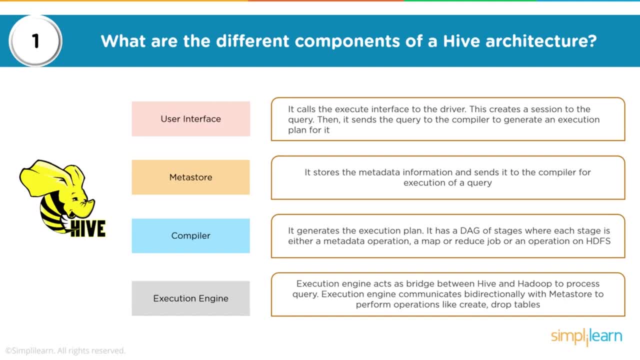 Hive is a data warehousing package of a Hive architecture. Now when we talk about Hive, we already know that Hive is a data warehousing package which basically allows you to work on structured data or data which can be structurized. So normally people are well versed with querying or basically processing the data using SQL queries. A lot of people come from database backgrounds and they would find it comfortable if they know structured query language. 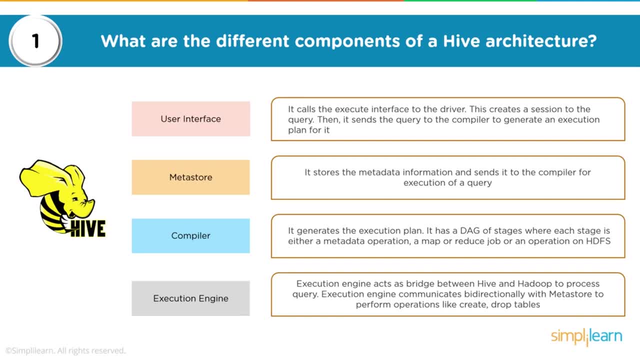 Hive is one of the data warehousing package which sites within a Hadoop ecosystem. It uses Hadoop's distributed file system to store the data and it uses RDBMS usually to store the metadata, Although metadata can be stored locally also. So what are? 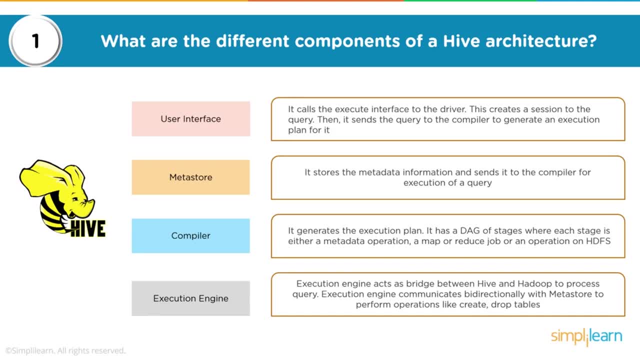 the different components of an Hive architecture, So it has a user interface. So user interface calls the execute interface to the driver. This creates a session to the query and then it sends the query to the compiler to generate an execution plan for it. Usually, whenever Hive is set up, it 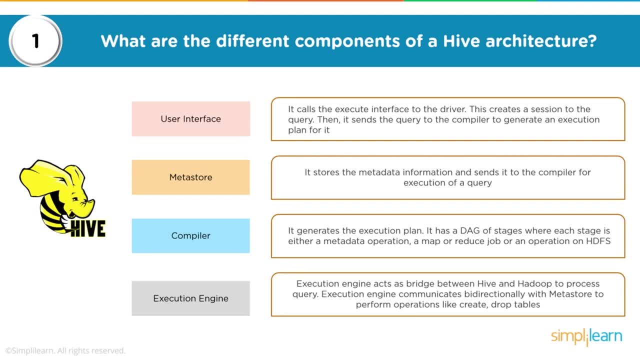 would have its metadata stored in an RDBMS. Now, to establish the connection between RDBMS and Hadoop, we need ODBC or JDBC connector jar file, and that connector jar file has a driver class. Now this driver class is mandatory to create a connection between Hive and Hadoop, So user interface. 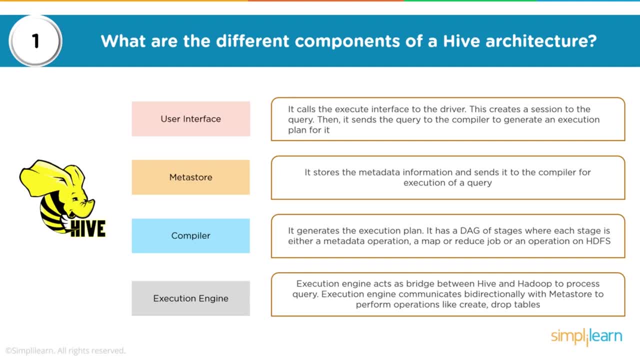 creates a connection between Hive and Hadoop. So user interface calls the execute interface to the query and it creates this interface using the driver. Now we have meta store. Meta store stores the metadata information. So any object which you create, such as database table, indexes. 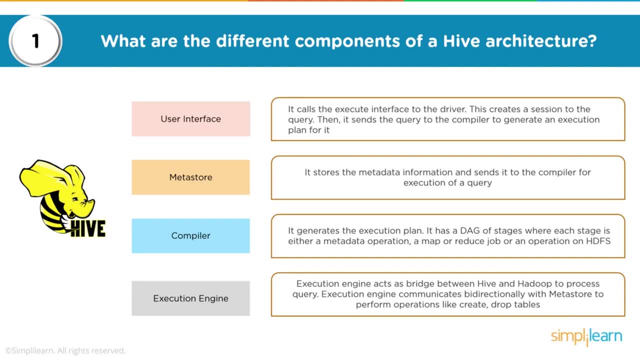 their metadata is stored in meta store and usually this meta store is stored in an RDBMS so that multiple users can connect to Hive. So your meta store stores the metadata information and sends that to the compiler for execution of a query. What does the compiler do? 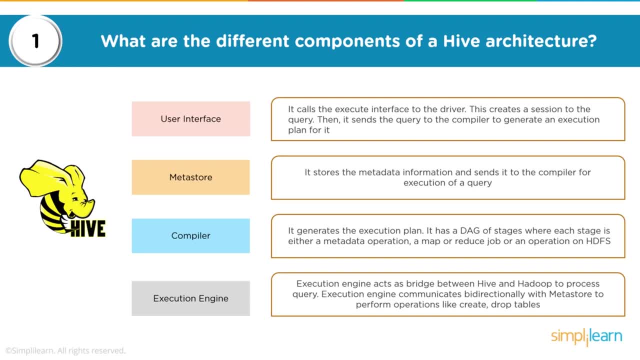 It generates the execution plan. It has a DAG. Now DAG stands for direct acyclic graph, So it has a DAG of stages, where each stage is either a metadata operation, a map, or reduce job or an operation on SDFS. And finally we have execution engine that acts as a bridge between Hive and Hadoop to process. 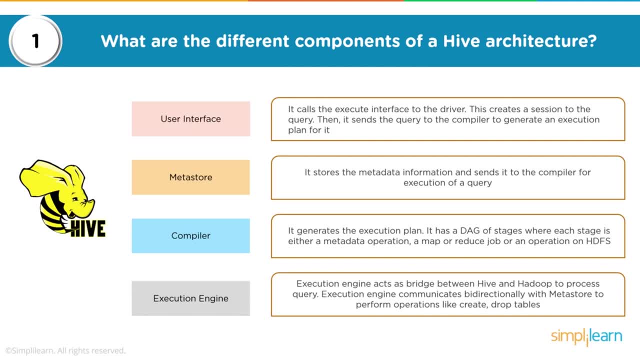 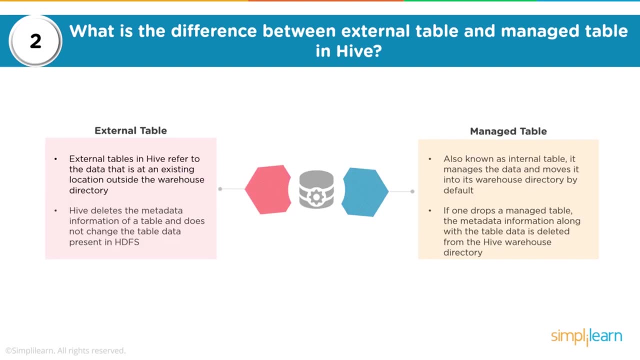 the query. So execution engine communicates bi-directionally with meta store to perform operations like create or drop tables. So these are the operations that are used to process the query. These are four important components of Hive architecture. Now what is the difference between external table and managed table in Hive? So we have various kinds of table in Hive, such as: 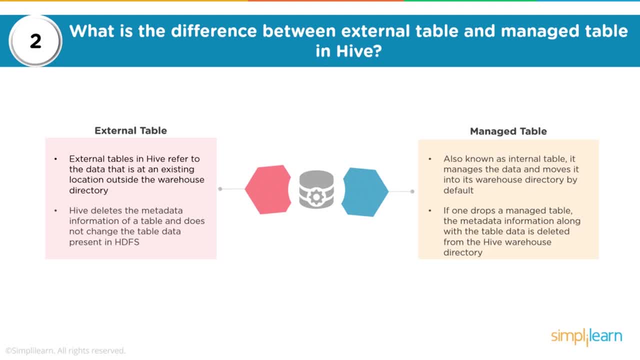 external table. managed table partition table. The major difference between your managed and external table is in respect to what happens to the data if the table is dropped. Usually, whenever we create a table in Hive, it creates a table that is dropped. So if the table is dropped, 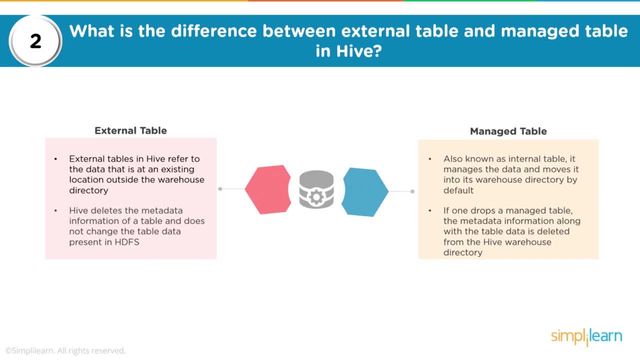 a managed table, or we could also call that as an internal table. Now, this manages the data and moves it into warehouse directory by default. Whether you create a managed table or external table, usually the data can reside in Hive's default warehouse directory, or it could be. 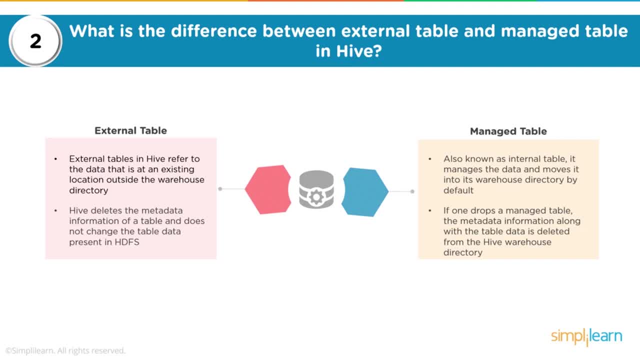 residing in a location chosen. However, when we talk about managed table, if one drops a managed table, not only the metadata information is deleted, but the table's data is also deleted from SDFS. If we talk about external table, it is created with an external keyword explicitly. 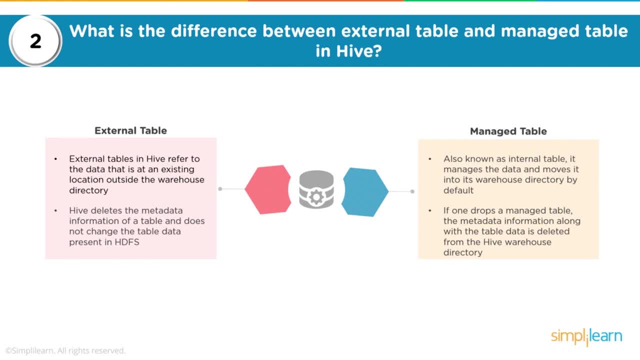 and if an external table is dropped, nothing happens to the data which resides in SDFS. So that's the main difference between your managed and external table. What might be the use case if somebody asks you, There might be a migration kind of activity or you are. 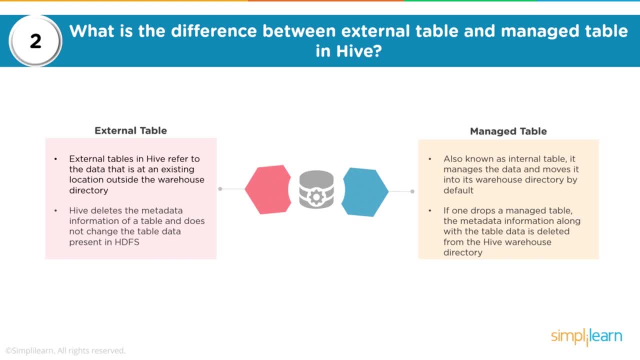 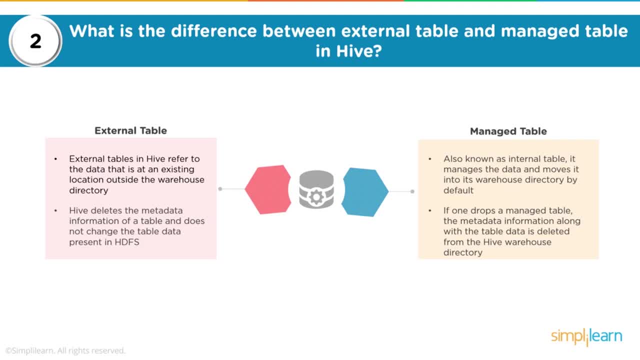 all the data on SDFS and then you could create a table by pointing to a particular directory or multiple directories. Now you could then do some testing of your tables and would decide that you might not need all the tables, So in that case it would be advisable to create. 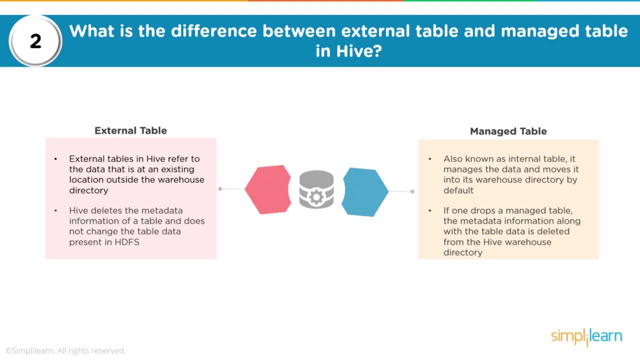 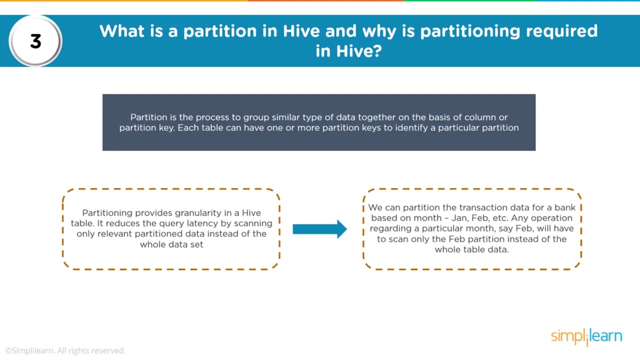 external tables so that even if the table is later dropped, the data on SDFS will be intact, unlike your managed table, where dropping of table will delete the data from SDFS. also, Let's learn a little bit on partition. So what is partition in Hive and why is partitioning? 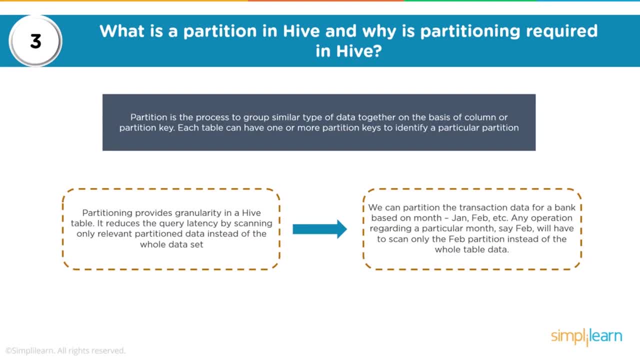 required in Hive, if somebody asks you that Now, normally in world of RDBMS, partition is the process to group similar type of data together, and that is usually done on basis of a column, or what we call as partitioning key, Now each table usually. 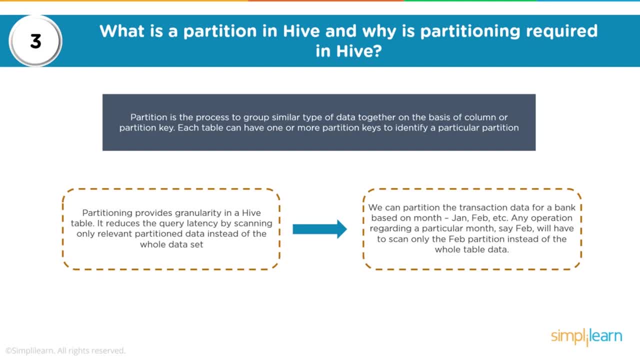 has one column in context of RDBMS which could be used to partition the data. And why do we do that? So that we can avoid scanning the complete table for a query and restrict the scan to set of data or to a particular partition. In Hive we can have any number. 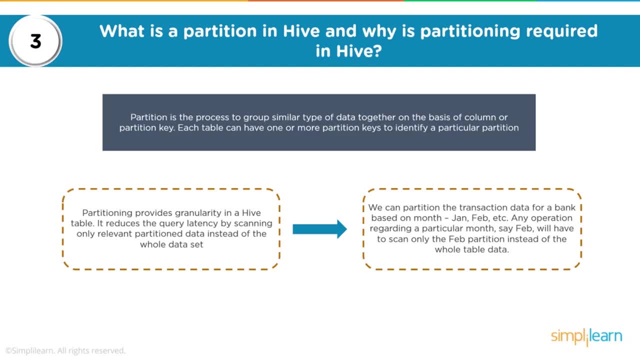 of partition keys. So partitioning provides granularity in Hive table. It reduces the query latency by scanning only relevant partition data instead of holding the data within a data set. We can partition at various levels. Now, if I compare RDBMS with Hive, in case of RDBMS, 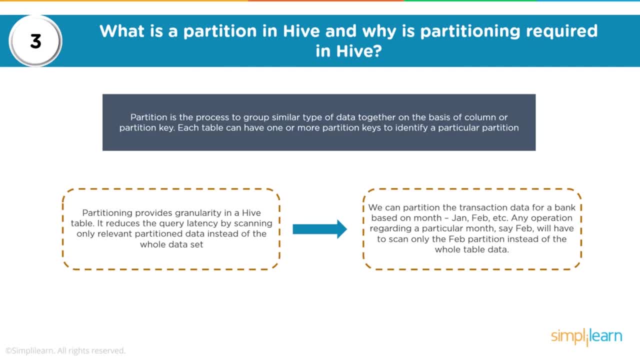 you could have one column which could be used for partitioning and then you could be querying the specific partition. So in case of RDBMS, your partition column is usually a part of the table definition. So, for example, if I have an employee table, I might have employee ID, employee name. 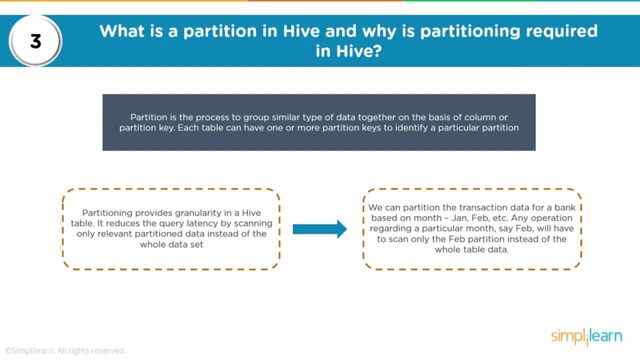 employee age and employee salary as four columns and I would decide to partition the table based on salary column. Now, why would I partition it? Because I feel that employee table is growing very fast. It is, or it will have, huge amount of data and later when we query the table, 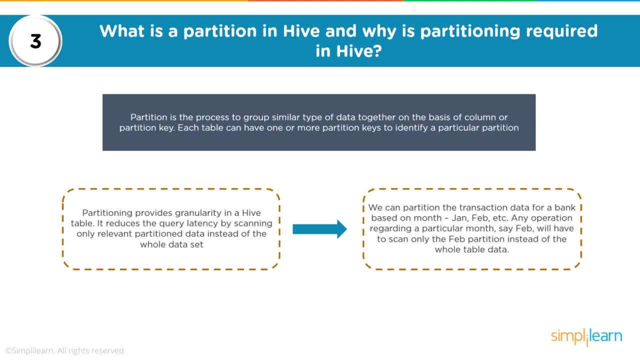 we don't want to scan the complete table, So I could split my data into multiple partition based on a salary column giving some ranges. In Hive it is a little different. In Hive you can do partitioning and there is a concept of static and dynamic partitioning. But in Hive 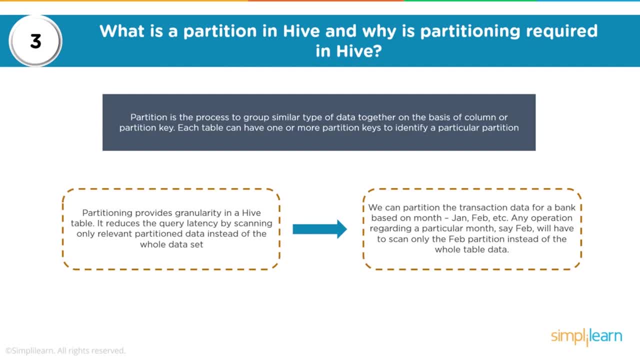 the partition column is not part of table definition. So you might have an employee table with employee ID, name, age and that's it. That would be the table definition. But you could then have partitioning done based on salary column, which will then create a specific folder. 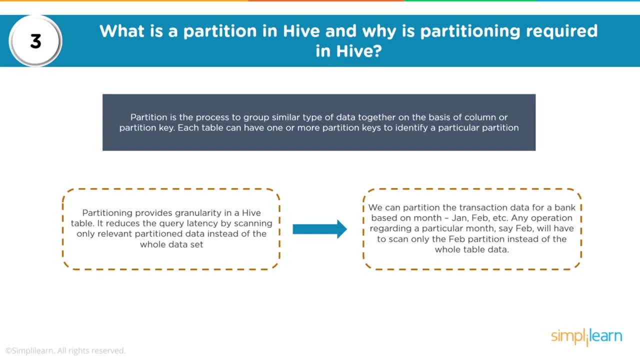 on SDFS. In that case, when we query the data, we can see the partition column also showing up, So we can partition the transaction data for a bank, for example, based on month, like Jan, Feb, etc. And any operation regarding a particular. 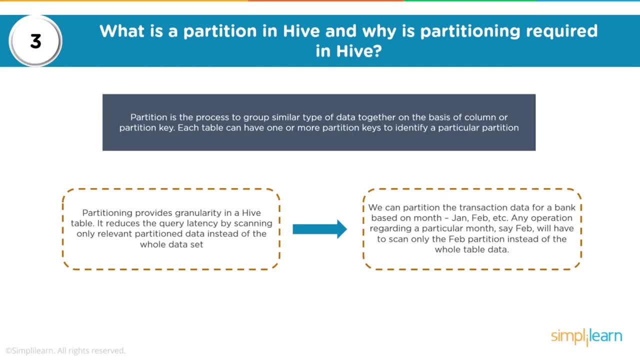 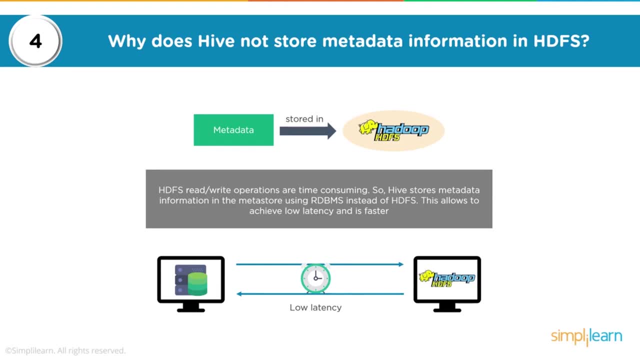 month will then allow us to query that particular folder. That is where partitioning is useful. Now, why does Hive not store metadata information in SDFS? If somebody asks you so, we know that Hive's data is stored in SDFS, which is Hadoop distributed file system. However, the metadata is either stored locally, 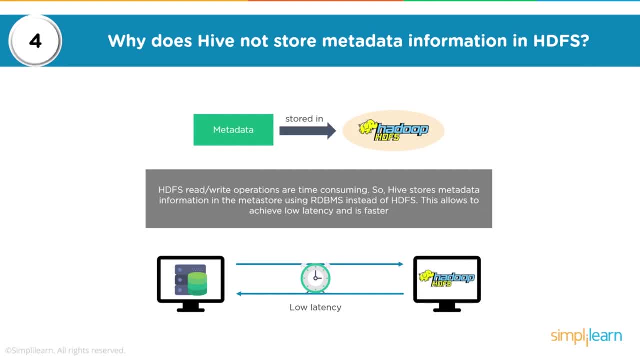 and that mode of Hive would be called as embedded mode, or you could have Hive's metadata stored in RDBMS so that multiple clients can initiate a connection. Now this metadata, which is very important for Hive, would not be stored in SDFS. So we already know that SDFS read and write. 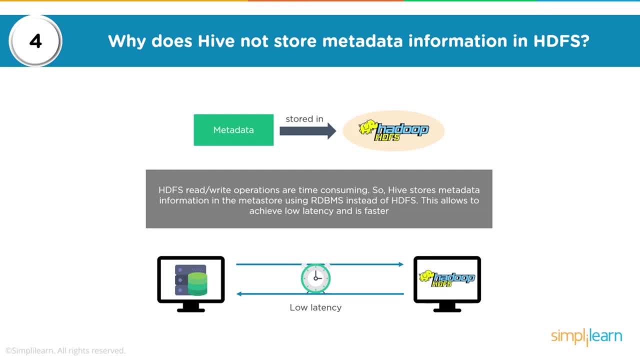 operations are time consuming. It is a distributed file system and it can accommodate huge amount of data, So Hive stores metadata information in Metastore, using RDBMS instead of SDFS. So this allows to achieve low latency and faster data access. Now if somebody asks what are the 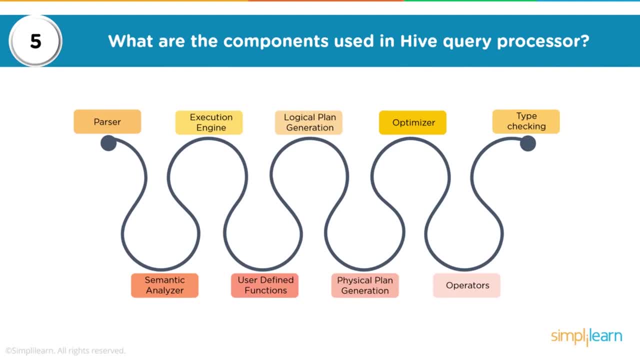 components used in Hive query processor. So usually we have. the main components are your parser, your execution engine, logical plan generation, optimizer and type checking. So it will go through a parser and parser would check the syntax, it would check for objects. 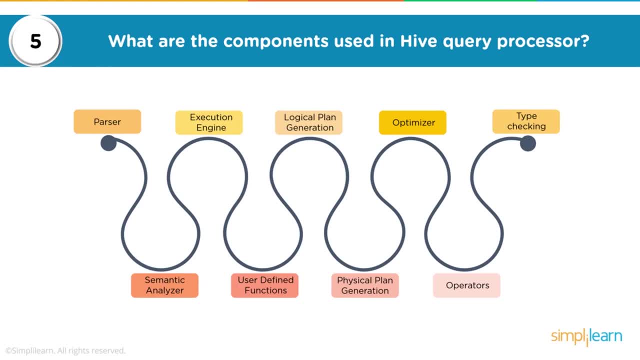 which are being queried and other things to see if the query is fine. Now, internally you have a semantic analyzer which will also look at the query. you have an execution engine which basically will work on the execution part. that is the best generated execution plan which could be used to. 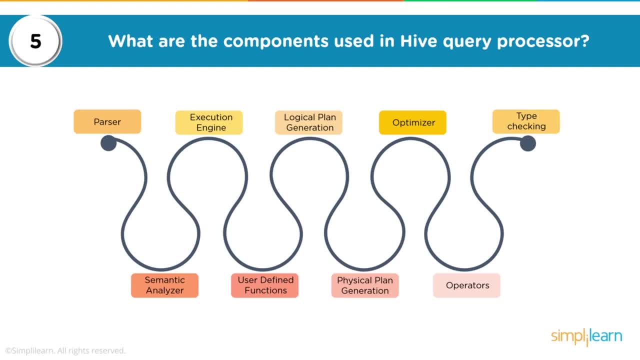 get the results for the query. You could also have user defined functions which a user would want to use, and these are normally created in Java or Java programming language, And then, basically, these user defined functions are added to the class path. Now you would have a logical plan generation. 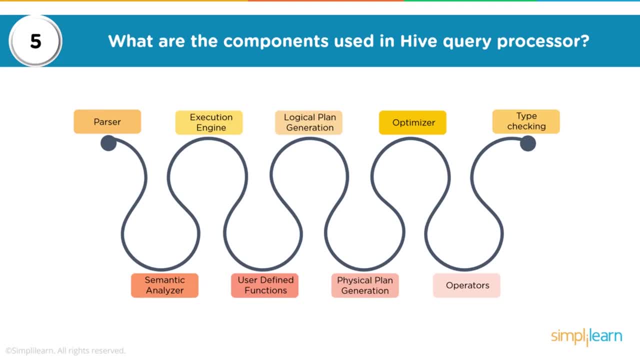 which basically looks at your query and then generates a logical plan or the best execution path which would be required to get to the results. Internally, there is a physical plan generated which is then looked in by optimizer to get the best path to get to the 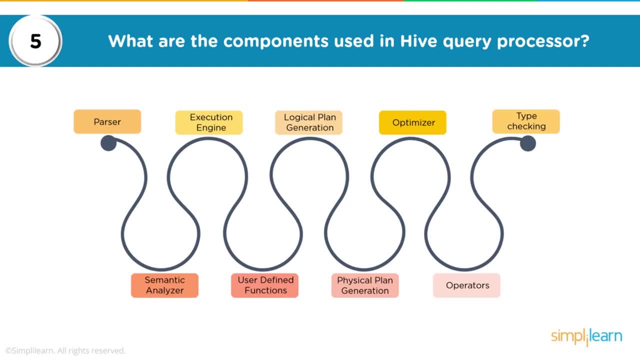 data, And that might also be checking your different operators which you are using within your query. Finally, we would also have type checking. So these are important components in Hive, So somebody might ask you, if you are querying your data using Hive, what are the 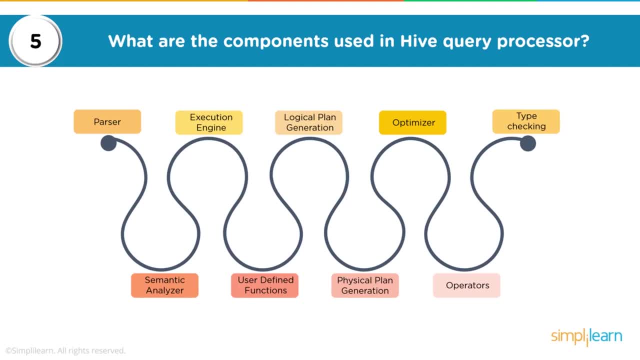 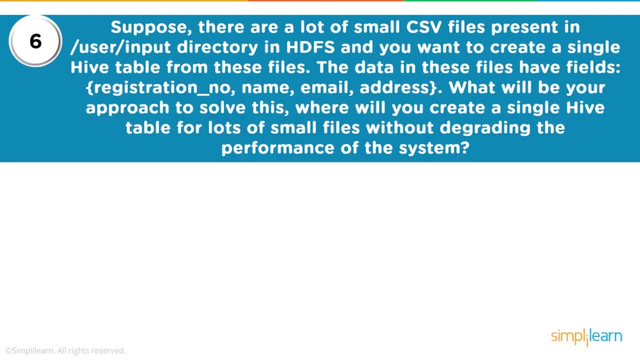 different components involved, Or if you could explain what are the different components which work when a query is submitted. So these are the components. Now let's look a scenario based question. Suppose there are a lot of small CSV files which are present in a SDFS directory and you want to create a single Hive table. 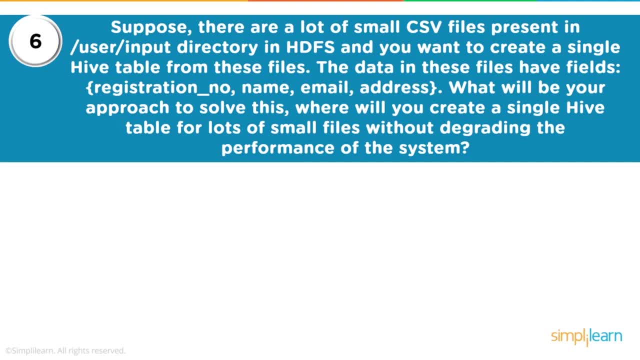 from these files. So data in these files have fields like registration number, name, email address. So if this is what needs to be done, what will be your approach to solve it? Where will you create a single Hive table for lots of small files without degrading the performance? 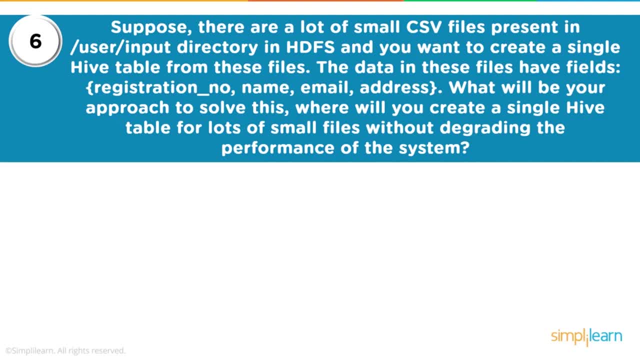 of the system So there can be different approaches. Now we know that there are a lot of small CSV files which are present in a directory. So we know that when we create a table in Hive we can use a location parameter. So I could say: create table, give the table name. 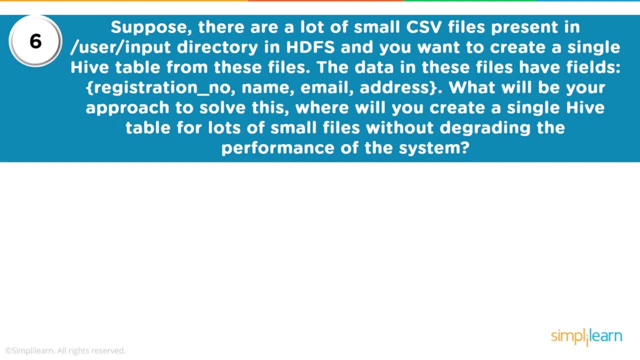 give the column and their data types, I could specify the delimiters And finally, I could say location and then point it to a directory on SDFS, And this directory might be the directory which has a lot of CSV files. So in this case I will avoid loading the data in the table, because 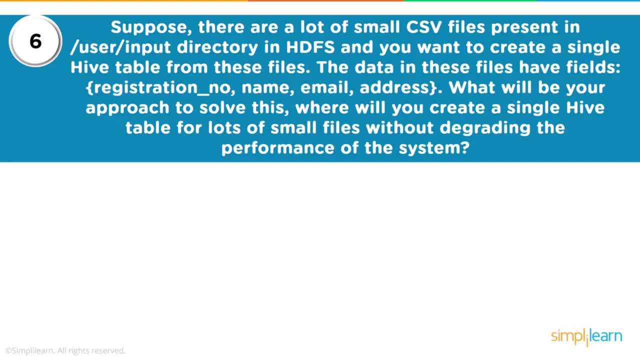 table being point- table pointing to the directory- will directly pick up the data from one or multiple files. and we also know that hive does schema check on read, so it does not do a schema check on write. so in case there were one or two files which did not follow the schema of the table, it would not. 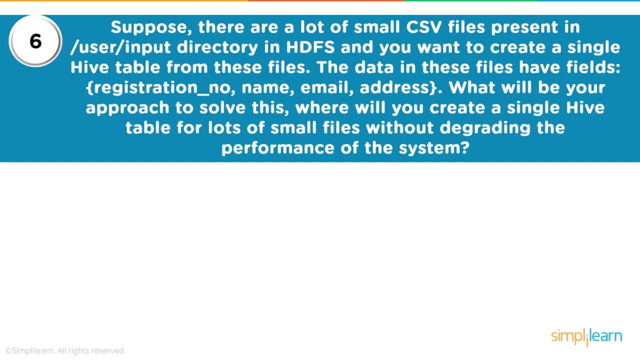 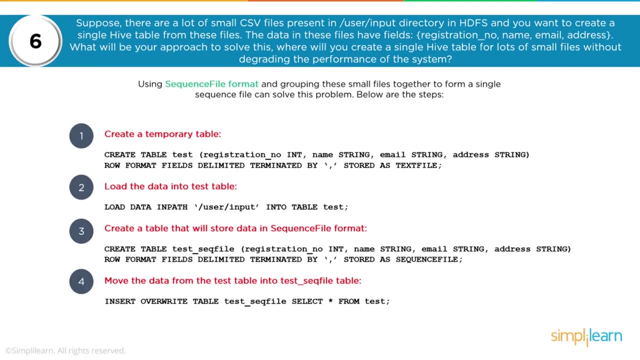 prevent data loading. data would anyways be loaded only when you query the data. it might show you null values if data which was loaded does not follow the schema of the table. this is one approach. what is the other approach? so let's look at that. you can think about sequence file format, which is 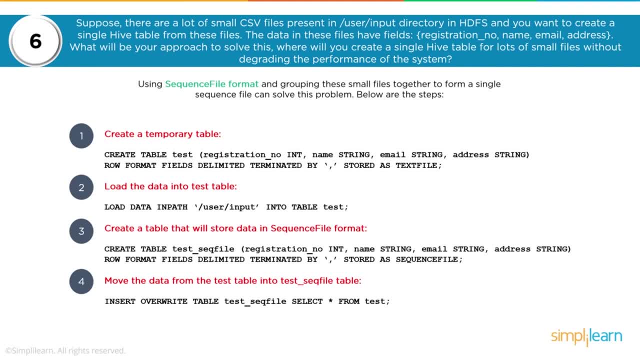 basically a smart format or a binary format and you can group these small files together to form a sequence file. now, this could be one other smarter approach so we could create a temporary table. so we could say: create table, give a table name, give the column names and their. 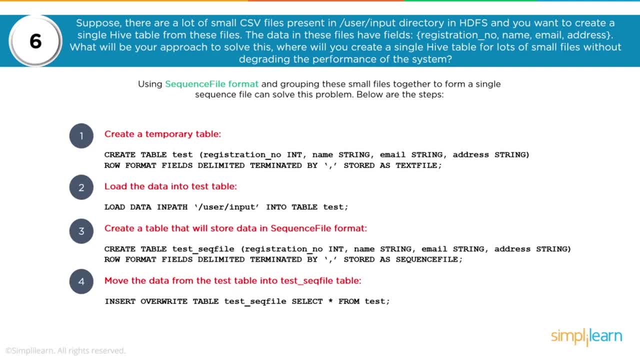 data to the table and then we could create a temporary table. so we could say, create table types, we could specify the delimiters as it shows here, that is, row format and fields terminated by, and finally we can store that as text file. then we can load data into this table by giving a local. 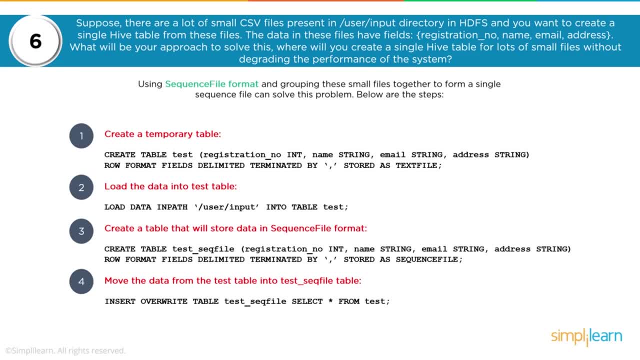 file system path and then we can create a table that will store data in sequence file format. so my point one is storing the data in this text file. point three would be storing the data in sequence file format. so we say: create table and then we can load data into this table and then we can load. 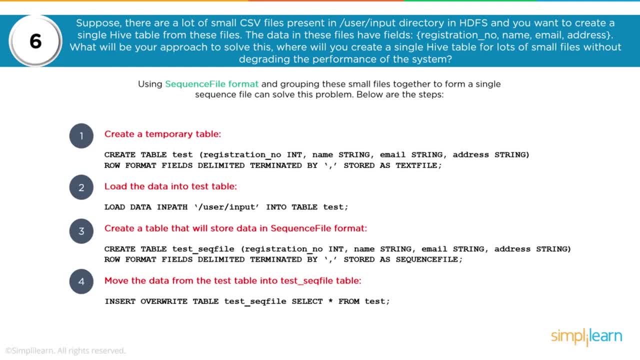 table give the specifications. we say row format, delimited fields are terminated by comma, stored as sequence file. then we can move the data from test table into test sequence file table. so i could just say: insert, overwrite my new table as select star from other table. remember in hive you. 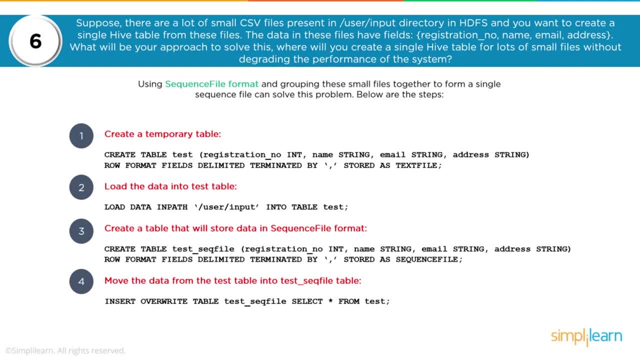 cannot do insert, update, delete. however, if the table is existing, you can do a insert overwrite from an existing table into a new table so we can move the data from test table into test sequence table. so this could be one approach where we could have a lot of csv files or smaller files. 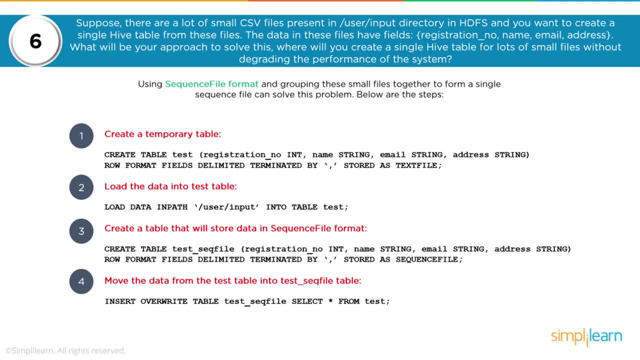 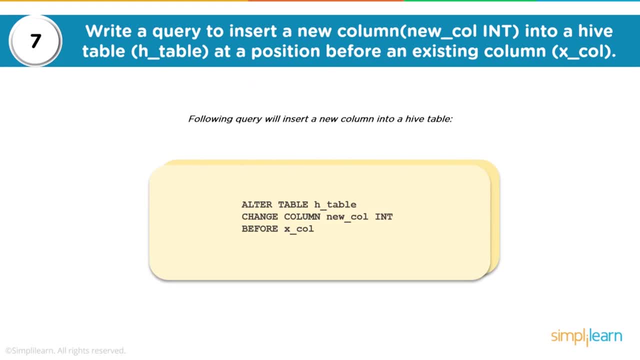 clubbed together as one big sequence file and then store it in the table. now, if somebody asks you write a query to insert a new column that is integer data type into a hive table and the requirement might be that you would want to insert this table at a position before an existing column, 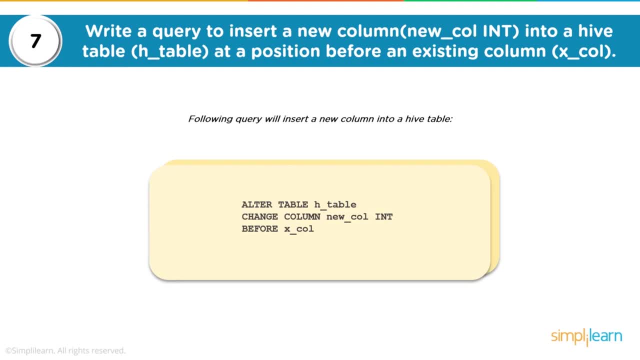 now that's possible by doing an alter table, giving your table name and then specifying change column, giving you a new column with the data type before an existing column. this is a simple way wherein you can insert a new column into a hive table. what are the key? 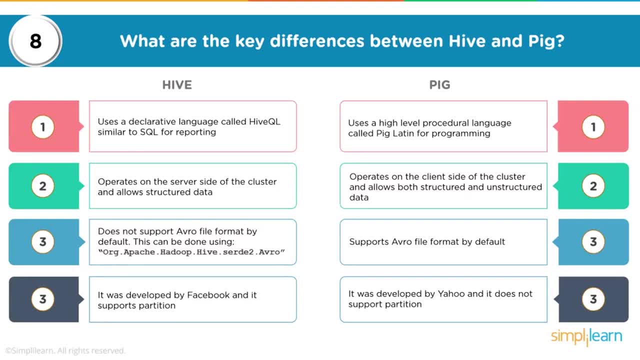 differences between hive and pig. now, some of you might have heard, hive is a data warehousing package and pig is more of a scripting language. both of them are used for data analysis or trend detection, hypothesis testing, data transformation and many other use cases. so if we compare hive and pig, hive uses a declarative language called hiveql, that is. 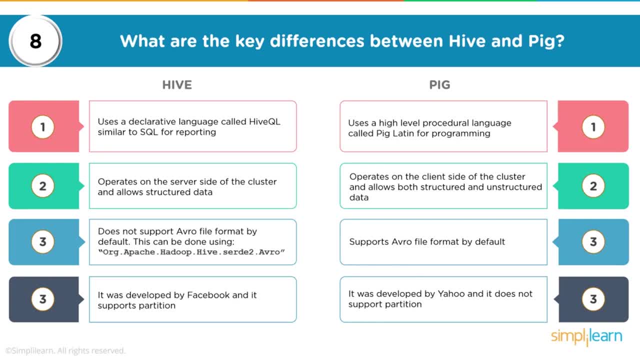 hive querying language similar to sql and it is for reporting or for data analysis. even for data transformation or for your data extraction. pig uses a high level procedural language called pig latin for programming. both of them, remember, use map, reduce processing framework. so when we run a query in hive to process the data, we use a high level procedural language called pig latin. 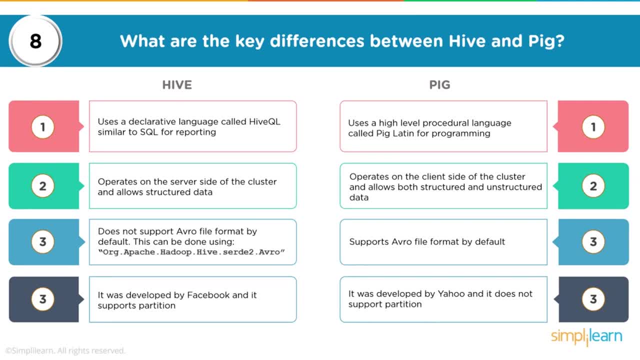 or when we create and submit a pig script. both of them trigger a map reduce job unless and until we have set them to local mode. hive operates on the server side of the cluster and basically works on structured data or data which can be structurized. pig usually works or operates on the client side. 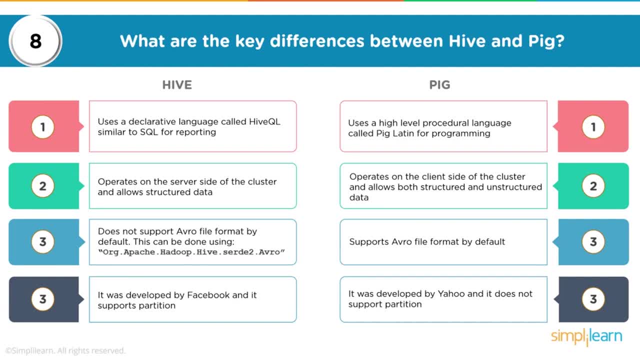 of the cluster and allows both structured, unstructured or even, i could say, semi-structured data. hive does not support avro file format by default, but it does support avro file format by default and it does not support avro file format by default and it does not support avro file format. 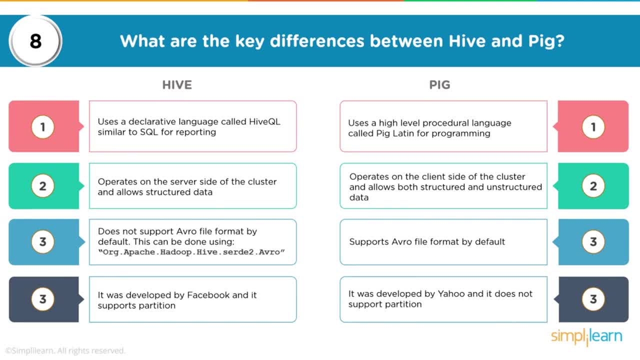 however, that can be done by using the right serializer, deserializer, so we can have hive table related data stored in avro format, in sequence file format, in parquet format or even as a text file format. however, when we are working on smarter formats like avro or sequence file or 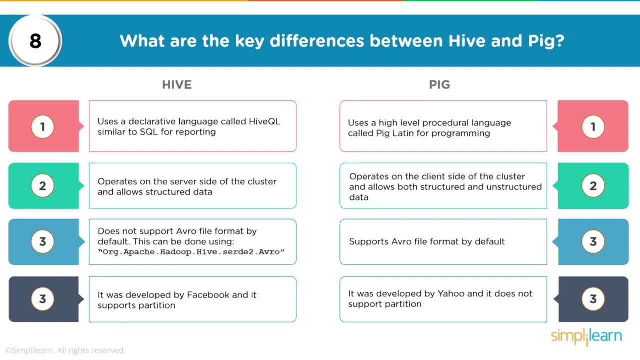 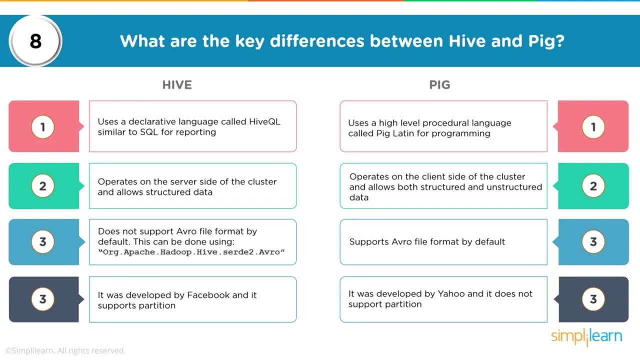 by default. hive was developed by facebook and it supports partitioning, and pig was developed by yahoo and it does not support partitioning. so these are high level differences. there are lots and lots of differences. remember, hive is more of a data warehousing package and pig is more of a. 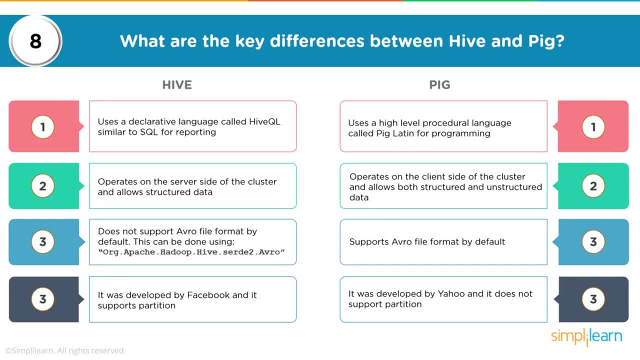 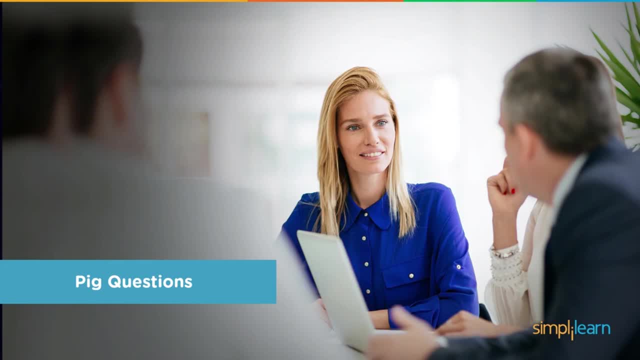 scripting language or a strictly procedural flow following scripting language, which allows us to process the data. now let's get started, so, let's get started, so, let's get started, so let's get started now, let's get more, and let's get more deeper and learn about pig, which is, as i mentioned, 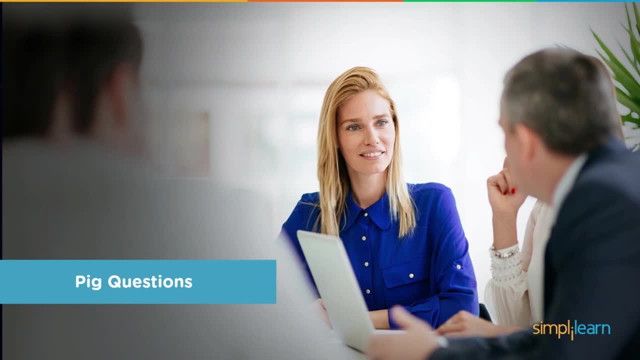 a scripting language which can be used for your data processing. it also uses map reduce, although we can even have pig run in a local mode. let's learn about pig in the next section. now let's learn on some questions about pig, which is a scripting language, and it is extensively used. 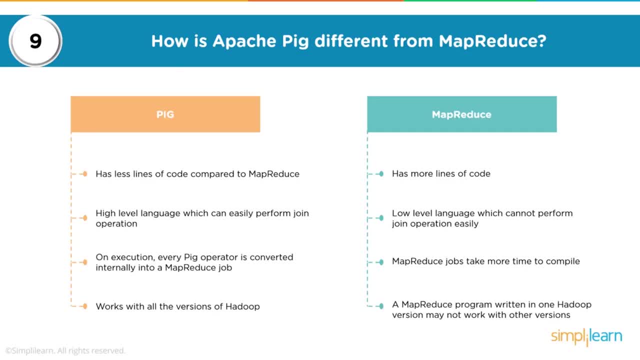 for data processing and data analysis. so the question is: how do you use pig to run your data? so the question is: how is apache pig different from map reduce? now, we all know that map reduce is a programming model. it is it's quite rigid when it comes to processing the data, because you have 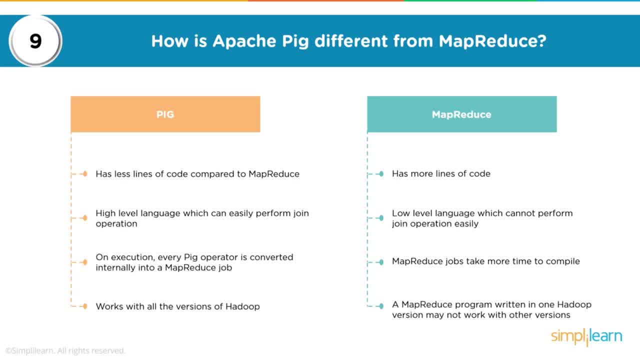 to do the mapping and reducing you have to write huge code. usually map reduces written in java, but now it can also be written in python. it can be written in scala and other programming languages. so if we compare pig with map reduce, pig obviously is very consistent with map reduce. 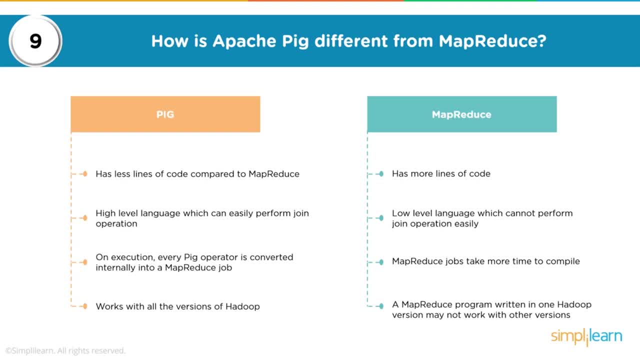 it has less lines of code when compared to map reduce. now we also know that pig script internally will trigger a map reduce job. however, user need not know about map reduce programming model. they can simply write simple scripts in pig and that will automatically be converted into map reduce. however, map reduce has more lines of code. pig is high level language which can. 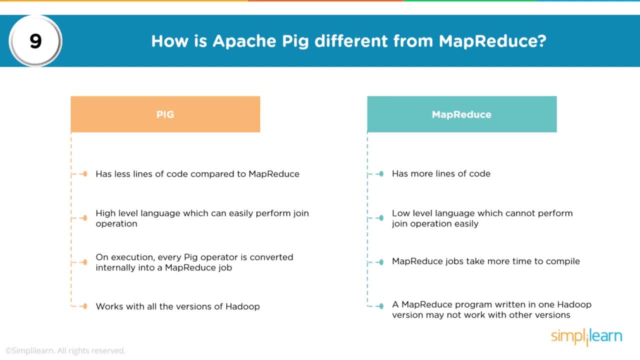 easily perform join operations or other data processing operations. map reduce is a programming language which can easily perform join operations or other data processing. is a low level language which cannot perform job join operations easily. so we can do join using map reduce. however, it's not really easy in comparison to pig. now, as i said, on execution, 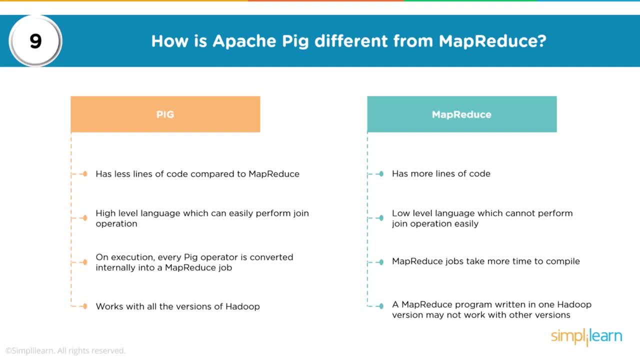 every pig operator is converted internally into a map reduce job. so every pig script which is run which would be converted into map reduce job. now, map reduce overall is a batch oriented processing so it takes a lot of time to do that. so it takes a lot of time to do that. so it takes a lot of time to do that. 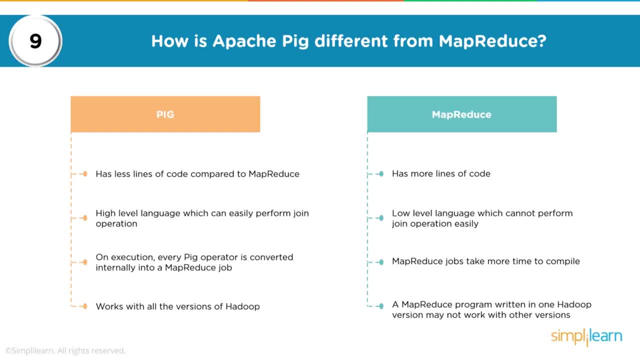 takes more time to compile. it takes more time to execute, either when you run a map reduce job or when it is triggered by pig script. pig works with all versions of hadoop and when we talk about map reduce program, which is written in one hadoop version may not work with other versions. it. 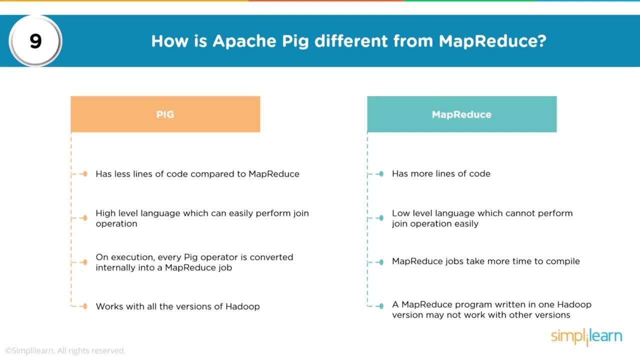 might work or it might not. it depends on what are the dependencies, what is the compiler you're using, what programming language you have used and what version of hadoop you are working on. so these are the main things that you need to know about hadoop and what version of hadoop you are working on. so 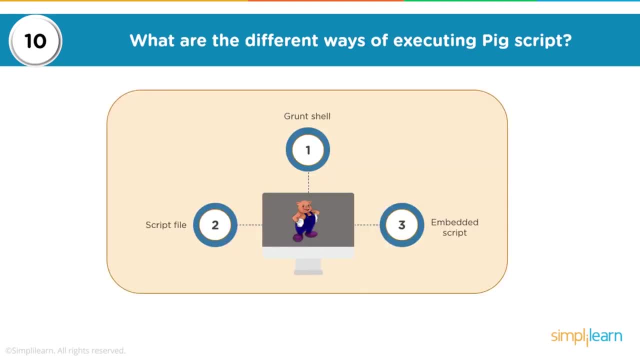 these are the main things that you need to know about hadoop and what version of hadoop you are working on. so so this would be a reason why i put into forecast: running ha까 adesso are the different ways of executing your pig script now. what are the major? 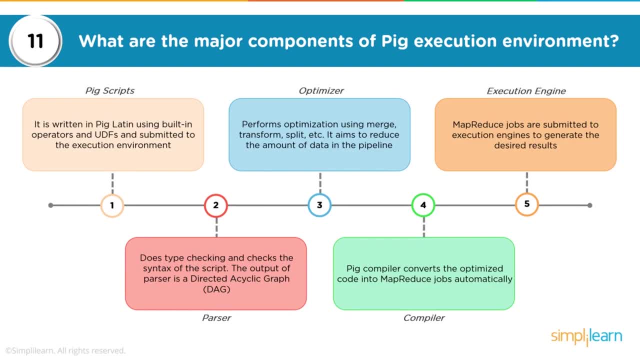 components of pig execution environment. this is: this is a very common question. interviewers would always want to know different components of hive, different components of pig, even different components which are involved in Hadoop ecosystem. so when we want to learn about major components of pig execution environment, here are some. so you have pig scripts now that is written in pig. 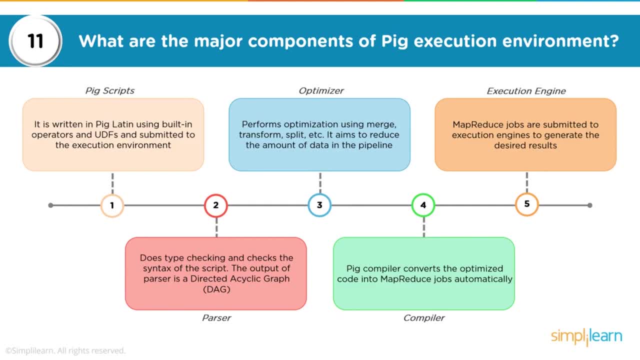 Latin, using built-in operators and user-defined functions and submitted to the execution environment. that's what happens when you would want to process the data using pig. now there is a parser which does type checking and checks the syntax of the script. the output of parser is a tag direct acyclic graph. so 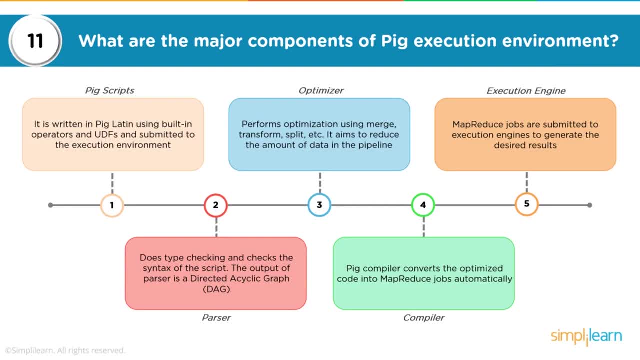 look in Wikipedia for tag. so tag is basically a sequence of steps which run in one direction. then you have an optimizer. now this optimizer performs optimization using merge, transform, split, etc. it aims to reduce the amount of data in the pipeline. that's the whole purpose of optimizer. you have a internal 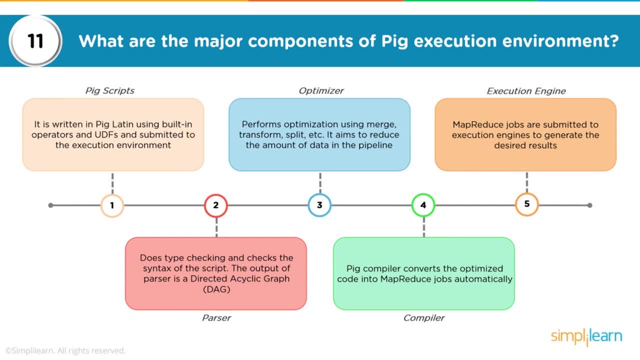 compiler, so pig compiler converts the optimized code into a map reduce job. and here user need not know the map reduce programming model or how it works or how it is written. they all need to know about running the pig script which would be internally converted into a map reduce job. and finally we have an execution engine, so map. 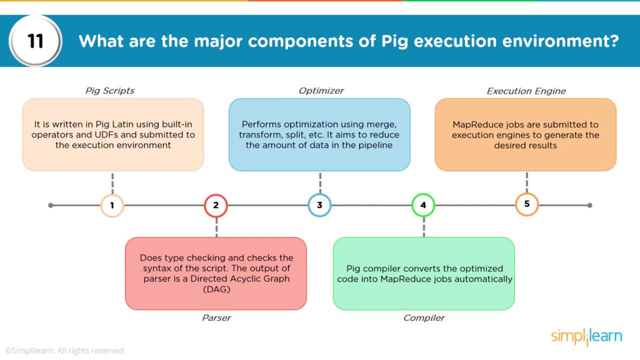 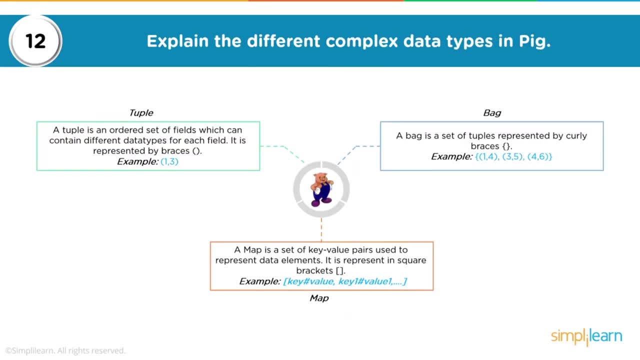 reduce jobs are submitted to the execution engine to generate the desired results. so these are major components of pig execution environment. now let's learn about different complex data types. in pig supports various data types. the main ones are tuple, bag and map. what is tuple? or tuple, as you might. 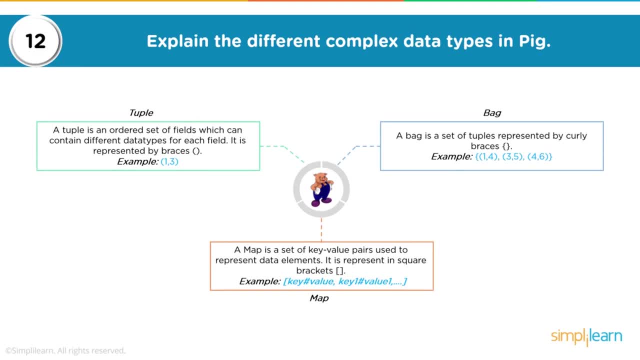 have heard. a tuple is an ordered set of fields which can contain different data types for each field. so in any you would have multiple elements but that would be of same types. list can also have different types. your tuple is a collection which has different fields and each field can be. 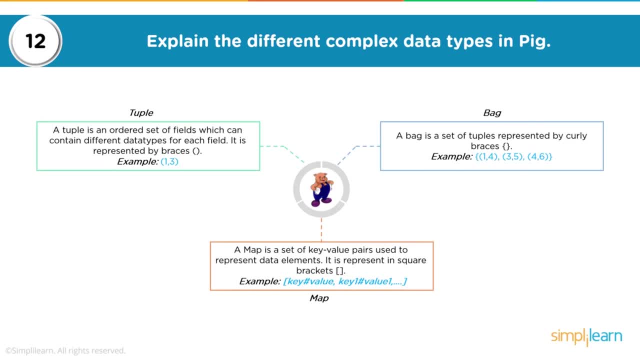 of different type. now we could have an example as 1 comma 3 or 1 comma 3 comma, a string or a float element and all of that form. a tuple bag is a set of tuples, so that's represented by curly braces. so you could also imagine this like a dictionary which has various different 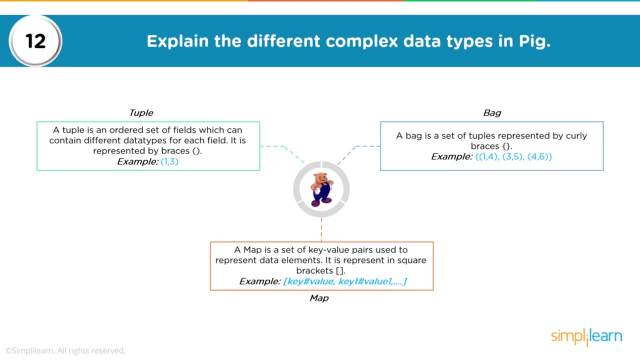 collection elements. what is a map? map is a set of key value pairs used to represent data. so when you work in big data field, you need to know about different data types which are supported by pig, which are supported by hive, which are supported in other components of a. do so tuple, bag, map array, array buffer. 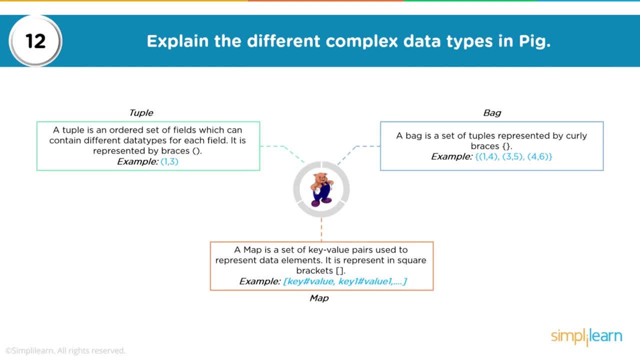 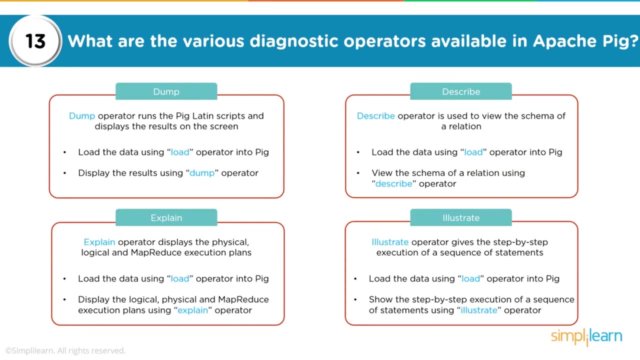 you can think about list, you can think about dictionaries, you can think about map, which is key value pair. so these are your different complex data types other than the primitive data type, such as integer, character string, boolean, float and so on. now, what are the various diagnostic operators available in Apache pig? so these are some of the operators, or 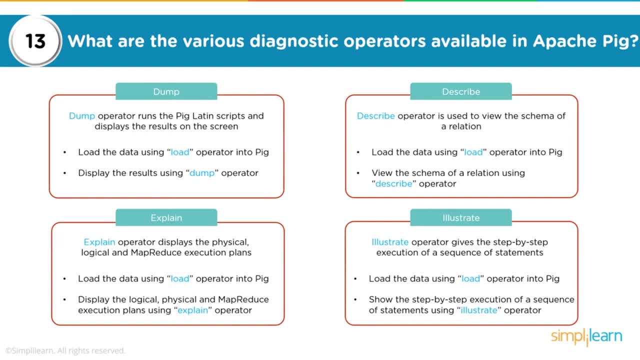 options which you can give in a pig script. you can do it dumb now dumb operator runs the pig Latin scripts and displays the result on the screen. so either I could do it dumb and see the results- the result would look like this output on the screen- or i can even do a dump into and i could store my output in a particular file. 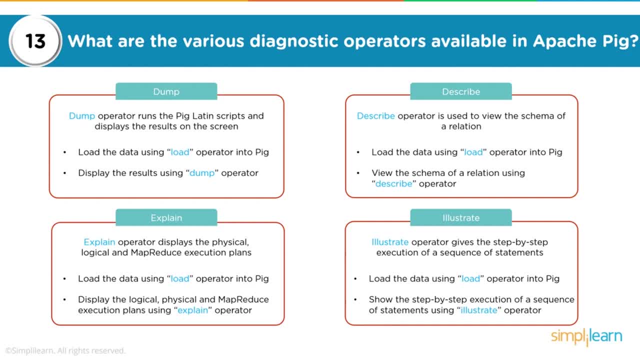 so we can load the data using load operator in pig, and then pig also has different internal storage, like json loader or big storage, which can be used if you are working on specific kind of data, and then you could do a dump either before processing or after processing, and dump would 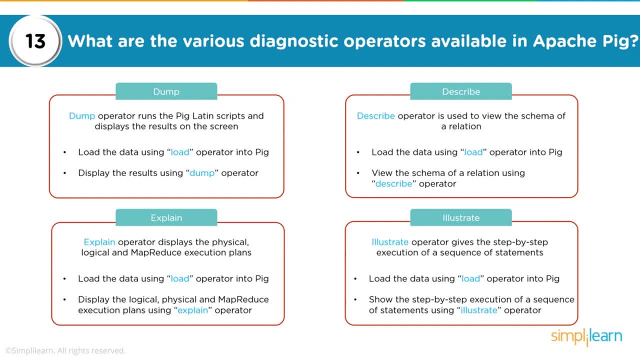 produce the result. the result could be stored in a file or seen on the screen. you also have a describe operator now that is used to view the schema of a relation, so you can load the data and then you can view the schema of relation using describe operator. explain as we might. 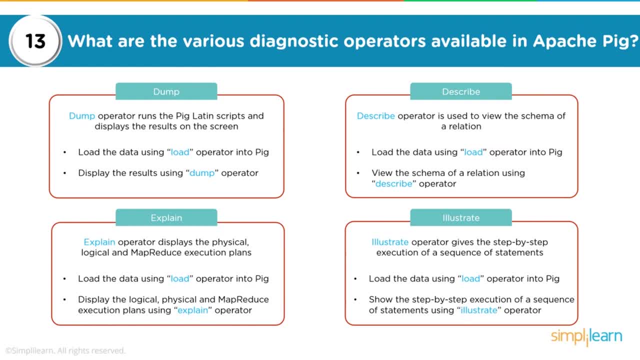 already know, displays the physical, logical and map reduce execution plans. so normally in rdbms when we use explain, we would like to see what happens behind the scenes when a particular script or a query is used, so we can see what happens when a particular script or a query is used. 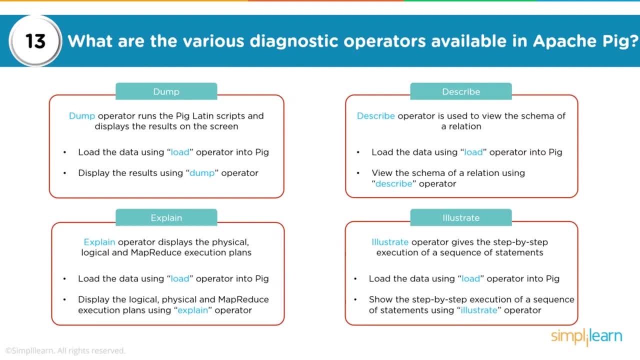 runs. so we could load the data using load operator as in any other case, and if we would want to display the logical, physical and map reduce execution plans, we could use explain operator. there is also an illustrate operator now that gives the step-by-step execution of sequence. 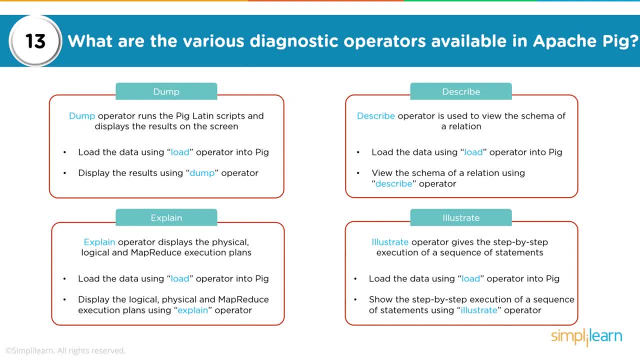 of statements. so sometimes when we would want to analyze our script to see how good or bad they are, or would that really serve our purpose- we could use illustrate. and again you can test that by loading the data using load operator and you could just use a illustrate operator to have a look. 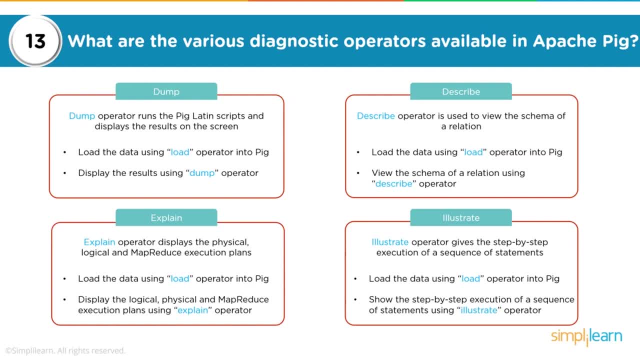 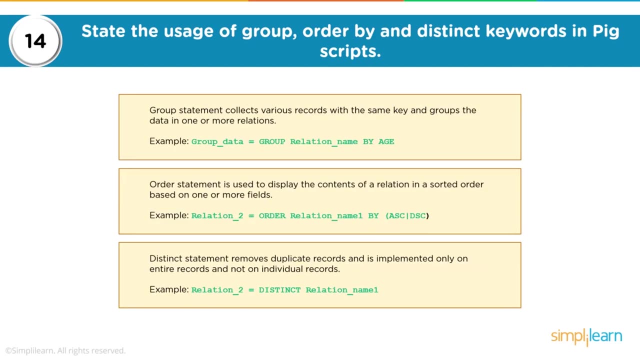 at the step-by-step execution of the sequence of statements which you would want to execute. so these are different diagnostic operators available in apache pig. now, if somebody asks, state the usage of group order by and distinct keywords in pig script. so, as i said, pig is a. 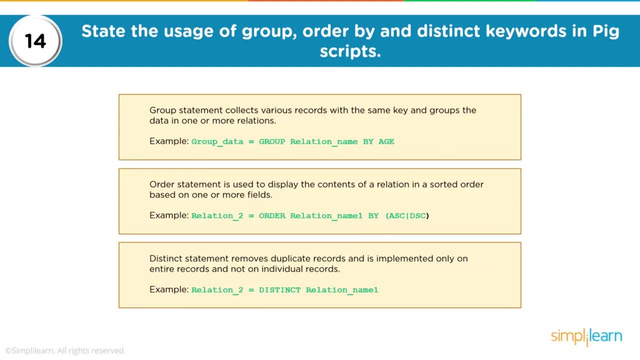 scripting language so you could use various operators. so group basically collects various records with the same key and groups the data in one or more relations. here is an example. you could do a group data, so that is basically a variable. or you can give some other name and you can say: 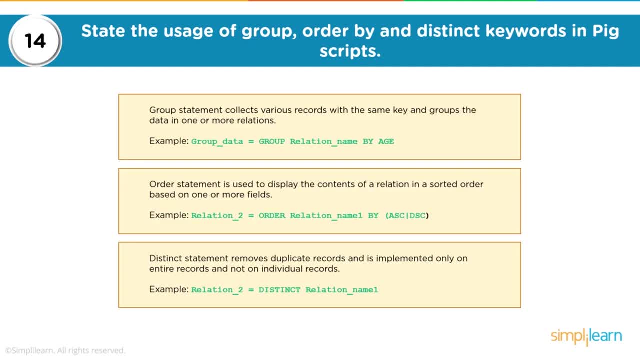 group relation name by age. now, say, i have a file where i have field, various fields, and one of the field is a relation name. so i could group that by a different field. order by is used to display the contents of relation in a sorted order, whether ascending or descending. 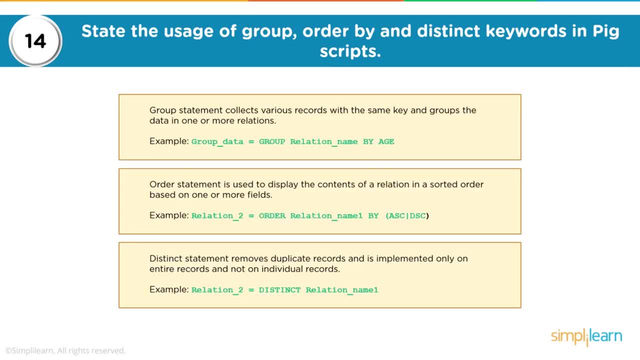 so i could create a variable called relation two and then i could say order relation name one by ascending or descending order. distinct basically removes the duplicate records and it is implemented only on entire records, not on individual records. so if you would like want to find out the distinct values and relation name field, i could use distinct. what are the? 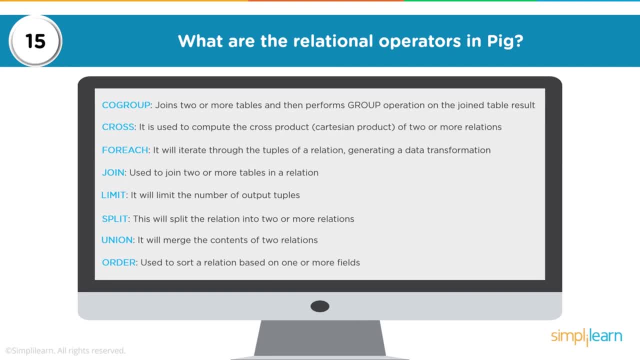 relational operators in pig. so you have various relational operators which help data scientists or data analysts or developers who are analyzing the data, such as co-group, which joins two or more tables and then performs group operation on the join table result you have cross. it is used to 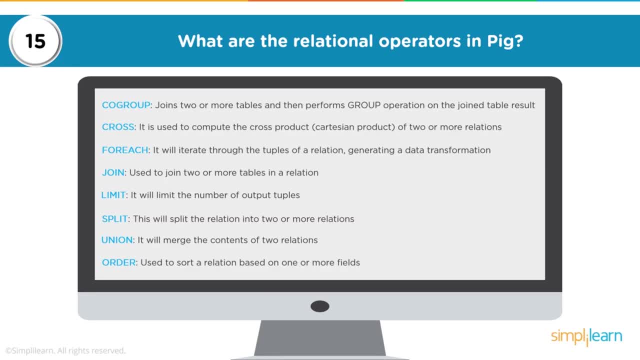 compute the cross product, that is, a cartesian product of two or more relations for each is basically to do some iteration, so if it will iterate through tuples of a relation, generating a data transformation. so for example, if i say variable a equals and then i load a file in a and then i could create a variable called b where i could say for: 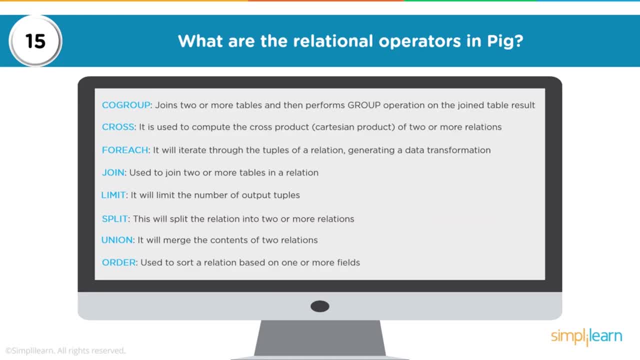 each a. i would want to do something. say, group join is to join two or more tables in a relation. limit is to limit the number of output tuples or output results. split is to split the relation into two or more relations. union is to get a combination, that's it will merge the contents. 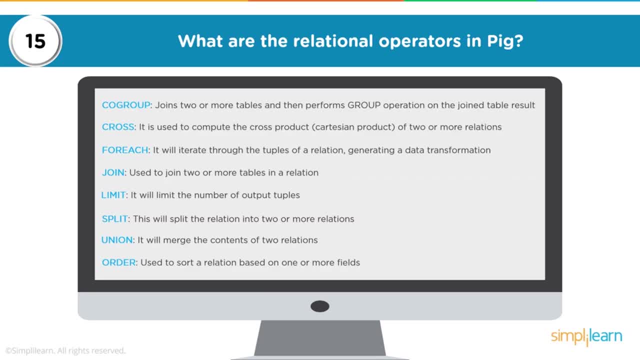 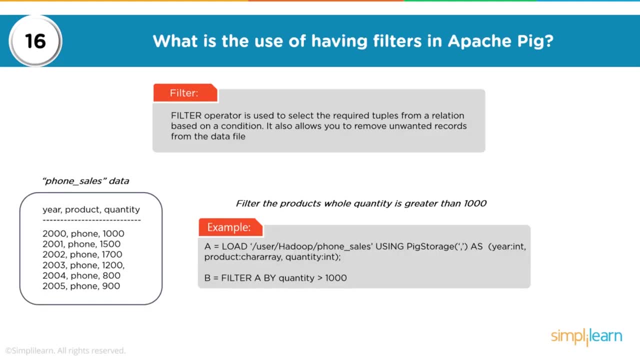 of two or more relations and order is to get a sorted result. so these are some of the functional operators which are extensively used in pig for analysis. what is the use of having filters in apache pig now say, for example? i have some data which has three fields: year, product. 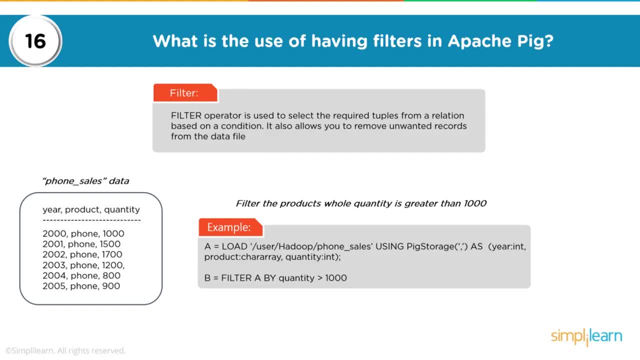 quantity and this is my phone sales data. so filter operator could be used to select the required values from a relation based on a condition. it also allows you to remove unwanted records from data file, so, for example, where quantity is greater than thousand. so i see that i have one row wherein, or multiple rows where, 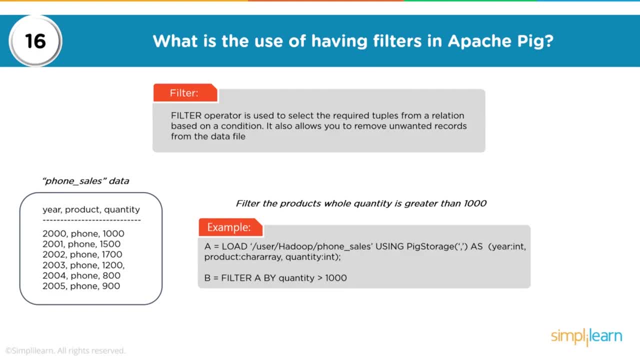 the quantity is greater than 1000, such as 1500, 1700, 1200. so i could create a variable called a. i would load my file using pig storage. as i explained earlier, pig storage is an internal parameter which can be used to specify the delimiters. now, here, my delimiter is comma. 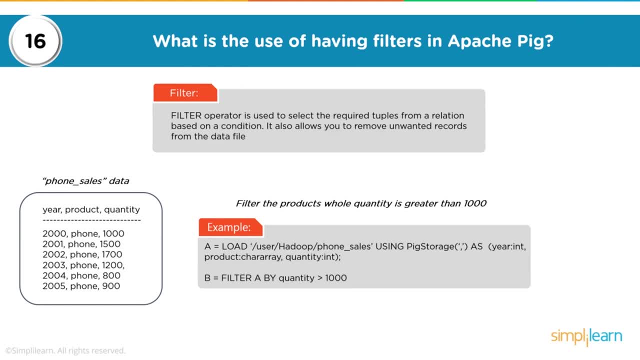 so i could say using pig storage as, and then i could specify the delimiter as, and then i could specify the data type for each field. so, here being integer, product being character array and quantity being integer, then b, i could say filter a, whatever we have in a- by quantity greater than. 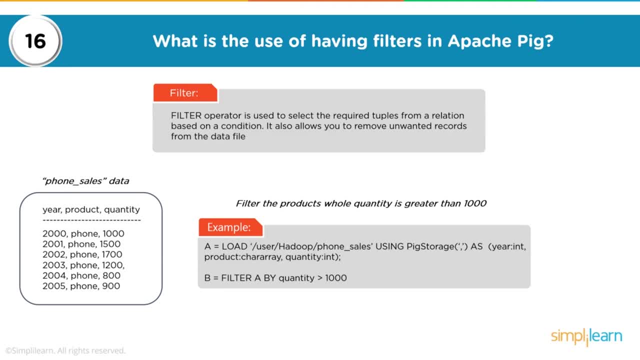 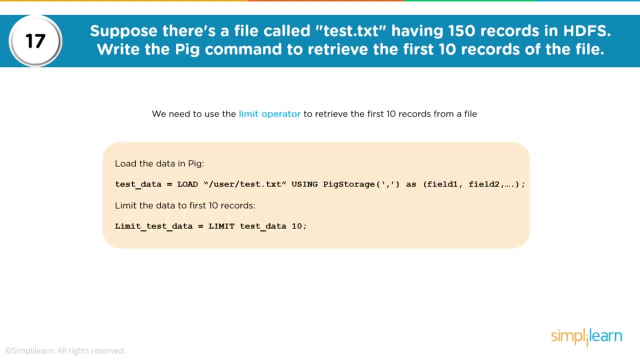 1000. so it's very concise, it's very simple and it allows us to extract and process data in a simpler way. now suppose there is a file called testtxt, having 150 records in his dfs. so this is a file- it has 150 records, where we can consider every record being one line and if somebody asks you 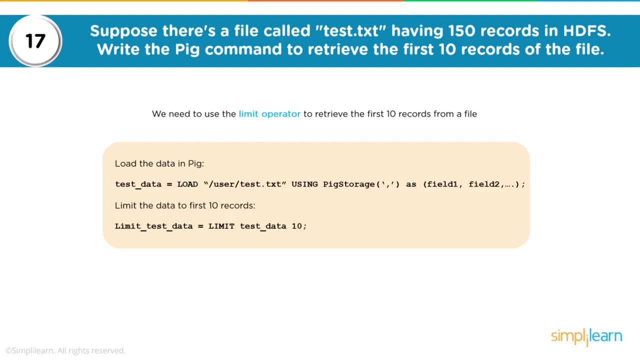 to write a pic command to retrieve the first 10 records of the file. first we will have to load the data. so i could create a variable called test underscore data and i would say: load my file using pig storage, specifying the delimiter as comma, as, and then i could specify my fields whatever. 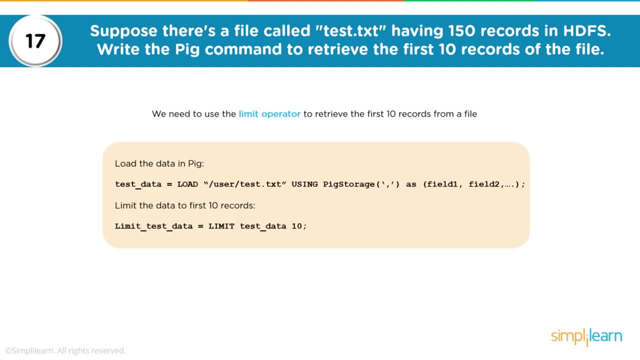 fields our file have. and then i would want to get only 10 records for which i could use the limit, so i could say limit on test data and give me 10 records. this is very simple and we can extract 10 records from 150 records which are stored in the file on sdfs. now we have learned. on pig, we have. 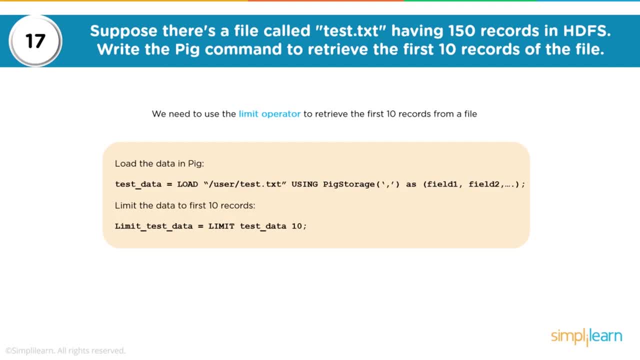 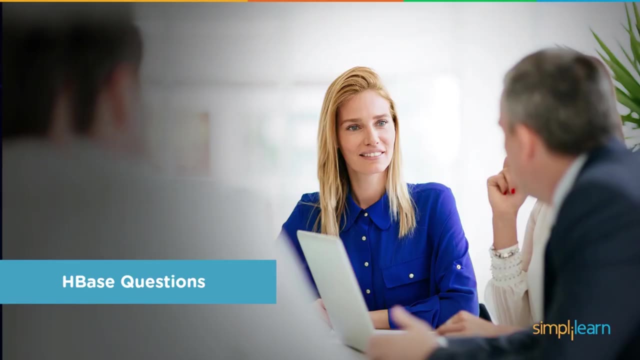 learned some questions on hive. you could always look more in books like programming in hive or programming in pig and look for some more examples and try out these examples on a existing hadoop setup. now let's learn on hbase, which is a no sql database. now hbase is a four dimensional database in comparison to your. 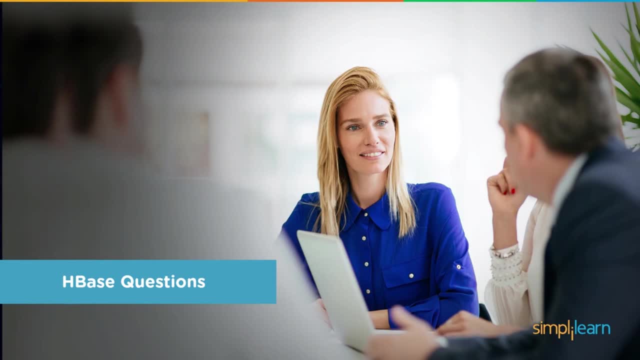 rdbms, which usually are two dimensional. so rdbms have rows and columns, but hbase has four coordinates. it has row key, which is always unique, column family, which can be any number, column qualifiers, which can again be any number per column family, and then you have a version. so these four coordinates. 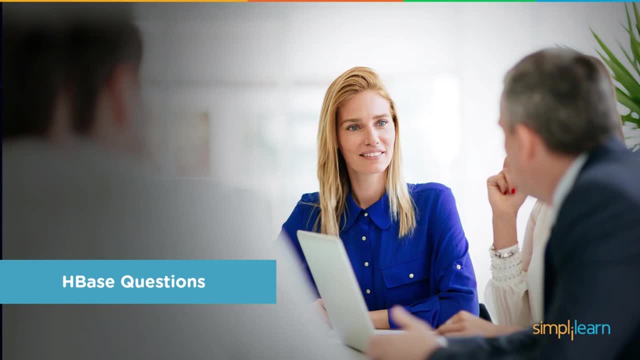 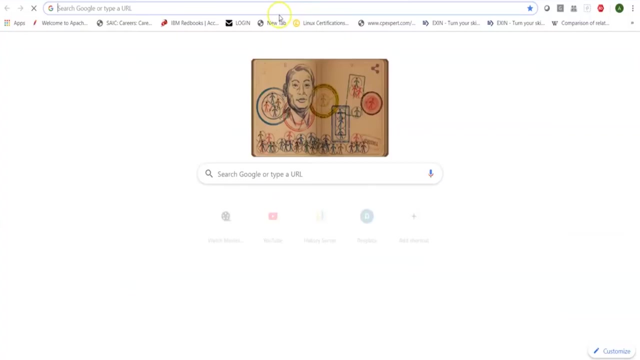 make hbase a four dimensional key value store or a column family store which is unique for storing huge amount of data and extracting data from hbase. there is a very good link which i would suggest everyone can look at if you would want to learn more on hbase and you could just say: 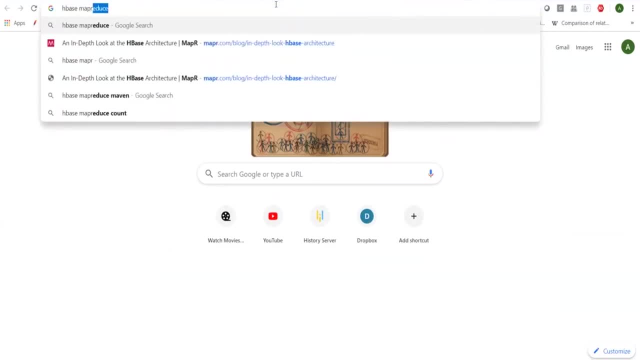 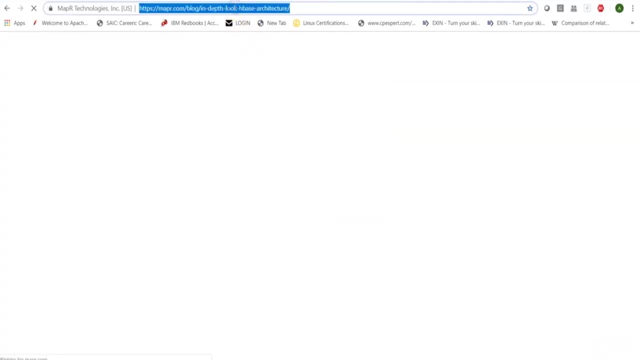 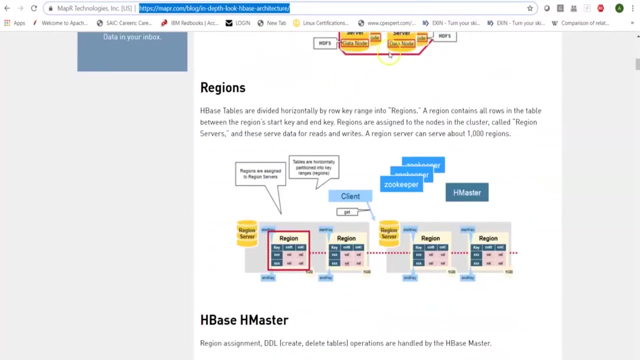 hbase mapper and this basically brings up a documentation which is from mapper, but then that's not specific to mapper and you can look at this link which will give you a detailed explanation of hbase, how it works, what are the architectural components and how data is. 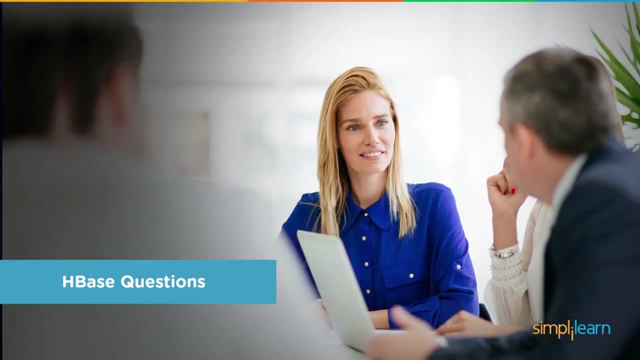 stored and how it makes hbase a very powerful no sql database. so let's learn on some of the important or critical questions on hbase which might be asked by the interviewer in an interview when you're applying for a big data admin or a developer position role. so what are the key? 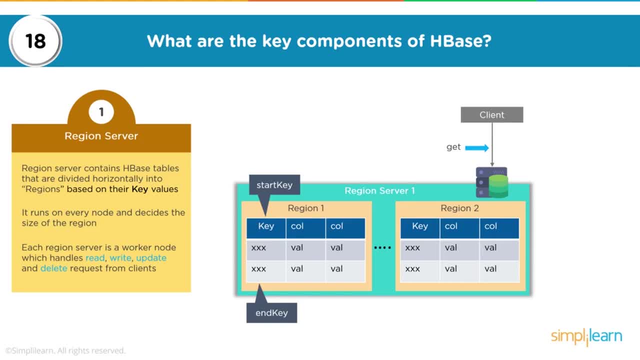 components of hbase. now, as i explained earlier, on the specific questions related to no sql database, I said this is one of the favorite questions of interviewers where they would want to understand your knowledge on different components for a particular service. HBase, as I said, is a 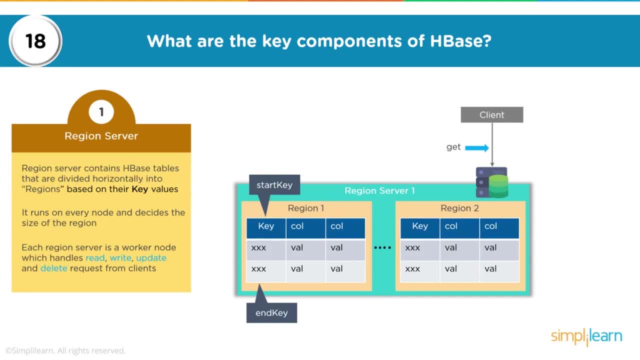 NoSQL database and that comes as a part of service with Cloudera or Hotendworks And with Apache, Hadoop, you could also set up HBase as an independent package. So what are the key components of HBase? HBase has a region server. Now HBase follows the similar kind of topology, like Hadoop. 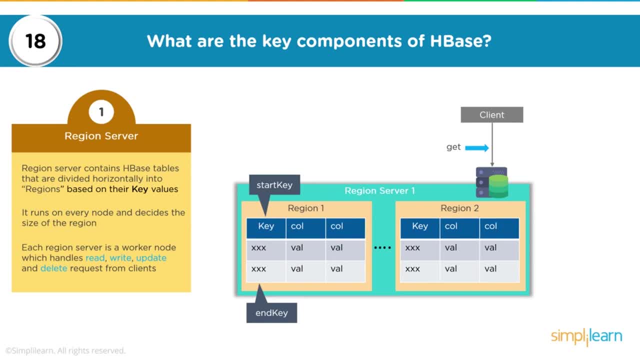 Now Hadoop has a master process, that is, name node, and slave processes such as data nodes and secondary name node. In the same way, HBase also has a master, which is H master, and the slave processes are called region servers. So these region servers are usually co-located with data. 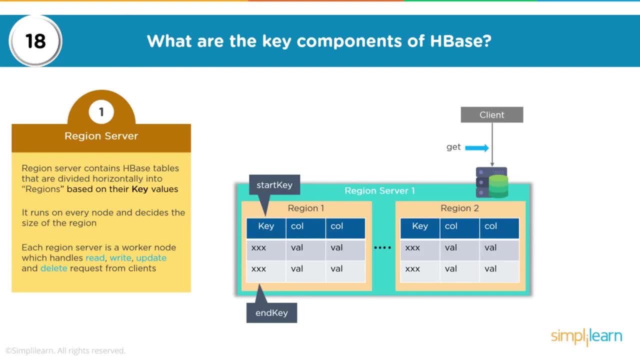 nodes. However, it is not mandatory that if you have 100 data nodes, you would have 100 region servers, So it purely depends on admin. So what does this region server contain? So region server contains HBase tables that are divided horizontally into regions, Or you could say group of rows. is 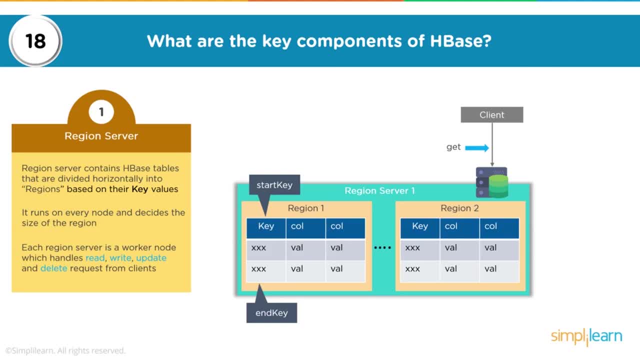 called regions. So in HBase you have two aspects: One is group of columns which is called column family, And one is group of rows which is called column family, And one is group of rows which is called regions. Now these regions, or these rows, are grouped based on the key values, or I would 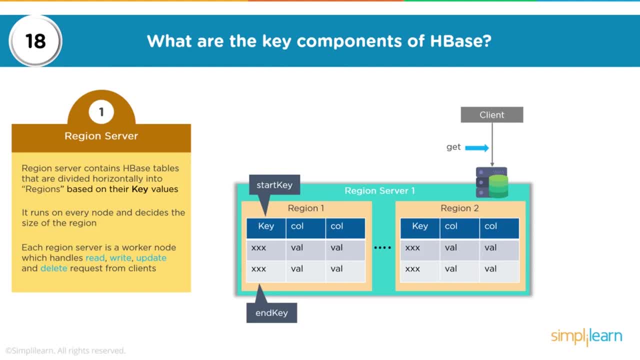 say row keys, which are always unique. When you store your data in HBase you would have data in the form of rows and columns. So group of rows are called regions, Or you could say these are horizontal partitions of the table. So a region server manages these regions on the node where a 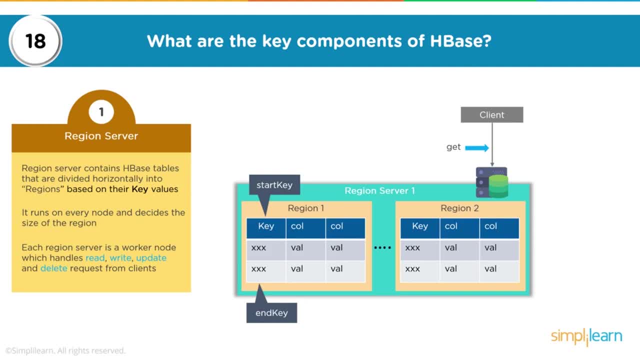 data node is running. So region server can have up to 1000 regions. It runs on every node and decides the size of region. So region server, as I said, is a slave process which is responsible for managing HBase data on. 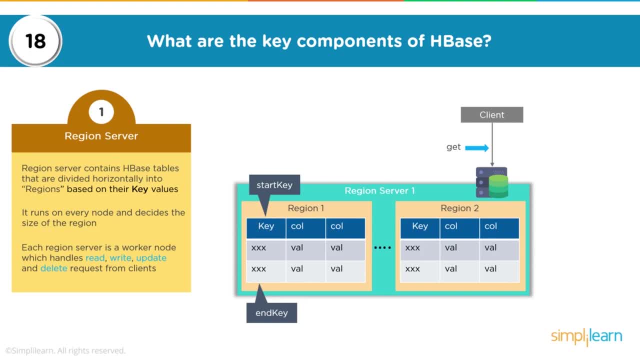 the node. Each region server is a worker node or a worker process co-located with data node, which will take care of your read, write, update, delete request from the clients. Now, when we talk about more components of HBase, as I said, 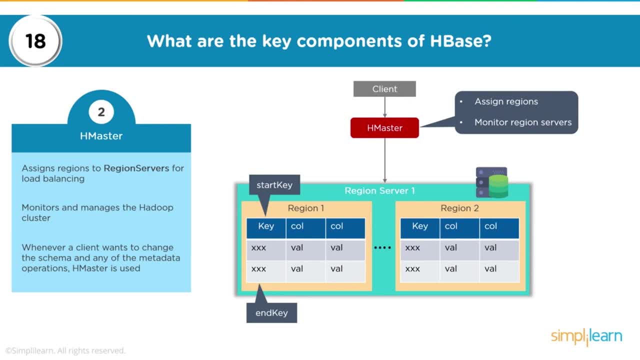 region server is a master, So you would always have a connection coming in from a client or an application. What does HMaster do? It assigns regions, It monitors the region servers, It assigns regions to region servers for load balancing, And it cannot do that without the 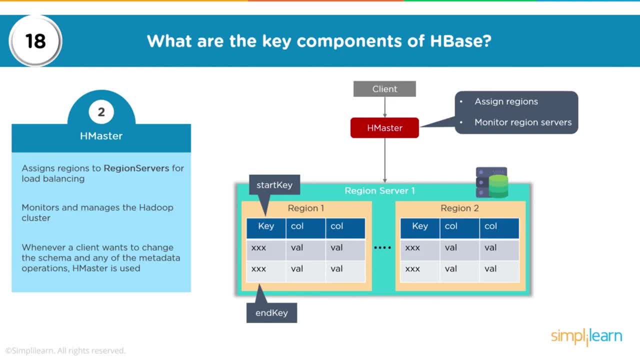 help of ZooKeeper. So if we talk about components of HBase, there are three main components: You have ZooKeeper, you have HMaster and you have region server, Region server being the slave process, your HMaster being the master process which takes care of all your table operations. 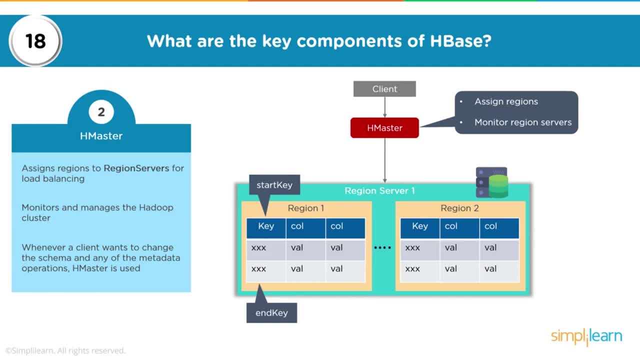 assigning regions to the region servers taking care of read and write requests which come from client. And for all of this HMaster will take in help of ZooKeeper, which is a centralized coordination service. So whenever a client wants to read or write or change the schema, 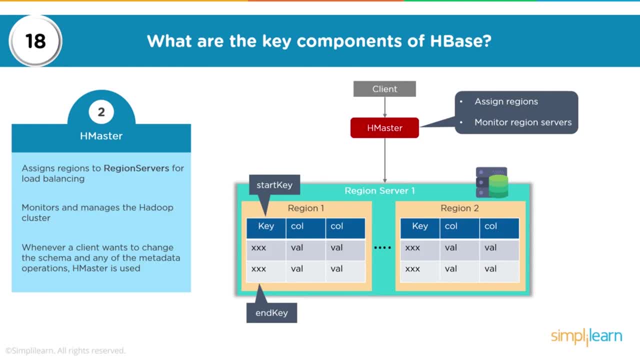 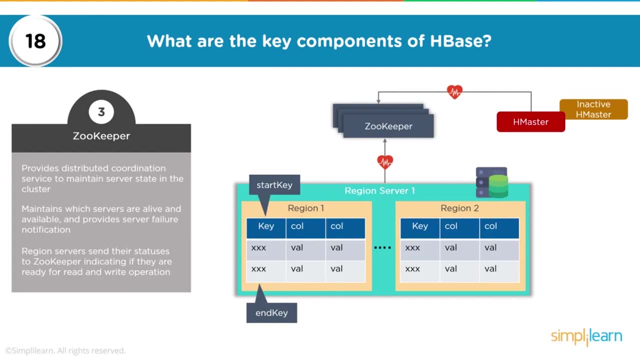 or any other metadata operations, it will contact HMaster. HMaster internally will contact HMaster. HMaster internally will contact HMaster. HMaster internally will contact HMaster. So you could have HBase set up also in high availability mode where you could have an. 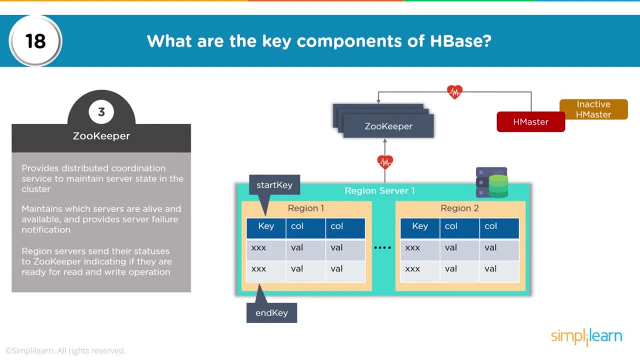 active HMaster and a backup HMaster, You would have a ZooKeeper quorum, which is the way ZooKeeper works. So ZooKeeper is a centralized coordination service which will always run with a quorum of processes. So ZooKeeper would always run with odd number of processes, such as three, five. 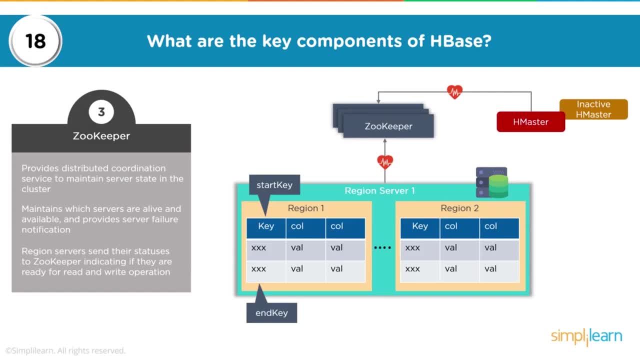 and seven because ZooKeeper works on the concept of maturity consensus. Now ZooKeeper, which is a centralized coordination service, is keeping a track of all the servers which are alive, available, and also keeps a track of their status For every server. 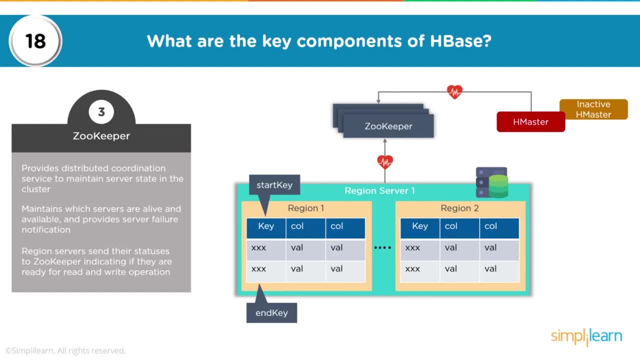 with ZooKeeper is monitoring. ZooKeeper keeps a session alive with that particular server. HMaster would always check with ZooKeeper which region servers are available alive so that regions can be assigned to the region server. At one end you have region server which are sending their status to the 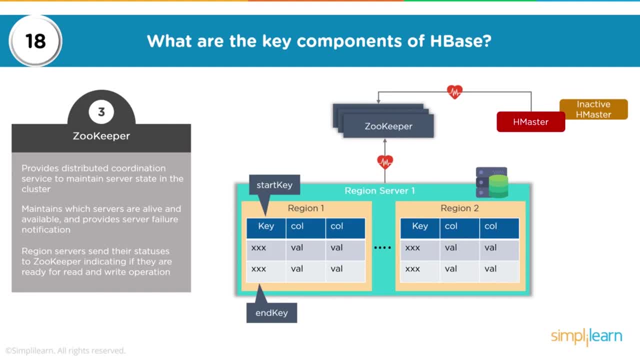 ZooKeeper indicating if they are ready for any kind of read or write operation And, at other end, HMaster is querying the ZooKeeper to check the status. Now ZooKeeper internally manages a meta table. Now that meta table will have information of which regions are residing on which region. 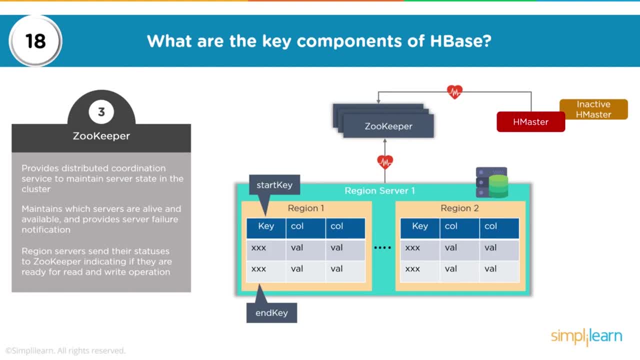 server and what row keys those regions contain. So in case of a read activity, HMaster will query ZooKeeper to find out the region server which contains that meta table. Once HMaster gets the information of meta table, it can look into the meta table to find out the row. 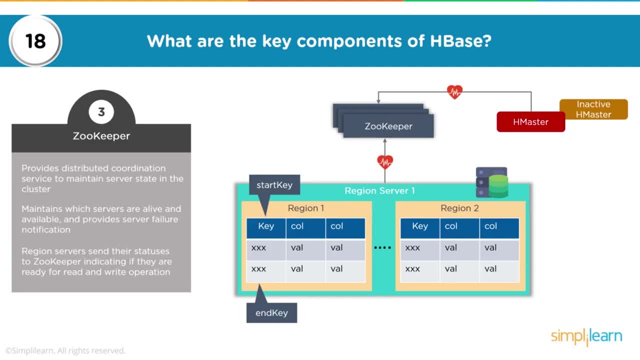 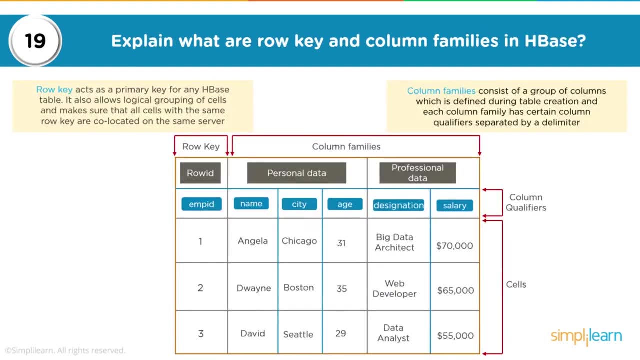 keys and the corresponding region servers which contain the regions for those row keys. Now, if we would want to understand row key and column families in HBase, let's look at this and it would be good if we could look this on an Excel sheet. So row key is: 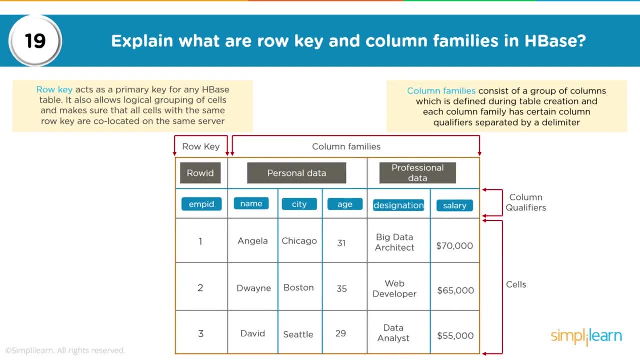 unique. It acts as a primary key for any HBase table. It allows logical grouping of cells and makes sure that all cells with the same row key are co-located on the same server. So, as I said, you have four coordinates for HBase. You have a row key which is always unique. You have column. 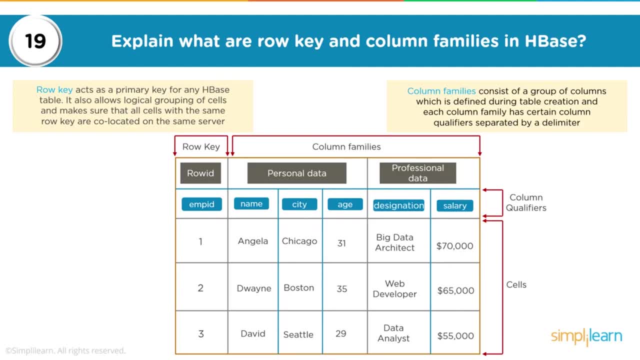 families, which is nothing but group of columns. And when I say column families, one column family can have any number of columns. So when I talk about HBase, HBase is four dimensional And in terms of HBase it is also called as a. 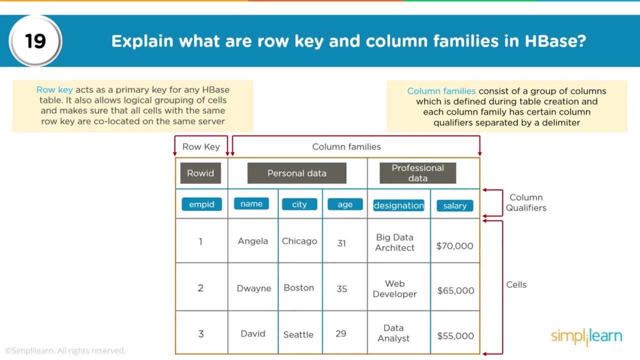 column oriented database, which basically means that every row in one column could have a different data type. Now you have a row key which uniquely identifies the row. You have column families, which could be one or many, depending on how the table has been defined, And a column family can have any. 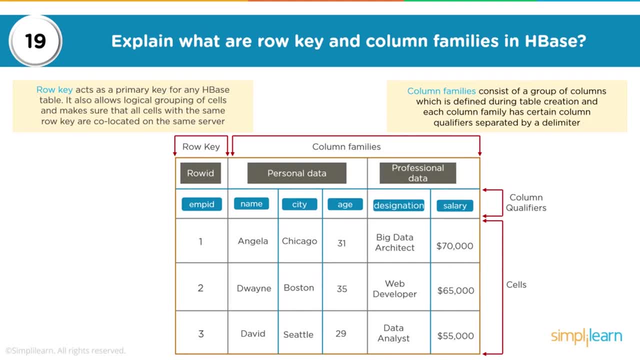 number of columns. Or I could say for every row within a column family you could have different number of columns. So I could say for my row one I could just have two columns, such as name and city, within the column family. For my row two, 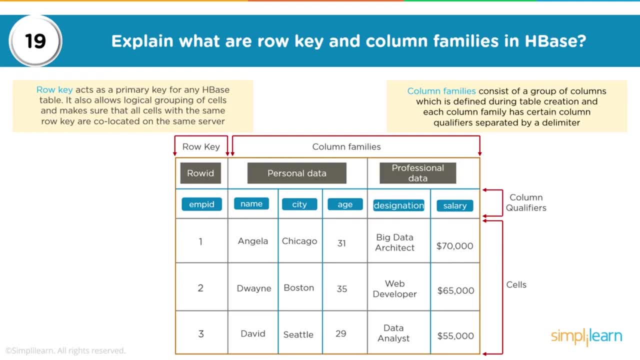 I could have name, city, age, designation, salary. For my third row. I could have thousand columns and all that could belong to one column family. So this is a horizontally scalable database. So column family consists of group of columns which is defined. 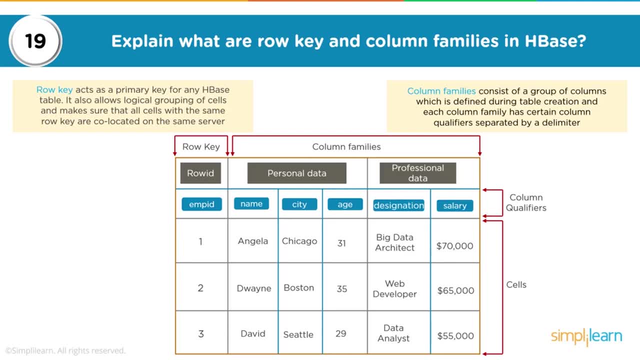 during table creation And each column family can have any number of column qualifiers separated by a delimiter. Now a combination of row key, column, family, column qualifier, such as name, city, age and the value within the cell makes the HBase a unique four dimensional. 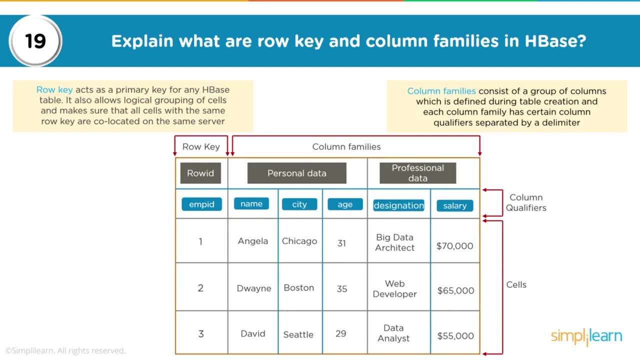 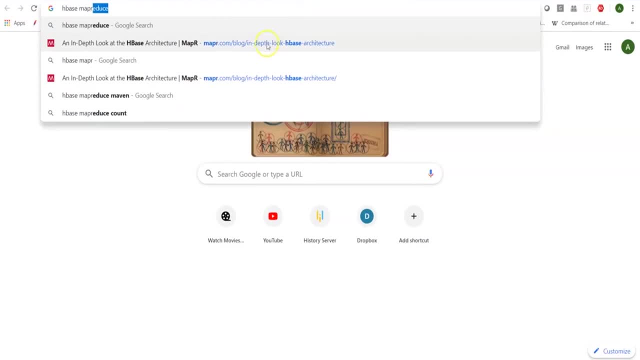 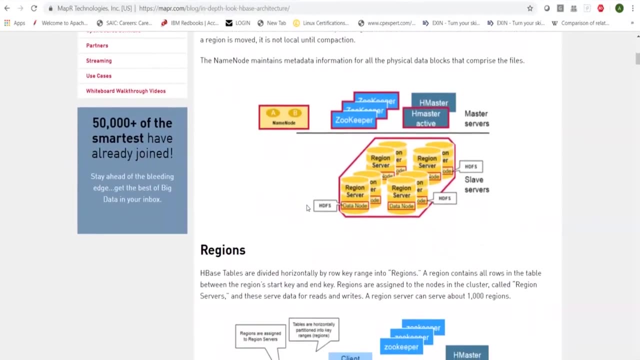 database For more information. if you would want to learn on HBase, please refer this link, which is HBase, and this gives a complete HBase architecture. That is, three components of name node. three components that is name node, region servers and ZooKeeper- how it works. 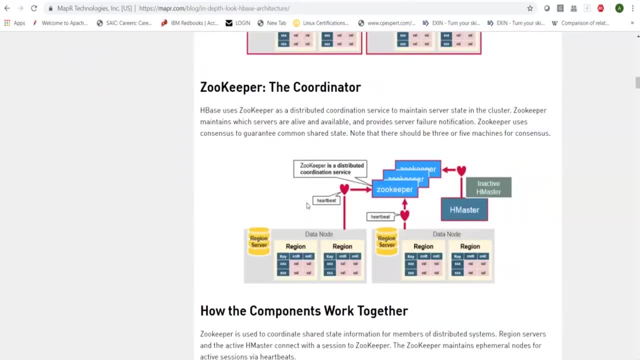 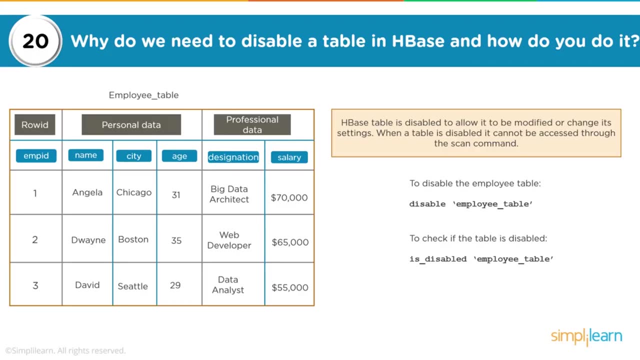 how HBase HMaster interacts with ZooKeeper, what ZooKeeper does in coordination, how are the components working together and how does HBase take care of read and write, Coming back and continuing? why do we need to disable a table? So there are different. 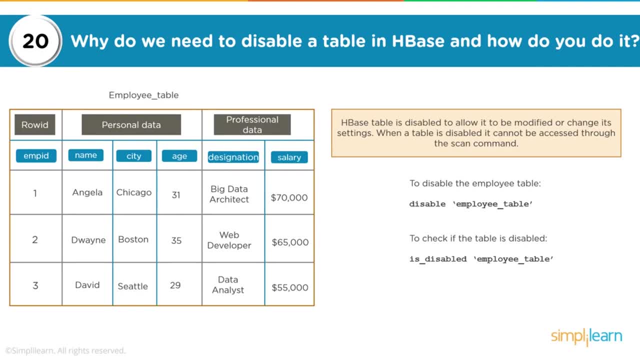 table operations, What you can do in HBase, and one of them is disabling a table. Now, if you would want to check the status of table, you could check that by is disabled and giving the table name or is enabled and the table name. So the question is: why do we need to disable a table Now? 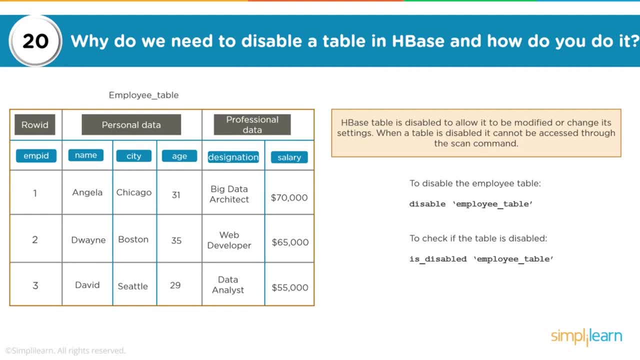 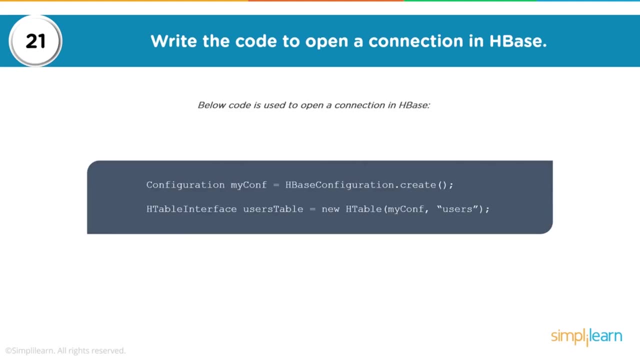 if we would want to modify a table or we are doing some kind of maintenance activity. in that case we can disable the table so that we can modify or change its settings. When a table is disabled, it cannot be accessed. This is through the scan command. Now, if we have to write a code to open a connection, 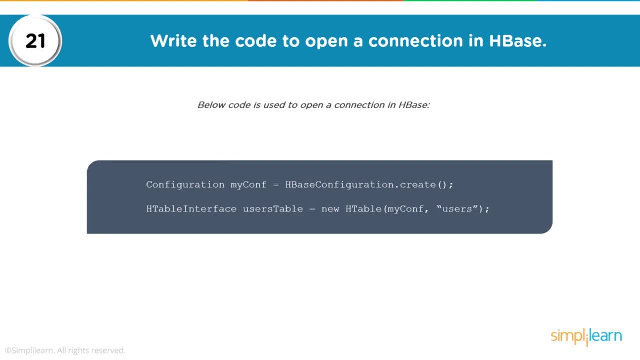 in HBase. Now, to interact with HBase, one could either use a graphical user interface such as Hue, or you could be using the command line HBase shell, or you could be using HBase admin API if you are working with Java, or say HappyBase if you are working with Python. 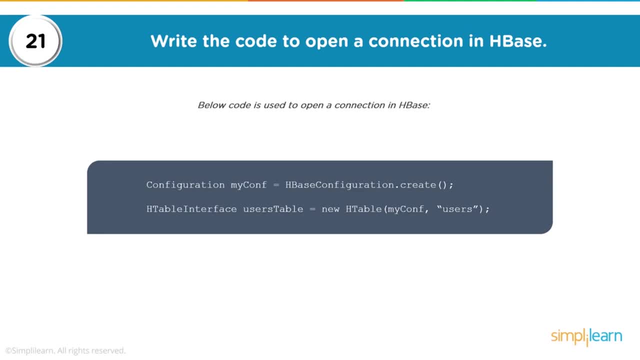 where you may want to open a connection with HBase so that you can work with HBase programmatically. In that case, you can use the command line HBase shell, or you could be using HBase admin API if you are working with Java. 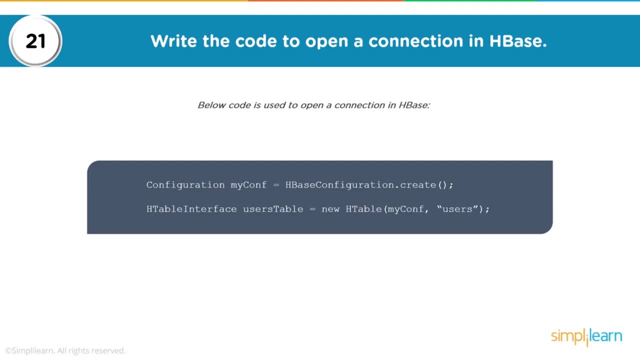 In HBase we have to create a configuration object, that is configuration myconf, and then create a configuration object and then you can use different classes, like H table interface. to work on a new table, You could use H column qualifier and many other classes which are 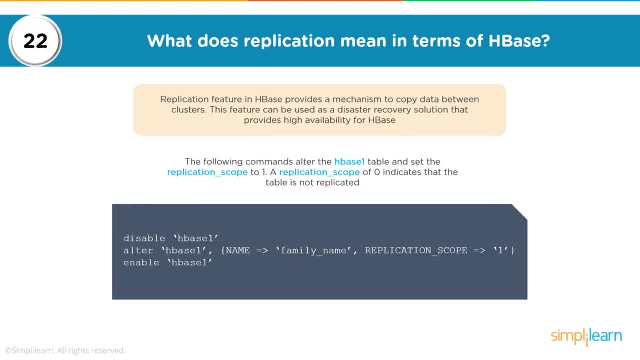 available in HBase admin API. What does replication mean in terms of HBase? So HBase, as I said, works in a cluster way And when you talk about cluster, you could always set up a replication from one HBase cluster to other HBase cluster. So this replication, 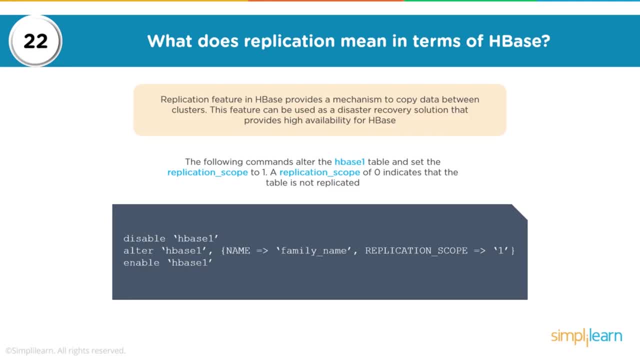 feature in HBase provides a mechanism to copy data between clusters or sync the data between different clusters. This feature can be used as a disaster recovery solution that provides high availability for HBase. So if I have HBase cluster one where I have one master, 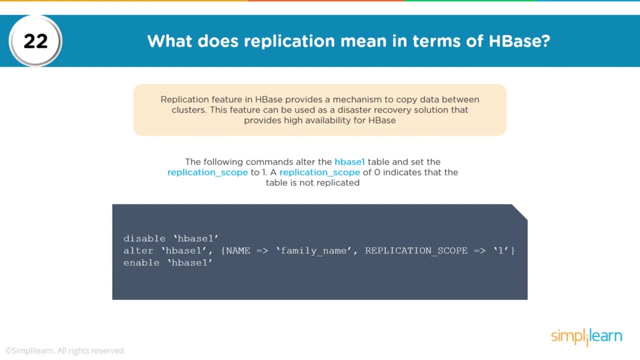 and multiple region servers running in a Hadoop cluster. I could use the same Hadoop cluster to create a HBase cluster, HBase replica cluster. or I could have a totally different HBase replica cluster, where my intention is that if things are changing in a particular table in cluster 1, I would want them to be. 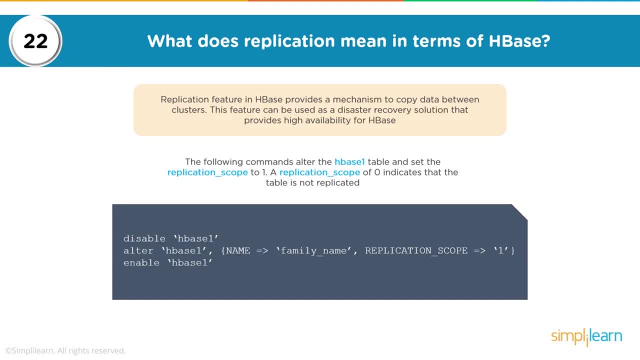 replicated across different clusters. So I could alter the HBase table and set the replication scope to 1.. Now, a replication scope of 0 indicates that table is not replicated. but if we set the replication to 1, we basically will have to set up a HBase cluster where we can replicate. 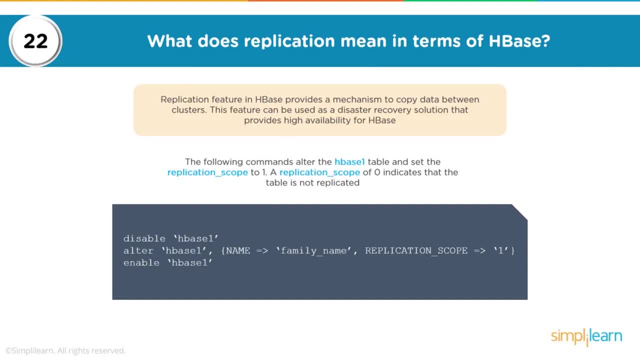 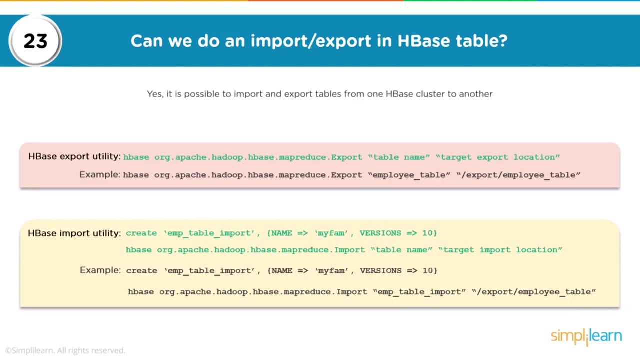 HBase tables data from cluster 1 to cluster. So these are the commands which can be used to enable replication and then replicate the data of table across clusters. Can we import and export in HBase? Of course we can. It is possible to import and export tables from one HBase cluster. 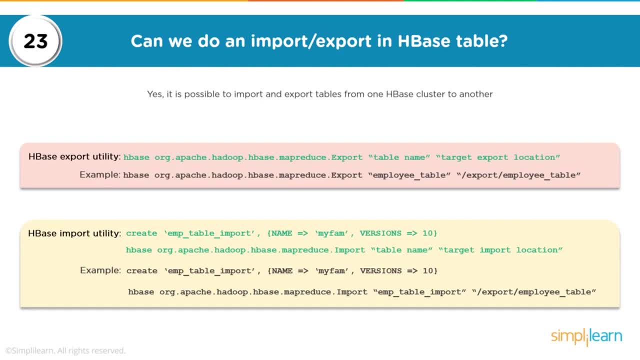 to other HBase cluster or even within a cluster. So we can use the HBase export utility Which comes in this particular package. give a table name and then a target location So that will export the data of HBase table into a directory on SDFS. Then I could create a different. 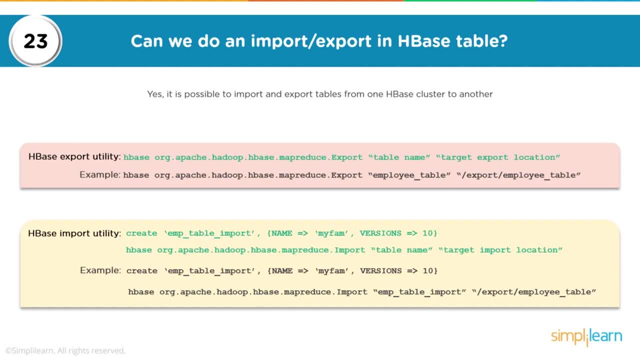 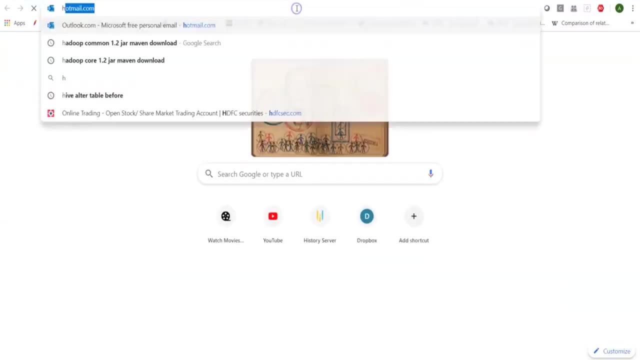 table which would follow some kind of same definition as the table which was exported, and then I could use import to import the data from the directory on SDFS to my table. If you would want to learn more on HBase import and export, you could look at. 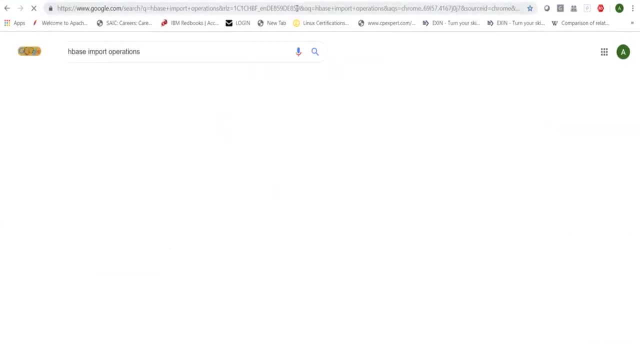 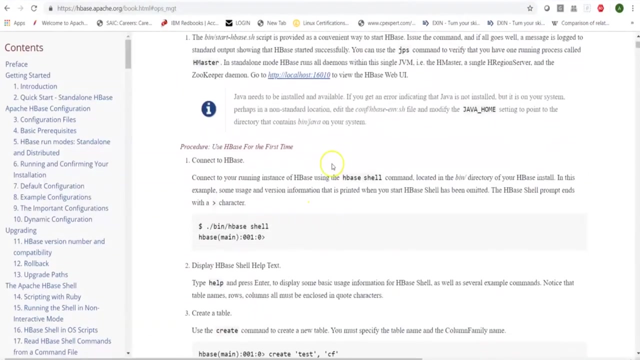 HBase import operations. Let's search for the link- And this is the link where you could learn more about HBase import export utilities, how you could do a bulk import, bulk export which internally uses MapReduce, And then you could do a import and export into HBase tables. 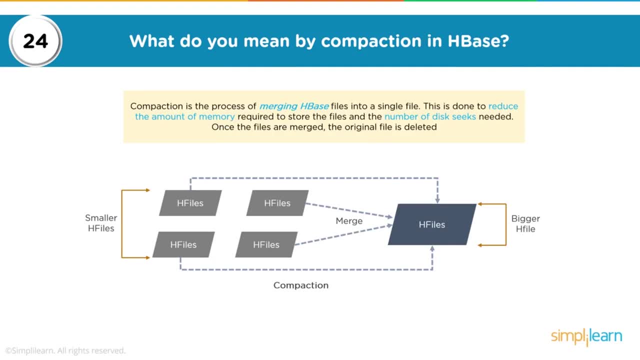 Moving further. what do we mean by compaction in HBase? Now we all know that HBase is a NoSQL database which can be used to store huge amount of data, So we can import and export data from data. However, whenever a data is written in HBase, it is first written to what we call as 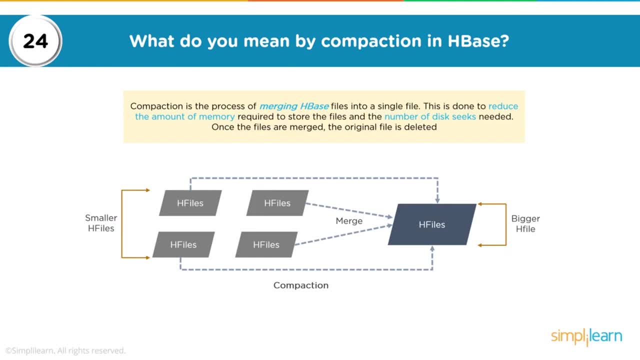 write ahead log and also to memstore, which is write cache. Now, once the data is written in ball and your memstore, it is offloaded to form an internal HBase format file which is called H file, And usually these H files are very small in nature. So we also know that SDFS is good when 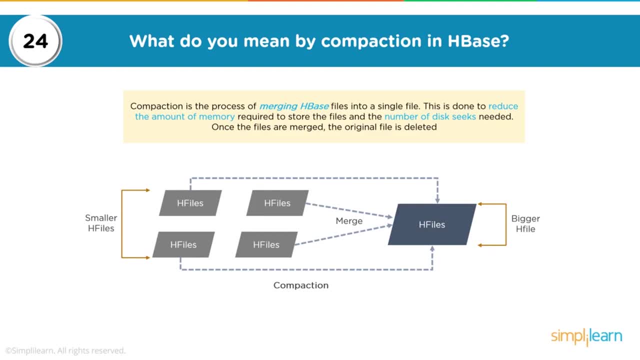 larger files in comparison to large number of smaller files due to the limitation of name nodes. memory Compaction is process of merging HBase files, that is, these smaller H files, into a single large file. This is done to reduce the amount of memory required to store the files. 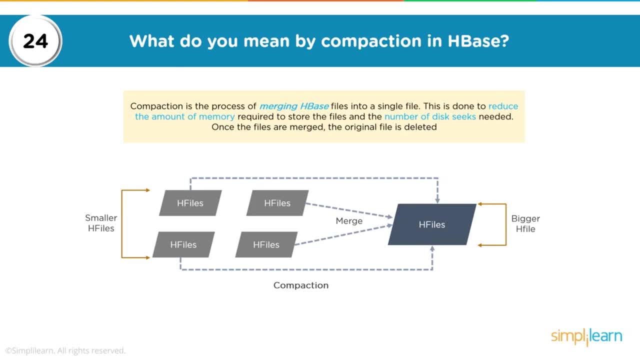 and number of disk seeks needed. So we could have a lot of H files which get created when the data is written to HBase And these smaller files can then be compacted through a smaller file. So we could have a major or minor compaction, creating one big H file which internally would 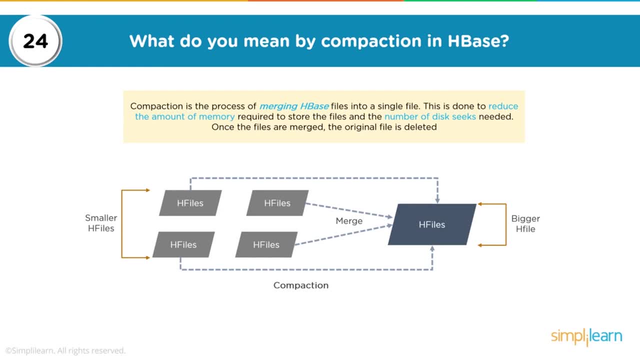 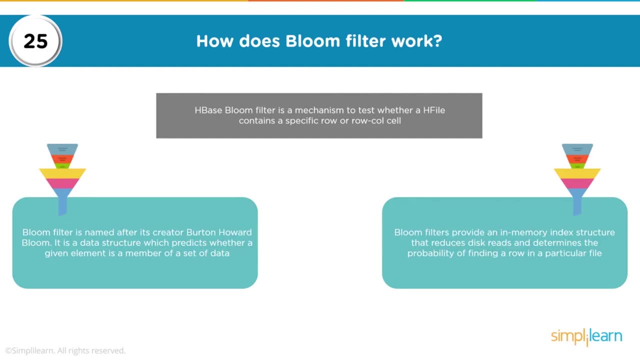 then be written to SDFS and SDFS format of blocks. That is the benefit of compaction. There is also a feature called bloom filter. So how does bloom filter work? So bloom filter, or HBase bloom filter, is a mechanism to test whether a H file contains a specific row or a row column. 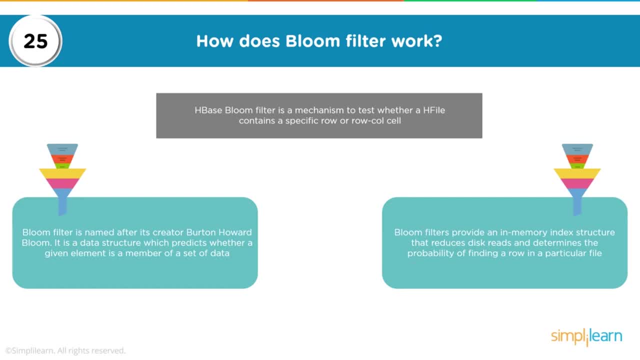 cell Bloom filter is named after its creator, Burton Howard. It is a data structure which predicts whether a given element is a member of a set of data. It provides an in-memory index structure that reduces the disk reads and determines the probability of finding a row in a particular file. This is one of very useful features of HBase. 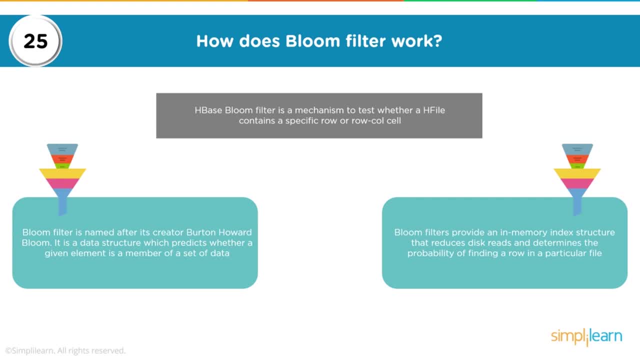 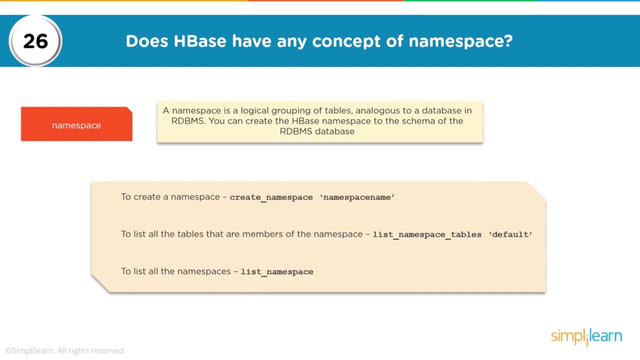 which allows for faster access and avoids disk seeks. Does HBase have any concept of namespace? So namespace is when you have similar elements grouped together, So namespace. yes, HBase supports namespace. So namespace is a logical grouping of tables analogous to a database in RDBMS, So you can create HBase namespace to. 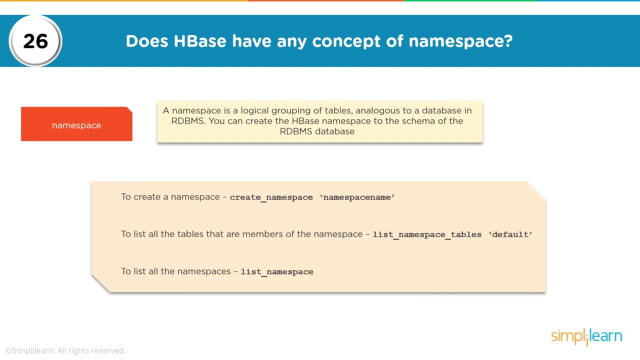 the schema of RDBMS database. So you could create a namespace by saying create namespace and giving it a name, And then you could also list the tables within a namespace. You could create tables within a specific namespace. This is usually done in production environment where a cluster might be multi-tenant cluster. 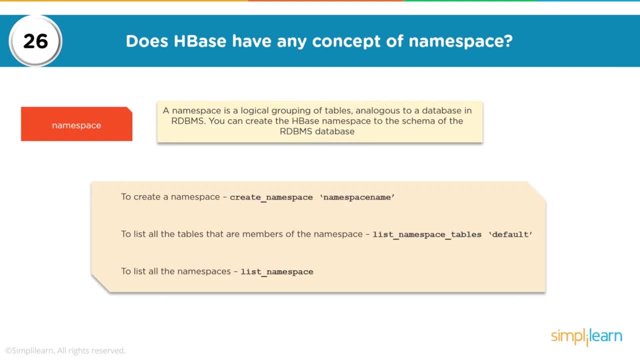 and there might be different users of the same NoSQL database. In that case, admin would create specific namespace And for specific namespace you would have different directories on HDFS and users of a particular business unit or a team can work on their HBase objects within. 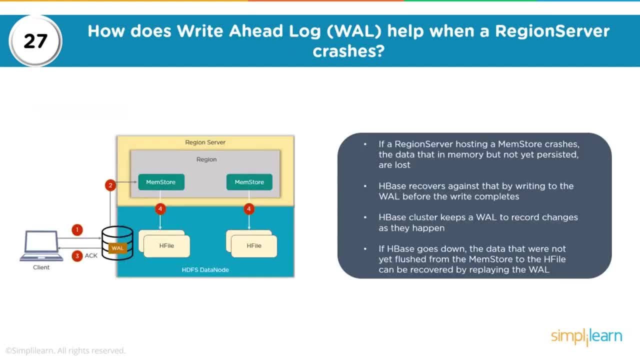 a specific namespace? This is a question which is, again, very important. It's important to understand about the writes or reads. So how does write ahead log wall help when a region server crashes? Now, as I said, when a write happens, it will happen. 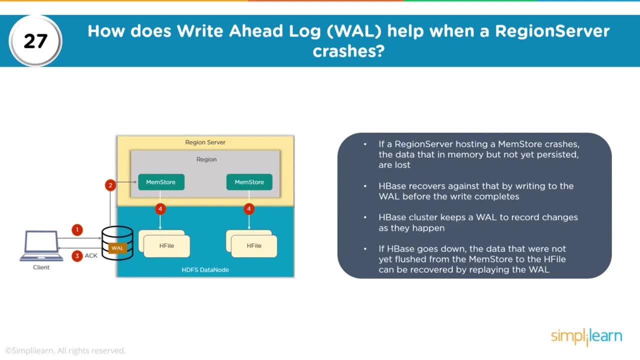 into memstore and wall, That is your edit log, or write ahead log. So whenever a write happens, it will happen in two places: memstore, which is the write cache, and wall, which is an edit log, Only when the data is written in both these places and based on the limitation. 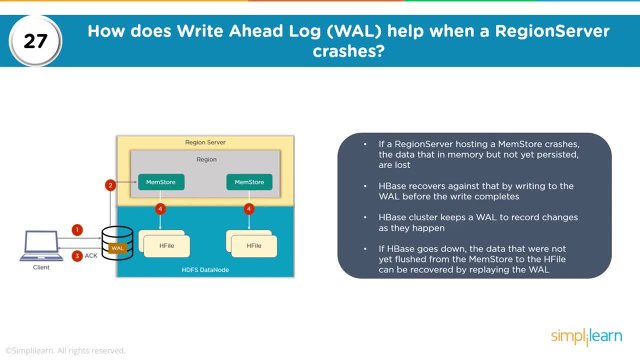 of memstore, the data will be flushed to create an HBase format file called hfile. These files are then compacted and created into one bigger file which will then be stored on HDFS. And HDFS data, as we know, is stored in the form of blocks on the underlying data nodes. So 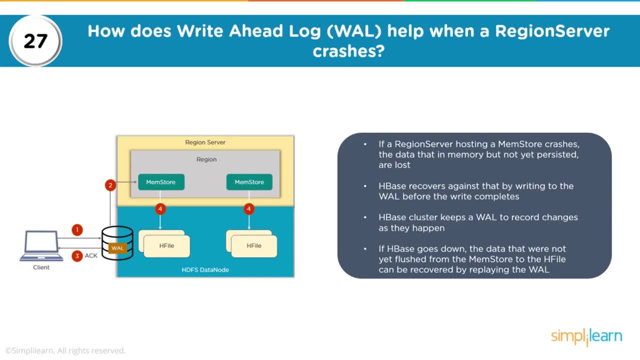 if a region server hosting a memstore crashes, now where is region server running? That would be co-located with data node. So if a data node crashes or if a region server which was hosting the memstore write cache crashes, data in memory, the data that in memory which was not. persisted is lost. now how does hbase recover from this? as i said, your data is written into wall and memstore at the same time. hbase recovers against that by writing to wall before the write completes. so whenever a write happens, it happens in memstore and wall at the same time. 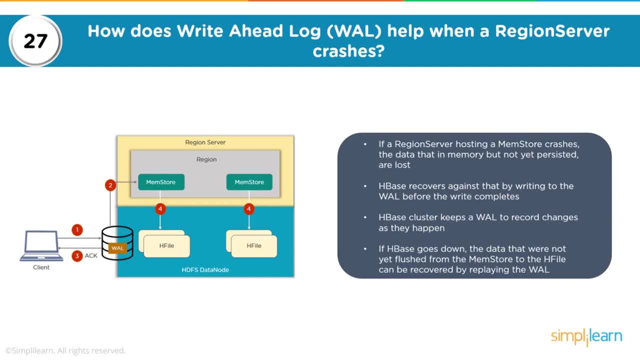 hbase cluster keeps a wall to record changes as they happen and that's why we call it as also an edit log. if hbase goes down or the node that goes down, the data that was not flushed from memstore to hfile can be recovered by replaying the write ahead log, and that's the benefit of your edit log. 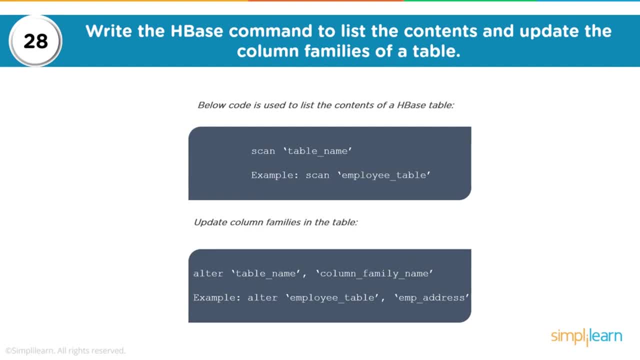 or write ahead log. now, if we would have to write hbase command to list the contents and update the column families of a table, i could just do a scan and that would give me the data that was not flushed from memstore to hfile, and that's the benefit of your edit log. 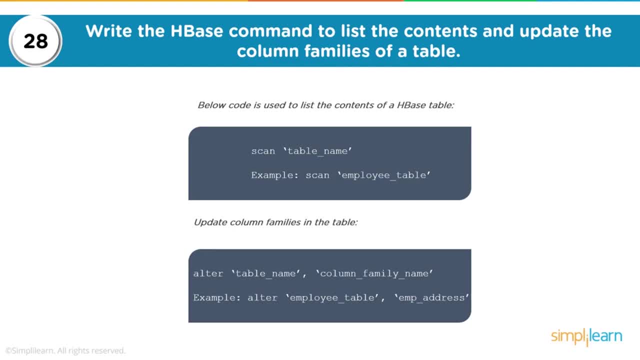 complete data of a table. if you are very specific and if you would want to look at a particular row, then you could do a get table name and then give the row key. however, you could do a scan to get the complete data of a particular table. you could also do a describe to see what are the different. 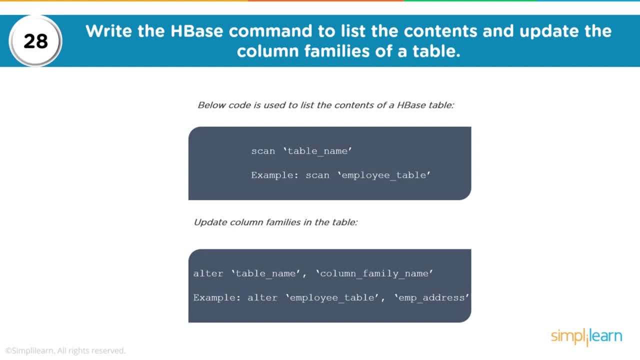 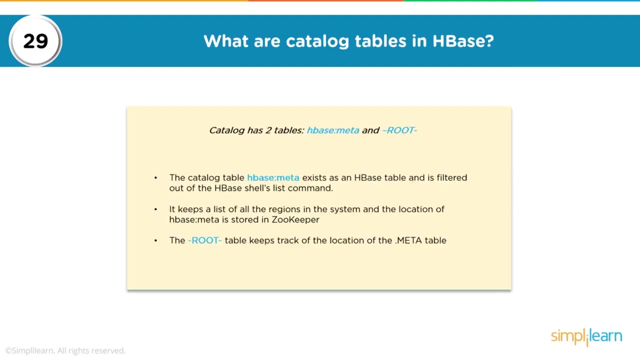 column families and if you would want to alter the table and add a new column family, it is very simple. you can just say alter, give the hbase table name and then give you a new column family name which will then be added to the table. what are catalog tables in hbase? so, as i mentioned, 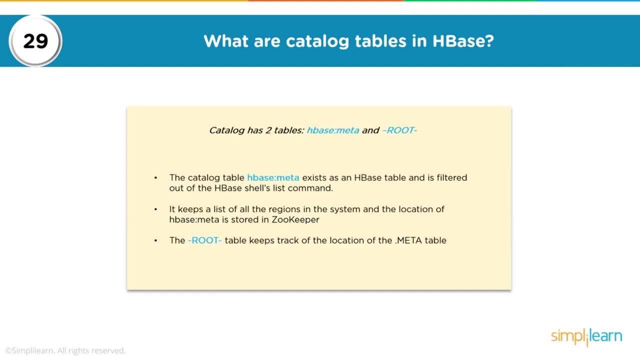 your zookeeper knows the location of this internal catalog table, or what we call as the meta table. now, catalog tables in hbase have two tables. one is hbase meta table and one is hyphen root. the catalog table hbase meta exists as an hbase table and is filtered out of hbase shells list command. 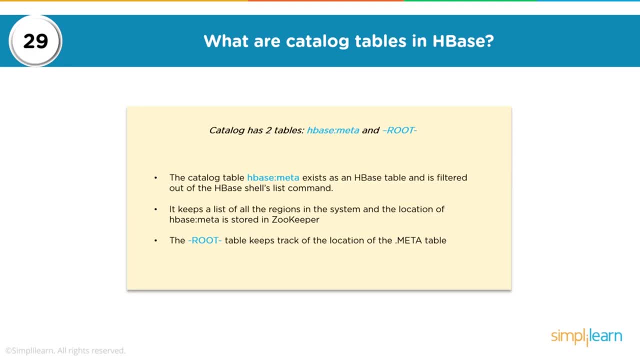 so if i give a list command and i give a list command and i give a list command and i give a list command on hbase, it would list all the tables which hbase contains, but not the meta table. it's an internal table. this meta table keeps a list of all regions in the system and location of hbase meta stored. 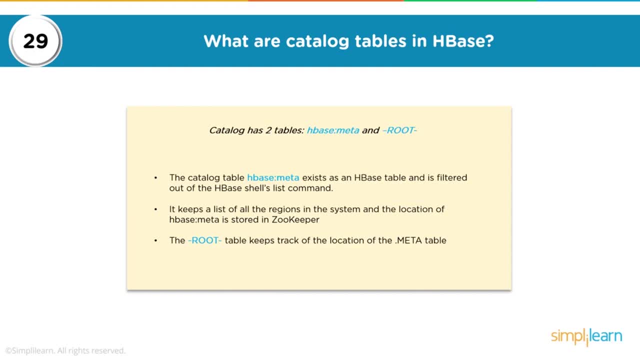 in zookeeper. so if somebody wants to find out or look for particular rows, they need to know the regions which contain that data and those regions are located on region server. to get all this information, you need to know the regions which contain that data and those regions are located. 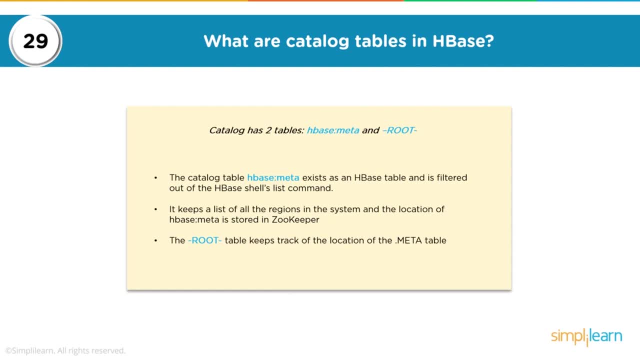 one has to look into this meta table. however, we will not be looking into meta table directly. we would just be giving a write or a read operation. internally, your hbase master queries the zookeeper. zookeeper has the information of where the meta table exists and that meta table which is existing. 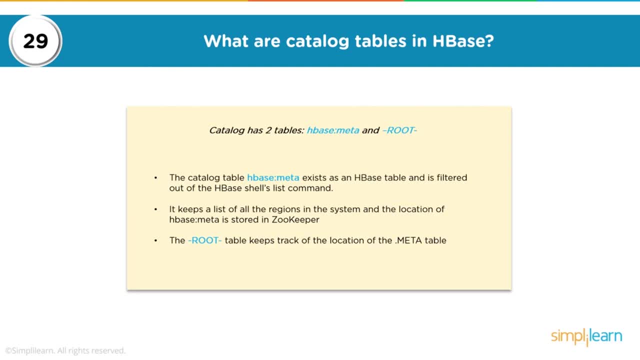 on region server contains information of row keys and the region servers where those rows can be found. your root table keeps a track of location of the region server and the region server contains data. so if somebody GOES right to the region server, that will create that data, and if somebody 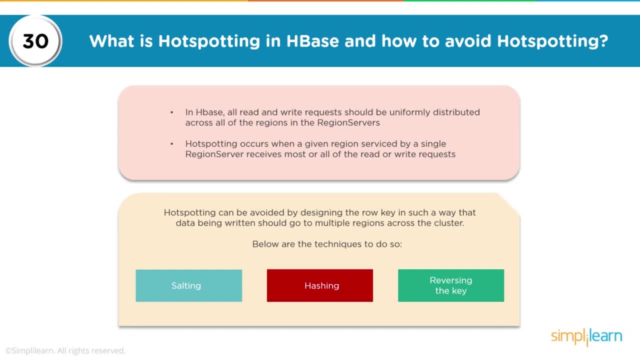 at the region server connection strucks to the region server which is inside the region server. that's whenroz Nh or hbase forremansizetcom. so then we need to make it happen. if you need to create that data integration rules. basically any site would replace the data, so we need a. 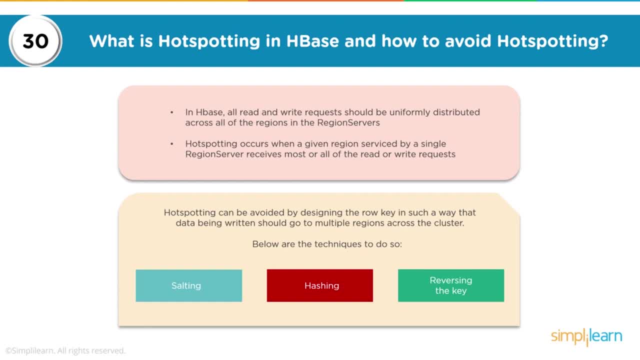 public dedicated data where idle data etc. and the address or location of this data transfer should not be turned into aernist of any Seoul data. the interface should not read into any lok disk or this voting problem. normally developers remove the phrase rightly. takes care, you can also show around the virtual isarten, whoever you are operating, in which I thought. 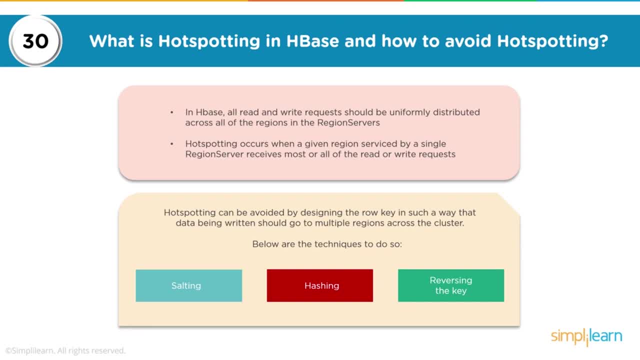 anyways is not. which have the email address? are you with whatever in yourTwoCenter? is the? So you would have your data stored across region servers in the form of regions, which are horizontal partitions of the table, And whenever read and write requests happen, they should be uniformly distributed across all the regions in the region servers. 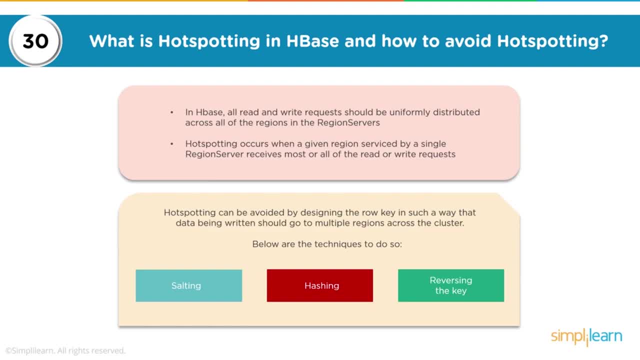 Now hotspotting occurs when a given region serviced by a region server receives most or all of read and write requests, which is basically an unbalanced way of read write operations. Now, hotspot can be avoided by designing the row key in such a way that data being written should go to multiple regions across the cluster. 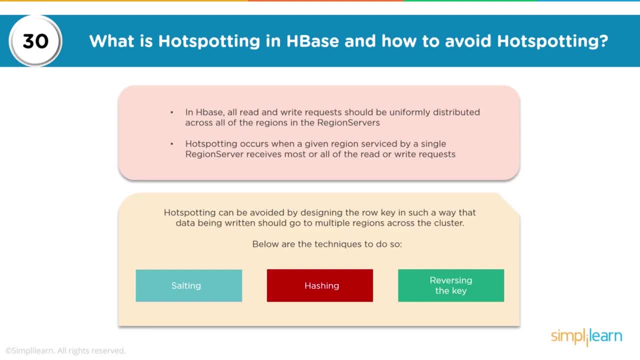 So you could do techniques such as salting, hashing, reversing the key and many other techniques which are employed by users of HBase. We need to just make sure that when the regions are distributed across region servers, they should be spread across region servers. 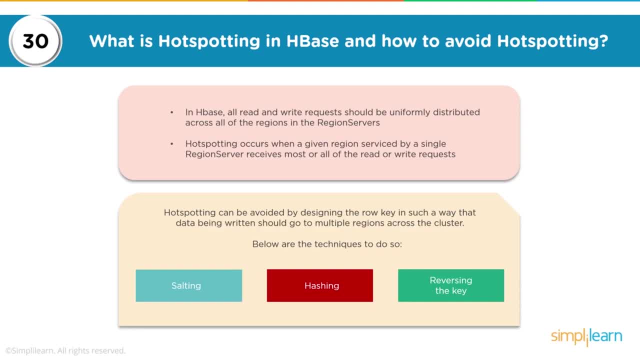 so that your read and write requests are distributed across region servers, So that your read and write requests can be satisfied from different region servers in parallel, rather than all read and write requests hitting the same region server, overloading the region server, which may also lead to the crashing of a particular region server. 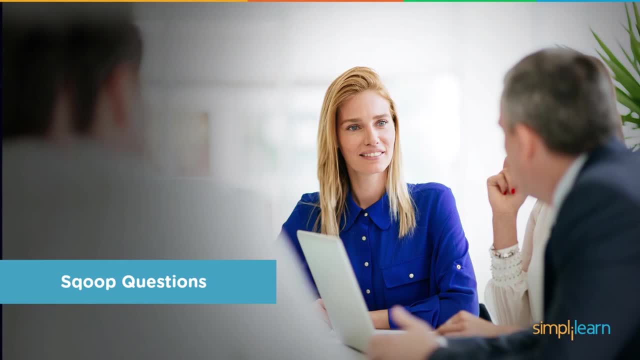 So these were some of the important questions of HBase, and then there are many more. Please refer to the link which I specified during my discussion and that gives you a detailed explanation of how HBase works. You can also look into it. 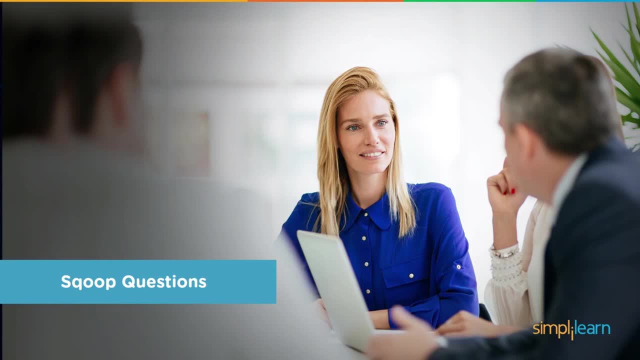 HBase Definitive Guide by O'Reilly or HBase in Action, and these are really good books to understand about HBase internals and how it works. Now that we have learned on Hive, which is a data warehousing package, we have learned on PIG, which is a scripting or a scripting language, 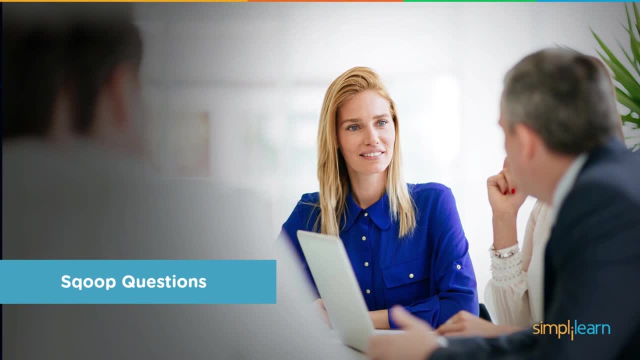 which allows you to do data analysis, and we have learned some questions on a NoSQL database. Just note it that there are more than 225 NoSQL databases existing in Microsoft And if you would want to learn and know about more NoSQL databases, you can just go to Google and type nosqldatabasesorg. 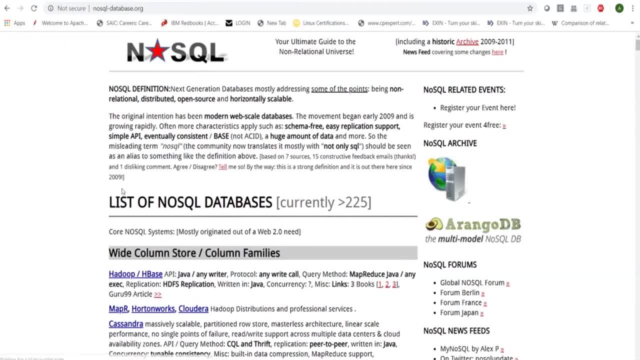 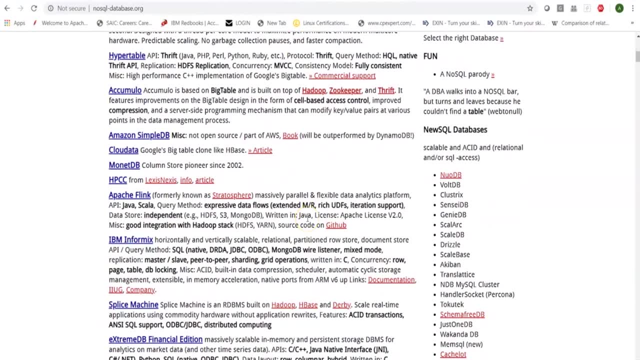 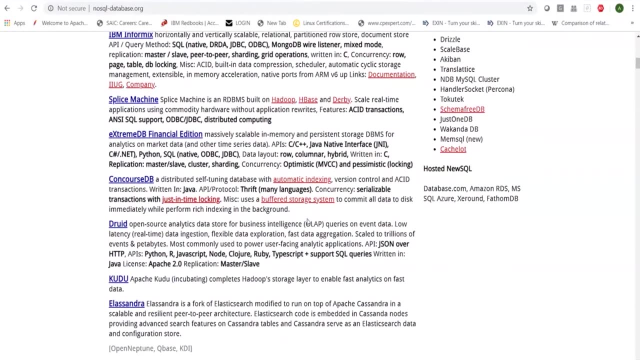 and that will take you to the link, which is for NoSQL databases, and this shows there are more than 225 NoSQL databases existing in market, and these are for different use cases, used by different users and with different features. So have a look. 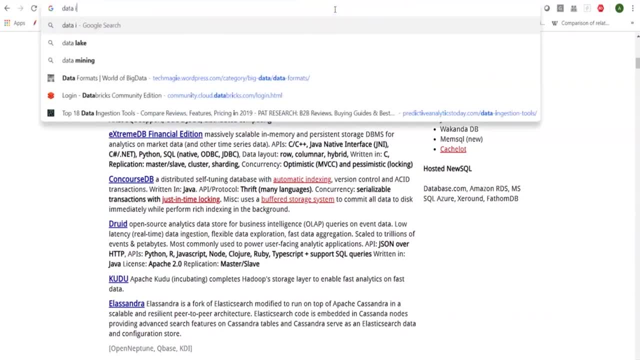 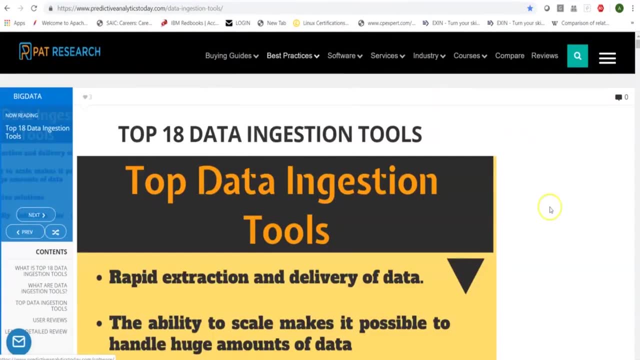 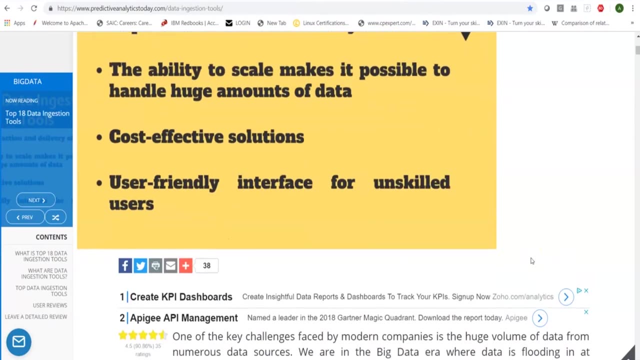 Now when you talk about data ingestion, so let's look at data ingestion and this is one good link which I would suggest to have a look at, which lists down around 18 different ingestion tools. So, when you talk about different data ingestion tools, some are for structured data, some are for streaming data. 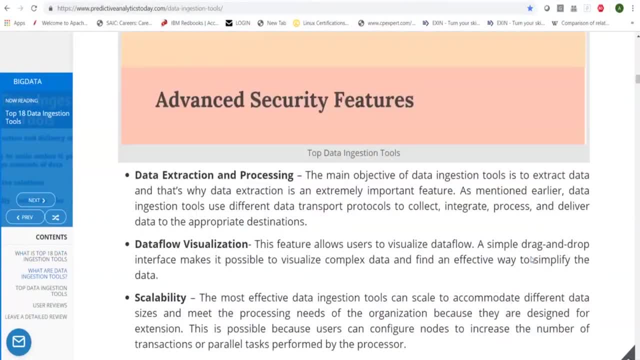 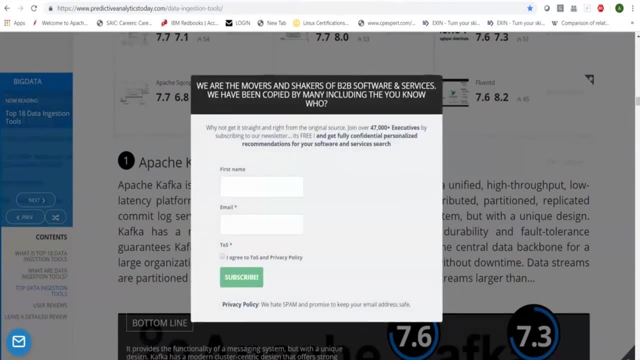 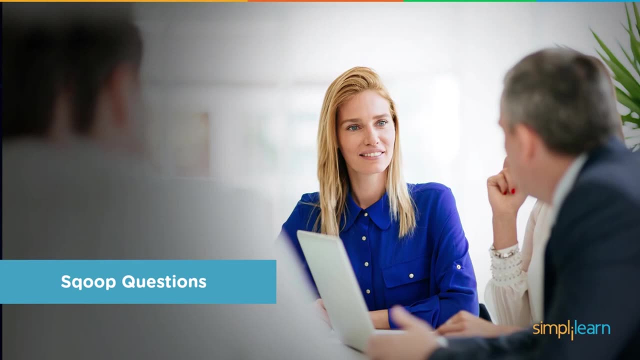 some are for data governance, some are for data ingestion and transformation and so on. So have a look at this link, which also gives you a comparison of different ingestion tools. So here let's learn about some questions on Scoop, which is one of the data ingestion tools mainly used for structured data. 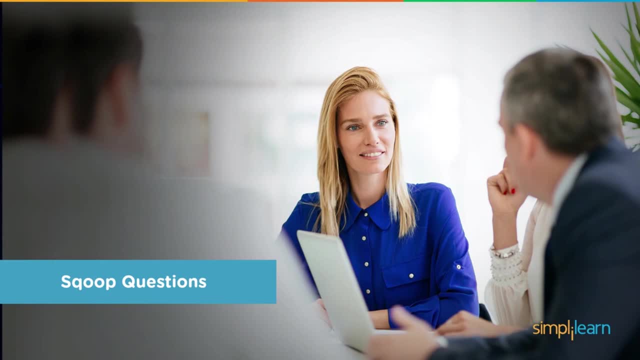 or you could say data which is coming in from RDBMS, or data which is already structured and you would want to ingest that. you would want to store that on SDFS, which could then be used for Hive, which could be used for any kind of processing. 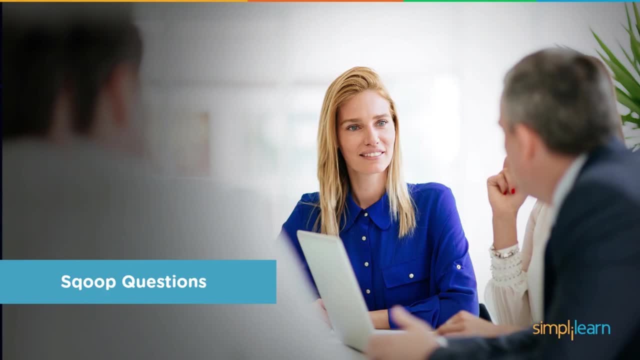 using MapReduce or Hive or Payless or Spark or any other processing frameworks, or you would want to load that data into, say, Hive or HBase tables. Scoop is mainly for structured data. It is extensively used when organizations are migrating from RDBMS to a big data platform. 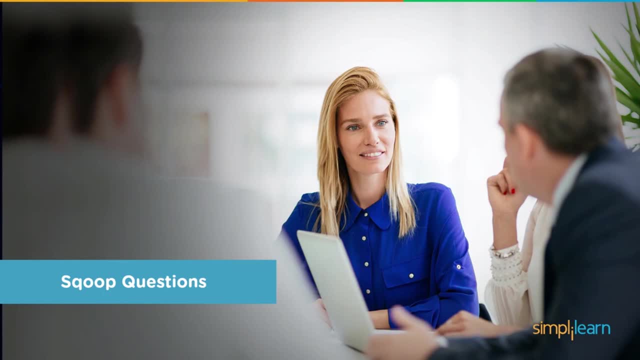 and they would be interested in ingesting the data. that is, doing import and export of data from RDBMS to SDFS or vice versa. So let's learn about some important questions. So let's learn about some important questions on Scoop which you may be asked by an interviewer when you apply for a big data-related position. 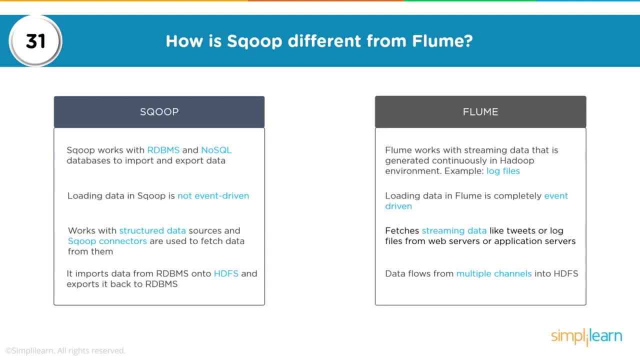 How is Scoop different from Flume? So this is a very common question which is asked. Scoop, which is mainly for structured data, So Scoop works with RDBMS. It also works with NoSQL databases to import and export data. 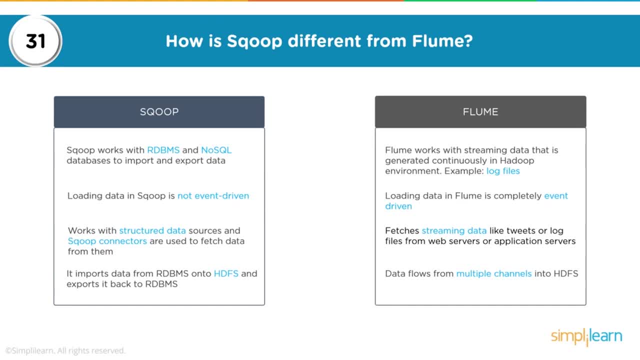 So you can import data into SDFS. You can import data into data warehousing packets such as Hive directly Or also in HBase, And you could also export data from Hadoop ecosystem to your RDBMS. However, when it comes to Flume, Flume is more of a data ingestion tool which works with streaming data or unstructured data. 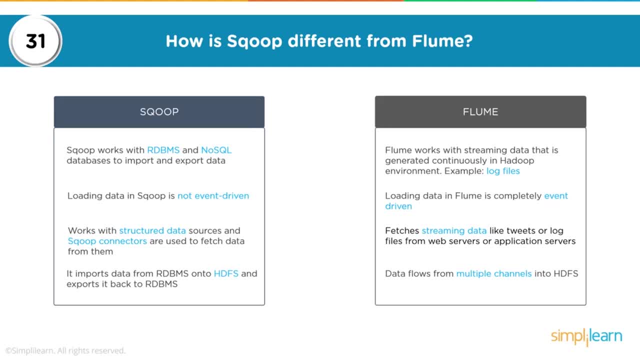 So data which is constantly getting generated, for example log files or metrics from server or some chat messenger and so on. So if you are interested in working on capturing and storing the streaming data in a storage layer such as SDFS or HBase, you could be using Flume. 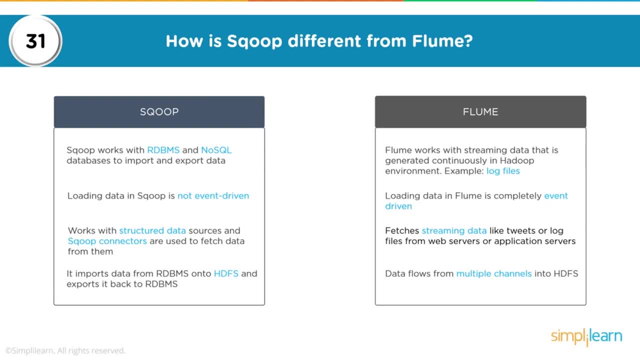 There could be other tools also, like Kafka or Storm or Chukwa or Samza, NiFi and so on. Scoop, however, is mainly for structured data. Your loading data in Scoop is not event-driven, So it is not based on event. 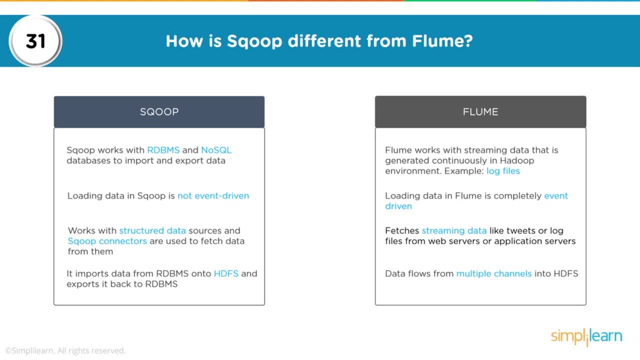 It basically works on data which is already stored in RDBMS. In terms of Flume, it is completely event-driven, That is, as the messages or as the events happen as the data is getting generated. you can have that data ingested using Flume. 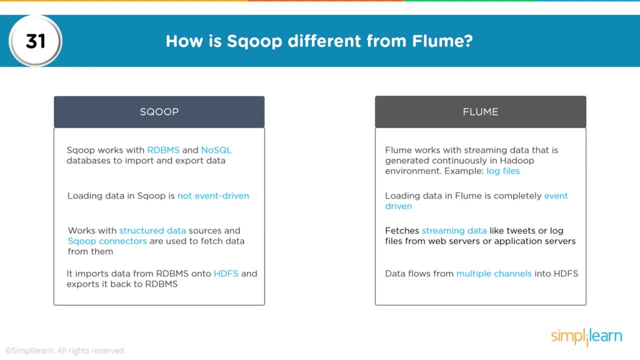 Scoop works with structured data sources and you have various Scoop connectors which are used to fetch data from external data structures or RDBMS. So for every RDBMS, such as MySQL, Oracle, TV2, Microsoft SQL Server, you have different connectors which are available. 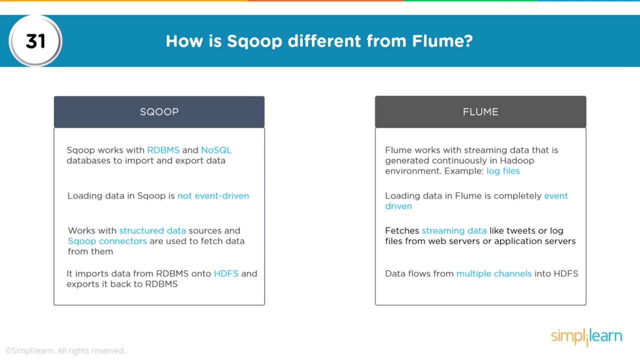 Flume. It works on fetching streaming data, such as tweets or log files or server metrics, from your different sources where the data is getting generated, And if you are interested in not only ingesting that data which is getting generated in a streaming fashion, but if you would be interested in processing the data as it arrives. 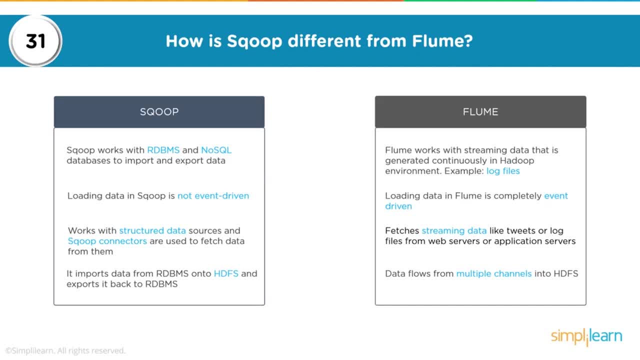 Scoop can import data from RDBMS onto SDFS and also export it back to RDBMS. Flume is then Used for streaming data. Now you could have one to one, one to many or many to one kind of relation. 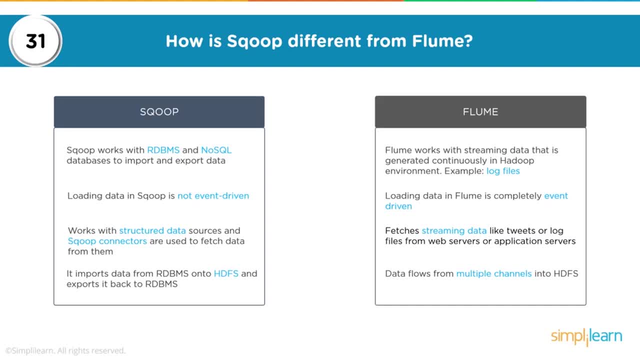 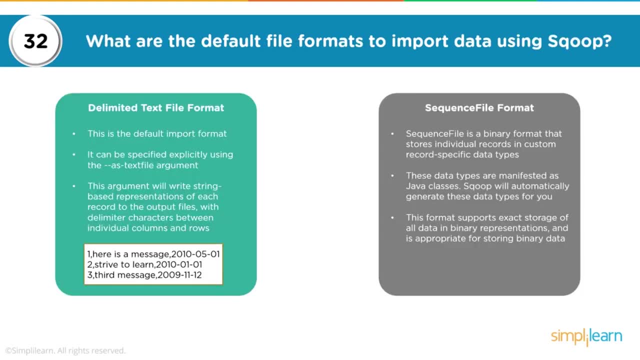 So, in terms of Flume, you have components such as your source, sync and channel. That's the main difference between your Scoop and Flume. What are the different file formats to import data using Scoop? Well, there are lots and lots of formats in which you can import data into Scoop. 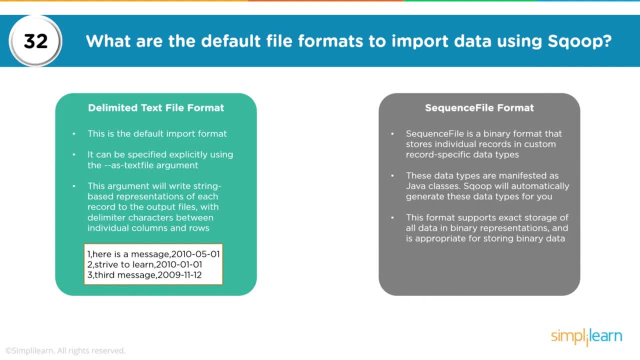 When you talk about Scoop, you can have delimited text file format. Now that's the default import format. It can be specified explicitly using as text file argument. So when I want to import data from an RDBMS, I could get that data in SDFS using different compression schemes or in different formats using the specific arguments. 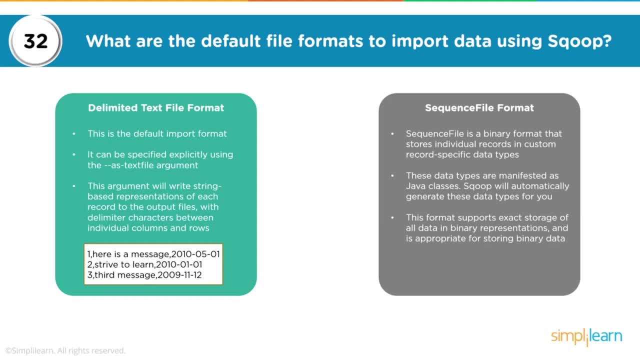 So I could specify an argument which will write string based representation of each record to output files with delimiters between individual columns and rows. So that is the default format which is used to import data using Scoop. So to learn more about your Scoop and different arguments which are available, you can click on scoopapacheorg. 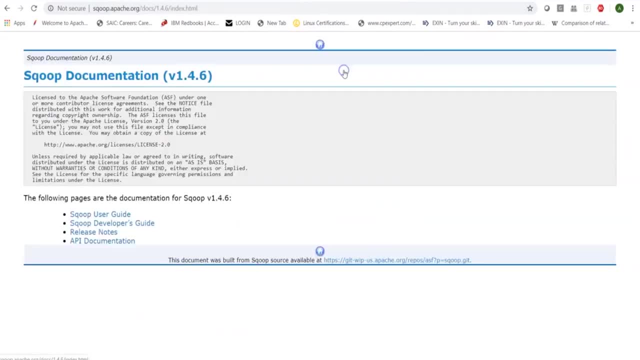 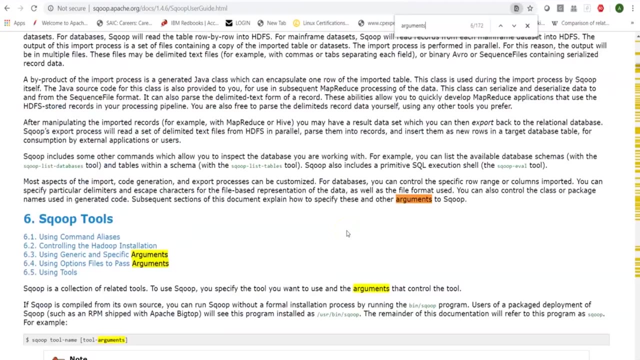 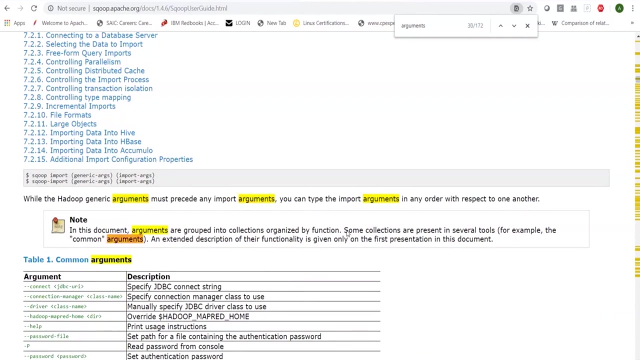 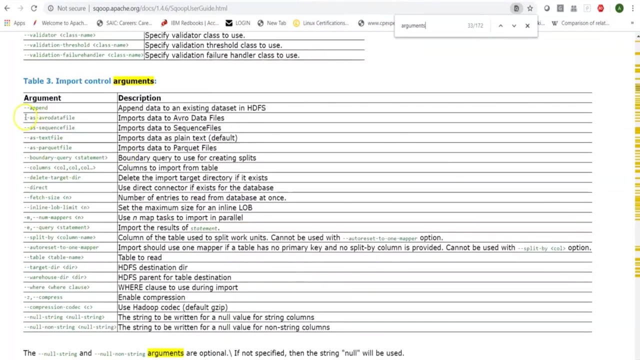 You can look into the documentation- and I would suggest choosing one of the versions and looking into the user guide- And here you can search for arguments and look for specific control arguments which show how you can import data Using Scoop. So here we have common arguments, and then you also have import control arguments, wherein we have different options, like getting data as app row, as sequence file, as text file or parquet file. 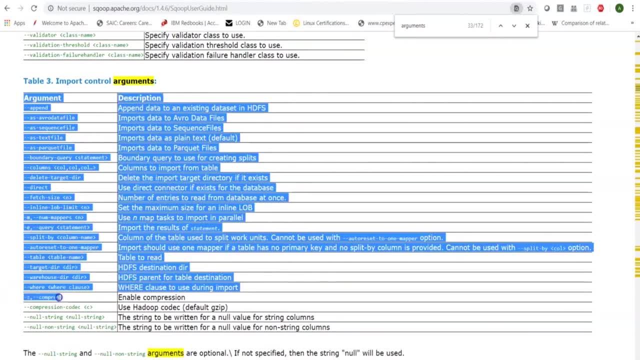 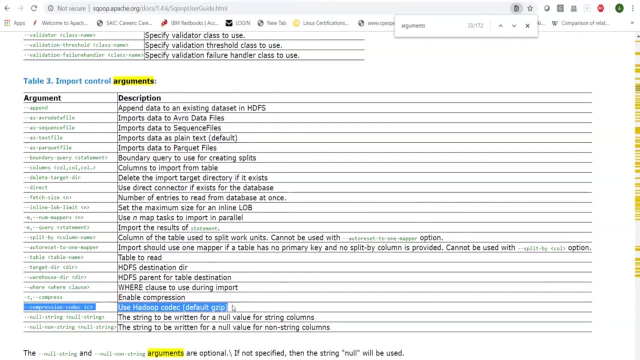 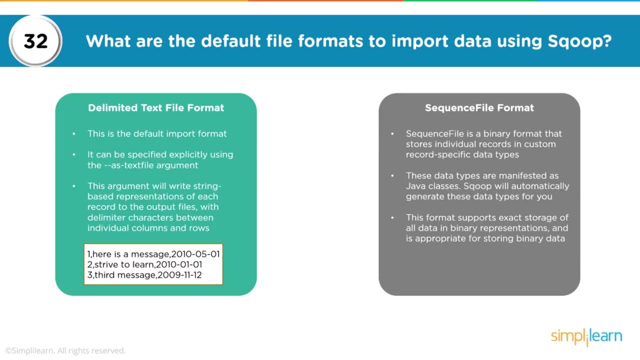 These are different formats. You can also get data in default compression scheme, that is, gzip, or you can specify compression codec and then you can specify what compression mechanism you would want to use when you are importing your data using Scoop. When it comes to default format for flume, we could say sequence file, which is a binary format that stores individual records in record, specific data types. 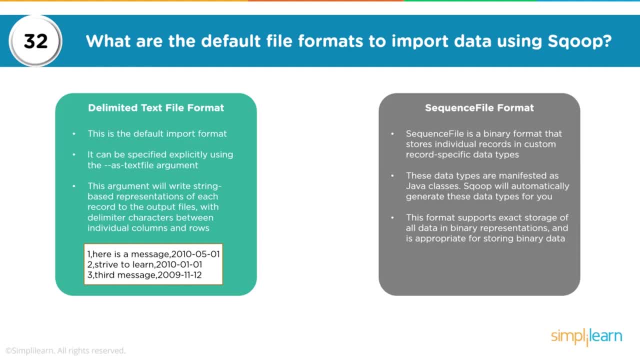 So these data types are manifested as Java classes and Scoop will automatically generate these data types for you. So Scoop does that. When we talk about your sequence file format, in terms of your Scoop you could be extracting storage of all data in binary representation. 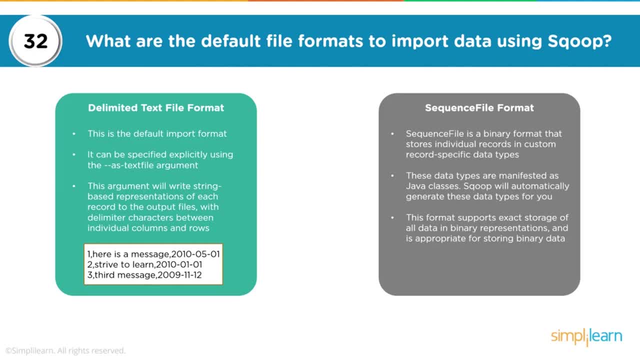 So, as I mentioned, you can import data in different formats, such as app, row, parquet sequence file, that is, binary format, or machine readable format, and then you could also have data in different compression schemes. Let me just show you some quick examples here. 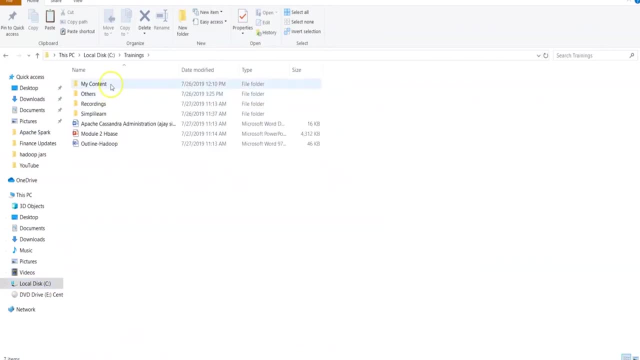 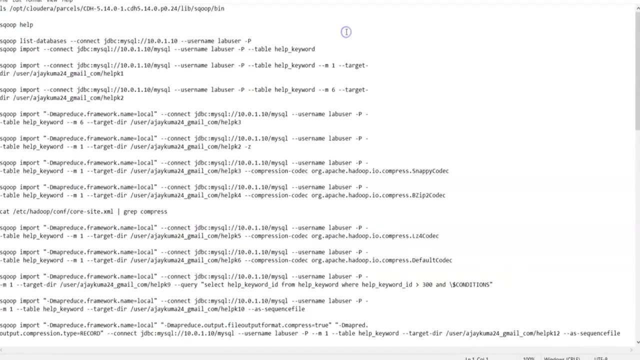 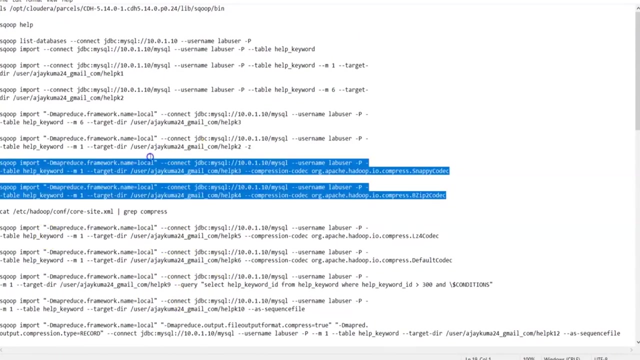 So if I look in the content and here I could search for a Scoop based file where I have listed down some examples. So if I would want to use different Compression schemes, Here are some examples. Have a look at these. So I'm doing a Scoop import. 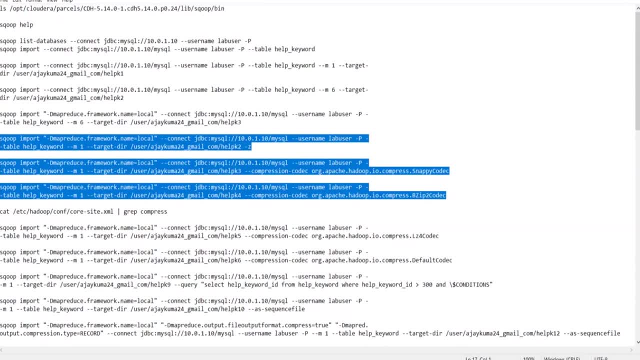 I'm also giving an argument so that Scoop, which also triggers a map reduce job, but I would say map only job. So when you run a Scoop import it triggers a map only job, No reduce happens here. and you could specify this parameter or this argument on the command line map reduce, dot, framework, dot name, so that you could run your map only job in a local mode. 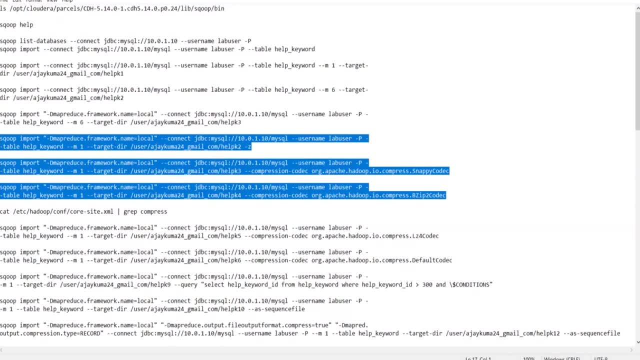 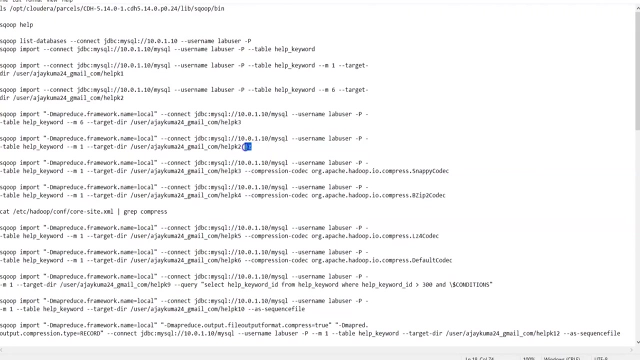 To save time, or that would interact with yarn and run a full-fledged map only job. We can give the connection and then connect to whatever our DBMS We are connecting, mentioning the database name. give your username and password, Give the table name, give a target directory, or it would create a directory same as the table name, which would work only once, and then I could say minus Z to get data in a compressed format. 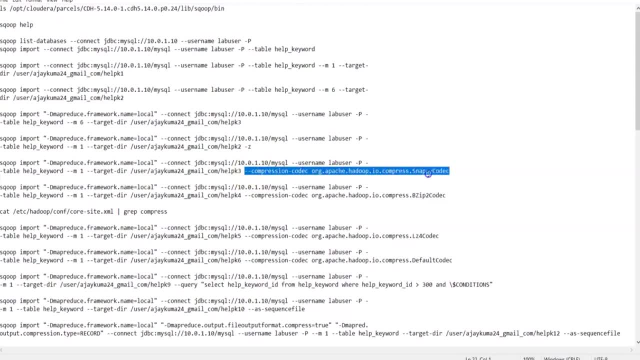 That is gzip, or I could be specifying compression codec and then I could specify What compression codec I would want to use. say, snappy is LZ for default. I could also run a query by giving a scoop import and when I'm specifying a query- and if you notice I've not given any table name because that would be included in the query- 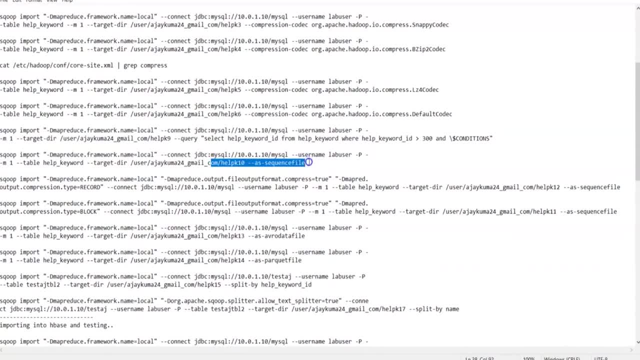 I can get my data as a sequence file format, which is a binary format, which will create a huge file. So we could also have compression enabled and then I could say: the output of my map job should use a compression At record level for my data coming in sequence file. 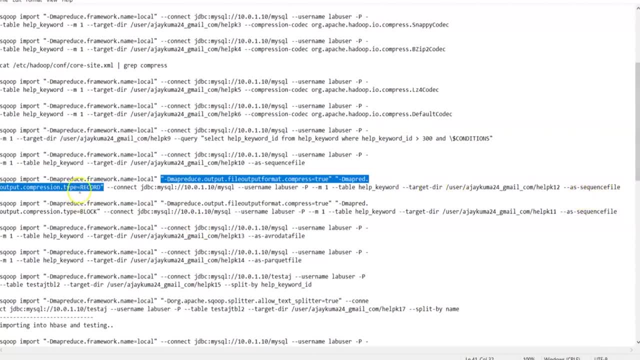 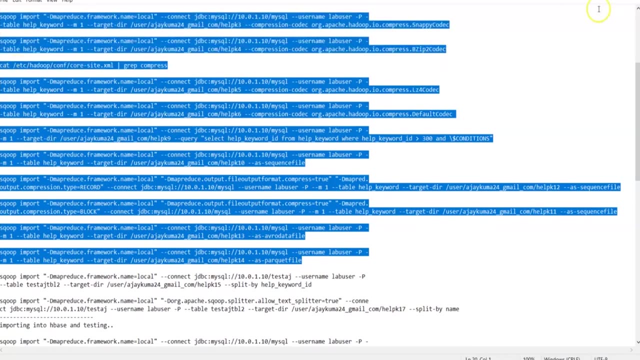 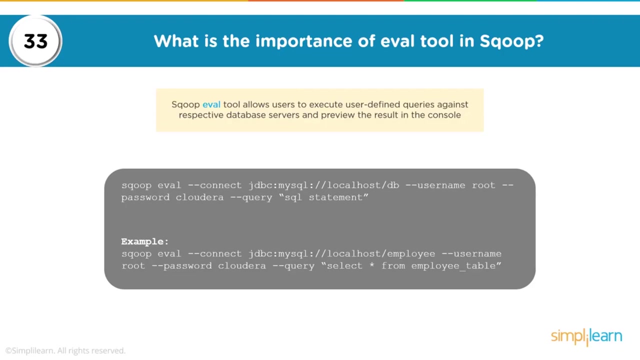 So sequence file or a binary format supports compression at record level or at block level. I could get my data in a Avro file where data has embedded schema within the file, or a parquet file also. So these are different ways in which you can set up different compression schemes, or you can even get data in different formats and you could be doing a simple scoop import for these. looking further, 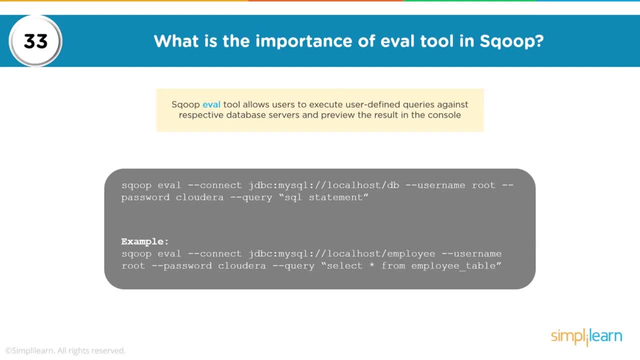 What is the important Tense of eval tool in scoop? So there is something called as eval tool. So scoop eval tool allows users to execute user-defined queries against respective database servers and preview the result in the console. So either I could be running a straight-away query to import the data into my HDFS or I could just use scoop eval, connect to my external RDBMS, specify my username and password and then I could be giving in a query. 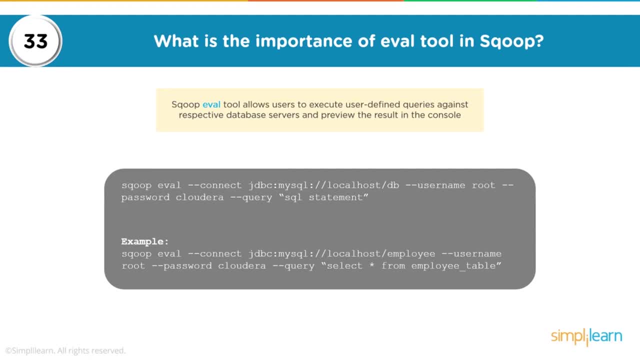 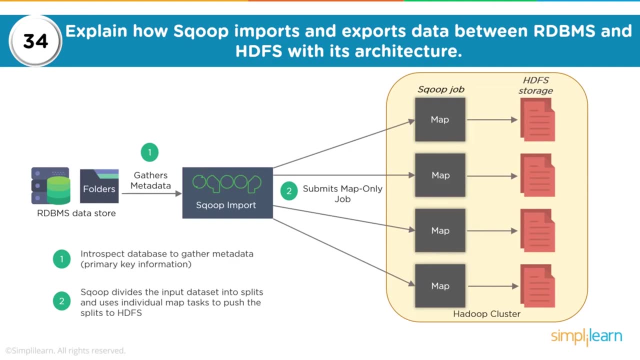 To see what would be the result of the query which we intend to import. Now let's learn about how scoop imports and exports data between RDBMS and HDFS with its architecture. So RDBMS, as we know, has your database structures, your tables, which all of them are logical, and internally there is always metadata which is stored. your scoop import connects to an external RDBMS. 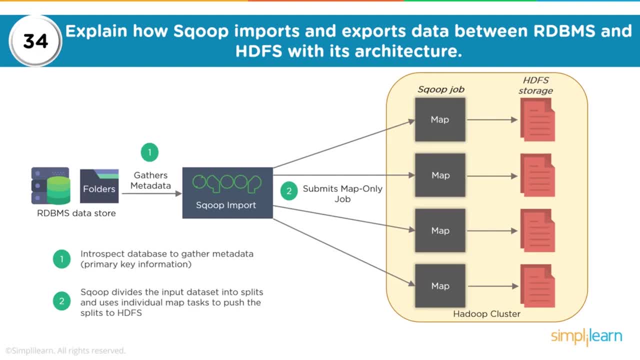 And for this connection It uses an internal connector jar file which has a driver class. So that's something which needs to be set up by admin. but they need to make sure that whichever RDBMS you intend to connect to, they need to have the JDBC connector for that particular RDBMS stored within the scoop lib folder. 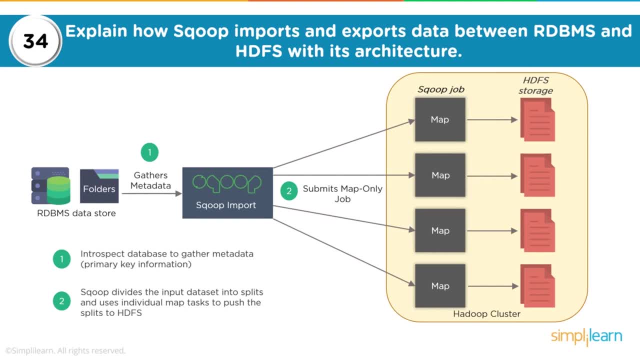 So scoop import gets the metadata and then for your scoop command it converts that into a map only job Which might Have one or multiple map tasks. Now that depends on your scoop command. You could be specifying that you would want to do a import only in one task or in multiple tasks. 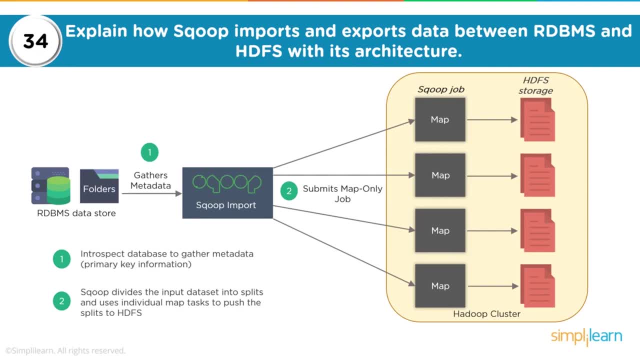 These multiple map tasks will then run on a section of data from RDBMS and then store it in HDFS. So at high level we could say scoop will introspect database to get gather the metadata. It divides the input data set Into splits and this division of data into splits mainly happens on primary key column of the table. 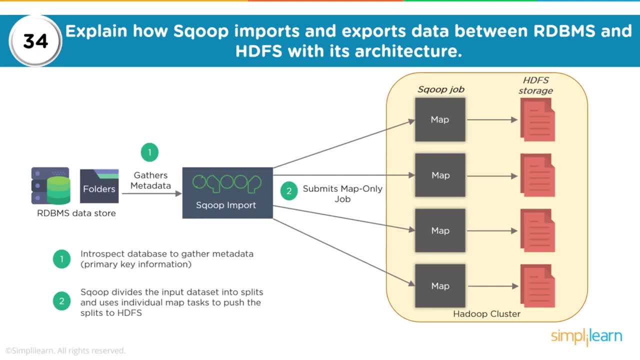 Now if somebody might ask: what if my table in RDBMS does not have a primary key column, then when you're doing a scoop import, either you will have to import it using one mapper task by specifying hyphen- hyphen M equals one- or you would have to say split by parameter to specify a numeric column. 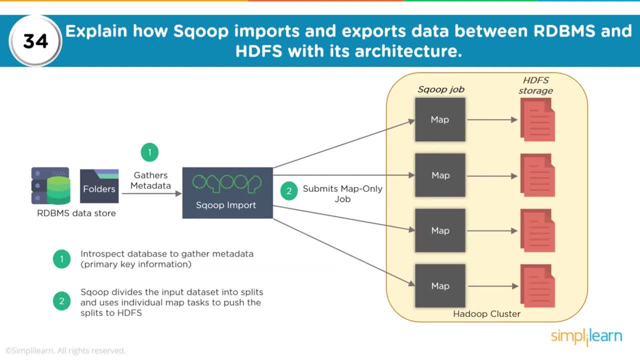 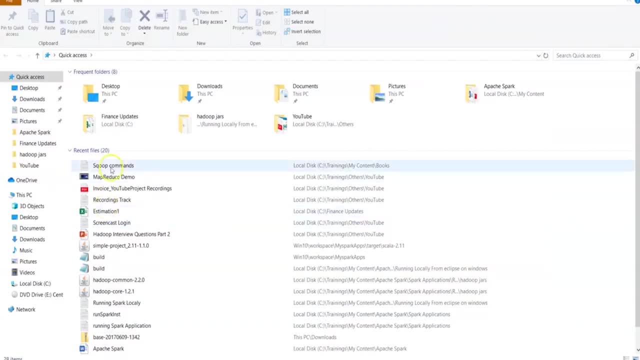 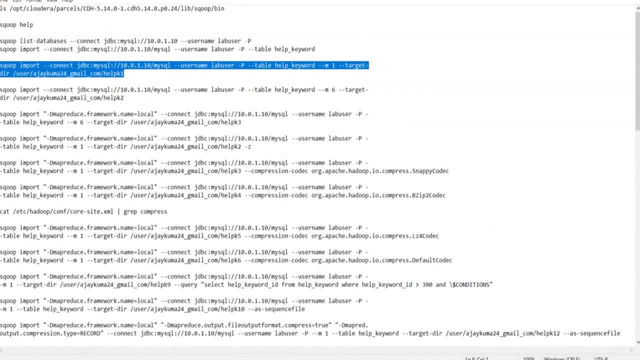 From RDBMS, and that's how you can import the data. Let me just show you a quick example on this So I could just look in again into the scoop command file and here we could be looking at an example. So if you see this one, here we are specifying: minus minus M equals one, which basically means I would want to import the data using one map task. 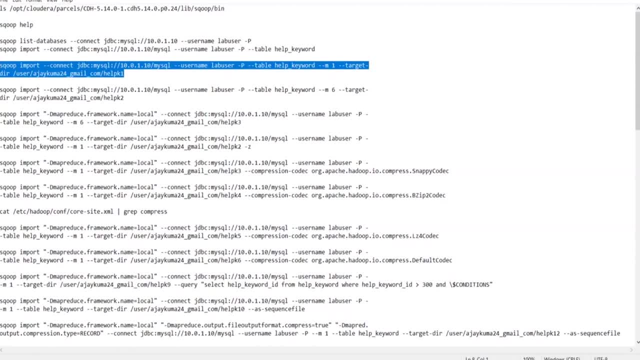 Now, in this case, whether the table has a primary key column or does not have a primary key Column will not matter. but if I say a minus minus M is six, where I'm specifying multiple map tasks to be imported, then this will look for a primary key column in the table which you are importing. 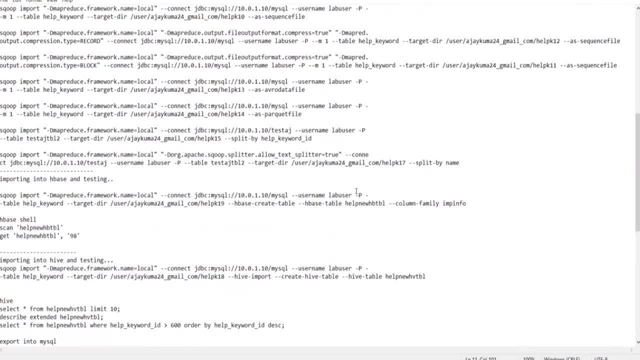 Now, if the table does not have a primary key column, then I could be specifying a split by and then specify the column, so that the data could be split into multiple chunks and multiple map tasks could take it. Now, if the second scenario Is your table does not have a primary key column and it does not have a numeric column on which you could do a split by, in that case, 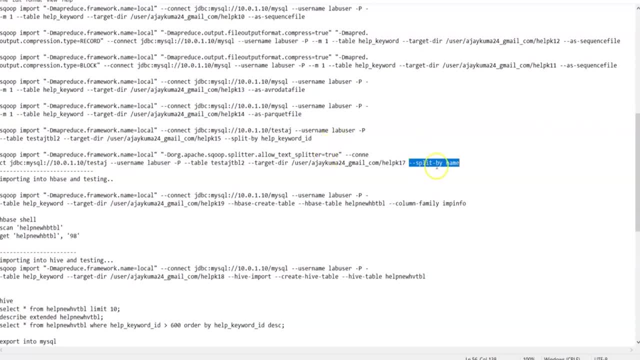 And if you would want to use multiple mappers, you could still say split by on a textual column, but you will have to add this property so that it allows splitting the data which is non numeric. All of these options are given in the scoop, Apache dot org. link. 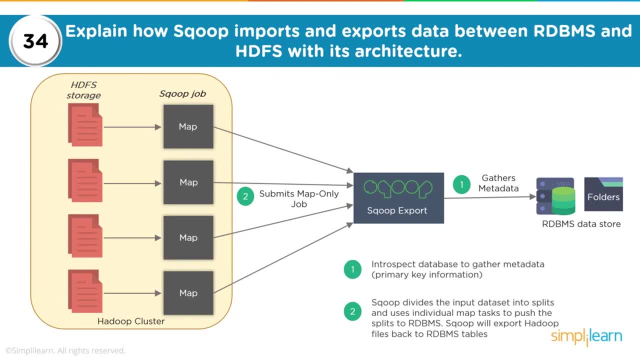 Going further, house scoop imports and exports data between RDBMS and SDFS with its architecture. so, as I said, it submits the map only job to the cluster and then it basically does a import or export. So if we are exporting the data from SDFS, in that case again there would be a map only job. 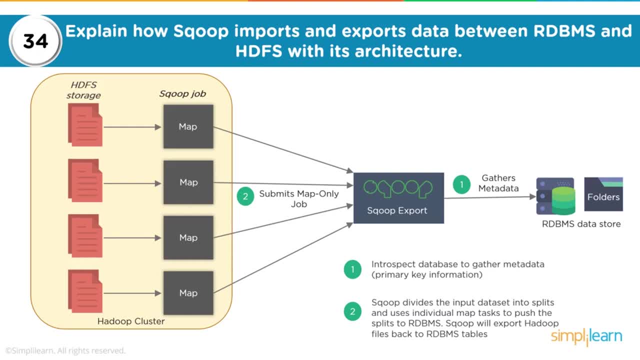 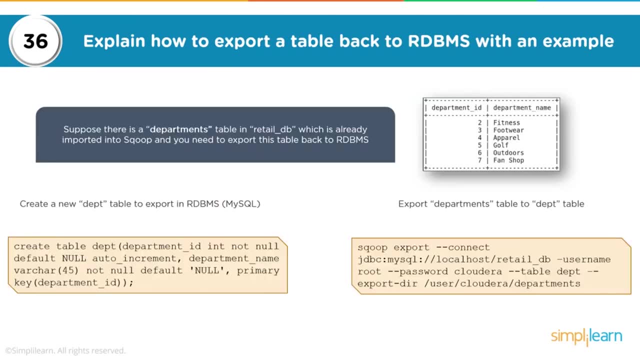 It would look at multiple splits of the data which is existing which your map only job would process through one or one table map task and then export it to RDBMS. Suppose You have a database test DB in MySQL, We, if somebody asked you to write a command to connect this database and import tables to scoop. 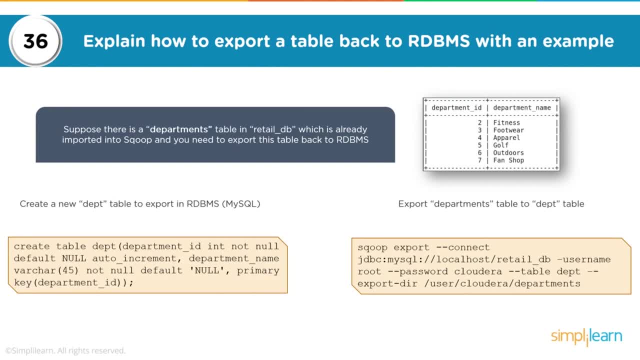 So here is a quick example, as I showed you in the command file. So you could say: scoop import. This is what we would want to do. You connect using JDBC. Now, this will only work if the JDBC connector already exists within your scoop lib directory. 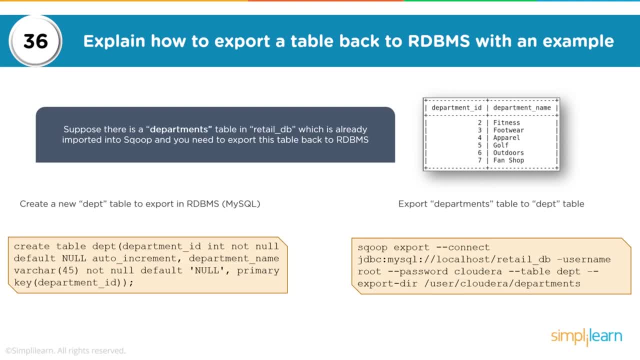 Edwin has to set up that so you can connect to your RDBMS, You can point to the database. So here our database name is test, underscore DV. I could give username and then either I could give password on the command line or just say capital P so that I could be prompted for the password, and then I could give the table name which I would want to import. 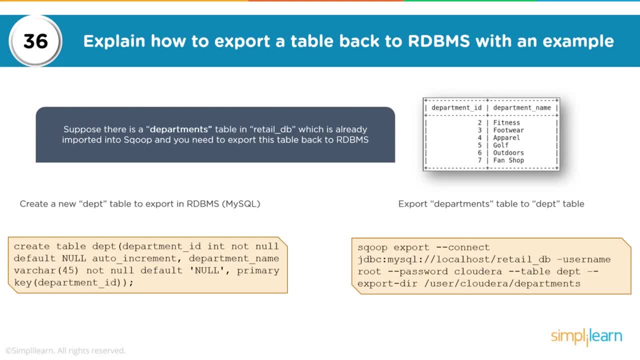 I could also be specifying minus minus M and specify how many map tasks do I want to use for this import. as I showed in previous screen How to export a table Back to RDBMS Now, for this we need the data in a directory on HDFS. 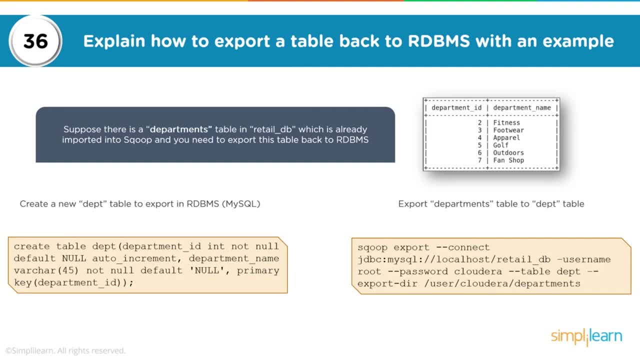 So, for example, there is a department stable in retail database which is already imported into scoop and you need to export this table back to RDBMS. So this is the content of the table. Now create a new department table in RDBMS So I could create a table specifying the column names, whether that supports null or no. 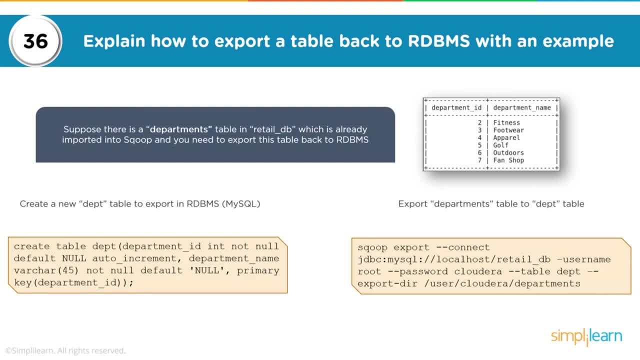 If that has a primary key column, Which is always recommended, and then I can do a scoop. export. I can connect to the RDBMS specifying my username and password, specify the table into which you want to export the data and then you give export directory, pointing to a directory on HDFS which contains the data. 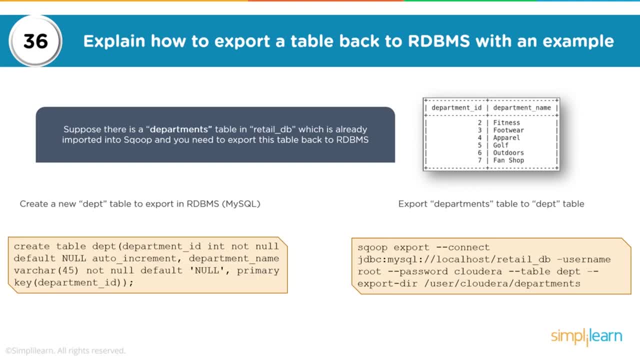 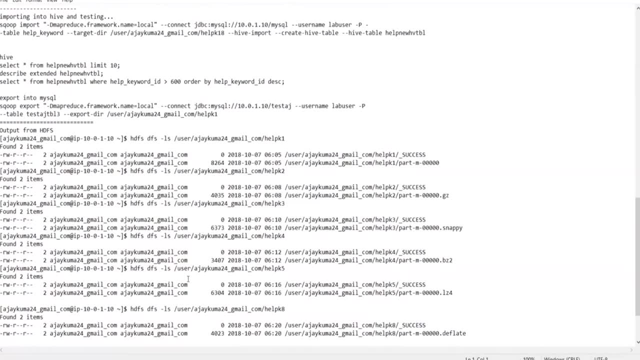 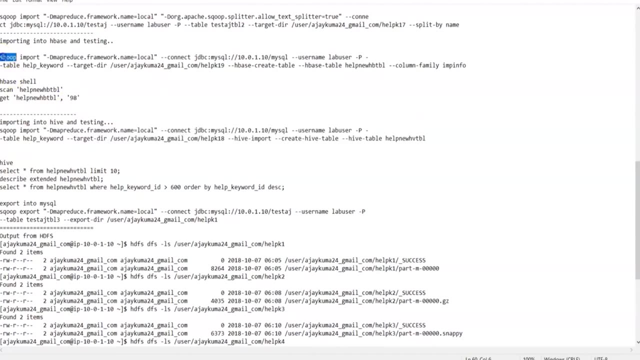 This is how you can export data into table. seeing example on this So I could again look into my file, and here I have an example Of import. This is where you are importing data directly into hive, and you have scoop import, where you are importing data directly into HBase table and you can then query your HBase table to look at the data. 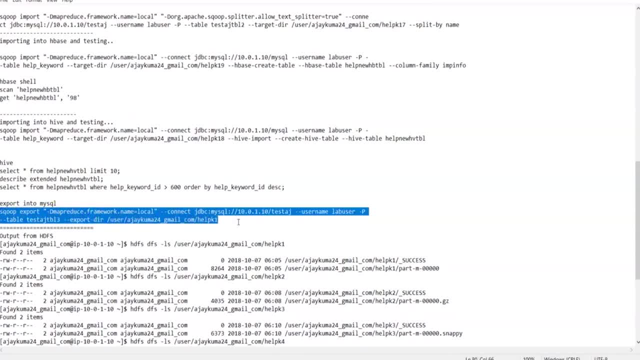 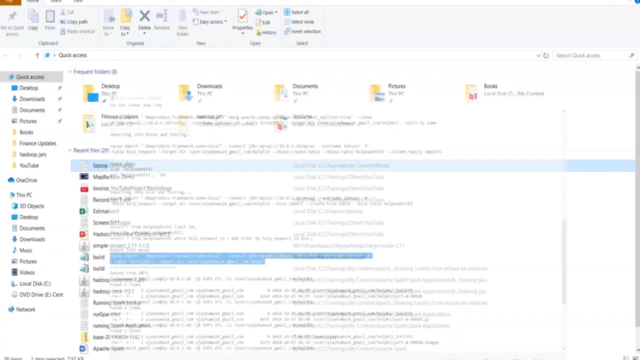 You could also do a export by running your map only job in a local mode, connecting to the RDBMS, specifying your username, specifying the table where you would want to export and the directory on HDFS Where you have kept the relevant data. This is a simple example of export. looking further, 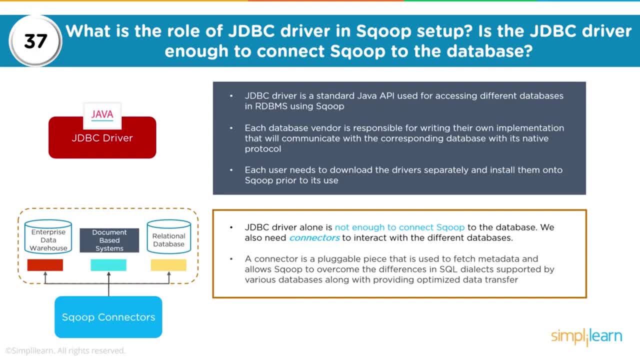 What is the role of JDBC driver in scoop setup? So, as I said, if you would want to use scoop to connect to an external RDBMS, we need the JDBC ODBC connector jar file. Now one or admin could download the JDBC connector jar file and then place the jar file within the scoop lib directory. 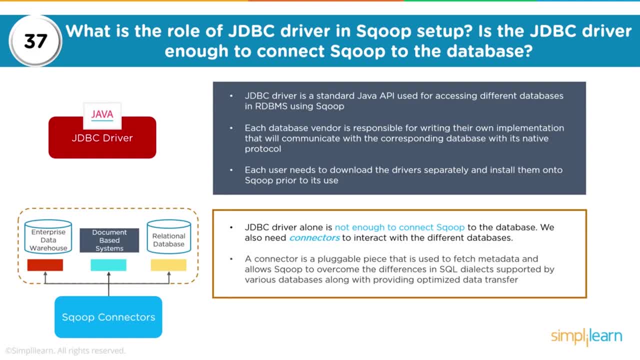 Wherever scoop is installed, and this JDBC connector jar file contains a driver. Now, JDBC driver is a standard Java API which is used for accessing different databases in RDBMS, So this connector jar file is very much required. and this connector jar file has a driver class, and this driver class enables the connection between your RDBMS and your Hadoop structure. 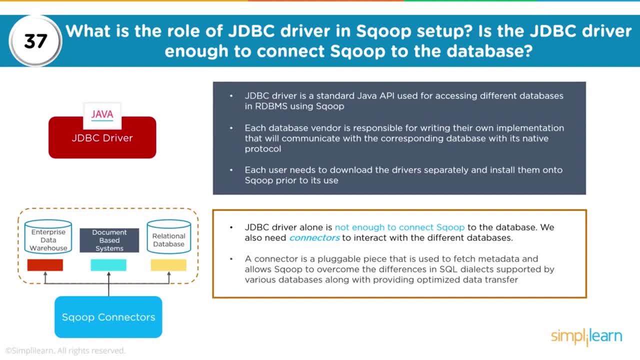 Each database vendor Is responsible for writing their own implementation that will allow communication with the corresponding database, and we need to download the drivers which allow our scoop to connect to external RDBMS. So your JDBC driver alone is not enough to connect to scoop. 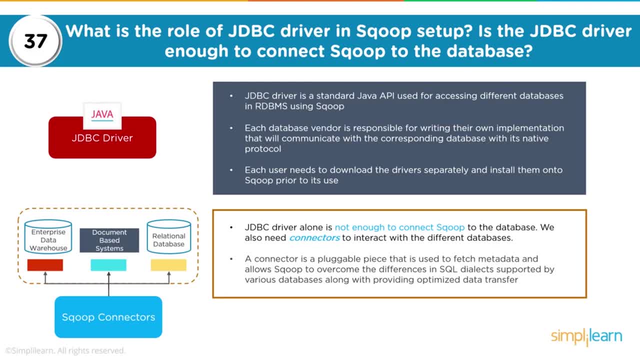 We also need connectors to interact with different database. So a connector is a pluggable piece that is used to fetch metadata and allow scoop to overcome the differences In SQL dialects. So this is how connection can be established. So normally your admins would when they are setting up scoop and Hadoop. 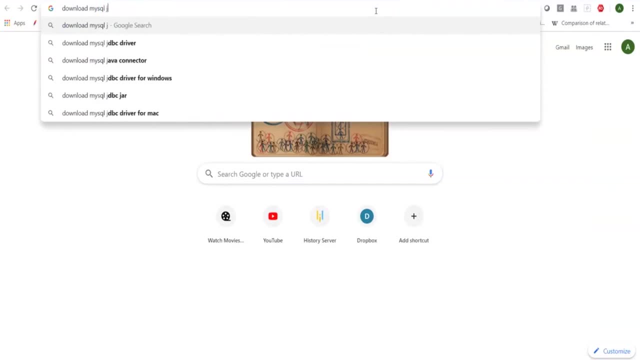 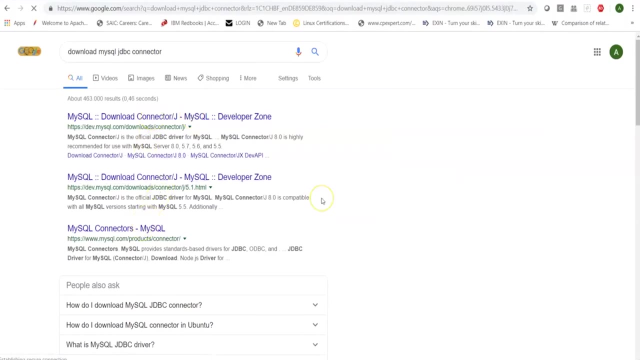 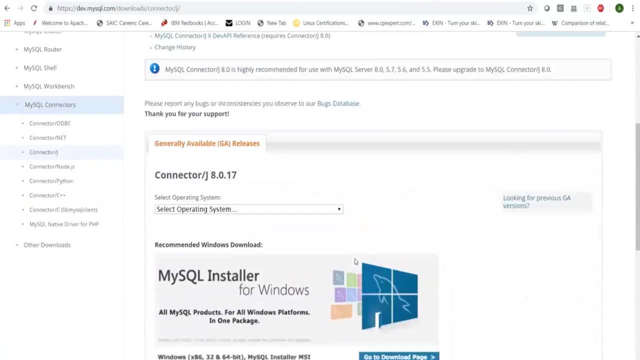 They would download, say, MySQL JDBC connector and this is how they would go to the MySQL connectors. If you are connecting to MySQL, similarly for your other RDBMS, you could be say, going in here, You could be looking for a previous version, depending. 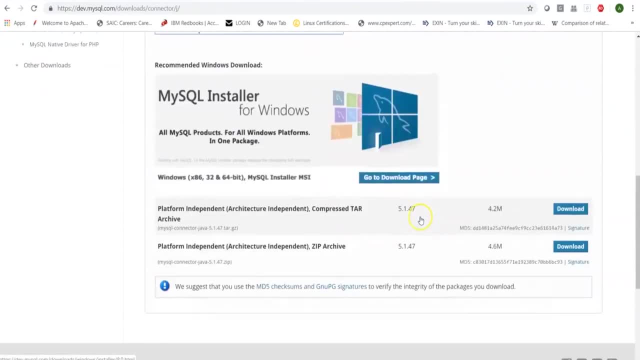 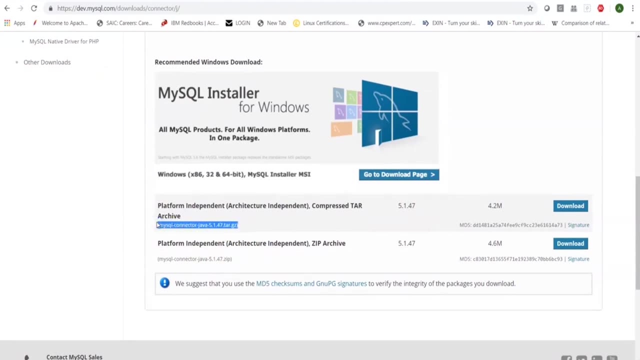 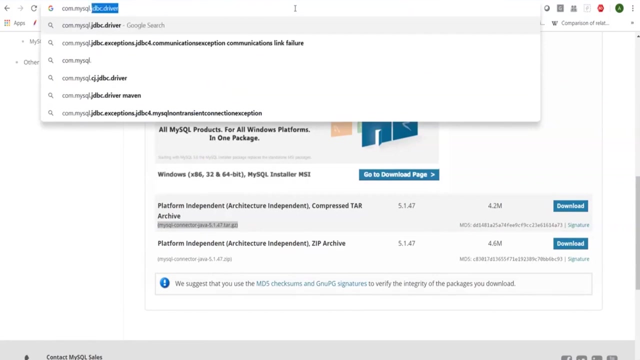 You could be going for platform independent and then you could be downloading the connector jar file. Now, if you untar this jar file, you would see a MySQL connector jar And if we look in, com Dot. MySQL, dot. JDBC, com dot. MySQL, dot. JDBC, dot. driver, 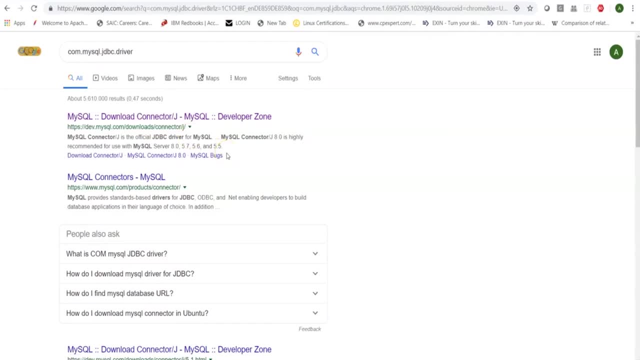 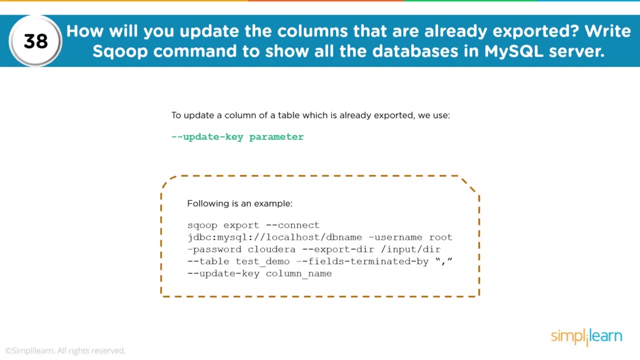 So this is the package which is within the connector jar file and this has the driver class Which allows the connection of your scoop with your RDBMS. So these things will have to be done by your admin so that you can have your scoop connecting to an external RDBMS. 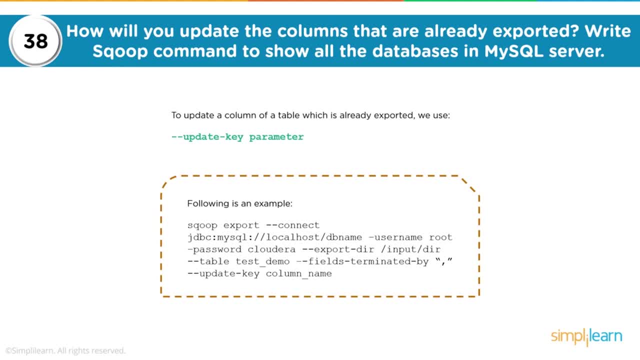 Now, how do you update the columns that are already exported? So if I do a export and I put my data in RDBMS, can I really update the columns that are already exported? Yes, I can, using a update key parameter. So scoop export. 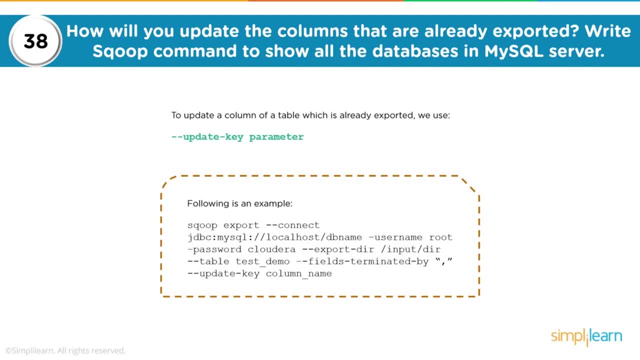 Command remains the same. The only thing I will have to specify now is the table name, Your fields terminated by, if you have a specific delimiter, and then you can say update key and then the column name. So this allows us to update the columns that are already exported in RDBMS. 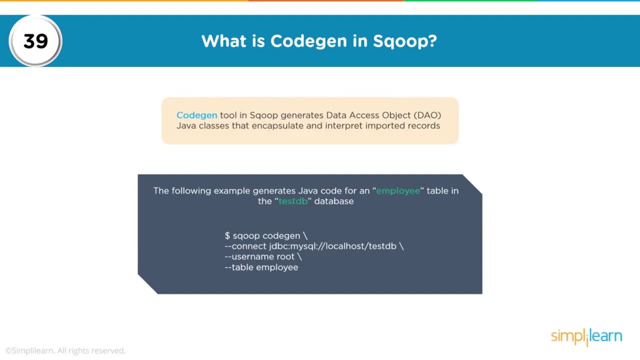 What is code gen? So scoop commands translate into your MapReduce job or map only job. So code gen Is basically a tool in scoop that generates data access objects, DAO, Java classes that encapsulate and interpret imported records. So if I do a scoop code gen, connect to an RDBMS using my username and give a table. 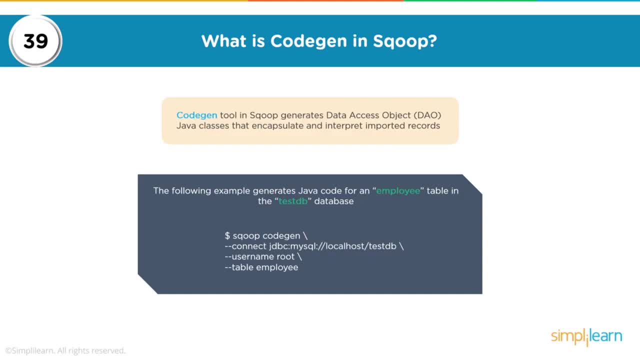 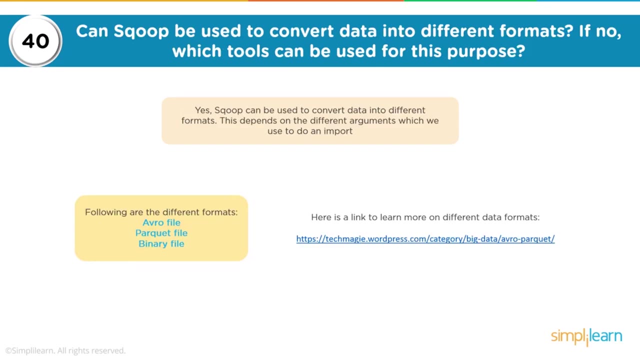 This will generate a Java code for employee table in the test database, So this code gen can be useful for us to understand what data we have in this particular table. Finally, can scoop be used to convert data in different formats? I think I already answered that right.